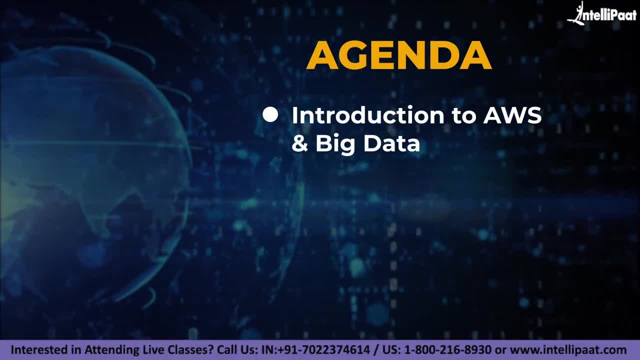 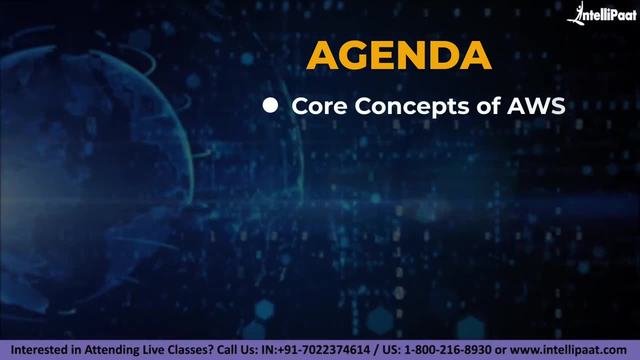 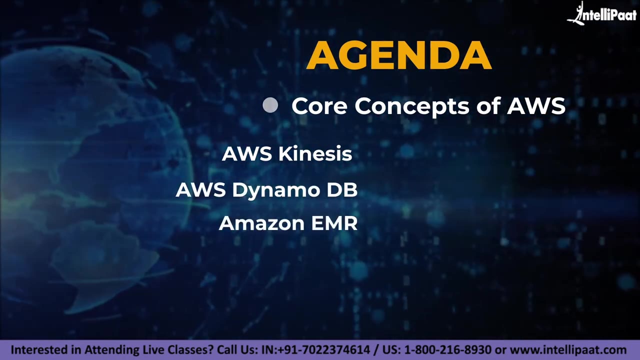 Firstly, we will begin with introduction to AWS and Big Data. Post that we will tell you why to use Big Data. on AWS Post that we will be learning few core concepts of AWS like AWS, Kinesis, AWS, DynamoDB, AWS, EMR, AWS, Lambda AWS, Glue AWS, Redshift AWS, AWS. 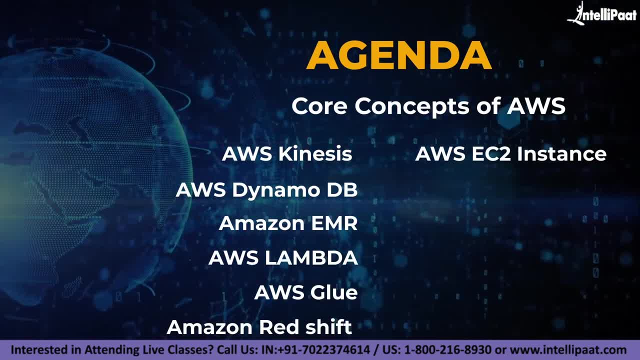 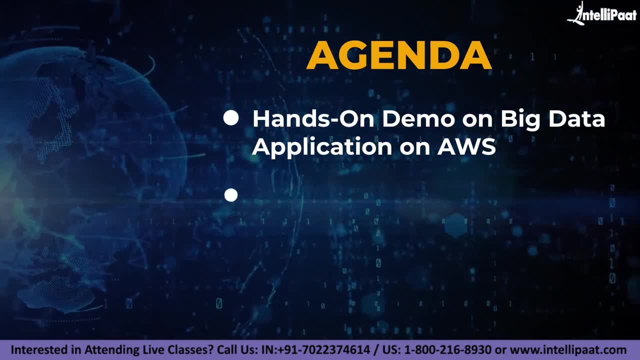 And we will be learning how to use AWS for Big Data workloads- AWS EC2 Instance. After that, we will be covering a hands-on demo on how to build Big Data applications on AWS. Then, finally, we have covered AWS and Big Data Hadoop. interview questions and answers. 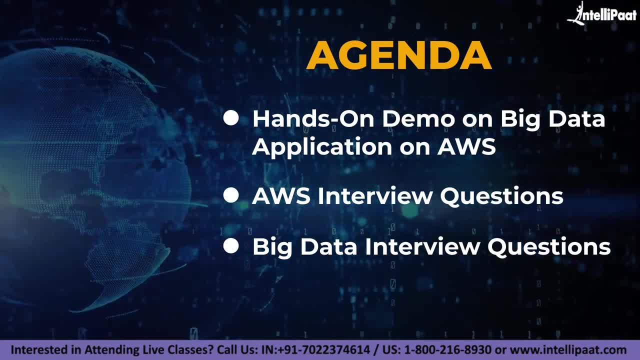 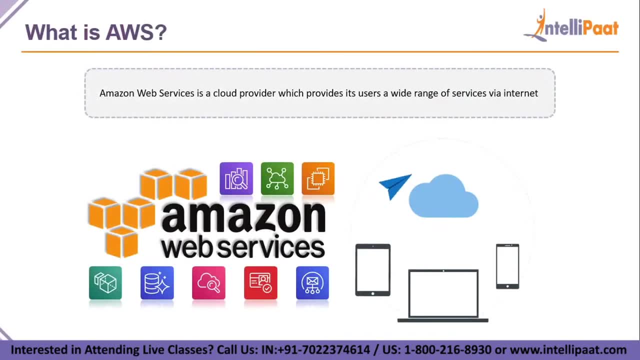 So, guys, this is the agenda of the video. This session is going to be very interesting, So stay tuned and watch the video till the end. So let's get started with it. What is AWS? So first let me give you the full form: the expansion of AWS. 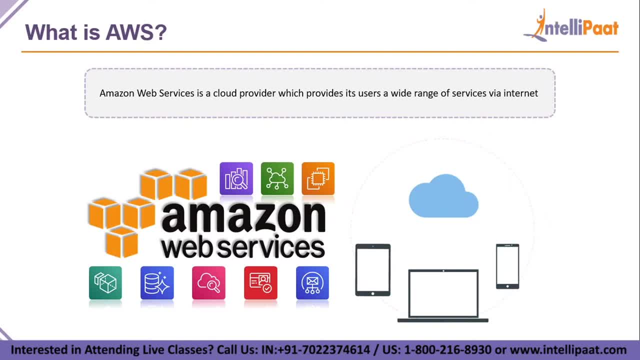 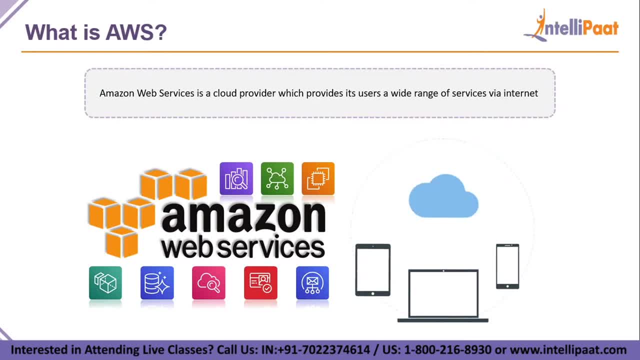 But what is a cloud provider? So to understand what is a cloud provider, you should first know what is a cloud service. So let me tell you in the most simplest terms what a cloud service is. Cloud service is something which is on another person's computer which you are trying to access through the internet. 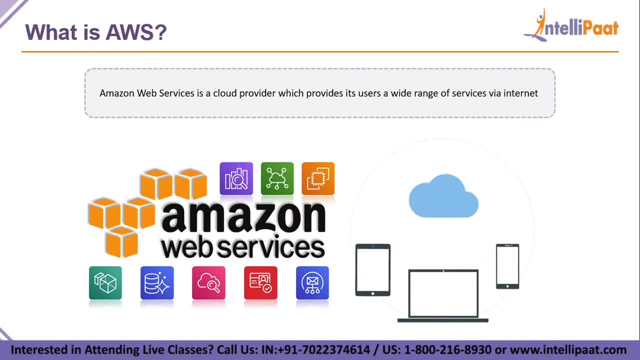 So let's say I have 10 computers, So in that I'm just using one, and nine computers are redundant for me, I'm not going to use them. So what I'll do? I'll just rent it out through the internet. 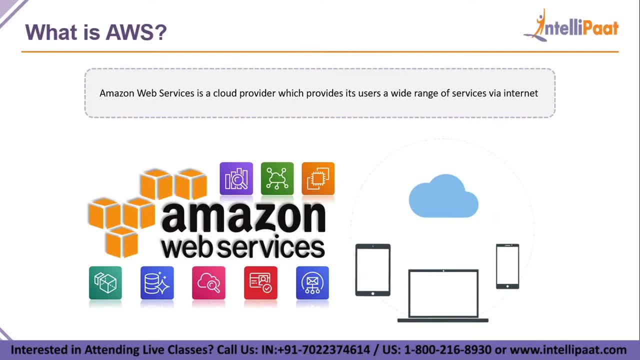 So I'll be running virtual missions on these PCs, So you will be able to create a virtual machine on my system and use it for yourself, And you will be paying me for that. So you are renting something through the internet. So a cloud service. 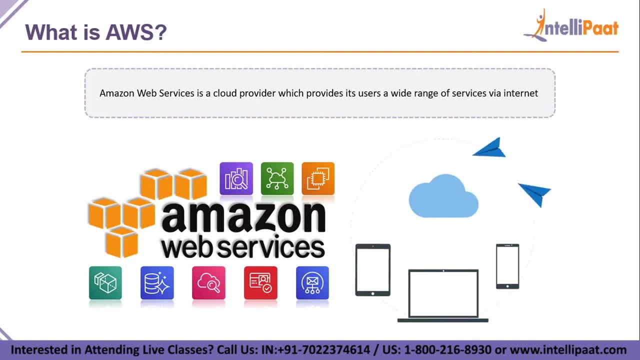 So let's say, even Gmail is a cloud service, But Gmail provides you An application over the internet. So you're using an application over the internet, but you do not know where this application is hosted on. Obviously, this application is hosted on a server somewhere in America or somewhere in Europe or any data center. 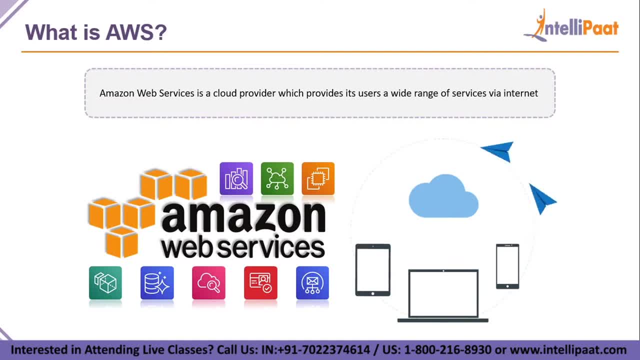 So somewhere it is hosted So that particular computer has these files and you are accessing these files or these applications through the internet. So that is a cloud service. So any service, any website which is which you are viewing On your browser. 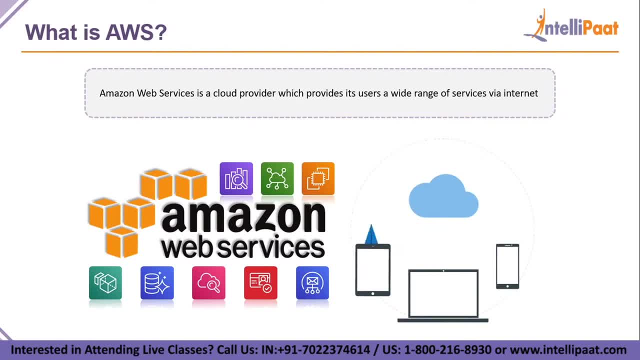 So you go to googlecom and type in: uh sorry, uh, if you go to a browser and just type in googlecom, you get a website. So that website is fetched from a server which is running on the glue- Google cloud. 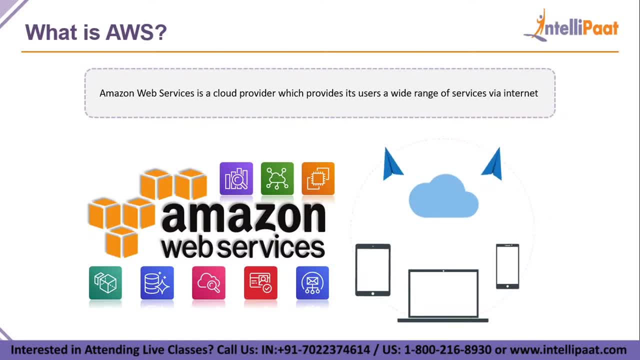 So even googlecom is a cloud service. So now there are other types of cloud services as well. So what do I mean by other types? So we've discussed about application sourced around. that is, googlecom, Gmail, Google sheets. So now come here. 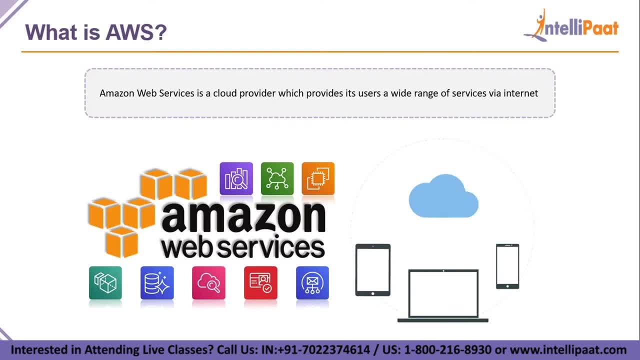 So, if you are coming to other types, there are two more types. One would be infrastructural and one would be platform based. infrastructural in the sense you can rent or you can basically uh, uh, get your own PC. Uh, so you can get your own computer, but the thing is you will get access to the operating system, not the hardware components. 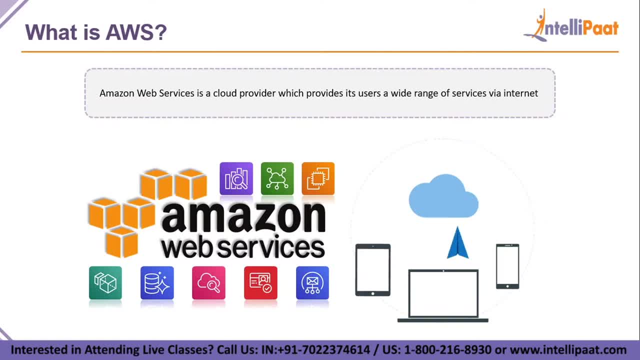 You will have complete access on the operating system. You can install anything, You can add any kind of files, you can do Uh, you can host your applications on them. You will be paying for that usage, but you will not be given hardware level permissions, you, but you will be given OS level permissions. 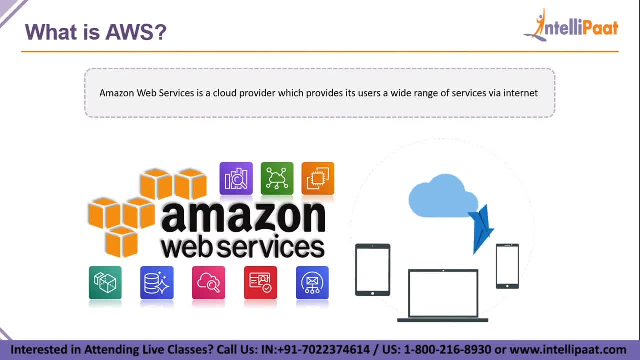 So you can get a server which is hosted on AWS, Another one which he was saying is platform. platform In the sense you will be given a website on which you can create your own application through that platform, which again will be hosted on AWS. 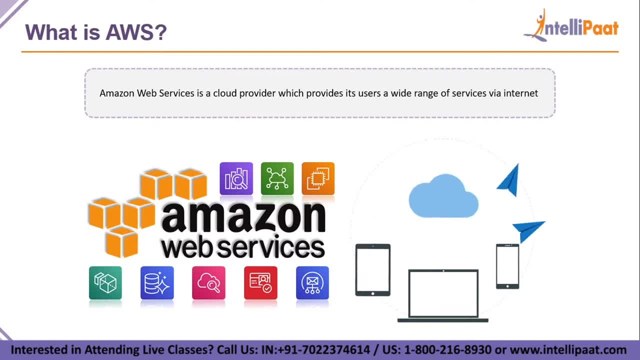 So here we are discussing AWS. That's why I'm giving AWS examples. So I've given you a basic. The three types: One is infrastructural, That is, you will get servers platform, where you will get a platform to design applications and also get uh servers automatically for that. 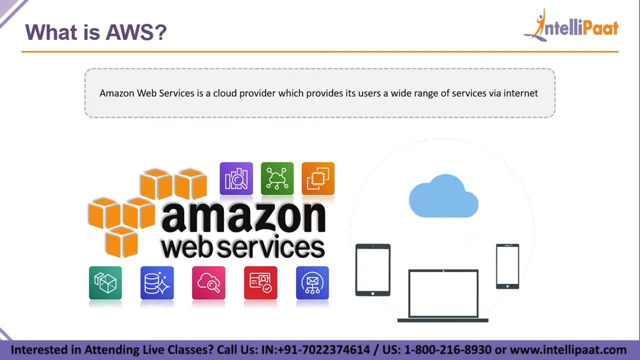 Third is the applications like Gmail, uh, Google sheets, So I'll give these. uh. so, for infrastructure, I'll give a service. for platform, I'll give a service which is available in AWS later in this session. So now we understood what is a cloud service. 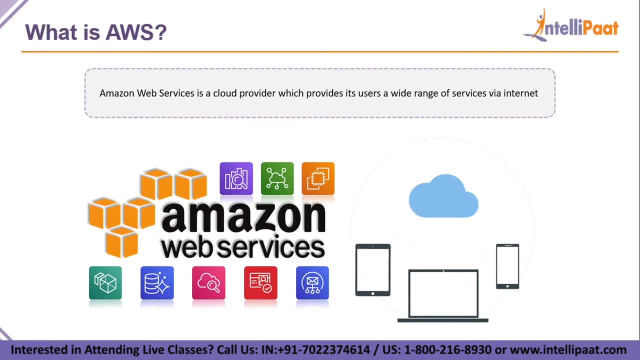 Now, a cloud service is something Which you get over the internet. Now, a cloud provider is a company who provides these cloud services. So Amazon web services is a cloud provider who provides these services over the internet, and they have a lot of different services and we'll discuss about them later. 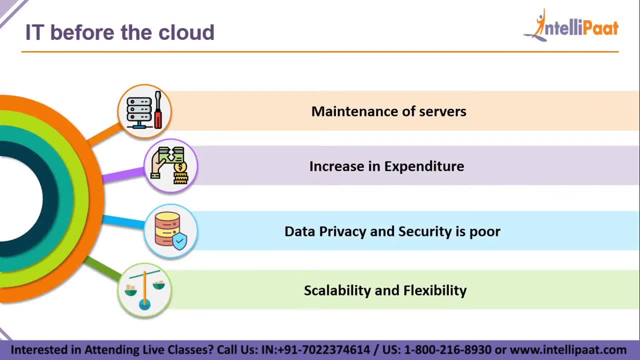 Now, uh, it before the cloud. So before we used to buy servers. so for any application you want to host, you will have to buy a few servers and then configure it. uh, install applications, Install softwares and then copy your code to that, make it run and then make it online. 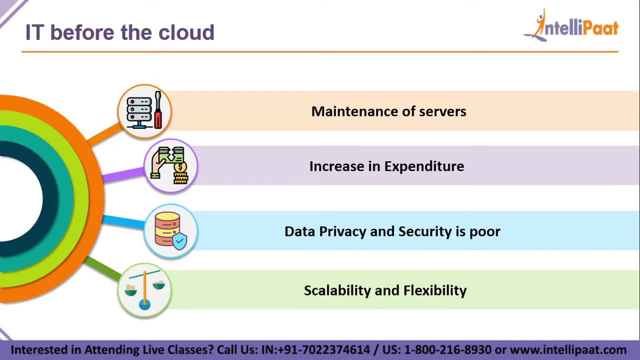 So this takes a lot of time as well as once it is running, you will also have to maintain them, So the maintenance costs will be very high, And that is one of the reason people started to shift off with cloud computing and then increasing expenditure. 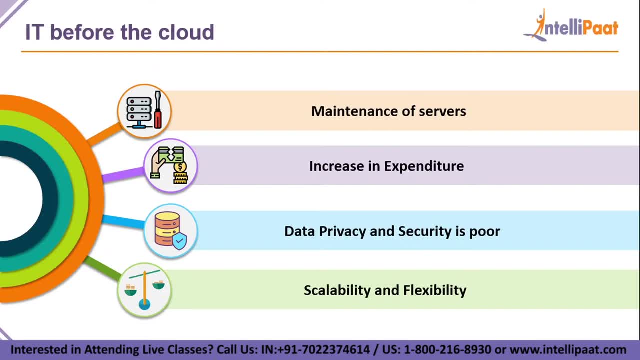 Uh, obviously, if you want to buy more servers, you need more capital, and to maintain them, uh, you'll have to hire professionals and for them you'll have to pay, So that also increases. This is the expenditure. data privacy and security is poor because you will have to hire security professionals. 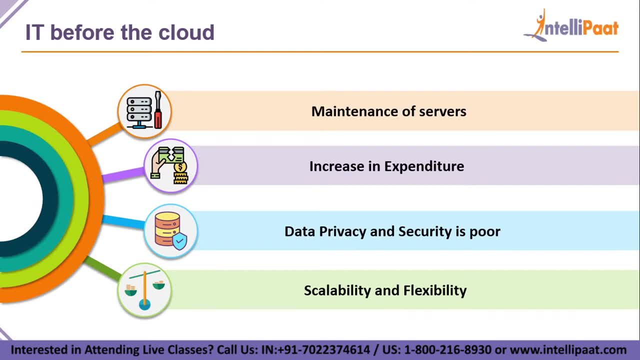 A lot of security professionals. If you are having a lot of servers, take care of it. If not, obviously your security will be poor because, uh, you will not be active all the time. Any security professional cannot be active all the time to keep on checking if there is a bug or if there is a loop loophole. 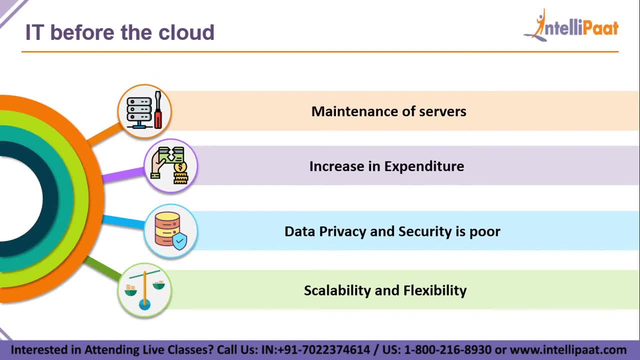 And then finally, scalability and flexibility. flexibility in the sense: if you have 10 servers, you cannot easily uh, give back to Servers and reduce your expenditure. You cannot do that If you bought 10 servers. and scalability in the sense. 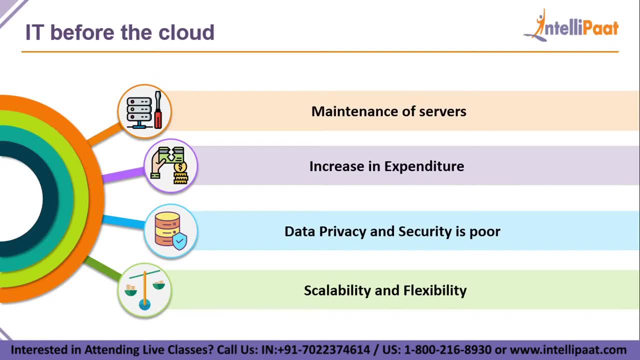 So if you have an application which is utilizing 10 servers, now suddenly the traffic is increasing, So now you want more servers, So you go buy five more servers and now you have 15 servers. right now the application is using all 15 servers, but suddenly one day or for one week you don't have any spike in traffic and it is only using 10 servers. right now. 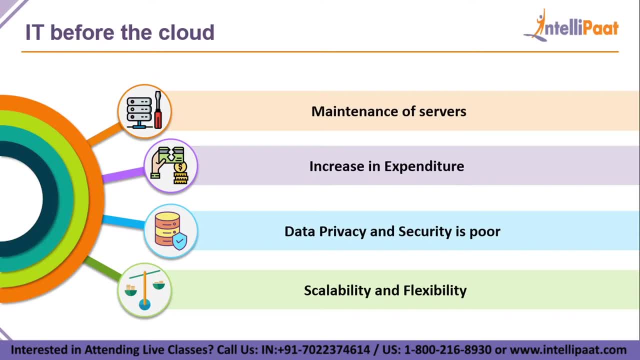 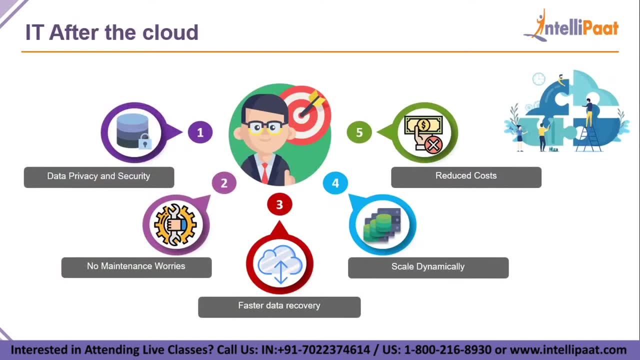 So now The five servers are sitting there idle, costing you money, So this again was an issue. So then cloud came into the picture. So they gave you better data security and data privacy because, uh, they have uh hired 3,500 plus security professionals for their data centers and their data centers. 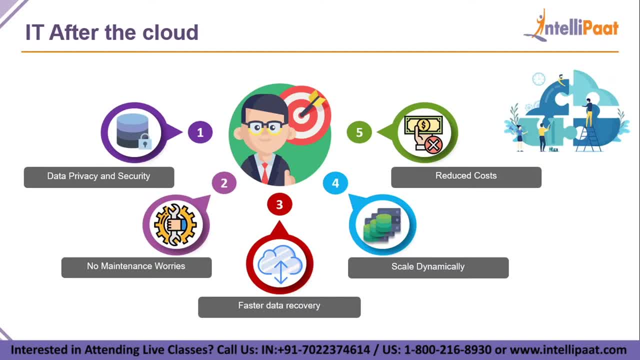 Architecture is obviously more secure and complex than a private company's data center. And then no maintenance worries, They'll take care of all Maintenance, they'll monitor it, They'll maintain it, They'll patch it up. faster data recovery. So if you have your servers and if you have data in it, if your servers are destroyed in some natural calamity, then you'll not be able to recover that data back. 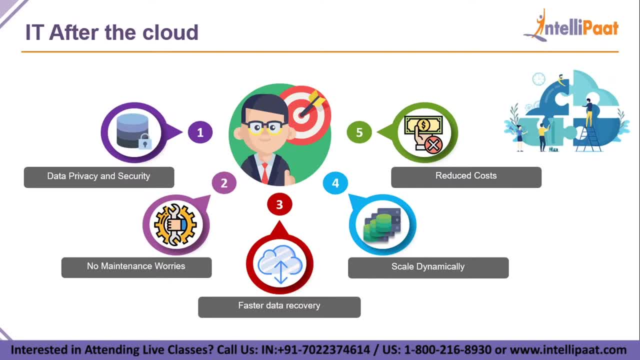 But if your data is stored on the cloud, you will. you can have a backup somewhere else in another region, Even though that data center is down. you can get a backup of the data from another data center scale dynamically. So in cloud you don't need to buy more servers. 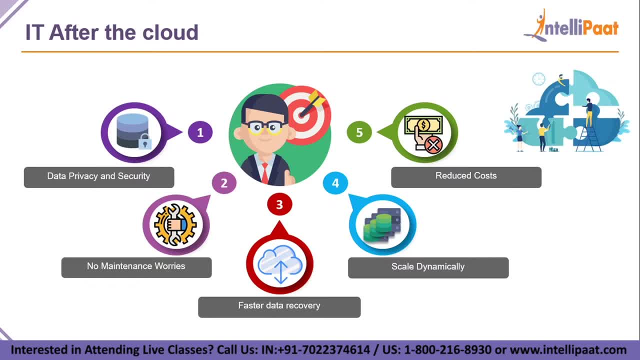 You just have to provision Five more servers. And so let's say the same example: you have 10 servers for an application- traffic spikes, So you get five more servers. So now 15 servers are used. Suddenly traffic goes down. You, you only need 10 servers right now. 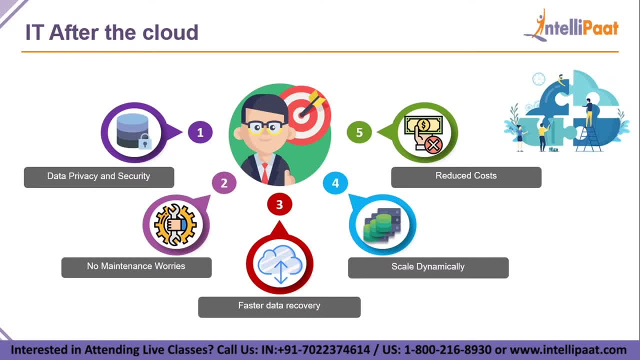 You can deprovision or terminate those five servers and use only these 10 servers, So this is very cost efficient and then reduced costs. Obviously, if a cloud provides a scale, a dynamically scaling option, obviously it'll reduce your costs. You don't need to worry. 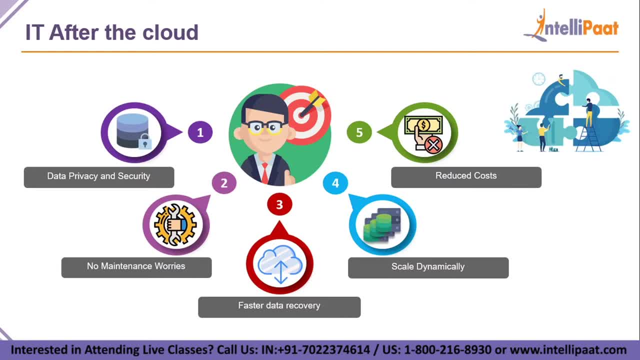 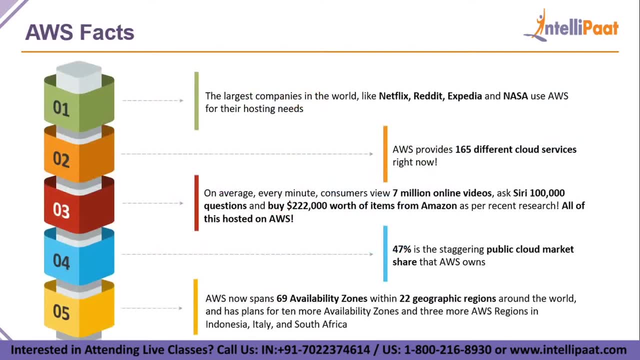 About maintenance. that will reduce your cost. You don't need to worry about security- Again, that will reduce your cost. Now some facts about AWS. We'll just rush through this. So top companies like Netflix, Reddit, Expedia and NASA use AWS for their hosting needs. 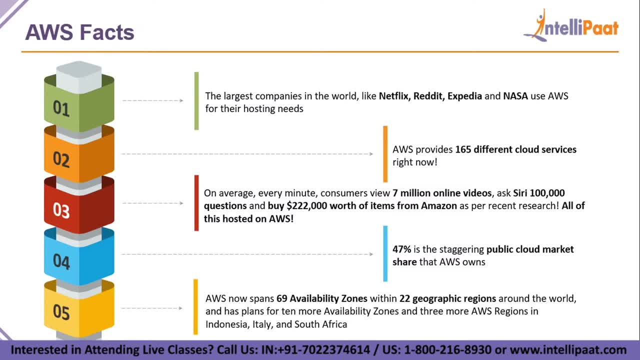 And then AWS currently has 165 different services and it is increasing every single year. And then, on average, people view 7 million online videos- 7 million online videos- And they ask Siri 100,000 questions. buy $222,000 worth of items from Amazon. 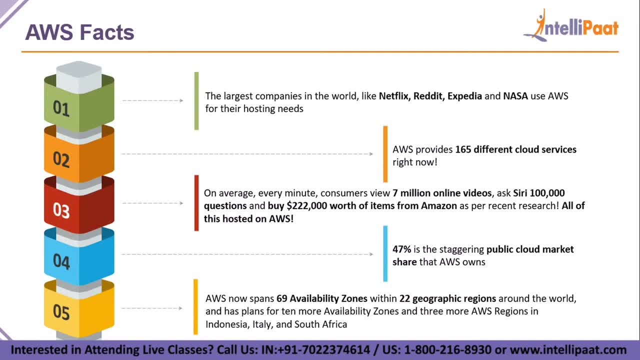 And all of these websites and applications are hosted on Amazon web services. Now also, AWS owns a 47% market share in the public cloud industry, which is the highest, And they are at the number one position. And also AWS has 69 availability zones across 22 geographic regions, including India. 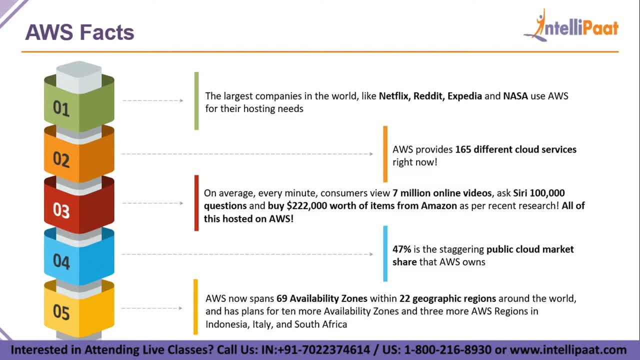 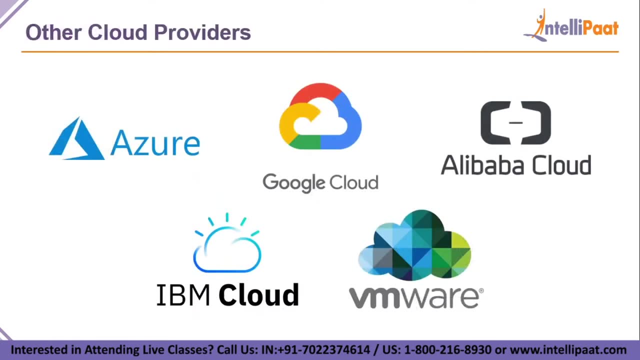 USA and all across Europe. So now they are also trying to bring 10 more availability zones in three different regions, which is Indonesia, Italy and South Africa. So these are some AWS facts just to show how big is AWS and other cloud providers, as your Google cloud, Ali cloud, IBM cloud, VMware. 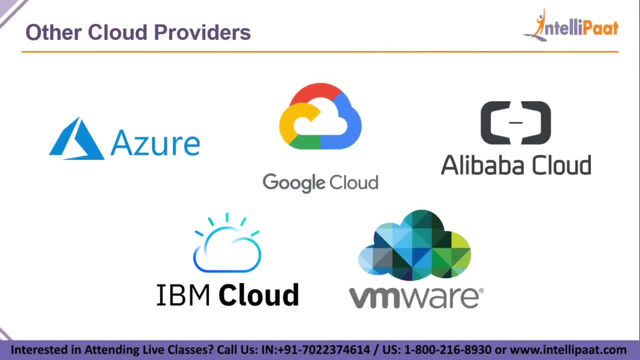 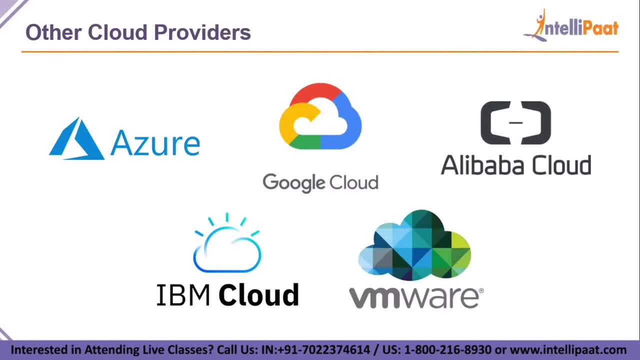 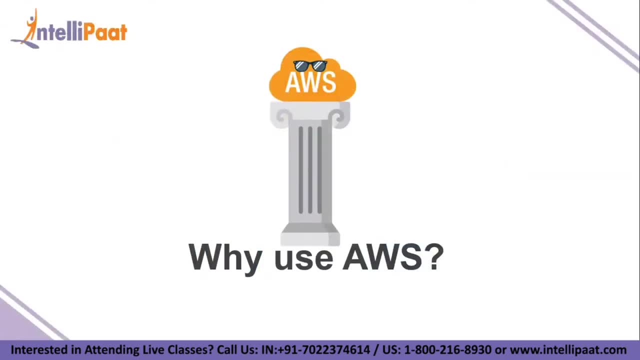 Mostly we ignore them because the top three are AWS, Azure and Google, And so in this session we are looking into AWS. So, moving ahead, we'll check out. why should we use AWS? So we've discussed about AWS and we also saw other cloud providers. 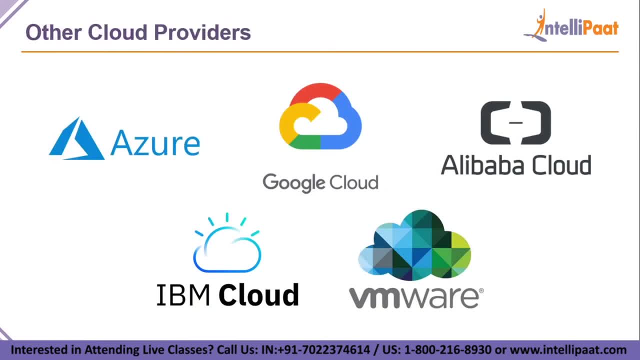 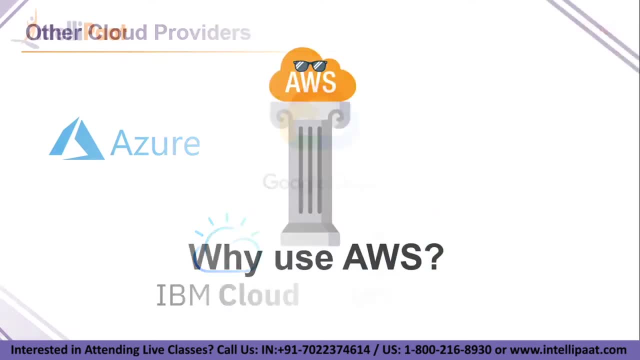 Now you would be thinking that why should I not use Azure or why should I not use Google cloud? So you can use Azure or Google cloud, but why should you use AWS? That we'll look at now. So first of all, we're going to talk about AWS. 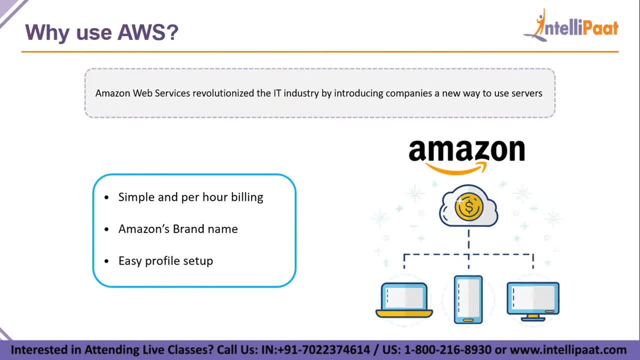 So first AWS launched. so AWS were not the first cloud providing company, but they were the best cloud providing company, So just a rhyme. So AWS came into picture in 2006 with EC2 and S3. These were the first services which came up. 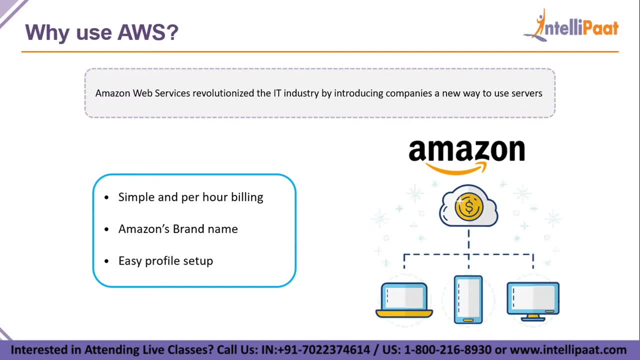 So they revolutionized the IT industry by introducing a new way to use servers. So normally an IT company will buy servers, configure it, put their application, run it. But when AWS came into picture, they told that. they told companies that you don't need to buy servers. 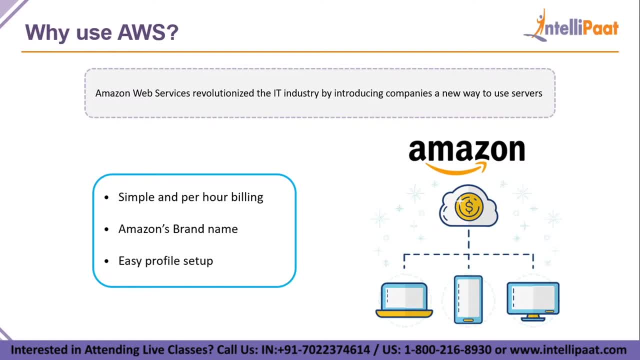 We'll buy servers, we'll take care of them. Just give your application to us, We'll host it on them. So, basically, you won't give your applications code You, they give you the permission to host your application on their data center and it will be running. 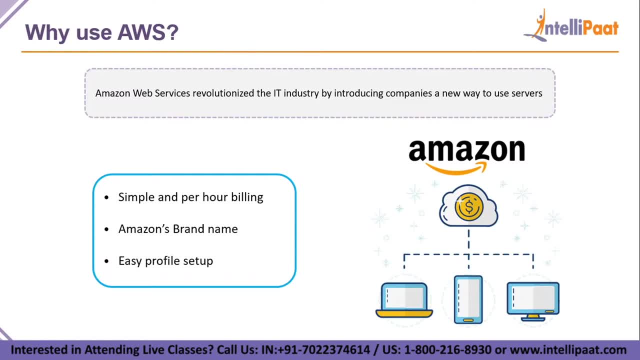 You just pay for the servers which is used. They'll take care of maintaining. So this was a great gift for any IT company, because it will reduce their costs as well. It'll reduce their maintaining needs and they can concentrate more on developing the application rather than hosting it. 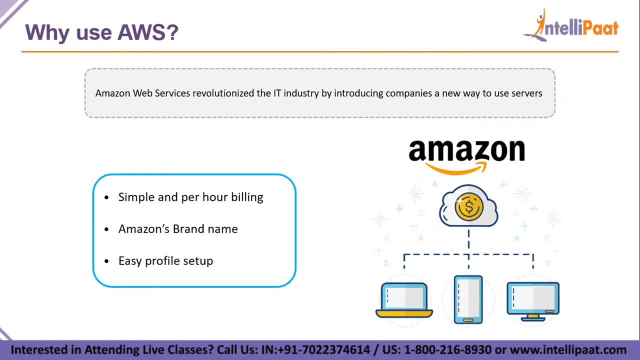 Then other other things. why you should use AWS is. other pointers are: first, simple and per hour billing. That is, if you're using a service and if you're using it just for an hour or two hours, you wouldn't get billed for a month. 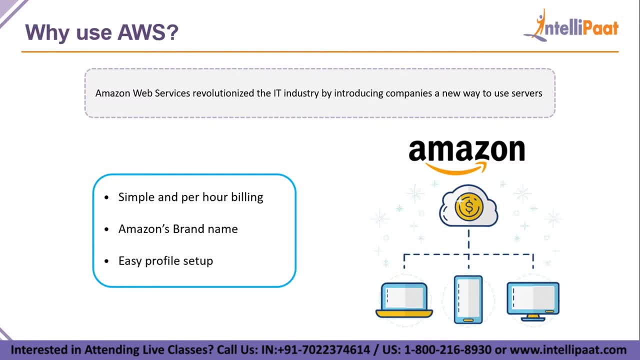 You just get billed for one or two hours which you have used Amazon's brand name. Obviously, Amazon is the largest e-commerce company in the world. They have other things like there is Amazon prime video, there is Amazon music, there is Amazon Kindle. 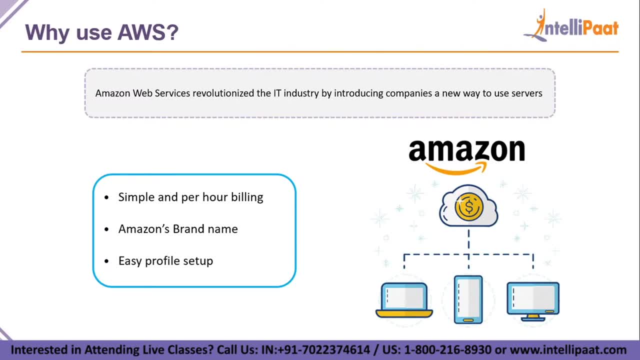 So there is so many things, And Amazon is one of the biggest names in the internet industry, So that is one plus. third one is: it is very easy to get started with AWS. It is like creating a profile for your Facebook account, but just one more step. 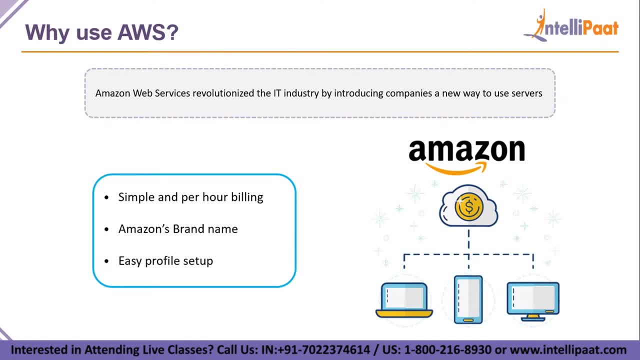 You will have to provide your credit or debit card details so that if you're using some services, obviously you will get billed. But AWS also provides a free tier. We'll discuss about that later. So right now, these are the three major factors why people prefer AWS. 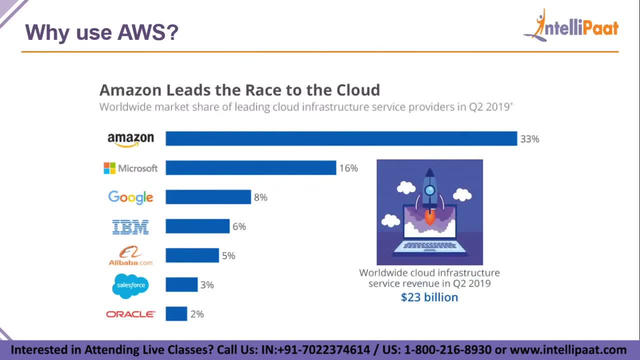 And I already told you that AWS is leading. So this particular chart is just for three month period on, So quarter two of 2019.. So in quarter two of 2019, Amazon had 33% share, Microsoft had 16% and Google had 8% and other companies. 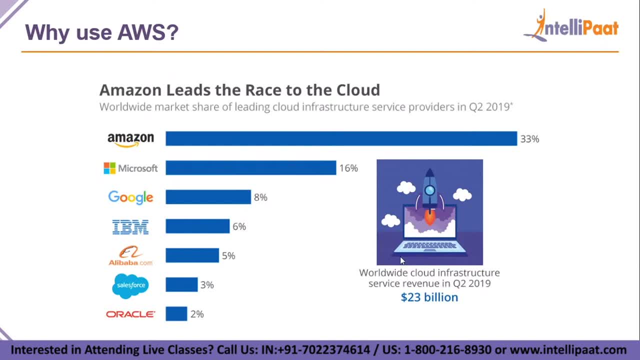 You can just look at it. You can just look at them. Uh, so worldwide cloud infrastructure service revenue was $23 billion And in that $23 billion, 33% was AWS revenue. So this shows how big is AWS And obviously, if a service or if a cloud provider is huge enough, many companies are going to use it or they're already using it. 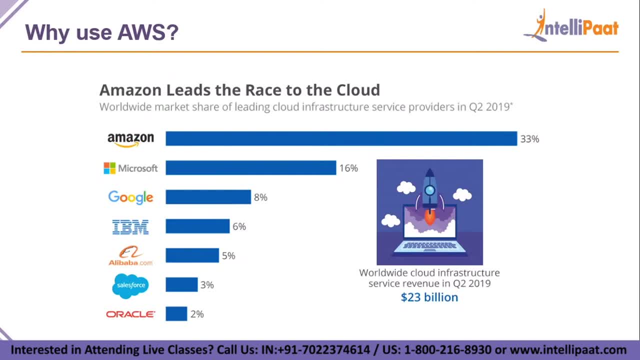 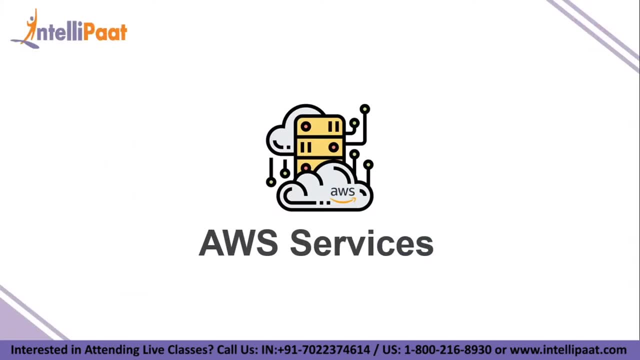 So if a lot of companies are using AWS, so if you learn AWS, obviously there is a lot of jobs. There's a lot of job opportunities. Okay, So now we've discussed various factors. We discussed what is AWS and why should you go ahead with AWS. 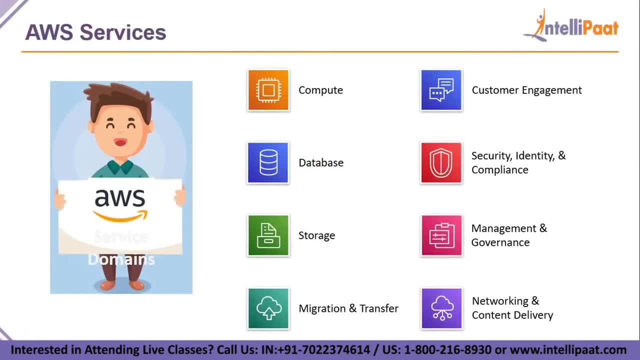 Now let us look at some AWS services First. these are some domains on which AWS has services. So compute, uh, compute in the sense, a server, a database engine. So, uh, a database engine which you can host on that server. 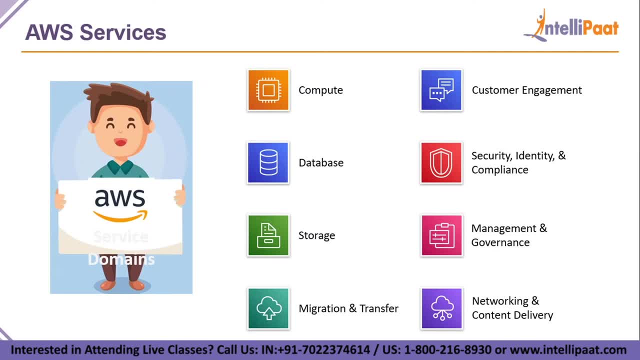 So they also have separate database services, but as a compute service you have these And you have database services. you have storage services. you have migration and transfer services. This is a very uh- these are very uh- amazing tools in migration. 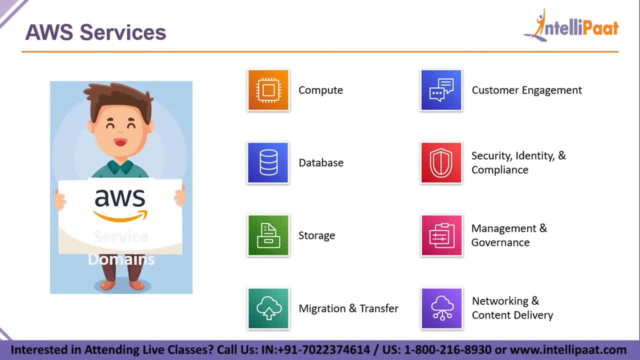 So there are uh database migration services and there is a virtual machine migration service as well. So in a database migration service you can directly migrate a database hosted on your on-premise system- uh on-premise server- to the AWS cloud in just a few minutes. 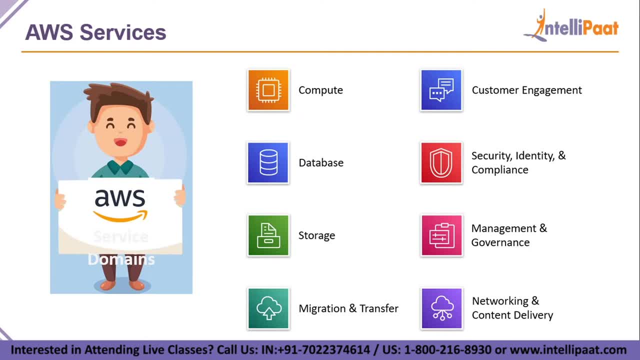 So you can do that, And then customer engagement. You have a customer engagement applications as well, like chats and email services. Then you have security, identity and compliance. Obviously, you need security and also identity services for AWS, because there might be multiple users using a single AWS account. 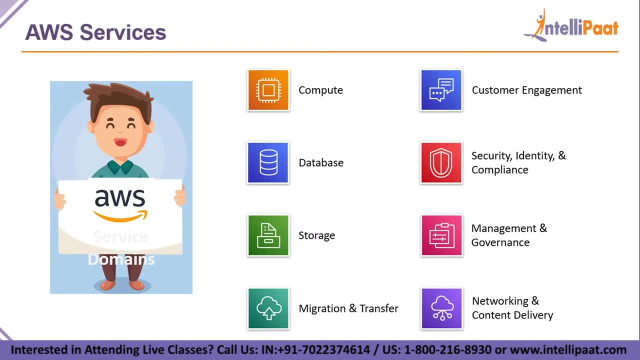 And for that you need identity and then management and governance. So obviously we'll have to monitor and manage your AWS account. Even though AWS is managing your servers, you will have to manage your AWS account, And for that you have monitoring and managing services, and then networking and content delivery. 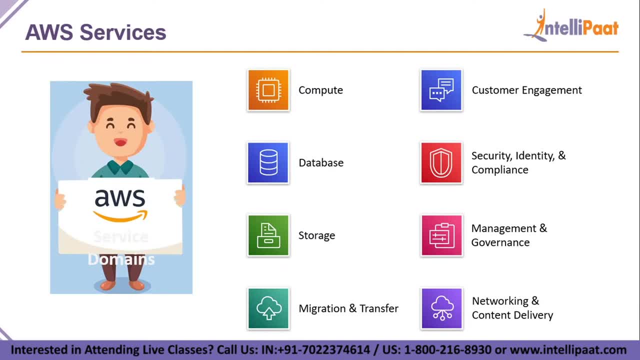 So for these services- that is, compute, database and storage- to run, they should be running inside a network. So to create a virtual network for yourself, So let's say, uh, you're creating virtual network and launching two servers within that and, uh, any other- so another server outside of it, in another network, cannot communicate with it until you give permissions for that. 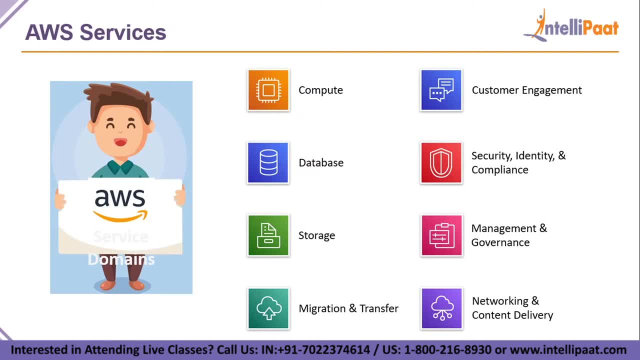 So you can Create your own private networks and also content delivery. That is you can. you can also have a CDN, a content delivery network. Uh, so YouTube uses a content delivery network, but YouTube uses Google's own content delivery network. 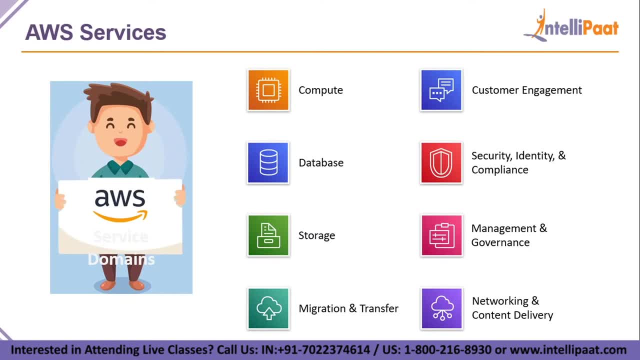 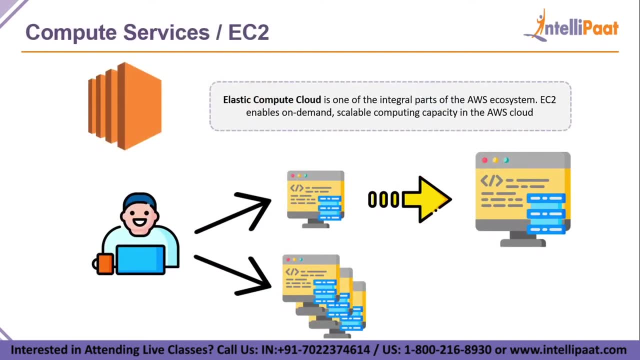 And in AWS also, they provide a CDN called cloud front, and you can use it for your own streaming needs. Okay, So now let us discuss few services. So see, uh, EC2 is a compute service and this is the Most. 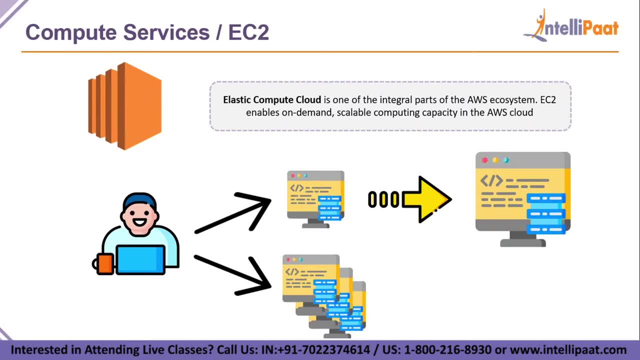 Integral part of AWS itself. So because most of the AWS services uses EC2 for one on one or another reason. So first let me tell you what is EC2.. So the full form of EC2 is elastic compute cloud And. 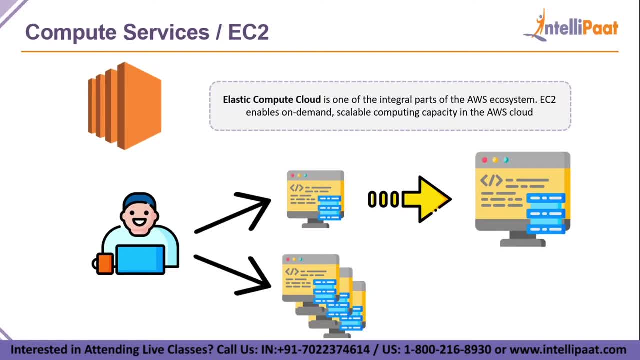 EC2 is basically an on-demand server uh system. So EC2 enables on-demand scalable computing capacity in the AWS cloud. So what does that this mean? is it provides you a virtualized server running on the AWS data center Which you can just launch in a couple of seconds and use it for your own needs. 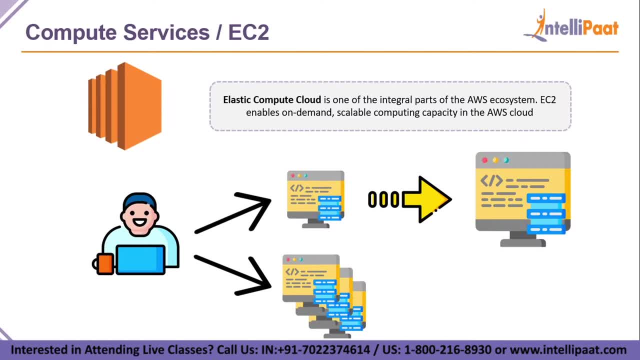 You can use it, uh, uh, so you can use it as your own PC. Uh, you can use it to launch applications, You can use it to host applications. So, uh, instead of buying your own server, you can just launch a virtualized system which will be like 10 to 20 times cheaper than, uh, maintaining your own server. 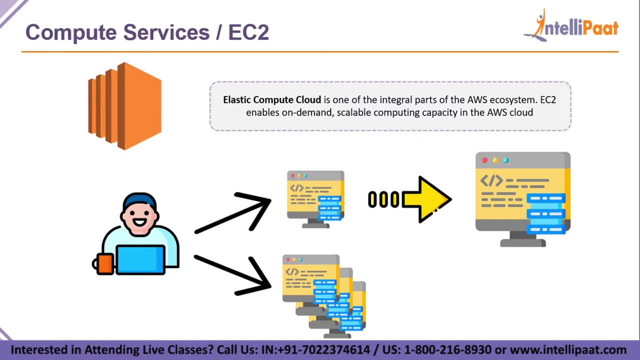 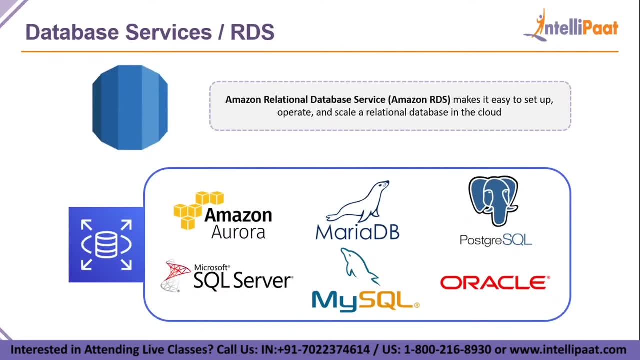 So this is easy to. I'll go more in depth in the hands-on And. And then comes RDS. RDS is a relational database service, So it is the. it is a service which gives you an uh relational database over the AWS cloud. 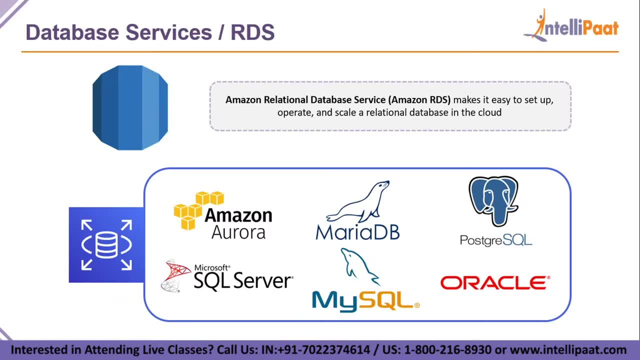 And these are the options. that is, MariaDB, uh, PostgreSQL, SQL Server, MySQL and Oracle And Amazon. Aurora is a sub feature of RDS where you can launch PostgreSQL and MySQL databases, but they will be much faster because it's a different architecture. 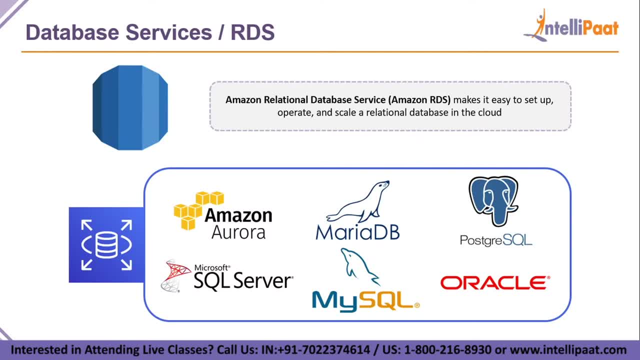 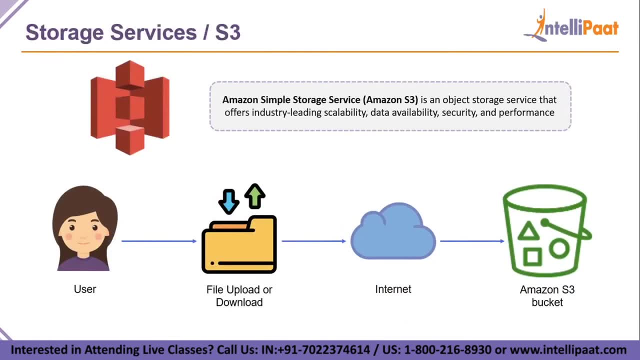 So we'll not go into that. We'll discuss that in a Session. So this is one of the service which is commonly used in AWS. and then comes S3, the most used AWS service. So S3 is a storage service. 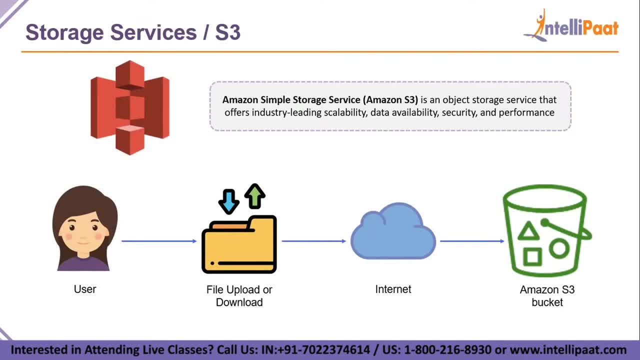 Basically it is a binary storage service. You can store anything you want. Everything will be stored as an object Uh. so you can store an audio file, You can store a text file, You can store a video file. So all of this uh is stored inside bucket. bucket is like a repository. 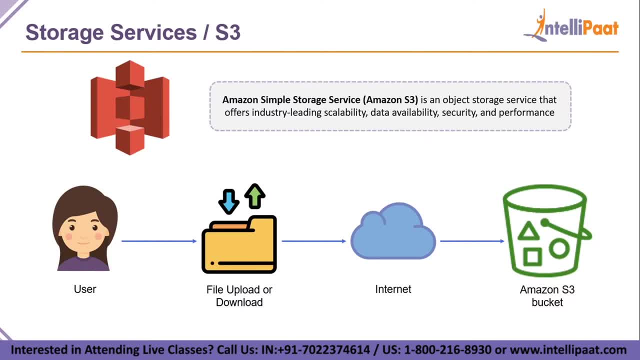 So in S3, there is no hierarchy concept, There is no File hierarchy concept, So there is no folders. Every single file is stored in the bucket. You can create virtual folders So it will seem like there is a folder, but it is just creating paths. but every single file is stored in one single bucket where you can just leave your hand inside and search for the right object and pick it up and use it. 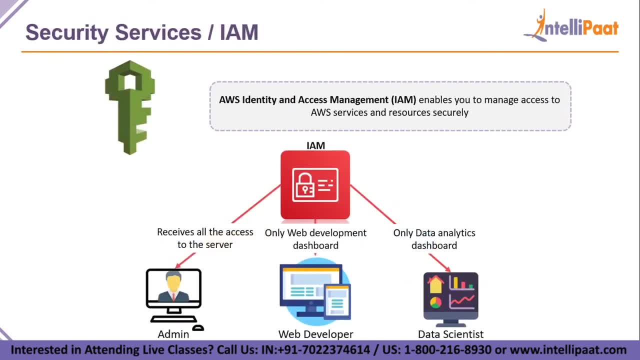 So this is the S3. And then there is IAM. This is a security service. So let's say, for example, you have an admin, cloud admin, You have a web developer and you have data scientists working in your company. Now for the admin, you want to provide all the- uh, all the access. 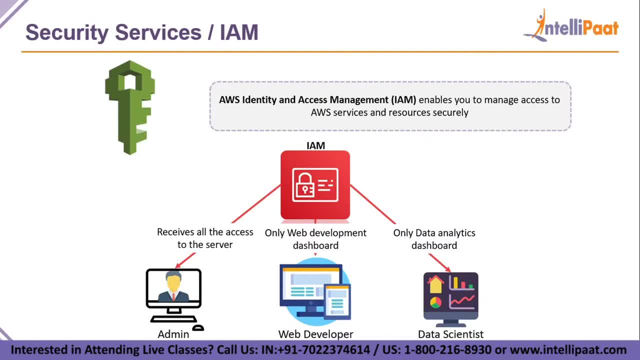 So this admin should be able to add users, remove users, give permissions to those users. second web developer: So you should provide uh permissions to this particular web developer only to the web development dashboard or to any services which he requires, like databases, uh EC2 or elastic bean stock. 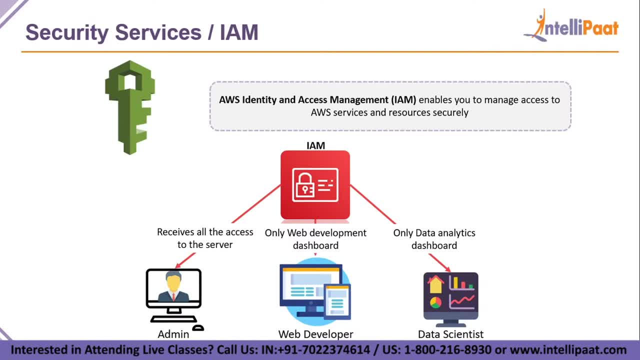 So you can give permissions to this web developer To only access these services and for a data scientist, you can only give access to uh the services which he requires. You don't need to give a permission for every single service in AWS. 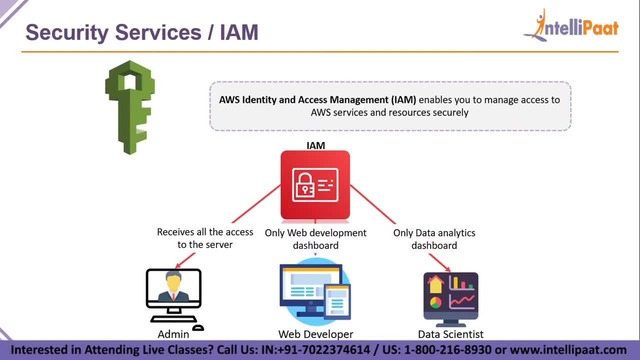 So if the data centers just needs five services, you can give permission for this data scientist to use only those five services and he'll not be able to use any other service. So this is why you use IAM to give permissions to create users, to create groups and you can also do a lot of other security. 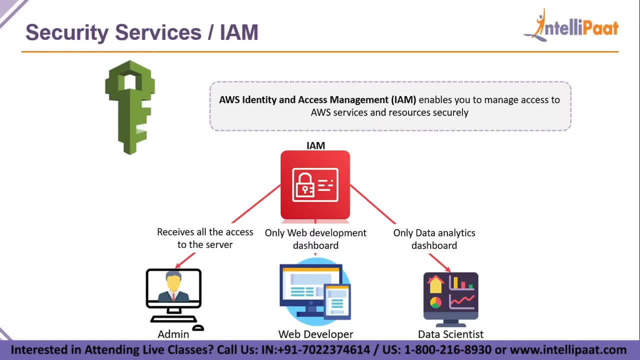 Uh, uh, security, uh features. It has multifactor authentication as well. So there is a lot of features. We are not going to go deep into IAM right now. Uh, this is one of the important servers you'll have to learn if you are going to start off with AWS. 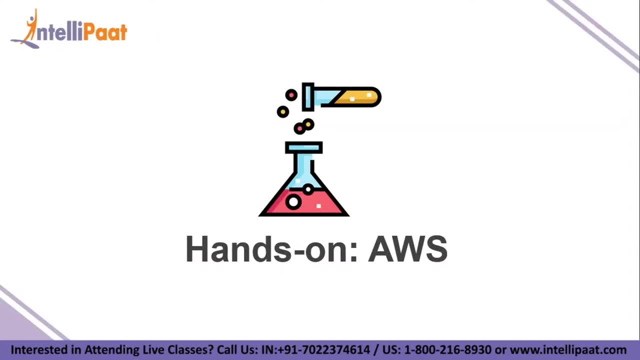 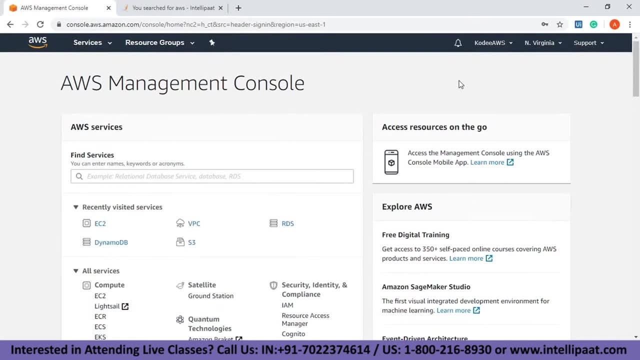 Okay, So now we've discussed these few services, Now let us do a quick hands-on. Okay, So I have already logged into my AWS management console, So this is how it looks and this is my username, And if you click here, you can see. 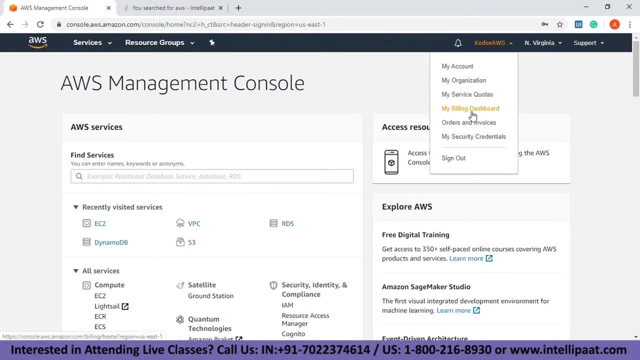 My account, my organization and then billing dashboard. here you can see if you have any bills or not and you can create billing reports and stuff. And here you can see your security credentials. I'm not going to go deep into this because it's a very huge concept. 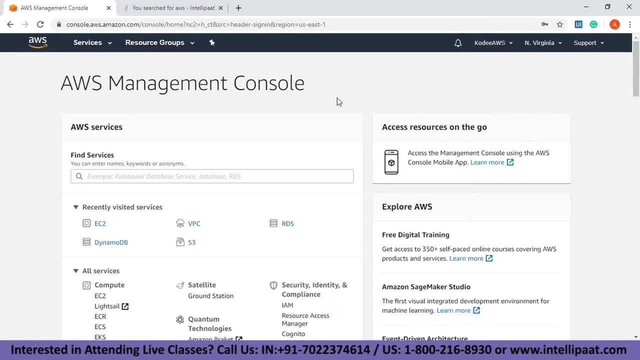 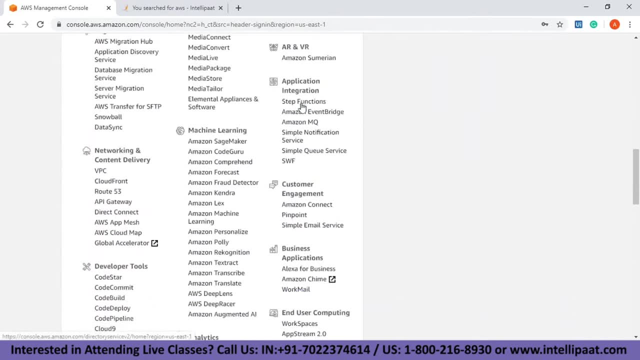 Okay, So now this is how your management console looks. So now you can see these are the recently visited services and coming down, you can see all these services available here And there are these many services. So learning AWS is not That you'll have to learn all of these services. 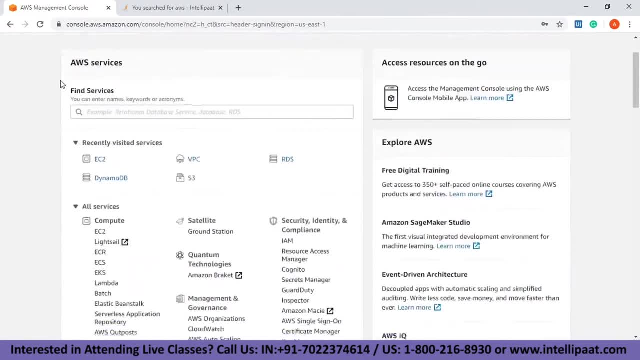 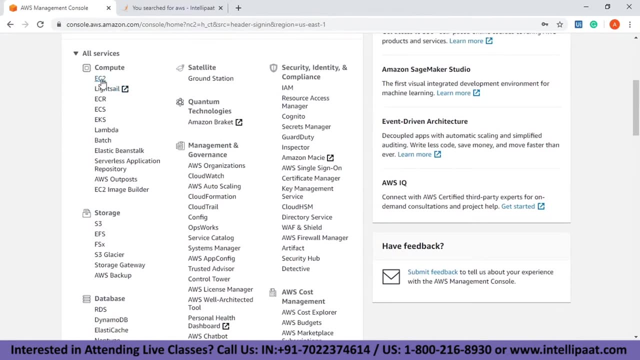 Nobody can do that. Even Jeff Bezos cannot do that. but you will have to know enough services for you to do something uh effective for a company. So let's say, you've learned EC2, you've learned uh uh databases. that is RDS. 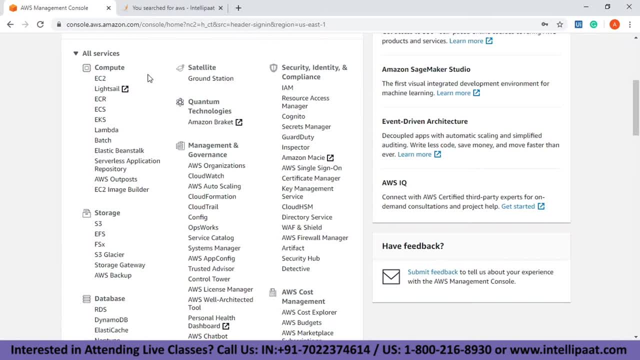 You've learned DynamoDB, you've learned S3, and, let's say, you've learned around 10 services. So now, with this 10 services, will you be able to create an architecture which can host an application successfully and also be highly available? 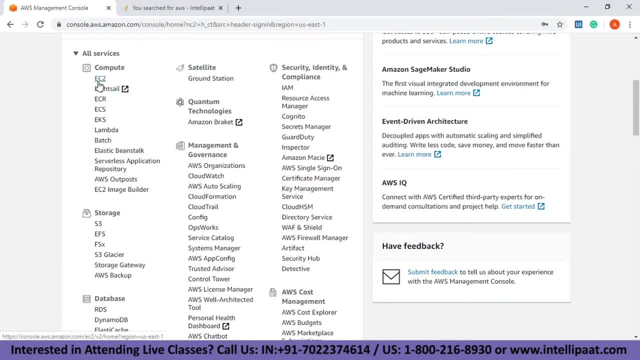 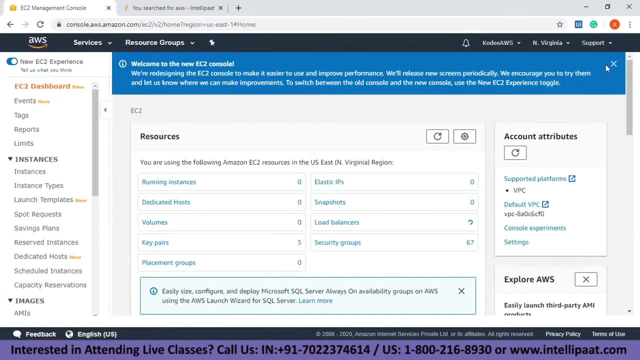 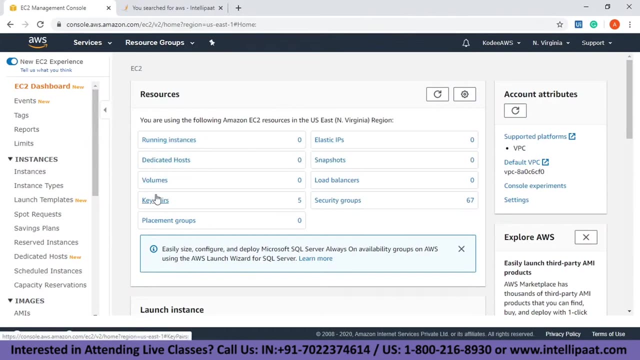 If you can do that, You can easily get a job in AWS. So now let us do a quick demo in EC2, because this is the most basic thing you'll have to learn first. So this is the EC2 dashboard. So now you can see running instances: uh, dedicated hosts, volumes, key pairs. 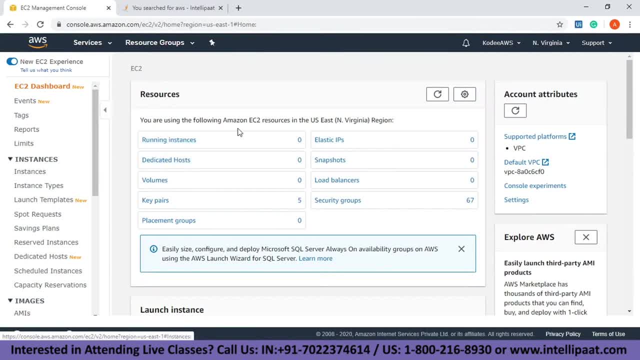 So I'll explain first: running instances. So this shows how many instances are running, that is servers. uh, in AWS, servers mean instances. Uh, we don't call them servers directly, We call them instances And volumes. obviously, if you are running a server for the storage purposes, you need a volume. 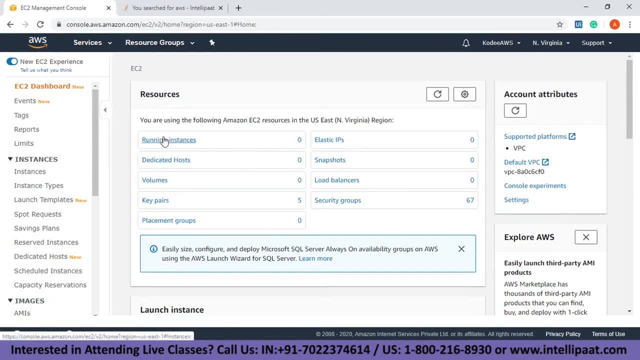 So it will automatically create a volume and to log into this particular instance you need a key pair. So the private key is with you. The public key is stored on the server, So while logging in you will have to provide the private key. 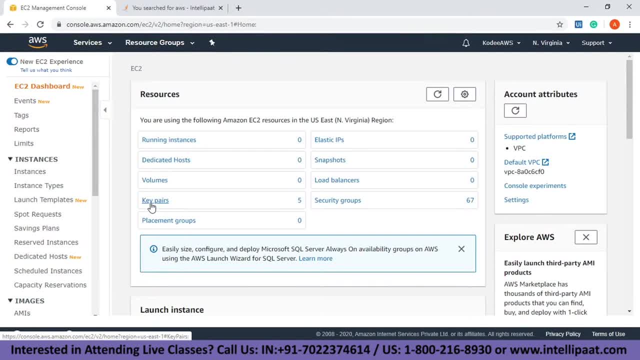 And if the private key is able to decrypt the public key, only then you will be given access to the server. So this is to prevent unauthorized access. So this is very- this is a very secure Method. So if you provide your private key to another person, uh, obviously they'll be able to log into your server, so you should not give access to them. 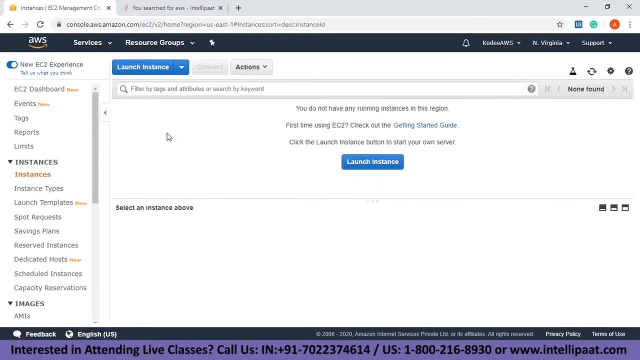 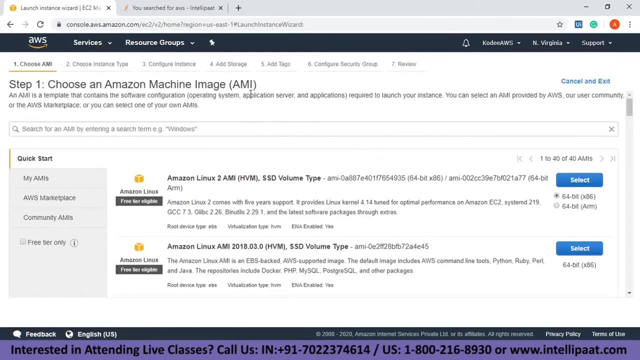 So now let's get started. I'm clicking on this, So I'm going to launch an instance, So I'm going to basically launch a server, So I'm going to launch an Ubuntu server. So first thing you'll have to uh, first thing, after clicking on launch an instance, is AMI, and AMI is uh, uh, let's say it is a copy of a server. 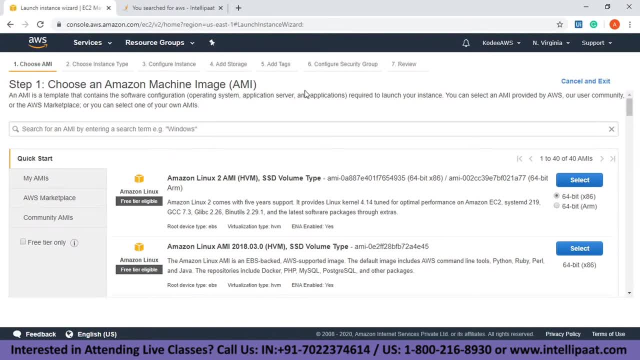 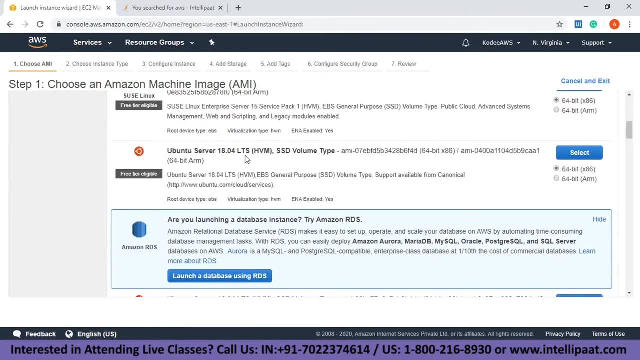 It is called an Amazon mission. So what is the purpose of an AMI? is so he? uh, let me come down. So here you can see an Ubuntu server 18.04 AMI. So this AMI is the? uh, it is like the ISO file which you use to create a virtual machine on your local system. 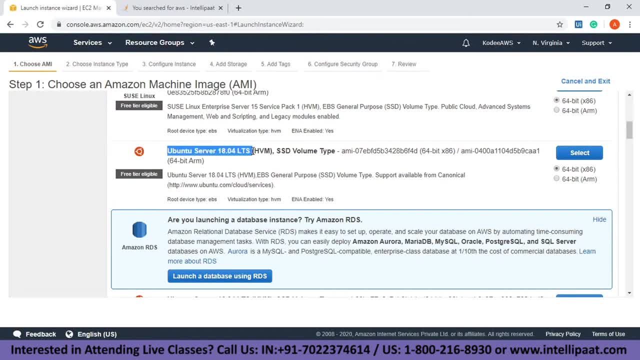 So this is the uh exact same thing, like an ISO file, but for a cloud system. So now, if I use this AMI to create, this AMI will already have all the configuration Files which, uh, which I require to create a Ubuntu server, to create a Ubuntu OS, to run an Ubuntu OS on a server. 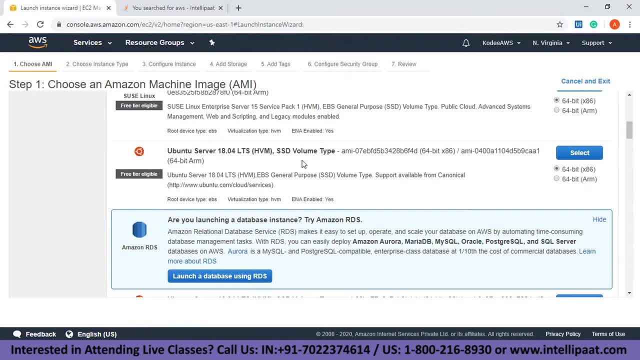 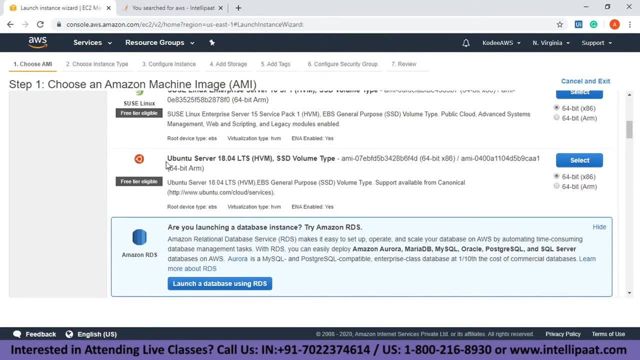 So this AMI will already have all the configurations. It will run everything for me and set up a Ubuntu server for me. So this is the most basic thing you'll have to learn about AMI. So if you use an Ubuntu server, AMI, uh, so you will get a Ubuntu instance. 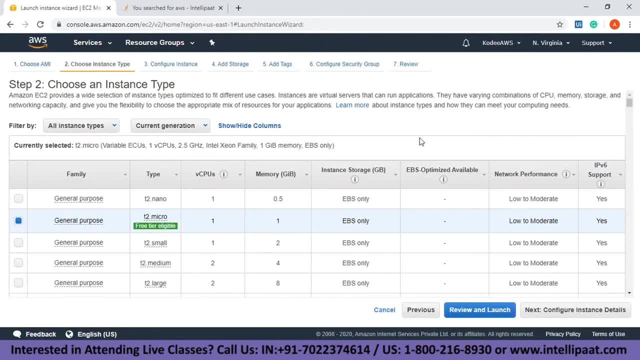 So now I'm using this. next is choosing an instance type. So there are so many Instance options, guys. So first it will automatically select the free tier eligible uh instance type because, for practice, uh, you don't need to go ahead with a large one. 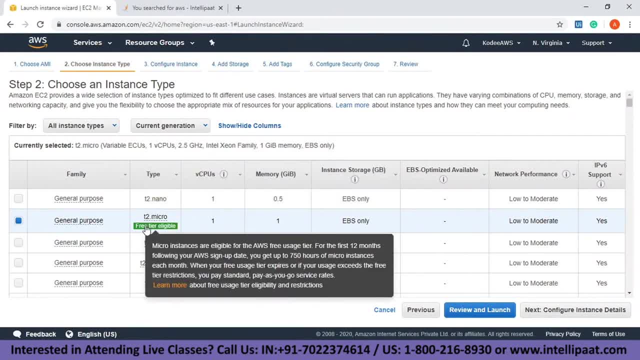 Free tier eligible is fine. Why free tier eligible in the sense you don't get billed? We'll discuss about this later. Uh, there is a free tier uh capability in AWS, So you can see, this particular uh free tier instance will give you 750 hours of free usage. 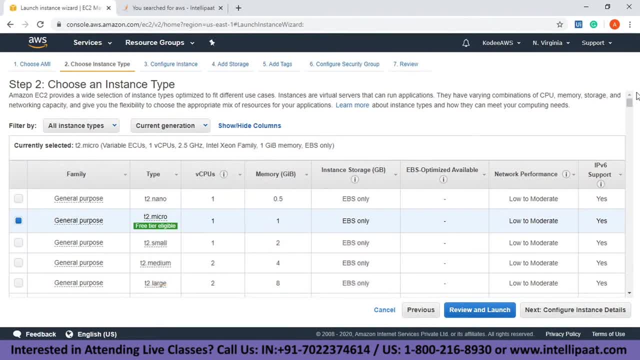 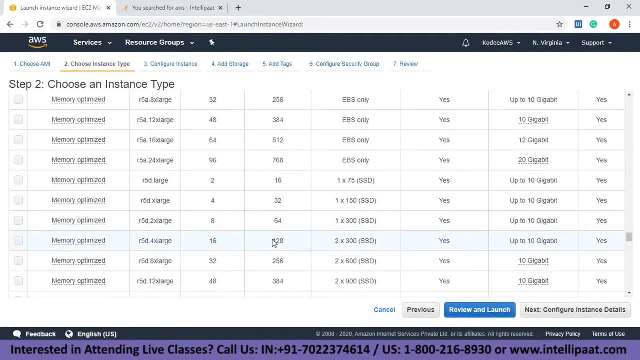 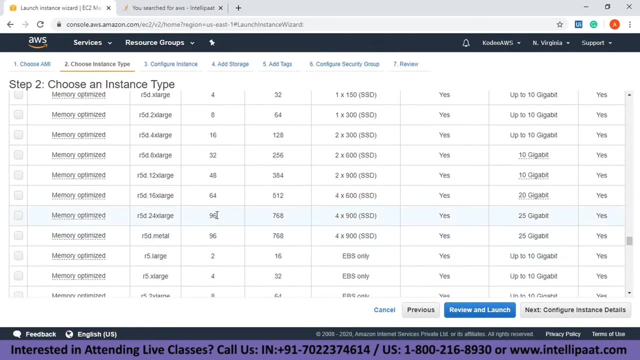 You don't get billed for that 750 hours, So let's go ahead with it. But there is also huge servers, So you can see if you want. uh, let's say, if you want a server with 48 virtual CPUs and 384 gigabytes of Ram, or if you want a server with 96 virtual CPUs and 768 gigabytes of Ram, you will still get a server like that. 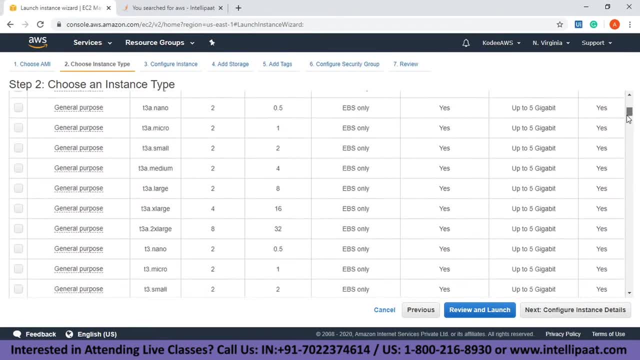 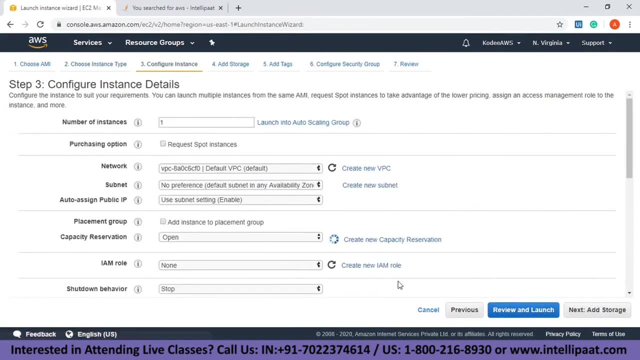 But these are very expensive services And if you even run them for a minute you will get billed a lot. So don't do that. Go ahead with a free tier eligible server. Next, configuring instance details. I just need one instance, So I'm not going to go to the network and subnet concepts. 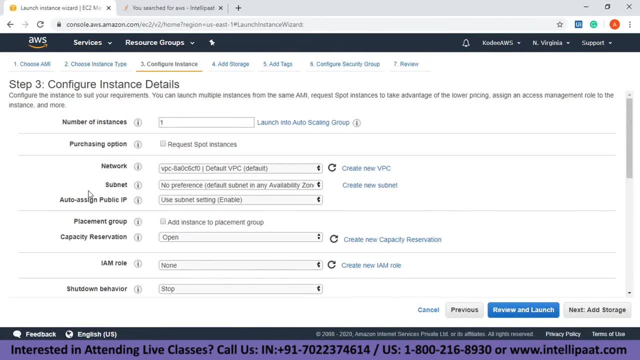 These are uh again. huge concepts are coming down here. So enable, so it'll already be enabled, So do not disable it, because we are launching a public server, So I should be able to launch a website in it. So to check out the website in your, uh, in your browser, you need a public IP address. for the instance, 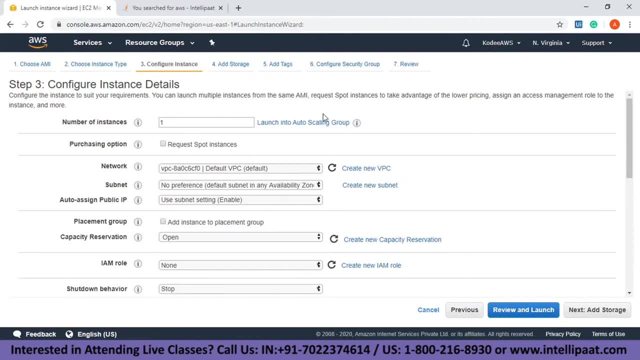 So To get a public IP address, You Will have to enable auto assign public IP, Otherwise you will have to creating the instance. You will have to manually uh assign one. So now this is done. Next, eight GB of storage is more than enough for my Ubuntu system. 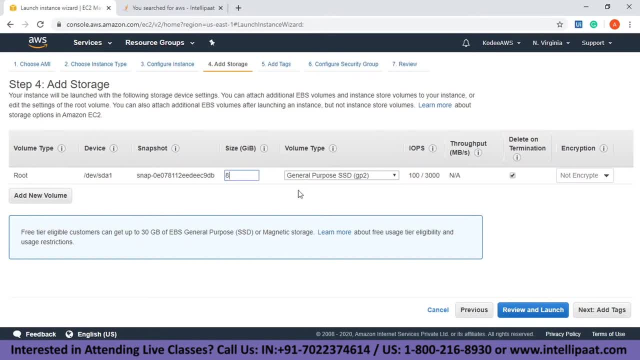 If you want more, you can just change the size over here and this will be your root directory. You can create one more volume If you want to. you can create multiple volumes and that is no issue. Next tags: tags are basically two uh trial. 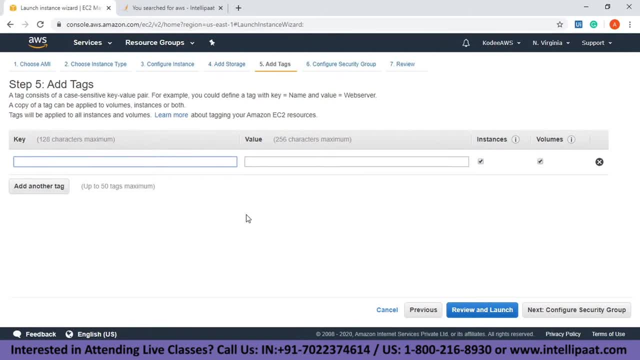 So let's say you have, uh, 10 different instances And in that five different instances are for a website and other five are for general purpose. You're just having them for other issues. So now you can just tag all that five servers which are for your website as web servers. 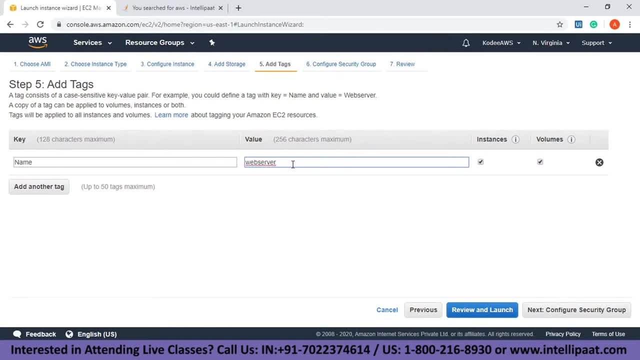 And So you can give it web server, And then if you just type in web server in the search bar, you will get all those five instances. So this is just to keep track of it. So you can Give a tag if you want to, and it is not, uh, it is optional. basically now, SSH. 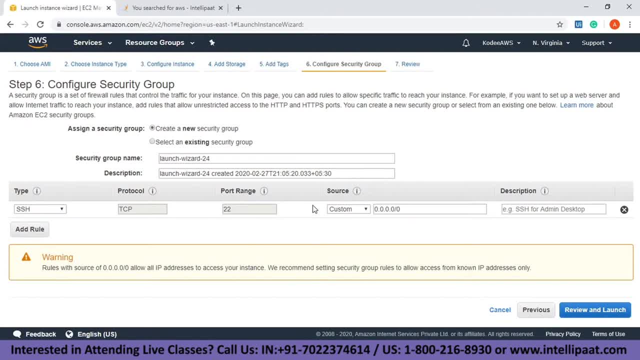 So to SS, uh, sorry, to SSH into an instance, uh, you will have to provide the SSH permissions. So the port number 22 is for SSH. that is secure shell. So why secure shell in the sense? Uh, so, as I told you, uh, you will get a key pair. 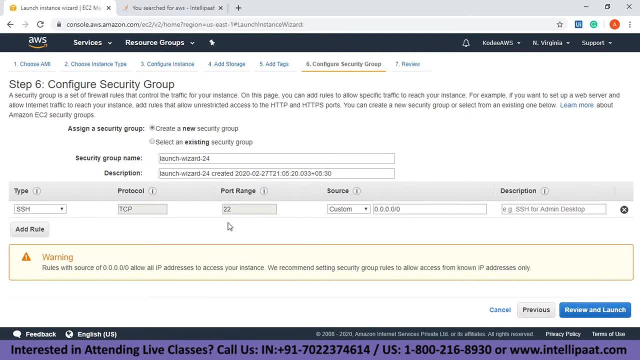 The public key will be on the server. The private key will be on your system, That is, your local system. So now what you'll have to do is you'll have to provide your Private key to the server. but how will you provide it? 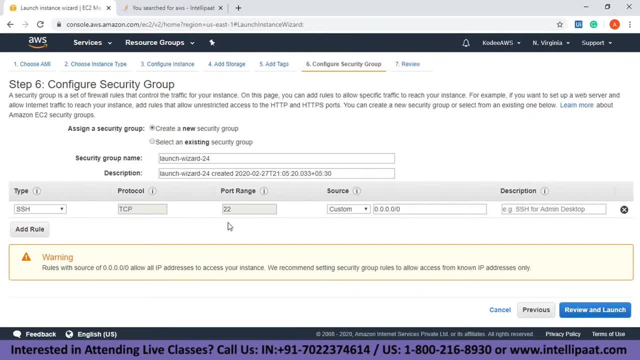 So you will provide it through a secure shell. You'll be providing it through SSH, So for that you need SSH and for logging in you need a service called putty. So I've already have it installed And if you want that, it's pretty simple. 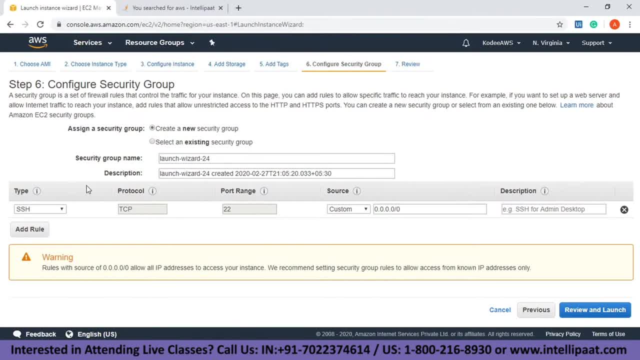 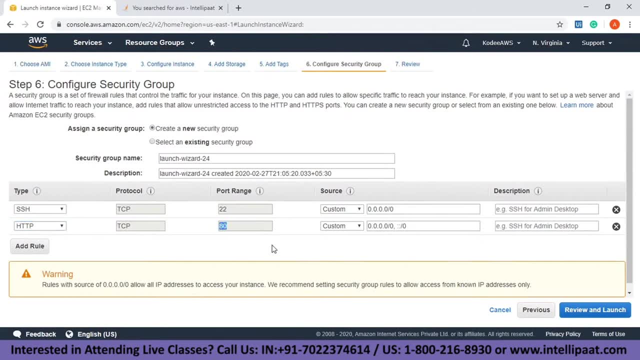 Just type in download putty and you'll get it, So no issues. And also, I'm going to launch a web server, So I'll just uh go HTTP, So port number 80, because I'll be launching a web server which requires the port number 80.. 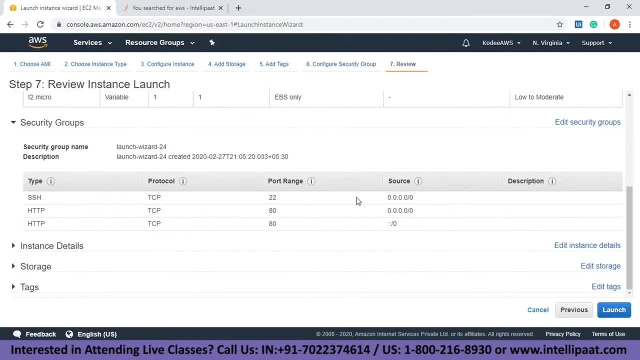 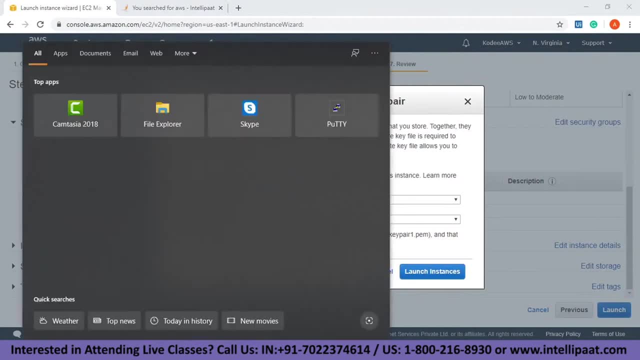 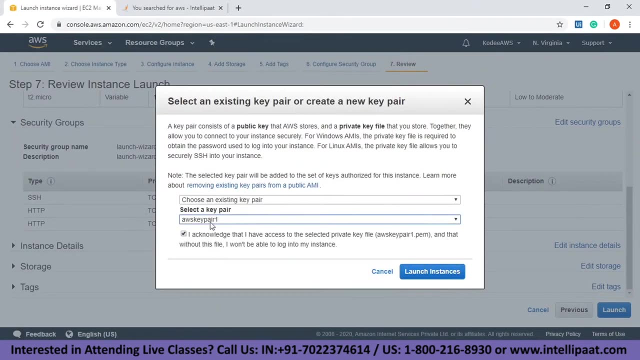 So I'm just using it next and then review your server and then click on launch, So I think. so I have this keeper. I'll just check once I it's not available, So I'll create a new one. Yeah, So, uh, I'm creating a new one. 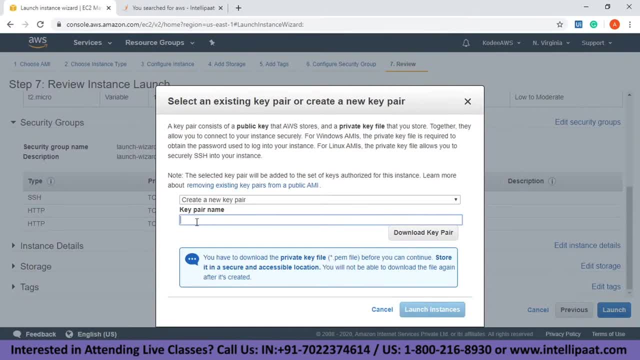 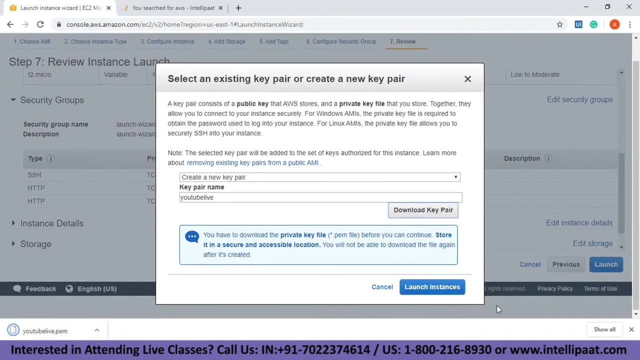 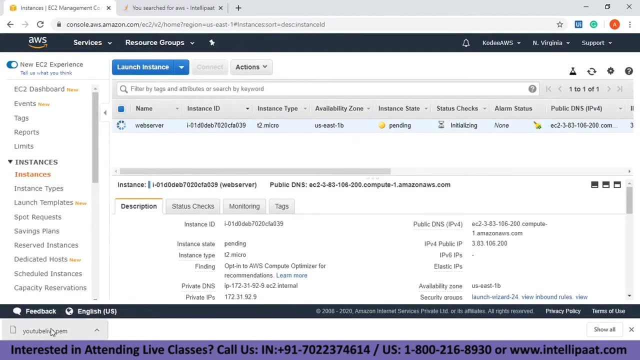 I'm giving a name for it as uh YouTube live and download it, So it'll be in my downloads, Let it be So. now I'm launching the instance. So now the first part is done. The second part is to convert your uh PEM file, because if you are having an uh Ubuntu system or a Linux system, you can just use the PEM file directly using the SSH command. 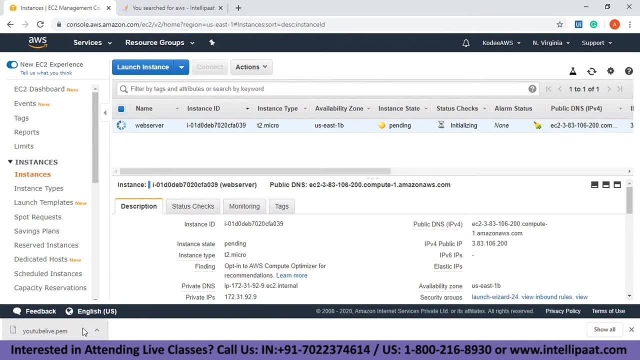 But if you're using a Linux system, you will either have to have a Linux emulator or you will have to convert this PEM file into a PPK file- PPK in the sense: putty private key file, because you're using putty. 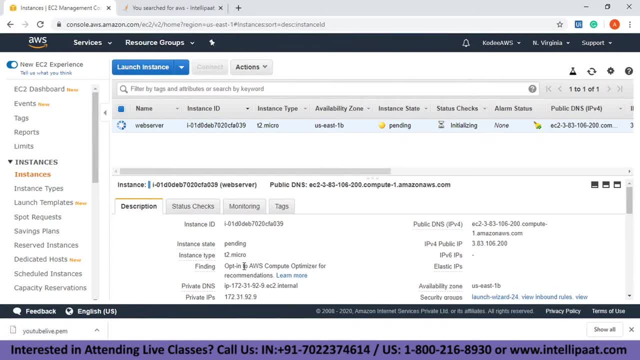 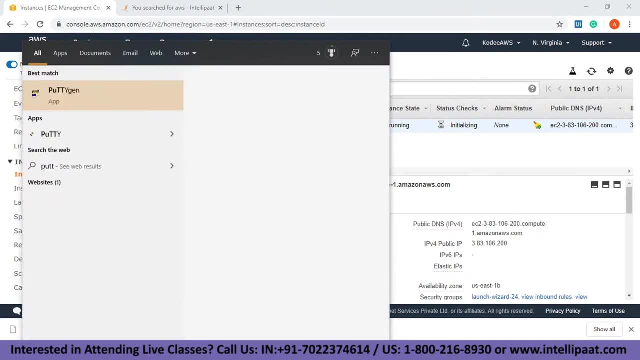 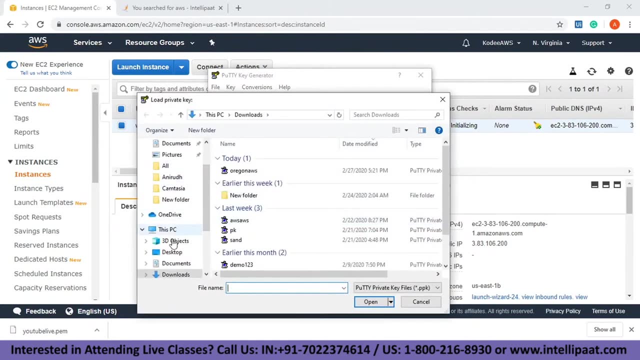 To do SSH. So putty only accepts a PPK file, so that you will have to convert. So if you have downloaded and installed putty, it'll also install a software called party gen. So in petition, uh, go to load and go to downloads, and it's not available. 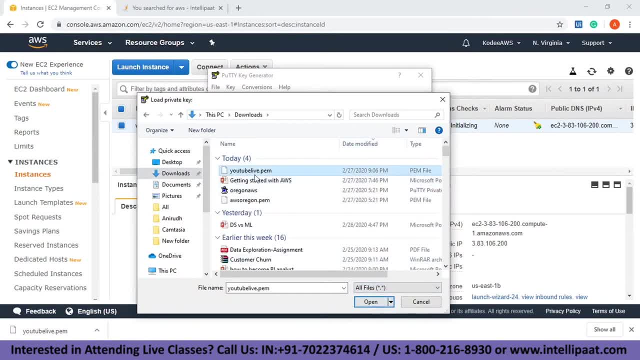 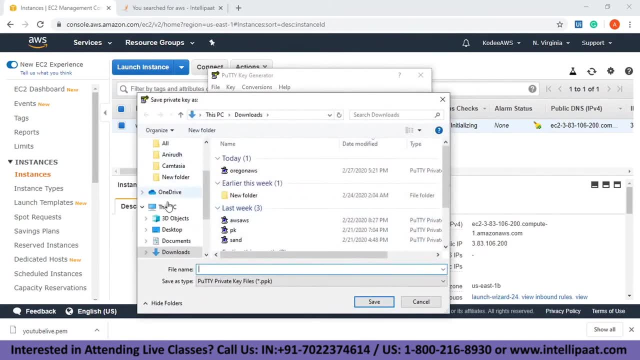 Oh, sorry, It's searching for party private key files, all files, And you can see the YouTube lab dot PEM file over here. I'm opening it and I'm saving the private key and I'm saving it in my desktop as YouTube live. 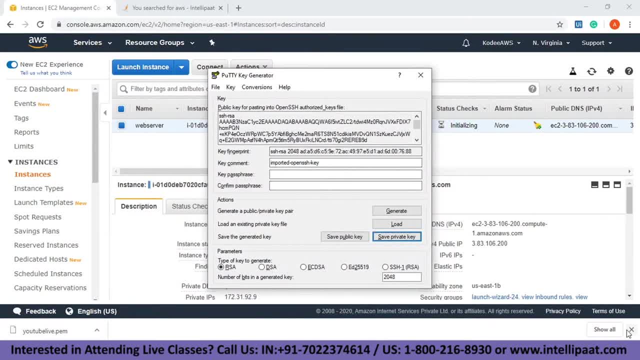 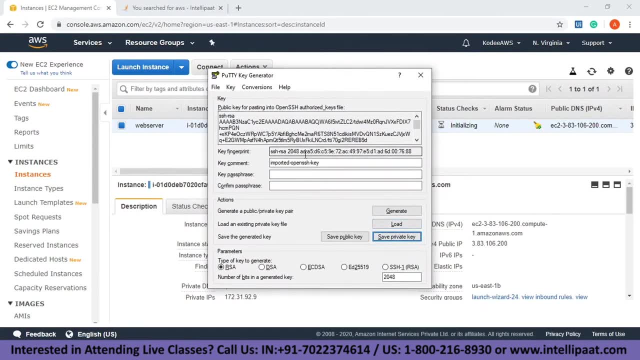 You can give it any name. I'm giving it the same name. So right now I've converted it using the party gen software. So just load your uh PEM file and it'll automatically generate a private key. then save the private key and close it. 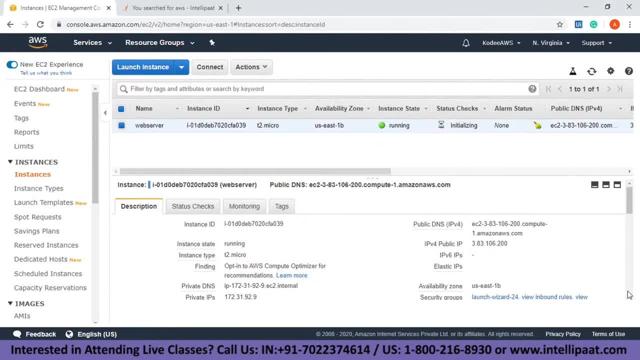 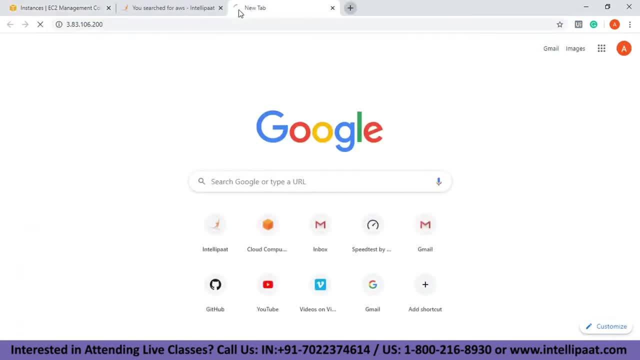 So done. Even my instance is running right now. So one more thing I wanted to show you is: you can see a public IP address over here. Okay, So now if I copy this and paste it here, you will not see any website running, because I don't have a web server running in my instance. 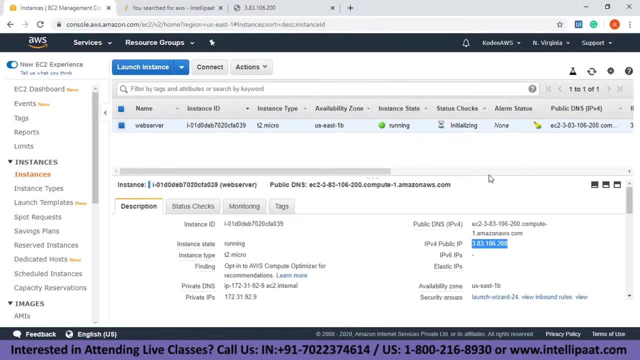 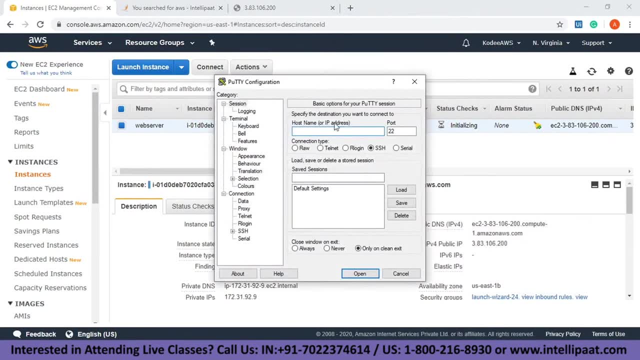 So once I run it, once I run my web server, you will be able to see that. So for that you'll have to log into your instance. So copy your public IP open party. paste your public IP under host name or IP address. 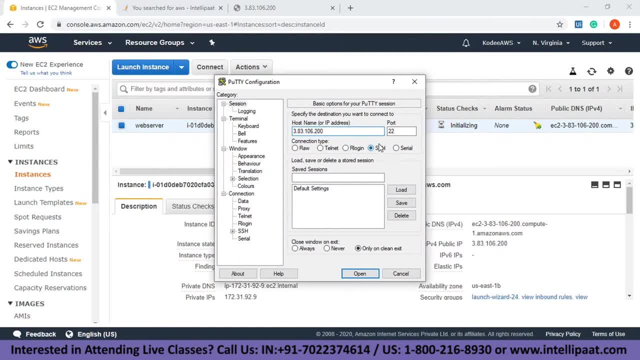 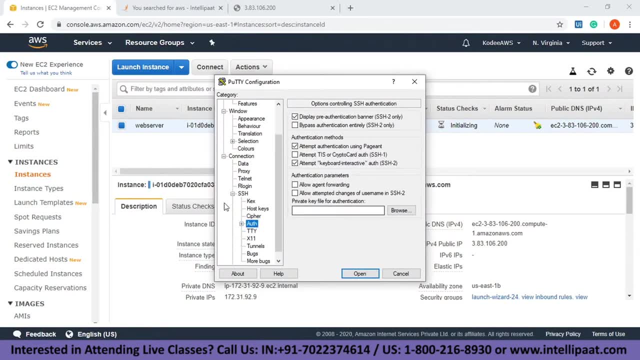 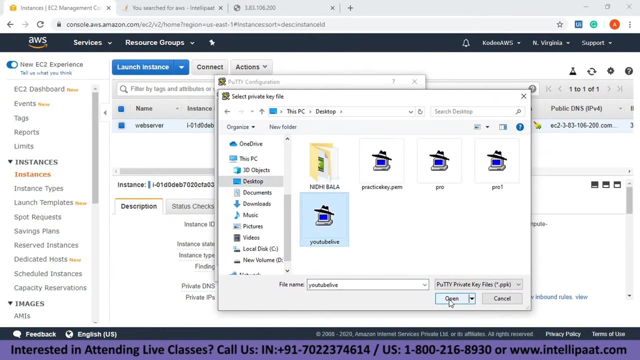 Port number is 22. connection type is SSH, which is secure shell. Then Go to SSH, expand it. go to authentication. under authentication, click on browse. choose the private key file, which is, uh, basically connected with your instance, because my instance has the public key of YouTube live private key. 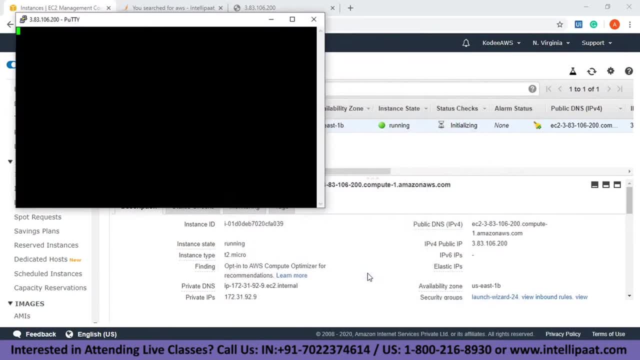 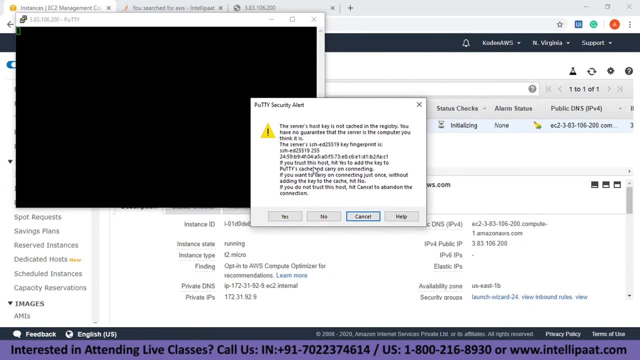 So I'm going to choose that and I'm going to hit open. So, if you get this particular security alert, uh, so basically, uh, it means that, uh, you trust this host. If you trust this host, just click yes. 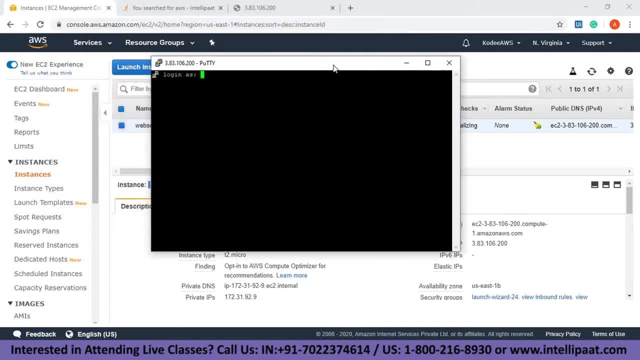 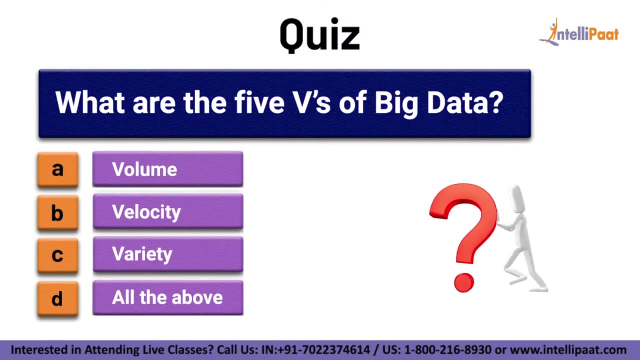 And you'll be given permissions to log in. So I've launched a Ubuntu system. So for me the username would be Ubuntu. If you have launched a Linux system, the username would be EC2 user. Just a quick info, guys, test your knowledge of big data by answering this question. 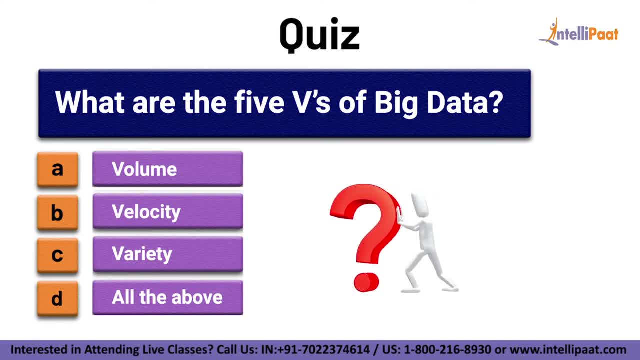 What are the five V's of big data? A, volume, B, velocity C, variety D: all of the above. comment your answer in the comment section below. subscribe to Intellipaat. know the right answer? Now let's continue with the session. 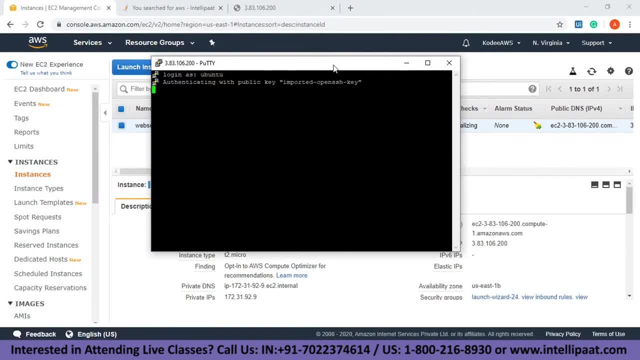 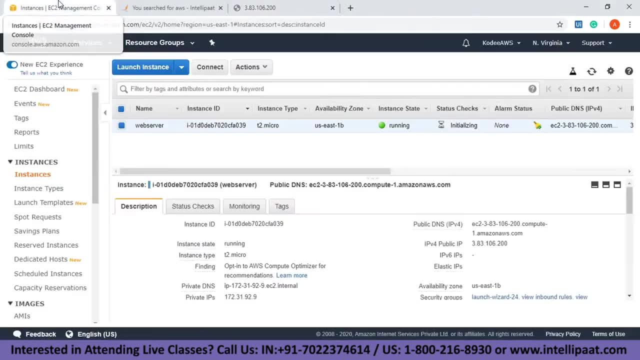 So this is the Ubuntu system, So I'm going to go with Ubuntu and it'll log in. So I'm successfully logged in. Okay, So now, right now, there is no web server, So what I'm going to do? I'm going to run a web server. 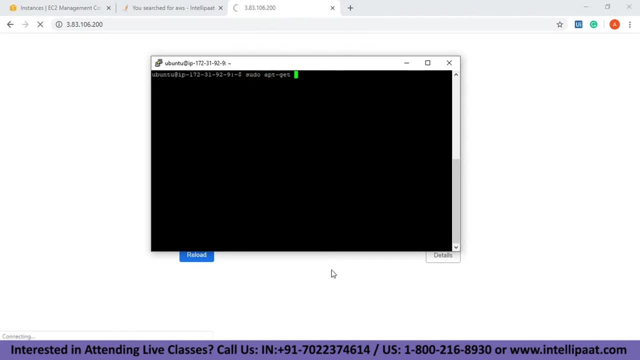 So there's a web server called Apache two So you can learn about that later. You can just do a Google search of Apache two and learn what is it, because I'm not going to go into Apache two, So it is pseudo APD. get install Apache two. 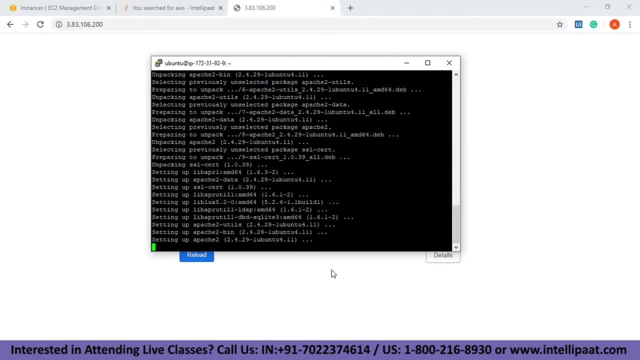 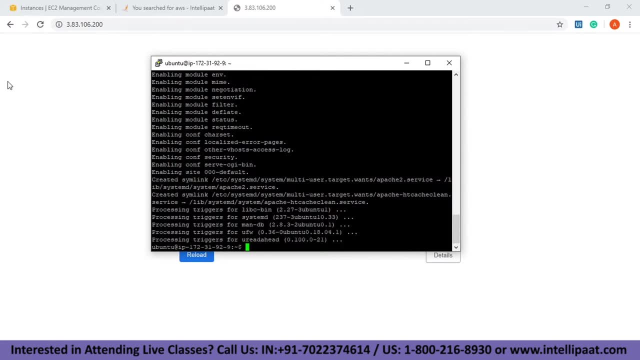 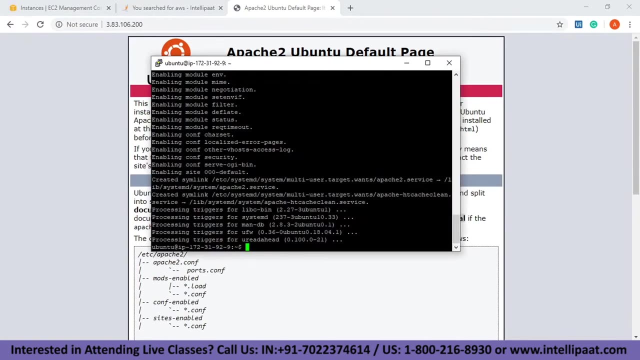 Yes, And now it'll install a web server. So once it is installed successfully, if I refresh this, you will be able to see the web server. You will be able to see a default web page. Let me refresh this. And now you can see a default web page running in my public IP, which is my instances public IP. 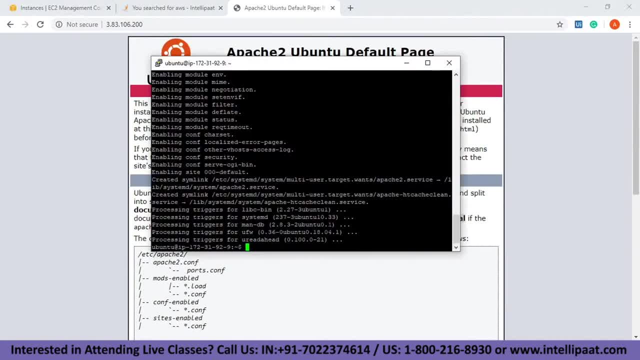 So where is this file? So let me show you that as well. So now let me open this folder. So under VAR, under WWW and inside that, there is a file folder called HTML, And if I do an LS, you can see an index dot HTML file over here. 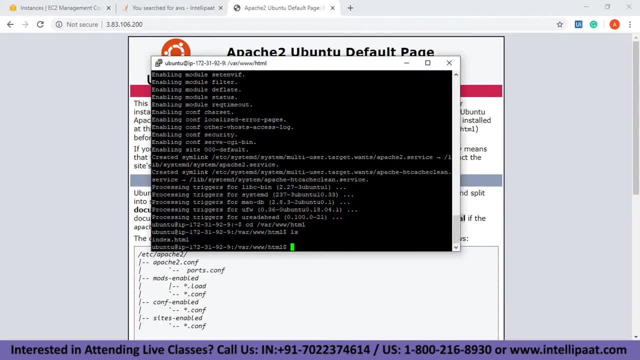 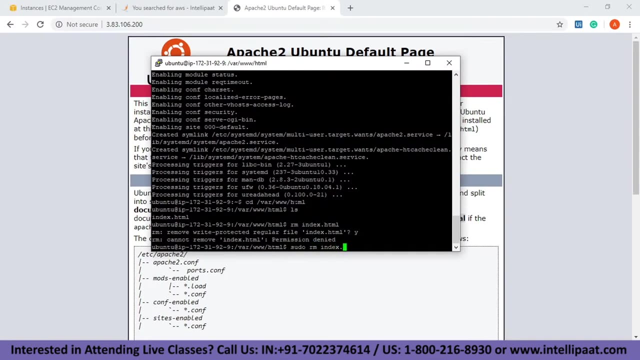 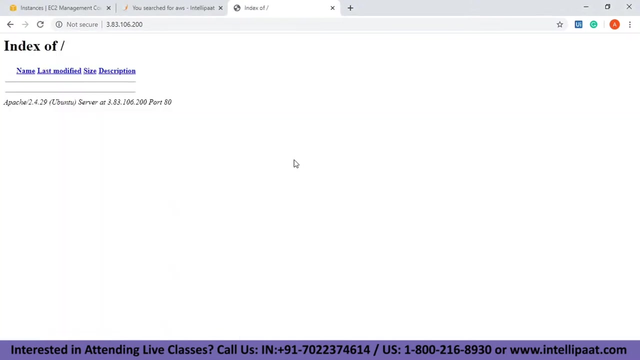 So this is that file, So let me remove this file. So I don't have permission, So I'll have to use pseudo. So now there is no index or HTML file, So now you can not see the webpage. Okay, Now let us create a index dot. 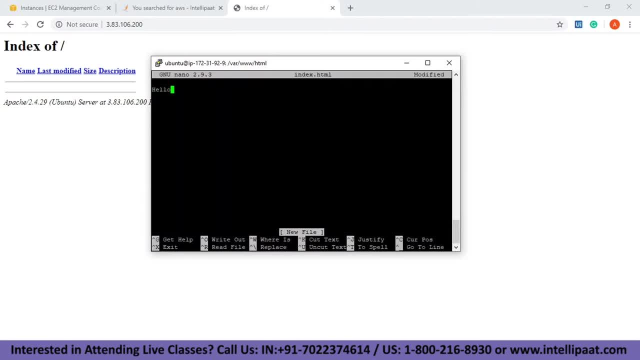 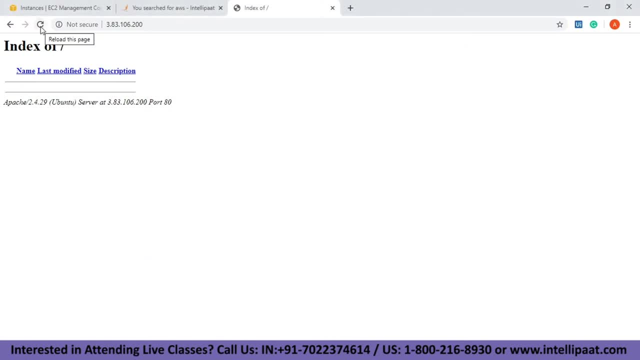 HTML File. I'll just type in hello world and save it. Okay, Now if I refresh this, you should be able to see the hello world page. That is, I've successfully hosted my website on my own server, So this is how you do it, guys. 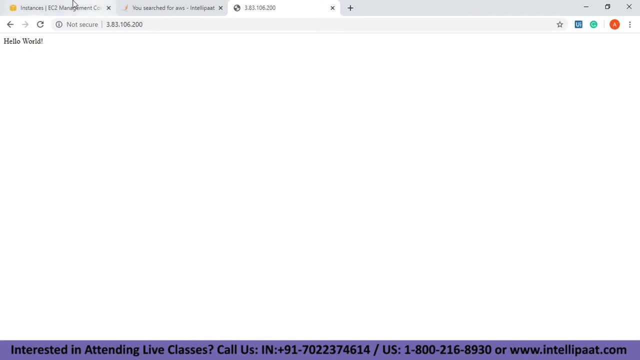 You can easily get started with AWS. So I think you understood the easy to part and it's pretty easy to get started with it. And let me go back to the slides. So we've done The hand On Introduction to big data right. 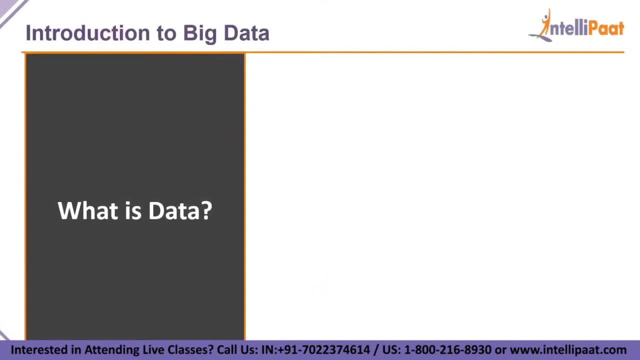 For those of you who are completely new to the entire concept of big data, we're going to be going through this step by step, So understanding the concept of what data means in the first place is extremely important, because these days, data is quite a generalized term. 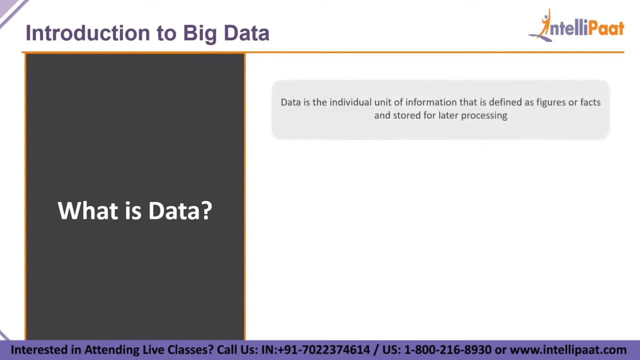 It actually covers a lot of things, but there are categories associated to it. So, firstly, by definition, data Is the individual unit of information that is defined as figures or facts and is stored for later processing onto your computer hard drive. It could be anywhere, essentially any storage device, and it is divided into three parts. 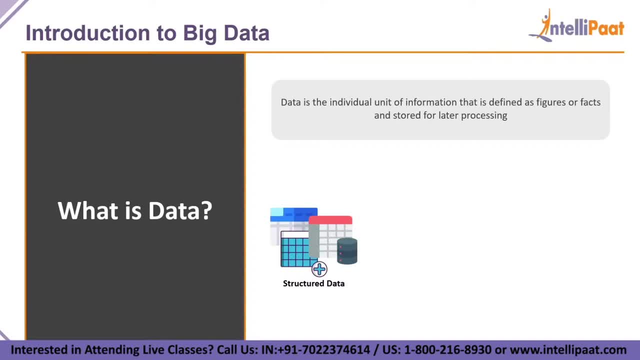 So the first is structured data. Now, for those of you who are coming from an SQL background, the sort of data you're quite familiar with, this is the data that is present in SQL tables with proper rules and proper columns. Right, It's in proper queryable form, so to speak. you can query it pretty easily. 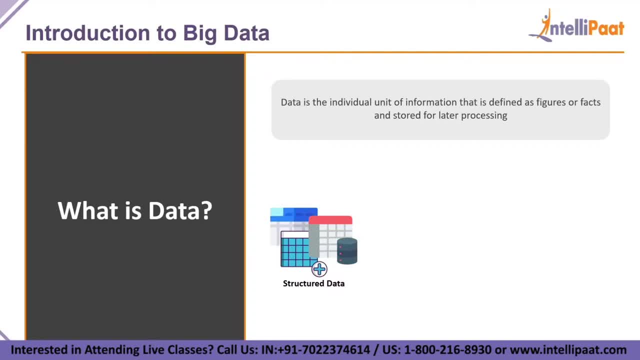 There is structure to it and it is the most organized form of data that exists. Secondly, we have semi structured data. Now, this is a combination between completely random order of data and some sort of a structure associated to it. So, for instance, you have files like JSON files, CSV files, and those files have a particular format associated to them. 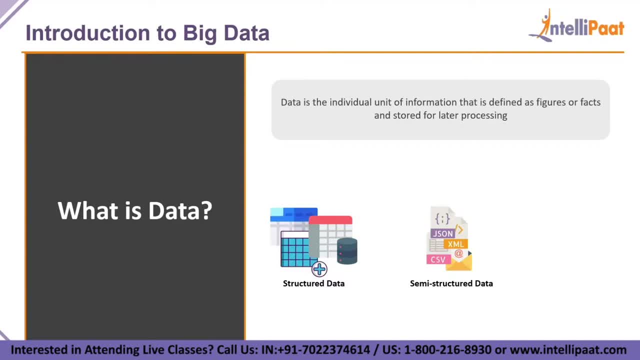 For instance, in CSV files, which is an abbreviation for comma separated values, all of the data records are separated by commas and delimited by line changes. So essentially it mimics an SQL table with proper rules and proper columns, except it is in the form of a file. 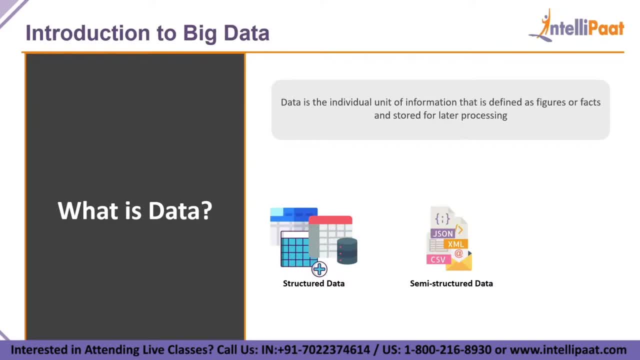 And you have just provided commas between the data records to differentiate between the column. So that is what essentially CSV is. So in a file format it does have some structure to it. That is why that file format is called a semi structured file format and the data is called semi structured data. 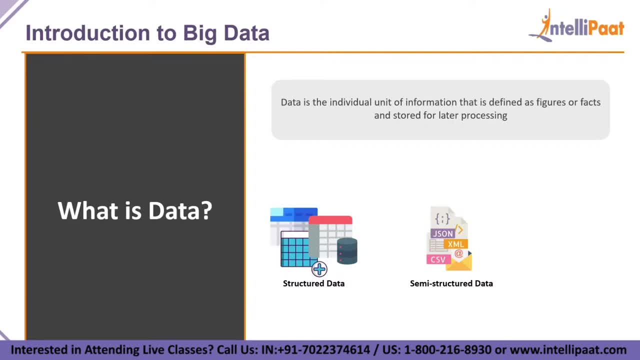 And so is the case with JSON and XML and other semi structured data sets as well, And finally, we have unstructured data. Now, this is completely random in nature, As you can see. the examples that we can see are JPG, PDF, MP3.. 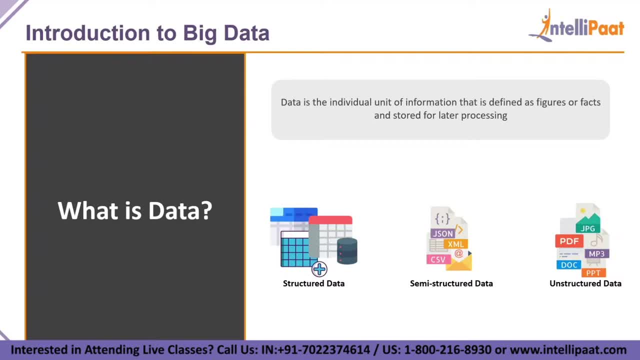 So if you were to convert these data formats- Files- into text files and see the contents of those text files, you will see completely random order of information. it would make absolutely no sense, right? So that is what unstructured data is now. unstructured data is the most challenging data because to derive some structure out of it, you need a lot of computing resources, you need to understand how the data behaves and a lot of other aspects as well. 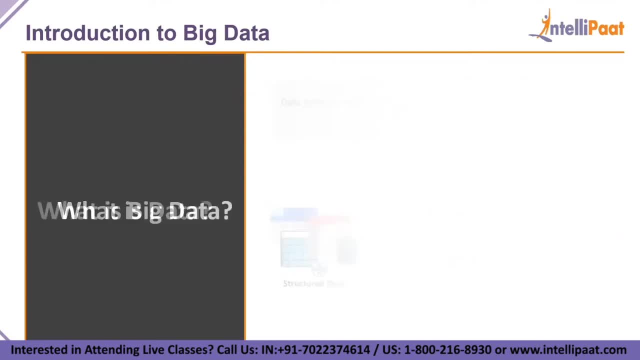 So these are the three types of data that exist Now. big data has a definition. It is, it has a distinction. it simply does not mean that the data is extremely large in size. there are other criterias as well, right? so there are five criterias in total, and these are called the five V's of big data. 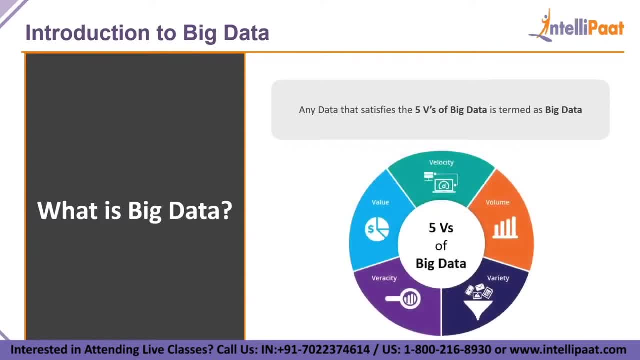 So what are the five V's of big data? These are the five V's of big data: velocity, volume, variety, veracity, value. let us go through them one by one. Velocity: the rate at which the data is being. 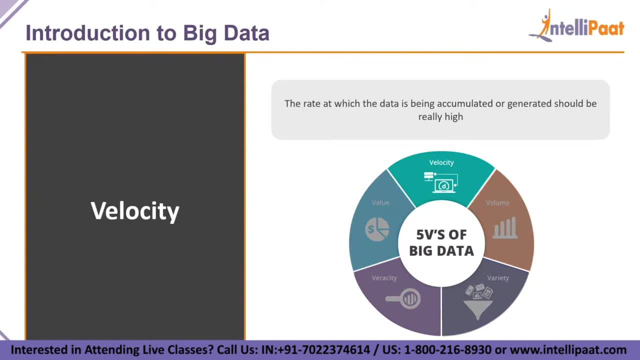 accumulated or generated should be really high right. So say, for instance, you're working for an organization where data is coming in in real time, say per minute or per hour, per second. in that sort the data has a really high volume per second or a really high volume per minute. 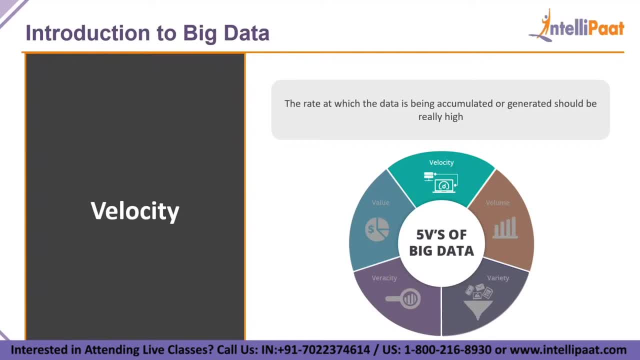 In that case the rate of the data is really high. the rate of the accumulation of data is really high. So in that case it satisfies the criteria of velocity. So if it's anywhere between the high and the low it's really high. 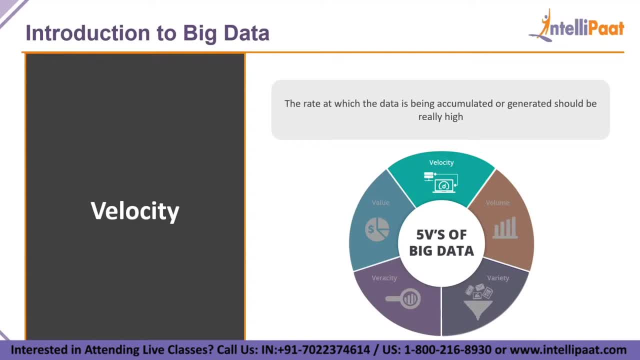 Higher- gigabytes to terabytes to petabytes in a day. then you can account for velocity in that particular aspect And then we have volume. Volume means the most obvious thing about big data is that it's big. So anywhere you're storing big data, it should be extremely large in size, from terabytes to petabytes. that accounts for volumes. 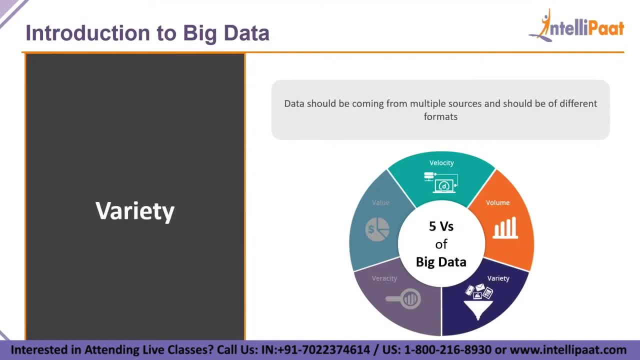 Next, we have variety. Variety means that the data should not be coming from a single source and the data can be of multiple file formats or data formats as well. so, for instance, if you're working for a big e-commerce organization like amazon, so you have something like user data, you have something like sales data, so both are. 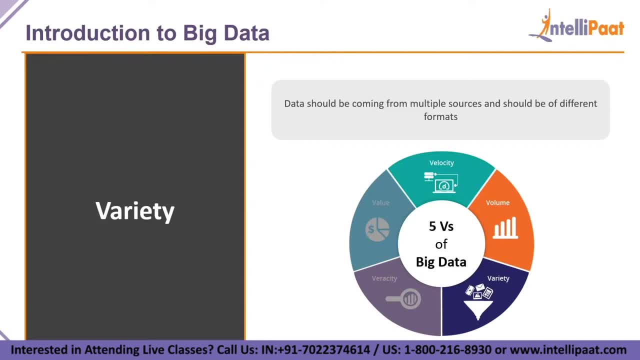 two separate databases- right. but for people in the higher management, they need to see this data all collaborated together- right, so they will combine that data and see it together. and basically, when you're combining data from multiple sources together and seeing it in a combined view, you're accounting for variety as well. so any big data case, you need to have variety in the data as. 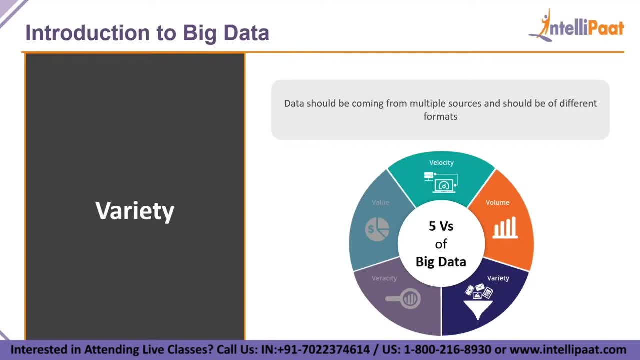 well, the data cannot simply be of a homogeneous source. and then we have veracity. veracity means that the data should not be error free. so basically, that means that the data should have some noise in it. data should have some missing values in it. the data should have some wrong or inconsistent values. 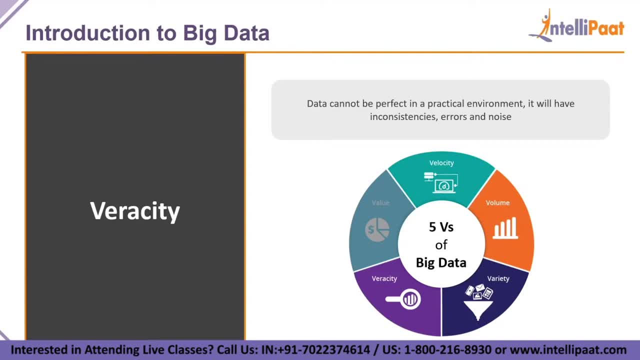 in it. so that basically means that any data set that you'll pick that is based on real world values will always have inconsistencies in it. right say, for instance, if somebody is generating a data set out of facebook, so a lot of people on facebook have created fake accounts as well with fake. 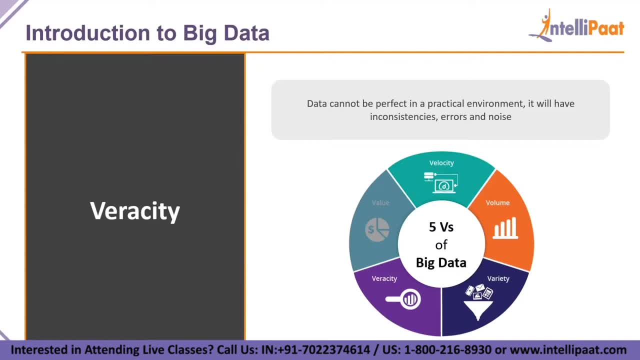 details, right? so if you were to perform a marketing survey, right, you cannot actually look at these fake accounts and decide your marketing strategy based on that. you need to be careful about that. so the data should have veracity as well, because any real world data set will have that and, finally, value. so whatever columns you're picking, whatever data you're, 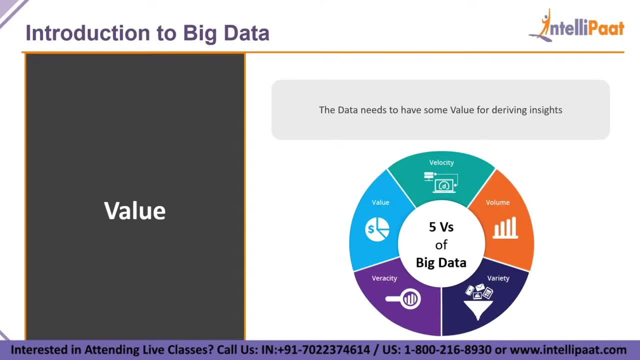 picking should have some value to it, right? say, for instance, you have a data set filled with complete random numbers- 100 random numbers- and you have a data set which has the academic records of students in a university, right? so you will not consider the data set which has 100 random numbers? 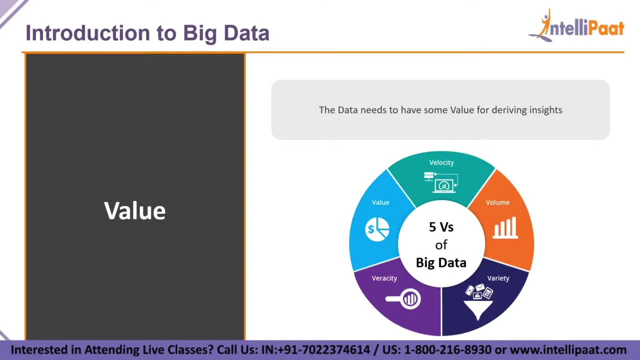 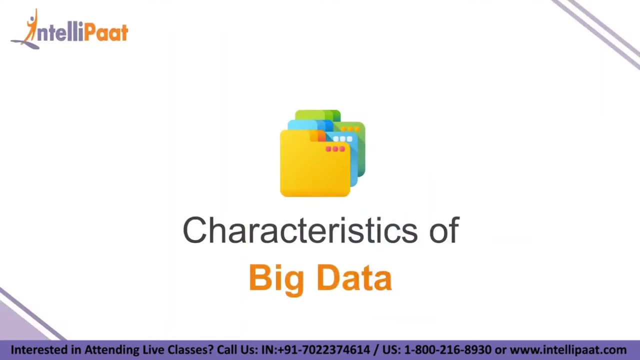 as the data set with value, because you cannot create any analytical model with it, because it is just a set of random numbers, they don't have any value in the real world sense of things. so now that we understand the initial concept of big data and the distinction between data, 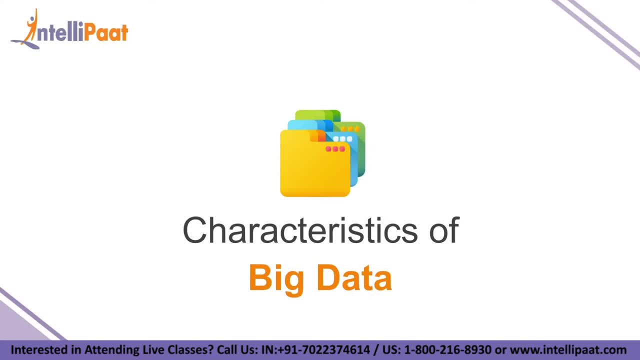 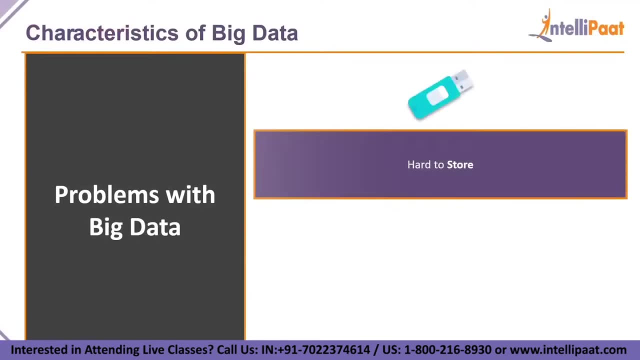 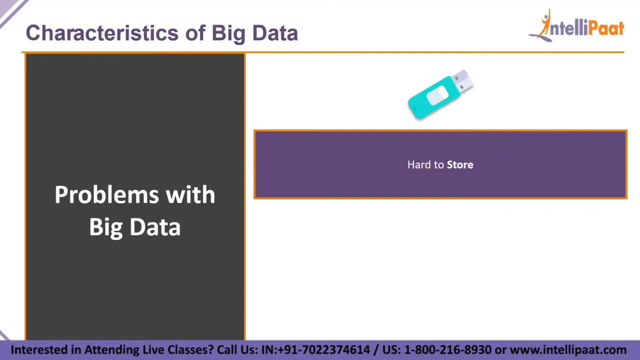 petabytes, and these days we hardly have 500 gigabytes to one terabyte of hard drive spaces in our laptops or in our working computers right at maximum we have two terabytes right. so it's quite a difficult issue to store big data on those computers right. so that is the first problem. 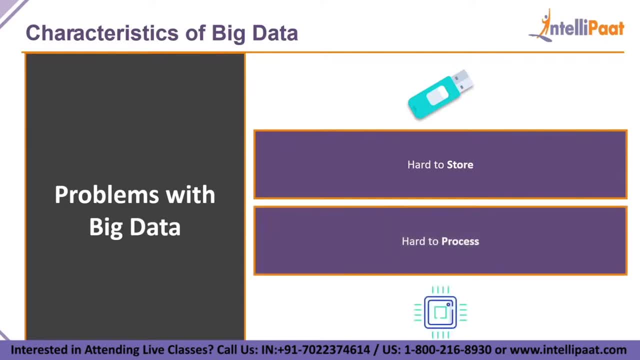 that we have with big data. the second problem that we have is that it's really time taking to process right. so, for example, if we have a big data and we have a lot of big data and we have a lot of records- right- so, for instance, if you have a data set with 10 records, 10 rows, it's very easy to 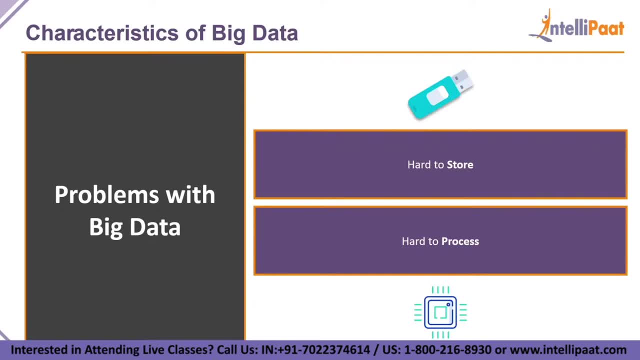 process, it'll all happen almost instantly, right? but if you have a data set with the billions of records, right, which may be the case in big data, then obviously it will take a lot of time to process that, maybe days to months, depending on the processor speed that you have, depending on 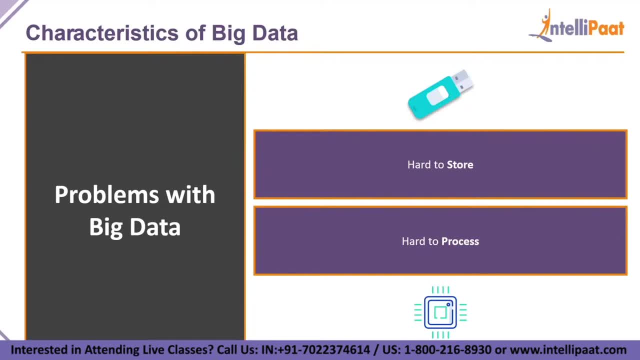 the number of cores that your processor has, depending on the number of threads that your processor can run simultaneously. so that's a big problem that we have with big data. and right, so these are the two primary problems that we have with big data. so even if we had a 10 terabyte, 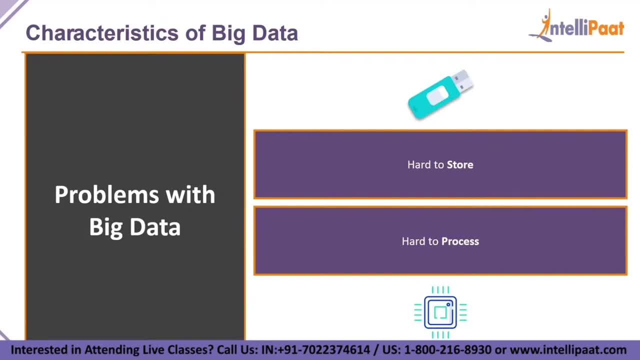 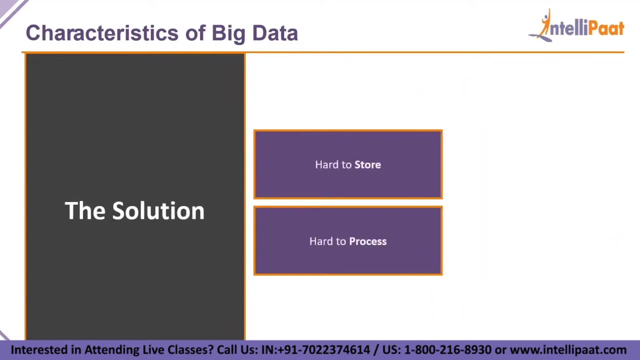 hard drive right and we were storing one terabyte of big data on it, right? we still need a very, very powerful processor to be able to process that one terabyte of information. so, with these problems arising, solutions also came up. the solution for the storage issue was Hadoop HDFS, and the solution 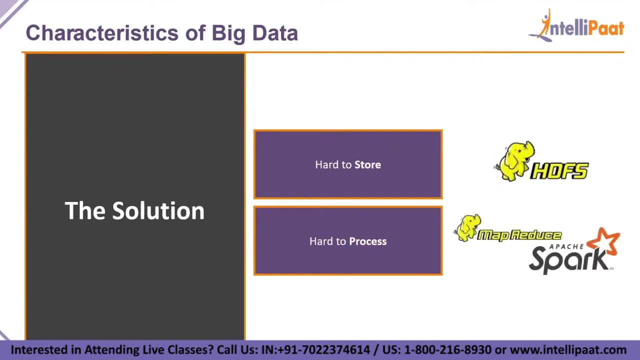 for the storage issue was Hadoop HDFS and the solution for the storage issue was Hadoop HDFS. for the processing issue was initially Hadoop MapReduce and then, in the modern times, it is Apache Spark right. so these are the technology stacks or frameworks I should say, that solve the big data. 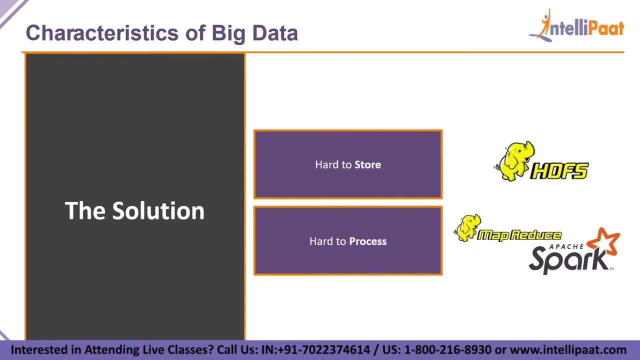 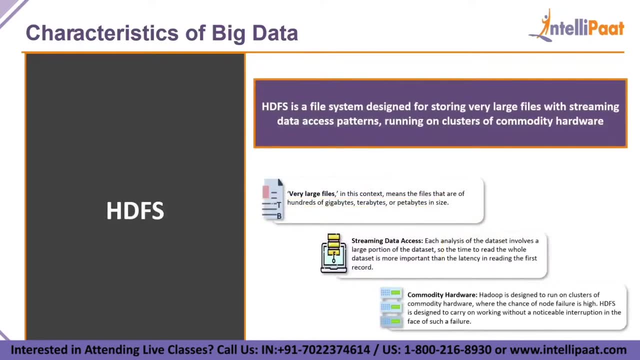 problem, right? so let us understand these frameworks and how these frameworks work and how big data clusters work- right? so firstly, let us understand what HDFS is now. HDFS is an abbreviation for the Hadoop distributed file system, so it's quite similar to the file system that you have on your 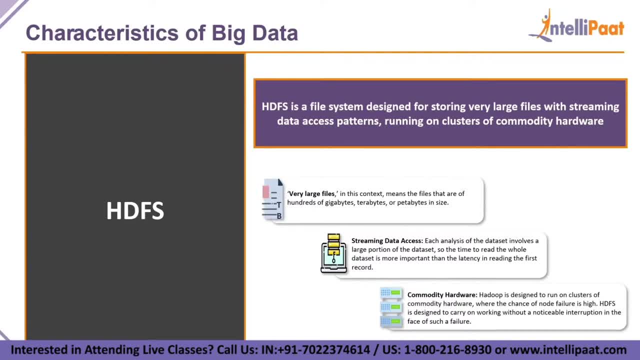 own computer, like you see in your Windows Explorer or your Mac file explorer right or your Linux file explorer. you look at the file system over there. it's quite similar to that, except this file system is collaborative in nature, right? so that means this file system is not just based on one computer. 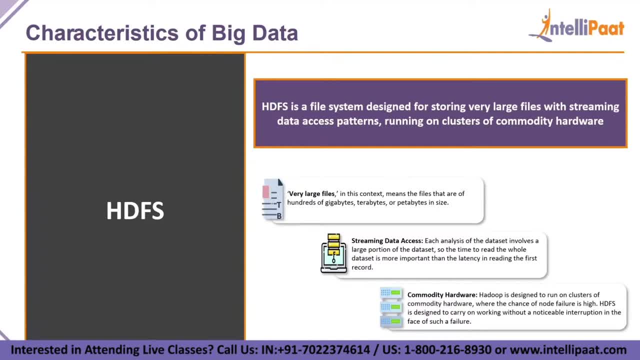 it is based on the entire cluster of computers that you have on your computer, right? so that's why it's called a Hadoop distributed file system, because it's based on a cluster of computers that you're connecting together in a network to create your Hadoop or big data cluster. so it might be. 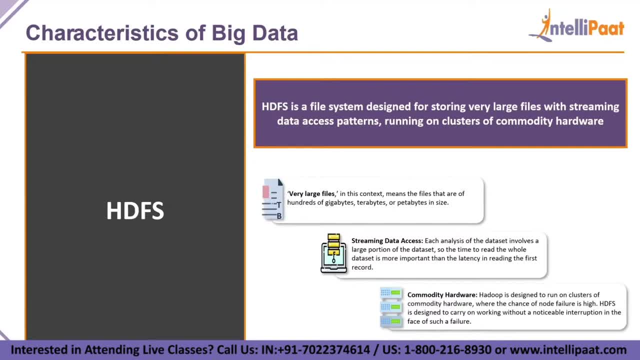 confusing. let us go through this step by step. so Hadoop is a Hadoop distributed file system is designed for storing very large files with streaming data access patterns running on clusters of commodity hardware. so very large files means that the data can be gigabytes to terabytes and petabytes in size. the HDFS manages that storage. 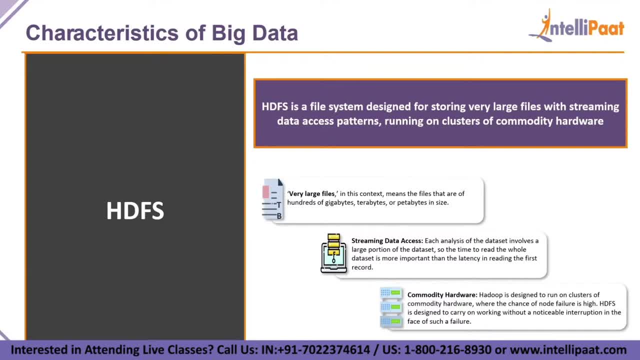 very large files means that the data can be gigabytes to terabytes and petabytes in size, flawlessly streaming data access. each analysis of the data set involves a large portion of the data set, so the time to read the whole data set is more important than the latency in reading the 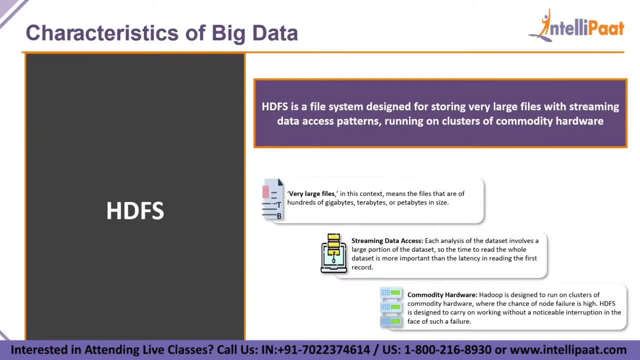 first record, right. so basically, that means that, even if the computers are far off, right, even other computers are not connected together at a very close range, right, if they're connected remotely to together, right, that is not an issue, as long as the internet speed is good, right. so, for instance, the 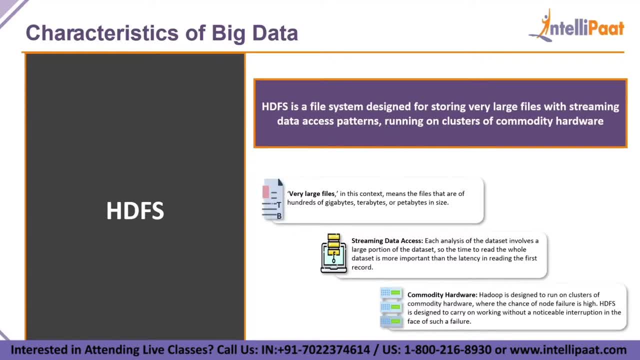 latency might be high between two particular computers, but once the request response starts right, you still have a constant speed between those two computers and the jobs will run without any issue. so that is what streaming data access means. basically, the latency is not that relevant unless you are doing something where latency matters and you're not able to get the data out of it. so that's why it's called a Hadoop distributed file system. 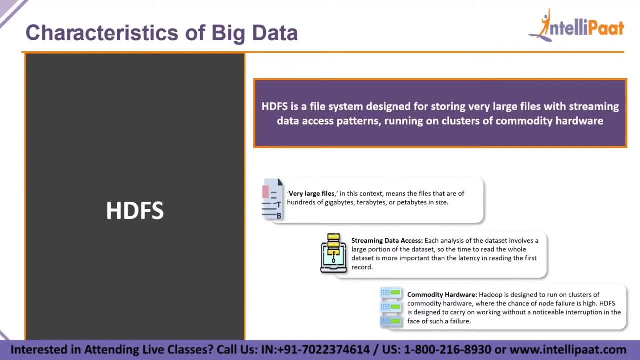 matters a lot. then we have commodity hardware. so commodity hardware was a concept that came up back when Hadoop was created. it was when hardware was really expensive, when RAM was really expensive. so what it essentially means is that, instead of buying entire servers with a high RAM, high hard drive space, what you can do is you can 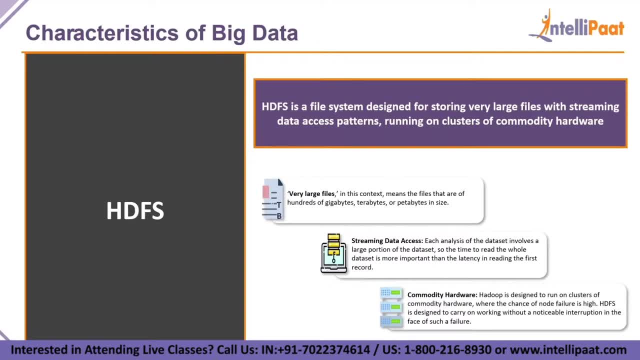 install Hadoop on commodity hardware, which means you can install it on the computer, uh, computers that you have in your computer. you can install it on your computer. you can install it on your computer in your own office spaces, the everyday workstations. right, you can just reserve a certain section. 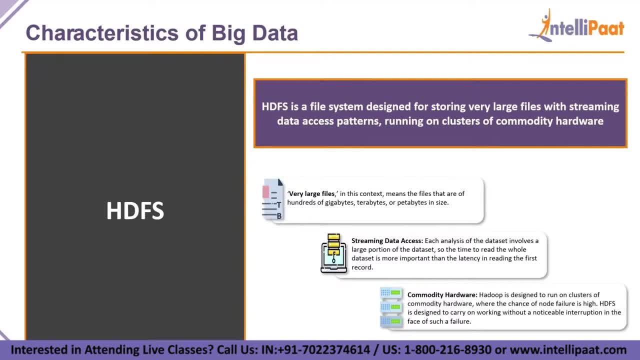 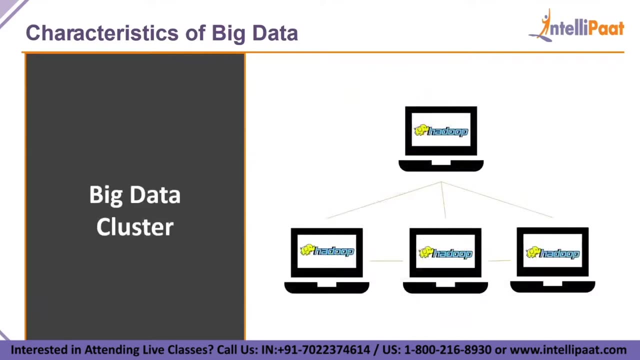 of those workstations and dedicate it to your Hadoop cluster. so instead of investing in an entire server farm for your Hadoop cluster, for your big data cluster, you can simply use the computers that you already have. so that is what commodity hardware means. so next up, let us understand the architecture of a big data cluster right. so you have LAN wires in. 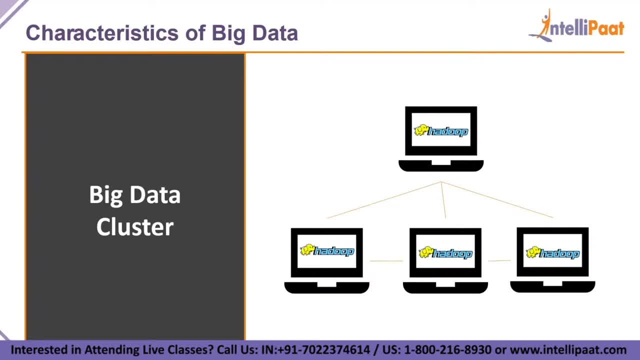 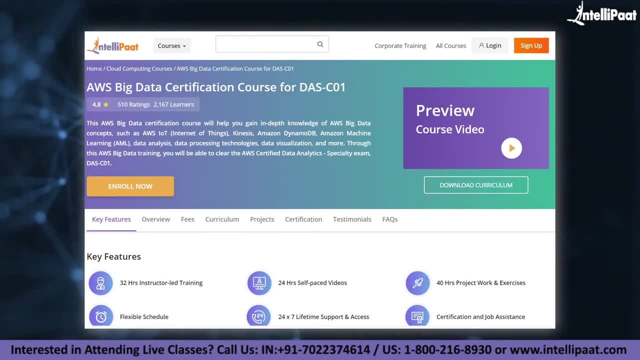 your office space. right you are, you have wi-fi in your office space. so what it essentially means is that whenever- just a quick info, guys- Intellipaat provides AWS Big Data certification course mentored by industry experts, the course link of which is given in the description below. now let's continue with the session. 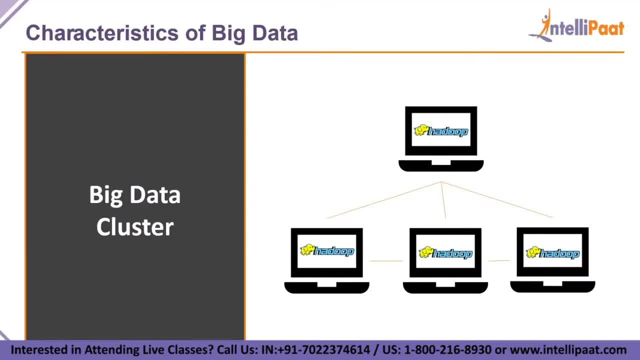 you are configuring Hadoop on your cluster on your network, right? and you're telling all of these systems to be low level on your cluster, on your network, right? and you're telling all of these systems to be to be low level. so if you don't have an indoor data cluster, then you'll do it with прид. You can do it withromTC if your computer is something using microred used by a kan in your system, but aren't you you? You are configuring Hadoop on your cluster, on your network, right? and you're telling all of these systems to be low level. 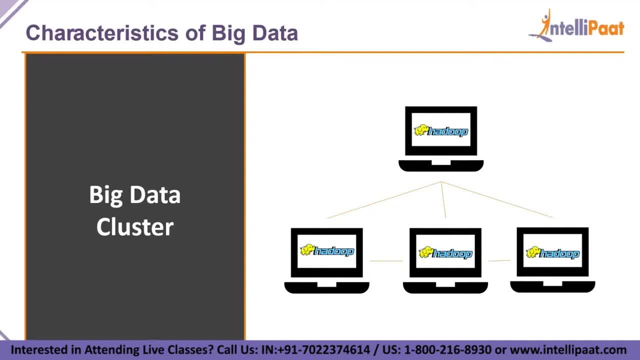 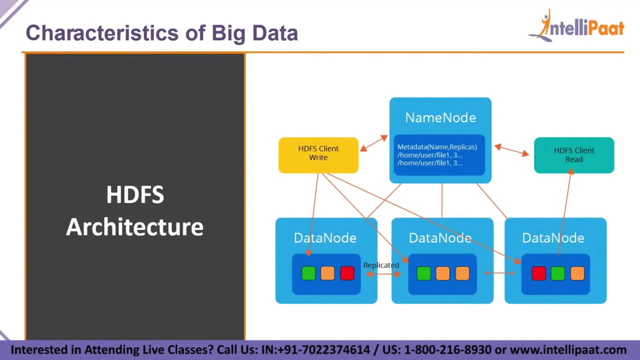 find each other. when they start functioning, they will start sharing files with each other as well when required, and all of that happens seamlessly without you knowing any of it right. so that is the advantage that you get with hadoop. so if we were to map the previous diagram to a more refined and 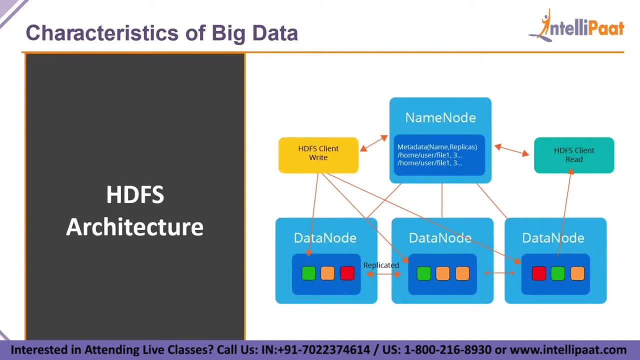 detailed hdfs architecture. so we can see that we've converted one of those computers into a name node. so we've basically configured one of the computers into a name node and the remaining three we've configured as data nodes, right, and we've installed hadoop on all of them. so what? 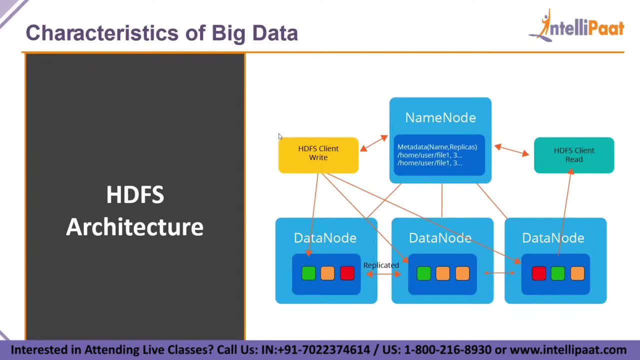 happens essentially is, say, for instance, you are a client or you're somebody who's trying to access this particular cluster, so you, you have a file to upload. essentially you have a petabyte file or a terabyte file to upload, right, so you will contact the name node first. the name node will tell you. 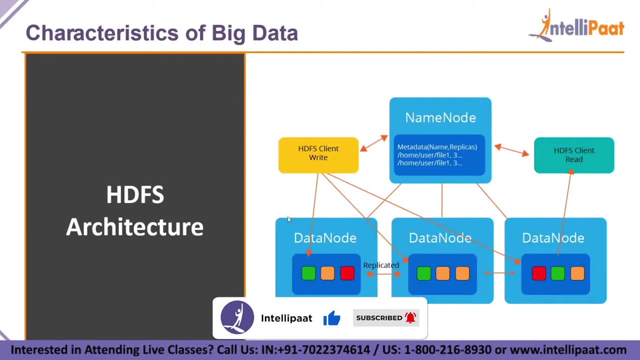 which data nodes have free space, right? so once the name node tells you which data nodes have free space, you are connected to the data node that you need to be connected to and then you start transferring your file there. but it does not end there. what happens is say, for instance, you have 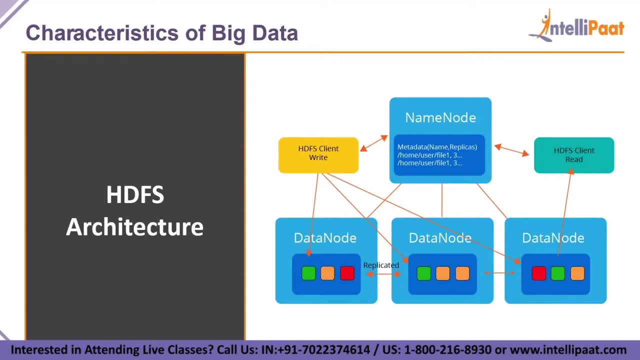 a one terabyte file, right, but it is almost a certainty that these data nodes will not have that much of free space, any single one of them. so what will you do? you will divide this file into three parts, right, depending on the uh, depending on the size of the file. 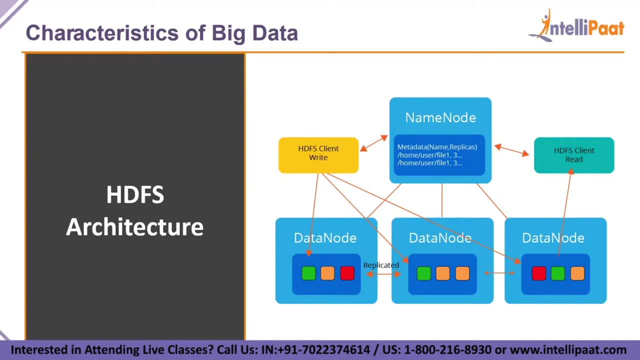 depending on the block size that is configured into your hdfs, this file will automatically be divided into a lot of blocks, right? so for now, for example, sake, let us assume that that one terabyte file has been divided into three blocks, right? so the first block will represent by green, the second 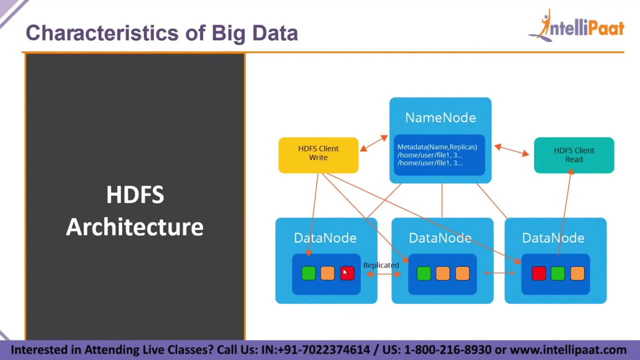 by this orangish color and the third by this reddish color, right? so you've uploaded that file and say, for instance, the green part get uploaded or gets uploaded on data node one, the red part gets uploaded on data node three and the orange part gets uploaded on data node two, right? so keep in mind that there may be a lot of. 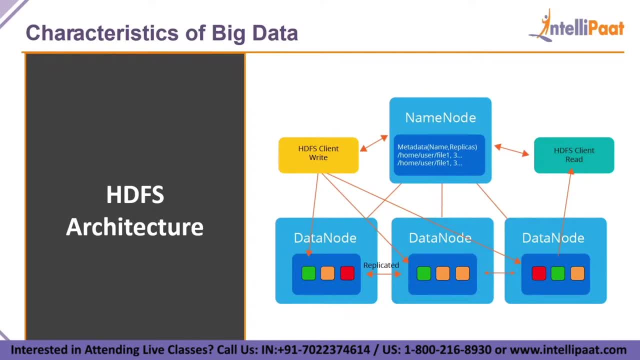 other data nodes as well, but right now we are going with an example of only three data nodes, right? so what happens after that? the file has been divided into three equal parts and it has been stored in three data nodes- right, but what? what happens when you try to access it? right, when you're a client, when you try to read that file, you'll see that file as 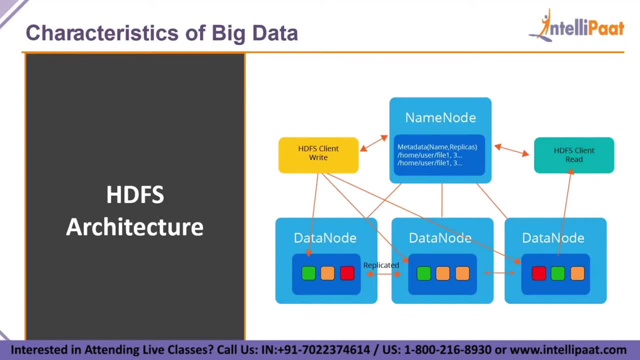 a one file. you wouldn't see it as three divided files. you will see it as one file. the combination of files and the division of files when we are writing it and reading it is managed entirely by the hdfs. so the next thing that is very important is data replication. so basically, 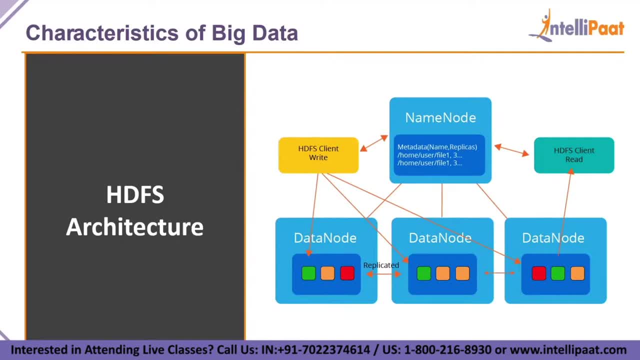 in order to provide provide a data loss prevention feature, hdfs has come up with a feature called data replication, where you can set up a replication factor. right, so say, for instance, you have set up a replication factor of two. so what will happen? you store one block of data on data node one. 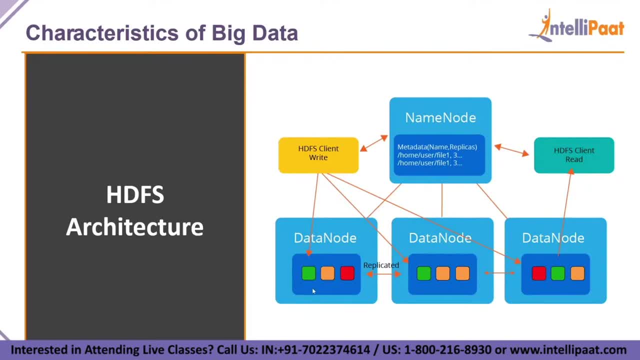 the data node one's block. the screen block will automatically be replicated two times on the nearest two data nodes or wherever the data nodes have available space, one would be stored on data node two, the other would be stored on data node three. so in this particular case, even if data node one fails or something goes wrong with data node one, you still 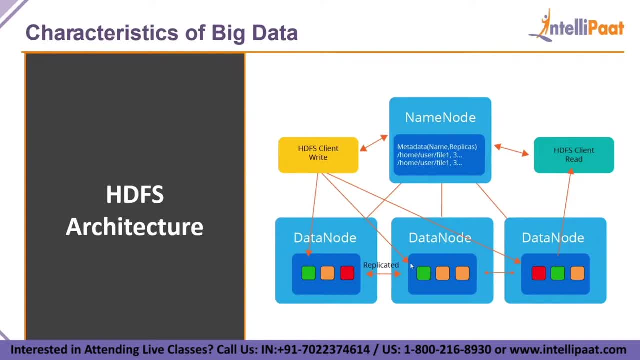 have access to the first part of the file, right? so that is the advantage of data replication: so you can set up auto data applications. whenever you store anything on the hdfs, it will automatically be replicated across the cluster as well, so that if any damage occurs, you still have access to the entirety of the file. 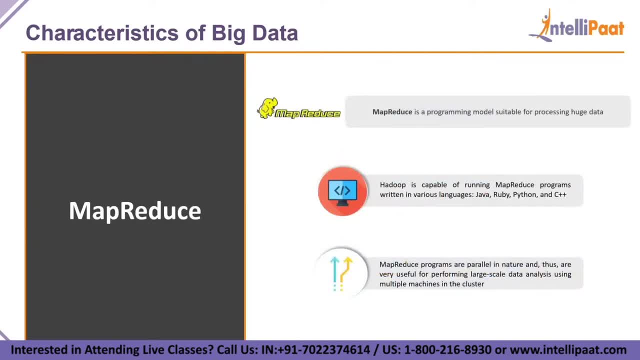 so the next thing that we want to talk about is what is the process of data replication? so we can understand what map reduces, so we know how storage happens in hudu. now we can understand how processing happens in hudu, like there are two parts involved in any big data procedure. so first, 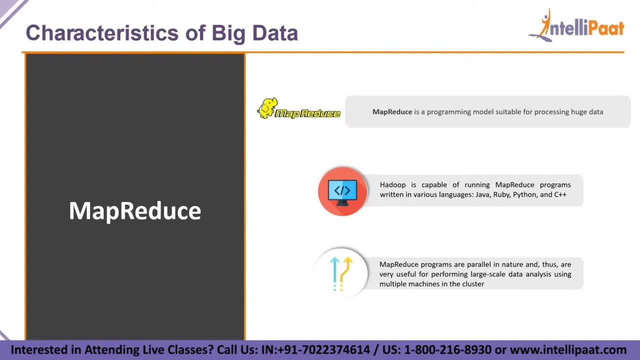 is storage. the second is processing. map reduce is the programming model suitable for processing huge data. right, so map reduce is unlike anything you've ever seen. if you are not uh aware of the domain of hudu and you are not familiar with the domain of hudu and you don't know how to use it, you can. 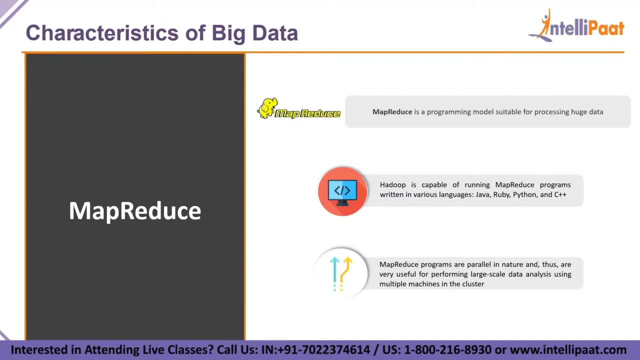 just click on the upper right corner of the page and you will see a menu which is called map reuse and it's capable of running multiple map reduce programs written in various languages, like java, ruby, python and c plus plus. so you have my map reduce libraries available for these particular 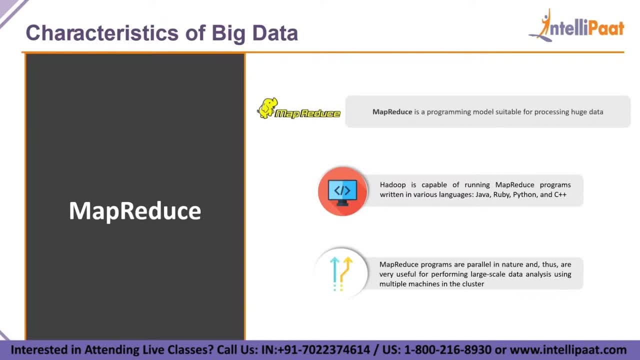 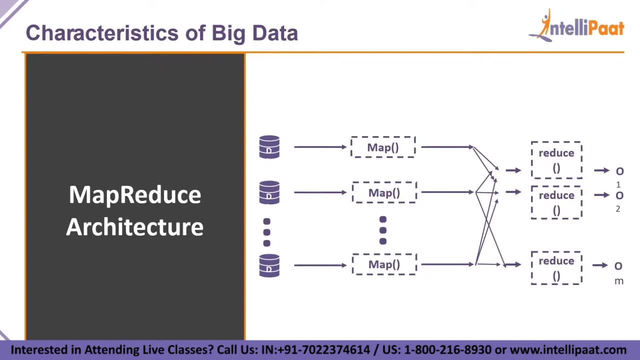 languages and map reduce programs run in parallel, so they are very useful in performing large-scale data analysis using multiple machines. in the cluster architecture that we were dividing data and storing it across nodes in a cluster across three data nodes. so for instance here let us imagine these are these three data nodes. 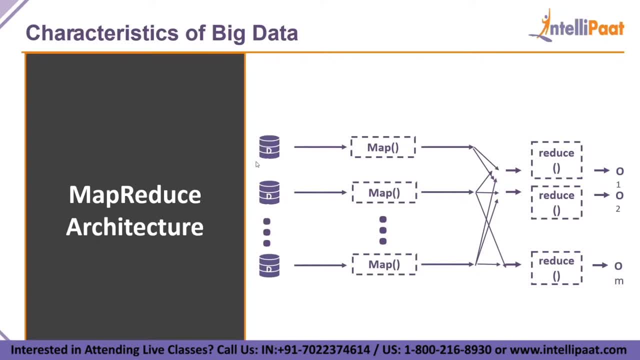 right. so this particular data node contains the green part, this contains the orange part and this contains the red part, the third one, right. so what will happen next is that you'll map it. so, firstly, any procedure, any data analytics procedure that you're performing, whatever is present in your code, it will execute in a map reduce format. so, firstly, the data will be mapped. 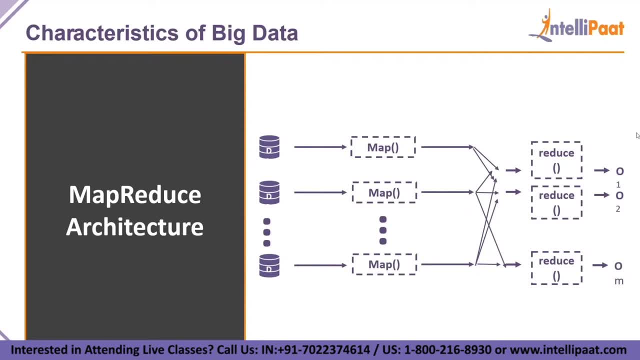 so it will be converted into key value pairs. and then the next step is: same keys will go to one reduce operation. so, for instance, if there are key values with the key being one, all of the keys, which are one, and the values corresponding to them, will go to one reduce operation. 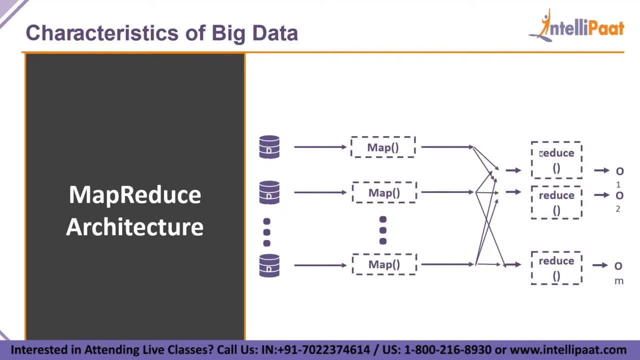 and all of the keys, which are two, will go to one reduce operation, you right, and then you'll finally get your output. essentially so, to sum it short, to give you the brief explanation of this, each data node is executing their part of the file on their processor itself. they are not actually collaborating until the output has been generated. 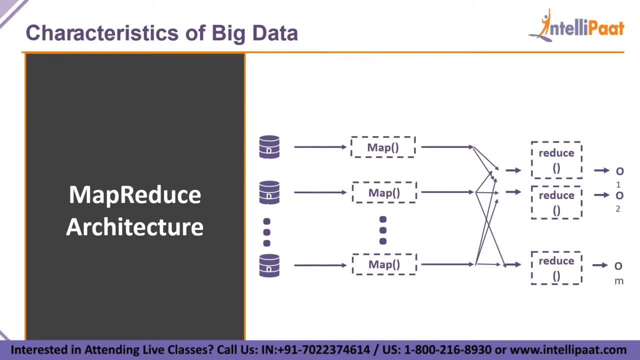 right, once the output has been generated, they all combine their output and show it together. so that is what parallel processing means. so instead of performing this entire operation on one computer, this entire terabyte of file, we have divided that one terabyte of file into three parts and we are executing each terabyte, each part. 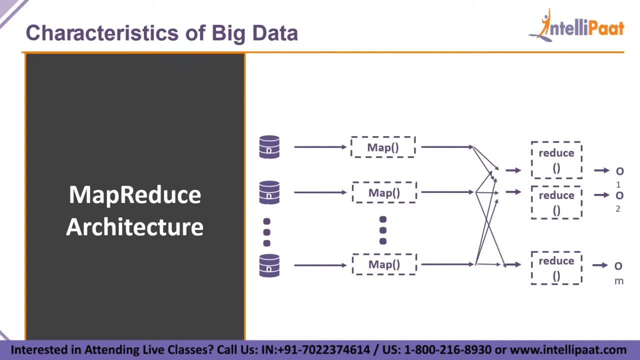 of that file on their respective node using their processor, dividing the entire time of the operation by three, so you can understand how efficient this can make things. so, depending on your cluster size, you can further reduce the time network time and you can also reduce the time network time. 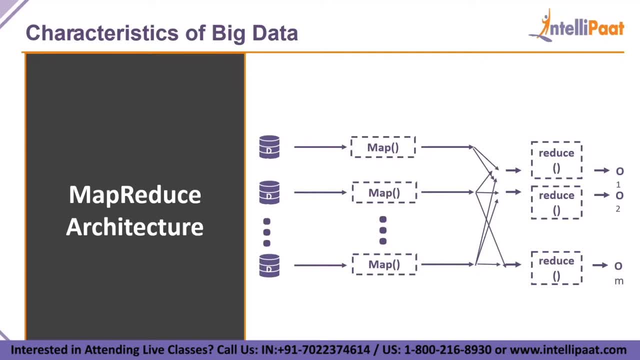 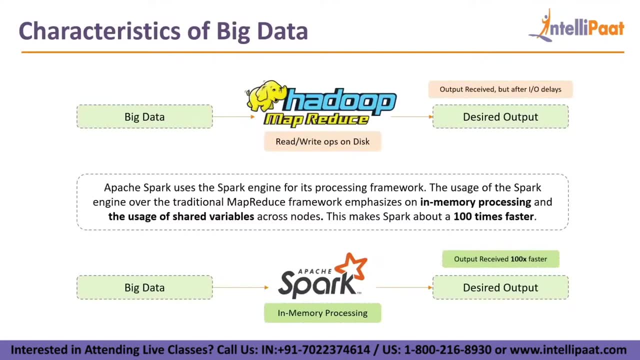 take to perform this operation as well, and we also discussed about Apache spark, right. so there is one other technology that is used today, because MapReduce, like we just discussed, is now sort of redundant, right, but based on the same concept, essentially, we have Apache spark. so, for instance, 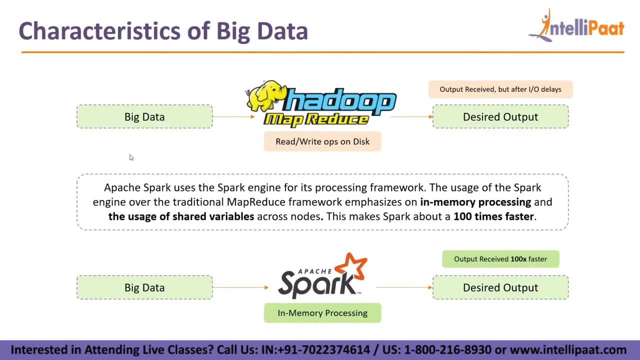 let us look at the distinctions between MapReduce and Apache spark. you have a big data set available to you right over here, then you pass it through a MapReduce program, and then you get your desired output. the problem with that, though, is that earlier on, when MapReduce was built, in the early stages, where RAM was extremely 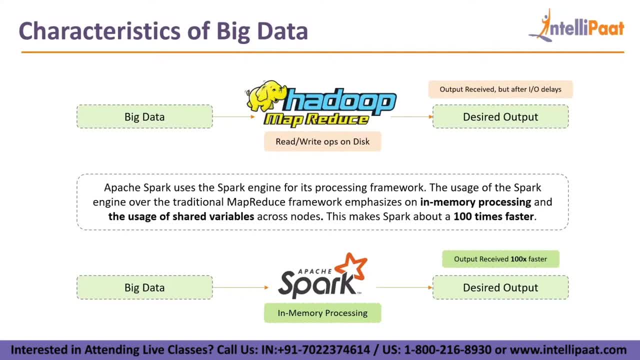 expensive. we used to use hard drive space as a sort of replacement for RAM, because RAM was really less. you had like 500, 512 megabytes of RAM on one computer and you had a terabyte of file, or say you had a 2 GB block size on your particular node, right? so it would take you four steps essentially to 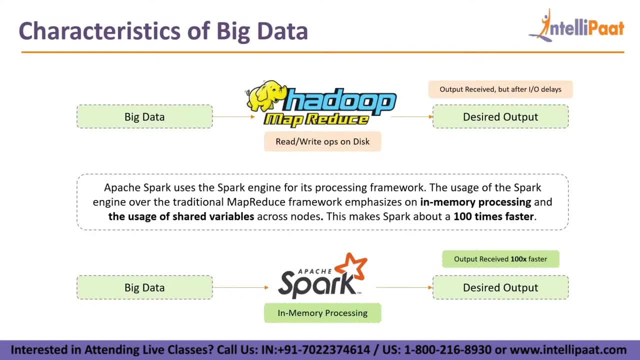 process all of that data if we were to go by it roughly. so problem with that is: every time you're transferring that 512 mbs of data to your RAM, you're having some latency issues with read and write operations. so every time you transfer data from your hard drive to your RAM it takes a bit of 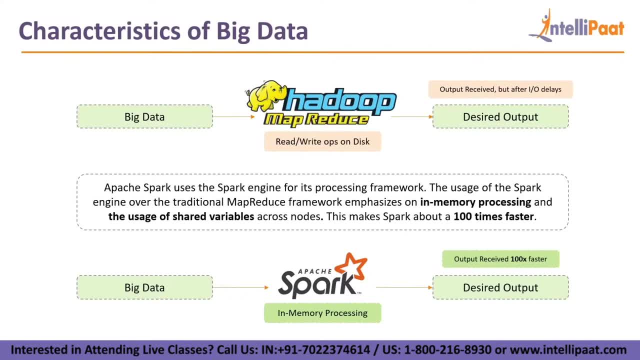 delay right and if you are dealing with extremely large amounts of data, that little bit of delay over time can add up. so when that adds up your process of getting your output becomes slow. so we can see that there are read write operations on the disk. so you're transferring the data into the RAM. the data is 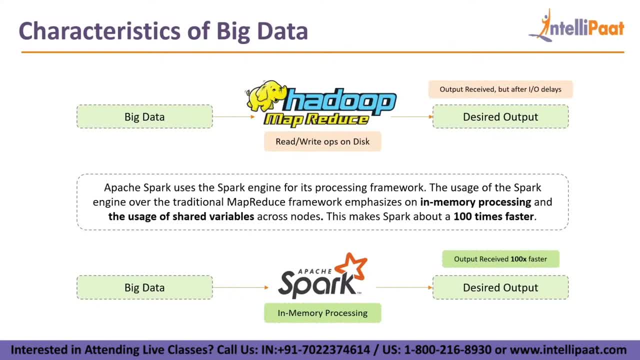 going into the CPU, it is being processed, it is being put back into the RAM and then being put back into your hard drive, right, so that time taken between for the data to transfer between to and fro between the hard drive and the RAM is adding up. essentially, So you're getting your output but with input output delays. 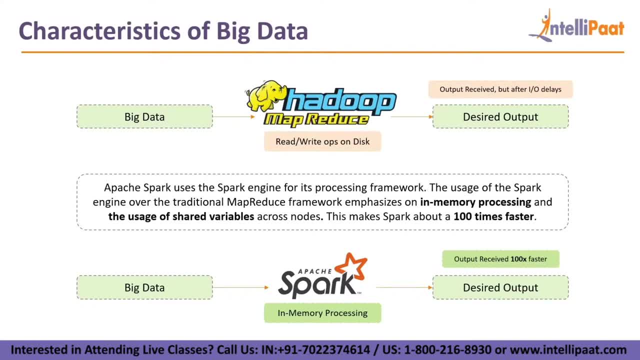 So as random access memory or RAM or physical memory got cheaper, we came up with the technology called Apache Spark, which uses the Spark engine right. So Spark engine is something that speeds up this entire process over a hundred times compared to MapReduce, depending on the size. 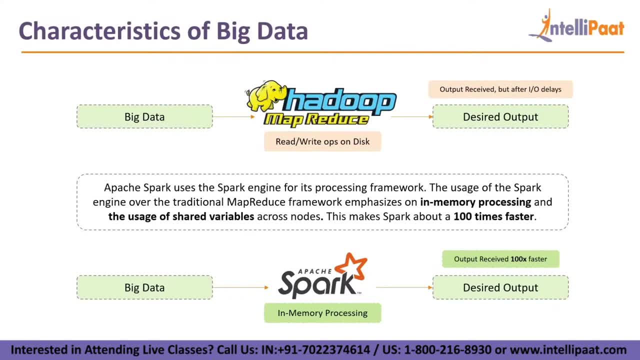 of the data. For lower sized datasets the difference is not that noticeable, but for higher sized datasets you can definitely see the difference between the performance of Apache Spark and Hadoop MapReduce. So Apache Spark does this by using in-memory processes. 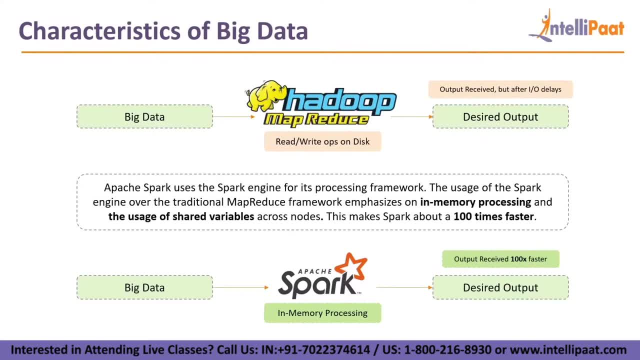 and the usage of shared variables across nodes, something that MapReduce did not do. So what does in-memory processing mean? In-memory processing means that when you transfer that data and say, for instance, now that RAM is cheap, you have like 64 gigabytes of RAM in mobile phones. 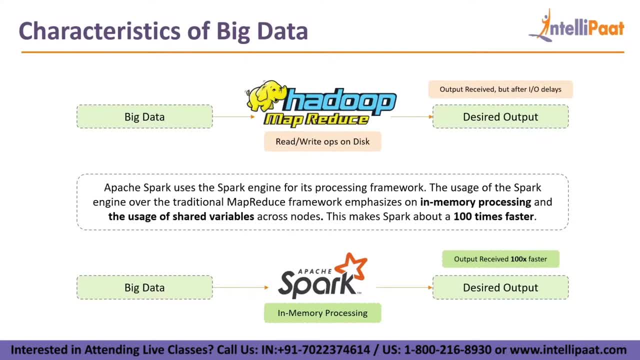 today. That is how cheap RAM has become- You can simply transfer the blocks of data that you have on your respective node on the data node. Now that data can be transferred to the card slot- and since the card slot is also an example of this- you can take a piece of your RAM and transfer the entirety of that in the RAM. 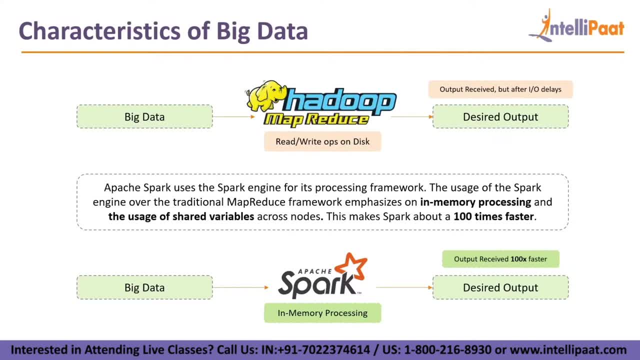 in just one go rather than four tries. So what that will do is you'll have the entire data available in your RAM at all times during the entirety of the execution of the job. So until you are closing down your Spark session, like until you're closing down your Spark job- you will have the entirety of the dataset available in your RAM. So that basically reduces any possibility of your system. 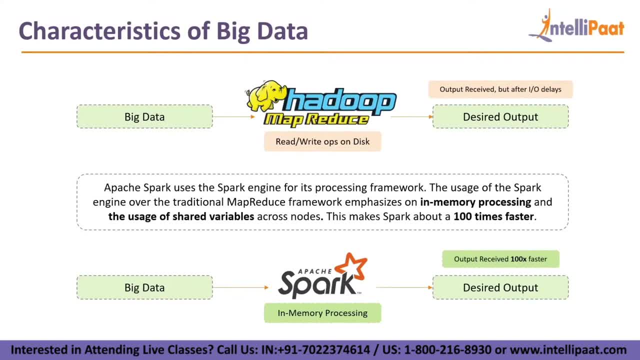 input output. delay between the CPU and the RAM and the hard drive. because you're not dealing with the hard drive after the initial transfer. you're not dealing with it anymore. once the hard drive has transferred the data to the RAM. the RAM will store that data until the execution of the entirety of the 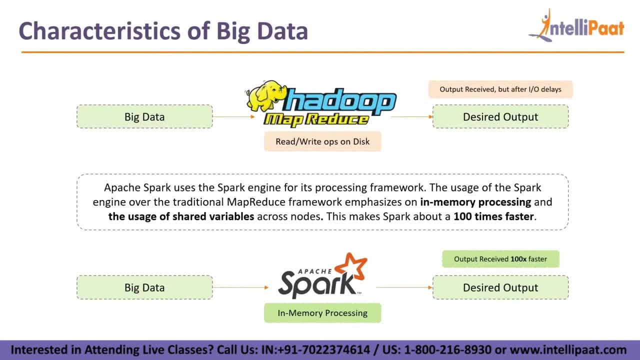 program and then, once the execution has happened, the output can go back into the hard drive. so you are essentially minimizing all sorts of input output delays. so this is what in-memory processing is, and essentially the usage of shared variables across nodes can help with a lot of logical aspects in. 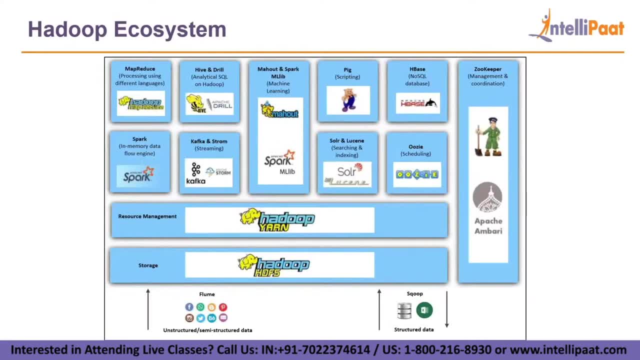 programming as well. so let us look at the Hadoop ecosystem as well. we have looked at some technologies. we have looked at HDFS, map, reduce and spark. there are other technologies as well. the foundational elements obviously are the HDFS. so this is the storage system and everything that is happening. 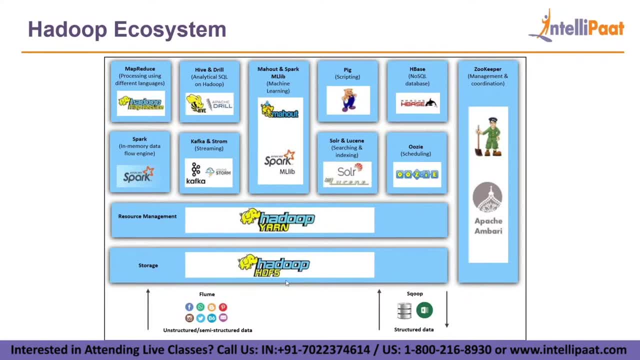 in the big data ecosystem is because of the storage system. so let us look at flume. flume is something that helps you integrate your HDFS with online api's and services, for instance, data coming in from Twitter or Facebook. you can configure your flume to ingest that data from time to time and you will get that. 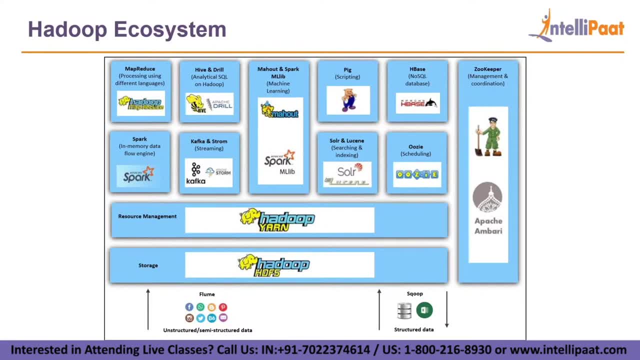 data stored into your HDFS automatically. we have scoop for people who are in the RDBMS business. they can essentially integrate HDFS with their RDBMS service by transferring data to and fro using the service we call as scoop. and there are other services as well. we're not going to be going through all of them for. 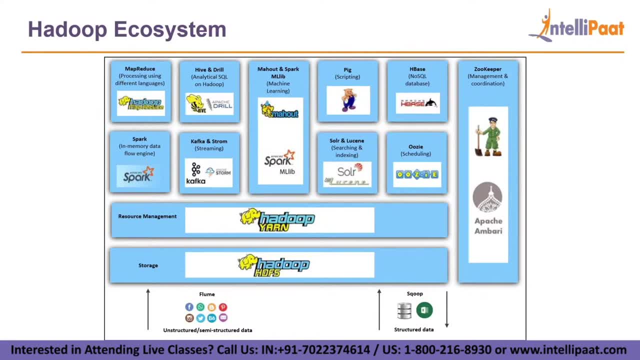 instance, we just understood what map reduce means. we also have hive, so a hive essentially is something that uses map reduce or to perform data warehousing and querying on the data present in the HDFS, so hive can be used for that. you have spark machine learning library, so right now we discuss spark. 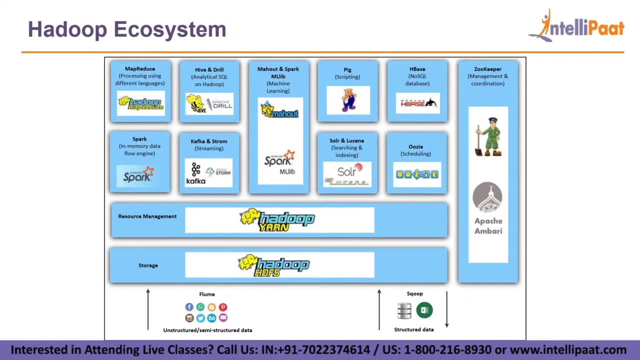 processing. so you have other options as well, available with spark. so, using the same format that spark uses, you can also create machine learning models out of spark for sorts, creating scripts using the map reduce concept. you can use pig. you have each base, which is essentially a no SQL database, present. 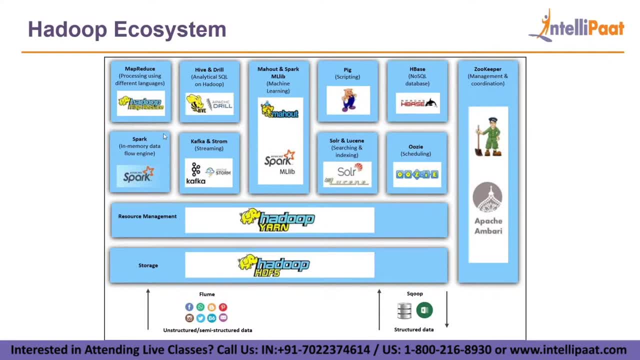 for the HDFS data. we obviously discussed spark. we have streaming data. we have most of the data is available in the database, so we have device application. we have other devices and, of course, the email and the phone that is supported by the htfs data. you can use it for sister applications. So that is why we are here. 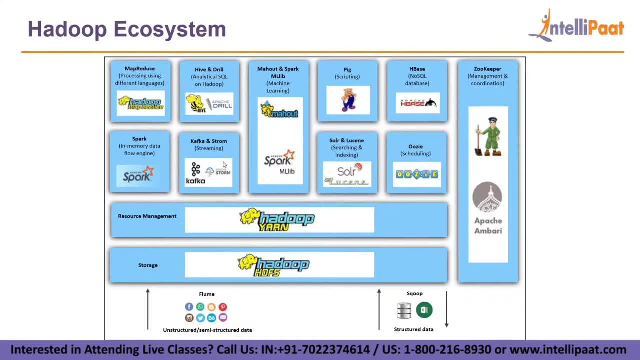 services available which transfer the data in real time to your HDFS. So, say, Kafka will stream the data coming from a particular source into your HDFS continuously. You have other services as well. You have Uzi for scheduling and you have Yarn for resource allocation. So Yarn, essentially. 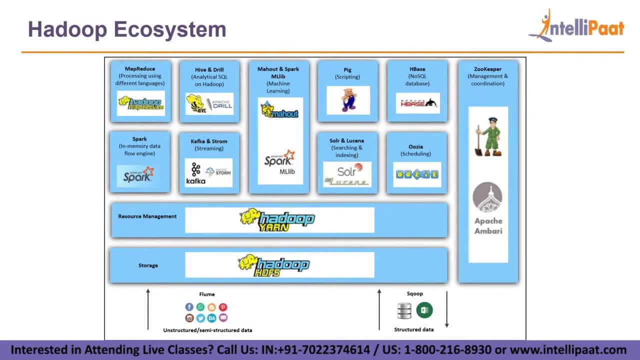 what it does is it allocates resources. So, for instance, any job that you try to run on your Hadoop server, Yarn will look at the resources that are available, It'll queue your job up and then eventually it'll get your job executed by allocating resources to these data nodes to 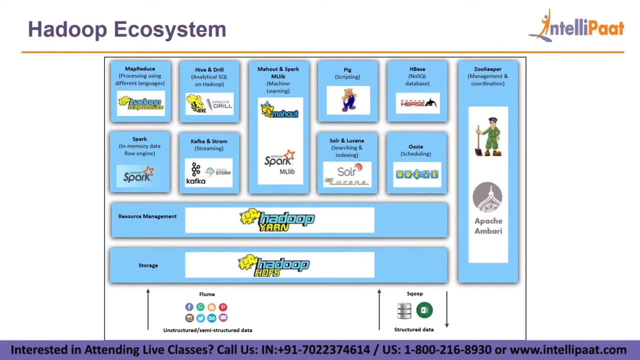 execute that job. And if you're looking for a UI to manage all of this, for instance if you don't want to deal with command line terminals, you also have UIs available, And one of these UIs is Apache Ambari. 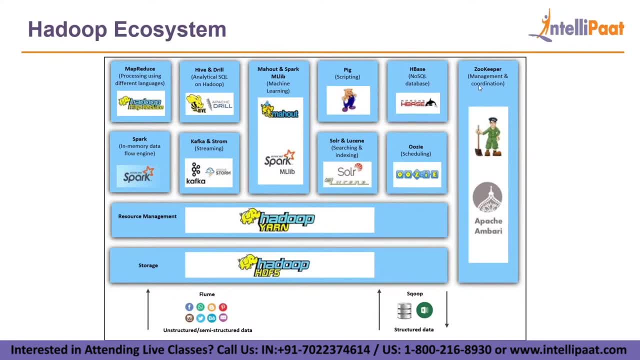 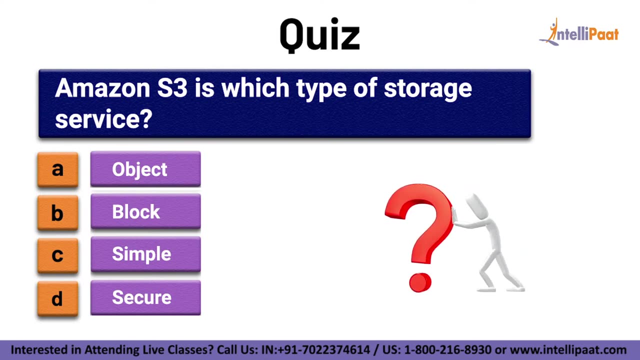 It has ZooKeeper in it, which helps you manage and coordinate all of these services and frameworks that are running on your Hadoop cluster. Just a quick info, guys. Test your knowledge of AWS by answering this question. Amazon S3 is which type of storage service? 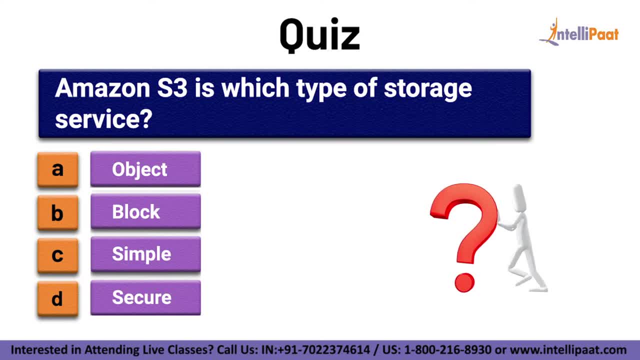 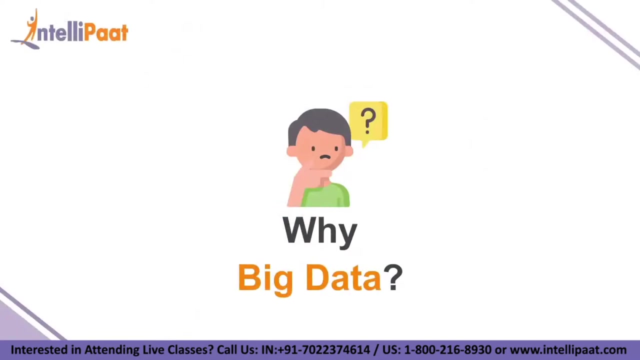 A, Object B, Block C, Simple D, Secure. Comment your answer in the comment section below. Subscribe to Intellipaat to know the right answer. Now let's continue with the session. So why big data? Why is this field so relevant, right? So let us take an imaginary scenario. 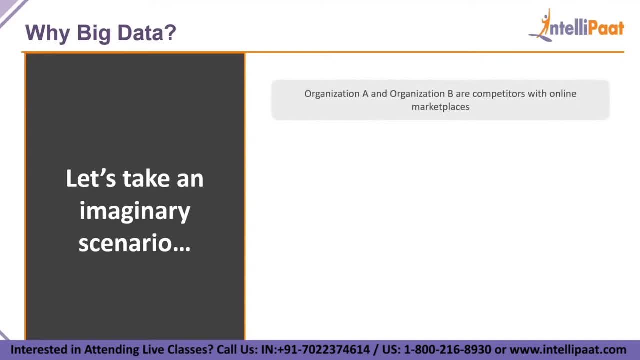 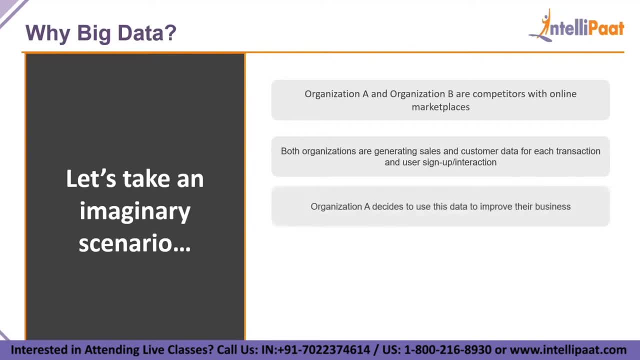 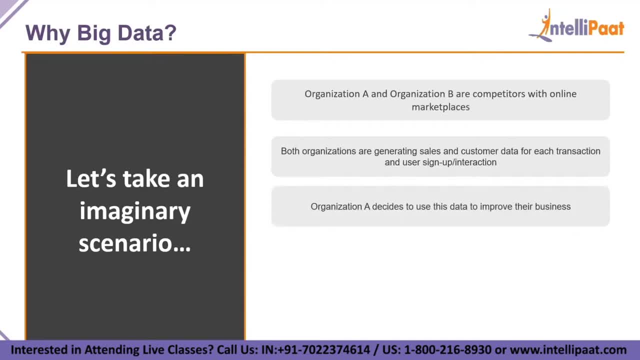 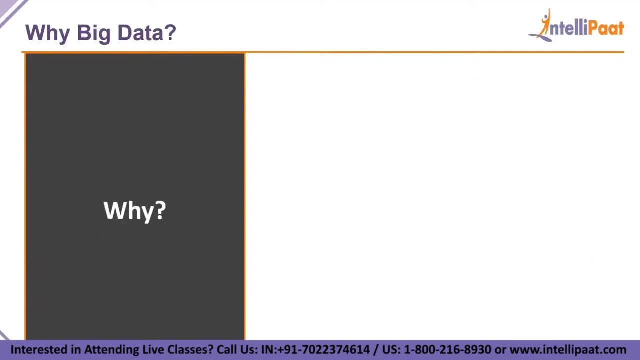 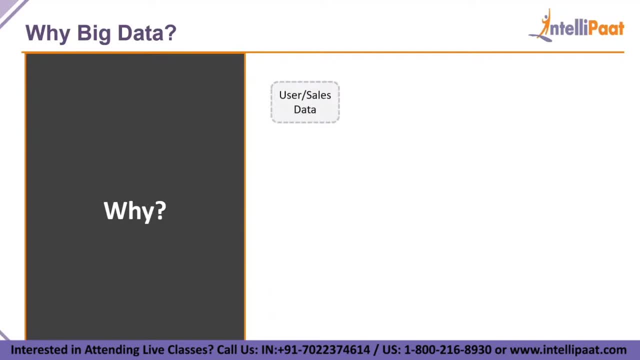 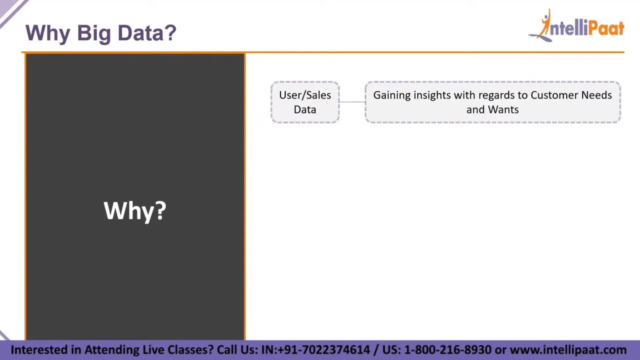 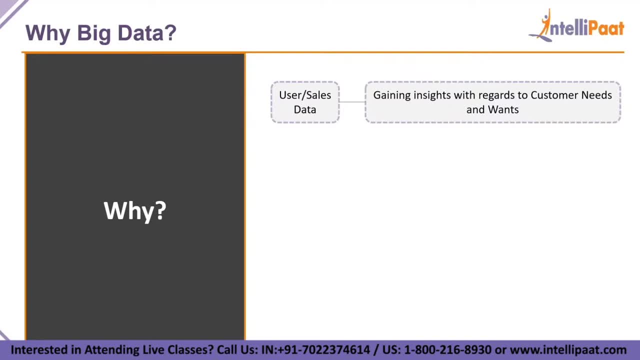 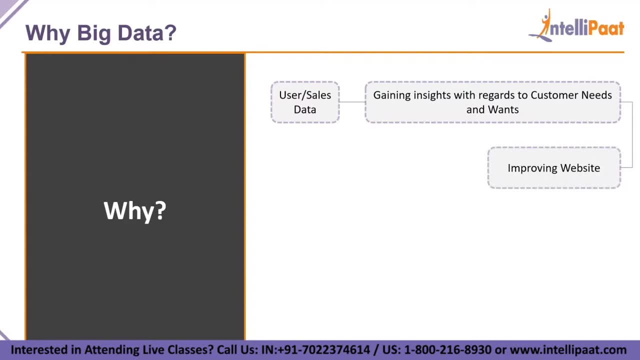 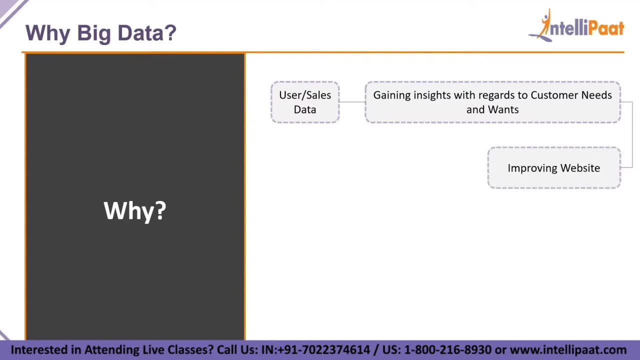 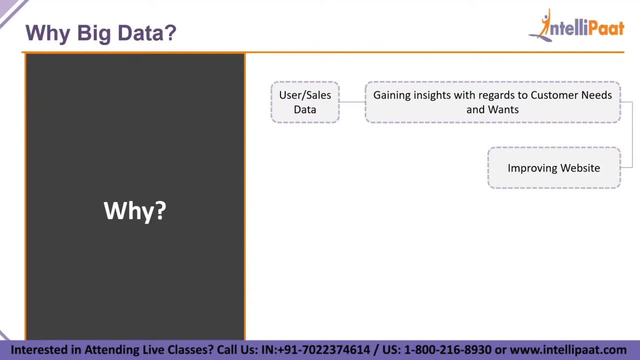 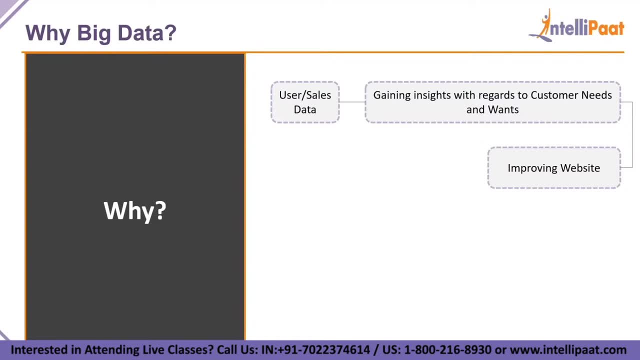 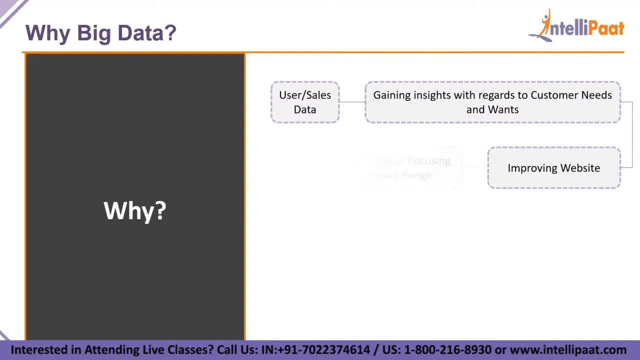 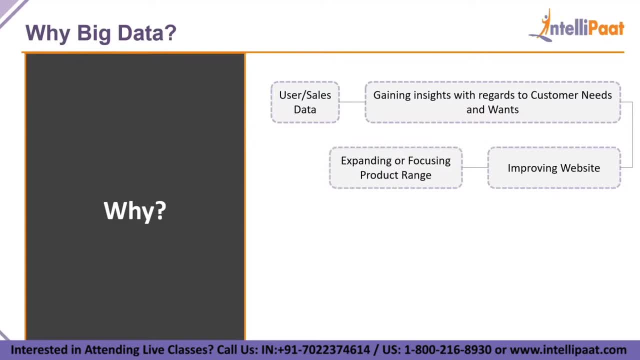 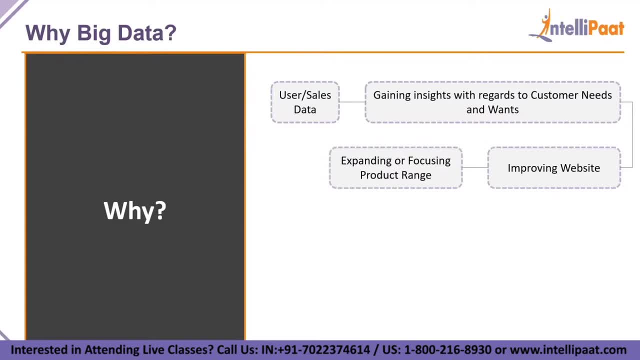 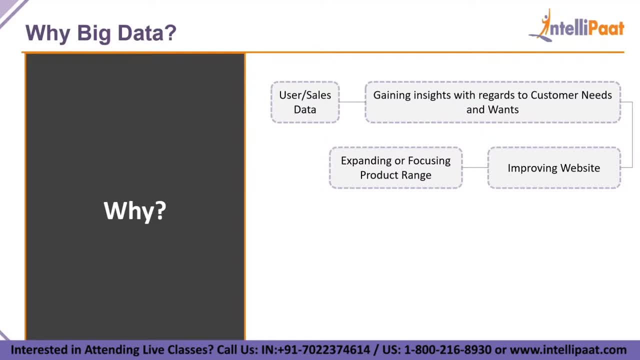 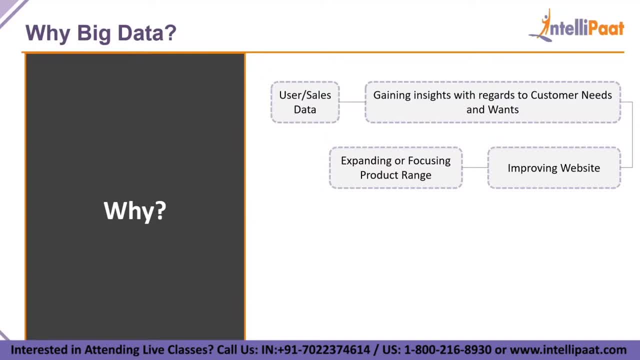 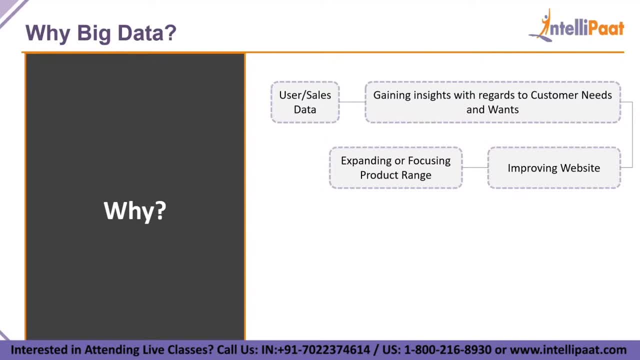 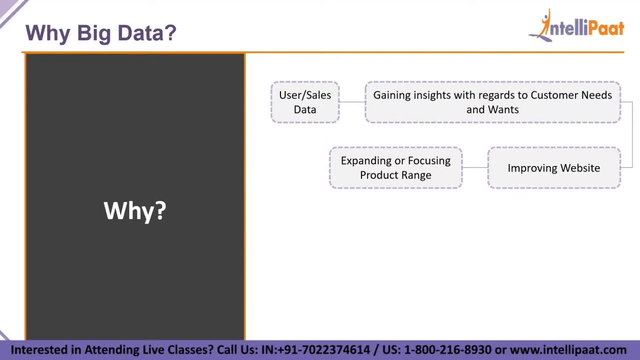 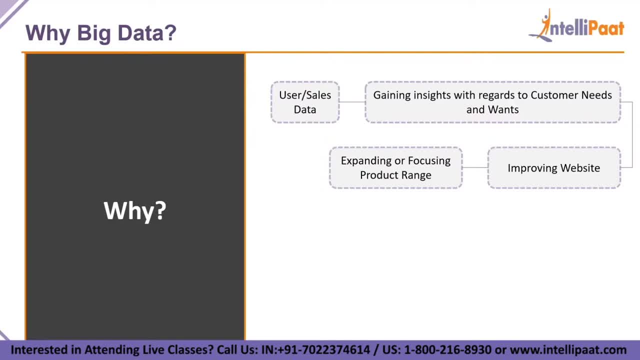 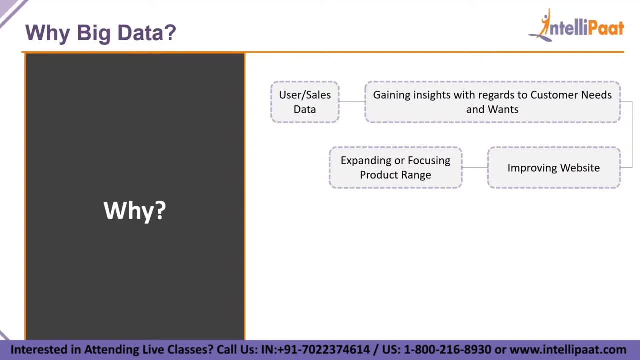 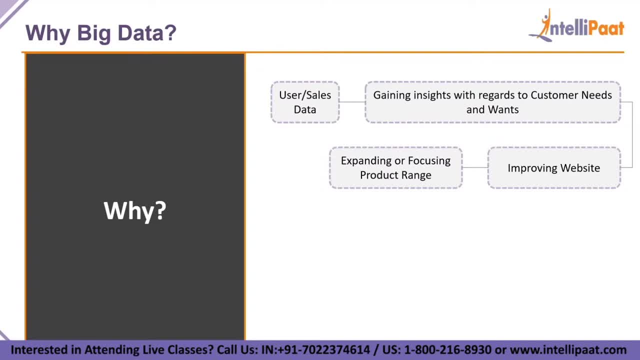 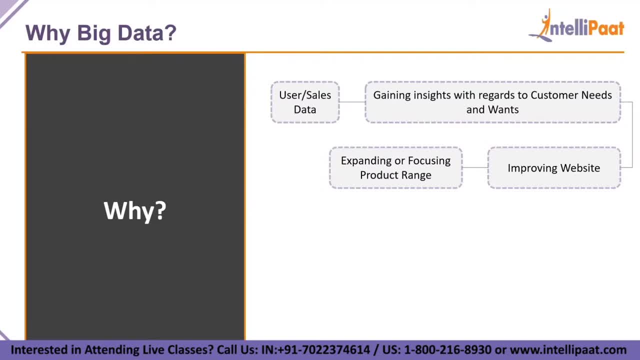 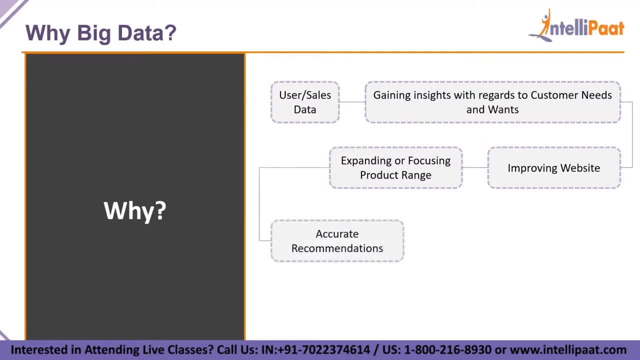 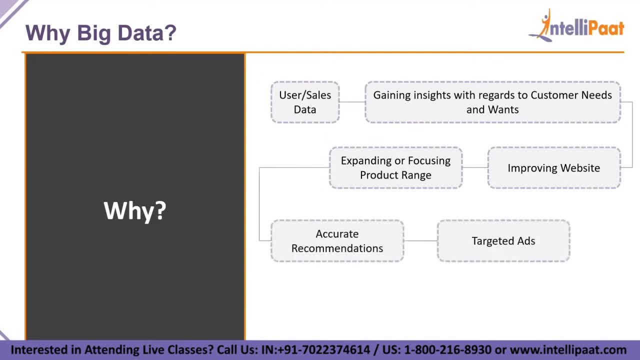 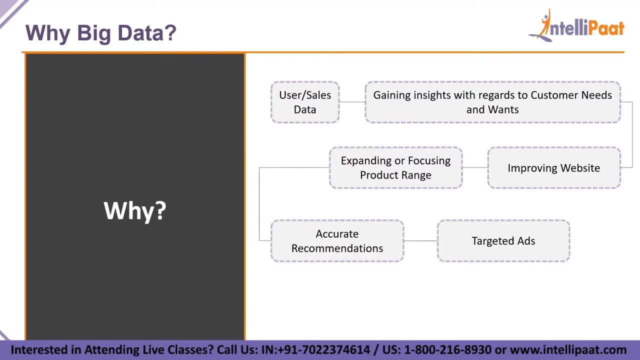 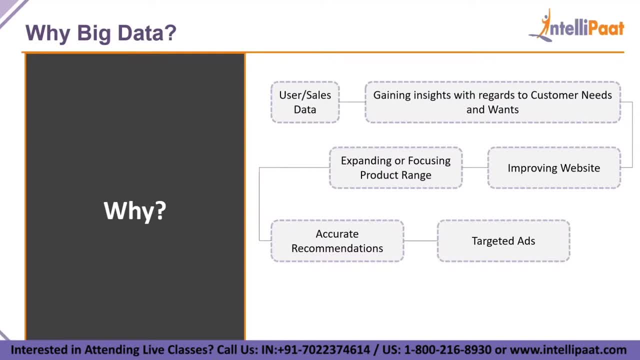 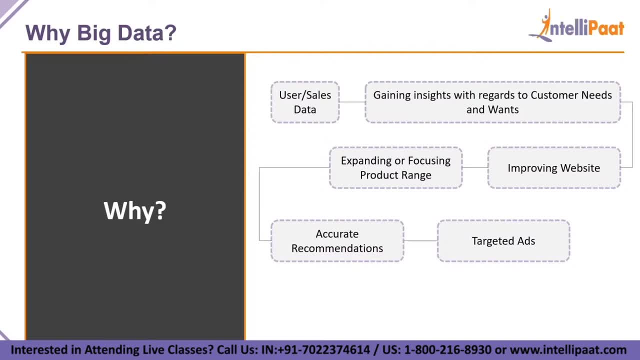 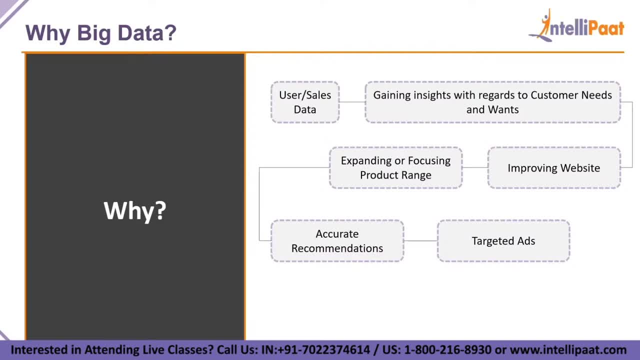 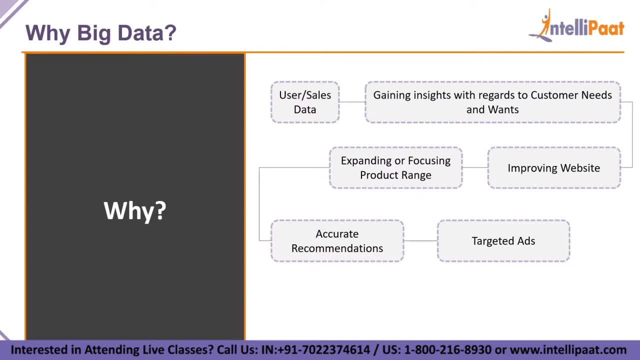 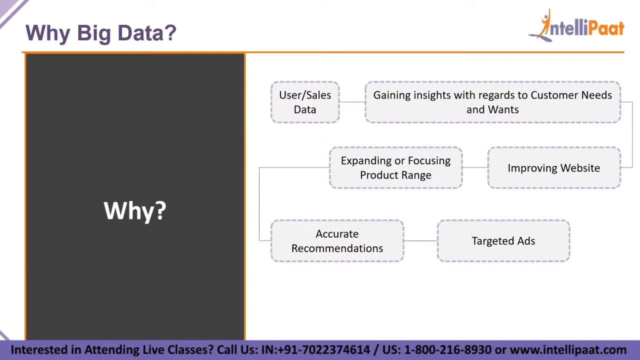 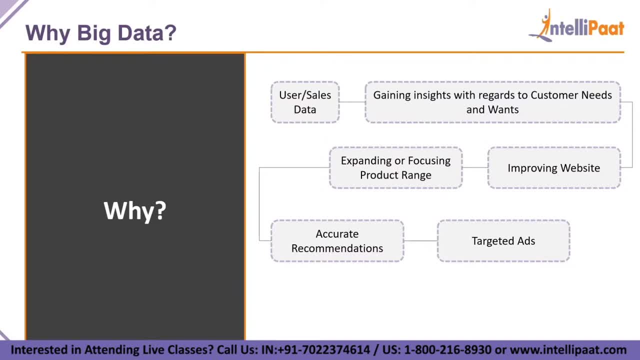 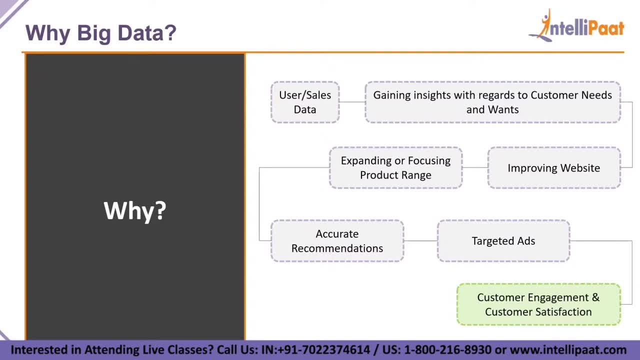 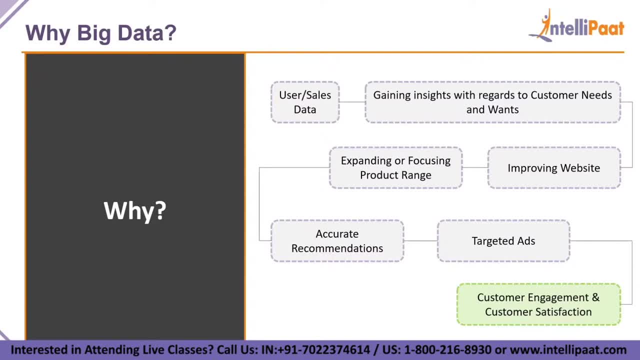 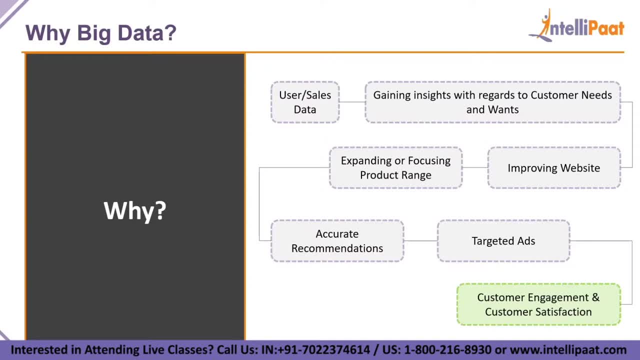 analytics model or the machine learning model, simply assesses and aggregates what the customer likes and shows that product to the customer, shows the exact recommendations that the customer actually needs and gives the customer a good user interface. there is customer engagement and there is customer satisfaction. these are the two key things in the success of any business and that 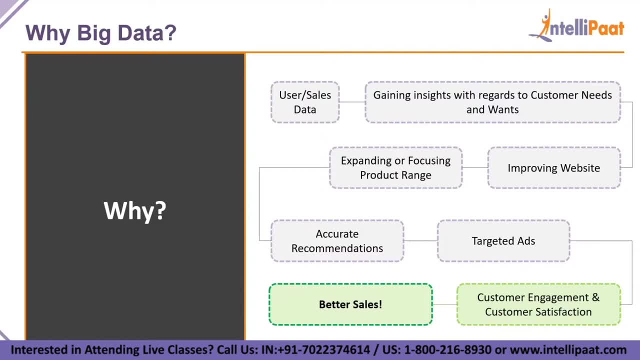 results in better sales, obviously, and that could also result in the organization getting the entirety of the market share as well. so kind of a similar story with amazon as well. because they have such good data science and data analytics models present within their algorithms, they have succeeded and they have gotten to the apex of the e-commerce industry. nobody even comes close. 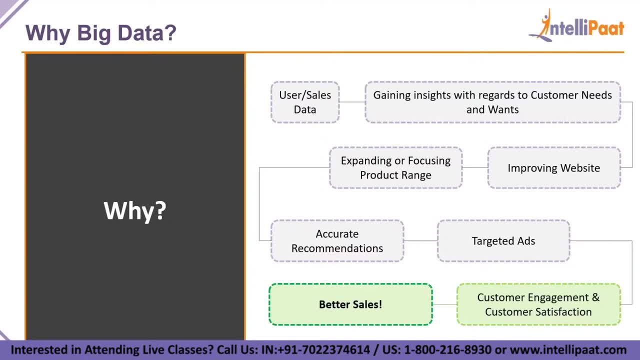 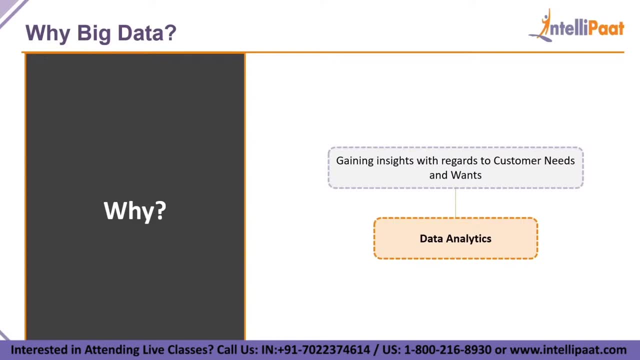 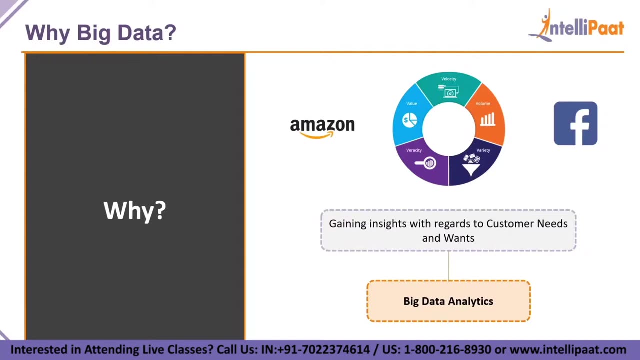 so that is how important this is: big data as a concept in general. so gaining insights with regards to what the customer needs and wants, that is, data analytics. and gaining insights with what the customer needs and wants when the data satisfies all of the five criteria that we had discussed. when the data is essentially of an 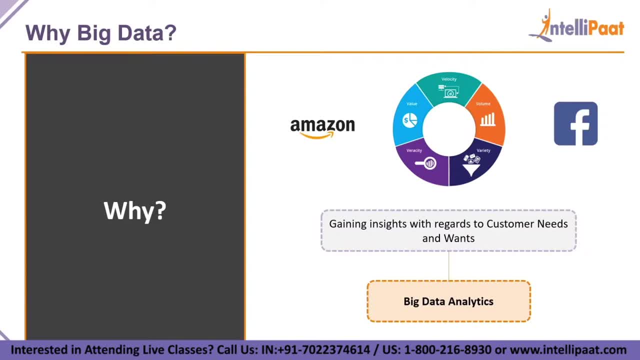 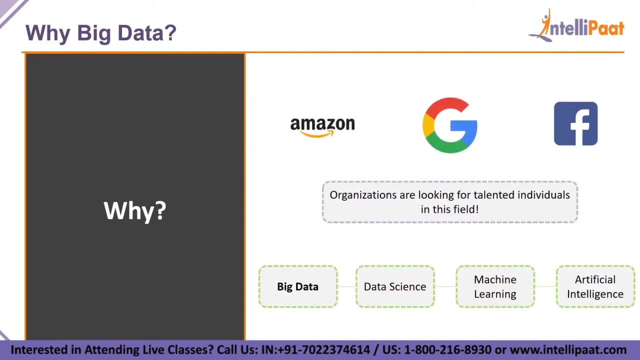 enormous scale, which would be the case for Amazon or websites like Facebook. right then, this entire process is called big data analytics. so organizations are looking for talented individuals in this field. big organizations, because a lot of organizations are generating data in that magnitude, so there is also a learning sort of. 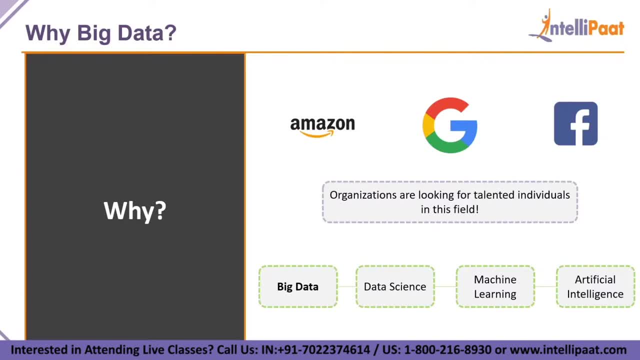 progression that is involved with big data. for instance, you will start with data analytics, you can get into big data, right, and then you can get into data science with big data. you can get into machine learning with big data and artificial intelligence with big data. so, rather than transitioning, listening withği Great work, the data analytics to an effective process beyond nemanth and data doctor大的 data, so we hope to bring next year a similar process. so the next slide is in three. today we will focus on education and learning services, for example, data analytics and data analysis. marketing and network and data analytics. 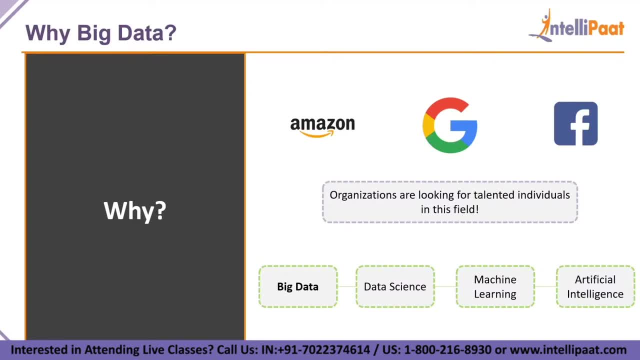 matters can sense major segment of making Internet. we will also start in longer term and serve in advance. second thing is that, as we started on online, our dimension is actually how exactly these areas of technology, rather than transitioning from a normal data analytics career to a data science career, where 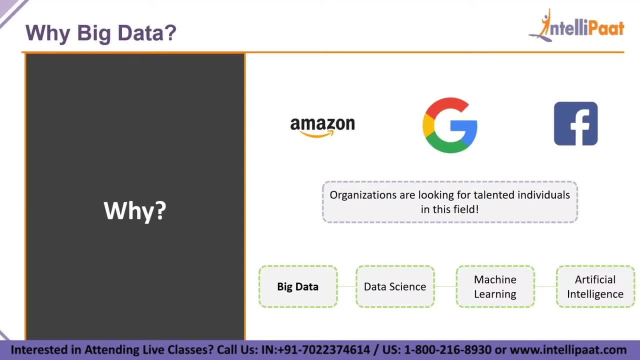 you're not accustomed to big data. when you know big data, you can essentially create more accurate- way more accurate- models in data science and machine learning, because your data set is extremely large. you know how to handle streaming data right. you can create these models way more accurately. 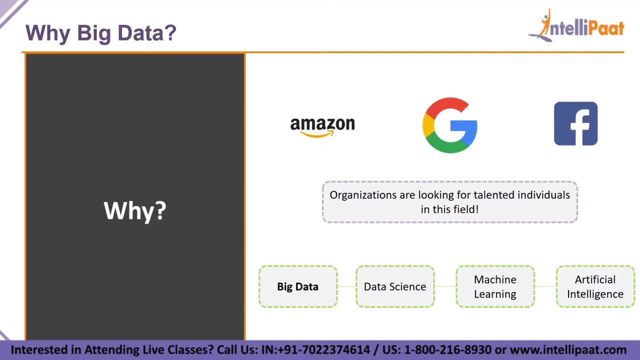 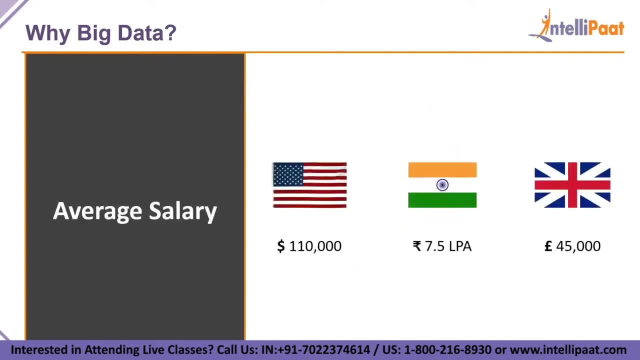 than anybody with just a normal data analytics experience. so that is the advantage that you get with big data as well. it gives you an edge in the industry. so the average salary in the united states for a big data analytics expert or a developer in the united states it's about 110. 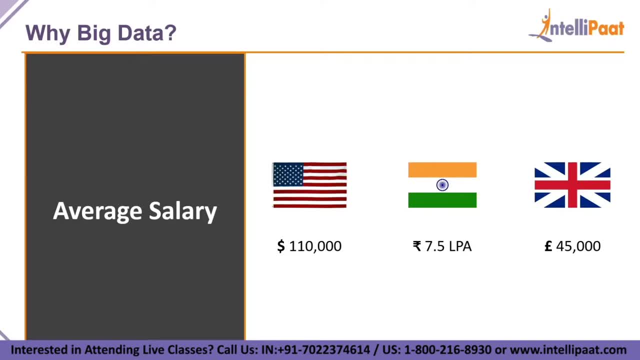 000. in india it's about 7.5 lakhs per annum. in the uk it's a good 45 000 pounds. so keep in mind this is the average salary right. so if you're getting into the field, you'll obviously get a lesser. 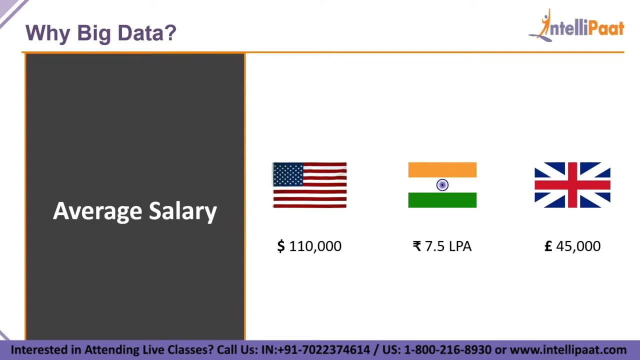 salary than that, but you, the more experience you get. uh, these salaries are not basically providing you with a limitation. you can gain more salary in it as well. you can expand your career, you can learn more technologies and you can increase your salary based on the experience as well. introduction to aws- big data. 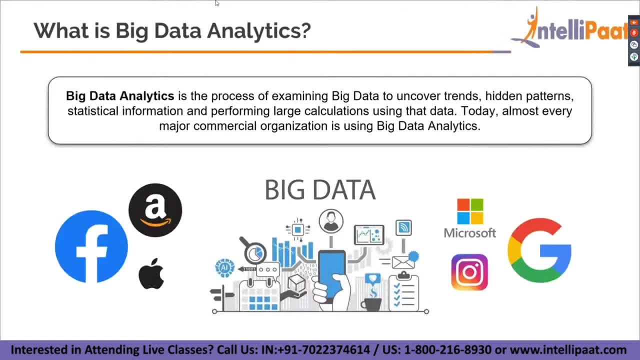 okay, so first of all, uh, let's say big data analytics, because that's what we'll be doing once you have a large set of data. if you have a large set of data, the main objective is to get some meaningful data or meaningful trend out of it. so let's say: 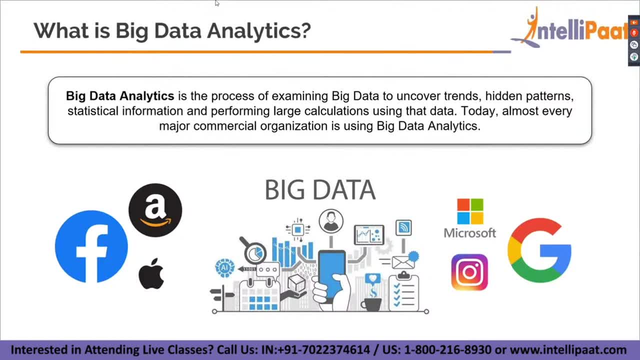 there is a company and they want to grow. so what do they do is they'll be gathering a lot of data, maybe from the user end, maybe from the applications end. once that data is collected, they'll process that data. once that data is processed, they will try to uncover some trends and they'll try to 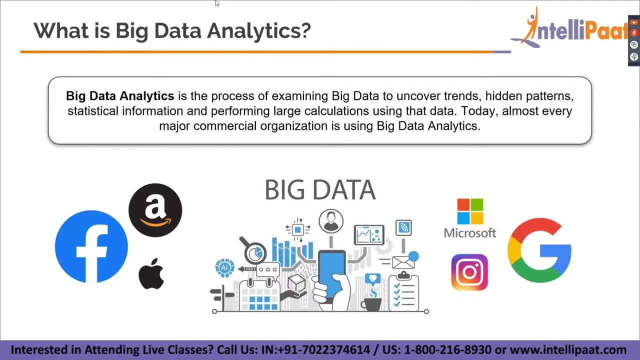 check some statistics which may be helpful for the business to grow. so you can see that today almost is using big data analytics. so if they obviously use, so these companies- facebook, amazon, apple, google, instagram, microsoft- so these all are major companies and obviously they'll be using big. 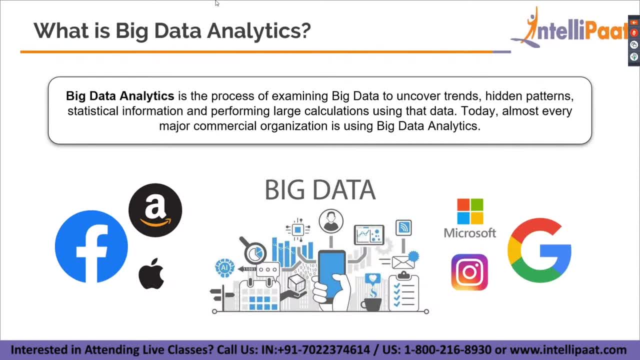 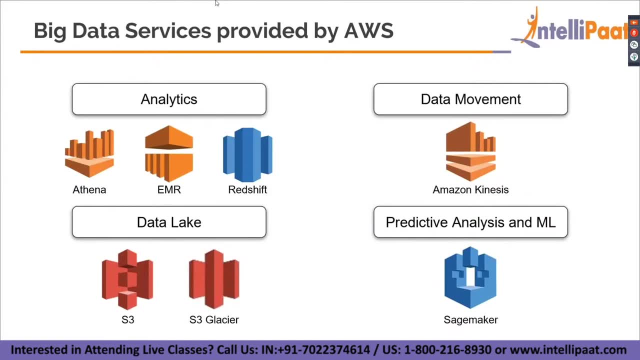 data, and so that's why big data is really important and big data is used everywhere. okay, now we've seen what exactly is that, so it's simply from a large set of data to get meaningful information. is big data analytics. so to do that, we have a lot of services, like in the local system. 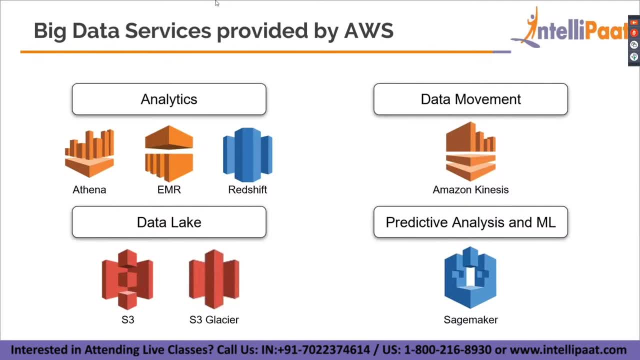 we can upload, or, in the on-premise setup, we can configure using the hadoop tools, using all the softwares provided by the hadoop ecosystem. so instead, if you don't want to use that, you can go with the cloud. so again, in cloud, there is azure, there is gcp and also aws. so now, as we are looking, 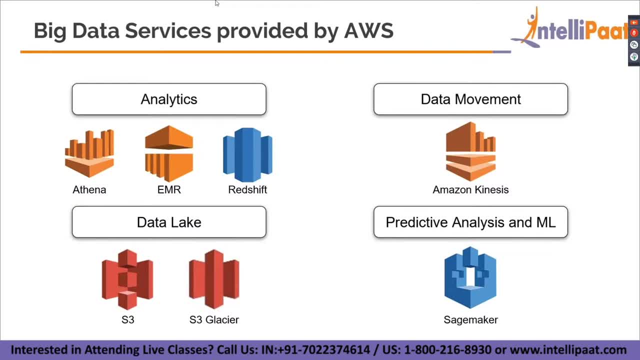 into aws. first let's look at the services provided by aws. so there are four divisions in big data services provided by aws. one is analytics, one is data movement, one is data lake and finally predictive analysis and machine learning. so first of all in analytics there is athena, and then there is emr, and then there is redshift, so athena is. 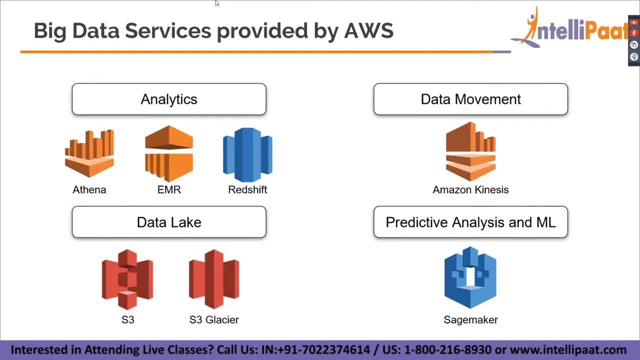 basically a query analysis software provided by aws. then comes elastic map reduce, which is basically a tool to provide the hadoop ecosystem on a cloud level. and third, redshift is a data warehousing tool. and then, coming to data movement, this is for real-time data streaming. for example, if you are watching youtube, when you click on a video, 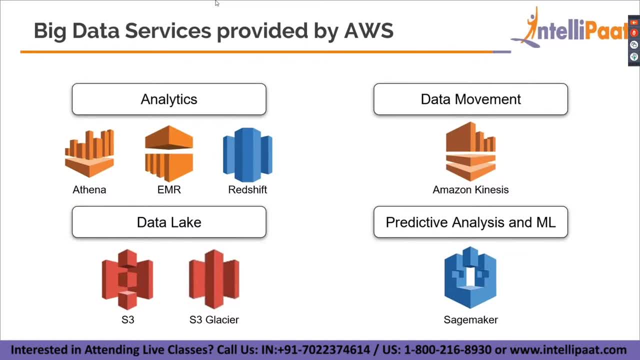 the video will be loading as well as you'll be watching the video. so basically, the data is gathered from somewhere and also you are able to access the same data at the same time. so for that you will be able to use amazon kinesis, and then comes data lake. so obviously to, let's say, to: 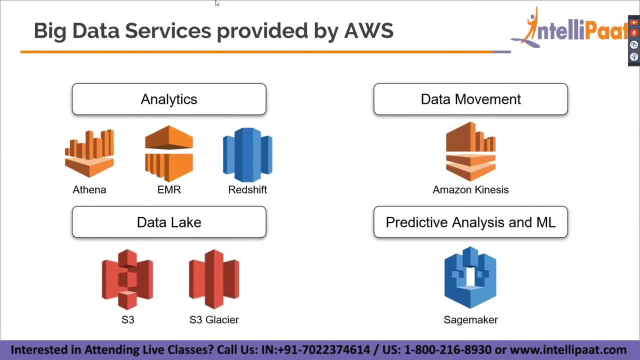 you actually need to store data somewhere, so s3, and s3 glacier takes that part. so s3 is where you store your data. if you want to backup or archive your data, you can go with s3 glacier. and finally comes sage maker. so sage maker is an ml tool, so it's a machine learning tool, if you know a little. 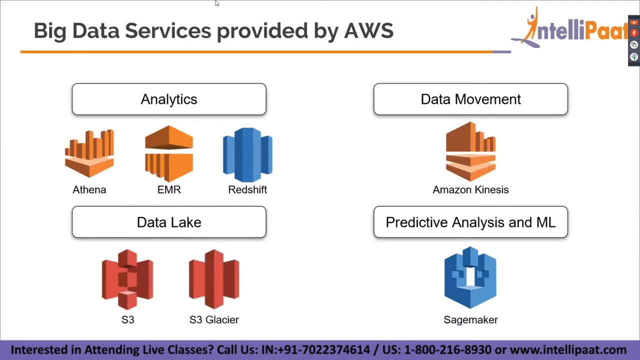 about aws. there was a tool called amazon machine learning. currently it is deprecated and everyone are used. moving to sage maker, because sage maker has all the built-in ml algorithms, for example k-means clustering. so if you want that, if you want to use that algorithm in your processing pipeline, then you can go with sage maker. it already has the. 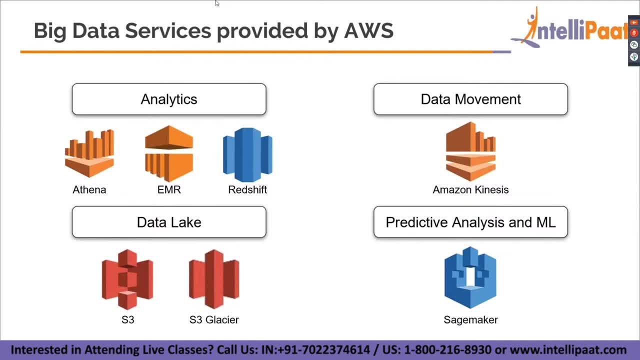 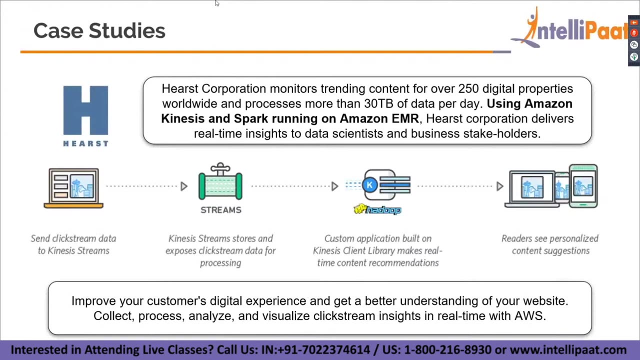 built-in algorithm. you can just implement it. so these are the services provided by aws. so now, using these services, how do company get benefits out of it? so that's what we are going to discuss in our case studies. first of all, we'll be looking at two different companies. one is hearst. 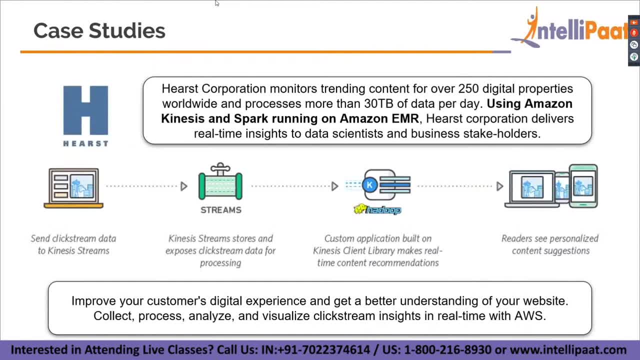 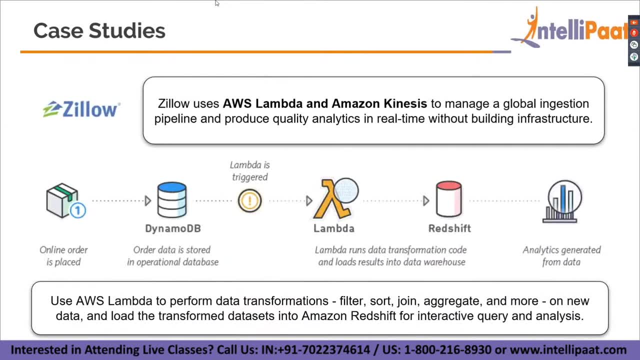 and one is sage maker and the other one is aws. so we're going to be looking at two different companies. one is zillow, so you might not have heard of these companies, but hearst is a magazine company and zillow is basically an e-commerce firm who sell products. so, coming to hearst, so 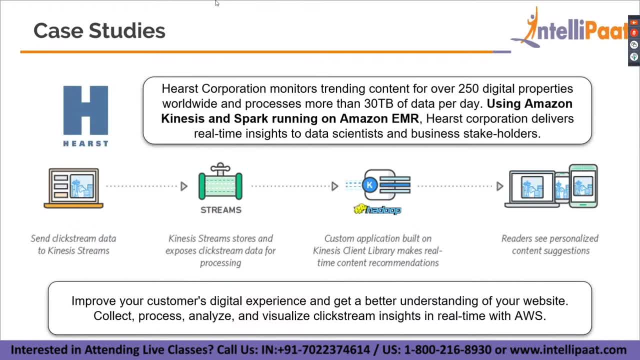 hearst corporation monitors trending content for over 250 digital properties worldwide and processes more than 30 tb of data per day. so 30 terabytes of data per day is quite a huge amount, and to handle that much of processing power you obviously need powerful systems. and therefore comes in amazon with kinesis to 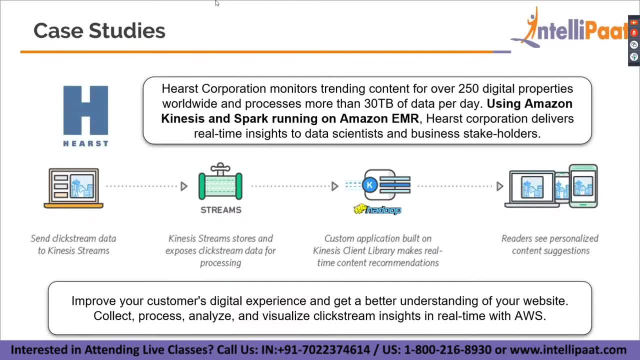 stream data, then spark running on emr to process data. so hearst corporation uses this to deliver real-time insights to data scientists as well as business stakeholders. so that's pure company part. so you can see the diagram in the below that. so first send clickstream data to kinesis streams. 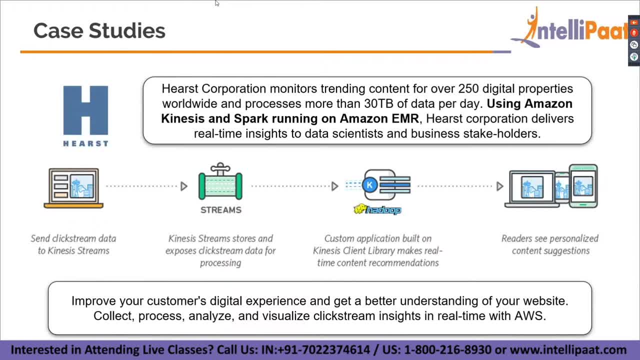 for example, if i'm a user, i'm reading the kinesis data. and i'm reading the kinesis data. let's say i'm reading a blog on uh sport. let's let's say i'm reading on a blog about cristiano ronaldo. so now once, i'm reading about that. so the next possible thing, uh, the algorithm. 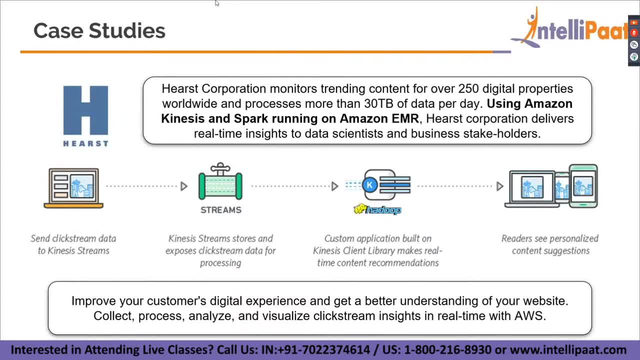 should understand is that i am interested in sports, i'm interested in football, so this person should be given football related content so that data will be taken. so kinesis takes all that data and it streams and it pushes into the client library which is running on the emr system. so on emr, there is an spark- uh, spark system running, so you would. 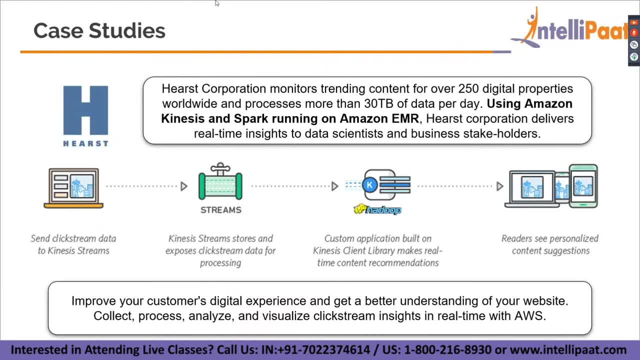 have embedded your code in that so that processes the data and obviously after that the reader- which is i am- i'll be getting suggestions which are personalized, that is, if i'm reading about football, i'll be getting articles related to football. so you can see at the bottom: improve your customer's. 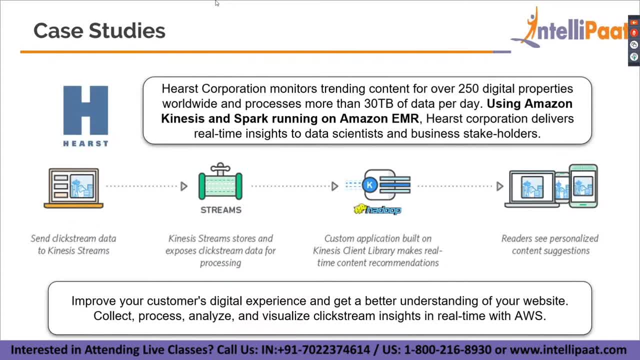 digital experience and get a better understanding of your website. collect, process, analyze and visualize clickstream insights in real time with aws. so to do this, you can see, you can use kinesis and spark. so that's what this organization is doing right now. so this is one of 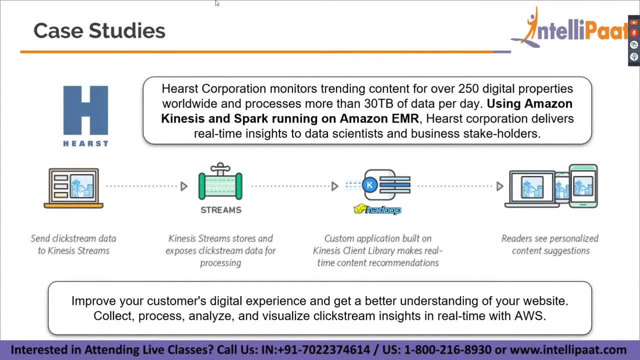 the uh, one of the real-time case studies, and i think you can understand this part why. how exactly is big data on aws useful for them? one more benefit is that they don't even need to manage anything over here. everything will be managed by aws. you will just have to set it up now. 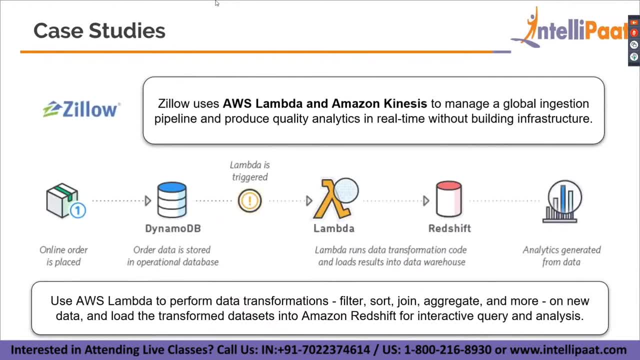 next case study is zillow. so, as i told, zillow is a e-commerce platform, so zillow uses lambda and kinesis. so i didn't discuss about lambda, because lambda does not actually fall under the category of big data. lambda is basically a background. let's say, to be more simpler, it's a software. 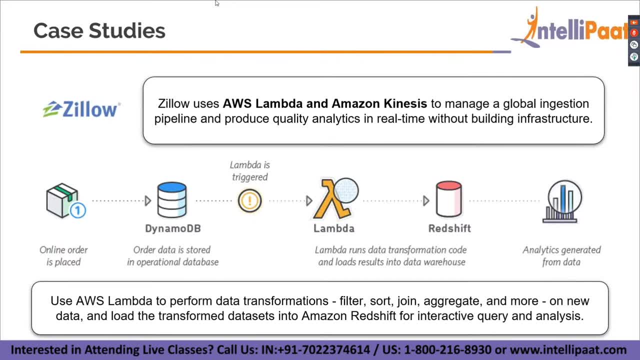 where you can put your code and whenever there is an event occurred. once that event occurred, this lambda function will be triggered and that code will run once. so this is why we use lambda, so let me explain that more clearly- so to manage a global ingestion pipeline and produce quality analytics in real time without building infrastructure. so zillow is using aws. 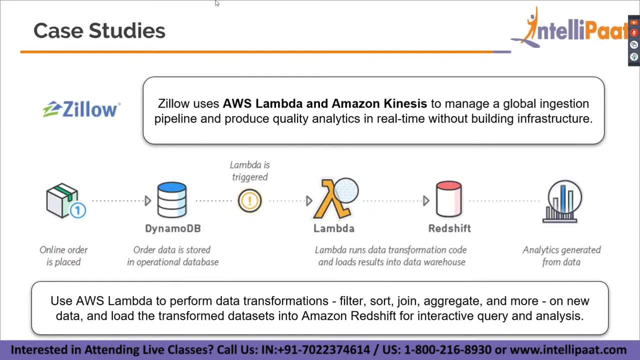 because they don't want to build an on-premise setup. they don't want to build an infrastructure because that needs a lot of capital. instead they are opting aws. so first, uh. now coming to the diagram. so an order is placed, so i'm buying. let's say i'm buying a bottle. so once i bought a bottle, 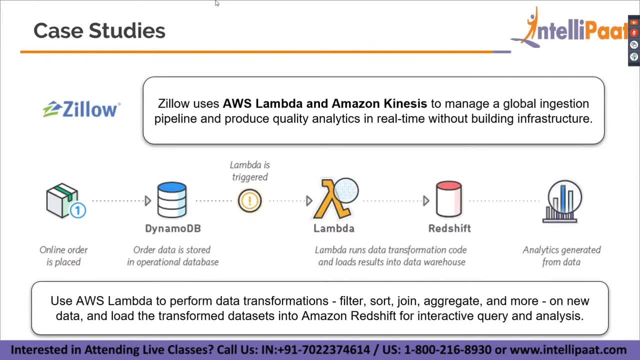 that data. obviously, once the order is placed it will be stored in a database. so let's say: that is dynamo db. so zillow is using dynamo db. so order data is stored in the operational database. so once that data is stored in dynamo db, so in lambda you have options to set up triggers. so let's say in lambda: 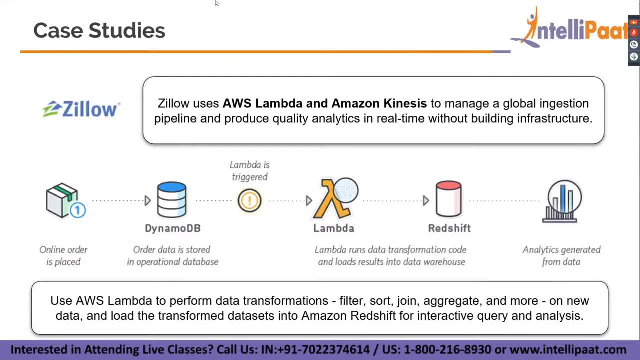 our trigger is going to be uh. whenever data is getting into dynamo db, lambda should be triggered and once it is triggered, the code in lambda will run. and once the code runs, the data is transformed. that data is pushed into redshift, which is the data warehouse, which is 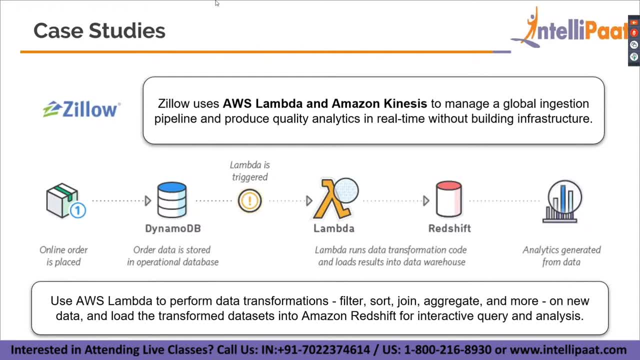 mainly used for analytical processing, that is, to get data out of it and make visualizations and analysis from it. so for analysis you can use any tool of your kind. you can use power bi, you can use tableau, you can use amazon quick site. so you have a lot of possibilities. but the 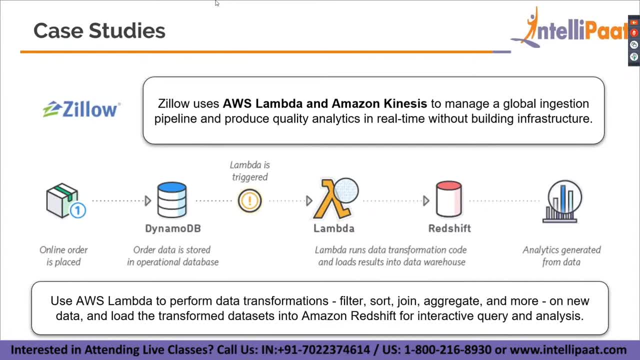 main part is you are storing data in dynamo db, which is a no sql database, comes lambda. whenever data is stored, lambda is triggered, lambda runs a code and that pushes the data into redshift, which is then used for visualizing data. so if you read the last para, that is, use aws lambda to perform. 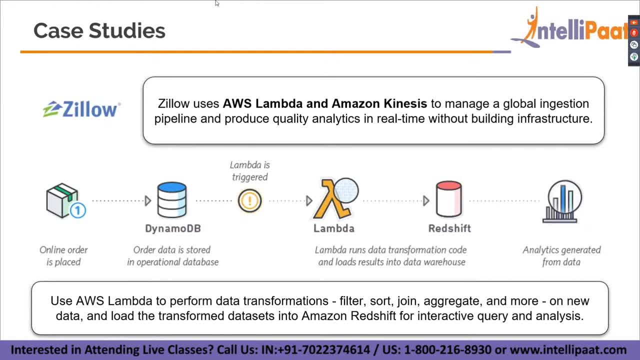 data transmissions- sorry, transformations, filter, sort, join, aggregate and more on new data and load the transform data sets into amazon redshift for interactive query analysis. so let's say, if you're uploading raw data to redshift then there is there is no use for that. data is stored in dynamo db. so 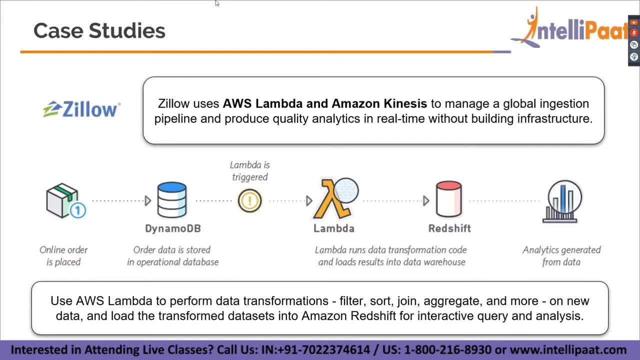 for that, because uploading raw data does not give you any uh ease of access. but if you transform your data into easily readable format for the computer and easily queryable format, then if you push it into redshift it will be very easy for analytical processing. so we've seen the case. 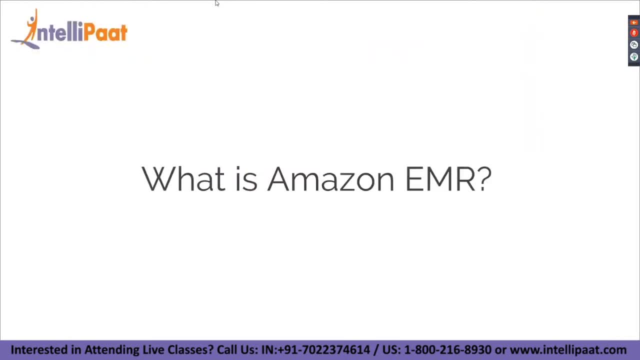 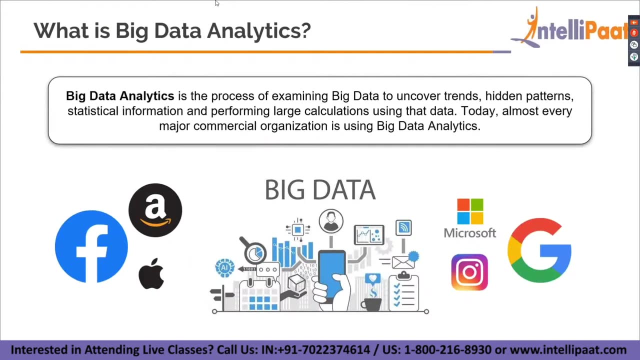 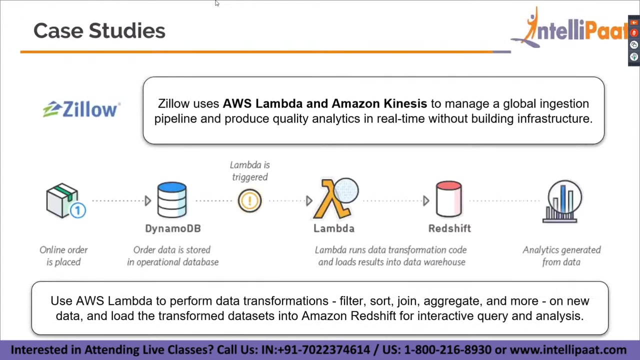 studies. one was for uh hearst and one is for zillow, okay, so we've seen that. we saw, yeah, we saw about uh, what is big data? then we saw the tool and we saw the case study. so one more thing why people prefer aws is there is no upfront cost. 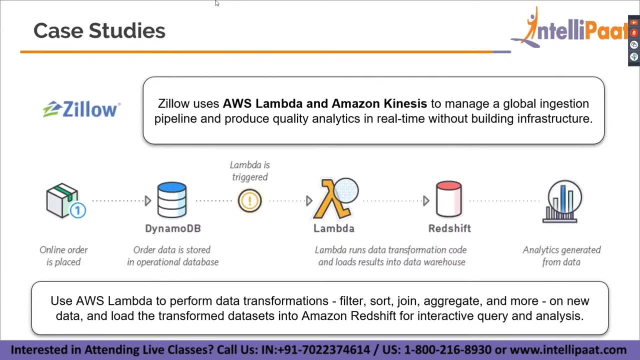 you only pay for what you're going to use. for example, if you're using a dynamo db for two hours, you'll only pay for that two hours. also, it is very easy to manage you. it is scalable. that is, let's say, if you're currently having one table in your database and it has 10 gb of storage, if you enable. auto scaling. if the data is incoming and there is a lot of data to handle, it will automatically scale your database size to 20 gb and then increments like, let's say, data is again coming in 30, 40, so it will be incrementing automatically. you don't need to worry about that. 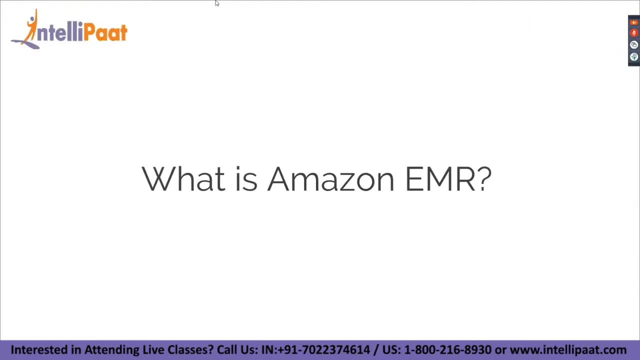 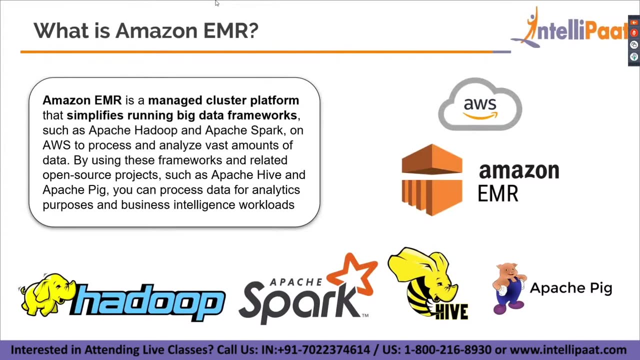 okay, so we saw that. now let's see what is amazon emr? okay, first of all, amazon emr is called elastic map reduce, so it is a managed cluster platform- that's sorry, managed cluster platform- that simplifies running big data frameworks such as hadoop spark. so the thing is to understand this much more easily. i think you should have a little. 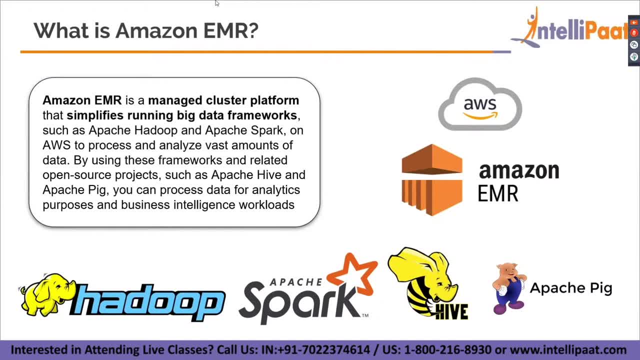 bit of idea about big data. so, because there is no use of explaining, uh, hadoop right now, because we are going to look at how, uh, these softwares for big data is used on aws- so just gather some little bit of idea. what is hadoop? what is spark? okay. so now on aws to process and analyze vast amounts of data? okay, so this is the 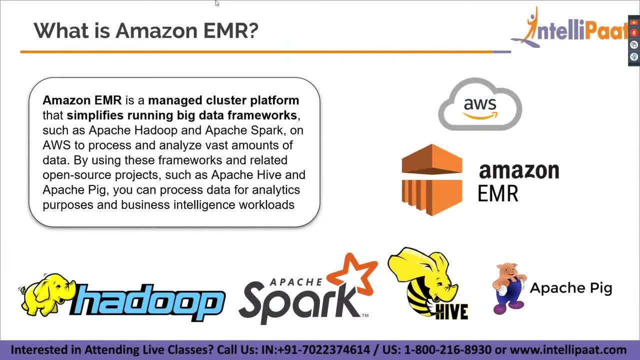 purpose of emr. by using these frameworks and related open source projects such as apache, hive, apache pig, you can process data for analytics purposes and business intelligence workloads. so, first of all, emr is called elastic map reduce and it is a managed cluster platform, so this will 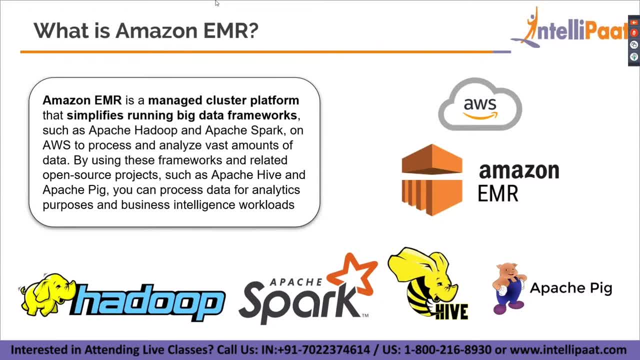 simplify big data frameworks. so let's say you want to run hadoop on the cloud. so instead of running a server, downloading hadoop in that and configuring every single step, you can just go ahead with amazon emr. just type in the name of your cluster, choose the softwares, choose the big data tools which you need. once you've done that, you can give. 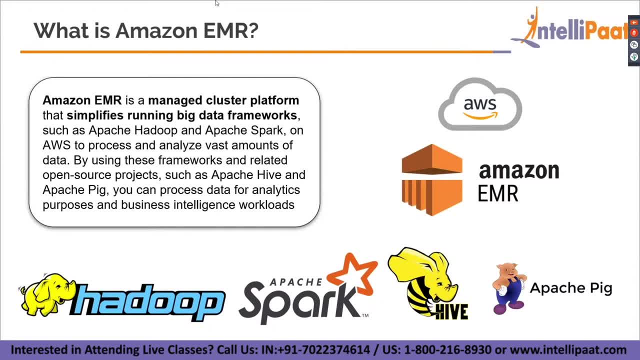 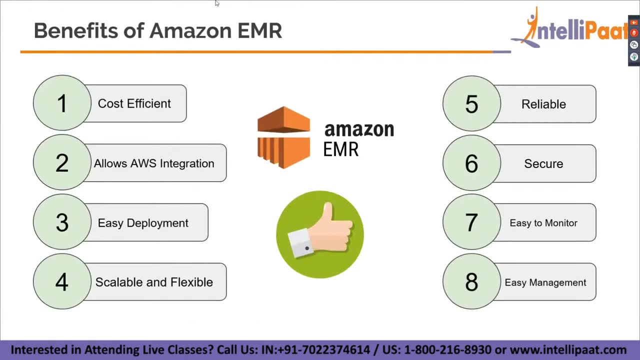 how many nodes you want. that is, the master and slaves. so let's say one master, two slaves. you can have that. once you mention that you'll have to provide a role and that's it. you'll just have to do the rest for you. so that's how simple amazon emr is. now let's look into the benefits of amazon. 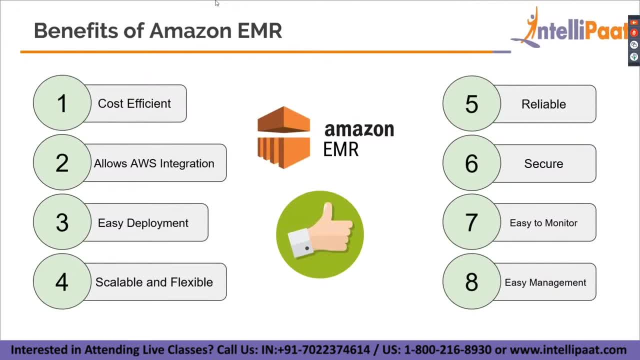 emr. so first of all, if you look into this, there is cost efficient, so that, as i told, you'll just have to pay as you go. then allows aws integration. you can integrate it with other aws services. then comes easy deployment. as i told you, you'll just have to give in. 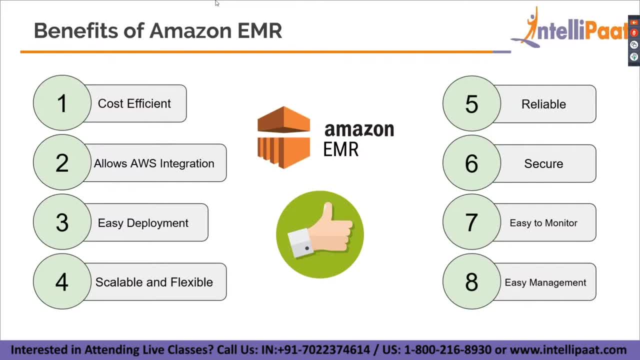 few details and hit, click. it'll automatically do that and then comes scalable and flexible. so, as i told you, there is auto scaling available and also it is flexible because you can terminate it, you can stop it whenever you want. it is reliable because they provide you an sla of 99.9. 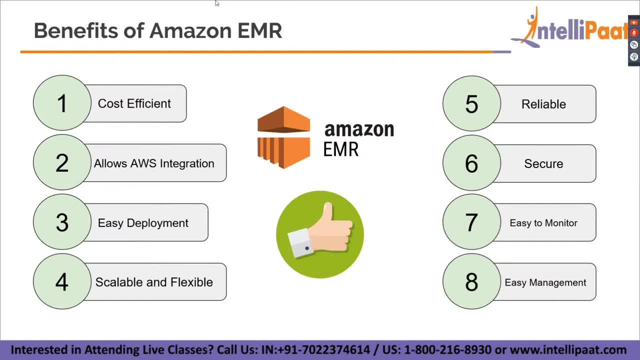 which basically means it never goes down, it is always on and then secure. so obviously aws provides you a lot of security features. you can use iam, which is for identity and access management, where you give permissions to users if they want to use it, and then you can use it for other services as well. 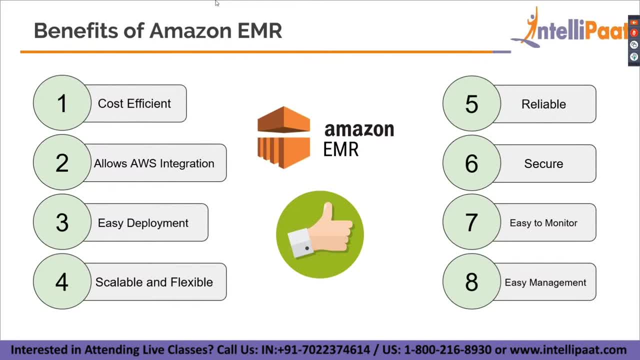 have. if they have the permission, they'll be able to use this particular service, emr, if they don't have the permissions, they'll not be able to use it. and then easy to monitor. so there is a service called cloudwatch, so it is automatically integrated with all the aw services, so you don't have to even. 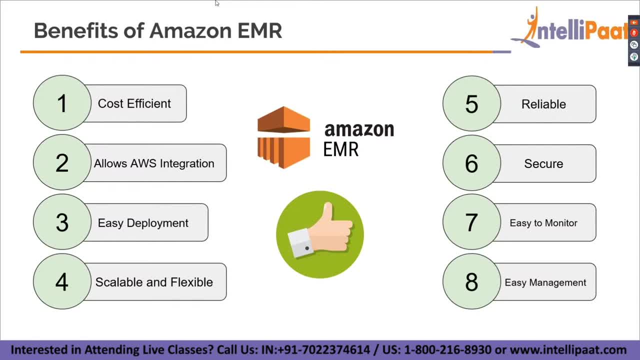 do anything, you can get the metrics automatically. finally, easy management. you're not going to manage anything, you're not going to patch anything, you're not going to add any code, you're not going to debug it. everything will be taken care by aws. you'll just have to set it up and that's it. so we've. 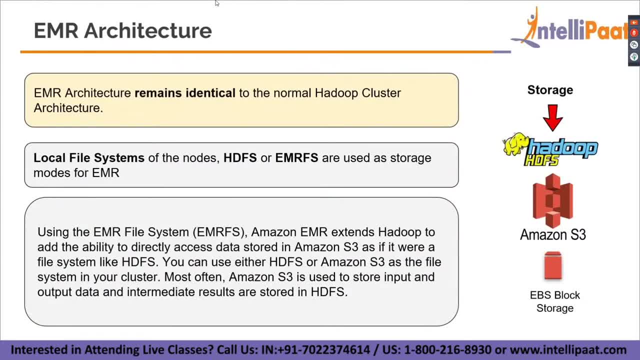 seen the benefits, as well then the emr architecture. so how exactly it? uh, so how exactly it is? what is that hosted in the cloud? so that would be your question, right? so let's say, in your local system you would have the how to pick a system because you'll know you will be downloading it and then 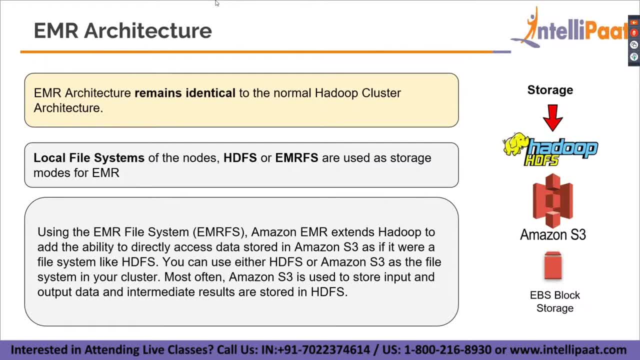 you will install it, you will configure it, you will set it up in the cloud. it is almost the same. so you can see that emr architecture remains identical to the normal hadoop cluster architecture. local file systems of the nodes, hdfs or emrfs, are used as storage nodes for emr, so you 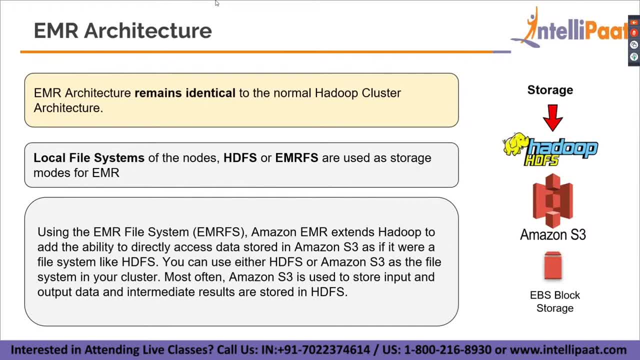 can use the local file systems of the nodes, that is, local file systems in the sense the local file systems which is hosted in the cloud, so that local file system is basically amazon s3. so s3 is the back end for hdfs. so, as i told you, s3 is used for storage, so s3 is also used for storing hd. that is. 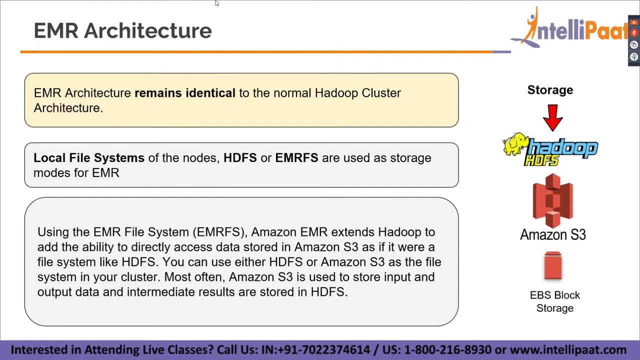 storing files in it. so using the emr file system, that is, emrfs. amazon emr extends hadoop to add the ability to directly access data stored in amazon s3. it is not that you will have to push the data into hdfs and then you'll. you will have to analyze it. instead, you can store the data in amazon s3. 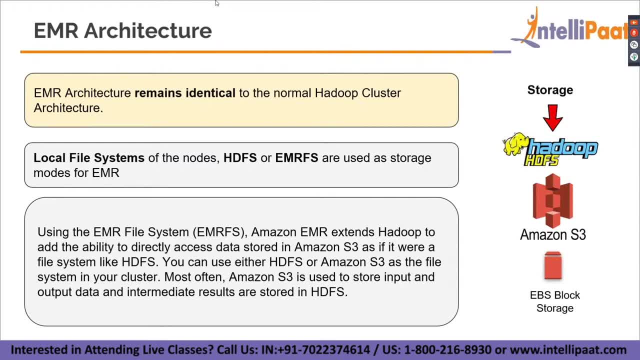 and directly from s3, sorry, yeah, so directly from s3, you will be able to query and analyze the data. most often, amazon s3 is used to store input and output data and also the results are stored in hdfs. so these are the temporary files are basically stored in hdfs. the input data and 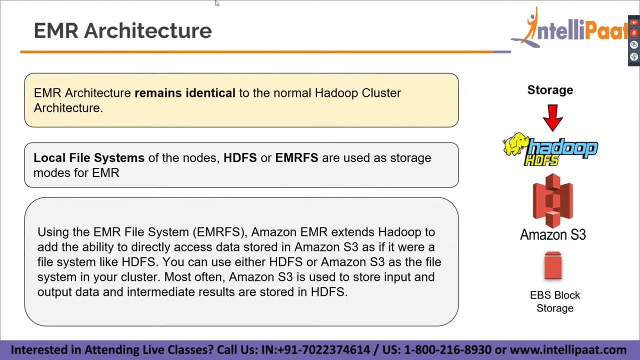 the output data. both are stored in s3. so this is how it basically works, guys, it's pretty simple, uh. if you know about the big data services, it is the same architecture on aws as well. so if you don't know the architecture, i uh tell you. so i ask you to go, and please go and check. 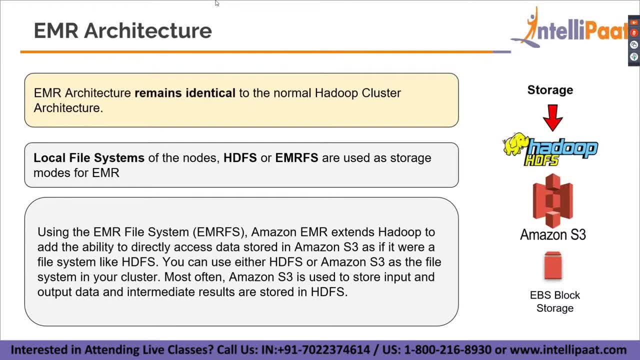 that out, check out hdfs, check out hadoop, check out map reduce and all that. so once you get, uh, an idea of that, you will get an idea of how it is hosted on the cloud, because it's similar. so let's say it will have a back-end server running and in that 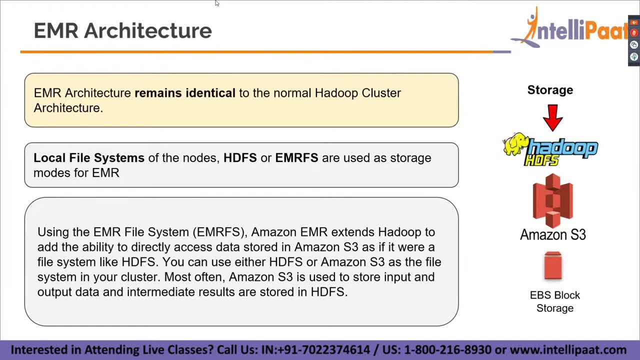 case, the hdfs will be installed, configured and everything would be set up over there. and once that is set up, guys, uh, amazon s3. it is pretty simple. i'll show you how to start up with that as well, and then you will be able to set up, uh, whatever service you want: hive, hadoop, spark. 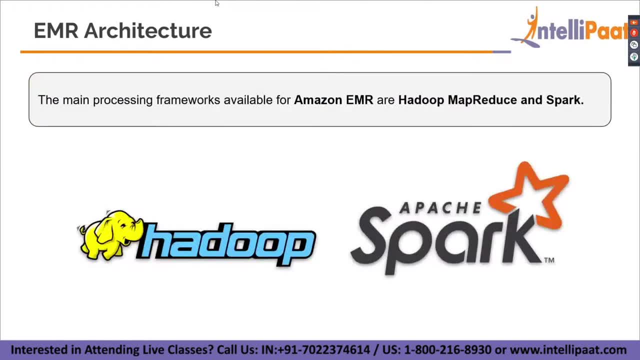 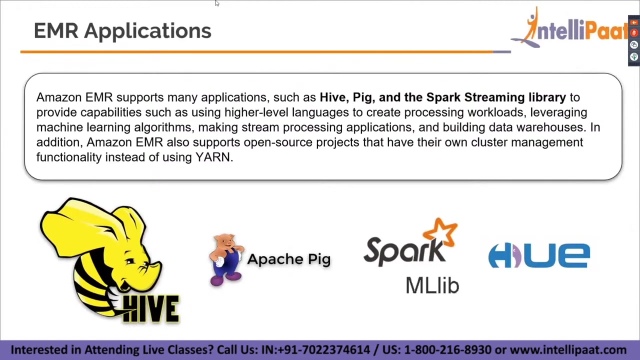 uh, hitch base anything. so this is the basic architecture. okay, so the main processing frameworks available for emr is hadoop, map, reduce and spark. so one more thing: the most popular frameworks are hadoop and spark. there are other frameworks which you can use on emr as well, but the most popular ones are hadoop and spark. okay, so now emr applications, that is. 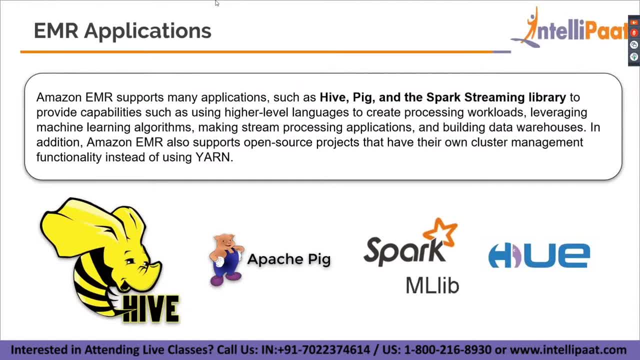 what are the other applications available on emr? as i told you, you can see over here, it supports many applications: hive pig, spark streaming platform. it supports yarn, it supports hue. it supports mostly all the uh apache products, that is, the hadoop ecosystem products, so you can go ahead and look into that uh more. 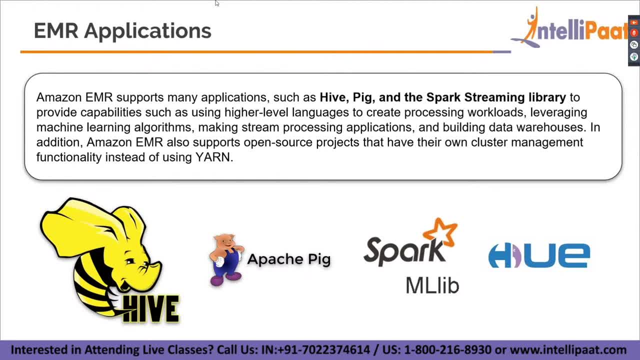 so we'll not be covering this a lot now. next i'll be doing a hands-on using hive on emr, so let's do that. so in addition, amazon emr also supports open source projects: that that have their own cluster management functionality instead of using yarn. so instead, 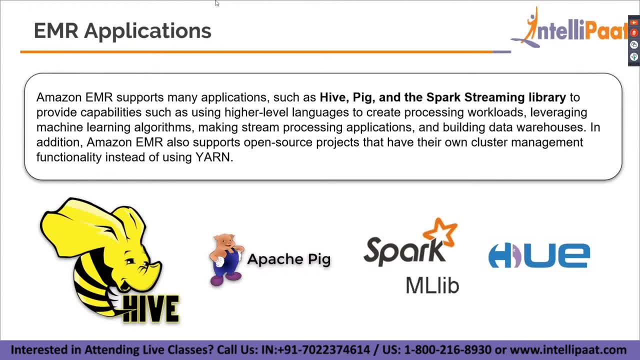 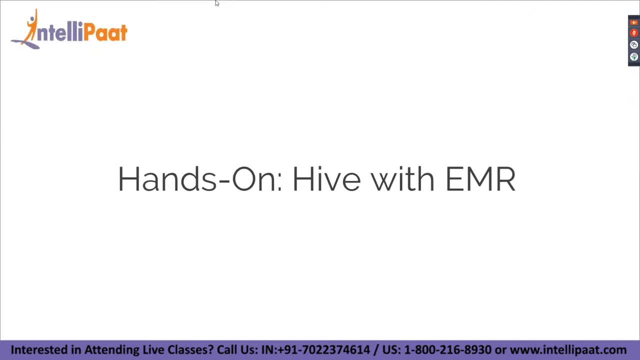 of using yarn. if you are using your own resource management, then that is also fine, so emr allows that as well. okay, guys, so we've seen that, so now let's do an hands-on on amazon. so this is basically getting to know session. so you will get to know how to start off with aws and aws- big data. 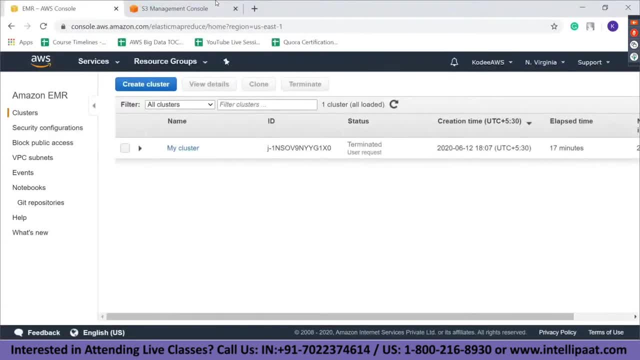 so, first of all, to start off with this, you will need an aws account. so i suggest you to get an aws account soon and start practicing, because this session will be available in our youtube channel and you can go through over that. okay, so right now i'm already in the emr console. i'm 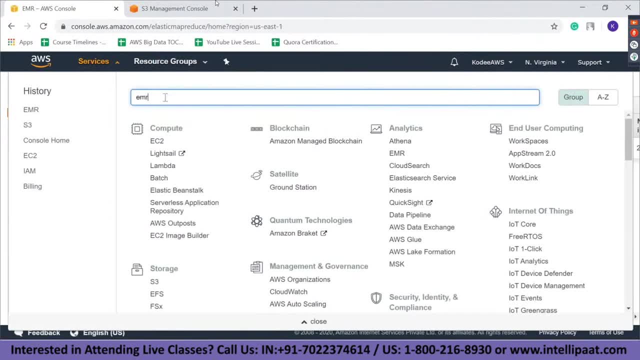 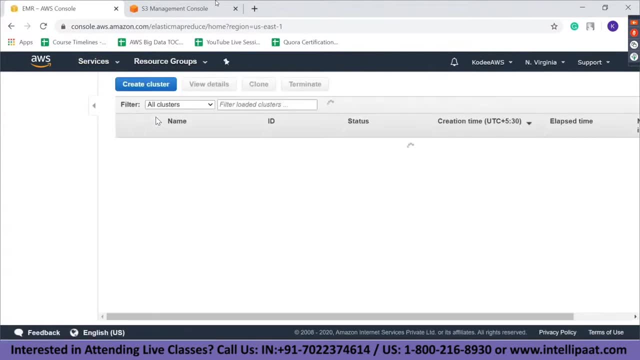 logged in and it's pretty simple and you can just search emr over here and click here and you will be inside the emr. yeah, so i am here. so just once again, i'll have to show you s3. okay, first of all, let's uh create a bucket here. so what we are going to do, we are. 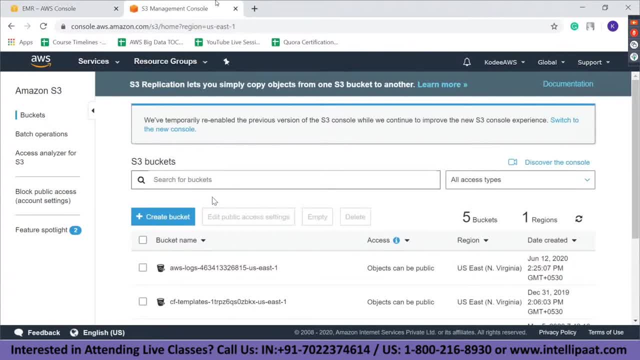 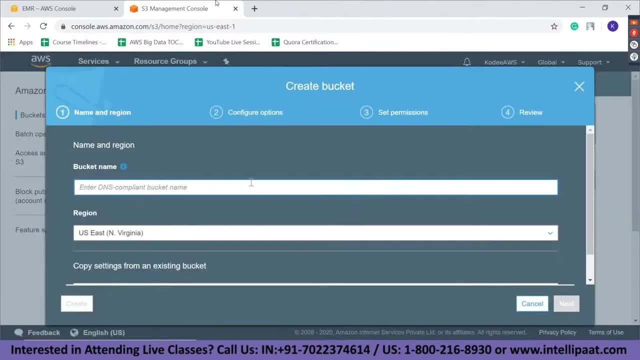 going to create a bucket to get our output, so our output will be stored in the bucket. we are going to create a bucket to get our output and then we are going to create a bucket. so this is the. this is very simple. click on create bucket, provide a name. so let me give as youtube live webinar one. 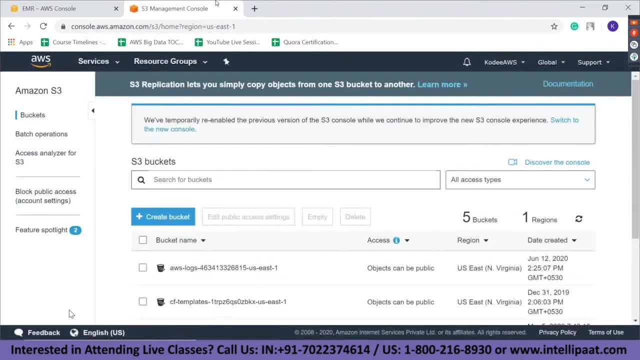 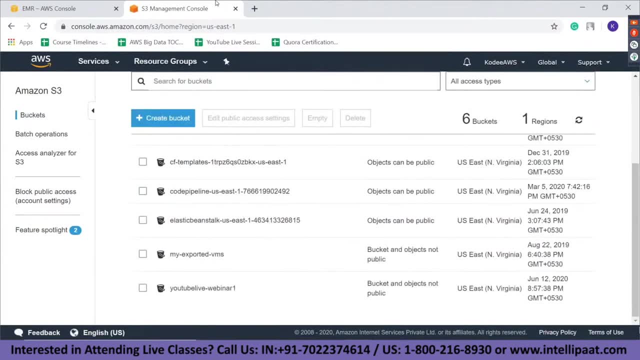 and i'm going to just create. i'm not going to set up anything, i'm just going to create this. so it is this simple: to start a bucket. so a bucket is basically a repository or a folder where all the files are stored. so it's pretty simple, guys. you'll just have to remember that. so a bucket is. 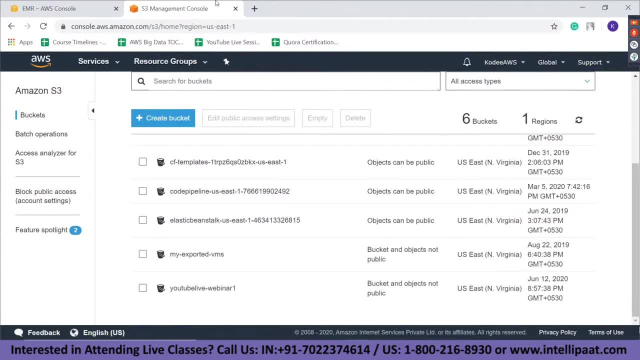 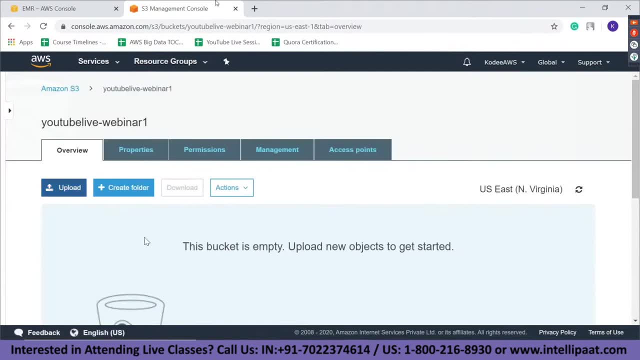 where you can store all kinds of files. it may be video, audio. all kinds of binary files can be stored here. so we've created a bucket so you can see. there's an upload option as well, but we're not going to upload anything over here right now because this bucket is for our output. okay now? 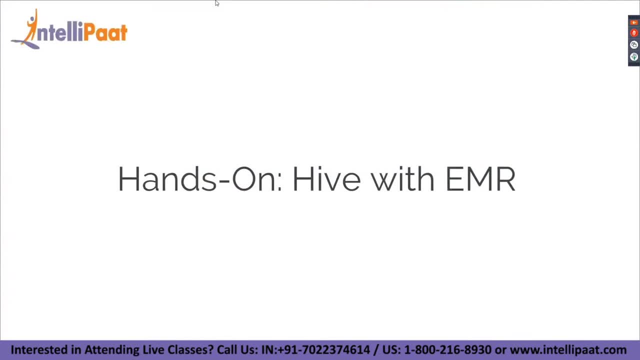 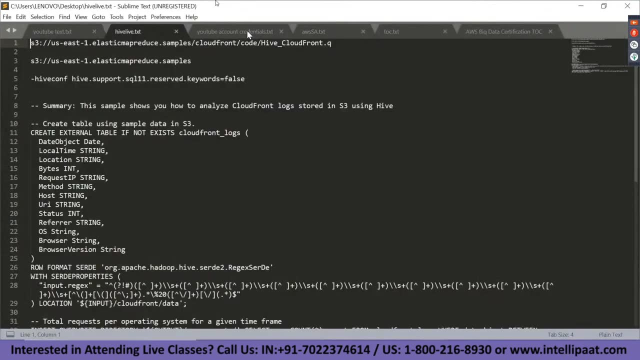 let's start with emr. but before starting off with emr, i'll just get a file once again. yeah, so the file is over here. just a second, i'll just close these. yeah, okay, so we are going to create a cluster. so while creating a cluster, i'll be explaining that. 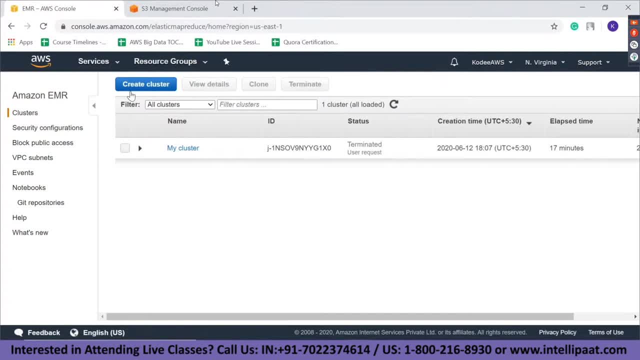 so first of all, to start off with emr, get yourself an aws account. but there is no free tier in emr, so there will be a small charge. it will be around, let's say 0.04, so let's say 0.04 dollars, something like that. it will be a very small amount so you can go ahead with that. but 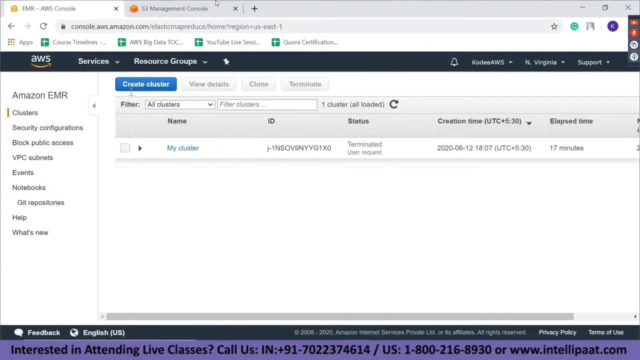 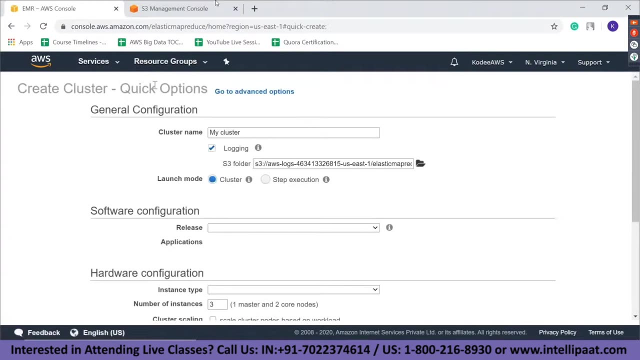 make sure that you terminate your uh cluster immediately. so create cluster. so first of all, to start off with emr, as i told, you get an account, then you can start off with this. then come to amazon emr, go to clusters, click on create cluster. okay, so now it's the simple setup. it's very, very. 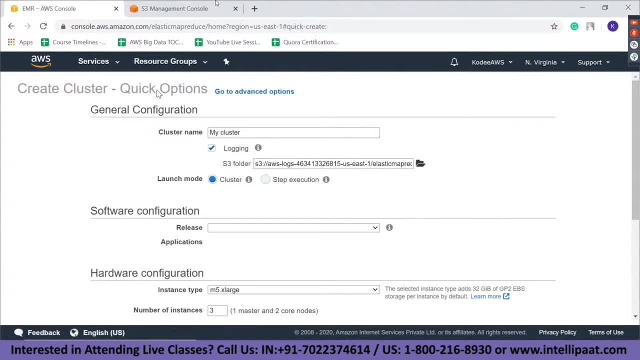 simple, yeah, okay. so first of all, give your cluster a name. i'm going to name it as webinar cluster, okay, and then let logging be on. logging in the sense: whatever happens, the setup, the, let's say, the configuration, everything will be loaded and it will be stored in this folder. 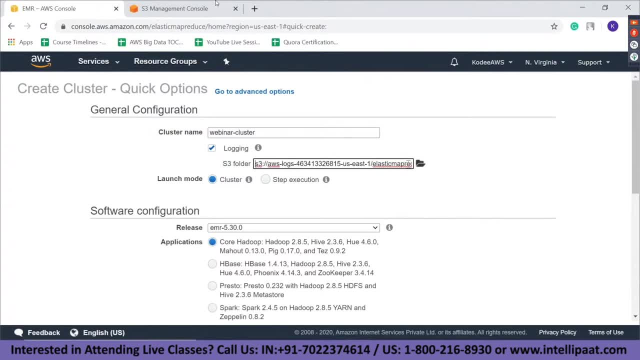 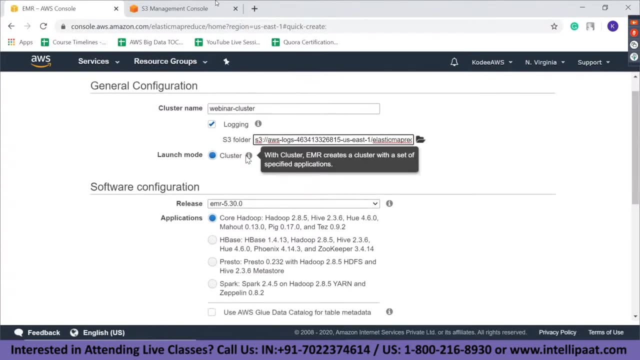 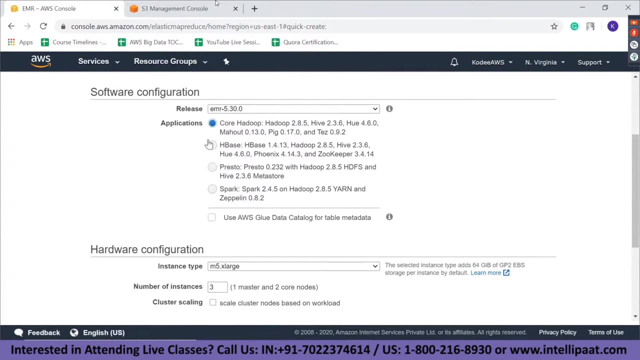 so it will be stored in this folder, in s3. so let it be, that's fine. next coming down. so this is going to be cluster. we are going to uh, start with a cluster and software configuration. so this is where you'll have to choose guys. so here you can see code hadoop. that is hadoop, hive view, mahout pig and test. 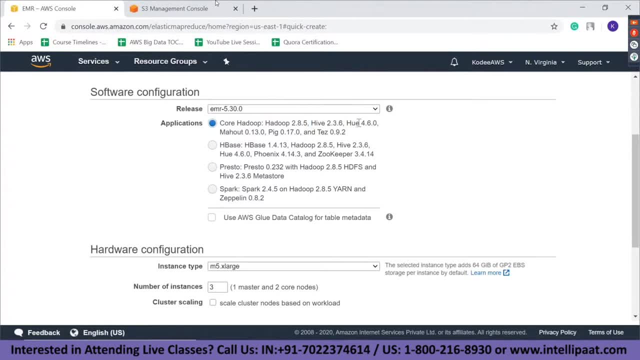 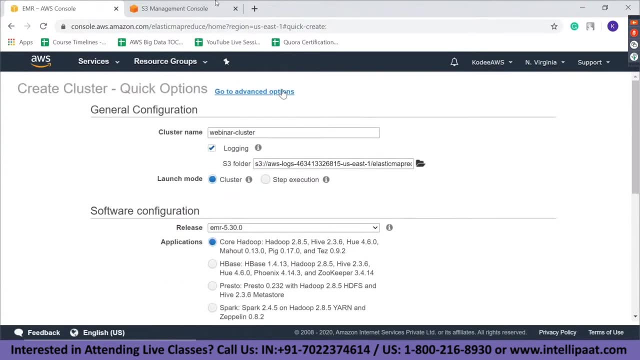 so, anyway, we are going to only use hive, so i'm going to choose first one. then there is for hbase, presto and spark. if you want more options, if you want to choose multiple services, you're going to need a little bit more. so this is the first one you can use and after that you can. 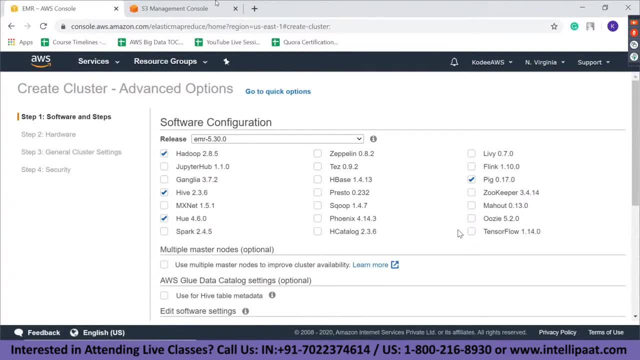 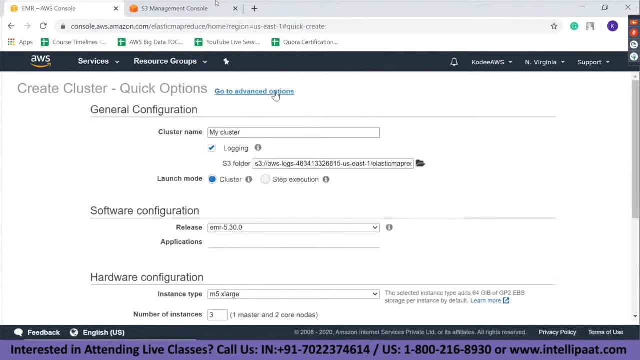 go to advanced options and so, and you can see here you get to see all the available applications. you can choose whatever application you want. example: tensorflow, zookeeper. if there is kafka, then there is flink test. you can choose whichever you want and then you can set it up. but right now, 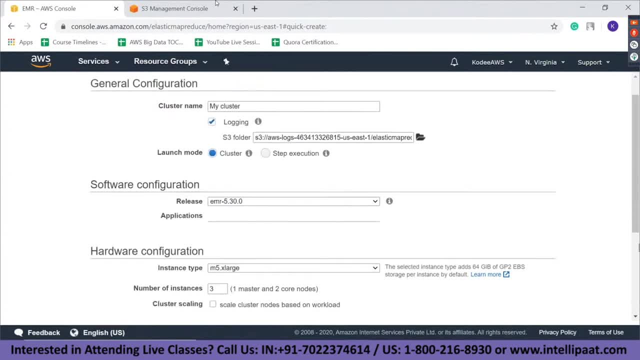 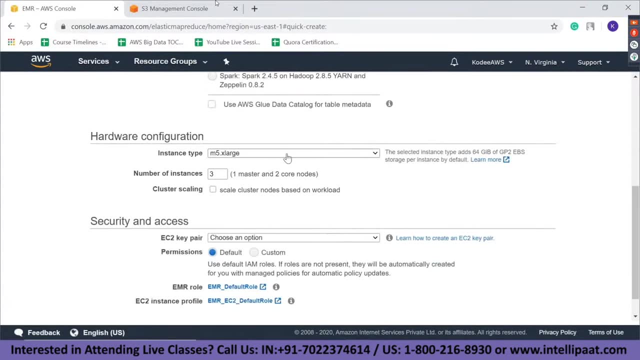 we are going to go with quick options because it's easier to understand at the start to change anything, and so you can see. yeah, so i'm going to go with core hadoop and this is the most basic instance type in emr. so let it be, and the number of instances are going to. 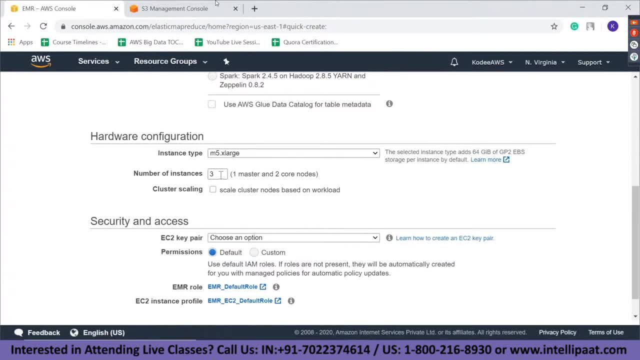 be three. there will be one master and two core nodes, which is basically one master, two slaves. so that will be a master slave architecture, and then i'm going to choose an ec2 key pair. anyway, we're not going to use this, but if you want to log in to the hadoop system and check out what is, 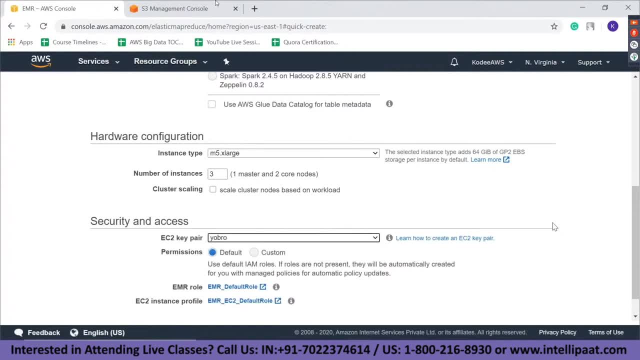 happening inside of it. you will need this, but anyway, we're not going to open it, but still i'm showing you. uh, so, key pair. you can learn about the key pairs and how to log in with the key pair from our other aws tutorials in our youtube channel. you can check that out. 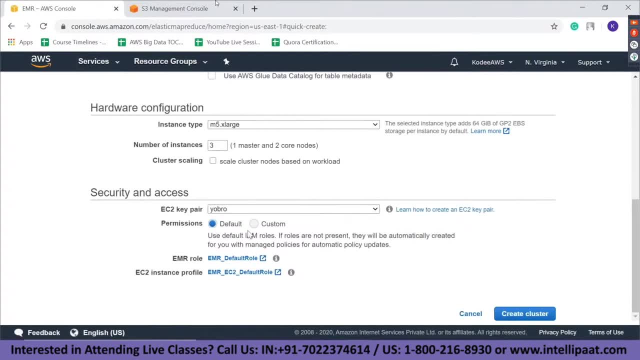 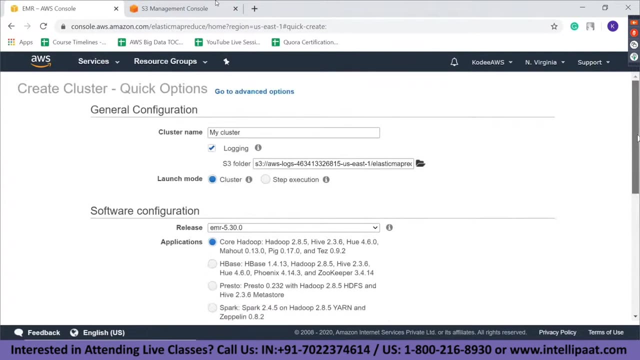 okay. so, uh, this is my key pair and choose a permission. i'm going to go with default because it is already configured, as we will be taking the data of uh, pushing the data into s3, so i'm going to go with this. uh, yeah, okay. so now you can see this and if i hit create cluster, it will start, but i'm not going to do. 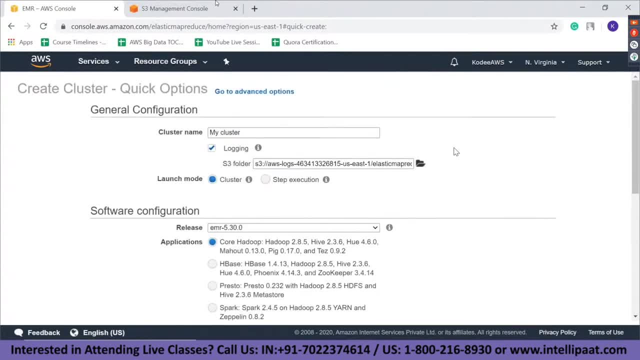 because i'm going to go and do this exact same thing in advanced options. i think i understood this part. if i click create cluster, it will create a cluster. so there's there's one small step in this, that is, we'll have to, uh, mention the input data. 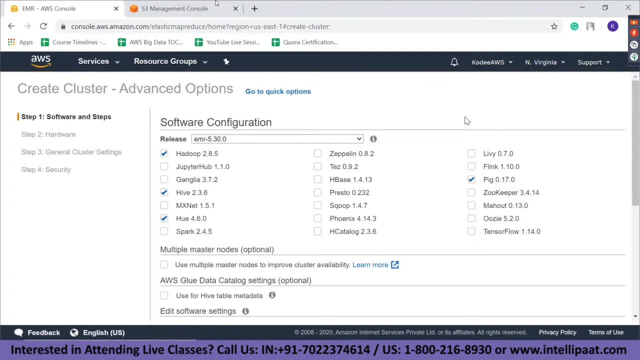 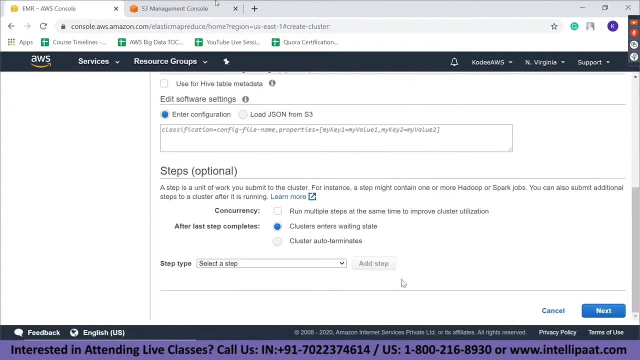 and the output folder where the uh result has to be stored. so i'm not going to make any changes. it is going to be the exact same configuration. i'm not going to change anything. the only change we'll be making is adding a step. so our step would be a hive program, because that is what 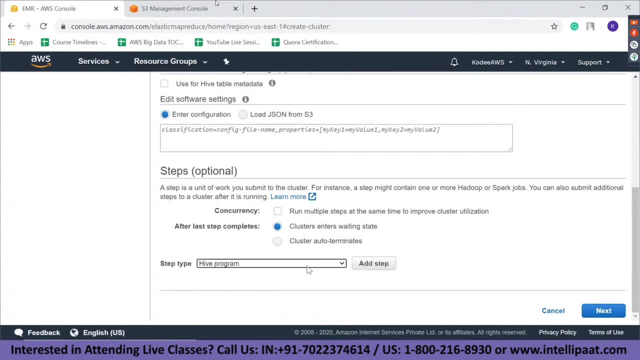 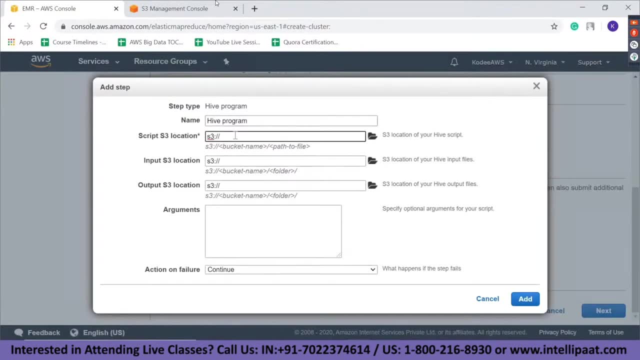 we're going to do. we are going to include a hive script, so i'm going to click that and i'm going to click add step. okay, so you can see script s3 location. so we'll have to provide the location of where the script is available. then we'll have to provide the s3 location of the input files and 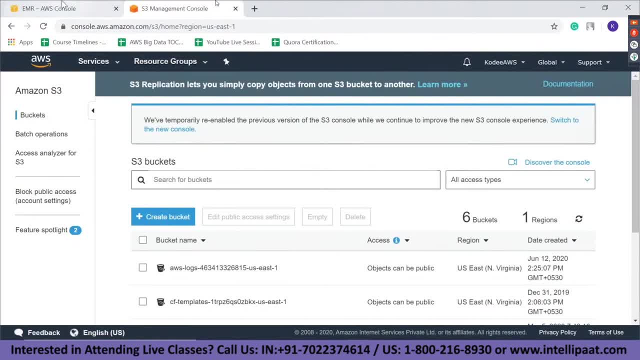 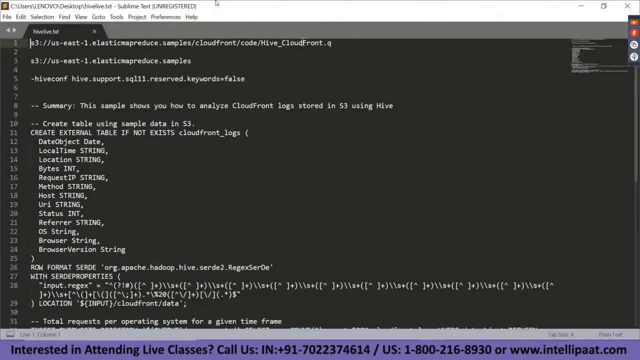 then we'll have to provide the output location which we created, okay, and an argument, okay. so that is fine coming down. so this is what i wanted to show you guys. so if you want to check out this, you can just go ahead with the documentation provided by aws for amazon emr. so this is one. 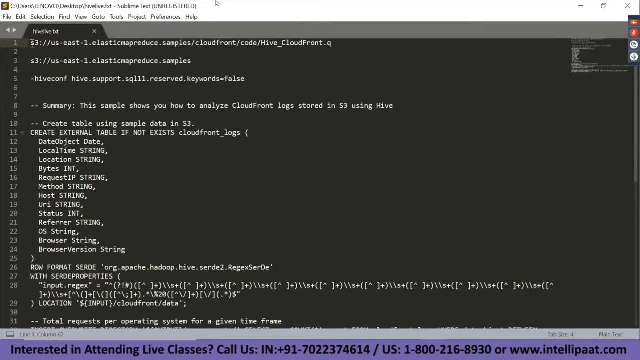 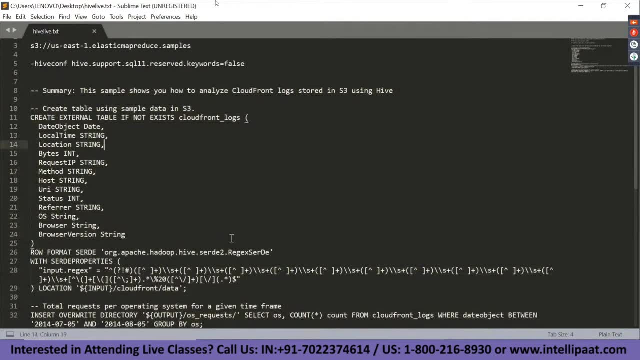 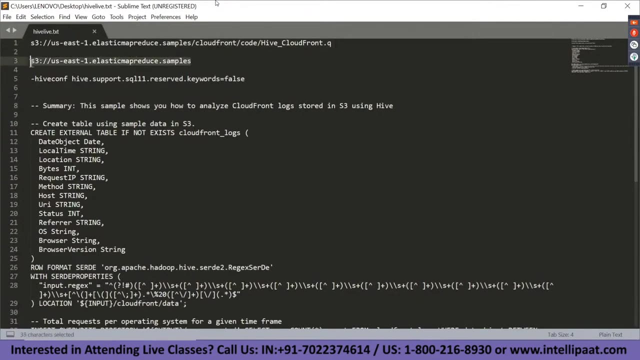 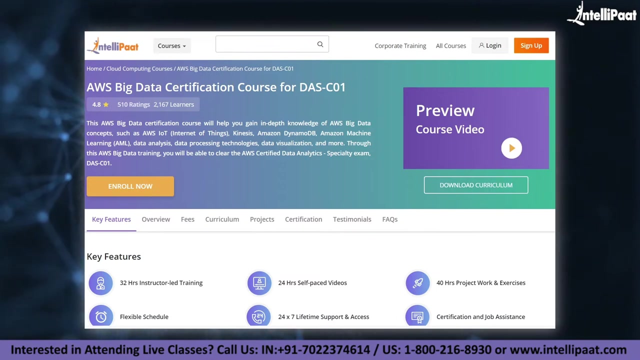 of the tutorials they provide. so this is the script link. so the script is over here. i'll explain to you about this. this is the script, this is the script link and this is the input folder. so, as you can see, just a quick info, guys. intellipaat provides aws big data certification course. 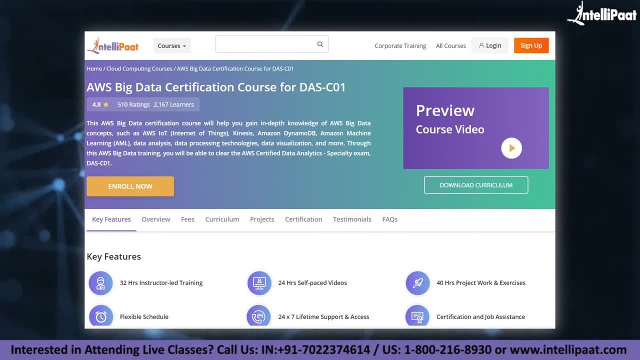 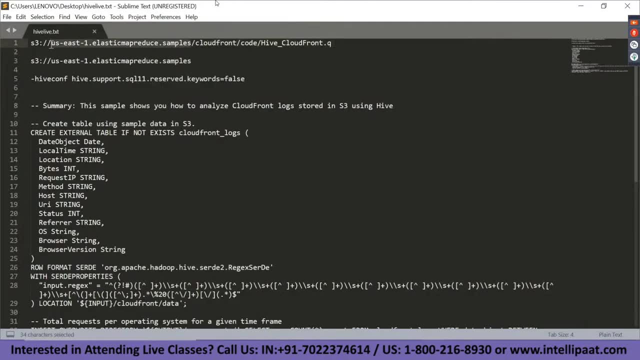 mentored by industry experts, the course link of which is given in the description below. now let's continue with the session. this is the input folder of the s3 bucket and inside this bucket there is a sub file called cloudfront. inside that there is a sub file called code. 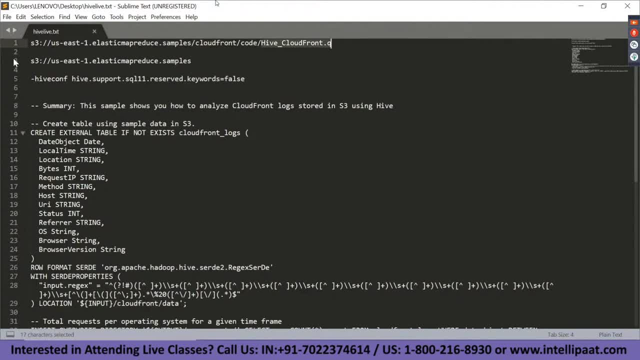 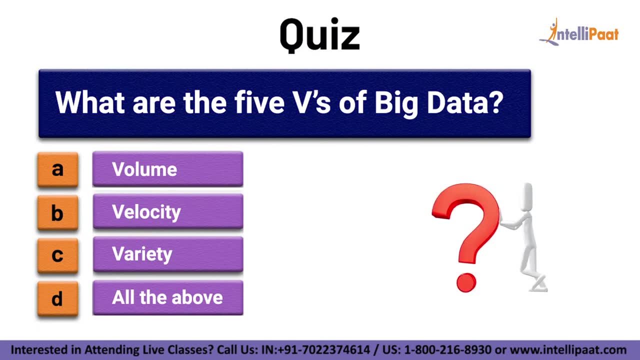 and inside that there is the script file- okay, that is fine. and then there is the input. just a quick info, guys, test your knowledge of big data by answering this question. what are the five v's of big data? volume b, velocity c, variety d- all of the above? comment your answer in the comment section below. 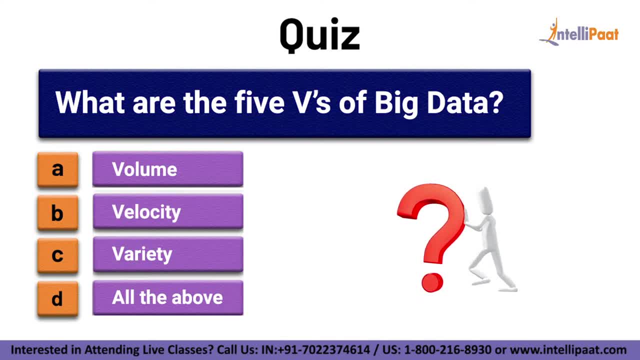 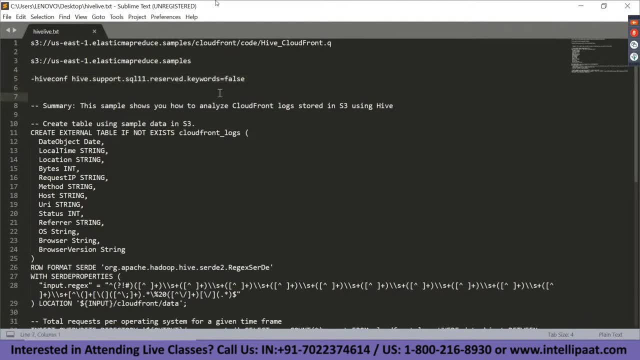 subscribe to intellipaat. know the right answer. now let's continue with the session. okay, and this is basically a command which aws told to add in the argument section so that if there is any uh keyword mismatch, it will automatically take care of it. okay, that is fine. next coming to summary. so this is the script which will be running in hive. 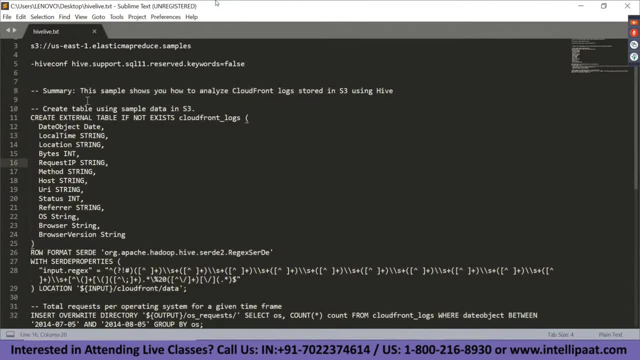 okay, so you can see this and this is pretty much pretty much it uh what exactly we are doing right now. so this sample shows you how to analyze cloud front logs stored in s3 using hive. so we are using hive on emr to analyze logs which are generated from cloud front, but we are not going to do 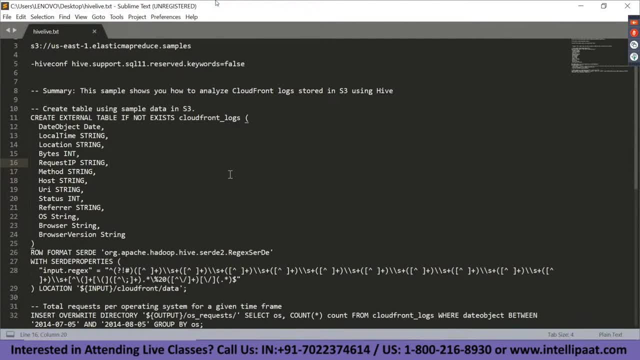 anything in the cloud front. that logs are already stored in s3, but not in mine, in a official sample repository. so we are going to take that data, push it into hive and once it is in hive this script will run. this script will process the data and give us the output and we can download. 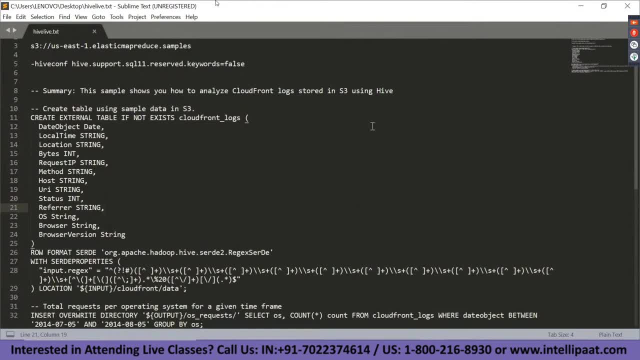 it and check the acquired results. so to check that, first of all you'll have to set it up, and before that you can see over here you will have. so this script is creating a table, so it's creating a date. it's- uh, you can see local time, location bytes. 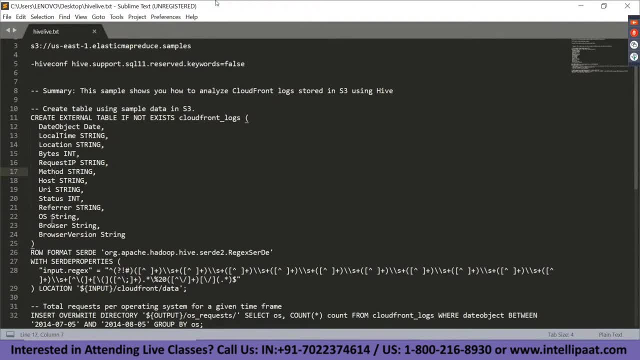 host, os and browser. so what we're going to do is we are just going to get the count of the os inputs. so, coming down, you can see total requests per operating system for a given time frame. so what result we are going to get is, for example, there is mac os, there is windows, there is. 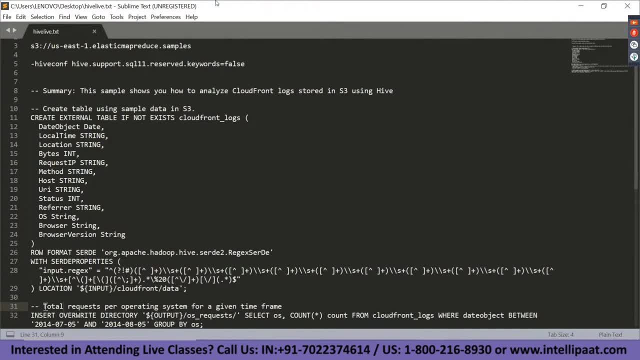 ubuntu, then there is android, so all of that operating systems. so let's say, in cloud front there is an application running: uh, so up to cloud front is basically cdn. okay, so there is. so let's forget about that, let's just concentrate on this. there is an. 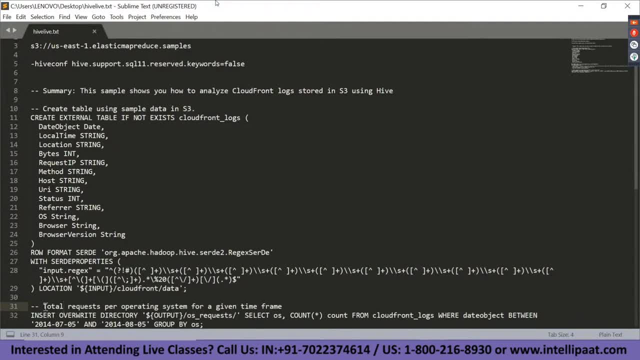 application running guys, so that application could be accessed from all kinds of operating systems: from a windows system, from a mac mac system, that is, an apple laptop, or from an iphone, from from a safari browser, uh, which is an ios, then there is uh, ubuntu, then there is android. so 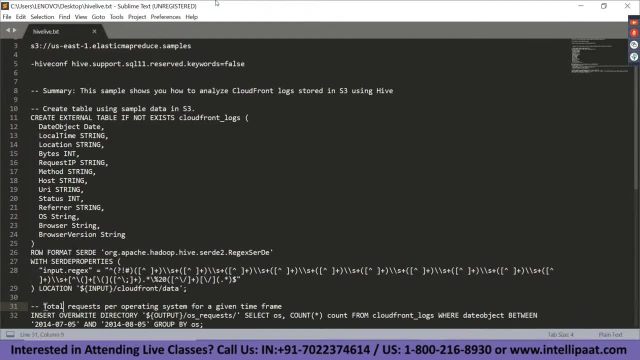 that application could be accessed from all these operating systems. so the output will be the operating system and the number of hits this particular application got from that operating system. so this data is already available. so it's not going to be dynamically changing. it is static data. okay, so i think i've explained to you this part. now let us start off with configuring. 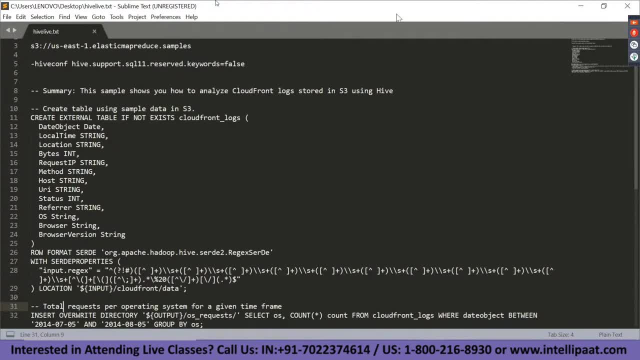 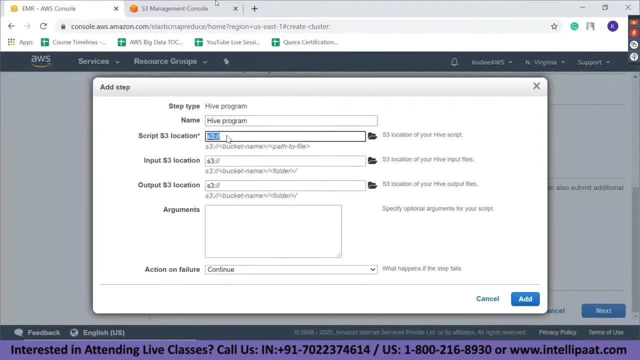 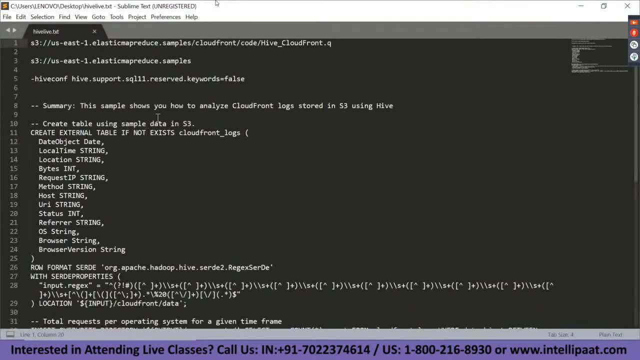 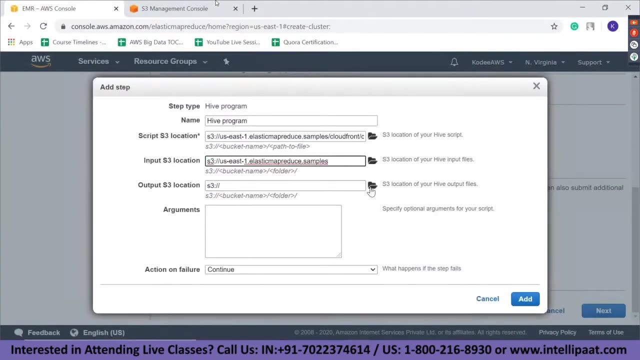 s3 location. so this is the s3 location, so i'm going to provide this done. next is the s3 input location, which is this. i'm going to provide this. next would be our output s3 location. so for this, we can search over here, and this is the bucket which should contain our output. 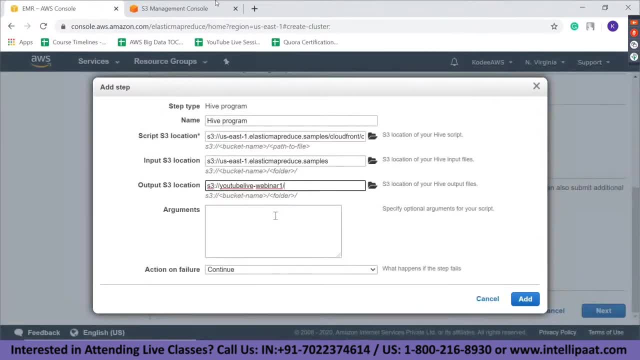 files. so i'm going to click it, select- okay. next is the argument. i'm going to copy this and paste it over here. so now this action on failure is: if this particular code or this particular process fails, it should continue and create this particular cluster, or you can cancel and wait. so basically, the cluster will be stopped. 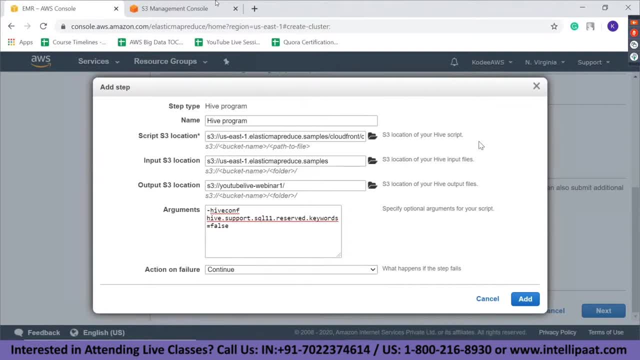 and then terminate cluster. if this particular little uh for this script we are running fails, then this cluster will be automatically terminated. if you give terminate cluster- but i'm not going to give that, i'm going to give continue- if this step fails, our cluster will still be active. 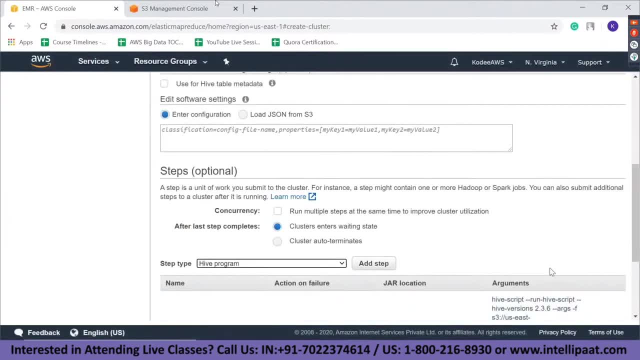 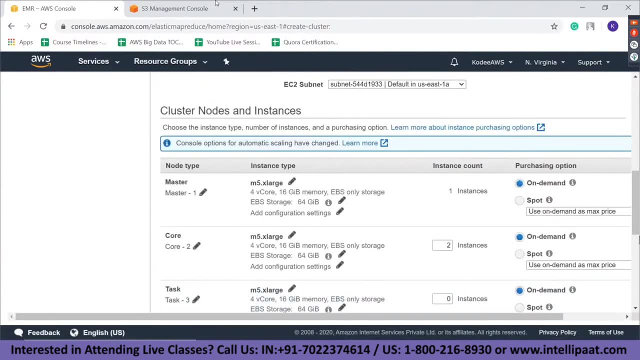 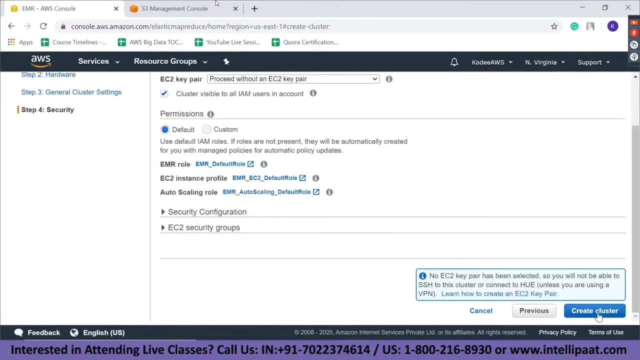 so that's what it means. so now i'm clicking on add and you can see we have set this up. that is the only extra step i'm just going to give next. next, i'm not going to change anything. yeah, so you can review it once so you can see it is proceed without an easy to keep it. 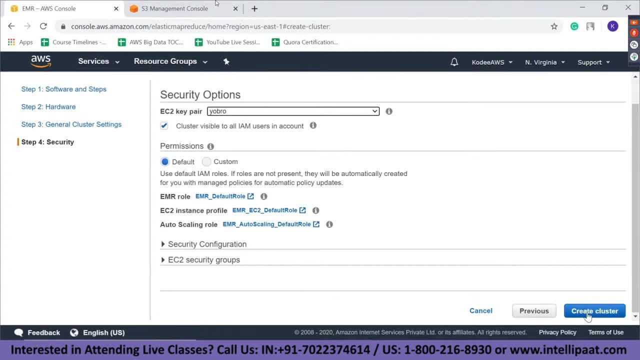 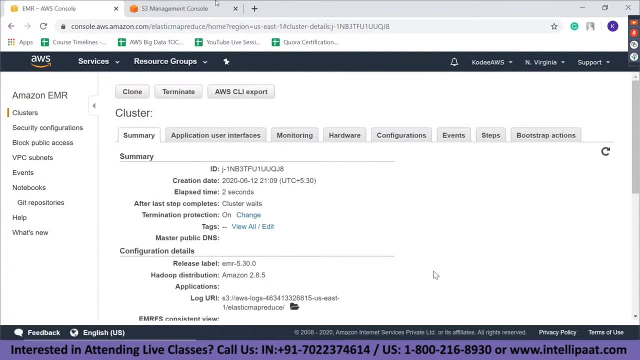 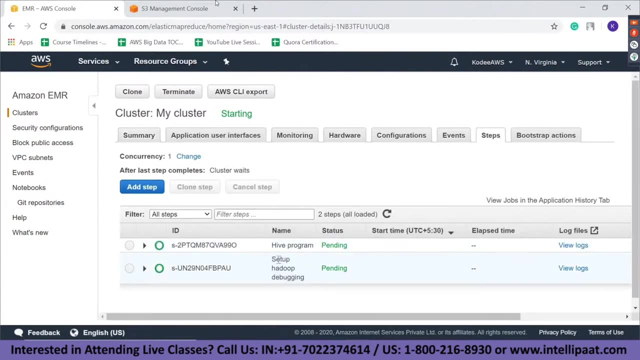 i'm going to give my key pair and create cluster. so, guys, it will take from 5 to 10 minutes to create this. so you can see the steps over here. you can see: first, this step will be completed. that is, the setup will be completed. then hadoop. 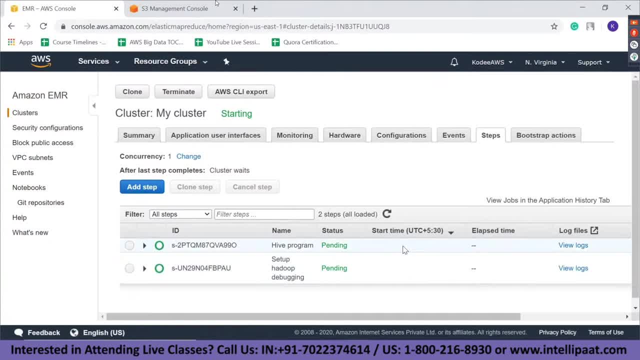 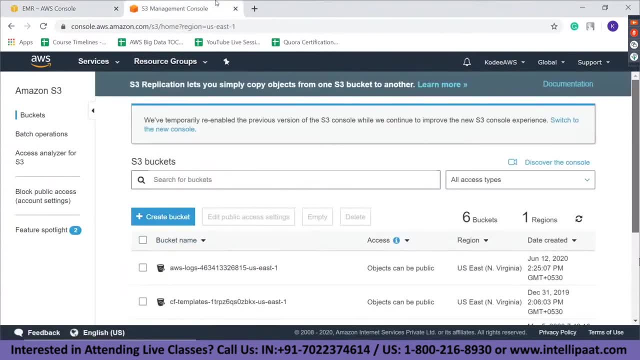 and debugging. everything will be completed. once that is done, the hive program will start running within the cluster. once that is done, we'll be able to see our output. so if i open this bucket right now, you'll not be able to see. let me just refresh. yeah, so i'm inside. 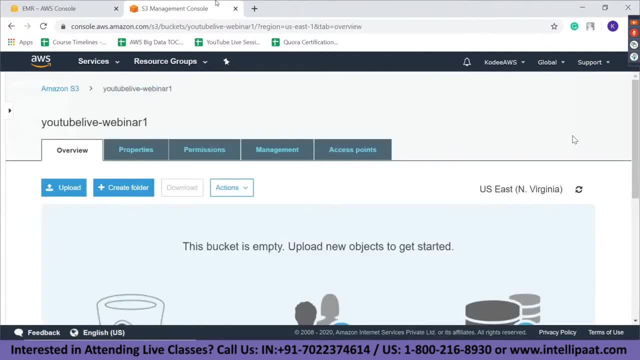 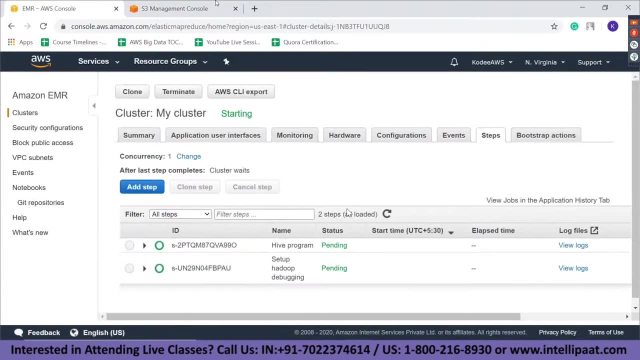 the bucket. so right now there are no files inside this bucket. once this is done, we'll be able to see that. so, as i told you, it will take some time. so let me go to let me click on clusters here you can see i already had a cluster which i terminated. so you can see it is my cluster, because once i 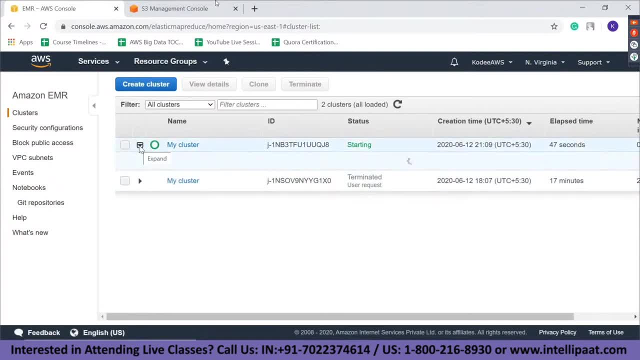 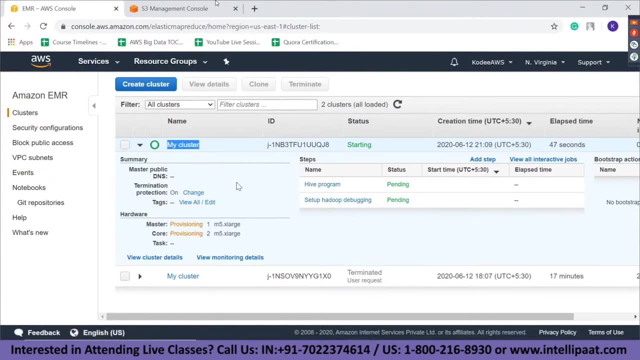 went into adjustment. here you can see that i already found my finely defined cluster. here you can see i already have my finely defined cluster. here you can see that i already have my advanced options. I did not change the clusters name, So it was my cluster only. So it's the same. 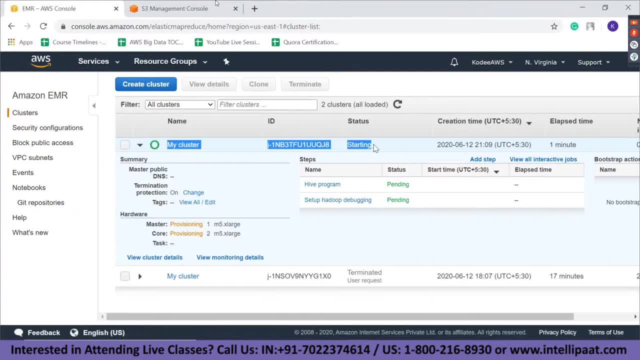 it is right now starting, and once we see complete over here, then this process will start. and once this is complete, this process will start and only then we'll be able to see the output. So then we'll download the file and see the output. guys, So I think that's clear right now. So the thing. 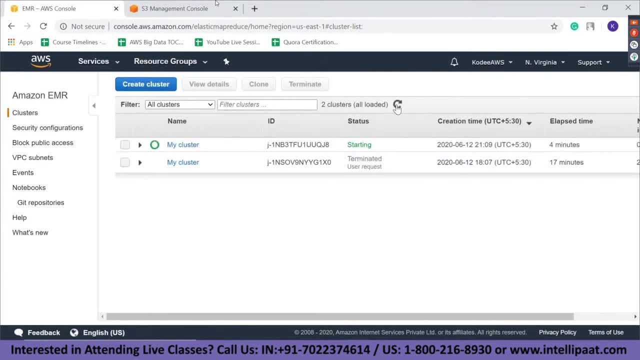 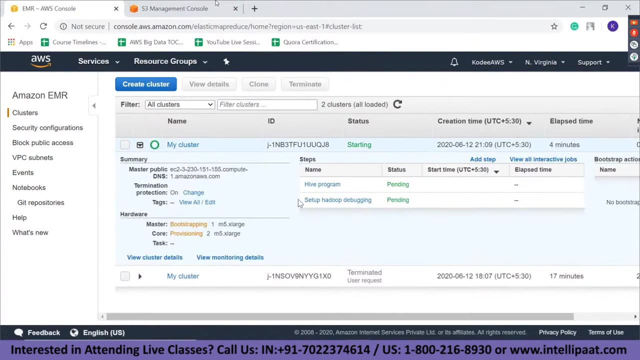 is will not be. we're not going to wait here and just sit idly. Yeah, it's still working ahead. So this process is still starting. So, as I told you, it will take from five to 10 minutes to this getting completed. The thing is, we added a step before we launched. you can also add a step once. 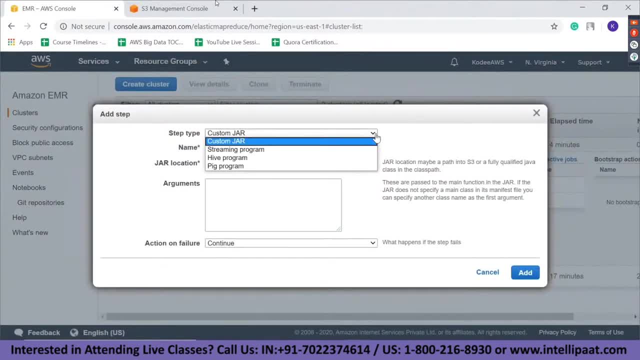 it is set up So you can see here you can also add this. Sorry, you can also add a step. Once you've created your cluster, you can choose a pig program, a hive, a streaming program or a custom jar program. So if 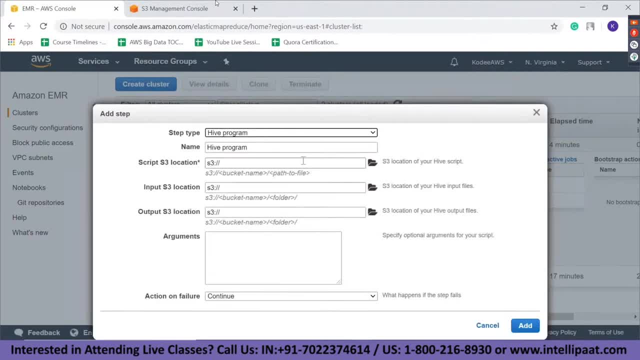 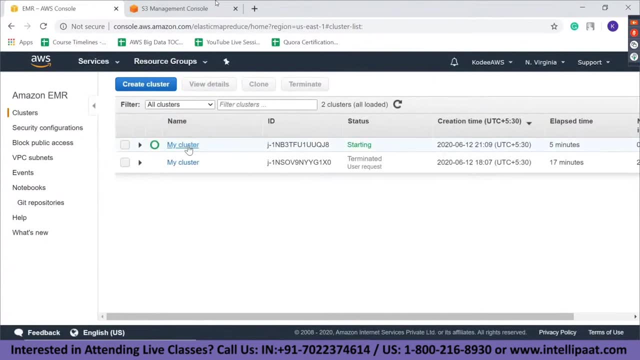 I want to add another high program. it's again the same setup And you can do that. Okay, so you've seen this. it's still starting, So there is nothing else to do over here. The only thing we'll have to see is our demo completing, Okay, so while doing this, I'll also explain the other 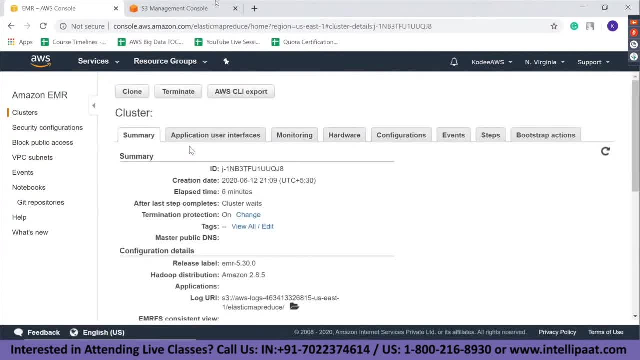 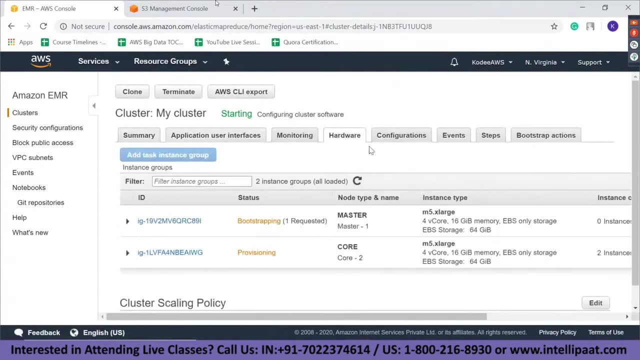 things about this cluster, Because there's no need to waste your time as well, Because it's everybody's precious time over here. Okay, so, coming to hardware, you can see this because we wanted to launch three instances. One is sorry when, as a master instance, two core instances, you can see the two. 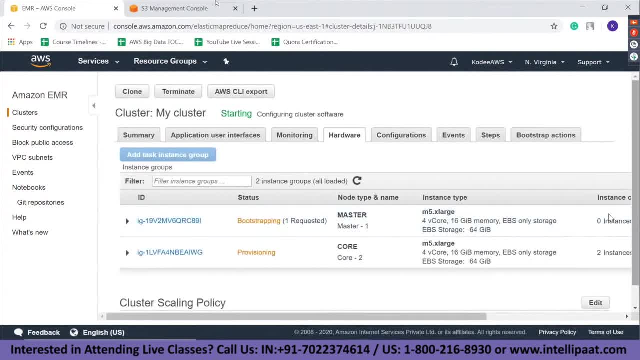 core instances are created. the master instance is currently under creation And so right now we have not enabled any scale. and since all of these data sources have been saved and when we launch the cluster, we can see that instance is lovely as well. 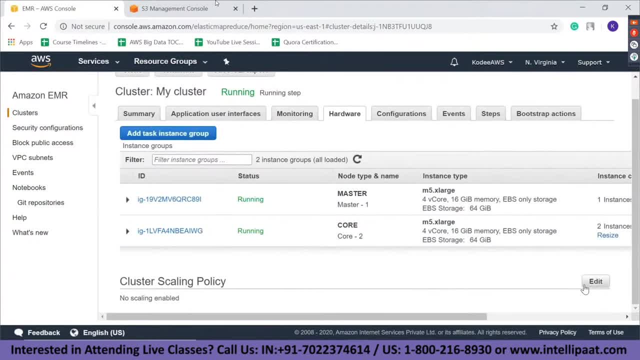 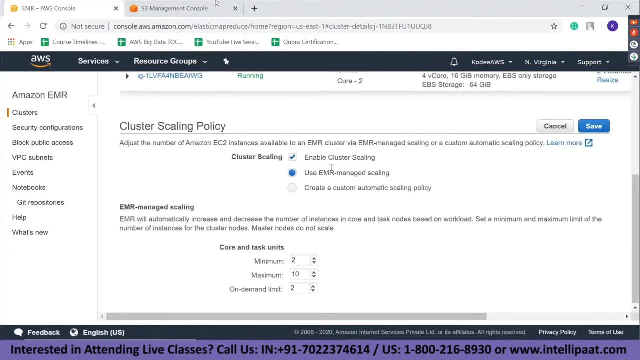 policy. let me explain to you about the scaling policy. so it is basically for auto scaling. click on edit, come down so you can see: enable cluster scaling. use emr, named scaling. so come come over here. emr will automatically increase and decrease the number of instances in core and task. 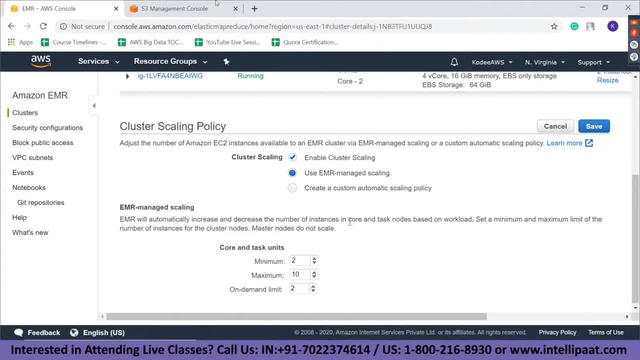 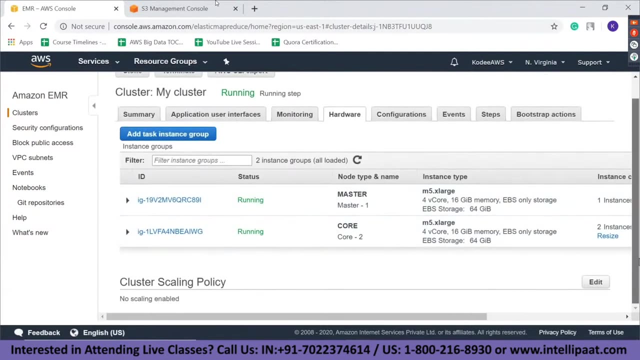 nodes based on workload. so if the workload increases, it will automatically increase the number of instances. the workload decreases, it will automatically decrease the number of instances. okay, let me close. this i'm seeing running over here. yeah, so the instances are running, guys, so you can check out the steps over here as well. you can see the instances are running. 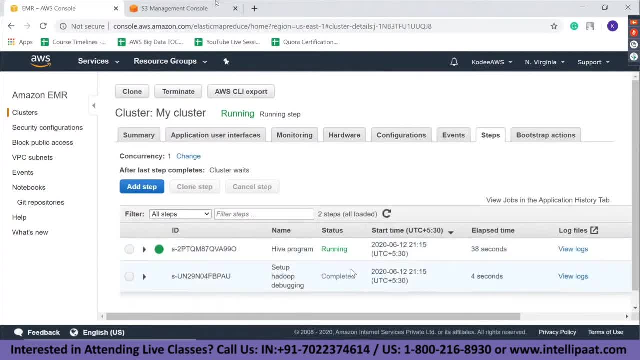 but the steps are still pending. so now this step has completed. so once the instance is run, it got set up in four seconds. if you want to check out this logs, just click over here. and so right now there are no logs. so once the log is created, you can just refresh and see over here. 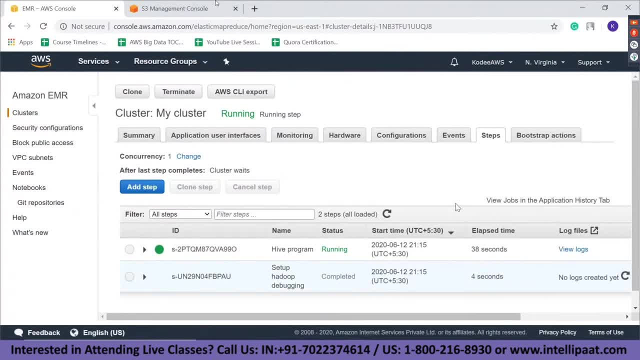 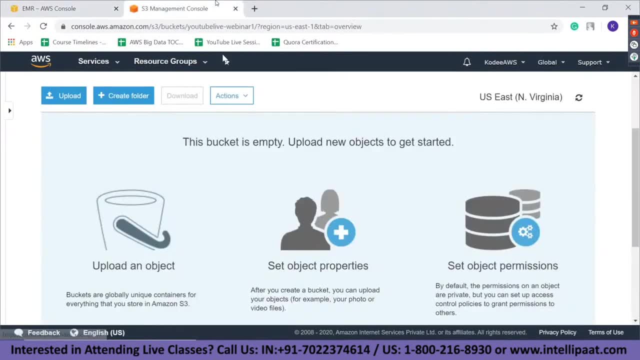 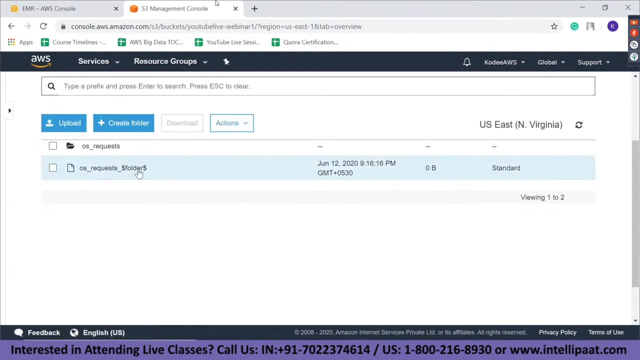 and that logs will be available in s3 and you can go check out those logs. but this step is still running and now it is completed, guys, so let's go over here, refresh this and hope that we get an output. and we got an output. so let me open this folder and let me download this. 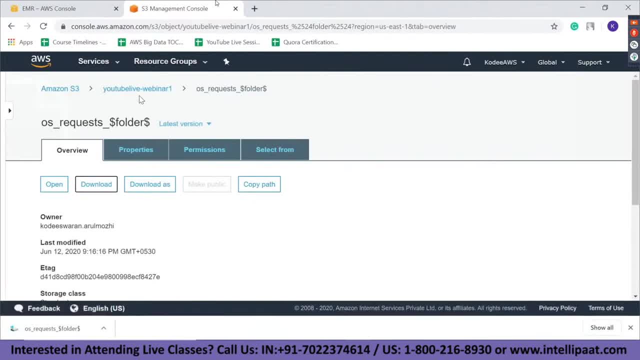 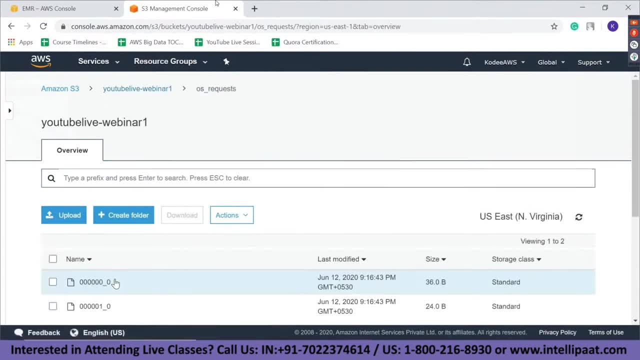 okay, sorry, that's not the, for that's not the folder which we want to download. we can download that or we can go inside and download this. so the thing is we have two nodes. that. so why do we have two nodes? is that we'll be splitting work and giving it to each instance, that is, the half, or 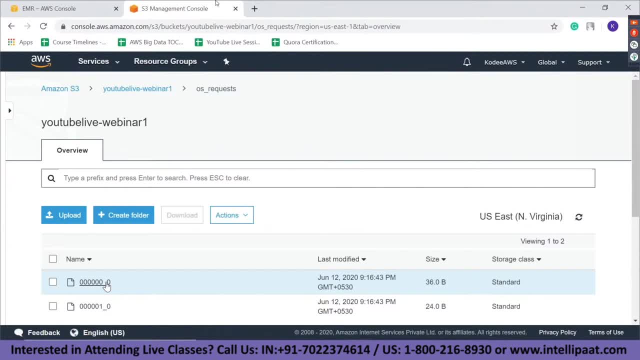 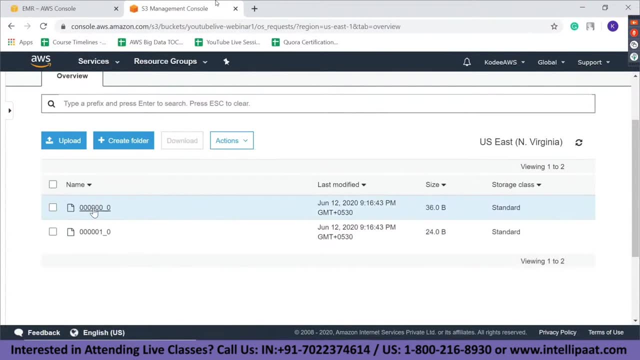 some of the work will be given to the first instance and some of the work will be given to the second instance. so you see two files over here, so we're going to give it to the second instance. so this file would have been, uh, processed in the first instance. this file would have been processed. 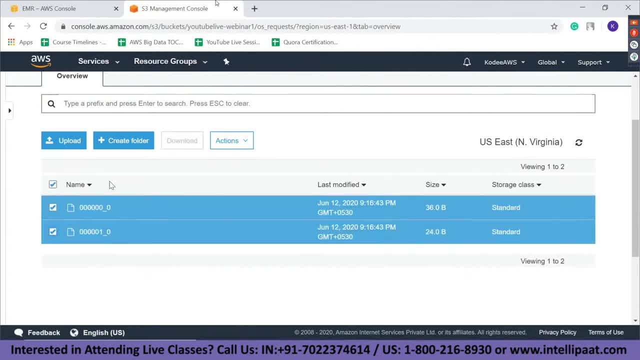 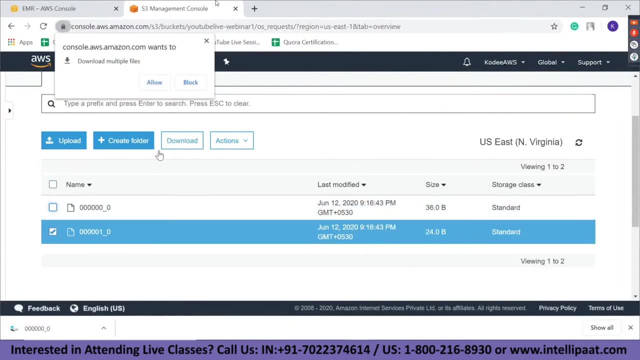 in this second instance. so now let's download. sorry, i think it's not possible. let me click, download the first one. click and download. sorry, i downloaded it multiple times. okay, so we've downloaded it. i'll go to the folder. so, as i told you, the output would be. 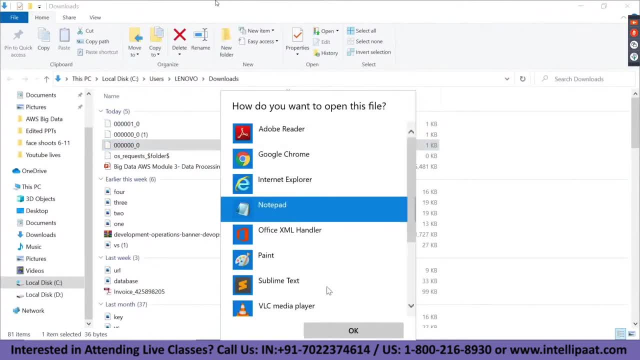 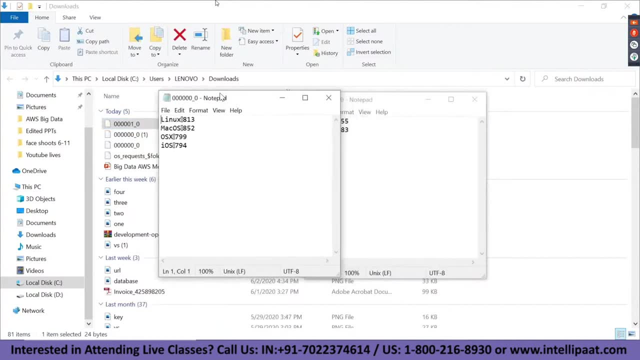 uh, the os name and the number of hits, and you can see this. let me open this as well. okay, i think you're able to see right now. you can see: android: 855 hits. windows: 883 hits. linux: 813. mac 852, osx, which is for the apple laptops, uh, macbooks, so it's 799 and in ios, it's. 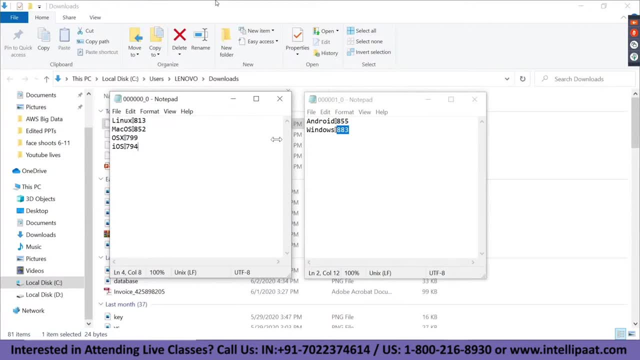 794. so we've got the files, guys. so let's go ahead and open this up. so let's go ahead and open this up over here. so this is this- actually means that our program ran successfully. we created a hive- sorry, we created an emr cluster successfully. we ran a hive program on it and we also got an output. 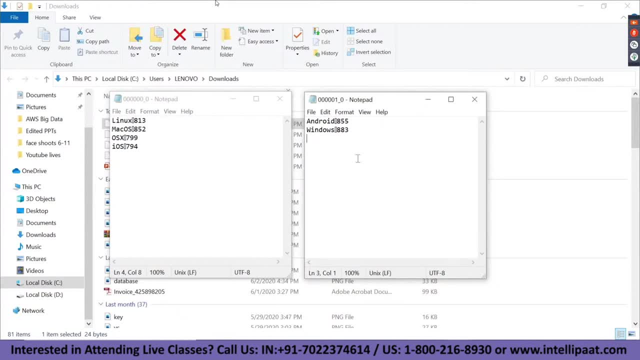 the thing is this file is very small. that's why we got an output in less than a minute. but if your file is very, very large and it takes a lot of time to process, then obviously it will take around 10 to 15 minutes, according to the size of your file, and sometimes it can also take a horse. 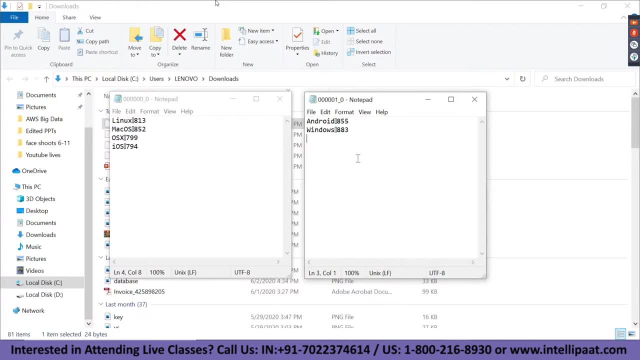 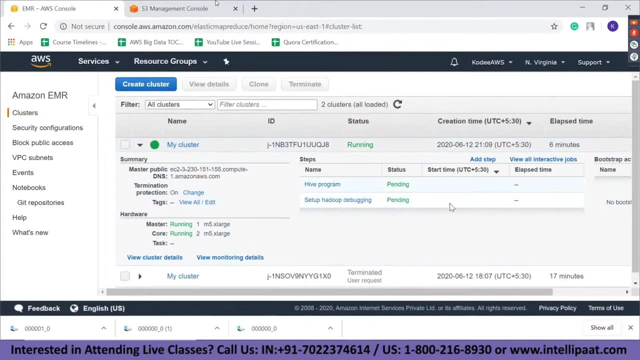 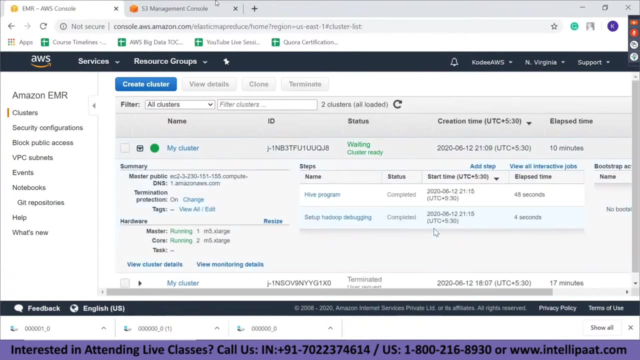 because you might have, uh, let's say, petabytes of data. okay, so, going back over here, we have successfully created the cluster. we ran a hive program and both of the steps have succeeded. you can just click here. yeah, so both of the steps have been come, succeeded, so it is waiting because right now there is no process running. 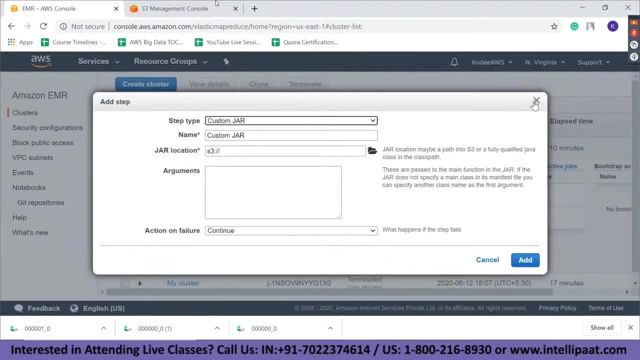 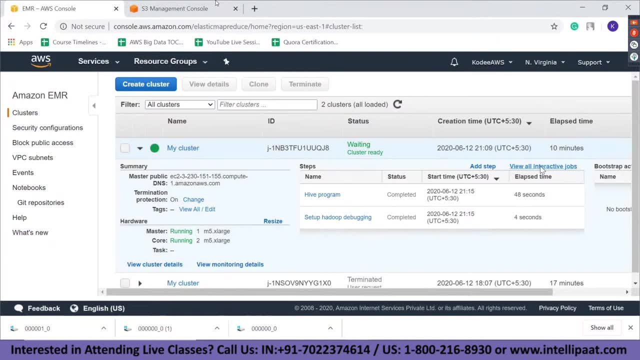 if you want to add a process, you can click on step and add another program to run your program and process data. so you can do that. you can see all the interactive jobs over here. if there is any current job running, you can see the job. so, for example, we were running this hive. 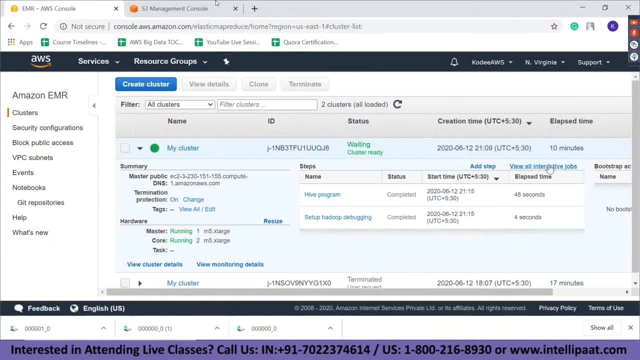 program. so while running we could have seen that job over here. so the thing is, this cluster can be shared among other users in my aws account so that all of them can run a job at the same time and we can check all the jobs running over here. 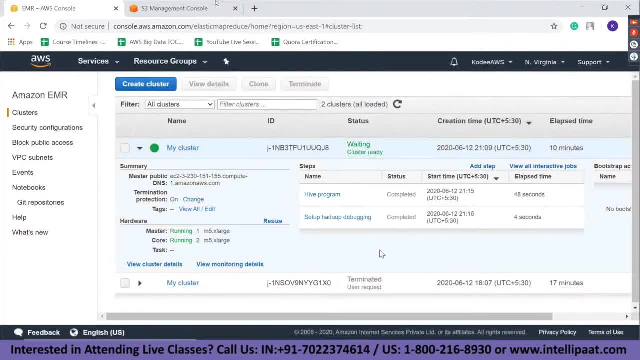 so i think that's pretty much it. so it's pretty simple to start off with this. it's pretty simple to create a cluster, run your own program with your own input data set. the thing is, while running the hive program, we gave an input data link. so instead of providing that link, you could, you could provide. 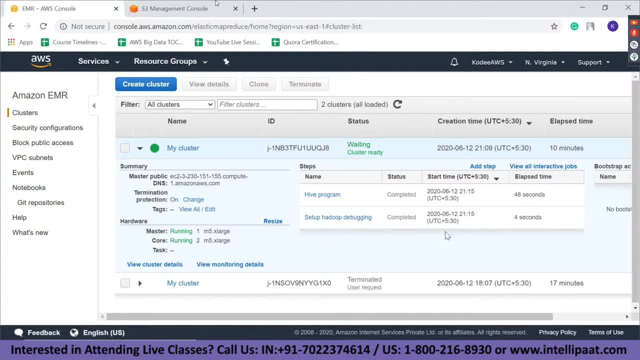 your own data set and you could provide your own hive script and you could provide your own output location. so output location is pretty simple. you can just give any location which you want, but the input script and the input data location should be provided and that's it. it will automatically. 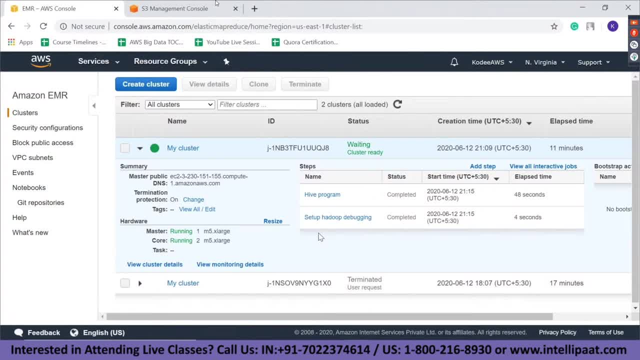 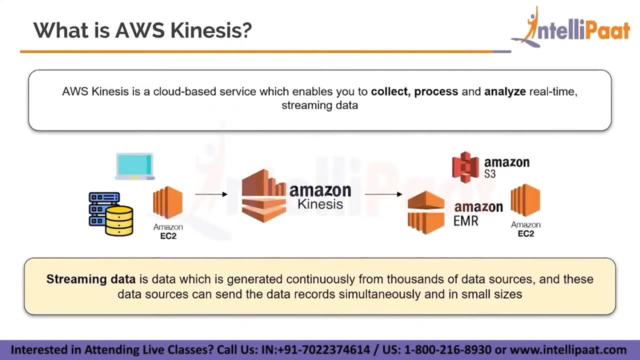 run the script and get your data processed. you can download the upload and take the data and do whatever you want with it. so what is aws kinesis? it's basically a cloud-based service and it is used to collect, process and analyze data in real time, so this data is termed as streaming data. 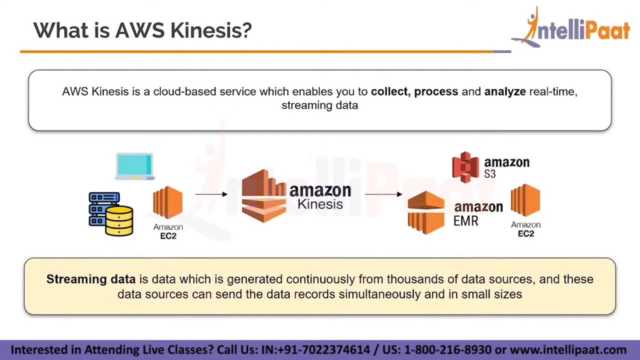 because it is being streamed in real time. so in the diagram, as we can see, the data source could be some relational database or a computer or an ec2 instance. it is sending the data as a producer to the amazon kinesis stream and then the amazon kinesis stream is then outputting that data to either s3 or emr or ec2. 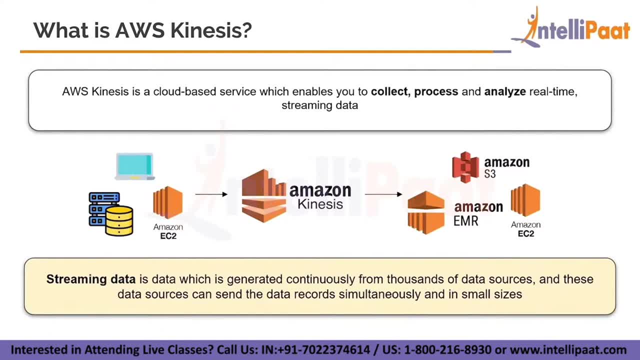 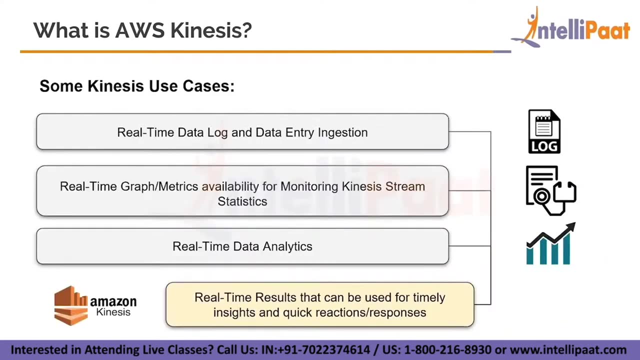 or various other instances as well. so to define streaming data, it's basically generated as a continuous data source, so it's being streamed continuously and it could be a culmination from thousands of data sources and these data sources could be sending these records simultaneously as one another. so there are many use cases for aws kinesis as well. we can analyze log data with this. 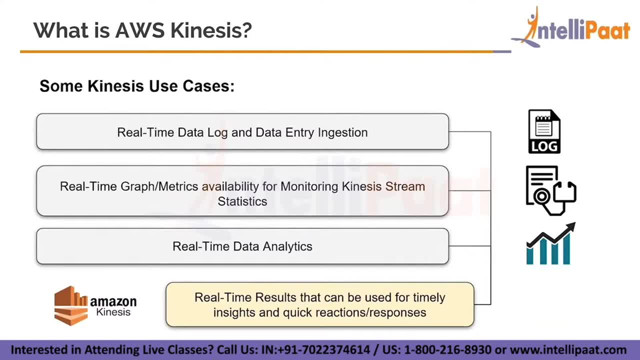 so a lot of web applications and applications in general generate a lot of log data in a continuous manner. if we want to process that data, analyze it and generate some insights out of that data, because because it essentially becomes a big data case in that regard, so we can use kinesis to basically 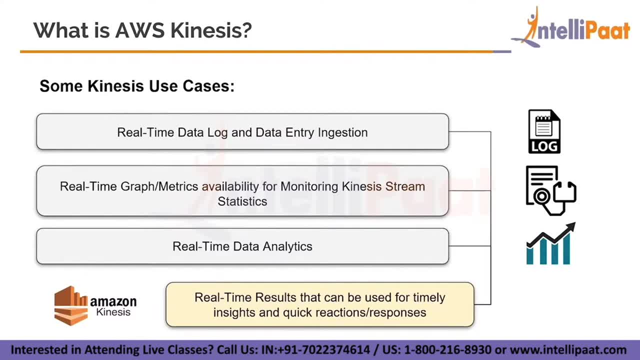 stream that data to our processing element, we can get the real-time graph and metrics for the kinesis stream. so while we are sending the data that we are sending, we can also analyze the statistics and the usage rate of that particular data that we are continuously sending to our 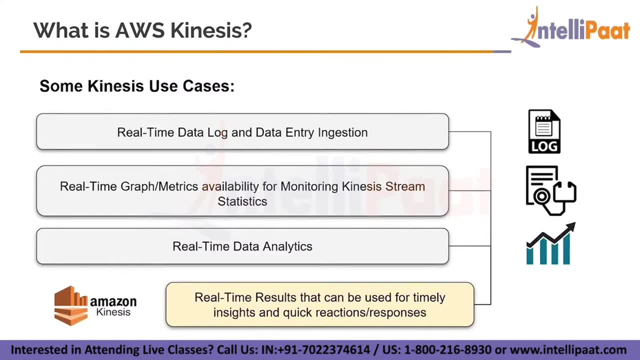 kinesis stream and we can also perform real-time data analytics. kinesis does not only act as a pipeline, it can also act as a processing element in itself. we can simply attach lambda functions to the kinesis stream and it can basically process and transform our data while in the stream itself. 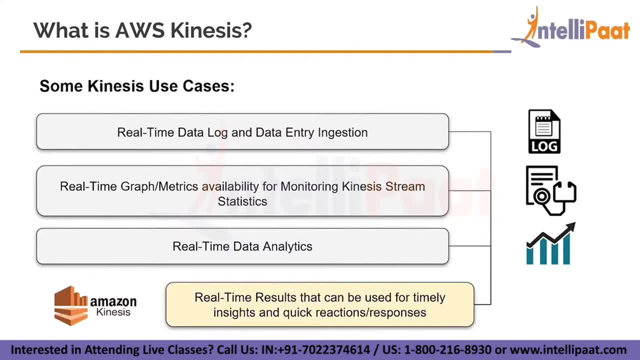 so, uh, it's basically used for timely insights and quick reactions and responses, because when data is taken from kinesis, the data is then automatically transferred to the kinesis stream, being generated at a rapid rate and continuously. we need a tool that can essentially process and 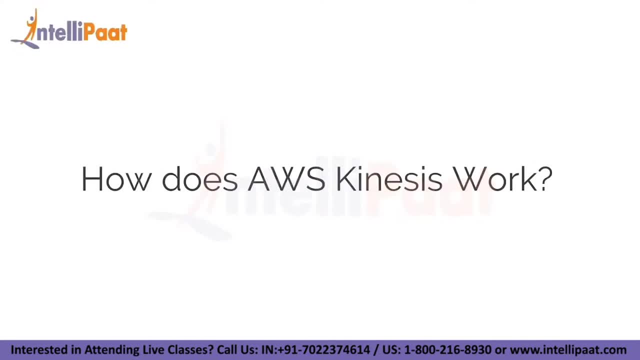 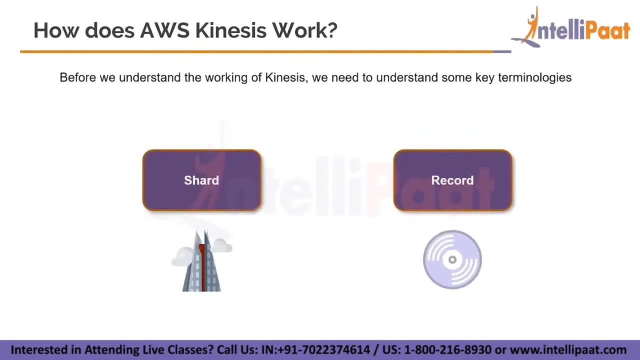 analyze that data in that manner only. So how does AWS Kinesis work? Before we actually understand the workflow, we need to understand some key terminology. So these key terminologies include a shard and a record. So to further define these, shard is the base throughput unit. 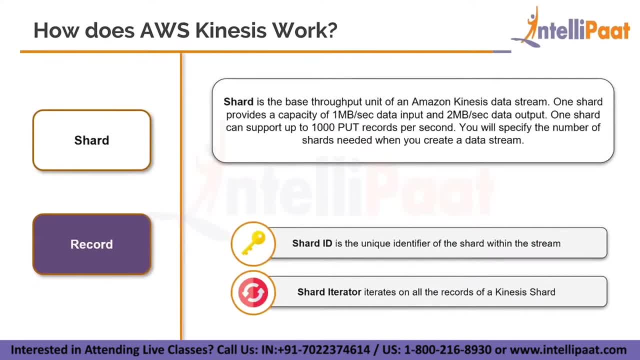 of a Kinesis data stream. So in input you get a maximum capacity of one megabytes per second and for output you get a maximum capacity of two megabytes per second. So one shard can support up to a thousand put records per second. So you can put a thousand records into the stream. 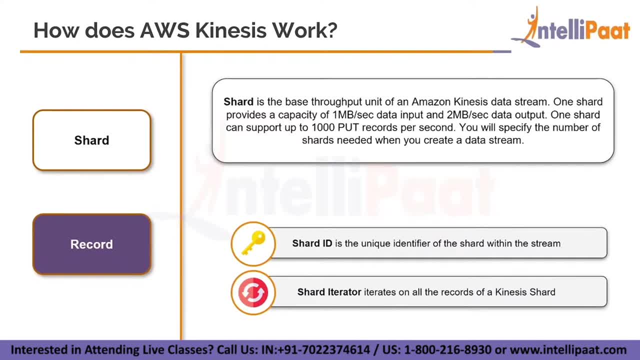 in a second in that particular shard and you can also increase or decrease the number of shards that you need when you are creating a data stream. Obviously, it would be priced on that criteria only, but you can specify the number of shards depending on the use case that 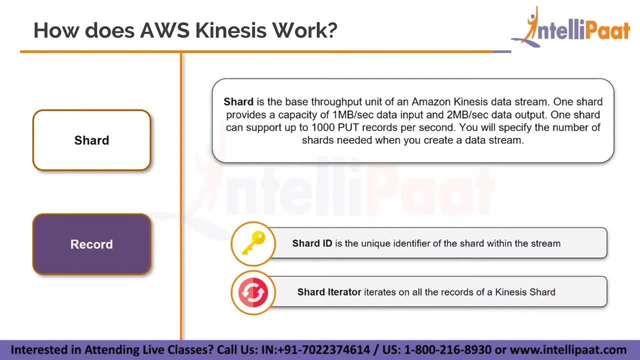 you have. So there are two elements to one particular shard. One is the unique identifier for that shard, which we call the shard ID, and the second is the shard iterator. So within the shard you have, at max, a thousand records at any given time. So you can basically have this. 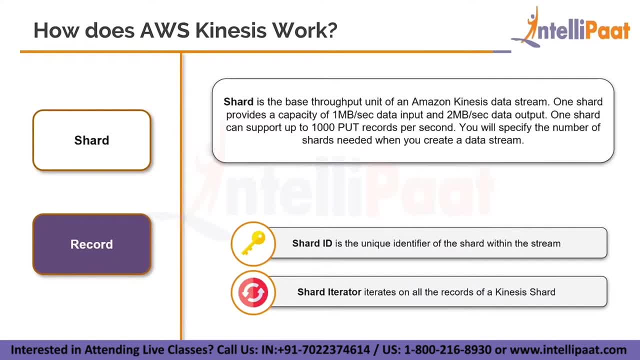 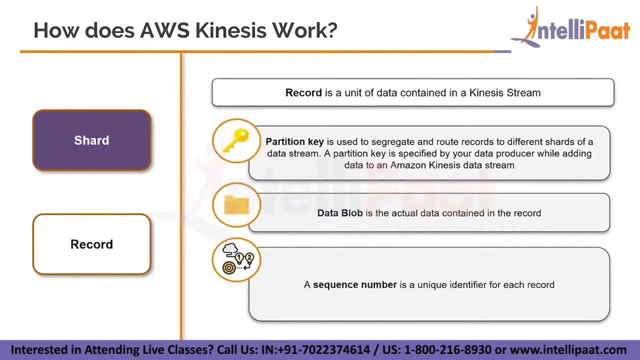 iterator value which can basically iterate throughout those records within that particular shard. So then you have a record, So it's basically a unit of data that is contained inside a Kinesis stream. So, as we were discussing before, within one shard you can put up to 1000. 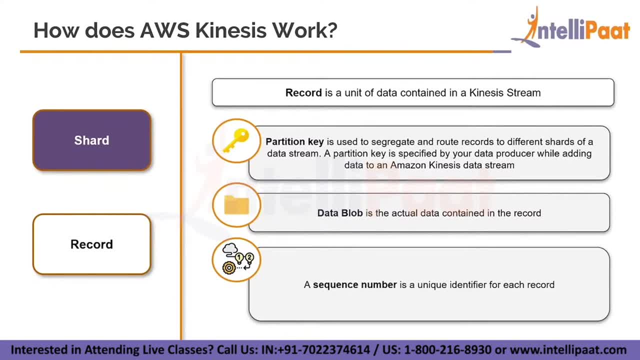 records per second. So that is what a record is. It's basically the data element that is contained within a shard, So it's not just pure data. Obviously, it needs to have some identifiers associated to it, So the first is the partition key. It is used to segregate and route records to. 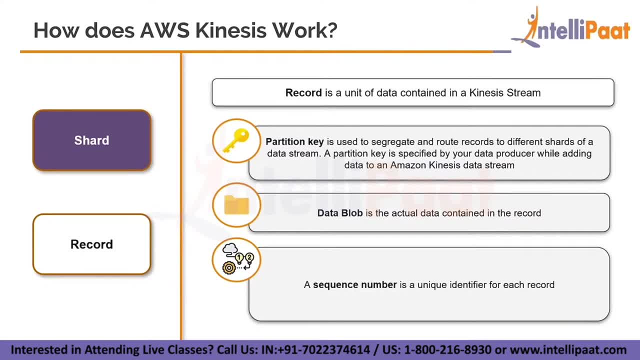 different shards of a data stream. So while you are sending your data to your particular Kinesis stream, you can use a particular partition key to basically direct that stream and direct that data that you have to a particular shard. So say, your Kinesis stream has three shards. 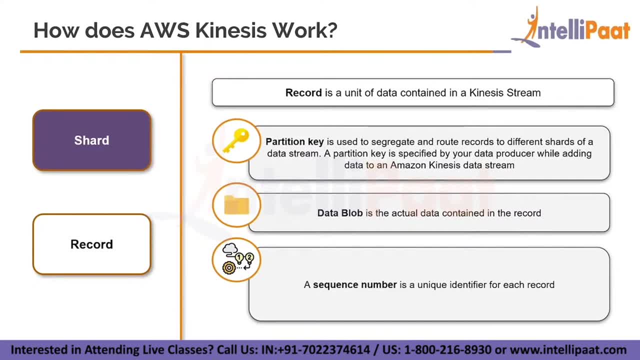 and you want to send your data to a particular shard Out of those three, you can specify the partition key based on the shard. So then you have the data blob. The data blob is the actual data that is contained, So it could be a string value. 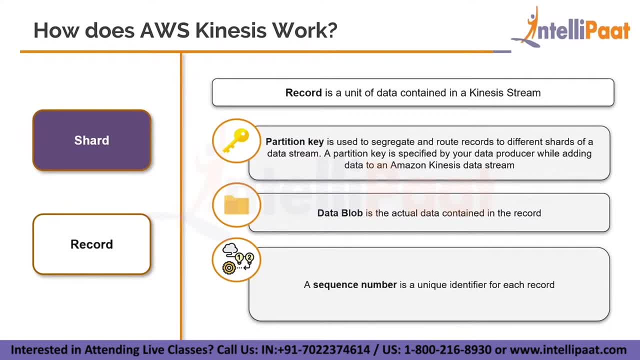 it could be some sort of a dictionary value, it could be anything. It's basically the data that you are trying to send to your Kinesis stream, And then there's a sequence number, So each record needs to be identified with a particular unique identifier. So that is. 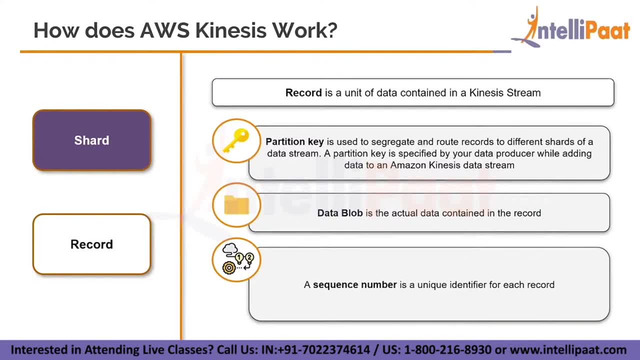 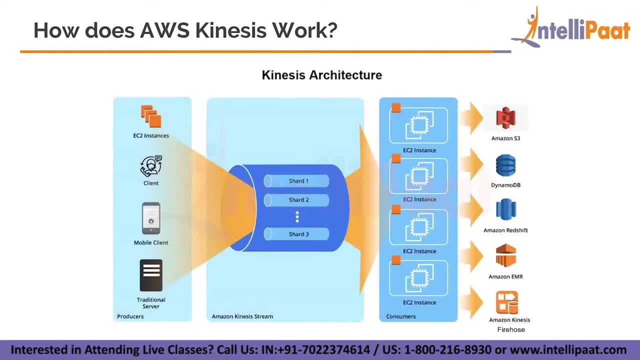 the sequence number. So this basically differentiates your record within a shard between other records present within that shard. So let us now get to the workflow. So this is the base Kinesis architecture. So, as we can see on the left hand side, 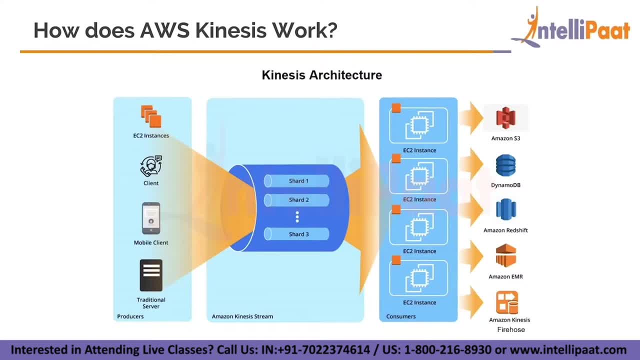 we have as our sources. we can have EC2 instances, we can have a client, we can have mobile clients and we can have our traditional server as well. So these are our producers, because these are the elements that are creating the data, And then we have our pipeline, this Kinesis stream. So this 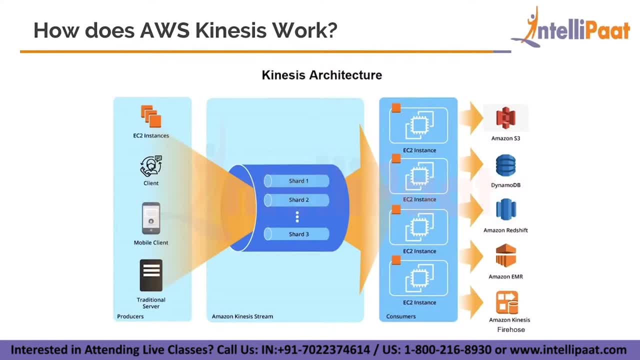 is one Kinesis stream which contains, in this case, only three shards, And it's basically transmitting data to consumers. So these consumers also are configured to take in this data that is being sent by the Kinesis stream, And these EC2 instances, optionally, can send this data furthermore. 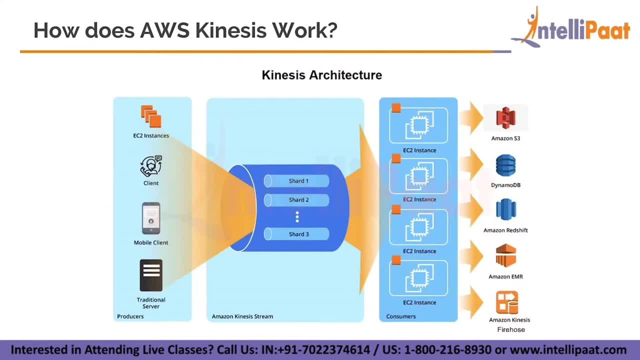 into Amazon S3 buckets. we can send them to DynamoDB, Redshift, EMR and Kinesis Firehose, for that matter, and so on and so forth. So let us now look at the workflow of how all of this works. So 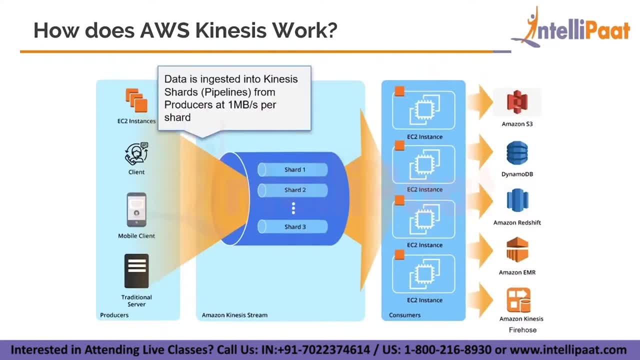 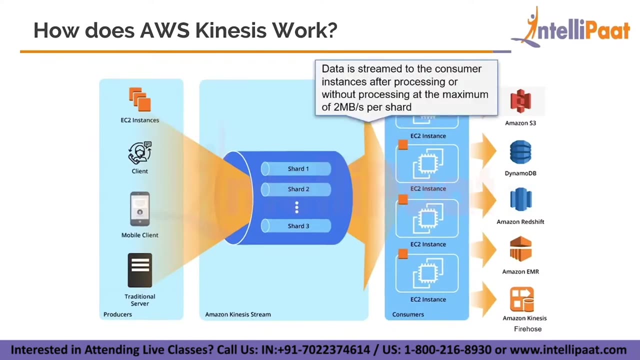 first thing that happens is the data is ingested into the Kinesis shards. So, as we discussed earlier, it could be ingested at a maximum of one megabyte per second per shard, And then, after it has been ingested, and put into the pipeline, then, depending on whether it was processed or not, 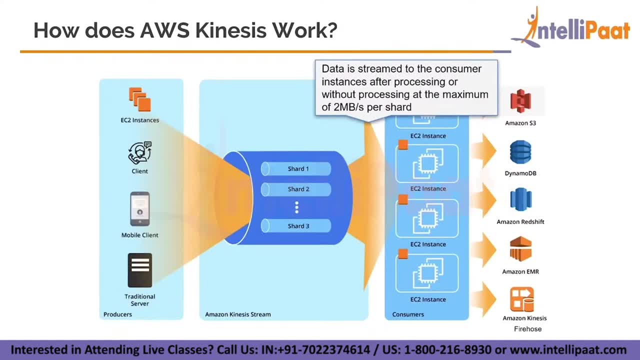 within that Kinesis stream. it is then streamed to the consumer, So the consumer could be EC2 instances or basically Amazon Firehose. for that matter, The capacity at which the data is outputted is at around two megabytes per shard, So per shard can. 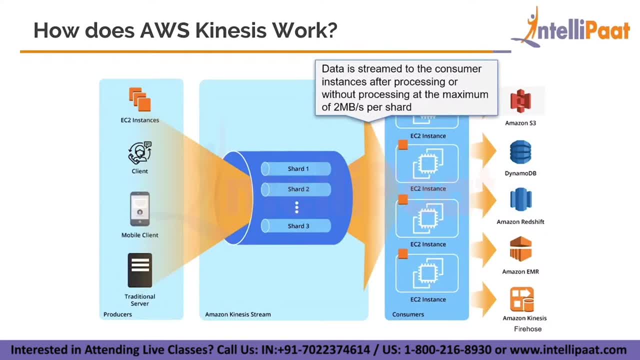 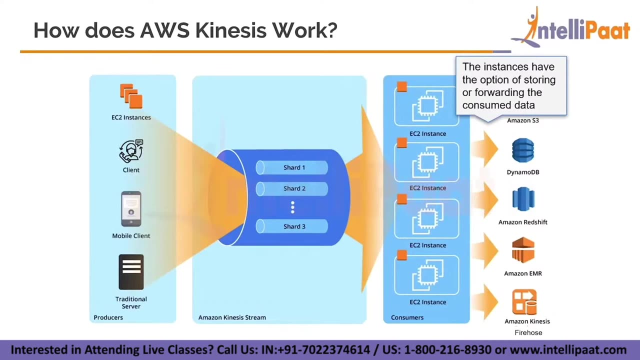 only output the data at a maximum of two megabytes per second, And after it has been put into the EC2 instances, after the traveling has been done, then the EC2 instances have the option of forwarding the consumed data to the further elements. So, coming to the hands-on section of how to actually 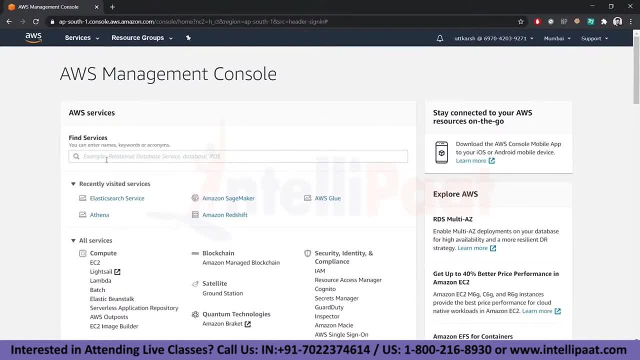 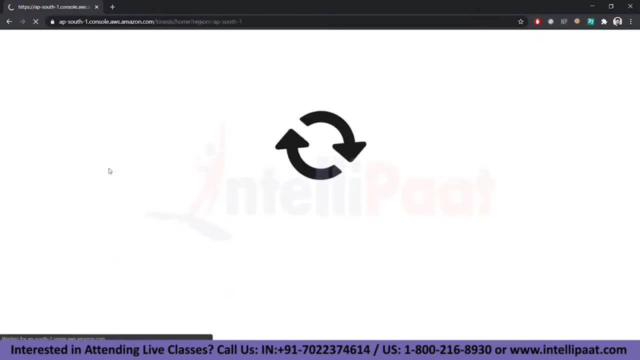 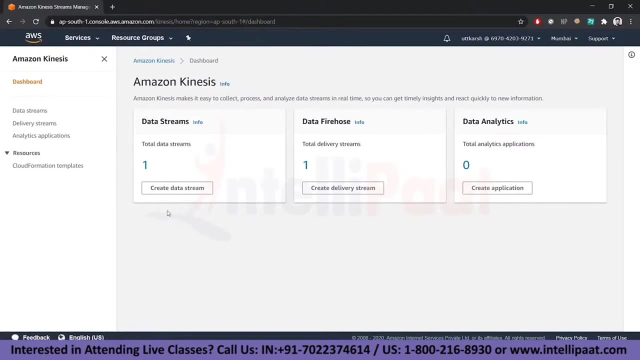 Kinesis stream. there are two ways to do it. The first way is obviously via the user interface that Amazon provides by itself, So you can simply type in Kinesis and you'll be greeted with a lot of options. So the first way you can actually create a data stream is by creating a data stream. 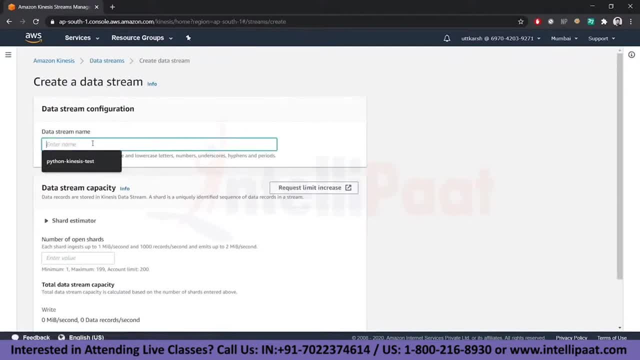 itself and then typing some name. So in my case, I can type name like Kinesis stream one. So this is my stream name, right? So this is my stream name, right? So this is my stream name, right? So the number of shards that I would want to use right now for our test case is only one. 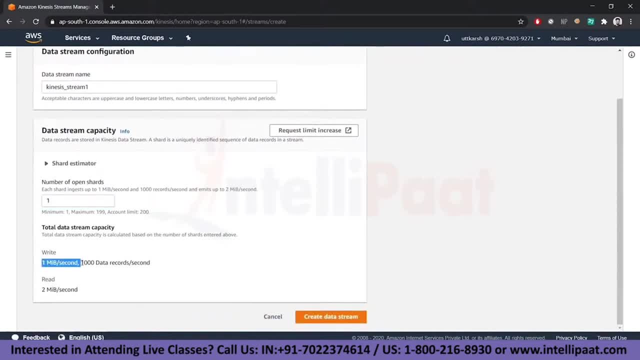 So, as you can see, it already gives you the statistics related to that one shard option that you just put in, which is the write of one megabytes per second and the read of two megabytes per second. You click on create and it will create your data stream. 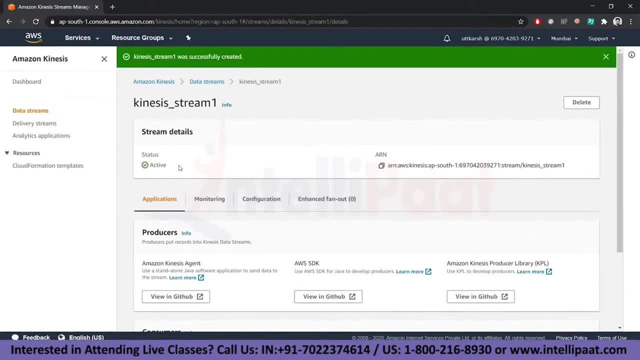 So, as you can see, the status is now creating. So now our stream has successfully been created. Now, depending on the name that you've put for your stream, you can now configure your producers and basically transfer your data to these streams. There's also other ways to actually implement. 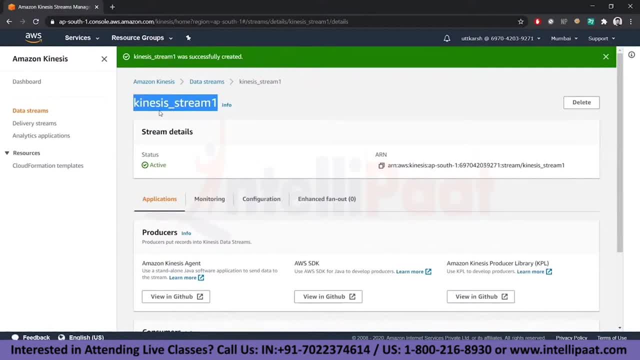 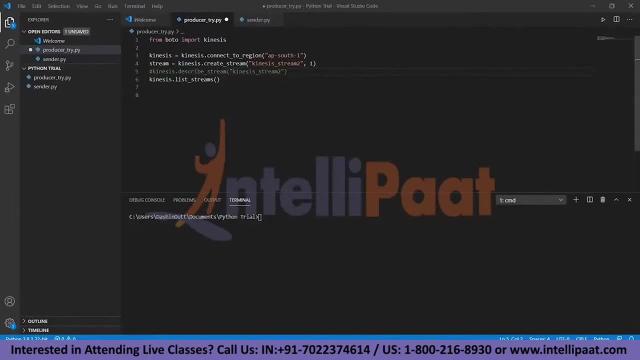 this. I'll show you that. So there's one other way you can actually create a stream. It's by using Python and the Borto library that comes with Python for AWS. So we'll show you that in just a second. So the other way you can create a stream is by simply writing the code for it. So in 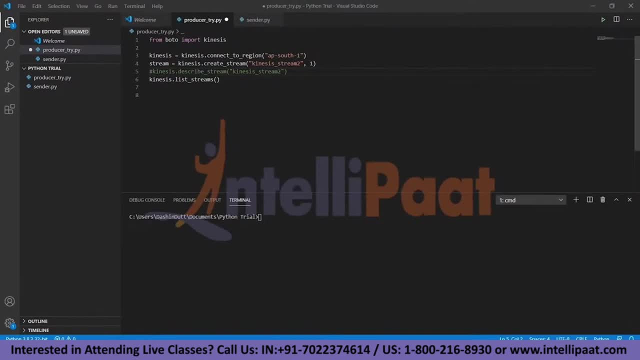 my case, I've used Borto from Python, So from the Borto library I've imported the Kinesis module. So this is what you will need to access the Kinesis elements of your AWS. So the credentials have already been set up. So it has been provided how to set up the credentials for your particular. 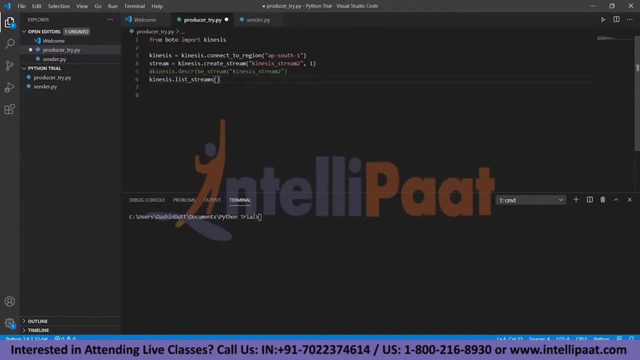 Amazon account, your IAM user role, So those things have already been set up, So we don't need to worry about that And we can simply go about creating our stream. You can install Borto by simply typing in pip, install Borto, And it will basically tell me that. 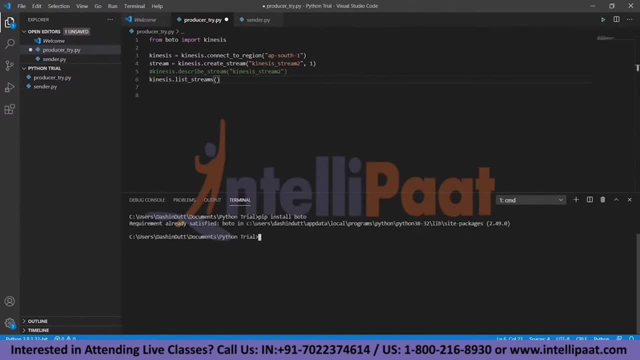 my requirement is already satisfied because I have already installed Borto. But if you're doing it for the first time, it will basically install for you for the first time. So the next thing that we will do is basically specify a reason. So we'll create a variable, we'll call it Kinesis and we'll 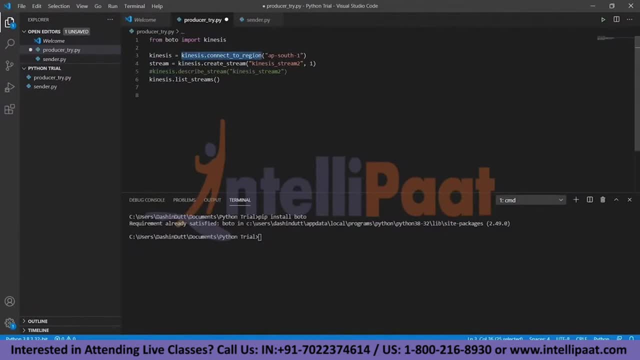 invoke the Kinesis connection To region clause and given the location of your particular Amazon region. So in my case it's Mumbai, So it's AP South one, right, And then we'll create our stream. So for stream, we'll create a variable and equate it to dot, create stream and given the stream name and given 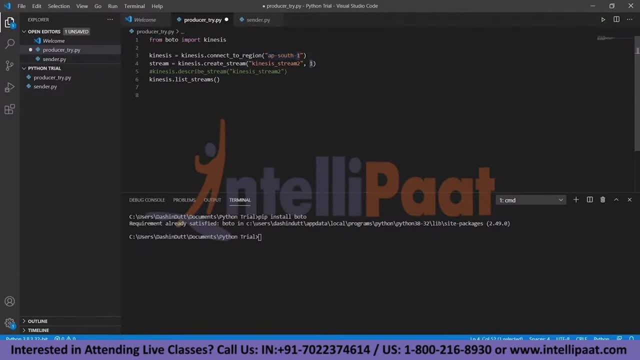 the number of shards for that stream. So I won't only give one shard for my stream, but you can give as many shards as you would like, depending on the use case that you have. For testing purposes. it is highly recommended that you only go. 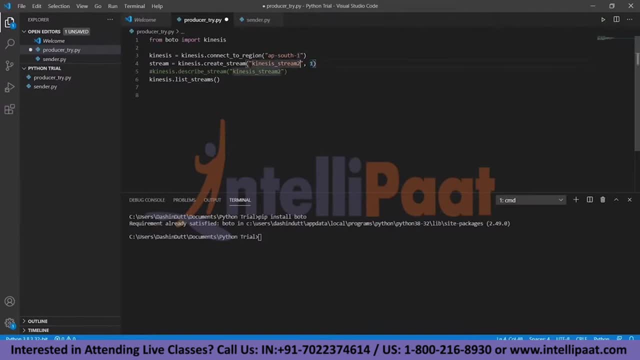 with one stream. Okay, so you can give this any name that you want. So in my case I'm giving it the name Kinesis stream two, since we've already used one with the UI creation of the stream, And then you can simply save the file and then you can run your Python file. So to run it with 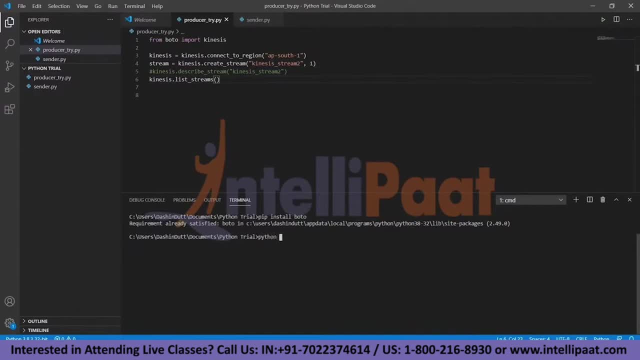 the present working directory. simply type in Python and then simply type in the file name that you've just created, which is producer underscore, try dot py. So when you type it and enter that, it will basically create your stream. The only caveat is you need to have your 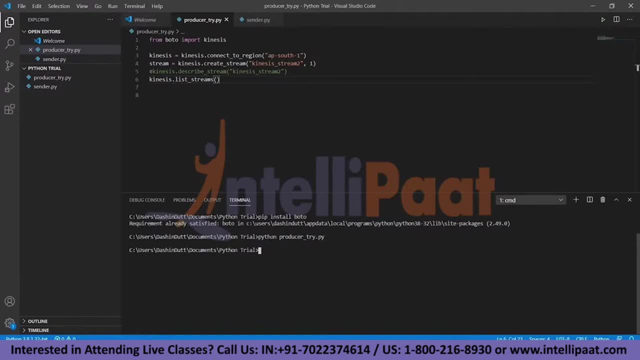 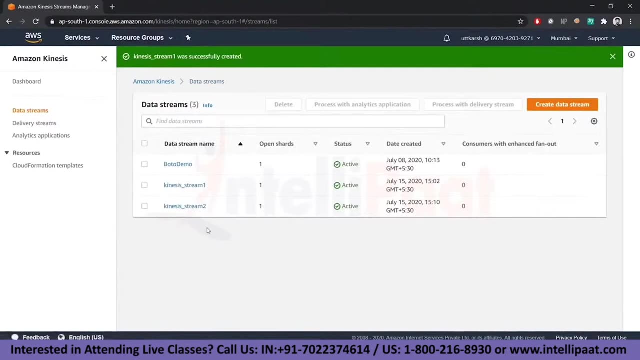 credentials already configured, which have been instructed to you. So if you simply go back to our Kinesis dashboard and go to our data streams, right. So, as we can see, there's another stream that is now active, which is Kinesis stream two. So this is the other stream that we just created. 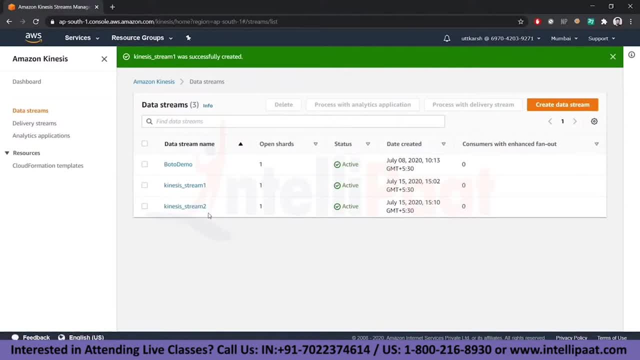 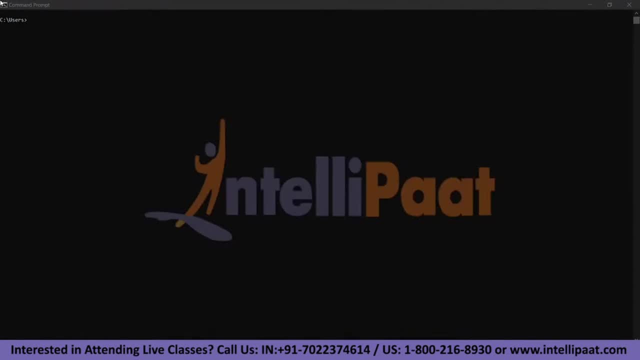 So that is how simple it is to actually create a stream: a Python Boto library And, lastly, if you want to create a stream using the AWS CLI, you can also do that. So once you have your credentials set up, you can simply type in: 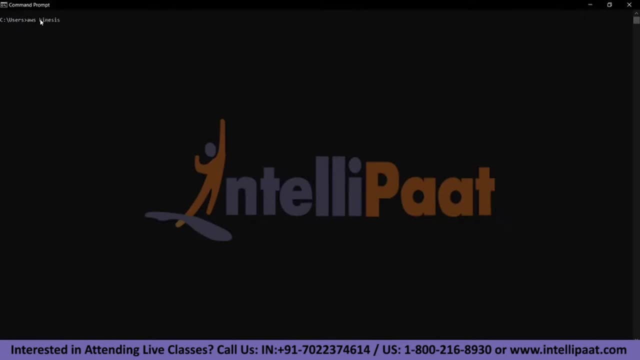 AWS Kinesis to invoke the Kinesis clause and then simply type in: create, hyphen stream- the stream name. So you need to specify the stream name So you can call this stream name. You can call this anything that you would like, So I'll call this Kinesis underscore stream three. 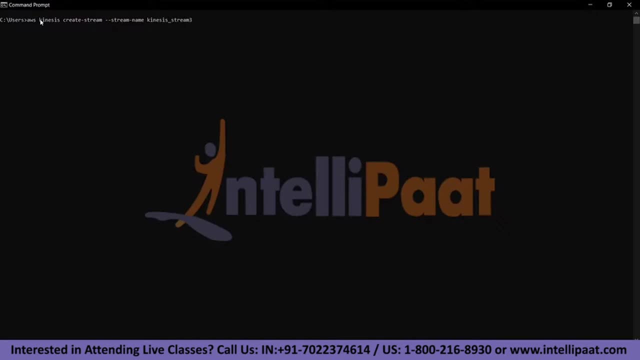 since we've already used two and one, and then you can give them the short count. So in my case I'm giving the short count of one and then you press enter. So that will basically create your stream number three. So if I simply refresh this, 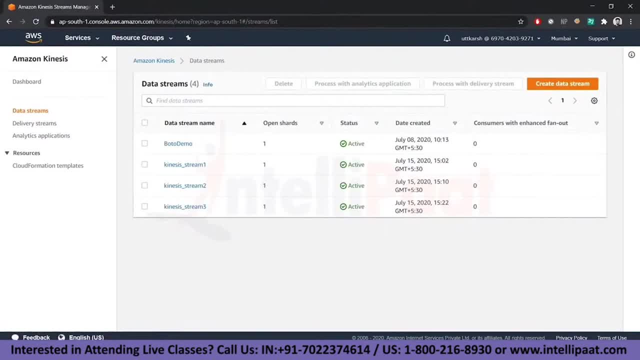 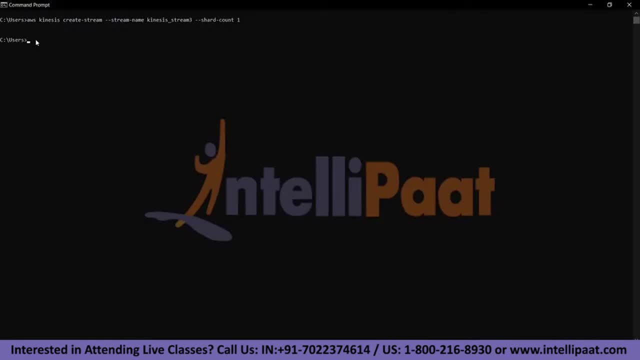 as we can see, we have a third stream which is now active. right, There are a lot of other things you can do with the AWS CLI So you can describe the stream. So describe the stream and type in AWS Kinesis and type in simply. 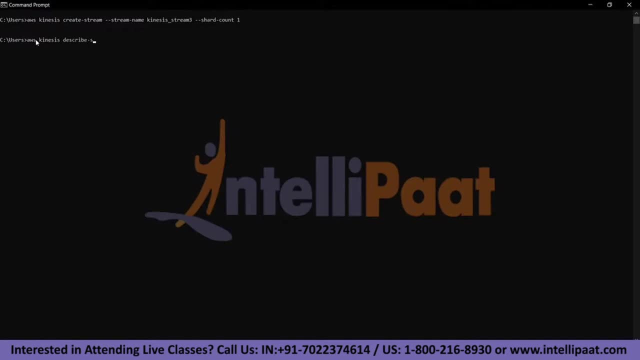 describe stream. So Kinesis underscore stream one. So this is a stream name that we want to describe, And then we press enter So it gives us the description of that stream, So it gives us the shards in basically a JSON format. So, as we can see, there's only one shard and we have a lot of 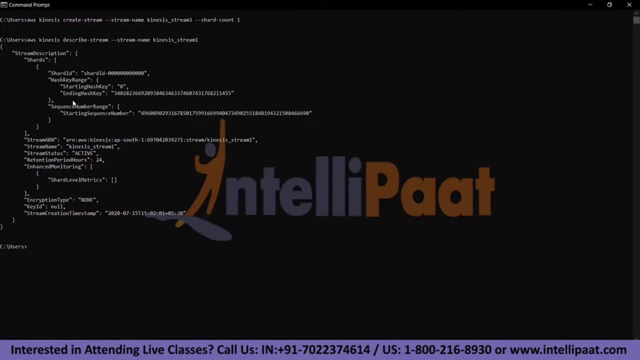 in stream one, So we only get the shard ID and all of the variables for only one shard and the stream name, the stream status that is currently there, the retention period for that stream- So it retains data for the maximum of 24 hours- and a lot of other elements as well. 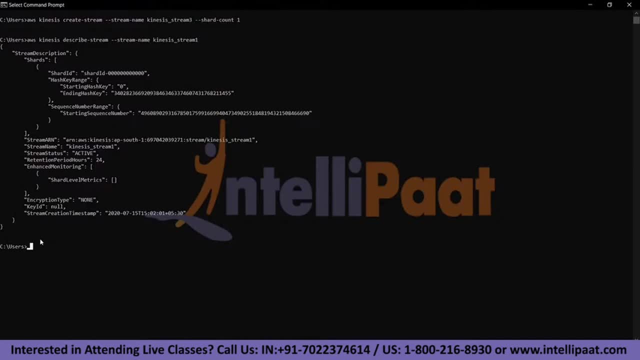 So the other thing that we could do is list all the streams that we've created. So to do that, we can simply type in AWS, Kinesis And list streams. So it basically gives you the stream list for your particular account, your IAM user. As you can see, we have four streams, So the first one was the default. 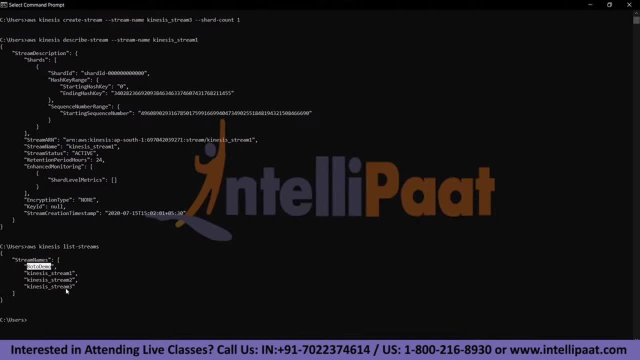 one that I had created earlier on Voto demo and the three streams that we just created. Say, now that you want to put some data into your stream, you can simply type in AWS, Kinesis, Put record. because you now want to put a record into your stream. 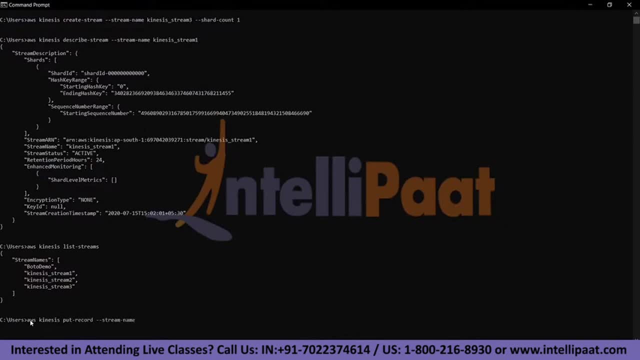 Your stream name that you want to put your record into. Let us take stream number three to put our record into. So Kinesis, underscore, stream three, The partition key. So this could be anything that you would like. So in my case I would be simply typing in 123.. You could type in anything that. 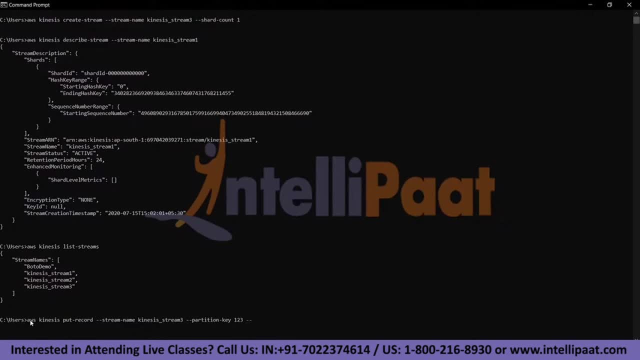 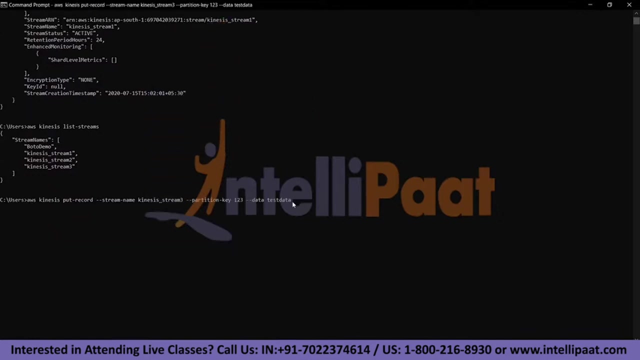 you would like here and then you would finally give the data. So let us give in some test data So when you press enter, it will basically create your stream. add your data within the stream. So, as we see, as we can see, our data has been added into the stream And we can see which shard. 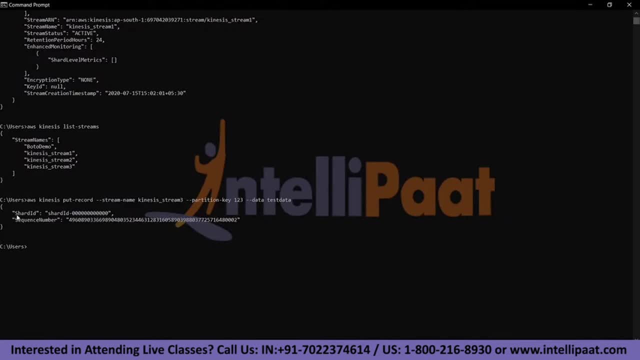 ID has taken that data, which shard has taken that data and the sequence number for our particular data record. So that is our sequence number. Next, we are going to add our data. So the next thing that we could do is get the shard iterator for that particular shard. 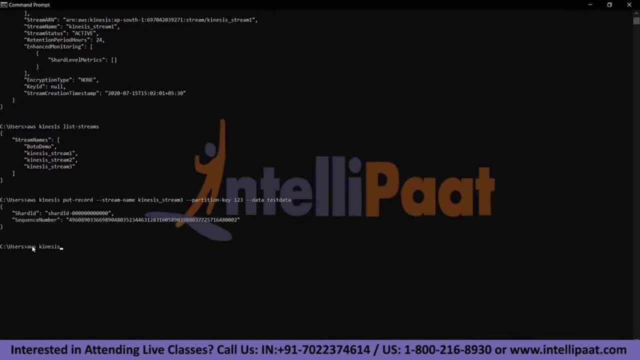 So for that we can simply type in AWS Kinesis, get shard iterator shard ID. So we can simply take in this the shard ID that we are concerned with right now is this particular shard ID. So take that and paste it over here And then we simply type in the shard iterator type. We trim anything that is. 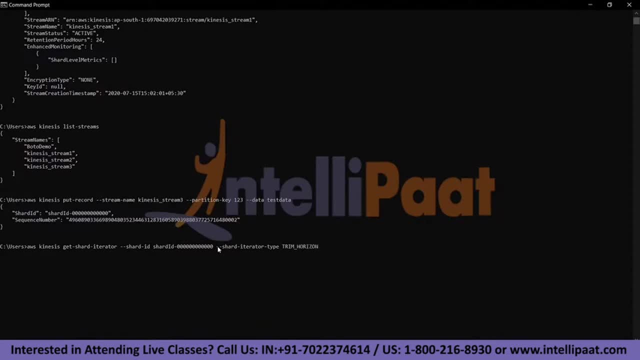 there, like spaces or remaining spaces, And then we give them the stream name, which is, in our case, Kinesis, stream three, And then we press enter. So then it gives us the shard iterator. So now we can use this iterator, this particular iterator, that we have to get all of the records. 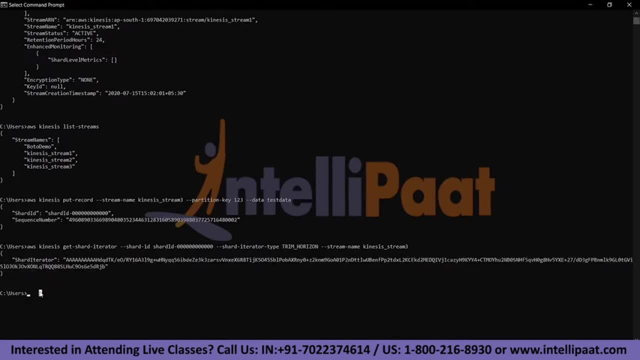 that are present in this particular shard right. So we can type in AWS Kinesis, get records, shard iterator. So, based on the shard iterator, we'll get records, And then the next thing that you could do is simply paste this particular iterator. So that's not the iterator we can. 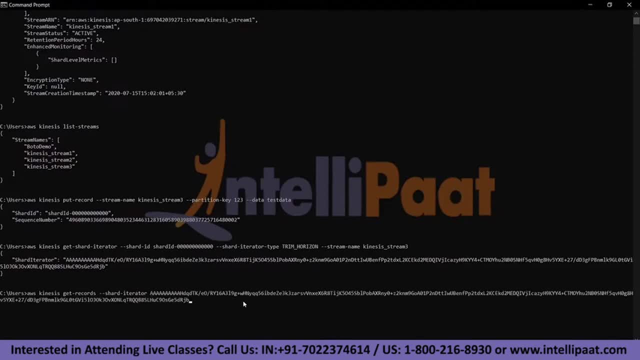 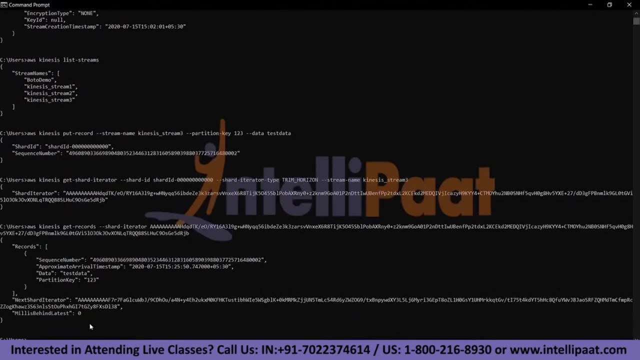 simply copy this and paste it over here So we get our iterator as well, And then we simply press enter, So it will basically give us all of the records that are present within that shard Once we have the shard iterator. And lastly, we can also delete streams that we've just created. So to delete. 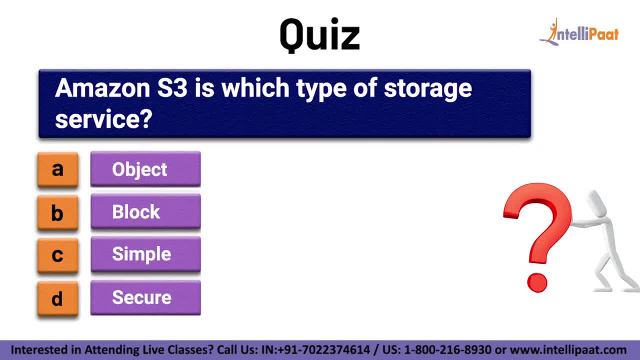 streams. we can simply type in AWS. just a quick info, guys. test your knowledge of AWS by answering this question. Amazon is three. is which type of storage service a object, B, Block C, Simple, D, Secure? Comment your answer in the comment section. 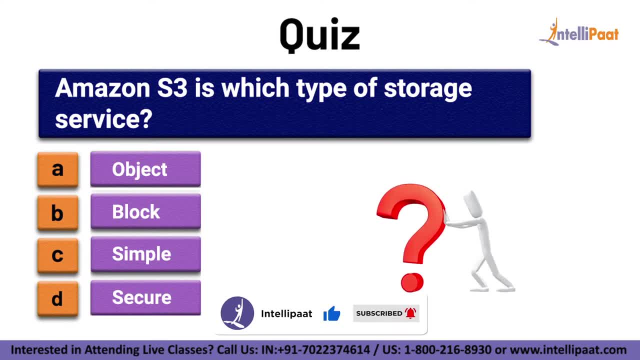 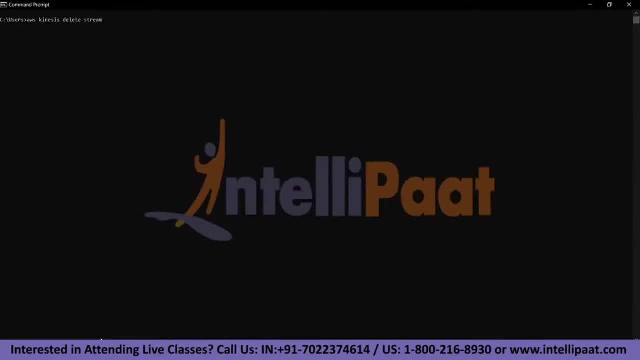 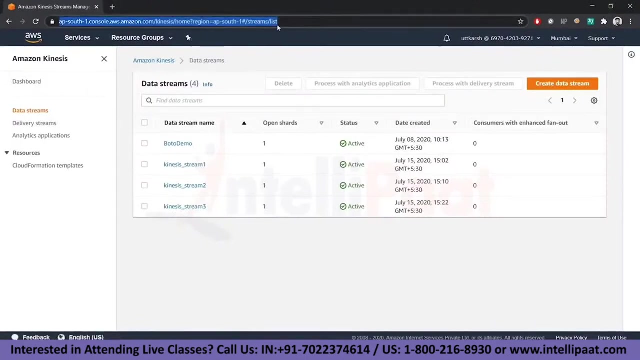 below: Subscribe to Intellipaat to know the right answer. Now let's continue with the session. Kinesis- delete and then specify the stream name. So let us delete the third stream, Kinesis, stream 3, and press enter. So now, if we go back and check our AWS and simply refresh this, 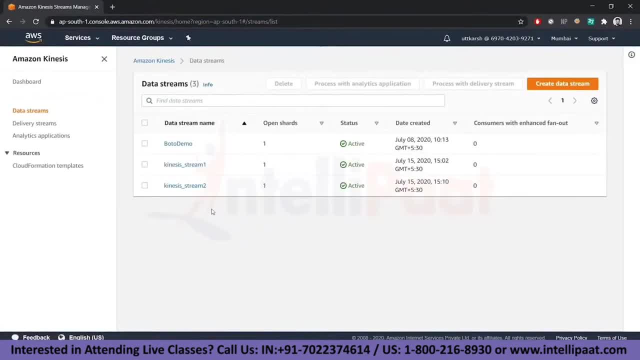 So we can now see that the stream 3 has disappeared. So these are some of the ways in which you can basically manage and handle the streams that you create using Kinesis. So you can do it with the live user interface. You can basically create a Python file and get the Botto library, which is the AWS library. 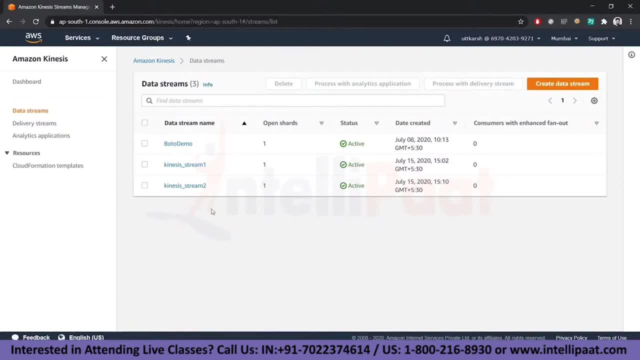 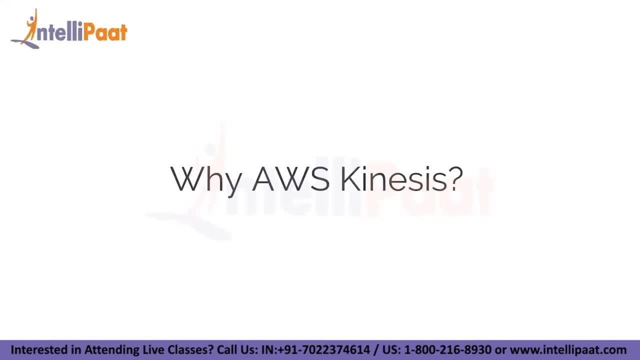 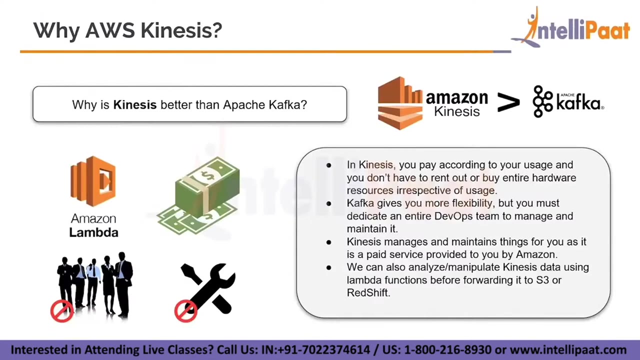 for Python and use the Kinesis module within that, Or you can simply use the AWS CLI as well. So why is AWS Kinesis actually better? So the obvious point of comparison comes as Apache Kafka, And with Apache Kafka you obviously have to own or rent an entire server to basically. 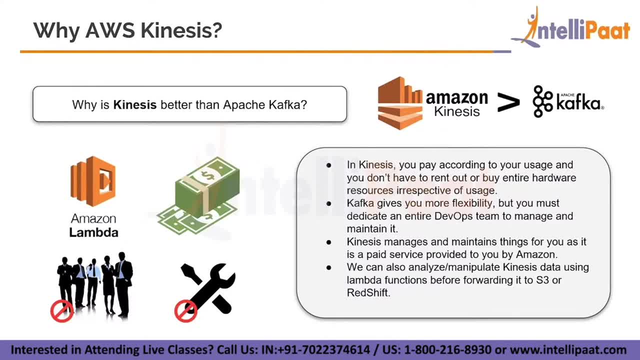 maintain that streaming service, But with Kinesis you only have to pay for your usage And Kafka may give you a whole lot of flexibility, but you do have to dedicate an entire DevOps team to manage and maintain it. Basically, Kinesis manages and maintains everything on its own. 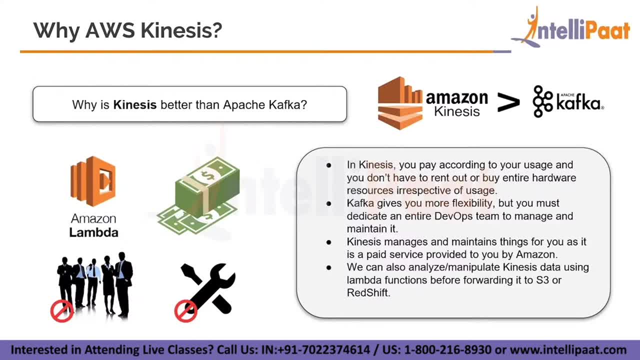 So you don't have to dedicate an entire team or basically any individual for it. AWS is fully scalable in nature, so you can increase and decrease the stream on just a click of a button. You don't really have to get into all of it. 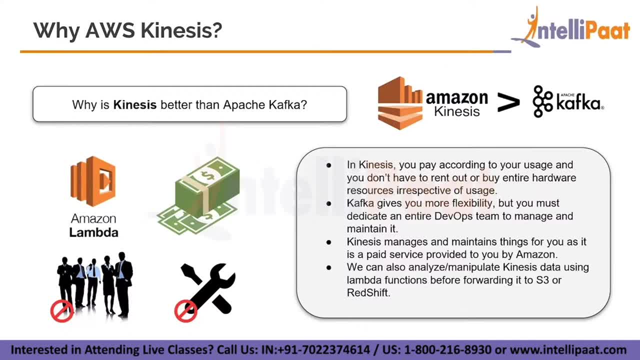 And you can also have the option of manipulating the data that is present within your Kinesis stream before actually forwarding it to S3 or Redshift or any other appliance that is provided to you by AWS. So these are a lot of benefits that you get while you're using Kinesis, which is a fully 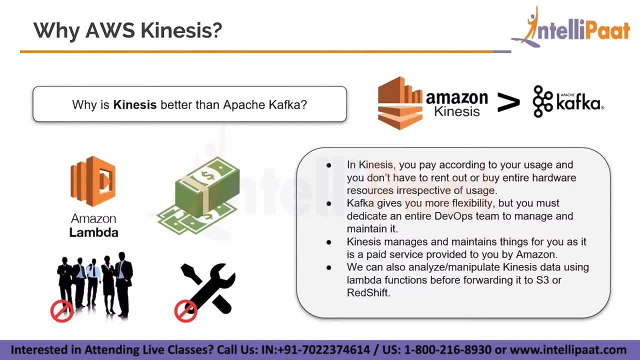 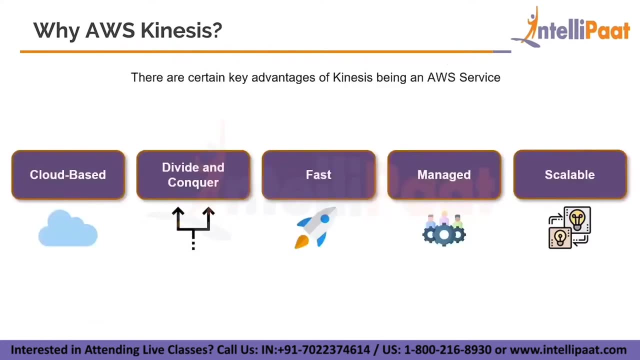 managed service, So there's also a customer service implementation that you can use If you are facing any difficulties. So no maintenance, no team, saving on money And you can basically manipulate the data that you're getting in your stream. So the key advantages include: it is cloud-based. AWS Kinesis is cloud-based, so it's on the. 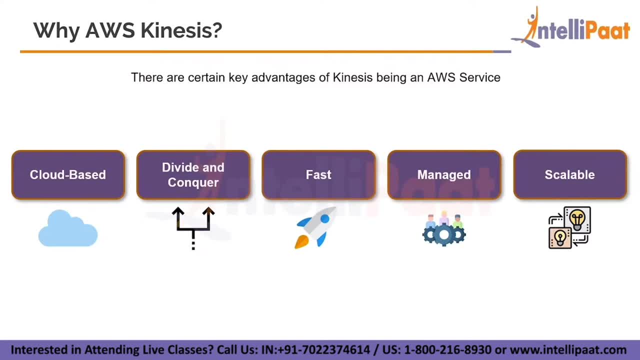 cloud You can use divide and conquer, It is fast, it is managed and scalable. Let us now dwell into how these advantages are. Let us now dwell into how these advantages are. Let us now dwell into how these advantages are. So the key advantages are basically elaborated. 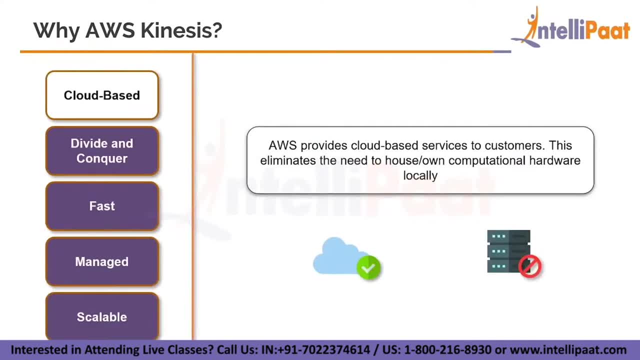 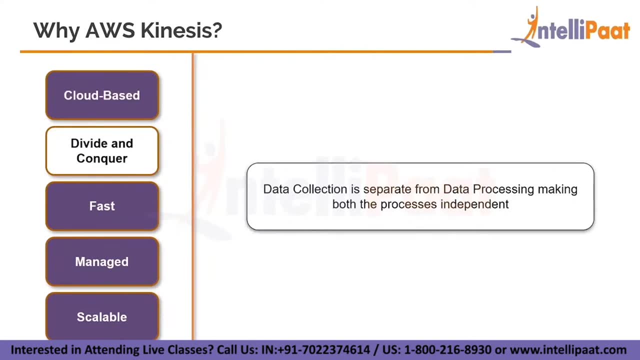 It is cloud-based, which means that you don't have to own any computational hardware. Data collection is separate from data processing, So both of these elements have been separated. You collect the data in a different phase of the Kinesis lifecycle And the data is processed in a different phase of the Kinesis lifecycle. 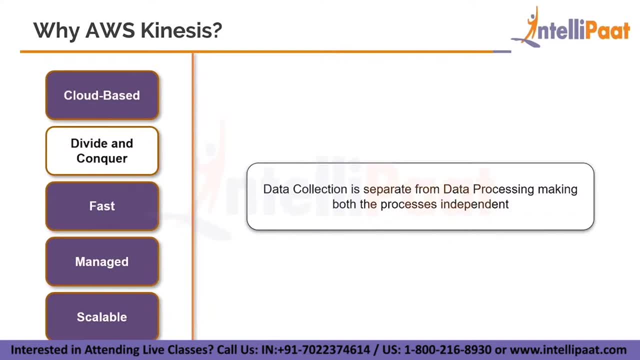 So it doesn't really matter how much data you're collecting on one side. That will be done in the capacity that has been allotted for it. It is fast. so, as we discussed before, one shard has the maximum input capacity of one megabytes per second and a maximum output capacity of two megabytes per second. 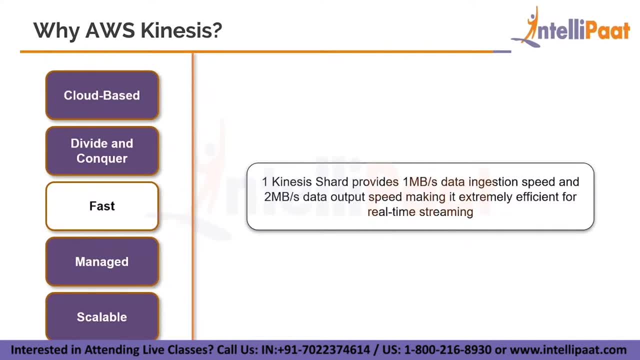 So it's very, extremely efficient, actually for real time streaming, And it is fully managed by Amazon, So you only need to concern yourself with the task at hand, No maintenance is involved, And fully scalable. So, depending on the use case, basically you can increase the number of shards and decrease. 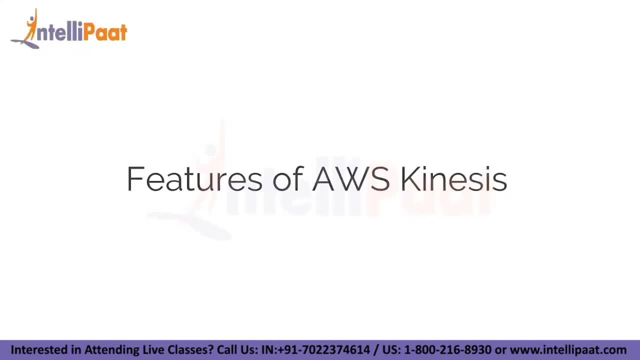 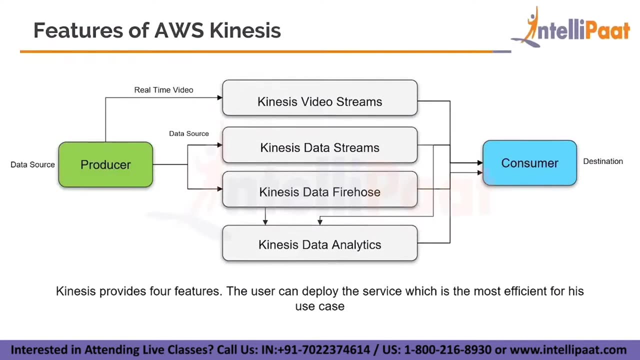 the number of shards. Features of AWS Kinesis. So there are namely four features for AWS Kinesis. The first is video streams, The second is data streams, Third, data firehose And the fourth data analytics. So if you have a real time video that you want to stream, basically with complete synchronicity. 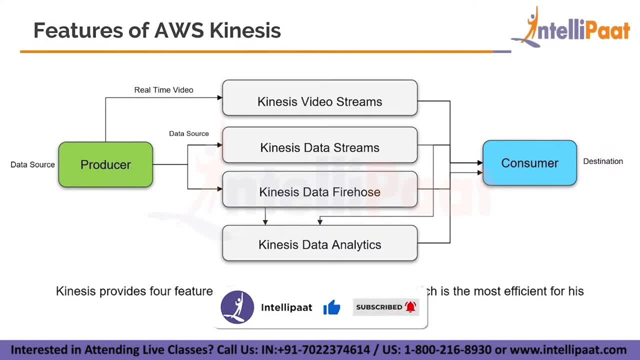 you will basically use the Kinesis video streams feature, Which will stream the video in real time. Then if you have a data source, a file format, data source like JSON, then you can use data streams and data firehose, And often both of them in combination as well. 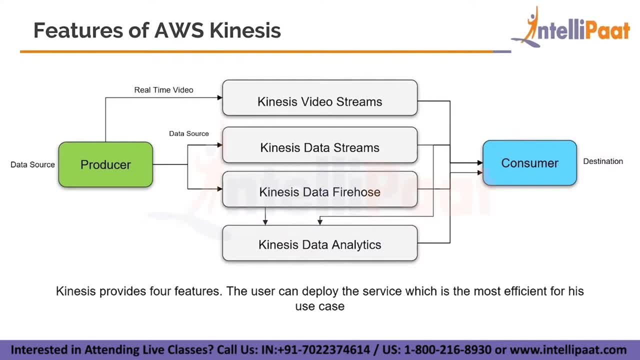 Say, if you want to perform some analytics on this data, you can use Kinesis data analytics by getting the output of the data streams and data firehose to data analytics And then eventually give that output to the consumer as well. So in the video streams. 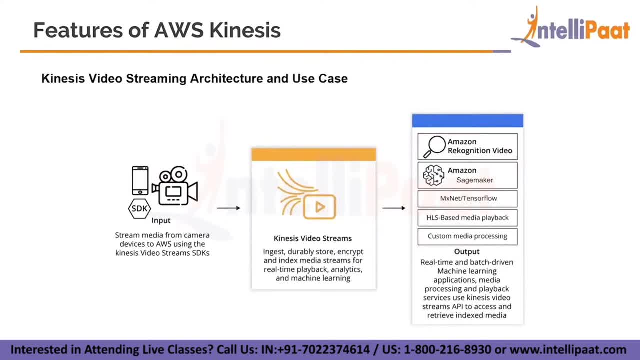 Streaming architecture. we can see if you have a phone, if you have a camera. you can send that data through an SDK to your Kinesis video streams. That video will be sent in real time and you can perform some analytics and ML on that. 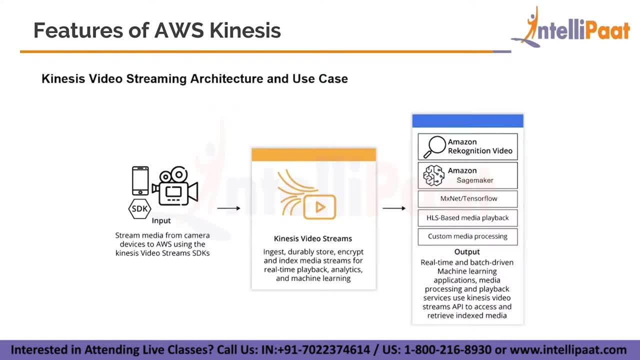 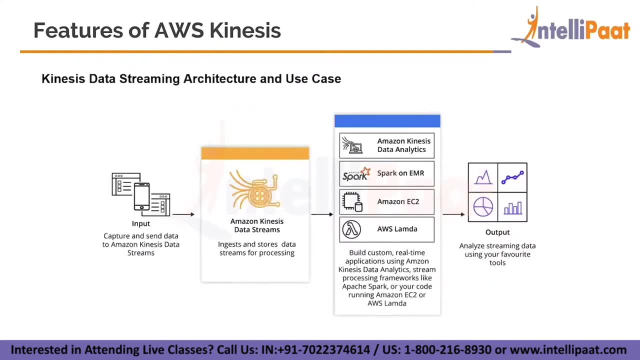 video that is being given to this particular stream and then send it and the output to Amazon recognition or Amazon SageMaker or any other AWS tool, Then you have Kinesis data streaming. So if you have simple files that you want to send that are being generated at the bottom, 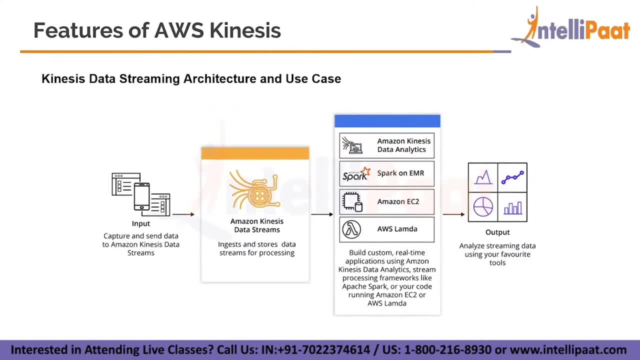 of the producer source. you can use a Kinesis data stream for this, and then it will ingest that data and, furthermore, it will transmit that data to a particular Kinesis data analytics stream or Spark on EMR EC2, or even send that data to AWS Lambda for further transformation. 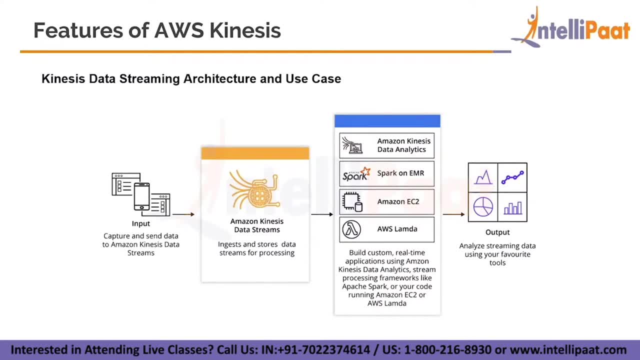 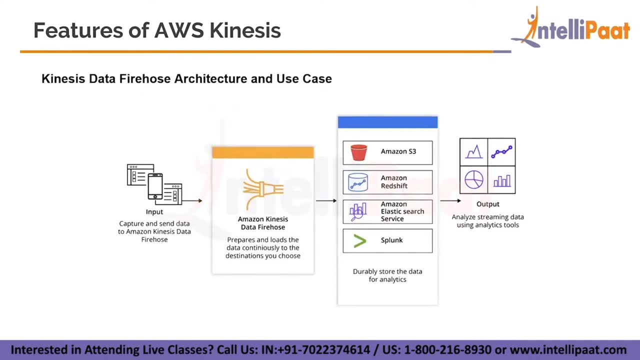 And then, eventually, you can create your analytical output from all of that. So if you have your input data coming from a Kinesis stream- or a normal input source, for that matter- you can take that data and load it continuously in the destinations that you would choose. 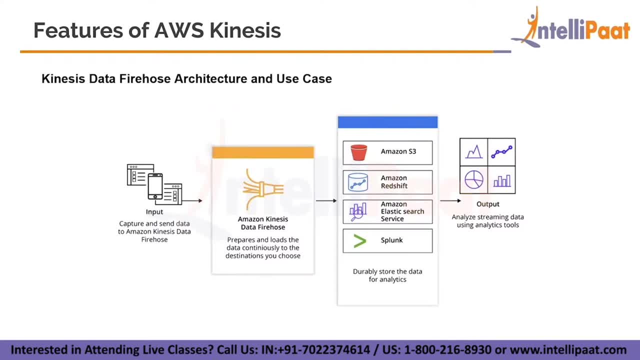 So Kinesis Firehose basically eliminates the middleman. You don't need an EC2 consumer instance that would transfer that data to Amazon, S3 or Redshift or any other AWS service. You can directly store your data in S3 and Redshift with the use of data firehose and 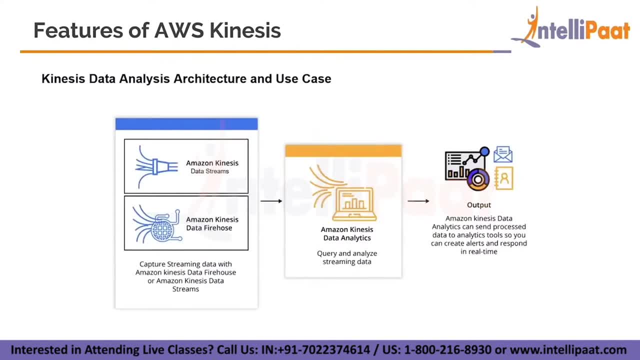 then eventually get your output in the end, And then you have your Kinesis data analysis. So, as we discussed before, the input source for a Kinesis data analytics stream could be a data streams or could be a data firehose source, right? 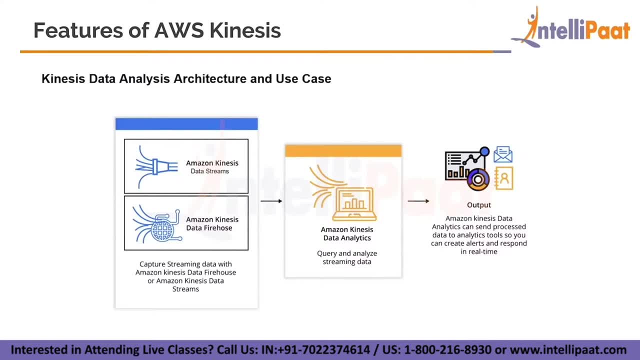 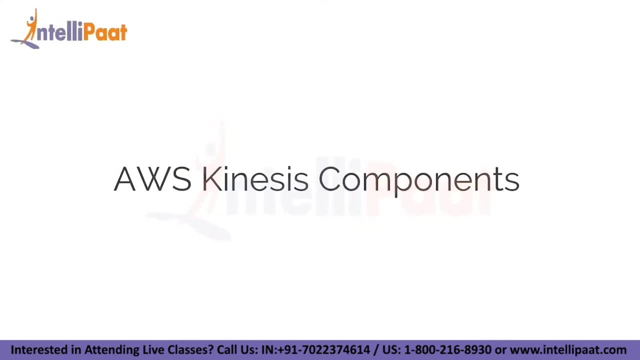 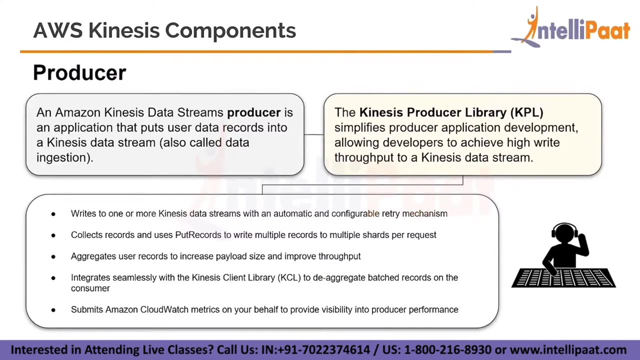 And then, when the data goes, you can perform some analysis and querying on that data and then eventually get your insights and output. AWS Kinesis components. So now we move on to the components that constitute AWS Kinesis. So the first element and the foremost element is the producer. 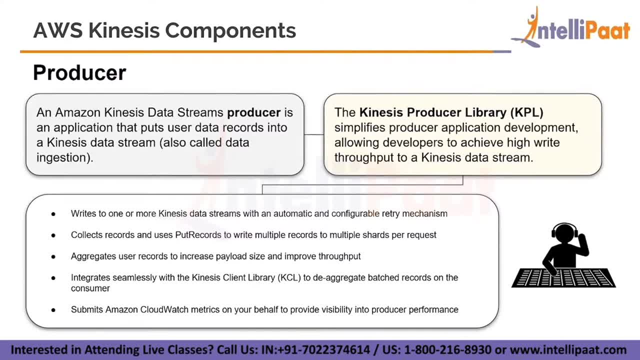 So this is the element Involved in the Kinesis data analysis process that generates the data, So this producer puts the records into the Kinesis data stream, and this process is called data ingestion. You can use the KPL library for this, and this simplifies the application development process. 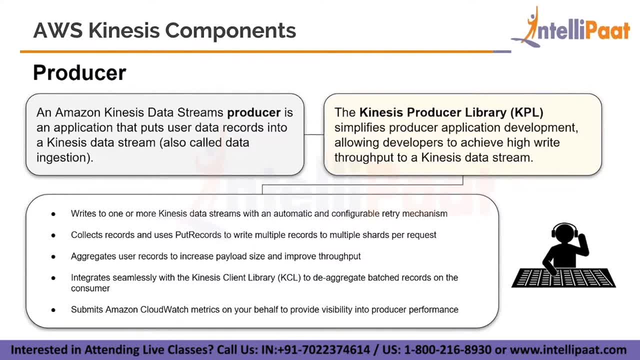 because you can use this library to perform these functions with just the invocation of a particular command. So the functions include rights to one or more Kinesis data streams with an automatic and configurable retry mechanism. So if it fails, the attempt to upload that data into the stream fails once it can retry. 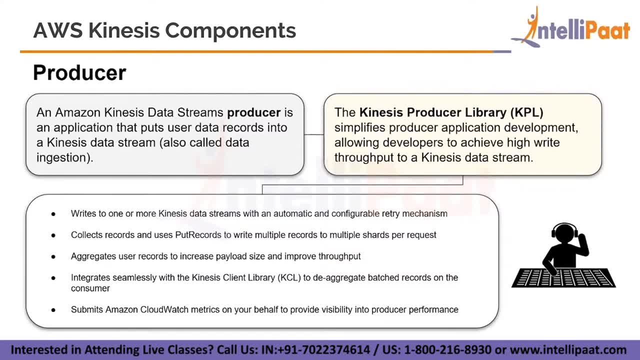 again, and then it collects the records and uses the put records function to write multiple records into the multiple shards of that particular stream. upon request, It aggregates the user records to increase the payload size, So you can basically manipulate the payload size that you want to deposit into the stream. 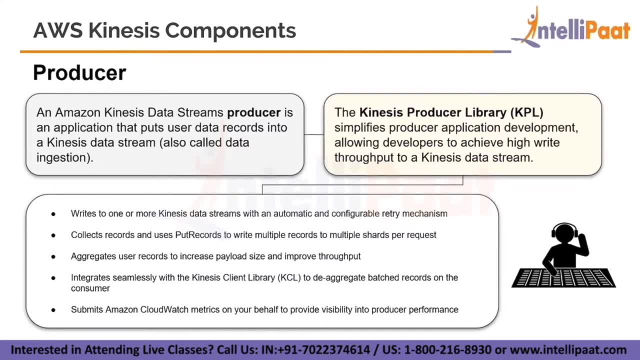 It integrates seamlessly with the Kinesis data stream. So this is the KPL library. It integrates seamlessly with the Kinesis client library, which is the KCL, and basically you can de-aggregate the patched records on the consumer. So once the data reaches the consumer, you can basically de-aggregate the records that. 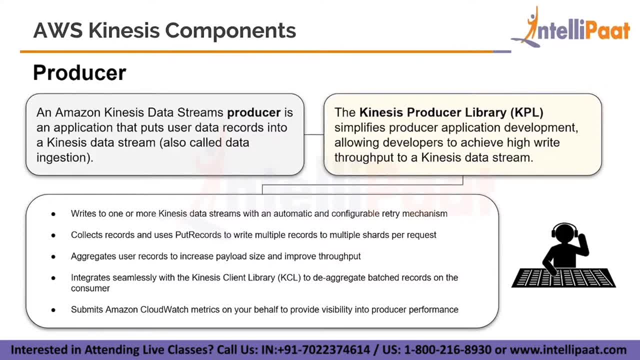 have been patched specifically for the sending purpose, So it's kind of like de-encryption, and then you can also submit the statistics and logs of your producer to Amazon CloudWatch to basically monitor how the producer has been performing and the health of the producer. 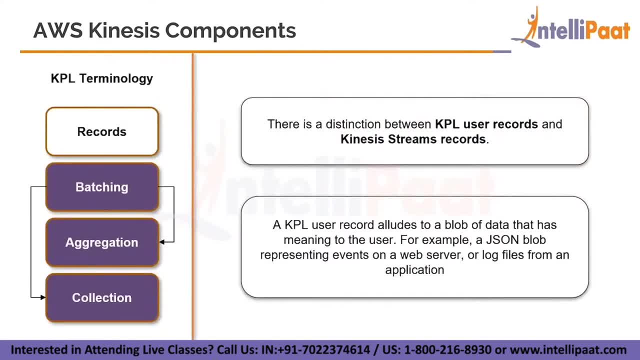 So that's it. So let us look at some KPL terminology. The first is records. So there's a distinction actually between the records that we discussed earlier on in Kinesis streams and KPL user records. So let's see what that is. 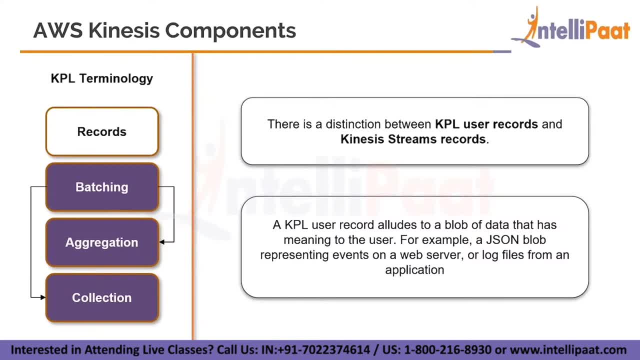 So the KPL record basically references to a blob of data that has meaning to the user. For example, you could take a JSON blob that represents all of the events happening on a particular web application And the log files from that particular application. so that could be an example of what a KPL user 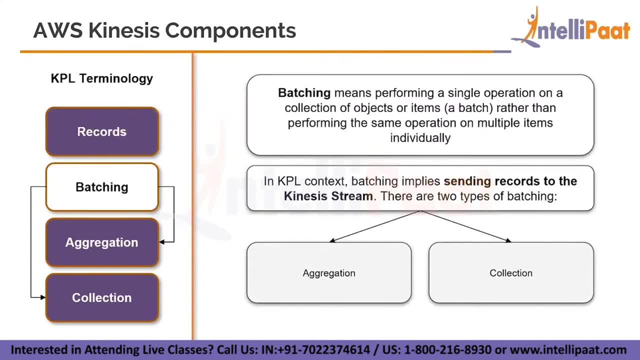 record could be. And then we have batching. So batching means performing a single operation on multiple or a collection of objects. So that means that you have multiple records that you want to deposit to your Kinesis stream, So you'll basically put them through a batching process so that all of this data is properly. 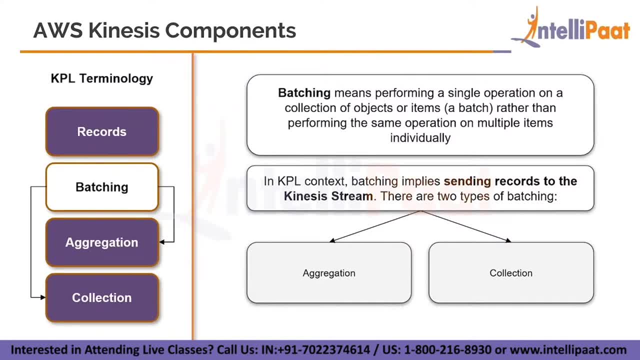 collected and bunched up together So that you can send them in a batch, In a stream, in a very organized way, And then they can be de-aggregated or de-batched when they reach the consumer eventually. So there are two types of batching. 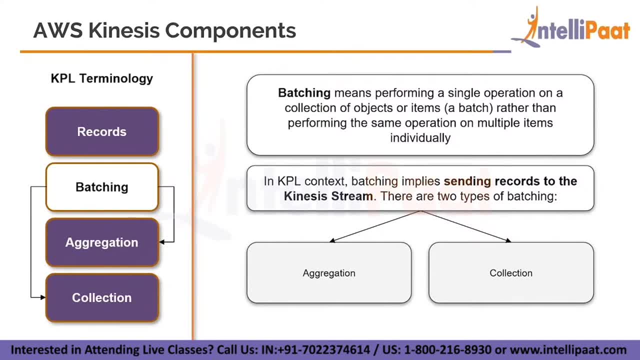 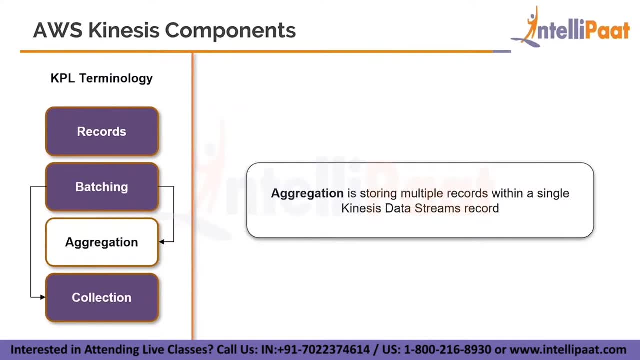 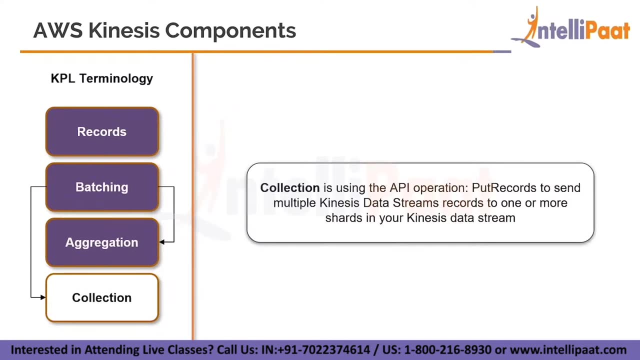 One is the aggregation and the other is collection. Let us look at what both of these are. So aggregation is storing multiple records within a single Kinesis data streams record, So one record will be containing multiple records. So one way you can achieve that is aggregation and the other is collection. 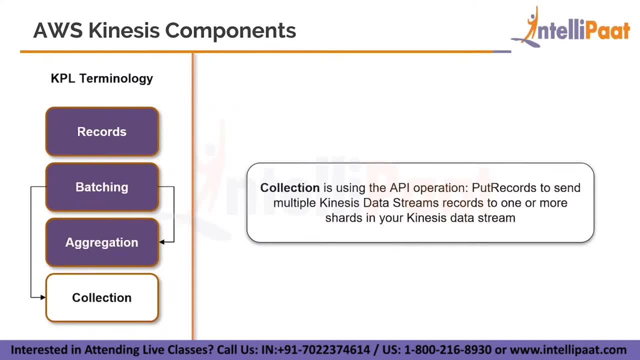 So this is basically an API operation. You can use the put records function to send multiple Kinesis data streams records to one or more shards in your Kinesis data stream. So this basically implies put records as a function can be used when you have multiple. 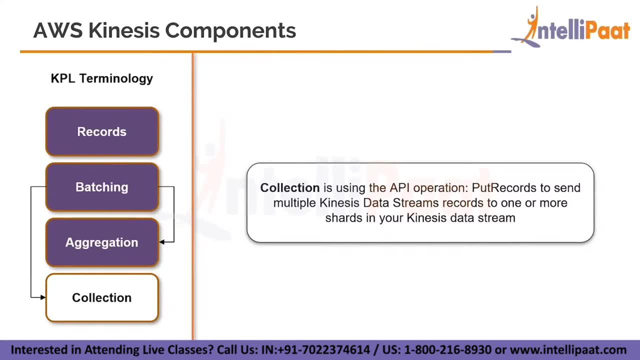 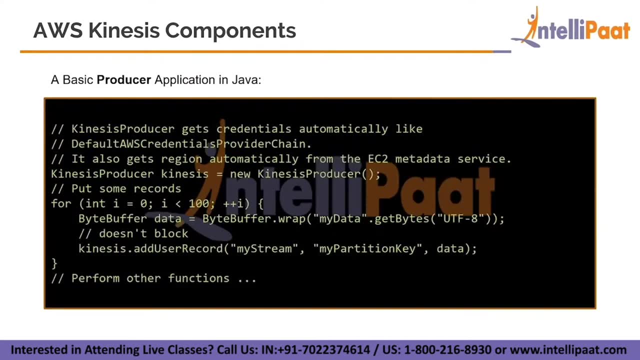 data stream records that you want to send to multiple shards or one shard in your Kinesis data stream. So this is an example of a basic producer application in Java. So you're sending a hundred records over here. So it's the loop. It's from zero to nine. 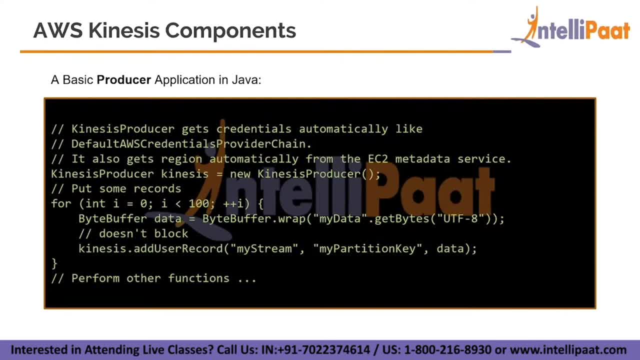 It's about 99,, which is about a hundred, And you're specifying the stream that you want to deposit your data into, which is my stream, and you've specified a partition key and also specified the data that you're sending And, in the consumer it uses, the KCL library does the same thing. 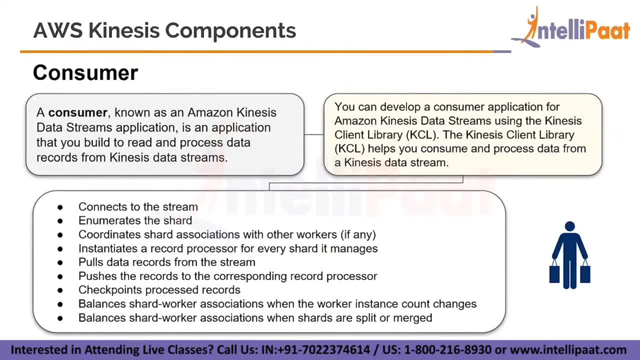 It ingests the data that is being received from the Kinesis data stream. It basically iterates upon the shard and you can get the data that is present within the shard with the shard iterator. So here we can see. this is the code to get the shard iterator for that particular shard. 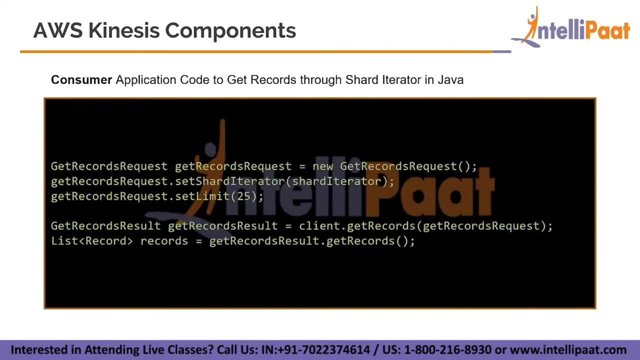 that you want to extract the data from. And here, as we can see, once we've received the shard iterator, once we've enumerated it, we can basically set the shard iterator as a shard iterator which we've received. We can set a limit to the records that we want to extract. 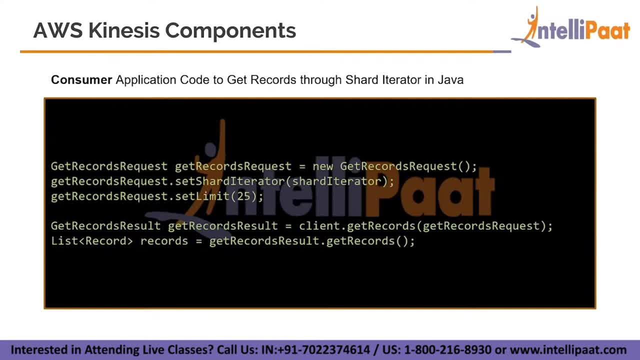 In this case, we set the limit at 25 and then we can eventually get the records once we've set up the configurations. So it's basically we're creating a list, Okay, We're calling it records and it's storing all of the records that is being received. 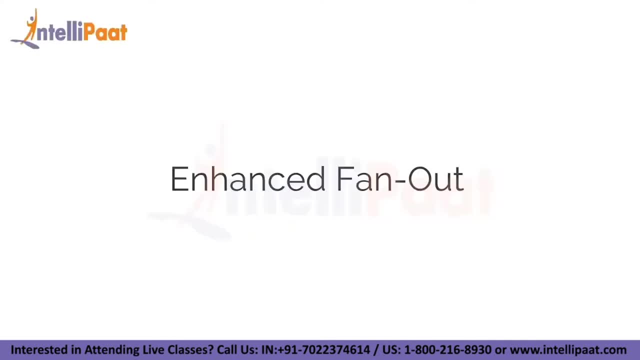 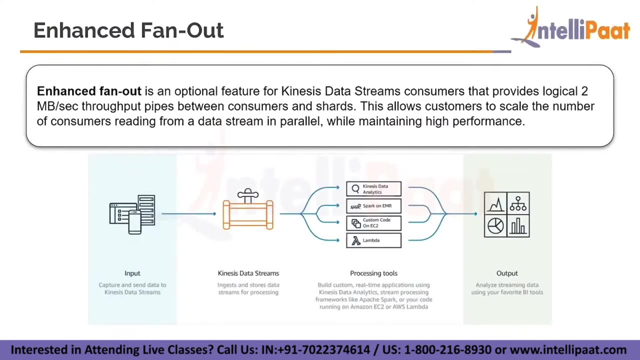 by the shard iterator. Enhanced fan out is one of the other features provided by AWS Kinesis. So say, if you want to scale the number of consumers that are receiving the data from your Kinesis stream, you can use the enhanced fan out feature. 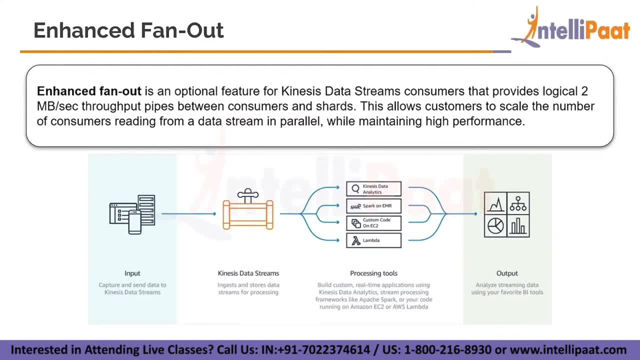 This is usually done when all of the consumers have to process the data that's being saved by them in parallel, And it is done to maintain High performance. So it basically, as we can see in the diagram, the shards are basically having multiple fan. 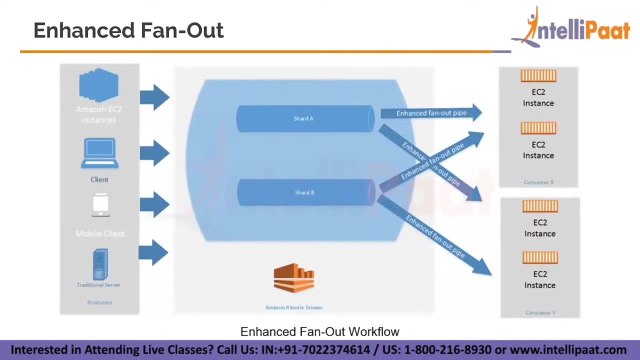 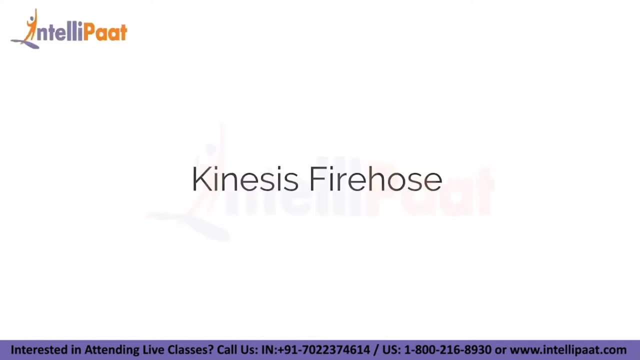 out pipes Right. So the first pipe is going to one EC2 instance and the other pipe is going to the other EC2 instance. So parallel computation is achieved by this methodology And this is an optional element that you can add to your Kinesis streams. 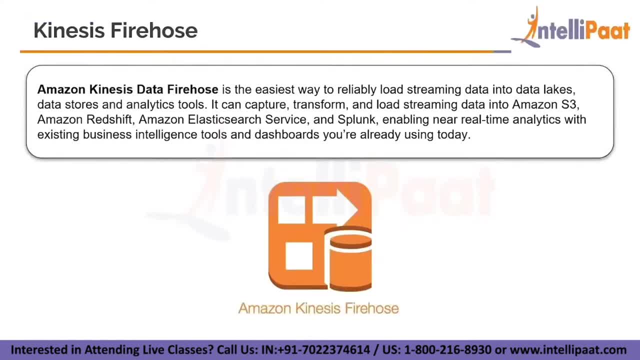 Kinesis Firehose. So this is an additional element on top of the model. Okay, So this is the way the data is being streamed. So in the case of normal Kinesis streams, it is the easiest way to transfer the data, or? 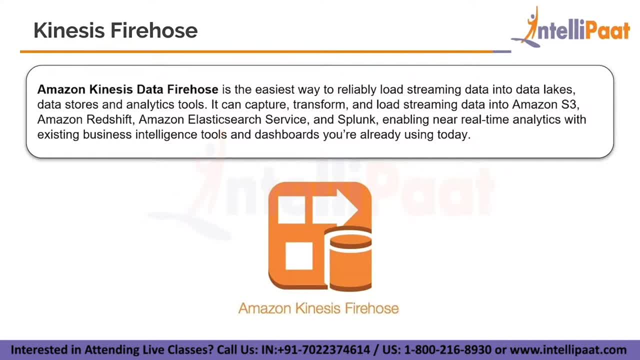 load the data, the streaming data that has been received, into data lakes like S3 and Redshift and Elasticsearch, And essentially enabling real time analytics and achieving business intelligence use cases with the dashboards of business intelligence and other analytical tools that we are already using today. 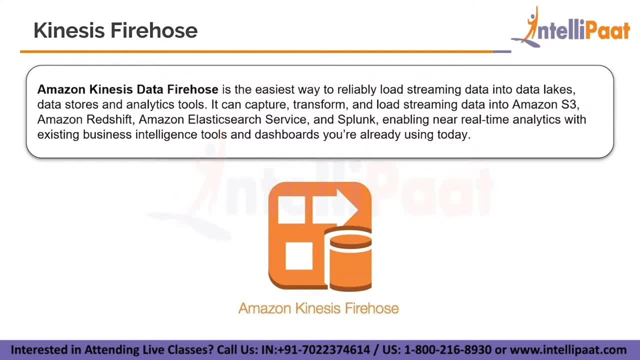 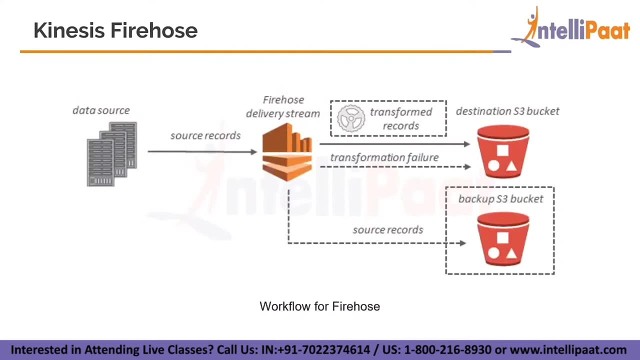 Right. So it's basically. It takes the data, does not need a consumer per se. it will directly transfer that data into a data lake which we can now directly query or warehouse according to our needs. so this is the uh workflow of how the kinesis firehose works. so you have your data source. the data source sends its source records. 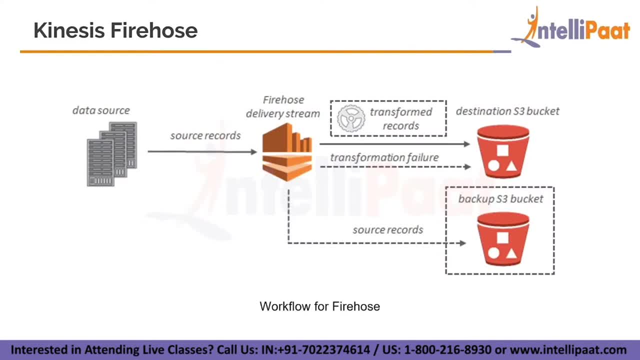 it sends its records. uh, so there are two ways it could go about now. so there is a backup s3 bucket and there's a destination location which is your destination s3 bucket, so see if there is some sort of a failure, if there's some sort of transformation failure or lambda failure. so if you say, if you 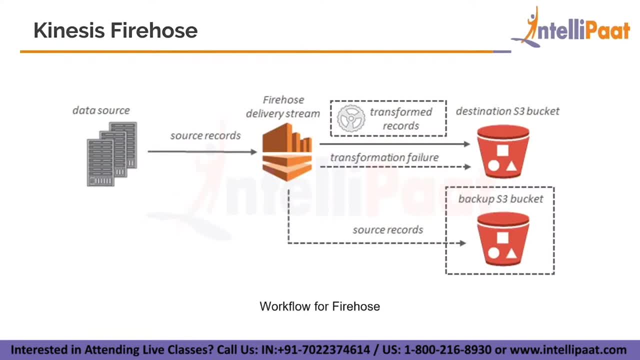 added a lambda function to your firehose delivery stream and that lambda function uh runs into some sort of error, right? so you don't want to lose the records that have been just received by your firehose delivery stream. so you can put up a backup s3 bucket so that data will be transferred. 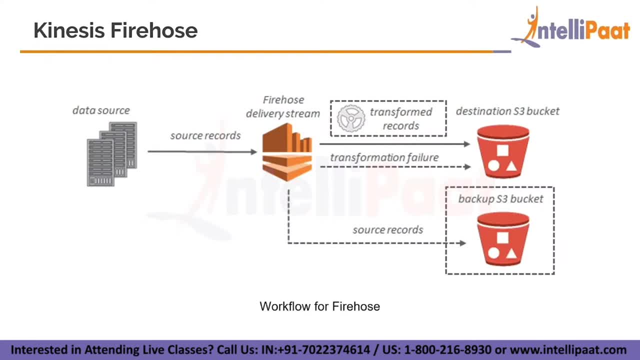 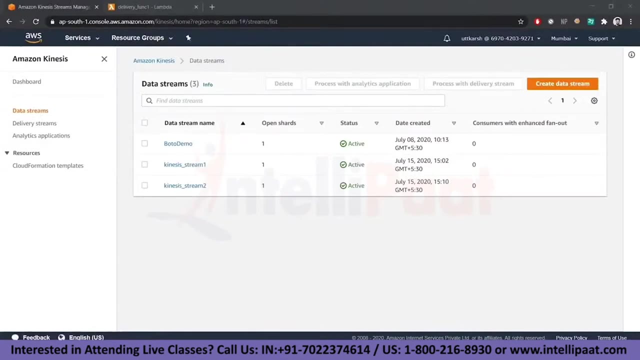 over there and uh, it's not basically lost in translation, and if the lambda function is successful and there are no errors, then definitely the data will directly go into the destination s3 bucket as well. so one of the ways we can use our delivery streams, or kinesis firewall streams, is by attaching them. 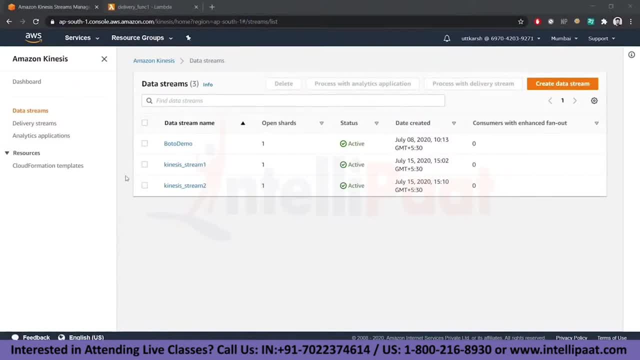 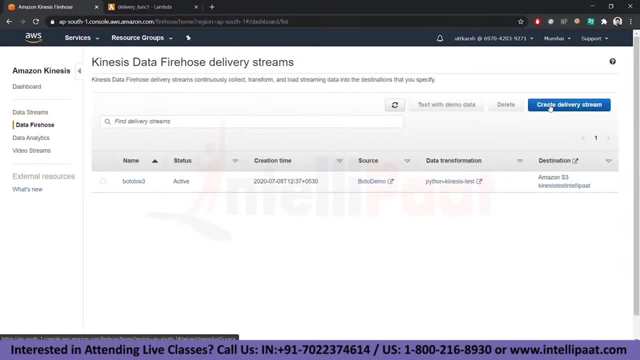 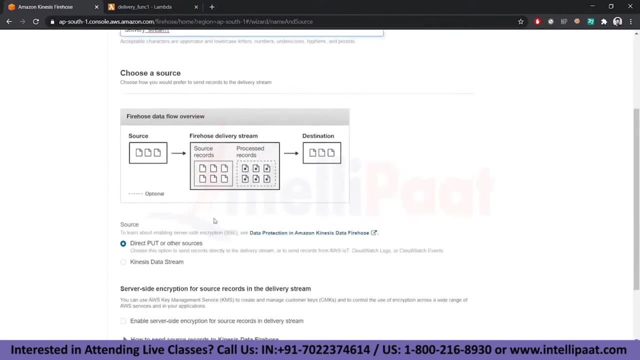 to our existing cases. streams, right, these data streams that we have, so you can simply click on delivery streams and click on it: create delivery stream option. so, uh, you can name the stream anything you want, so i'll call this delivery stream one. you can choose the source, uh, so let us choose a kinesis. 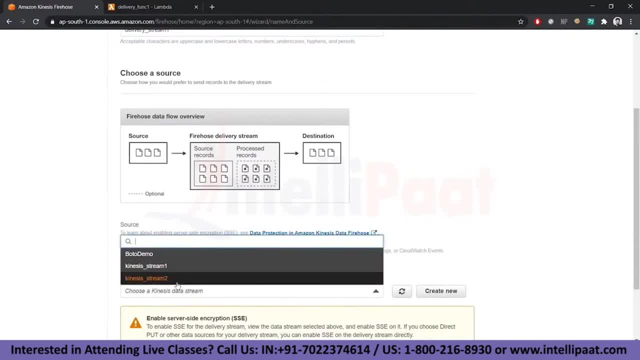 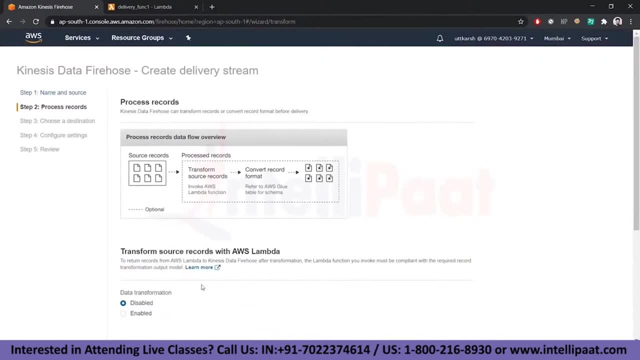 data stream that we've previously previously created. so you can choose any of these, click on next and then you can specify some data transformation functions if you want- right now we're not going to do that- and you can also convert the format in which the data is being. 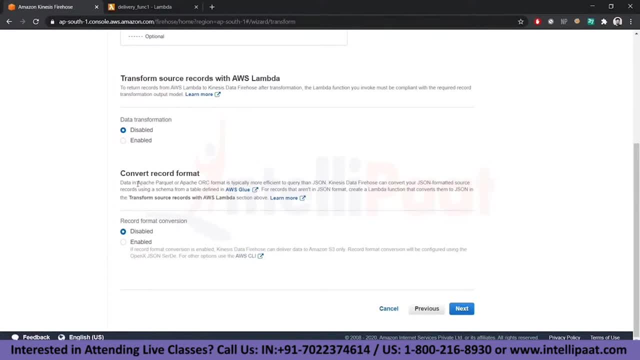 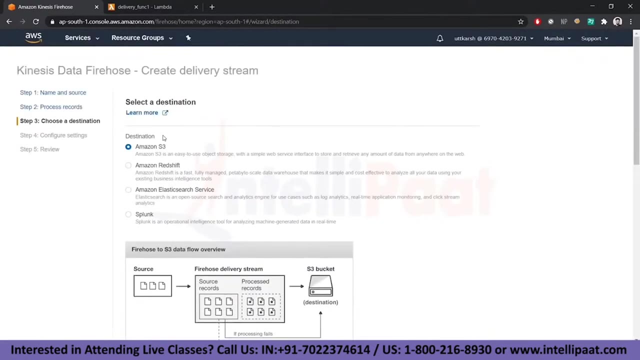 received into the format that you would like. so, uh, apache. if the data is being received in apache format, you can convert that uh with the data record format conversion and then you click on next and then we have to specify a destination. so in our case we want to specify amazon s3 as. 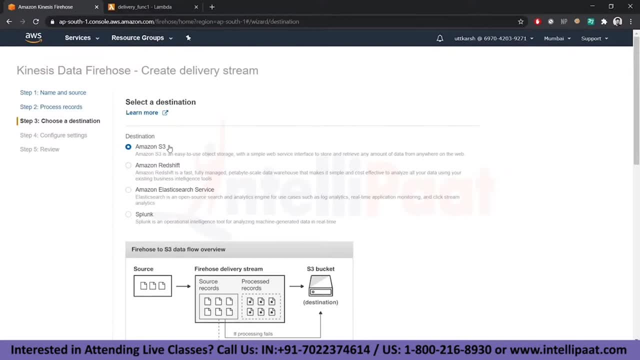 our destination. so our kinesis data stream will send us the data to our kinesis fire hose stream and then the fire hose stream will deposit that data into an s3 bucket. you can specify which bucket we want to deposit our data into. so we can specify uh from here. we want to use our kinesis data. 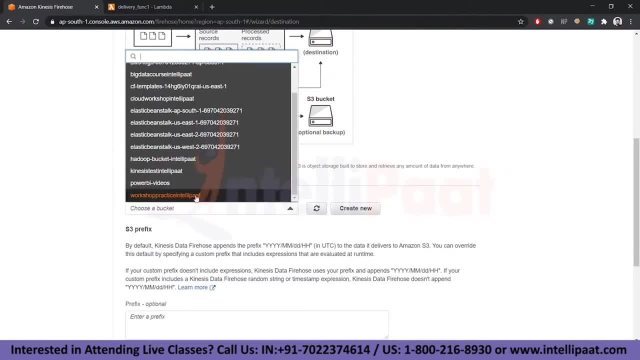 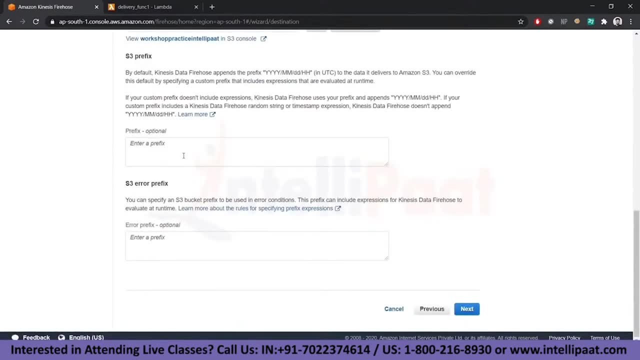 or we can simply go to s3 and create a bucket. so let us specify some workshop practice bucket and then we can specify some prefix for the records that are going to be accumulated in our s3 bucket. so all of the records will start with the name that we specify over here. we are not. 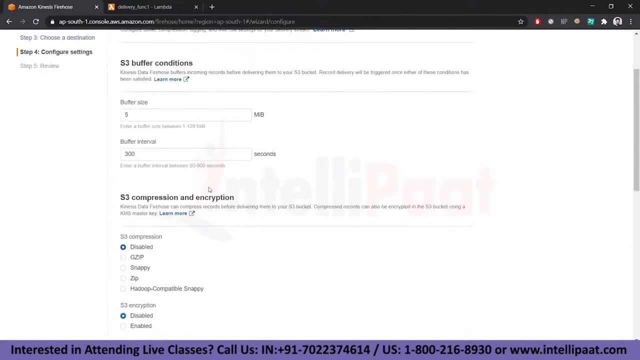 going to specify anything right now and click on next, we can specify the buffer size. so, as we can see the in the description, uh, the data fire hose buffers the incoming records before delivering them to the s3 bucket. so the record delivery will only be triggered once the buffer size has been. 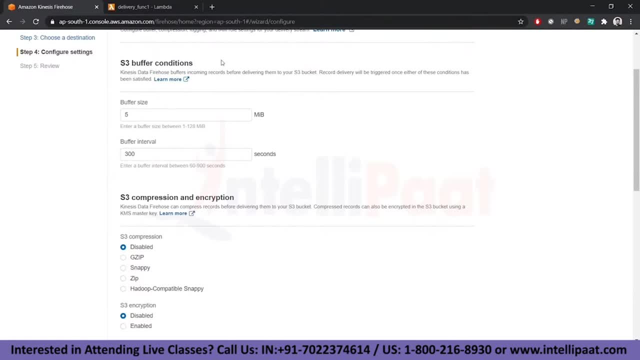 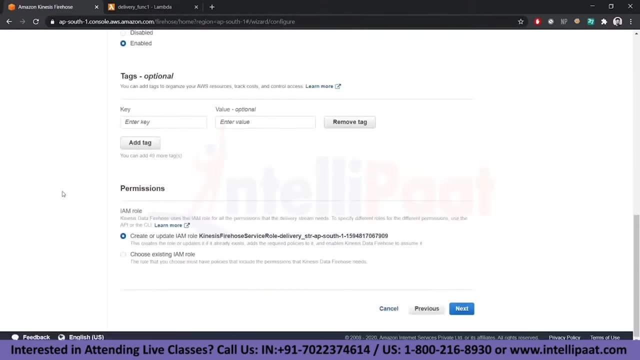 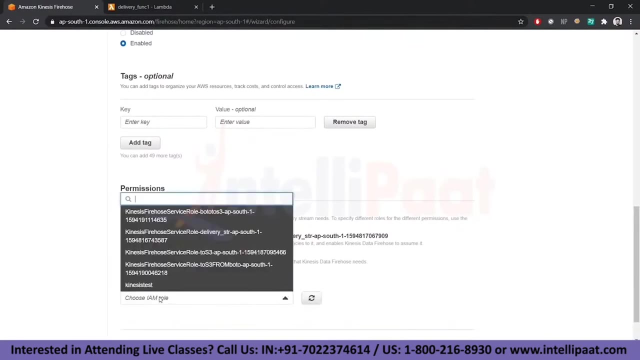 reached. so these conditions have to be reached before the delivery actually occurs. we can specify conversion formats and we can also specify error logging, so let us now create this stream. so i'm going to choose an existing iam role. just a quick info, guys. intellipaat provides aws big data certification course. 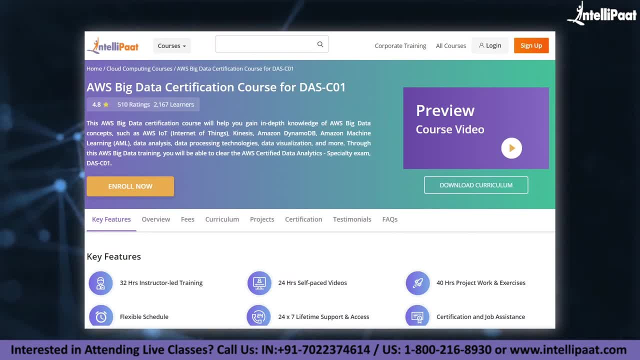 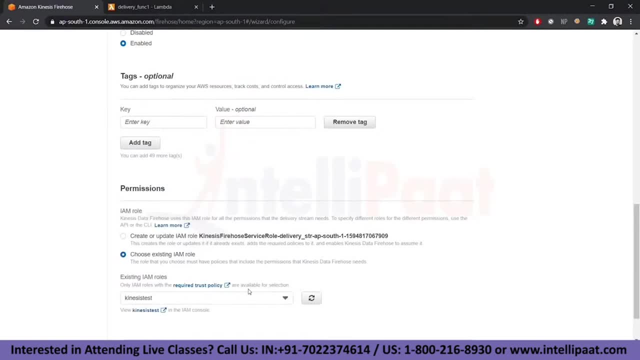 mentored by industry experts, the course link of which is given in the description below. now let's continue with the session. so this is the kinesis test role that i've already created. so this has all of the permissions that are required for you to run your kinesis fire hose. 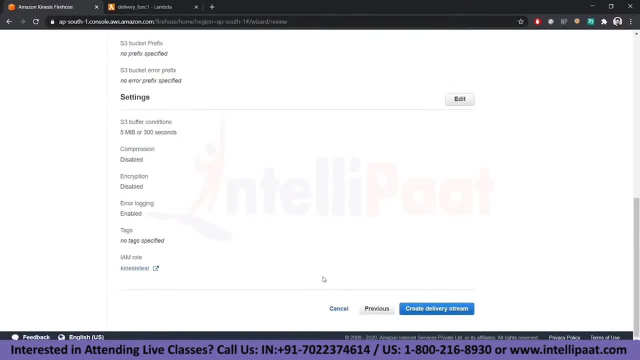 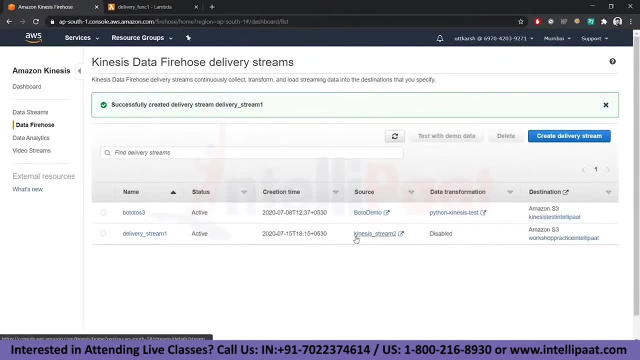 delivery stream, click on next and then eventually click on create delivery stream, so that will create our delivery stream. uh, and as we can see in the source it, it says kinesis stream too, so it's taking data from the kinesis stream that we had earlier created. 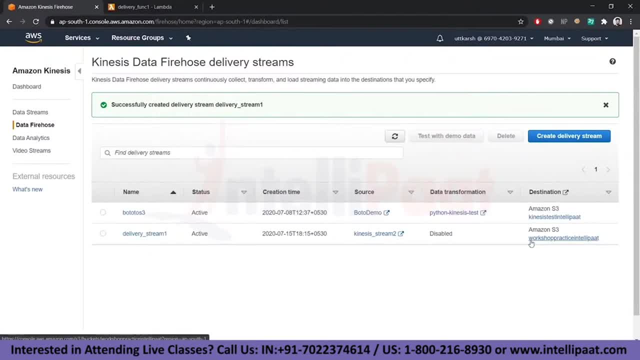 and the destination is the uh folder as the bucket that we've created in our amazon s3. so once the data is being accumulated in our kinesis data stream and it satisfies the threshold conditions uh, that are sort of needed to be achieved for the data to be delivered, 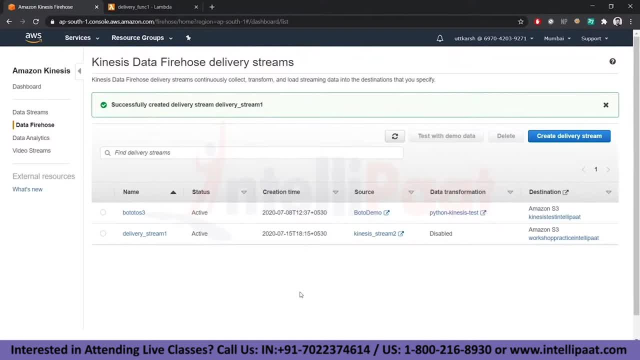 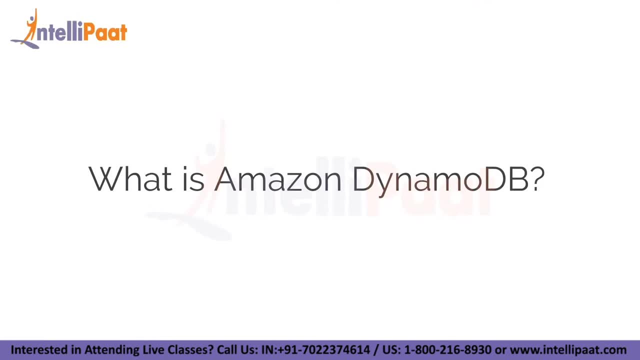 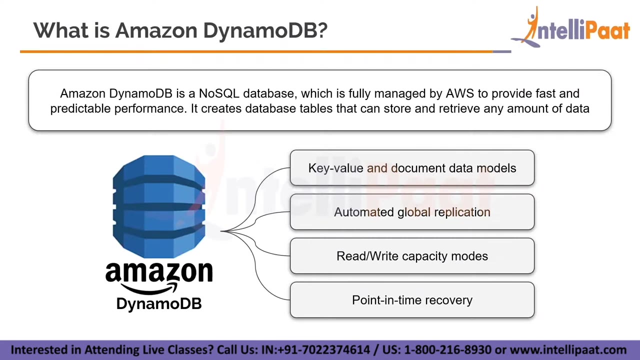 s3 in our fire hose stream. it will be delivered to the workshop practice intellipaat bucket in our s3. what is amazon dynamo db? amazon dynamo db is a no sql database. it is fully managed by aws and it provides a really fast performance. the main advantage of amazon dynamo db is that you can 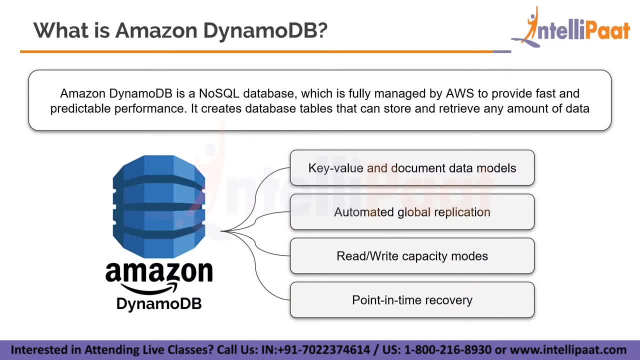 store any amount of data and retrieve any amount of data that you basically have. so, uh, it very well satisfies all the requirements that you need to be able to run your kinesis data stream in our fire hose stream and it also satisfies our big data use case. the four features available for amazon: 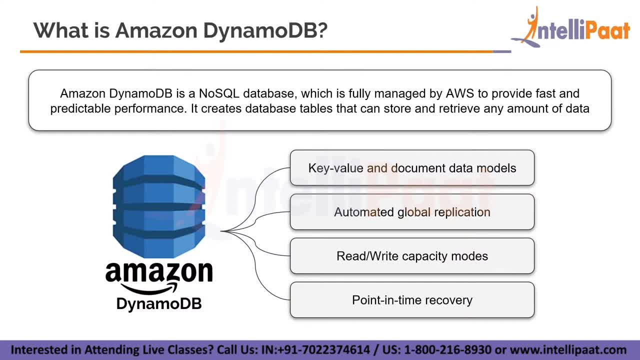 dynamo, dvr, key value and document data models. so json like document data models and automated global replications, which means your data is replicated or backed up. in case of any data loss or hardware failure, you can still retrieve your data. two read and write capacity modes, which are 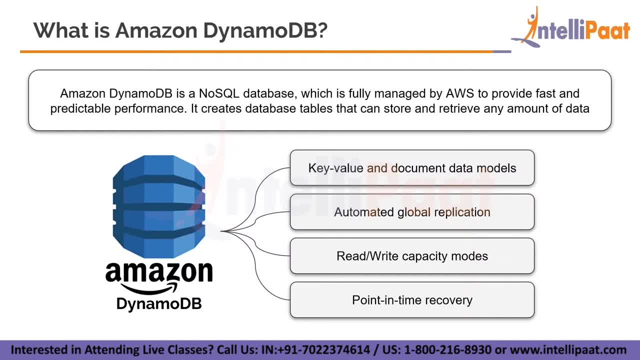 provisioned and on demand. so if you know your use case and how many read and write operations you would require, you would use the provisioned capacity mode, and if you don't know, you can use the on-demand capacity mode. it basically depends on how much pricing you want for your particular dynamo db use case and 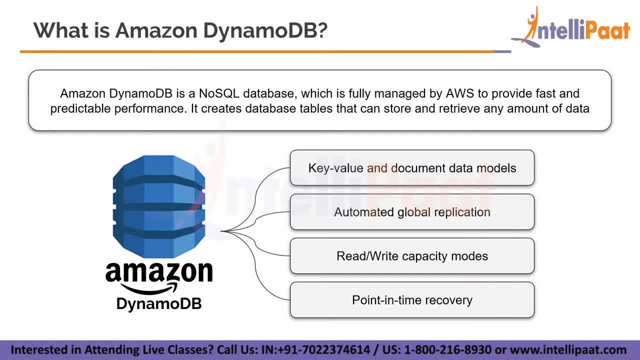 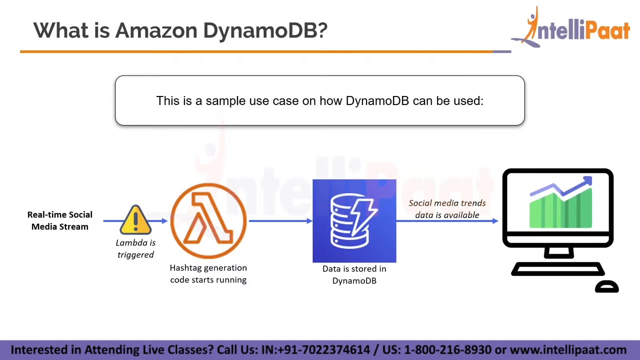 the fourth is point in time recovery, so you can recover your data and restore it to any point in time in the past. so that is available as a feature for amazon dynamo db. so let us look at a sample use case of amazon dynamo db, of amazon dynamo db. so say you are generating some social media data. the stream is coming. 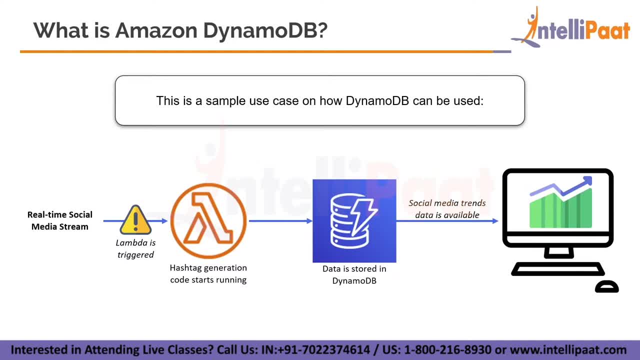 when the stream comes, a lambda function is triggered and the code within that lambda function, which is a hashtag generation code, starts running. once it starts running, it basically stores the data within your dynamo db database. so once it has been stored and cataloged within your dynamodb database, you can simply query this data and visualize it and create your trends. 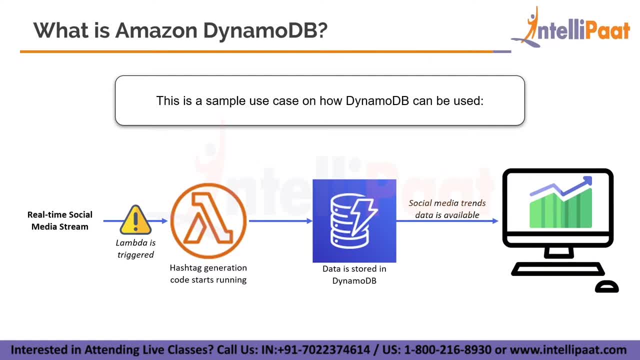 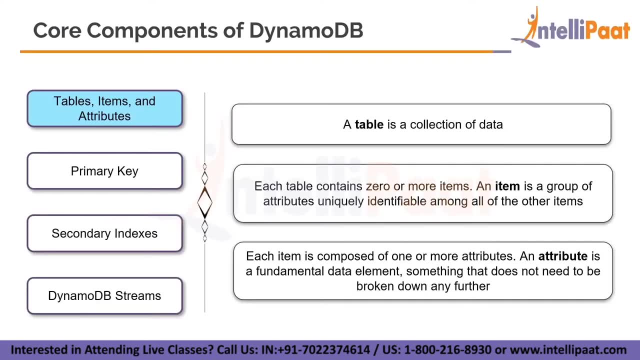 create your analytical models. so this is one of the use cases that is possible for Amazon DynamoDB- core components of DynamoDB. so there are four core components that constitute DynamoDB. the first of these components is tables, items and attributes. so, like in SQL, you have tables in DynamoDB as well, and each 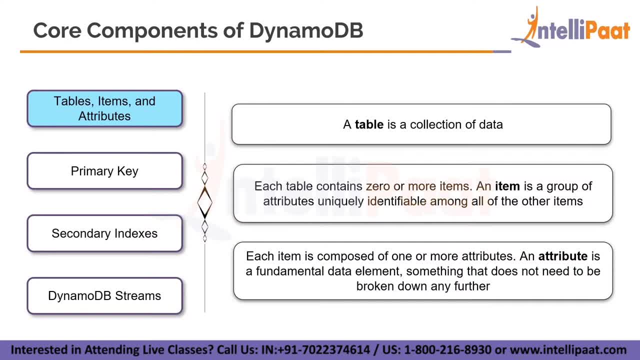 table can contain multiple records. in this case, these records are called items, and these items are basically key values, and these key values correspond to some values. these values are called attributes. so there is a combination of items and attributes. so this is what constitutes a table, which is a. 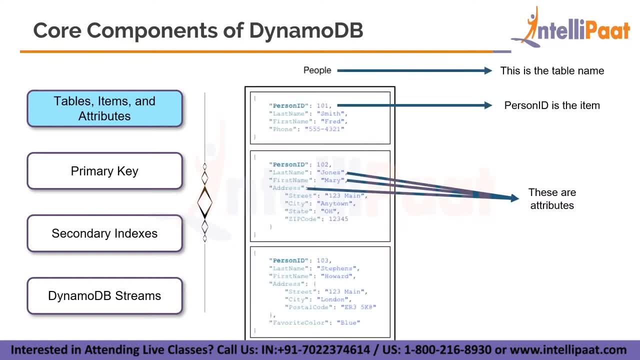 collection of data within DynamoDB. so here we can see that person ID. on the left hand side, which is the item, is also the key. that is what basically is the section. it's kind of similar to what a column name is in an SQL table and on the right hand side is the value associated to that item. now this value. 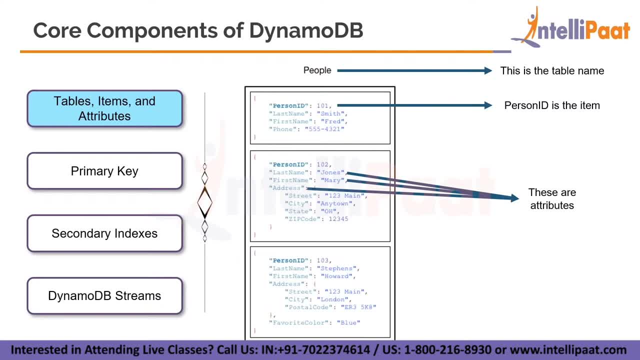 is called an attribute, so an attribute could be singular. or if we go to the second box on the bottom, we can see that the address item has multiple values or attributes associated to it. so it's a nested list within address, a nested dictionary with an address. so 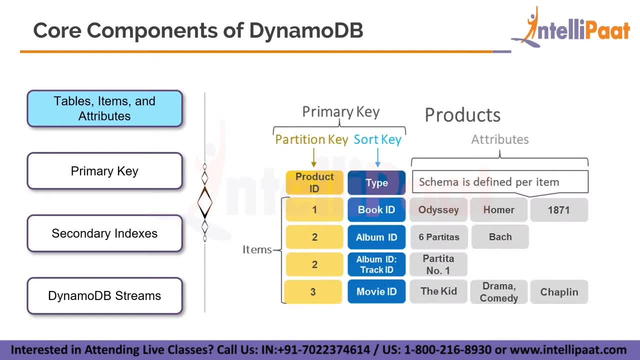 attributes could be multiple as well. so on the left hand side there is the unique identifier, which is known as the primary key. like in SQL tables now, this primary key can be constituted of a partition key and a sort key. so a partition key is basically what makes the separation. as to define the 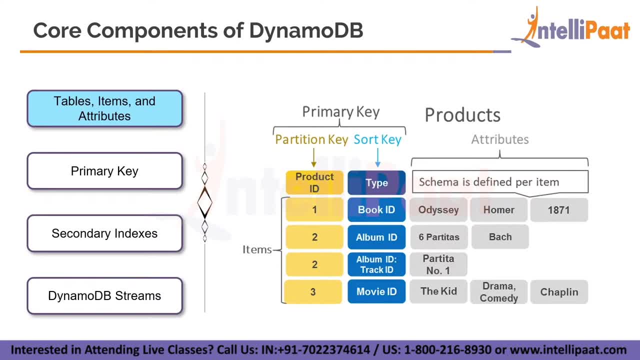 difference between attributes. so here are three product IDs in the partition key: 1, 2, 2 and 3. so it basically is a summation of three. so in two specifically we can see that the first two contains an album ID, while the second two contains an album ID and within the album ID it also. 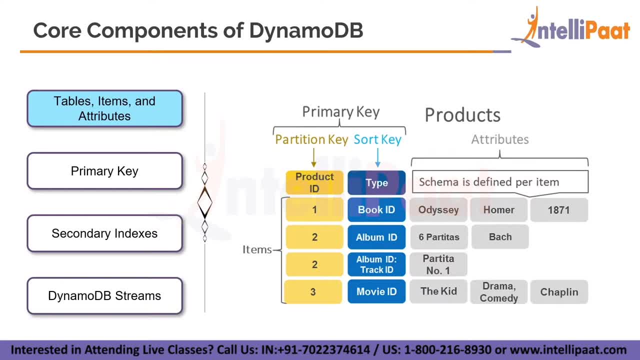 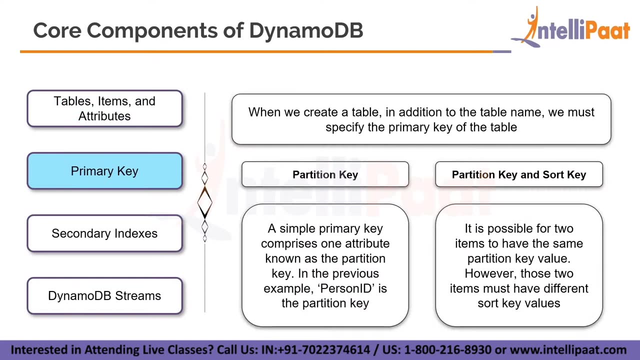 contains a track ID, so this is to more uniquely identify a particular attribute. so this is the basic format of how a DynamoDB table looks. so we'll get more into this once we get into the hands-on section. now let us look at the primary key in detail. so the primary key is constituted of a partition key or it. 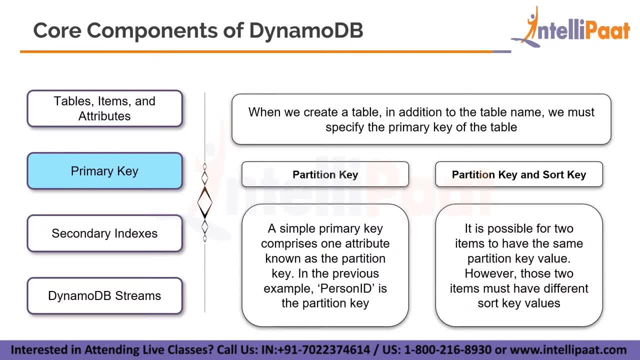 could be constituted of a partition key and a sort key. so when we create a table we must also specify the primary key of the table. a simple primary key comprises of only one attribute, so there is only the partition key that is involved in it, and then there is no sort key. so the primary key of a partition key is a. 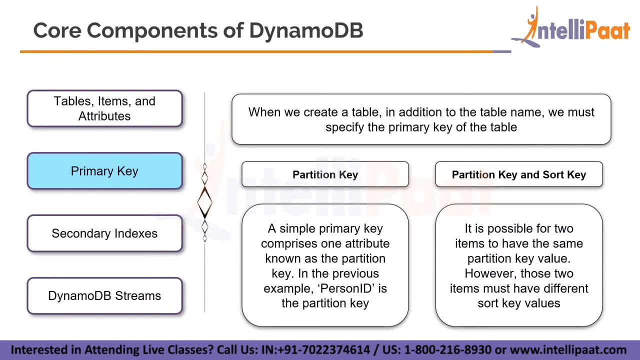 key right. so in the previous example the person id was the partition key. it is also possible to have a partition key and a sort key, but these two items must have different sort key values. so even if the partition key value is the same for two particular records, there should be different. 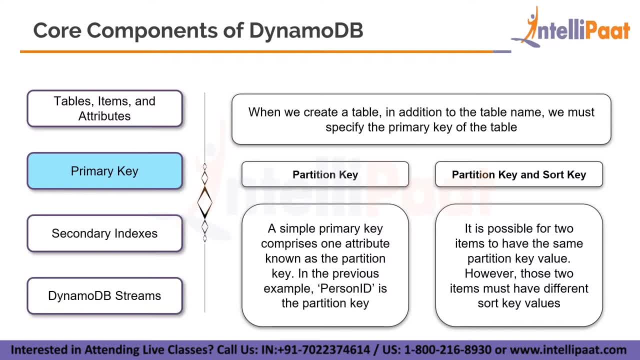 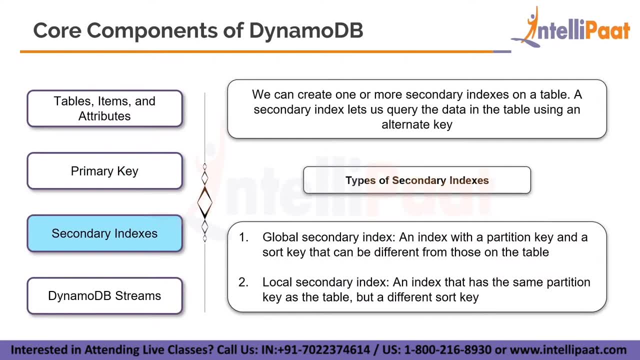 sort key values to uniquely identify the attribute associated to that particular item. then we have secondary indexes, so we can create one or more secondary indexes on a table. it basically lets us query the data using an alternate key. say, if we don't want to use the primary key, we can also. 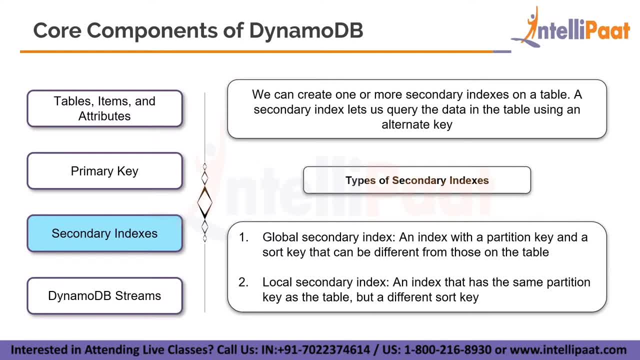 uniquely identify attributes using an alternate key as well. so there is a global secondary index that you can have, which is basically an index with a partition key and the sort key that can be different than those already present on the table. and then there's a local secondary key, which is basically the same partition key as the table, but 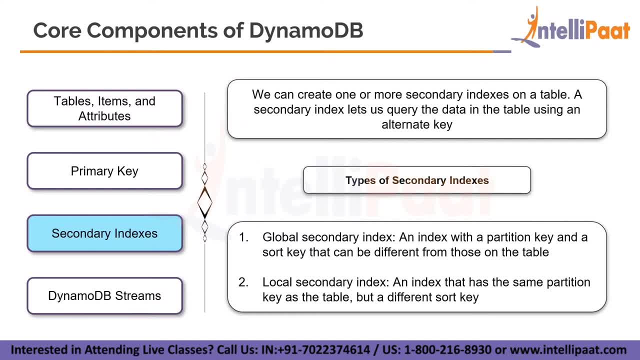 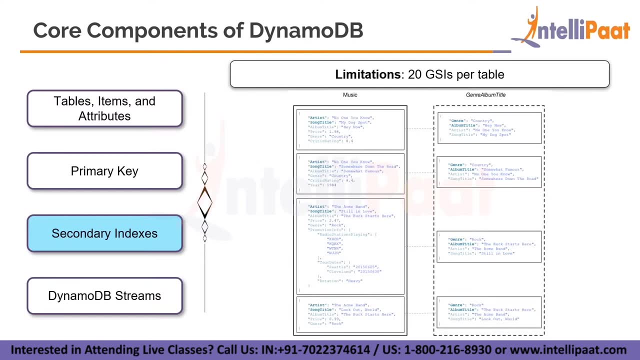 has a different sort. key all of this is to access data in a more unique format. so DynamoDB offers you very much a flexible environment in which you can access the data that is present within your repository. there is also a limitation of 20 GSIs per table, which means you can have a maximum of 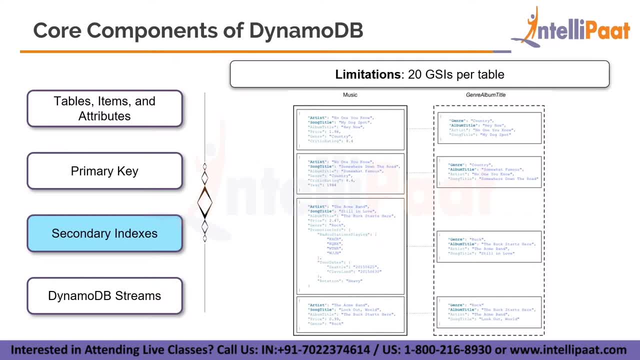 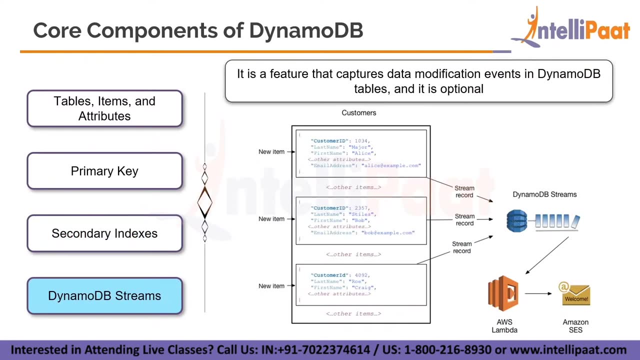 only 20 global secondary indexes, so you can have a maximum of only 20 global secondary indexes per table, which was earlier 5 but now has been increased by Amazon. you can obviously request for a further increase by putting in that request to AWS. and then there are also DynamoDB streams, so 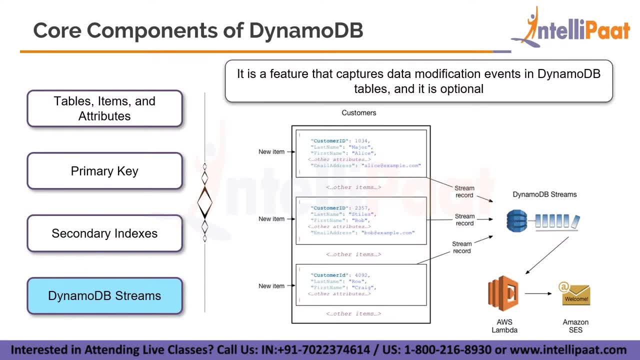 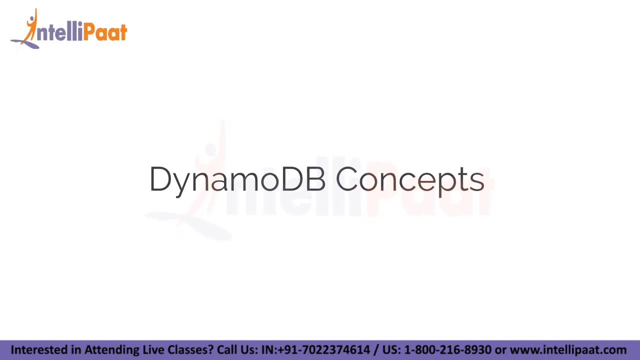 if you want to stream the records, you can do that as well. DynamoDB allows you to stream your records in a format so you can send these streams to AWS Lambda and then the lambda can process it and send it forward to Amazon further services as well. dynamodb concepts. so there are a few concepts related to dynamodb. 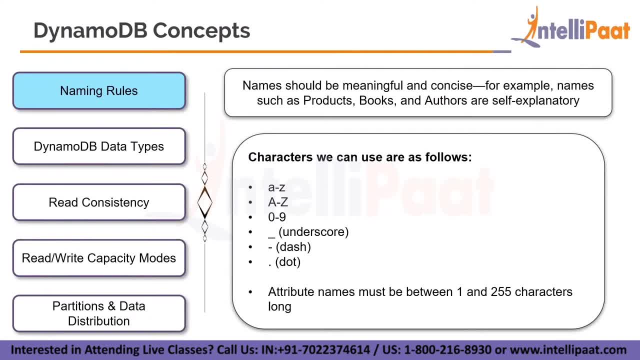 the first includes the naming rules. so in item names we can only use the following characters, so small characters, uh, cap characters 0 to 9 digits, underscore, dash and dot. and the other rule is that the attribute names must be between 1 to 255 characters. then there are dynamodb data types. 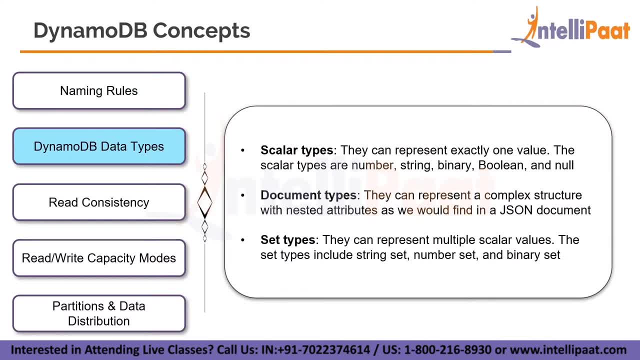 so there are scalar data types, which basically correspond to one value. these values could be number, string, binary, boolean and null. then there are document types, so these types usually represent complex structures with nested attributes, like we would find in json files. and then there are set types, which are basically 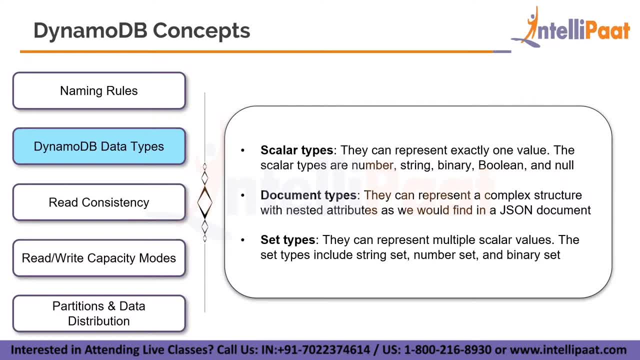 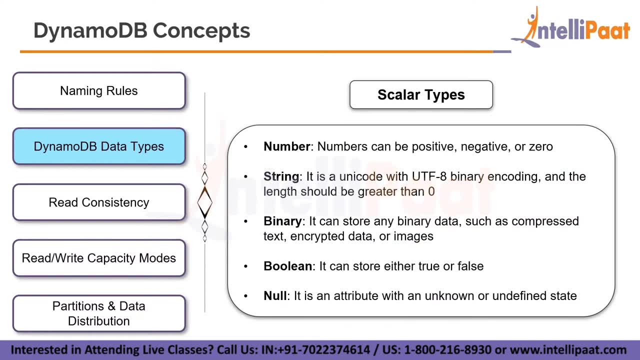 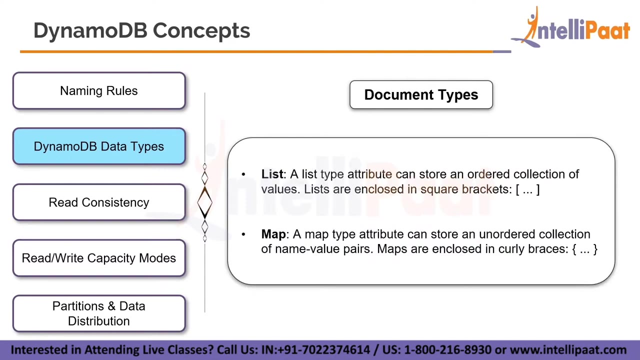 nested scalar values, so one set could be included within a particular scalar value in itself, so that those are sets essentially. so let us look at scalar types. so sailor types include numbers, strings which have the utf-8 binary encoding. then there's binary boolean and null. there are document types which could include lists and maps. so the maps are what we see in. 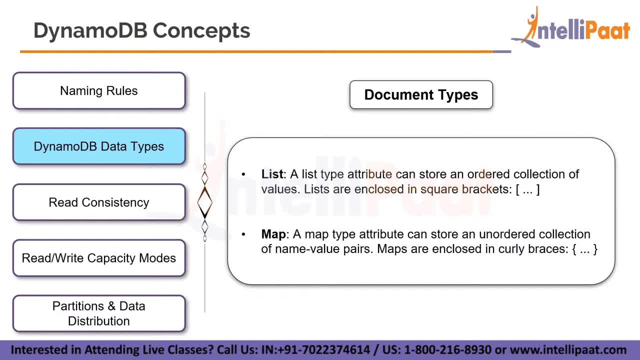 the common json for a set of numbers, and then there are set types which include numbers and formats which are key. value pairs and lists are basically: when we have an item name, we can correspond a list to it. now, these lists could be an ordered collection of values. so these are. 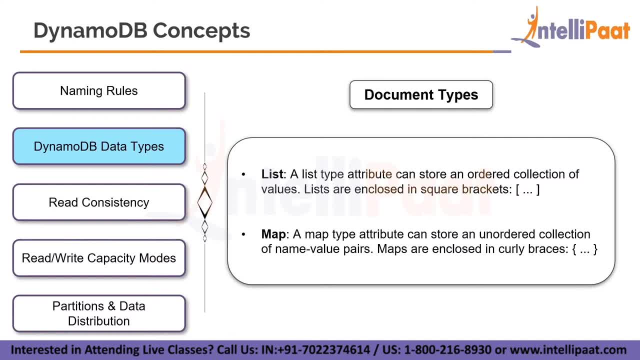 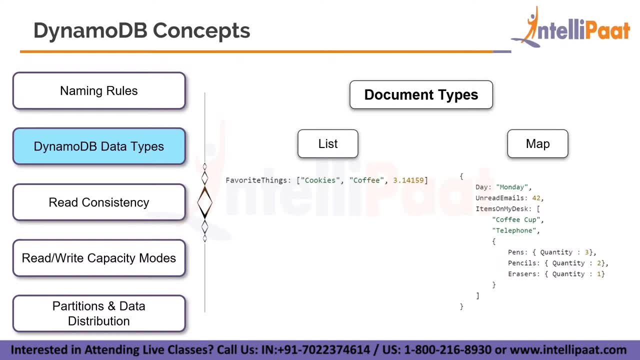 enclosed in square brackets. the brackets are what makes the difference. so let's look at an example. so say we have a item name- favorite things. so it says it is basically corresponding to a list which includes cookies, coffee and a numeric value map. so within map we can see that all of the item names are corresponding to an attribute. 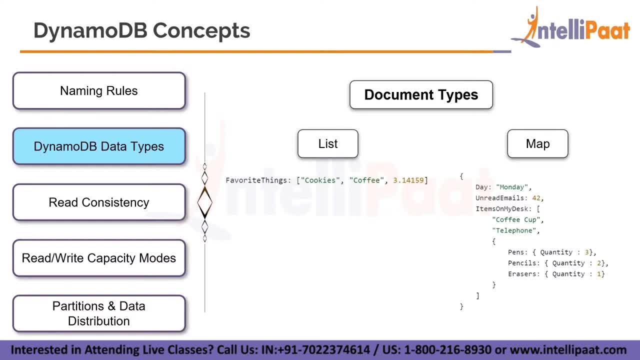 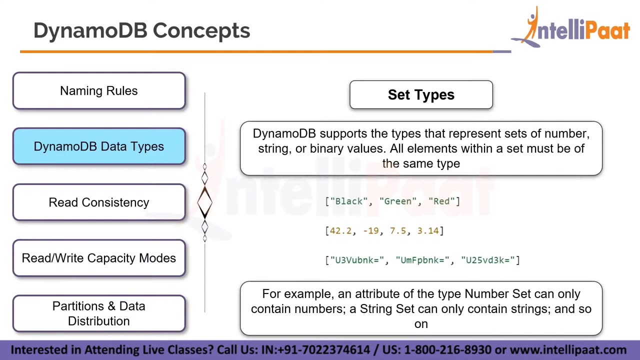 and not a list. but we can have lists somewhere in between as well. so wherever there are square brackets, those are lists, but when they are curly brackets, those are maps. so sets. sets are one other thing that dynamodb supports. so these are sets of numbers, strings or binary values, but with sets the. 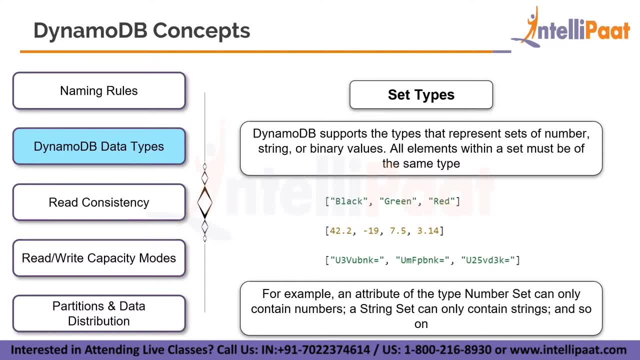 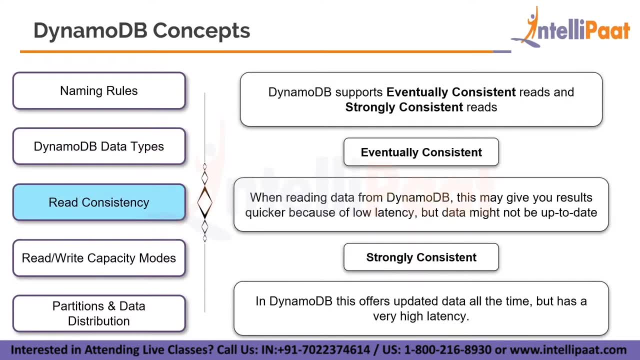 set of numbers, string or binary values, it should be the same. so if it's string, it should be string all throughout. if it's numeric, it should be numeric all throughout. there are two types of consistencies in dynamodb so we can select any of these read consistencies, so the eventually. 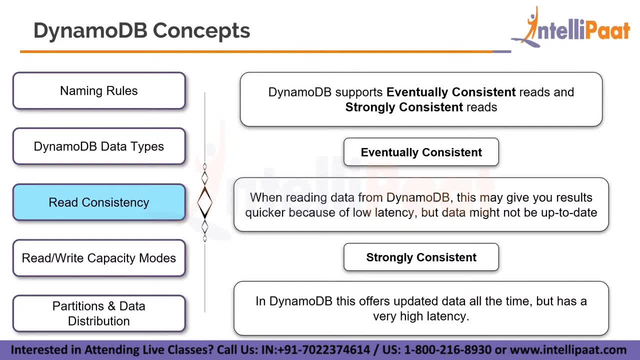 consistent implies that the data is already loaded, so that is why it is accessed with a low latency, but it might not be up to date. so with the current uh data status, but with strongly consistent, the data is loaded upon demand, which means there is a very high. 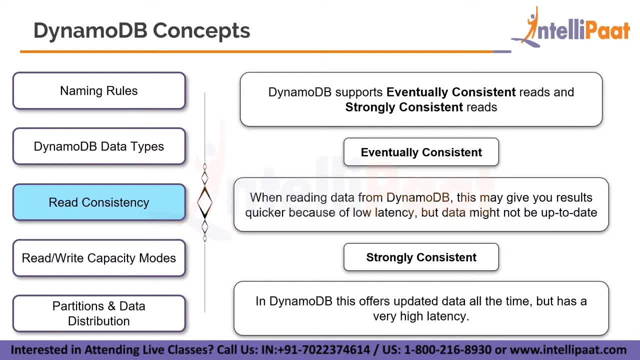 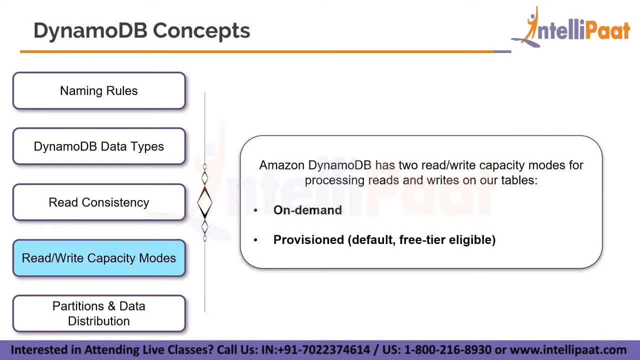 latency, because the data is accessed from the source, but it gives us the updated data, which is the data that is available at the current point in time, all the time. then there are uh capacity modes, the read and write capacity modes. so the first, as we discussed earlier, is on demand, and 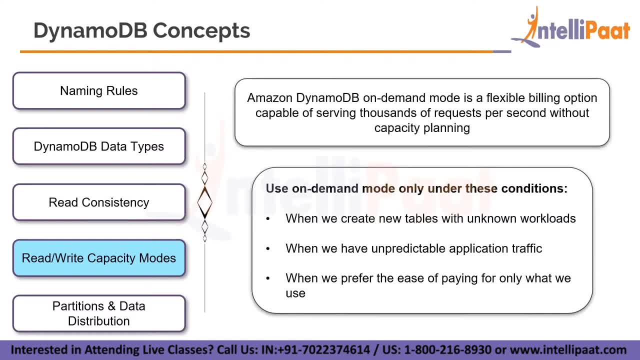 the second is provisioned. so with on demand, you can basically pay for as much as you use, depending on the number of read and write operations that have been performed. so this is used when we have to create tables with unknown amounts of data, when there is unpredictable traffic, application traffic, 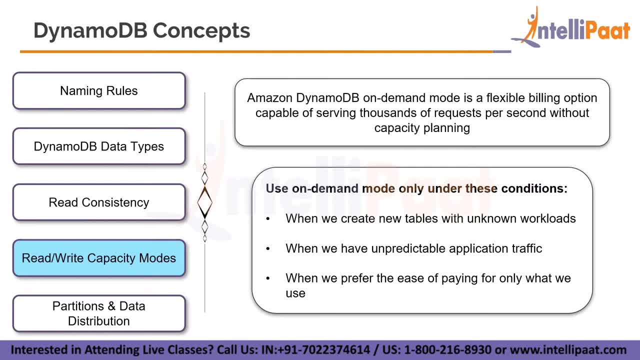 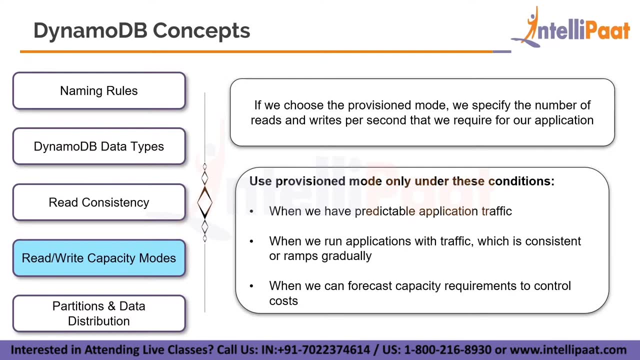 so the data capacity, the data amount is unpredictable and we only want to deal with paying for whatever we are using. we're not pre-allocating resources, we are paying as we are using the service, and then there is provisional. so, uh, in the provision we already know, uh, what is the application traffic? we already have some idea of it, so we 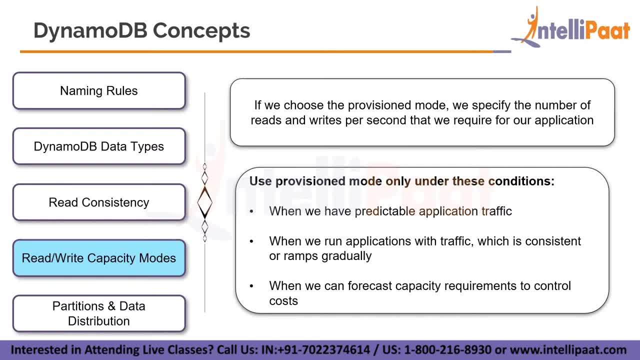 already know how much we have to provision ourselves with and when we run applications with traffic which is consistent or ramps gradually right. so basically we have a model of how the traffic is going to ramp up and whether, when, we can forecast the capacity requirements to control cost. so we can already have the modeling, we already have the idea. 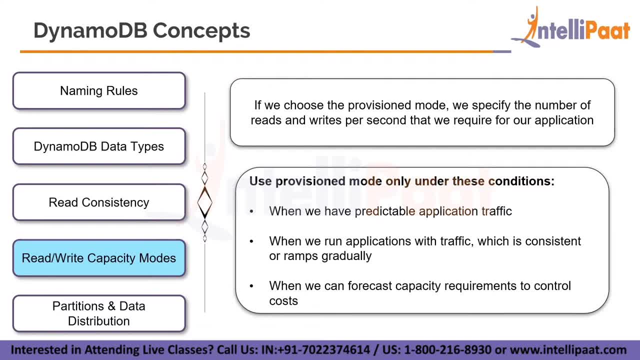 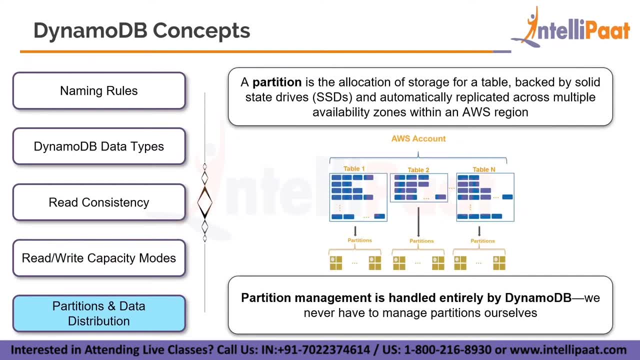 of how much read and write operations we would be performing. so the last concept is a partition. a partition is an allocation of storage for a table backed by ssds, which are solid state drives. so these drives have a much higher performance than normal ebs volume or hard drives. 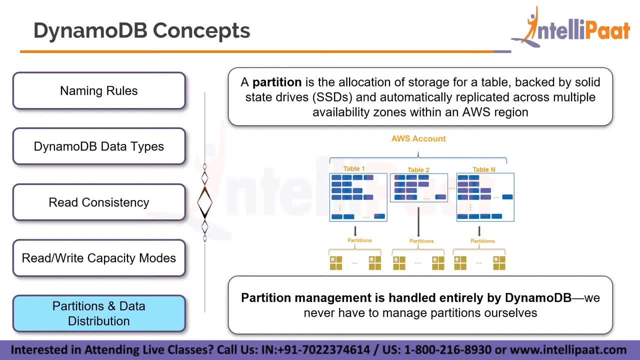 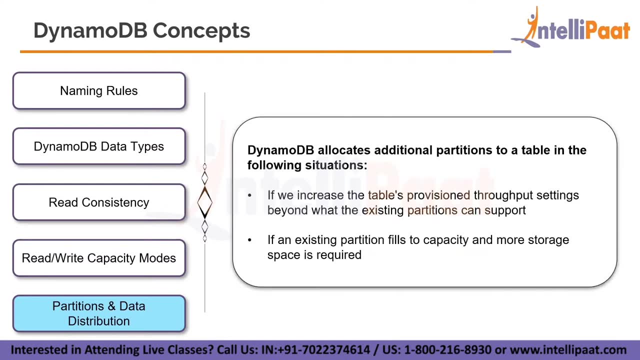 and these are automatically replicated across multiple availability zones within the aws region. so the partitions are also replicated to prevent data loss. the partition management is entirely handled by dynamo db. we don't have to concern ourselves with that. dynamo db also allocates additional partitions to a table in the following situations: 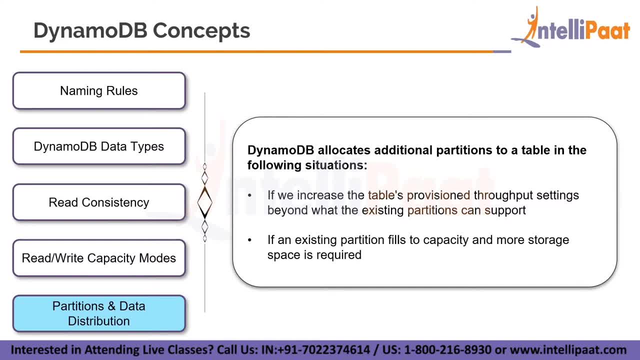 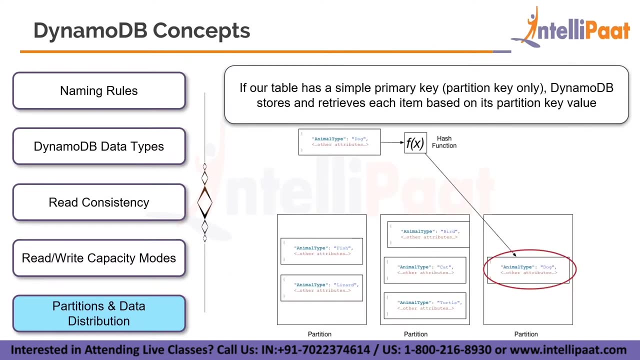 if we increase the table's provision throughput beyond what the existing partitions can already support, or if the existing partition fills to capacity, which means there is no more space left anymore and then there's more storage space required. so, if we look at this, if our table has a simple primary key, which is the partition key, 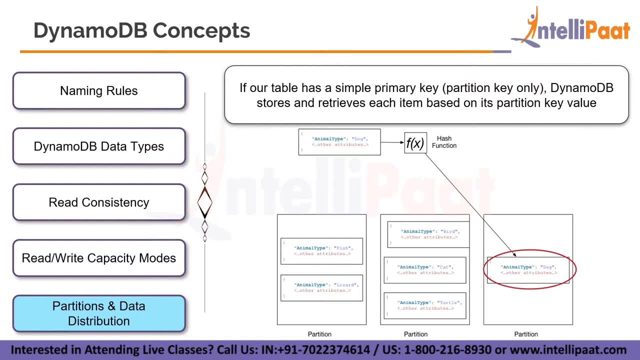 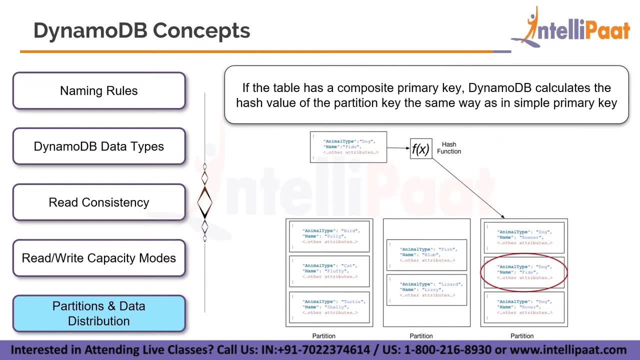 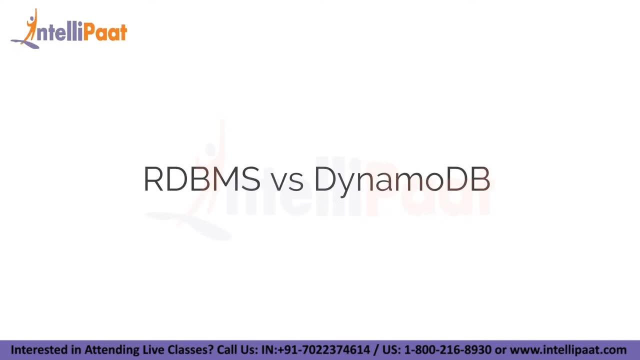 dynamo db stores and retrieves each item based on the partition key value. if it has a composite primary key, dynamo db calculates the hash value corresponding to that partition key and then refers to it after the hash function has been calculated. rdbms versus dynamodb. now let us look at the differences between a. 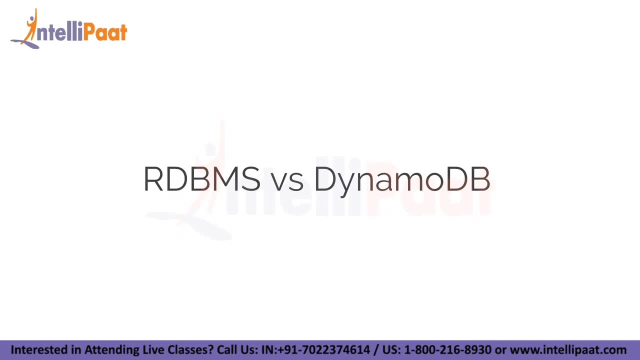 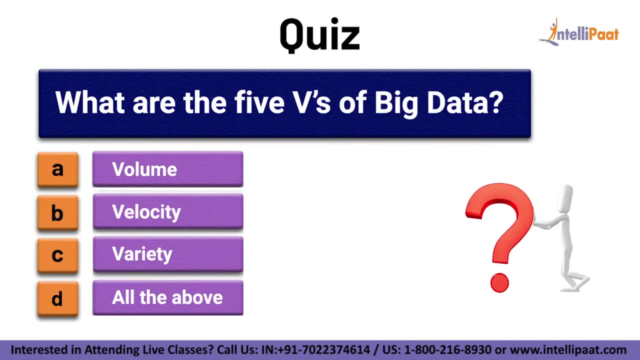 partitioned relational database management system and dynamodb. so, uh, the first is optimal workloads. so just a quick info, guys, test your knowledge of big data by answering this question. what are the five v's of big data? a, volume b, velocity c, variety, d. all of the above comment your answer in the comment box. 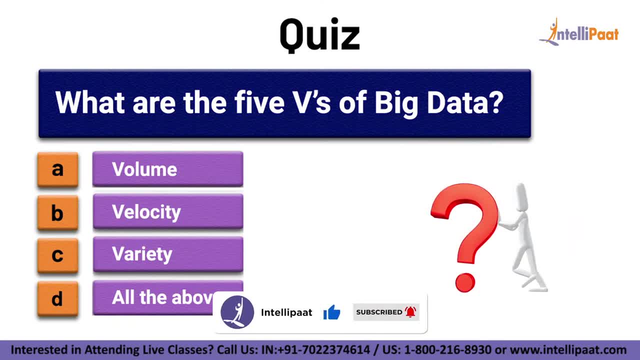 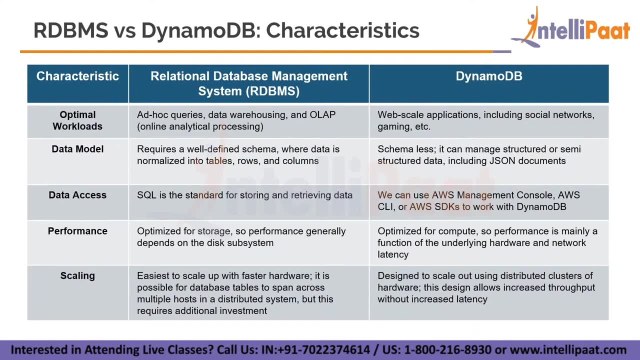 section below: subscribe to intellipaat. know the right answer. now let's continue with the session. uh. data warehousing and OLAP, which is online analytical processing and ad-hoc queries, are the forte of relational database management systems, but with dynamo db we have huge use cases. 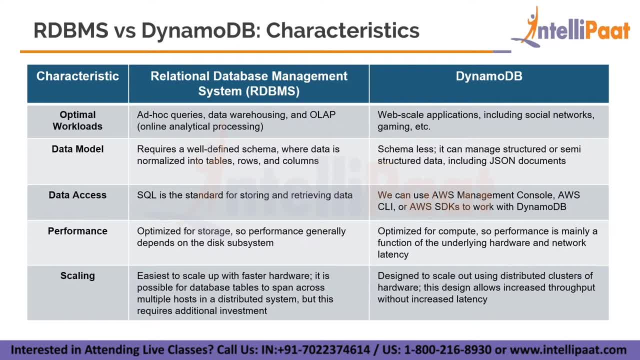 we can basically store information related to web scale applications, which would include social networks in gaming. so two completely different cases of ohs and page. ohs provides a lot of data use cases. with rdbms we are essentially accomplishing data warehousing and olap, while 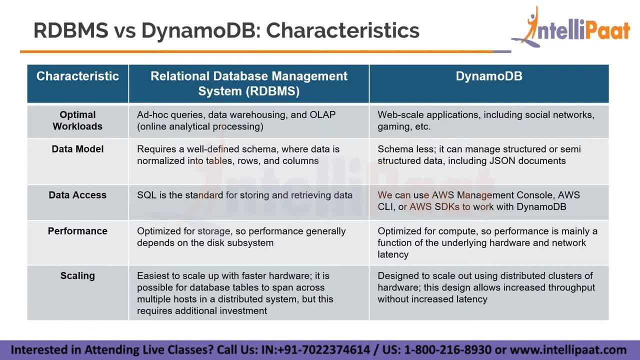 with dynamodb we can basically store all of these huge amounts of data. data model includes that rdbms is obviously corresponding to databases which are very well structured, so it has a very defined schema where data is normalized into table rows and columns, like sql, and dynamodb is schema. 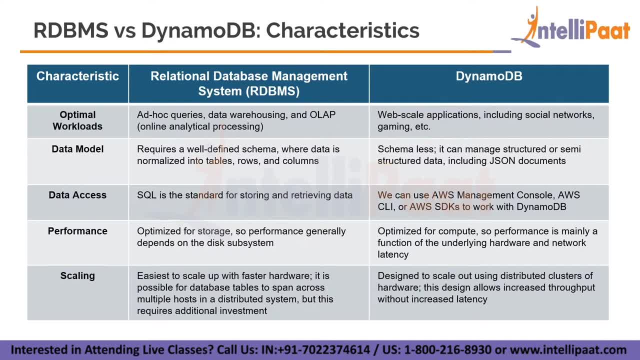 less schema. less is a no sql format which is comprised of json like documents. it can manage structured or semi-structured data. in that regard, data access sql is the standard of storing and retrieving data. when it comes to rdbms, mysql, if you use this oracle, db and such so on and so forth. 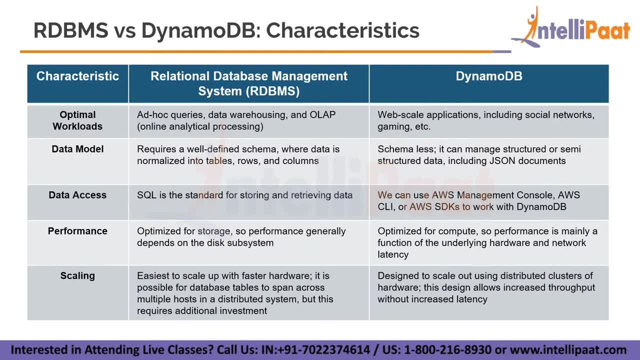 and with dynamodb we can use the aws management console or the aws cli or even the software development kits provided by aws itself to access elements within dynamodb. the performance. so rdbms is optimized for storage, so it depends on the computer configuration that you have. that basically evaluates the performance that 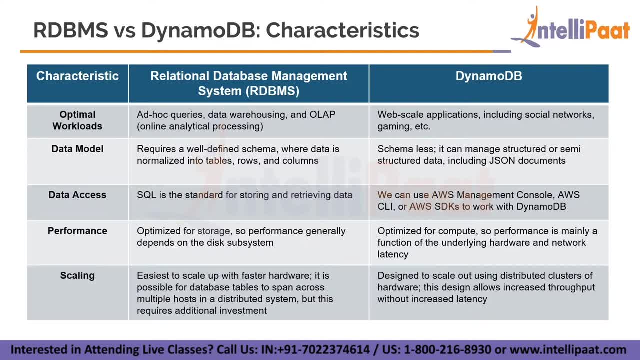 your relational database management system will perform at and dynamodb. it is optimized for computation. it's not optimized for storage. so performance is a focus in dynamodb. so it uses the underlying hardware and network latency. and those are the main focuses when we are dealing with dynamodb. scaling: you can scale up the rdbms when you have faster hardware. it is also possible. 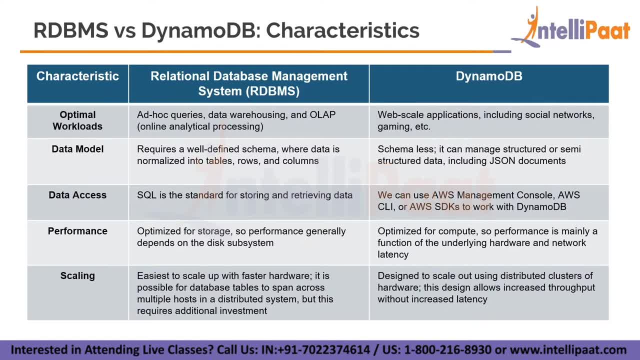 for database tables to span across multiple hosts in a distributed file system but it requires a lot of maintenance fees and additional investment to actually make that synchronization. but with dynamodb and it is designed to scale up or down on distributed clusters of hardware based on the use case. that 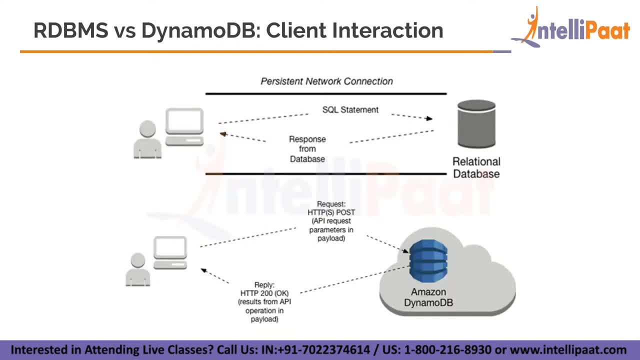 you may have. so we can see the differences in the workflow here. so there's a persistent network connection. when we are dealing with the relational database, we as a client put in an sql statement and the database gives us the response. but uh, when we are dealing with amazon dynamodb, we can simply put: 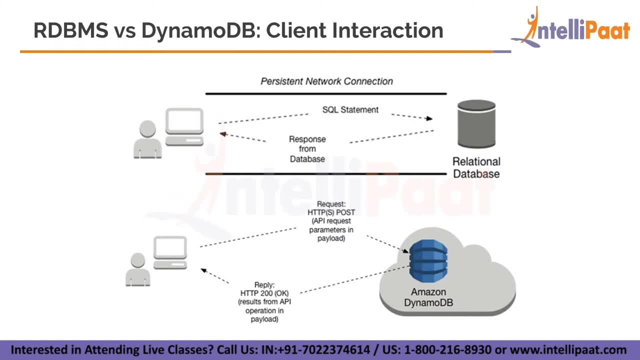 in a web request while we are using the aws dashboard and you can see that we have a lot of. when the request goes into the DB, it gives us the result back and the comparison models. when they're dealing with a large amount of data in a relational database, you would have to invest a lot for hard drive space. you 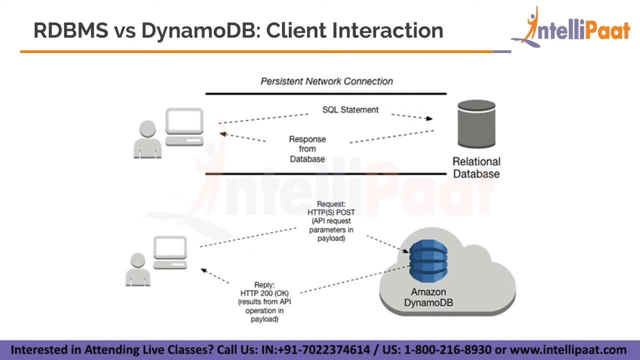 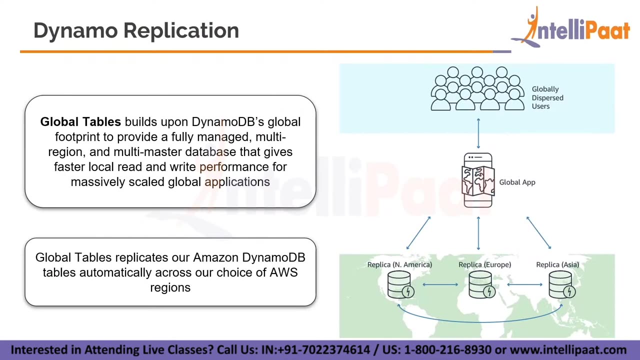 would have to invest a lot of computational elements, but with Dynamo DB you only have to, in most cases, pay for what you use and it computes things really fast. Dynamo replication- so, as we discussed before, there is global automated replication- and Dynamo DB, so there are global tables that are built. 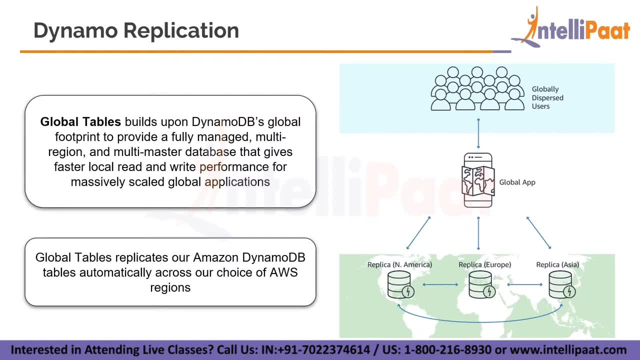 upon Dynamo DB's global footprint to provide a fully managed multi region and multi master database that gives faster local read and write performances for massively scaled global applications. so the availability of global tables allows us to enforce replication of data so we can replicate these tables across various 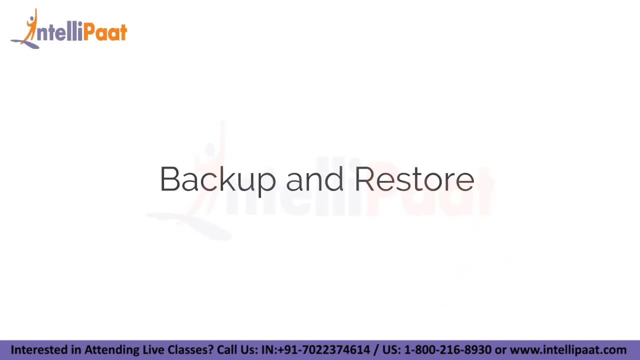 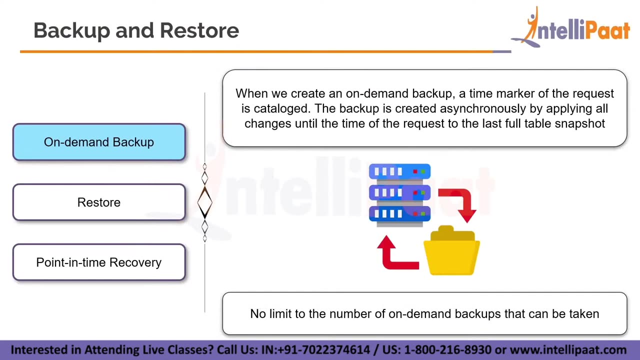 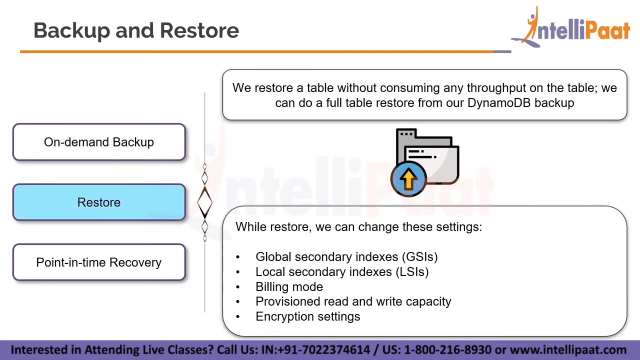 AWS regions for faster access, all the data that is in our source distribution. so, as we are referring to today, we have this package, we can have this another configuration and you can also have this: a multi standard backup for past dashboards, a multi standard backup to any throughput on the table. we can do a full table, restore that DynamoDB backup. 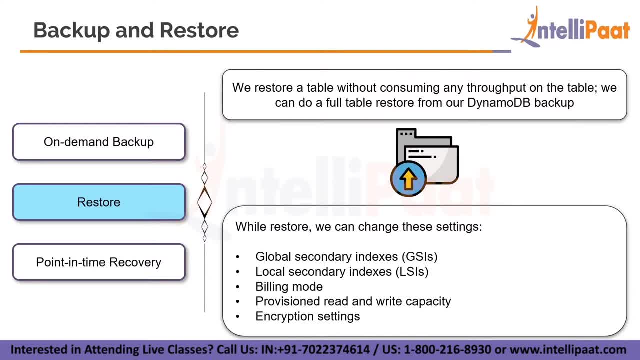 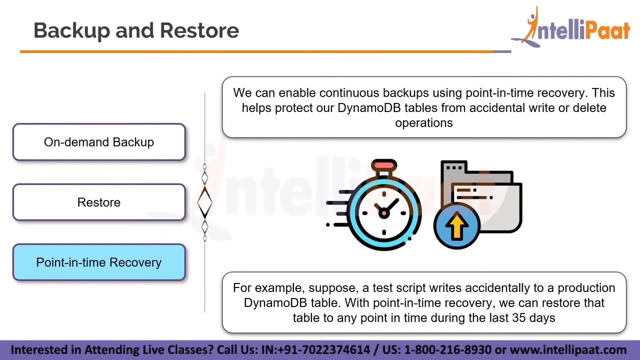 so while restoring, we can change the following settings: global secondary indexes, local secondary indexes, the billing mode, the provision read and write capacity, the encryption settings of the table. and then there's point in time recovery. we can enable continuous backups using point in time recovery, so AWS will automatically enable snapshotting of the database at points. 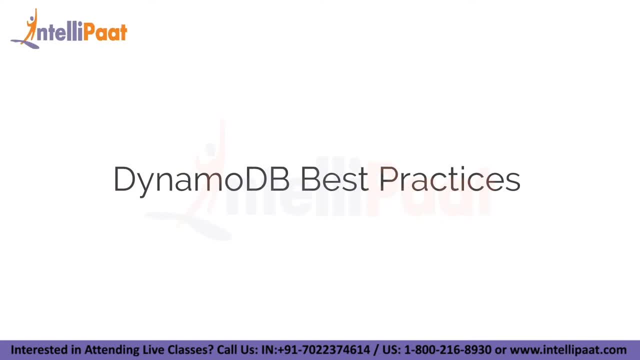 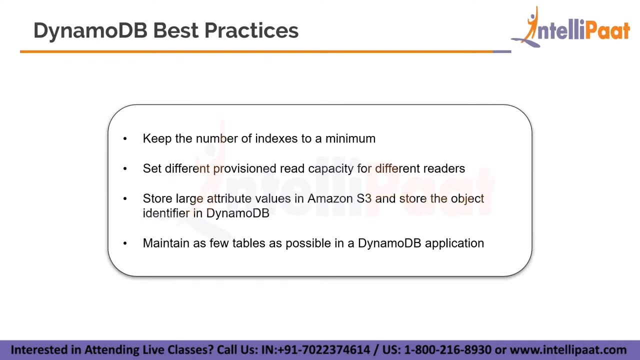 in time. so there are certain practices that you could follow when using DynamoDB. keep the number of indexes to a minimum. you don't want a large number of indexes. send different provision to read capacity for different readers. so, based on the role of the reader of the DynamoDB database that you have, you can 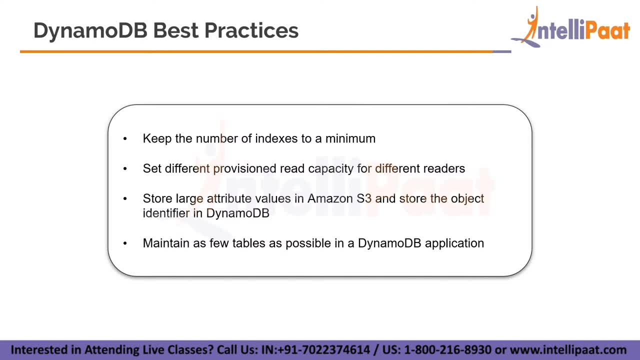 set up different provisionings and you can store large attribute values in Amazon s3. so say, if you have an extremely large value and store that in s3 and simply point to that value using an identifier in DynamoDB. maintain as few tables as possible in a DynamoDB application, so you want to minimize the 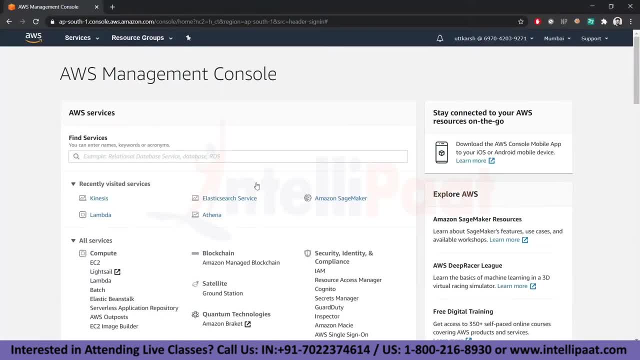 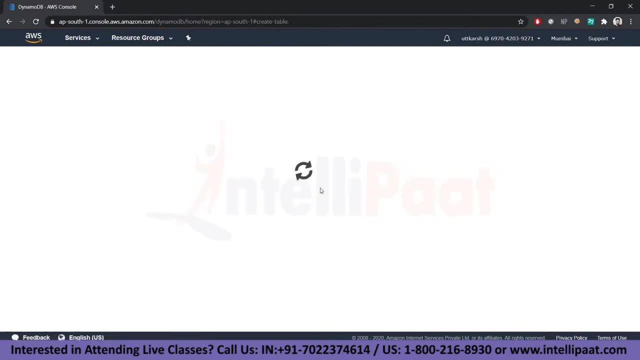 number of tables that you use for convenience. so let us create a table in DynamoDB. so simply type in DynamoDB for that and when up the service so it very conveniently gives you the option to create a table. just click on that and then you can name the table anything that you would like. so let us name this. 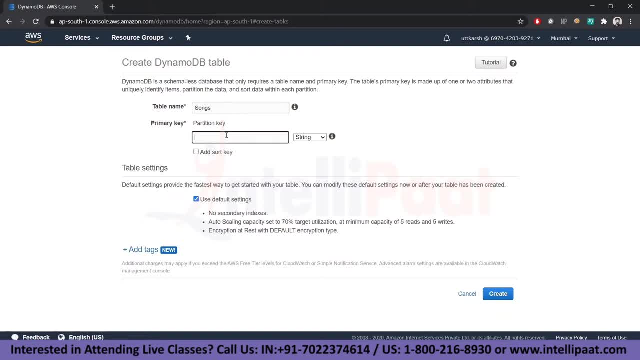 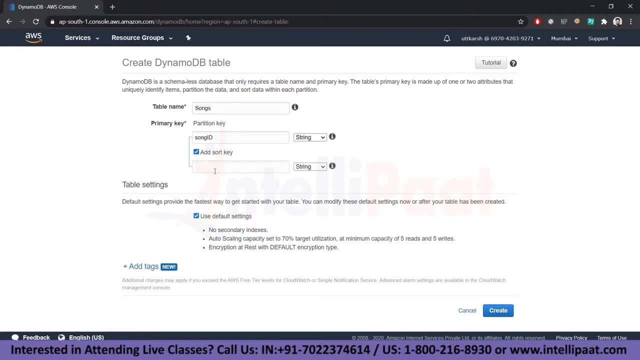 songs and the primary key could be the song ID, so we can name it that and we can also add a sort key, so this could be the album name, maybe the artist ID or the album name, and we can change the song ID to a number. simply click on create. 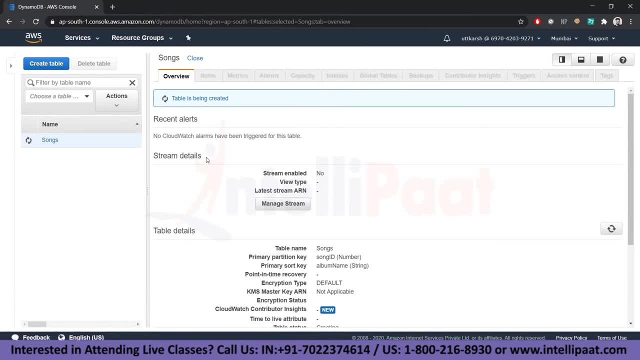 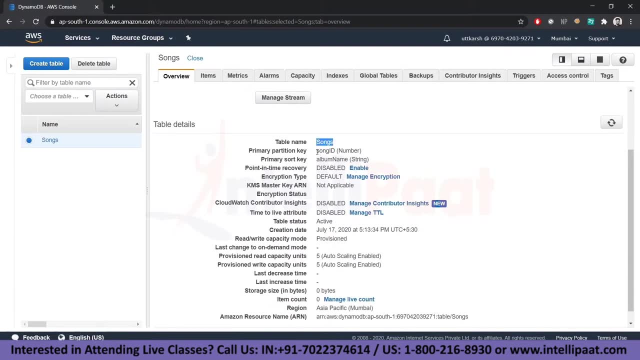 so it will take some time but the table will be created. so we've successfully created our table. so the table name is songs. the primary partition key is the song ID, which is a number, and the primary sort key is the album name, which is a string. so now that we've created our table, we can load some data into it. 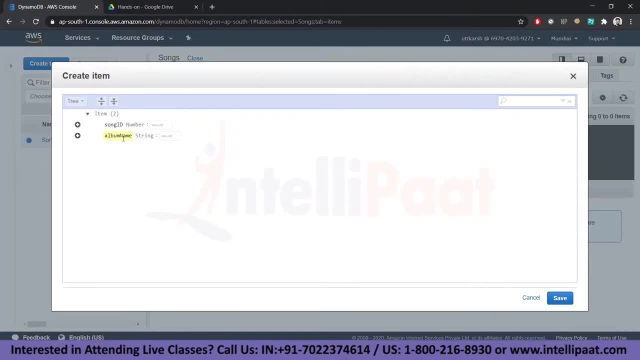 so click on items and we'll create an item. so this is the template that is there available for us. so song ID is the partition key and then we can add the, and album name is the start key, so we can simply add another if we want. so click on append after. 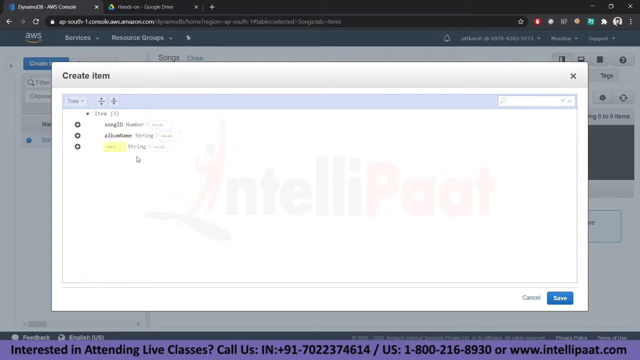 clicking on the plus sign and click on string, so we can add another element which is artist. and we can add another element as well and call this song name, and then we can give some numbers to it, so the song id could be one, the album name could be xyz. artist could be new artist. 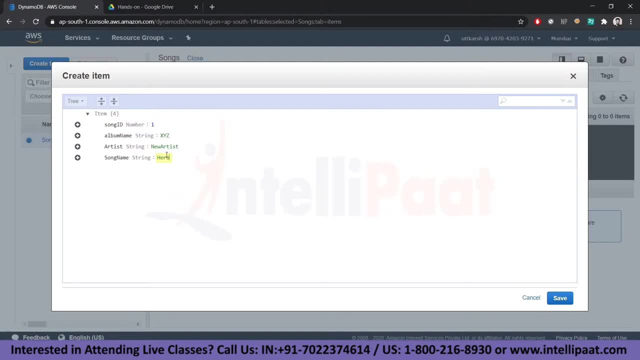 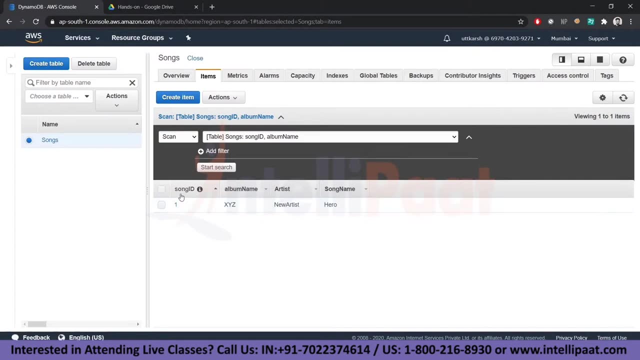 and the song name could be hero. so this is a sample or data record and we save that and we'll create a table, like structure which we can, where we can see the song id is the partition key with one, and then there's album name, and then there's the artist and then there's the song. 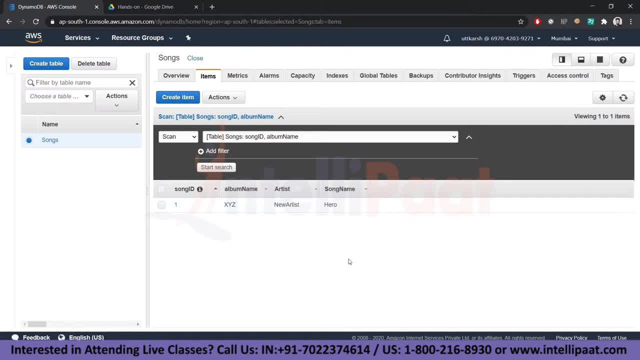 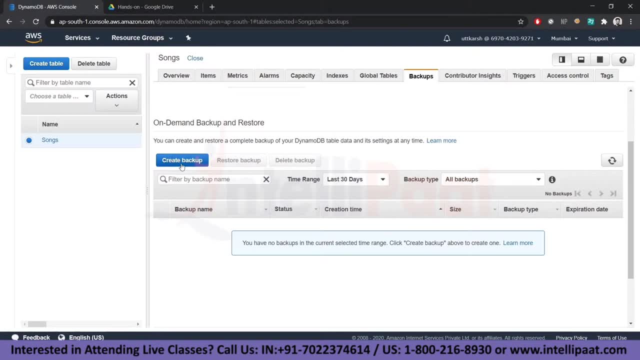 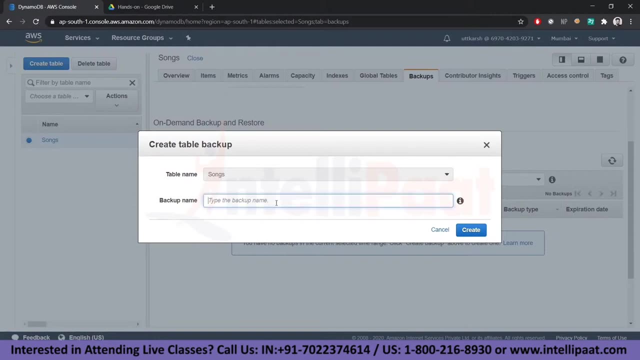 name. so we can do that in this regard also, so we can also create backups of these tables. if we simply go over to the backup section and we have our create backup option, we'll click on that. so the table that we have to backup is already selected. there are no other options and we can. 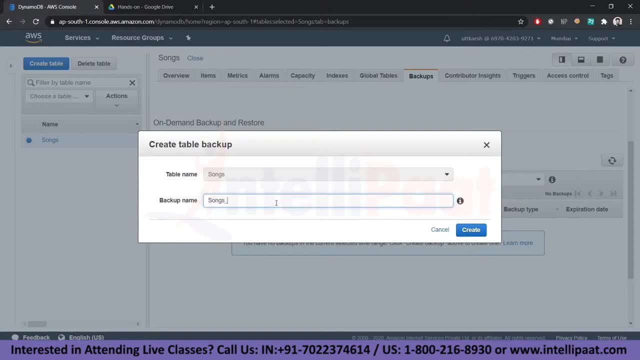 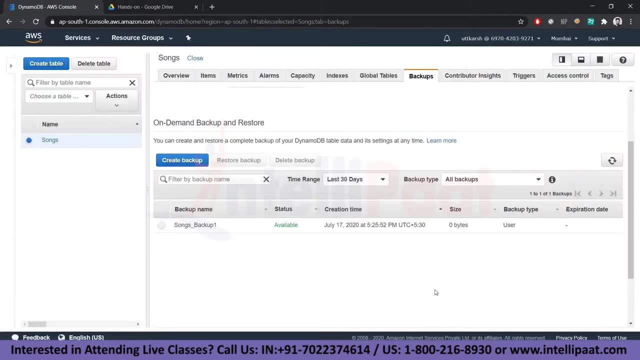 name this anything that we want the backup, so songs underscore, backup one and then simply click on create so the backup request is successful. so, depending on the table size, it will take some time and the table will be backed up. so in my case the table was really small so it backed up almost. 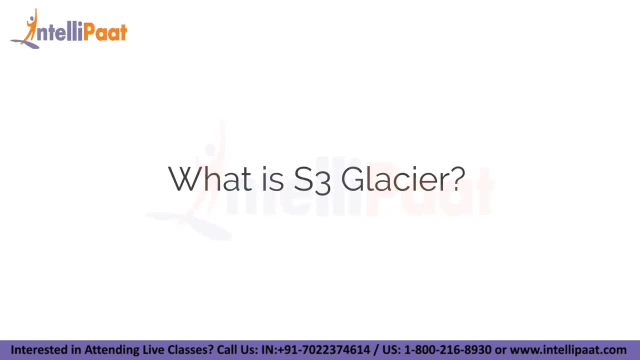 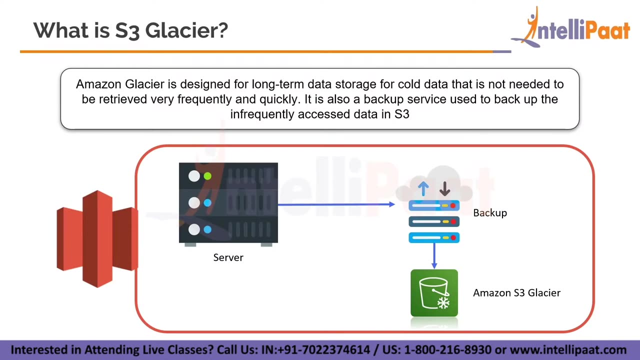 instantly. so here we have our backup. what is s3 glacier? so s3 glacier has been designed for long-term data storage, which means it is used to store data that we don't need frequent and quick access to. the most common use case for using s3 glacier is to store backup databases. so, say you. 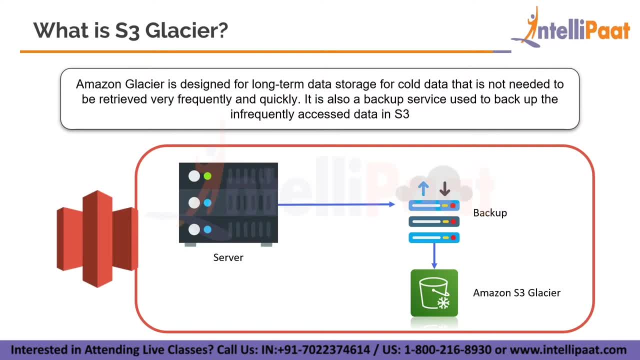 have any server for that matter- and it initiates a backup of the database that it is attached to. so the backup is then transmitted into s3 glacier, where it is stored until further requirement. so, since the backup is not something that we need frequent access to, we only need access to the. 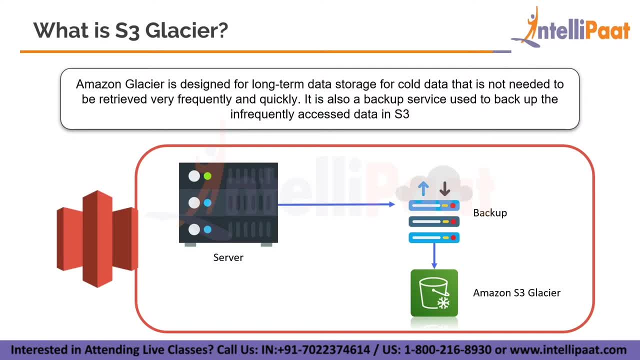 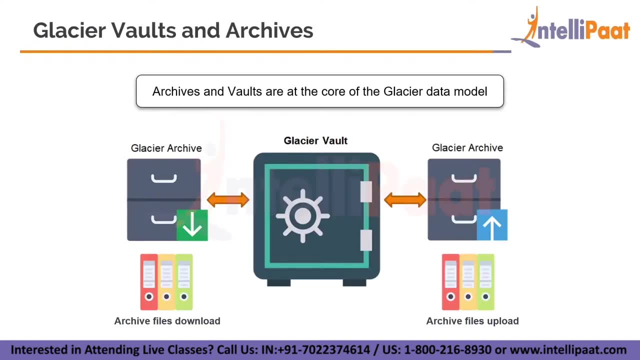 backup when something goes terribly wrong. so that is why it is stored in s3 glacier, glacier vaults and archives. so there are two building blocks for glaciers. so when we are uploading the data to the s3 glacier, we create an archive of that data, so an 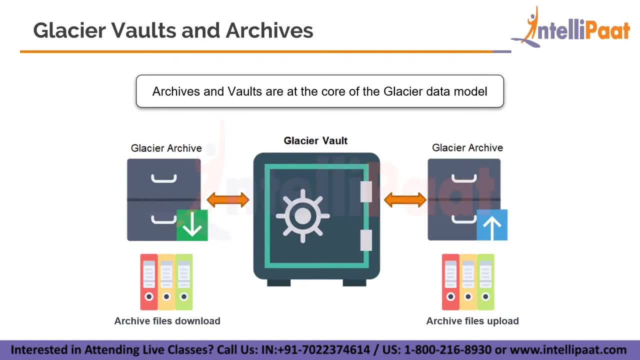 archive is a compressed format, a compressed version of that data, and it is then put into the glacier vault. we can put in a request later on to retrieve that data. so the glacier vault basically gives us that archive and it is then decompressed, be encrypted for us to get the data that we originally. 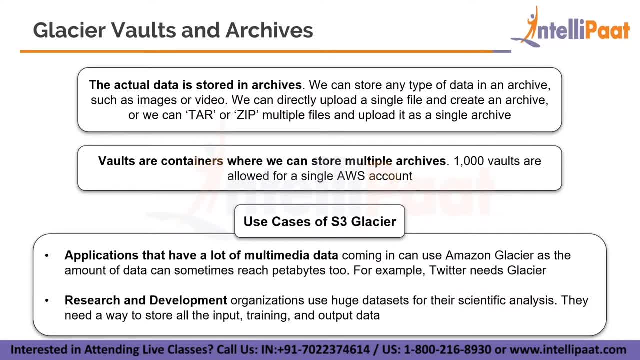 required. so the actual data that is stored in the archives is in a compressed format so we can directly upload a single file or create an archive. we can tar or zip multiple files and upload it as a single archive. vaults are containers where these archives are stored. thousand vaults are allowed per aws account. 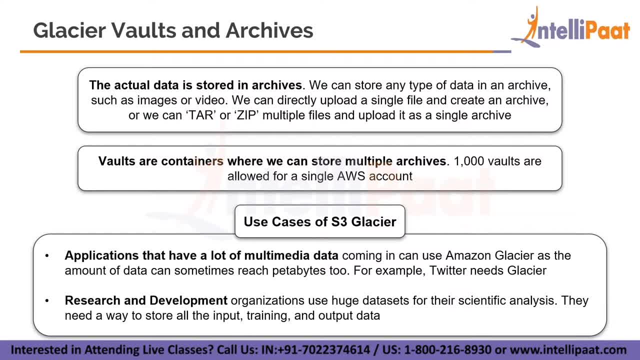 the use cases for s3 glacier: applications that generate a lot of multimedia data, which means images, movies, videos, anything multimedia- and these data sets can reach petabytes at times and we need to be able to compress them and use it, put them in a very manageable space. 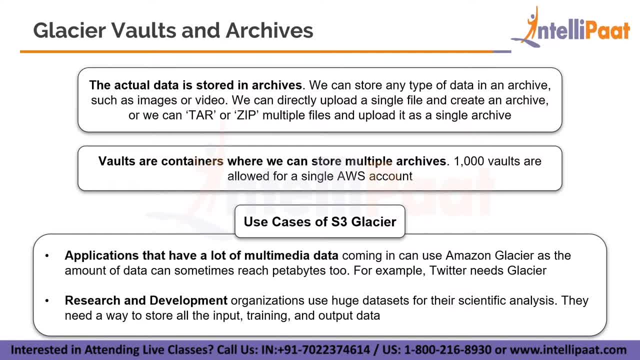 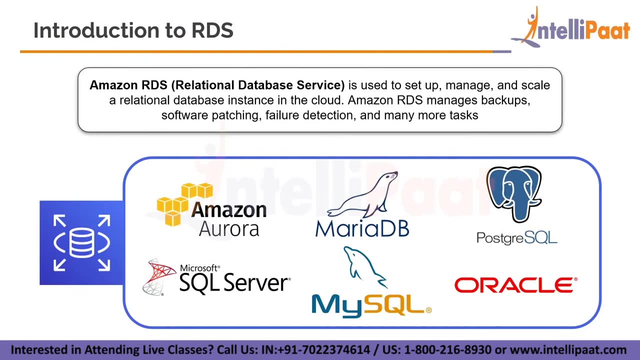 for them to be stored. so that is why we use s3 glacier and for research and development, because they have very huge data sets for their scientific analysis. they also need to store that data. lastly, amazon also provides you with rds, which is a relational database service, fully managed, fully. 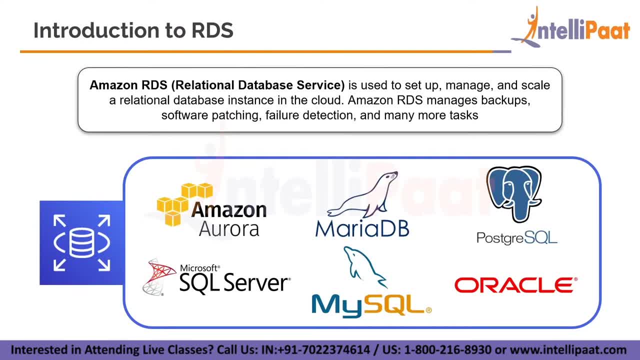 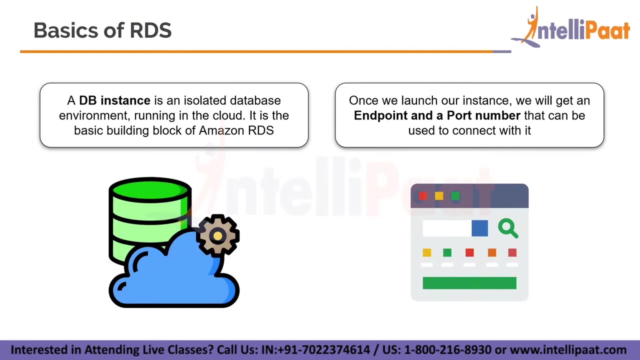 available, provided to you by amazon, and you can manage backups, software patching, failure detection and many more tasks. so some of these logos might be familiar to you: microsoft, sql server, mysql, oracle, postgre sql, maria tv and amazon aurora. so the basics of rds. a db instance is an isolated database. 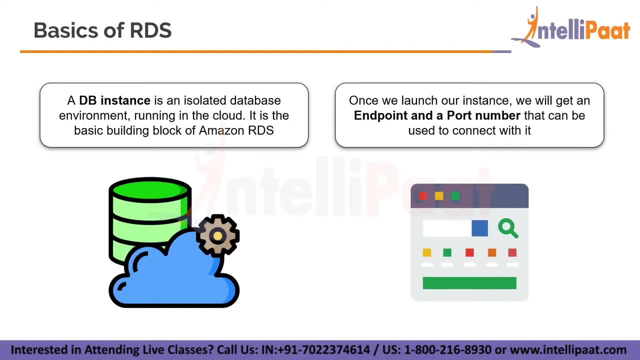 it is running in the cloud and this is the basic building block of amazon rds. this is what you would connect to and you would use certain credentials, which are the end point and the port number, to connect to that particular database. now let's start over the first topic. 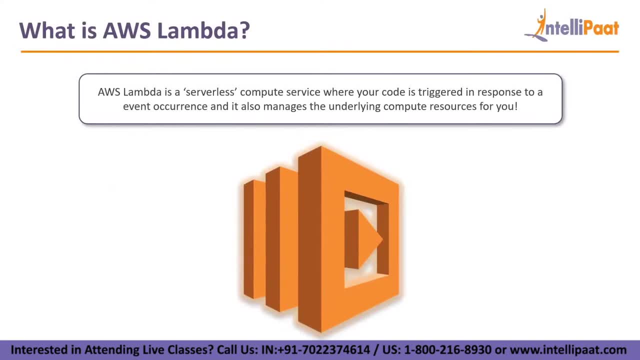 which is what is aws lambda. so aws lambda is a compute service, but it is a serverless compute service where your code is triggered in response to an event occurrence and it also manages the underlying compute resources for you. it is basically a compute service to which you need to provide any information regarding the operating system, regarding how much of ram you need. 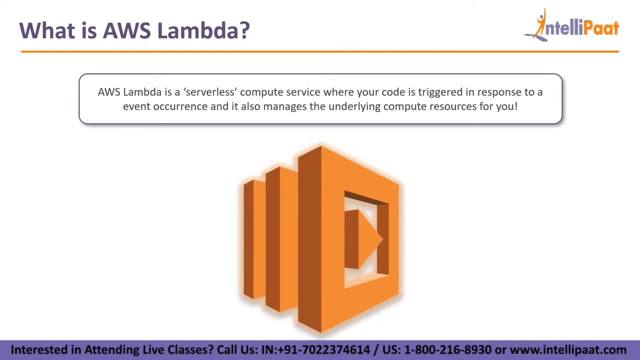 how much storage. you need nothing, so you just have to specify what runtime you want your code to run it. so you can choose either nodejs you can choose, java, phd, python you can choose that, but you don't need to provide anything else. you just have to put your code in there and either you'll have to run it. 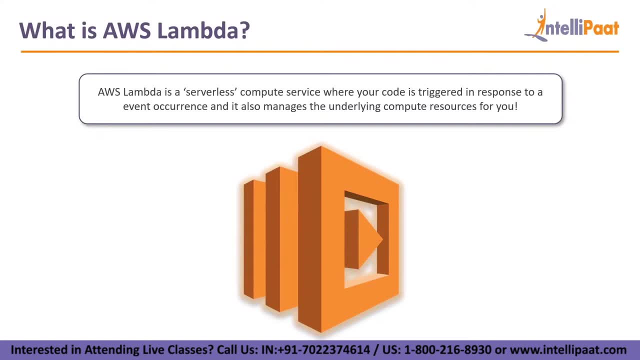 manually, or you'll have to set up a trigger which will automatically run the code for you and also manages the underlying compute resources. because even though you don't provision or you you don't mention any compute resources, you need obviously the uh, the lambda function which you create. 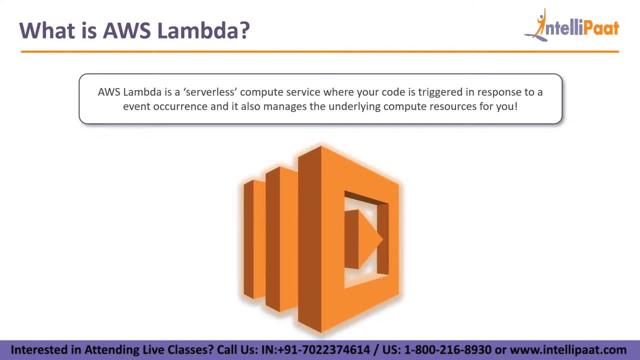 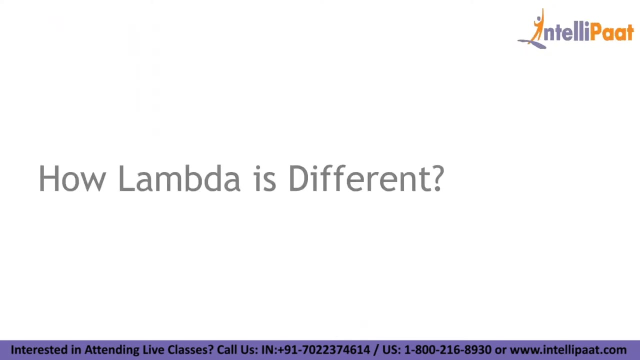 should run on some server somewhere in the adb data center, and all of that is managed by lambda itself. so, basically, it provisions a server or it provisions a location in which it runs the code for itself, so you don't need to worry about anything else. okay, so now how? 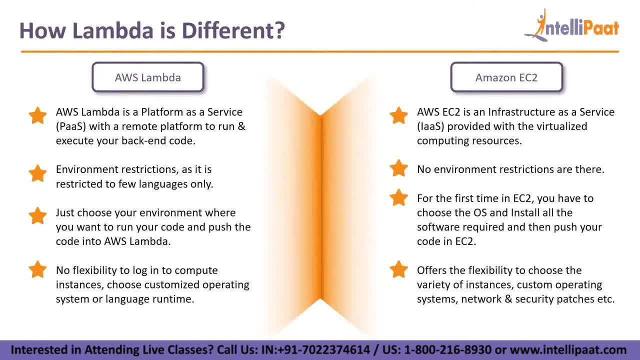 it is different from ec2 because in amazon ec2 we have so many other features which we don't have in lambda. so what exactly is the purpose of lambda here? the aws? lambda is a pass with a remote platform to run and execute your backend code. so basically, they provide you a website in which you 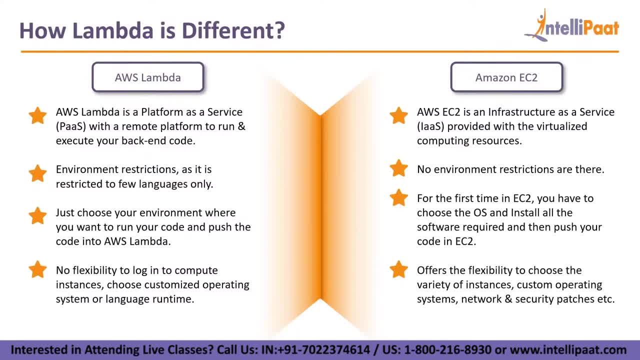 put your code and you run it on your desired platform or desired runtime. in amazon ec2, it's an infrastructure as a service in which you are provided with virtualized computing resources, which is hosted in the aws data center. so in this case, it's a website which is, which is obviously hosted. 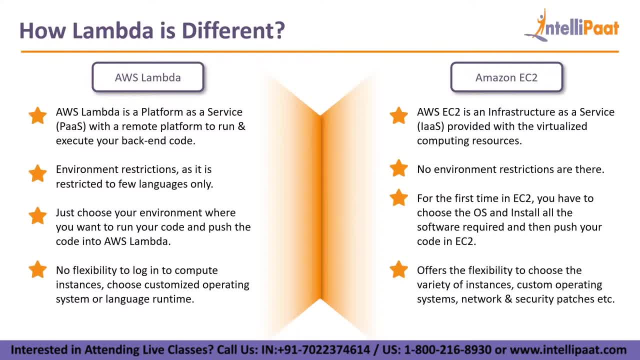 in the aws data center, which provides you access to the lambda tool in which you can run your code according to a certain trigger. but in this case, in lambda's case, you won't give, you won't be given access to the server itself, but in the ec2 part, you will be given access to the server completely. 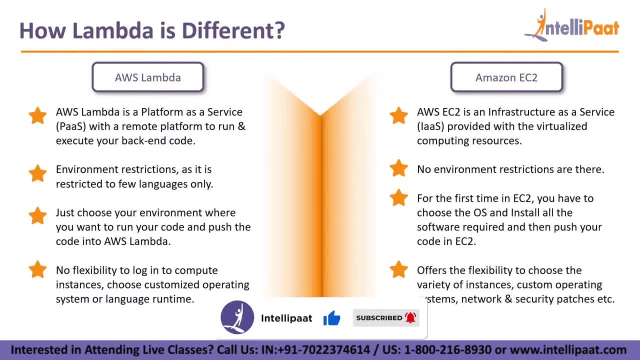 you can install any software you need. you can install whatever you want. you can upload certain images to it or you can upload certain code files to it and you can manually run it from there. but in lambda it is just a website in which you are uploading your code. then environment restrictions, as it is restricted to a few languages only. 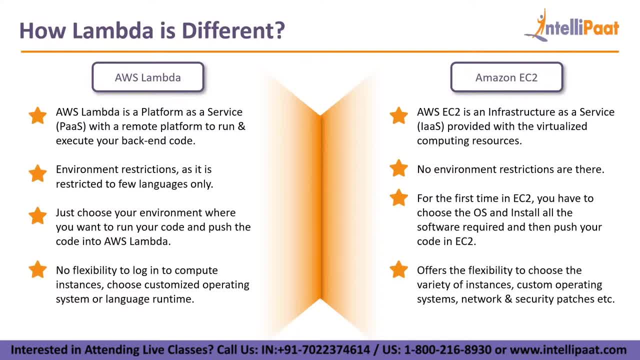 so in aws lambda. so there are some pre-loaded language runtimes which are the only languages which you can use. but in ec2 there is no restrictions because it is a virtual machine. you can install any software you want according to your needs. just choose your environment where you want to. 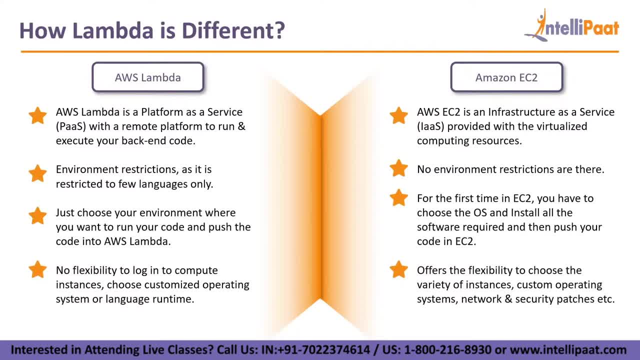 run your code and push the code into the lambda. so basically in lambda you just create the function, choose your runtime, push your code ec2. so you'll have to basically choose the operating system, which is the ami, and once you choose the ami, you'll have to log in into the ec2 instance and 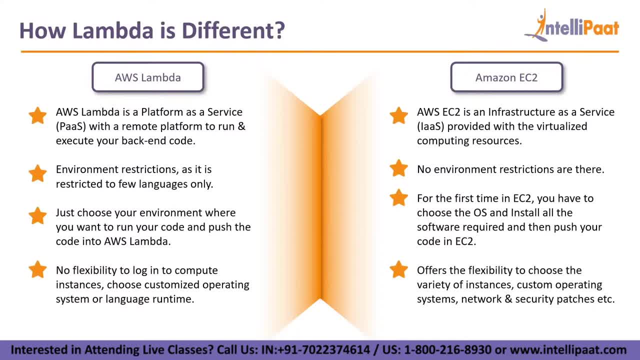 install all the software. only then you can get to the process of running your code. no flexibility to log into computer instances from customised operating systems or language runtime offers the flexibility to do that with various of instances, operating systems, network and security badges. so this may be one of the 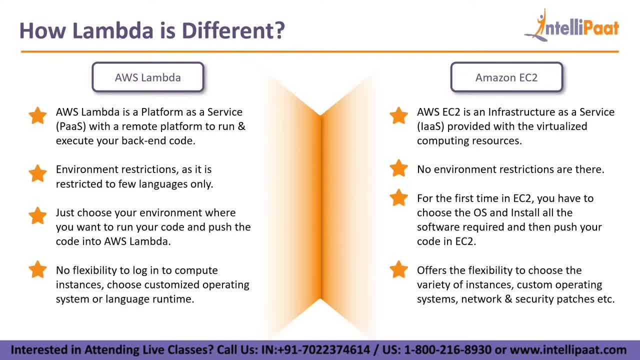 disadvantages of lambda. so in lambda there is no flexibility. basically you cannot log into the provisioned server and then rectify if there are any errors. but in ec2 you can do that because it is your serverこのι فedocio з. these are the main differences, guys. so one of 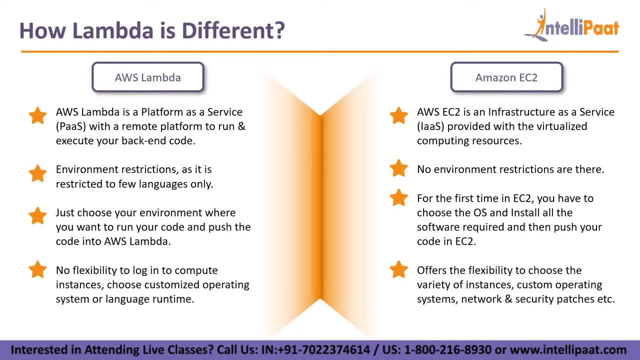 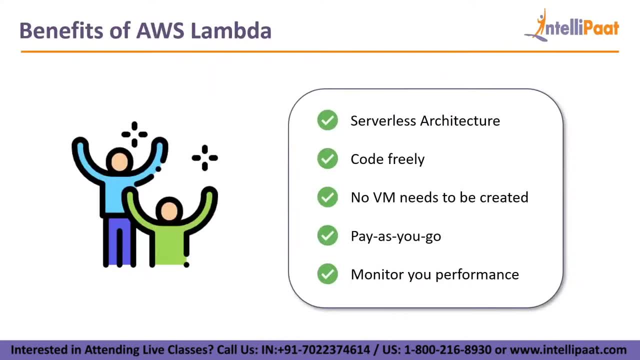 The main difference is it is serverless and EC2 is a server which is provided to you. Lambda is a platform which is provided to you. So what are the benefits? First of all, it's serverless architecture. Let's say you don't want to maintain the architecture, you just want to write a good code which you 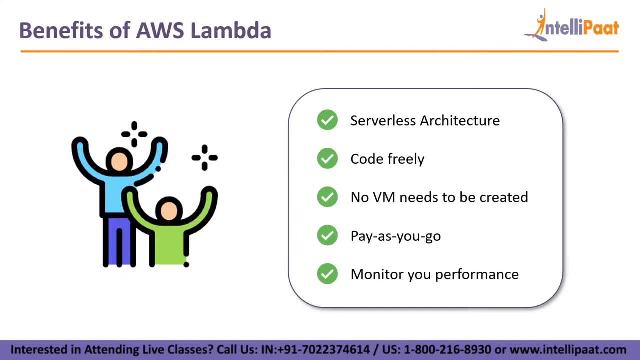 want to write a good program which you want to run, So in that case you don't need to worry about anything else. You can just use Lambda, which will give you a serverless architecture automatically and you can run your code on it. 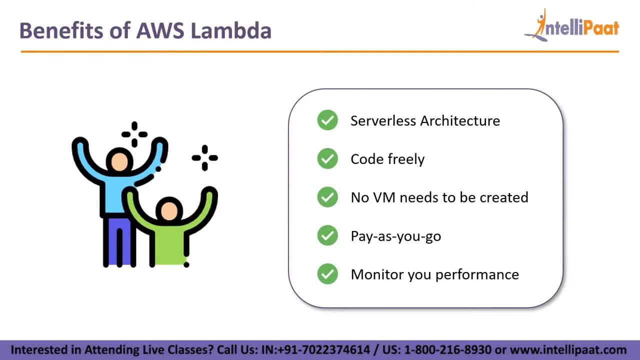 Code freely. you have a text editor or you have a code editor on the Lambda console itself. You can code over there and also it'll accept. you can basically choose the version of your runtime and you can change your code according to that. No VM needs to be created. 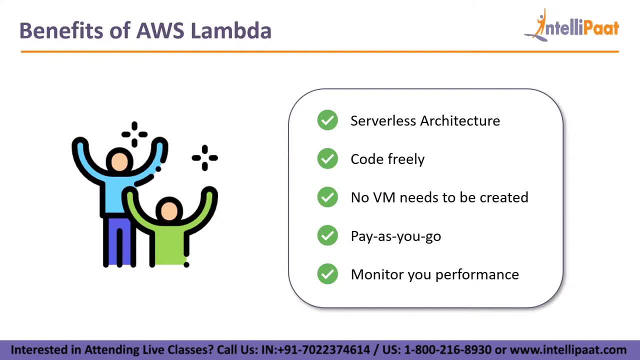 So, again, we know about this. We don't need to create a virtual machine, We just have to create the function Pay as you go. This is for every single AWS service. You pay for what you use. If you use, let's say, two EC2 instances, you only pay for the two EC2 instances. 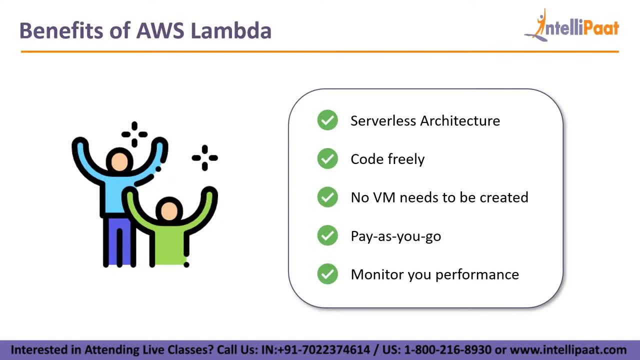 If they are stopped or if they are terminated, you're not going to pay for them anymore. Monitor your performance. A monitoring tab is always available in Lambda, which is in real time. you can go ahead and check whenever there is a change in that particular tab. 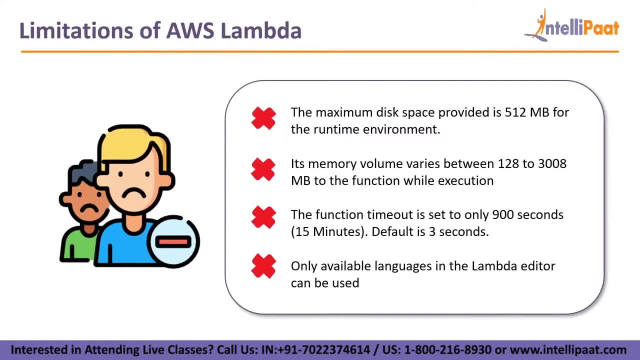 So now, what are the limitations to Lambda? So, as I told you, it's not a server, because it provisions everything for you. So if it does that, you cannot do all the tasks right. So in that case, whenever it is a platform as a service, there are all ways to do it. 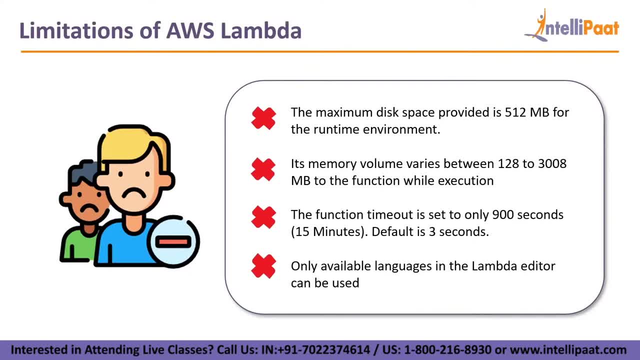 So in that case, whenever it is a platform as a service, there are all ways to do it. So, in that case, whenever it is a platform as a service, there are all ways to do it. So if it is a server, there is no limitation. you can use the complete server as much as. 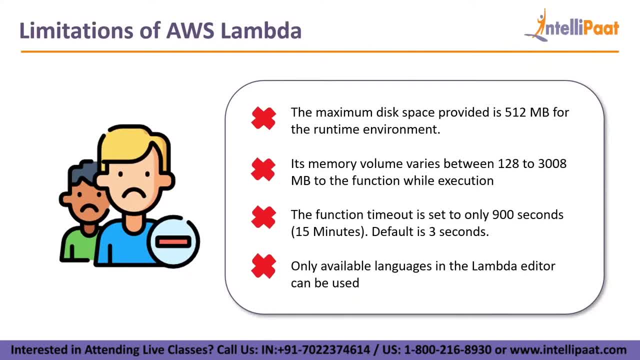 you want, however you want, But in in an environment like Lambda, you have certain limitations which you will have to abide to. If you go ahead of that, your function will not work. So now, the maximum disk space provided is 512MB for the runtime environment. 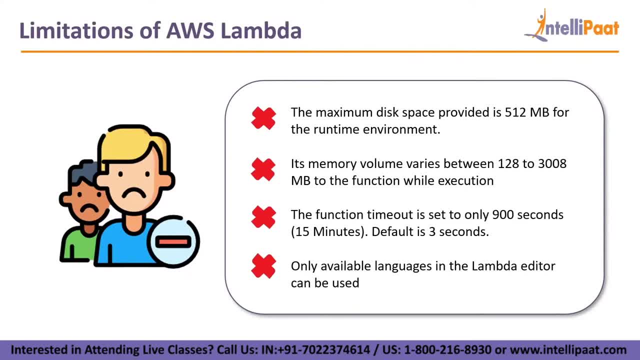 If you want to store certain temporary files while the function is running, then to get 512MB should save a bit more time. If you want to store some temporary files while the function is running, then at least mb for the runtime environment. so right now there is a new feature where you can attach an efs volume. 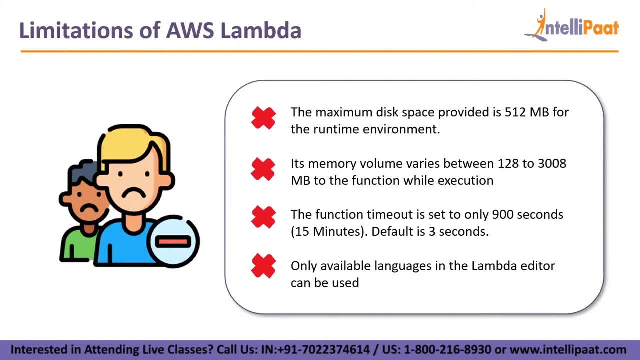 to lambda. so right now i think there is no issue. you can just create a huge efs volume and attach it to lambda to store all your temporary files. but if you don't want to use efs, you just want to use lambda. in that case you get 512 mb. its memory volume varies between 128 to 3008 mb. 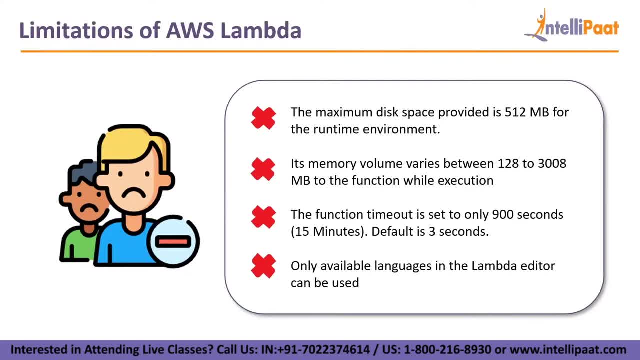 the function while execution. so while creating a lambda function, you can also vary the memory which you want to which that particular program has to be using. so let's say the minimum would be 128 whenever you create a lambda function. that would be the minimum. you can change it up to 3008. 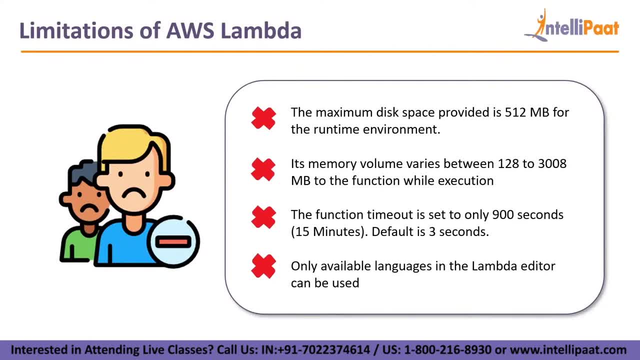 mb. so now, if your lambda function, if you think your lambda function requires a lot of memory to run, in that case you will have to run certain times, do some trial and trial and error and check how much mb your lambda function is using and then come to an average value. so let's say you run your function three times, it's using 200, 201 and 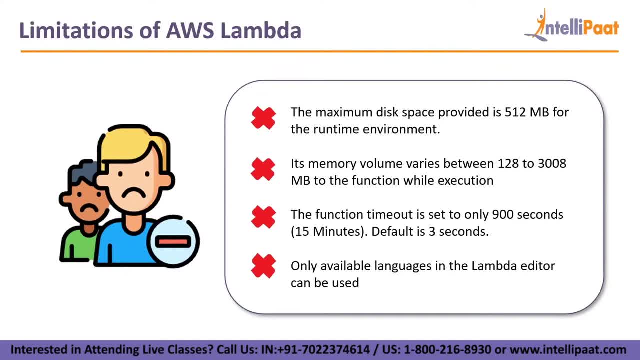 195 mb, so you can give around 220 to 230 mb of memory so that it does not like fail. and then function timeout is set to only 900 seconds. that is, if your lambda function is running for more than 900 seconds it will abruptly stop. the maximum function runtime is 900 seconds. if it, it cannot go beyond that. but 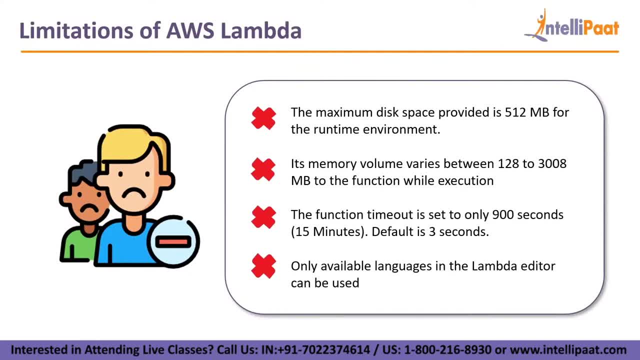 i don't think any code will run more than 900 seconds, whichever you put on lambda. so make sure your code does not take more than 900 seconds. also, the default is three seconds. you can make it lesser as well, but whenever you create around the function, the default timeout period is three. 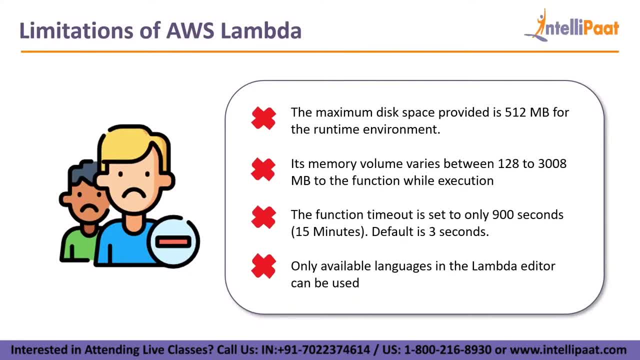 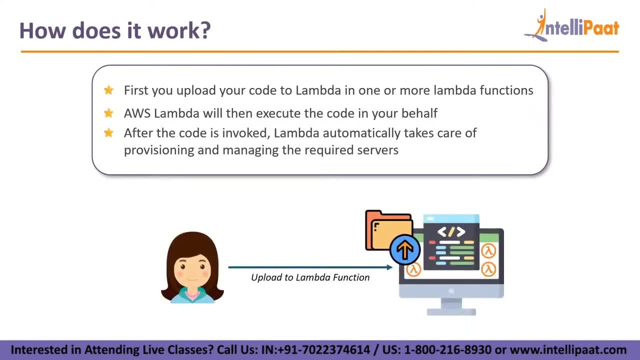 seconds, only language is available and the lambda editor can be used. so this will be the default we already discussed. now how does it work? first, you upload your code to lambda in one or more lambda functions, so you create a lambda function, or you create multiple lambda functions and you 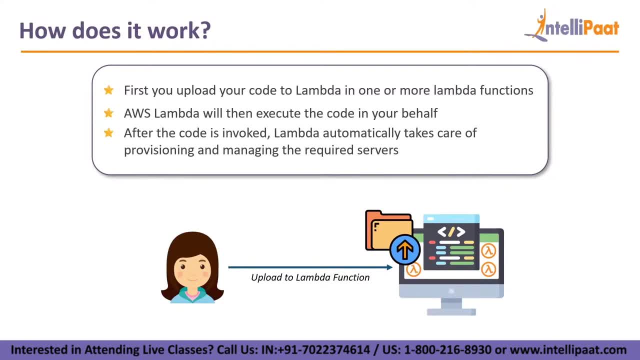 upload or copy and paste it code to lambda. once that is done, once you set up a trigger, then the trigger is triggered, obviously, and once that is done, the lambda function will start executing. if your code executes successfully, in that case, all well, all good. if it does not, then there is no use to that particular function. 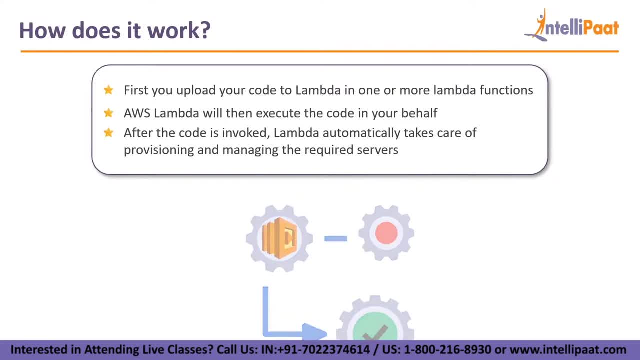 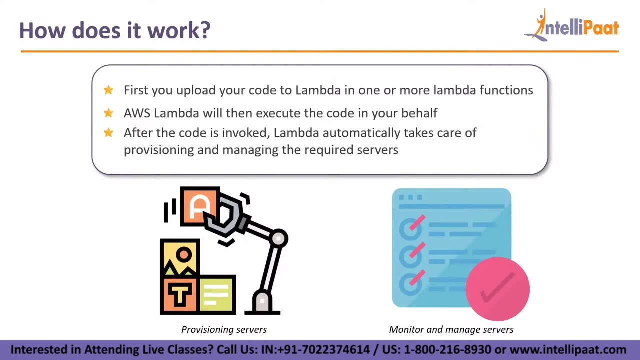 so now, let's say your code has been successfully run. so after the code is invoked, lambda automatically takes care of provisioning and managing the required service. that is, whenever your function uh is requesting, let's say your, your function is triggered right now, so that function has to run. 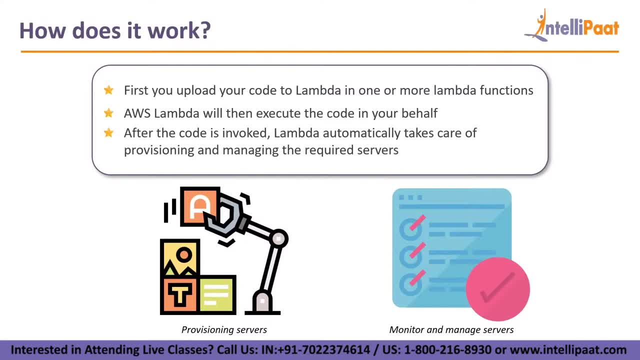 somewhere right? so if it doesn't, if it does not have computing resources, it cannot run your code in that case, that particular time. so already provisioned servers will be used for running your code and lambda will monitor and manage all these servers in the backend. so that is, you don't. 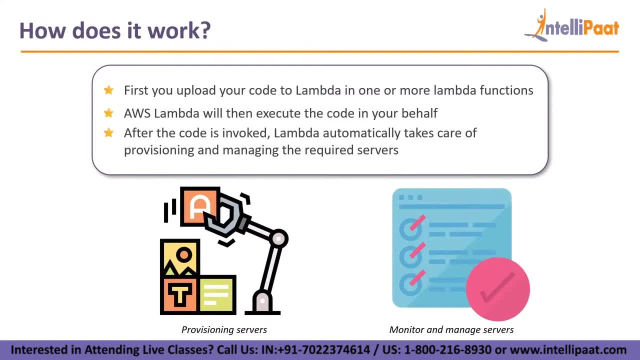 need to worry about anything because it is serverless, and so this is the basic uh idea of how it works. you upload your code, set up a trigger of any aws uh service whenever that particular trigger is, has been triggered or has been provoked. in that case, the lambda function will. 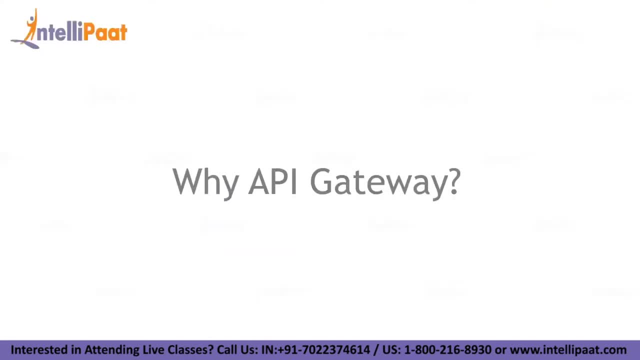 run and all of these steps will take place now. so you've seen about lambda. uh, i think you got a little bit of an idea about lambda, because this is a beginner level tutorial. we've not gone into the depth of lambda. if you want to check out lambda, you can check it out in our youtube page. 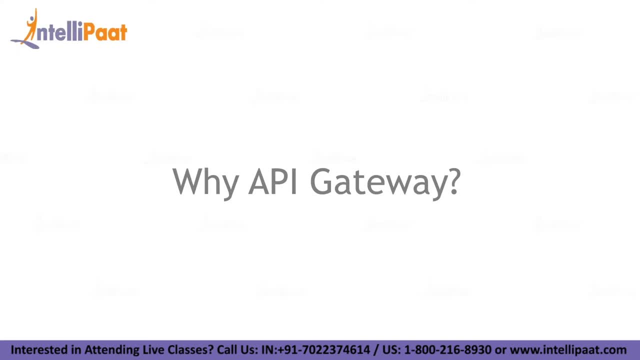 and also guys, make sure to subscribe to our channel and also leave a like if you like the video, if you like our efforts that we put every single day. um, yeah, so please subscribe so that you can get more of aws content and we will see you in the next video. bye, bye. 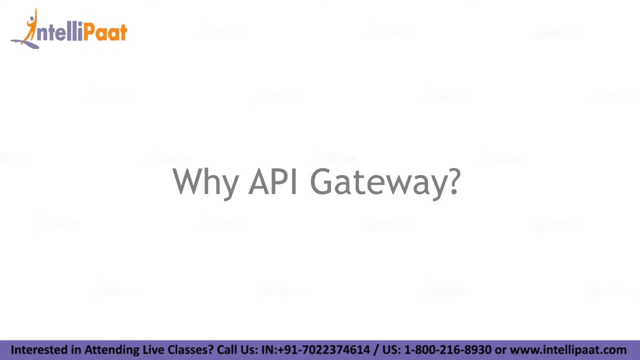 and also other technology content. okay, now let's flip into the api gateway. so we already saw lambda. so lambda is a serverless computing resource which you can upload your code to and it runs whenever it is triggered. so it is mainly used for backend purposes. now we're coming. 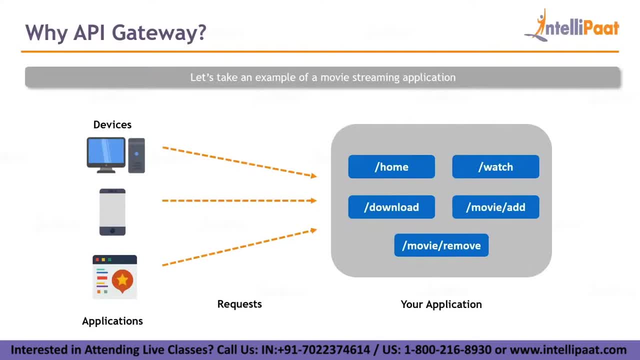 to api gateway. so why do we need api gateway? that is, that is the first thing we'll be looking into. so let's take an example of a movie streaming platform. so let's say you have certain devices. you can watch netflix in your pc, in your uh, let's say, in your mobile, also in your tv. so these are three different uh. 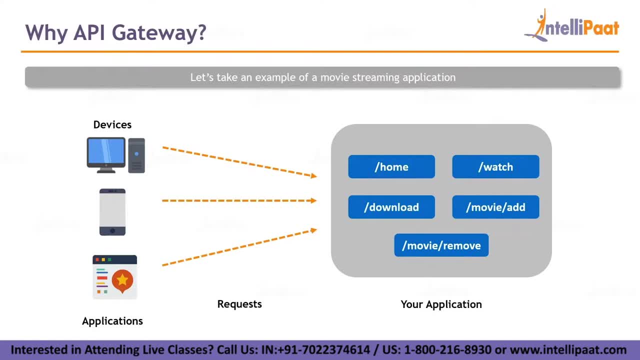 devices, which has three different applications running in them. so now the getting over here. so these are the requests to watch movies or get into the page. so the home page is basically the page in which all the movies are shown. watch page is the page for a particular movie, in which. so you can. 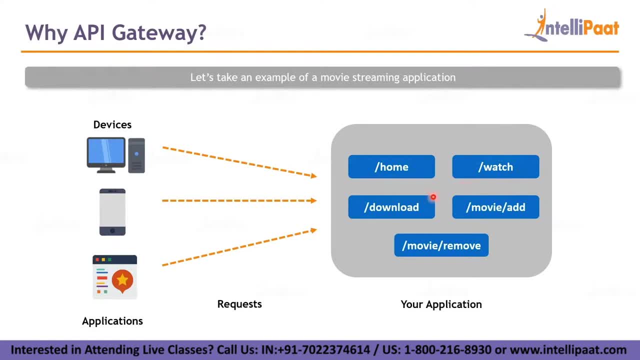 watch this movie or continue to get into the movie so you can download the download page. you can add a movie, you can remove a movie. so these are the five different operations in this particular streaming platform. okay, home page. you click on certain movie, you watch it here you can download. 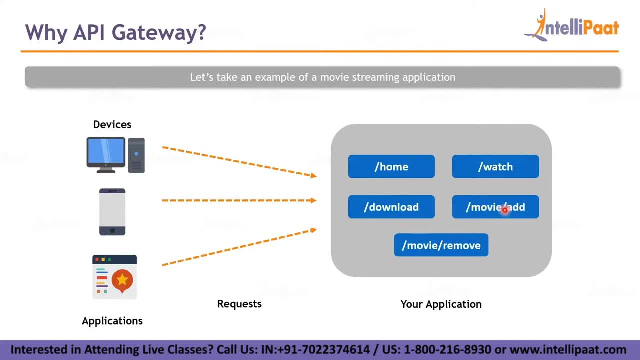 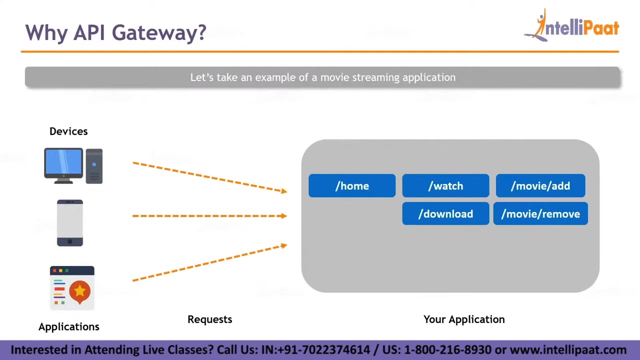 it in this particular url. you can check it out. you can add the movie to your streaming service from this particular url. you can remove it from this particular url. okay, now let's say your application is this. so this is your application. your application has five different pages and there are multiple devices which are trying to access your application. 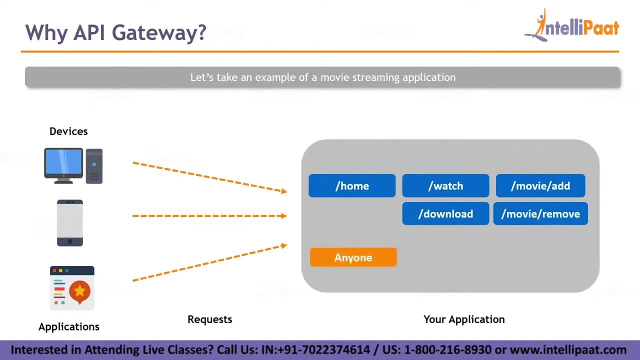 so now your home page should be available to anyone. so even if i don't have a subscription to your streaming service, even if i don't have subscription to netflix, i should be able to see all the movies available in netflix. so that is the first api anyone. 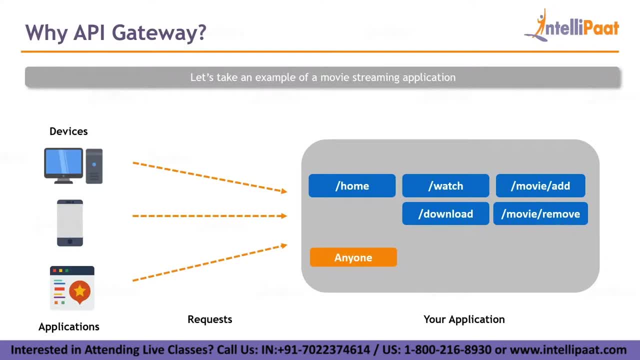 so anyone can access home. if any of these users, from any of the devices, with subscription or without subscription, go to netflixcom home, they should be able to see all the movies in that particular home page. next comes in login user. so if you have a subscription and you're logged in, 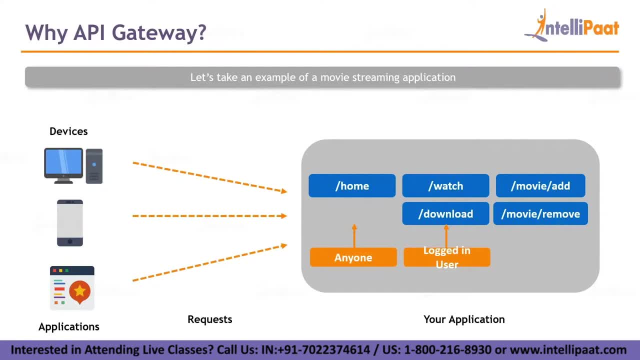 in that case you will be able to watch the movies in the streaming service and also download. so i think you know, if you own a streaming service, if you pay for a streaming service- let's say a hot star- or if you pay for crime or netflix, in that case you can watch it, also download it. 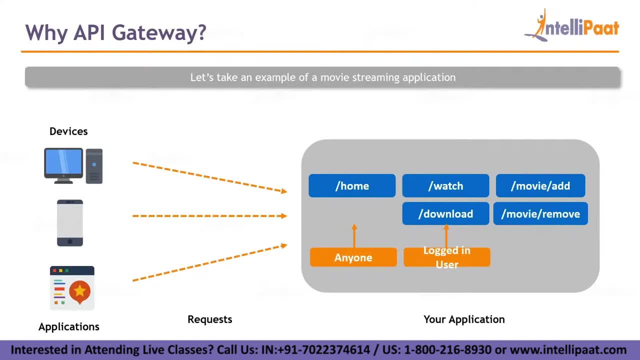 and you can only do that if you're logged in. subscribed user. that is the second api, which tests if the user is logged in and has a subscription. now coming to the third one, as an admin. so the admin is the person who adds movie to the streaming service and removes movies. 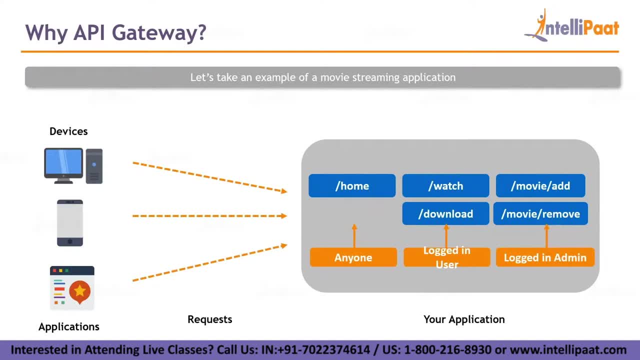 from the streaming service. so now normal logged and subscribed user cannot add movies from their local pc into the streaming service, right, because they don't have any rights. so now there's a third api called logged in admin. so now whenever you're trying to log in, the api logged in admin will check if this particular user is an admin. if this user is, 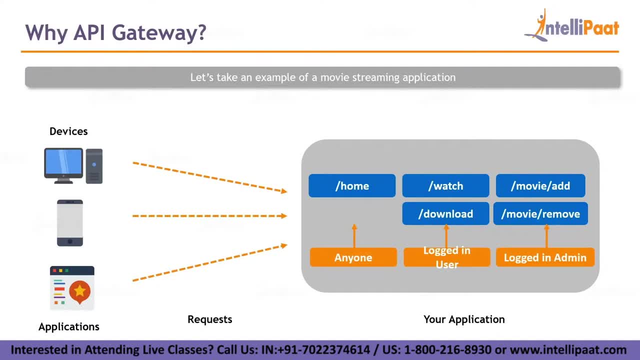 an admin. it will allow access to adding a movie and removing a movie. so these are the three different apis for one particular streaming application. so now you also have a fourth api which is used to secure the complete application. okay, so there are three apis within the application. 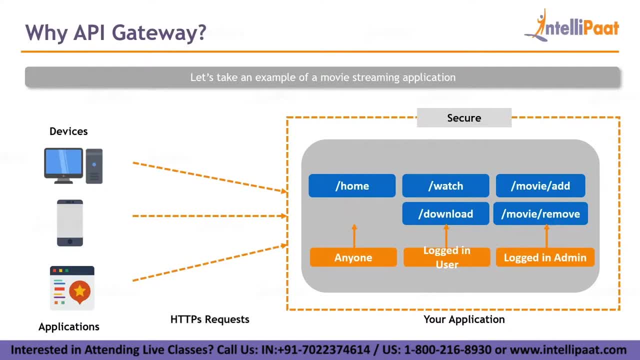 and also there is a fourth api to secure the complete application. so the problem which arises here is: everything is within this particular code, so everything is available in one single location. so now you can group all of these apis together inside your code itself, but still there would be. 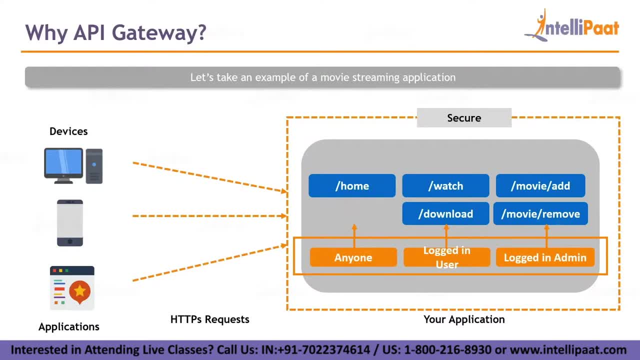 a problem. there won't be a single point of entry for all of these devices, because all of the devices get into the application only then the api is checked. so in this case the application might get slow. there might be a lot of errors sometimes. if let's say the secure api doesn't work, in that case it won't check any of the other apis. that 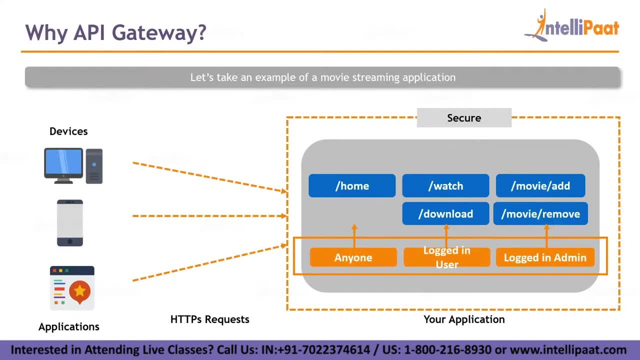 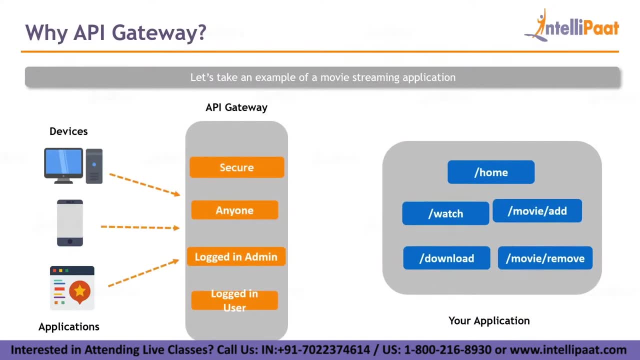 there is a lot of problems today. so now to solve this, an api gateway was introduced. so what did an api gateway do? so that's what we're going to see here. so an api gateway considered. this is the aws api gateway, so there are b4 apis available over here: secure. 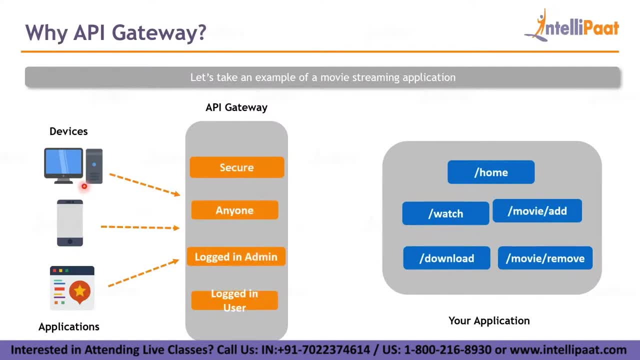 anyone logged in admin and login user. so whenever a user is trying to access your application, it goes through this particular api gateway, which is the single point of contact for any device which is getting in. so now, let's say i'm logging, i'm trying to access the website, i don't have a 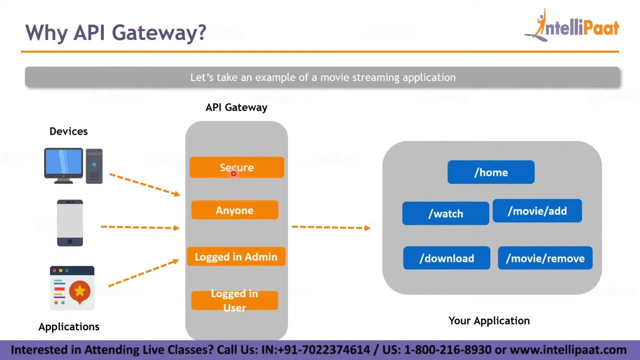 subscription. okay, so now the secure api is obviously securing my application, because the application is after or behind my api gateway, which is securing it already, as well, as the secure api is also used to secure it. so now, when i'm getting in, i don't have a login, so it checks with all the apis and i. 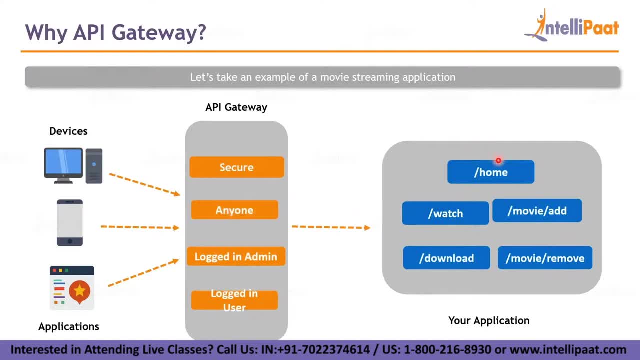 only pass for the anyone api, so it only allows me to view the home page. same thing. a second user is logging in and he's a user, normally a subscribed user. so now the user can go to home, watch and also download. a third user is logging in and it is the admin, so now all of this is allowed. 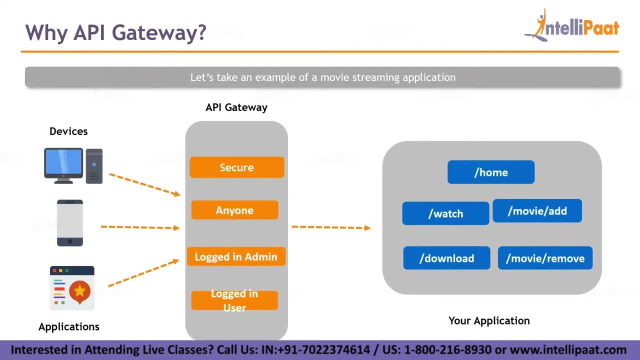 a single api gateway, which is going to be the door to your application, which makes it even more secure, is what exactly is an api gateway? and also, it's pretty much easy to manage an api gateway. so if you have all your apis clubbed together with your code, in that case it will be. 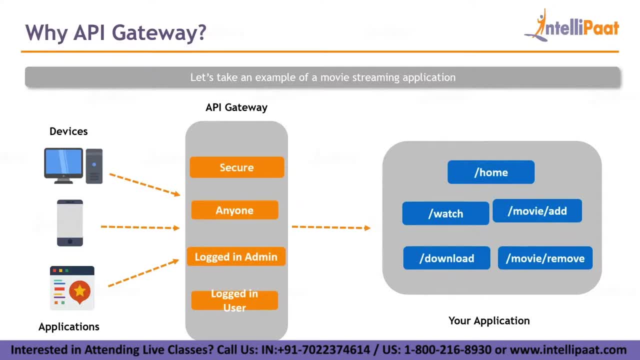 much easier to manage. so this is just an example of four different apis. but in a real-time application there's going to be hundreds of apis in place, so it will be really hard to manage. so if you have one api gateway in place to handle all of these apis, that would be much, much easier. 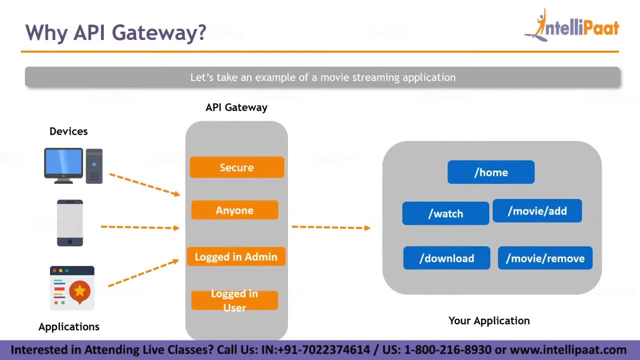 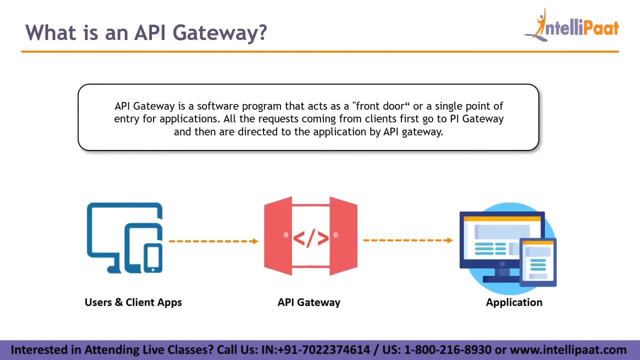 than having all of the apis to be available in the code, which just directly checks and redirects you to the correct page. so now, coming down now, what is an api gateway? as i told you, api gateway is a software program that acts as a front door or a single point of entry for applications, all the requests coming from clients. 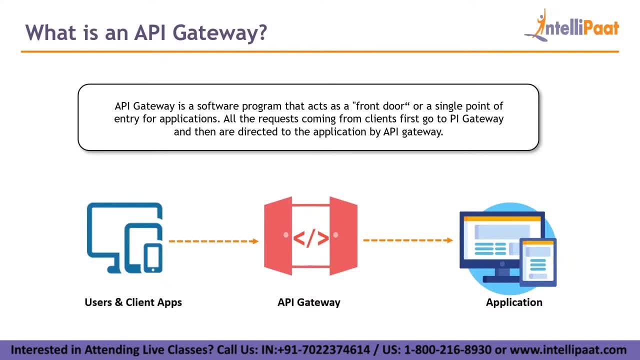 first go to the api gateway and then are directed to the application by the api gateway. so whoever the user may be- uh, however, they can get in the administrator or the ceo of the company itself or a normal user- whoever it is- they have to go through the api gateway. so api gateway is not a 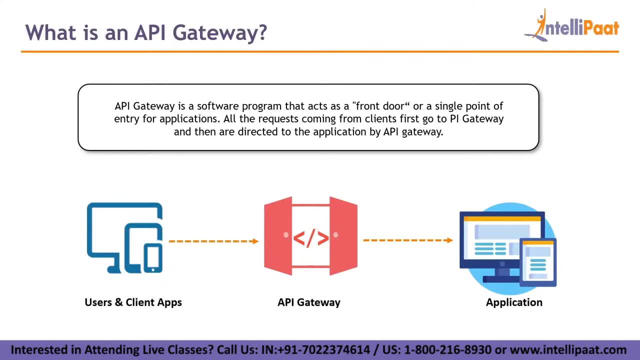 physical entity. it is a piece of software program which checks for certain accesses for the person who is logging in. so if the person does not have a login id, the application will only allow certain pages to be visible if they are logged in. more pages will be visible if they are logged in as. 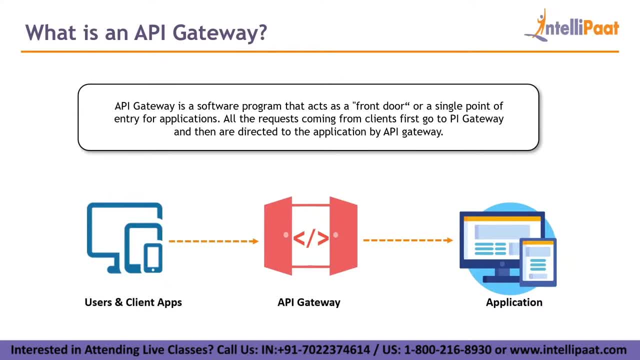 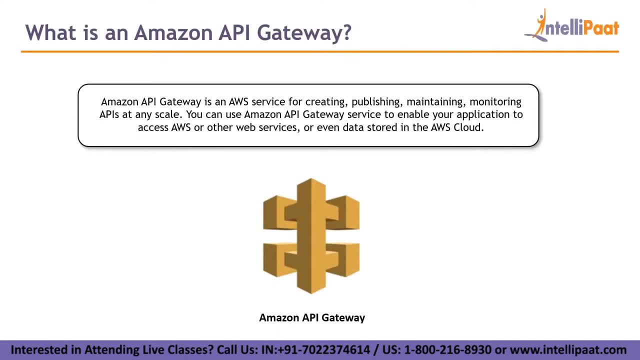 the administrator, all the pages would be invisible. okay, so we've seen this. so this is basically an api gateway. so now, what is an api gateway? it's pretty much the same, but this is just provided by amazon. so amazon api gateway is an aws service for creating, publishing, maintaining and monitoring apis at any scale you can use. 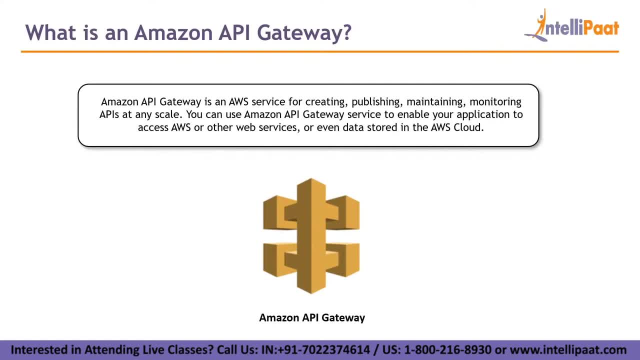 amazon api gateway service to enable your application to access aws or other aws web services or even data stored in the aws cloud. so you can use amazon api api as your front door to any application posted on aws or any of the other aws services which you don't want anybody to use before getting to your api gateway. so you can basically create: 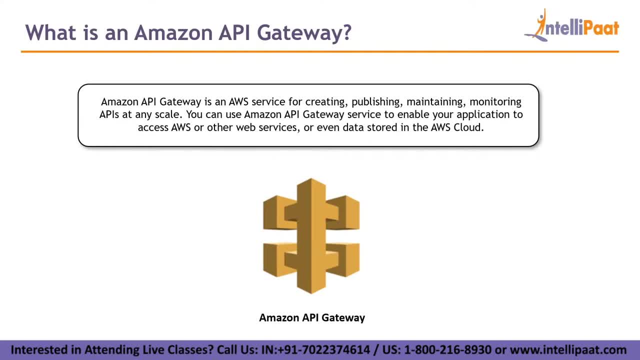 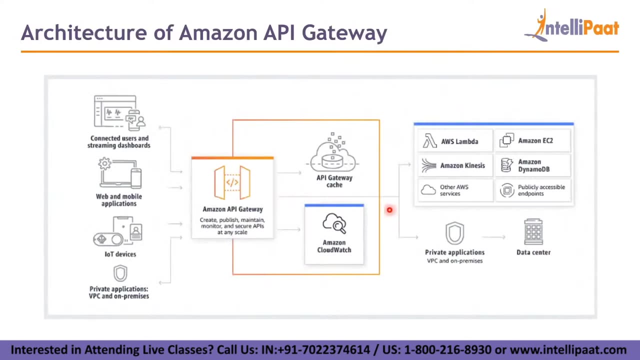 apis: publish it, maintain it, monitor it, and it can be at any scale. it can be a simple test, it can be a real-time production environment for a huge application as well. so api gateway can handle all of that. so now, finally, before going into the demo, let's look at this particular 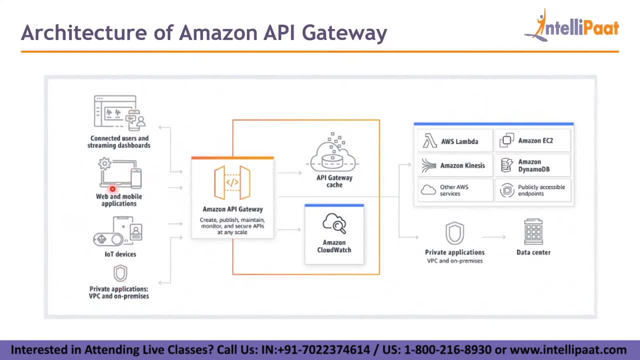 architecture. so these are the different types of users who are getting into, who are trying to get into the application. so now api gateway is the single point of contact for all of these users now getting in. there is an api gateway cache. let's say this particular user is always viewing just the home page of the application. so in that case the home. 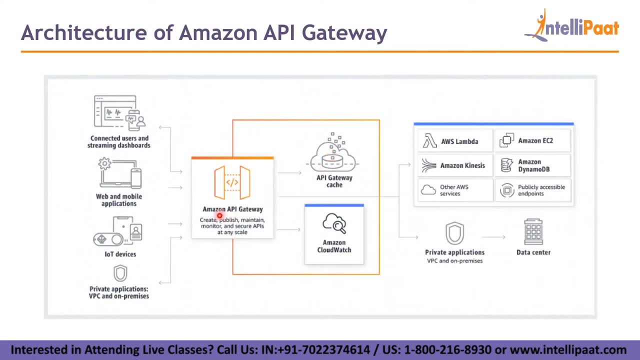 page will be available in the gateway cache. it will be picked up, given to the user immediately. it won't even go to the application. same goes with cloudwatch. so cloudwatch basically watches what is the api, how many times it has been invoked, if there is any problem. so this is just for monitoring. 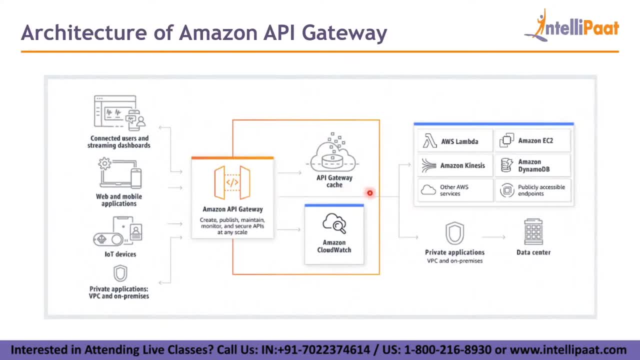 so now another user is trying to access and it gets in. so these are the aws services and these are the private applications. you can use amazon api gateway for both private applications and aws hosted applications. you can see here vpc and on-premises, so vpcs on aws. 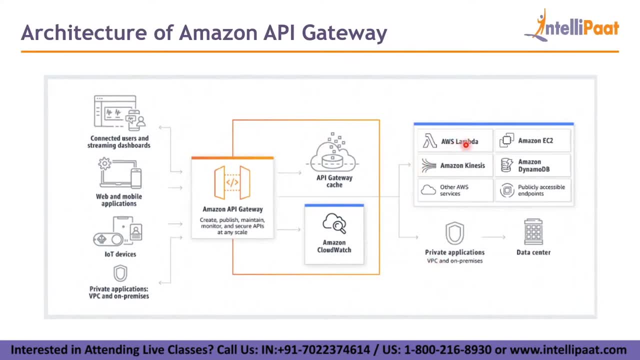 on-premises are private applications. so now, in our case, we'll be using lambda. so gateway is going to be the trigger for lambda, and whenever the person is trying to do a certain, let's say a certain task, and that tasks code is available in lambda, it has to be triggered. so 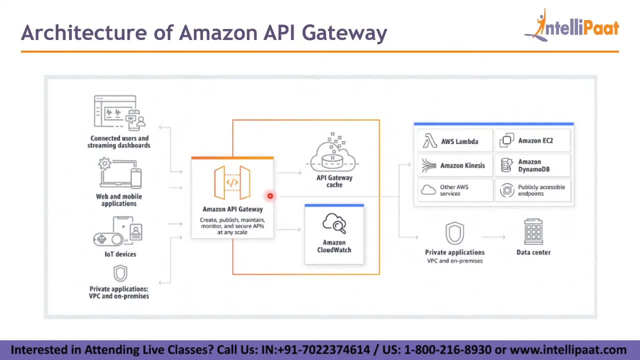 whenever they're entering to through the api gateway. that particular api which is within the gateway will trigger the aws lambda function and the lambda function will run and give back the result to the user and the result will go back through the api gateway itself. because it's this. 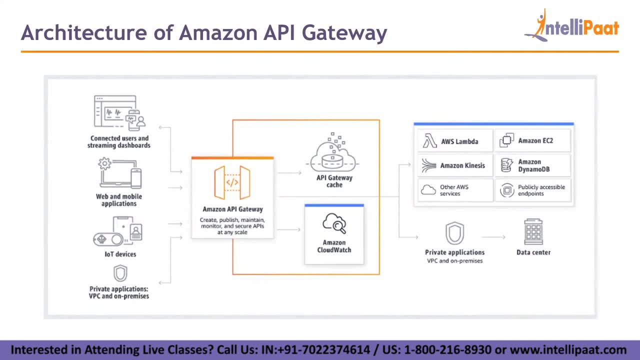 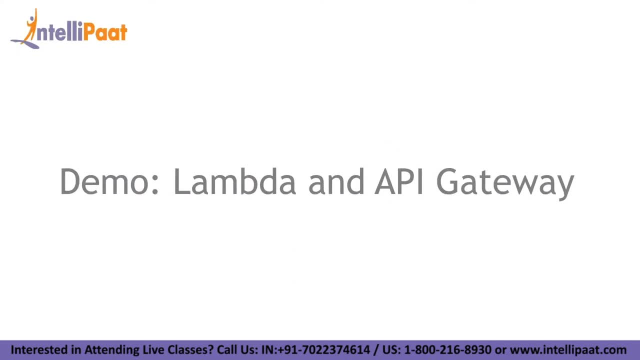 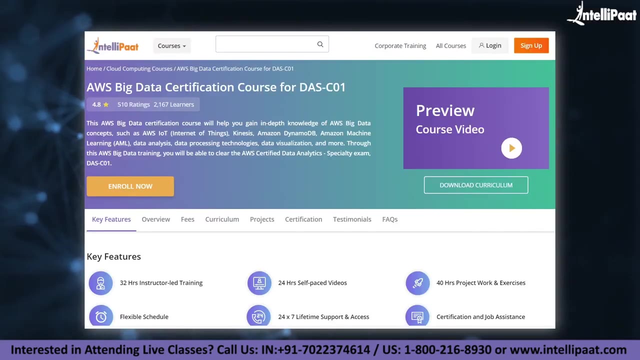 single point of contact. okay, so as we've seen this, now let's look into the demo for this particular session. so the demo would consist of lambda as well as the api gateway. here is the aws management console. first let me open lambda. just a quick info, guys: intellipaat provides aws big data certification. 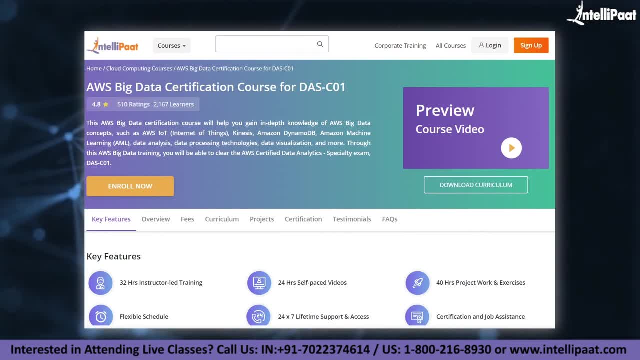 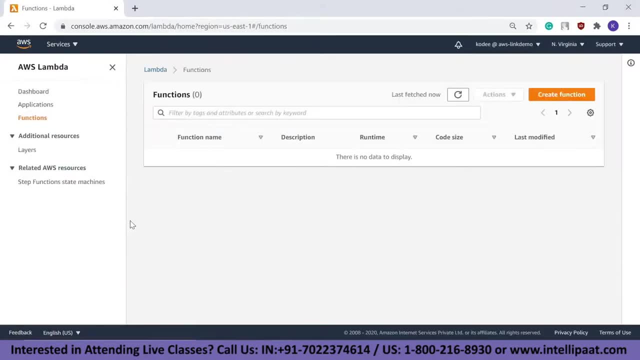 course mentored by industry experts, the course link of which is given in the description below. now let's continue with the session. okay, so before moving on with the aws case, make sure you have your own aws account where you can practice. so don't worry, this session will be available on our youtube channel once this. 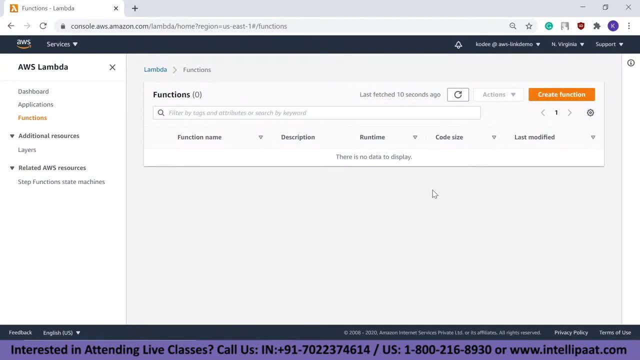 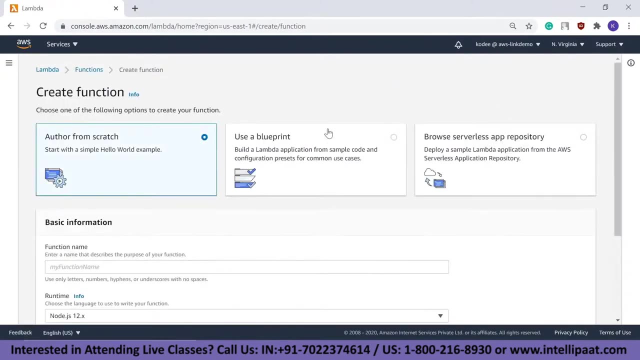 particular live ends. you can watch this particular video again if you want any more clarity in this demo. it's a pretty simple demo where we're creating a sample function which will be triggered by an aws api. so first let's start off with creating a function. so go to lambda, click on create a function. 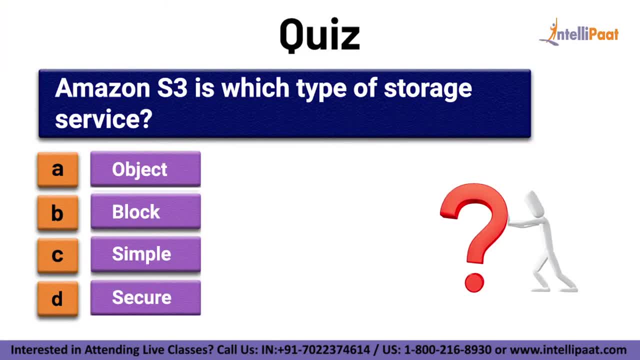 just a quick info, guys. test your knowledge of aws by answering this question. amazon s3 is which type of storage service? a? object b, block c, simple d, secure. comment your answer in the comment section below. subscribe to intellipaat to know the right answer. now let's continue with the session. 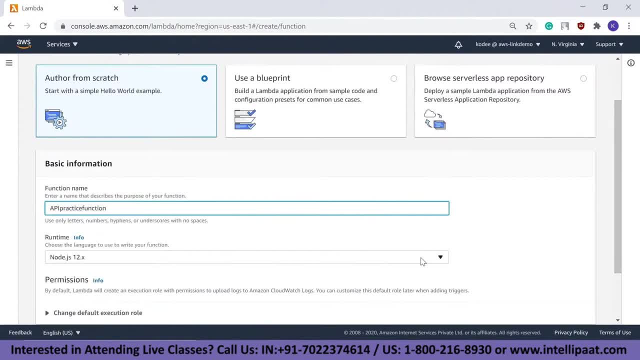 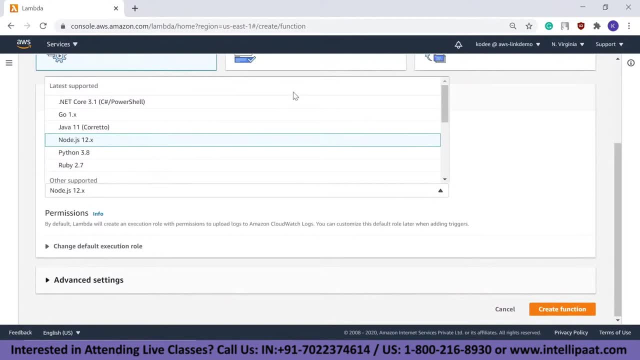 dá" come down, provide a name and we need to provide it as api practices function. choose any runtime you want, because i'm not going to upload any code. i'm just going to use the default code which is available. so let's choose python and click on create function. so, as i told you, you don't need to choose the operating system, you don't. 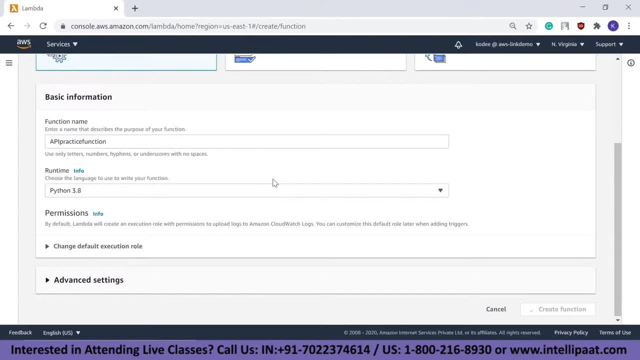 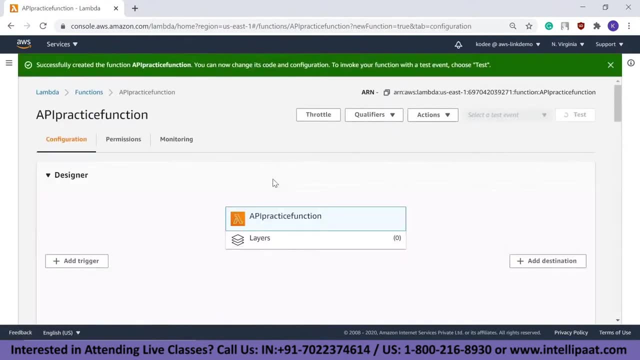 need to choose, or let's say, you don't need to choose the instance type or you don't choose anything here. you just need to pick theבi viber year. if you want to load the에서 ò, have to choose the runtime and create the function, and once you've created the 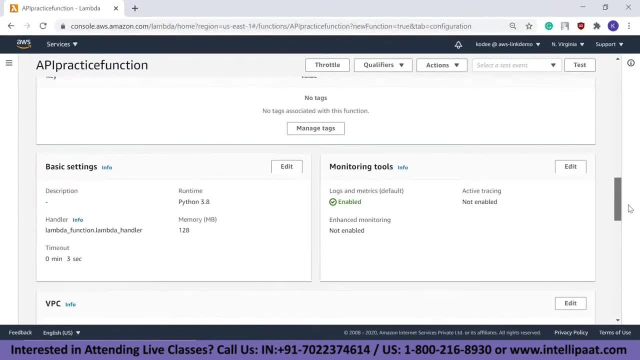 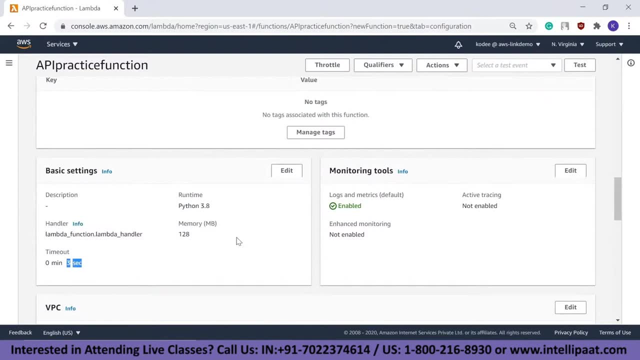 function, then you can basically change every single aspect of the function as well. coming down, you can see over here: memory is 128, timeout is 3 seconds. you can change this by clicking on edit over here, but I'm not going to do that because my function doesn't need more than that. 3 seconds is more than enough. 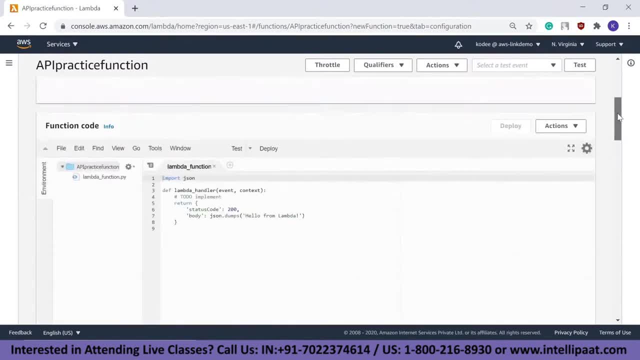 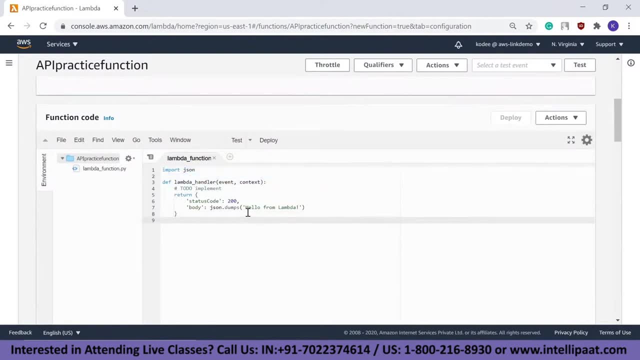 128 MB is more than enough. now, coming to the code you can see over here: import JSON lambda handler and it says hello from lambda. okay, so this is the sample function which will be running. this is the sample function which will be running, and this particular function will be called so whenever this lambda 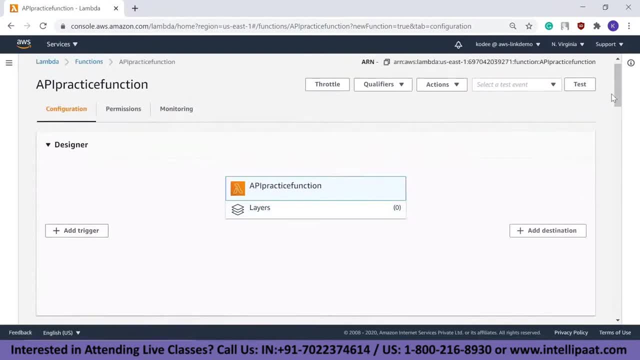 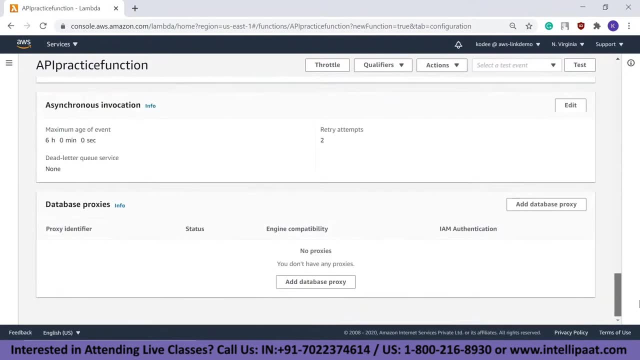 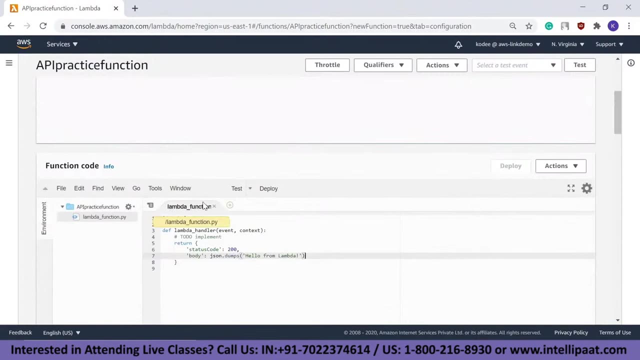 function gets triggered by a trigger which will be adding right now. this particular lambda function will be called. so why it will be called. I'll show you that. okay, so you can see. the name of the function is name of the code is lambda underscore function and the definition's name is lambda. 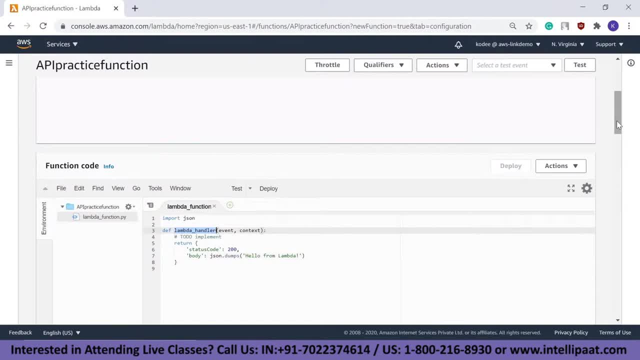 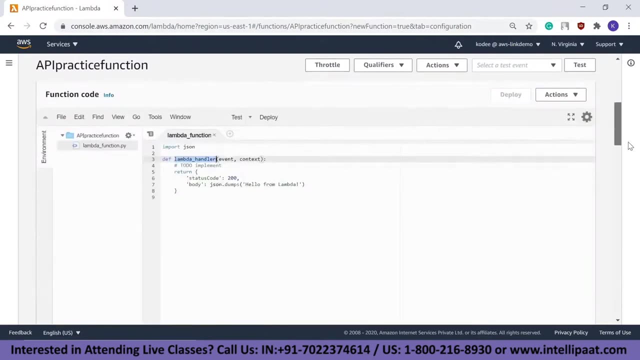 underscore handler. so now it will check for the lambda underscore handler function inside of the code which you have uploaded. so whichever code it is and you set for the lambda for handler function and that particular definition of that particular function inside the code will run. so now, before moving on with the API gateway part, 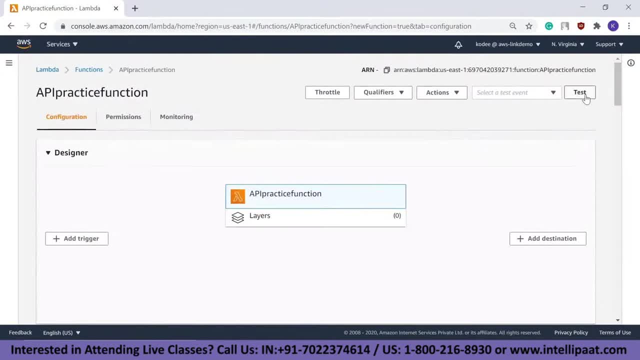 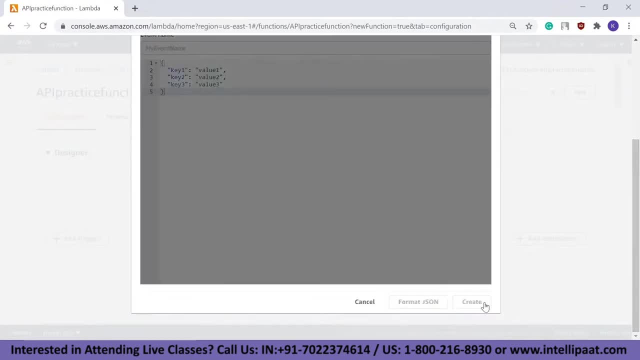 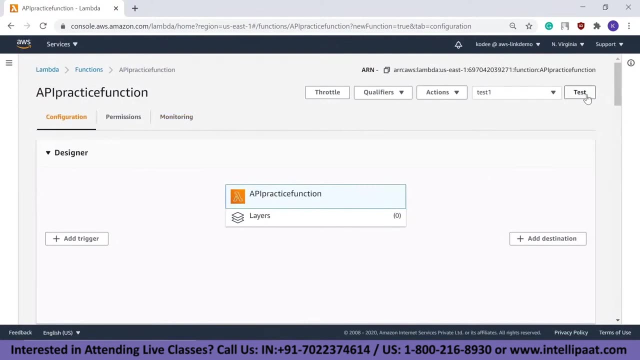 let's test this out. so to test it, you can just click on test, provide a name like test1, come down and click on create so it will show if the test is run once we click on this test. so we have set up a test by clicking on it, sorry, 1. 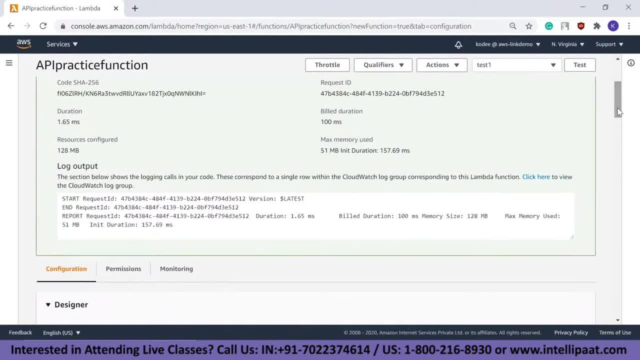 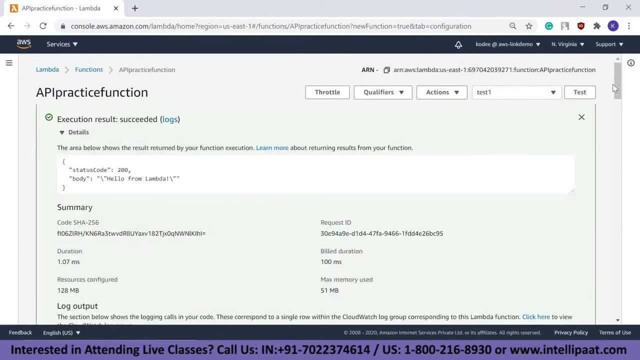 million invocations free, so you don't need to worry about that coming down. so maximum memory used is 51 MB. you can see that, as it told you, 128 MB is available. so I'm testing once again so you can see: maximum memory used is 51 MB. 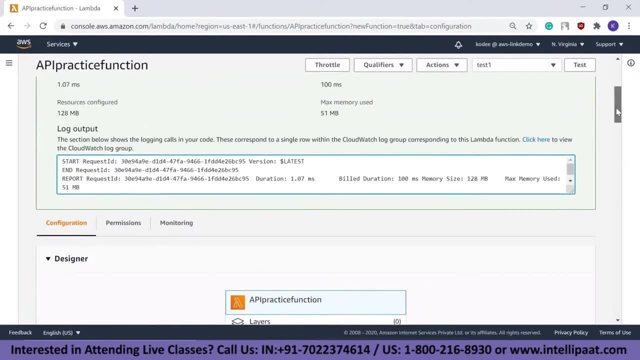 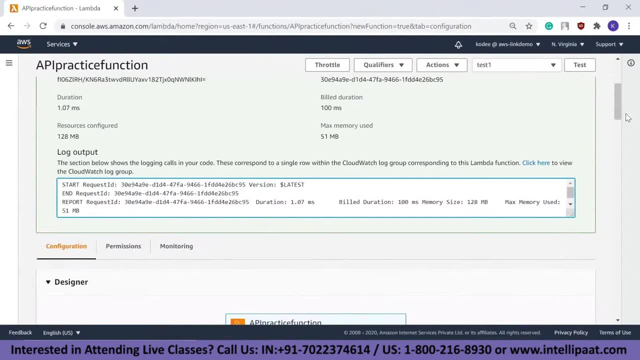 it does not go beyond that, so you can check your applications. so once you upload your code, you can basically test it and check how much memory it is using and according to that you can set up your memory so that you don't get charged a lot. so once this is done, test is complete. 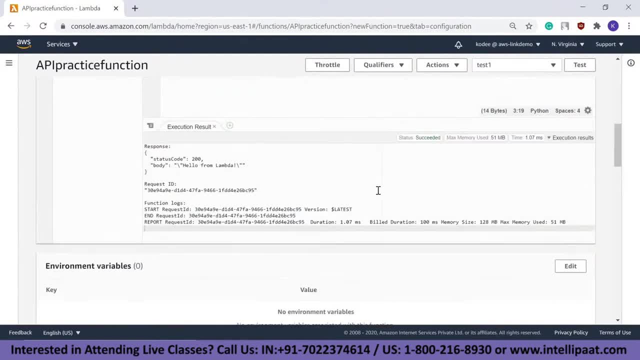 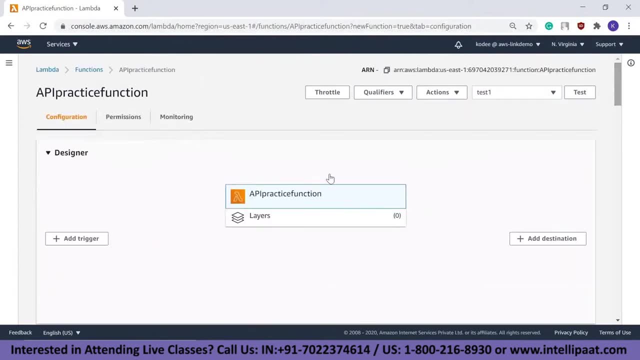 now coming down, so here also you can see it's the same thing which we saw at the top. okay, so now test is complete. the next step is to add a trigger. so our trigger is going to be API gateway, and whenever the API gateway is launched, then this: 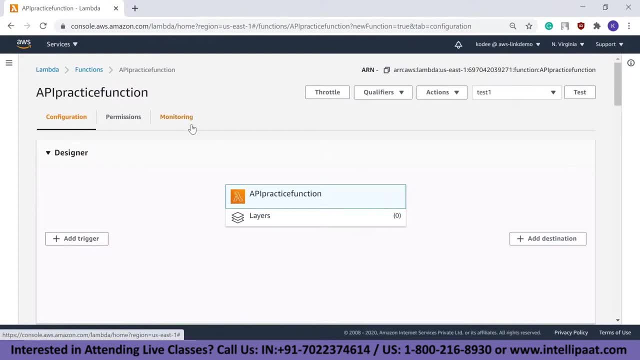 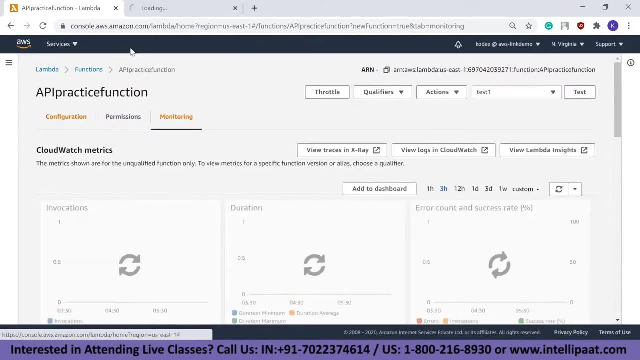 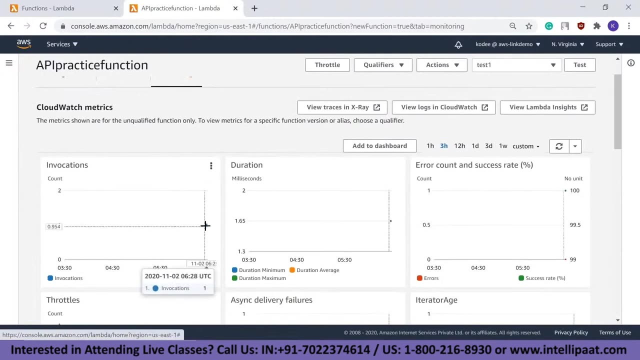 lambda function will get triggered. so how will you know if the lambda function got triggered? so to know that, you'll have to go to monitoring. so just open this in another tab and monitoring in another tab. so over here you can see there is one invocation. this is when we tested it and 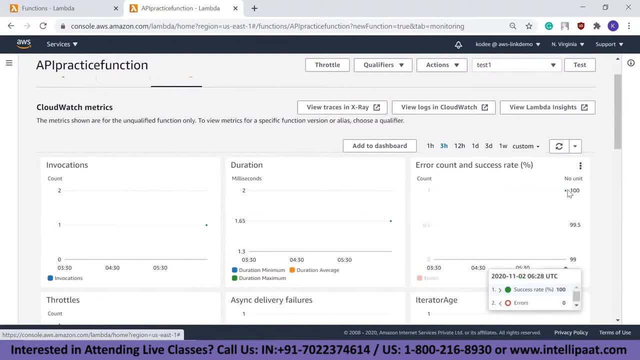 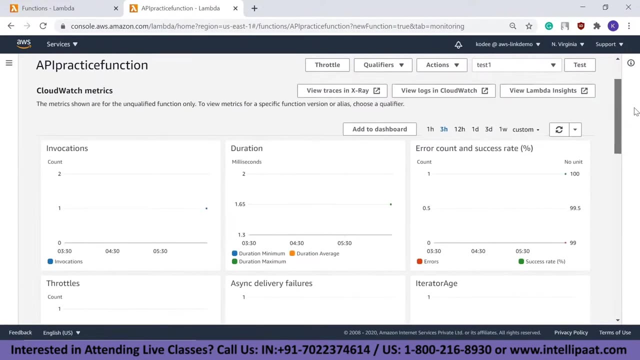 it was successful, you can see here. so the success rate is 100% because the one test we did was successful and yeah, okay, now coming down. so these are the metrics which you can look into the CloudWatch metrics dashboard. within the lambda function itself, main one is invocations. you can just check how many invocations. 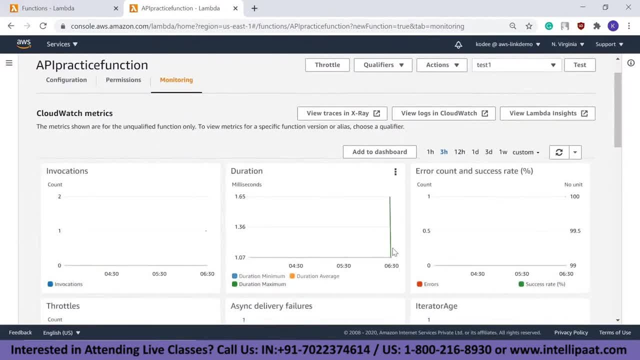 have been made, how many of them are successful? you can also see this, so you can see. there is one, and duration went from 1.65 milliseconds to 1.078 because we ran it for a second time, right, so that time it got reduced. okay, guys, so you've seen this, so now what we're going. 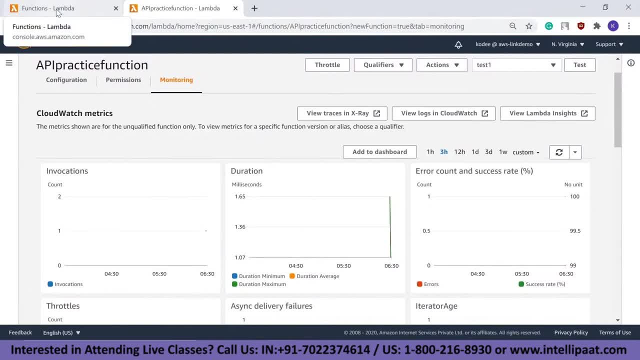 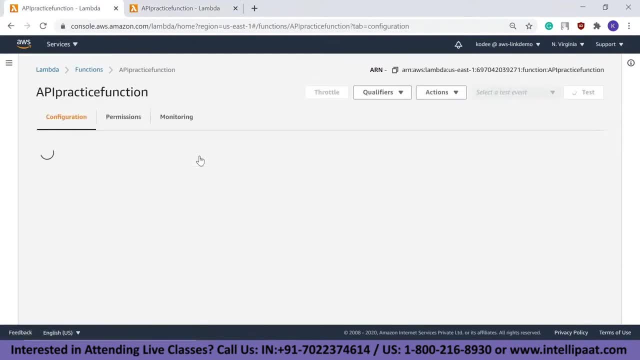 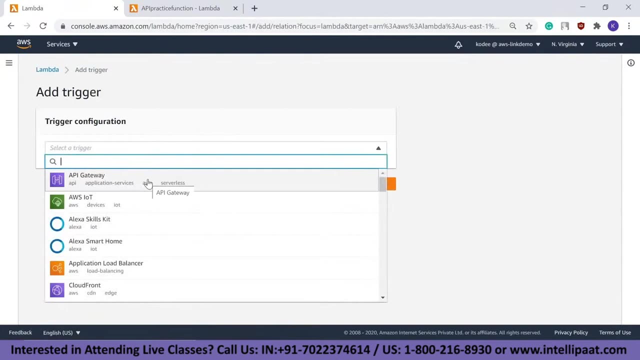 to do is we're going to create API gateway as a trigger and once you created a trigger, we'll run it multiple times. we'll run the API gateway multiple times so that we can check the number of invocations. now, clicking on add trigger, my trigger is going to be API gateway click. 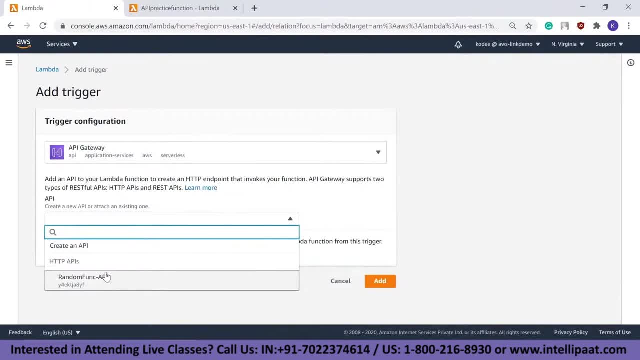 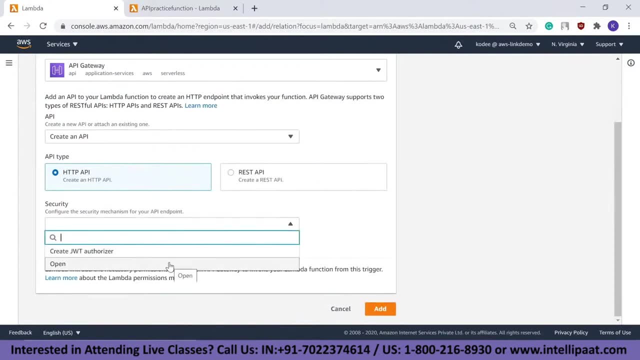 here if I'm creating an API, so I already have an API and I'm just going to create a new one: HTTP API security. you can leave it as open. anybody can use this particular API, but for now we're just doing it for the test. so there is there. 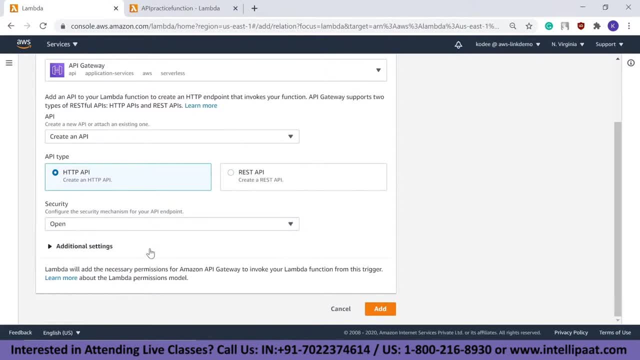 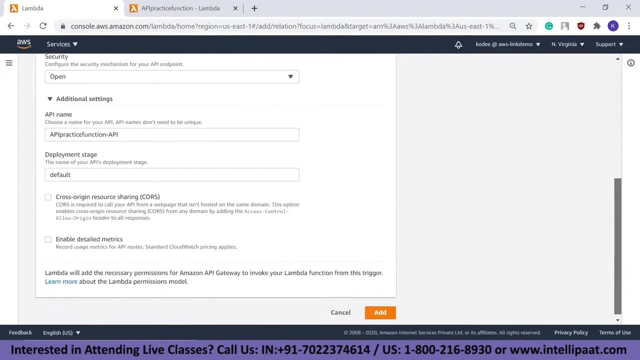 won't be any issue. but if you're going to use an API for your function, do not leave the security open and coming down. you can leave the API name as such. you don't need to change it. you can leave the deployment stage as default. so we are choosing HTTP because 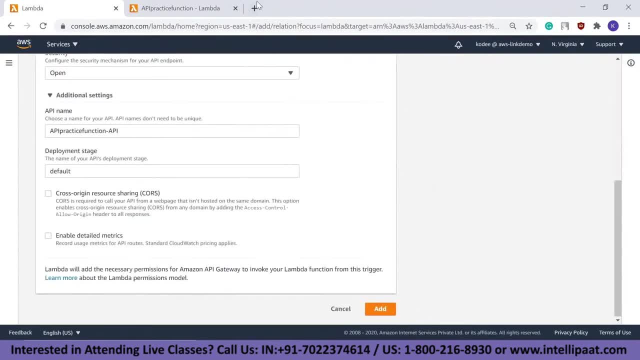 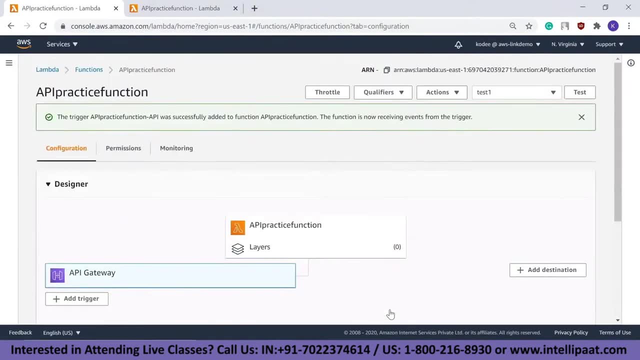 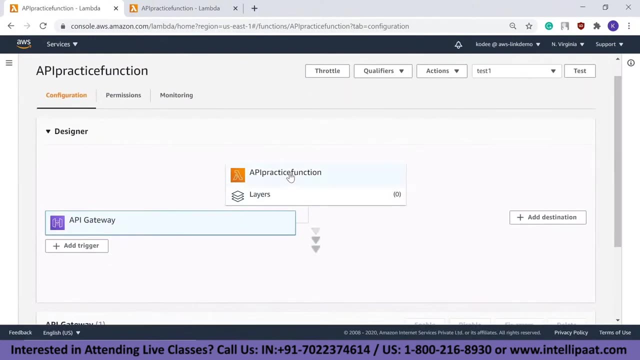 it is a lambda function which you will be seeing over here, so we'll have to see it in the browser. so we are using HTTP. now. I'm adding this as a trigger. so it's done. so the trigger has been successfully added now. if you click on this right now, if you click on this, you 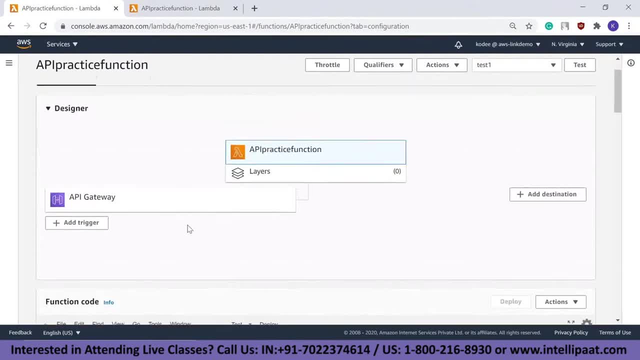 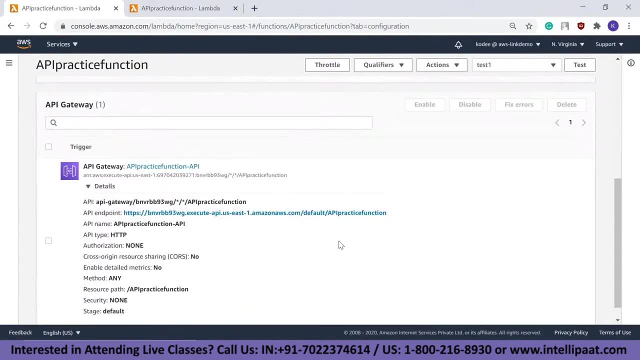 would see the code. right, you will see the code and the other things. you click on a API gateway, you'll be able to see the details of the API gateway trigger. now, when you click on details, I can see there is an API gateway endpoint, so I'm going to open this. I'm just 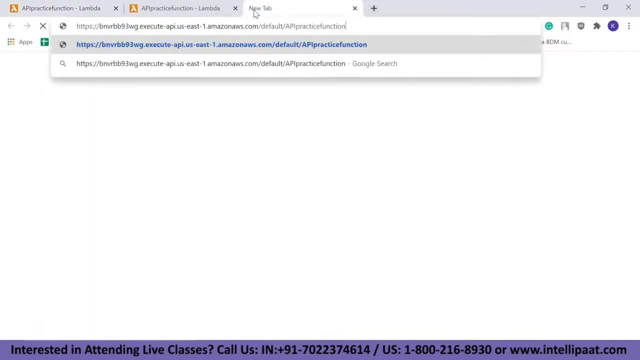 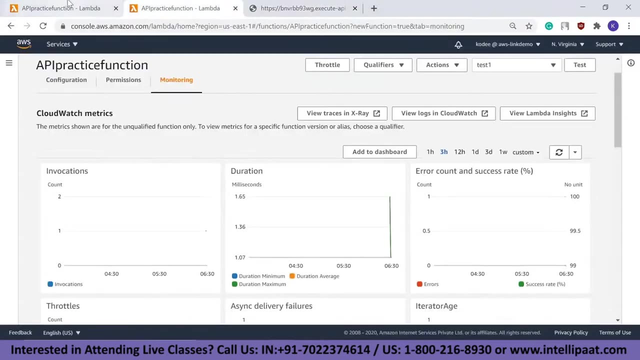 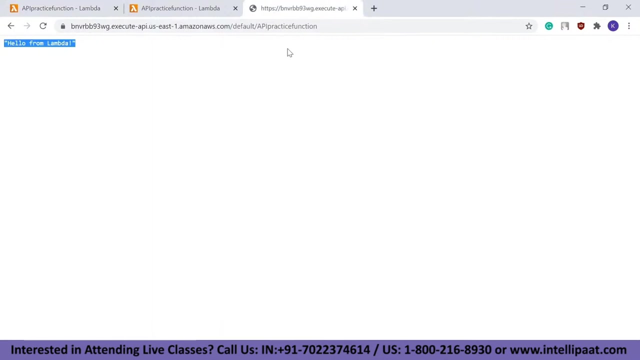 going to copy this first. running this, you can see there is a message from the code. so the codes message itself was: hello from Lambda, So that is what is being shown over here. This is the result which is getting shown, So now you can basically run it once again. 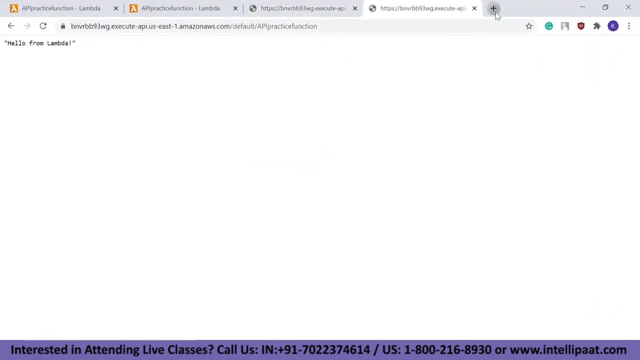 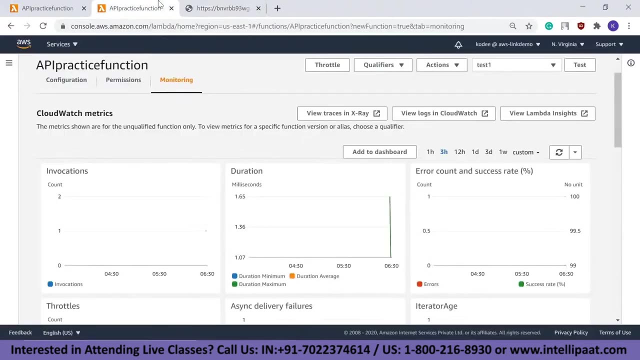 You can run it once again and run it once again. So this is just to check the number of invocations. So we ran it around five times. Let's go to the CloudWatch dashboard, So it won't be available in the same second. 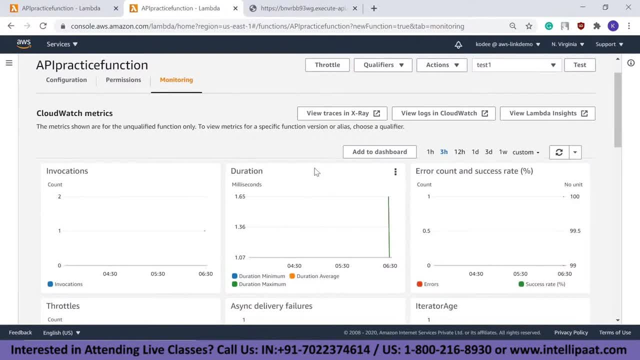 it won't be available in the next second Understand until you have enabled enhanced monitoring. If you have enhanced monitoring, in that case they're paying extra for monitoring and they'll give you real-time updates. But in this case you won't get real-time updates. 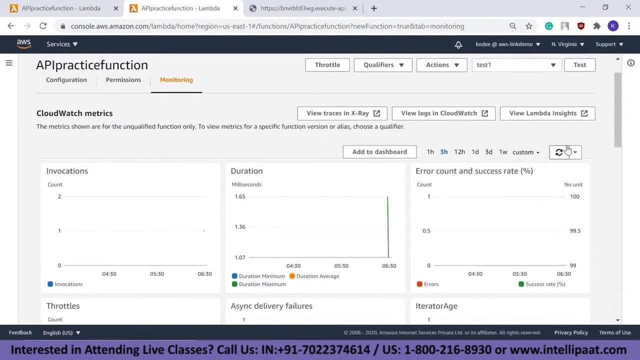 you'll get updates which are a little delayed, and that's what we'll be seeing over here. Right now it's still showing that there was only one invocation, but soon we'll see if there are more invocations arrived, So let this be here. 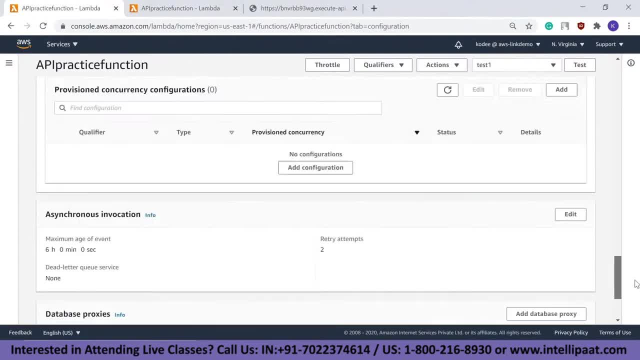 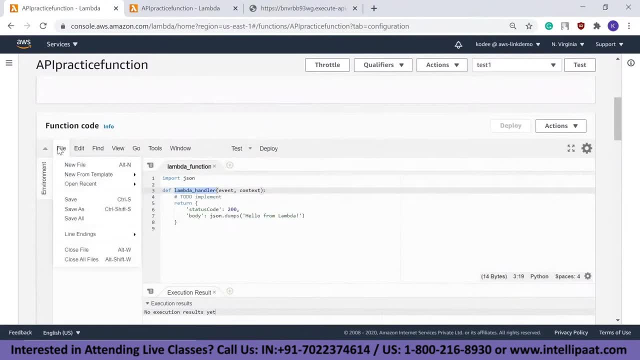 Let me go over here and let me show you if there are any other things which I have to show. Okay, so you have. okay, so this is what I wanted. So you can basically use this as your code editor or your text editor. 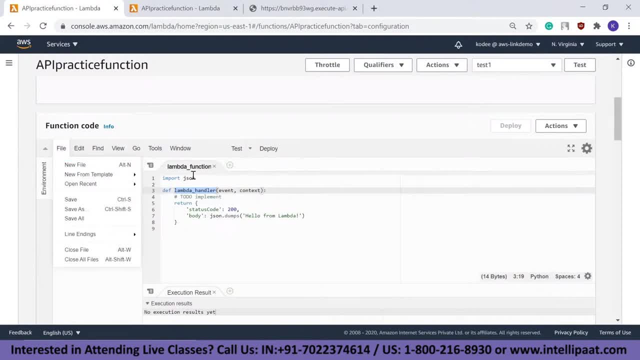 So you can just click create new files over here and start coding. You can edit your files, you can just use it like a normal text editor or a code editor And then, yeah, so you can upload a zip file which you have in your local PC. 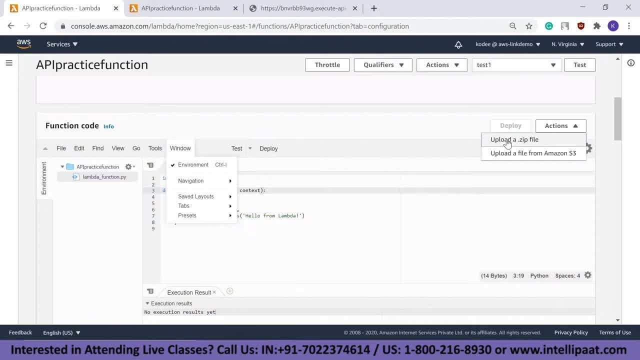 Let's say you have a complete application, which is, which has everything in it, So you can just zip it and upload it over here, or you can upload a file directly from Amazon S3, which you have stored over there And there you can change the memory. 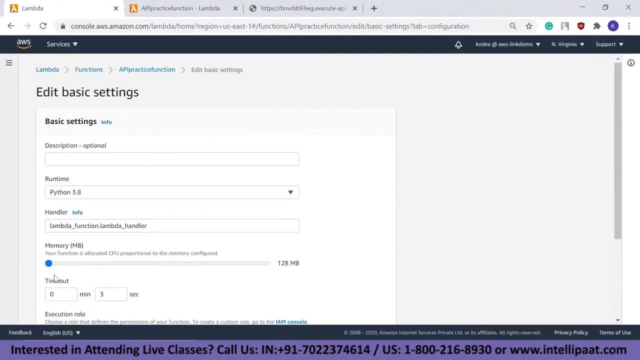 You can change the memory up to 3008.. You can change this up to 15 minutes. You can see this. the maximum is 15 minutes. If you go above that, you can't. So you can also keep it as one second, two seconds. 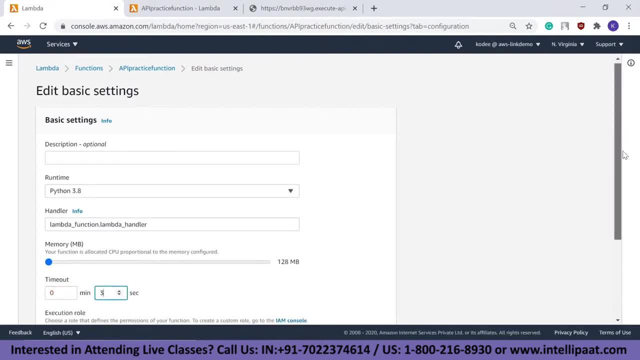 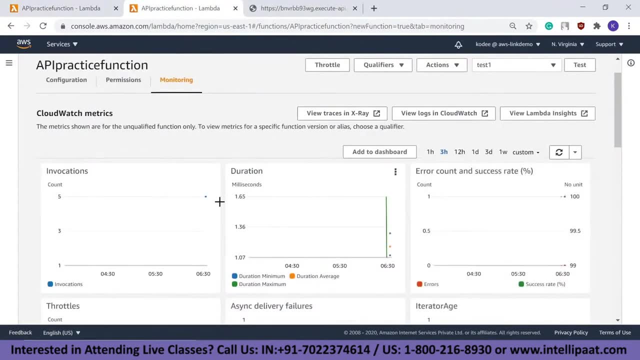 three seconds. three seconds would be the default value all the time, So I'm just going to leave it over here. Okay, now let's check the changes being shown here. Yes, you can see there are five invocations right now, So I invoke it five different times. 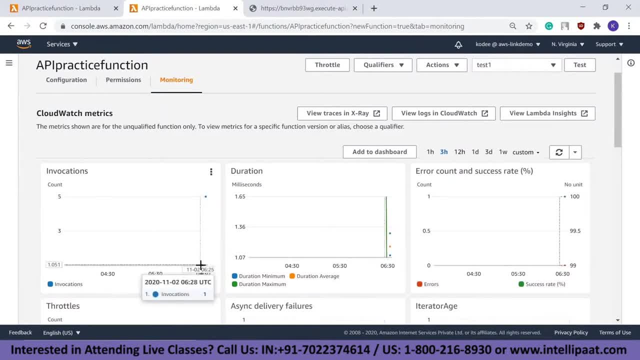 So last invocation, when I did there was one invocation, but with the API gateway we pasted the endpoint over here for five times And basically it ran the function for five different times And you can see. so invocations are five. 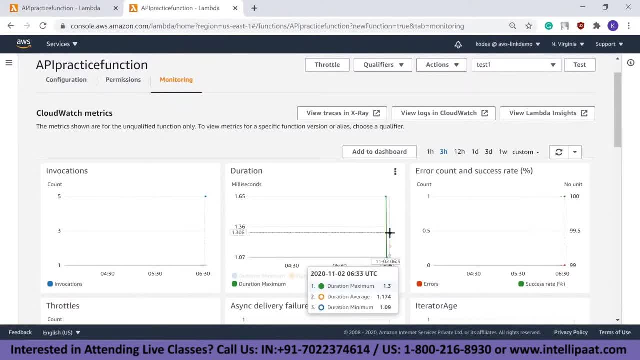 Now coming over here you can see the maximum duration. maximum was 1.3 milliseconds. Duration average is 1.174.. Minimum is 1.09.. So this is the maximum minimum time which it took to run each of those invocations. 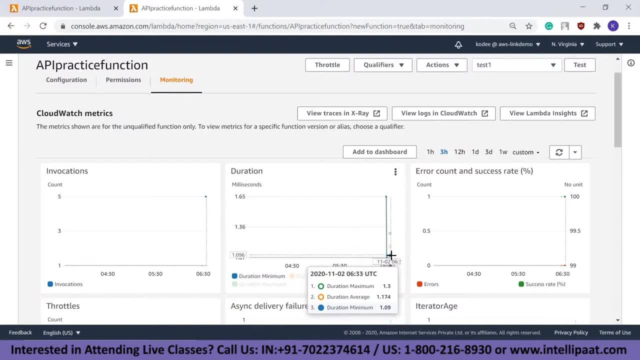 This is the minimum. This is again the average for the last time. Okay, now, coming over here, you can see again there is 100% success rate because all of my invocations ran successfully. So this is how we can use API gateway. 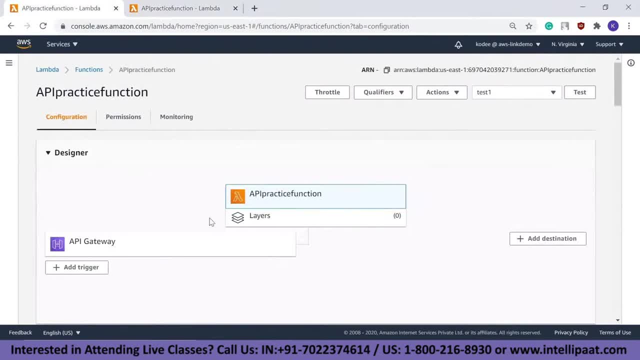 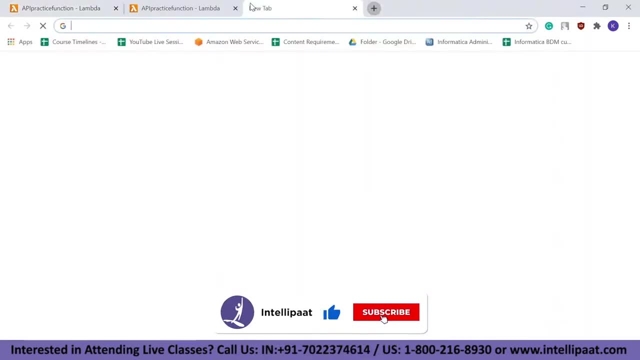 So I'm not directly triggering my Lambda function. I'm using my API gateway as the front end where I open a website. So let's say, you can open intilapadcom. You will not know that, but there is an API in the back. 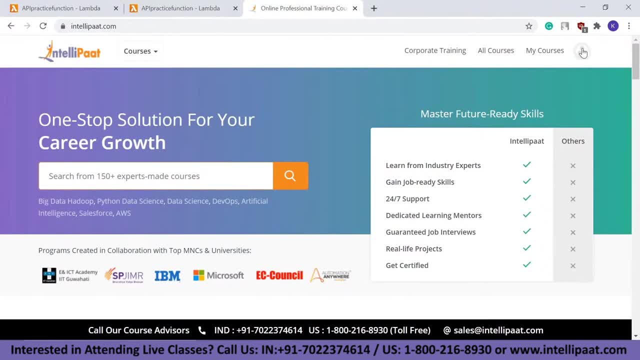 So right now I'm logged in. but if I'm not logged in, it'll open this website even though you're not a logged in user, because it allows anybody to access the homepage, but it'll allow to access the my courses page. 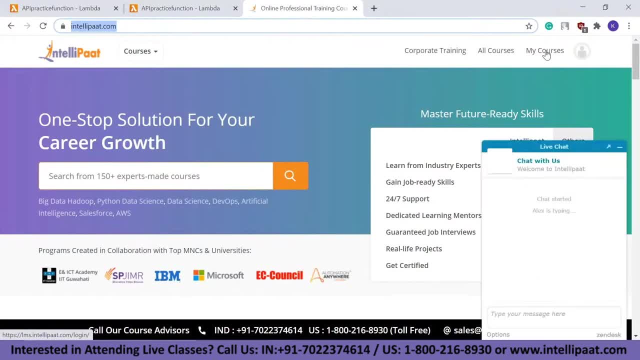 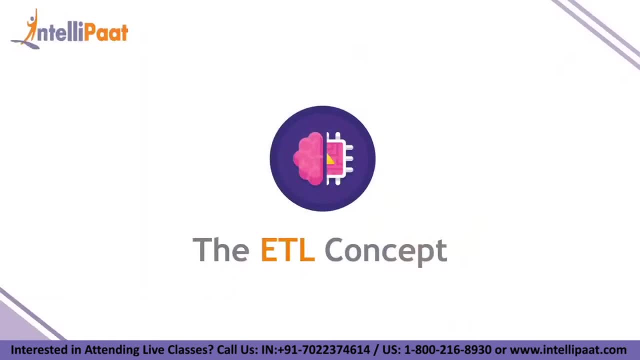 only if you're a logged in user. So that is the main use of your API gateway. So, firstly, we need to understand what the ETL concept is. So, in order to understand what AWS Glue is, which is an ETL tool, 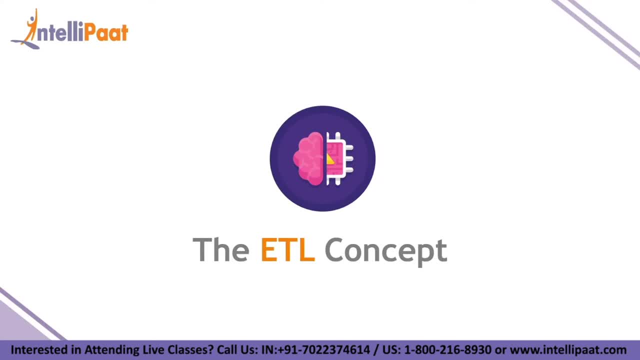 we need to understand what ETL means in the first place and what is the utility of ETL. So another thing to note, guys, we're also going to be implementing a hands-on with AWS Glue on the AWS platform, So stick around for that till the end of the video. 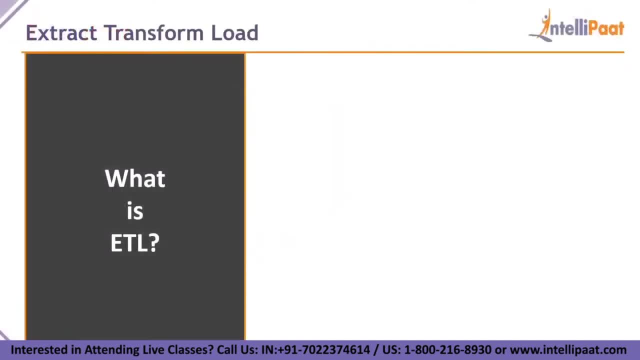 Okay, so let us understand what ETL is. ETL is a data integration process where three interrelated steps are existing. So the first step is extract, The second step is transform And the third step is load. right, So these have to be followed in a sequence. 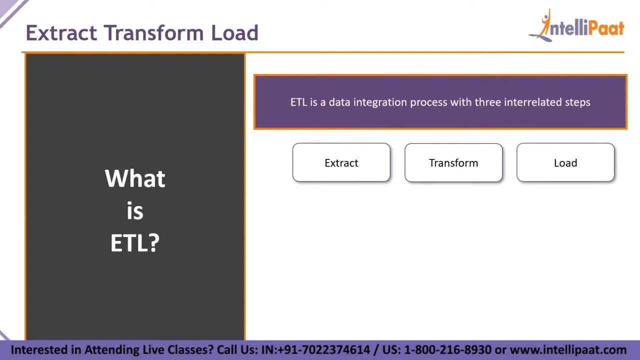 These are the three parts of the ETL process. but what do they achieve? So they achieve a data warehousing. So the primary function is to build a data warehouse or any data construct which provides a combined view of data from multiple sources. right, 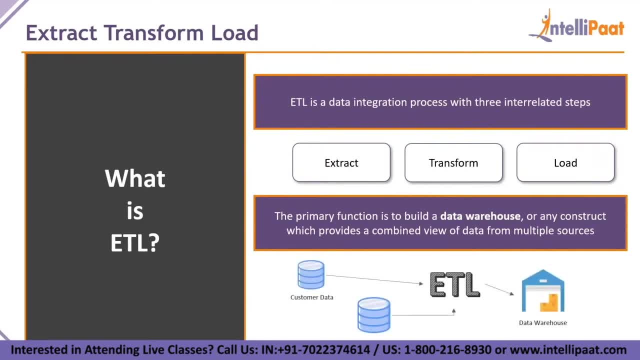 So, to elaborate on this, imagine you're working for an e-commerce organization as a data analytics expert and you're working with AWS, Glue or any other ETL tool or data warehousing tool. You'll have multiple data sources. So, for instance, Amazon has a customer data source. 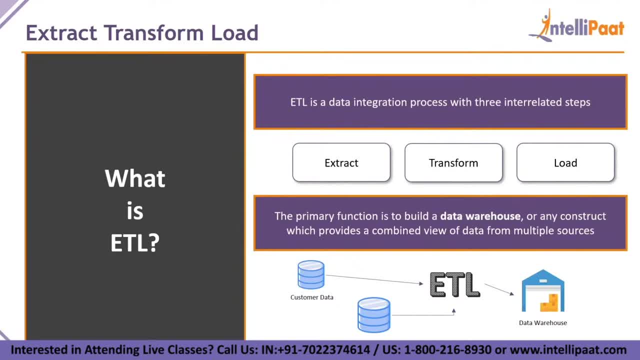 and Amazon has a sales data, obviously. So these are two separate data sources, right. But for a person who's sitting on a managerial position or a person who needs to get insights from a combined aggregate of all of this data, right? He will not be dealing with these two data sets separately. 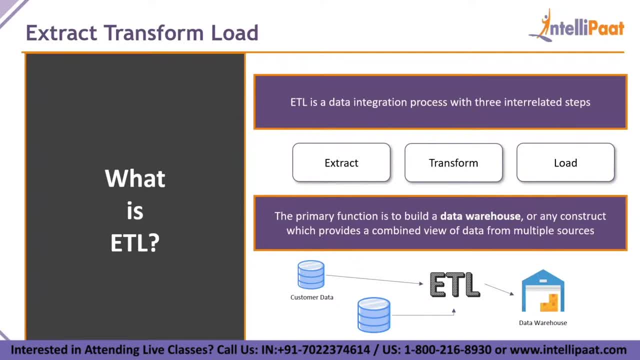 So your job would be to combine those two data sets. right You have. your job is to combine the important aspects of those two data sets using an ETL process or an ETL tool and putting that combined view or the combined analytics into a data warehouse. 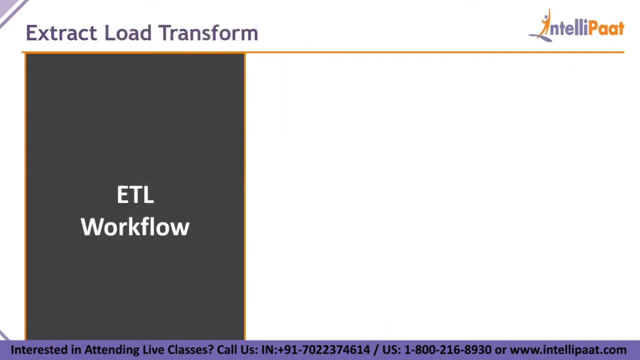 Now, data warehouse is a common place where the data is stored, And then you can use it for further insights. You can create charts out of it, You can create graphs out of it and you can show it to your boss. You can show it to the sales team or the marketing team. 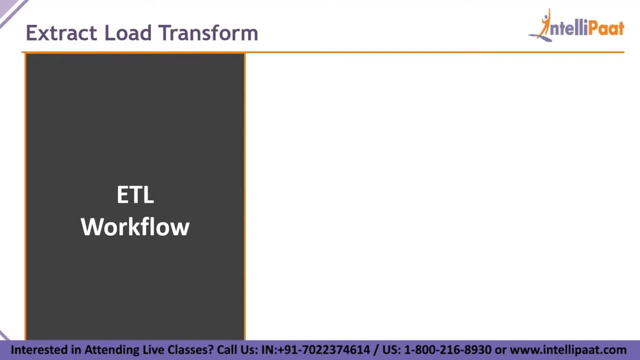 So the people with the non-technical expertise can also understand what is going on with the data. To further elaborate on the ETL process, right, We need to look at the workflow as well. So imagine you have three separate data sources. So one is coming from an RDBMS server. 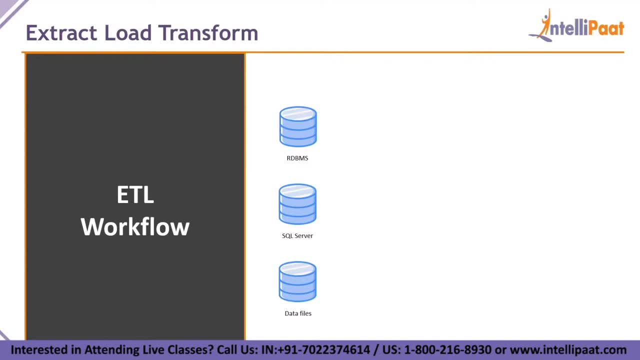 One is coming from an SQL server. One is coming from actual files present on some hard drive or SSD, Right? so these are the three data sources that you have currently. So the first step is obviously extract, right? So the first step in your ETL tool, 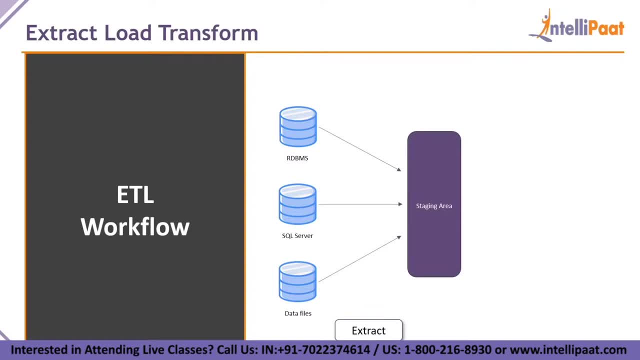 would be to extract this data into a staging area. So what does this staging area essentially do? Once the data has been extracted and put into the staging area, then you're going to be cleaning and processing it essentially. So that means that the data might have. 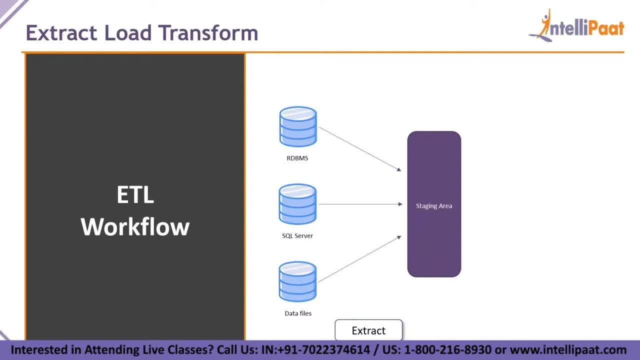 some inconsistencies in it, might have some noise in it, it might have a different format right, and it's coming from three different data sources, so, for instance, the data files that are coming in could be of json format. the sql server is obviously giving data in an sql format, in a structured format in the staging area when you're creating. 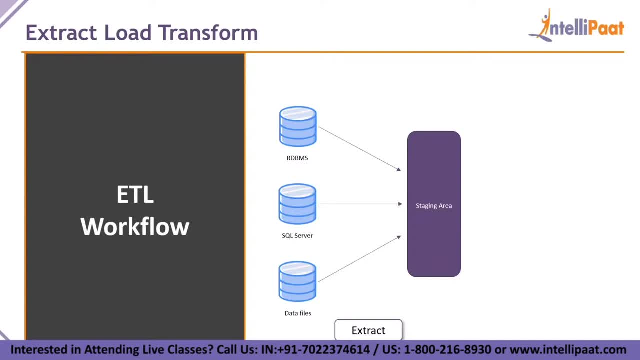 a combined view for a data warehouse, you need to make sure that all of this data is in a singular format, and in an sql format preferably, and the data is essentially cataloged. right, so the next step becomes the transformation process. right, so the transformation process refers to when. 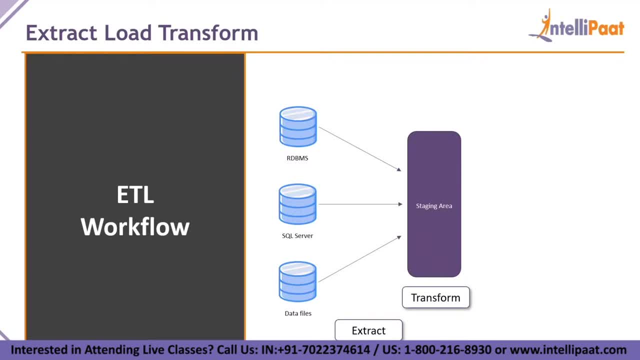 you're cleaning the data after the extraction and you're basically coordinating all of the data types that are there in the data and the data formats that are there and you're cataloging the data. then obviously you have the load. so the load comes in when all of the transformations have been. 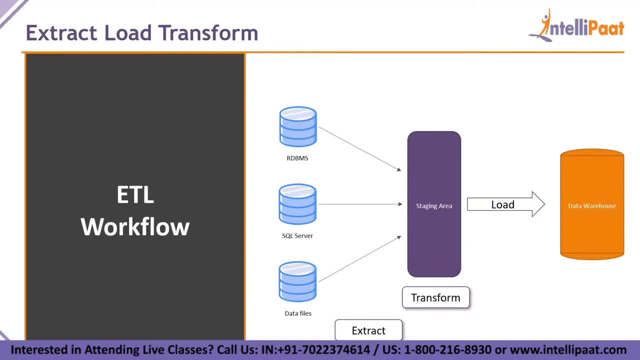 down each one and is all the damages associated with the data. now we can move on to the other end, and so why am i telling you that all of these information are already there, want to allow you done, And the next step is to put all of that transformation and data that has been transformed. 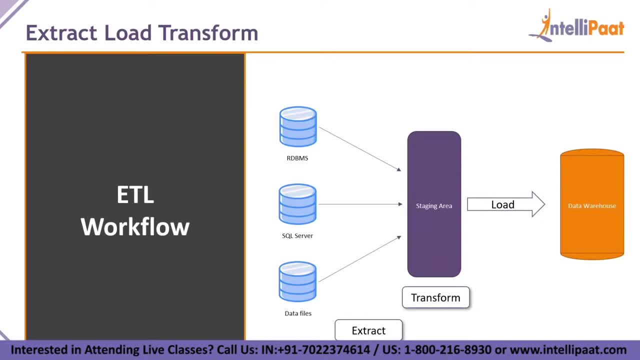 into a data warehouse. So this is what the ETL tool does: It takes the data from the data source and puts it into a data warehouse after it has transformed it. So now that we understand the ETL workflow, let us look at the advantages of data warehousing, because the entire aim that we have 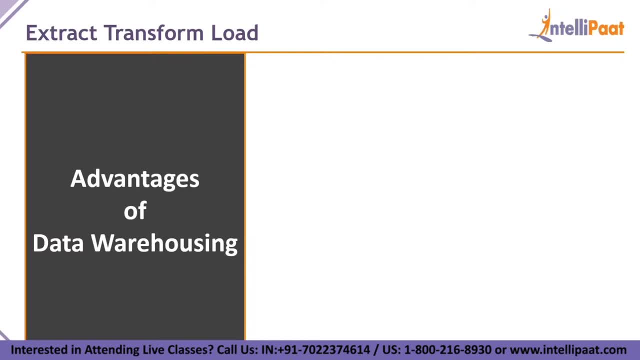 with using ETL is to create a data warehouse. So the question obviously comes up: why are we so inclined to data warehouse? What are the advantages of it? So the first thing is high scalability. High scalability implies that if the data is extremely large in nature- extremely large- 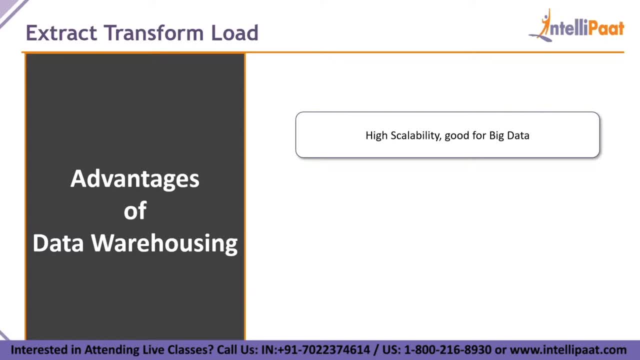 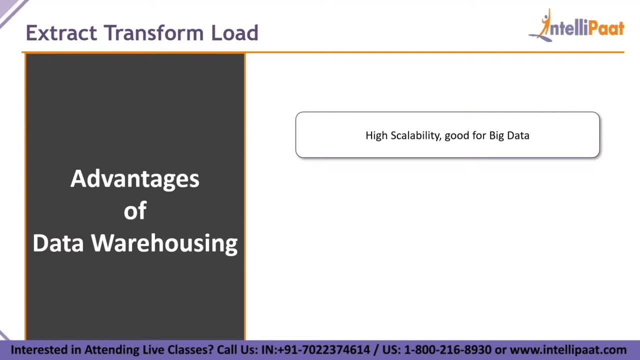 data warehousing. It is a very important part of data warehousing. It is a very important part of an option to basically increase or decrease the size of that data at will right. We don't have to worry about the hardware resources, particularly when we're dealing with this particular aspect. 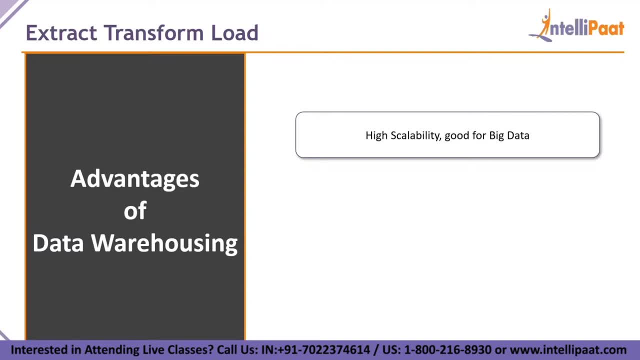 because data warehousing is a process where you're not actually transferring the data from the actual source to a target. What you're doing in data warehousing is you're keeping the data at the location it is, So you're not transferring it and you're not actually transferring it from the actual source to a target. 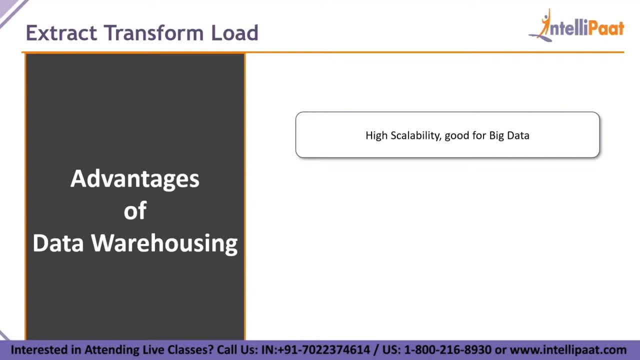 you're performing all your queries on the cataloged version of that data, right so that brings us to the second point. the second point is it increases the speed and efficiency of your data analytics process, right? so, since there is no input output delay, particularly, you're only fetching the 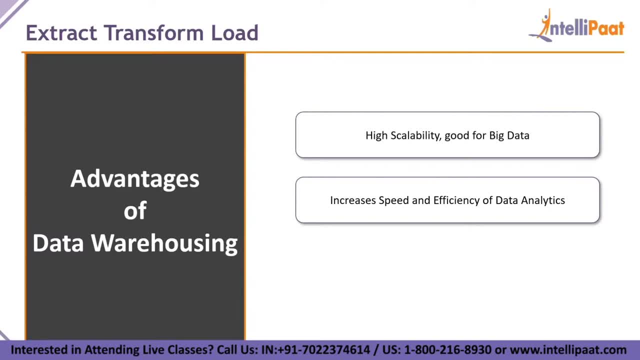 cataloged information. you're only fetching the metadata of the data and then you're performing your queries on the source itself. this efficiency and speed of this particular aspect is extremely good because there is no transfer that is happening and finally, you get the combined view of data. so for people who are coming from a non-technical background or for people who are 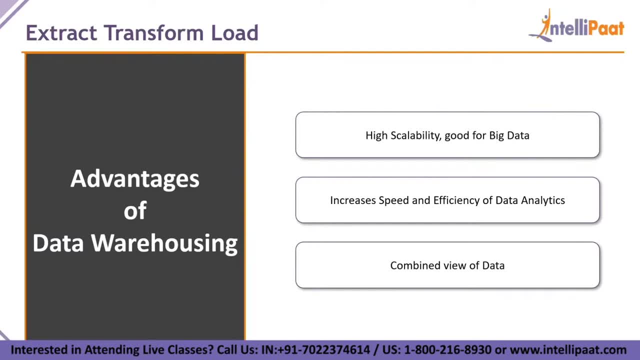 creating data visualizations right. having that combined and aggregate view of data is extremely important, because you cannot have five different data sources and then you can try to visualize it or show it to anybody. nobody will understand the meaning of what you have found or what your analytics model has been, so you need to combine all of it together to be able to query it in a 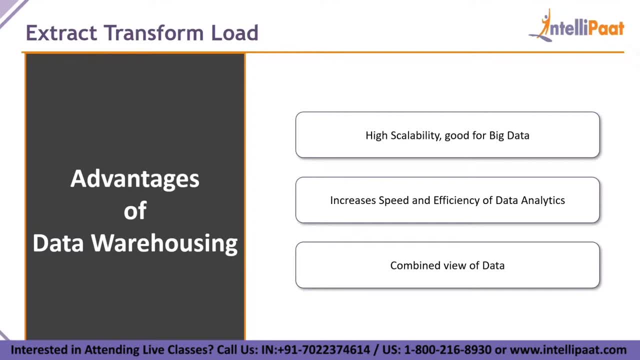 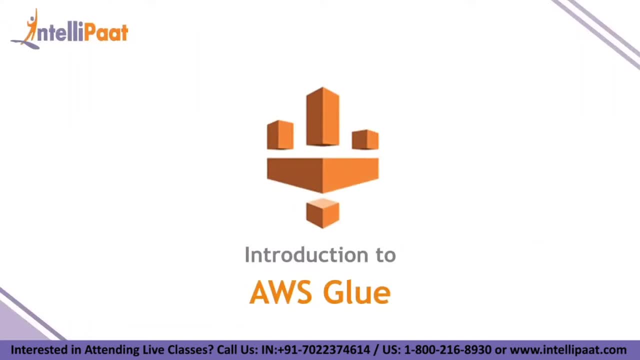 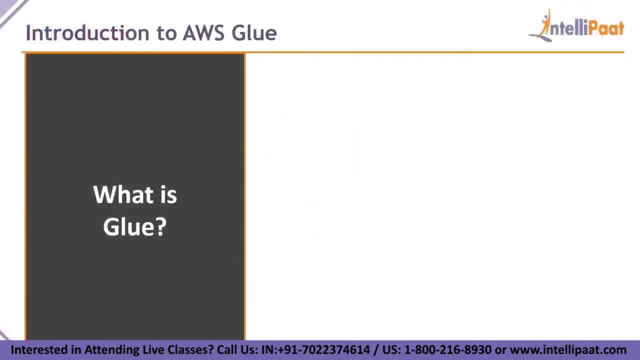 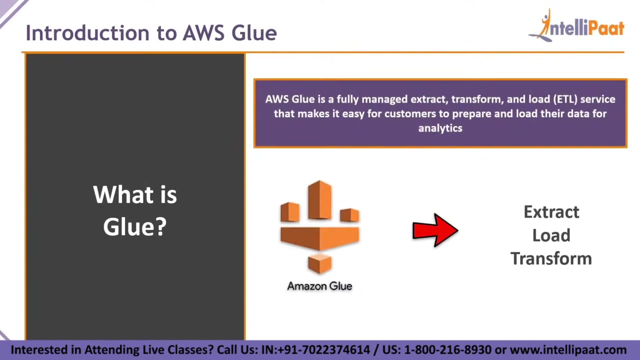 convenient fashion. so that also brings us to our tool that we are going to be using today. there are many data warehousing and etl tools out there, but aws glue is particularly suited for big data, right? so what is aws clue? aws clue is a fully managed extract, transform and load etl service, as we discussed earlier. that makes 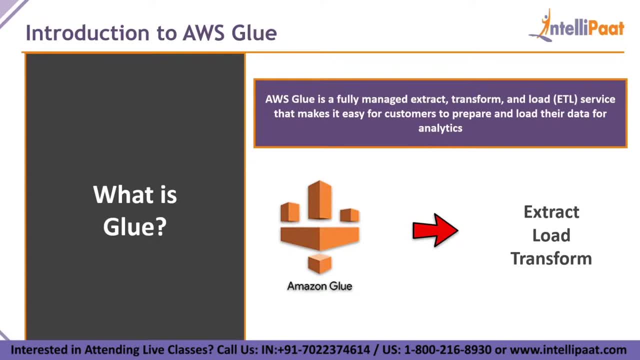 it easy for customers to prepare and load their data for analytics right, so that is pretty straightforward. it is especially suited for big data because with amazon you get a cluster based computing system right, you can deploy a lot of resources for your etl service, so you can increase. 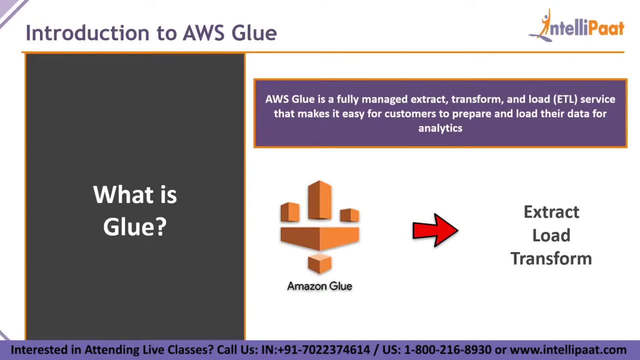 the speed of your service, or decrease the speed of your service at will, depending on the workload. uh, with the amount of resources that you've allocated to it, you don't have to have any local hardware, particularly to be able to run glue. so what are the benefits of glue? the first is: 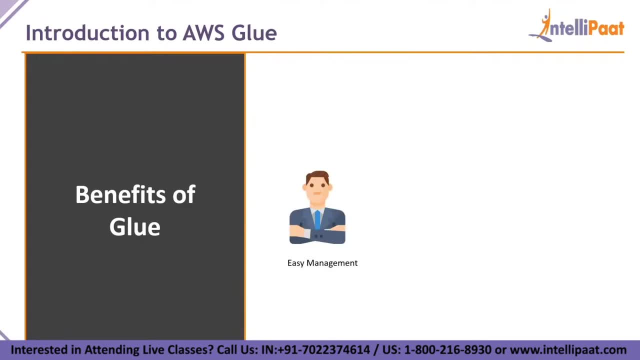 easy management because amazon manages almost everything for you. it has the options for you to allocate the specified amount of resources that you want to specify for your etl job- not more, not less right- and you can scale that up and scale that down pretty easily. so if you have any other issue, amazon manages all of the updates, all of the security patches, all. 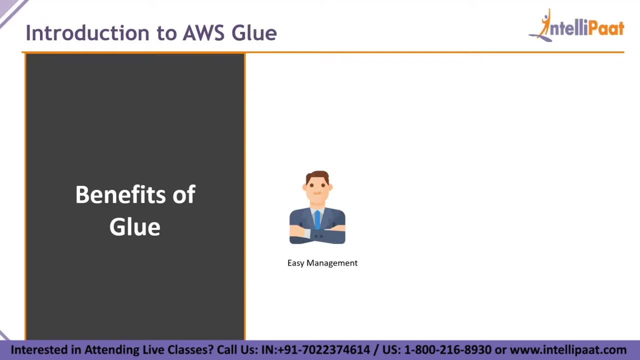 of the version upgrades. you don't have to deploy any maintenance or administrative engineers for that right. so the cloud's computing system makes it really easy for you to be able to data warehouse and use your etl tools with it. next up, it's cost efficient. so amazon is one of the 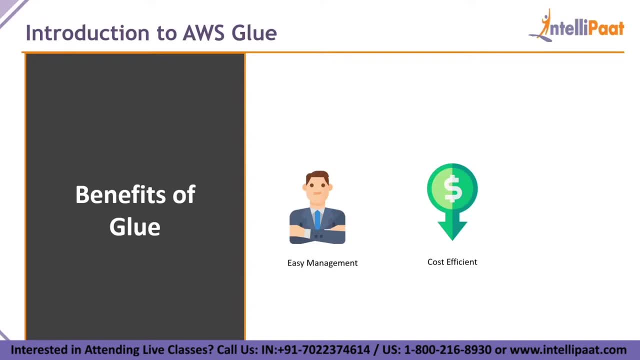 cloud services that comes at really affordable rates. right, it's also cost efficient because you can use it for a bunch of different reasons, i would say for as much of the resources that you're using. right, if you have a server in your own office space, if you have a computer, that is. 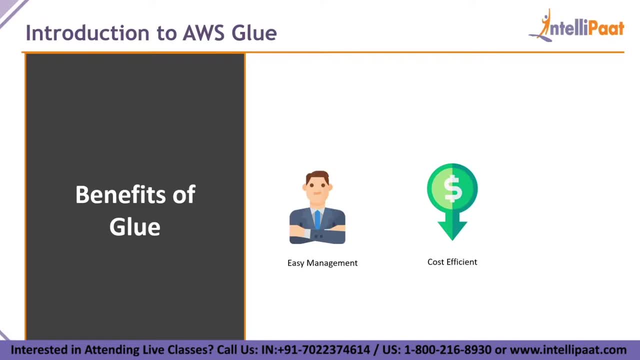 entirely dedicated to that. you still have to keep that running all the time and you have to pay rent for it. you have to pay the administrative team for it, with a maintenance team for it. right in amazon's case, everything is managed and you don't have to pay anybody anything for. 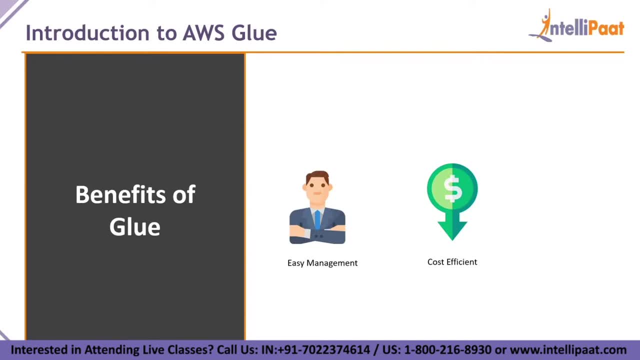 it and you're not renting anything. you only have to pay for the exact percentage or the amount of reason you use for when you use it. so that is why it's cost efficient as well. then we have superior functionality. so with aws glue you don't only get the primary benefits of etl tools, you also. 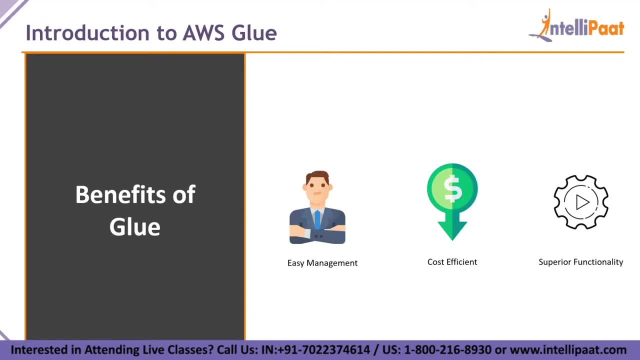 get superior functionality because it's easily integratable with big data. it's easy easily integratable with other services as well- other cloud and offline services and third-party services as well, because amazon, as an organization, aims to provide a compatibility with a lot of things that you would do in your data analytics or your data science career, and it also aims to 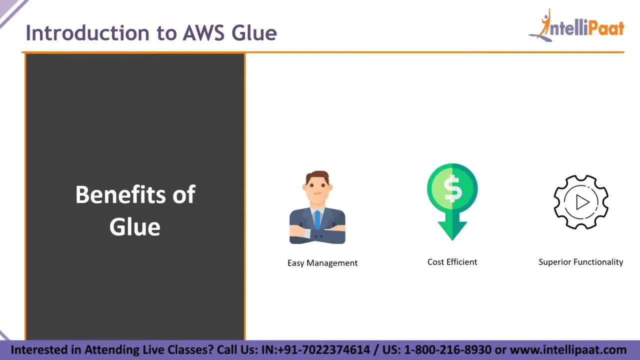 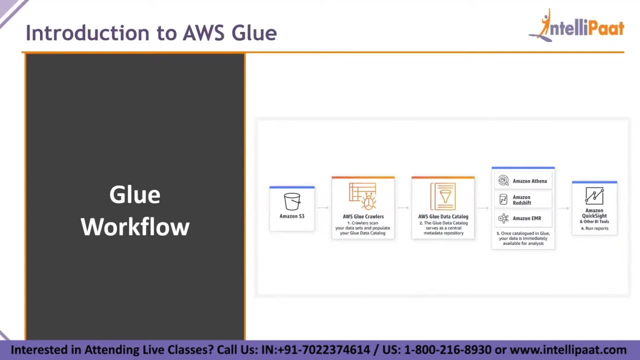 provide organizations with the most affordable and reliable cloud service there is. so let us look at the glue workflow as well before we actually get to the tutorial. so say, you have some data present in your amazon and cloud services. so let us look at the glue workflow as well before we actually get to the tutorial. so say, you have some data present in your amazon and 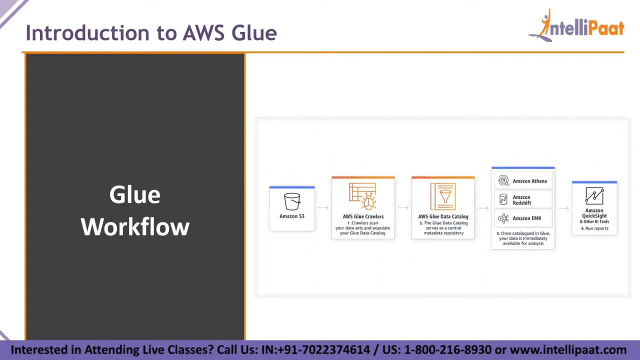 s3 bucket, amazon. s3 is a data storage service in aws and then you take some data using aws glue crawlers. now, crawlers are mini services present within aws glue that scan your data set right. they scan your data set. they generate the meta metadata out of that data set right. they catalog that data. 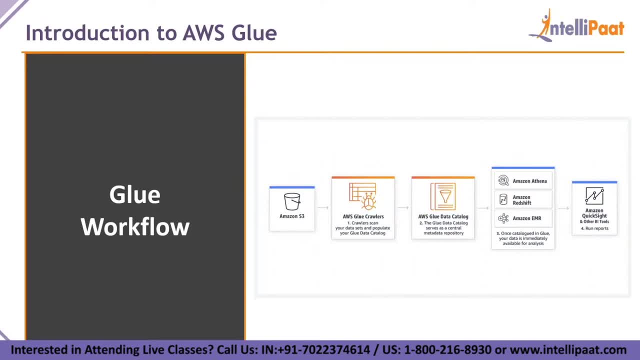 and they also create a virtual database out of this catalog data. right? so you have generated your aws glue data catalog after that point, right, that is the second step. right, it serves as a central metadata repository and then you can use this repository for a various plethora of services. 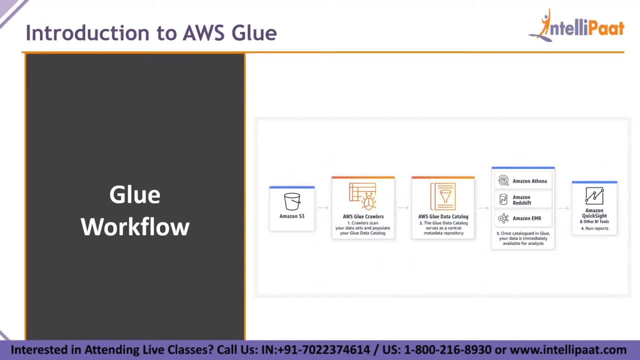 right now that your data has been cataloged, it has been transformed uh. after your glue service has ran on it, uh. you can then integrate it with other aws services like amazon athena, which is an actual uh data warehousing service, amazon redshift- same uh. you can use it with amazon emr services. 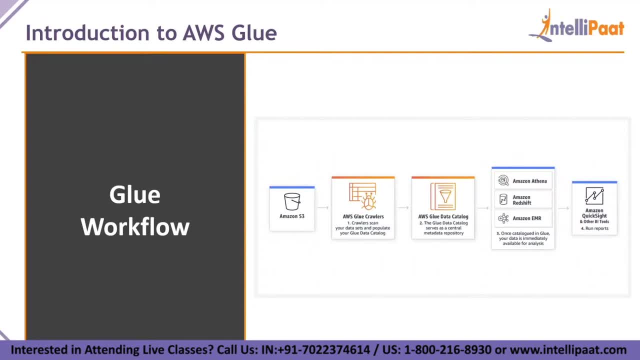 as well with say: uh, hive, right. so these are the three services that you can use it with, and there are other services as well. and then uh, once you have warehoused that data, you can essentially use your data visualization tools with it. so amazon quick site is a data visualization tool that is. 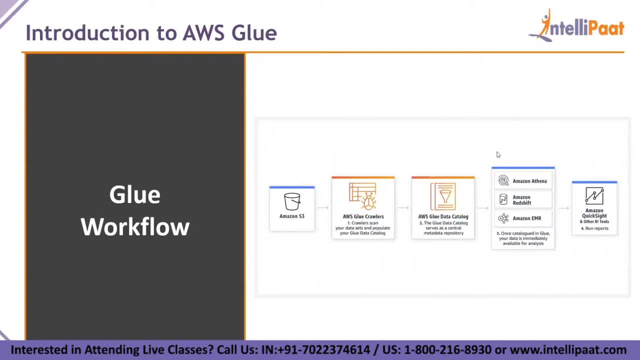 present in the aws services so you can integrate it with your data warehousing. the part that i want you to focus on particularly here: are these two blocks right? so this is the task of the data warehouse aws glue, which is the etl task, and then, from then on, this is. these are the data warehousing services. 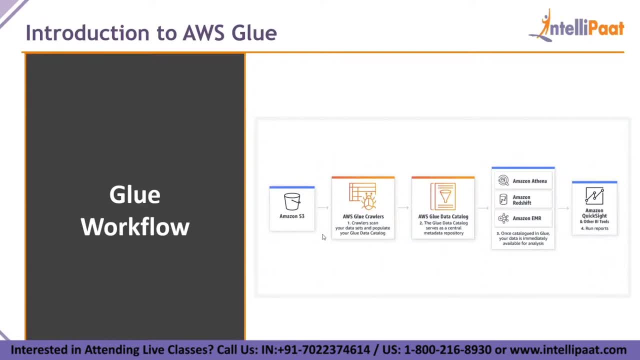 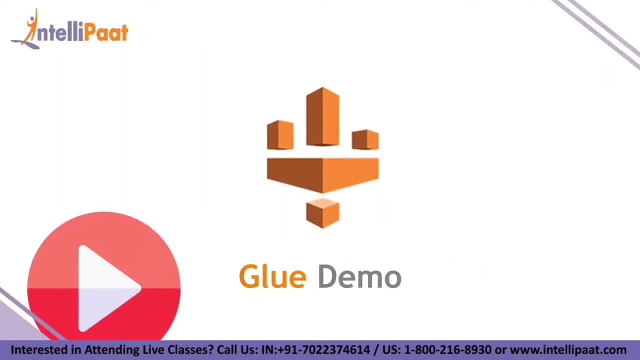 this is the data visualization tool and this is the storage service. so let us go to the glue demo that we have for today. we are going to be crawling some data out of amazon s3 and then we are going to be putting it back into amazon s3 after we've 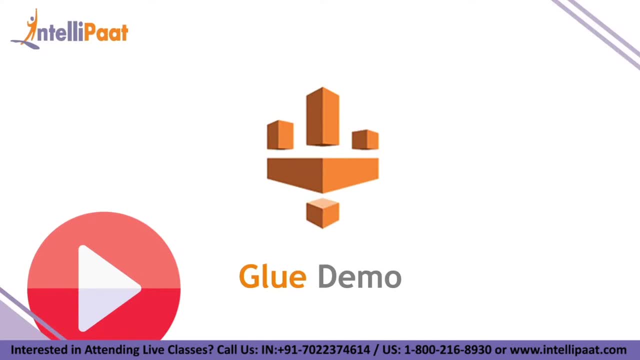 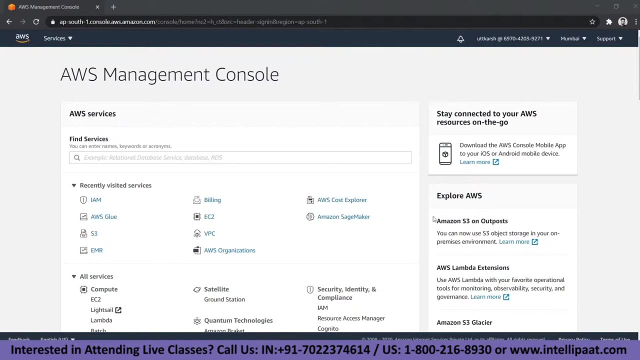 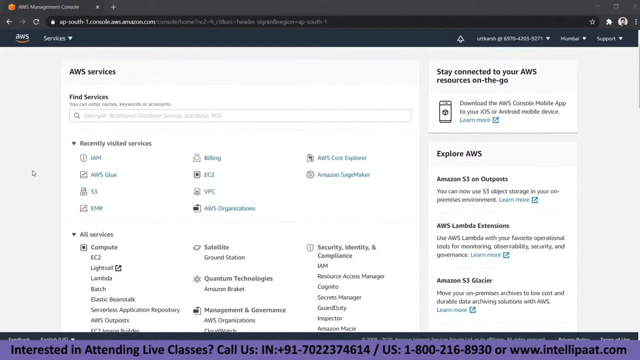 cataloged it. whatever we have cataloged and however we have transformed it, so we are currently in the aws management console. aws provides a very convenient console for you to select your services from, so the first thing that i want to do is upload my data set. actually, 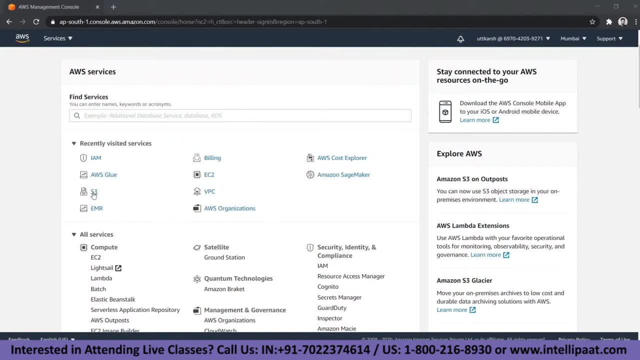 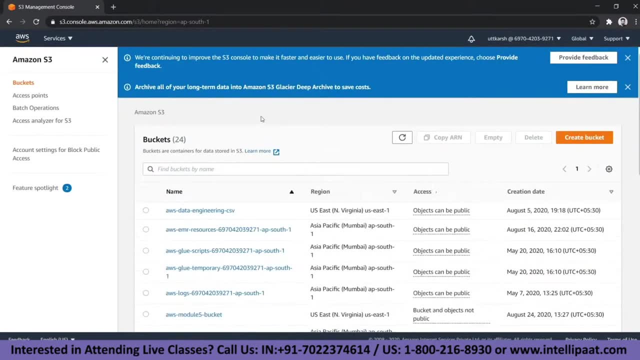 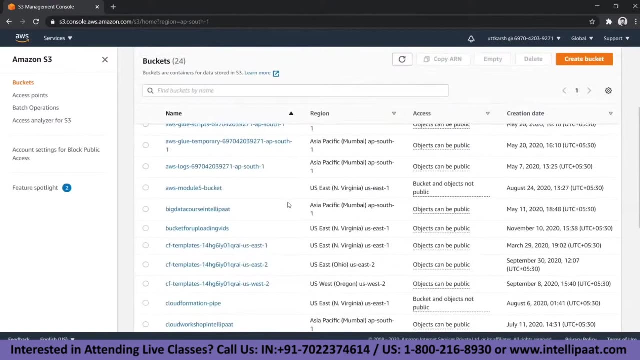 so i'm going to be selecting amazon s3, right? so this is essentially like your google drive, right? if you want to store extremely large data sets, you can go ahead and do that. you can go for the paid version of it, but if you want to store small things, uh, the default free. 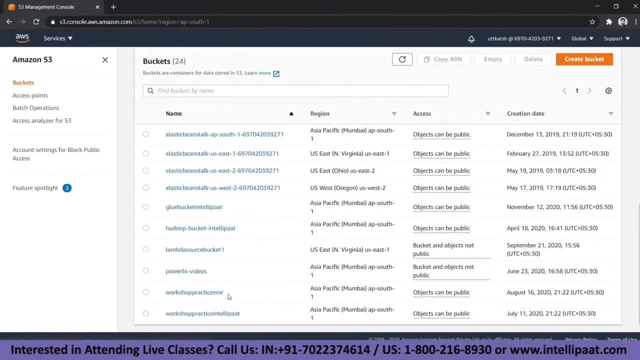 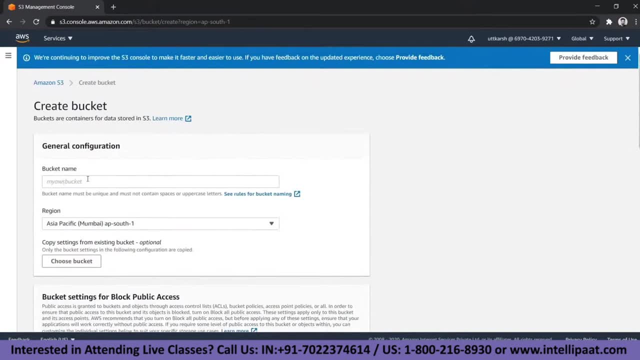 tier version works as well. you don't have to pay anything for storing small data sets, right. so the first thing that i would do is create a bucket. so in this bucket, since i don't want to deal with permissions specifically right now, i'm going to be allowing all public access. 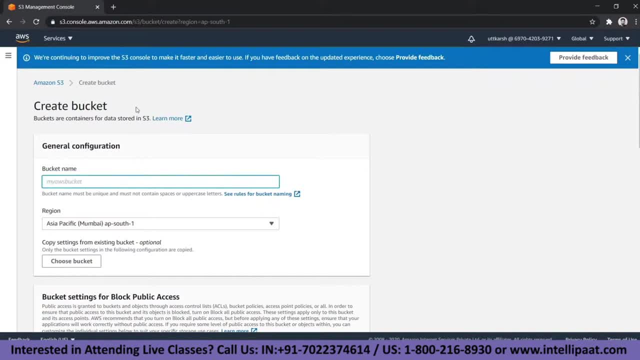 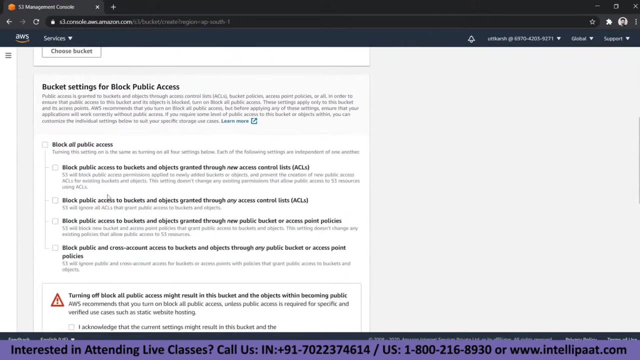 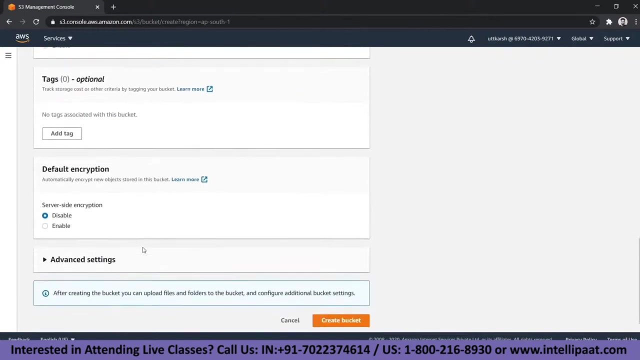 so the first thing that i would do is call my bucket something. so let us call this: um youtube glue right, let's call it that. maybe that name has been taken, but we'll see- and then untick this, which is block all public access. i acknowledge that it will ask you for a waiver and then 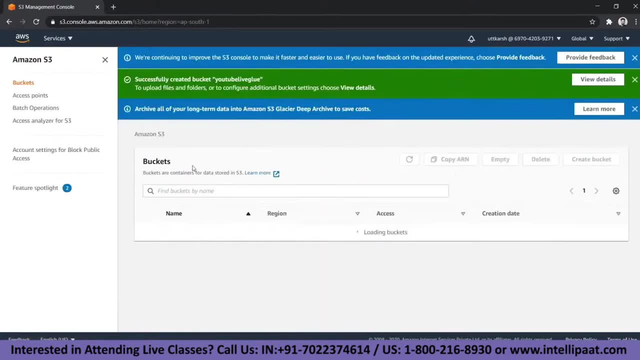 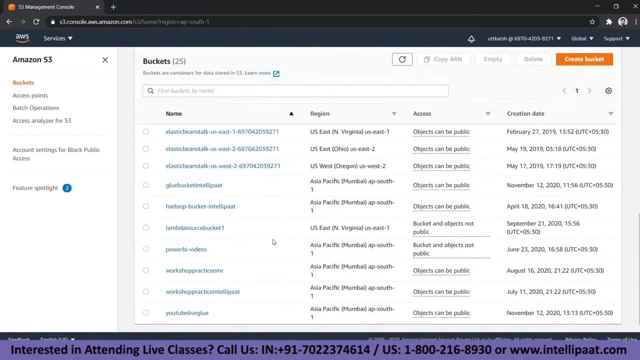 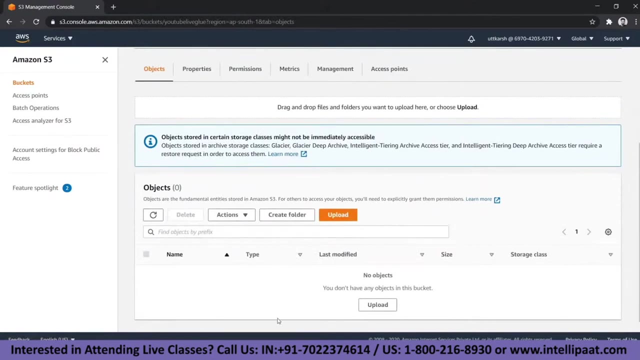 we will click on create bucket. right, so that name wasn't taken and we have created that bucket, which is publicly accessible. uh, in this particular scenario, right, so this is our bucket. we go into that. we create two folders that we are going to be using. so the first folder that we are 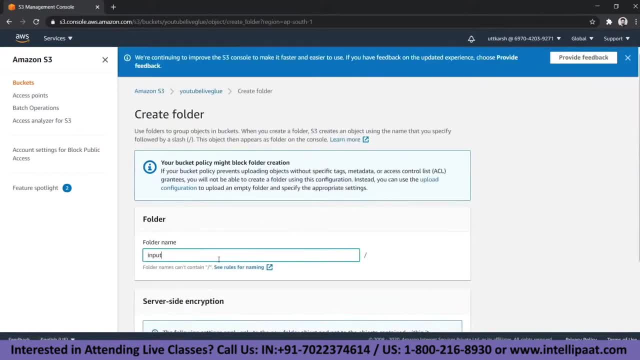 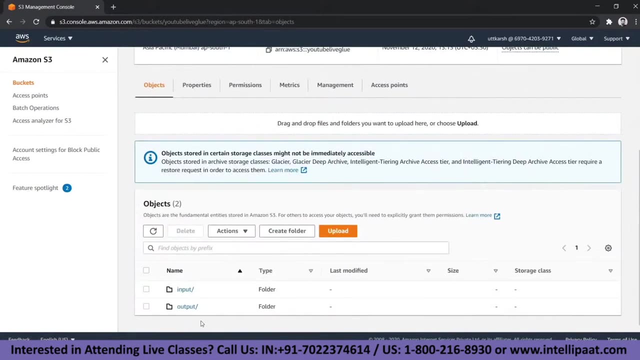 going to be using is the input folder, where we are going to be uploading our data set. we'll create that. and the second folder that we'll be creating is the output folder, and we'll create that as well. right, we have two folders now, and the input folder will be uploading our data set. 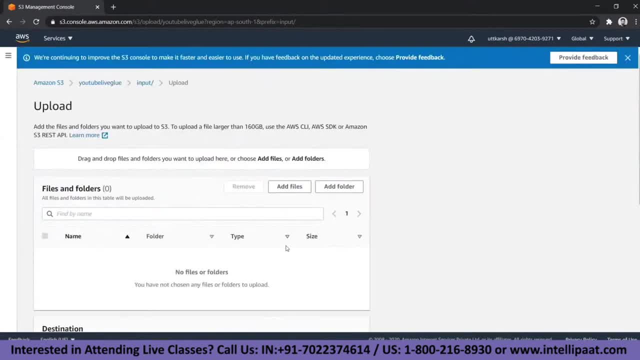 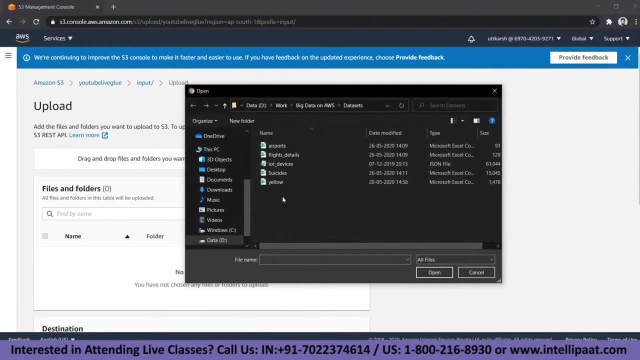 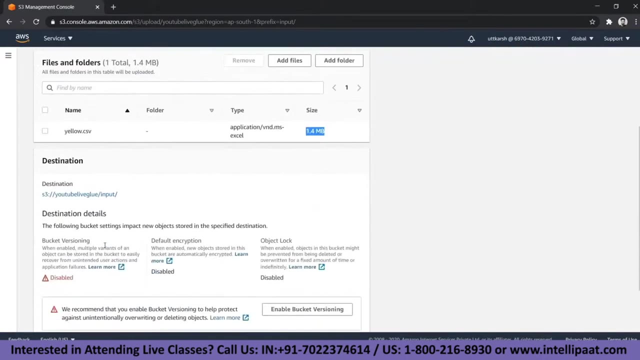 so we'll click on upload and go to add files and then we can select anything. so, uh, let us go for the taxi cab data that we have, the yellow dot csv it's of 1.4 mb, right, and then we're going to be clicking on upload. 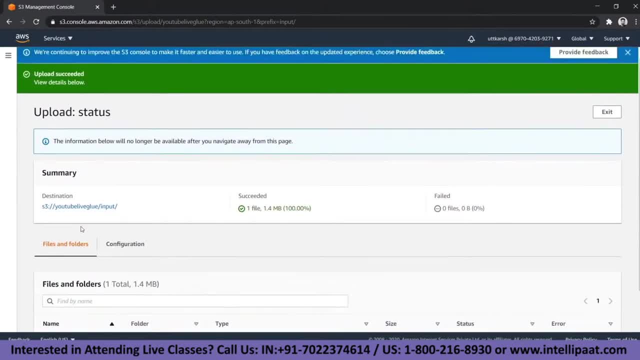 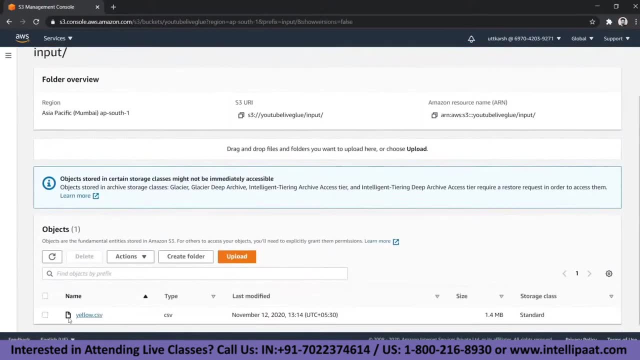 so it got uploaded. now it's there present in our folder. so if i look at the folder again, we have the input and we have our yellow dot csv within the input folder. now the aws task is done. for now this s3 task is done. so i'll go to glue now. so i'll open up aws glue. 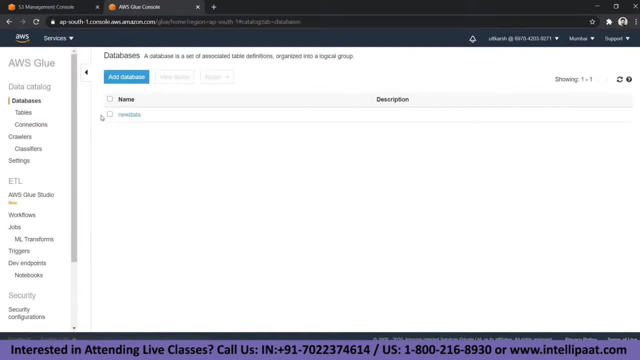 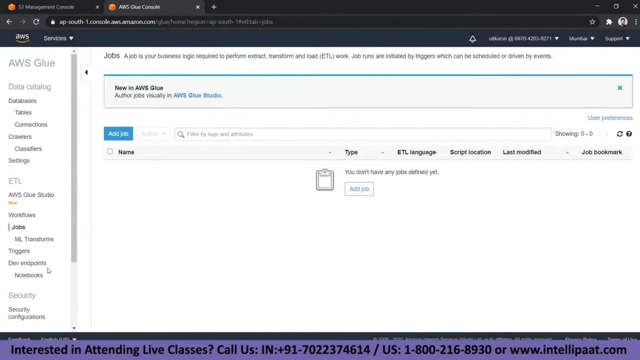 right, first i'll delete any databases that i already have to avoid any sort of conflict, and i'll delete my job as well. right, then i'll go to crawlers. so this is the part where we're actually, uh, uh, basically picking that data up from s3. so we'll delete this pre-existing crawler. 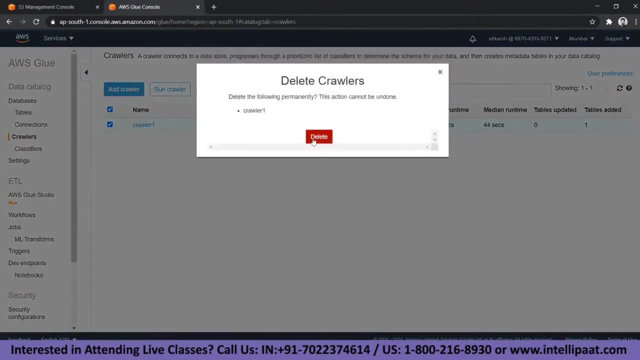 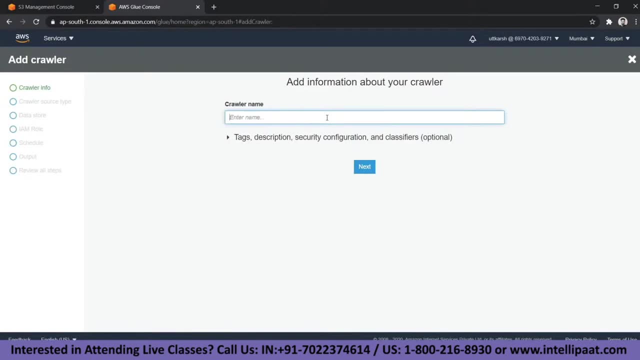 go to add crawler and create a new crawler, so let us call this yt live. and then we're going to create a new crawler, so let us call this yt live. click on add a Polit muscle and click on next. we are going to be choosing the source type as data. 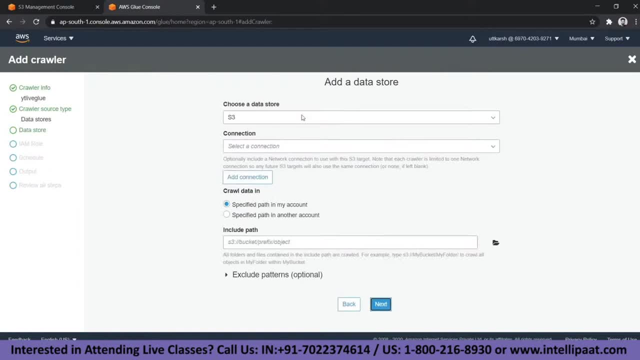 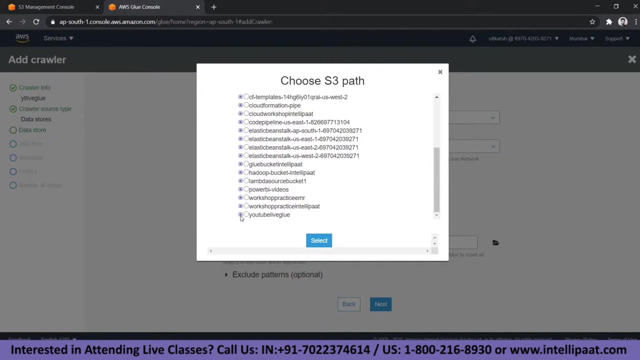 stores, which is in s3, and we're going to be crawling on everything that is present in that particular folder, in that particular directory. then the data store is s3 and i want to choose a specified path folder that I had created earlier on this particular bucket. so once I expand that, I have 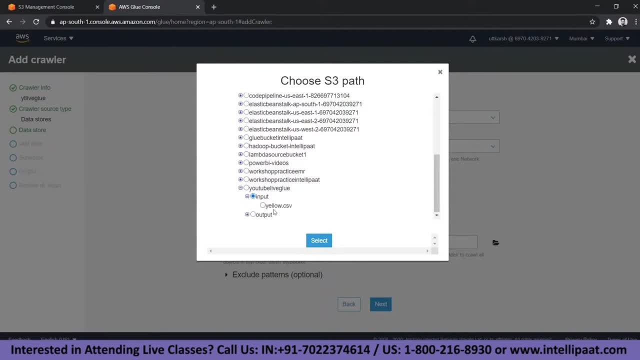 the option of selecting input and within input we have yellow dot csv. we're not going to be selecting that because we could have had multiple data sets. right in this case we only have one. but if you have multiple data sets, the best way to go about it is to select the folder that houses your data. 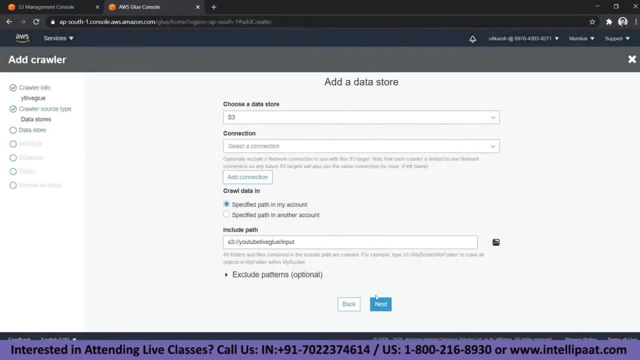 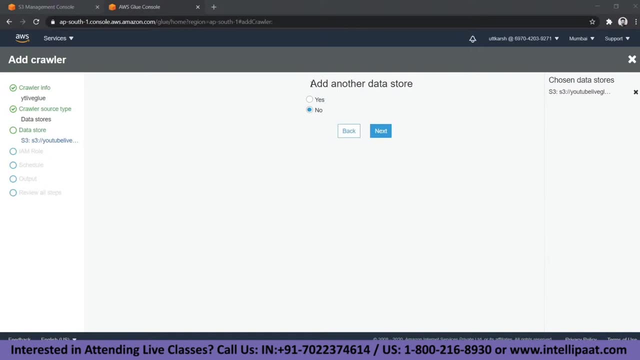 set rather than selecting the data set itself, and we'll click on next. it is asking us whether we want to add another data store. we don't, so we'll click on no and click on next. and then it is asking us to choose an IAM role. now in Amazon, there are a lot of permissions. 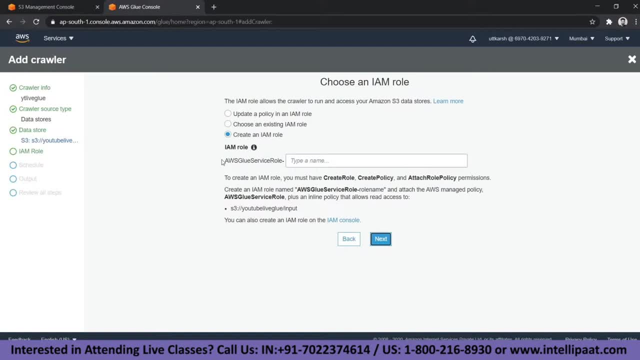 that you need to deal with right, because data security is a top priority for Amazon. so you need to specify roles for every particular task that you're doing, and it depends on your account privileges whether you're using a data store or not. so we're going to select IAM role and then 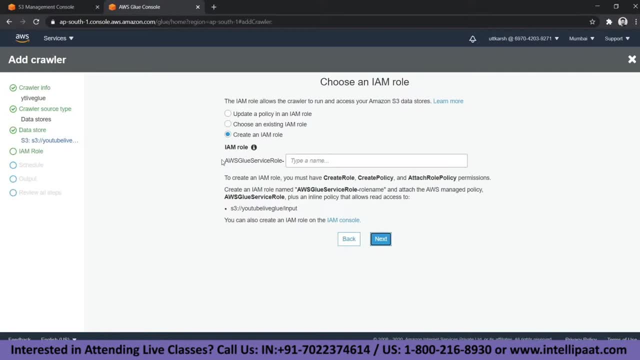 we're going to select IAM role, and then we're going to select IAM role, and then we're going to select you're working as an employee in an organization on their AWS account and how many permissions you've been assigned and which services you can integrate with which service. All of these things 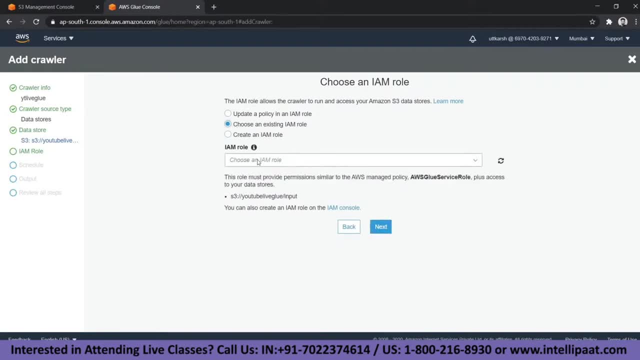 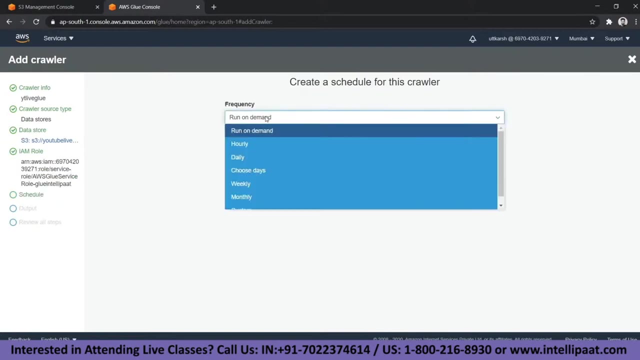 are dependent on IAM roles. So for this particular purpose, I have created an IAM role already which gives me access to the Amazon S3 bucket right. So there will be no permission clashes. And then I'll click on. next I'll select in the frequency tab. I'll select run on demand because 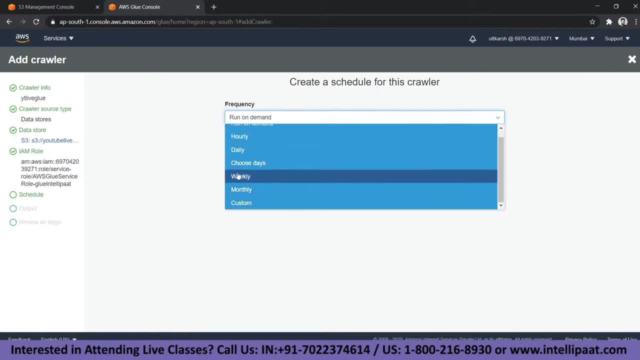 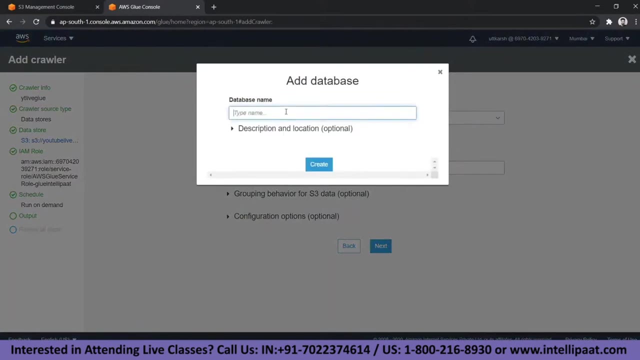 I don't want to run the scroller at a periodic level. I only want to run it whenever I click on run. I'll click on next, And then it asks me to create a virtual database, So I'll create one. So let us call this virtual create. 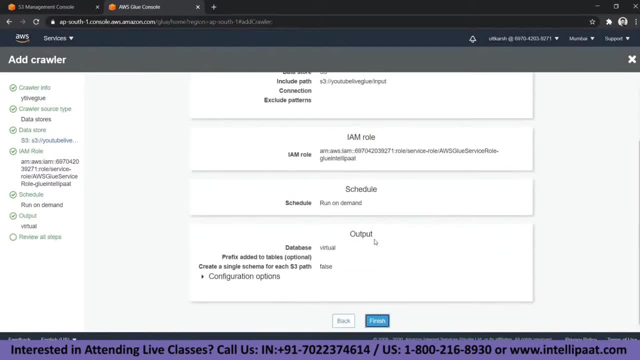 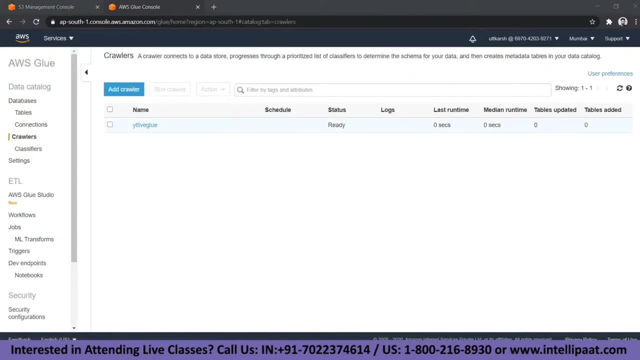 And then we'll click on next. So once we have done that, we'll click on finish. So since the crawler is set or to run on demand- it's not actually set to run periodically or automatically- we have to manually start it. So we'll click on the crawler and we'll click on run. 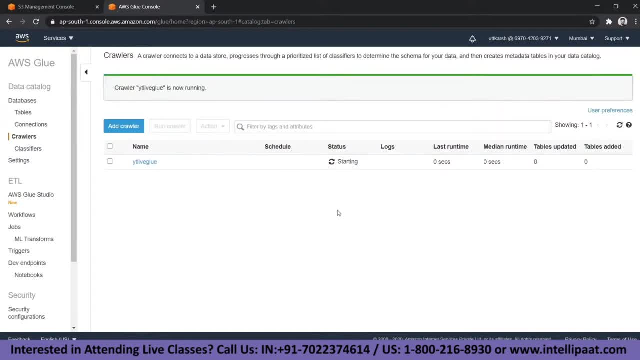 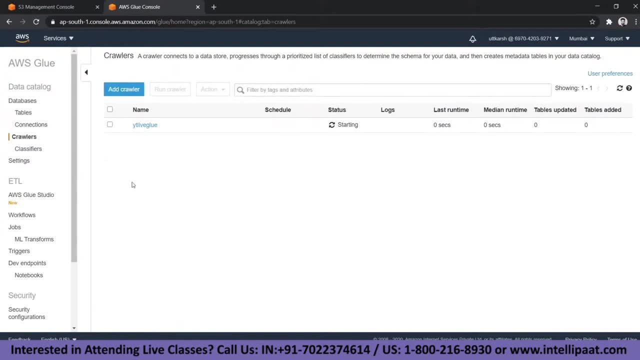 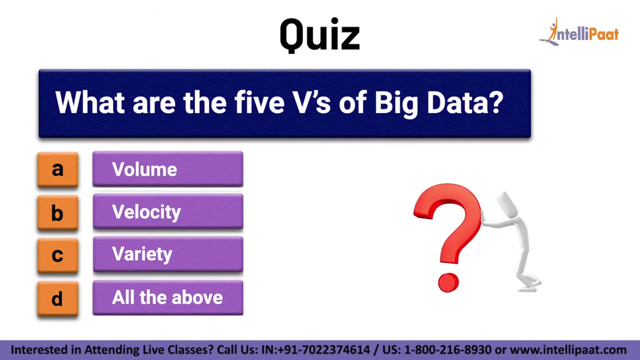 Now it is running. it will take some time and then it will create the virtual database with the data cataloged in it. Just a quick info, guys. test your knowledge of big data by answering this question: What are the five V's of big data? 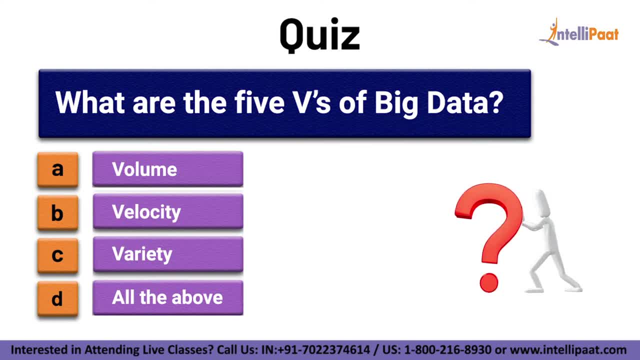 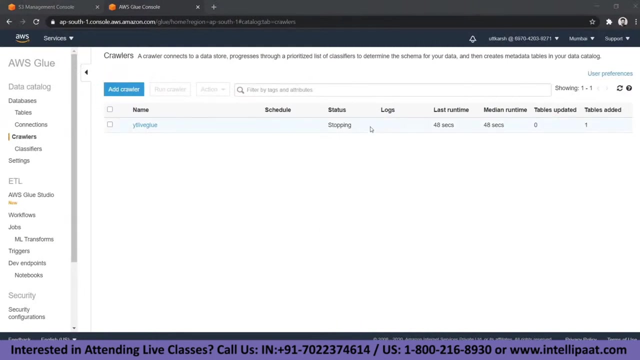 A, Volume B, Velocity C, Variety D- All of the above. Comment your answer in the comment section below And if you have any questions, feel free to ask them in the comments section. Now let's continue with the session. So as we can see now that the data crawler is now stopping, 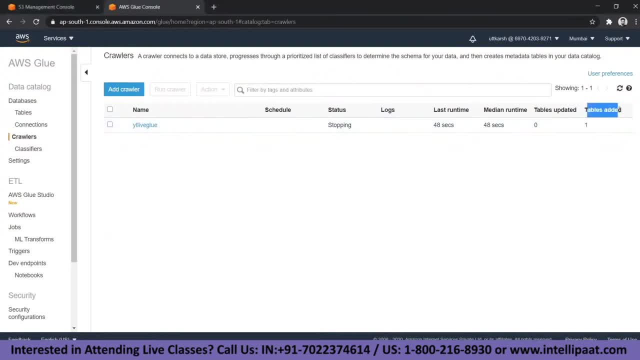 right and we can see that one table has been added. So it was earlier zero, now it's one. So we'll wait for it to be ready And meanwhile we can also check in the databases So once we refresh it we're able to see that a. 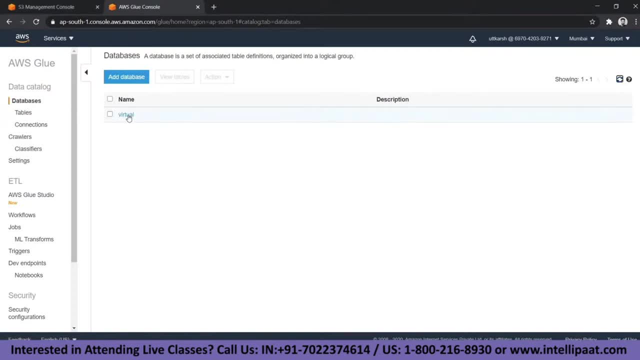 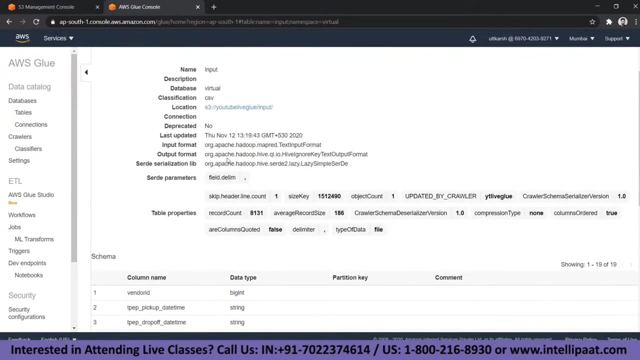 database called virtual has been created and once we open the virtual database and we click on tables in virtual, we can see that there is one table called input right. if we open that we can see that our taxi cab data set has been accepted and the metadata is obviously there. 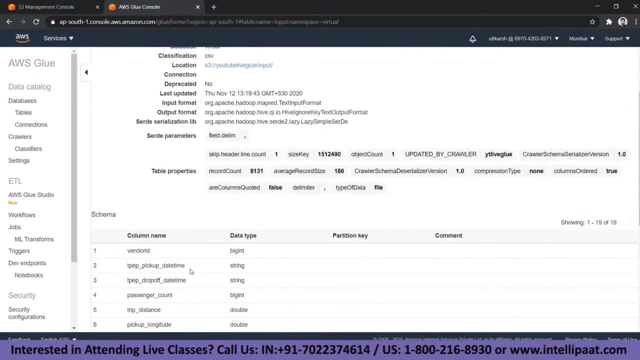 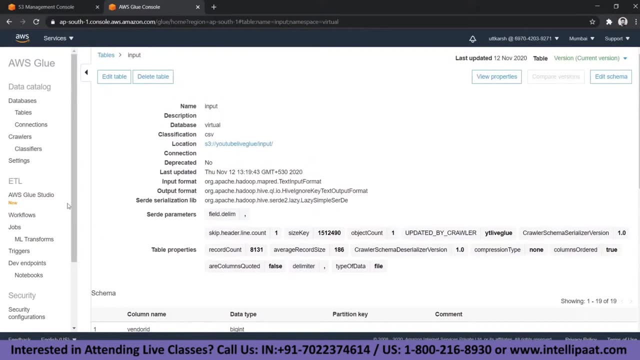 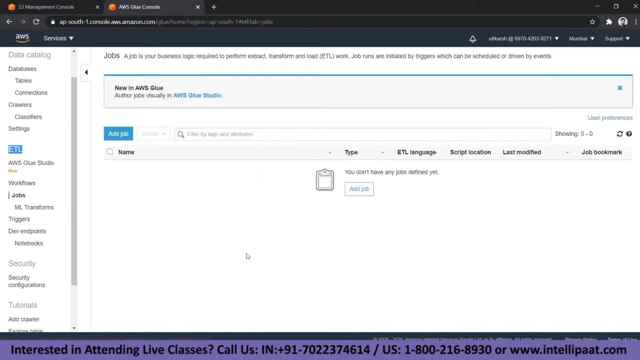 so we can see that and we can see the data types for each of the columns. so the next thing that we can do after creating the metadata is actually start our etl job. so for that we'll go to the etl tab over here and we'll click on jobs, right. so there are no jobs that are. 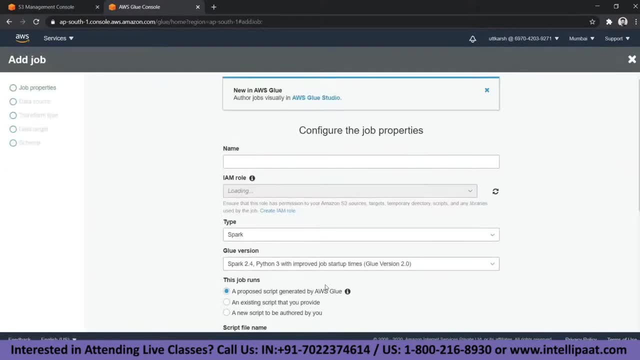 currently there that we can run, so we'll click on add job. right, so we can call this job anything. so let us call this job yt live job and we'll click on add job so we can call this job anything. so let us call this job yt live job. 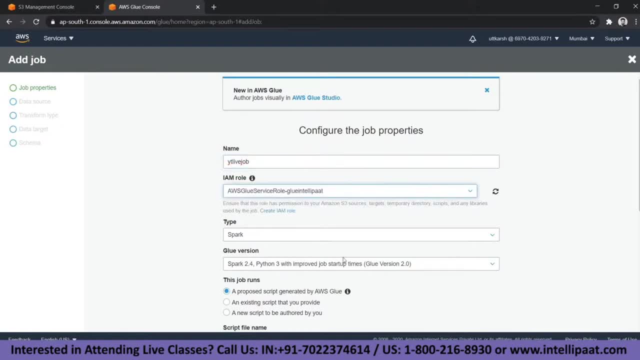 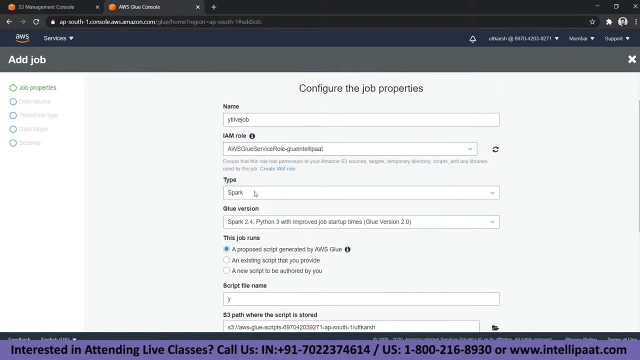 and we'll choose an iam role, we'll select the same iam role and we can select the technology stack that we want to run this on. so, for this particular case, we are going to be using spark, which is a very prevalent technology in the case of big data, and we're going to be going with spark with a 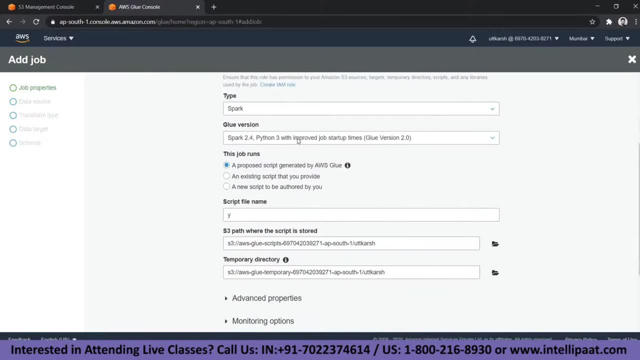 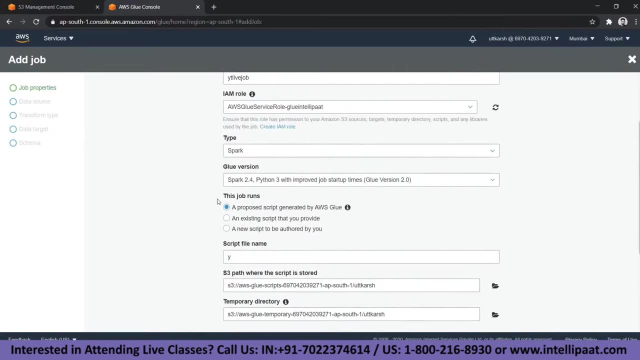 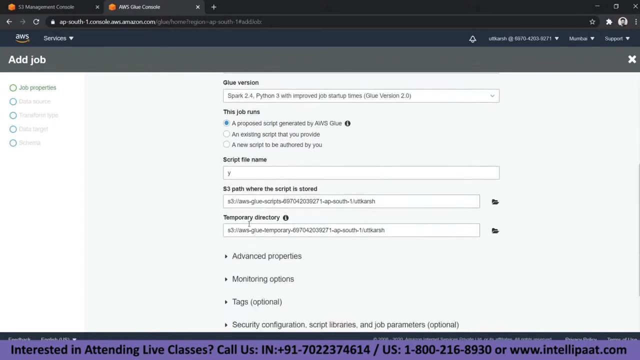 python uh language. so we're going to be using pi spark essentially, and then we have an option of customizing our script so we can use custom etl scripts. we're just going to be going with the proposed default script, that amazon gives us right, and then next up we will be actually. 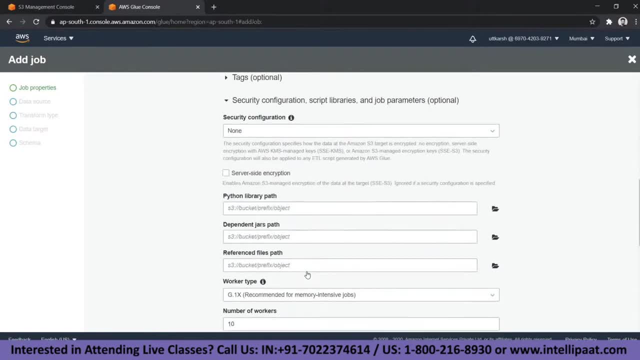 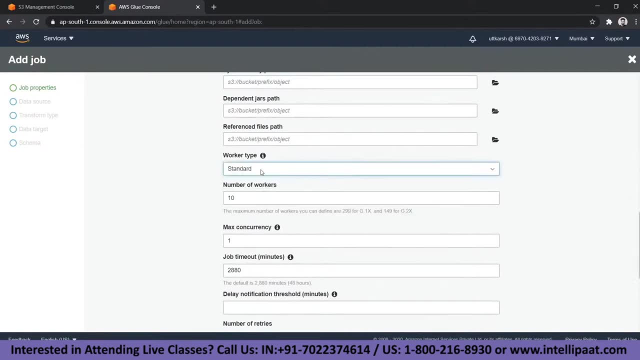 going ahead with the security configurations and actually reducing the number of resources and the amount of resources we're using. so we're going to be putting the worker type to standard right, because this is not a memory intensive job. the file is only a 1.4 mb, so we're not actually doing any. 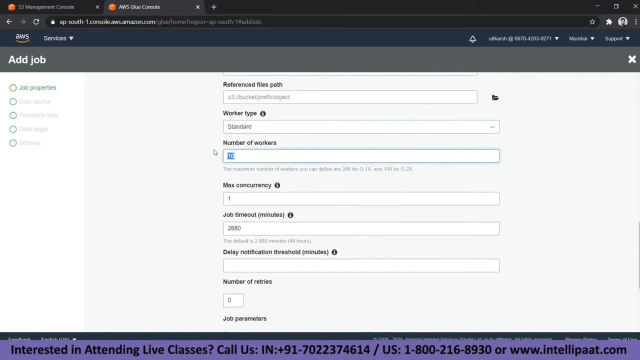 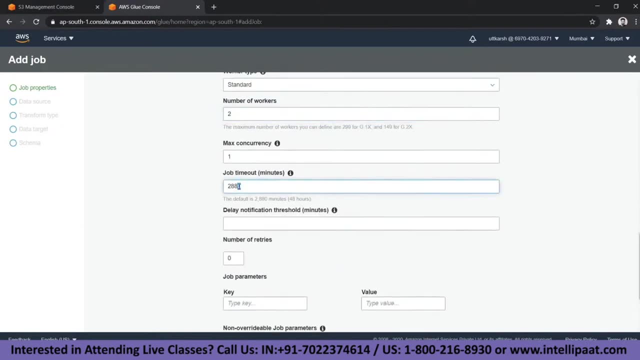 thing very memory intensive and the number of workers will reduce to 2 right and the job timeout is 2880 minutes. so this is for industry level job timeout standards. we'll put this to 10 because we're just doing a practice session over here and then we'll click on next. 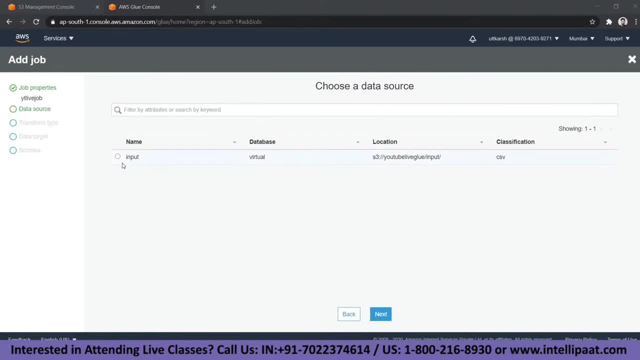 so next up we have to select our data source. so in this particular case, our data source is in the input. it's in the input table that we had virtually created, and then we'll click on next right, and the default option over here is change schema. so we'll go over there and click on next. 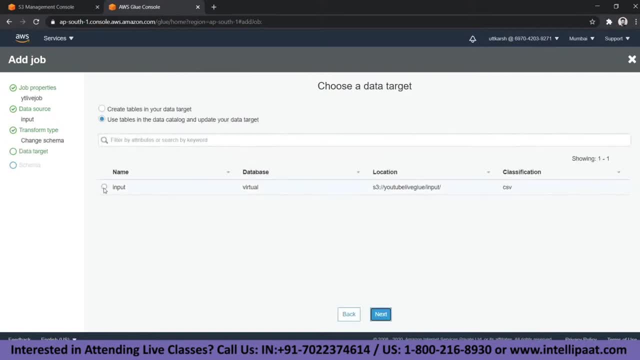 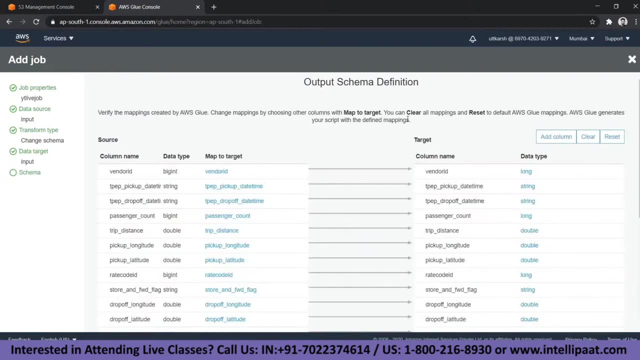 right, so the target in our virtual database would be input as well, because we're going to be changing our input schema, and then it gives us a rundown of how these things look. right, so default in s3 it was detected as bigint, but now some things have been by default detected as long. 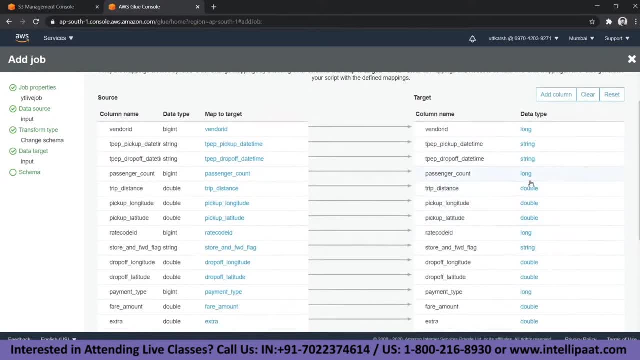 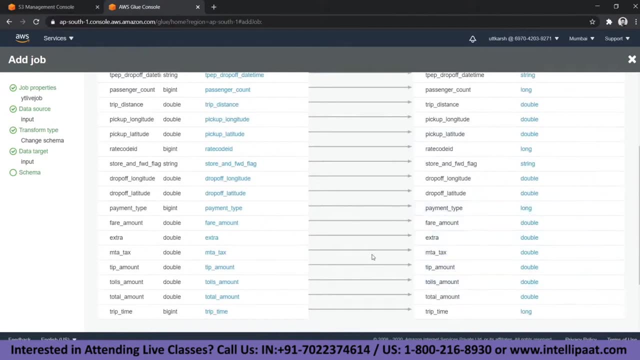 the times have been detected as string values. the passenger count has been detected as long. so all of the data types have been appropriately detected by amazon itself. but you have the option of adding new columns over here, resetting this to the default values. you can do anything with. 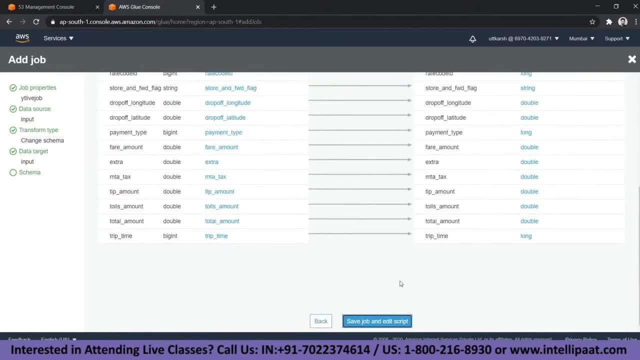 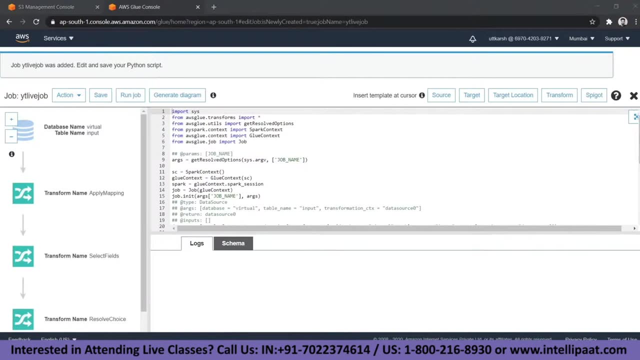 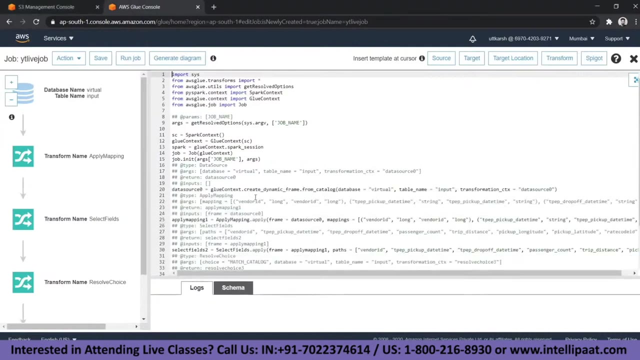 it for now. we're just going to go with what amazon has detected for us. we're going to save the job and edit the script. now, when we get to the edit script part of things, we can see the pi spark code that is going to be extracting, transforming and loading our data right. so this is the default script that you're. 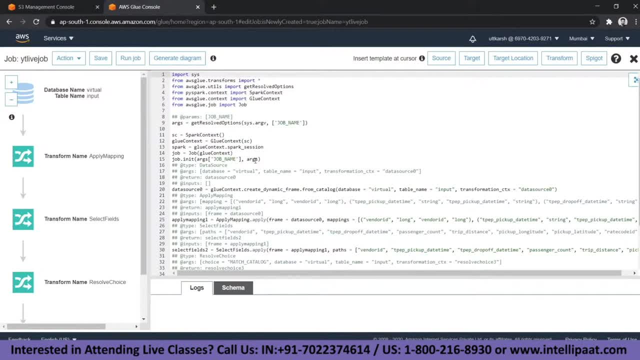 getting with amazon. you can write your own custom script for it, so i have one that is currently written already, so we are going to be using that in order to store our data, our transformed data, into our s3 bucket, the output folder that we had created earlier on. 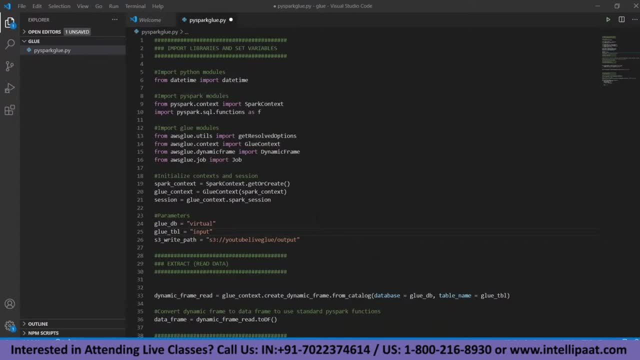 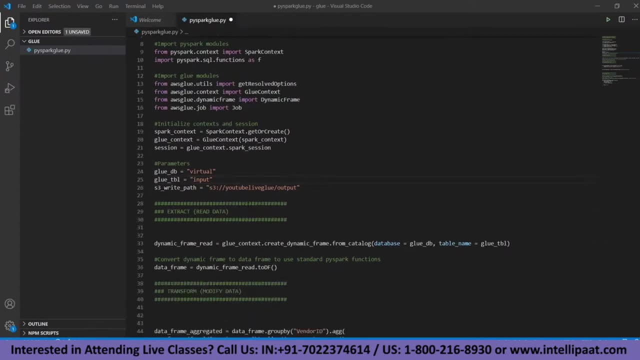 so i already have my pi spark code written for this. so we have imported a few modules from the aws glue package and we are going to be using them. so first thing that i have specified are the parameters. so the database that i have created is called virtual, the table is input and the right 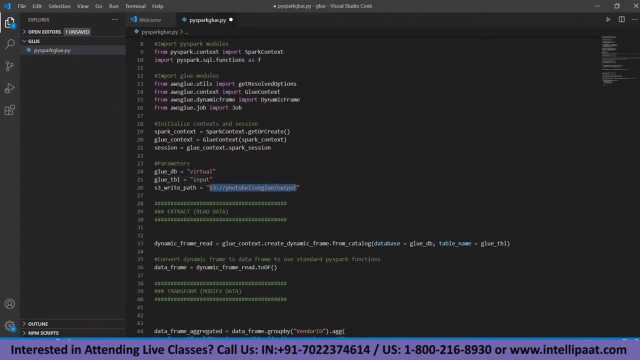 path is the output folder that we had created in our s3 bucket. so we have to specify all of that. so the first part is obviously extracting the data right. so this particular function create dynamic frame from catalog. so the data that has been cataloged in our virtual database we are taking 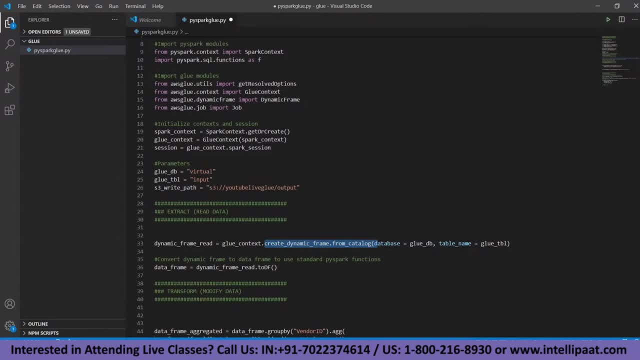 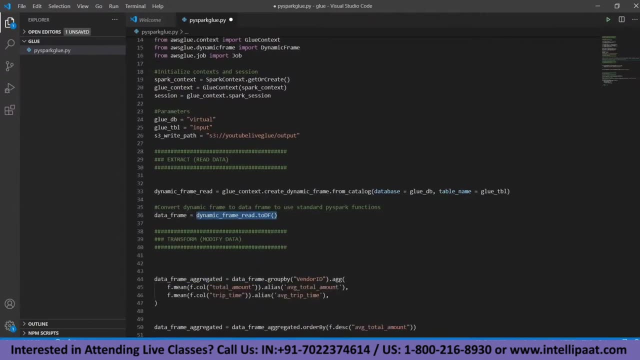 it from there and then we are essentially extracting it and we are converting it into a data frame. now data frame is quite similar to an sql table, where we can perform our transformations quite easily. and then we are creating another data frame. we are calling it data frame aggregated. 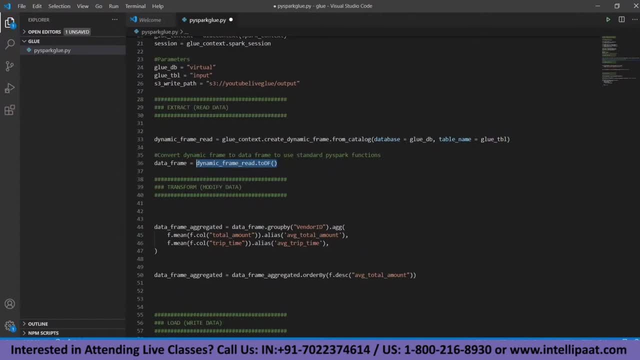 and this particular data that we are creating out of the old data contains the vendor id, which is the id of the cab driver, which could be one or two depending on the type of cab that the person drives. we have the total amount of the fare of the trip and we are averaging that to. 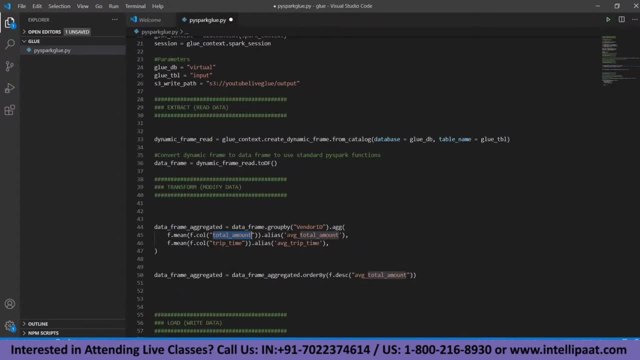 the average of the total amount. so So we're grouping it by vendor ID, and each vendor ID will display the average total amount and the average trip time taken right. So these are the two things that we're aggregating essentially, And then we'll get our final data set based on it. 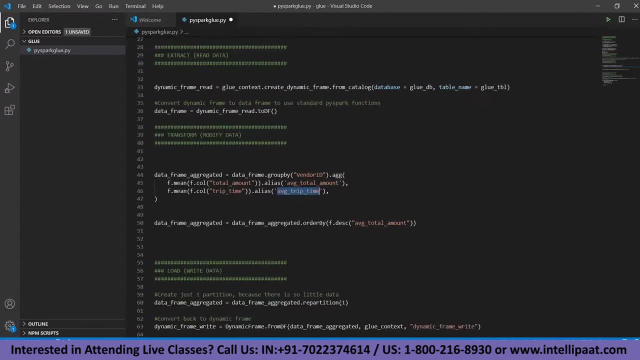 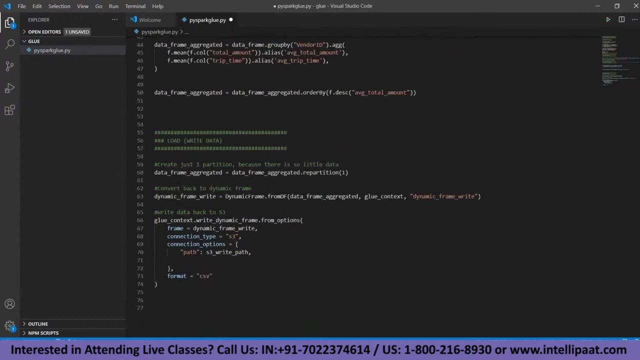 And we're also arranging this data frame in the descending order of the average total amount. So whichever vendor ID has the highest average total amount, it'll come at the top of the table And then finally, after the transformation has been done, the third part, which is loading. 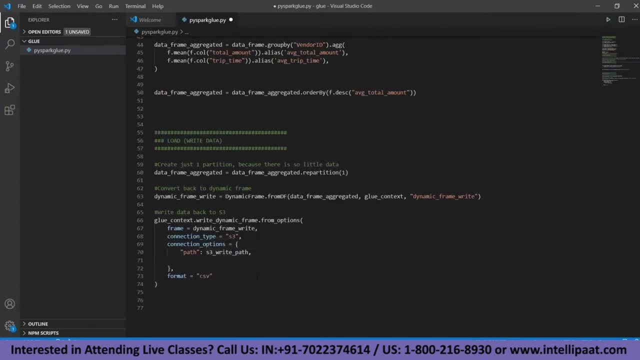 So we're essentially putting that data into S3, into the output folder. we're essentially loading it into S3.. We can also put it into Redshift or Athena, or we can put it into EMR as well. it is up to us. 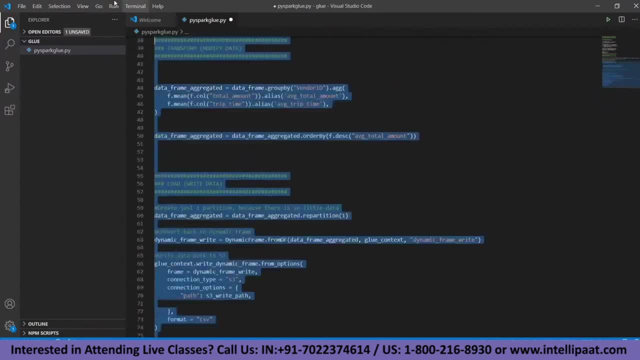 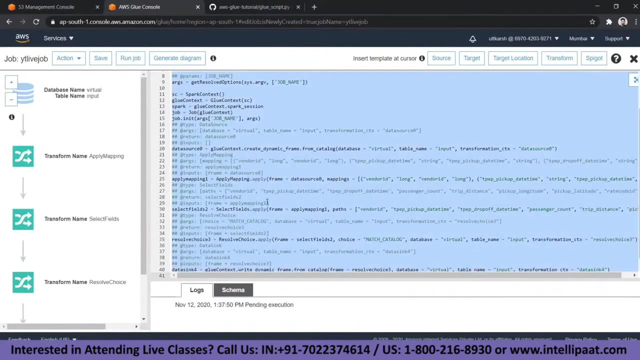 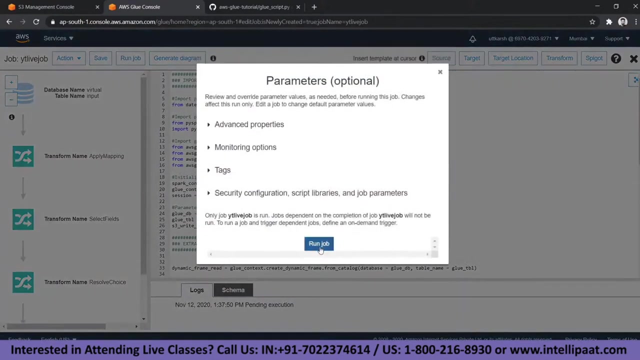 And the format is CSV again. So I'll copy all of this, right, And then I'll put it instead of this code. I'll select this and I'll remove that and put this code instead of that, And then I'll click on run job. 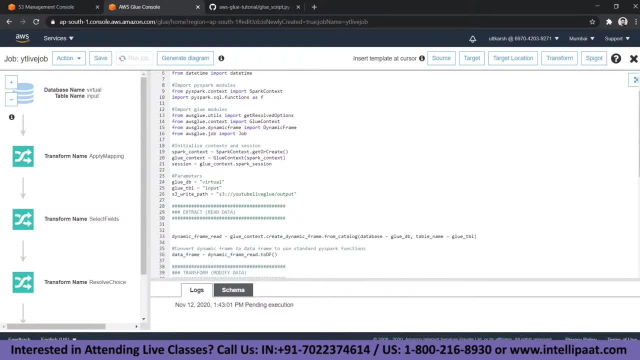 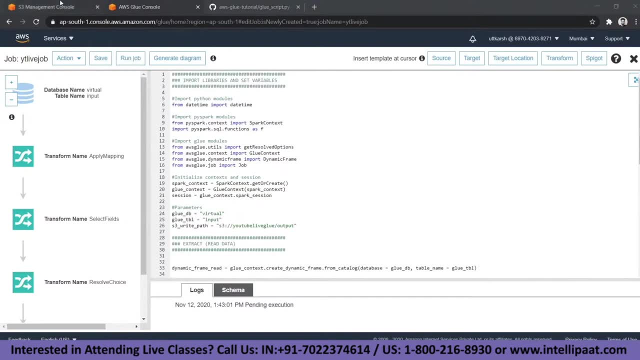 So the job is running, as we can see, and it'll take some time. So when we see that the running job process has finished, then we can simply go back to our S3 console. We have two folders. We had the input folder. 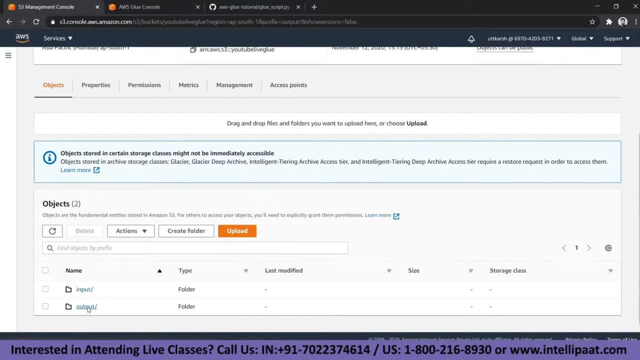 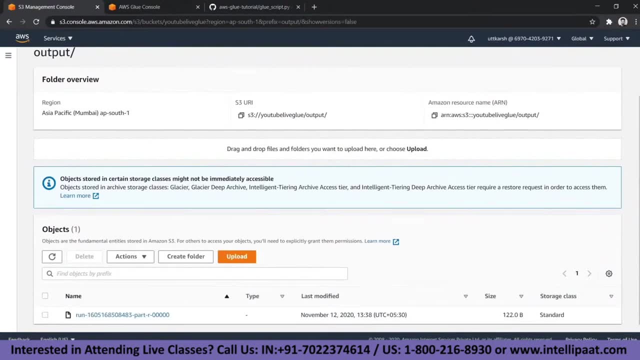 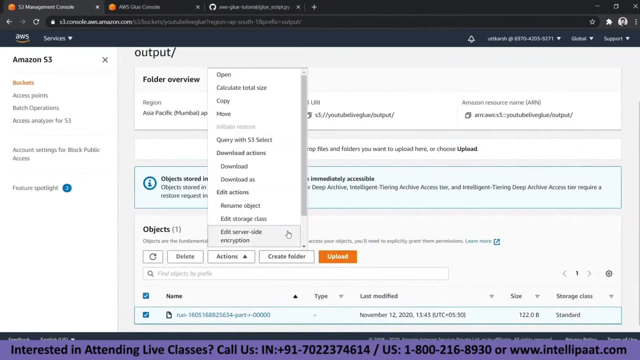 We'll open up the output folder to see if anything has been created. So we can see that a part file has been generated. It's of 122 bytes, So it means there is something in it. So we'll download this first. So we will click on it and we'll click on actions and we'll click on download as right. 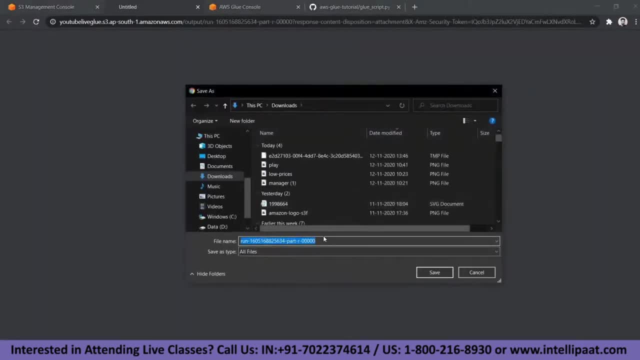 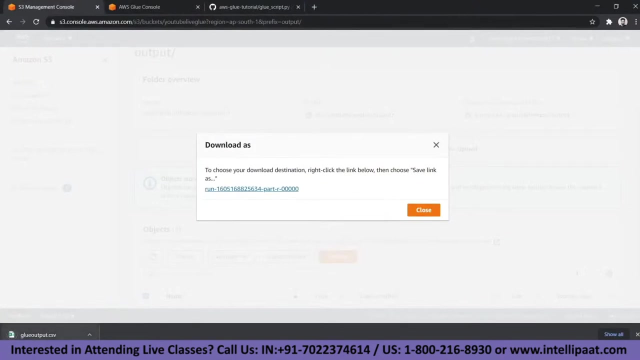 So firstly we'll click on this And then we'll put it over here and the downloads folder, we'll call it glue output dot CSV And then we'll click on save Right, So it's automatically saved as an Excel file and the CSV format will open it up. 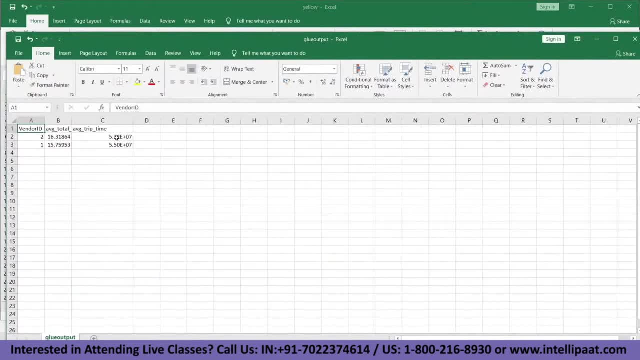 So we can see that the average trip time has been calculated and we have our average total fare as well, And it has been arranged in the descending order. So do we have the 16 first and the 15 second? So, similar to that, based on the sort of data that you'll have, you can do this in that. 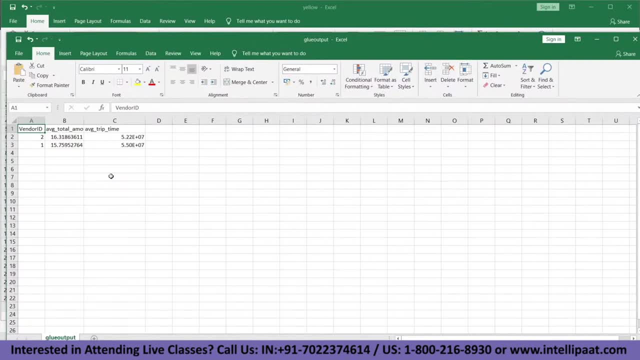 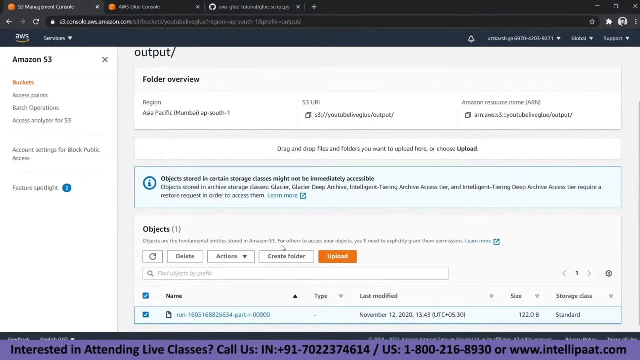 manner as well. So we can see that we had a data set initially. We transformed it. We have an aggregated data set now. Now we can perform some further analytics with it as well, using data warehousing tools. So that is about it for this particular tutorial on Amazon glue. 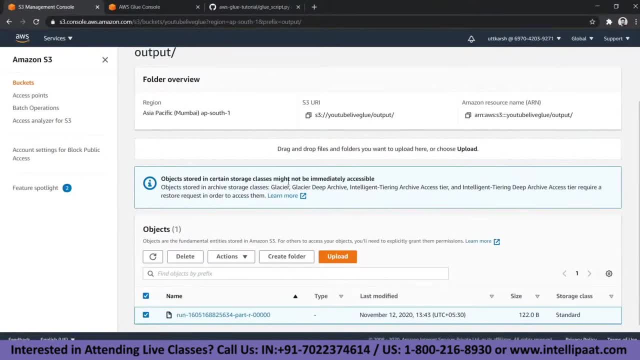 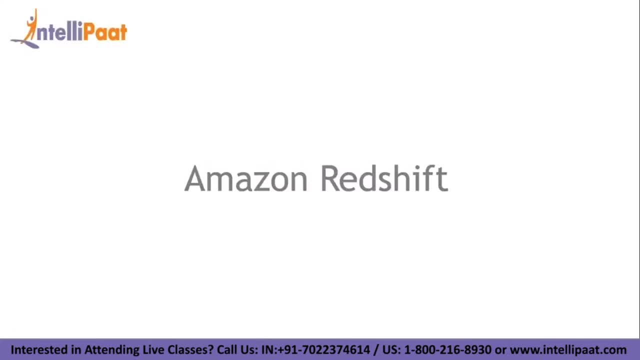 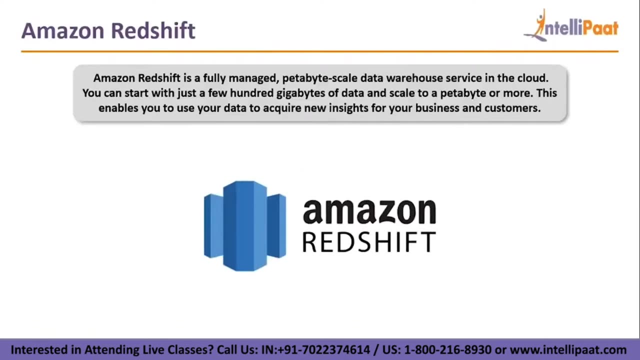 We can see how easy it makes things and how it could be beneficial in the cases of big data as well. Now let us see the data warehousing tool, which is provided by AWS. That is Amazon Right, So Amazon Redshift. So Amazon Redshift is a fully managed petabyte scale data warehouse service in the cloud. 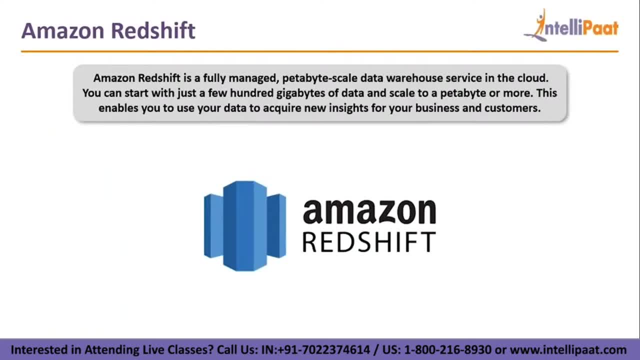 So you can scale this particular service up to petabytes. So you can start with just a few hundred gigabytes of data and scale to a petabyte or more. This enables you to use your data to acquire new insights for your business and customers. 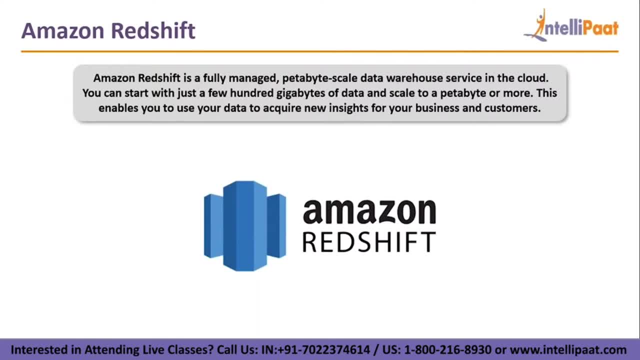 So it provides you so much of storage. You can store a lot of data, and also it has a different kind of an architecture, Which I'll show you. using that architecture, You can query results faster and, yeah, you can acquire new insights of your business. 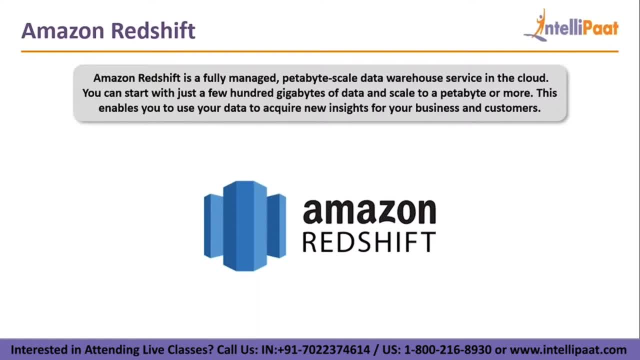 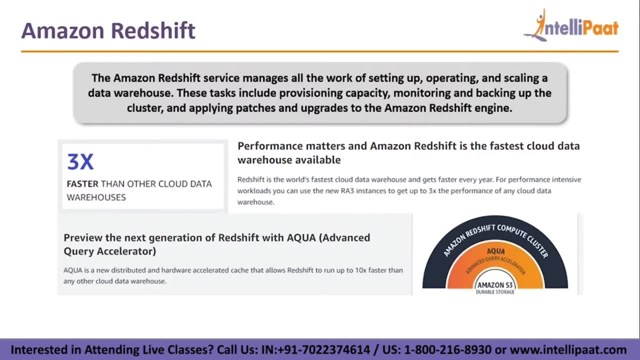 and customers as soon as possible after the data is loaded. and yeah, so now Amazon Redshift servers manages all the work of setting up, operating and scaling a data warehouse. It takes care of everything because that's what AWS does for us, and these tasks include: 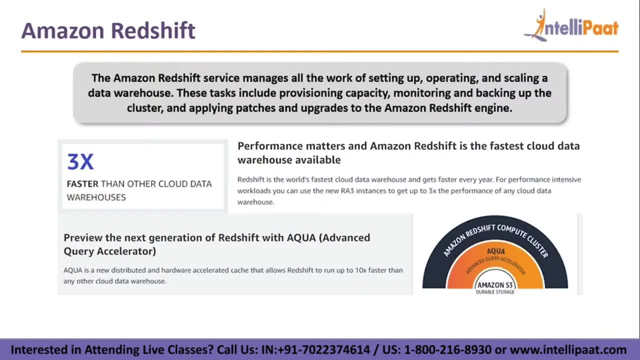 provisioning capacity, monitoring, your monitoring. you know, if we get metrics for almost every service, then backing up the cluster, we can back up using snapshots, automated backups and applying patches and upgrades to the Amazon Redshift engine. Yeah, there's also AWS, they do this for us and so, yeah, so three into faster than other. 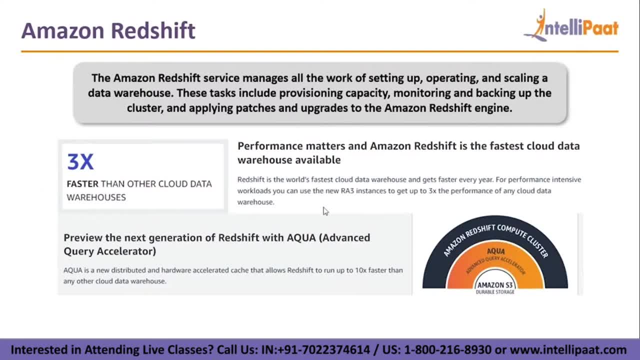 cloud data warehouses. So they give us the confidence that this is three times faster than the other data houses available. and yeah, so performance mass matters. and Amazon Redshift is the fastest cloud data warehouse available- Redshift- Redshift is the world's fastest cloud data warehouse and gets faster every year for performance. 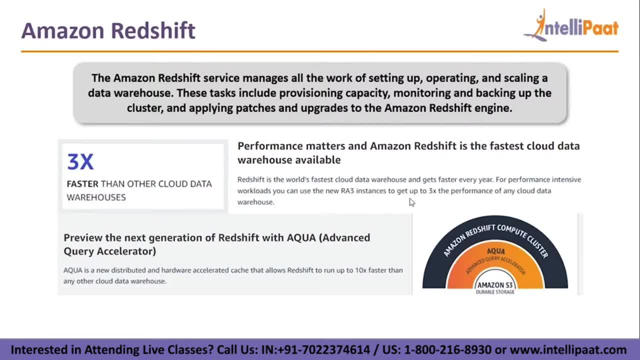 intensive workloads. You can use the new RA3 instances to get up to 3x the performance of any data cloud data warehouse. So I think this was announced in the recent reinvent event of AWS and also this aqua advanced query accelerator also was announced and this will be available in 2022, the 2020, not now. 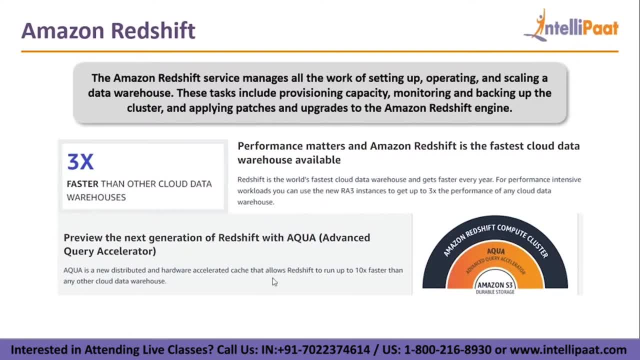 So aqua is the new distributed And hardware accelerated cache that allows Redshift to run up to 10 into faster than any other cloud data warehouse. So they have this system. They are building the system- I think it will be available in 2020, not right now- and also this aqua system when they build. 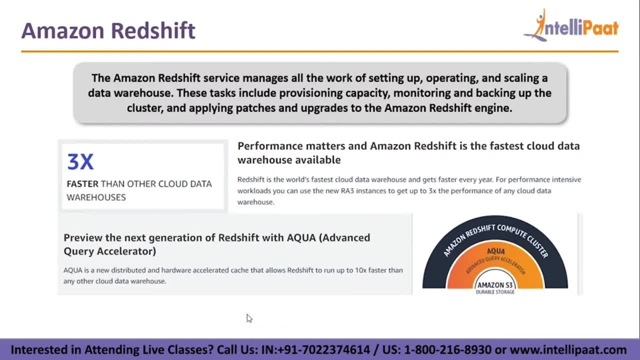 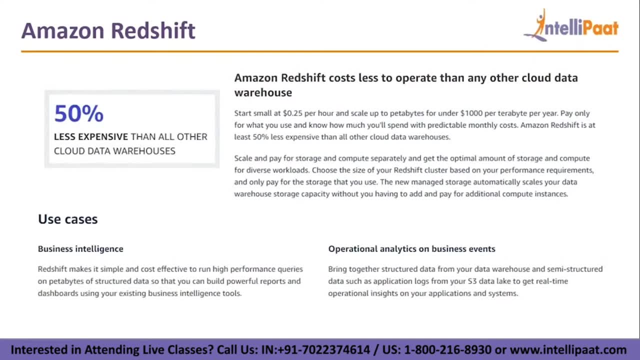 it. It will be compatible with the older Redshift versions also. Yeah, So yeah, this is the basic, basic information. and then one more is that it is 50% less expensive than all other cloud data warehouses. This is another product, Yeah. 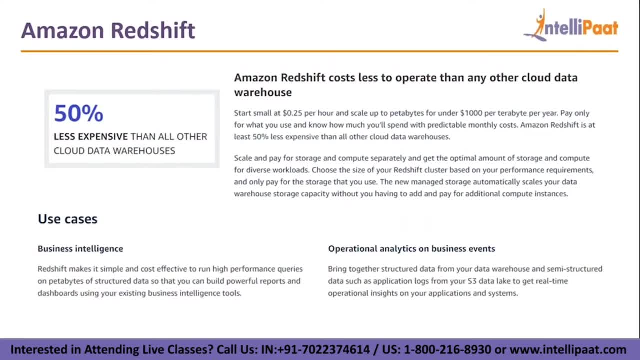 That's what they promise. They make us so. Amazon Redshift costs less to operate than any other cloud data warehouse. start small at 0.25 dollars per hour and scale up to petabytes for under thousand dollars per byte per terabyte a year. pay only for what you use. 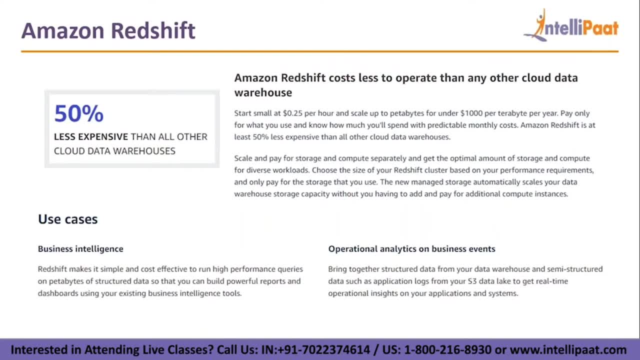 So that's exactly what every cloud service does for us: You. we only pay for what we use and know how much you'll spend, with predictable monthly costs. Amazon Redshift is at least 50% less expensive than all the other cloud data warehouse. 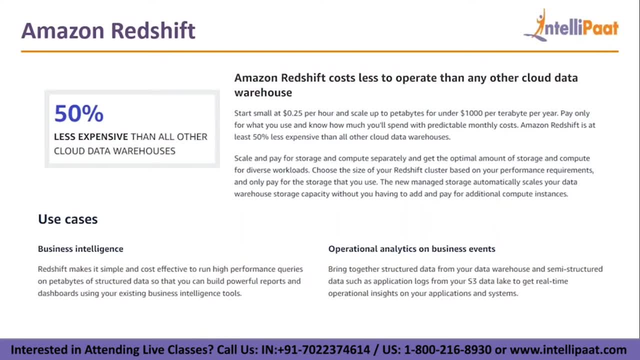 They are telling at least, so it might be even lesser expensive, scale and pay for storage, compute separately and get the optimal amount of storage and compute for diverse workloads. So basically, here you can, instead of choosing one instance which are both covers, the storage and compute, they give you options of selecting storage and compute separately. 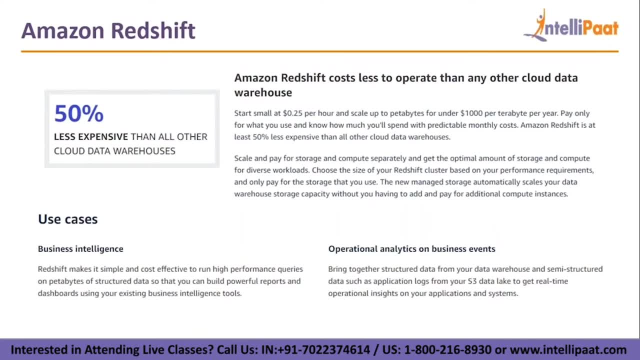 So you can provide according to your needs, choose the size of your Redshift cluster based on the performance requirements And only pay for the storage that you use. the new managed storage automatically scales your data warehouse storage capacity without you having to add and pay for additional compute. 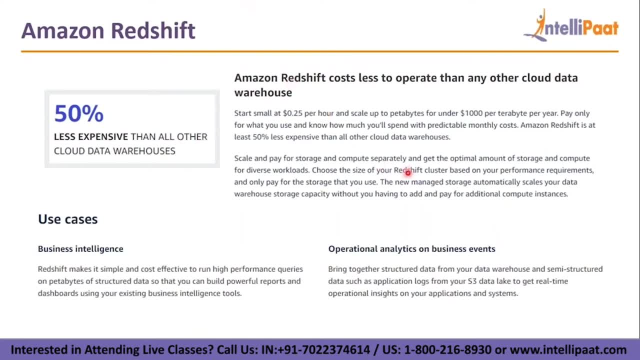 instances. So the new managed storage. So basically what they're saying is it automatically scales our data warehouse storage capacity for us. Yeah, So this is automatically done, We don't need to provision or we don't need to do anything, and yeah, so these are the. 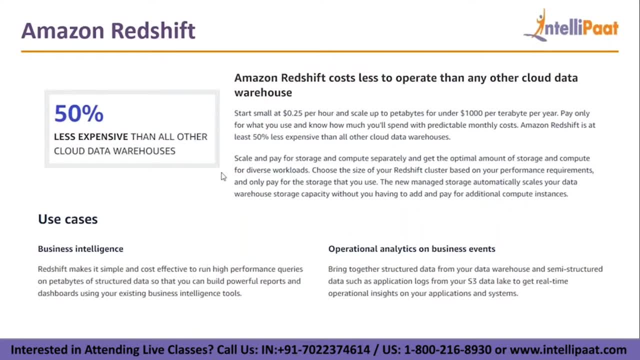 use cases. These are the two use cases provided. The first one is business Intelligence and the second one is operational analytics on business events. So first, business intelligence: Redshift makes it simple and cost-effective to run high-performance queries on petabytes of structured data so that you can build powerful reports and dashboards. 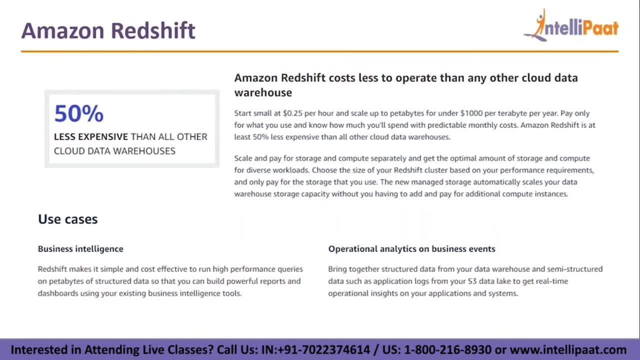 using your existing bi tools. So I, as I told you, you can run high performance queries on petabytes of structured data and you can use that data for creating reports and you can use, You can connect it with your existing bi tools and you can get insights out of it and operational. 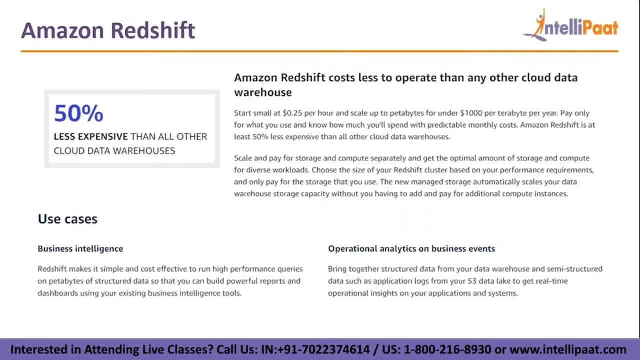 analytics on business events. bring together structured data from your data warehouse and semi-structured data, such as application logs from your S3 data Lake, to get real-time operational insights on your applications and systems. So, they are telling, we can combine both structured and semi-structured from two different services. 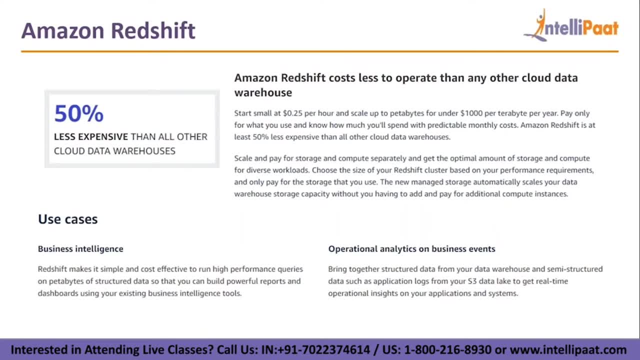 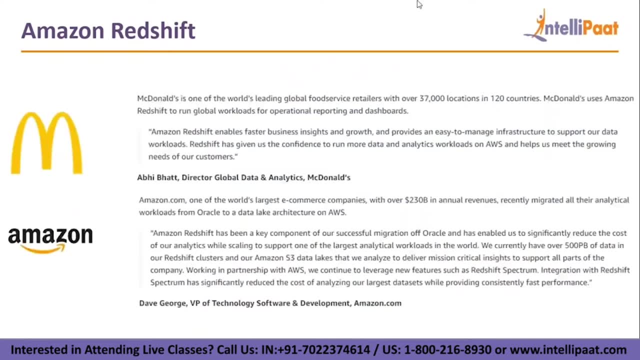 One is the data warehouse service, One is the data Lake service. Yeah, So these are the two use cases and this I wanted to show. that's it. this is nothing important. So these are a few companies. Yeah, Amazon uses Redshift, and so what they have said is: Amazon Redshift has been a key. 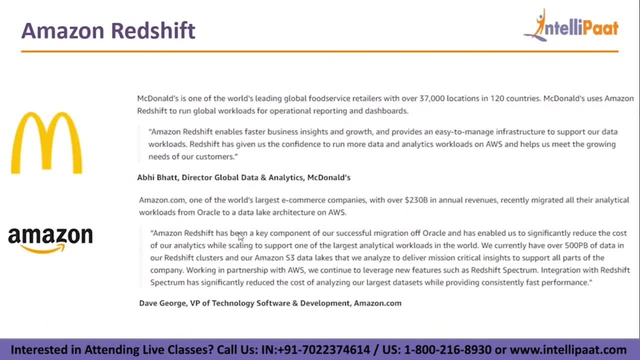 component of our successful migration of Oracle and has enabled us to significantly reduce the cost of our analytics while scaling to support one of the largest analytical workloads in the world We all know: Amazon. I think permanent $300,000 of transactions happen on Amazon. 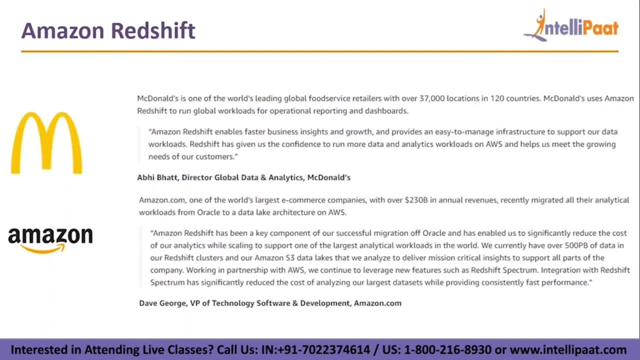 So a lot of products being bought. So, yeah, it is a very huge workload for them. So for that they're using Redshift and it's working well for them. and then coming to McDonald's, Amazon, Redshift enables faster business insights and growth and provides an easy to manage. 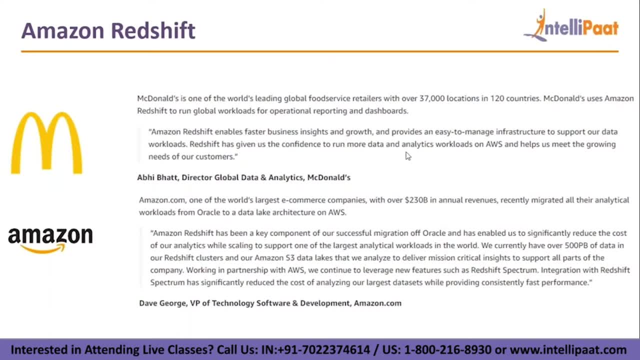 infrastructure to support our data workloads Redshift has given us- or this is just something they just talking, something about- reflective, So these are few companies which use Redshift right now. Okay, so now we've come. Yeah, so the that was just the introduction of Redshift. 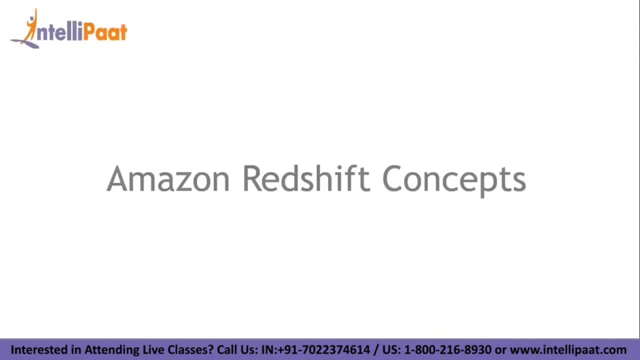 What? what is Redshift? It is a data warehousing tool provided by Amazon and the few companies using it. and those are the use cases. you can use it for analytics and you can use it for getting operational insights and you can use it as the data provider for your bi tool. 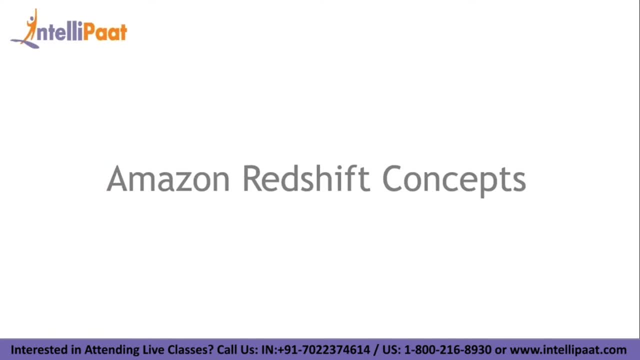 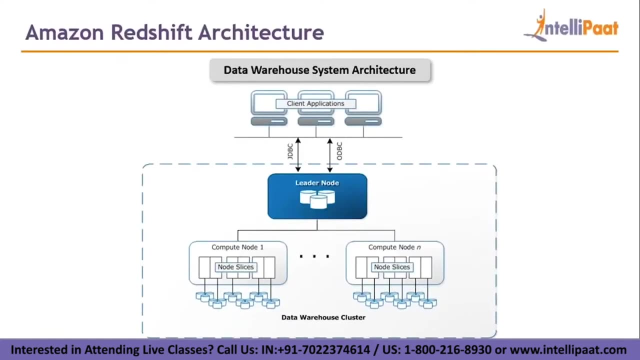 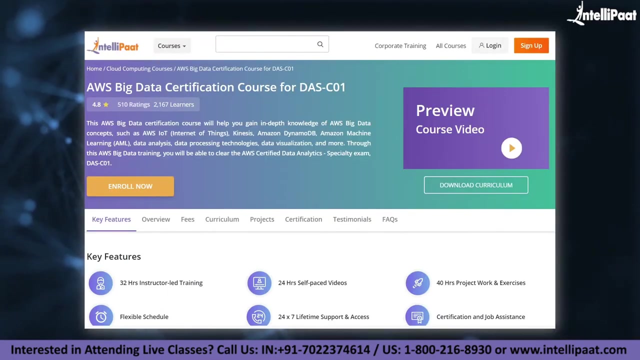 Yeah, so that's what we saw. now Let us look at the concepts of Amazon Redshift. So this is the architecture which they provide us AWS providers. So this is the architecture of Amazon Redshift. So these are the client applications. And so here this is the just a quick info, guys. 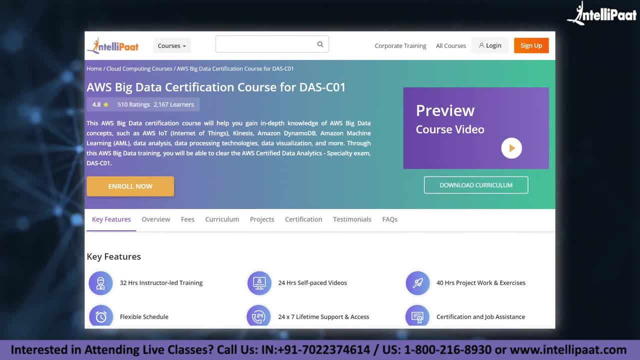 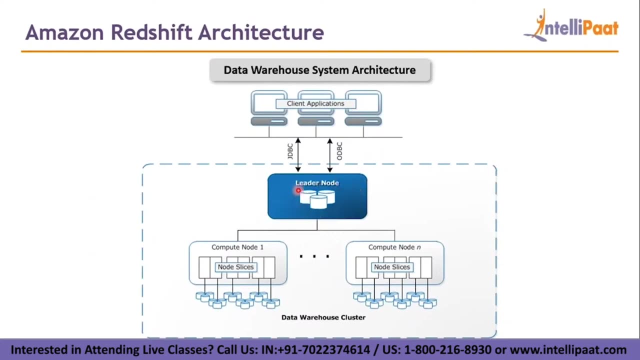 Intellipaat provides AWS big data certification course mentored by industry experts, The course link of which is given in the description below. Now let's continue with the session. data warehouse architecture of Redshift. So they have a leader node and they have multiple compute notes. 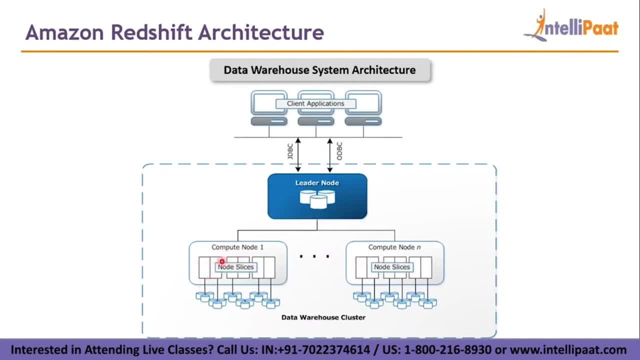 You can have multiple compute notes and all those compute notes have node slices also. So I'll explain all of these concepts right now. So this is the basic structure and they provide you two different connectivity options. One is JDBC, one is ODBC. this for open connectivity and this is for Java connectivity. 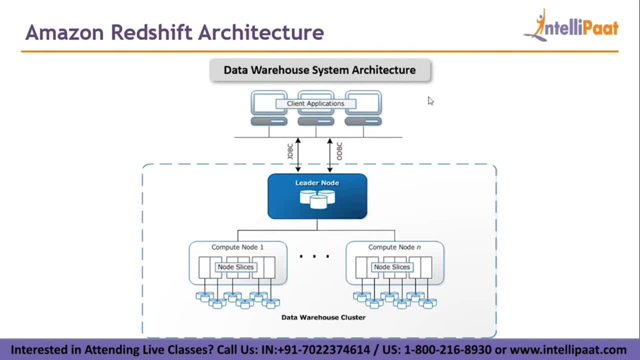 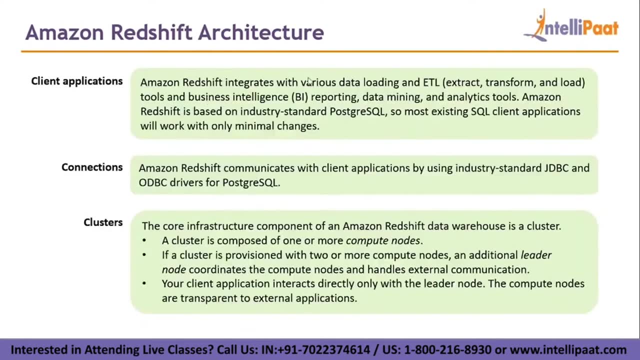 and you can use them to connect with your client applications. So this is the basic architecture of Redshift data warehouse Now, so client applications- in the sense Amazon Redshift integrates with various data loading and ETL tools and BI tools. So you can see BI tools, reporting, data mining and analytics tools. 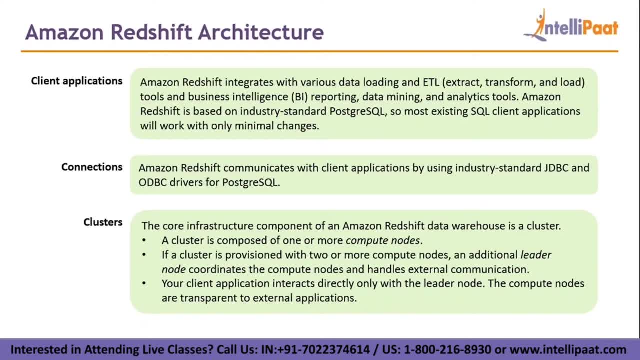 It integrates well with all of these tools and it is based on an industry standard, PostgreSQL. So basically the entire Redshift structure is built on a PostgreSQL database. So that's what they have used. So most existing SQL client applications will work with only minimal changes. 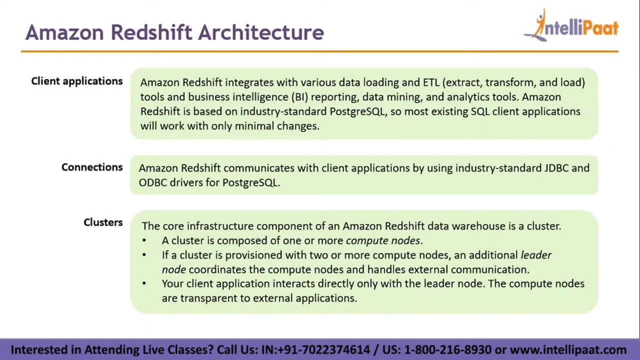 So I think you can use this with your MySQL workbench or SQL Server or other clients, So I think they work with it. and also, yeah, so as it is built with PostgreSQL, you can also use the PostgreSQL client. So, yeah, this is. these are the client applications. 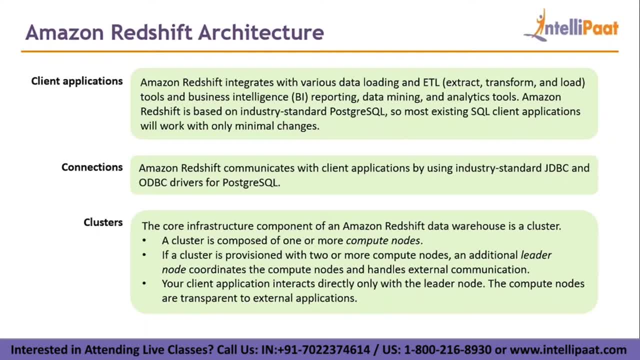 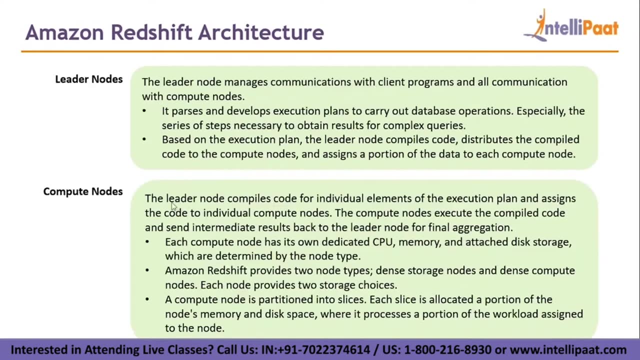 and connections. Amazon Redshift communicates with client applications by using industry standard JDBC and ODBC drivers. They provide both- you can use either of them- And clusters. so clusters, they are the core components, and so the leader node compiles code for individual elements of the execution plan. 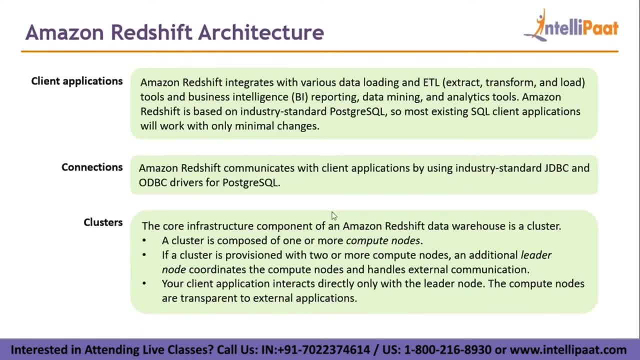 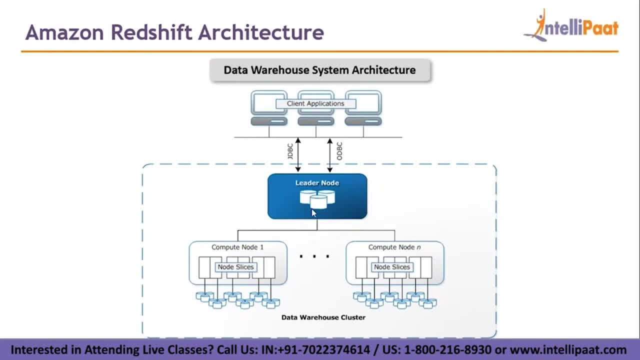 and assigns the code to individual compute nodes. So, for example, if a huge query, if a huge code comes in, so leader node takes in, takes it, it splits it up into a smaller workload, a smaller queries or smaller tasks. It provides it to the Available compute nodes respectively. 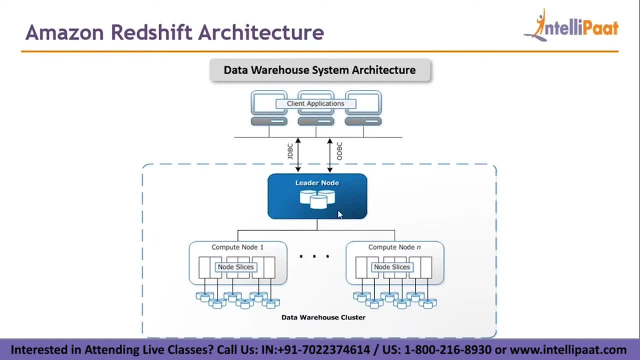 that the leader node decides how to provide it. So, basically, this concept is used so that the time it takes to query something reduces, and so you don't need to play anything for the leader node, You just pay for the number of compute nodes you create. 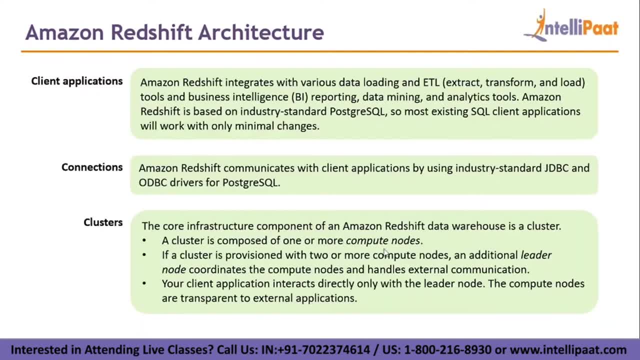 and yeah, a cluster is composed of one or more compute nodes. So basically, this is so. this part is the cluster. It can have one or more compute nodes. And then, yeah, if a cluster is provisioned with two or more compute nodes and additional leader node coordinates the compute nodes. 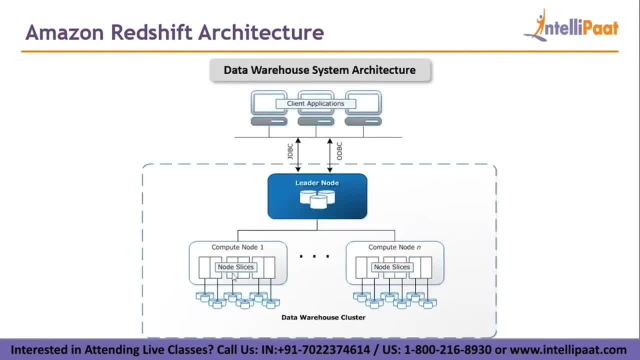 and handles external communication. For example, if you have only one compute node, if you created with just one compute node, there is no need of a leader node to distribute work among the other compute nodes, because there is only one node and all the work will be signed to that. 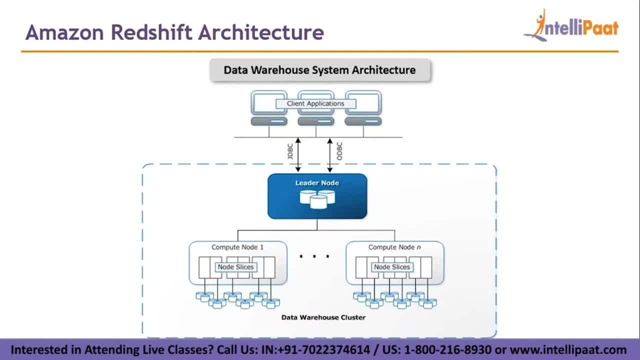 So there is no use of leader node. So what if you assign more than two or two compute nodes? then The leader node is automatically assigned and all the incoming queries, all the incoming transactions are taken care of, for leader node takes care of it. 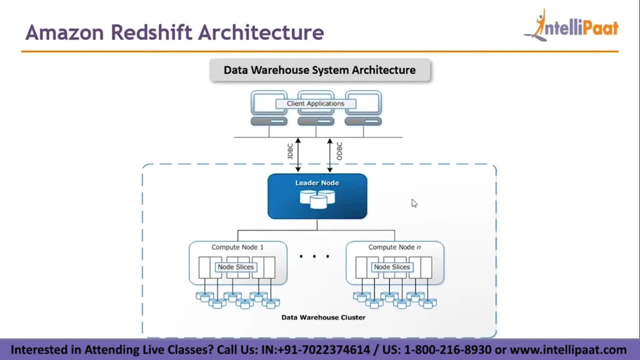 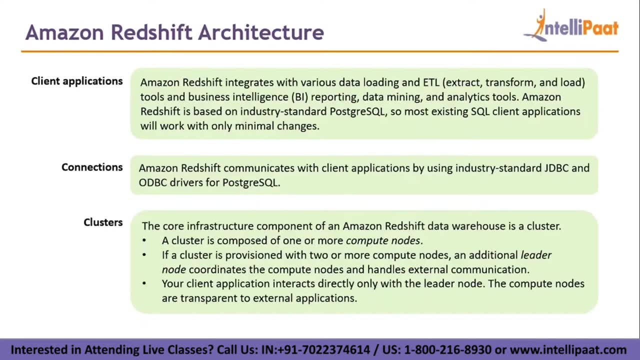 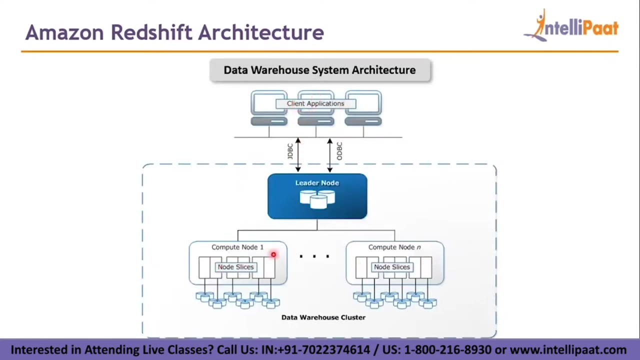 It divides into multiple smaller tasks and provided to the compute nodes accordingly, and your client application interacts directly only with the leader node. The compute nodes are transferred into the external applications, So these client applications do not contact the compute nodes available. If you have two or more nodes, two or more compute nodes, 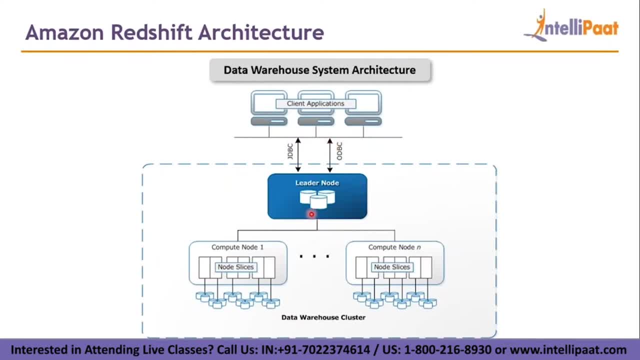 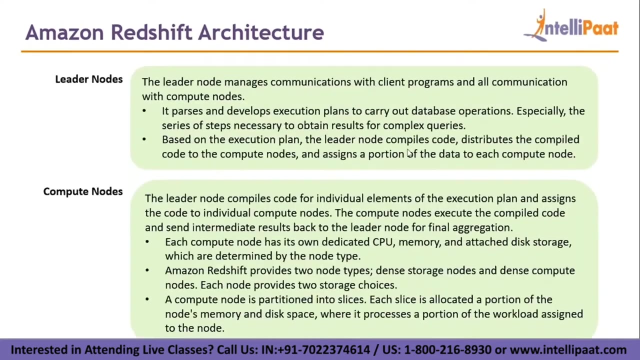 then your client applications. only point of connectivity is the leader node, not the compute nodes. So all the requests first go to the leader node, then it goes to the compute node. So that is what they are saying. and the next point: Yeah, the leader node coming to the leader node. 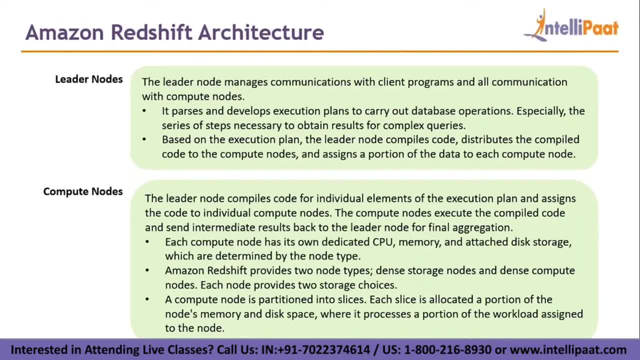 and the compute nodes. So the leader node manages communications with client programs in all communication with compute nodes. Yeah, it takes care of all the communication between the client programs and the compute nodes. So it stands in the middle, It's like a middleman and it passes. 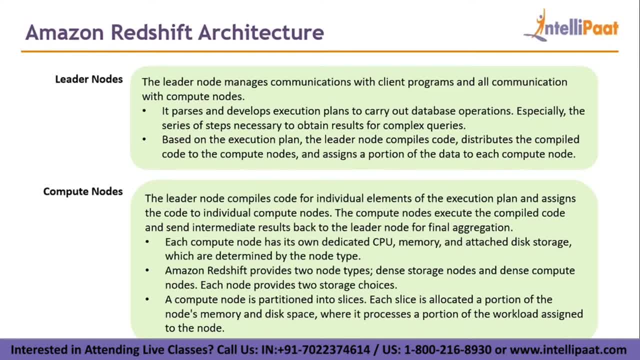 and develops execution plans to carry out database operations. So any kind of a huge database operation will be taken care of the leader node. The leader node will assign the work to the compute nodes accordingly. So yeah, especially the series of steps necessary to obtain results for complex queries. 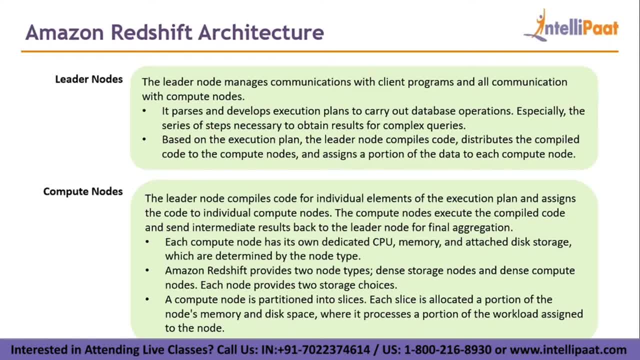 So if you enter, if you hit in a complex query, it first goes to the leader node? Yeah, it is. It's the first point of contact for any client application. So the leader node now splits it up accordingly. It splits it up in multiple parts. 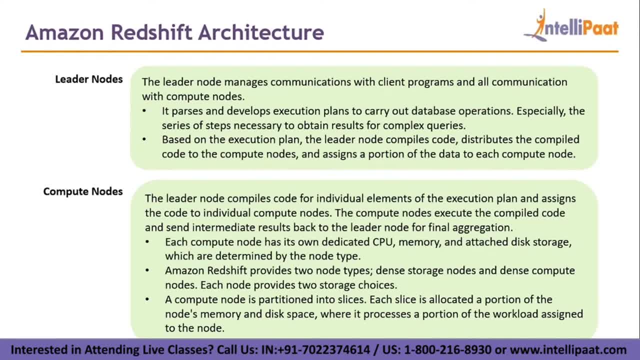 and provides it to other compute nodes which do their part and provide the results back, and the leader node aggregates them into a single result and sends it back to the client application. So this is why we need a leader node based on the execution plan. 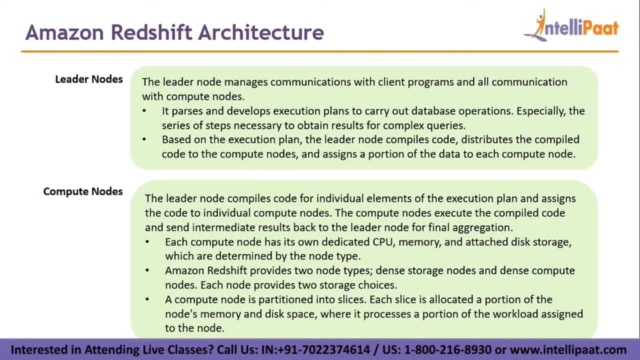 The leader node compiles code, distributes the compiled code to the compute nodes and assigns a portion of the data to each compute node. So, according to the execution plan, the leader node will compile the code, then distribute the compiled code to the compute nodes. So now coming to compute node part. 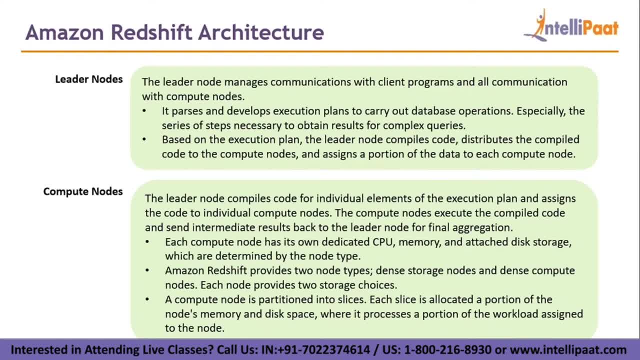 So the leader node compiles code for individual elements of the execution plan- that might be a huge execution plan which is currently executing- and assigns the code to individual compute nodes. Yeah, so the compute nodes execute the compiled code and send intermediate results back to the leader. leader node. 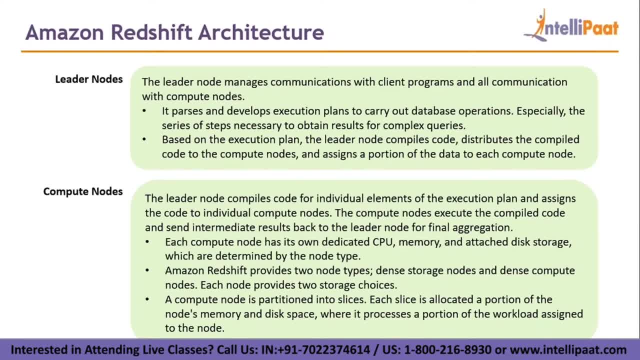 for final aggregation. So these code will be sent to the compute nodes. The compute nodes will run the queries. after running the queries, all that results will be sent back to the leader node, which will aggregate them, which will finally aggregate them and send it back to the client application. 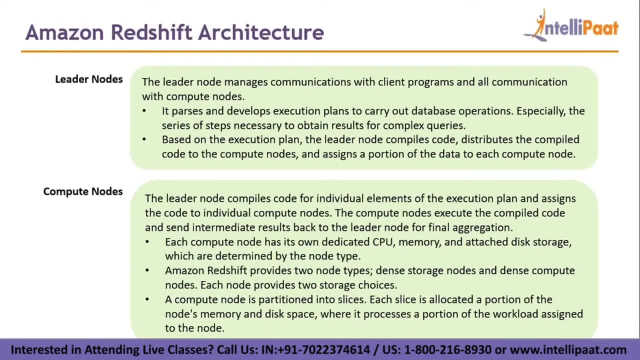 So each compute node has its own dedicated CPU, memory, attached disk storage, which are determined by the node type. So there are multiple node types also that we'll see while creating the rich of cluster. So basically every compute node will have its own CPU, its own memory. 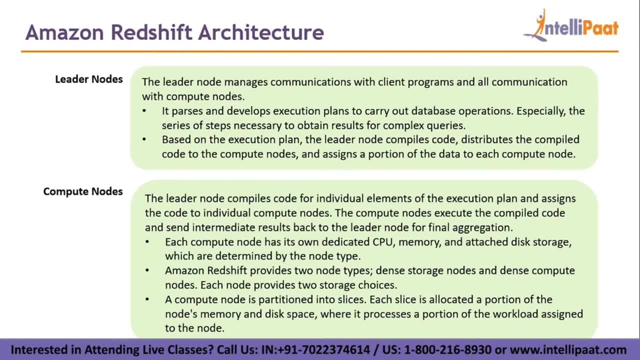 its own disk storage attached to it, and Amazon Redshift provides two node types: dense storage nodes and dense compute nodes. each node provides two storage choices. Okay, So basically these are different storage types. basically note type in the sense in the previous sentence. instance classes: 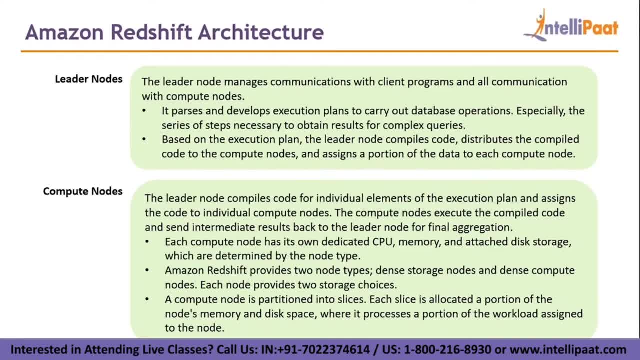 We saw instance classes right like that. There are multiple node types also, Yeah, so they have different specific specifications. that also will see. so there are two types of nodes here. one is dense storage notes and one one is dense compute node. So I think the dense compute nodes will have a lot of computing. 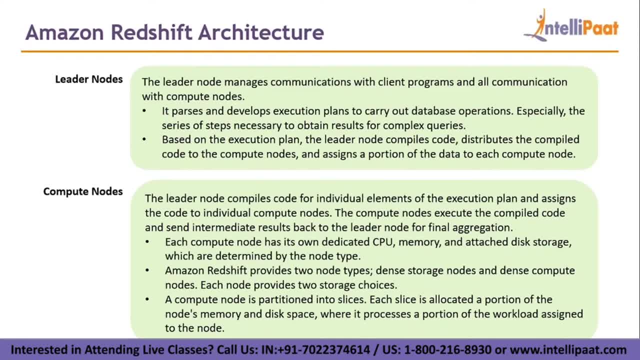 power and the dense storage nodes is used for scaling up your storage whenever you need or scaling down. Yeah, I think you cannot scale down. Yes, so scaling up your storage whenever you need it. So these are two different nodes which are entirely separate. 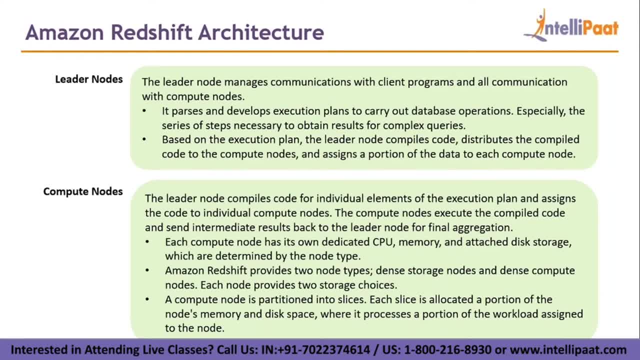 and these are assigned separately. as I told you, These are separate- the computer and the storage- and these storage can be auto scaled accordingly. AWS does it for us and same goes with compute, but you will have to change the instance type accordingly and a compute node is partitioned into slices. 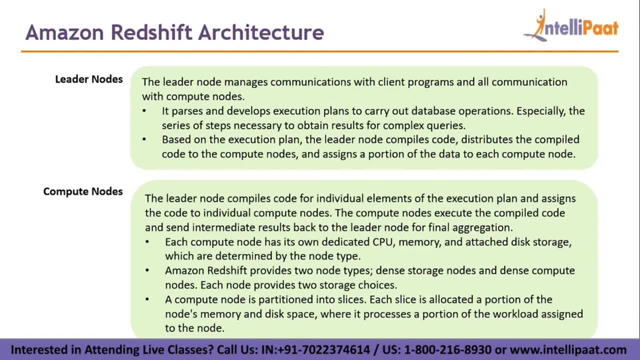 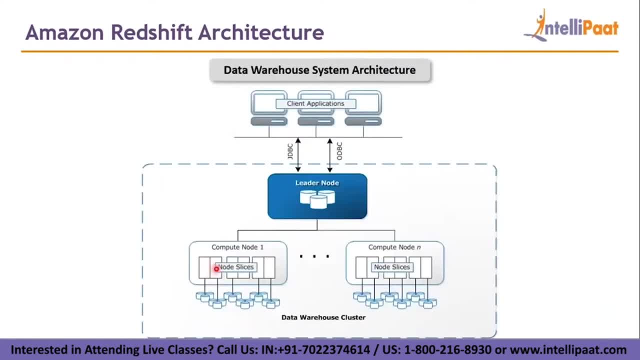 Each slice is allocated a part of the nodes memory and disk space where it processes a portion of the workload assigned to the node. So even the compute node has multiple node slices within it. So you can see this is the storage area. So all of these node slices has their own compute power have. 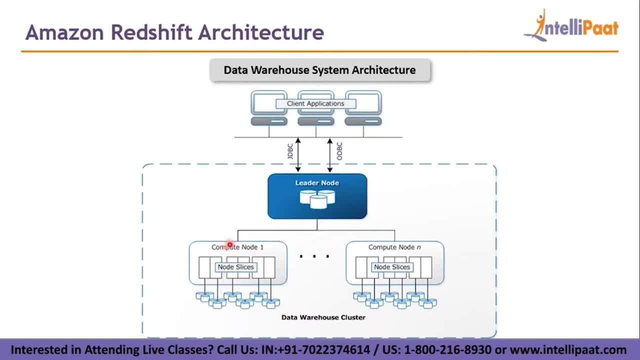 their own storage area. So now this compute node will be provided with a simpler query. Now this compute node, it will split that query into multiple parts if it requires multiple parts, if it cannot handle the workload in just one node slice. So what it does: it separates it and provides it to multiple node. 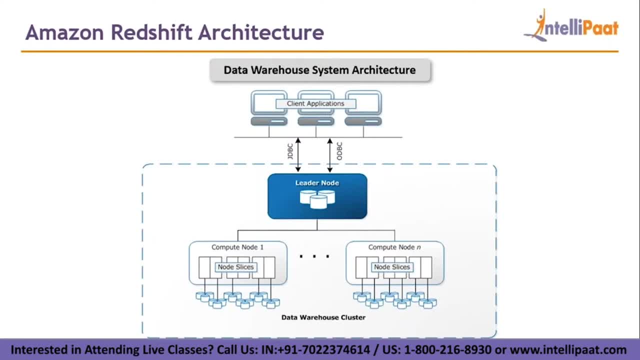 slices with. so these node slices are responsible for executing those queries or executing Those operations after they execute them. So the data obviously will be available in the storage area. It gets that back and sends it back to the leader node for final aggregation. So these are node slices. 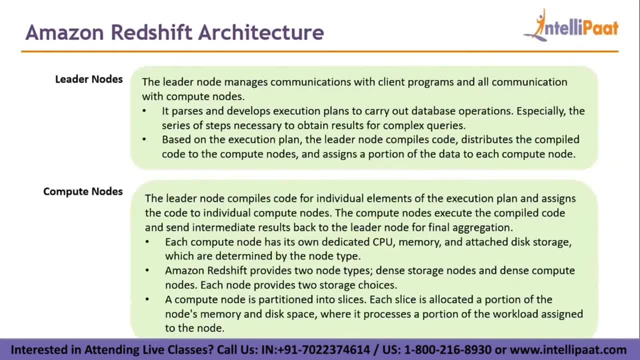 They are smaller parts of a compute node which have their own CPU. So they have their own memory and their disk space where they process a portion of the workload assigned to them. So the node slices will be assigned a portion of the workload which is assigned to the compute node and they execute them. 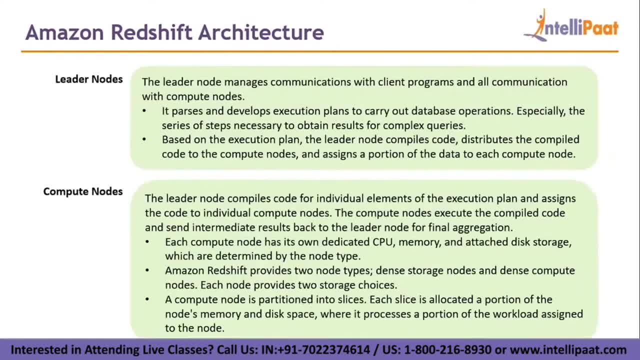 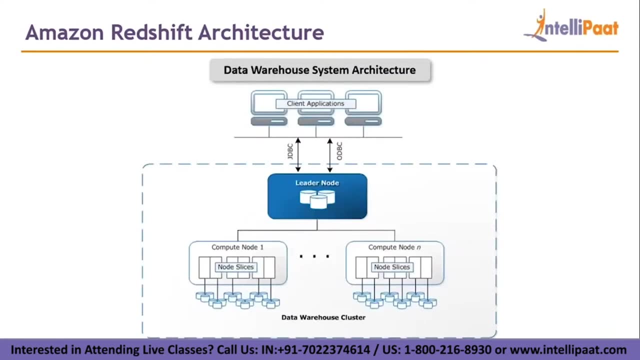 So these are compute nodes. Okay Now, these are the basic concepts of the redshift architecture. One is the connection, one is the cluster. under cluster, There are leader nodes and compute nodes. a leader node is a single point of contact for the client applications, then compute nodes. 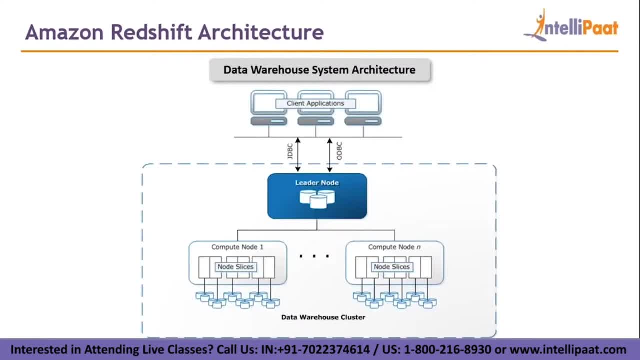 You have. you can have a number of compute nodes. We'll see how much. so if you have two or more compute nodes, then a leader node is automatically created and the leader node is responsible for splitting up huge workloads into smaller workloads and providing it to the compute nodes. 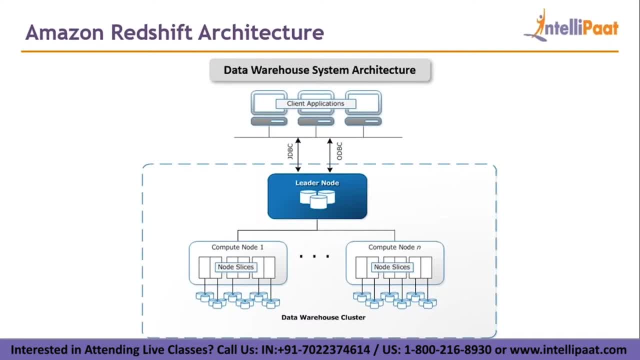 and the compute nodes have their own subversions. Those are node slices and these node slices have their own memory and storage space and the workload assigned to the compute node will be split up into smaller workloads, again given it is given to the node slices. 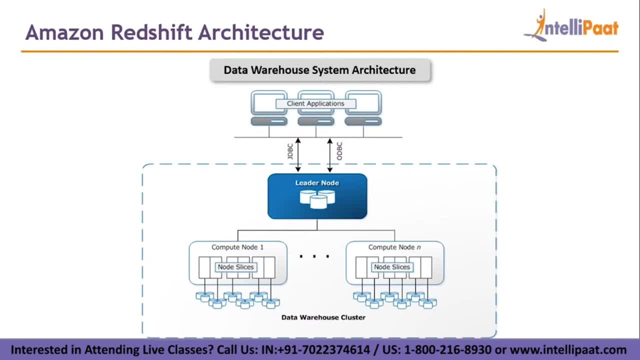 They execute their part, give it back to the compute node and the computer, don't give us it back to the leader node for final aggregation, and that finally, the collected result is sent back to the client application. So this is the architecture of redshift, now performance. 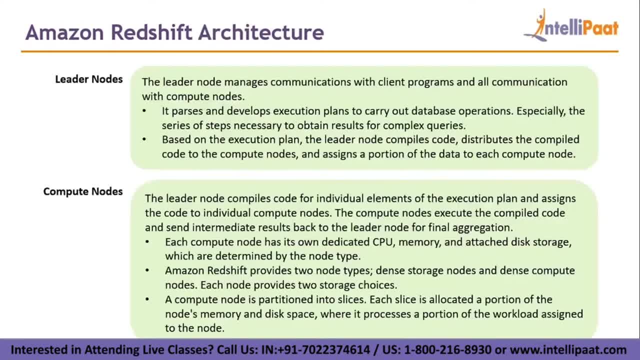 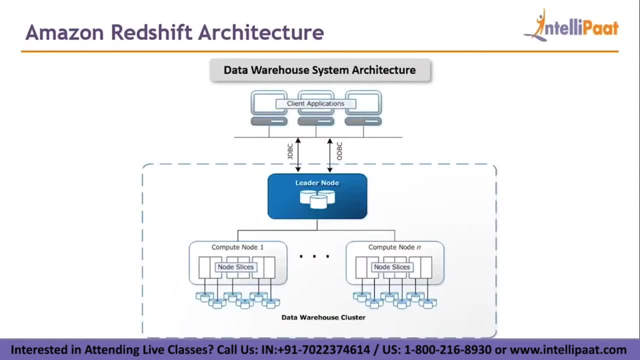 So why does? I'm sorry, I have a question. Yes, so the leader node like: is I'm that the only one like? is it just one size, single point of failure, or could you have multiple leader nodes, like unload, balance it or something like that? 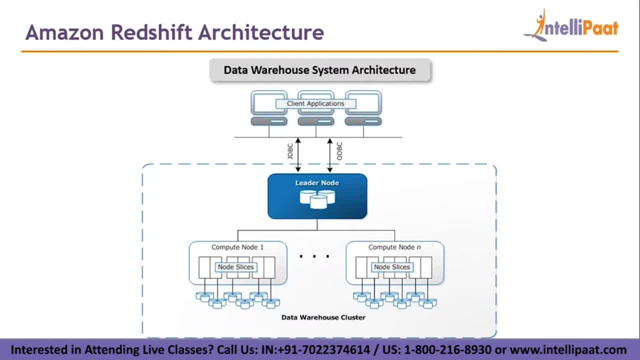 So I think the leader node is more of a logical thing. I think it's not like there is no separate compute head for that. the compute head or whatever you assign. I think they take it and create a leader node accordingly, because when you create a compute node, just one compute node. 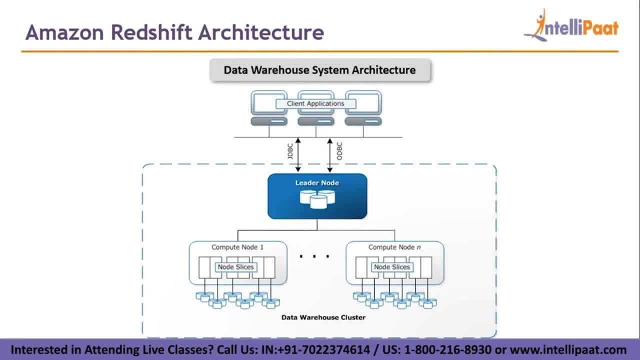 there is. there are no leader nodes, but I think actually there is workload management. So basically, what you'll do is: what is that? Yeah, so you can provide a particular compute node, a particular type of workload, but I think, coming to the single point of failure part, 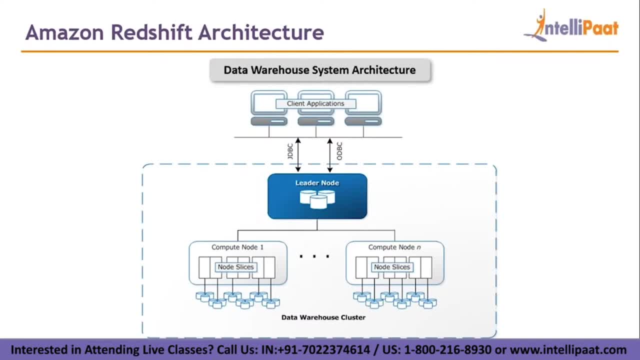 So right now, the basic Concepts in this architecture: one is the client application, which is totally away from the redshift cluster. then inside the redshift cluster, If you have multiple compute nodes, you will have a leader node. If you do not have multiple compute nodes, 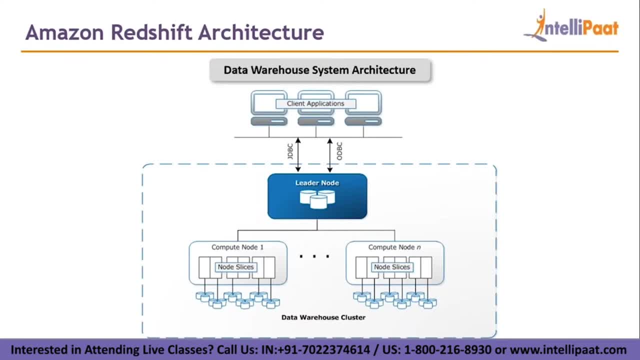 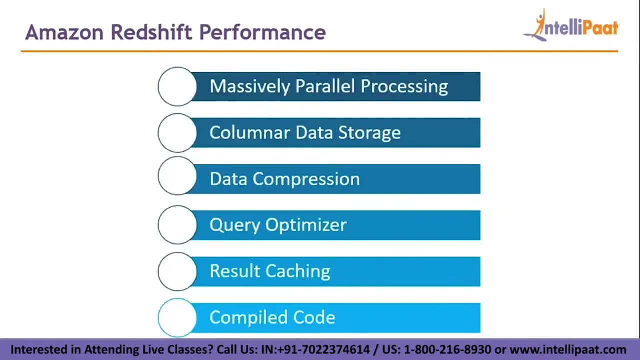 If you have a single compute node, then you will have no leader nodes, because there is only one compute node and inside compute nodes You have node slices and they have their own memory and storage. Okay, now coming to the performance of redshift. So there are six factors. 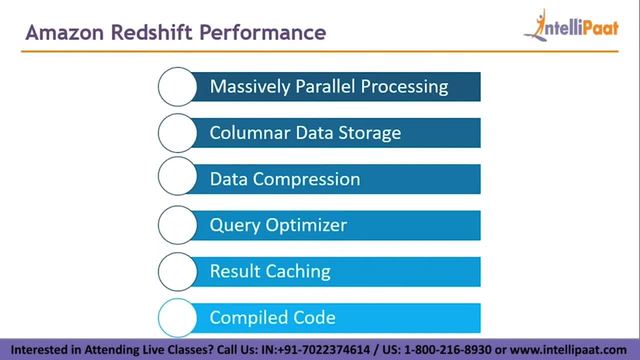 Which they climb to be available in redshift, which makes redshifts performance faster, because they told AWS promises that they. that is three times faster than any other cloud data warehouse, So redshift is the fastest data warehouse available. So you can see, these are the options. one is massively parallel processing. 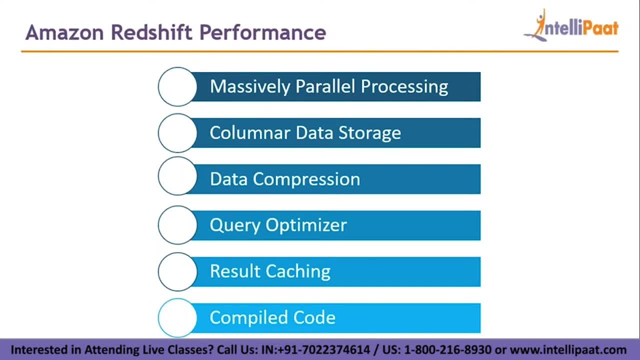 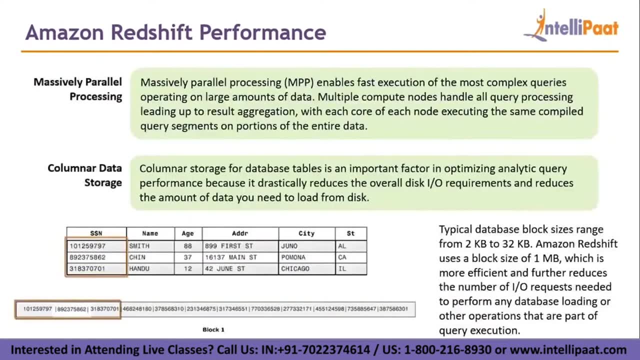 Second one is columnar data storage. Third one is data compression. fourth, query optimizer, then result caching and compiled code. Okay, So now let us discuss all of these concepts. So first, massively parallel processing. so, massively parallel processing enables fast execution of the most complex queries operating on small. 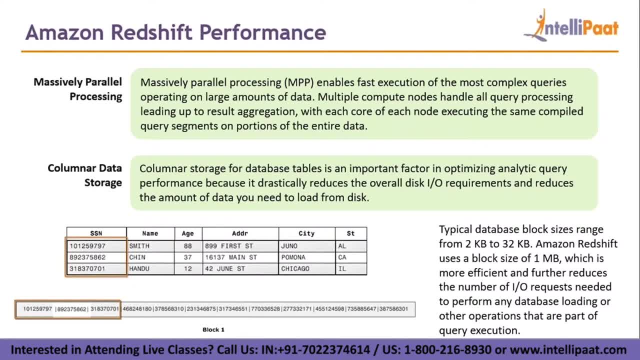 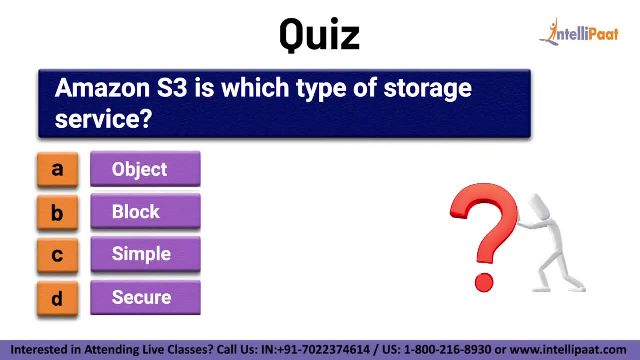 Sorry. operating on large amounts of data, multiple compute nodes handle all query processing leading up to a result aggregation which each core of each node executing the same compiled query segments on portions of the entire data. just a quick info, guys. Test your knowledge of AWS by answering this question. 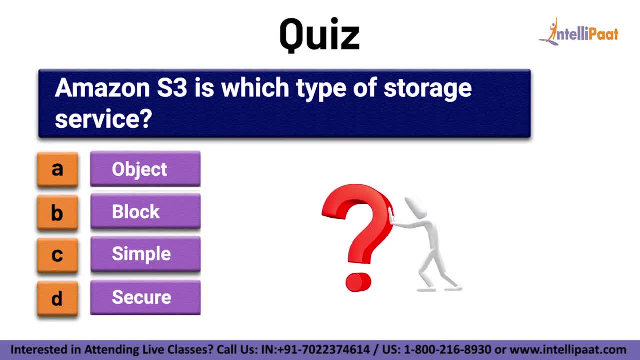 Amazon S3 is which type of storage service- A, object, B, block, C, simple, D, secure. Comment your answer in the comment section below. Subscribe to Intellipaat to know the right answer. Now let's continue with the session. 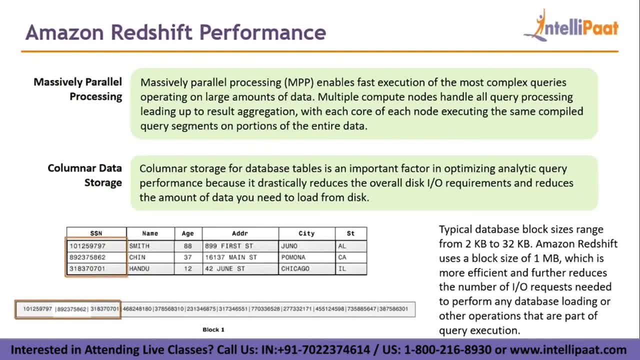 So this is what massively parallel processing is, the same thing, which was explaining about leader, what leader node does. So basically, massively parallel processing enables fast execution of complex queries. But why does it do that? Because it splits it up. it, as I told you, it, the leader node splits. 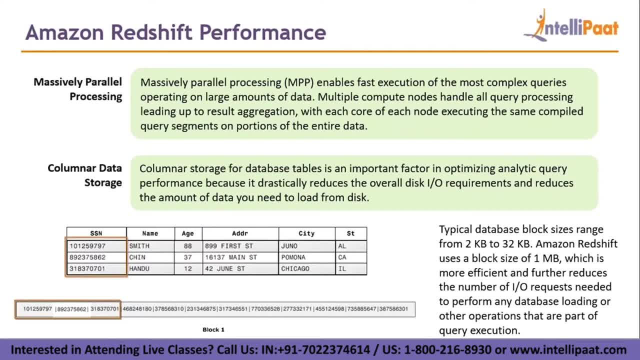 up the workload, provides it to the, provides it to multiple compute nodes and the processing is happening parallelly and all of this results are coupled up together and then provided. So that is what MPP, that is, massively parallel processing, and second one is columnar storage. 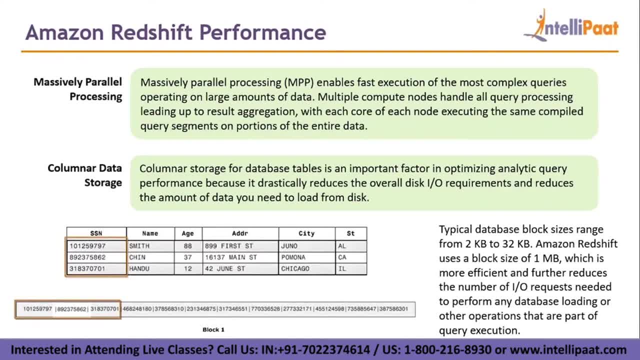 So I think there are two types. One is a row based, which happens in traditional databases. The database blocks will have 2 KB to 3- 32 KB, but in Amazon Redshift a block size can go up to 1 MB, which is more efficient and further reduces the number of input. 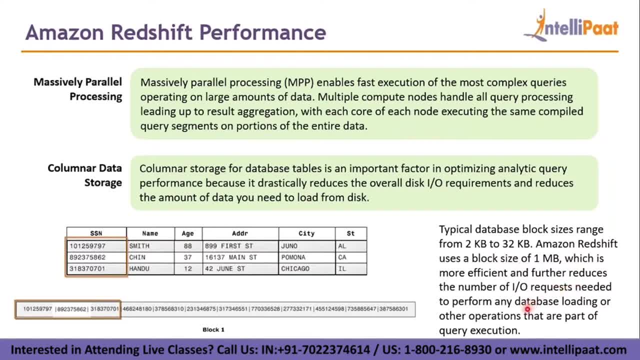 output requests needed to perform any database loading or other operations that are part of query execution. So in Redshift any data coming in will be automatically taken into a column, your storage, basically all the, for example, in a block, normally in a normal database, if in a row based database, this block 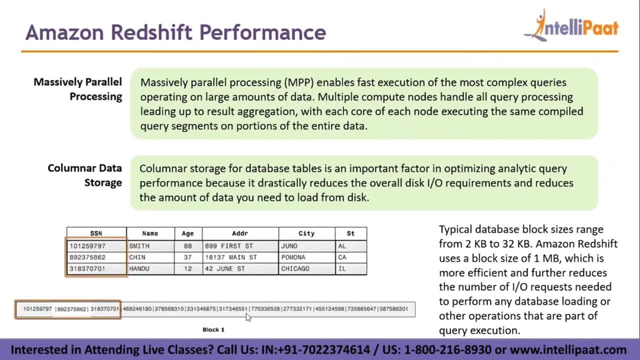 will not have only this columns data. So block one will have data of this particular row, but in Redshift, block one will have column of. it will have the data of this entire column in one block. So basically, if there are six columns, then there will just be six blocks. 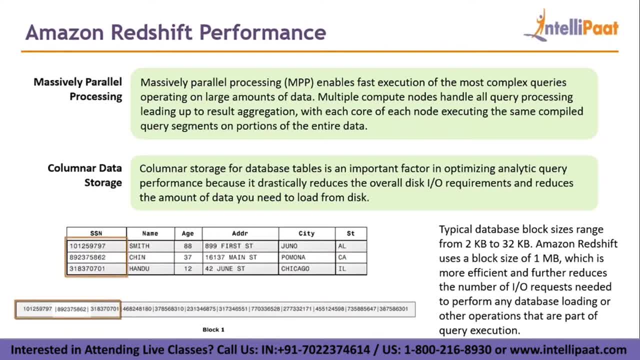 of which have all the column data in it. So I think for a analytic engine, for example for Redshift, for a data warehousing tool, columnar storage provides better performance. So we can see here, columnar storage for database tables is an important factor in optimizing analytic query performance. 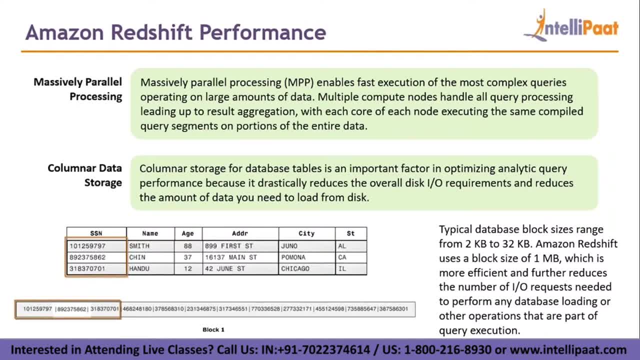 because it drastically reduces the overall IO requirements and reduces the amount of data You need to load from this. So, for example, if it is row based storage, then for each row there will be one block, So this will basically not take up a lot of storage. 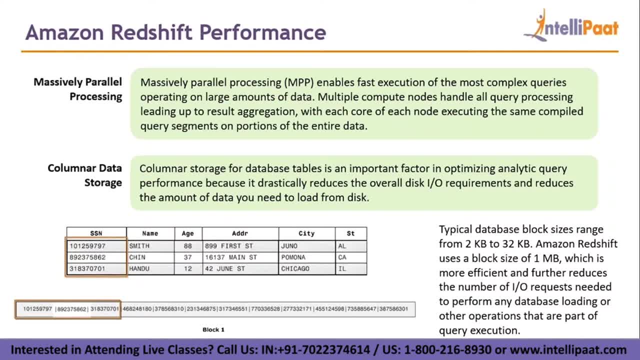 but it will take a lot of memory. So basically there will be a lot of blocks. So to take from, for example, if you just want to gather this particular column data, you will not be, so basically you will have to go through all the blocks. 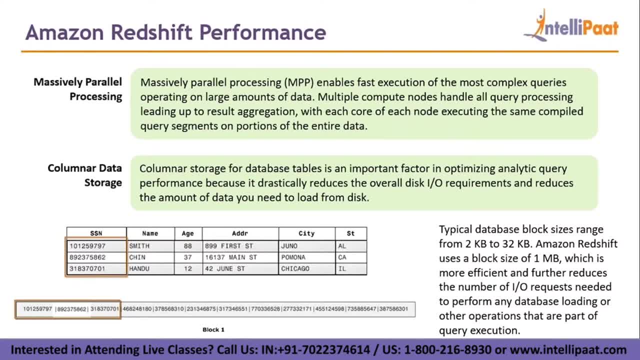 only if you go through all the blocks then you can get all the data back. but in a Data warehousing tool, basic thing is for analytics. So for analytics you need large amounts of data. You need large amounts of data to analyze something. So let's say you want to calculate the average age. 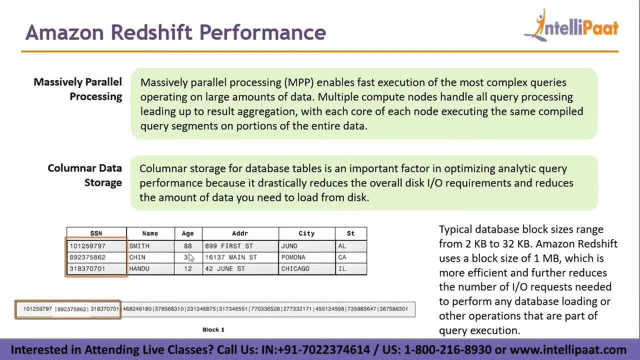 So let's say there are a hundred thousand records of age. So if you try to do that, if you try to analyze that, then if it is a row based storage, it will go into every block and gather that particular data and then it will do the process. 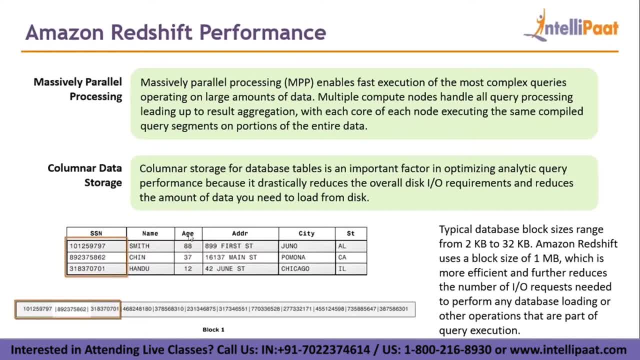 But if it is a, if it is a columnar storage, then it just takes this block, So there will be one single block and it just uses that. So I think this reduces the input out requirements and also it fastest, so it increases their performance. 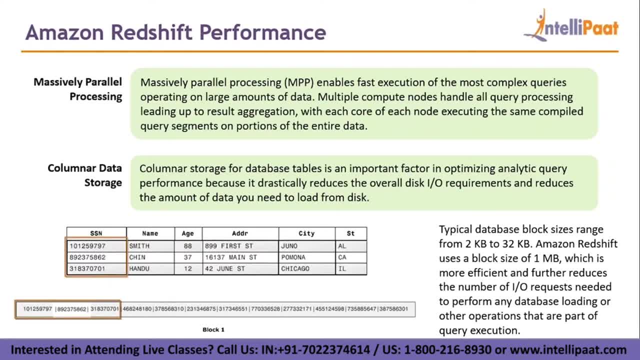 So, as told by Redshift to, Redshift uses columnar storage and because of that they're telling it is three times faster than using a row based database for analytics operations. It is three times faster. So if it is three times faster than a row based database, 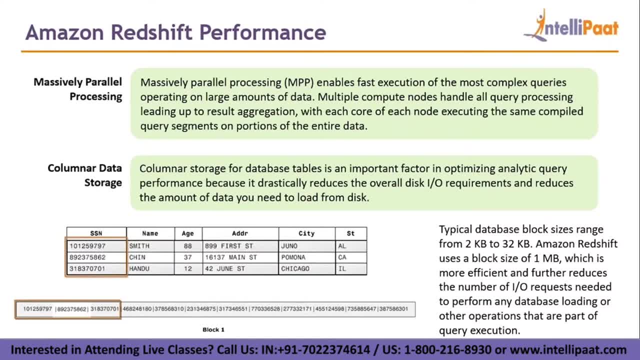 basically, it requires three times less, for example, one by third of the memory and the compute cap capability of a row based storage used for analytics. So this is where columnar data storage comes in. So this is the basic example they provide, and then data compression. data compression reduces storage. 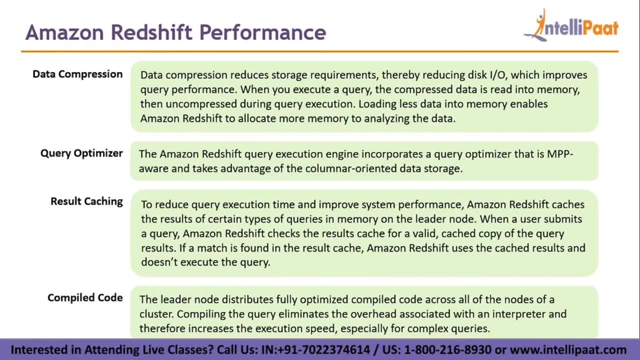 requirements, thereby reducing disk input output, which improves query performance. So data compression are yeah. So if you compress the data, it'll reduce storage requirements. So when you execute a query, the compressed data is read into memory, then uncompressed during query execution. So loading less data into memory enables Amazon Redshift. 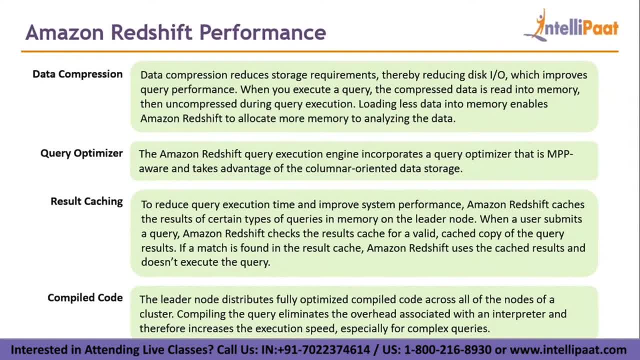 to allocate more memory to analyzing the data, So basically for loading data. So if it is compressed, so when that data is loaded into memory it is not taking up a lot of memory area. So now Redshift can allocate the remaining memory for analyzing that data. 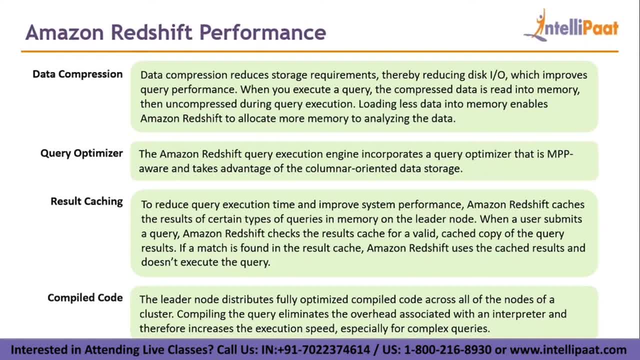 So once this compressed data is put inside the memory, then before query execution it is uncompressed, and then that data is used to analyze. So basically this takes lesser memory. So that's why they use data compression. So these are default concepts which they automatically use in Redshift. 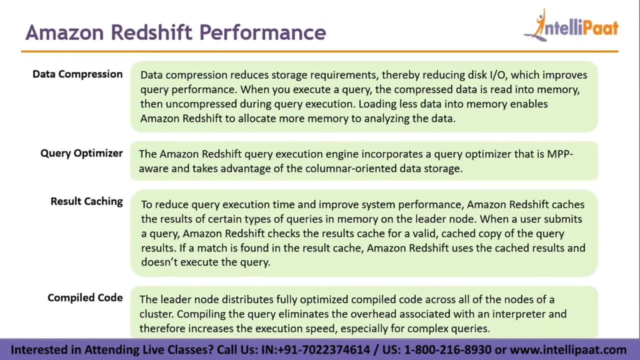 We don't need to enable these, So these are what they automatically use in Redshift. and then query optimizer: the Amazon Redshift query execution Engine incorporates a query optimizer that is massively parallel processing aware and takes advantage of the columnar oriented data storage. 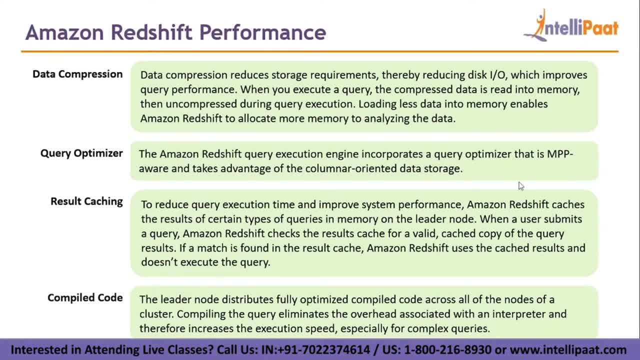 So, as he told you, Redshift has both massively parallel processing and the columnar data storage. So there is a query execution engine specially designed to take advantage of this columnar data storage and MPP. So there is a separate query optimizer inside Redshift. 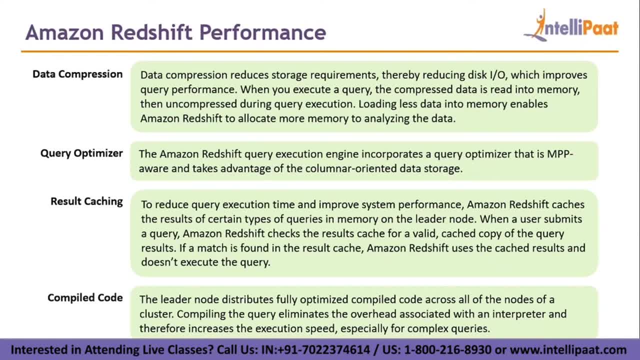 which is running for us, And this is what this is what it does. And then result caching, so to reduce query execution time and improve system performance, Amazon Redshift caches the results of certain types of queries in memory on the leader node. So, for example, for, let's say, multiple people are trying. 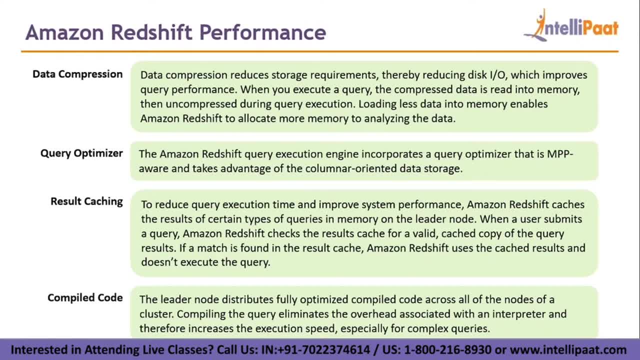 to analyze some particular query data. So they are querying the same thing from the same Redshift cluster again and again. So this query data- or it should- automatically stores it in the cache in the leader node. So once it stores that, then every time it can be taken. 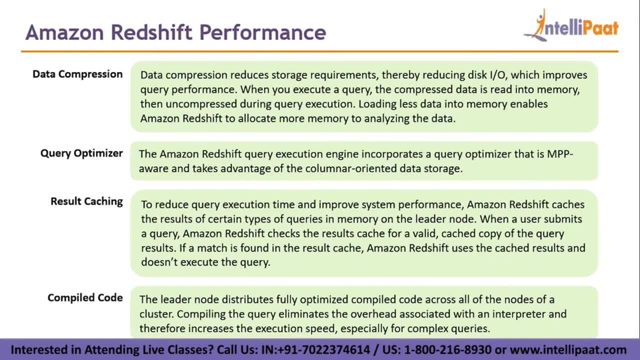 But it can be retrieved faster than going back to the compute nodes, then querying it back, getting it back, then providing the final result. So it also does result caching. So when a user submits a query, Amazon Redshift checks the result cache for the valid or cached copy. 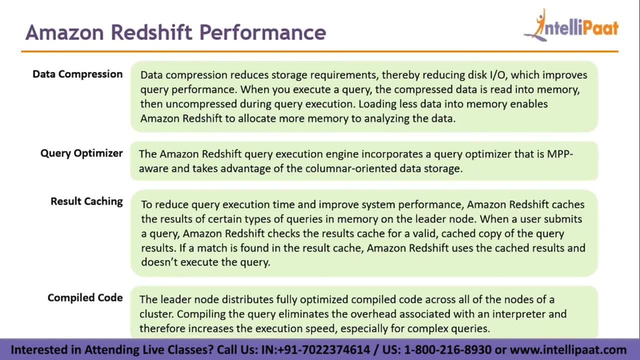 of the query result. if a match is found in the result cache, Amazon Redshift uses the cached results and does not execute the query. So when you run that query once again, basically it will not run the query execution. It does not happen. So this will improve the performance. 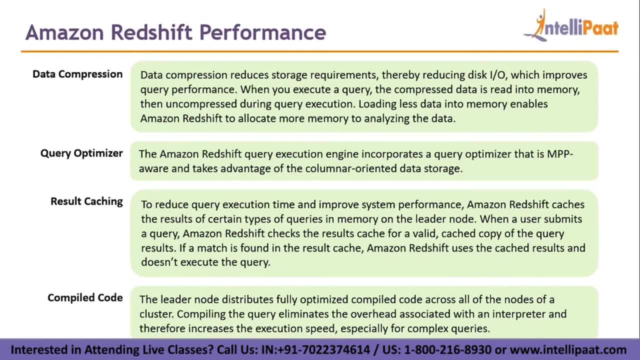 So it just takes the result from the cache and give it, gives it back, So the query is not performed. It is now the workloads are not assigned to the compute nodes and then compiled code. So the leader node distributes fully optimized compiled code across all of the nodes of the cluster. compiling the query eliminates 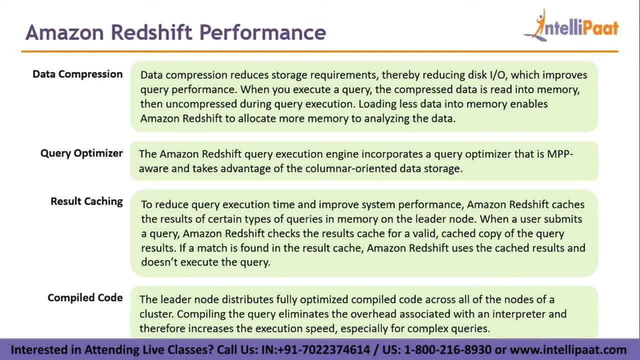 the overhead associated with an interpreter and therefore increases the execution speed, especially for complex queries. Okay, So basically the leader node: whenever there is a query coming in, it automatically compiles it first and it gives that compiled code. So I cannot make sense out of it. 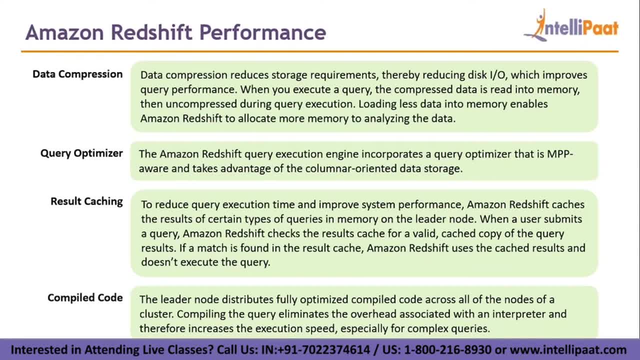 but this is what it does. So it, if you provide a particular set of a query set, So in that there are multiple queries running continuously, So it executes. that executes in the sense it compiles it in. it interprets whether there is there are any errors. 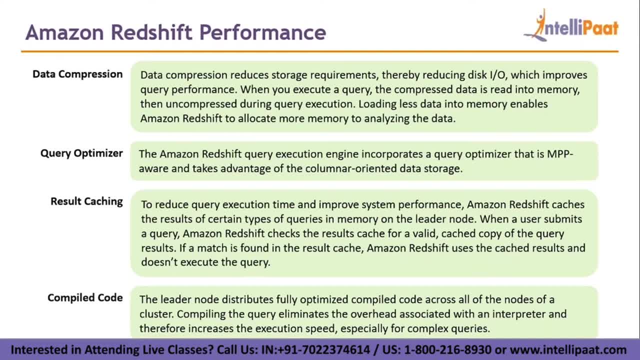 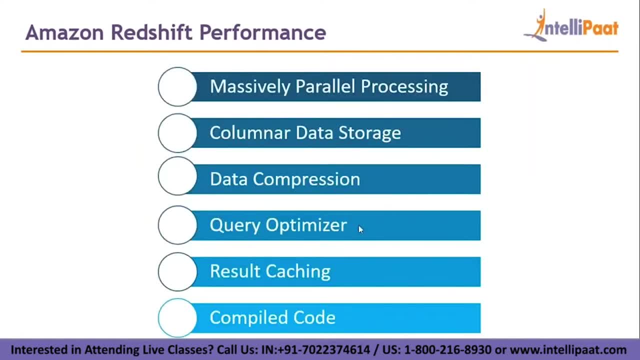 or whatever, and then it provides it, divides it into multiple workloads And provides it to the compute nodes. So these are the six major Concepts for improving Redshift performance, and these are already implemented in Redshift. There is no need to trigger them. 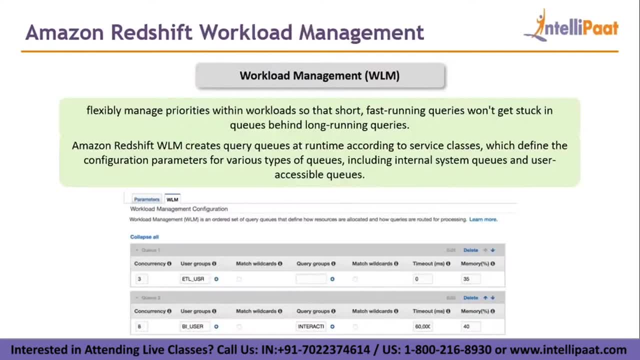 There is no need to do anything. Yeah, and so workload management or WLM, So flexibly manage priorities within workloads, so that short, fast-running queries won't get stuck in queues behind long-running queries. So you can set up, for example, 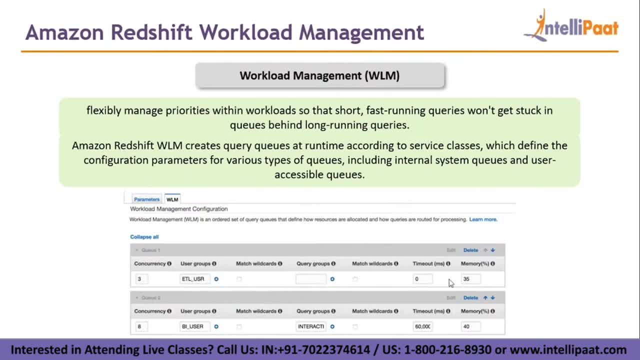 you can see over here concurrency Three user group and so this part will see so: 35% memory. So if this particular query is using 35% of memory, then it will be taken up by this queue If it is taking up 40% of memory. 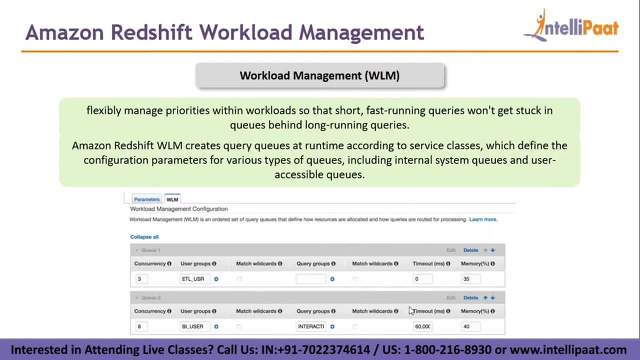 it will take up this queue. I don't know much information about this, So right now I just know this: you can create manual queues also, so you can provide 5% memory, then anything below 5%, and, yeah, anything below 5%, up to 5% will be taken. 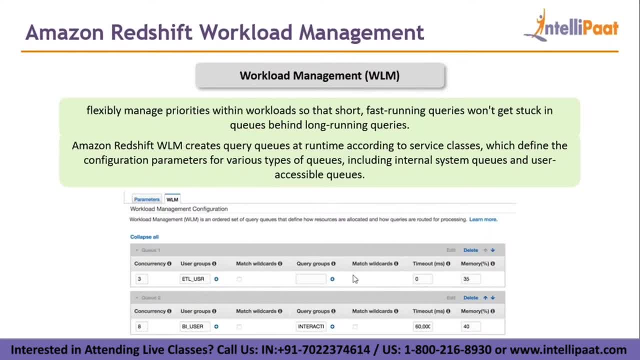 in that particular queue and anything below 35% will be in this queue. Like, for example, smaller queries do not need a lot of memory. They have. they occur faster. So for those fast-running queries you do not need to assign a lot of memory. 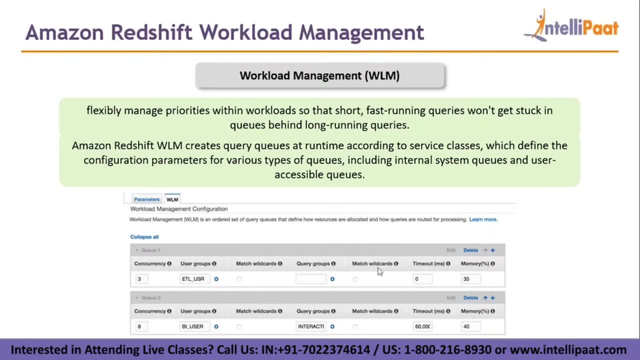 You can just create a manual queue which will automatically execute for us. So if you provide 5%, all the queries under 5% memory usage will be taken care of this queue, And so same thing. you can create multiple queues and Amazon Redshift WLM creates query queues at runtime. 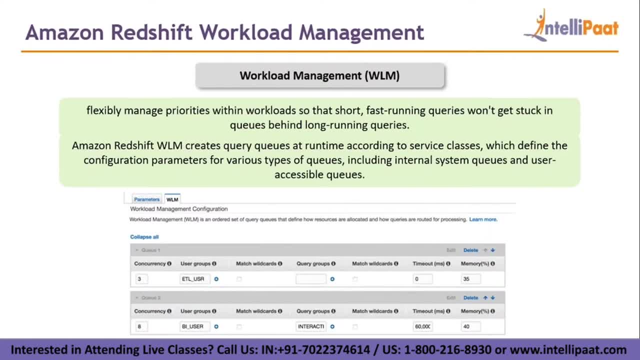 according to service classes. So which defines the configuration parameters for various types of queues, including internal system queues and user accessible queues. So you can create multiple. I think you can create 50, do not know the exact number. You can create that, and also there is a queue system implemented. 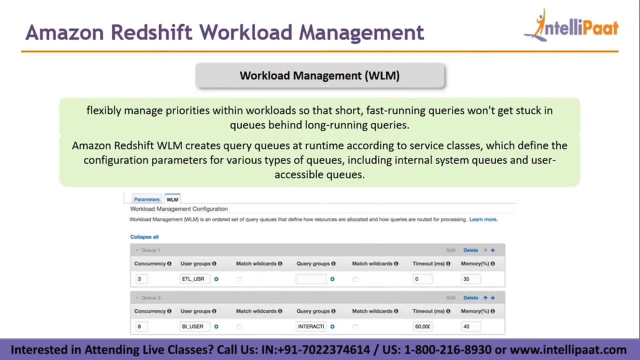 inside the redshift cluster. It is an automatic. you, I think again you'll have to set it up. So there are two types. one is automatic queuing system. One is this manual queuing system and launching a redshift cluster. So I launched one, so this will how it will look. 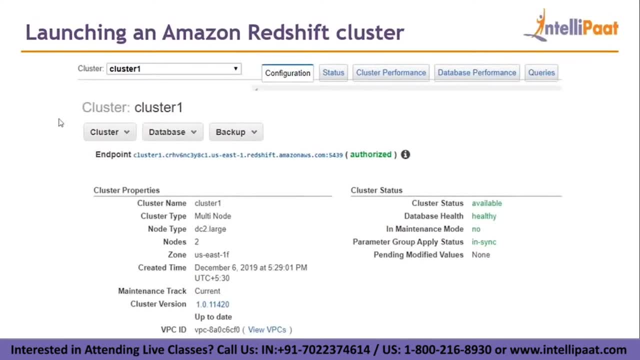 and also there are some bugs on the console. I don't know whether in this system, I'll just check that. so now. so this was my cluster name, cluster one. Then this was the end point which they provided. you can use this end point to connect with your SQL client. 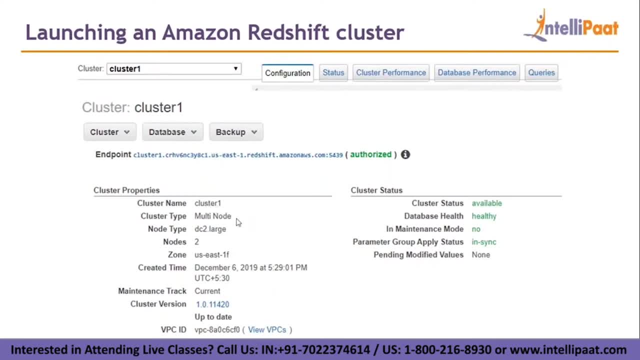 Yeah, so you can do that, then cluster one multi-node. So to see, I was multi-node because I chose two nodes and I chose the node type as DC 2 dot large and I didn't provide any preference. It took us East 1 F and create a time. 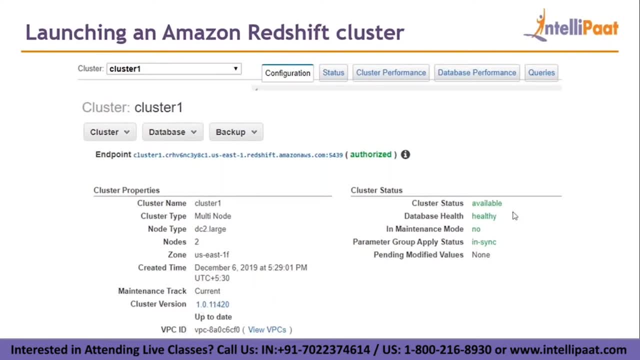 Yeah, maintenance track, PPC cluster status. It was available, It was healthy, It was not in maintenance mode. Yeah, something like this. So you get also other options. I'll also show that we look into all the concepts in the dashboard. We'll understand that completely. 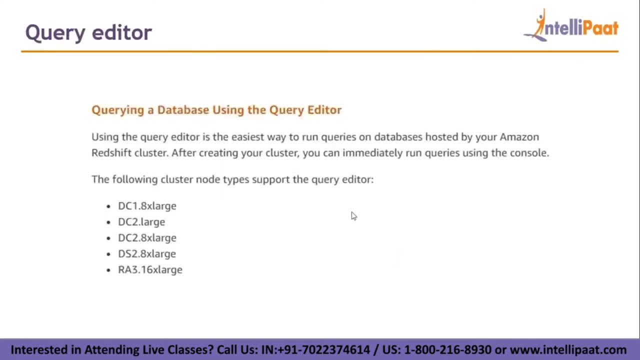 and then querying a database using the query editor, Because I'll not be using a SQL client, I'll be using the query editor provided by redshift and also I have some sample data to load. I also have some sample queries to execute, So I'll be doing that and then query editor considerations. 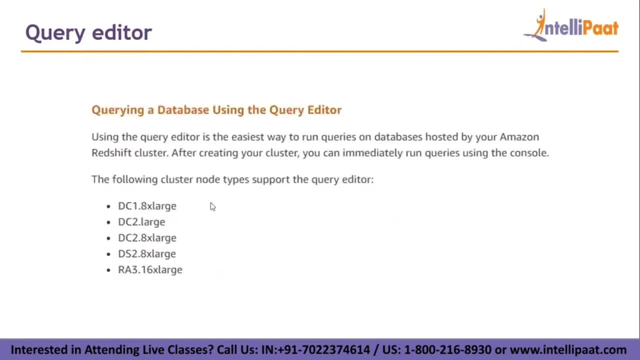 This once we complete the demo, then we'll come back here and look. look at that. and also, the query editor allows only these, that is, DC 0.8 into large These. this is the previous generation DC 2 dot large. DC 2.8 X large. 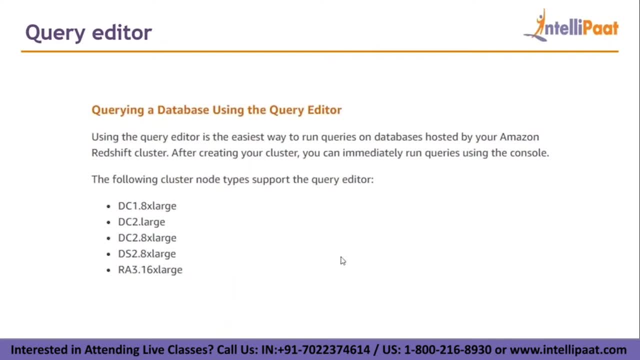 DS 2 dot 8 X large is allowed, not DS 2 dot large, and then are a 3.6 X large is load. So basically there are two node types, which is not allowed for using the query editor, So we'll be using DC 2 dot large. 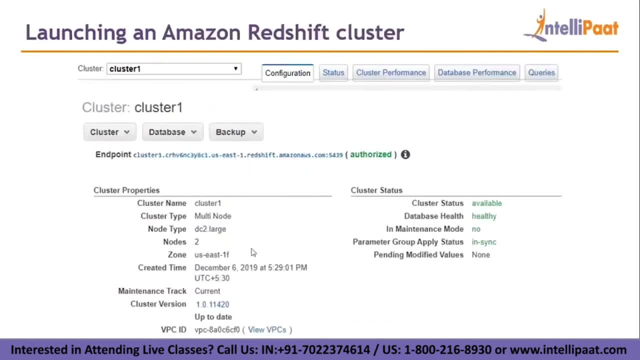 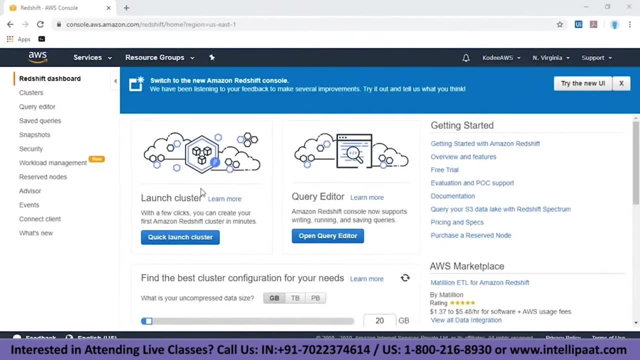 So no worries, We'll be able to access the query editor. Yeah, So now let's go over to the console. So this is the dashboard, and so there is this bug guy. So basically also never if you're in middle of some process, if you are creating the cluster. 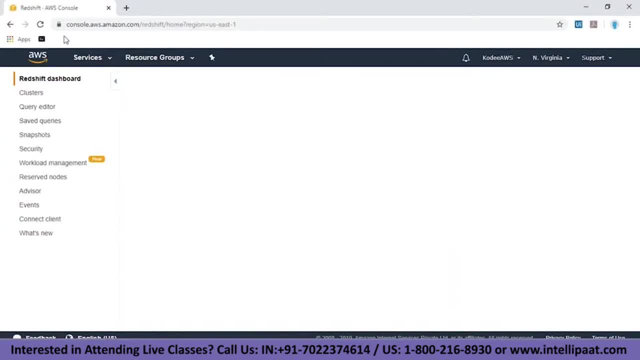 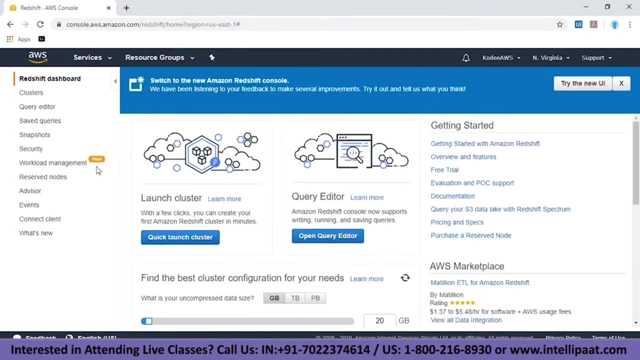 if you have typed something, don't click on this X, it goes off or something happens. So if you choose anything, you don't get this part. I don't know why. so Yeah, so this is the basic dashboard right now. So launch cluster and query later. 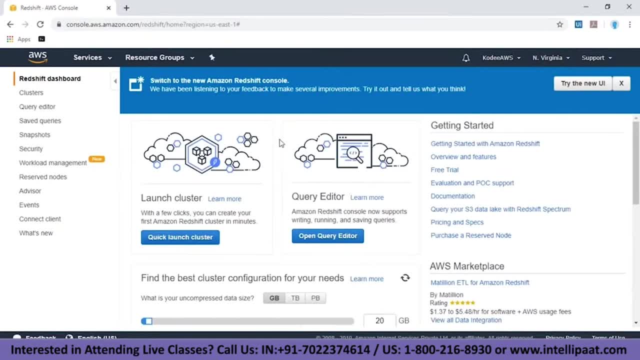 These are the two main services they provide in redshift. This is for launching a cluster, This is for querying the cluster we created. So these are the two services and find the best cluster configuration for your needs. So this is the tool they provide. 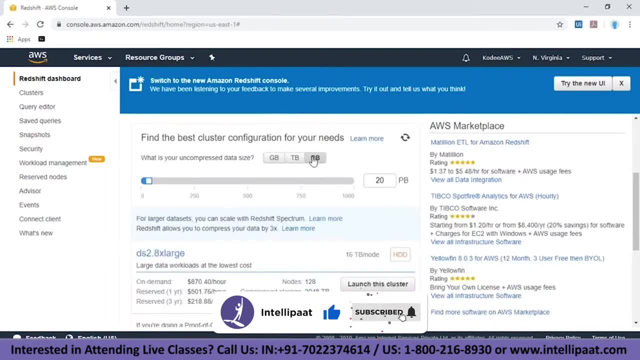 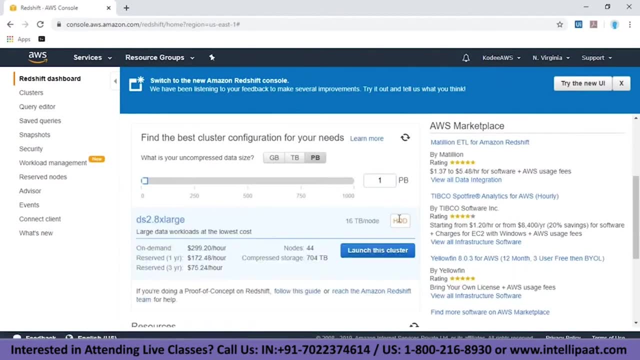 This is a service. So if you want to petabyte scale, then you can choose here and you can choose the number of petabytes you need. So five or one Or four, so three, let's say 20 again. So here they provide you a cluster name. 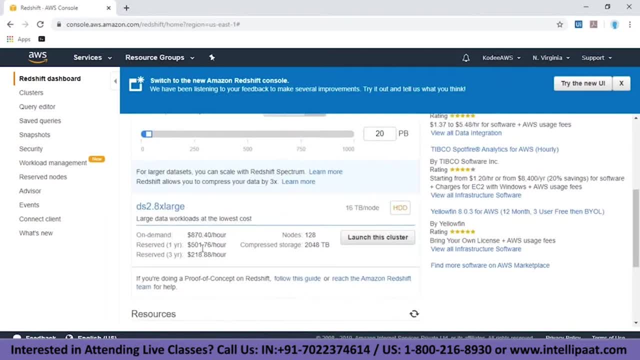 They provide you the amount. They also show this. or reserved for three years It's 218 dollars. reserved for one year It is 500 and 1.76 dollars per hour. per hour. This is not per year. This is for our and on demand. 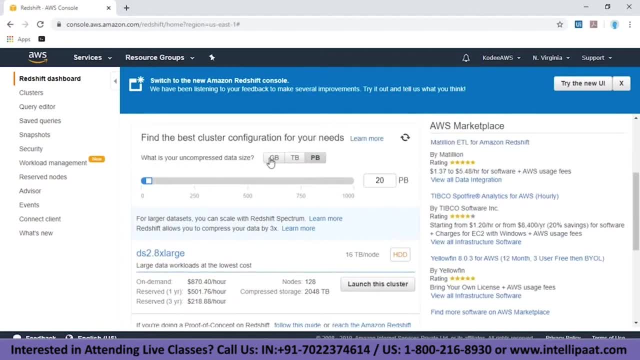 It is 870 dollars per hour. So this is one tool which which you can use for GB 20, GB DC to DC 2. Large: This is the node type will be using today. So for this, if you reserve it for one year, 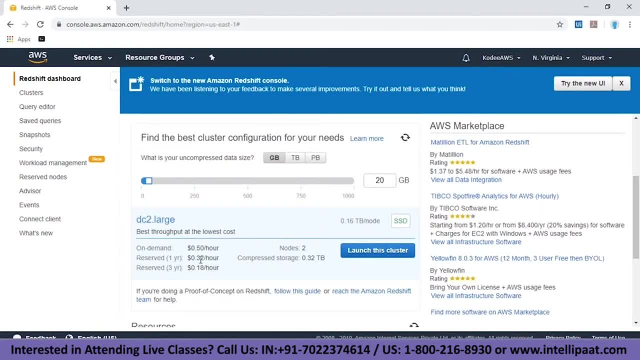 then every hour it is 3.32 dollars. If you reserve it for three years, every hour it's 0.18 dollars. So this is actually very economic If you reserve it for three years, if you are using it for three years, 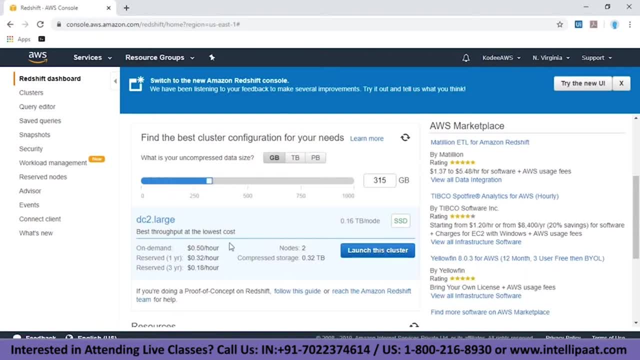 you can directly launch a cluster from here after choosing it. So like this, you can choose it from here and you can just select it for TV. So it provides gives you recommended options. So you can see recommended DC 2.8 into large, DS 2.8 into large. 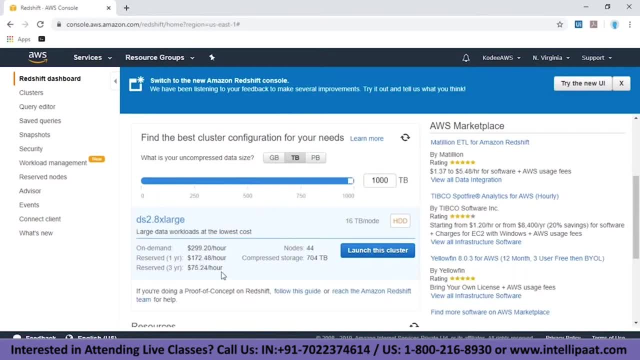 So the price also varies. It also shows you the exact amount for the storage which you take up question: Is there a maximum storage for the option, Like, for example, the large option? Yeah, I think thousand petabyte, for so this is the maximum capacity. 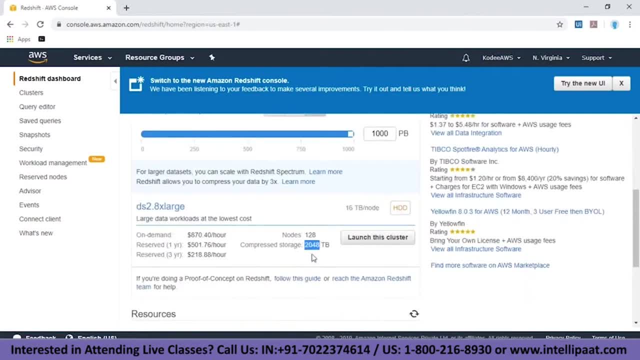 that is 128 nodes, 2048 DB compressed storage, this compressed storage. So basically you can scale up to thousand DB here and then 16 terabytes per node. You will have 128 node. You will be provided 16 TV every node at the start. 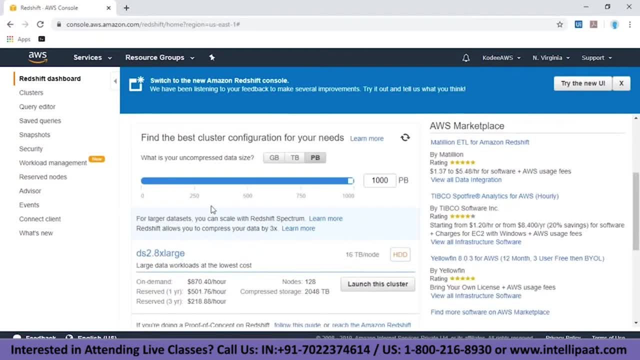 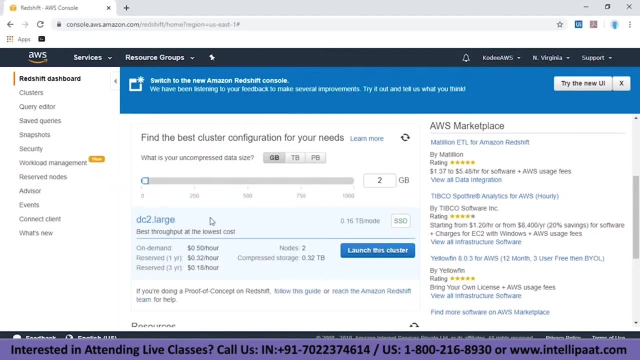 So I think this is the largest one. Oh, so the- that's the bar- changes, the option changes. Okay, So if I go to GB, provides me DC 2 large. No, there is one more instance. It's not shown here. 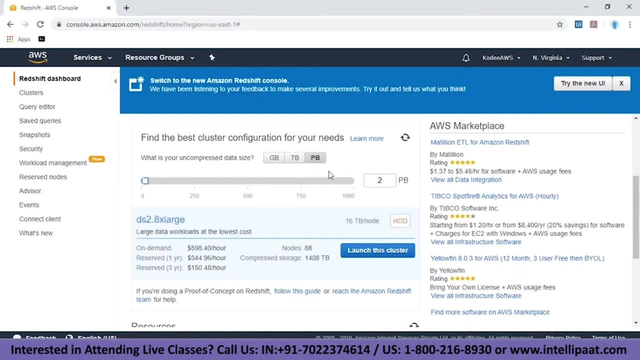 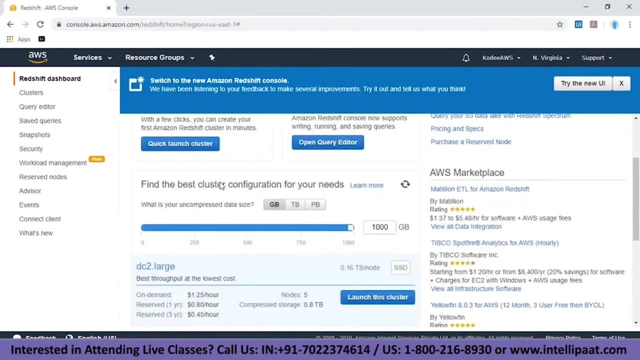 There is. that is the largest instance available, But here the biggest one is. they suggest only this. the largest one is, I think, RA 3 dot large. that I'll show now while launching the cluster. So then then you have this cluster Snapshots. 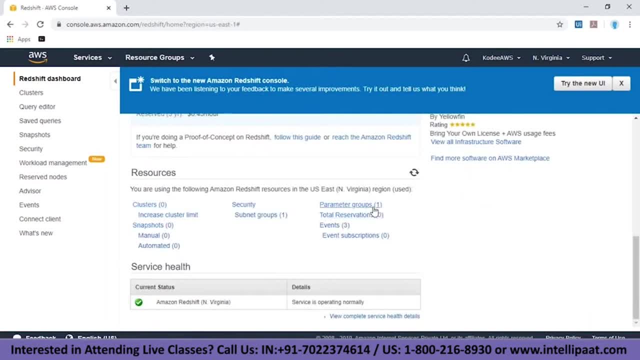 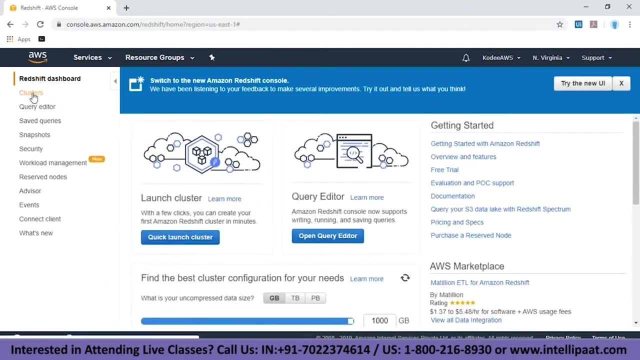 These are the basic things, So I created one. So there is one parameter group, three events, again events and even subscriptions, and these are the other options. This is for clusters, query editors, So if you run a query and if you want to save that query, 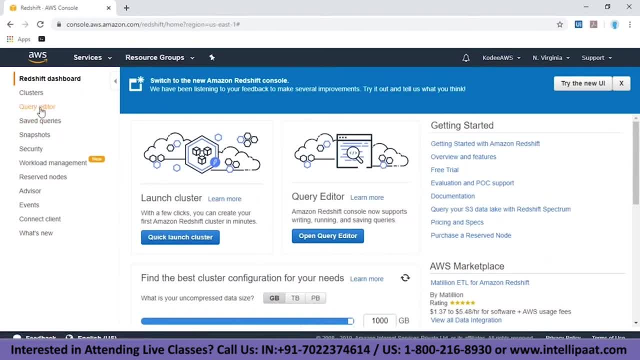 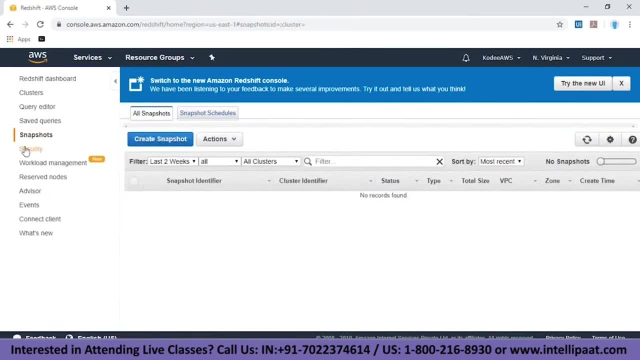 you can save it in saved queries. You can just there is an option for a save, just hit save, It will be saved. here I think I've saved one query up, So there is one query and then snapshot. I've not taken any snapshot. 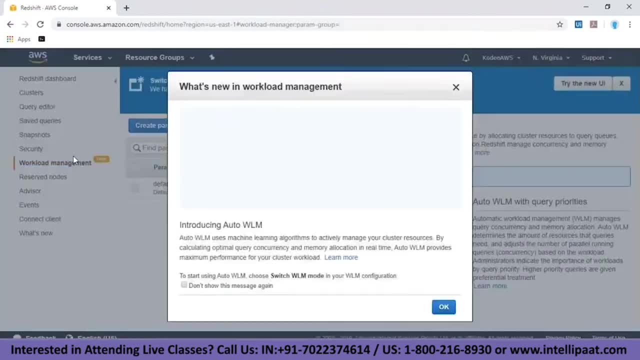 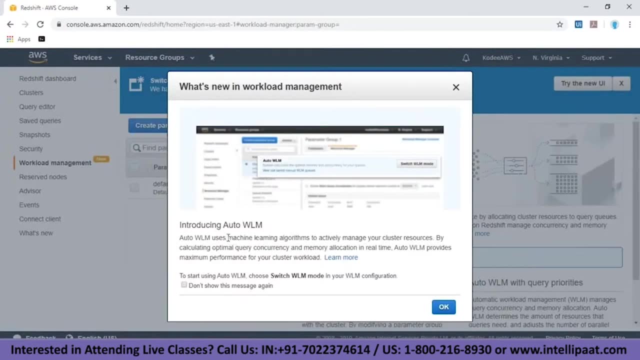 and I've not gone through security. then workload management: as I told you there, They have introduced newly introducing Auto WLM. So Auto WLM uses machine learning algorithms to actively manage your cluster resources by calculating optimal query concurrency and memory allocation. real-time Auto WLM provides maximum performance. 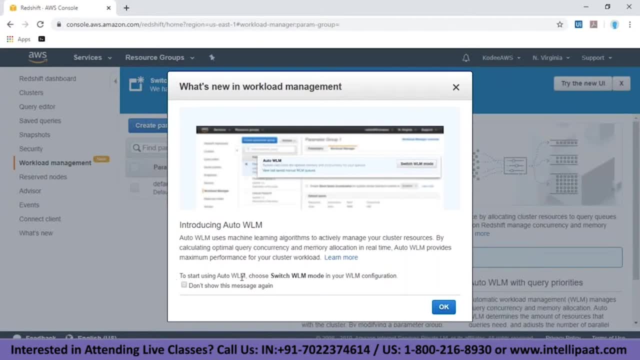 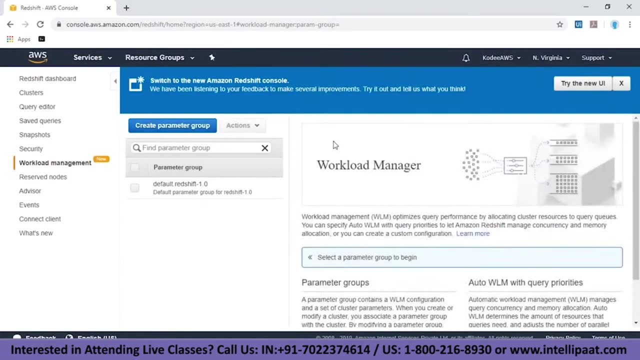 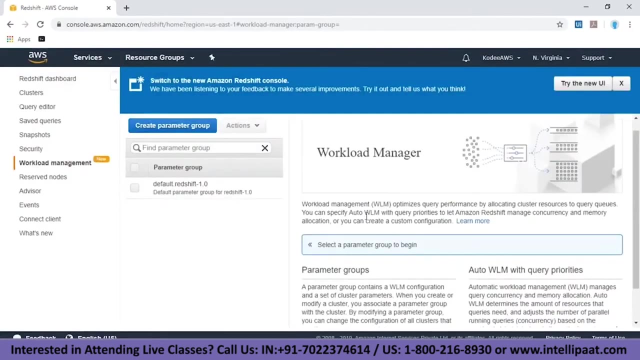 for your cluster workload. So to start with Auto WLM, choose switch WLM in your WLM configuration. Okay, So I think normally you get this. What is that Not a parameter group workload manager? So workload manager optimizes query performance for allocating clusters to query memories. 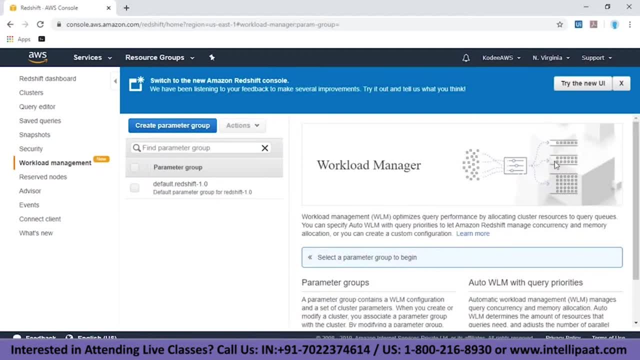 Yeah, so it creates my. you can create multiple queues, as I told here. So that is what they are depicting: data coming in. You can. you can manage your workload manager and you can create multiple queues. Okay, so that's fine. I'm not going to go inside that right now. 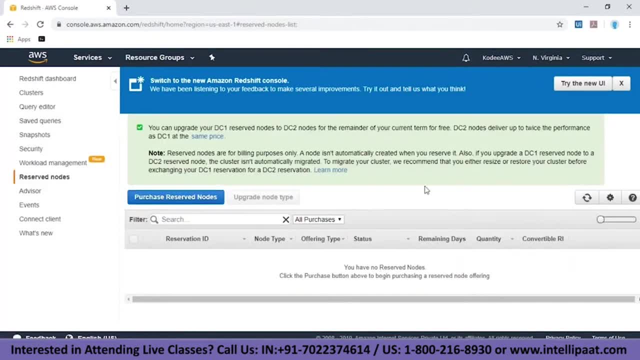 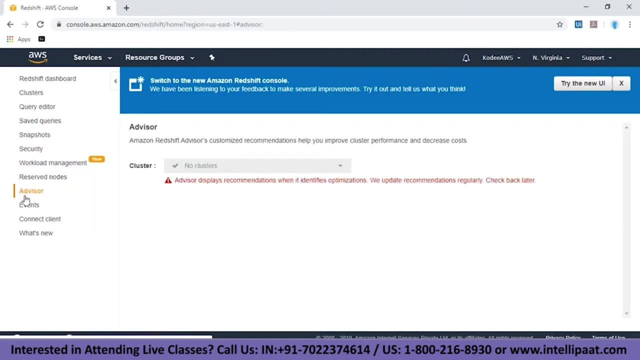 Then preserve notes. These are, as I was showing you. it showed on-demand pricing, then reserved for one year and for three years. You can purchase reserved notes here And I think advisor is a tool like recommendation engine for the Aurora cluster, for Aurora cluster. 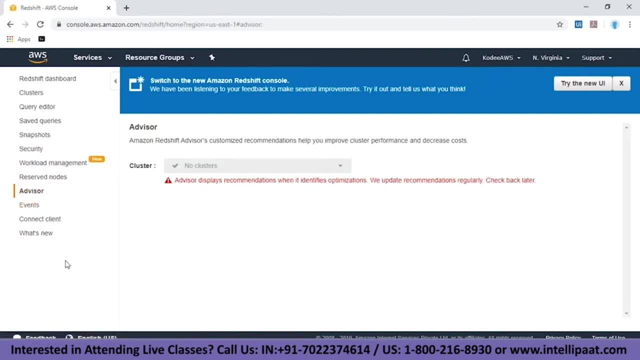 If you create an Aurora cluster, you have an option of recommendations here. If you click on that AWS or they automatically provide you some recommendations which you can implement or you don't need to Then events so you can see creating. Where are the ones? 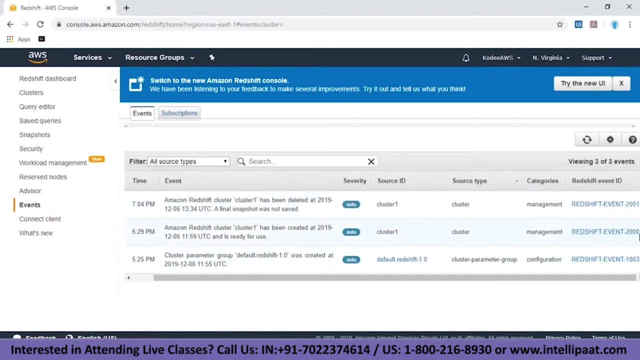 Yeah, so event to two, zero, zero one, two thousand thousand three. So even redshift has its own different types of events and I think you can. so this is basically informational. There is no severity. So basically, if it failed over, maybe that will create a event. 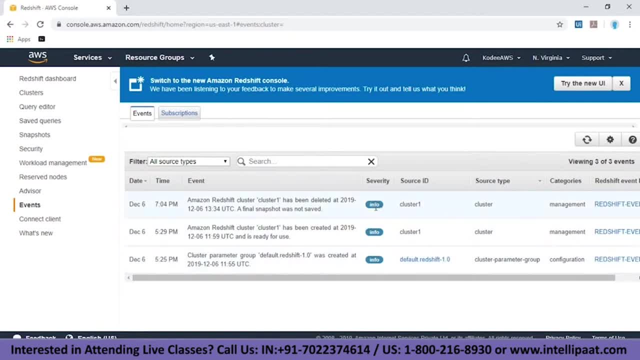 and it will provide a severity like a risk or high or something over here. and this is for Creation, This is for created, This is for deleted, That's it, And yeah, so this is connect client, So this is a for connecting client. 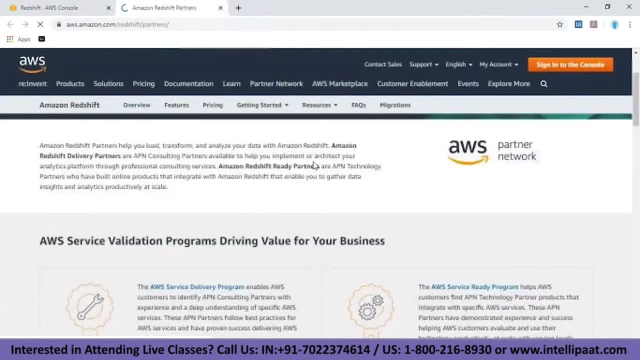 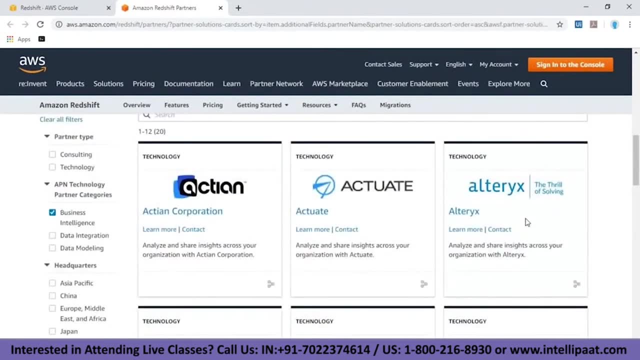 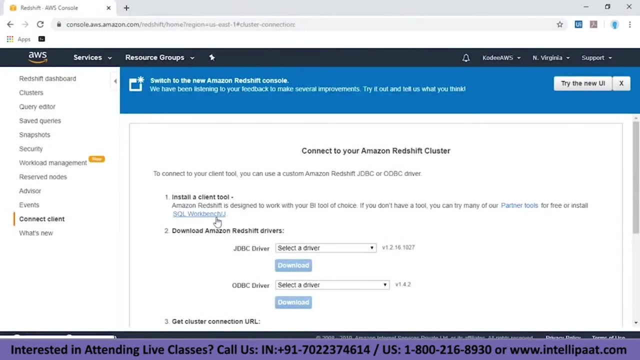 You can try these partner tools which they suggest. So I think these are those tools. I don't know Where are they, So I think you can use these tools which they are saying they are partnered, or you can just download the SQL SQL workbench. 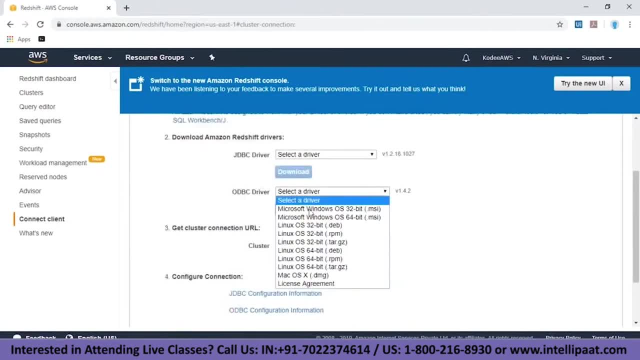 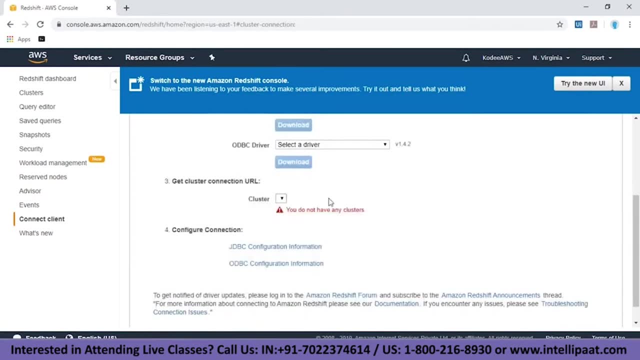 and you can select the JDBC, Or you can select the ODBC driver and download it from here itself, And so I don't have any clusters right now. So you'll have to choose one, will have to choose a cluster and you can download it and you can connect it accordingly. 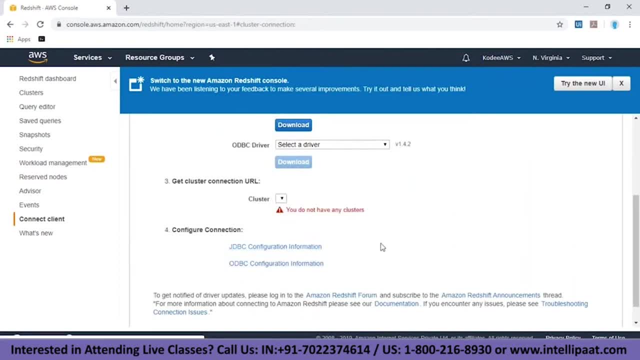 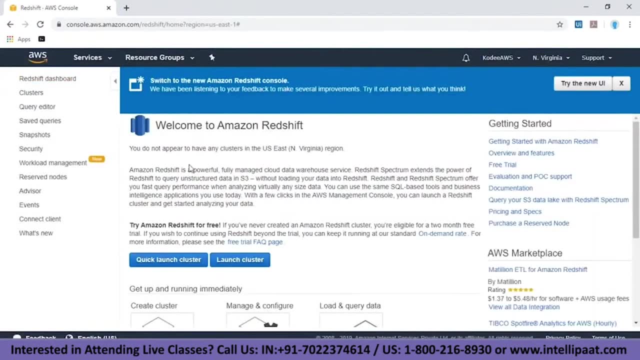 So you get configurations over here. So I'll not be connecting with JDBC or ODBC, I'll be using the query editor. Okay, So now let us start off with clusters. Let us launch a cluster. So again, there are two ways. either you can go with quick launch. 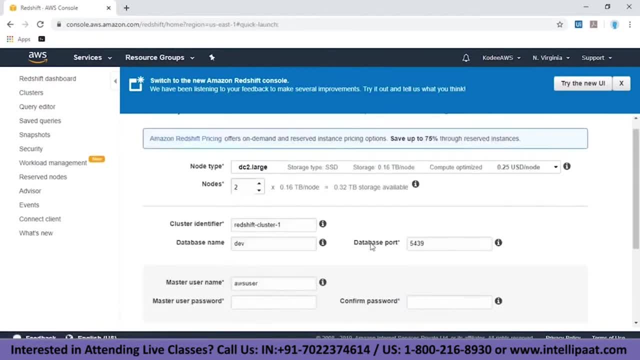 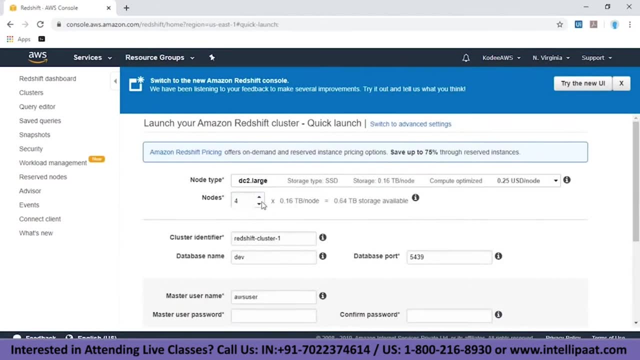 or launch cluster. So if I provide quick launch, it is just one page. You can choose the number of nodes here- one or two or three or four, and you can see if I choose 2.32 TB storage available. So if I provide 4.64, if I provide a number, 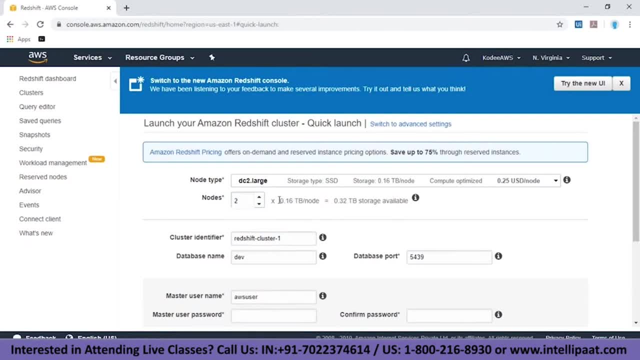 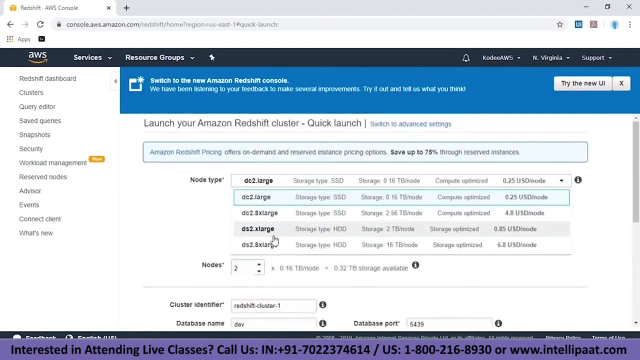 it increases accordingly because it's 0.16 per node And also you are provided with the instances over here, The type of the node types, So dc2 dot large, dc2, dot 8x large, dc2.. So these are the things we discussed. 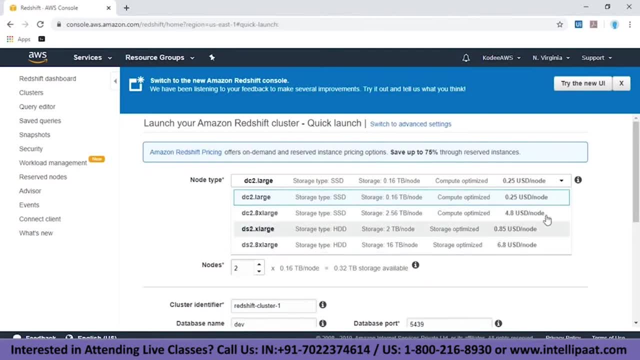 and also they provide the pricing here. Now I think this is better, better looking than Aurora. They don't provide the pricing for the instance classes and the storage they have provided per node for dc2 dot large. It's 0.16 per TB per node. 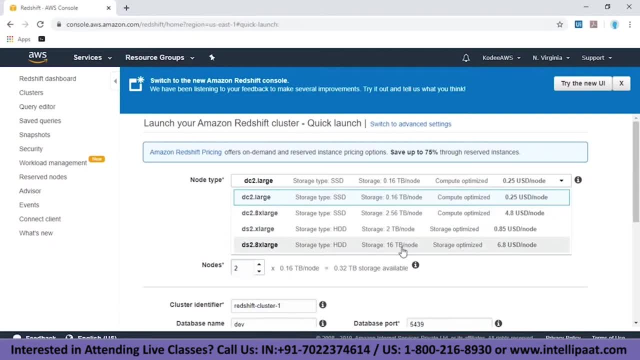 This is 2.56 per node, 2 TB per node, 16 TB per node, So these are dense storage engines. These are dense compute engines, So these are for compute, so they have lesser storage. and so, accordingly, if they have lesser storage, 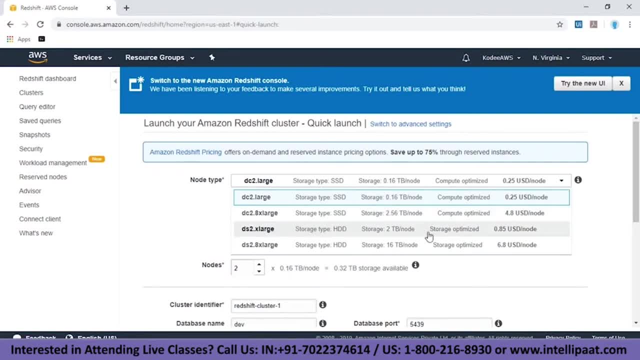 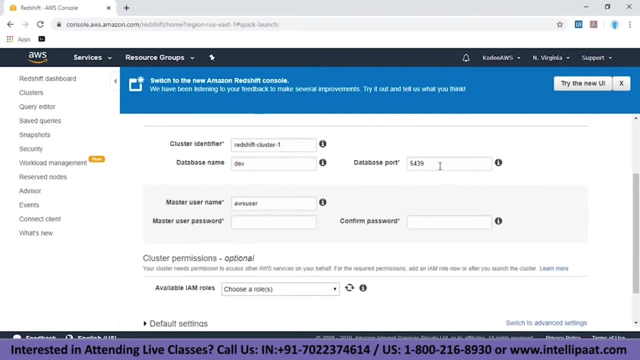 it is an optimal. they have optimal memory and here the storage is very high. You can store a lot of data in these two node types. You can choose them from here and after that you'll have to provide a name, then provide a database name and provide the port number. 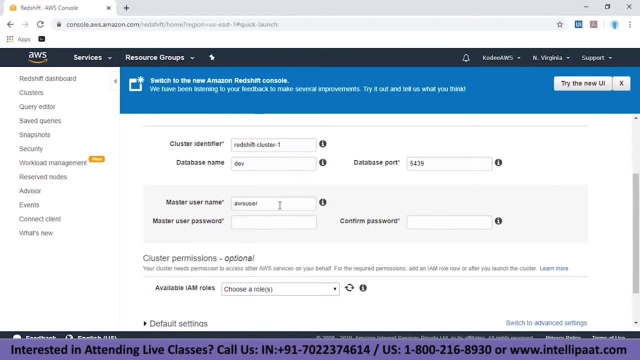 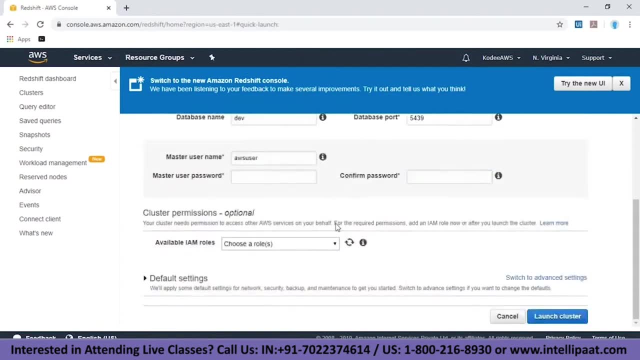 This is the default, It automatically takes it- and then master username: You will have to provide the passwords and if you are going to use any other service- So, for example, I'm going to show you how to load from S3. So you'll have to choose one of the roles. 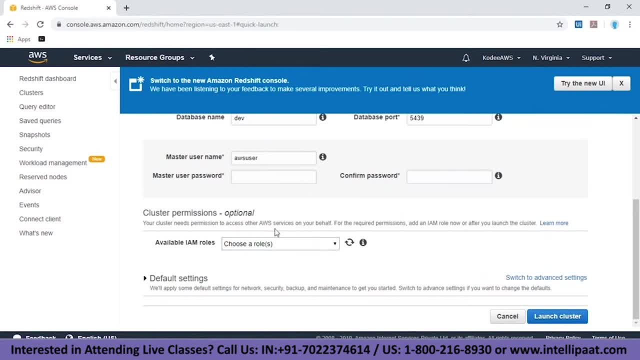 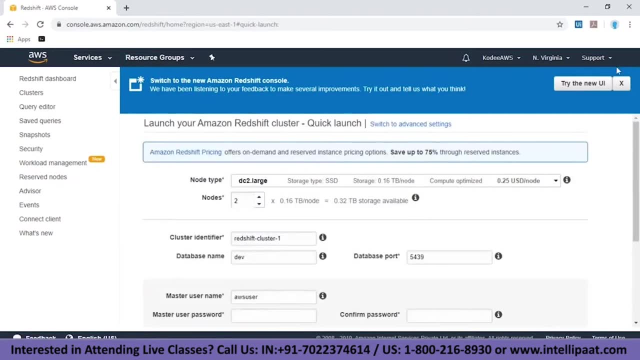 I'll also show what kind of a role to create. So first let us create the cluster and then we'll move on to that part. So either you can use the quick launch or you go. you can go to that one settings again If you have typed something, if you close this, 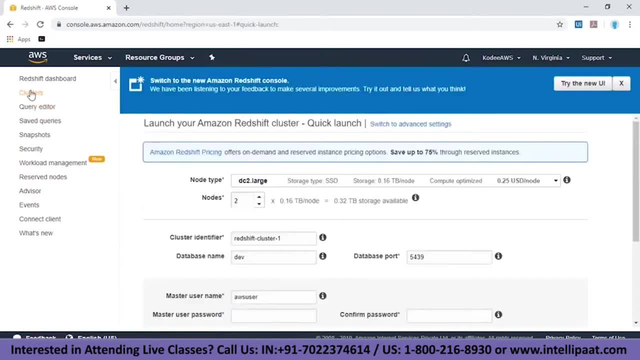 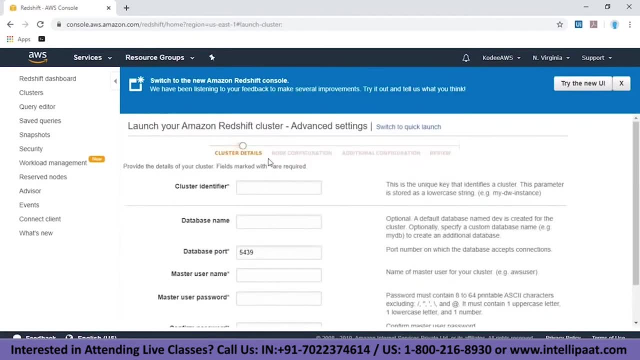 particular page goes off. So okay then, yeah, I'll just shift to advanced settings. So here you'll have to configure one by one. first You'll have to provide the cluster details, then you'll have to provide the node configuration, then some additional configurations. 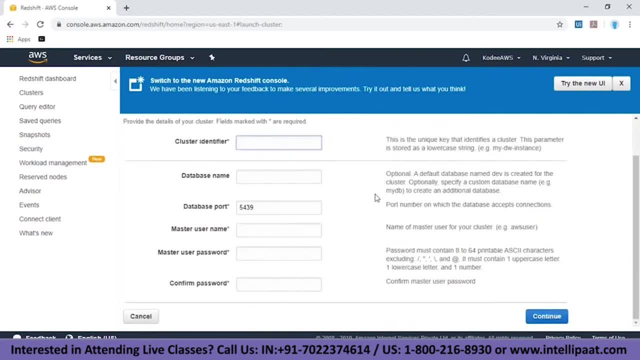 like, I think, security groups or something. Okay, So now, first cluster identifier. I'll provide cluster one. I don't have a cluster. then the database name, So optional. this is optional. This is not mandatory. You can see there is no star here. 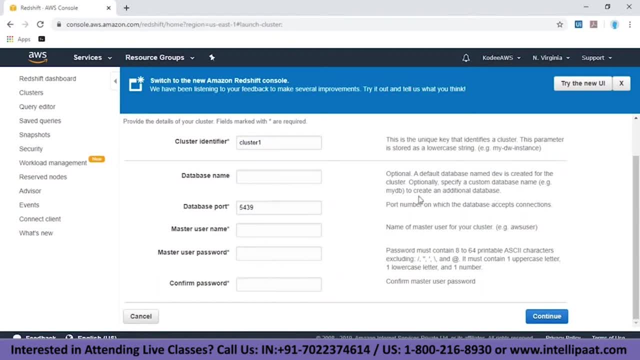 A default database named dev is created for the cluster. optionally specify a custom database- example my DB- to create a additional database. So a database is already created when you normally clear create a cluster. if you want an additional database before launching the cluster, then you can provide the name over here. 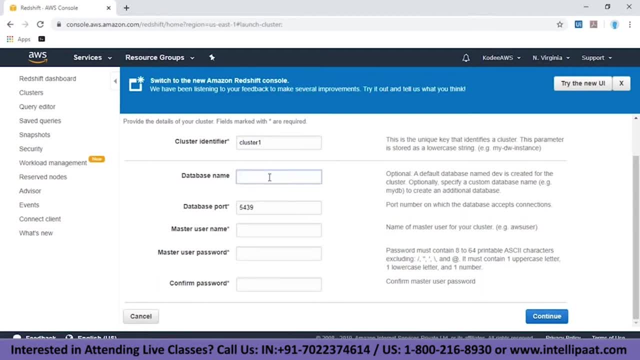 and then, after creating the cluster, you can create any number of databases inside that. So I'll provide a name. Let's say so dev, so just create one. Let's say test database name test, So I'll just give test one. I don't know. 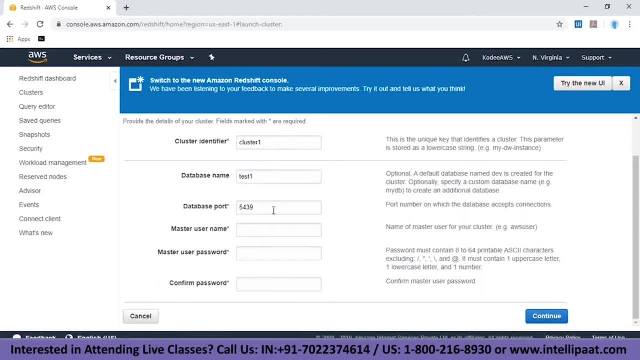 I don't know whether there is a test already inside. Okay, so cluster one: test. one port number is 5, 4, 3, 9. master user: I'll just go with admin for password: admin 1, 2, 3, but I think you'll have to provide a combination. 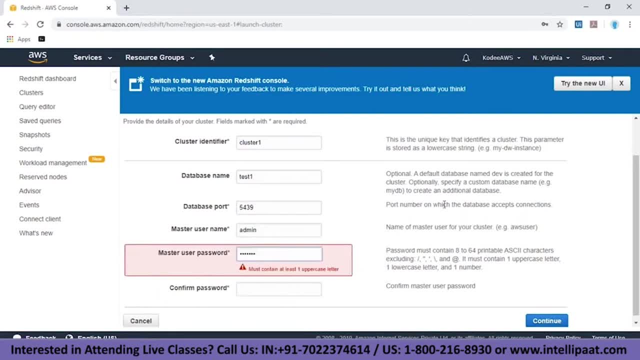 So it has to have one uppercase letter and also one number. So they provided that here, So I'm just going to make my a capital. So still, it's admin: 1, 2, 3 soda. So now continue. now here You'll have to choose the node type. 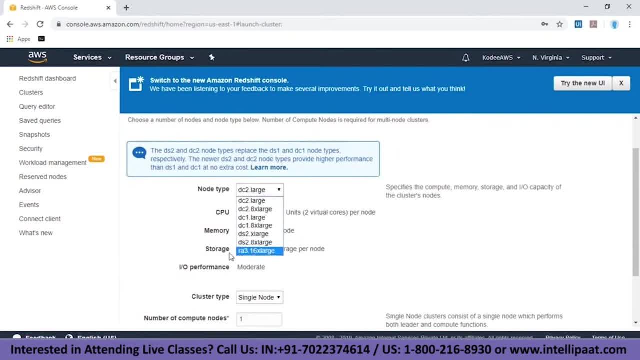 So here you can see, in quick launch You did not see this node type or you only saw DC 2. Large DC 2.8 X. large DS 2. Large DS 2.8 X. last these through D, These two are the previous generation node types. 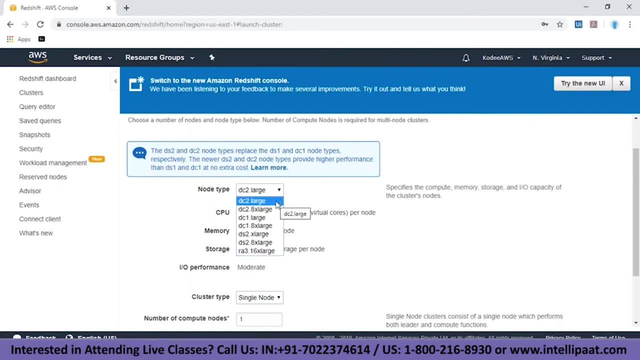 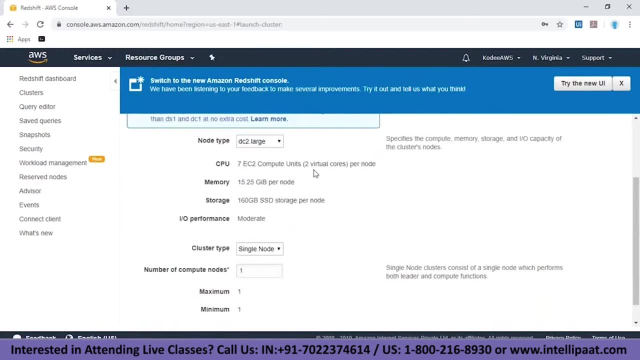 and this is the newest one. Yeah, so I'm just going to go with DC 2. Large, and again you also choose DC 2. Large, and here 7 AC 2 computer units to which will course. So for node, for node. 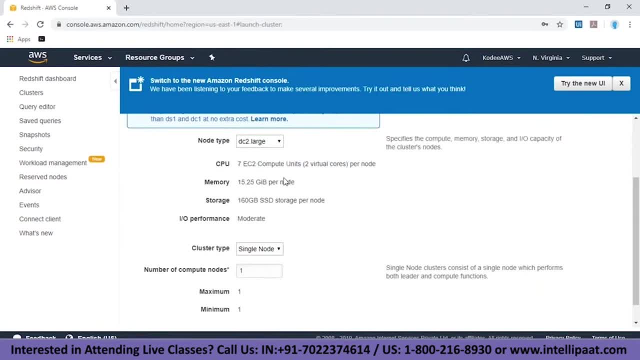 it provides seven different computer units. As I told you, there will be node slices. So these are them. So there will be, I think, seven node slices accordingly, and then memory: 15.25 gigabyte per node. That is, I think, yeah, so 15.25 gigabyte per node. 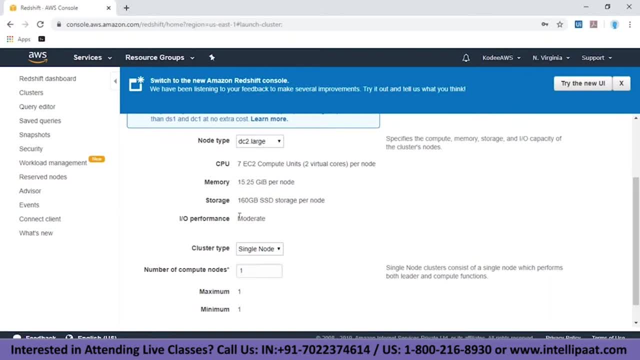 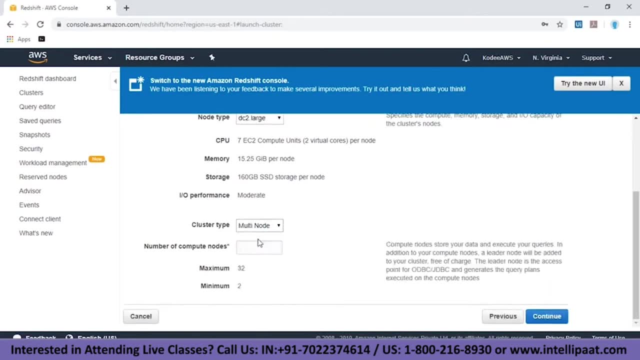 and then 160gb SSD storage per node- Yeah, moderate, Yeah. And then it can be the single node. single node, There is one option, one or multi node. the maximum number of nodes you can provide for a DC 2 dot large instance type is 32.. 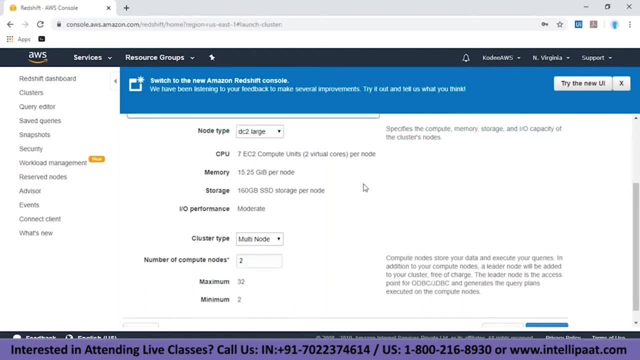 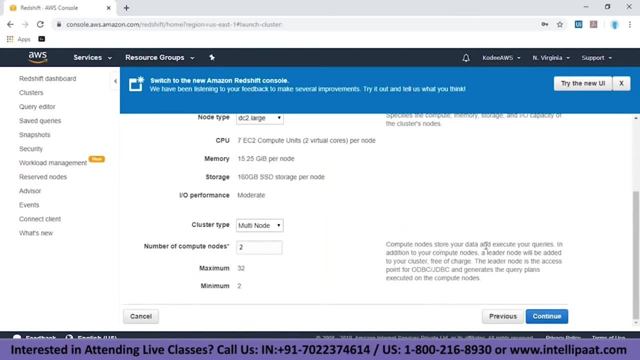 So I'll just go with two. I don't want a huge instance right now, So two is fine. So next, you can also read this: So compute nodes store your data and execute your queries. in addition to your compute nodes, A leader node will be added to your cluster. 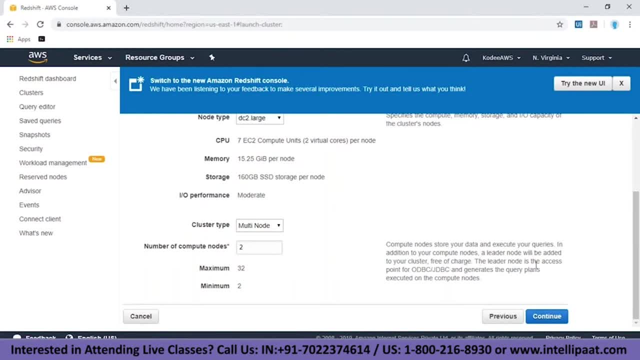 Free of charge. The leader node is the access point for the ODBC, slash JDBC and generates the query plans executed on the compute node. So also one of you asked whether data node is only one. is the is that might be a single point of failure. 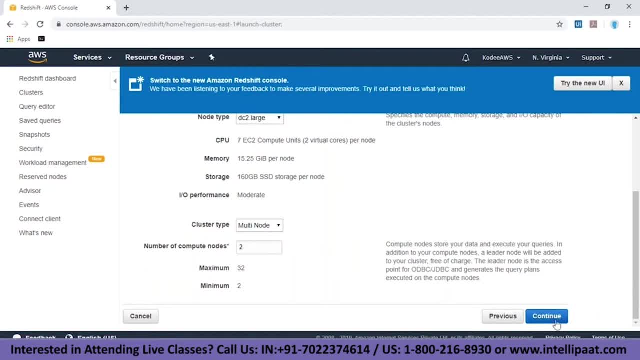 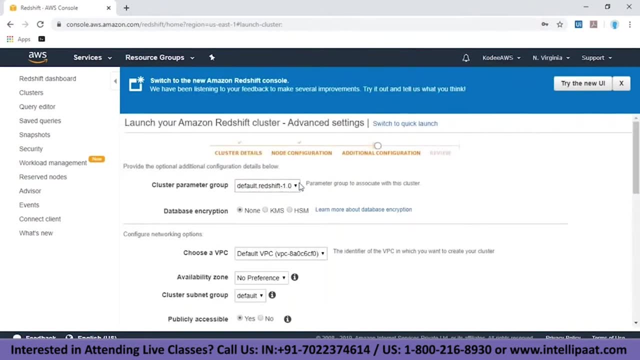 that also will look into right now. then continue. So default redshift. There is one parameter group already existing. It automatically took that, as he told you, a parameter group Would be a set of flags. They'll all be flags, You'll just have to provide the value. So it automatically takes a default one. If you want to create your own one, you can. you can create your. you can edit this, I think. and then database encryption: You can either go with none- You don't need right right now, I do not need- but you can go with KMS. 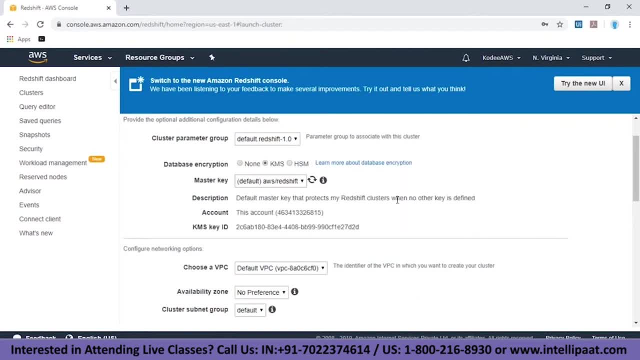 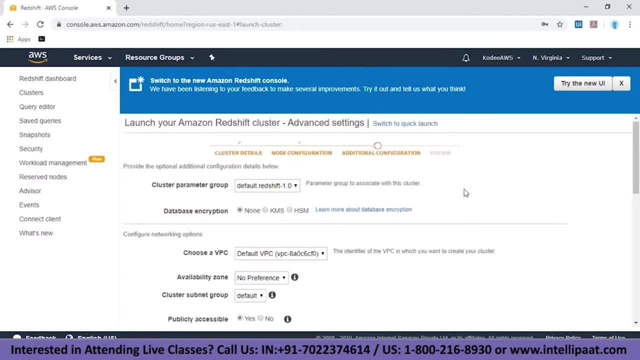 They encrypt it with their own default key, which is available in AWS. You don't need to do. anything is encrypted For this particular account, which is my account, So I'll just go with none right now and then VPC default is automatically taken. availability zone. 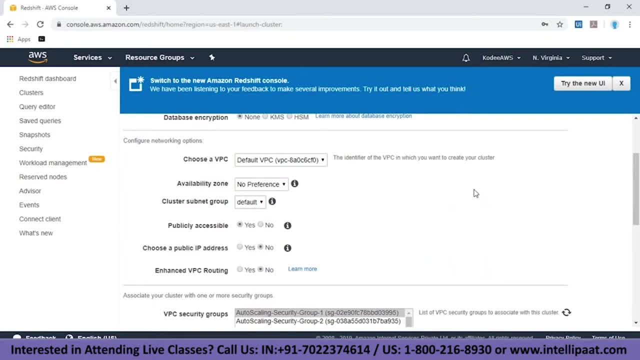 then I'll be able to connect with SQL client and then choose a public IP address. So here, what does they mean? is they provide an elastic IP address for this? So if I click yes, you can if you already have a elastic IP available in your AWS console. 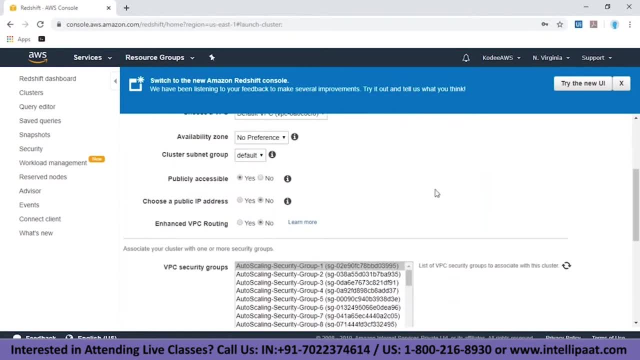 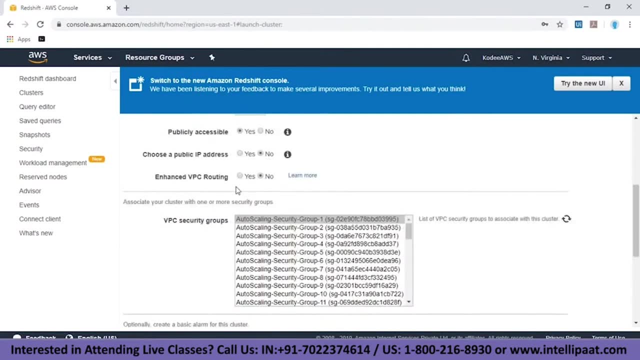 you can choose. if you do not have just provide No, they'll create on automatically and they'll assign it. to assign it to the redshift cluster and then in answer to VPC routing. So basically, if you click on enhanced VPC routing, all the queries 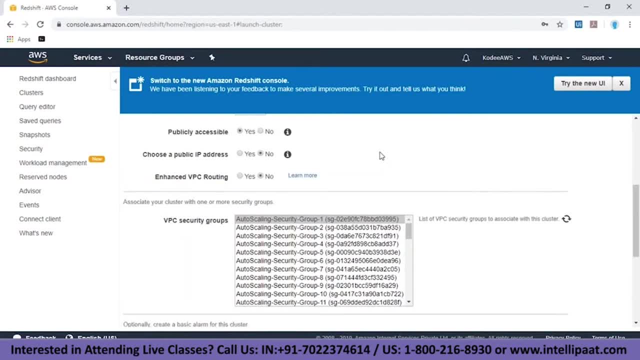 all the data going in and out will go through only with. all the data coming in or going out will go through one particular VPC. So you'll have to do much more configurations for that. You will have to create a VPC which does not allow data to go out. 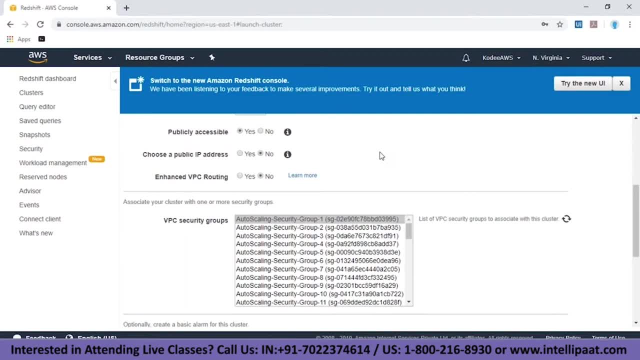 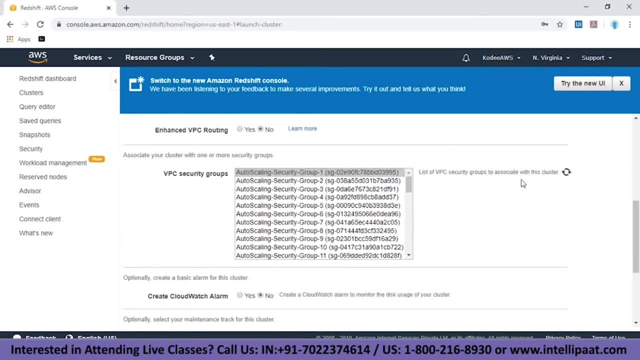 It should not be publicly accessible and all that. So that's what VPC routing basically means, and then list of VPC security groups to associate with this cluster. associate your cluster with one or more security group. So this, I think. you cannot select anything. 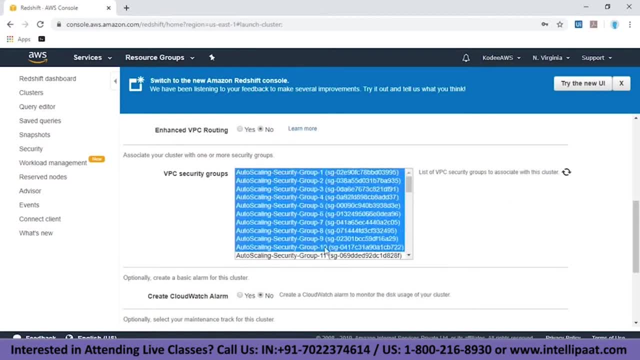 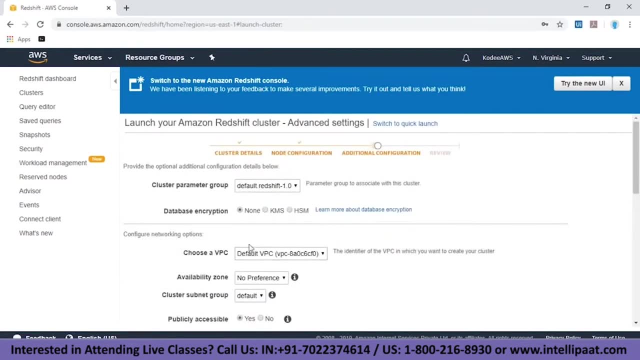 It is automatically. it automatically picks it up. but you don't need to provide anything because I said: choose a default VPC, It automatically takes my default security group. It does not take any other security group. if you provide another VPC, if that VPC is combined. 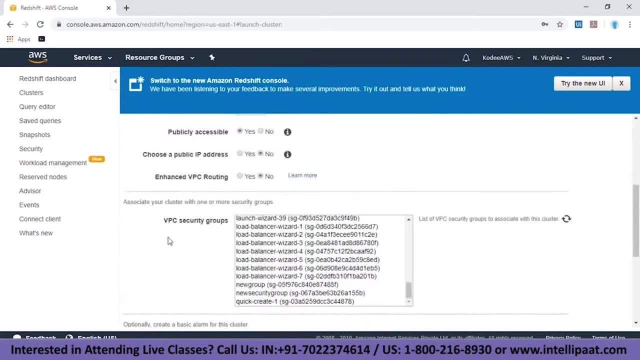 with a particular security group, then, yes, you can, that will automatically be taken, but right now there is default. Yeah, so this will be automatically taken for me, because that is my default security group, and then you can create a cloud watch alarm directly from here. 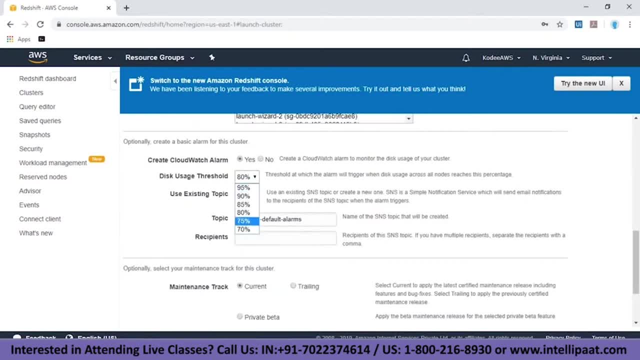 You can choose. So these are the only options provided in this console- There is 70 till 95- and use existing topic. So you guys all know what is a topic. just basically used to send email notifications and use existing topic in a sense. 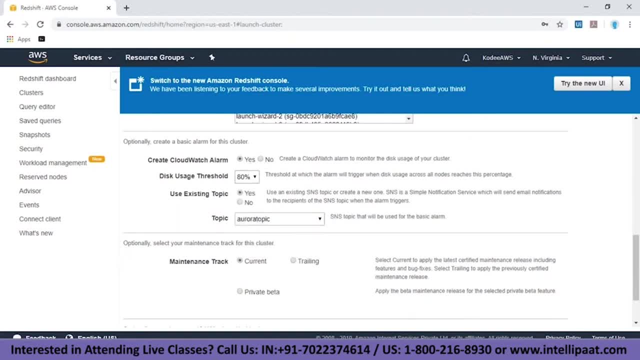 You will have to choose one, and that's it. You can create one from here. So, disk usage threshold- threshold at which the alarm will trigger when disk usage across all nodes reaches this percentage, So when the disk usage in all nodes are going to reach 80%. 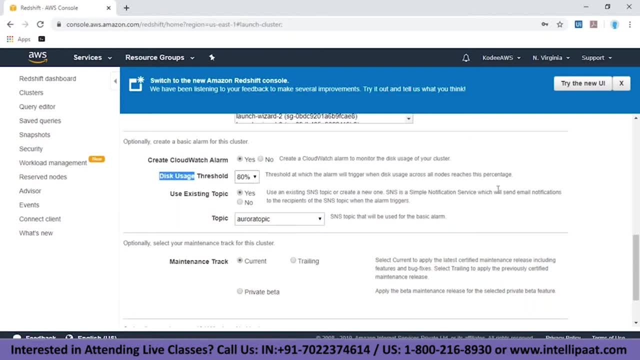 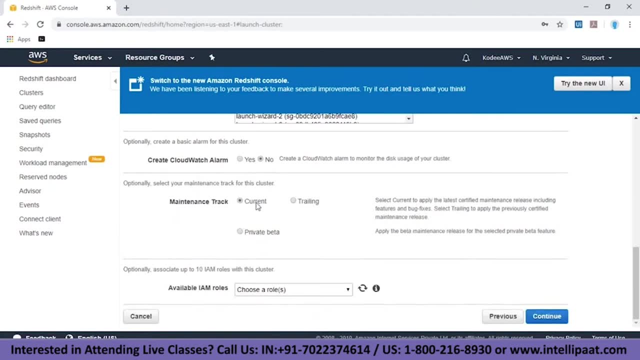 then this alarm will send to send an email to this particular topic, So I don't need a lamb right now. and then my maintenance track: current trailing and private beta. So if you choose private beta, you can basically preview the features, but you cannot. so I think don't choose this either. choose current. 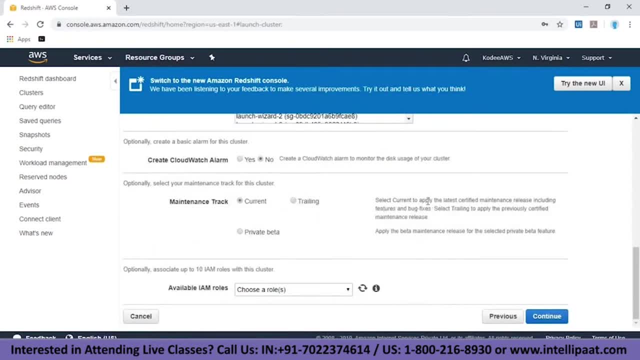 or choose trailing. so current. select current to apply the latest certified maintenance release, which includes the latest features and the latest bug fixes. If you choose trailing, it applies the previous. that is, the previous certified maintenance release, the one before this. So that is what trailing and this was current. 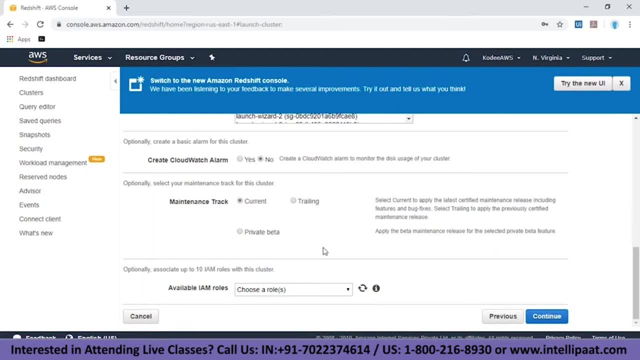 You can just go with current For the latest. So if you want to attach a, I am rolled right now. you can just directly go. I already have one. I can attach this or I can attach it later. So I'll attach that later. 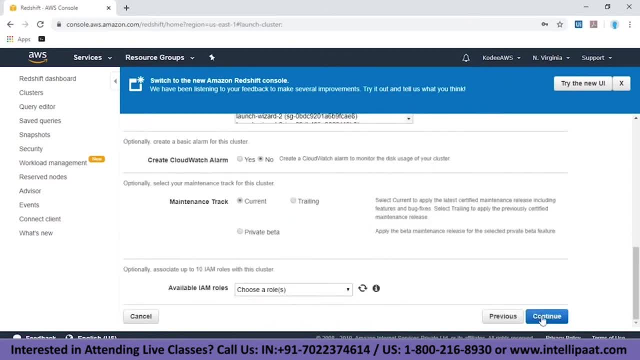 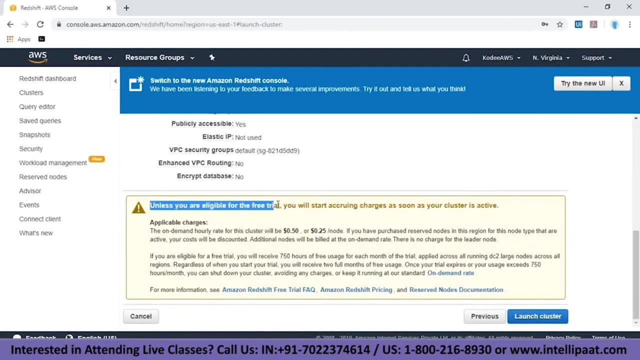 So, right now, let us launch this cluster. So these are the. we provided all the configurations. that is more than enough. and now, unless you are eligible for free trail, you will start occurring charges as soon as your cluster is active. So, as I told you, if you have not launched, so where is that? I'll take you home, I'll show you and show it. I just want to make you sure. So try Amazon Redshift for two months free If your organization has never created an Amazon Redshift cluster organization in the sense your AWS account. if you have never created a redshift cluster in your AWS account, you are eligible for a two-month free trail or for DC 2.. Large node: Yeah, you get 750 hours per month, enough hours to continuously run one DC to large node. 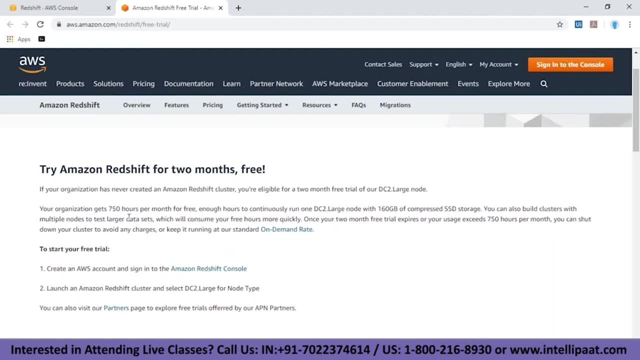 with 160 GB. So this, basically 750 hours from per month, is for one node. So if you run two nodes, that has will be divided between those two nodes. If you're on three, it will be divided between those three, four accordingly. So it goes on up to 32.. So if you run 32 nodes for DC 2. Large, then that 750 hours will get. it'll get over soon. So 750 divided by 32.. That's it. Yeah, so that's it. So what else? who's eligible? So you are eligible for the free trail if your organization has not created an Amazon Redshift cluster since July 1st 2014.. So if you have not created a cluster since 2014 or July 1st, 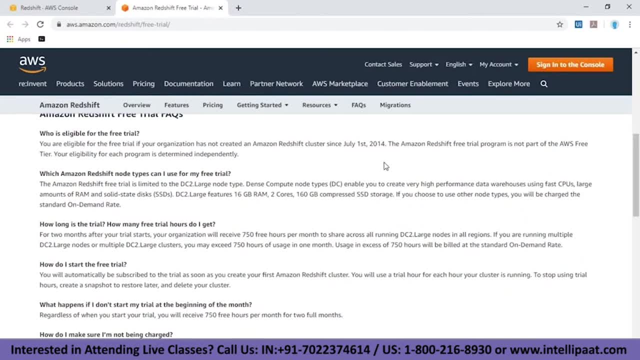 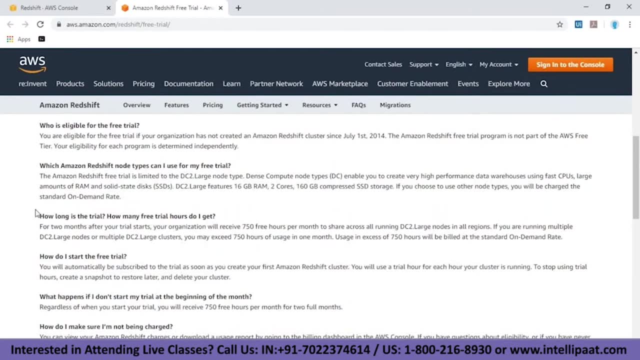 then you are eligible for this free trail program. Yeah, so I think most of you would have not created a cluster, So I think you'll be eligible for this free trail. Yeah, so others are the same. They state the same fact. 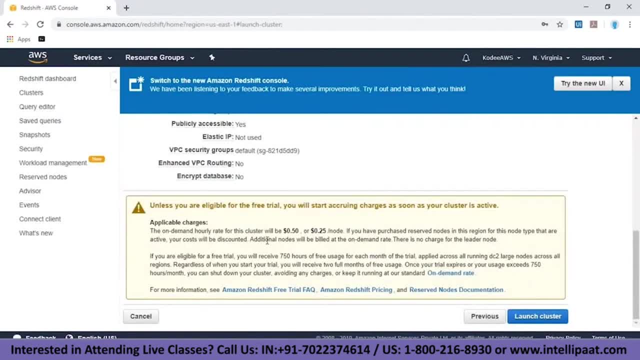 I just wanted to show that and yep So the if you do not have free trail, if somebody does not have a free trail, then the on-demand Harley rate for this cluster will be 0.5 dollars or 0.25 dollars per node. So for this there are two nodes, So plus a free leader node. So for the leader node you don't pay anything and 0.25 dollars. If you have purchased reserved nodes in this region for this node type that are active, your costs will be discounted. 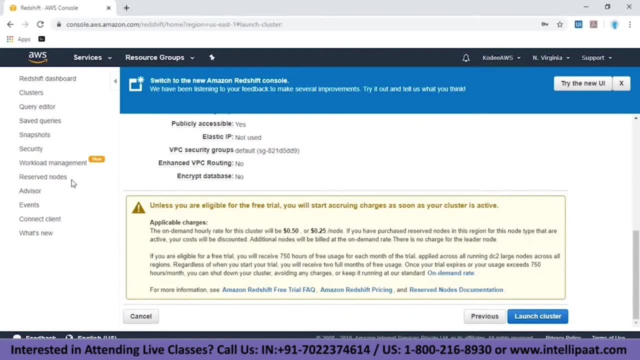 So basically, if you have a reserved, if you have bought a reserved node from here, so then in this region, so in North Virginia region, if you have bought a node, then that particular node, star, just will be discounted accordingly, And then there is no charge for the leader node. 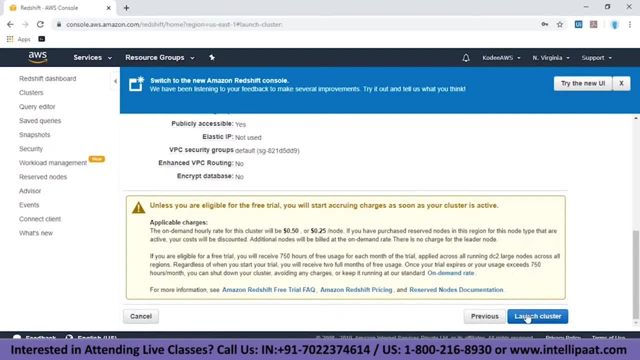 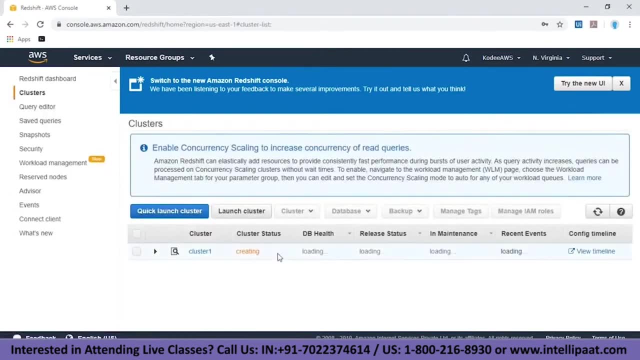 If you're eligible for free trail, they are there. It's the same thing, So I'll just launch the cluster. So now let us view all the clusters. I think it would have been created. It's creating. Yeah, it's still creating. 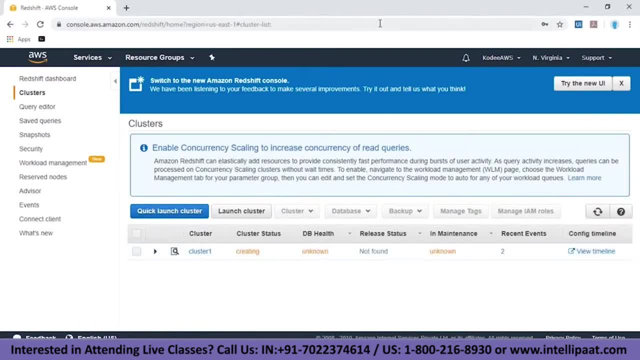 So once it creates, we'll be able to see inside that, We'll be able to see the endpoints and stuff. Let's wait until it gets created. I think it's available right now. This is a cluster is available right now. So three events happened. 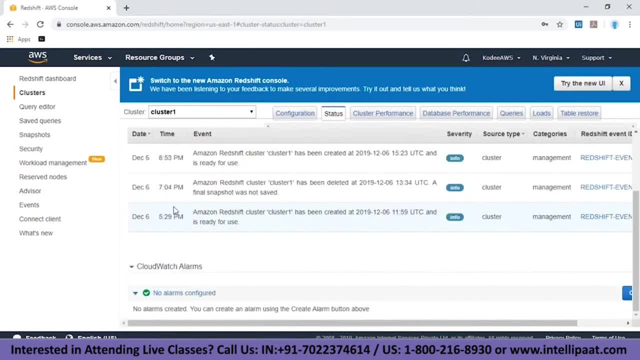 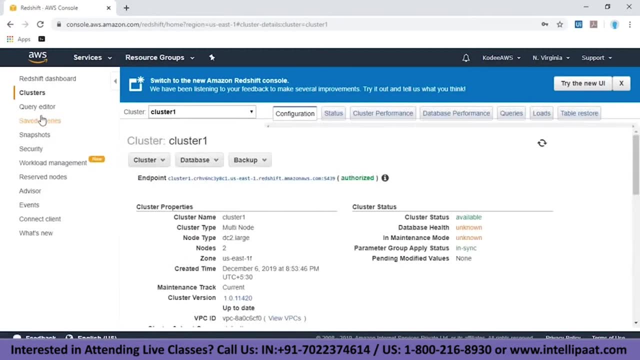 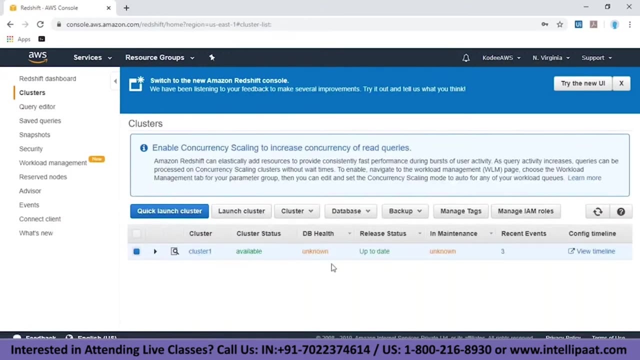 Created a deleted created. Oh, this was back, So right now it's created. Okay, Right now the cluster state is available. The DP health is still unknown. It'll check for the DB health and tell us. it'll also give us the detail. 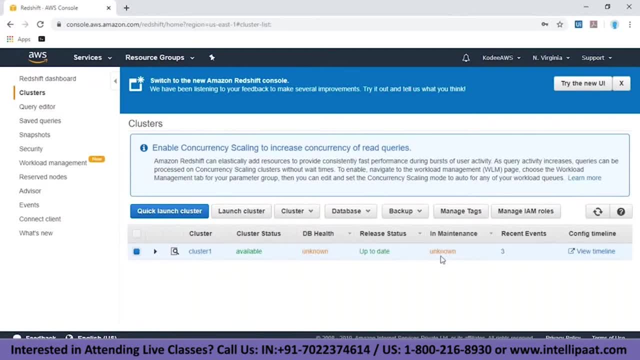 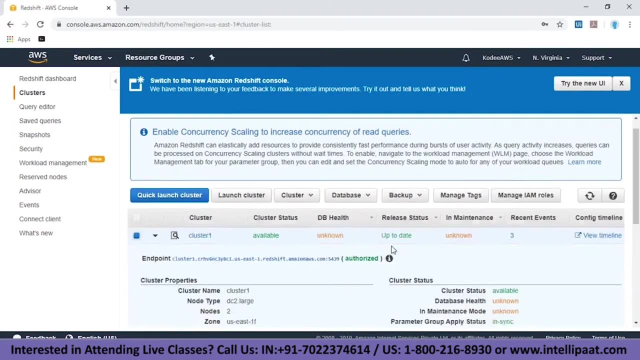 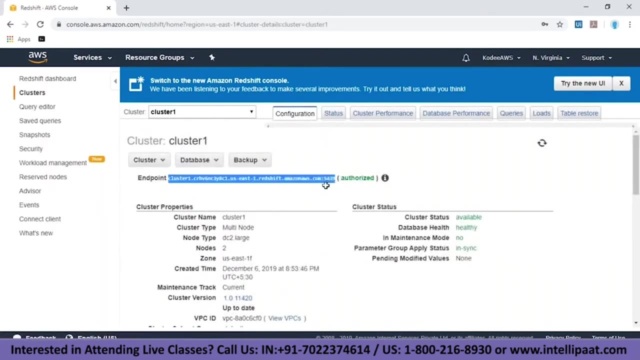 whether it is in maintenance or not. So it'll tell it's in maintenance or it'll provide not in maintenance, or something like that, and then coming down, So right now they have provided an endpoint. So yeah, so you'll have to use this endpoint to connect with your SQL client. 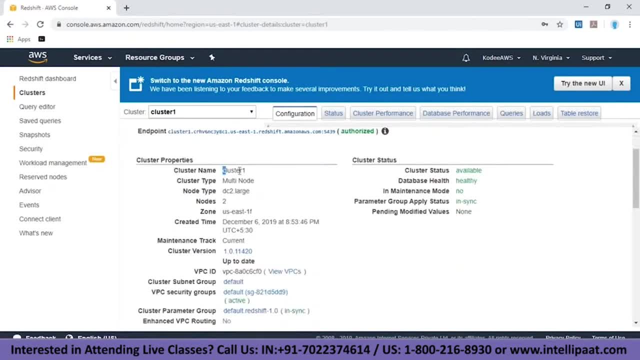 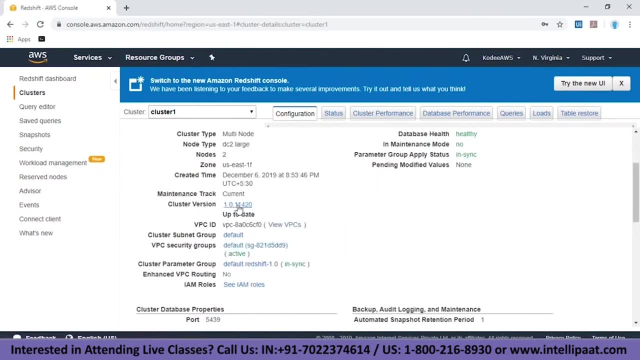 and then cluster properties. You have the name. it's multi node, node type to. it got created in 1f, the time and everything, the cluster version. It's up to date, the latest version. That's what I told, because if you scope, maintenance, track, current. 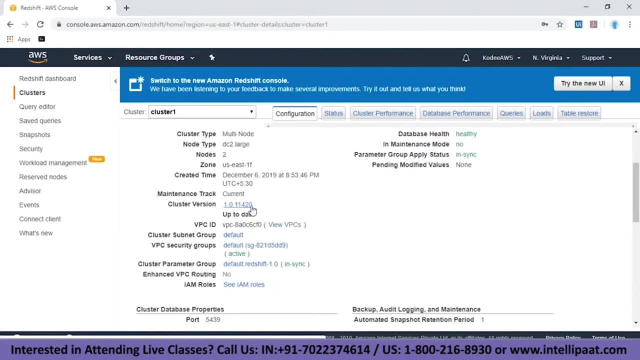 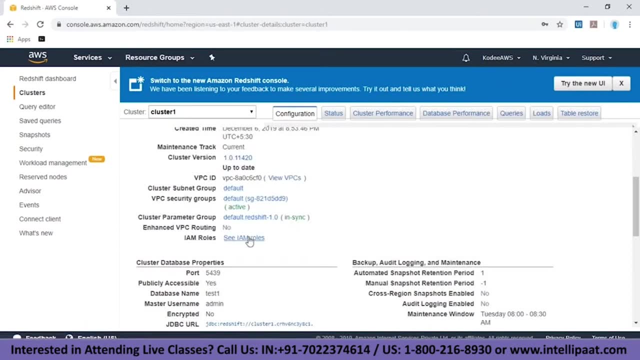 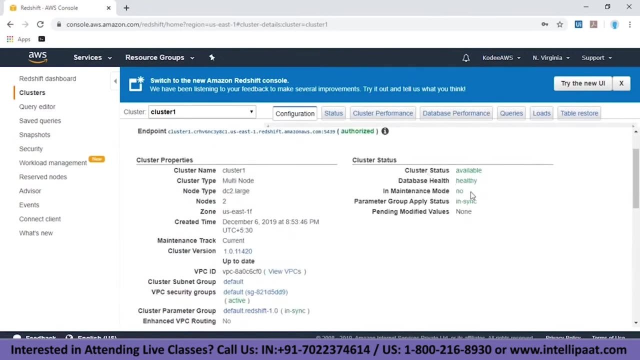 the latest reseal, sorry, the latest release will be used. and then VPC, then cluster subnet group, VPC parameter group. So I don't have any. I am group still. now. cluster state is available, So database health is also provided right now. It's healthy. 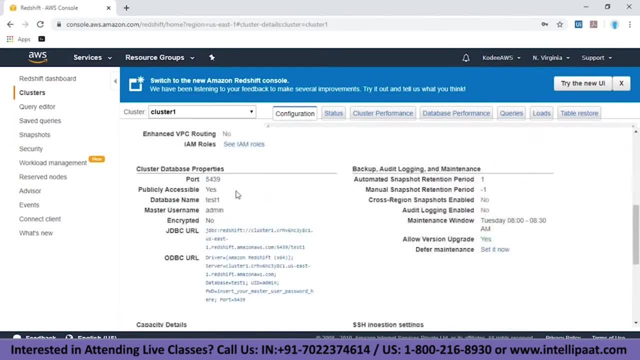 It's not in maintenance mode. Okay, fine, So now database properties. the port number is 5, 4, 3, 9.. It is publicly accessible. We created a database name called our video, created a database called a test one, and then we created master username admin. 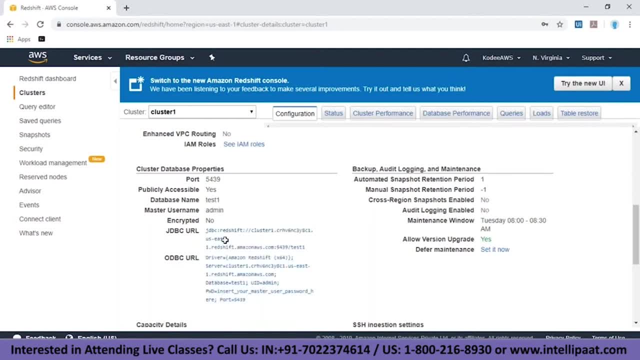 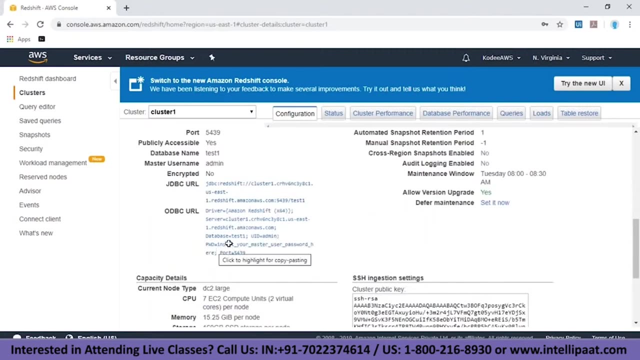 It's not encrypted, So they have provided for both. So basically, JDBC Redshift: colon the endpoint with the database name for ODBC, its driver Server name database test one UID admin password. You'll have to enter the master password and port number. 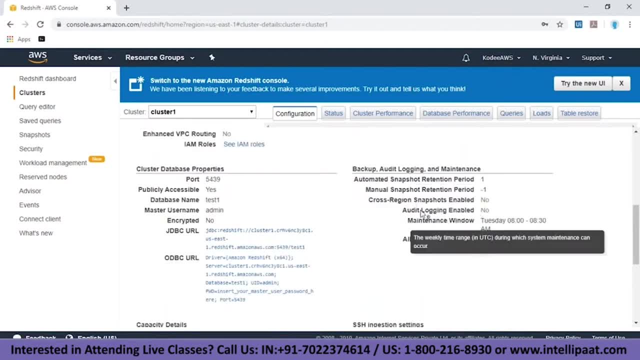 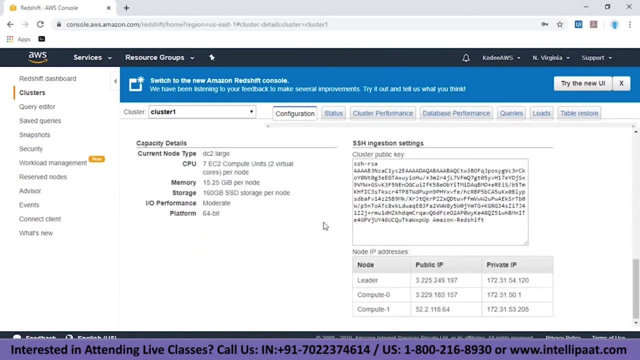 So this is the URL for JDBC and ODBC. and then, yeah, so this is backup, audit, logging and maintenance. a low version upgrade, Yes, Yeah, Okay, and here comes a capacity details: DC 2. Large. then we have total of seven easy to compute units, that is. 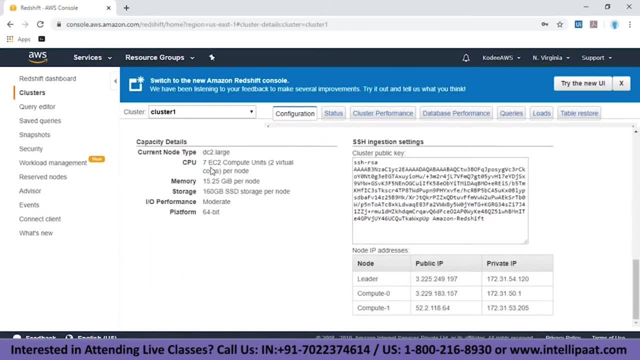 to which will CPU is per node. So according to that, there are seven easy to compute units, totally Okay, And 15.25 gigabytes per node. 160 GBS is the storage per node, moderate 64 MB, and this is the public key of the cluster. 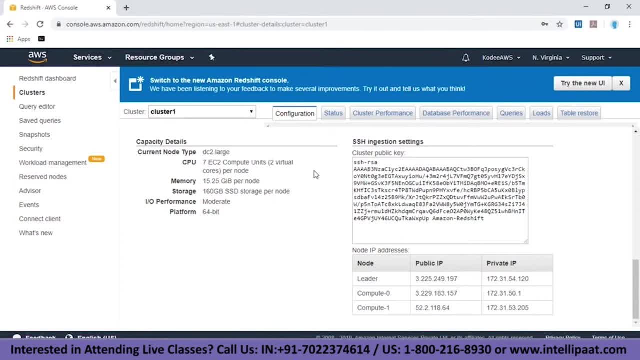 I think we can use this for SSH, So logging in with that, then send. they've provided the node IP addresses. So the leader notes IP address and private IP. is this, the compute notes public and this is compute 0, compute 1, so you can have up to compute 32.. 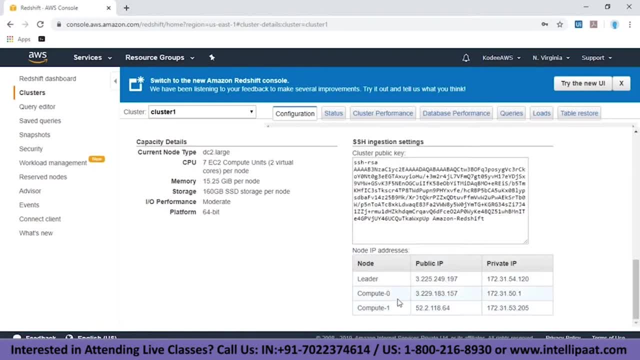 Sorry, This will be 31.. Yeah, compute 0, 1 or compute 1.. So, yeah, so, public IP, public IP and private IPs of these created nodes. So now, as one of you asked, are the? what will happen if there is a failure? 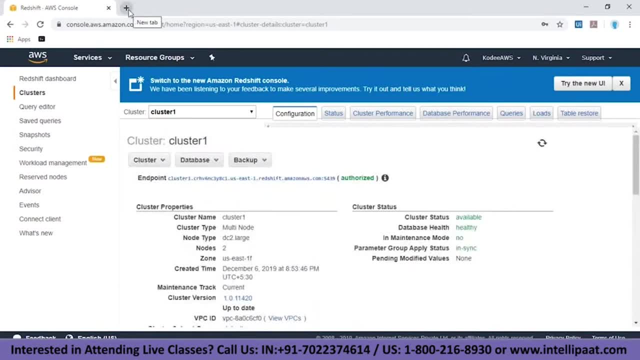 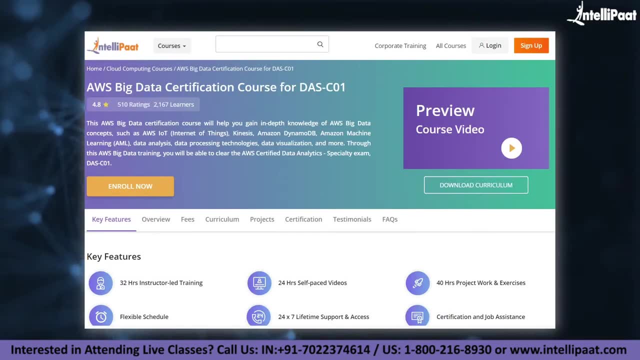 of the leader node that will check will go to the FAQ of Amazon rich shift. Just a quick info: guys into the pad. provides AWS big data certification codes Mentored by industry experts, The course link of which is given in the description below. Now let's continue with the session. 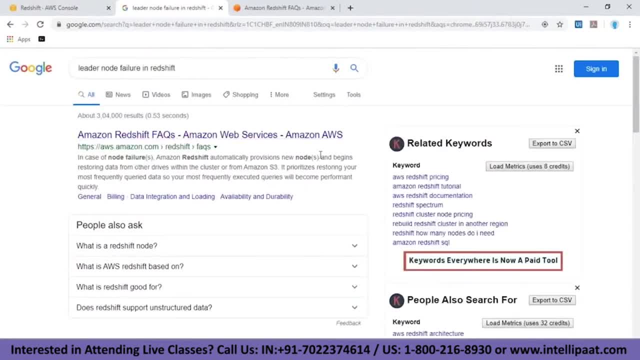 In case of node failures, Amazon redshift automatically provisions new nodes and begins restoring data from other drives within the cluster or from Amazon S3. It prioritizes your prioritizes restoring your most frequently query data on your most frequently executed queries will become performant quickly. 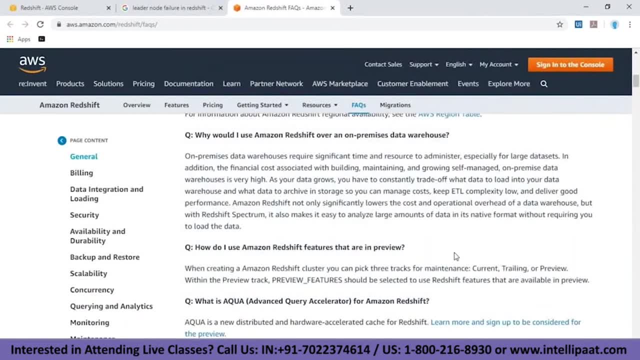 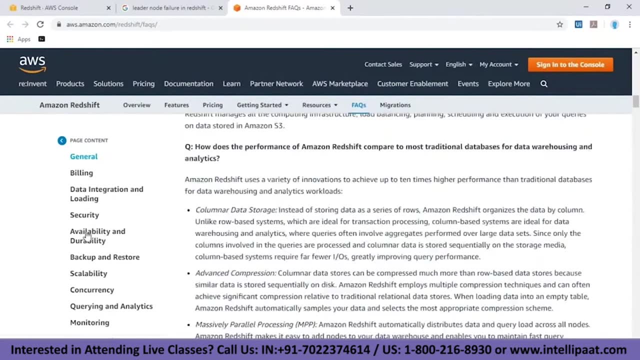 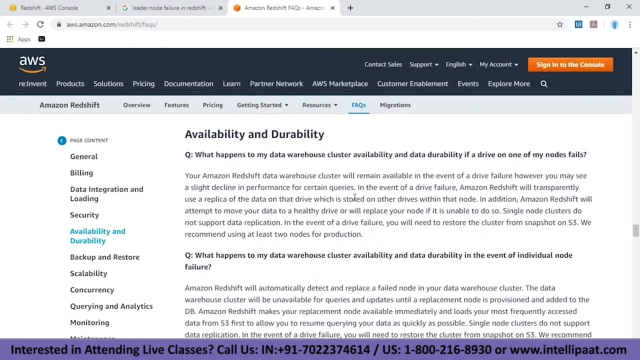 Okay, So now let us just check this. This is more informative than just reading that metadata. So I think over here. viability and durability. So what happens to my data warehouse cluster? availability and data durability if you drive on one of my node fails? 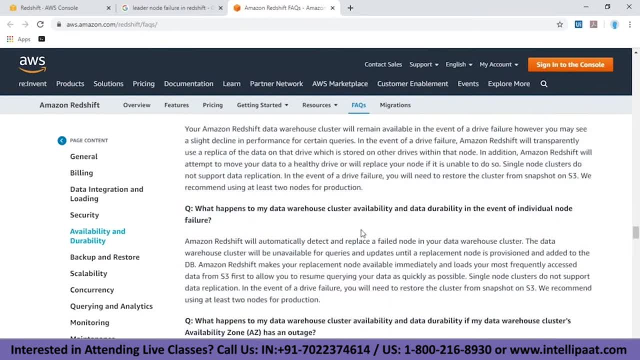 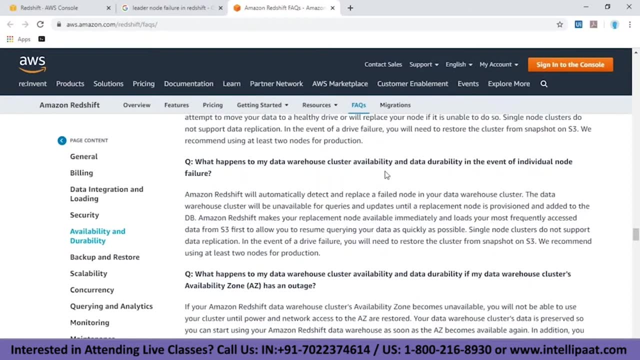 So this does not answer it. Yeah, So this is individual node failure. So individual node failure in the sense Amazon redshift will automatically detect and replace a failed node in your data warehouse cluster. So these this is automatically done if there is a failure in the in. 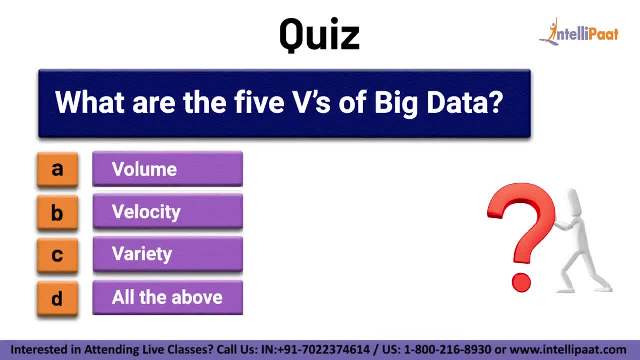 So, for example, we have two nodes. Just a quick info, guys, test your knowledge of big data by answering this question. What are the five V's of big data? A, Volume B, Velocity C, Variety D. All of the above? 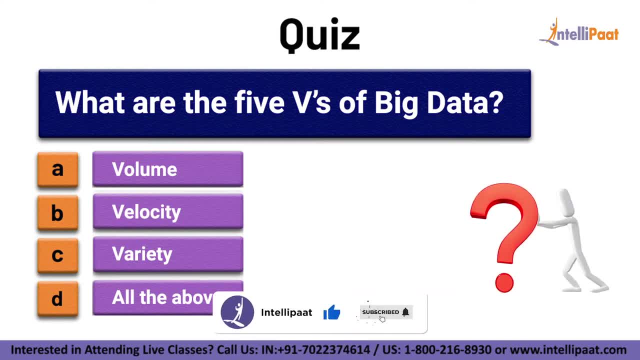 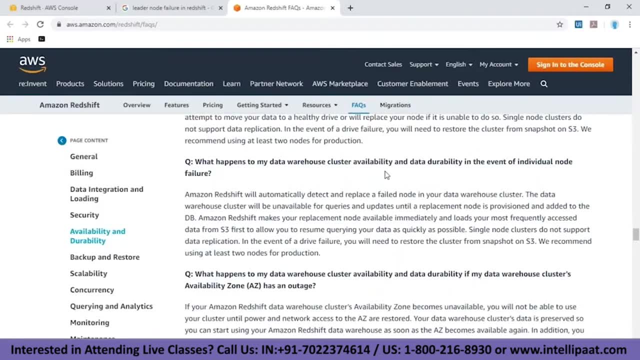 Comment your answer below, In the comment section below. Subscribe to Intellipaat. Know the right answer? Now let's continue with the session. The node has been there is a node failure, So yeah, it will be replaced. The data warehouse cluster will be unavailable for queries. 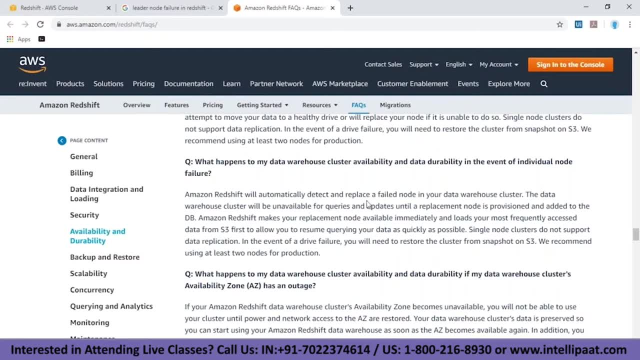 So that particular node. if one node fails, it will be unavailable for queries and updates until a replacement node is provisioned. So your entire warehouse is unavailable. when there is a node failure occurring and is provisioned and then added to the data warehouse, Amazon Richard makes your replacement node available immediately and loads your most frequently accessed data from S3. 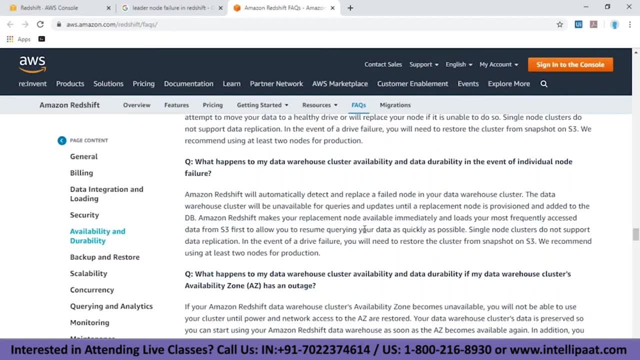 So the most data free data, which is frequently accessed. that data will be taken and first stored and later all the data is loaded back. Single node clusters do not support data replication. in the event of drive failure, You will need to restore the cluster from a snapshot on S3. 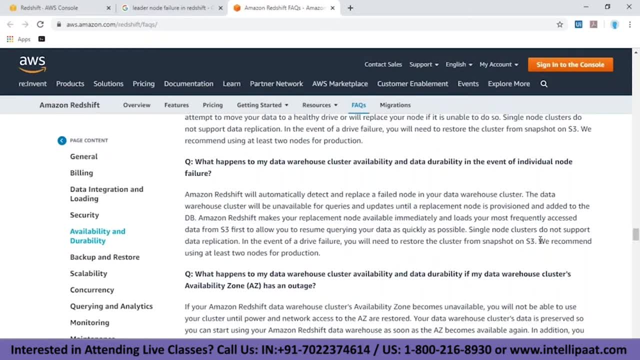 We recommend using at least two nodes for protection. So, yeah, This, at least they are telling us to use two nodes. So if, even so, that I think this is just for one node. So if one node fails, event of individual node failure, then your cluster will not be available. 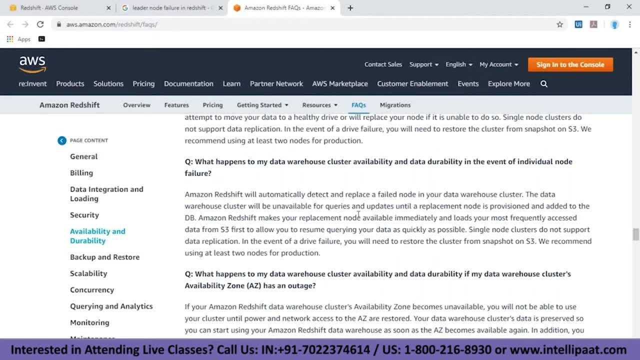 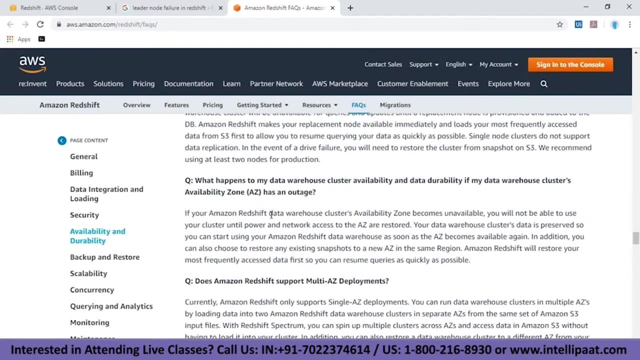 So if you have two nodes, if one node fails, at least that one node will be working, and then this is for the entire availability Zone has an outage. So if your Amazon Richard data warehouse cluster, the entire availability Zone is having an outage. if it is completely unavailable, 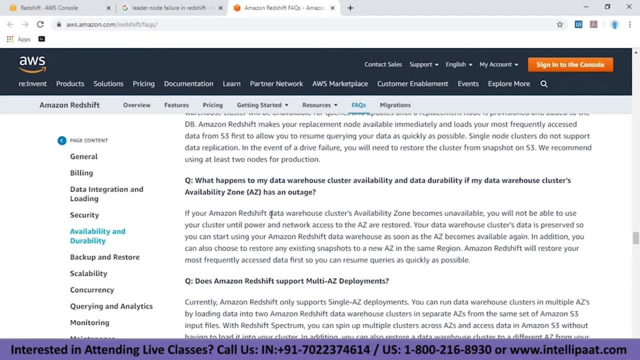 So you will not be able to use your cluster until power The network access is three to restore to that availability Zone. So yeah, your database, data warehouse clusters, data is preserved so that you can use. you can start using your Amazon Richard data warehouse as soon as the availability Zone is available. 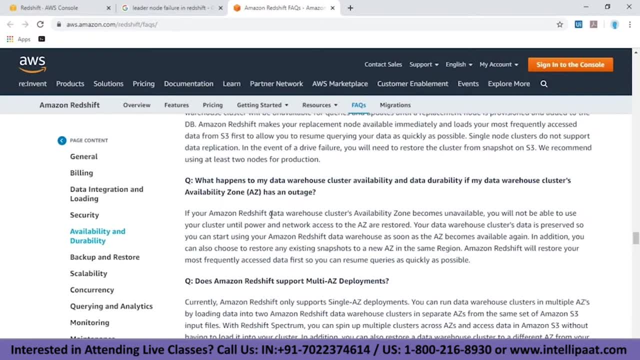 So the data is preserved, The data is not lost. If, when the availability Zone comes back up online, then that data again a new one is created or already the existing cluster is provided, is will be available. So yeah, It is will be available right now. 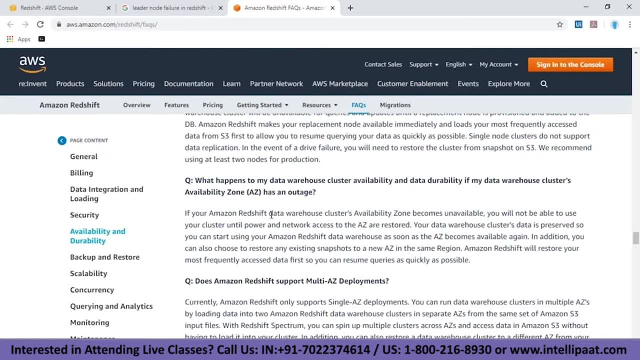 So you can start using it. and, in addition, you can also choose to restore any existing snapshots. Yeah, So if you created any snapshot, you can use that to create one more cluster and Amazon Richard will restore your most frequently access data first, So you can resume queries as quickly as possible. 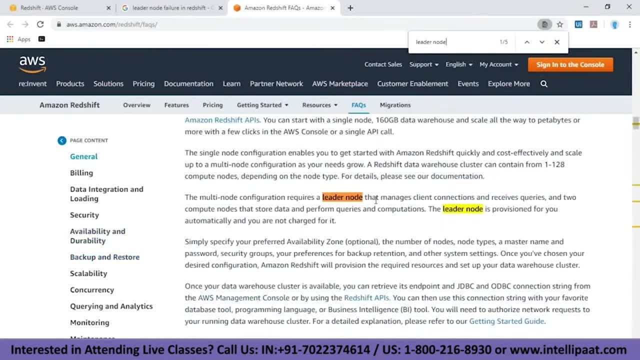 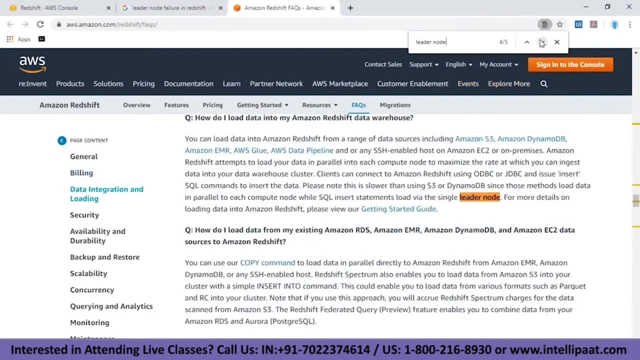 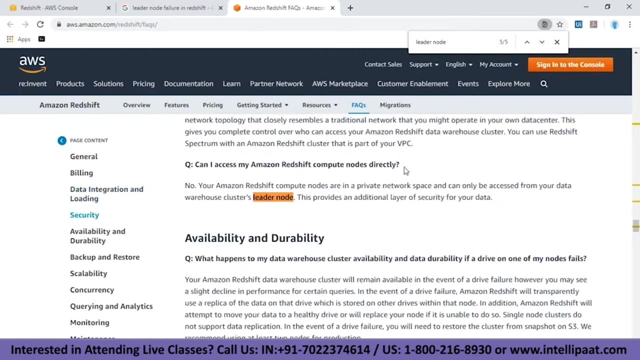 So I think yeah, so they have not provided over here. You will not be charged, only compute nodes will incur charges. It will be built for. okay, How do I load data inside? Okay, We are the single leader node. know where they have provided that. can I access compute nodes directly? 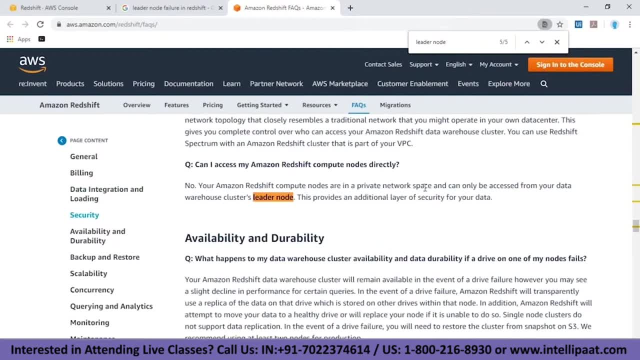 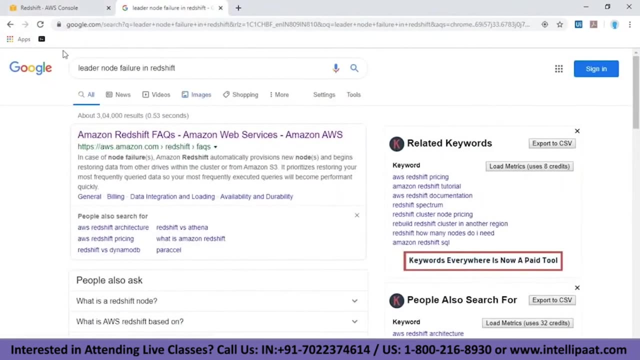 No, your redshift compute nodes are in a private network space and can only be accessed from your data warehouses, clusters, leader node. This provides an additional layer of security. I think there is no other goal. You will have to use leader node. So I think, even if there is a failure, they will provide a new one immediately. 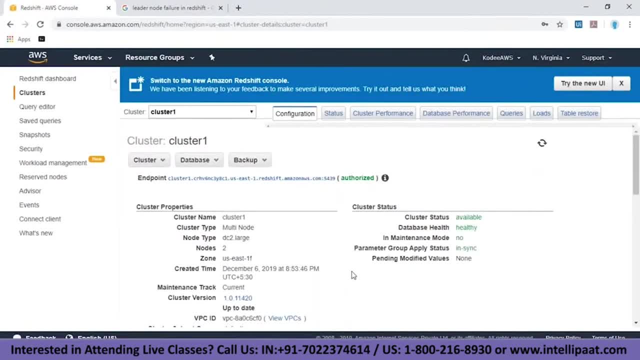 There is no other strategy either. You can have another cluster. So after that like, when there is a, when your cluster, one of the cluster- goes down, you can have another cluster in another region and just use that until this availability zone comes up. So I think there is no part of having a like. there is a leader, node, failure or something. 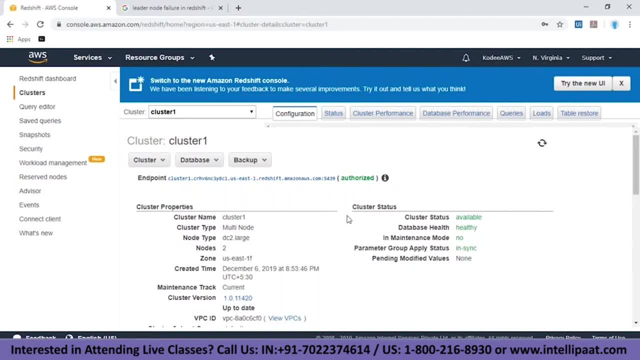 So even if the cluster endpoint is not an available, then I think you'll have to wait until it comes back up. That's the only chance here. But if the node goes down, then if you have two nodes, one node will be working. if, until the other node comes down, this node will be used if you have multiple nodes. 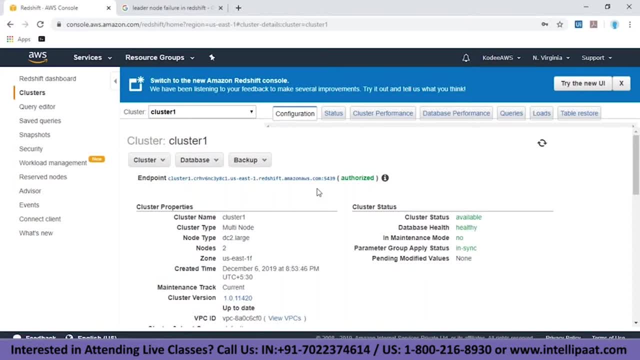 then it's better if you have a single node. if the node goes down, then, yes, your entire cluster will be down. no queries or nothing can be, nothing will be running. any queries coming in will be cancelled. any client connection will be cancelled. So yeah, so that's what if there is a case of leader node failure? 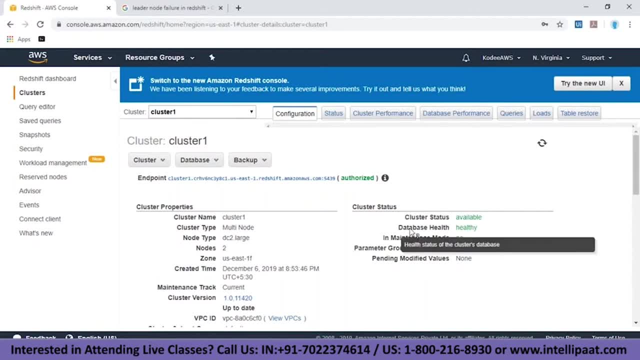 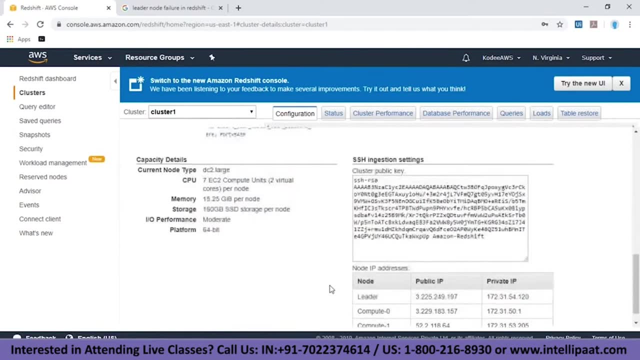 so you, you cannot do anything else until you, You can just wait until it comes back up. That's it. Yeah, So right now we have created a cluster. Okay, so coming back here, Okay, so we have created a cluster, guys. 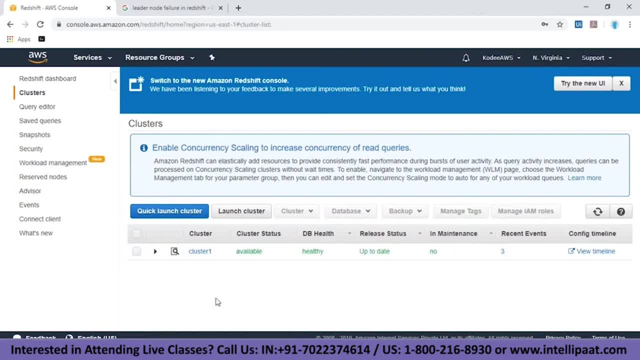 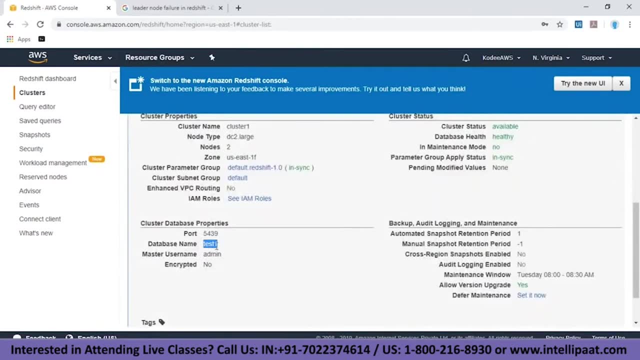 So that's it. It's a. you'll have to provide the information, and that's it. So now we have a database named as test one, So I'll show how to connect this database from your query editor. So now I'll open query. 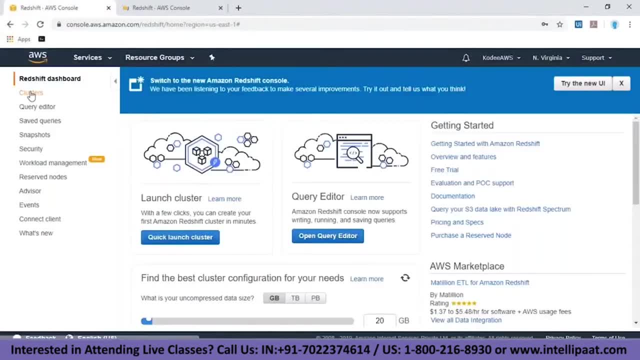 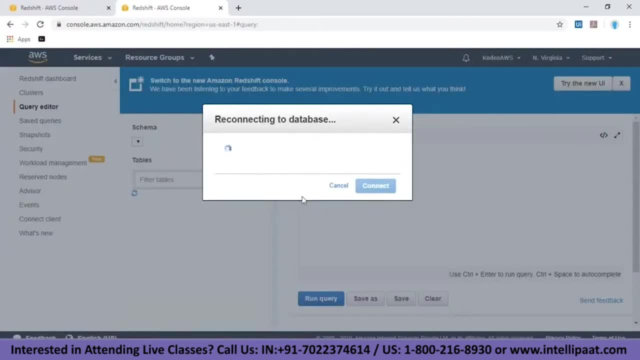 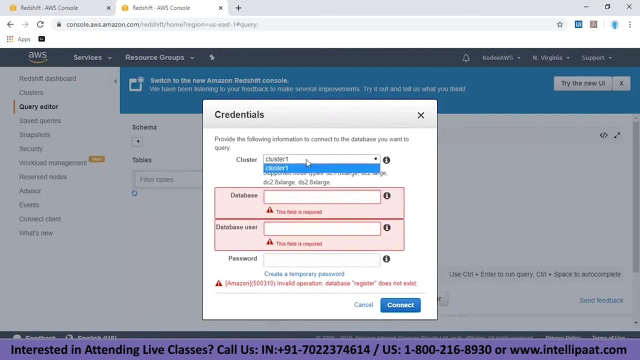 I'll open query editor over here. So when you click on query editor it shows this. So this was with the previous cluster. It's still trying, So now I'll just close this. So cluster one, cluster one, is the cluster name which I have right now. 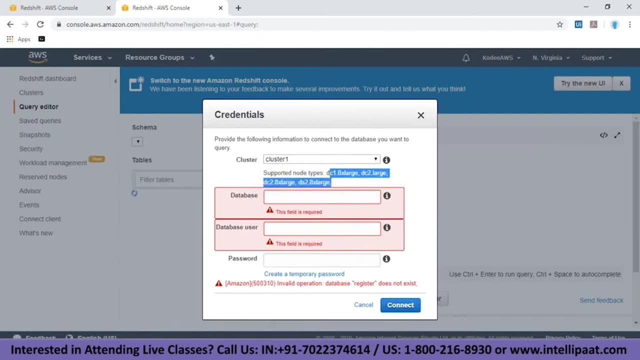 So the supported nodes for query editor are these four: DC 1 dot 8x large. DC 2 dot large. DC 2 dot 8x large. DS 2 dot 8x large. DS 2 dot large is not. you cannot use that particular node type in query editor. 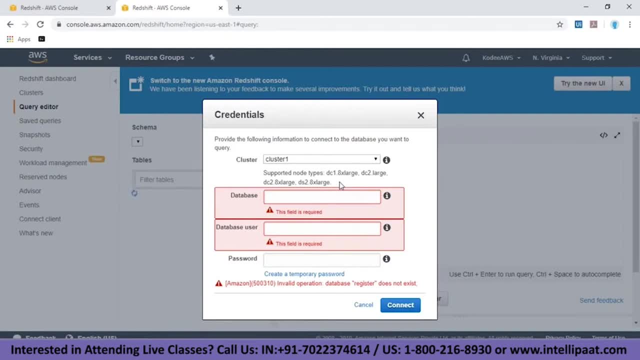 And then you can also. you are, you can also use the RA 3 instead node type. You can also use that. It's not provided here, But as I read the documentation, it was provided there, I should I. it is in the PowerPoint also. 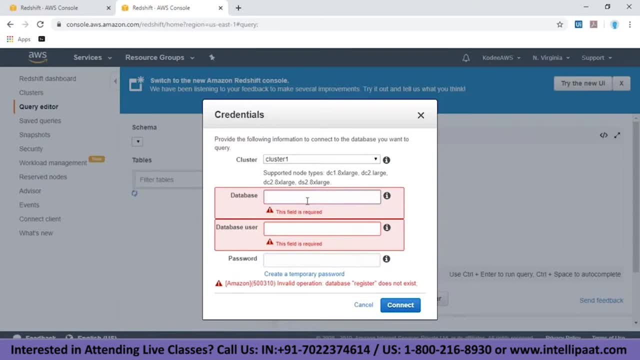 So yeah. so now to log in into this database. It's pretty simple: enter the database name. so you can enter the database name, 8x large. The database name, either dev or test one. So test one dev is already created. test One is the database. 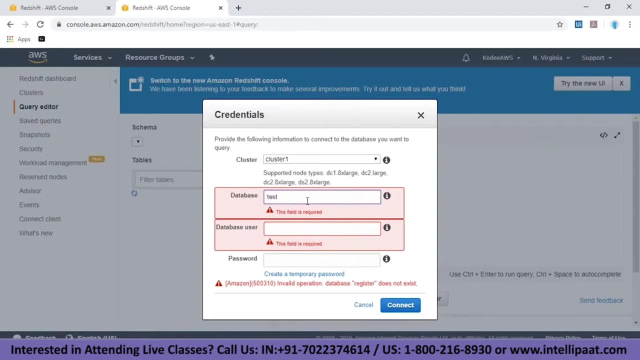 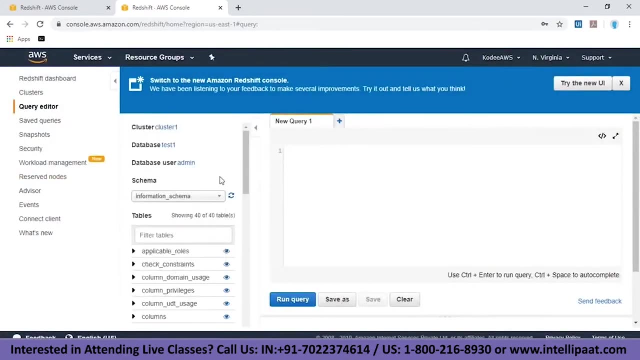 We put created while creating the cluster. So now hit test one: provide the database name, database username. I have only admin and then password and connect. So now it is connected. That's it. So the year you can see the viable databases or Yep. 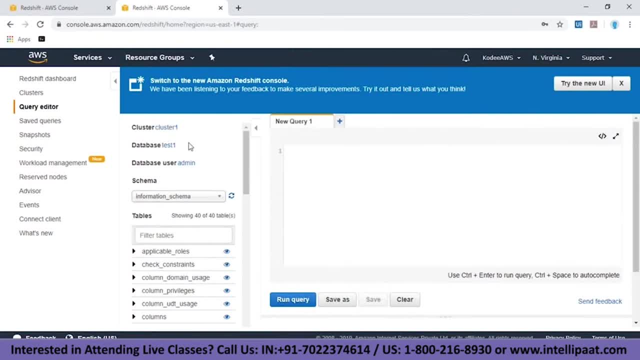 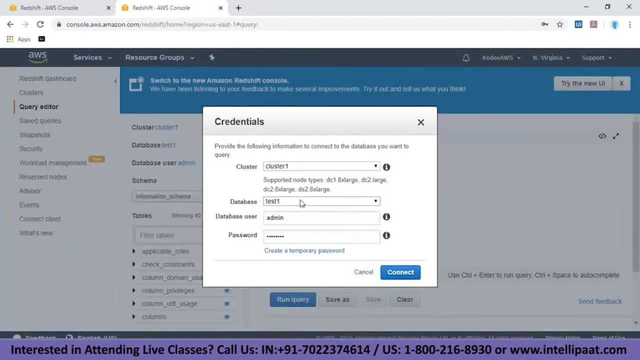 So this is the console, This is how it looks. provides the cluster name. It provides the database name. So here, Yeah. So if you click on the database, if you click on the database name, you will be shown the available databases. 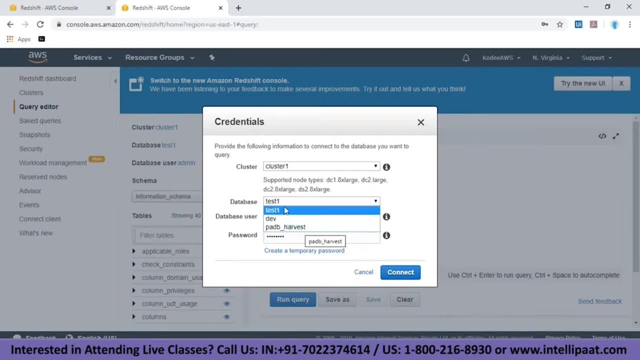 So you have dev here, You have another database- I don't know What is this- So you have these three databases here right now and you can shift. if you click dev and if you hit connect, you will be connected with dev and you can do that accordingly. 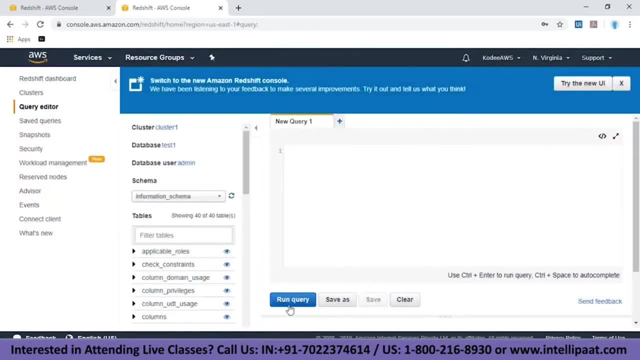 So now I'll close. So here you can type in a query And Run that query. So let's create a database here. create database, say, dev 2, and run the query. So query completed in point eight six one seconds. statement completed successfully. a statement completed. 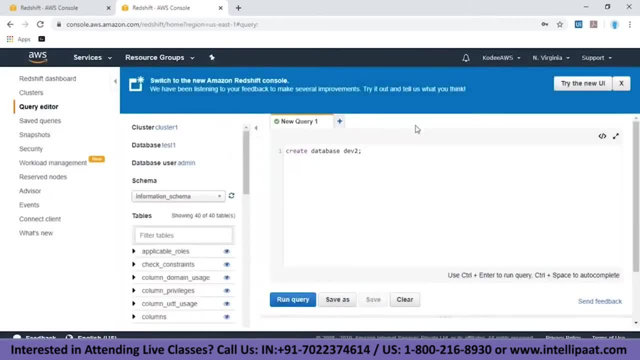 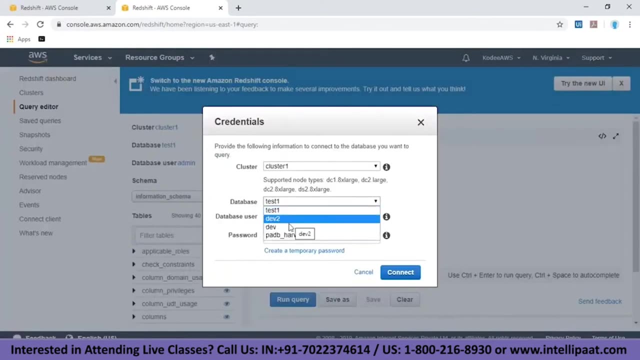 Yeah, So right now. So I think I'll have to wait for some time or So. we've created the database dev 2, but why is it not available? Let me check once again. Yeah, So now it is available. dev 2. we've created a database. 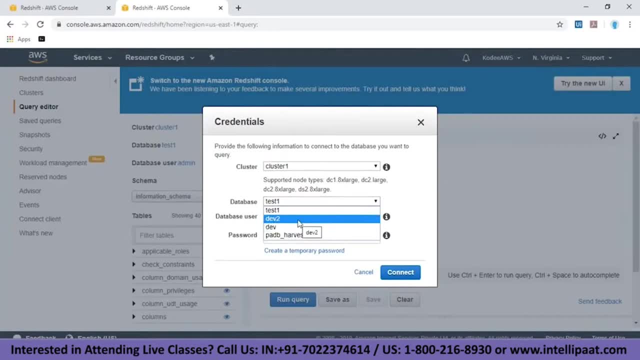 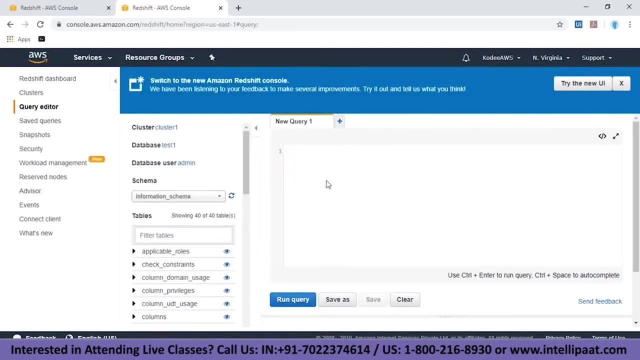 So this is how it's this, how simple it is used query editor over here. So that's it. So now, guys. So now let us do a simple demo, That is, I'll create a role, I'll attach it to this redshift cluster. 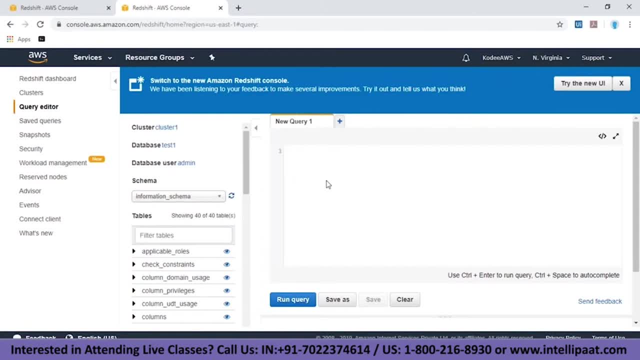 So what that role basically does it does is it provides the permissions to access S3 for this particular database, For this particular redshift redshift cluster. So once I provide this, from this redshift cluster we can query data which is stored in S3.. 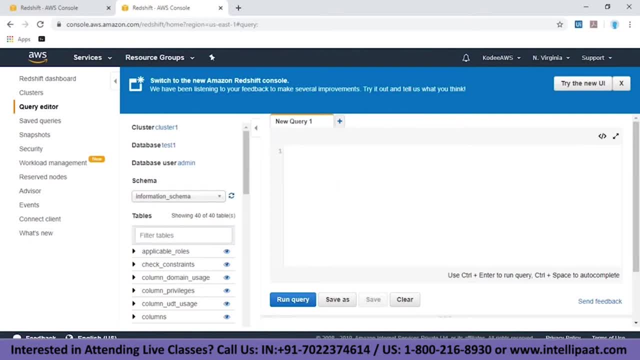 So I've already stored some data in S3 and I'll also show from where to get that sample data. There is a tutorial I followed which is AWS. again, I just follow AWS official white papers and documentations. So from there you can get the sample data and you can upload it to an S3 packet from there. 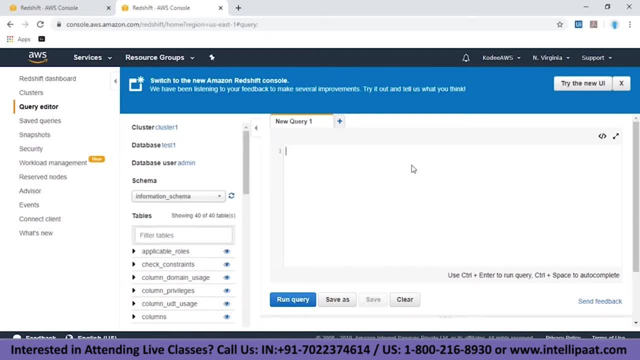 You can. you can provide the I am role to this particular redshift cluster. after providing it, You can just query it and create tables here. after creating tables, load data into this database. after loading data, You can query the data. So yeah, so let us start with that. 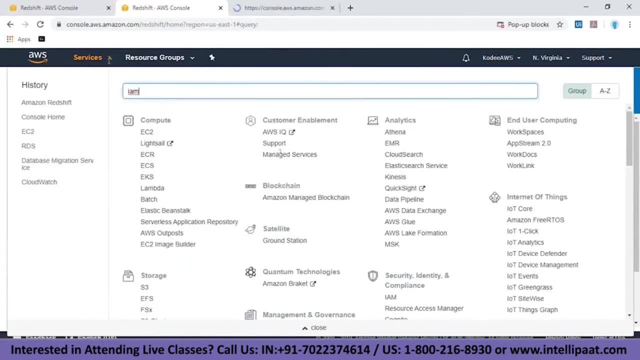 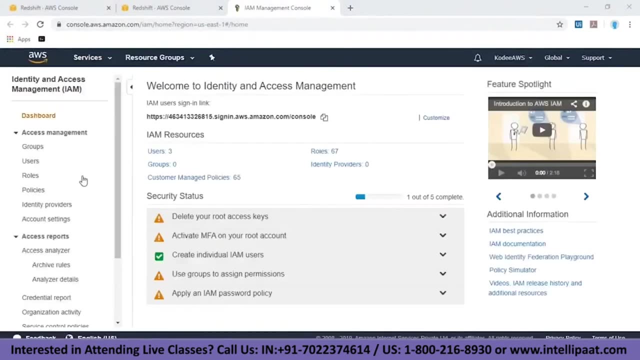 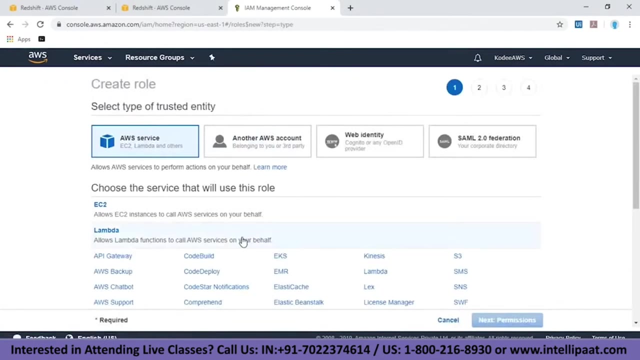 So for that, first I'll have to you open I am. So first I'll have to create a role. as I told you, I'll have to create a role. So role, create, role, or the service which I have to provide the permissions to is redshift. 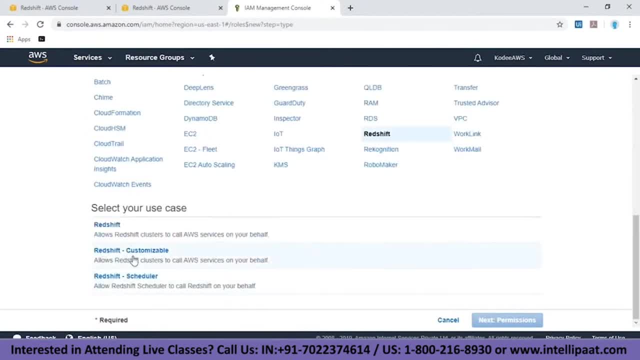 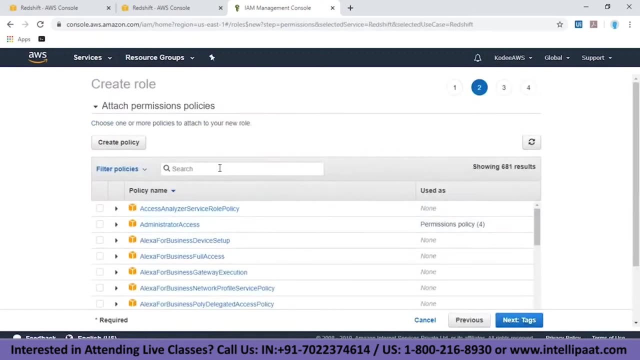 I'll have to choose redshift. redshift is over here, So I'll be choosing redshift, customizable. There is one thing called scheduler, and this is not for clusters. This is for clusters, So I'll just choose this. and then, here, you'll have to provide the permissions for redshift accessing S3.. 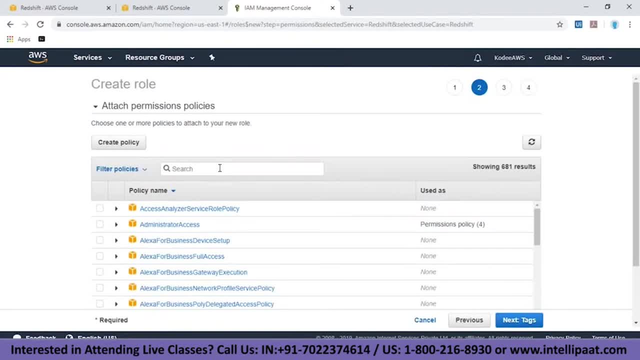 So redshift does not need any other access, It just needs to access to read objects inside S3.. So let's see, Yeah, so here is three reader. So there is this. that is Amazon S3 read only access. So this will allow the redshift cluster to only read the data from S3. 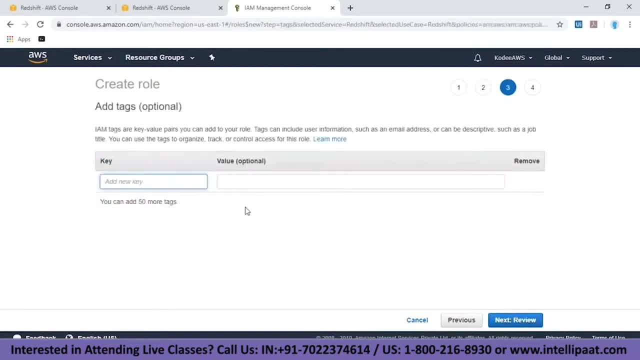 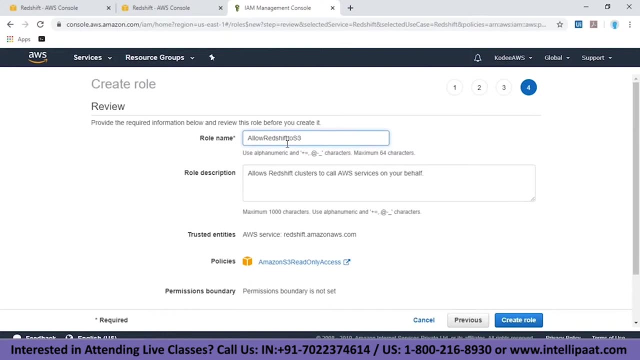 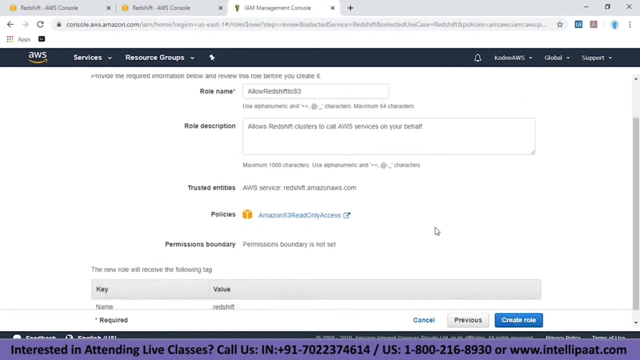 So I'll just click here: next tags. If you want, you can add a tag. Let's say name redshift. then review: provide a name: Hello redshift to S3.. And yeah, so this allows redshift clusters to call AWS services on your behalf and then create role. 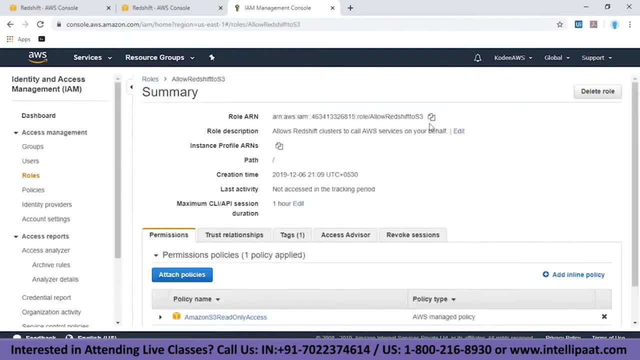 So the role? Yeah, so the role is created, So I'll just copy this: Vini, We will need this air and ahead in this demo, So I'll just copy this. So this is one. will just open another. save it here. 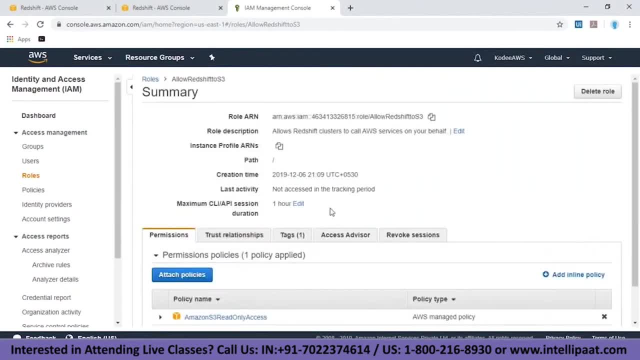 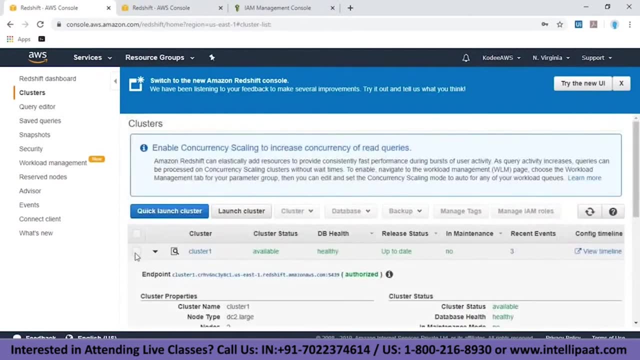 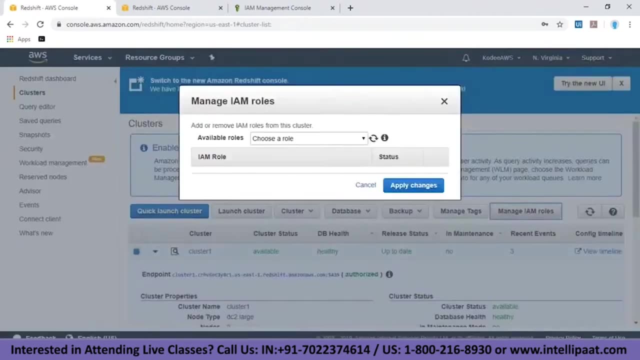 Okay, So now we've created this, so we are going to attach this role to our redshift cluster, So I'll go to my cluster To. I think I can more manage here itself. manager am roles. choose a role. This is the role. 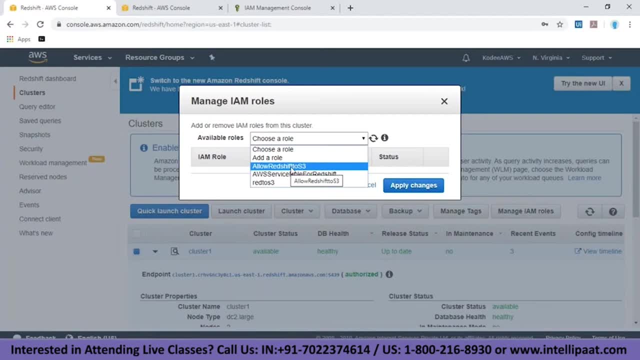 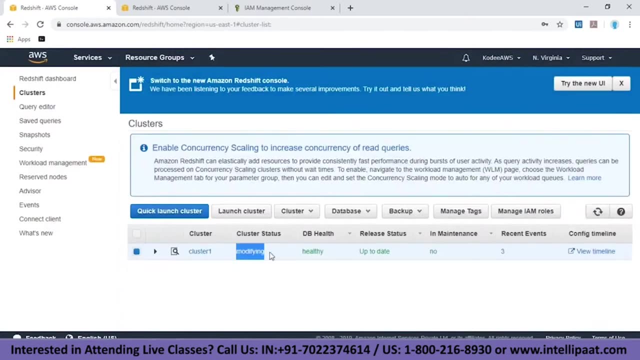 I created right now, That is, a lower redshift to S3. click on it and then apply changes. Yeah, so now it's modifying, So we have attached I am role to our cluster, So that part is done. So the next part, because we are going to lower taking data from S3.. 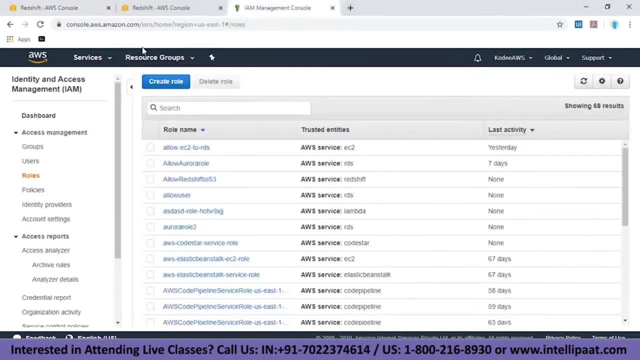 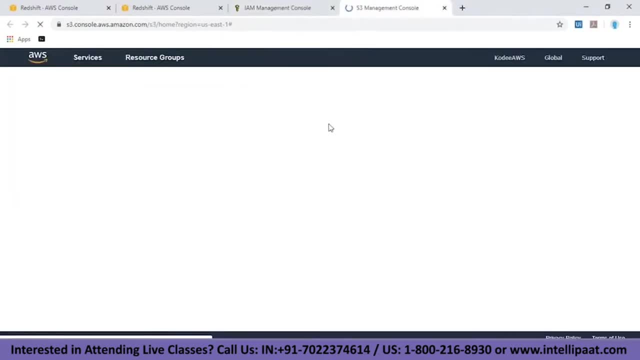 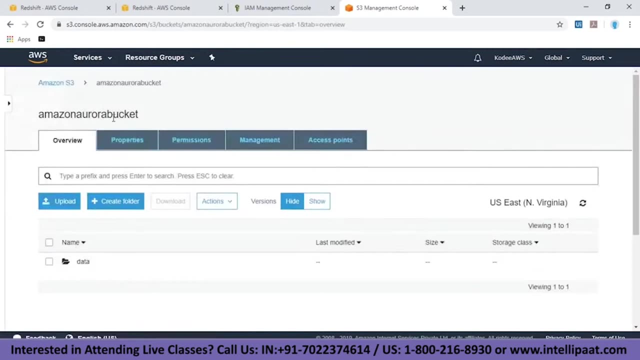 So now data should be available in S3.. So I'll open the S3 console. So I've already uploaded the files inside S3.. I'll show which bucket. Yeah, so it is Amazon Aurora bucket. the bucket visit created long back and I've created a folder inside that data. 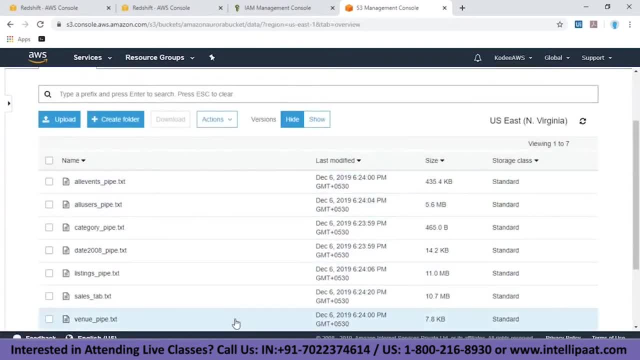 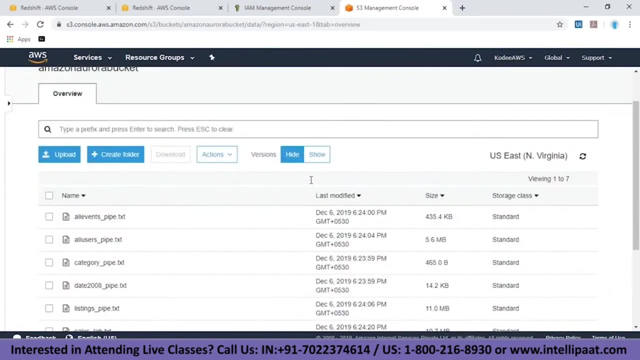 and inside that all the text files are available. So those text files, I have the zip file of that and I'll also show which documentation to go for, like which documentation you can go through and get the origin. You can get the load, this particular files, the zip file. 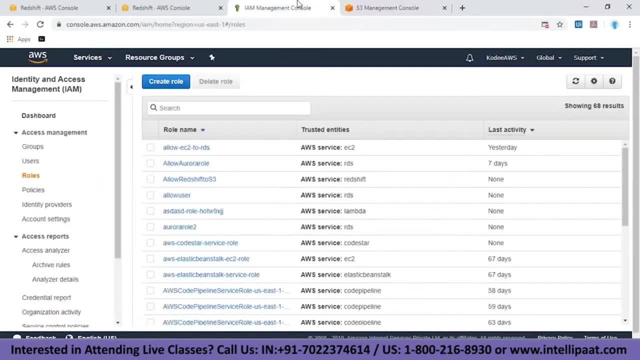 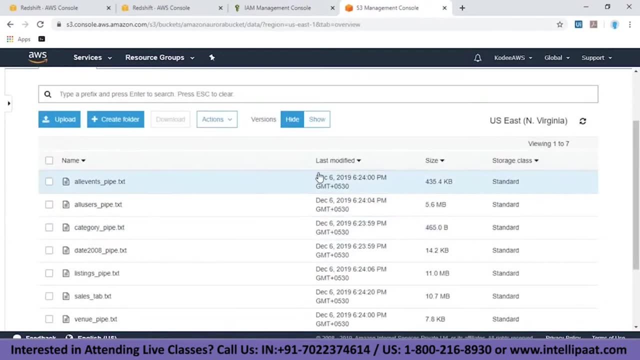 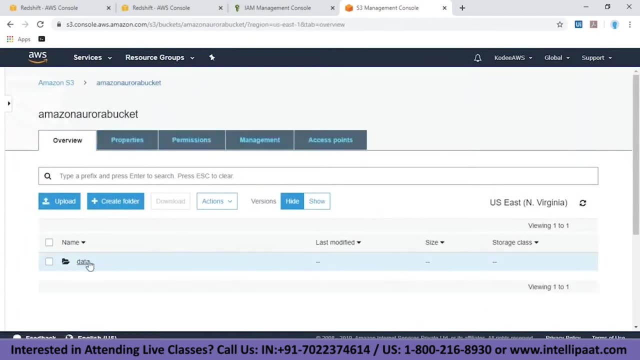 and also from where you can get the queries. So, yeah, so right now we have attached it to the cluster. Also, We have the data inside our S3 database, So it is over here. Yeah, So we created a folder, uploaded the data into it. 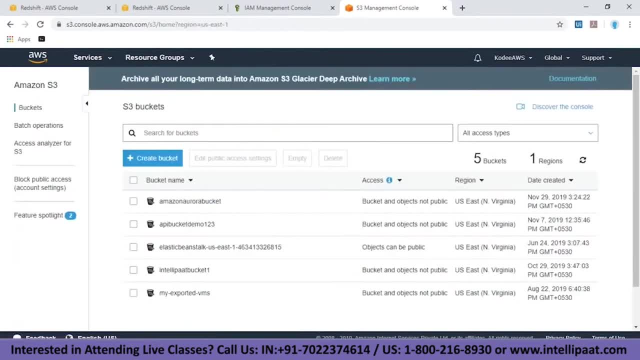 So right now my S3 is set, data is ready. Now I just have to run the queries accordingly to create tables. after creating tables, I'll have to load that data inside those tables. That will be my second part, after loading data inside that table. 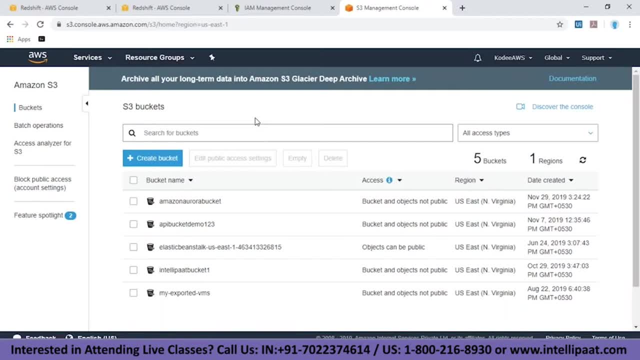 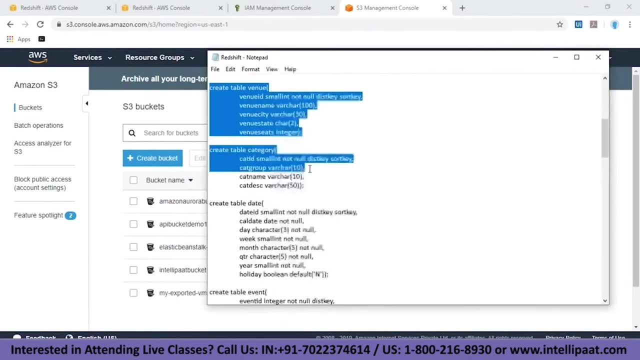 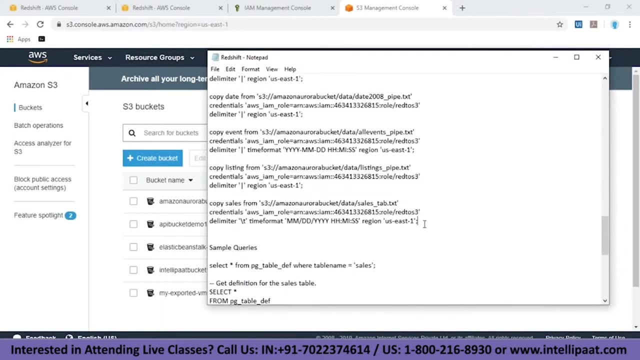 After that I'll have to query, start querying. So right now, let's just show that. so first I'll be creating these tables, After creating these tables, I'll be copying. So these are some more queries. So you would have taught why I copied the ARN. 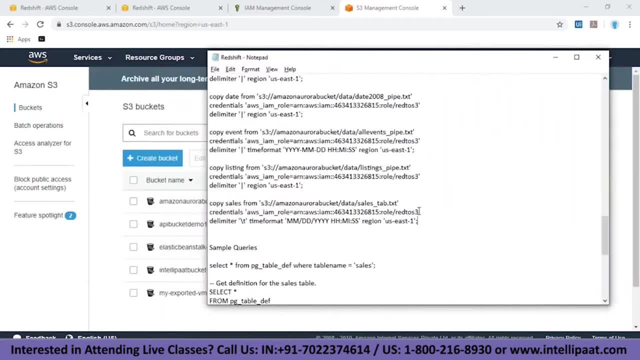 So basically I'll have to copy this ARN and paste it here So this will show. So basically, the query editor does not have access, So for that we'll have to provide this so that the S3 bucket knows that. so this particular IAM role. 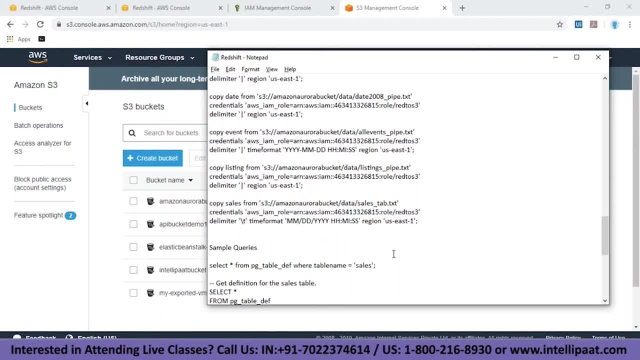 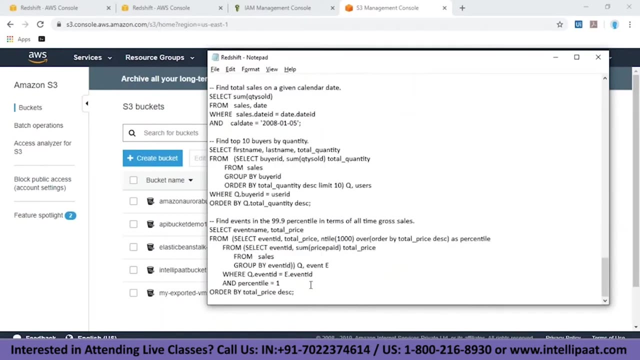 So basically, it allows the redshift cluster to access the data from S3. So while providing this ARN, the S3 bucket will automatically understand we can provide the data to it. So this is that. I also paste these in the end, and then these are some sample queries. which was available. 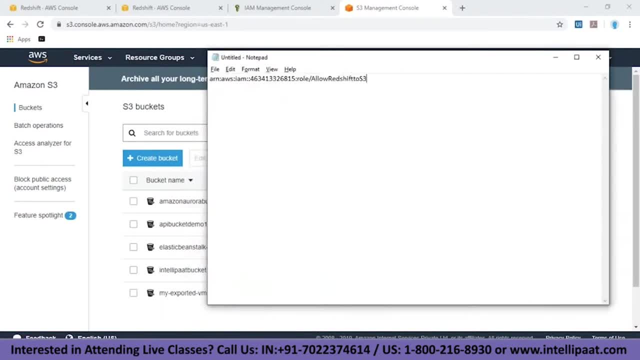 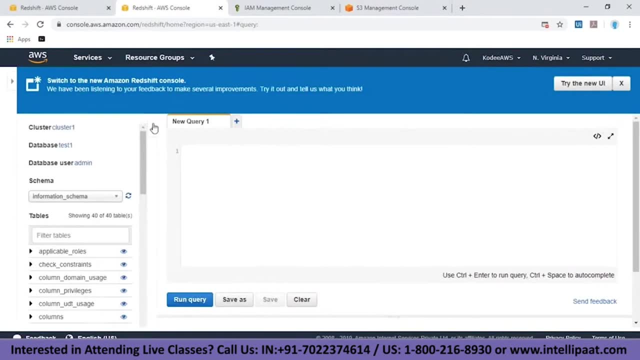 So yeah, so done. So now let us start off with this process. So first I'll go to my query editor and then I'll just do this and do this. Yeah, So now I have my query editor and here you can see the query results. 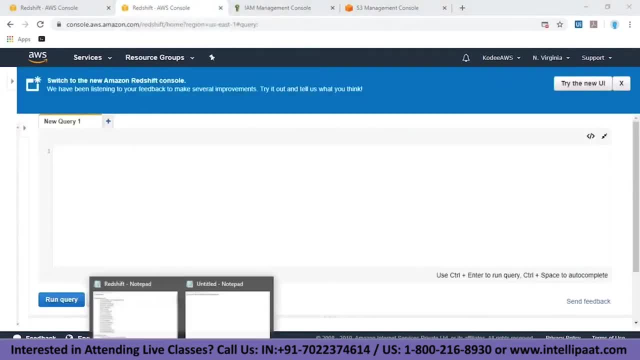 So now, Yeah, So now, first we'll have to create tables. So first I'll create this table. Run query, So completed, and point eight seconds, So done. I've created one table and now I'll load the data for that particular table. 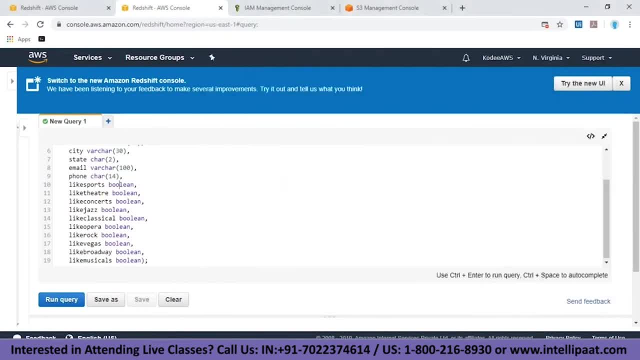 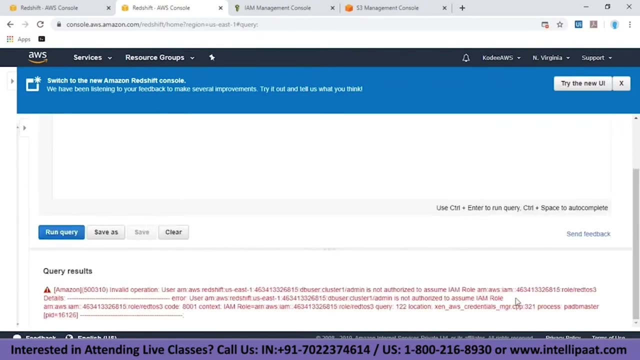 So now I'll just copy this. I can just paste it in this query And hit run, or I can create a new one and hit run. So I'll just run here. What is this? Oh, sorry, I did not change the role. 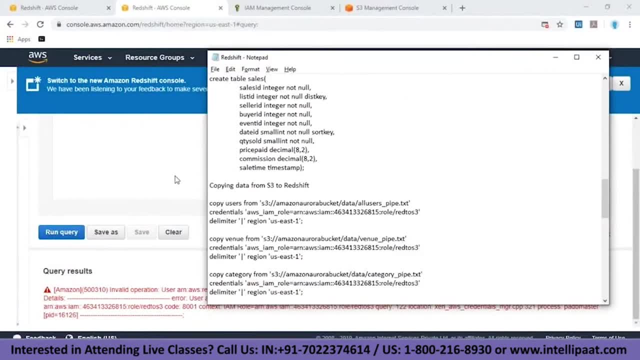 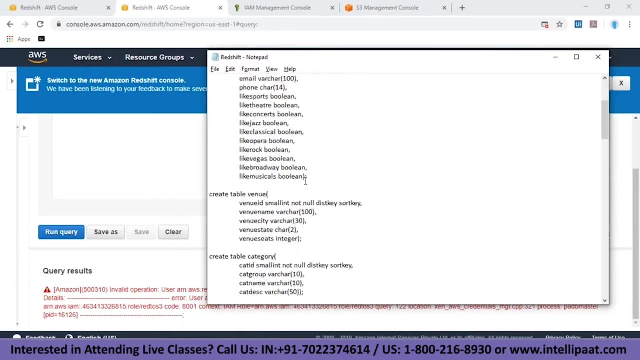 What is what's the copy user? So these are some for query editors. These are the commands for copying users In the sense: Oh, the table name, Yeah, Okay, Okay, Got it. Yeah, Confused with the user. 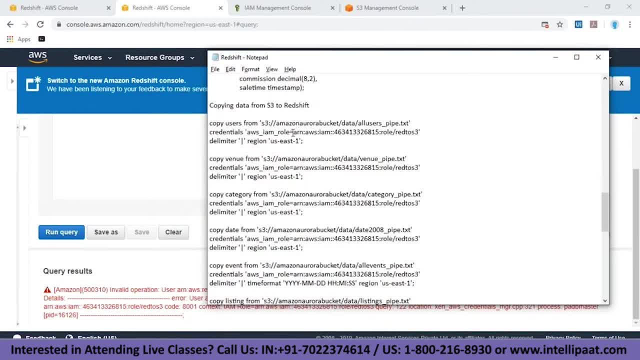 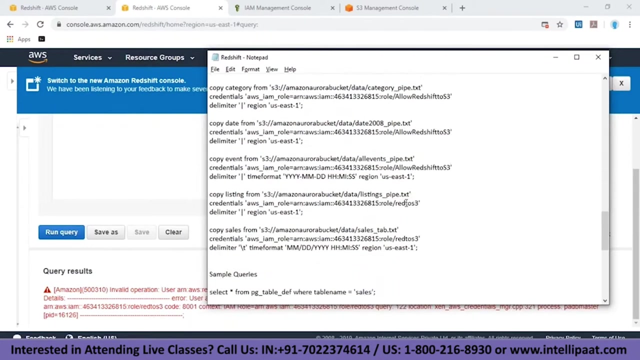 Okay, Okay. So now I forgot to change my ARN, That is, Amazon resource number of my IAM role, which I just attached to my rich of cluster, So I'll just paste it all over My queries. Yeah, So I that's done. 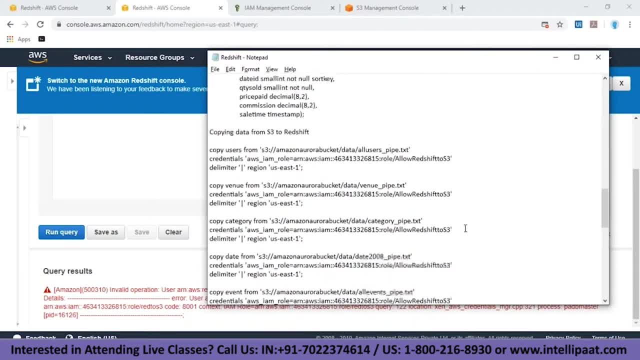 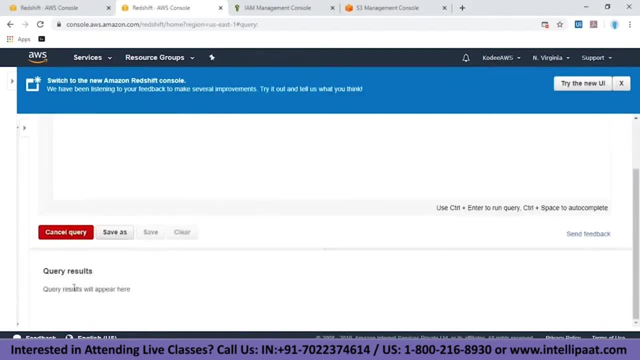 Okay, So now I think it will work. So yeah, it's, the query has run successfully. So now we can just use this one query to do all the operations, or we can open another query and do a different one. So now I will just create a new one. 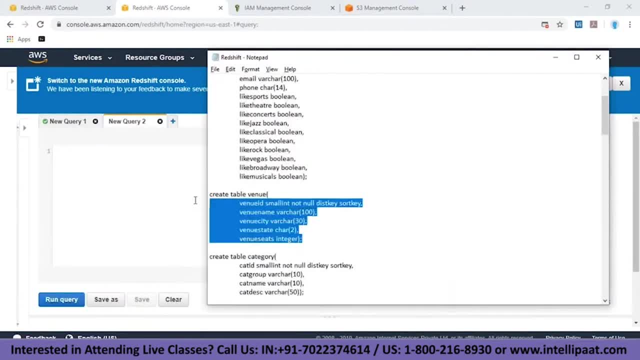 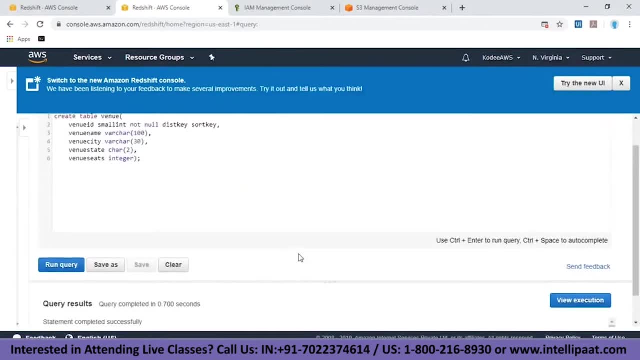 So this is my, So I will just put the new one. Do so we can draw. Do this so as also as a best practice. in the documentation They told: run one query in one query page. So one complete query in one query page. that I don't know why. 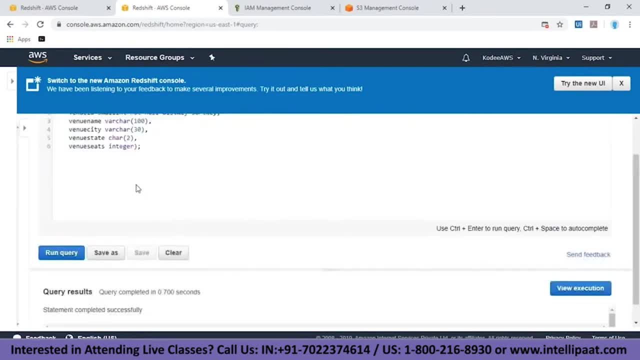 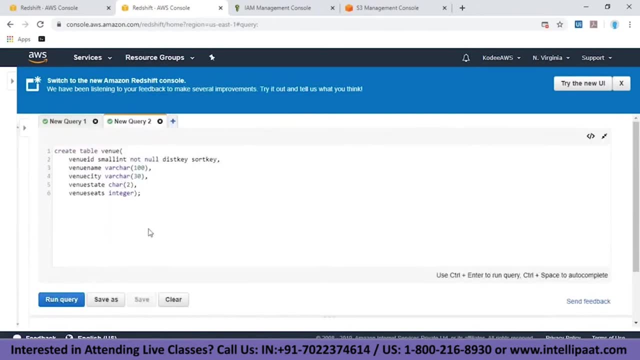 But that is what they have told. Sometimes when you run multiple queries, there are some errors occurring. here It's showing some some kind of intonation errors or something. So that's what it was showing here. So run one query at a time, then what you can run a query in the same query. 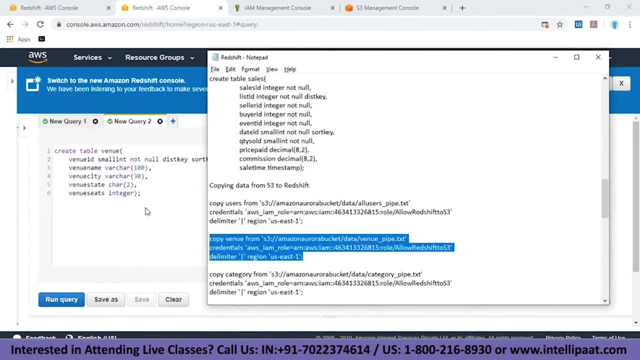 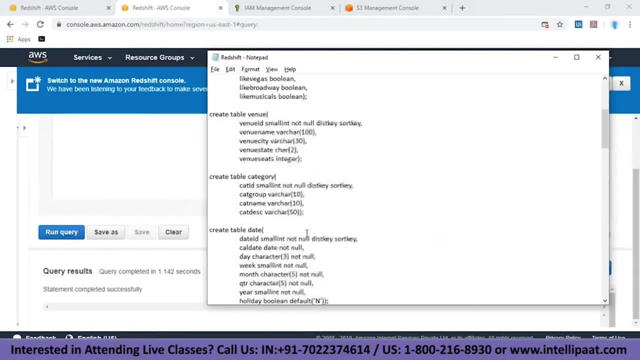 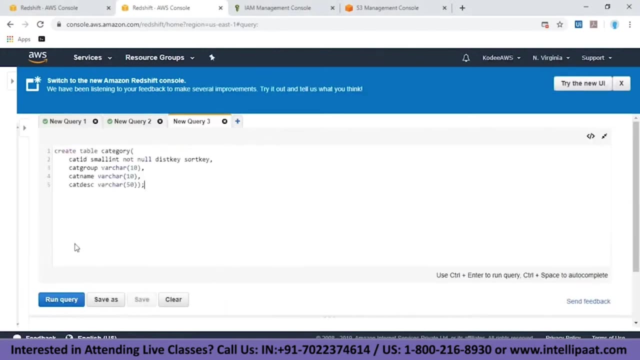 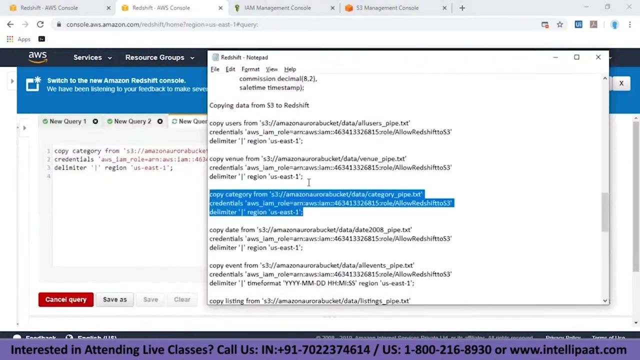 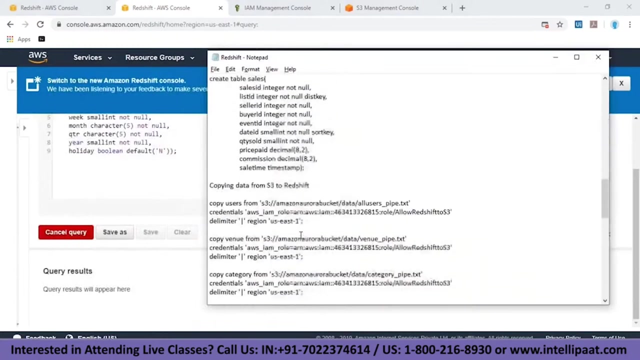 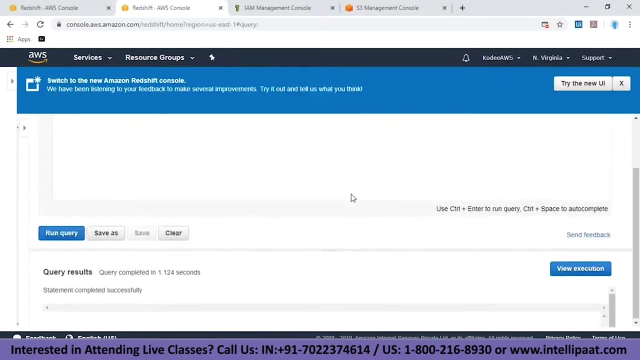 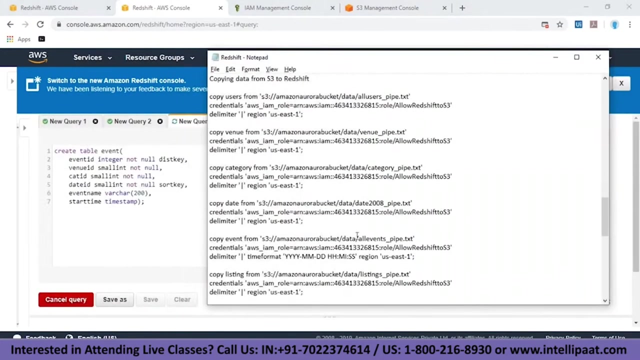 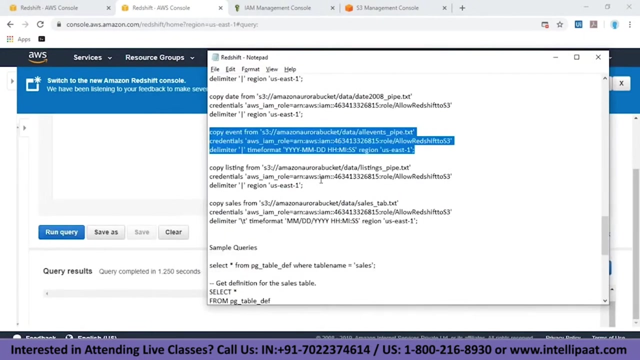 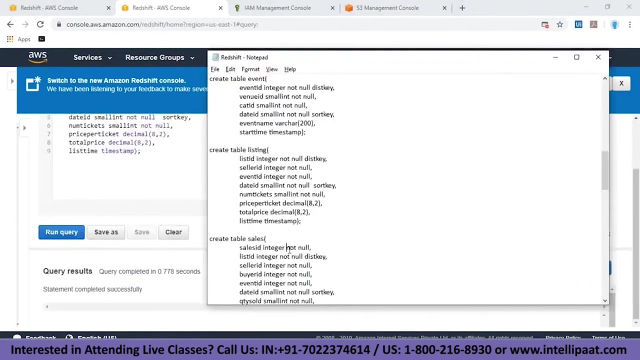 Dashboard multiple times. So I'll just Upload the content of this Done, then category. So just wait, I'll just do finish this off. Discrete multiple queries based run And Then date: Successful Done, Event Done. then there are two more listing And then sales just create one more. 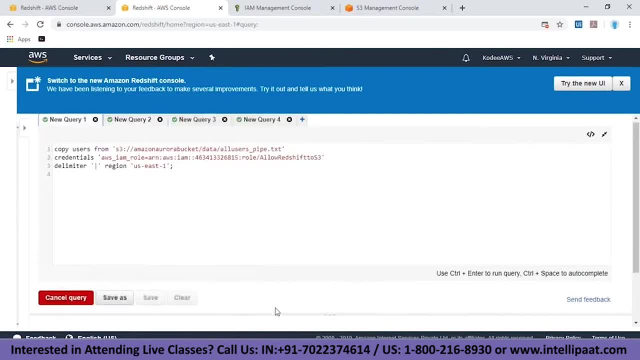 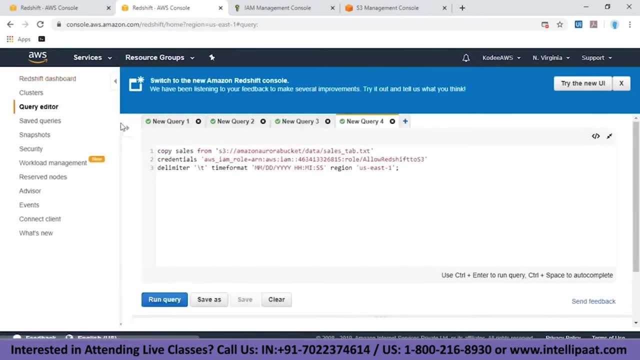 So every time you open, it shows the results. It's taking some time to show. Okay, so we've uploaded all the content inside our tables, but one more thing is You'll not be able to view that content here. That is the only problem. It is just to query. 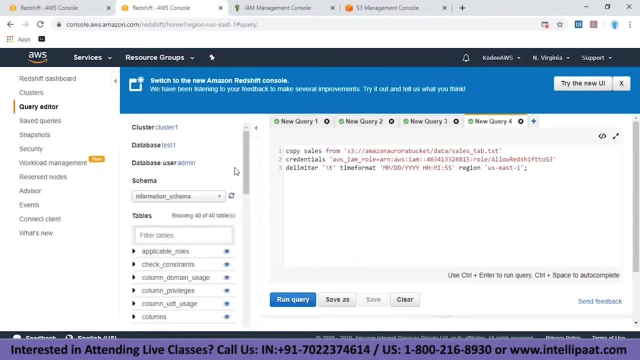 In query editor you will not be able to view the data you stored, So for that you will have to use an SQL client. but you will be able to run queries and then see the data. So yeah, that you can do. But there is no option for viewing all the tables available. 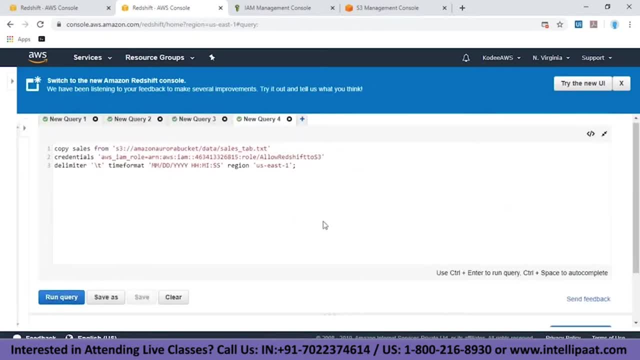 Like that. so you will just have to query all of them and see here: Yeah, So if it is a client or a workbench or something like that, you have everything. you have your own GUI Which you can use to see the tables available or the databases available and everything but in the query editor. 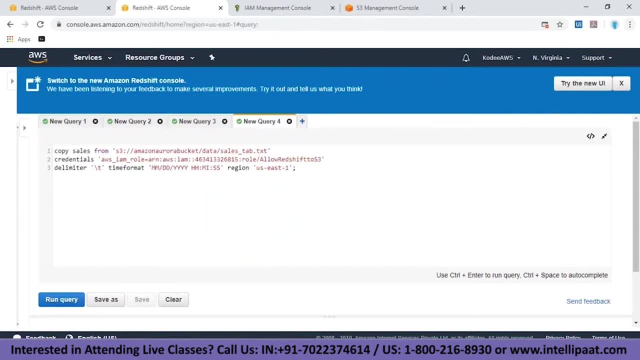 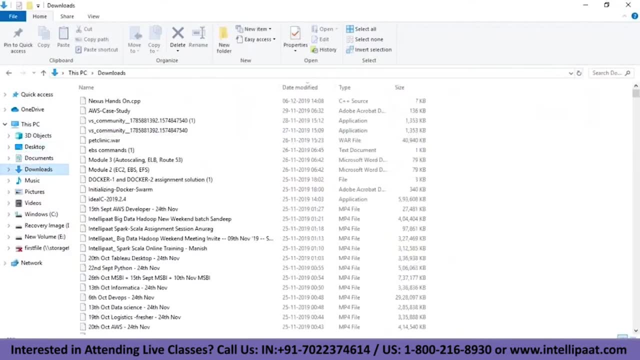 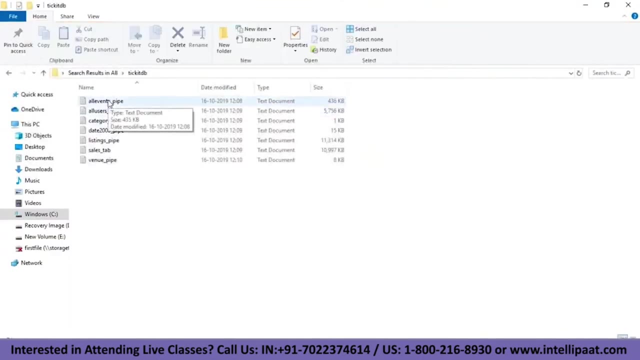 You can only query. that's the only option here. So now we have uploaded the content, So I'll also show What was in the content. So it was a Thing. the name of it was ticket. Yeah, So these are the files. they're all text file, so here you can see. 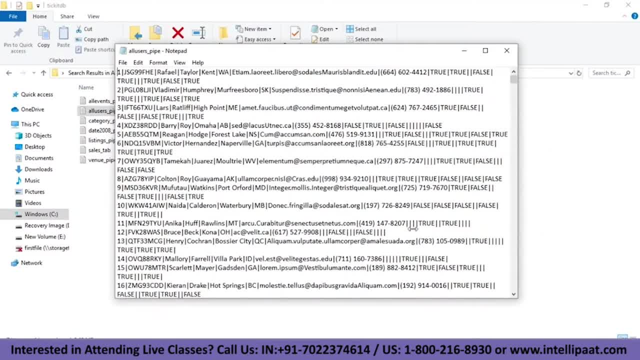 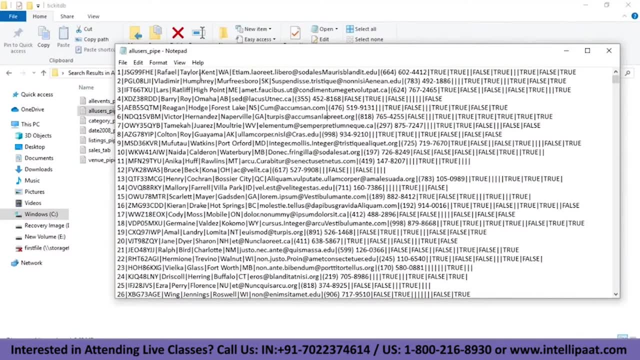 Just to say it's Loading up. So this is how the continuous available so you can see the number code or something. Whatever Is that name, middle name, Last name, so whatever order, and then The email, the number. some questions: true, true, false, true, true, false. shows all right. 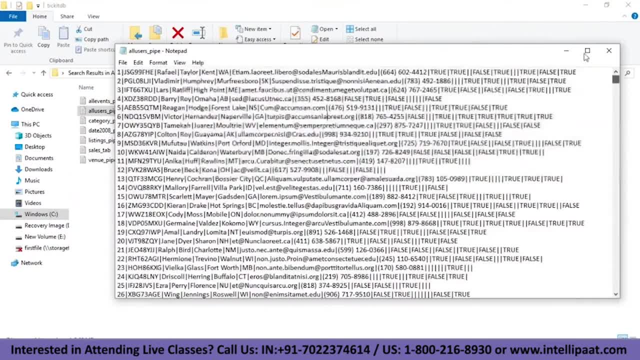 Okay, so, so you can see, there's a lot of data available. So these many queries- sorry, this money- are rows, So basically It will not be uploaded as single rows. So if it is uploaded as single rows every time, it will take a lot of time. 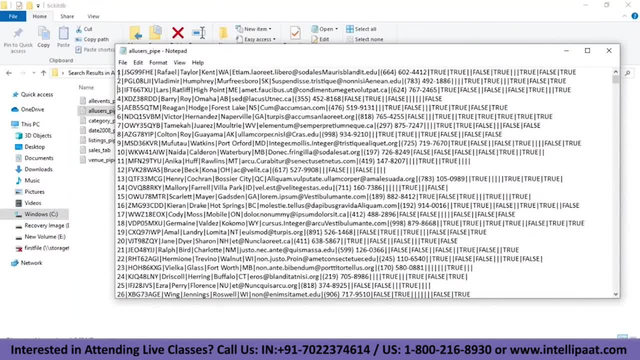 So what they do is they consider this entire Column as one row, one, one, one one. so they do that and they upload it. So, basically, it happens in the redshift and it happens transparently, which that's what you've promises us. They use columnar data storage, So I just wanted to show this. 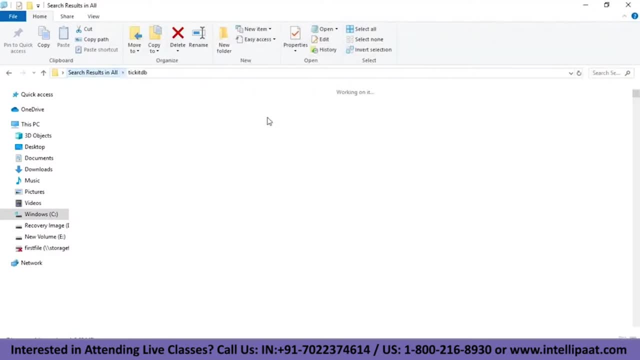 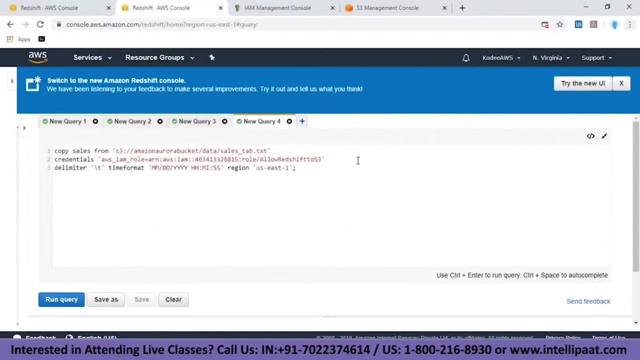 I also I'll give the link for downloading this sample data which you can use for practicing. Yeah, so now we have uploaded all the content. We have loaded the content from s3 into Redshift, so now we'll have. we'll just do some querying and practice it. 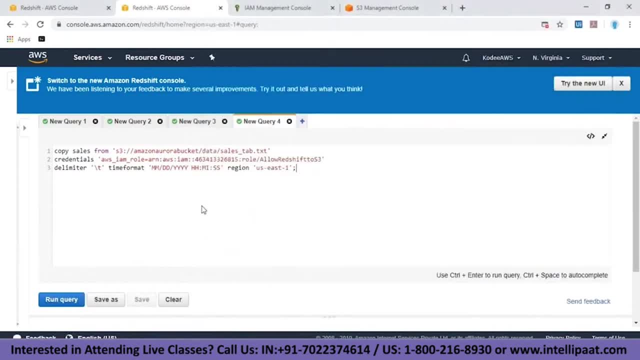 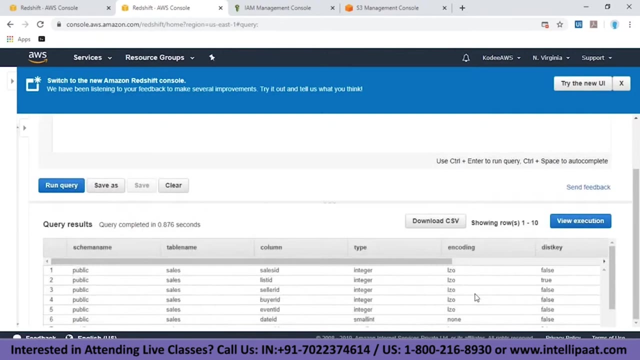 So sample queries. so this one is to get the Table definition, I think table definition of table name sales. Just push it up, Yeah. so table dimension definition over here, So you can see the query results over here and also you can download the CSV file from here and 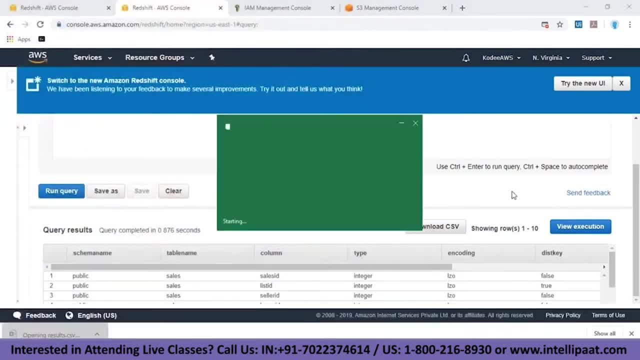 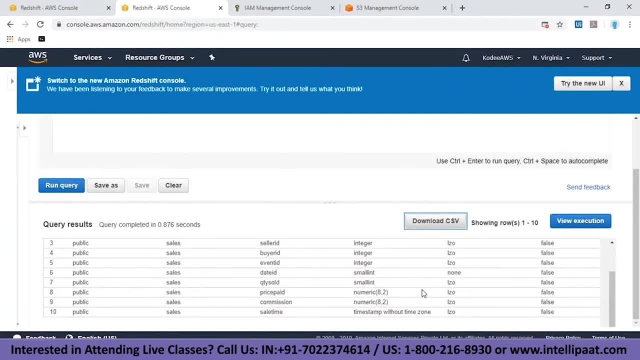 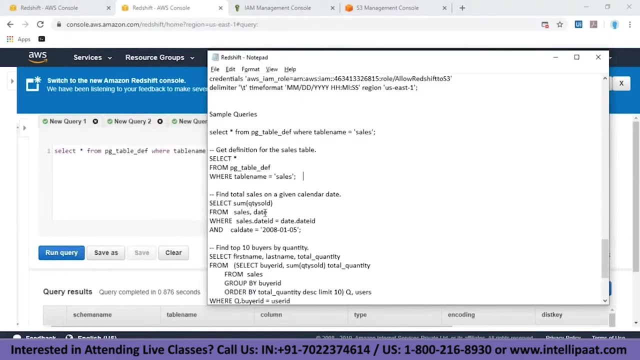 Just save and you can download it and you can also view the results here. Okay, so there is some problem with this. so you can also download the CSV file and view it, and that's it. and then another query: Select some this from sales date, where sales dot date ID is equal to date dot date ID. So they are just 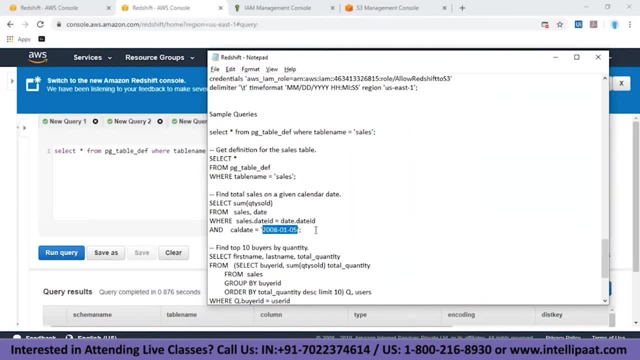 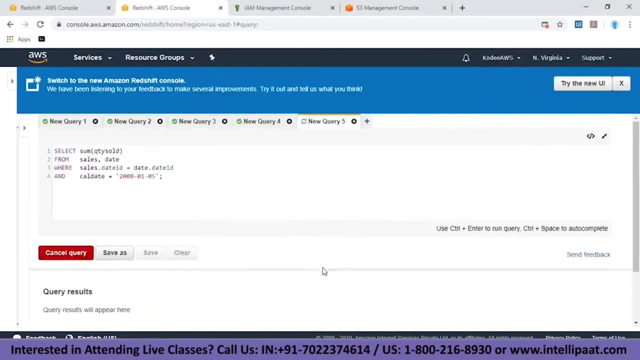 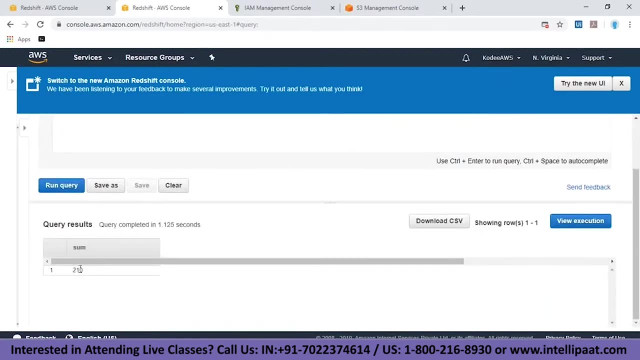 Doing that and calculating on the date. on this date They are calculating the sum of quantity sold. So now, When I run this query, I should get a number of sum. So yes, so we've got that number. so that is the only result we get, because that is the only result we needed. 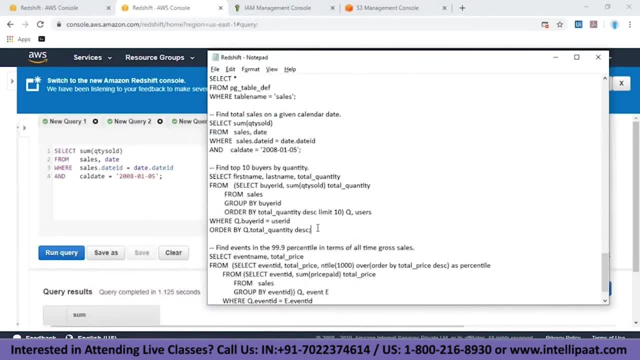 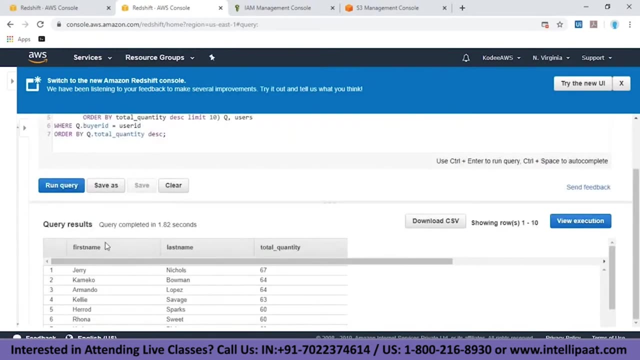 so this is one query, and then and Then there is this. so here they've provided the limit as 10.. Okay, so, So we'll get 10 rows of Output, so showing rows 1 to 10, so you can see first name, last name, total quantity. 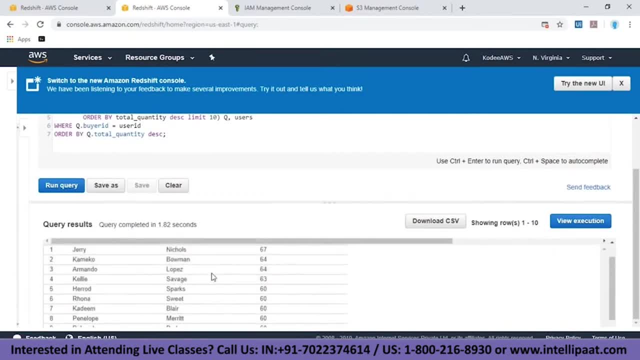 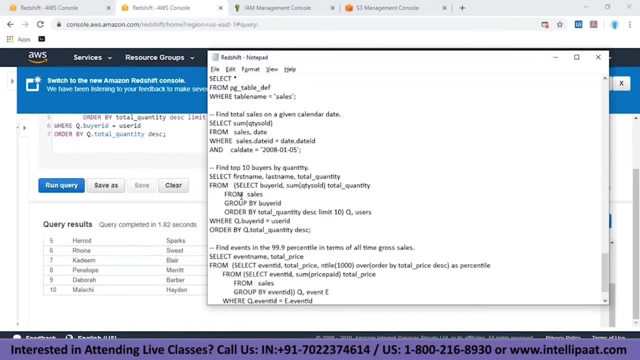 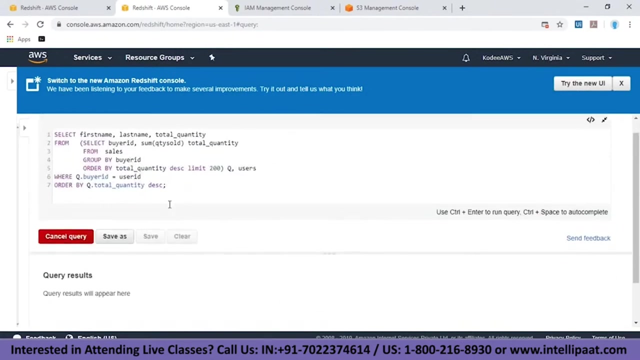 they have provided the name and Last name and the total quantity. So that's what mentioned here. select buyer ID: Some quantity sold. total quantity from sales group by buyer ID. order by total quantity limit. So we'll just change this limit to 200. I could have just changed here. 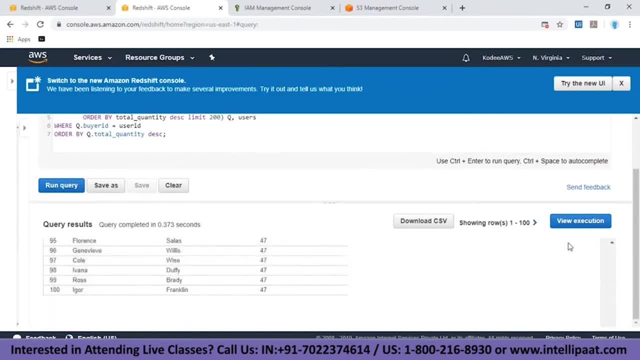 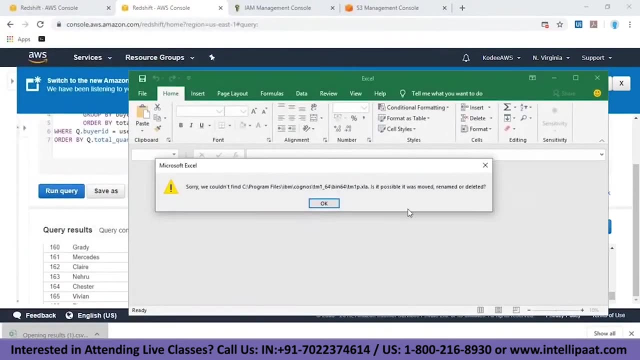 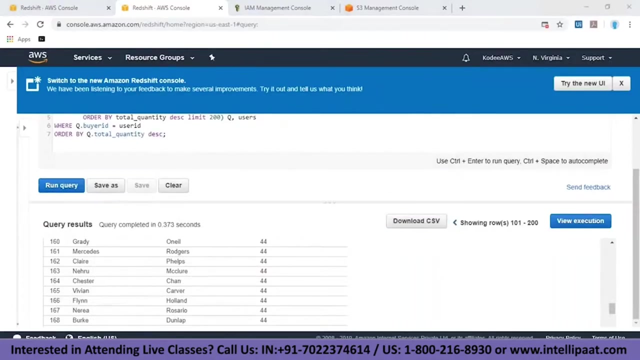 So They provided hundred rows here and then another hundred rows in the next column. So I think hundred rows is the limit for one particular Result column, and you can also download this entire CV CSV, CSV file and just look at the results for yourselves. Yes, so they have provided it here completely. Yeah, so this is one query. I'm just doing some sample queries. 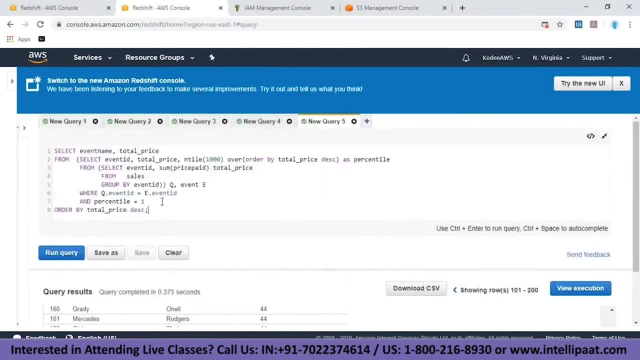 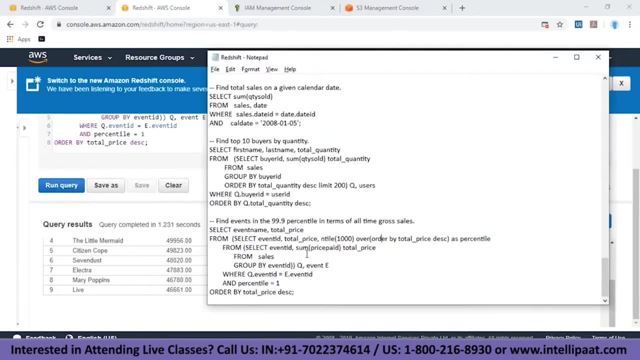 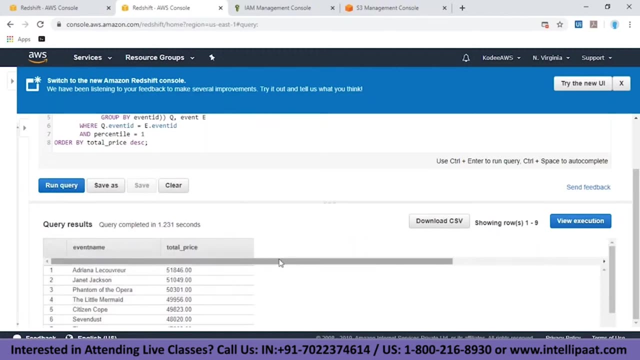 To show how it works. So then select And again another query, same thing so here. So yeah, that that you can see the query results are faster, Even though there is- there is not a lot of data, but still we can consider. but when there is really a large amount of data. 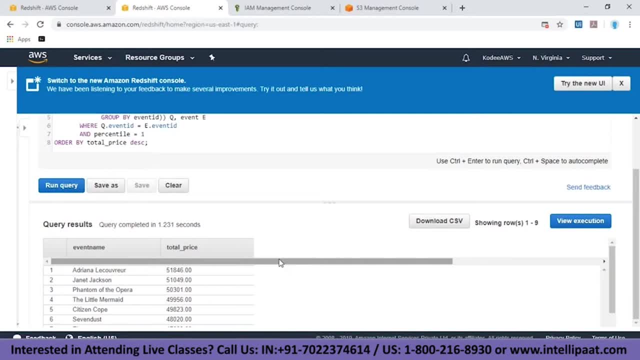 And you want to query some results. they happen very fast because, as I told you, that's what. that's how a redshift has been Architectured: it has one leader node and the multiple compute nodes which distributes the workload, and accordingly, complex queries are Divided into simpler queries and they are executed and the results are clubbed in later node and that final aggregation is sent to the client tools. 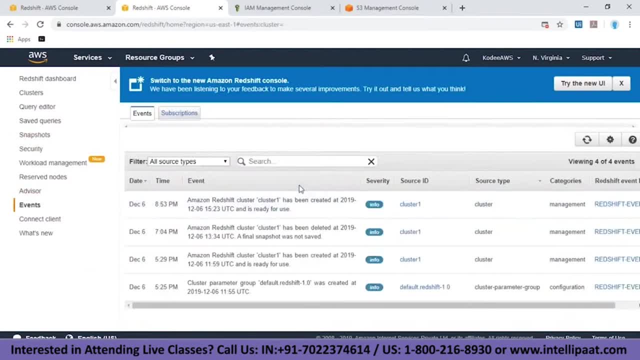 So yeah, so we've done query editor also. and one more, one question about: I am database authentication And so I tried. so basically, instead of: you'll not be able to assign roles to your on-prem setup, but you'll- you can use secret and secret access key and your access key to. 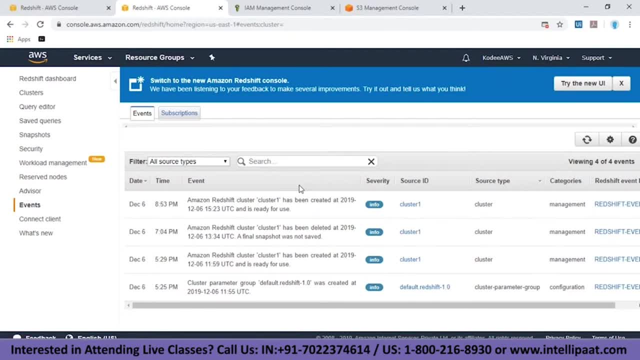 authenticate. for that particular I am users, you can provide programmatic access and Those users can use their secret and access keys to enable I am database authentication. But you can only use that for RDS instances, RDS databases, because only there you will be able to enable it. 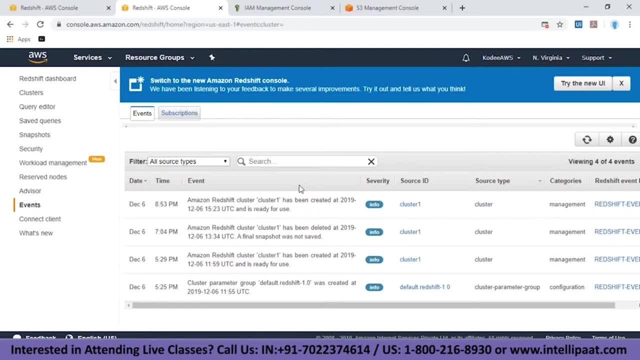 after that, you can just use that endpoint and, Yeah, you can use the security credentials to login, but you'll not be able to Use I am database authentication on your server, but you'll be able to use- what Is that? your secret access key and access key and also the token, and do that. 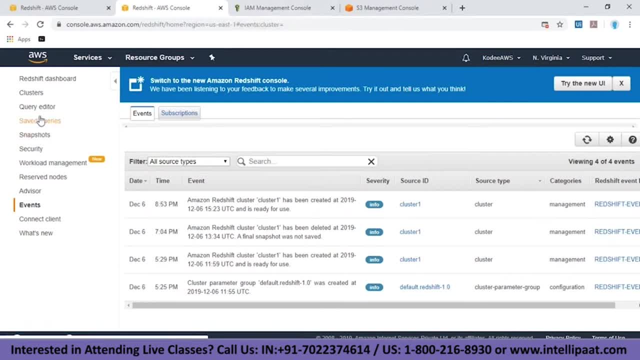 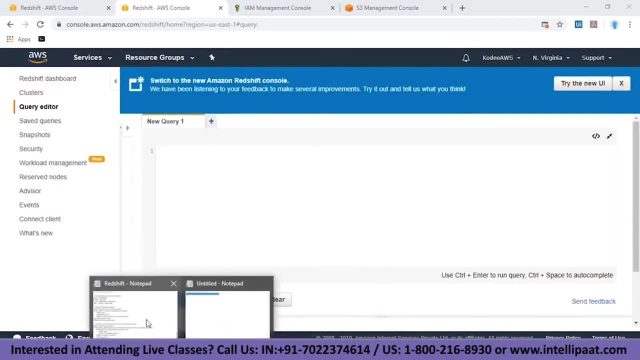 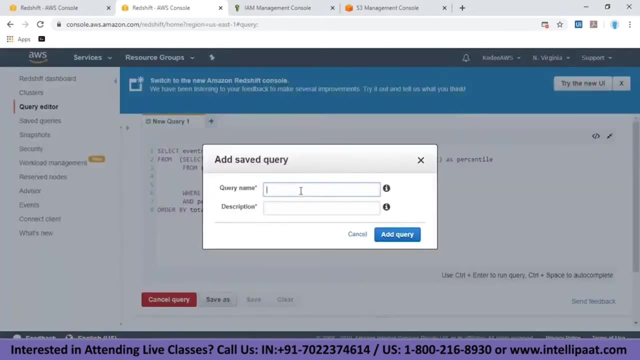 So that is the only option, Okay, So now coming back here. So saved query. So coming back to the query editor, I forgot to show one thing. So, for example, if you think you'll run this query often so you can just save it here, and just save it here, provide a query name. 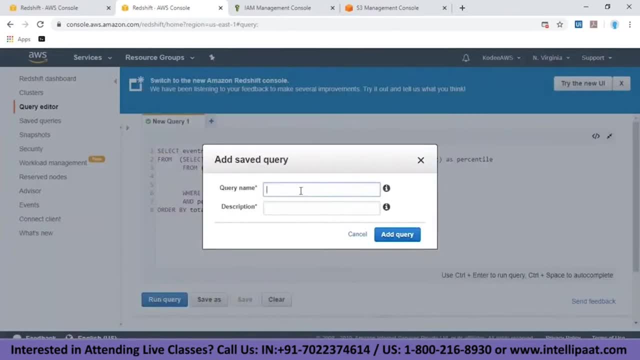 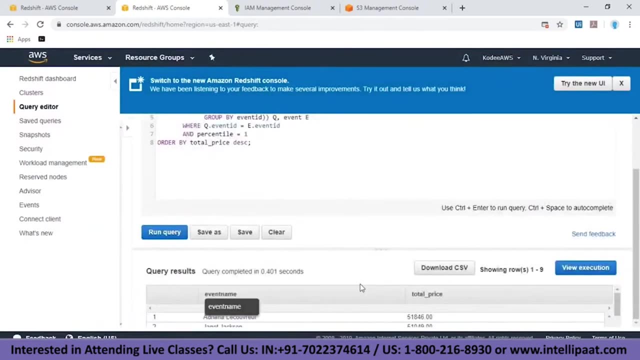 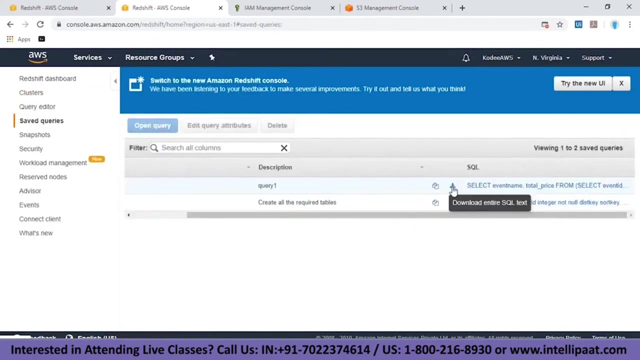 Let's say this is. I don't even know what query is this, So I'll just give query one and again query one. Add query. So done, queries saved: Yeah, so so here. So now go to saved queries. So this is saved query download. enter SQL text: 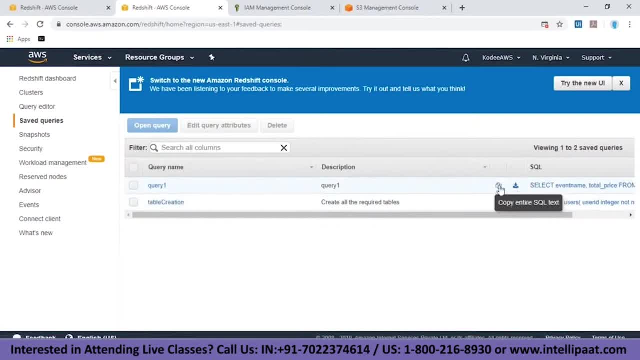 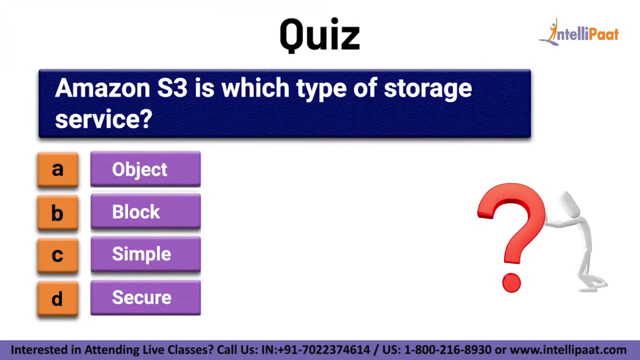 So you can download this queries as SQL text, or you can copy the entire SQL text and just if I just paste it here, Just a quick info, guys, test your knowledge of AWS by answering this question. Amazon S3 is which type of storage server? 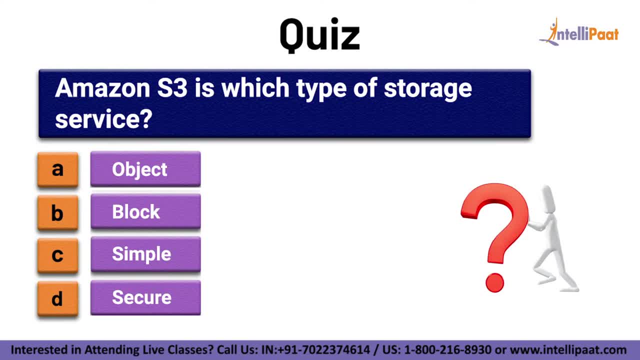 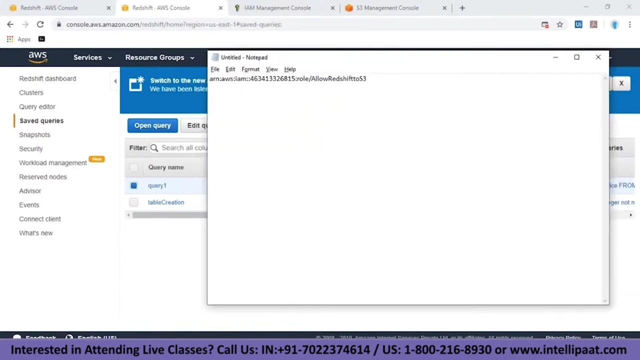 Is a object B block: See simple D: secure Comment your answer in the comment section below. subscribe to intellipaat to know the right answer. Now let's continue with the session. So we'll get it. So this is this pretty easy. 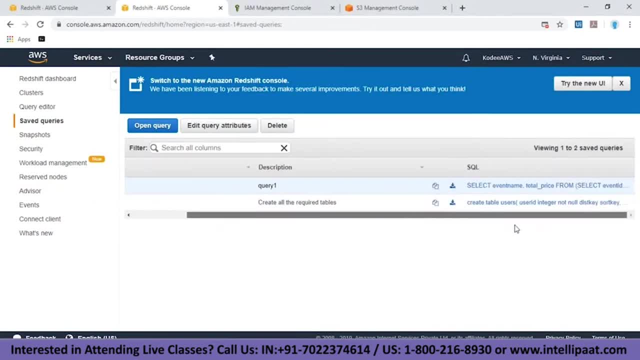 You can just save your queries over here And get them whenever you need. So also, this is easy to control. You can just search what query you need accordingly and get it and then, yeah, so this is pretty much saved queries, That's it. 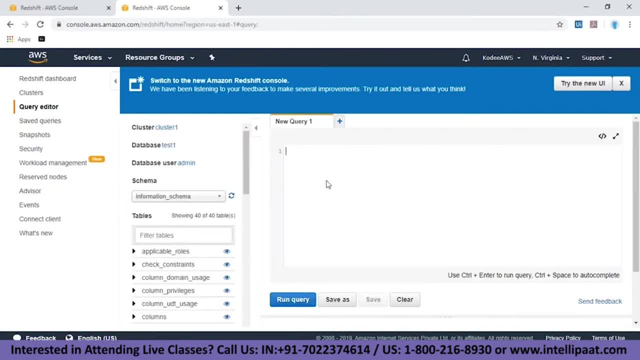 So now, guys, so now let us do a simple demo. with that is: I'll create a role, I'll attach it to this redshift cluster. So what that role basically does, it does is is it provides the permissions to access S3 for this particular rich, rich of cluster. 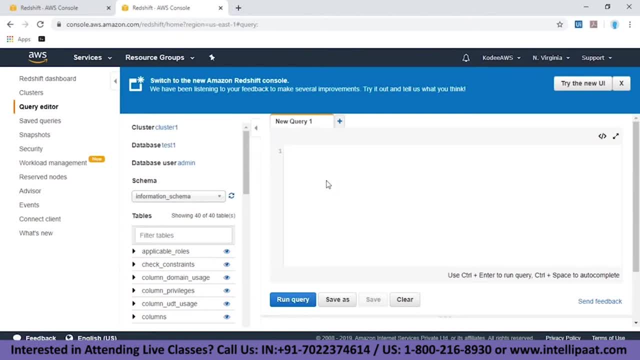 So once I provide this from this redshift cluster, we can query data which is stored in S3.. So I've already stored some data in S3 and I'll also show from where to get that sample data. There is a tutorial I followed, which is AWS again. 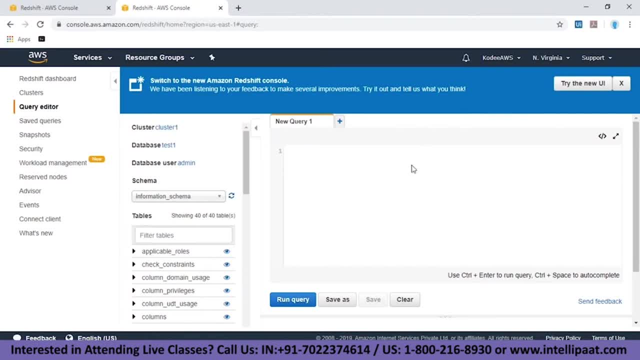 I just follow AWS official white papers and documentations, So from there you can get the sample data and you can upload it to an S3 packet. from there You can, you can provide the IAEA I am role to this particular redshift cluster after providing it. 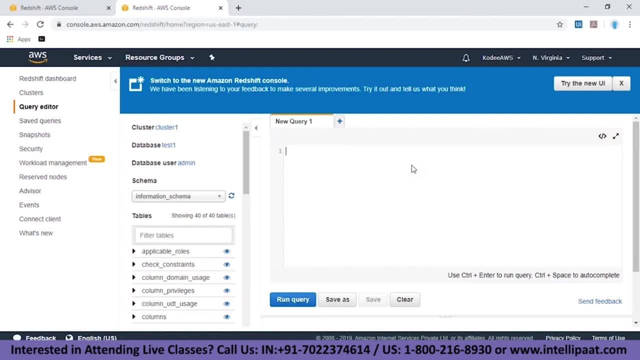 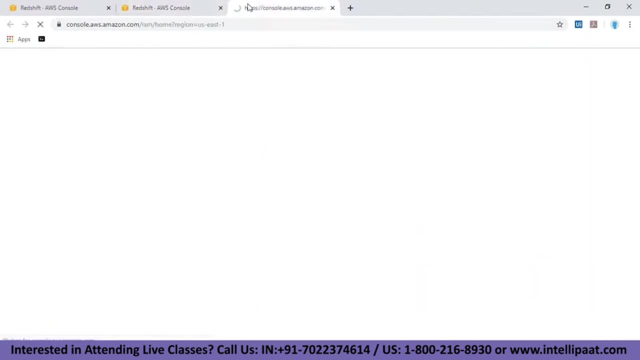 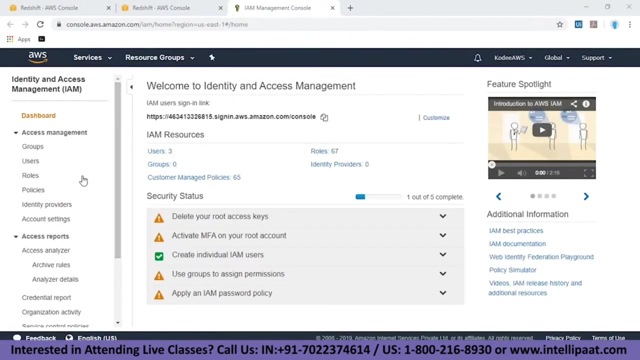 You can just query it and create tables here. after creating tables, load data into this database. after loading data, You can query the data stored. So yeah, so let us start with that. So for that, first I'll have to you open. I am so first I'll have to create a role, as I told you. 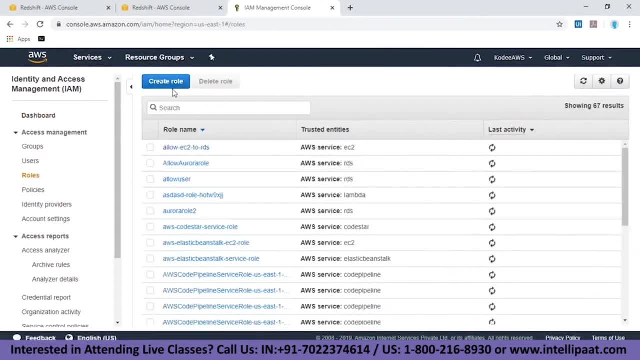 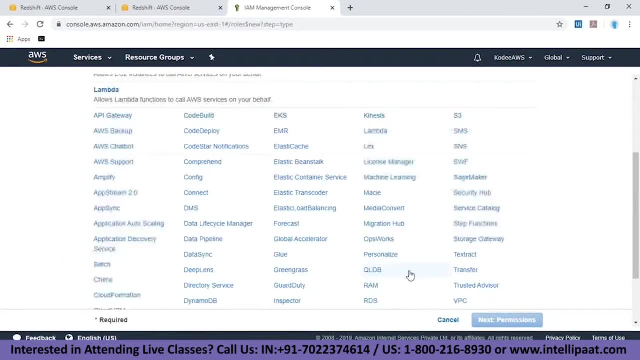 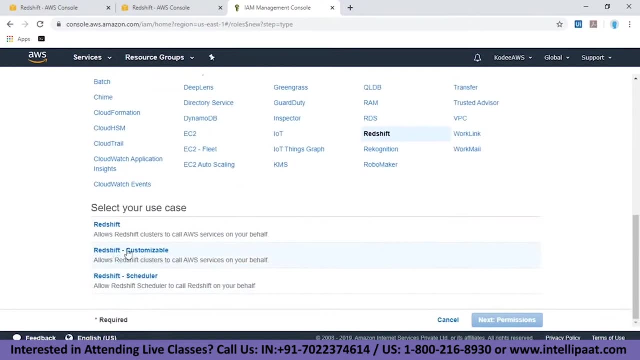 I'll have to create a role. So role create role, or the service which I have to provide the permissions to is redshift. I'll have to choose to redshift. redshift is over here, So I'll be choosing redshift. customizable: There is one thing called scheduler, and this is not for clusters. 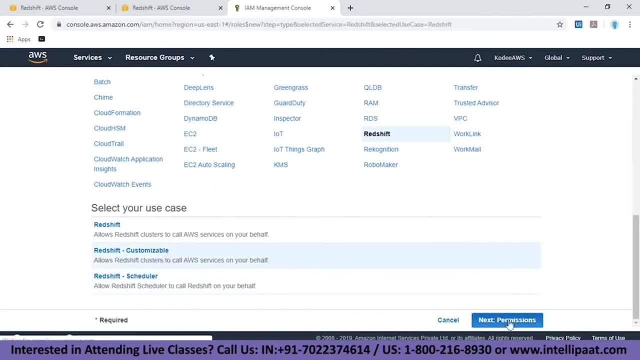 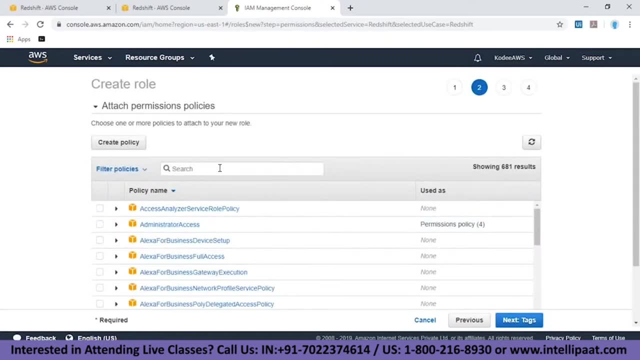 This is for clusters, So I'll just choose this, And then here you'll have to provide the permissions for redshift accessing S3. So redshift does not need any other access, It just needs to access to read objects inside S3.. 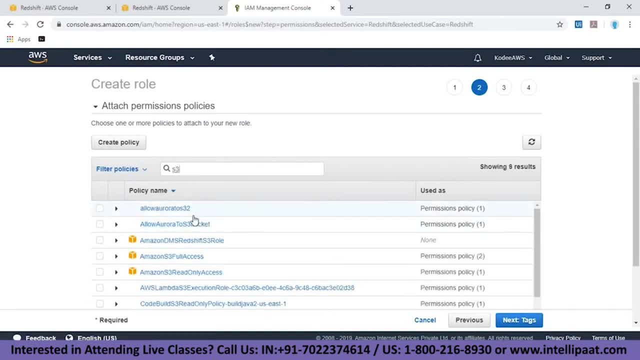 So let's see. Yeah, so here is three reader. So there is this. that is Amazon S3 read only access. So this will allow the redshift cluster to only read the Data from S3.. So I'll just click here. next tags: 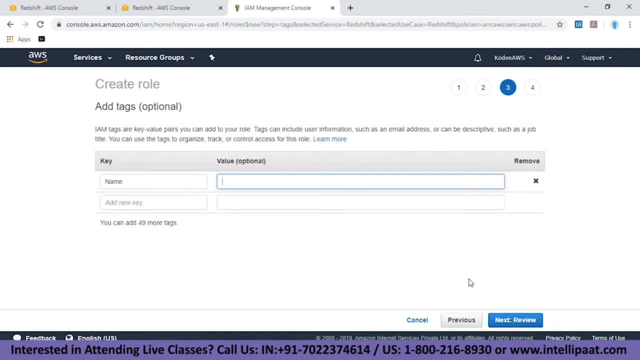 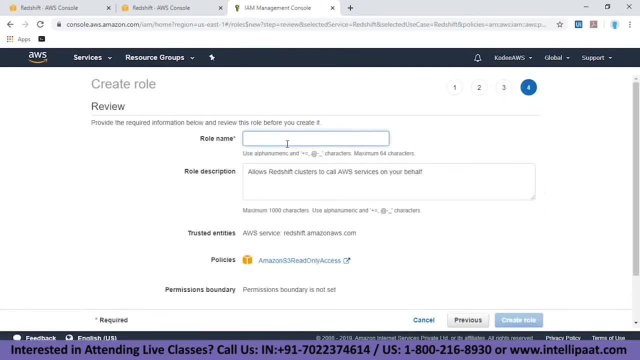 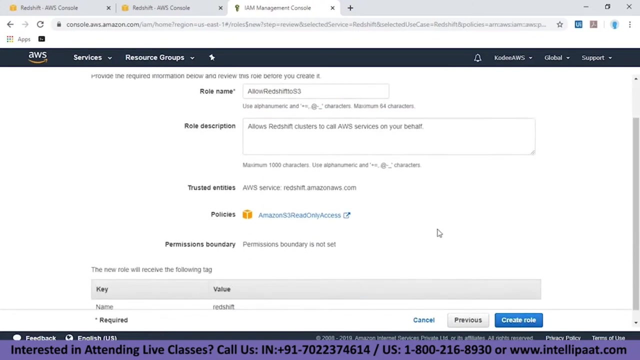 If you want, you can add a tag. Let's say name redshift. Then review: provide a name Hello redshift To S3.. And yeah, so this allows redshift clusters to call AWS services on your behalf and then create roles. 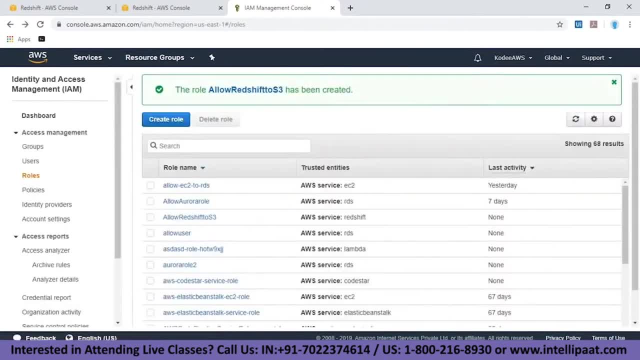 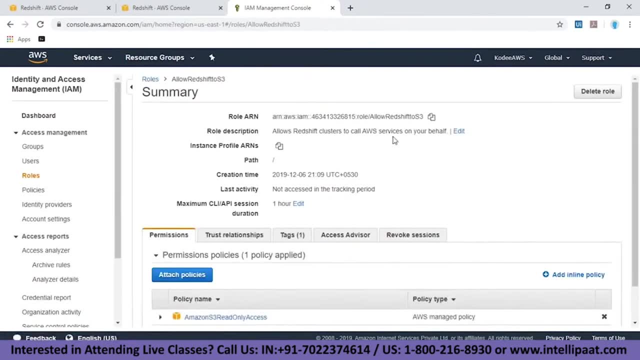 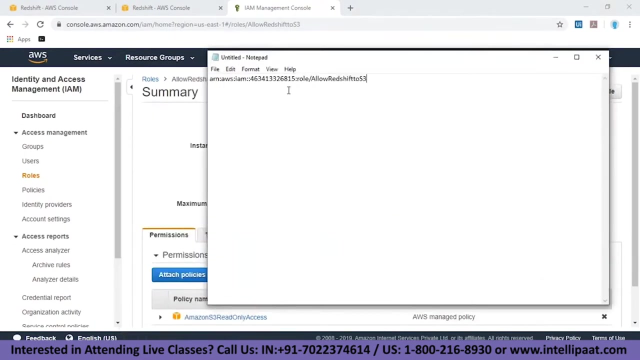 So so the role. Yeah, so the role is created, So I'll just copy this. We need, we will need this ARN ahead in this demo, So I'll just copy this. So this is one. I'll just open another. save it here. 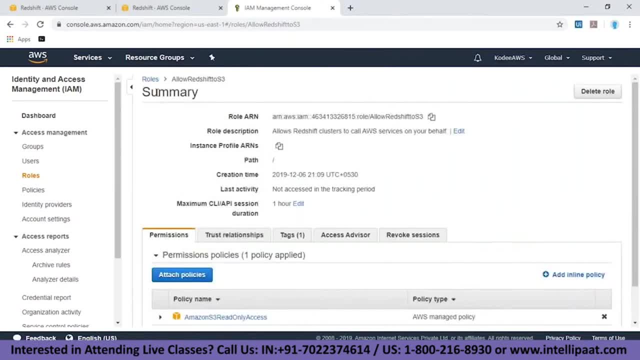 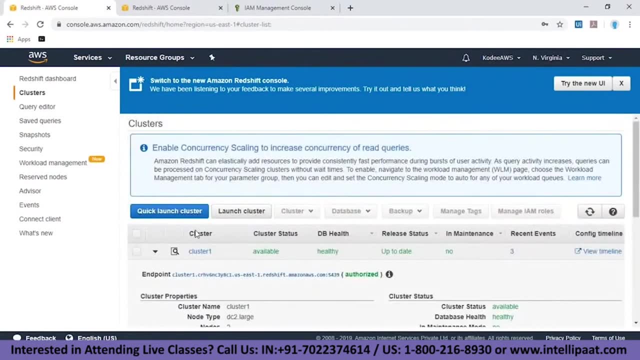 Okay, So now we've created this, So we are going to attach this role to our redshift cluster, So I'll go to my cluster To. I think I can more manage here itself. manager am roles. Choose a role. This is the role I created right now. 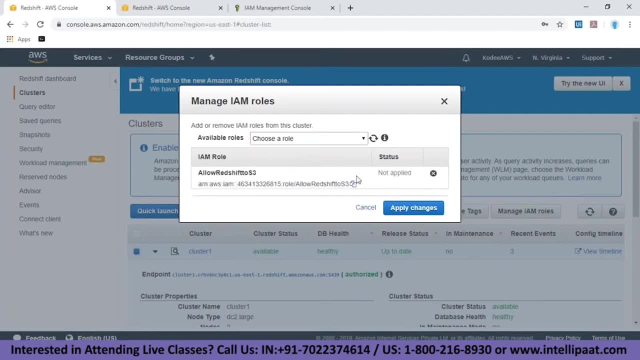 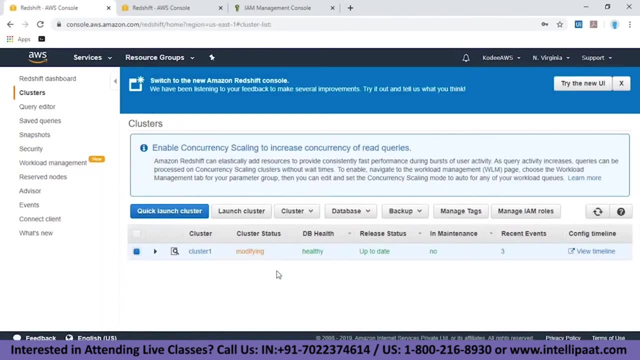 That is, allow redshift to S3, click on it and then apply changes. Yeah, so now it's modifying. So we have attached a IAM role to our cluster. So that part is done. So the next part, because we are going to lower taken data from S3.. 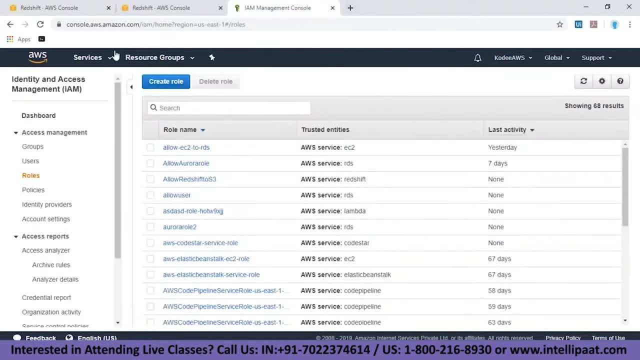 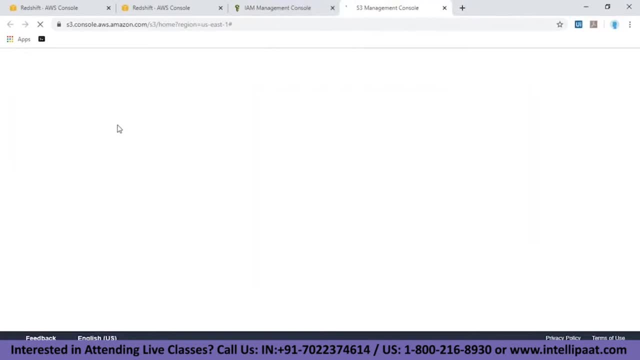 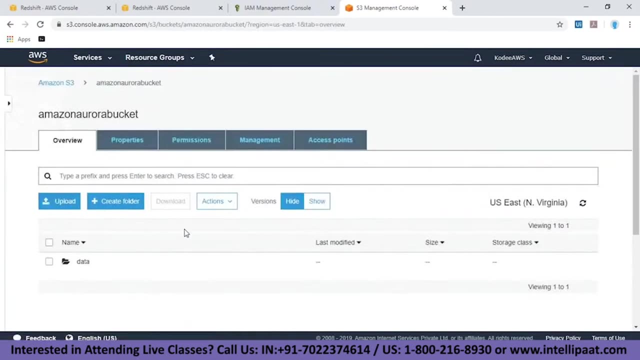 So now data should be available in S3.. So I'll open the S3 console. So I've already uploaded the files inside S3.. I'll show which bucket. Yeah, so it is Amazon Aurora bucket, The bucket which is created long back, and I've created a folder inside that data. 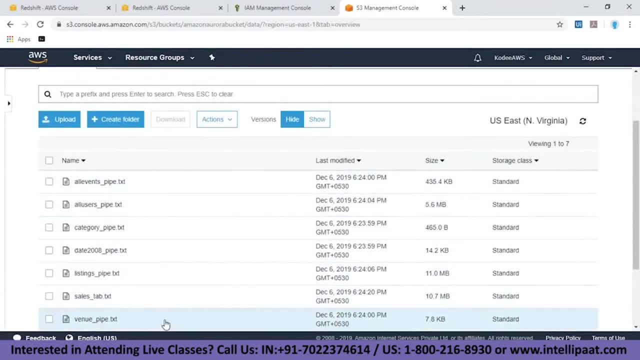 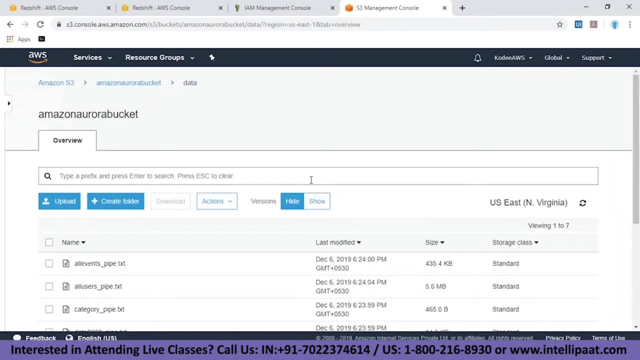 and inside that all the text files are available. So those text files, I have the zip file of that and I'll also show which documentation to go for, like which documentation you can go through and get the or is it? you can get the load this. 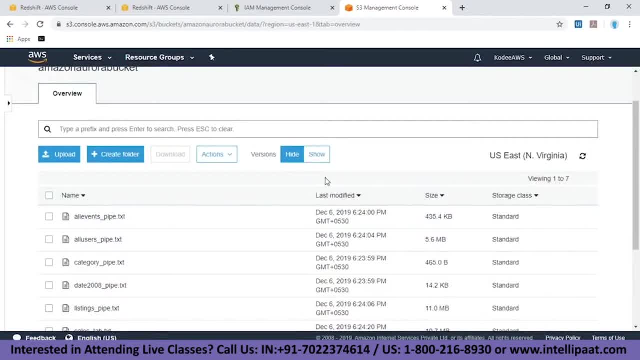 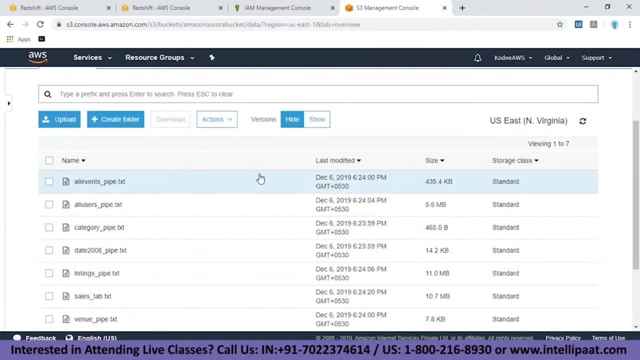 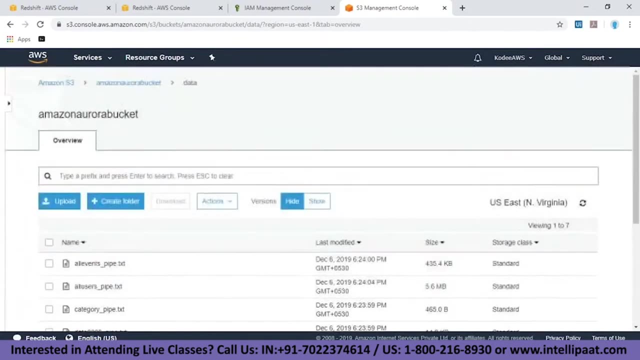 Particular files, the zip file, and also from where you can get the queries. So, yeah, so right now we have attached it to the cluster. Also, We have the data inside our S3 database, So it is over here. Yeah, So we created a folder, uploaded the data into it. 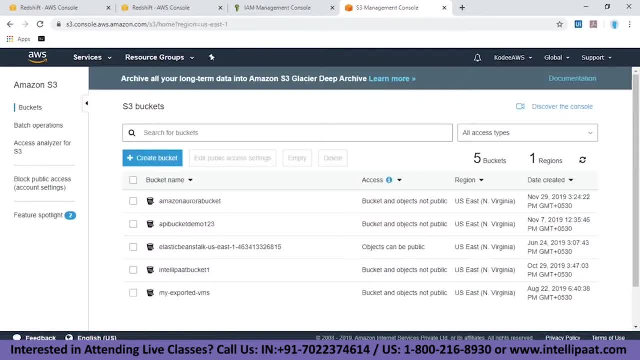 So right now my S3 is set, data is ready. Now I just have to run the queries accordingly to create tables. after creating tables, I'll have to load that data inside those tables. That will be my second part: after loading data inside that table, after that. 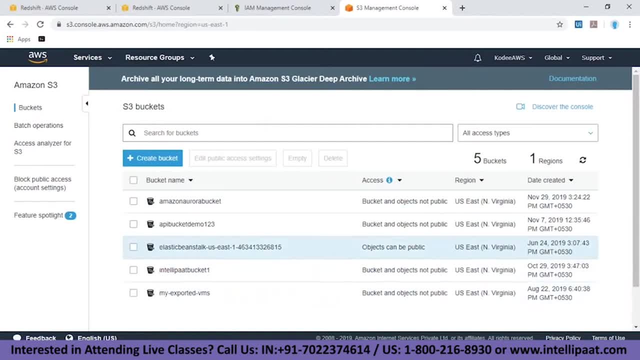 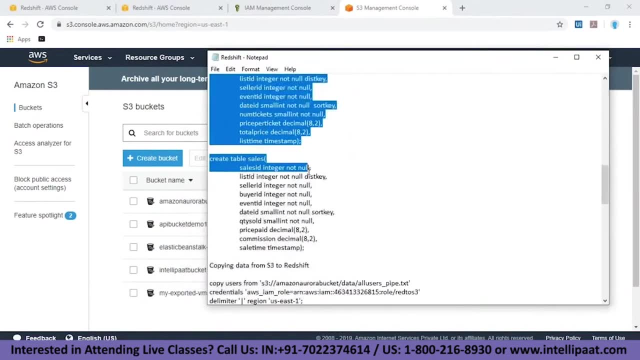 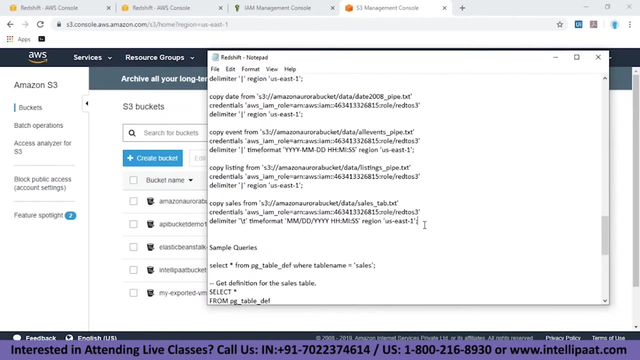 I'll have to query, start querying. So right now, let's just show that. so first I'll be creating these tables, After creating these tables, I'll be copying. So these are some more queries. So you would have taught why I copied the ARN. 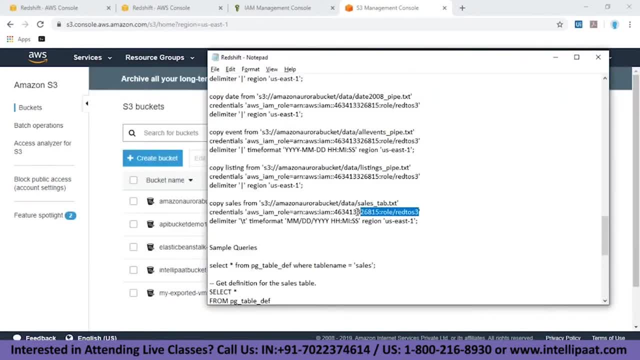 So basically I'll have to copy this ARN and paste it here So this will show. So basically, the query editor does not have access, So for that we'll have to provide this so that the S3 bucket knows that. so this particular I was a- I am role. 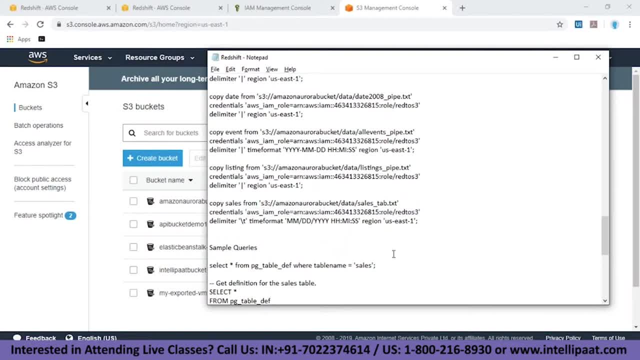 So basically, it allows the redshift cluster To access the data from S3. So while providing this ARN is the S3 bucket will automatically understand We can provide the data to it. So this is that. I also paste these in the end. 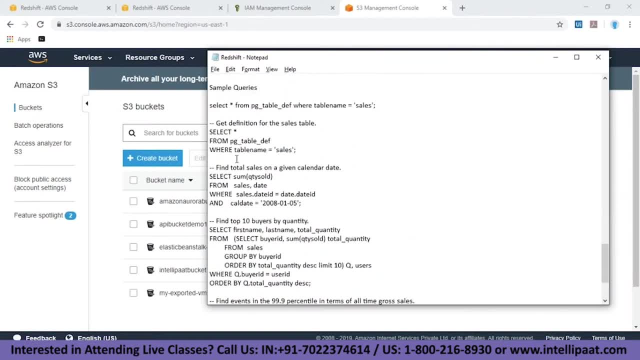 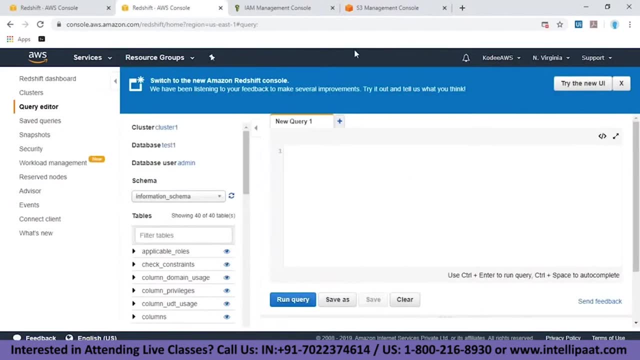 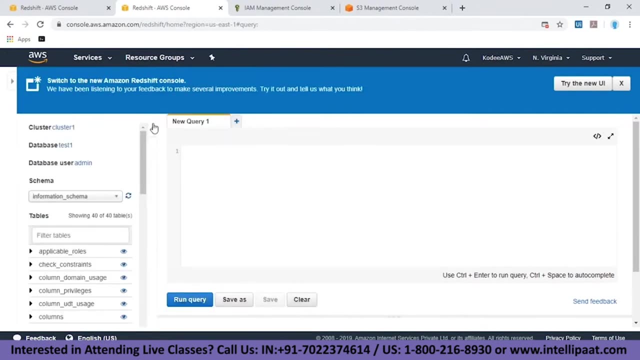 and then these are some sample queries, which was available. So yeah, so done. So now let us start off with this process. So first I'll go to my query editor And then I'll just Do this and do this. Yeah, So now I have my query editor and here you can see the query results. 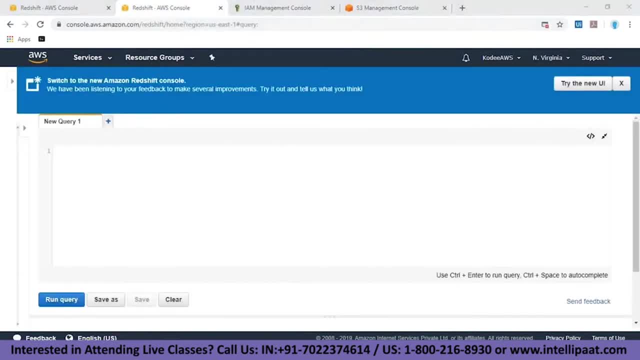 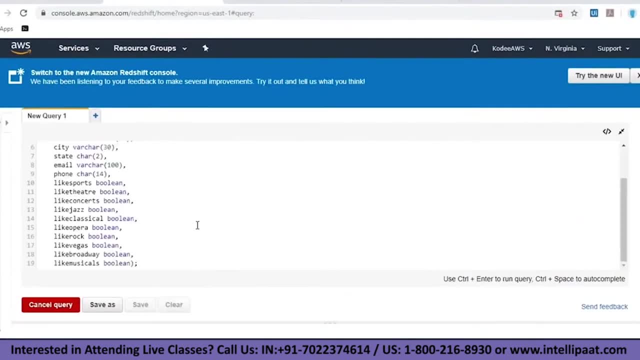 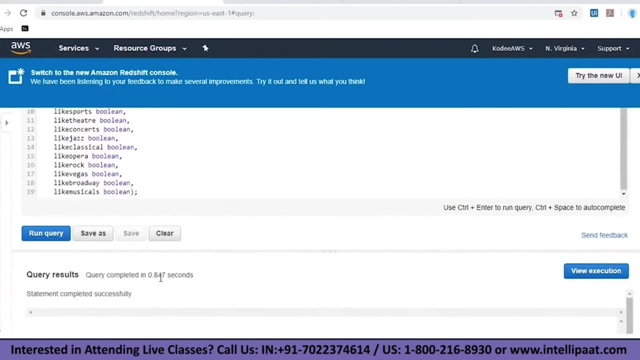 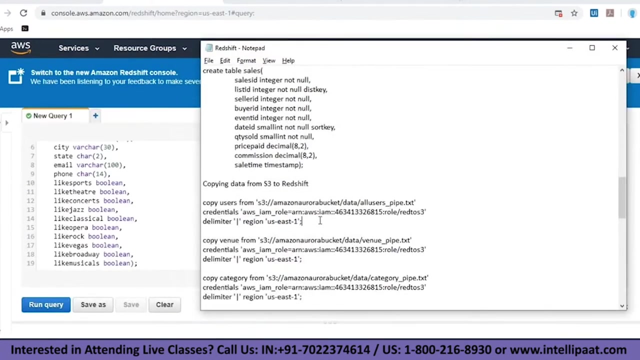 So now, Yeah, So now, first we'll have to create tables. So first I'll create this table. Run query, So completed, and point eight seconds, So done. I've created one table and now I'll load the data for that particular table. 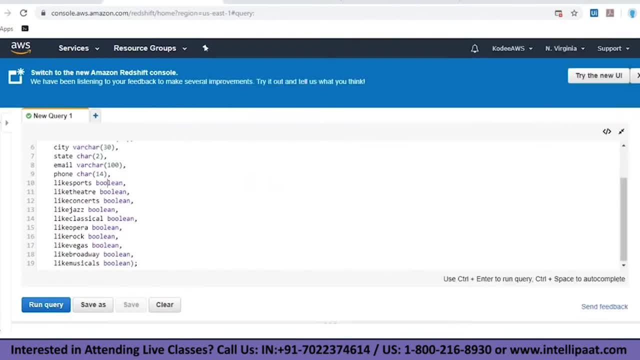 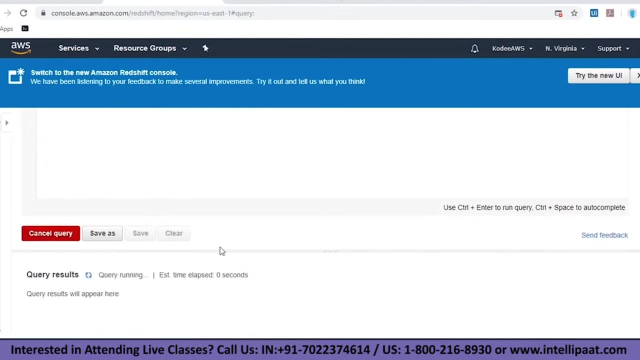 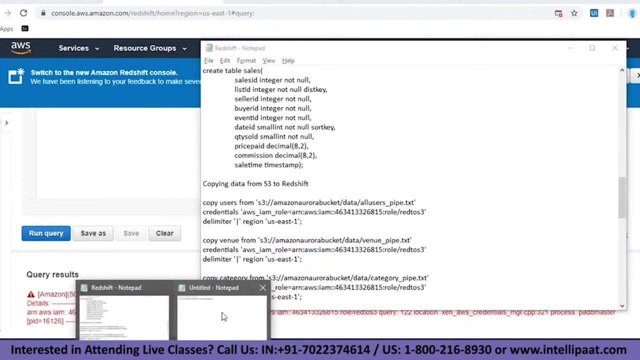 So now I'll just copy this. I can just paste it in this query and hit run, or I can create a new one and hit run. So I'll just run here. What is this? Oh, sorry, I did not change the role. 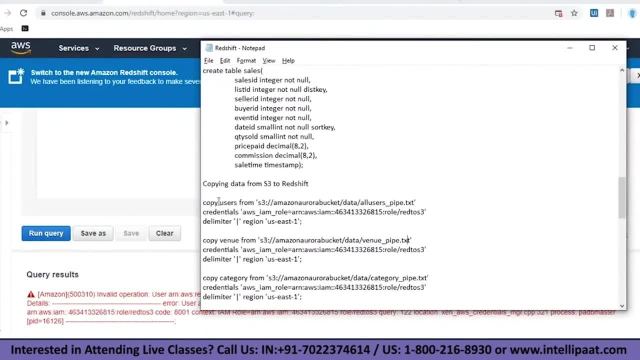 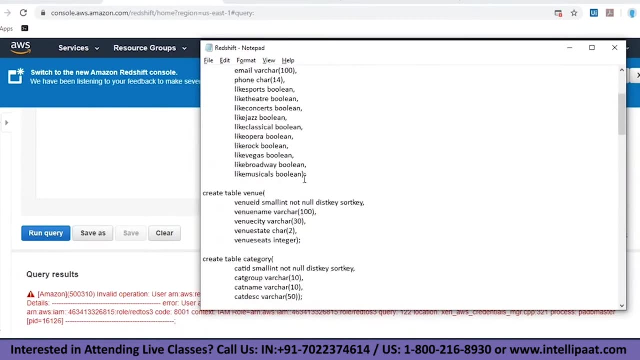 What is what's the copy user? So these are some for query editors. These are the commands for copying users in the sense: Oh, the table name, Yeah, Okay, Okay, Got it. Yeah, Confused with the user. Okay. 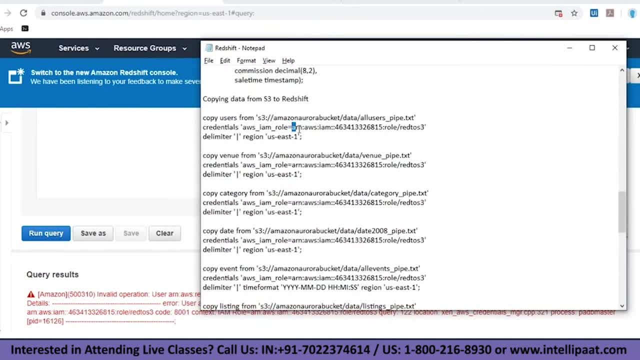 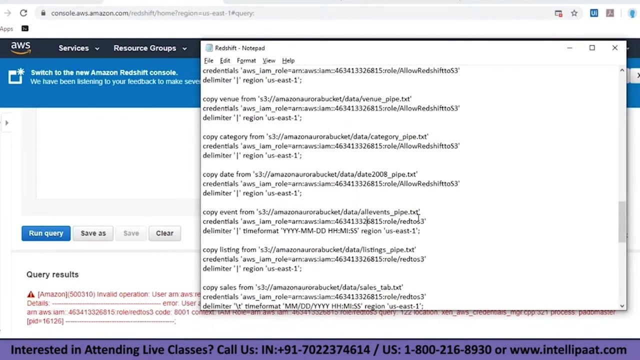 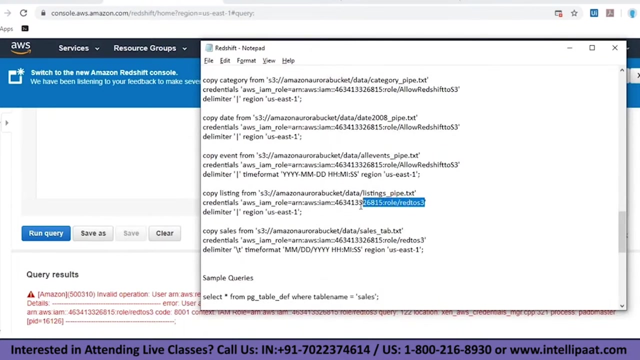 Okay, So now I forgot to change my ARN, that is, Amazon resource number Of my I am role, which I just attached to my rich of cluster, So I'll just paste it all over My queries. Sorry, Yeah, so I that's done. 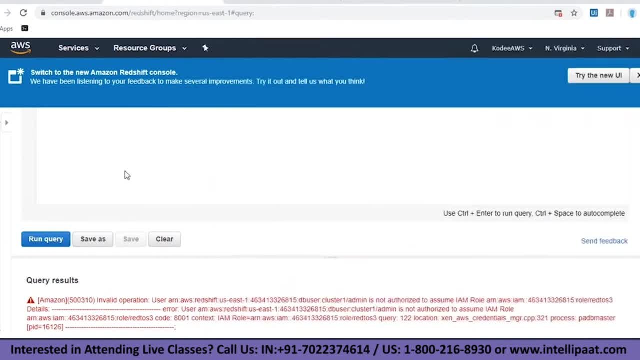 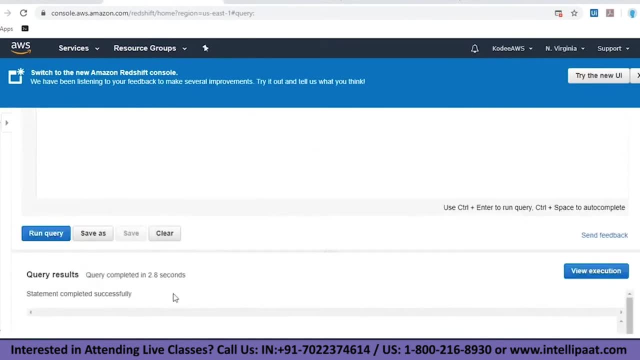 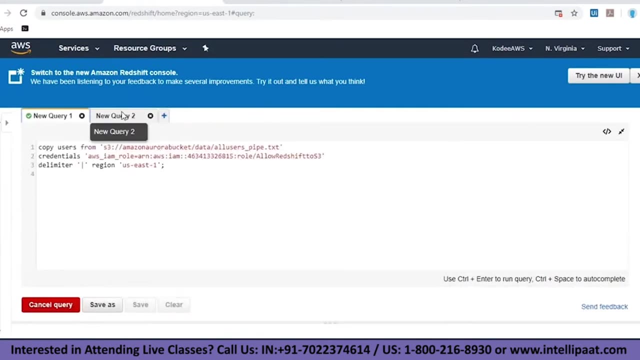 Okay, So now I think it will work. So yeah, it's, the query has run successfully. So now we can just use this one query to do all the operations, or we can open another query and do so. we can draw, do this So as also as a best practice in the documentation. 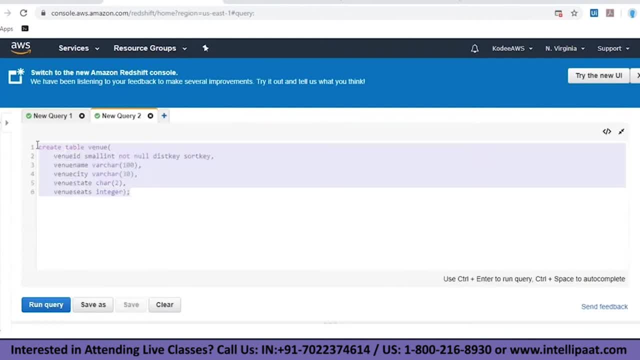 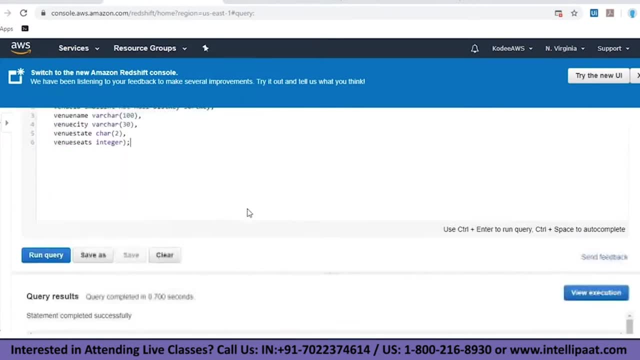 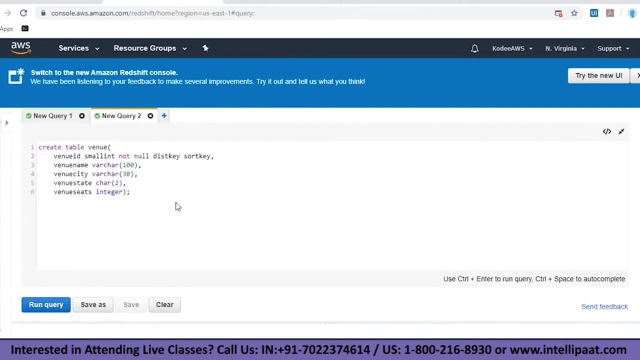 they told, run one query in one query page. So one complete query in one query page. that I don't know why, but that is what they have told. sometimes when you run multiple queries, there are some errors occurring. here It's showing some some kind of Intentation errors or something. 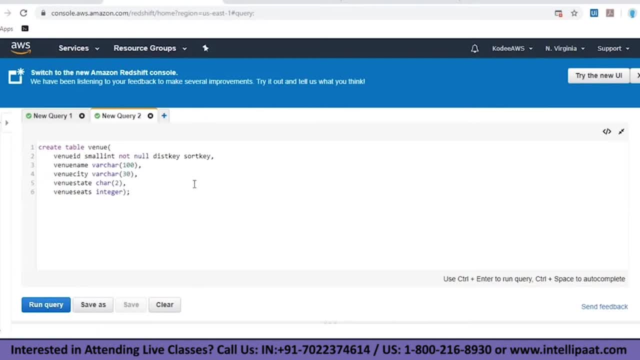 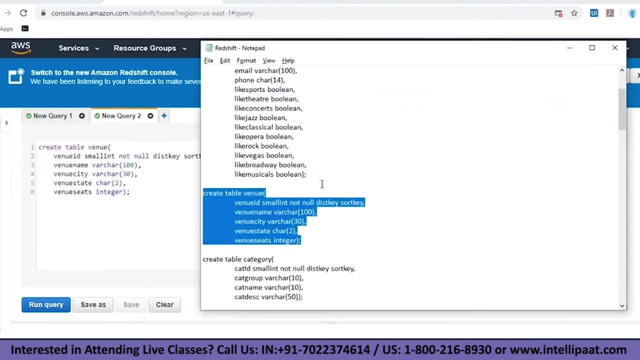 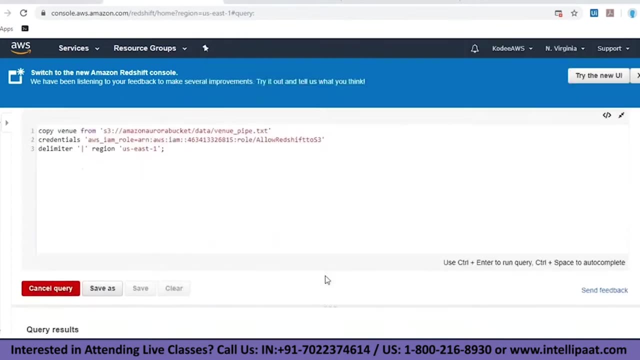 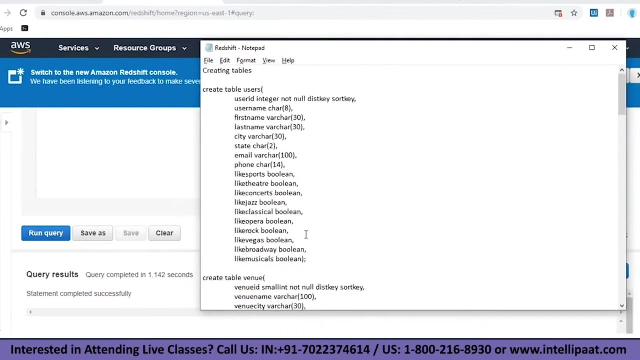 So that's what it was showing here. So around one query at a time, then, but you can run a query in the same query, So I'll just dashboard multiple times. So I'll just upload the content of this done Then category. So just wait, I'll just do. finish this off. 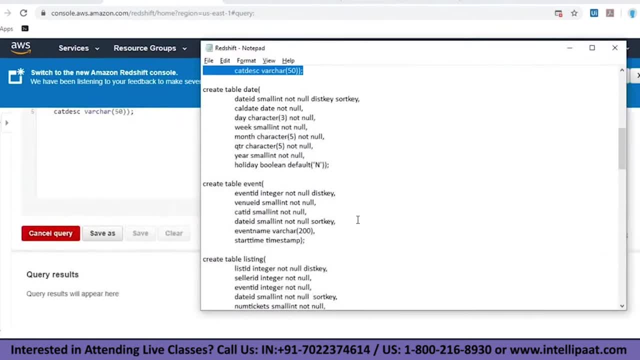 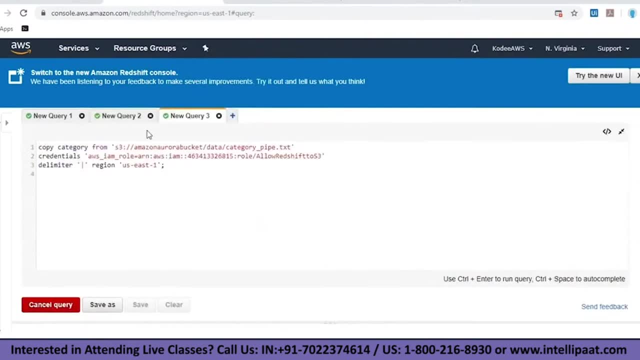 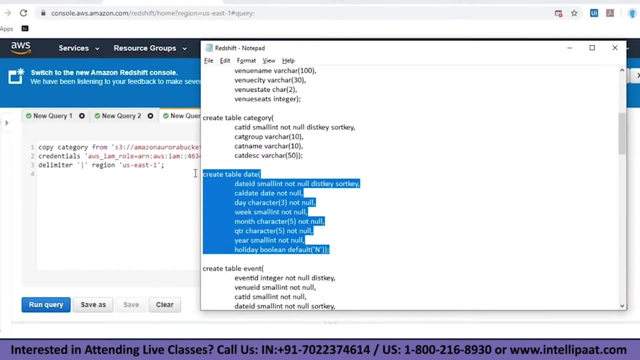 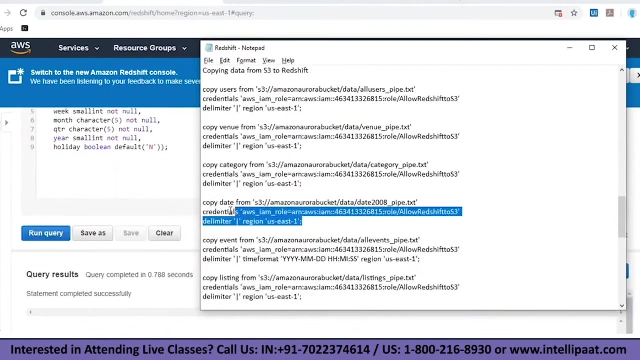 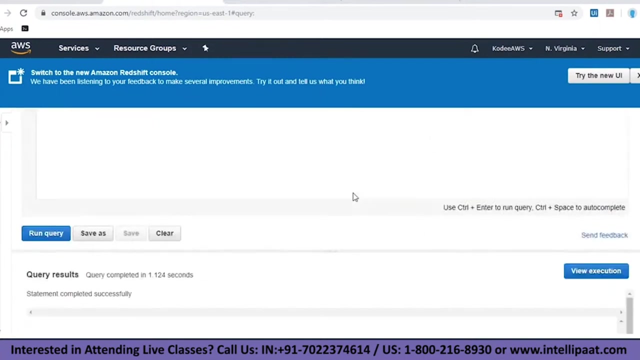 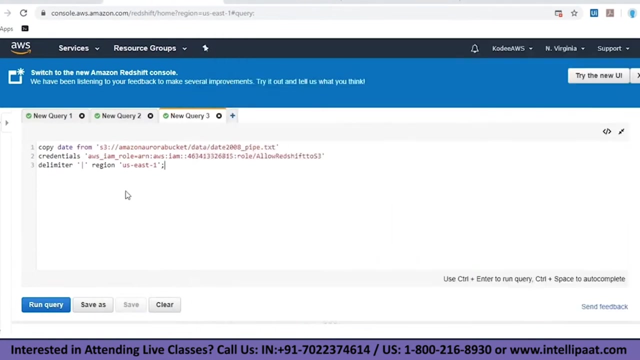 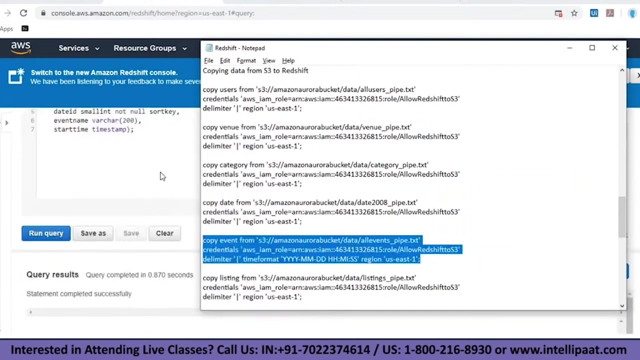 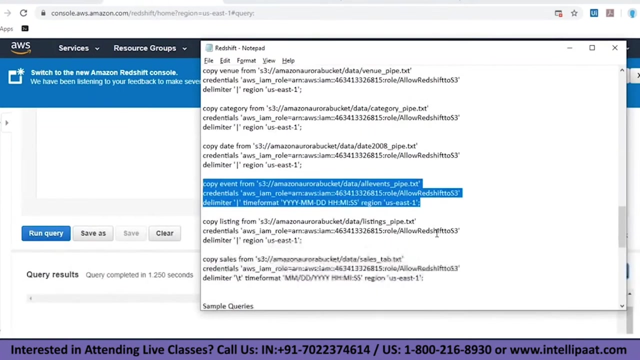 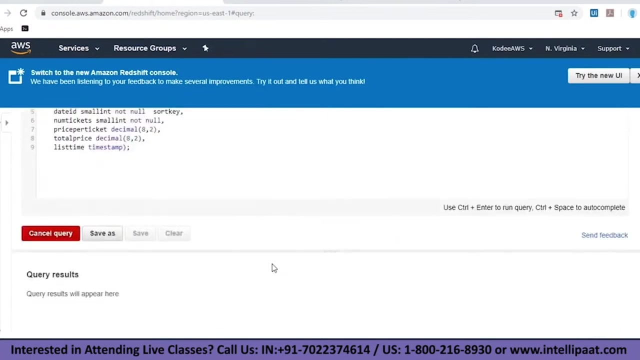 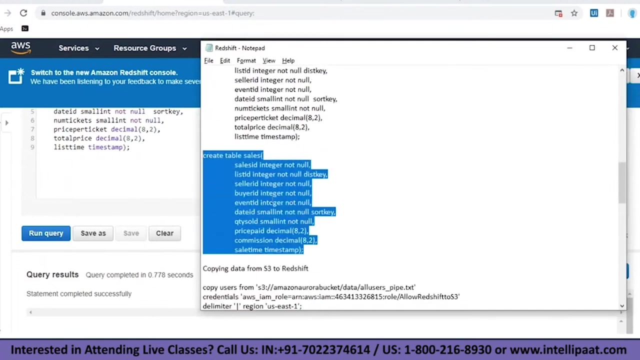 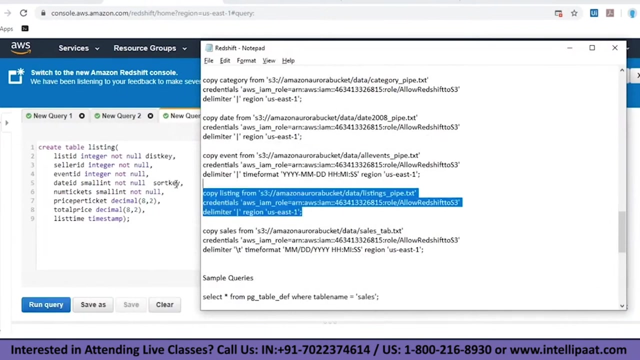 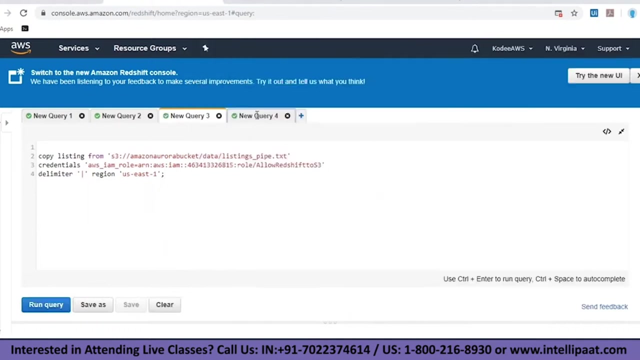 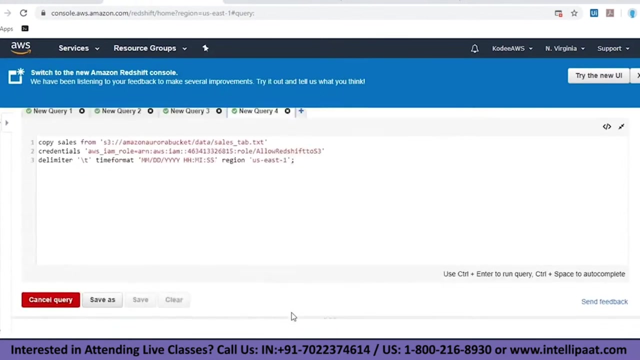 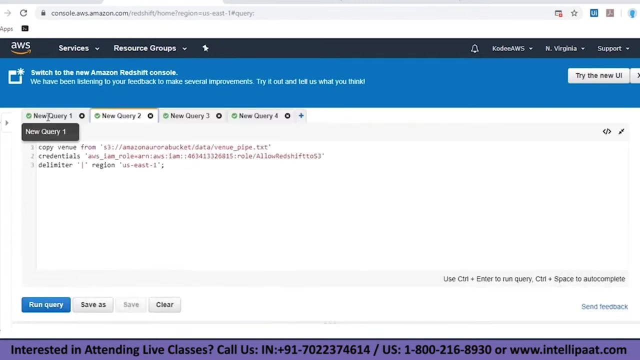 Just create multiple queries based run And then date: Successful, Done, event Done. then there are two more listing And then sales. Just create one more. Sorry, So Every time you open it shows the results. It's taking some time to show. Okay, so we've uploaded all the content inside our tables. But one more thing is: 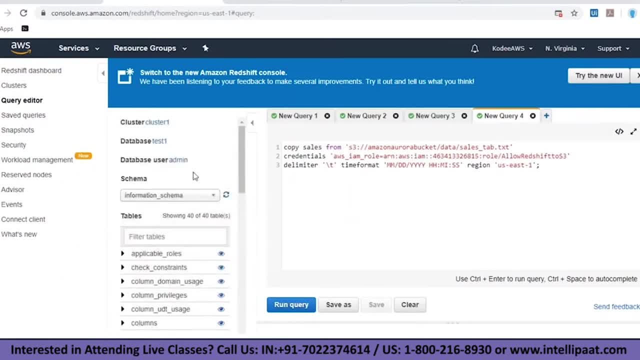 You'll not be able to view that content here. that is the only problem. it is just to query In query editor. you'll not be able to view the data you stored, So for that you'll have to use an SQL client. But you will be. 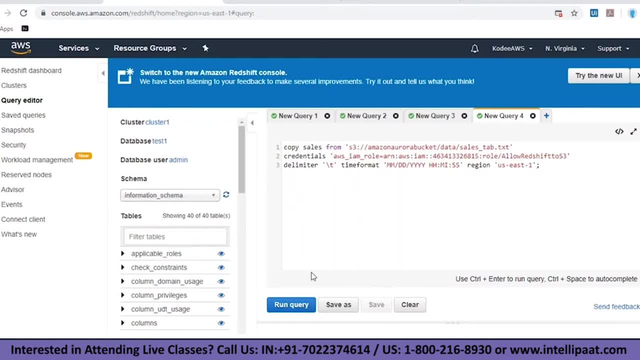 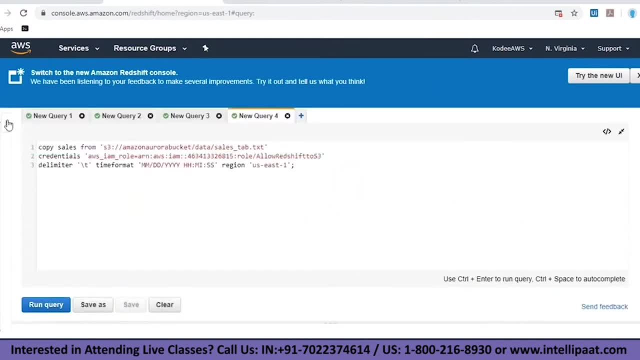 Be able to run queries and then see the data. So, yeah, that you can do, But there is no option for viewing all the tables available, Like that, so you will just have to query all of them and see here. Yeah, so If it is a client or a workbench or something like that, 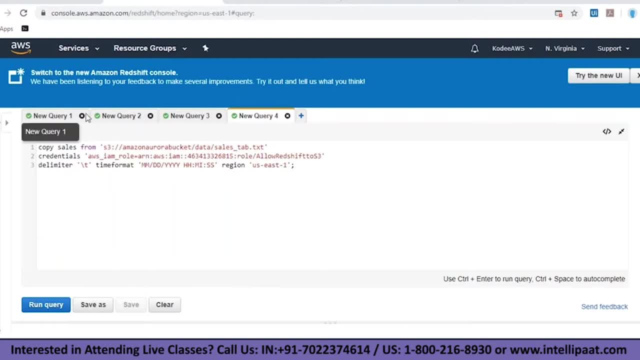 You have everything. you have your own GUI which you can use to see the tables available or the databases available and everything. But in the query editor you can only query. that's the one, Only option here. So now we have uploaded the content, So I'll also show. 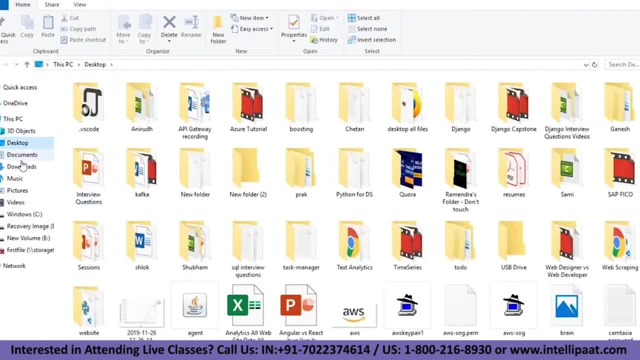 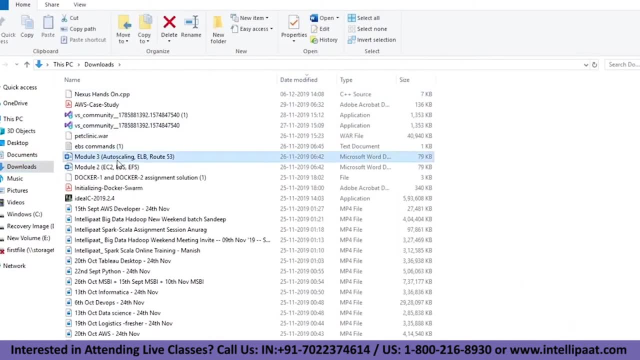 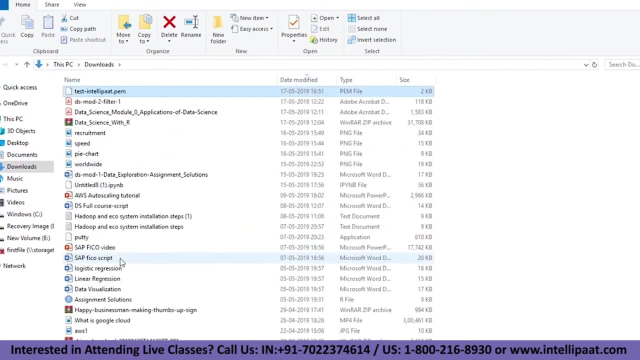 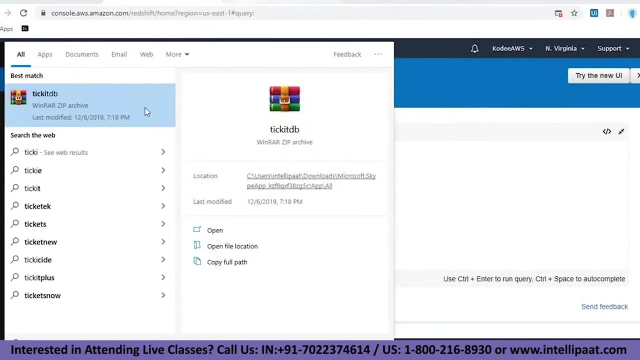 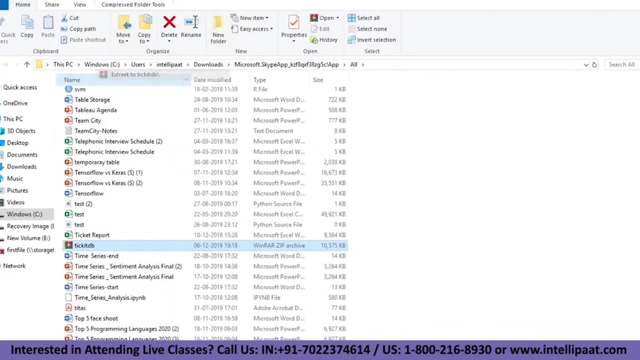 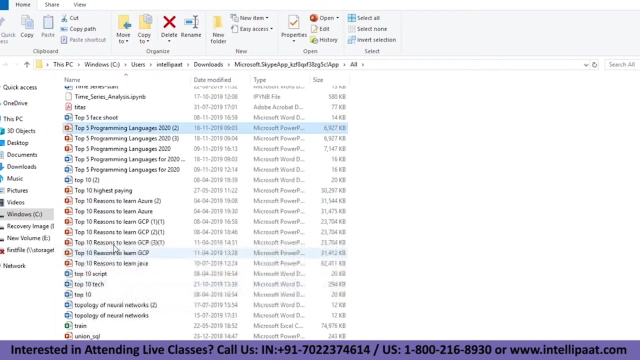 What was in the content. so It was it. There was it, Think the name of it was ticket. Yeah, So if we paste that data into here, you num Walter was, so You can do. I knew I we'll also do so, But for now I'll save that. We did it. 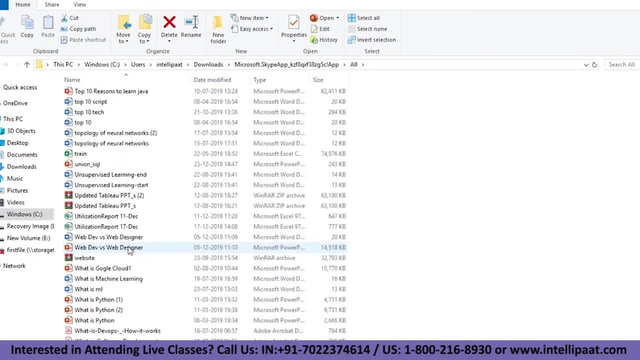 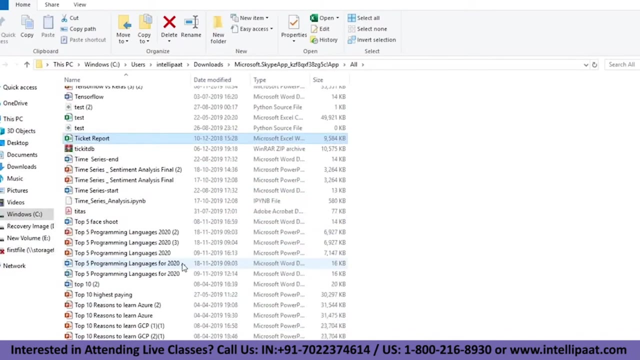 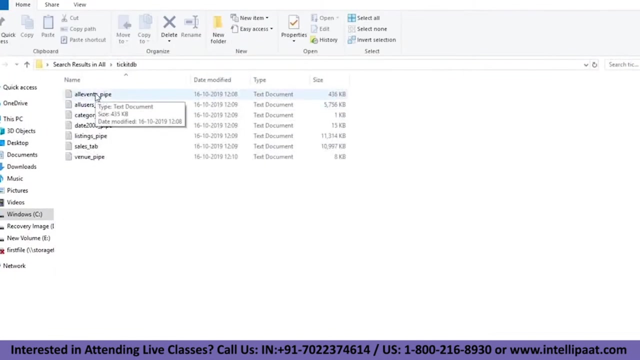 Okay, so Right, so It just So. Anyway, I'll just I'll just record Lead. You have to select a IS transparent image and which identity element? Yes, on the right side. Yeah, there is one. None options, is it here? so these are the files. they're all text file, so here you can see. 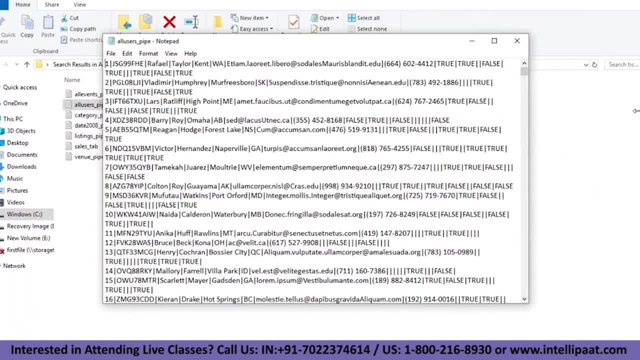 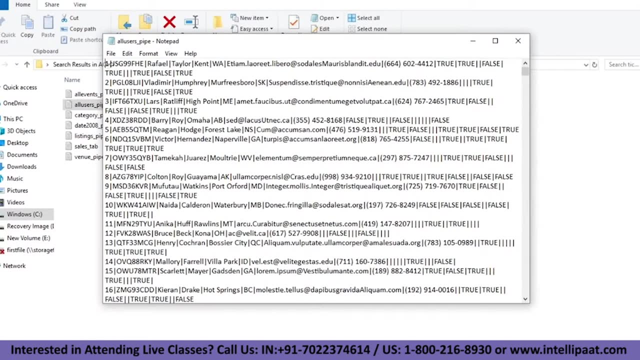 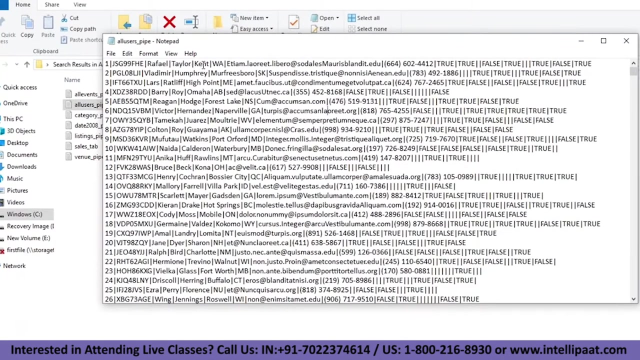 so just saying it's loading. yeah, so this is how the continuous available, so you can see the number, the code or something whatever. is that name, middle name, last name? so whatever order, and then the email, the number, some questions: true, true, false, true, true, false, or something. okay, so so you can see there's. 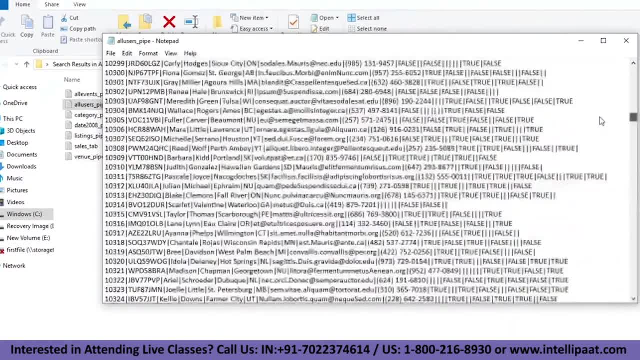 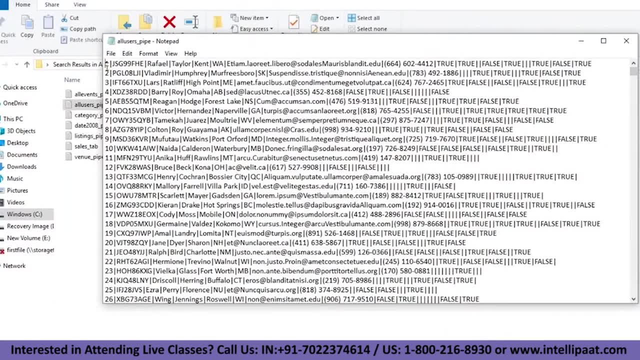 a lot of data available. so these many queries, sorry, this many rows. so basically, it will not be uploaded as single rows. so if it is a product as single rows every time, it will take a lot of time. so what they do is they consider this entire column as one row, one, one, one one. so they do that and they. 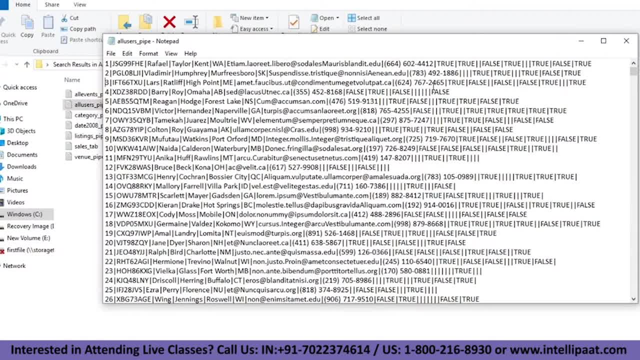 upload it. so basically, it happens in the redshift and it happens transparently, which that's what you promises us. they use columnar data storage, so I just wanted to show this. I also I'll give the link for downloading this sample data which you can use for. 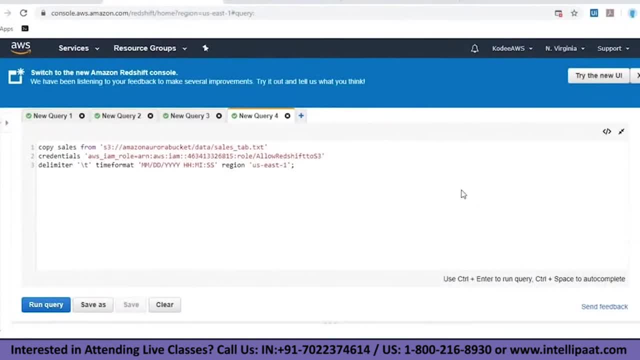 practicing. yeah, so now we have uploaded all the content, we have loaded the content from s3 into redshift, so now we'll have. we'll just do some querying and practice it. so sample query is. so this one is to get the table definition. I think table definition of table name is table name. is table name. is table name. 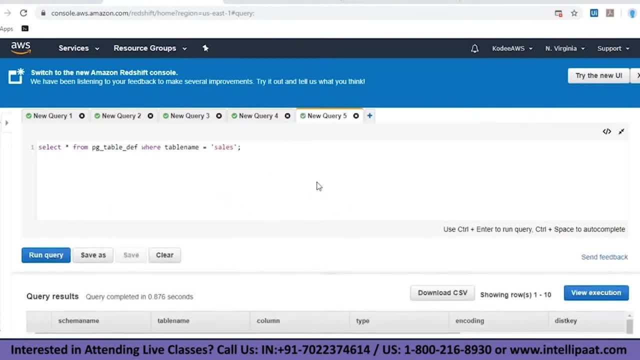 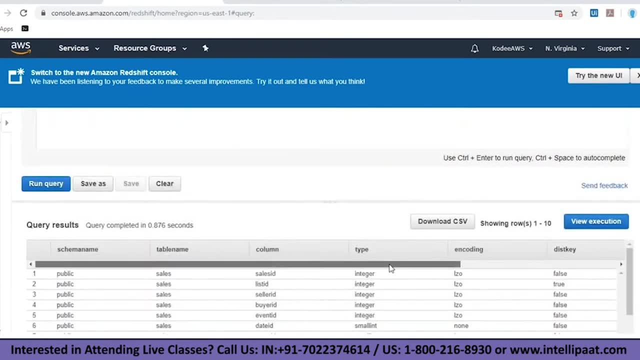 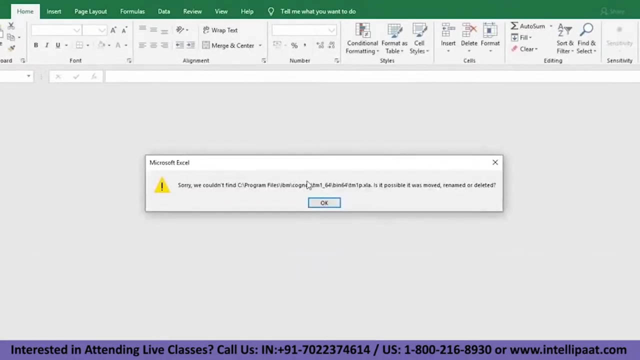 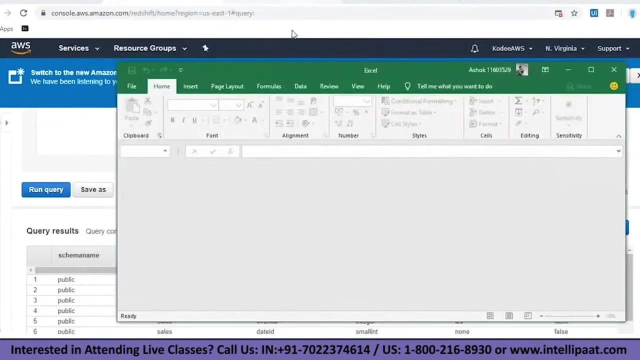 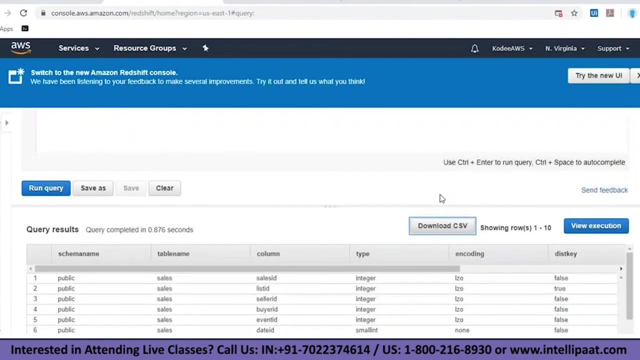 sales. just push it up. yeah, so table division definition over here so you can see the query results over here and also you can download the CSV file from here and just save and you can download it and you can also view the results here. you- I guess I'm there is some problem with this- so you can also download the CSV. 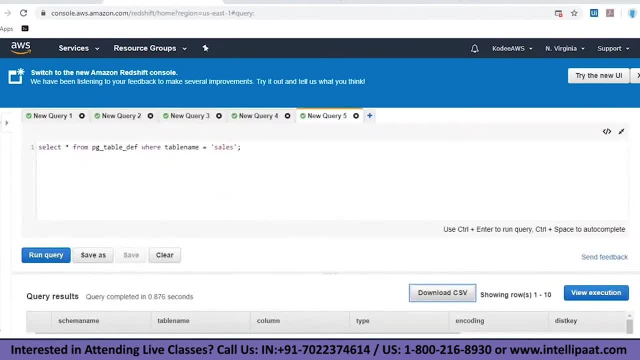 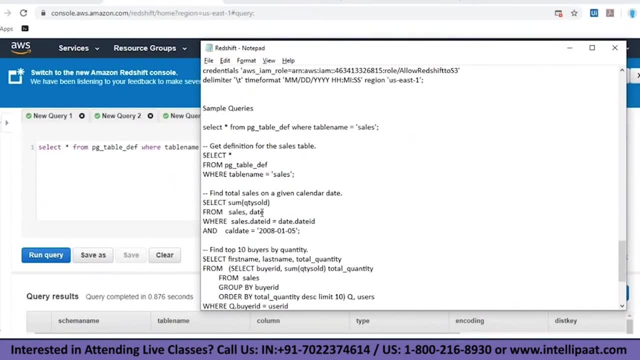 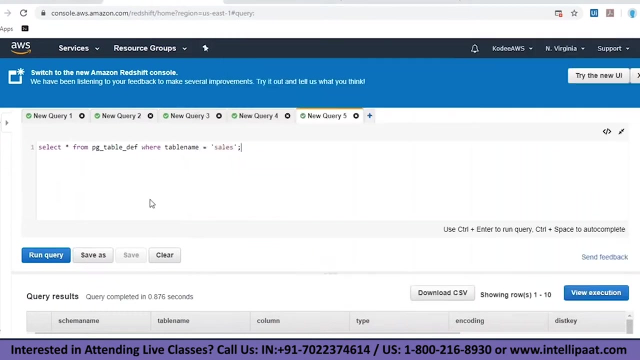 file and view it and that's it. and then another query: select some this from sales date, where sales dot date ID is equal to date dot date ID. so they are just doing that and calculating on the date. on this date they are calculating the sum of quantity sold. so now when I run, 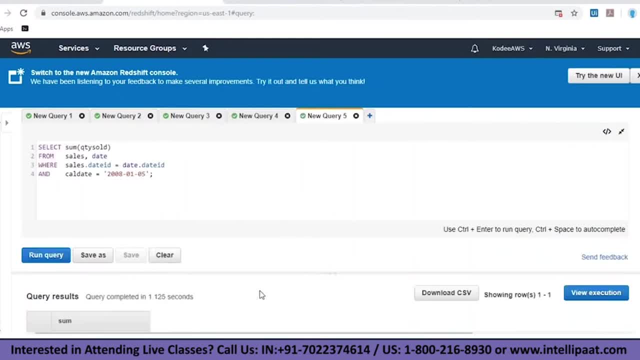 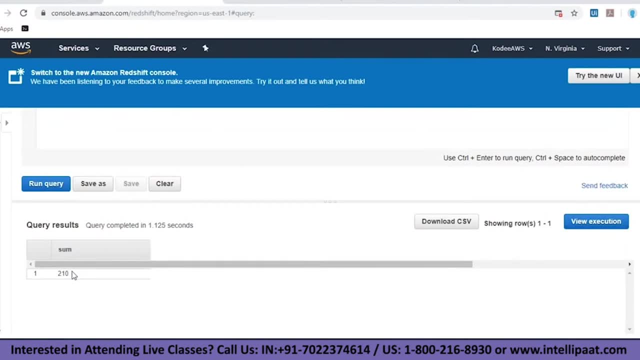 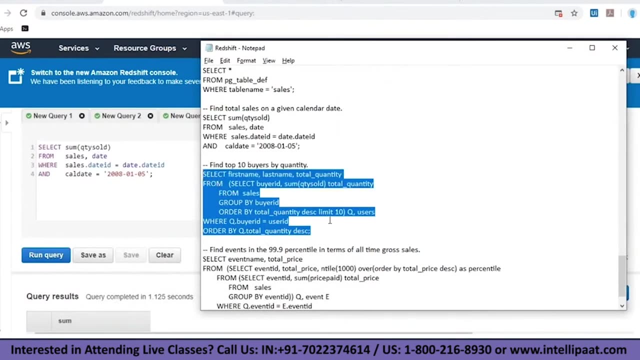 this query, I should get a number of some. so yes, so we've got that number, so that is the only result we get, because that is the only result we needed. so this is one query, and then and then there is this: so here they've provided the limit. 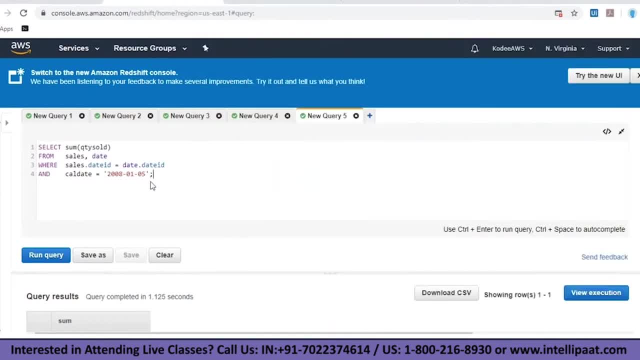 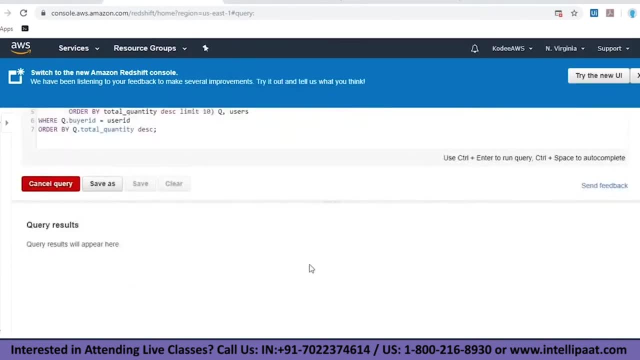 as 10. okay, so, so here they've provided the limit as 10. okay, so so. so we'll get 10 rows of output, so showing rows 1 to 10, so you can see first name, last name, total quantity. they have provided the name and last name. 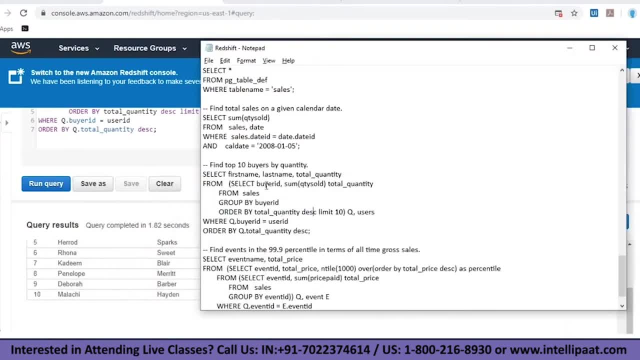 and the total quantity. so that's what mentioned here: select buyer ID, some quantity sold, total quantity from sales group by buyer ID. cube from sales community for sales trade: sure, so this particular way to know share is that you forecast. complete the current rate by feature on the. 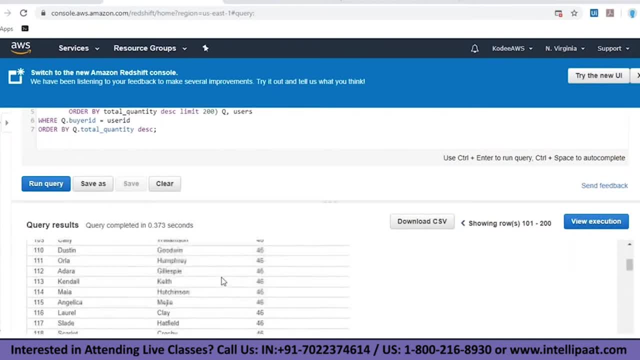 physical order by total quantity limit. so we just change this limit to 200. I will just change this limit to 100. I could have just changed here. so they could have just changed here. so they provided 100 rows here and then another hundred rows in the next column. so I think hundred rows is the limit for one. 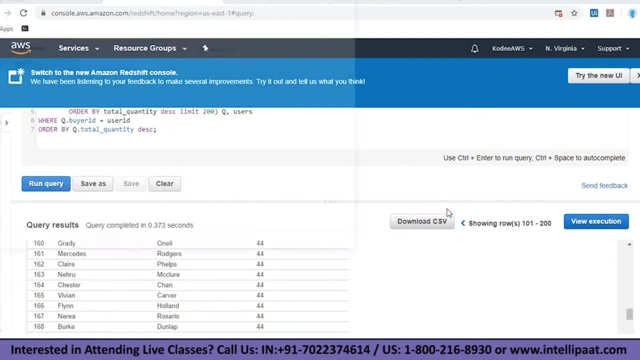 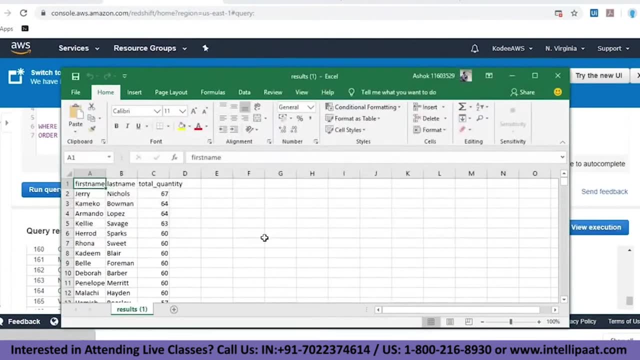 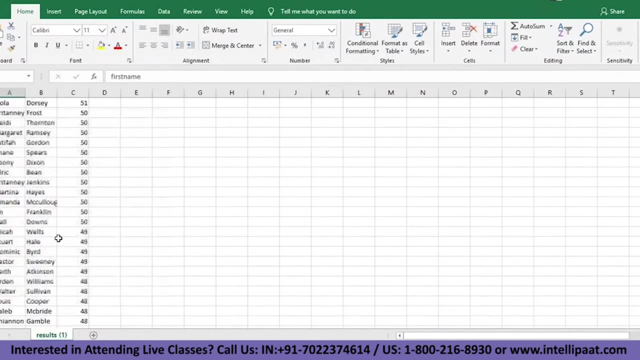 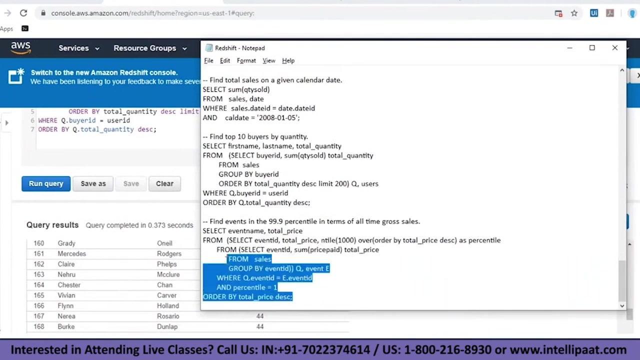 counted that. so these things change the term like this here. so if you are able to Result column and you can also download this entire CV CSV file and just look at the results for yourselves. Yes, So they have provided it here completely. Yeah, so this is one query. I'm just doing some sample queries to show how it works. so then select. 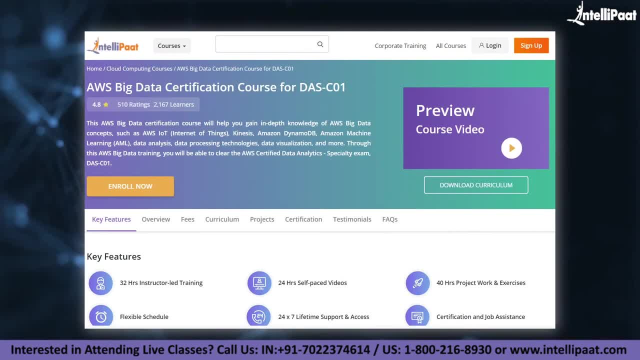 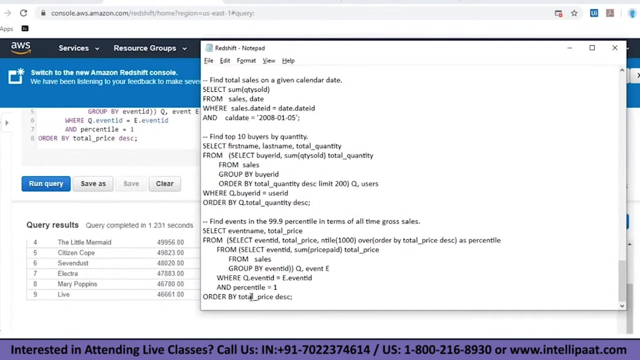 You Just a quick info, guys. Intel iPad provides AWS big data certification codes Mentored by industry experts, the course link of which is given in the description below. Now let's continue with the session. And again another query. same thing, so here, So that that you can see the query results are faster. 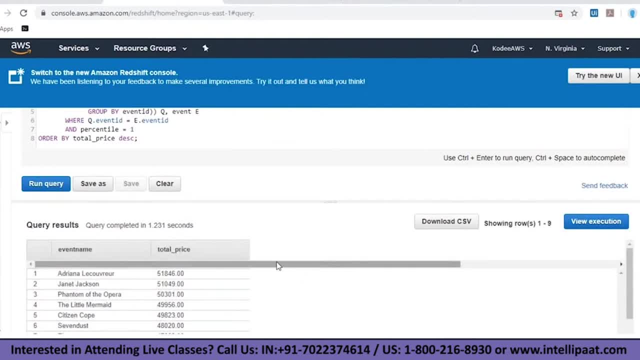 Even though there is. There is not a lot of data, but still we can consider. but when there is really a large amount of data And you want to query some results, they happen very fast because, as I told you, that's what, that's how a Redshift has been. 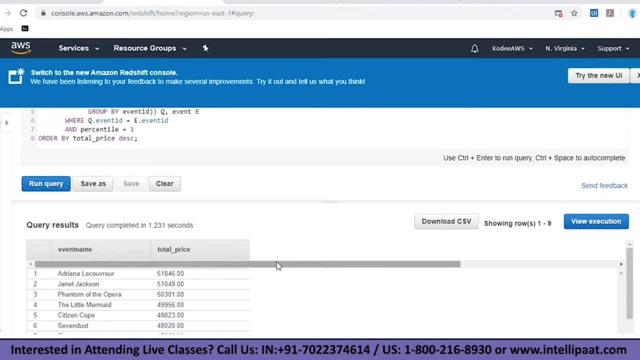 Architectured. it has one leader node and a multiple compute nodes which distributes the workload and accordingly complex queries are Divided into simpler queries and they are executed and the results are clubbed In later node and that final aggregation is sent to the client tools. So 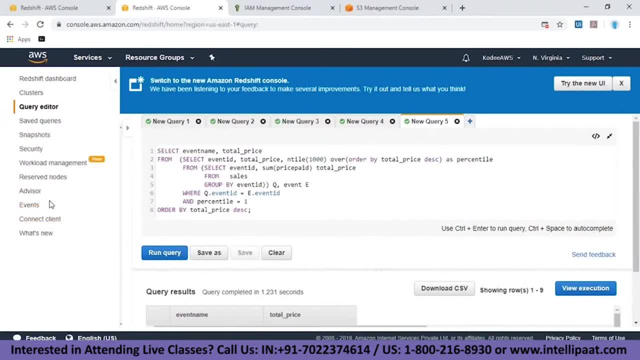 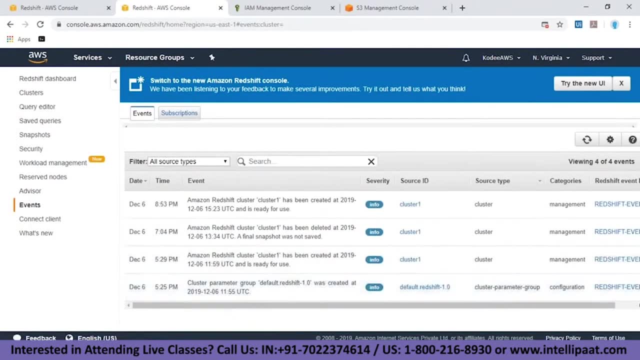 Yeah, so we've done. query editor also. Then the one more thing: I'll just show events and after events We'll see the monitoring part of this and then I think we will be able to do the cross-region replication of Aurora. We'll do that And yeah, so we'll do that. 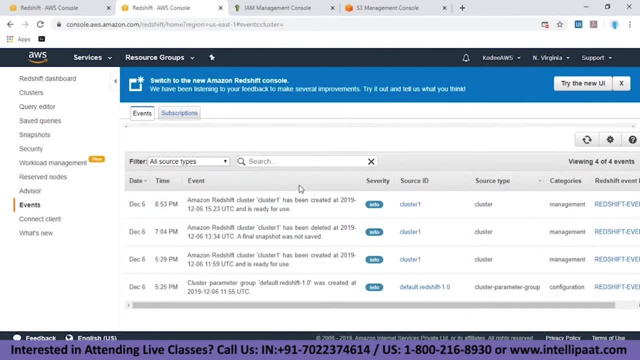 and one more. one question about. I am database authentication in the last session, so I tried. so basically, instead of: you'll not be able to assign roles to your on-prem setup, but you'll. you can use secret and secret access key and your access key to. 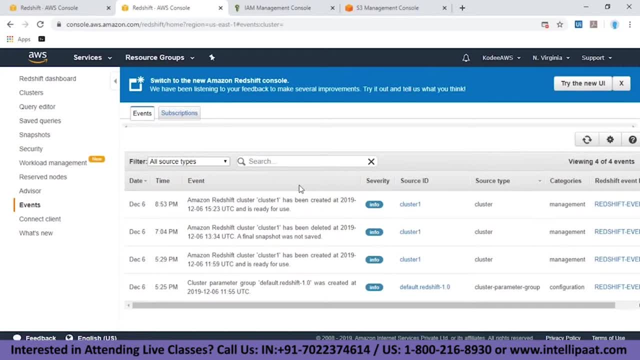 Authenticate. for that particular I am users. You can provide programmatic access and those users can use their secret and access keys to enable I am database authentication. But you can only use that for RDS instances, RDS databases, because only there you will be able to enable. 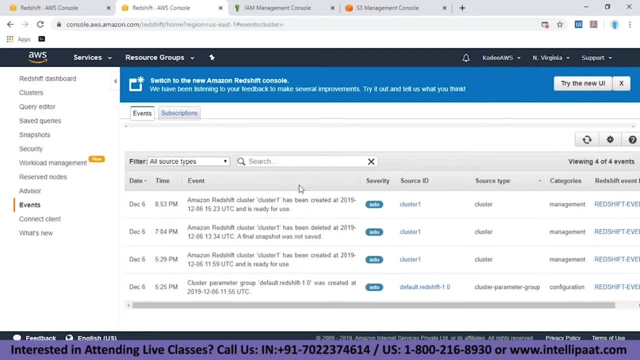 it. after that you can just use that endpoint and, Yeah, you can use the security credentials to login, but you'll not be able to use- I am database authentication on your server, But you'll be able to use- What is that, your secret access key and access key and also the token, and do that. so that is the only option. 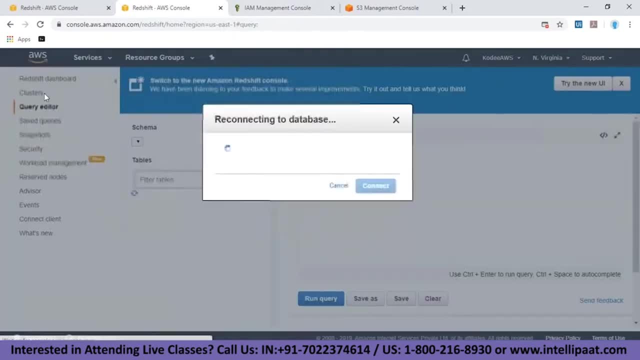 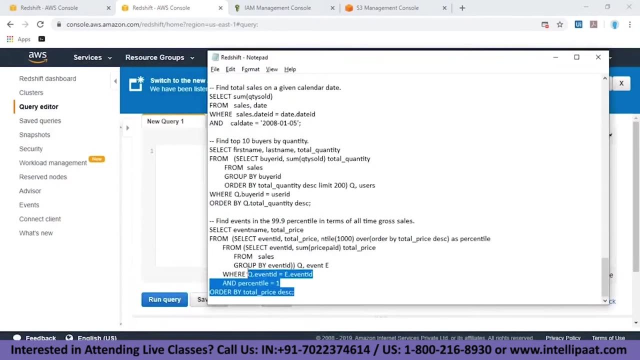 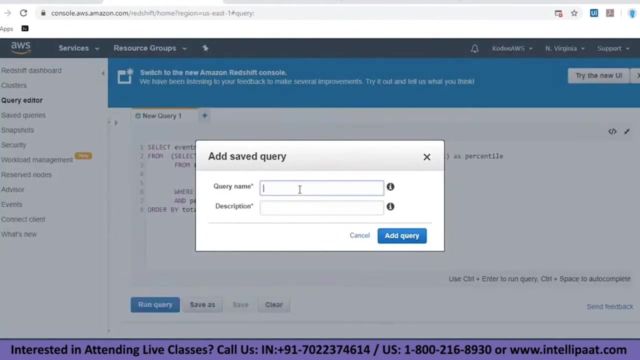 Okay. so now coming back here, so saved query. so Coming back to the query editor, I forgot to show one thing. So, for example, If you think you'll run this query often so you can just save it here, You just save it here. provide a query name. Let's say this is- I don't even know what query is this. 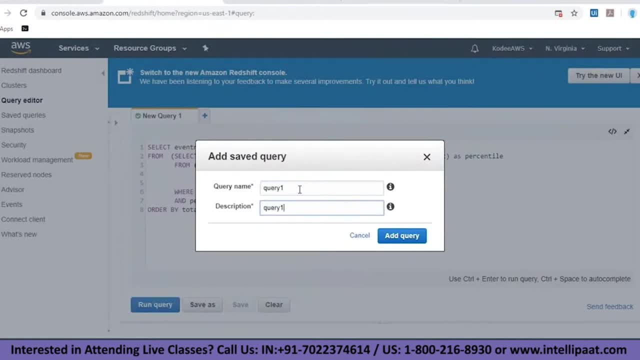 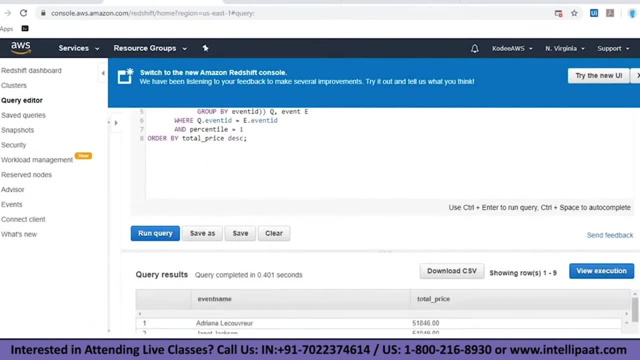 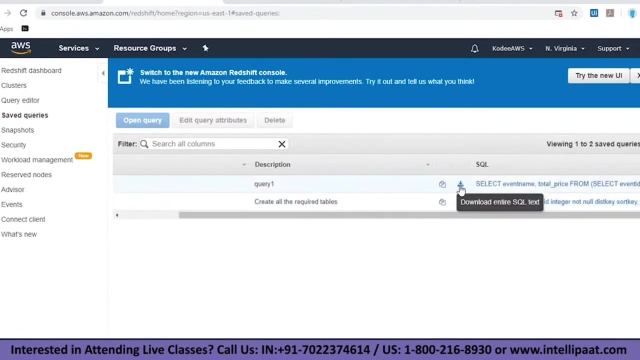 So I'll just give query one and again query one. Add query. so done. query is saved. Yeah, so so here. so now go to saved queries. so the saved query: Download. enter SQL a text so you can download this queries SQL text. or you can copy the entire SQL text and just if I just paste it here: 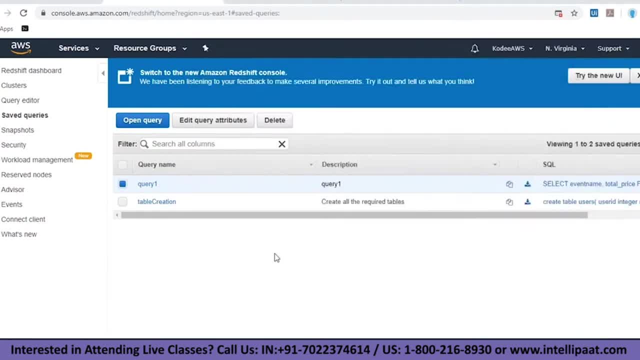 So we'll get it. So this is this pretty easy. You can just save your queries over here and get them whenever you need. So also, this is easy to control. You can just search what query you need accordingly and get it, And then, yeah, so this is pretty much saved queries, That's it. 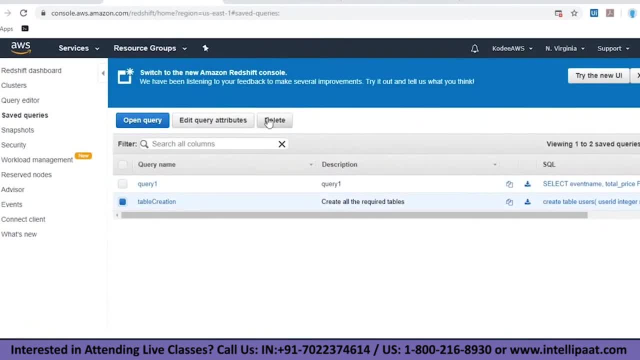 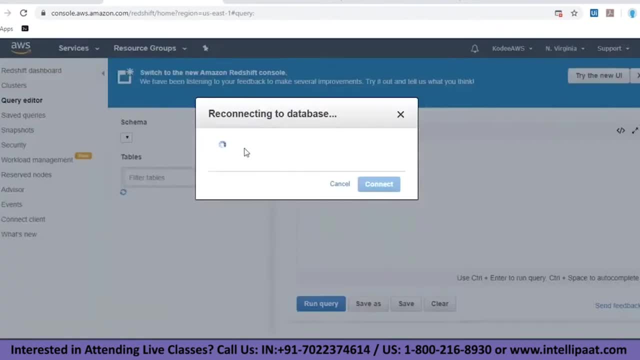 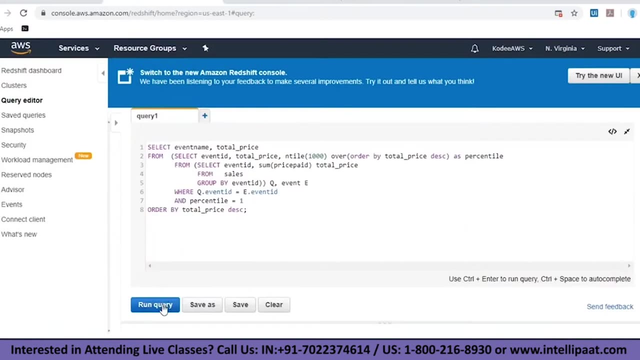 So that is for changing query attributes and also you can delete them whenever you need. just that's it. Yeah, So I think you'll not be able to. So you can also open that query in your query editor and after opening that query into the query editor, you can run. 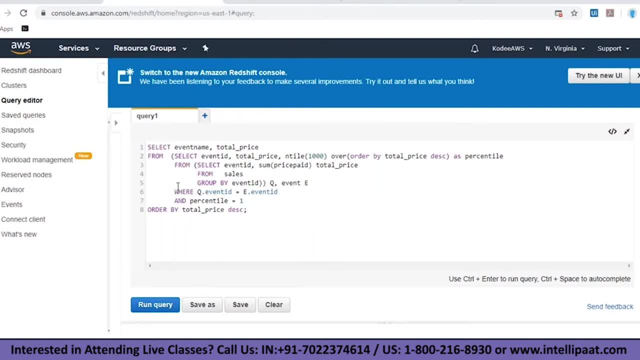 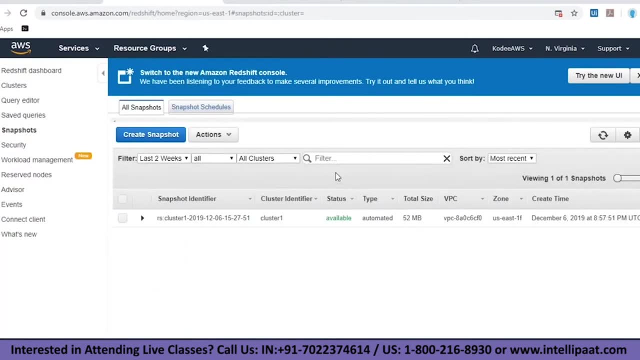 directly from here. you don't need to copy that and paste it over here and Do it, and you can. this is also one of the options. and then snapshots: Again, snapshot does the same thing and you can see here: an automated snapshot of 52 MB has been collected. 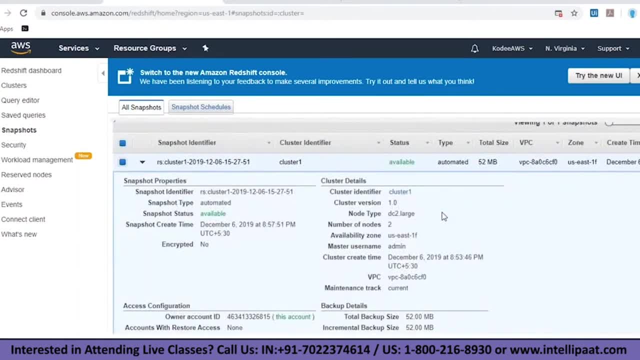 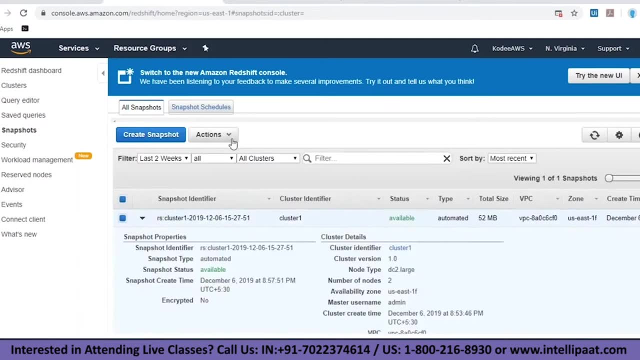 So this is for my cluster one. So now, at this point of time, if I want to restore my cluster, I can use this snapshot and restore this particular cluster directly from my snapshot at this particular point of time and it will Provide me the entire architecture, the end, same cluster, if you have two nodes. 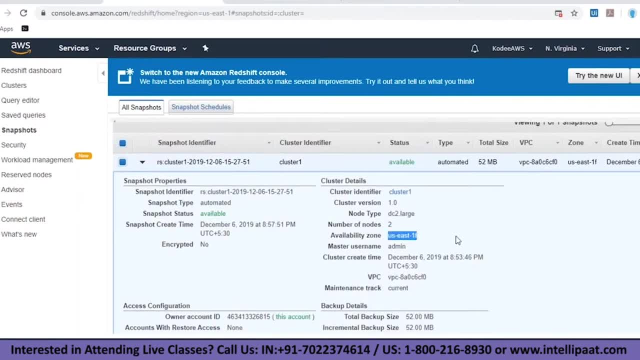 So you can see here the cluster details. two nodes: availability zone F. I don't know whether it provides in the same availability zone, if maybe the availability zone is not available, That's, that's the reason why you are trying to restore it. But it will provide. you can choose the availability zone while creating the cluster and you can see, you can choose the node type. 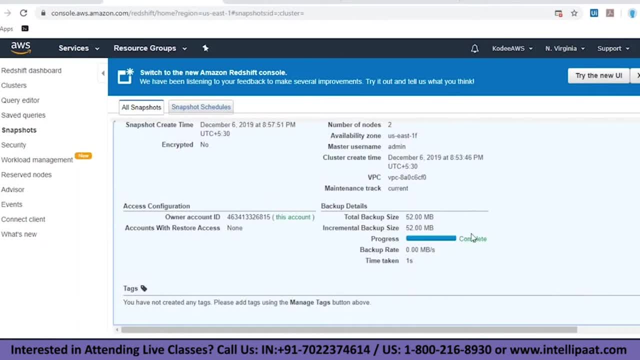 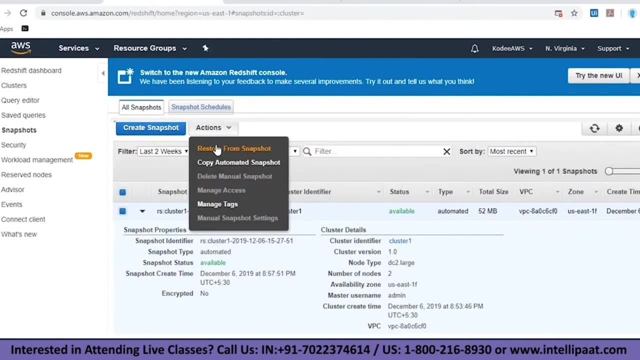 you can choose the number of nodes and everything. progress is a hundred percent completed and Yeah, so This is much time taken. one second. It took just one second to do this, So whatever. So now we can just Restore from a snapshot. if you click that, you'll get these options. 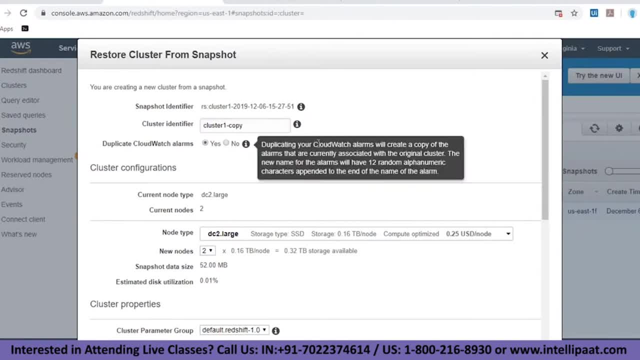 Cluster identify, you'll have to provide it if you have any cloud watch alarms already associated with your Existing or a chip cluster. if it is available, just provide yes. it will duplicate all of them. if you do not have a, You don't need to provide yes or so just provide no. it will not check for any cloud watch alarms. 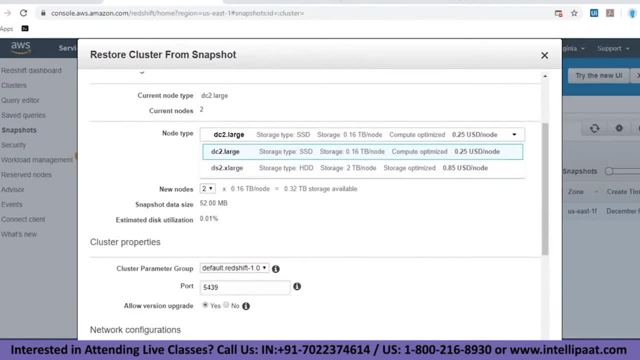 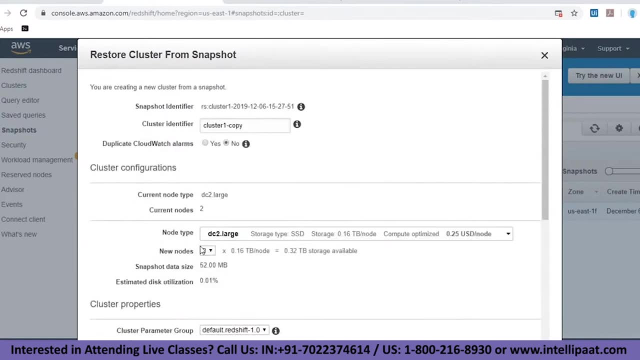 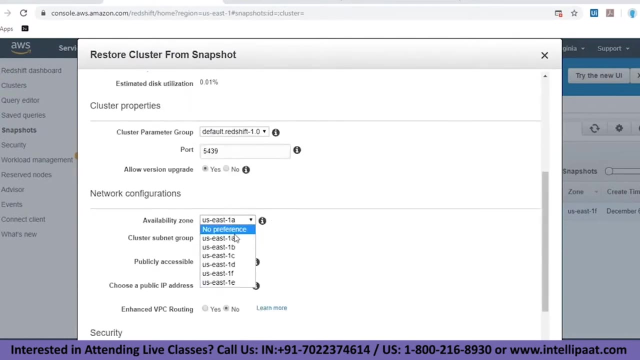 This will save some time. and then you can choose The node type. here you can choose the number of new nodes, so they only provide few options. snapshot size is 52 MB. You can choose the region over here: Cluster node- everything is taken default, So VPC. 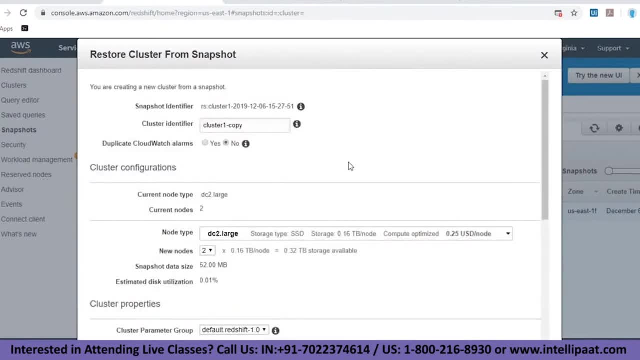 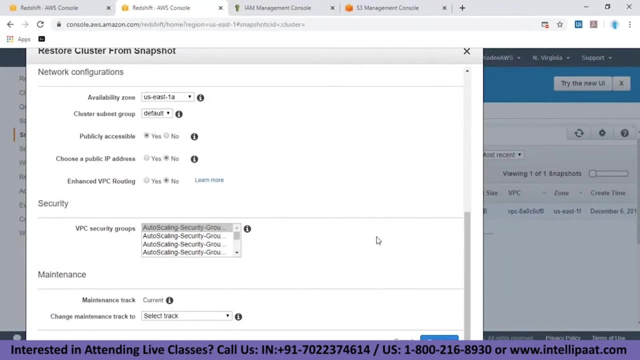 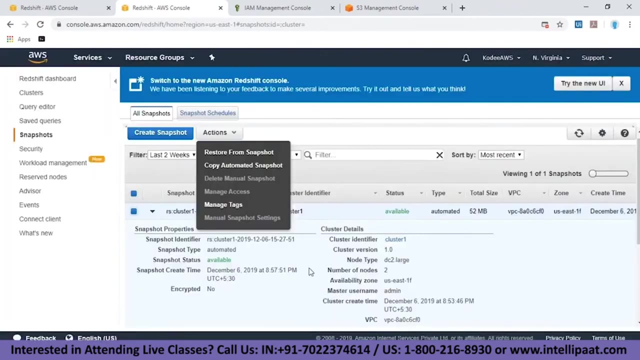 Group select track. it's going to be current. So, yeah, everything is fine. So this is more than enough. So restore is over here. so this is more than enough to restore your cluster. so just click on restore, let's see. Yeah, so done. so one more thing. 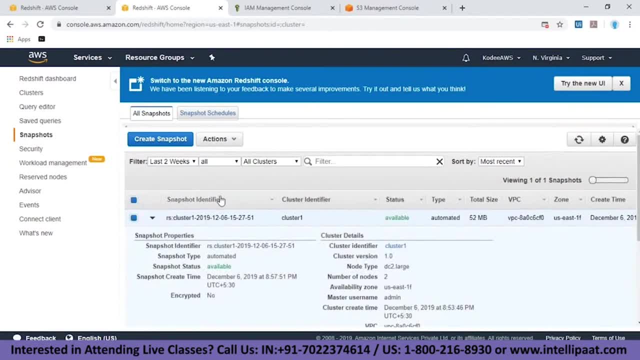 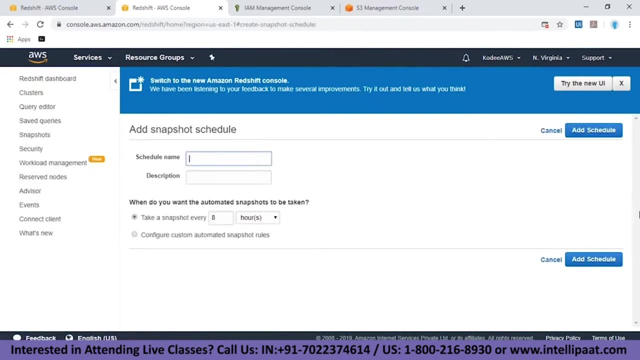 For this? Yeah, I think I. you can also add a snapshot as a schedule so you can provide a name. so let's say a snapshot One and provide a description and then Take snapshot every eight hours or eight minutes or one minute or whatever you want to. so I'll just provide a�vo gods. Configure custom automated snapshot. So take snapshot every 8th hour, 8 am To 8 pm. So take snapshot every weekend at every hour from 8 am To 8 pm. Take snapshot every week day at 12 am. 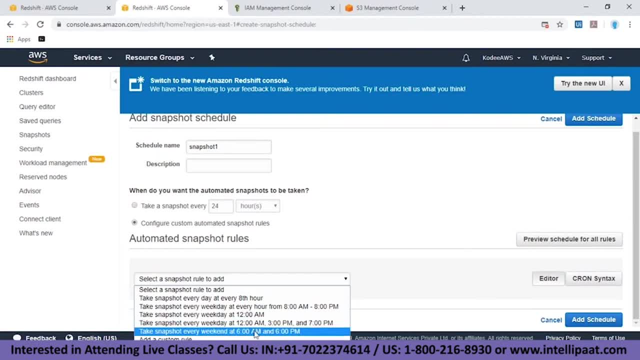 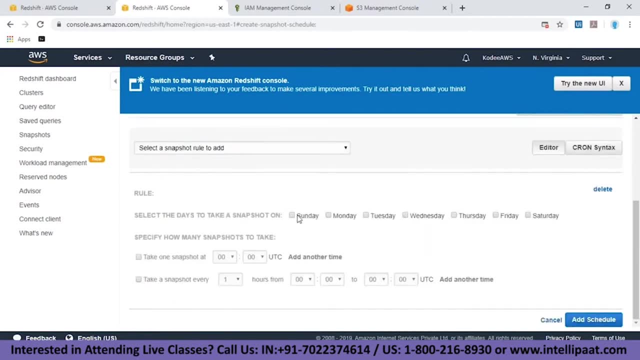 Take snapshot every weekday at 12 am, 3 pm And 7 pm. Take snapshot every weekend at 6 am And 6 pm. And also you can add a custom rule. So, custom rule: you can choose the number of days. 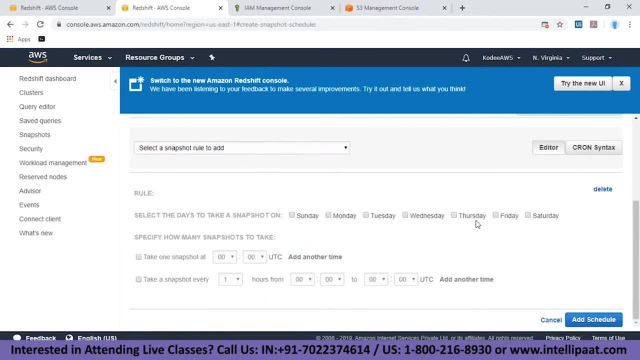 on which you will have to create a snapshot for and then after choosing the days and take one snapshot at. you can provide a time or take a snapshot at this particular time on all of these days. So this is UTC. You will have to look up to your time and UTC. 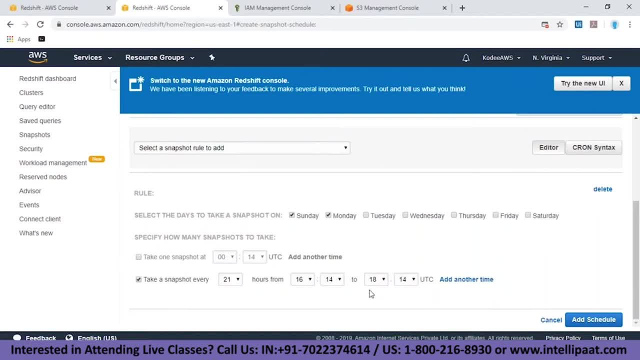 and then specify this. So this does not. so UTC is common, So you'll have to check for your country's timing with UTC and then provide this. so now, every Sunday and Monday at this time it takes, take a snapshot at every 21 hours from this time. 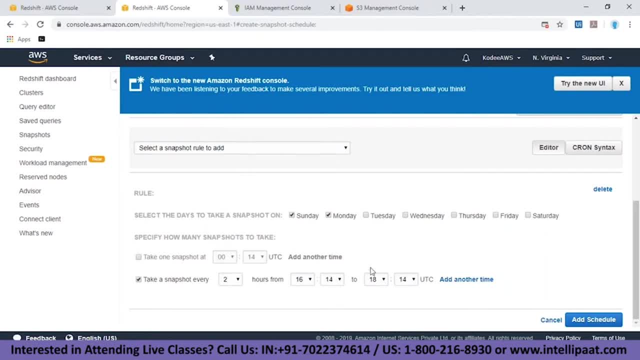 So I'll just make it do so every two hours from this time to this time, So from 4: 14 to 6: 14,. it will also basically create a, I think, Three snapshots here, one at 16: 14, 1 at 17 14, 18, 14.. 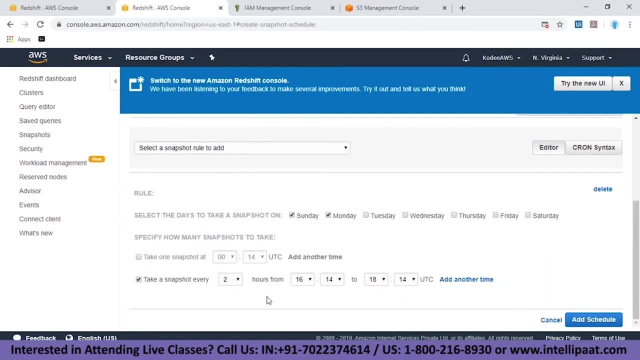 No, it's two hours from take a snapshot every two hours. So I think the it will create to. I don't know what exactly happens here, So if I provide one, so there will be take a snapshot every one hour. So everyone are in the sense. 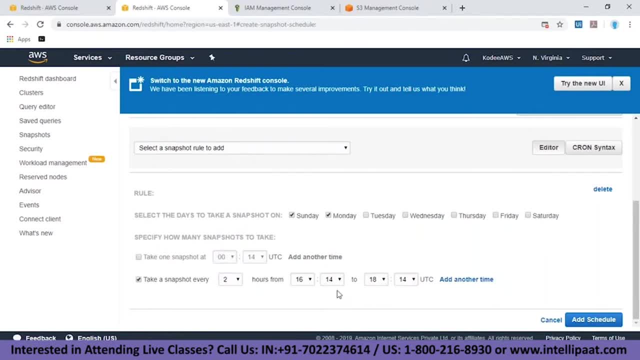 There will be three. two is confusing me. I'll have will have to test it out- Or how many it creates. So this I do not know. So the basic thing I want to say is: you can create a schedule. Also, you can create a custom rule. 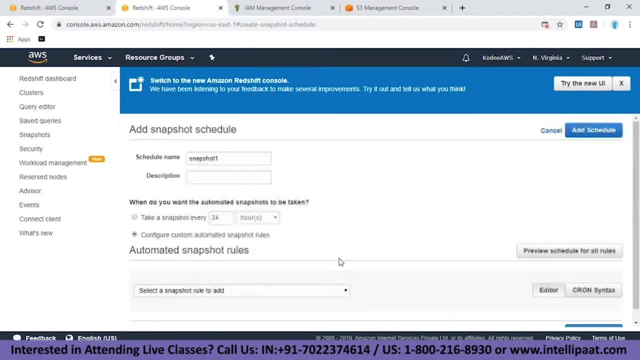 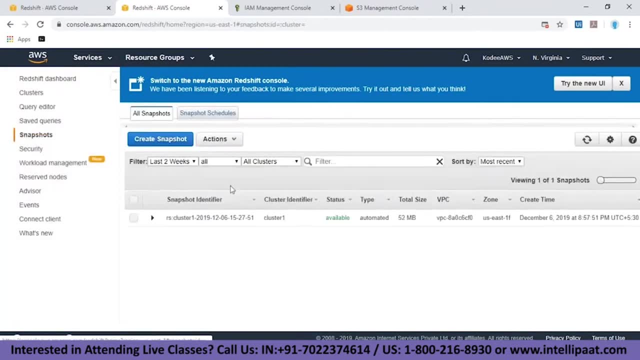 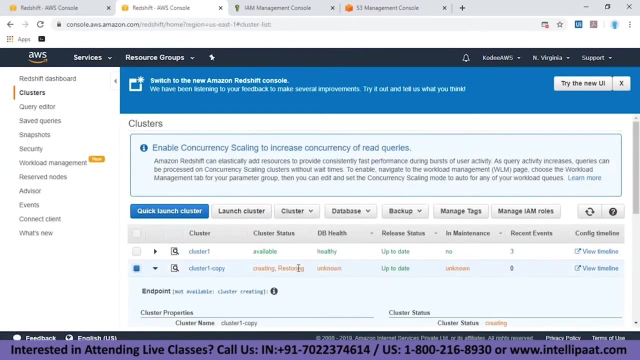 So that's how you do it. And then, so this is one so you can figure, configure this out and coming back. Okay, So now going back to clusters, so you can see here the cluster copy is creating and restoring. Yes, So before you continue, snapshot. 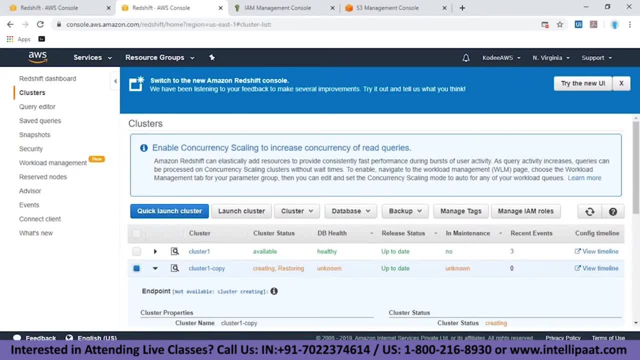 it's the way. a backup, right? Yeah, it's a backup, Okay, So does it take a full snapshot every time you run? Or it does It'll take a full snapshot at the current time. Okay, so that's not taking parts. 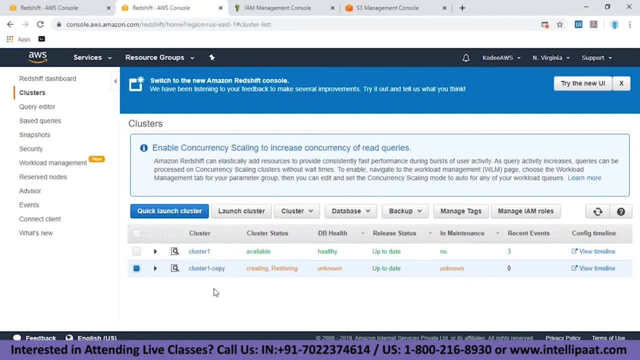 Yeah, Okay, So do you have approximately a size, like a estimate of size is, for example, if it's one terabyte of database? Yes, snapshot, does it back up all the files, or it's like the OS level of snapshots, not not to take the backup? 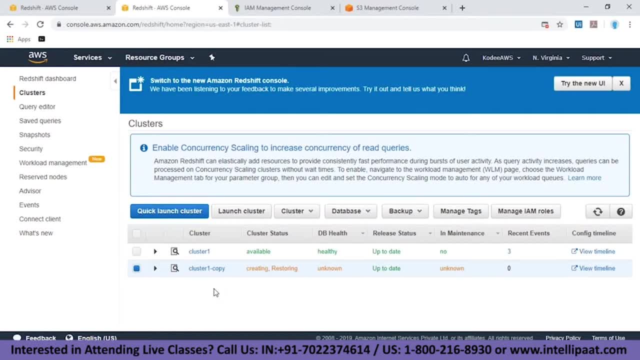 I don't understand what I mean, like the space optimized snapshot That's by West level. No, I think it takes all the data also, Because it was 52 MB and yeah, so I. it takes all the data And it stores in S3.. 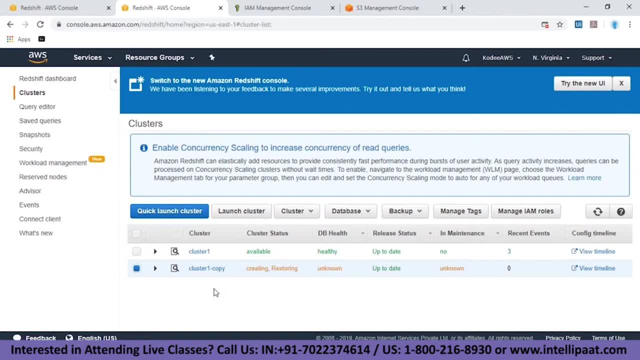 I think you get, so let's check that also. I would assume there's a retention. I don't didn't see that part like to allow you to specify how many snapshots you want to retain, Okay, so I think sort of it is custom. 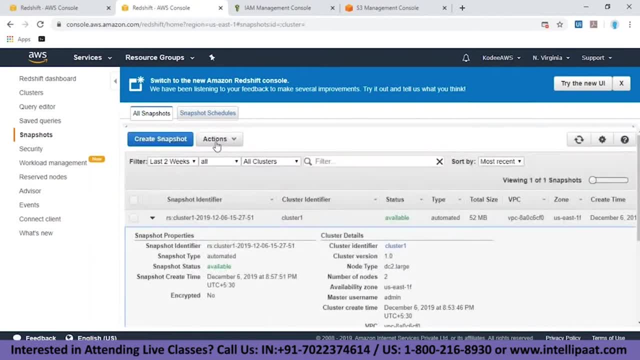 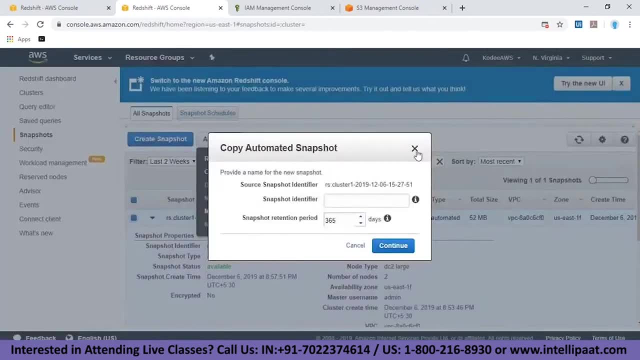 Automated. This is automated. Automated retention time. Second, I'll just snapshot retention period. Okay, it's over here. The number of days for which the manual snapshot will be retained. setting this parameter to minus one days retains the snapshot indefinitely. So, basically, if you have a snapshot, 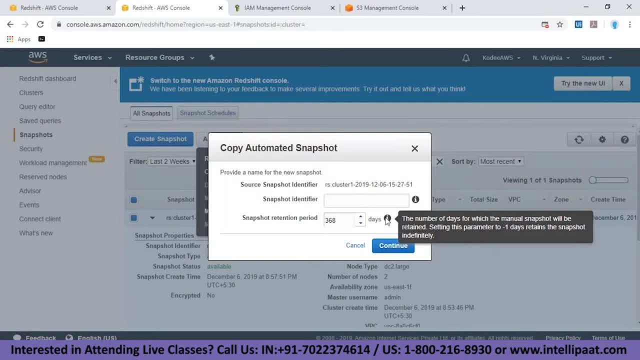 you can create a copy of it or like while creating the snapshot. I think you can provide this. So if this is minus one, then you can store this indefinitely until whenever you want. So then, after creating that snapshot, you can delete the existing snapshot. 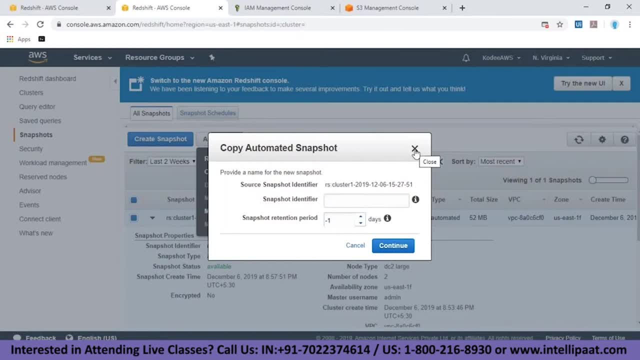 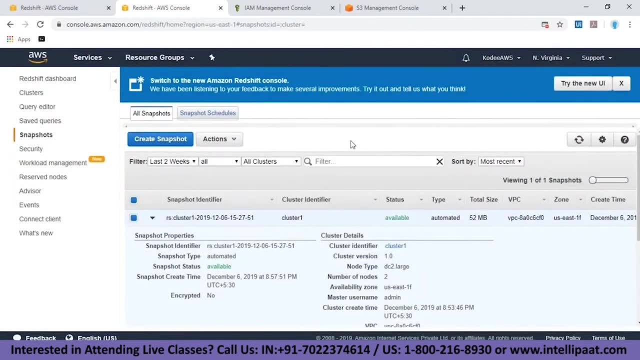 This is the copy. So I think: yeah, AWS chart this. do they charge you by storage to? Yeah, it is the S3 storage charge. backups are stored on S3. So you'll have to check how much data is stored. So, 52 MB. 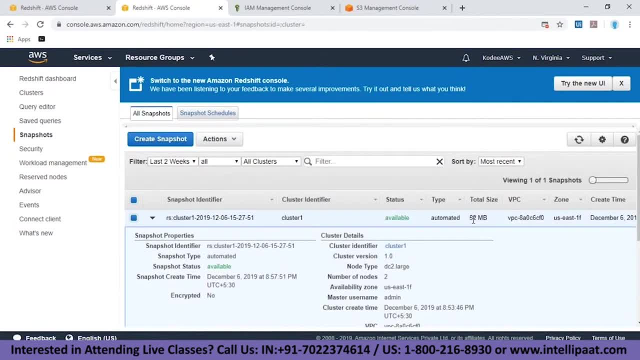 So if it is, for example, S3 provides you 5 GB of free tier storage every month. So if it goes beyond that, then you'll have to check. according to, S3 is on-demand storage costs, So all the backups, all the snapshots are stored in S3.. 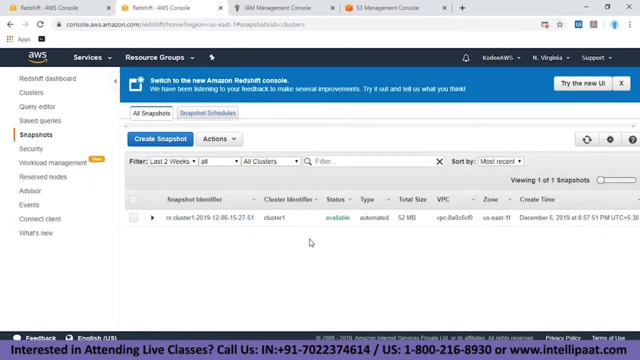 So you'll get charged if you go above 5 GB every month. So you know it's not a big deal. So you'll not be charged for that first 5 GB, Then after that you'll be charged according to S3 sir. 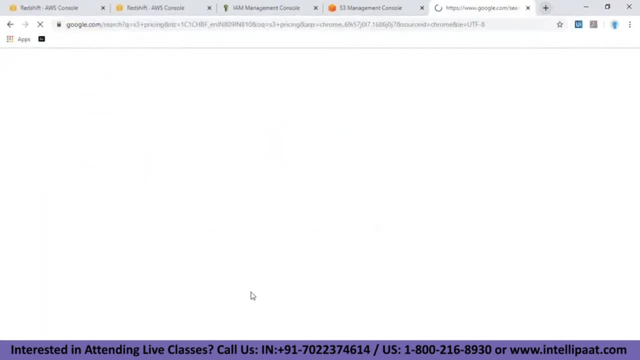 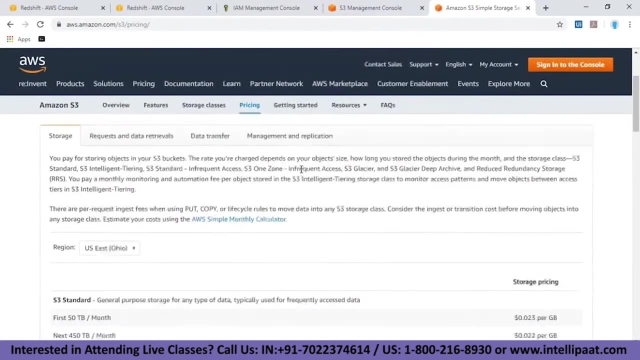 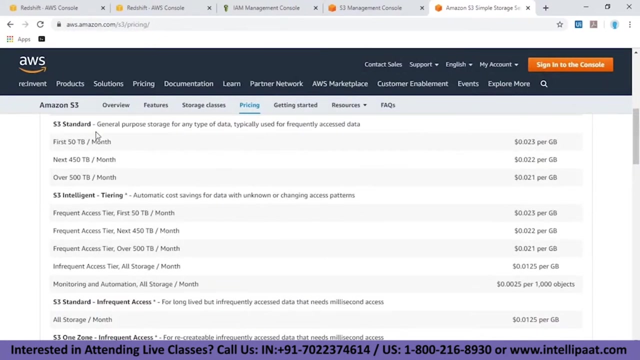 So let us check S3 pricing them. So because that is where all the snapshots are stored and that is important Storage. So yeah, for storage first, 50 TB per month is just for standard. So there are also storage classes in S3 for standard storage class. 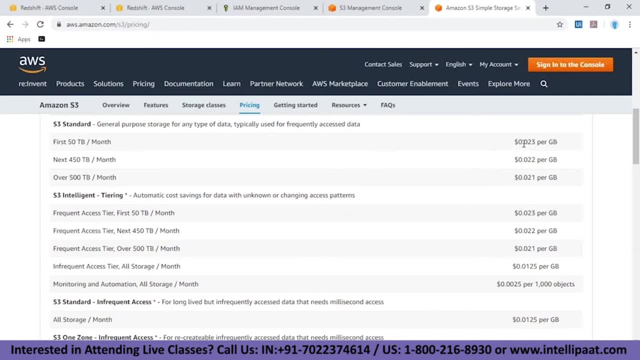 That is basically frequently accessed data. So for that it is a point zero, two, three dollars per GB. So so 50 TB. so you'll have to calculate it accordingly how much, and then for 450, for next 450 TB, It's point zero, two, two per GB and next 500 TB. 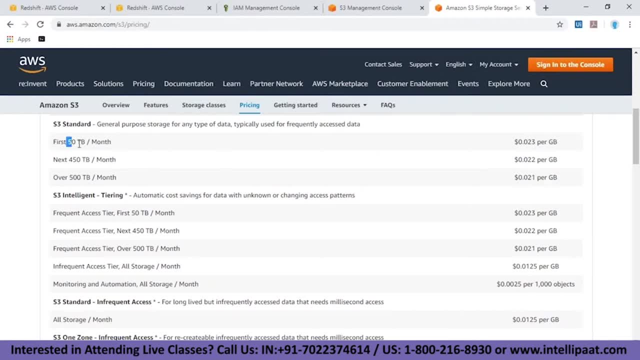 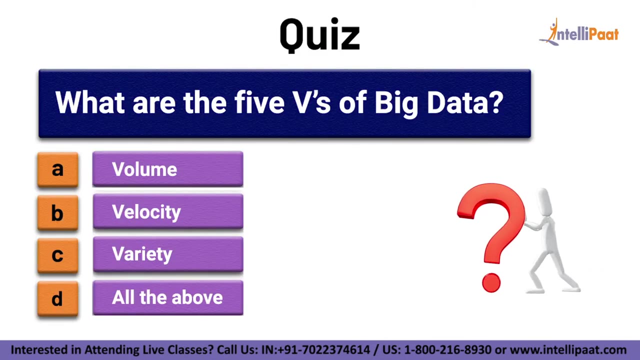 It's a point zero, two, one per GB. So basically the first 5 GB you won't get charged. after that, for every GB, you will get charged up to point two, three dollars. point zero, two, three Dollars. just a quick info, guys, test your knowledge of big data by answering this question. 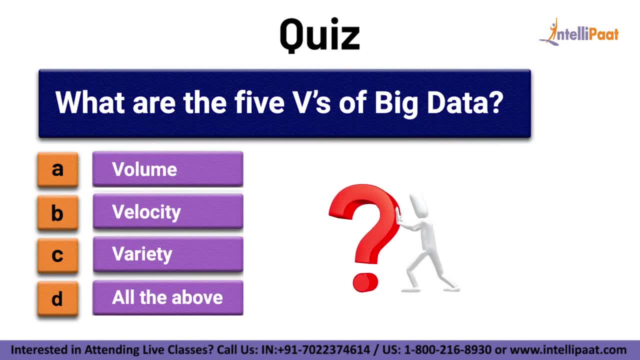 What are the five V's of big data? A, volume, B, velocity, C, variety D. all of the above. Comment your answer in the comment section below. Subscribe to Intellipaat. know the right answer? Now let's continue with the session. 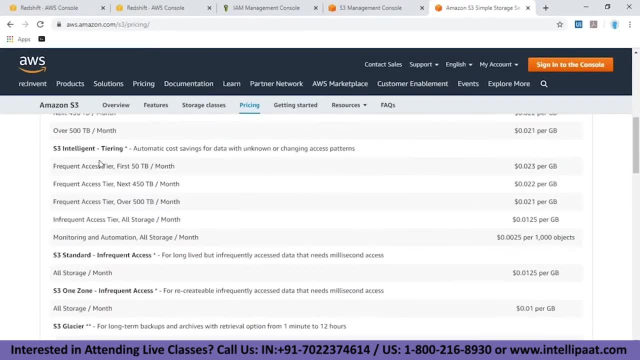 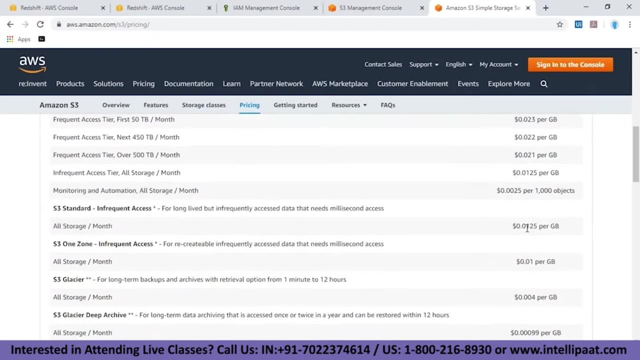 Up to 50 TB. then for other classes also the same. for S3, intelligent tearing, you get point zero, two, three, again for infrequent access, It is point zero one to five. So if you're not using your data that much, if it is just accessed once in a month, 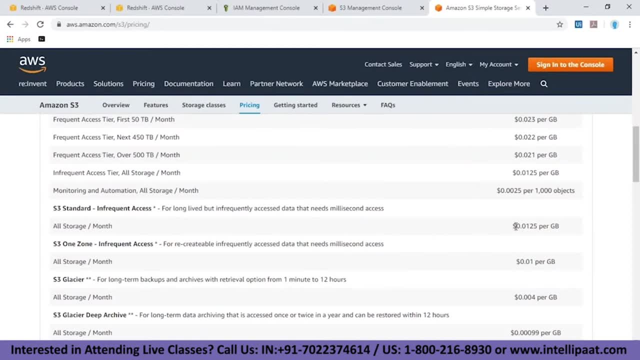 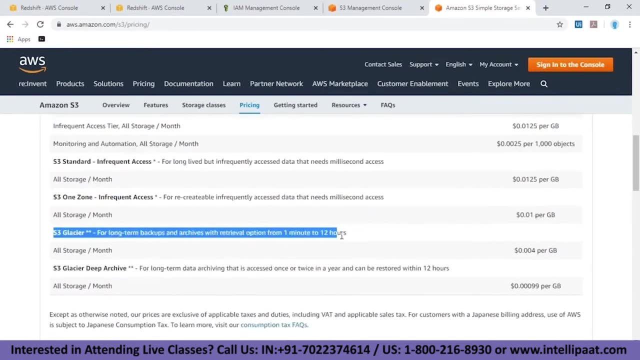 or something like that. then you can store in infrequent access. So this is for storage here, but backups- I think for long-term backups- S3 glacier will be taken By and it's very cheap. So it's a point zero zero four dollars per GB all storage per month. 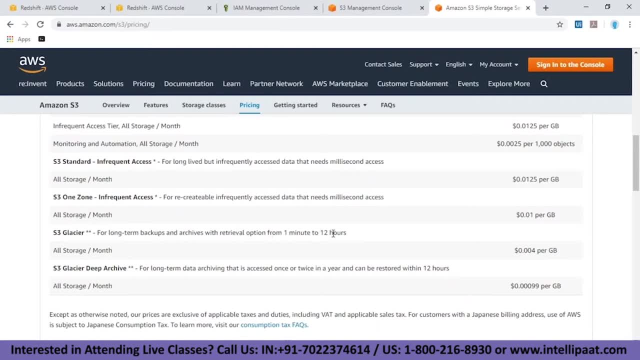 For long-term backups and archivals option from one minute to 12 hours. Okay, Long-term backups and archives within a retrieval option If your retrieval option for that data is within one minute to 12 hours. If you want to retrieve all the data within 12 hours, 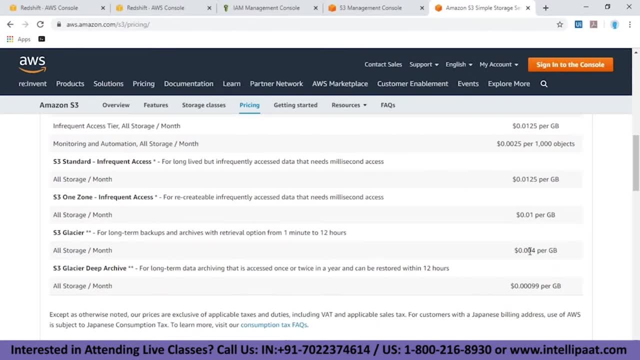 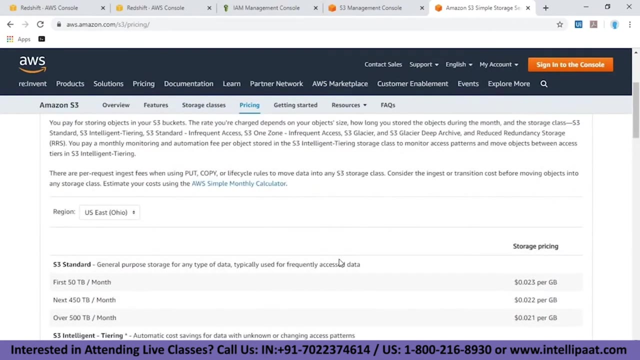 then you get charged point zero zero four GB. point Zero zero four dollars per GB for S3 Glacier. So S3 Glacier is the storage class for any kind of backup, for long-term backup. Yeah, so that's it. So these are these charges are for you storing it here. 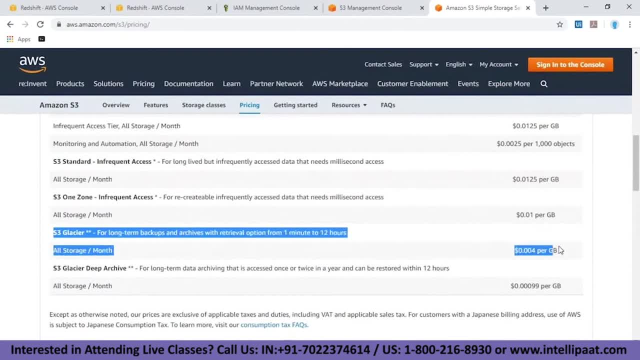 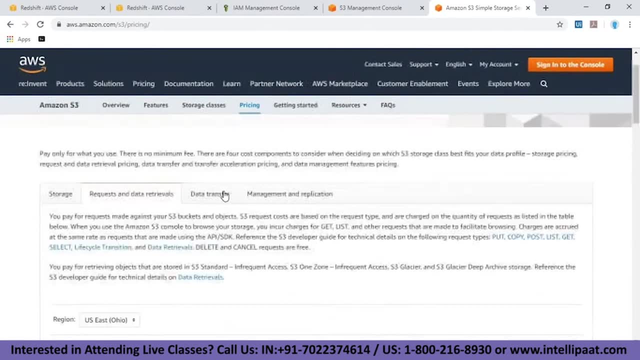 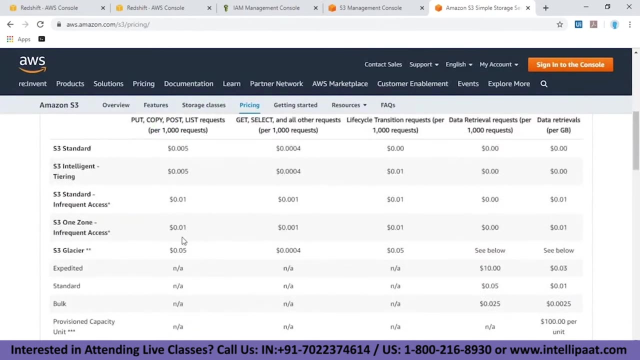 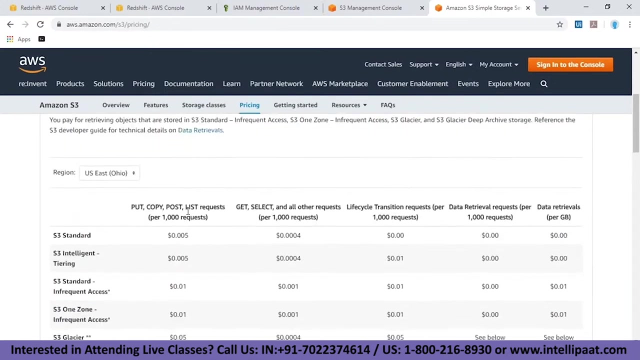 These charges. this is for backup. And then what else? this for requests and data retrieval. Yeah, so if you want to retrieve data, so for up to thousand requests of retrieval it costs point zero five. then This is for put for storing data. 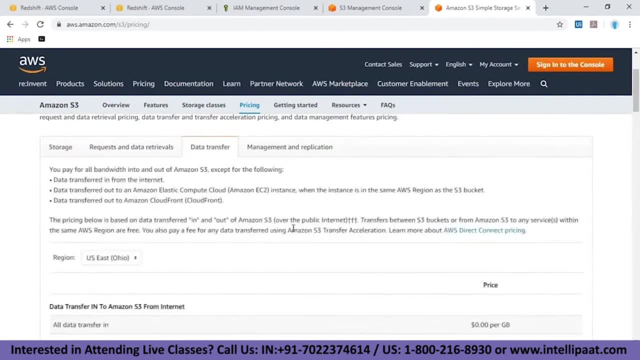 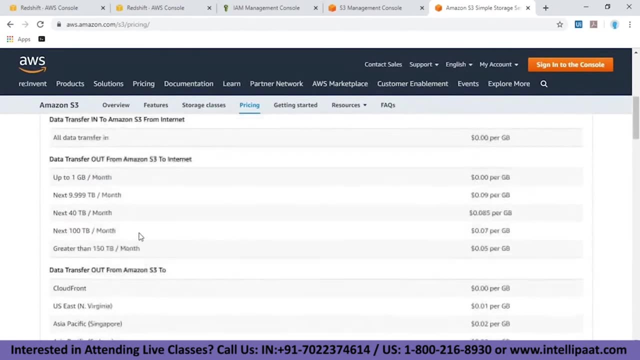 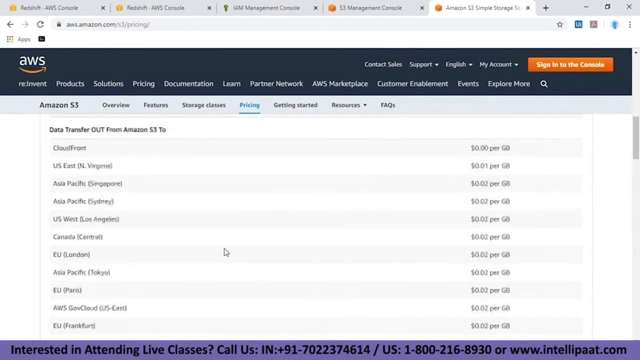 This is for getting. yeah, So for this. also in data transfer, this is data transfer in data transfer out. Yeah, so there are various concerns here. So basically you'll have to check for Glacier everywhere. These are for. these are common for all S3 storage. 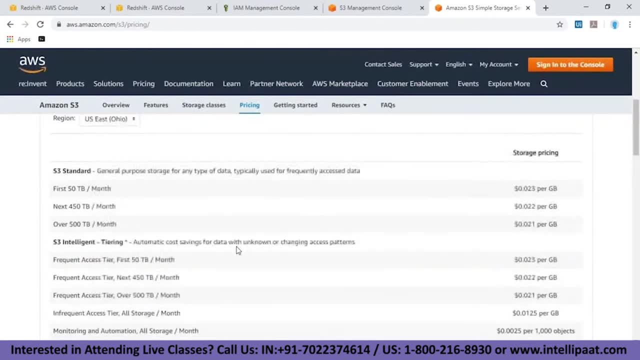 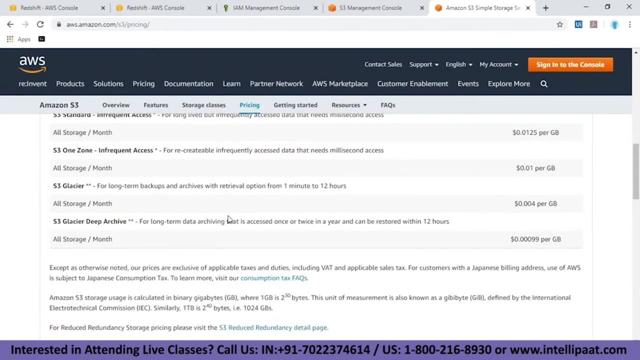 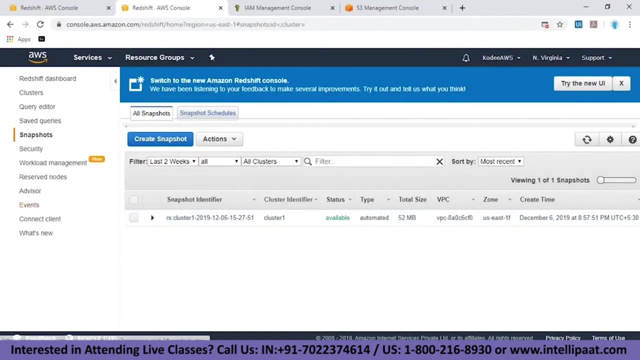 Classes. So the main pricing is here for storage, for storing your data. It is point zero zero, four dollars per GB for any number of storage per month. Okay, So now we are at snapshots, Then, yeah, snapshot schedules And then going to going back to cluster. 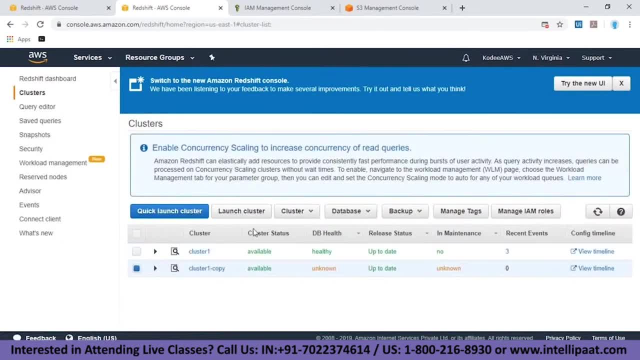 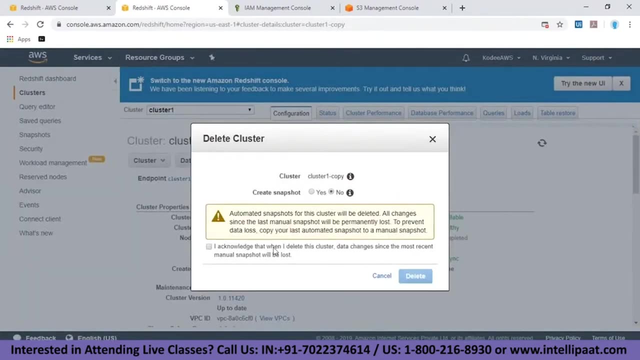 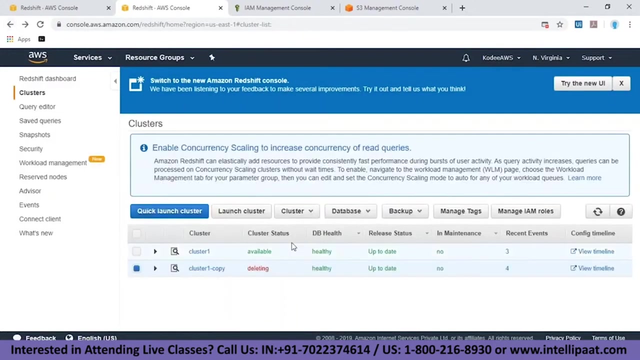 So, yeah, the even this is available right now, but I'll delete this. Yeah, so it has to be available. Delete cluster. I don't need a snapshot. delete, Yeah, Okay, so this was the restored copy of this cluster. 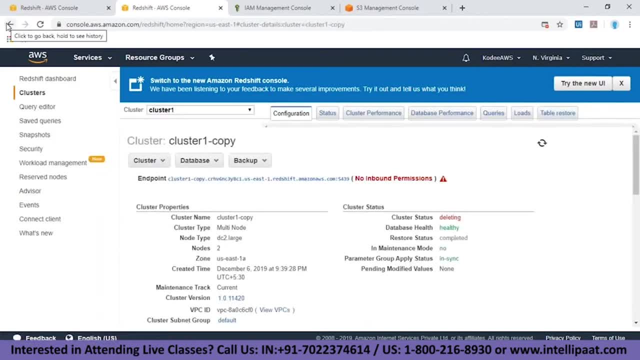 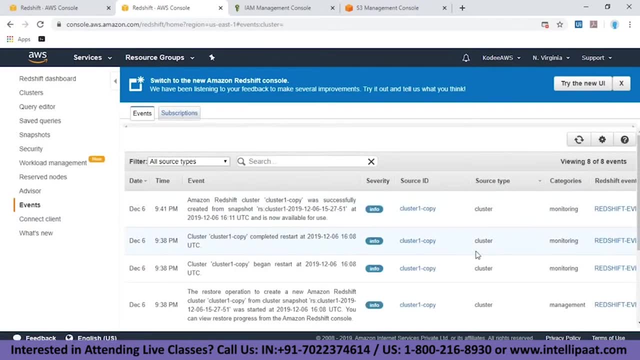 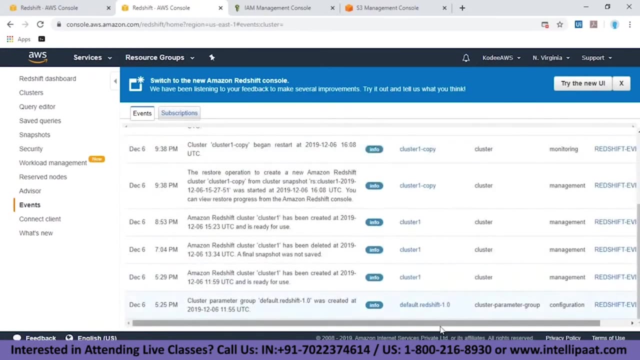 So yeah, so I deleted it done. Okay, So now we'll see events And then we'll go ahead and do the cross-region replication for Aurora. So events, events are the same for all kind of aw services. even here It is: see here. 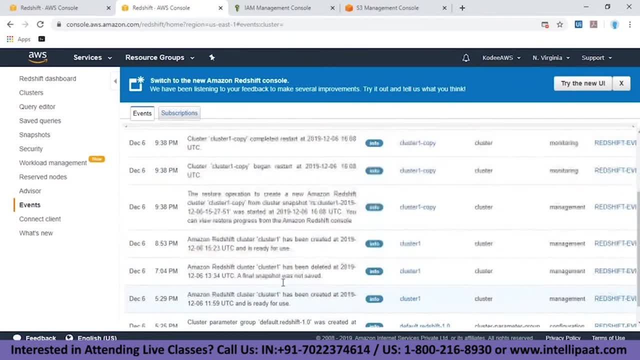 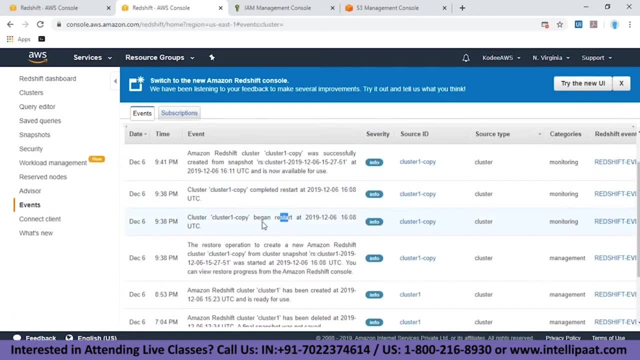 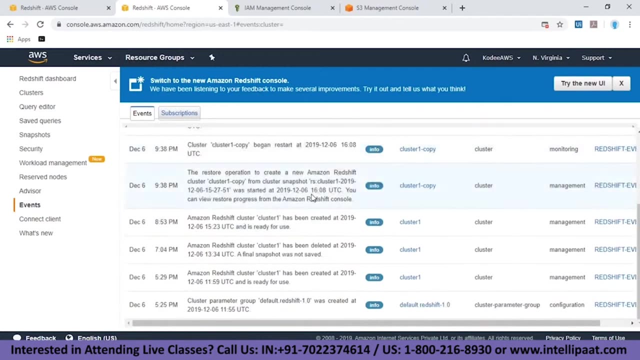 You can see the event numbers and here you can see what kind of an event It is: cluster copy one. then restart began, restart completed, restart was successfully create, created. So there are, these are various events, and again, here also you can subscribe, you can create a subscription event. 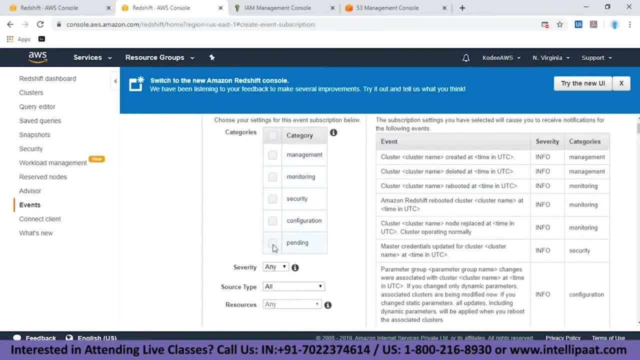 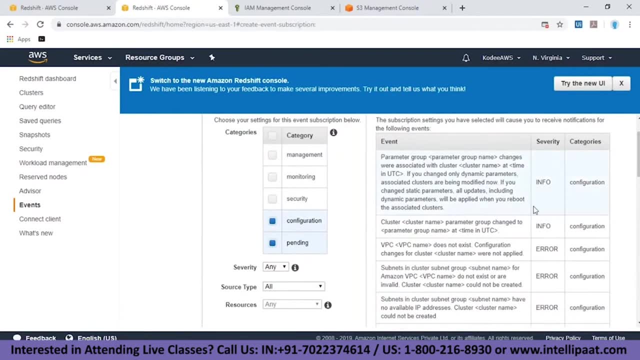 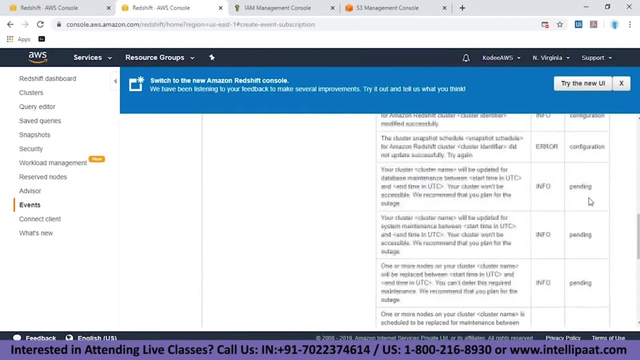 Choose the category. you can choose everything or just a particular thing, appending. So for pending, these four are the category. So these four events you will get to mail for configuration, for info or error or info. So these kind of configuration and pending, and so we've selected pending. 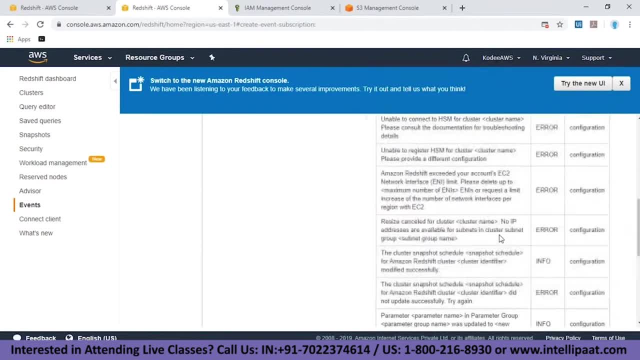 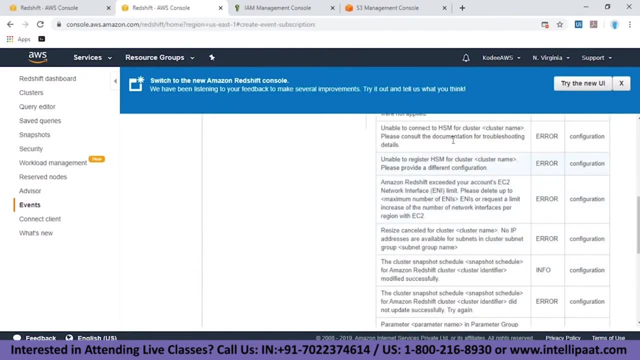 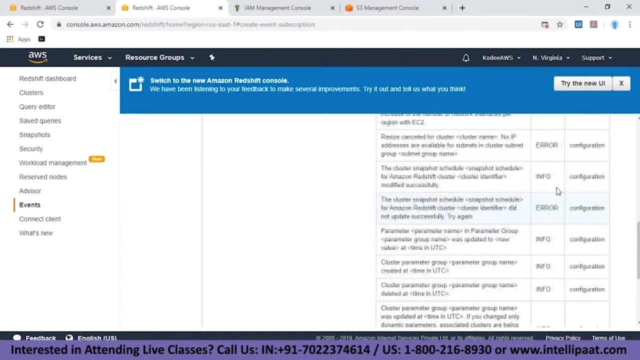 Also, so it's showing pending. So for all configuration categories. so that is a info errors, multiple errors And then yeah, so various errors and information. These are the events. for security It is can info error and for so it is for cluster security: security group deleted. security group- updated. security group created. 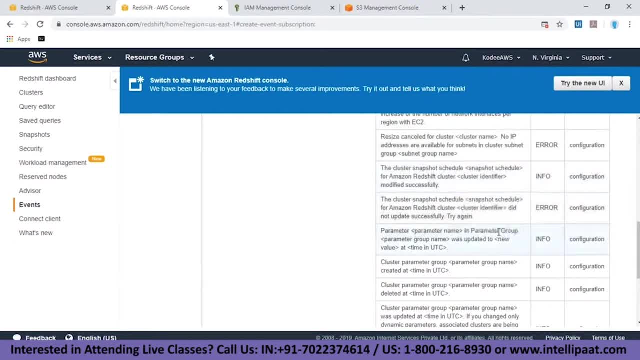 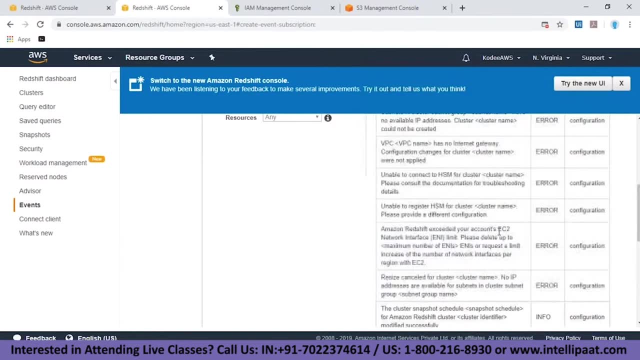 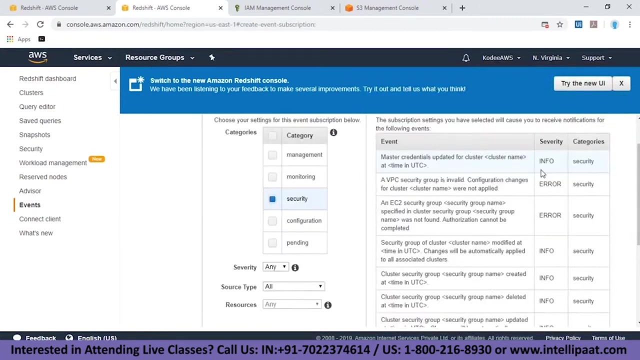 So these are for security, for monitoring, I think so. cluster rebooted, redshift rebooted. cluster node replaced. So whenever there is a node replaced, you also get an event so that AWS will. Oh, is my audio law? Yeah, it was my audio lost for some time. 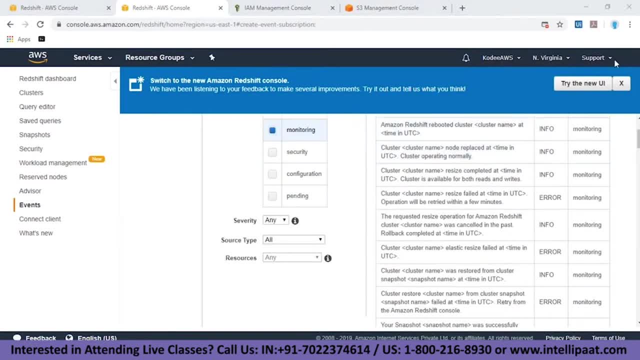 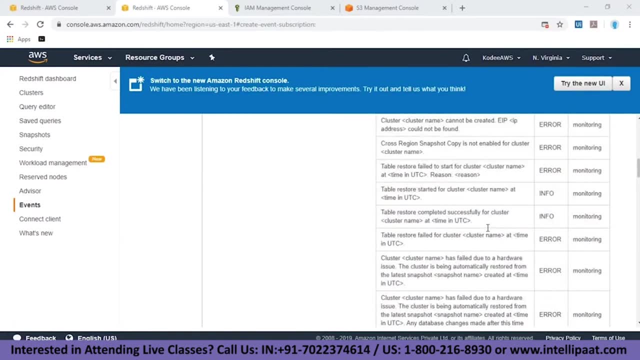 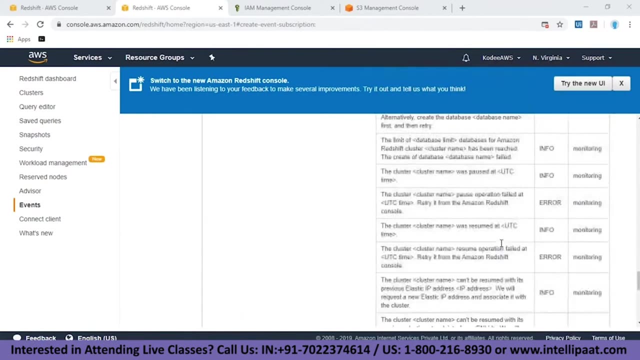 No, you're good. No, No, Okay, I was shown. audio was lost. Okay, I'll just continue. So for monitoring, Yeah, so there are various monitoring things. for monitoring, There are a lot of events because creation, deletion, failing, rebooting, then for alarms, for all kind of monitoring event. 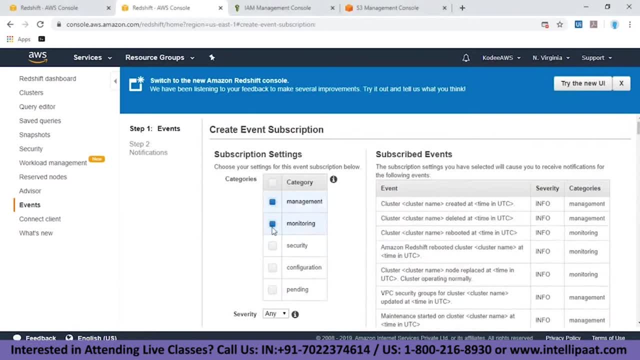 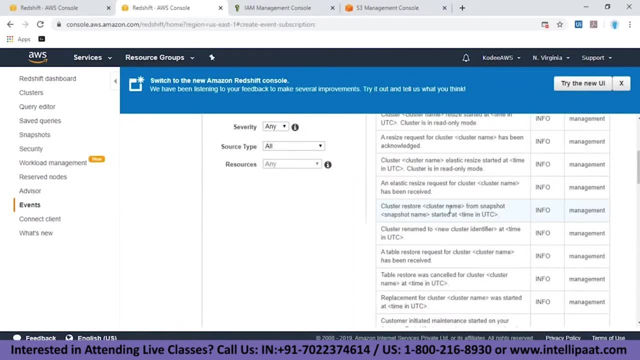 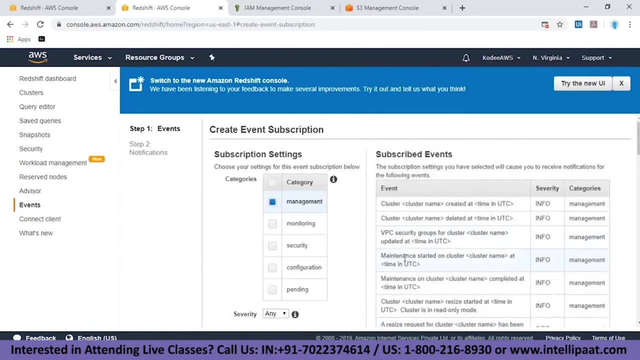 This is the only configuration which you need. just select monitoring and management. Okay, here comes created, deleted and what else It's not? restore from snapshot: Canceled frog clusters. So table restore then. Yeah, so all of these. basically, you can subscribe from here. 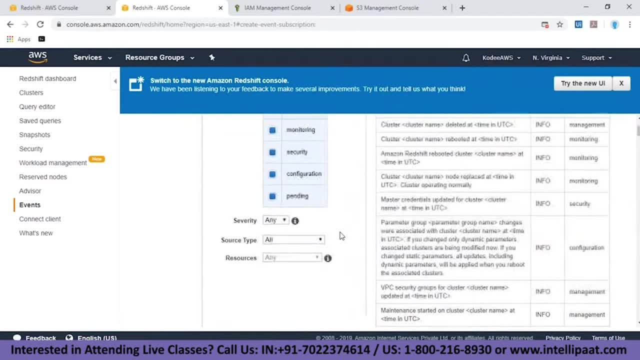 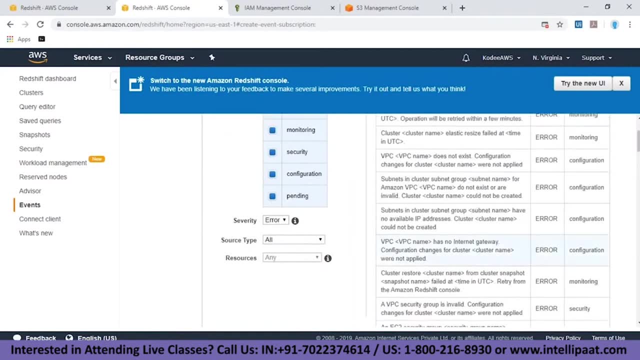 If you want all kinds of things, you can also take up the severity. For example, if you just want error, if you just want error event mails, so you just want. you don't want any information as your mail, right? You can just check it over here. 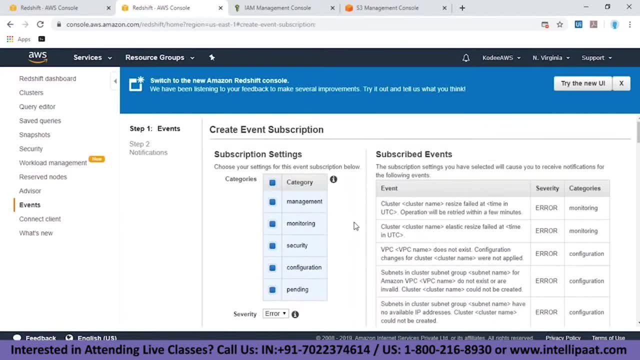 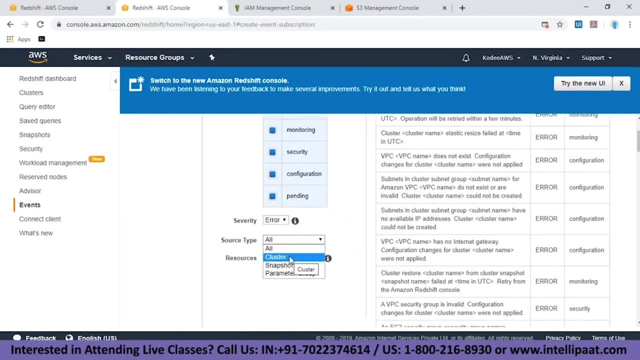 So if you just want errors which are occurring at your redshift cluster as mails, we can just choose that. choose the source type on which particular thing you want events for, for the cluster or for the snapshot or the parameter group. So you can just choose all and then, if you choose cluster, 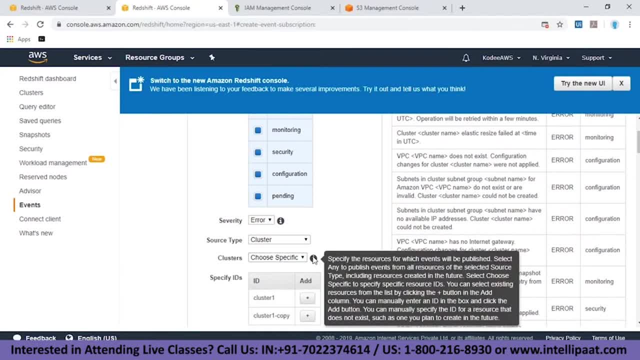 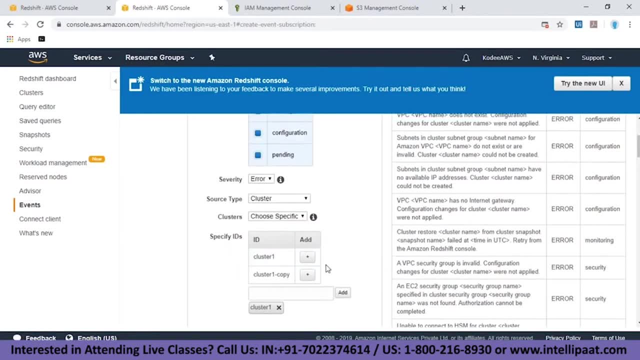 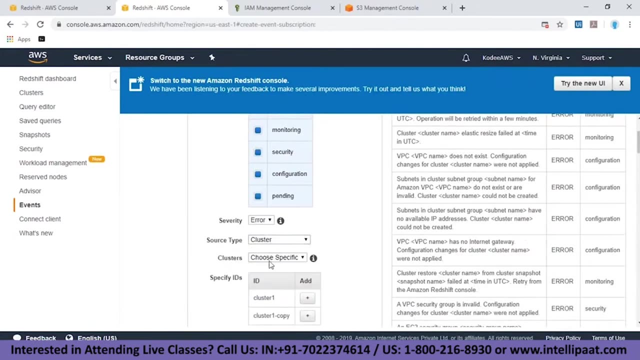 you can choose a specific cluster, You can choose one, or if you have any number of cluster, you can add it. So I'll just go with cluster one. Yeah, I've added it. then What else here? So here there is nothing then. 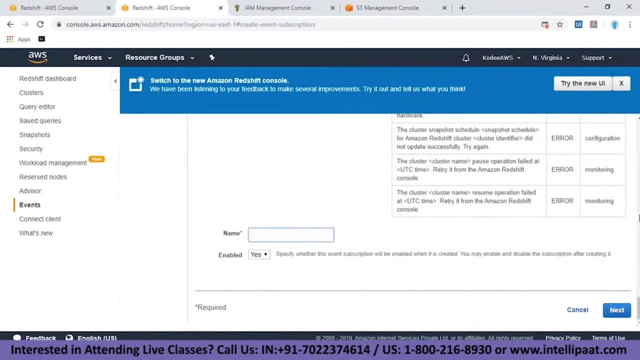 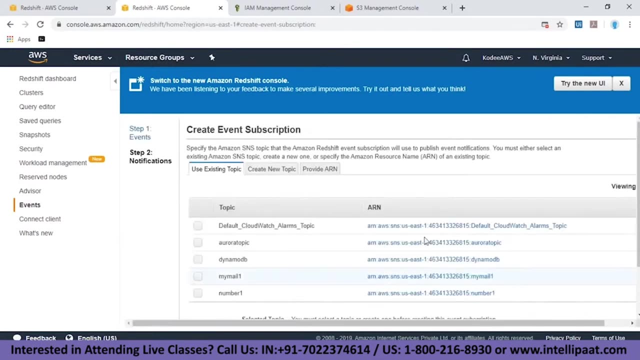 We'll have to go to next step. So you have to provide the name of the subscription, Let's say one. it is enabled. You can also, if you want to just create a subscription and want to enable later, click no here and the next. if you already have a topic create, choose it from there directly. 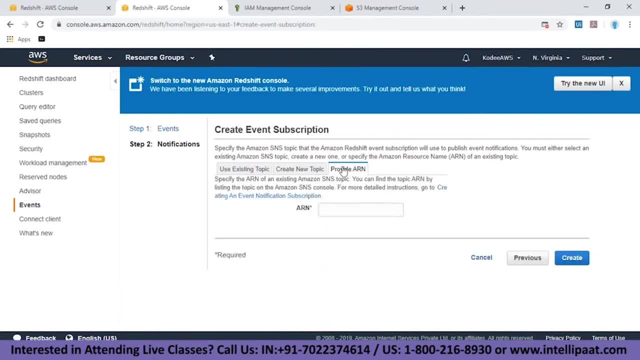 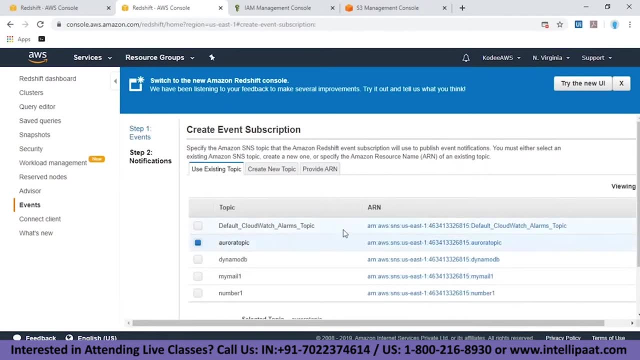 if you do not have created here and then if you, if you know the ARN of your topic, just provide it here. So I'll use the existing topic. I'm just clicking on Aurora topic which I created before create, so done. So now any for any year. 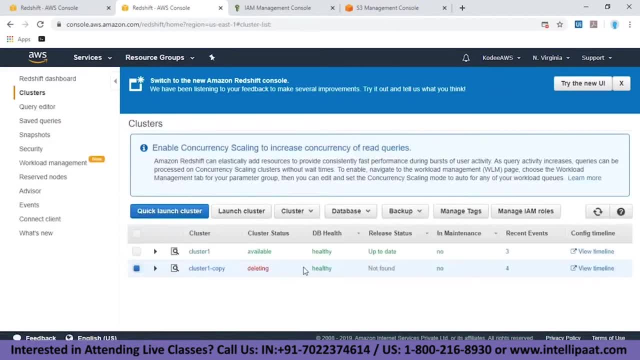 So it is active. My event subscription is active. now for any event I'll be getting mails. So even subscriptions and events are almost. it's not almost. it's the same for any kind of AWS service, Yep. So now we've seen that, so we've discussed today's concept. 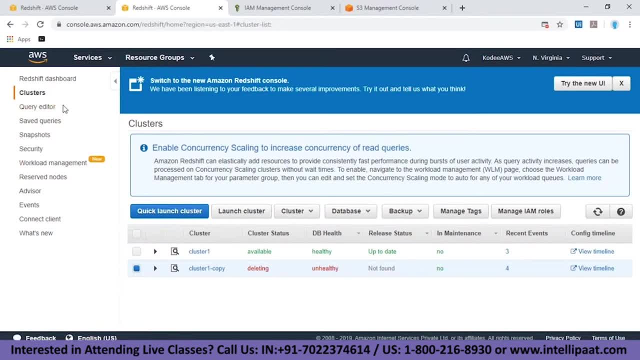 That is, we've discussed about rich of clusters. Then we saw query editors- how to edit, sorry, how to run queries there. Then we saw how to save queries. We saw how to restore. then after that, what else we saw. we saw events and also we'll see the sub node. 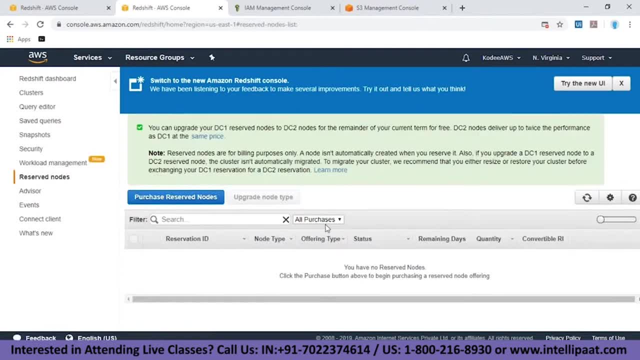 So if you want, if you're going to use this particular redshift cluster till for one year or two years or however how much ever you want, you can purchase from here. So you'll have to select the node type, you will have to select the contract you'll have to select. 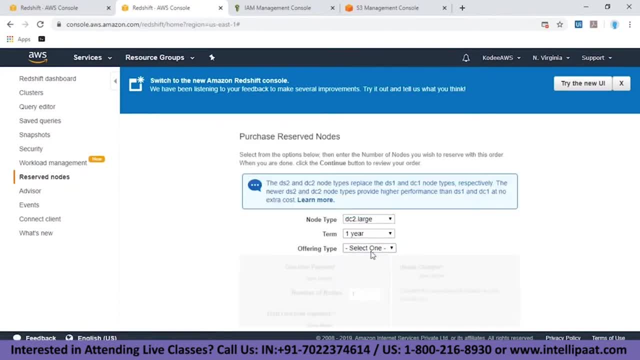 if you are going to provide it all up front, all the cost for a one year, all up front or so, for example, one time payment, thousand three hundred dollars or partial upfront, 750 dollars, and you will be charged point a, point zero, eight dollars. hardly and no front. you'll be charged point two, zero dollars per hour. 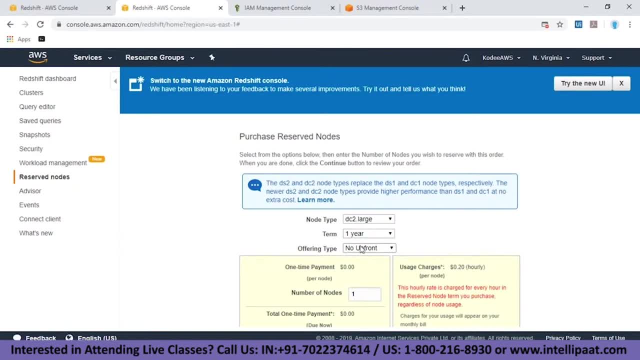 But your instance will be available for one hour with you. She's already one year with you, so it's all up front. It is thousand three hundred and single payment and also it differs with. so here this is total one-time payment due now. So anyway, 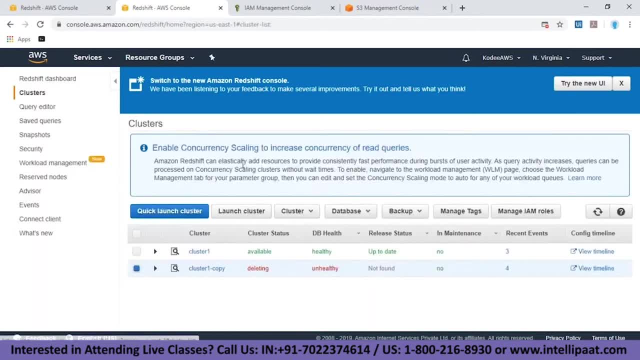 I'm not going to pay it, So I'll just go ahead. Yep, So now we've seen this. so for today, today's stuff, we've done. So now let us go ahead and do the Aurora Last region replication. before you continue, 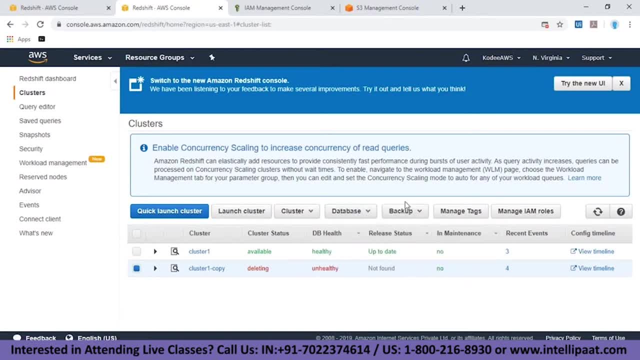 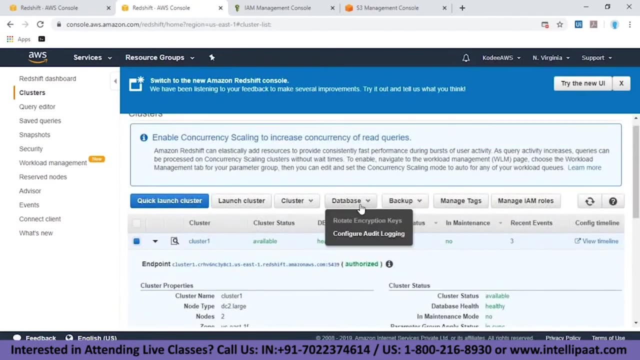 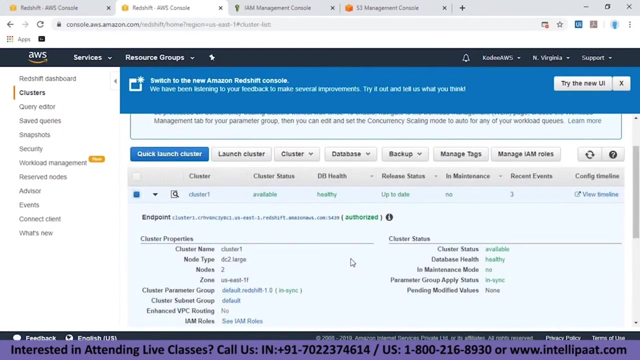 I. I was hoping that you might be able to dive into the no slices, But no slice, Yeah. so if you like, okay, so yeah, on the compute note, there's like distribution of the data across those slices, Yeah, I. 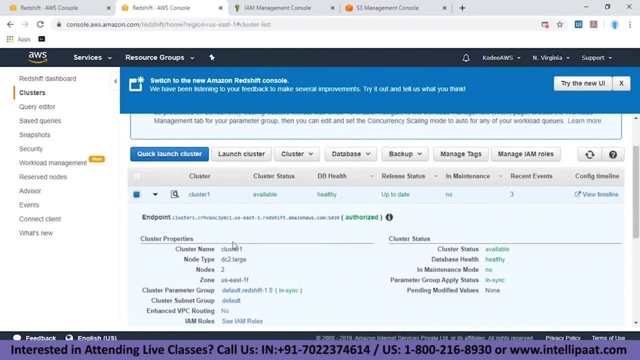 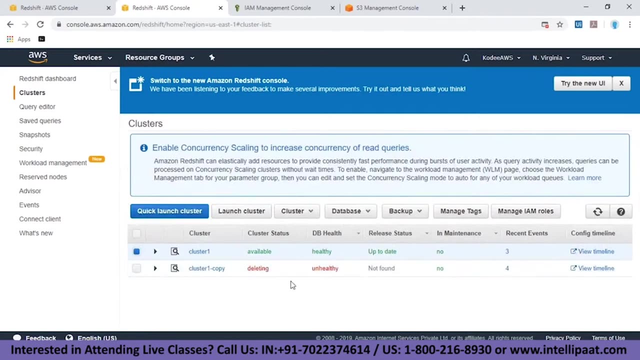 think we do not have a provision for that. I think that is automatically taken care by Redshift, because we do not have the authority to check what exactly, where exactly it is running or what it is running inside. So there are no provisions here. But the thing is, if you have two nodes, then in that two nodes. 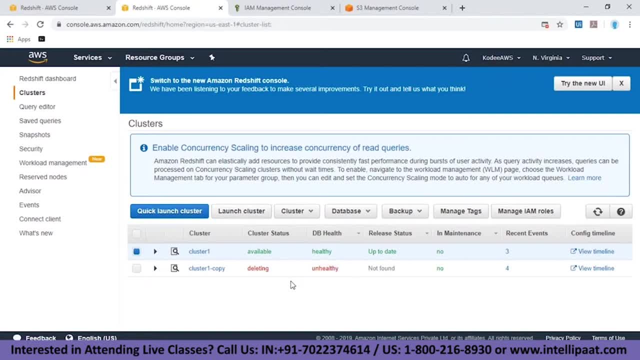 there will be multiple node slices and each node slice will have its own memory and storage space and the workload coming into that particular compute node Will be distributed across all those node slices. So everything will be happening parallelly and then the no compute node will gather the query data, send it back to the leader node. 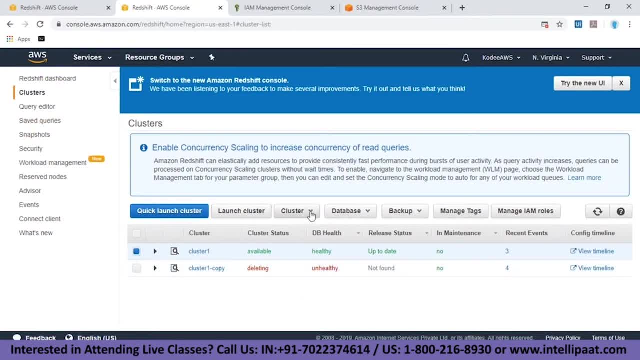 and it will send back to the client application, but there are no provisions here for that, I think. so What if I? yes, it's more of a deep dive into the database concept in terms of Redshift. I guess you might not have that insight. 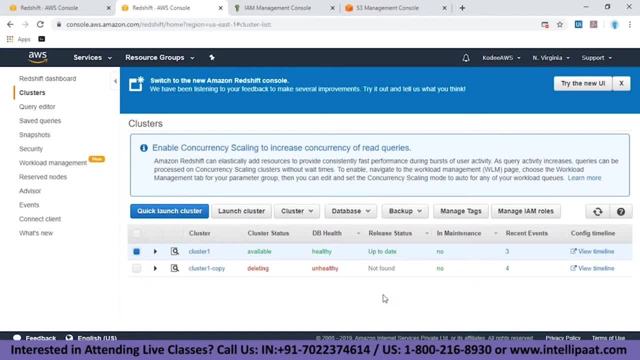 So I'll take it back to Nash and see if Maybe so. Yeah, So how are the how it runs on the data center for how exactly it works? Yeah, so we have Redshift and then we have a lot of tables loaded already. 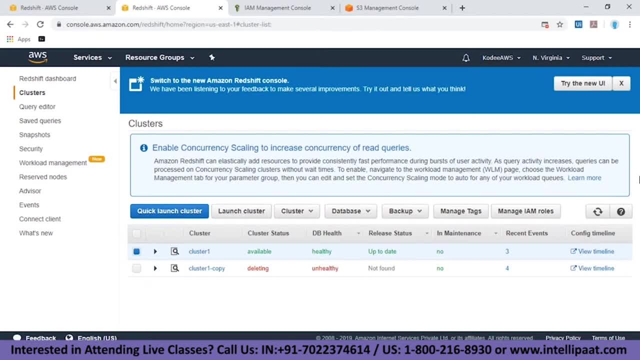 Okay, but we haven't used it for real, like for live processing, yet. Okay So, but we heard that the key- how to build the key, The sort keys and stuff like that and also avoid hot spots when the query hits particular- slides. So we want to distribute the data evenly. 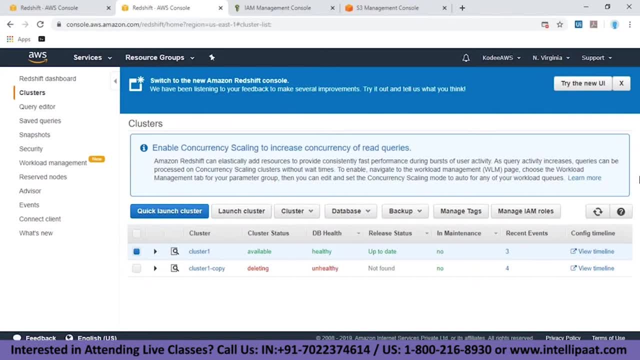 Okay, like inside the database, just a second. It's not so much of a yeah, I get it. So I think we'll be looking more into the data sources, then designing the warehouse, then maintaining the warehouse, analyzing, tuning performance. Yeah, So, yeah. so those things I'll cover in the next session. 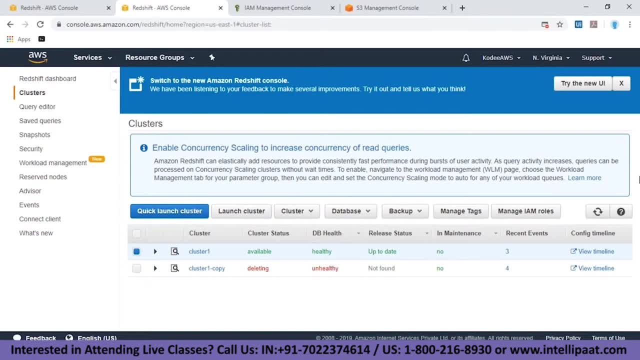 Okay, Yeah. So today I just want to cover the basics of Redshift, then launching it and showing what exactly is the, how exactly this dashboard works. So, yeah, I'll also, like I'll make, I'll teach you how exactly node slices and how the data is segregated across them. also in the next session. 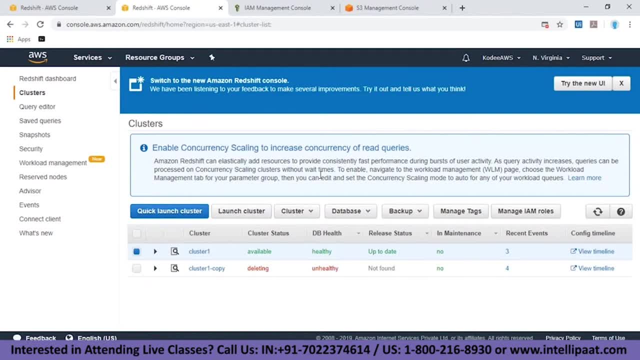 Okay, cool, Yeah, Yeah, Okay, Okay, So now, yeah, so here first we'll look at cross region replication here. So there is no provision for directly, like for example in Aurora. You can just click on an option, actions- and just hit cross region replication, and it'll do all the job for you. 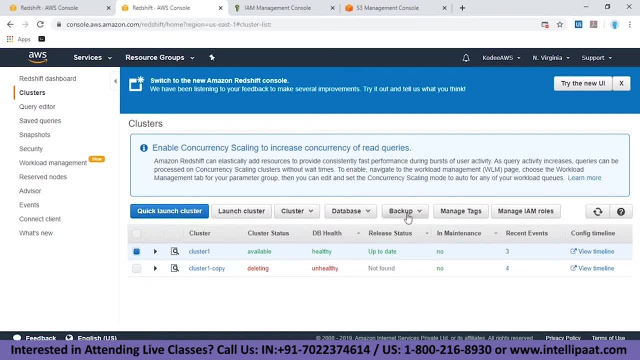 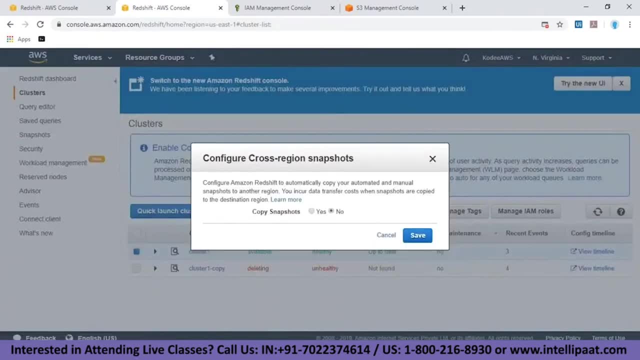 But here you should have a snapshot. You should go to backup and here you see, configure cross region snapshots Now. Now you'll have to hit it, So copy snapshots. you'll have to choose the region where you will have to copy it. 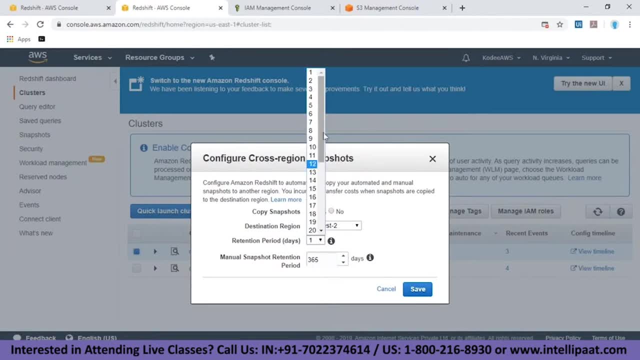 For example, let's say us East to, you will have to choose the retention period. So they've given 35 days manual snapshot Retention period. you can provide minus one, I think, the number of days for which manual snapshot will be retained. setting this parameter to minus one days retains the snapshot indefinitely. 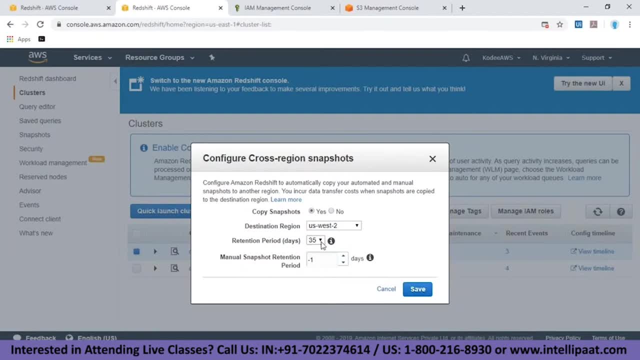 So, basically, this is for the automated snapshot. So, automated snapshot. the maximum retention period for it is 35 days. So what you'll have to do is you'll have to make a copy of it so that it becomes a manual retention, a manual snapshot. 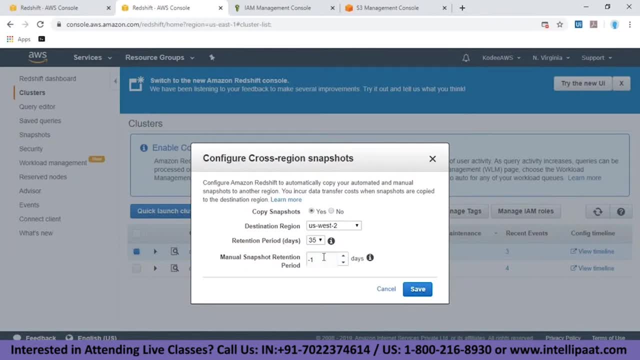 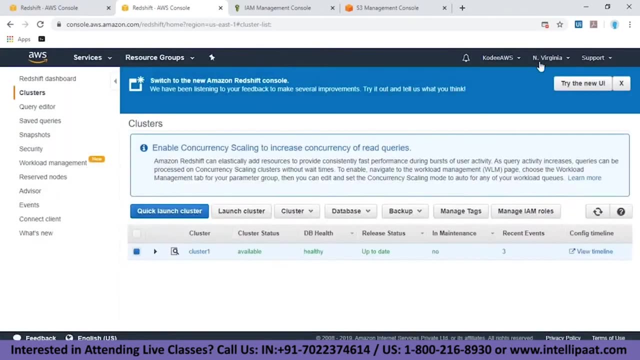 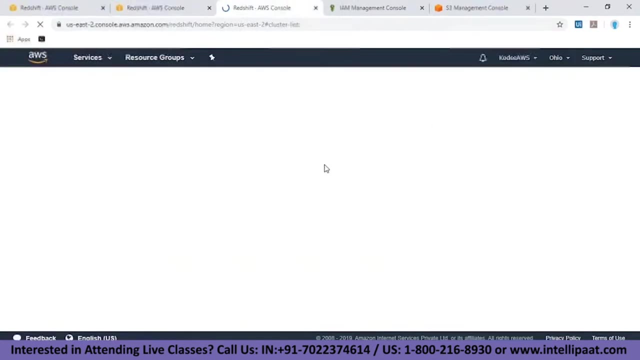 Then you can provide minus one. Basically, what that mean is what that means is: the retention period is indefinite. So now I'll save it. So now I've copied it, So now I have to go to. was it us East to or best to do? don't remember. I think I gave you a star East to. so the thing is, once it gets created here, Once it's copied in this region, then you can choose that snapshot and restore your cluster here also. So that's how you can do cross-region replication in Amazon. 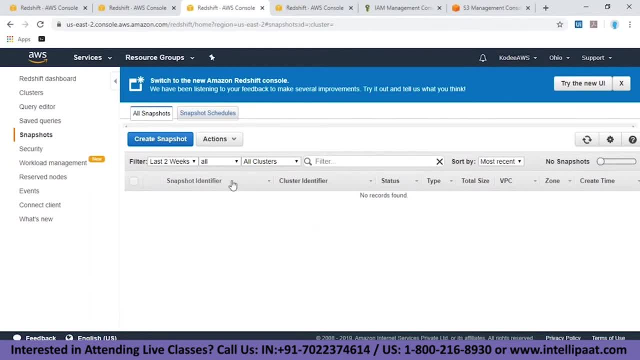 Aurora clusters. the snapshot data, the backed up data, will be the same here, but there is no interconnection between these two clusters. So, yeah, so this is how you do it in Redshift, but in Aurora you have a complete option for that. 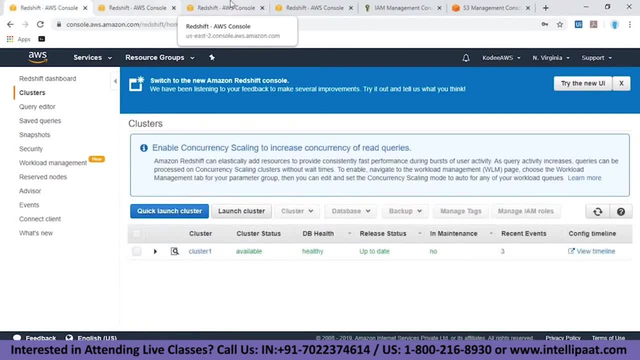 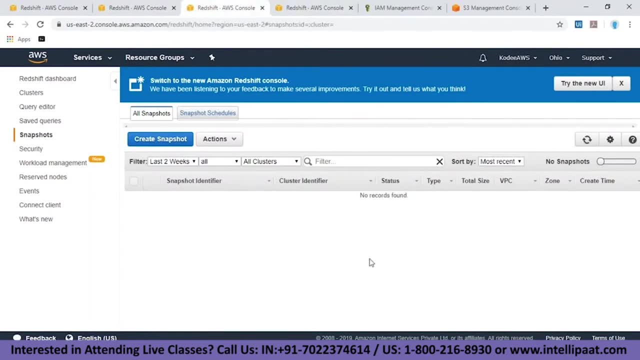 You have a separate button for that. So now we'll go there before you move. If I create a cross-region snapshot on the other side, on another region, and periodically I want to test it. So how long does it take to restore, based on the size? 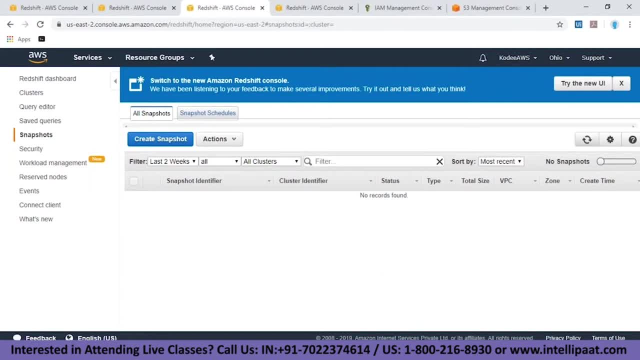 So it's what, whatever you show for different options, like earlier for great Glacier, for example, the cost for restore, So is it like the price gets charged at the point when I want to do a restore test and then they will start charging, and then 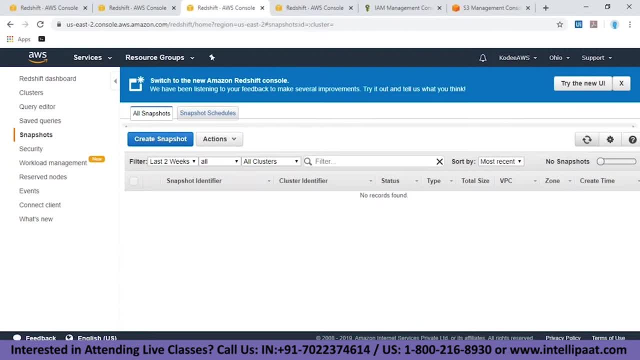 if I test finish, my test finished, and then I shut it down and then stop charging, like that, right? Yeah, So when you are retrieving data, only that particular time will be charged for retrieval of data. So when, once the retrieval- that is restoring from your Glacier stops, 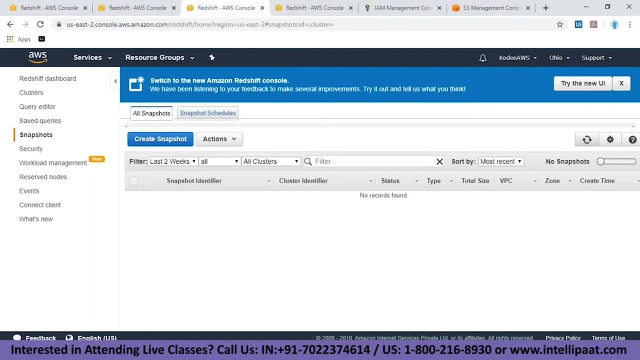 then you'll not get charged for that. So then when I do the restore from the snapshot and based on the SLA, I guess if I, for example, if I have one terabyte and based on SLA, I want to bring up the database, the entire warehouse in like, say one or two hours, say one hours. 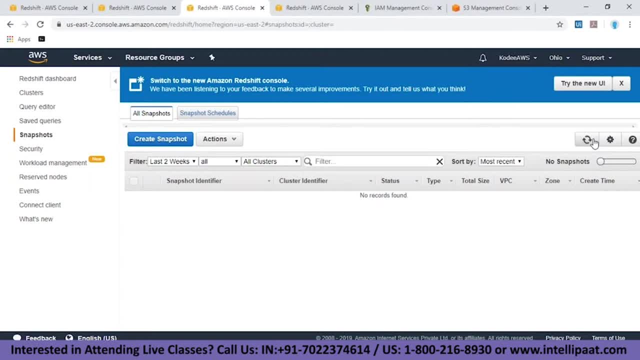 Okay, So then I would go to what you have just shown us: the speed and the charge will restore, right? And then, based on that, choose the options, right? I don't know. Yeah, Yeah, Yeah, The thing is so. I think you'll have to set it up accordingly. Amazon Glacier. 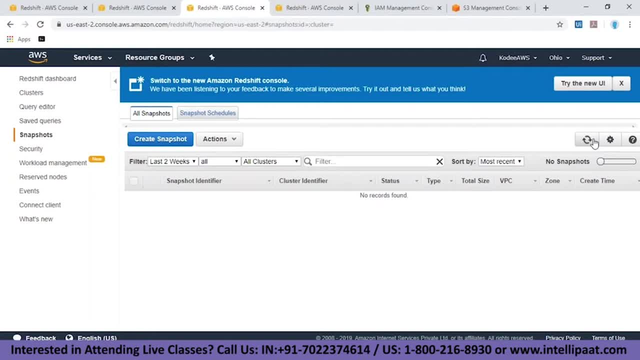 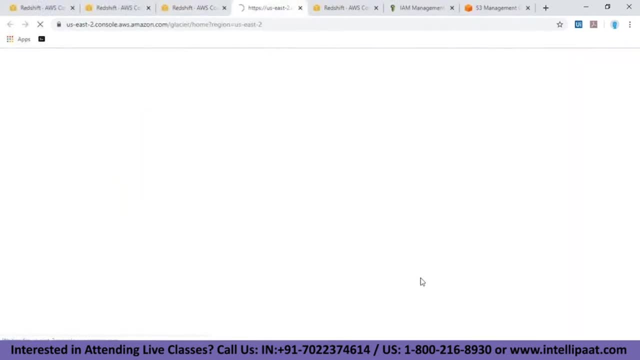 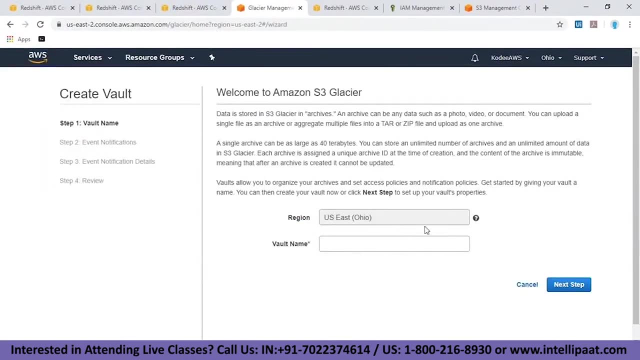 I think you have a separate option for that. also, You'll have to set it up. So let me check one second. So you have this, so I've not worked on this, but another basic thing: so you'll have to set up a vault and you'll have to store the data in this world. 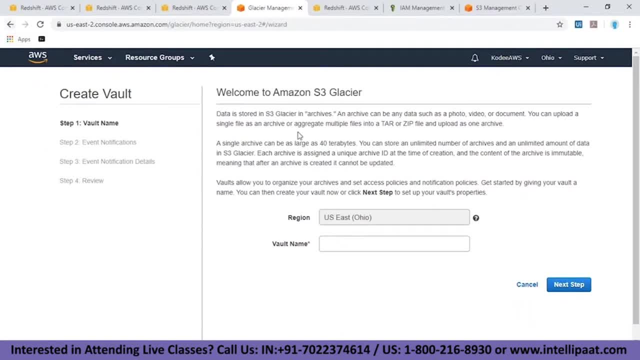 and for this world you'll have to provide some details. So for this, this particular world, for your data, So to retrieve these, you'll have to set like: this should be retrieved within one hour or two hours, I think it's like that. 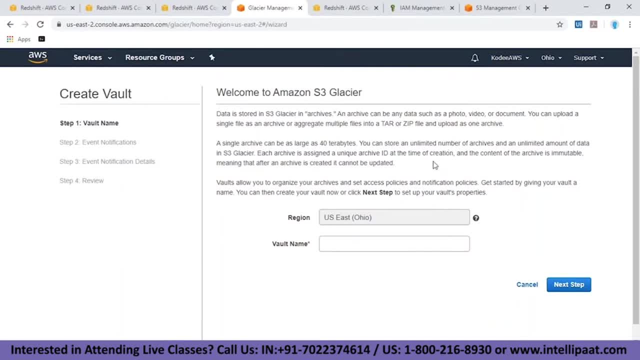 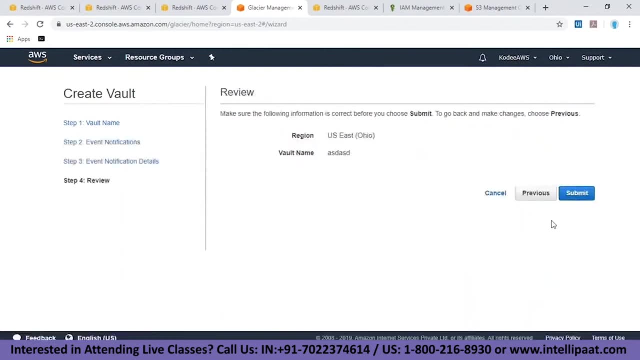 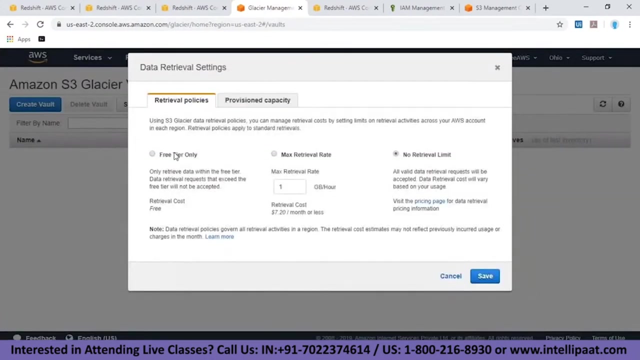 So once you do that, then once you retrieve, retrieve data, so yeah, so you'll be charged only for that particular time of retrieving it. So I've not worked on. so just a second Step: do not enable So free to your only retrieval cost. free within the no retrieval limit. 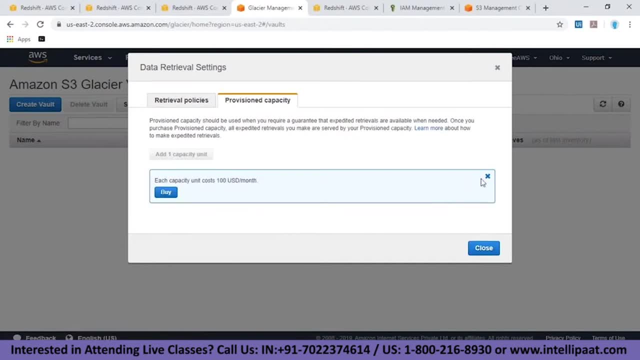 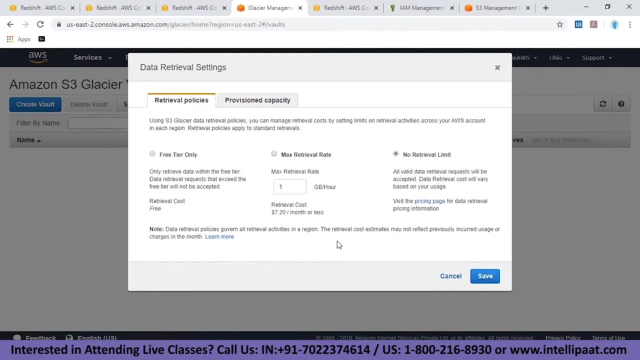 Max retrieval provision capacity. Each capacity in which was so much may reflect previously and could use it. or charges month Max retrieval rate. max retrieval rate: 1 GB per hour. Sure, of course it's not provided here, So I'll exactly do not know from there, from S3 Glacier, from where we'll have to configure that. but 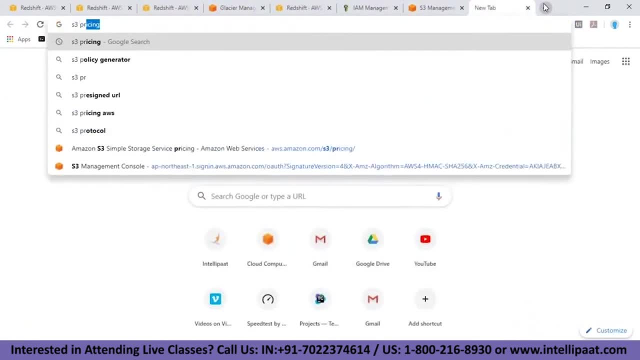 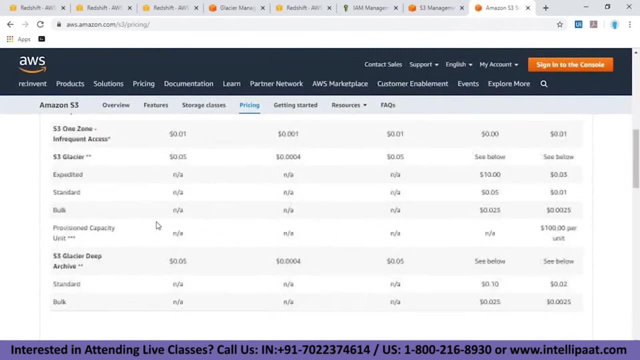 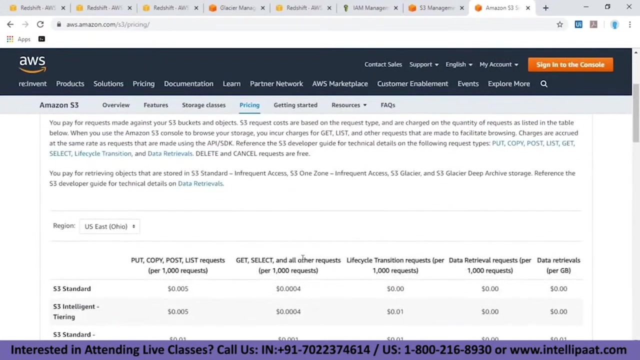 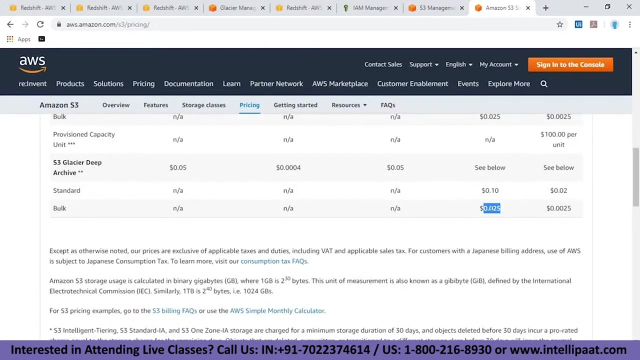 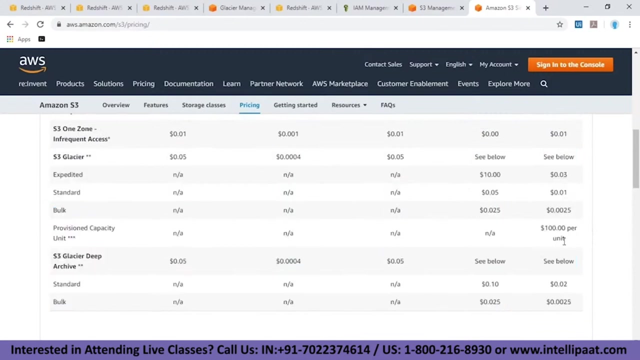 me check here. So Glacier, standard, bulk, This is for get and select data retrieval requests. So here standard and bulk. This is for Glacier, This is for Glacier, Okay, provisioned. so there are some various options: standard, bulk, bulk. I think there is. 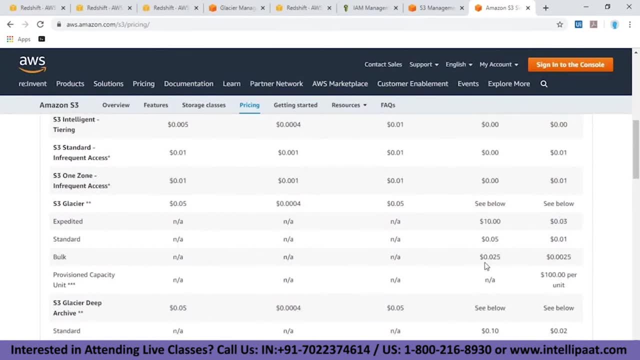 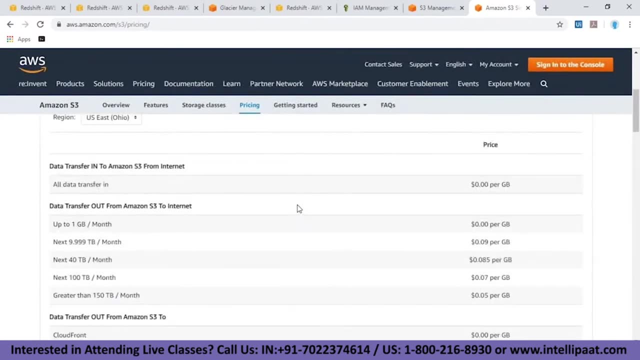 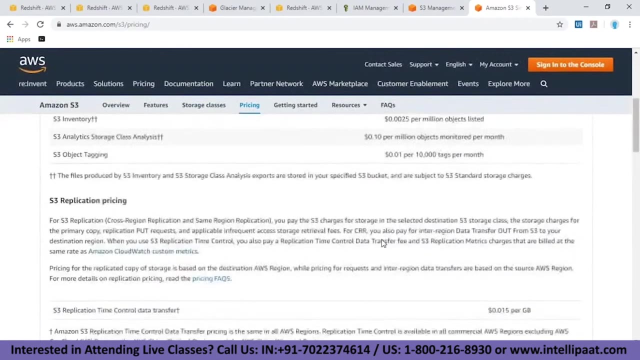 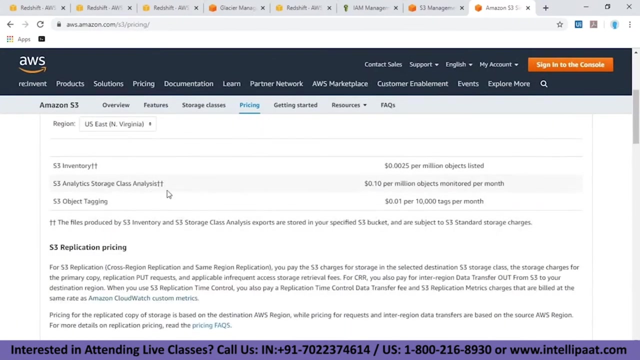 Some provisioned capacity for this, and after that you will be charged this much, but I do not know the exact amount. how much you'll get charged? Not here: Stereo transfer, management and replication. It's over here, See, not Virginia. It's not so much the price price. 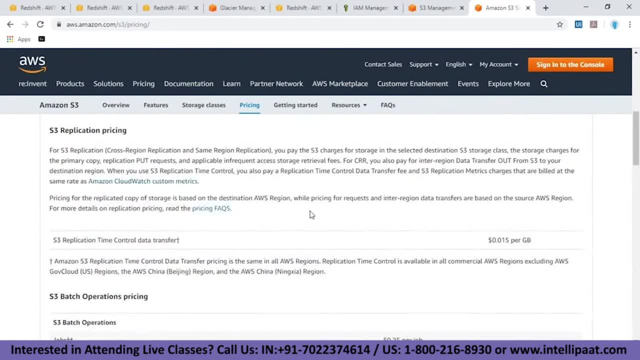 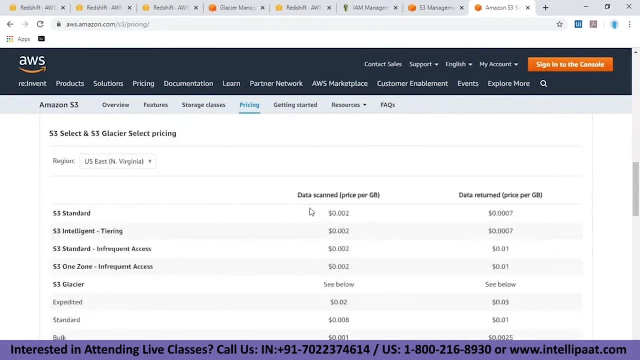 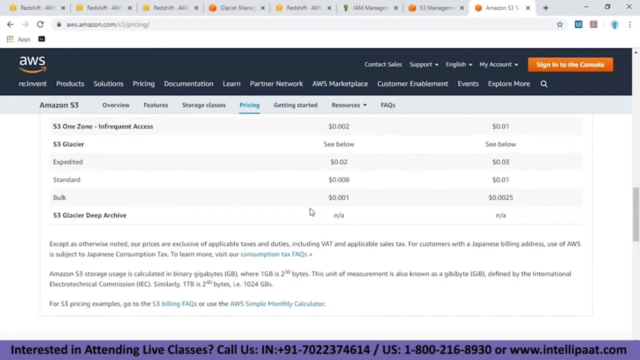 Oh, it's important, but the it's more of the timing. the timing, right. Yeah, the time is correct, Okay, Okay, So I do not know that right now. I'll check into that and, like before the session, like how I do. 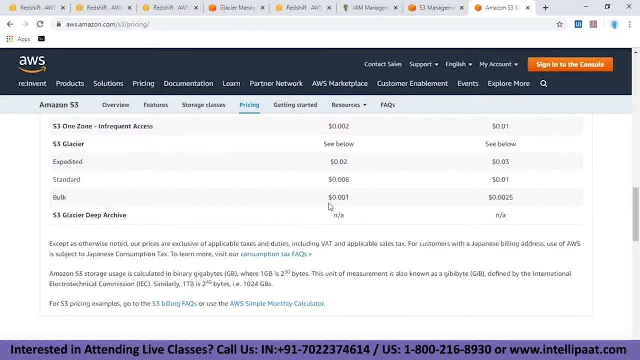 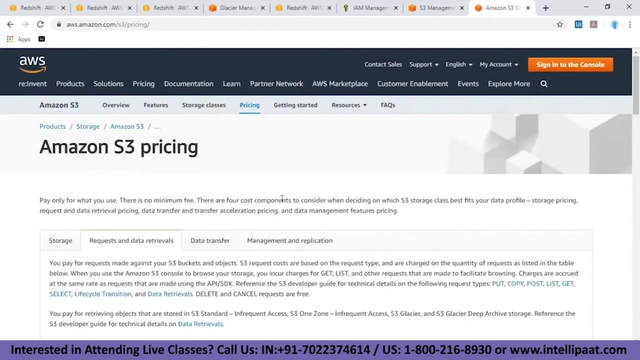 I'll answer that first, then I'll proceed with the session. So I'll see where we'll set it up accordingly, so that, for example, when we retrieve, if we set up one hour, it should restore within one hour All the data of that database and how much we'll get charged for that. 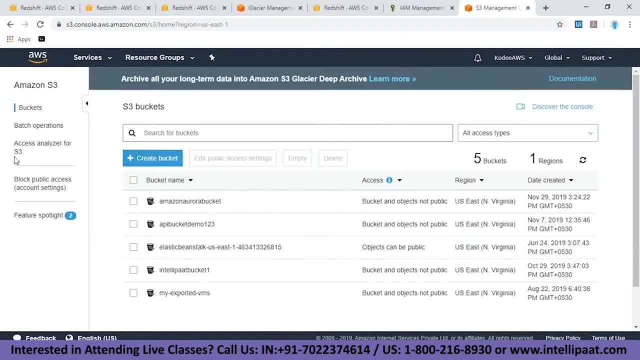 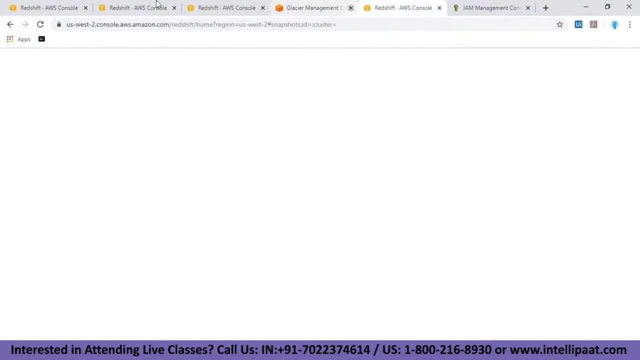 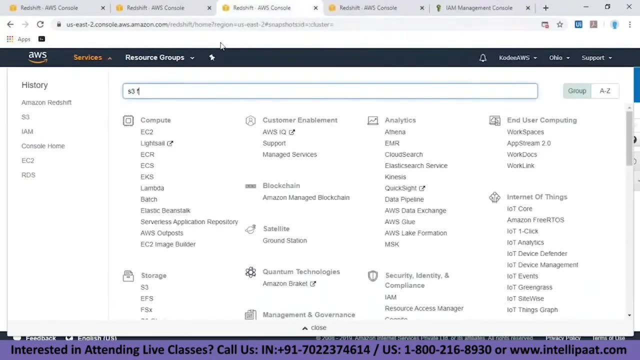 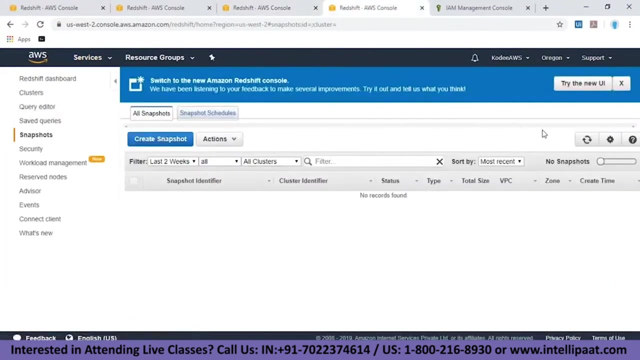 Yeah, Okay, I'll check that. So where was I here? So we are looking at that. So did it copy in Ohio, What is this is not Virginia. Okay, so What? you're saying Pennsylvania, So where's it going? 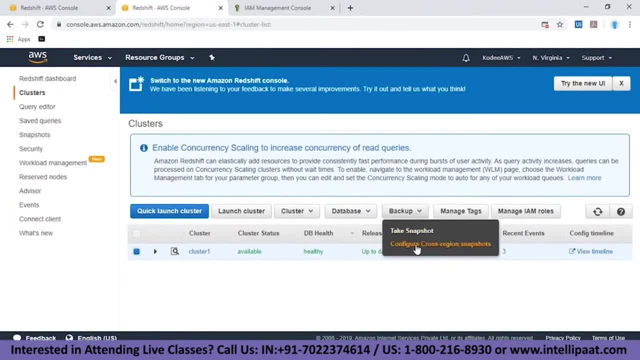 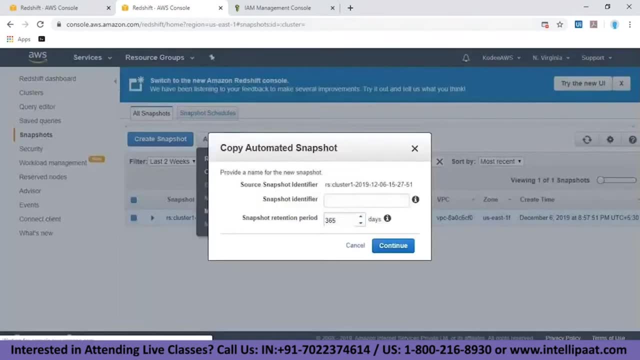 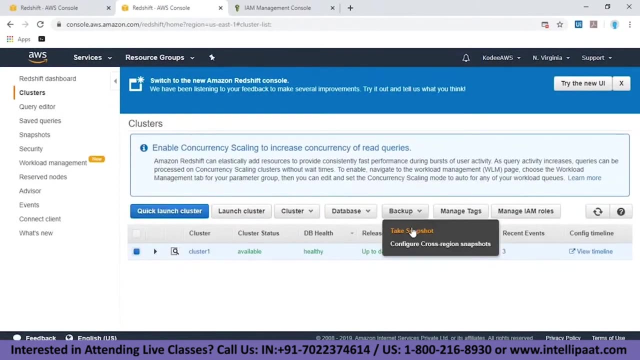 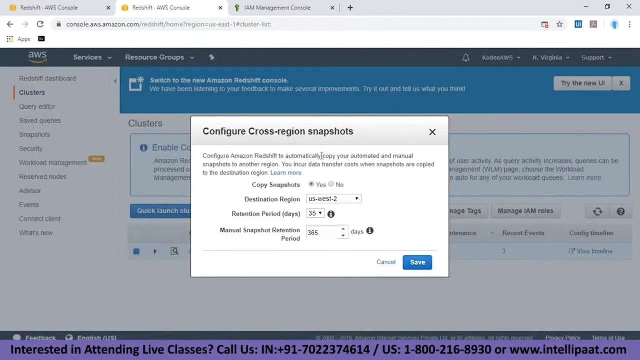 Okay, Okay, so fillаю, Okay. so here we go. here's my to is from California, So it is camera. We all know you have it right, You're theave. Okay, soaré, Configure them to automatically copy or automated in manual snapshots. You incur data transfer costs when snapshots are copied to the to the destination region. So if I create a manual snapshot right now, let's let me create one. So I think once it this gets created, I'll also get one in my the cross-region replicated snapshot. 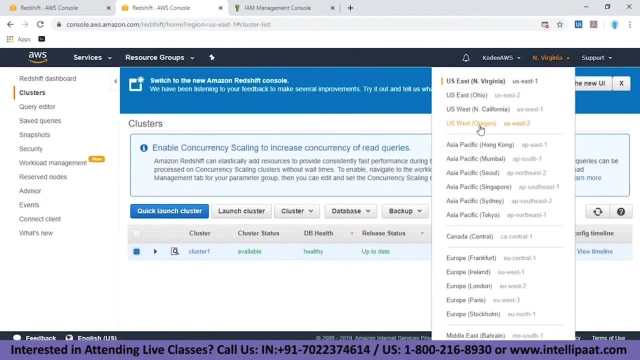 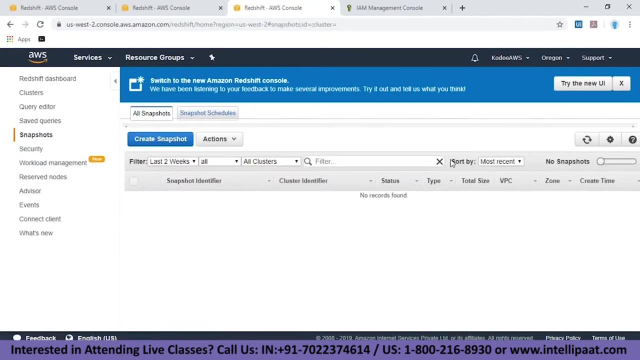 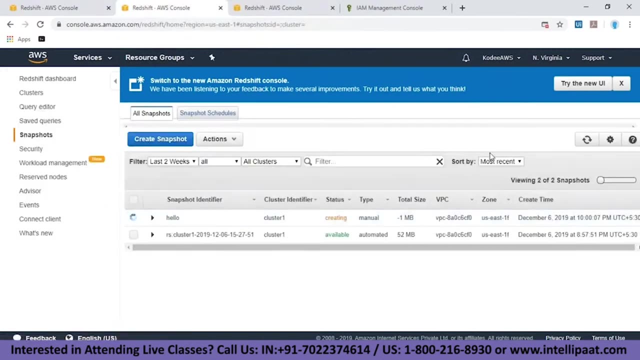 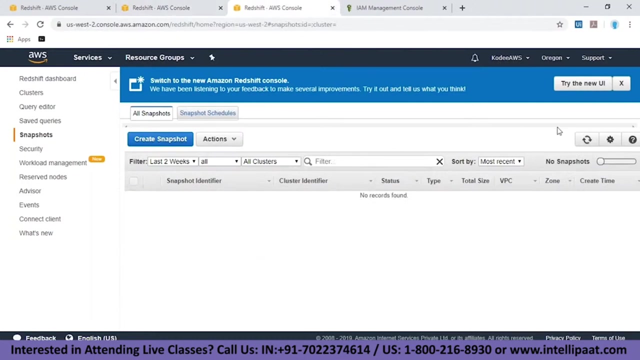 So where was that? us West to US West to Oregon, I think. once it gets created here, then it will be copied. So it's getting created. So minus 1 MB, So you can see the type. also this manual. So the thing is so when I configured it, the this, this one was already available. 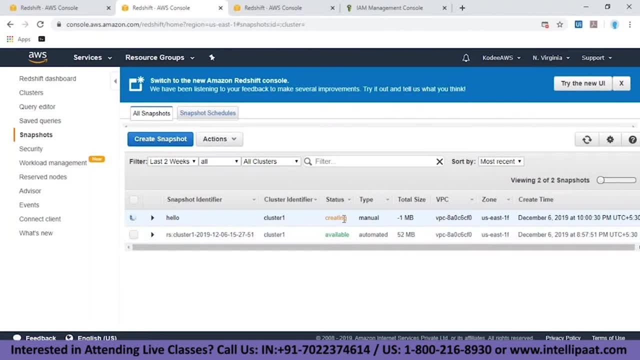 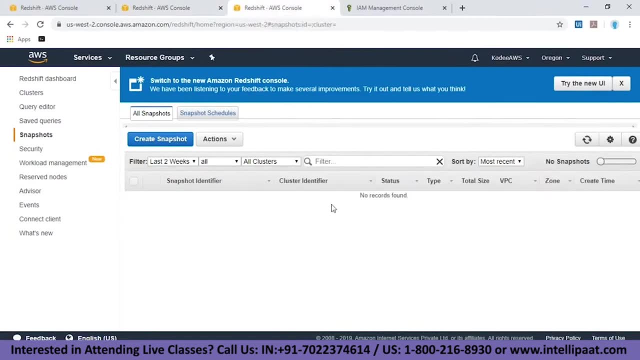 So the ones which will get created after that. that will be noticed once it gets created here. I think it will get created here, It will be copied here. So let's get created. We'll see whether it gets copied here or not at the end. So first, so we'll have to launch Amazon cluster, Aurora cluster And sorry, sorry days. So here, if you create Aurora database, then cross, do a cross-region replication. They enter database, architecture will be replicated there. Everything will be that. the data will be there, the same number of compute heads will be there. I'll just choose t3 dot small And yeah, so I've created the database. So. So right now it's getting Created. So once it gets created then we'll be able to do cross-region replication. So here there is one cross-region read replica. 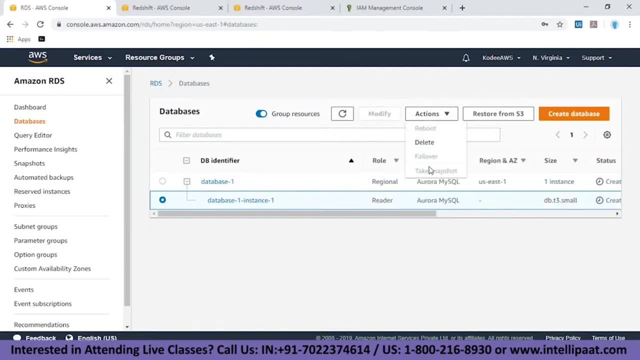 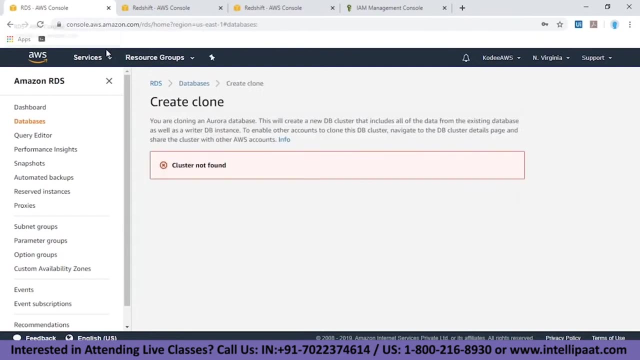 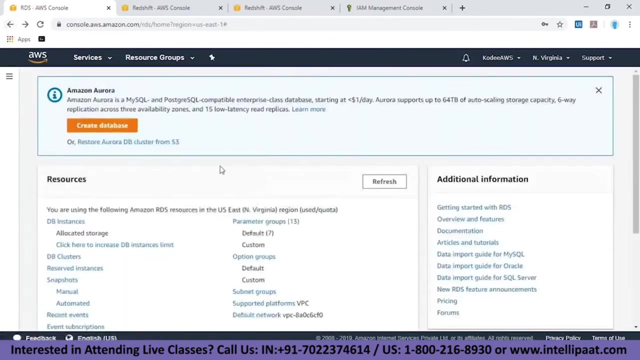 I think this is one. then I think, yeah, There is one cloning option. Where is that? Create, clone What this does. Okay, the database has not created. Just let's wait until it gets created. It's just Let's wait for it to get created. 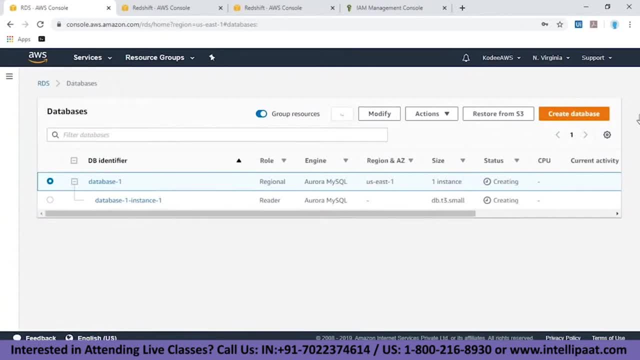 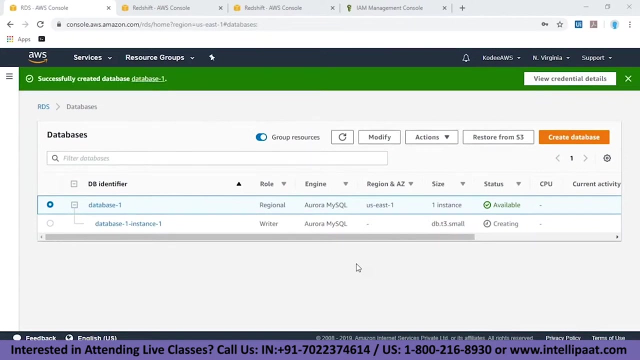 So I'll just wait for it to get created. So I'll just wait for it to get created. Okay, so this is a little bit more than that, So I'm just going to go ahead and do it. Let's see, Let's do it. 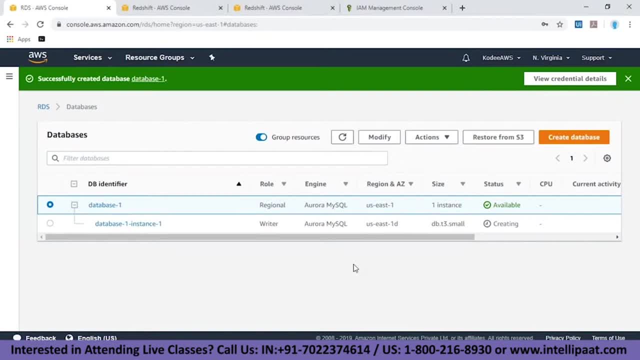 I'm going to double click on it. Okay, so it's going to create the new database. It's going to create the new database. Let's do the same thing over here. Okay, so, I'm going to do this one. So I'm going to do this one. 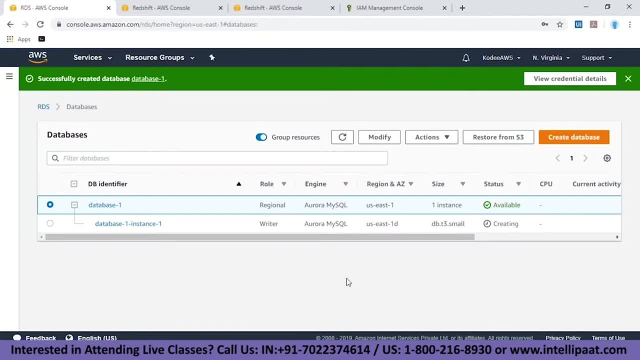 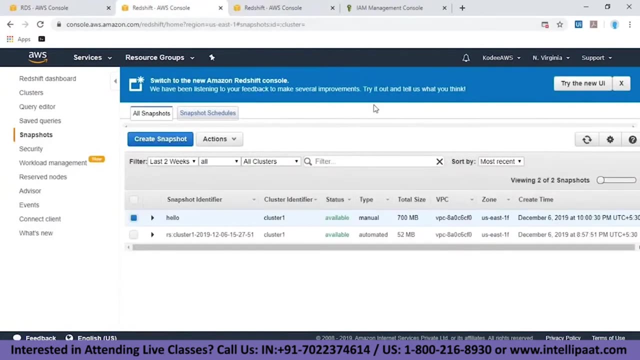 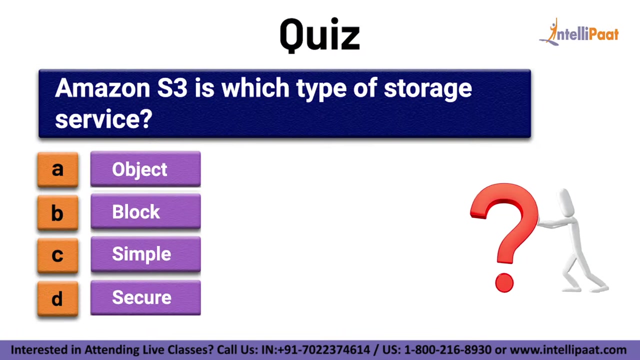 And then I'm going to do this one. Okay, Just a quick info, guys. test your knowledge of AWS by answering this question. Amazon S3 is which type of storage service- A, Object B, Block C, Simple, D, Secure? Comment your answer in the comment section below. 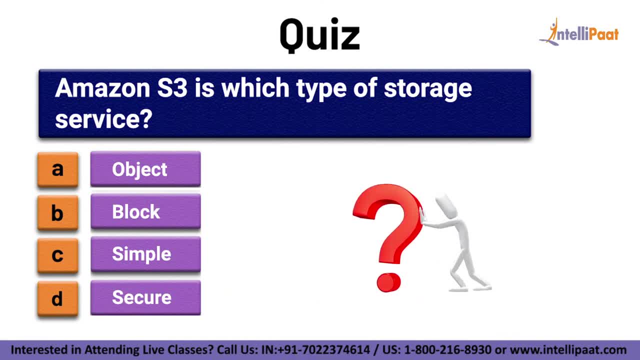 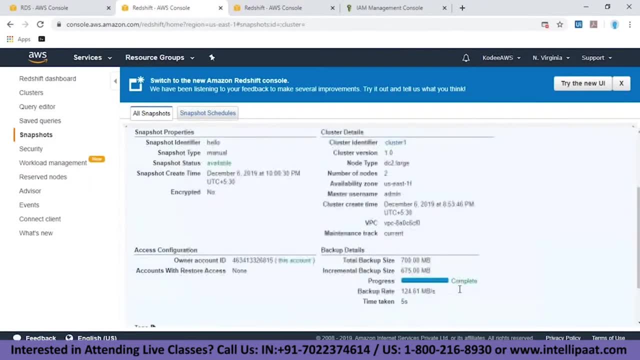 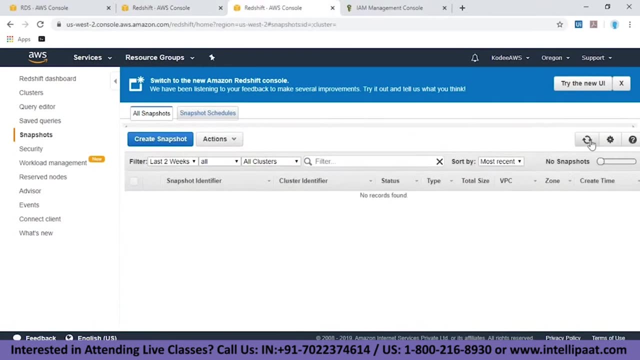 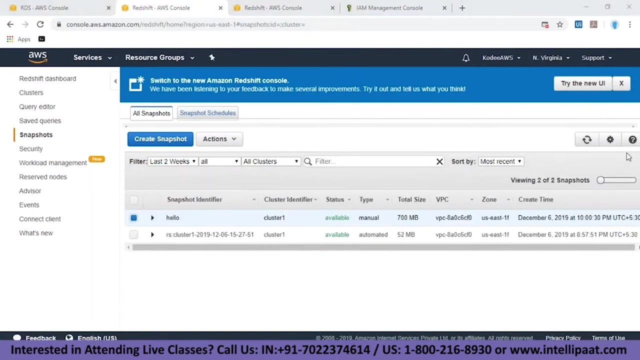 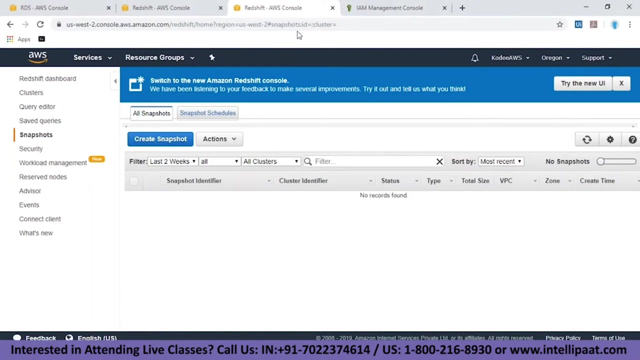 Subscribe to Intellipaat to know the right answer. Now let's continue with the session. Did we lose your voice, Kodhi? No, no, no, no, just checking. I've enabled cross-region replication, So what completed over here? I think it takes some time to start it up over here. 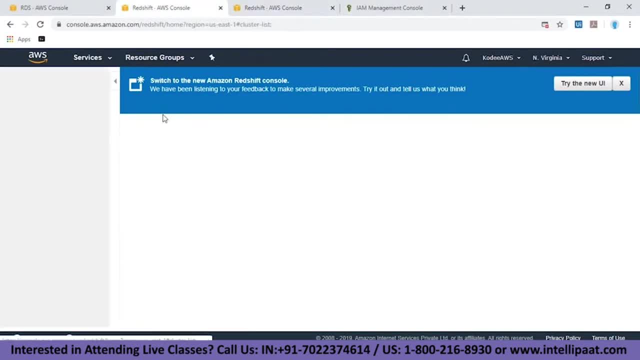 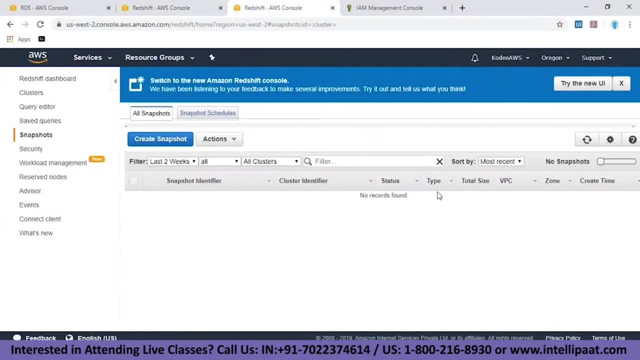 So I've mentioned us-east-2.. They've configured it for cloud. It's a cluster one. So, yes, us-east-1 copies snapshots. everything is done, So it should. Okay. so let's see this at the end. 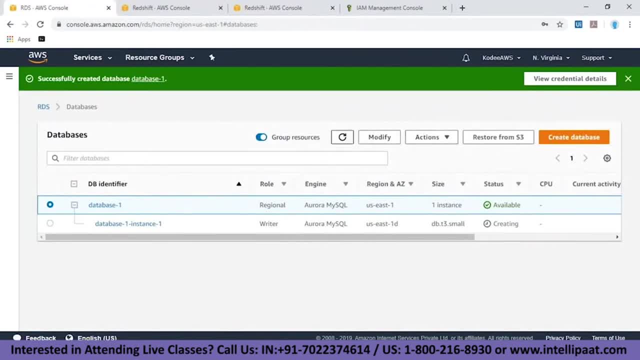 It's taking some time to do that. What's the concept of the cross-region replication? So the remote region, the database, it's read-only available, Or So the thing is So for a reader, for example, for one primary database in your local. so you can create five. In five regions you can create five read replicas. So like in one particular region you can create 15 read replicas for one primary database, So like that in five you can create up to five different read replicas in five different regions. 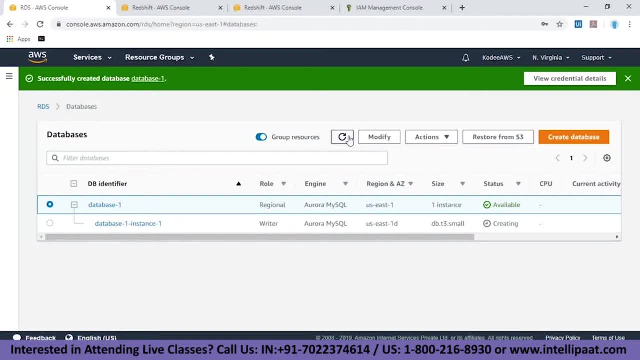 And for those regions, for every read replica you can create 15, up to. It's the same thing, Same concept, But the primary database is just one. When this primary database fails, then So you will have another database over here. 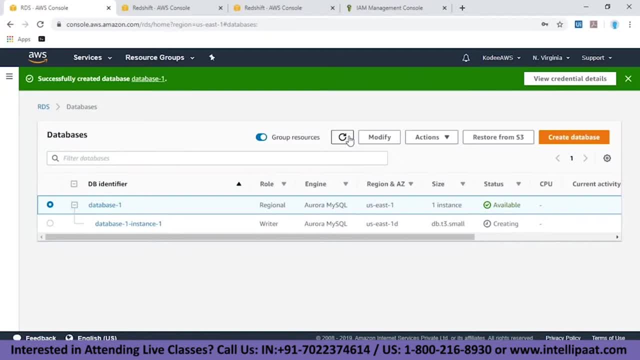 What is that? So, according to your priority, according to your entire priority, it'll create one more. For example, you'll already have a replica, So that replica will become your primary database, But you'll not be able to create a primary database directly using cross-region replication. In your In other regions, but you will have to take a snapshot, then go copy a snapshot to the other region And then you'll have to launch a new primary cluster. So if you use cross-region it'll just create read replicas. And plus that one read replica you can create up to 15 more read replicas accordingly. So your cross-region read replica database cluster, it can have up to 15 read replicas, 15 read replicas. So yeah, so that like that. 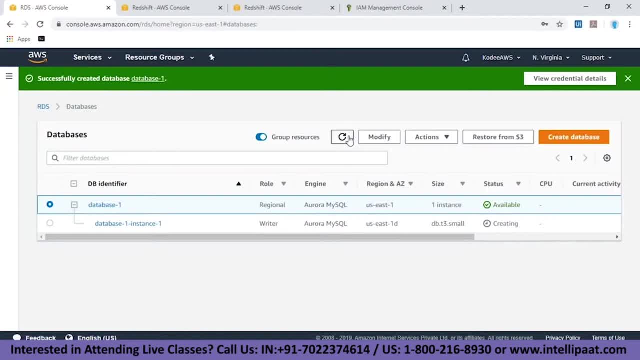 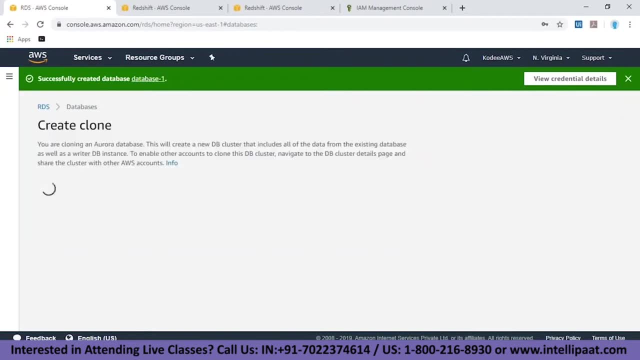 Okay, So it's not a the whole site. No, it's Okay. No, so for that you have to basically what I think you can, just a second, So it will be the same as reshift after to restore from a snapshot. 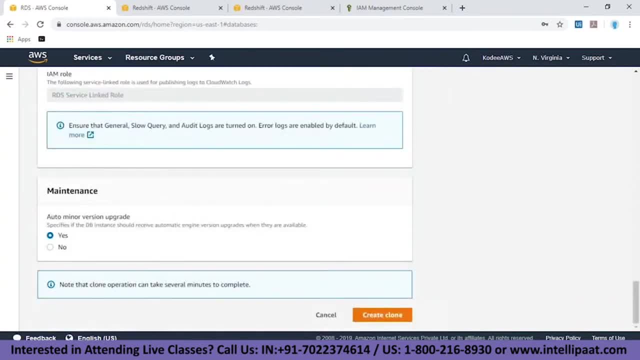 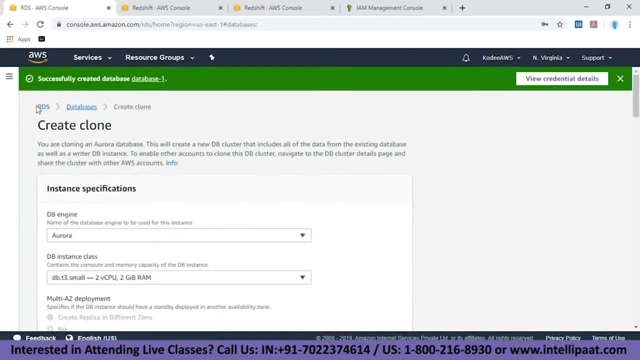 Yes, Yes, So for the entire DB cluster you'll have to do that. but for creating a cross-region read replica, then you can and do it directly. This is not the way. so for read replicas, I think you can. it's pretty simple. 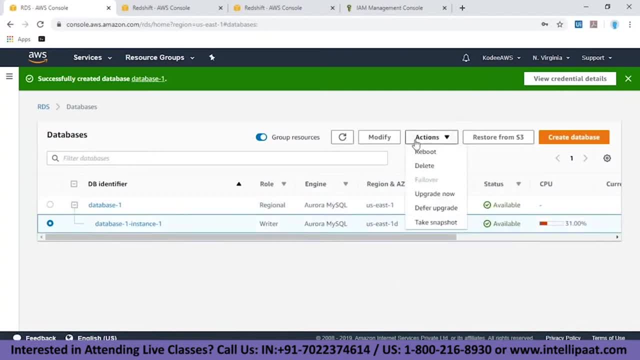 It's the same options. You can just go with this this takes. so this is your. this is going to be your primary database because it's a writer, So you'll have to take a snapshot of this and I think you can create a new one, or 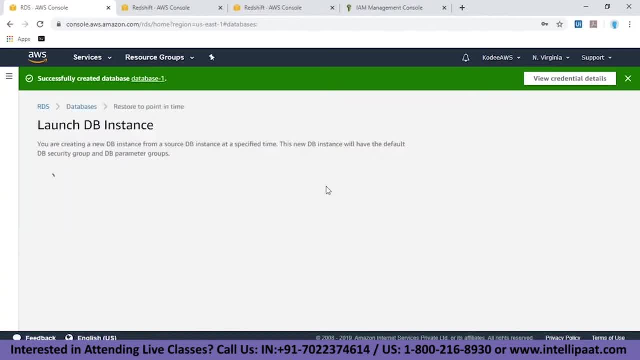 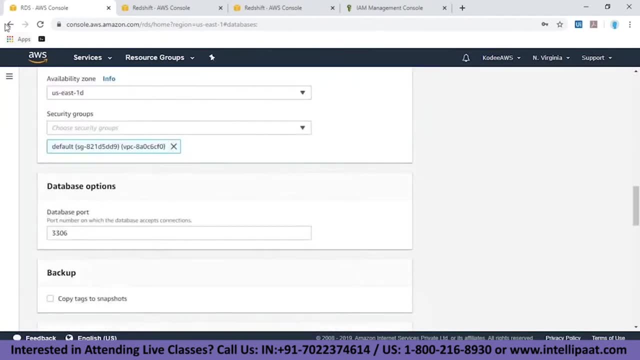 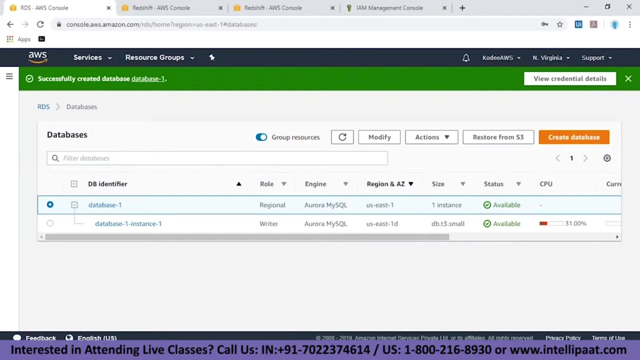 you can just think you can do this. Let's check. Okay, not, Yeah. so one of the option would be for the primary database. You'll have to take a snapshot of it and then create one more in the respective region on which you will have to create a DB. cluster, but for cross region replication, you will be allowed to create three replicas in five different regions. after creating those three triplicas, You can go to that reader And create up to 15 different Aurora replicas for that particular replica and also, yeah so, the connectivity between those three. 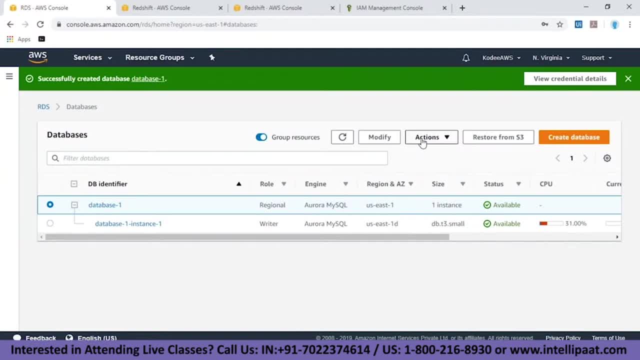 triplicas and this primary database instance will have a lag. So that is also provided in the documentation. It will have a lag, but that is the only way you can do so. the thing is between the source database cluster and these read replicas between regions. 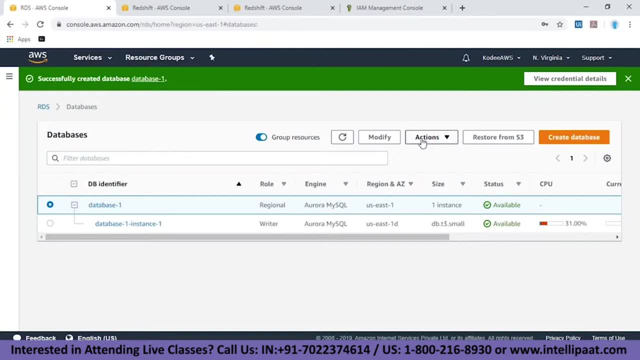 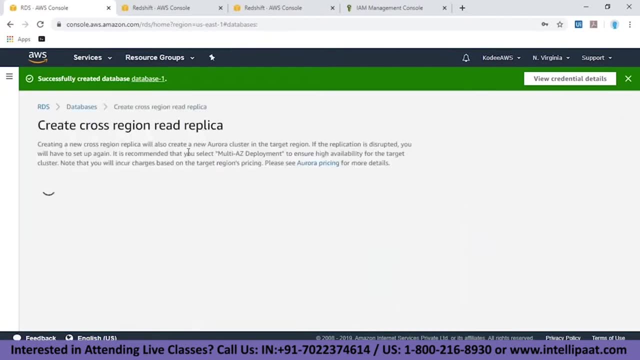 They have a. the networks are totally different, So obviously there will be lags. Yeah, So right now, let's just create one cross-region replica. So, create cross-region read replica. You'll have to just click on the database cluster or for what you. 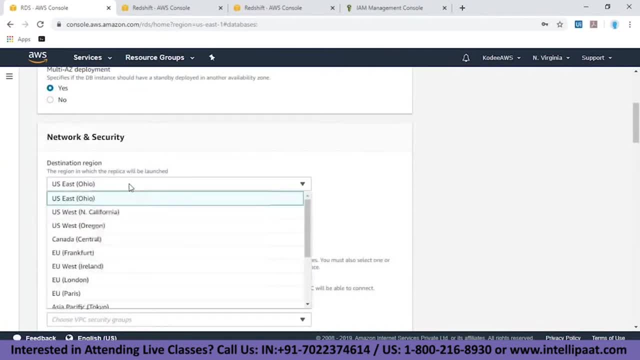 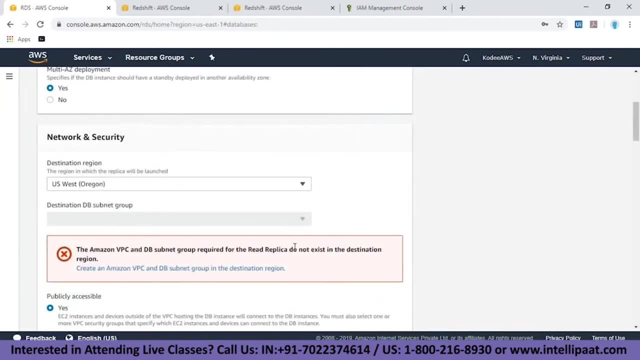 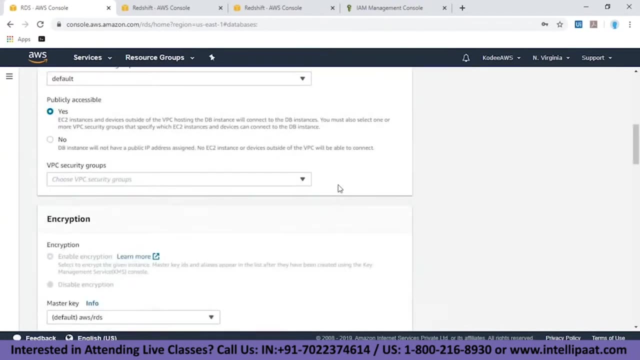 will have to create one. choose, then choose that region. I'll go to Oregon because it's already open. I'll go to Oregon, and so Amazon VPC- Okay, it does not exist in this region. So I think they only provide you certain regions. 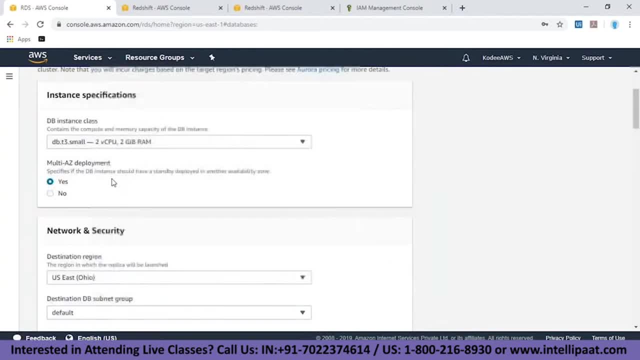 I think so. Yeah, they provided Ohio, So I went with Ohio. It's going to be. no, it's not multi-AZ. You can select your DB class here. Also, You don't need to have the same class as your primary if you are. 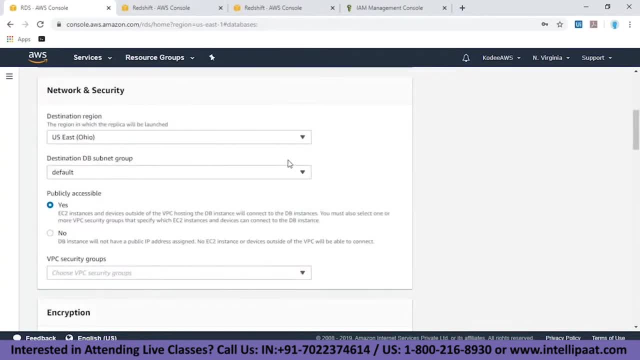 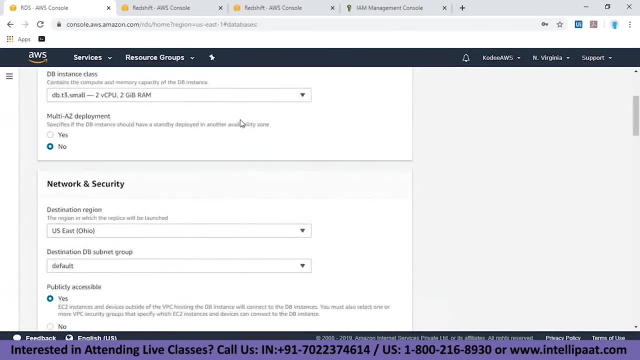 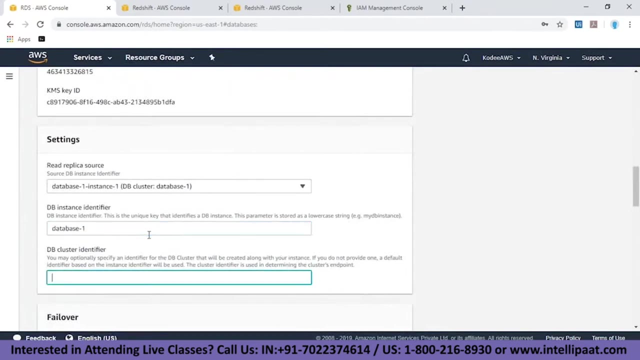 going to use this particular region infrequently, then you don't need to give a powerful instance type. You can just choose a normal one or less lesser powerful one. then every thing will be the same. just left to provide the identifier, one, cluster, one and then. so this is not required. 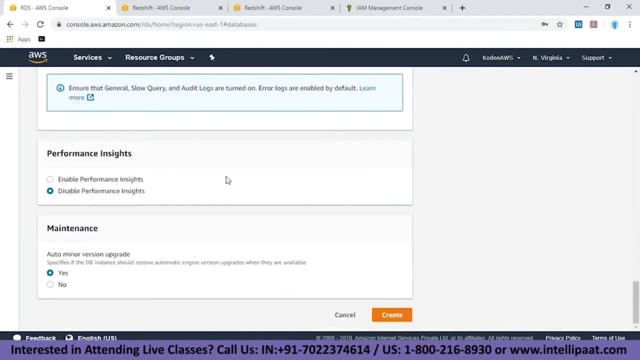 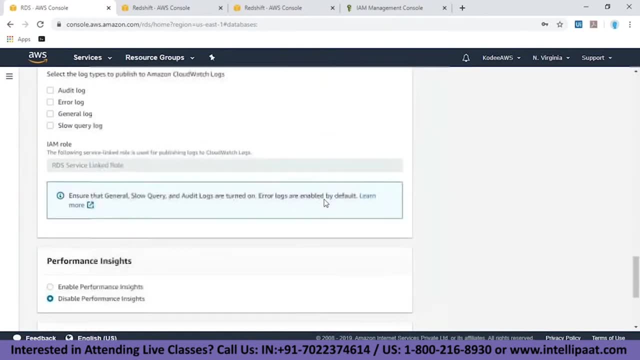 Okay, enhance monitoring. I don't want performance inside, So yeah. so now, if you create this, I think it's going to be a lot more complex, but it's not going to be too complicated, So I'm just going to do that. 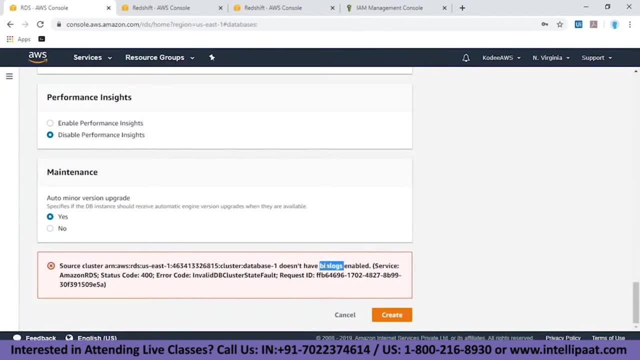 So I'm going to go back to this one So you can see that the database is still in the program. So if you have any more questions about this, please just put them in the comments section. Okay, we should also. they provide another thing. 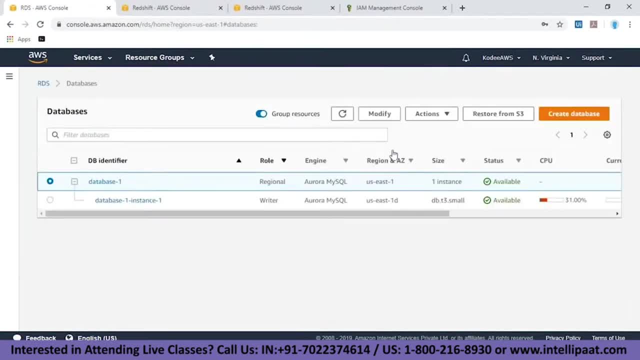 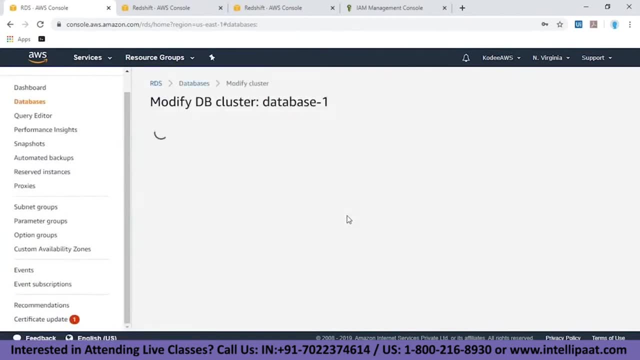 So database one doesn't have bin logs enabled, So we'll have to enable bin logs for this. So I think I'll have to go to the parameter group. So if I go to the parameter group, I see that it's not going to be the same. 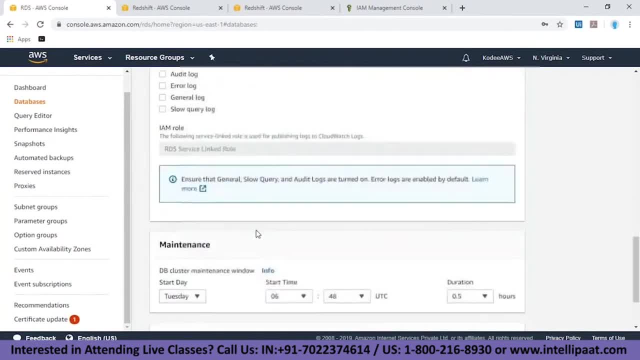 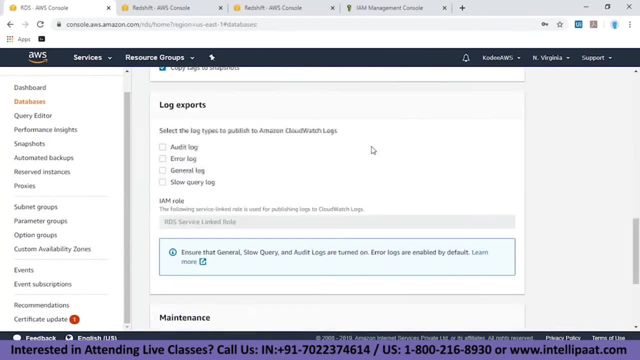 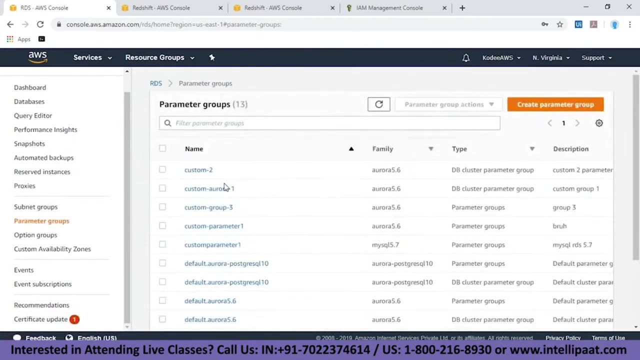 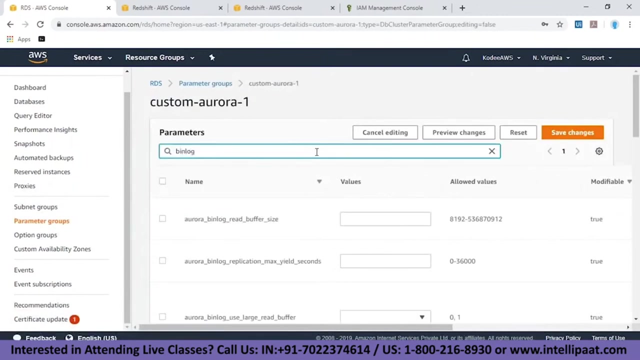 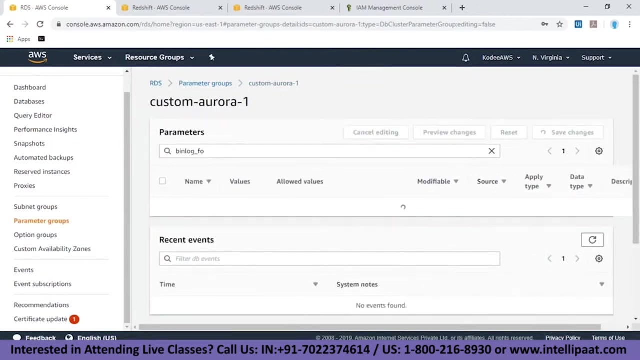 So I'm going to go to the parameter group. So if I go to the parameter group, which is the parameter group for this, change it to customer or a one parameter groups log it is on. I'll just make it, mix it so it is on, but still showing some errors. for that is it saved, think it's. 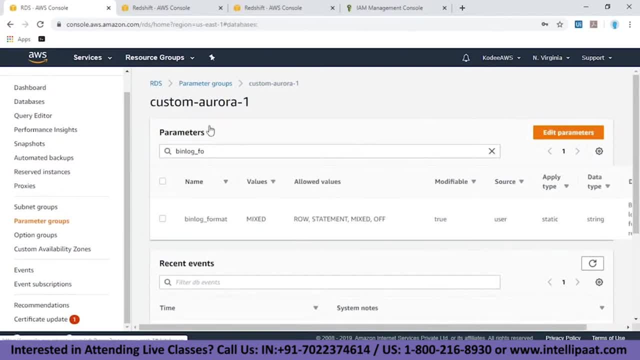 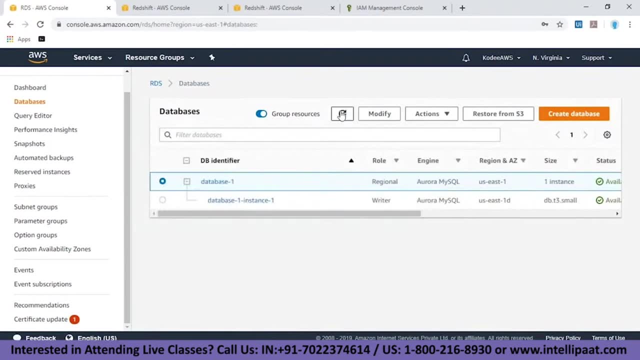 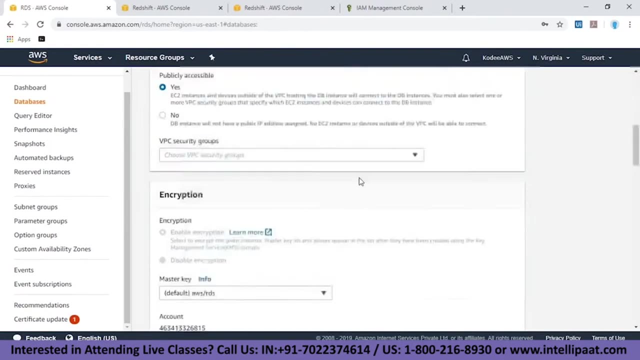 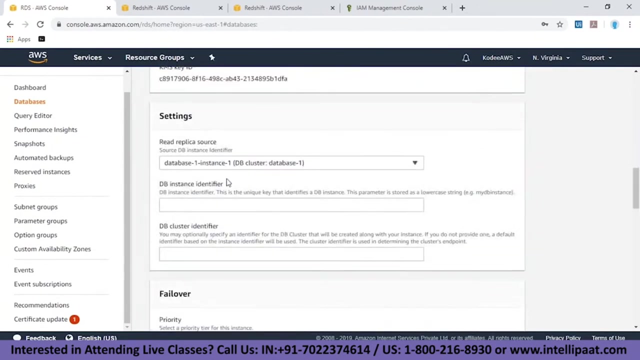 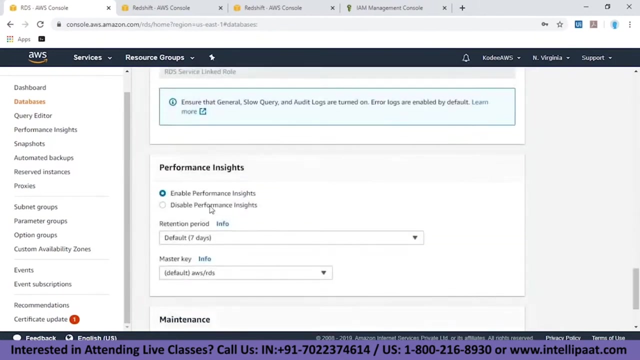 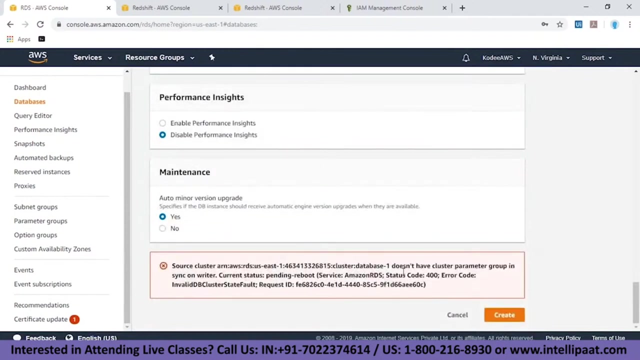 saved. let's mix it. okay. so now it is available. I think it modified. so now let's try once again. Ohio publicly access will know db1, db1 cluster, db, cluster 1 failover: nothing doesn't have cluster parameter group in the system and then it is showing some errors. for that is it saved. and now let's try once again. 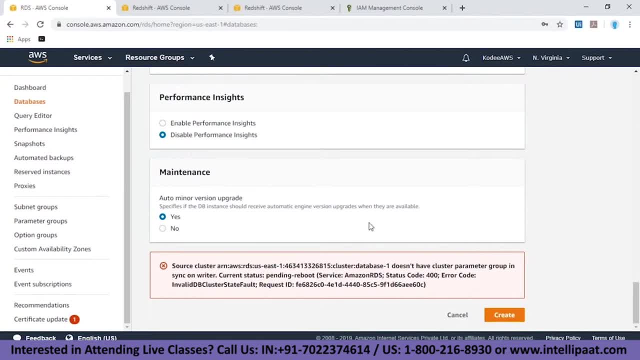 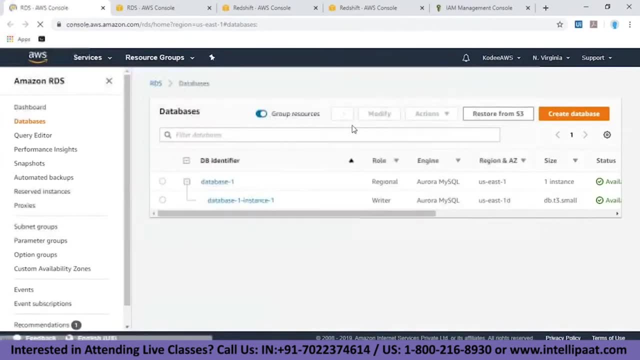 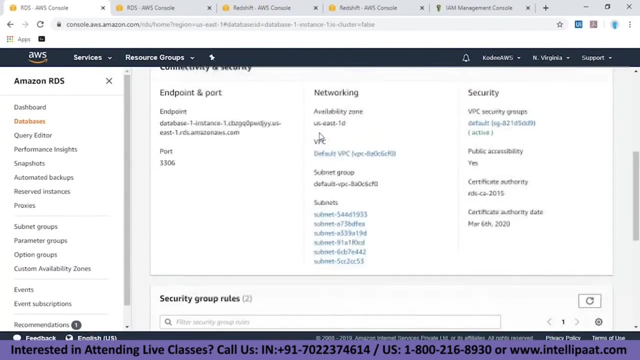 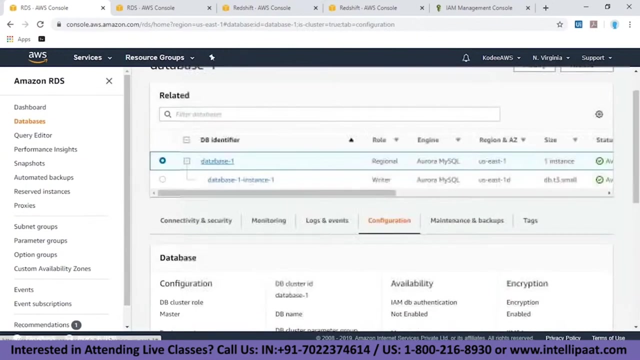 it is showing some errors. for that is it saved. and now let's try once again. sync on writer. it's still modifying. once it modifies will be. it's not on sync. oh yeah, I think I'll have to. there is that configuration. it is in sync, but I just 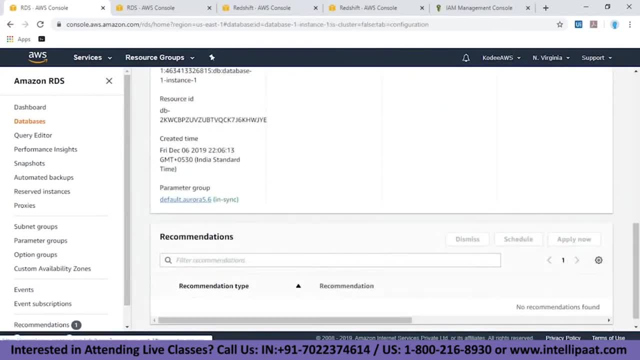 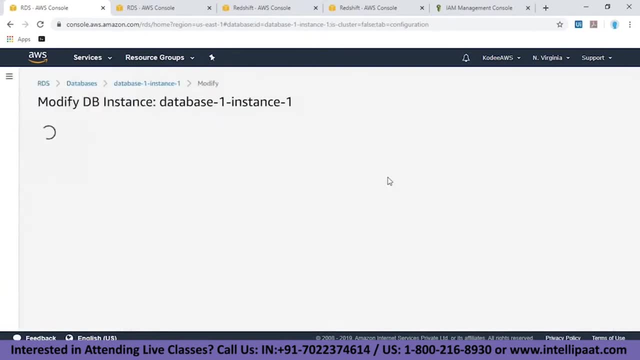 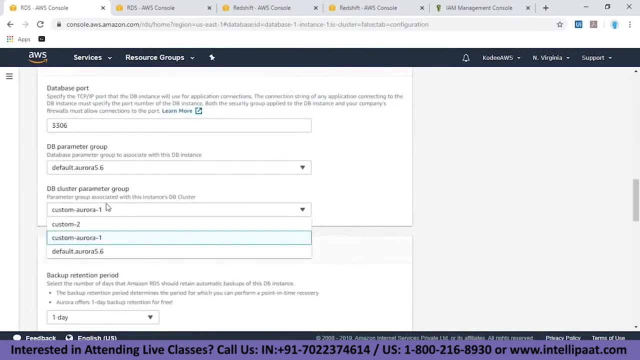 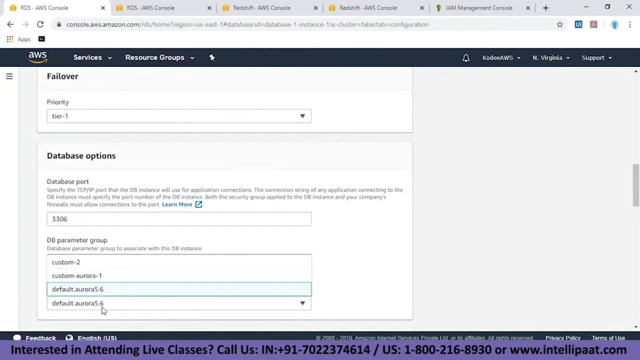 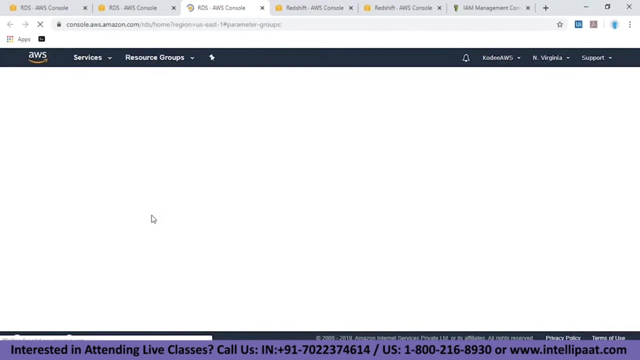 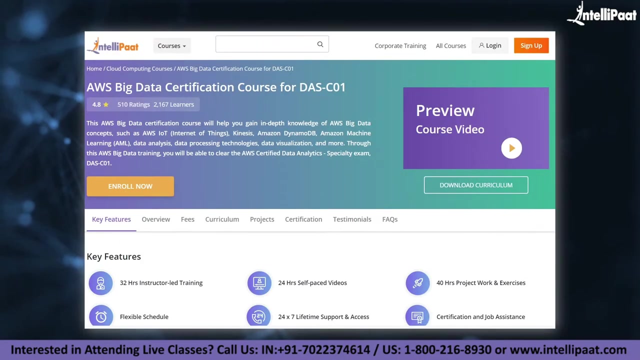 changed the parameter group. why is it cluster? cluster, parameter group one. I think that's just as I can. guys sell just a quick info. guys in telepath provides AWS big data certification codes mentored by industry experts, and the course link of which is given in the description below. now let's continue. 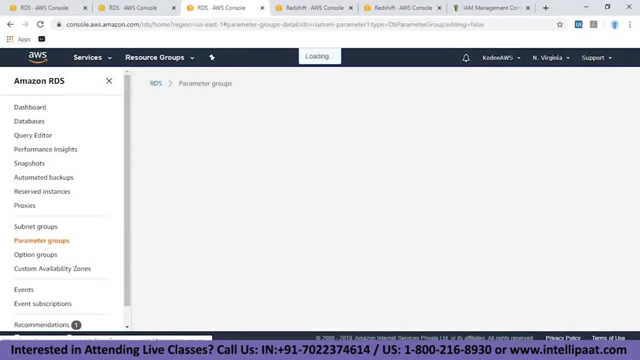 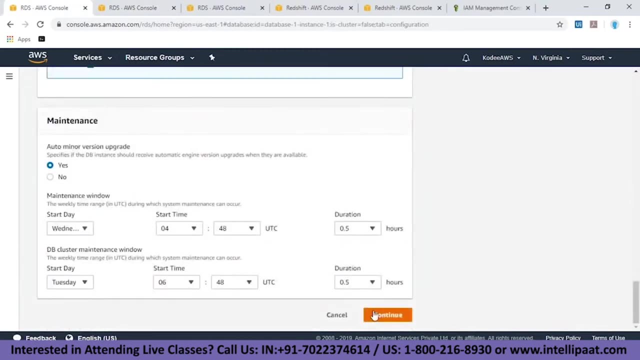 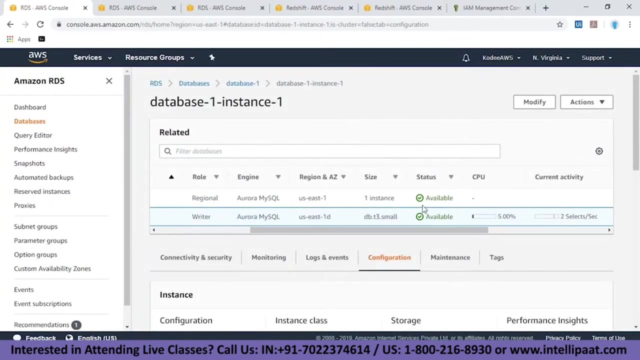 with the session, then log for my. it's not available for this custom Aurora, one selected customer over one also, so now we'll try once again. so the thing is for cross-region replication: your bin logging should be. binary logging should be on for the databases which you are doing, databases which you're doing. 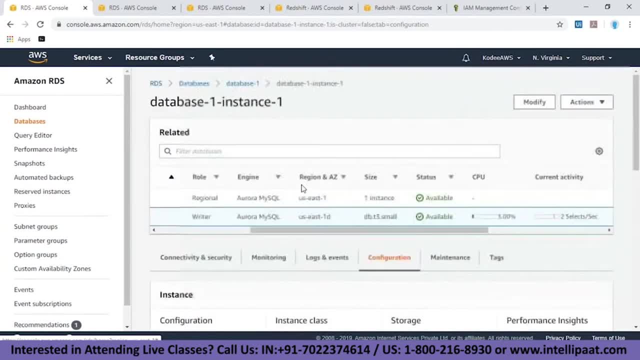 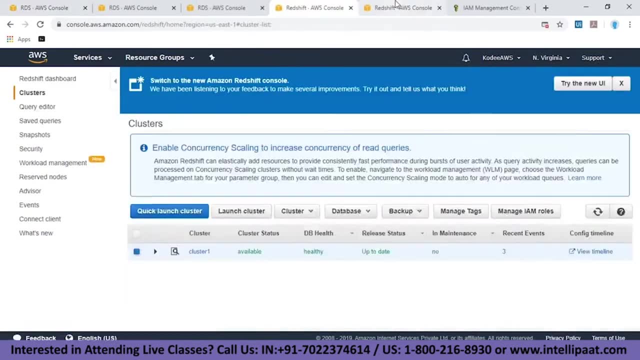 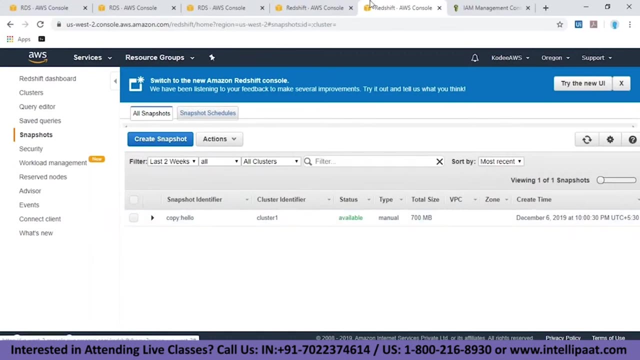 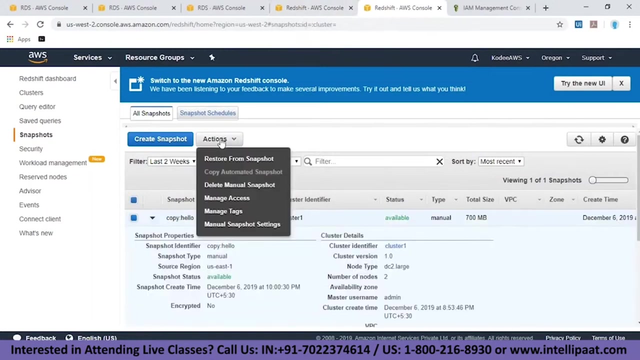 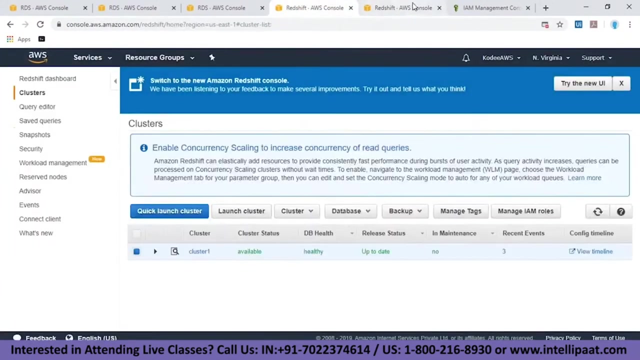 replication for so it's applying. you create here. yeah, so, so the copy has been created. and Oregon, so we've enabled cross-region or snapshot replication. so it has created, so now I can directly restore from my snapshot. yeah, so this is one thing we can do. I'll just delete these snapshots. okay, now, coming back, 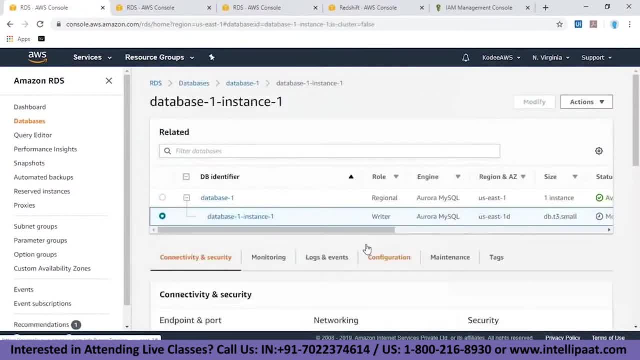 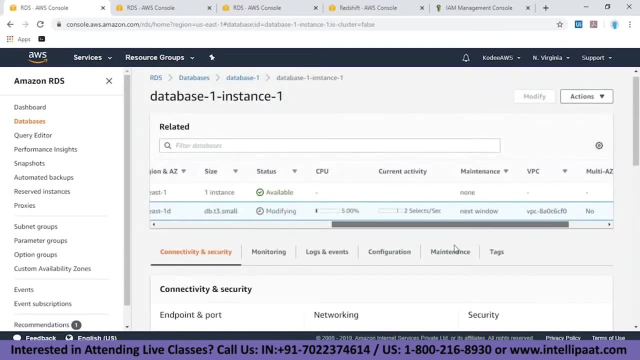 here it's modifying. so even in the last session we had the trouble of that been logging in RDS. but in our local MySQL databases we'll have what is that? we'll have the authority to change the configuration files so we we can change whatever we need. but here the only thing we'll have to do, 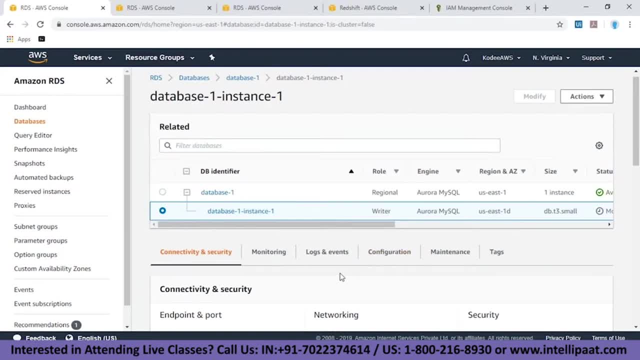 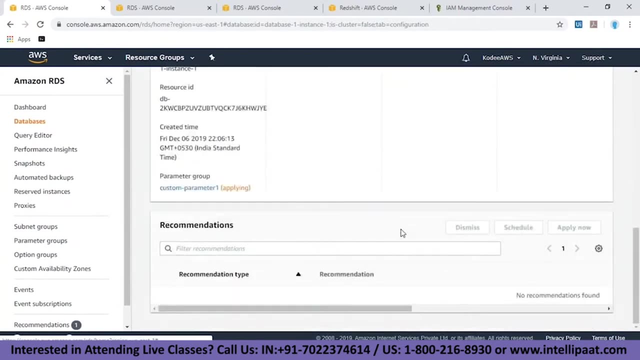 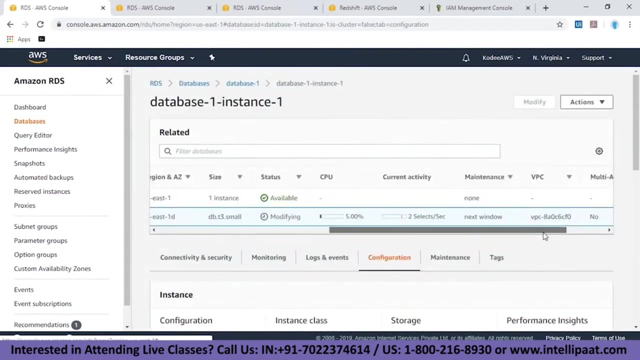 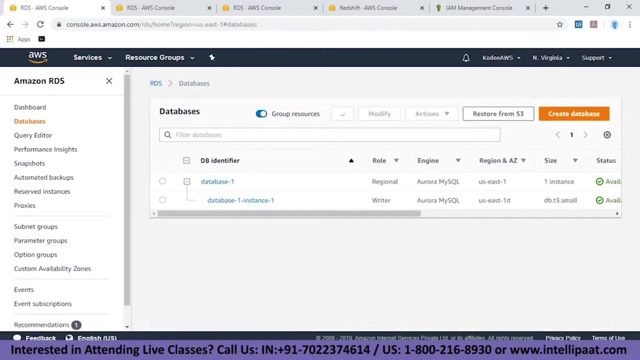 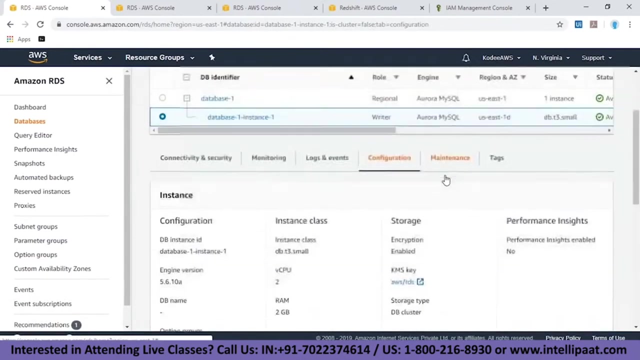 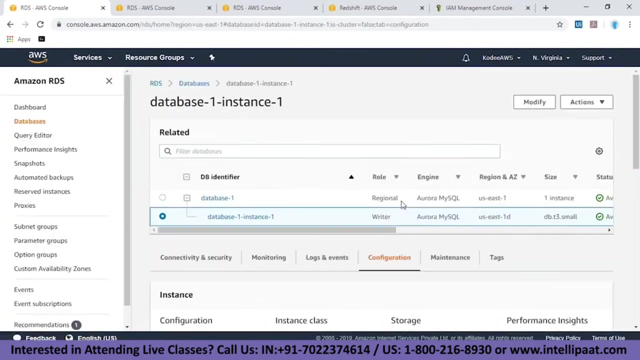 for enable bin logging is making bin log format either from mixer or it should not be off. it should be at least a row or statement or mix it. so if it is there, then bin logging is available. still taking some time. it's available pending reboot, so I have to reboot this. so once I reboot the changes will be made. so 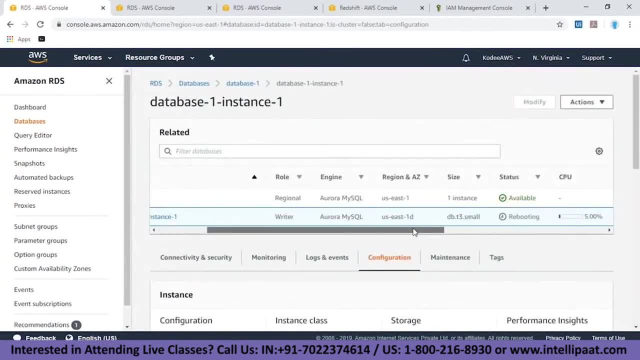 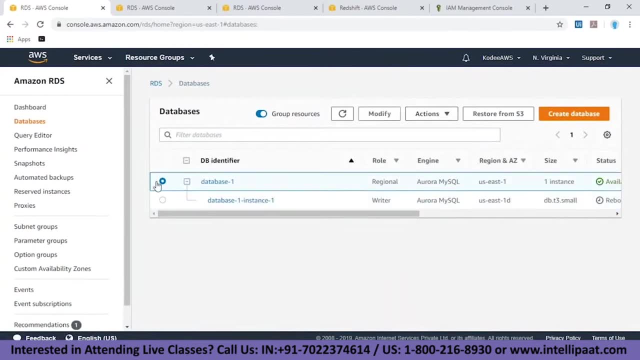 once the changes are made, then we'll be able to- uh, I think we'll be able to- cross-region replicate. so the thing is, it's just simple to cross-region replicate. you'll have to choose the database cluster and then you'll have to choose the database cluster and then you'll have to choose the database. 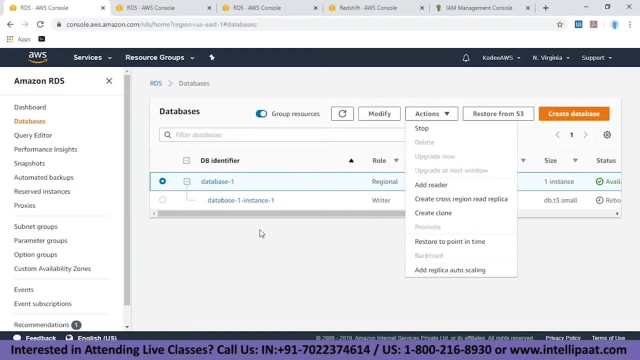 cluster and hit this, you can. if you want to create one more replica, go to add reader. if you want to clone this entire database- uh cluster, go to create clone. and if you want to restore to the last known snapshot, not the uh, so you can go with this. if you want to create or auto scaling for replicas. 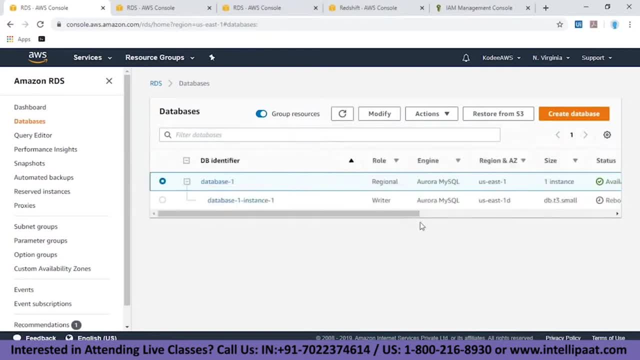 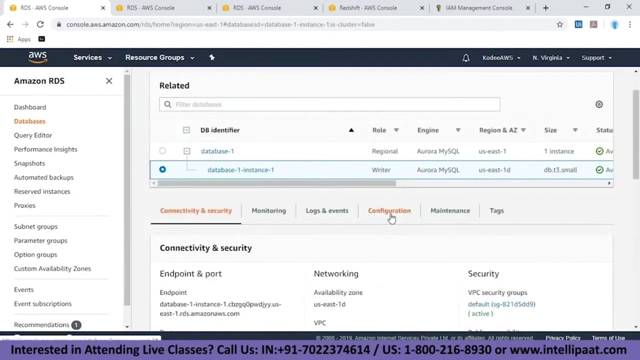 go with this, so yeah, so right now it has to reboot. once it reboots, we'll check once again for cross-region replication. I think it's available. so has occurred. we go back to configuration in sync. yeah, so I think we'll be able to do right now. let's 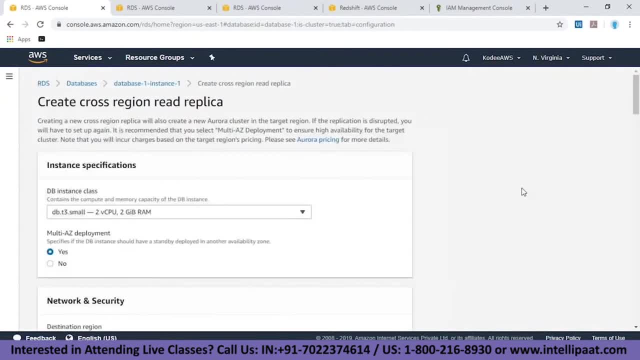 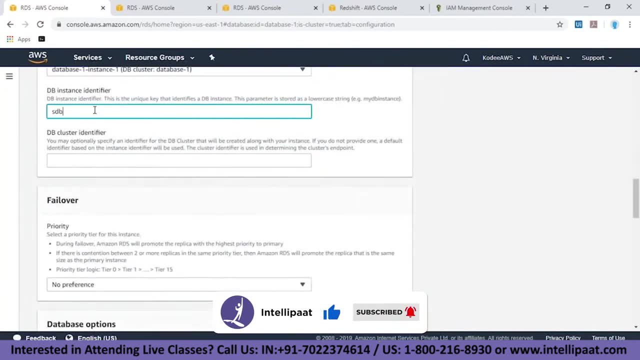 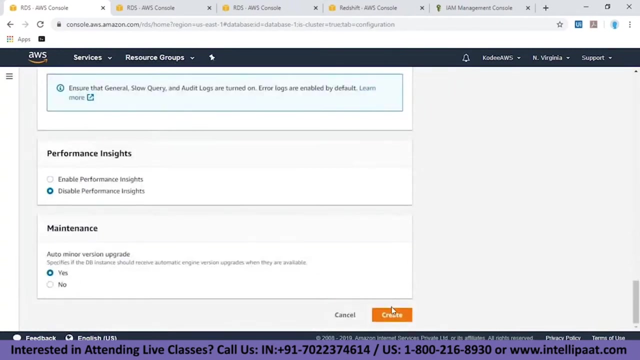 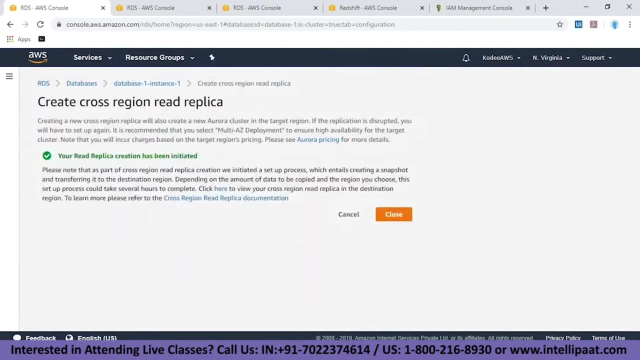 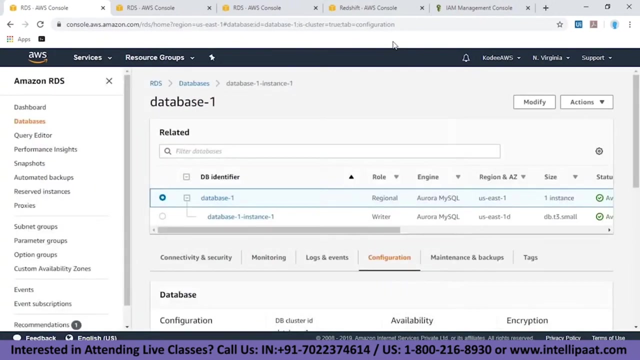 check once again. yeah so. so I did the same thing in the last session, but it still showed: bin log is not. what is that not enabled? so I don't know there are some bugs with this. so so right now the read replica has been initiated. so right now we'll have to go to Ohio region and check whether it is getting created or 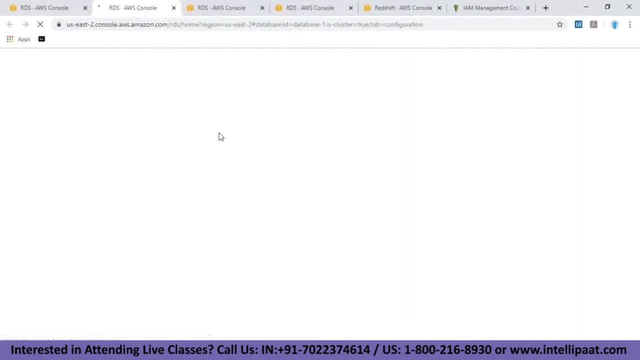 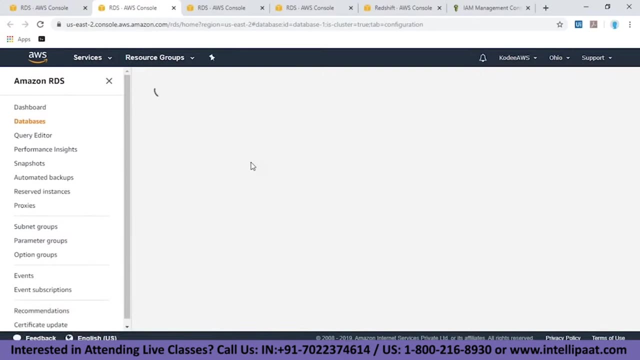 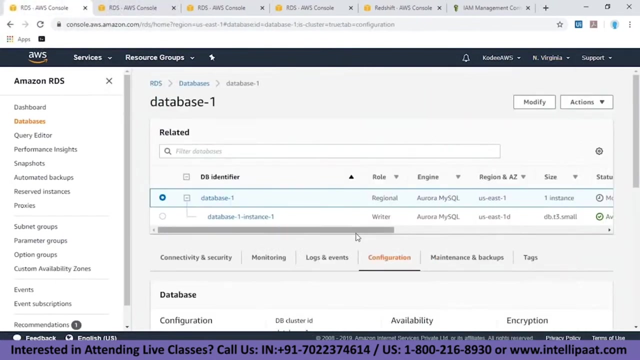 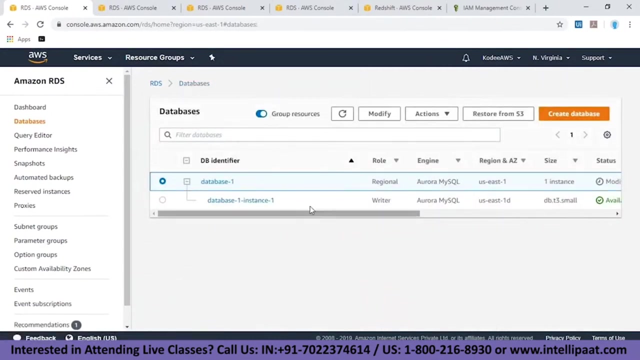 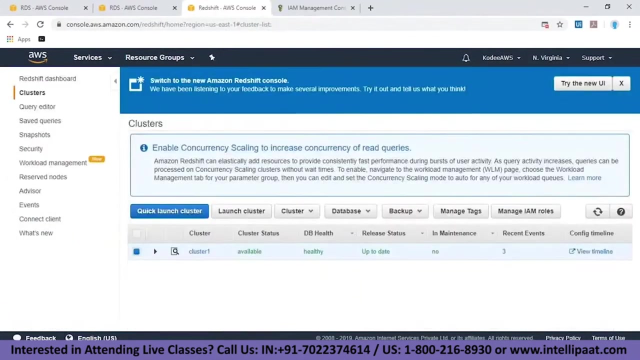 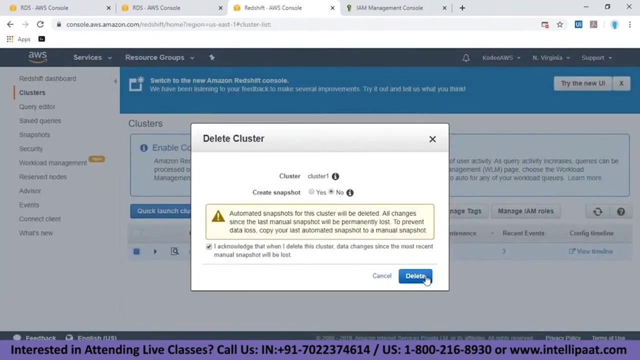 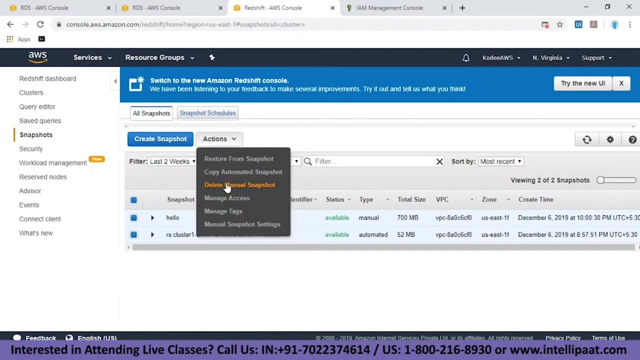 not okay, it's too slow. I said I don't know why, so I think once it completes there, I'll be able to see this: just close these, close these. I do not have a free, so I'll have to delete it. I have to delete my snapshots, so I think this will. 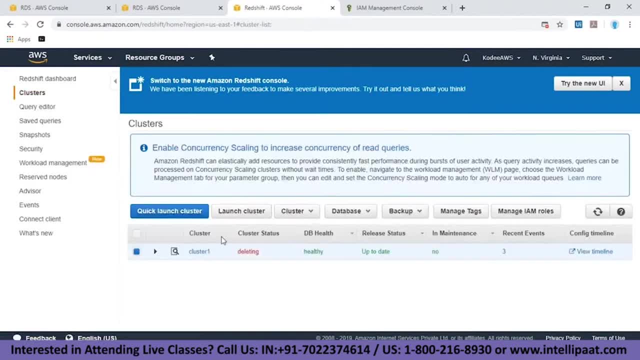 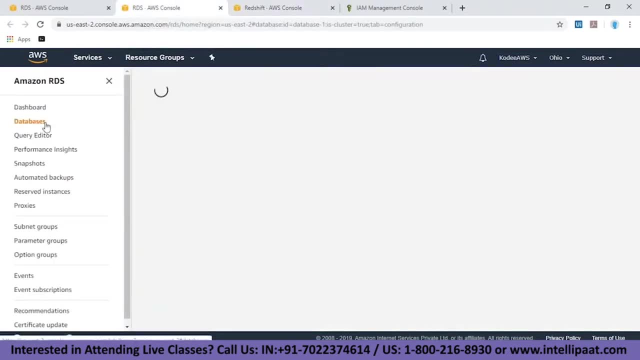 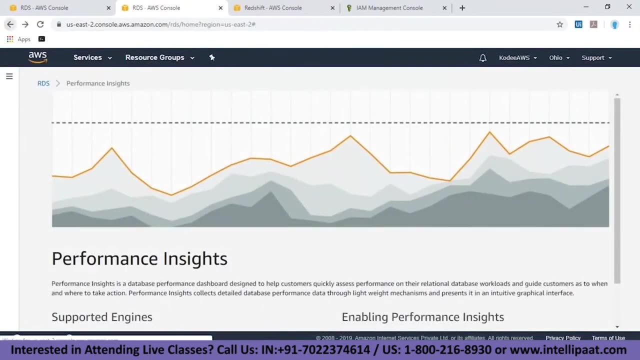 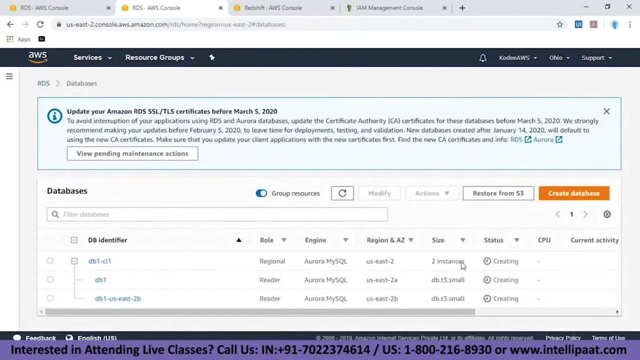 get deleted. once the cluster is gone, then, fine, it's still loading. yeah, it came, it came. okay, so there are. so yeah, so we've created. so there are two instances. I think I clicked on. yeah, so I unchecked multi availability zone, I guess. but okay, I do not. 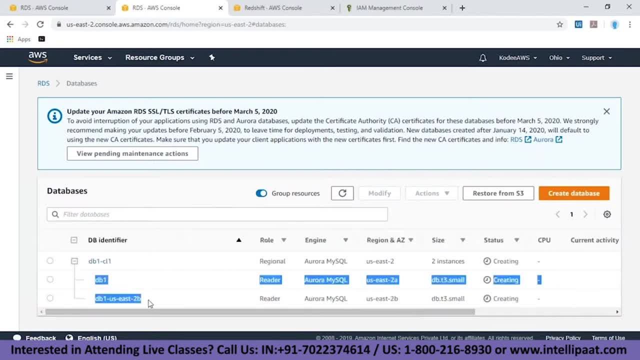 remember properly. so so it created two reader, because for me they both are readers, and you can see that over here, so I can see that over here. so I can see that over here, so I can see that over here. so it's a click of a button to create a cross-region replica for your existing database. 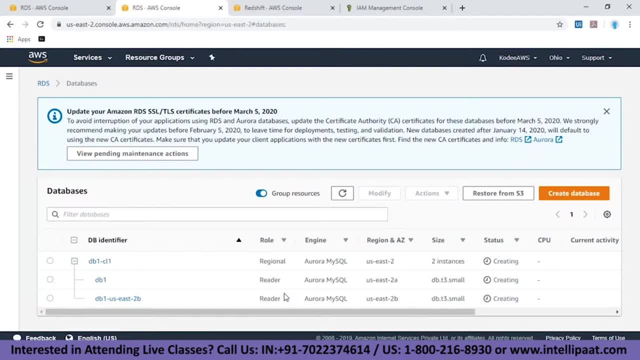 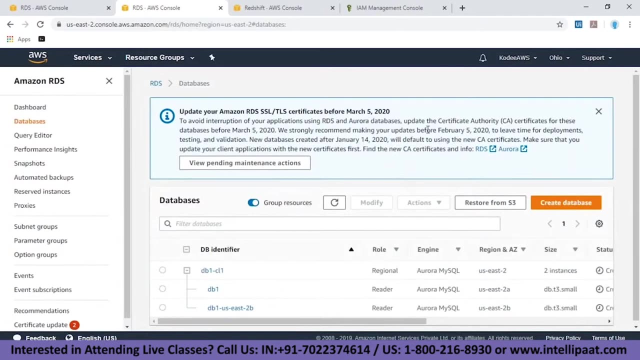 clusters. you cannot replicate your primary database instance directly. you'll have to take a snapshot of it. and after taking a snapshot of it, you will have to copy the snapshot to here, after copying the snapshot to the particular region where you'll have to create that database from. 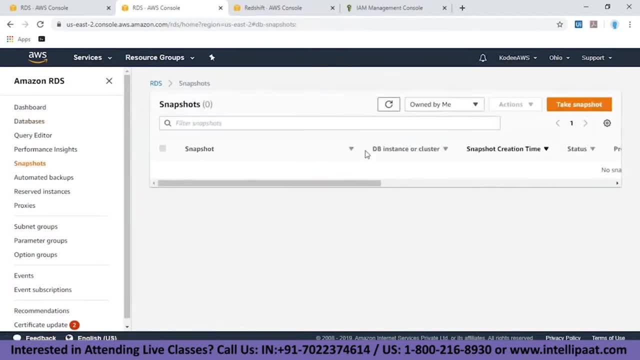 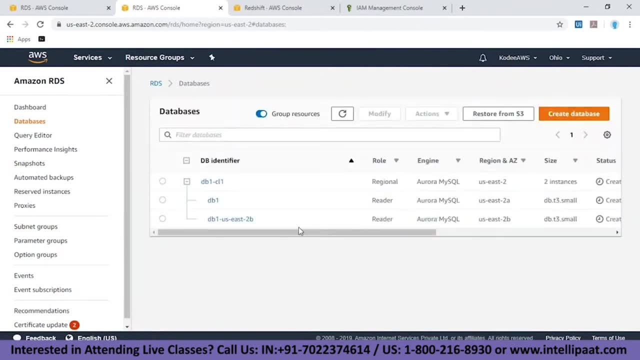 that you will have to use that snapshot. we'll have to use that snapshot to create a database cluster out of it. so that's how you'll have to do it. so right now it has just created a reader reader notes- sorry, not notes- so it has created reader instances. so DB 1, DB us, is to be. it has created 1 in 2 a and 1 in 2 B. that is multi. availability zone deployment. it automatically did it for us, so yeah, so it will take some time to first create after creating a database, so that's how you'll have to do it. so right now it has just created a database. so that's how you'll have to do it. so right now it has just. 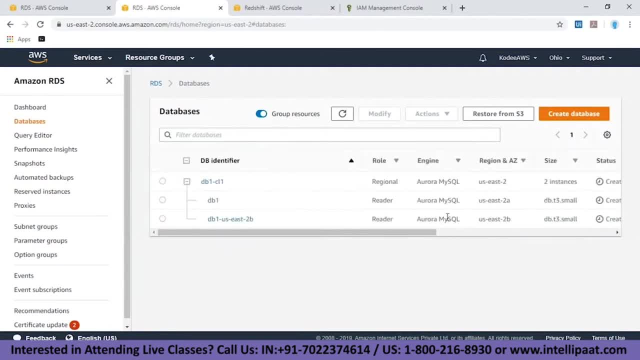 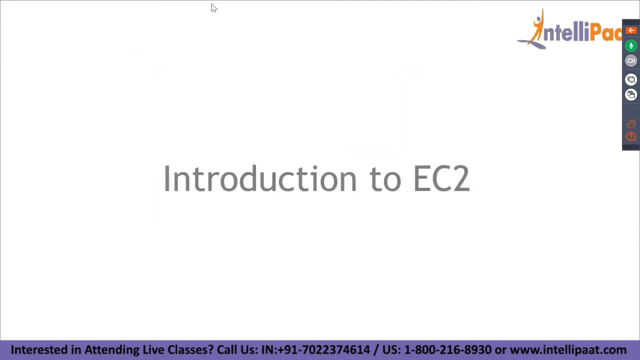 creating it has to copy the data so it will take some time to load. so this is how we do it. uh, we'll be looking into aws easy to it's introduction to easy. we're not going to concentrate much on the uh theory, so I'll just give you all the briefs, make you understand and 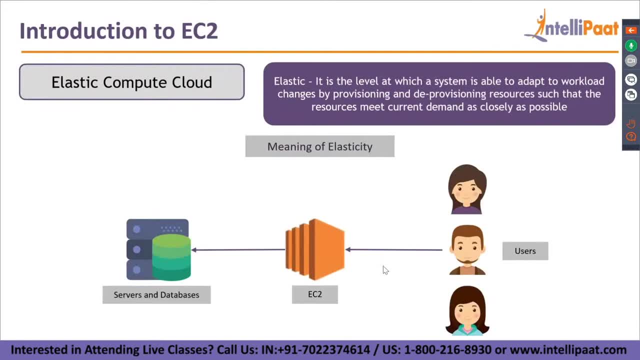 let's move on to them. now, coming to introduction to ec2: uh, ec2's full form is elastic compute cloud. so first let's understand the first word, which is elastic. uh, if you have a server in your online code connection, if you say that with, does OnPremise an我们需要 Polymer. 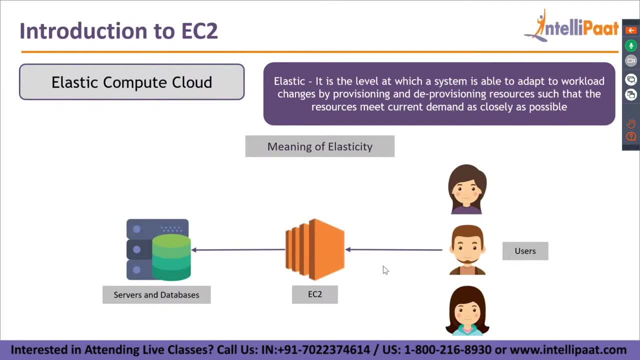 Umm for my setup. let's say you have five servicons to host your website. now you want a sixth server because your website's popularity is increasing. so your, your website is getting much and much more and more popular, so in that case you will need another server. so to get another server, what? 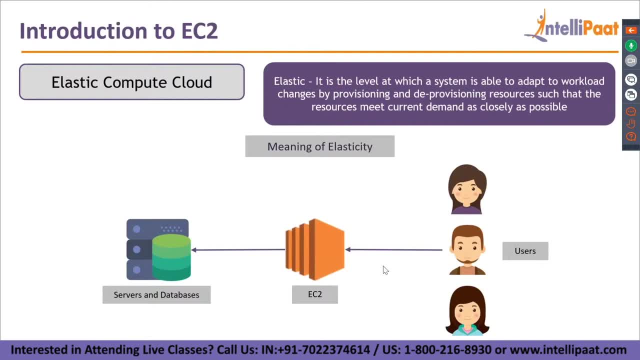 you do? you go and purchase a system, you bring it, you configure it with the appropriate softwares, you push your code into it, you set it up and you have six servicons right now, but, let's say, after two weeks, your websites' 12800'0003希望ентов. 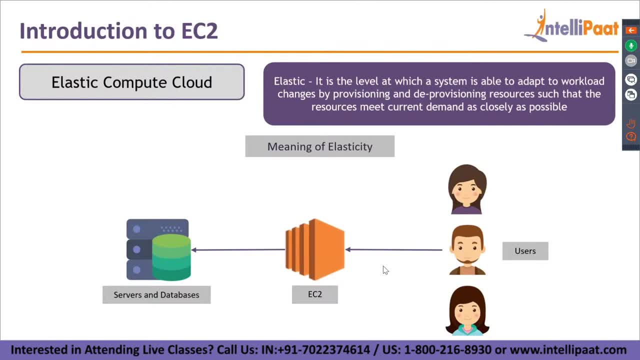 or your website's interest goes down by 50%. In that case, only three servers are needed right now, So you cannot just sell the other three servers because you have invested in them. And even if you sell it, they'll go for less price. 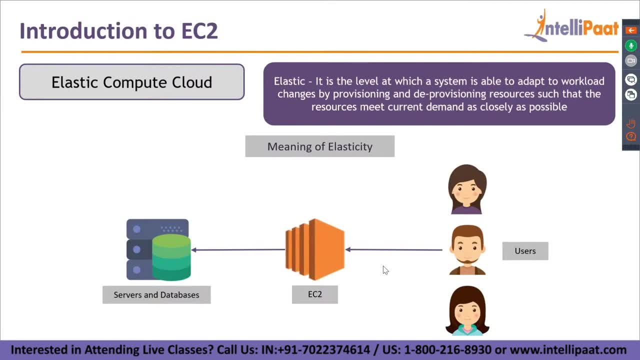 So exactly to solve that particular thing EZ2 came and the elastic part of it is the yeah. So that came to save us from that compromise setup that we'll have to invest capital to buy servers and then host our code in it. So now, elastic, it basically means it is the level. 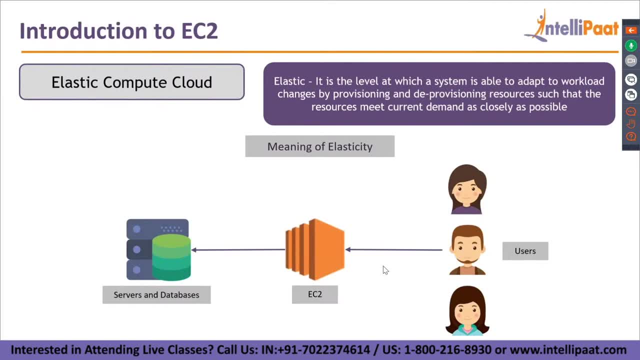 at which a system is able to adapt to workload changes, provisioning and deprovisioning resources such that resources meet current demand. So that basically means so the servers which you launch in EZ2, you can set up a scaling policy which basically determines to provision. 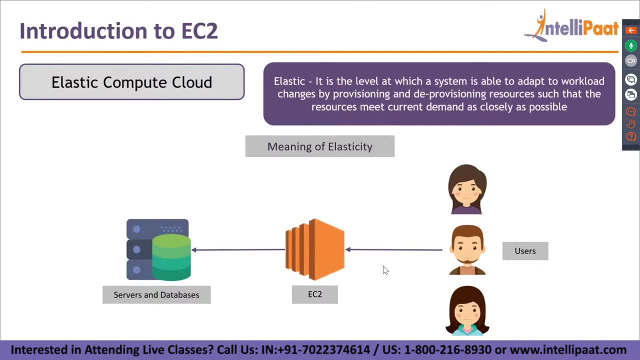 or deprovision the resources. That basically means increasing the servers or decreasing the number of servers according to the current demand. So there is a service for this, particularly called auto scaling. We'll not be looking into that. We might look into that in another session. 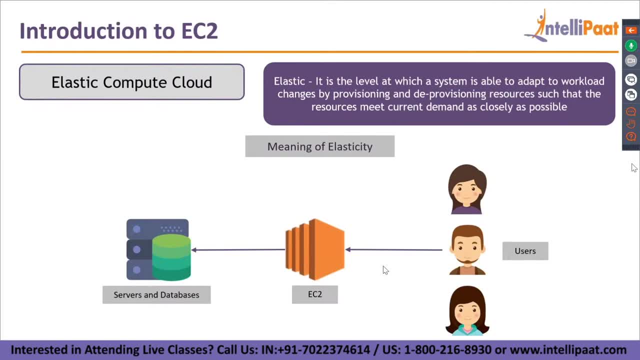 So that basically is Elastic Compute Cloud And also it is cost optimized because you only use, you only have the number of servers you need at that point of time. So right now you can see there are three users using EZ2 and EZ2 is provisioned a particular server. 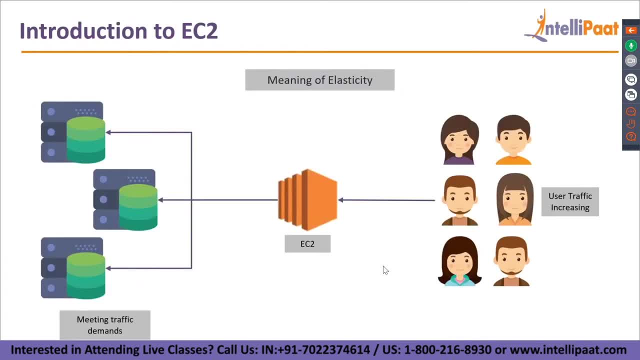 So this is the server which is handling these users. So now, let's say there are six users and you're using these servers, So each server can handle two different users. Now user traffic is increasing. Your website is performing well. You need three servers right now. 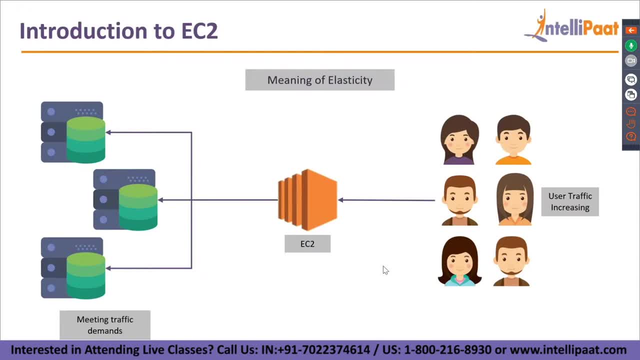 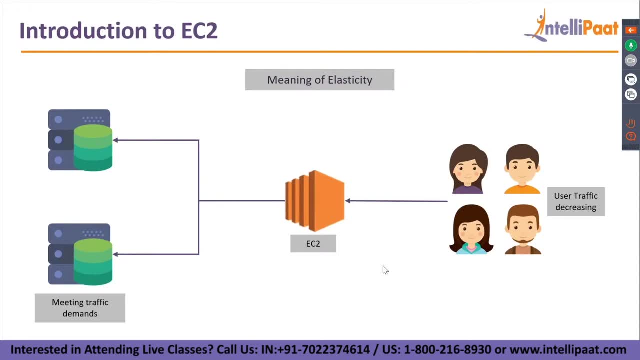 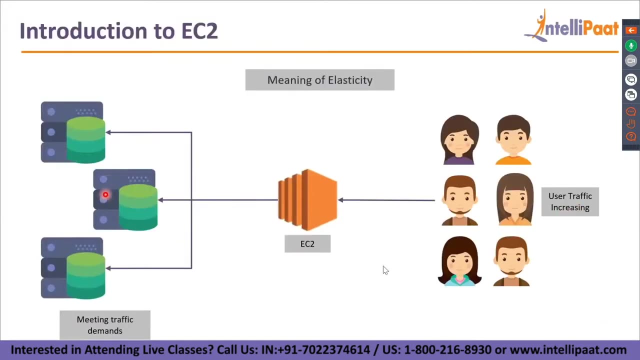 Without three servers, obviously your website would crash. Now, suddenly, your website's popularity decreased and your website's traffic is decreasing. Now there are only four users using a website, So if you have three different servers, there is no need. sorry If you're using three different servers. 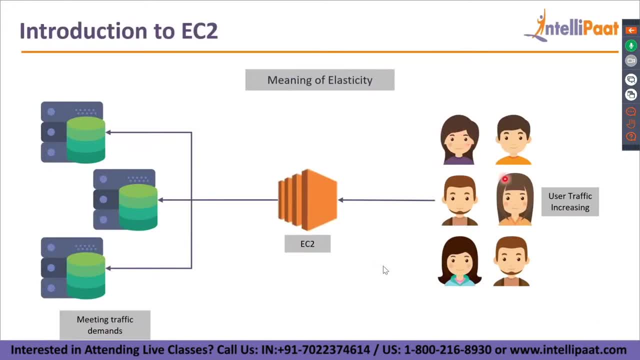 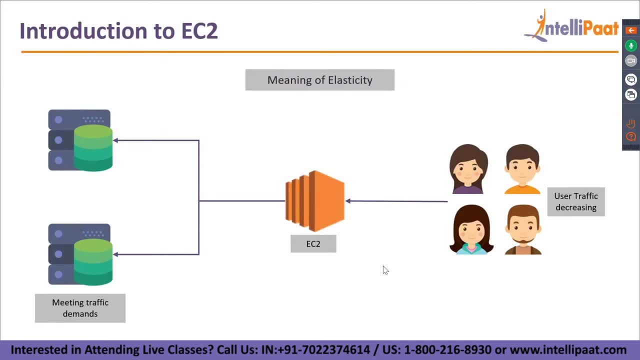 there is no need for one server because two of the servers- the servers- can accommodate four users, So EWS basically does that for you. So you can set up an auto-scaling policy which will decrease the server by one, And now you only have two instances running. 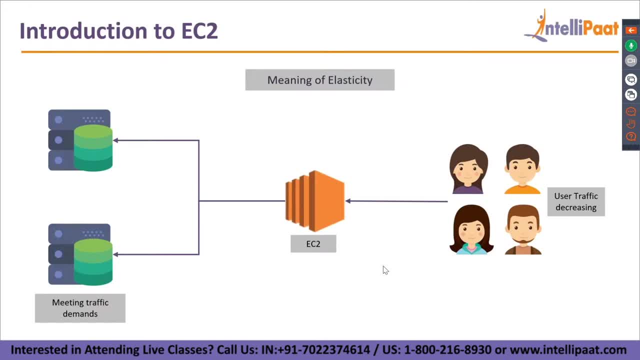 which can accommodate four users. So there are two things which you can benefit from this One is high availability: Your website will be always running, even if the traffic increases or decreases. Second one is scoped optimization, That is, you get, you only pay for the servers. 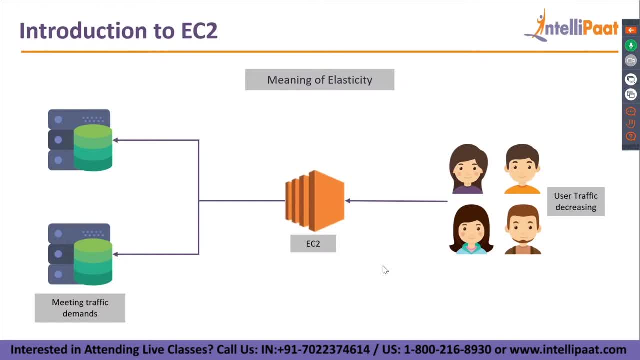 which are currently running, So when there is less traffic, if you want, you only have a minimum number of servers. That basically means you have reduced your cost a lot. Okay, now, coming to regions and availability zones, I wanted to introduce this. 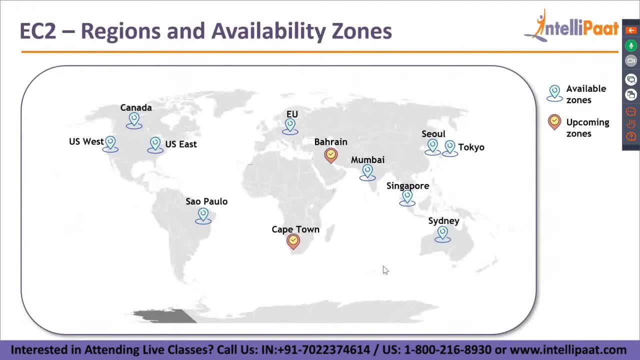 This is not a major concept which you can start off with while you're starting off with EC2.. So there are multiple regions in AWS. You can, let's say, if you're in Singapore, you can launch an instance or a server in US East. 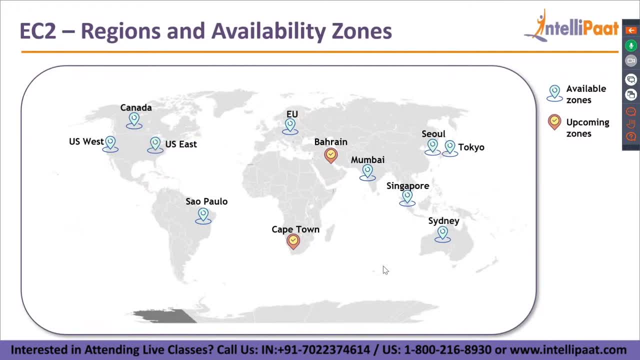 We can launch an instance in Seattle. So you can launch an instance in any of these locations you want. You'll just have to change the location in the AWS console. So the main advantage of this is, let's say, you are a developer in, let's say, in Mumbai. 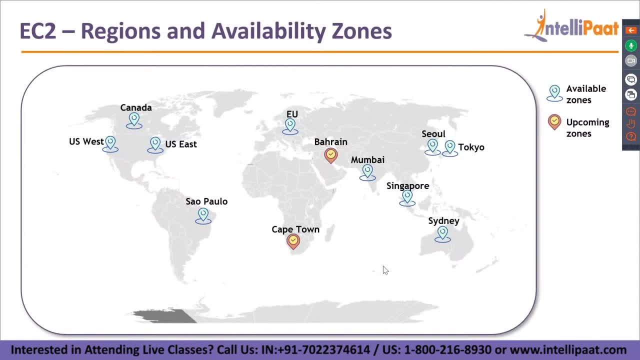 You create a website, you launch it on AWS, So right now you get to know that your customer base is global. There are some customers in Singapore and Sydney, So now you want to move your applications to Singapore and Sydney as well, So that the customers can get fast access. 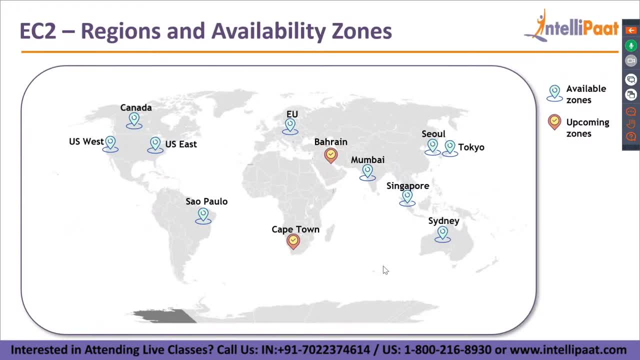 So now what you can do. if it is an on-premise setup, that is, if you have created a simple on-premise setup to host your application, you will if you want to create an on-premise setup in Singapore and Sydney. 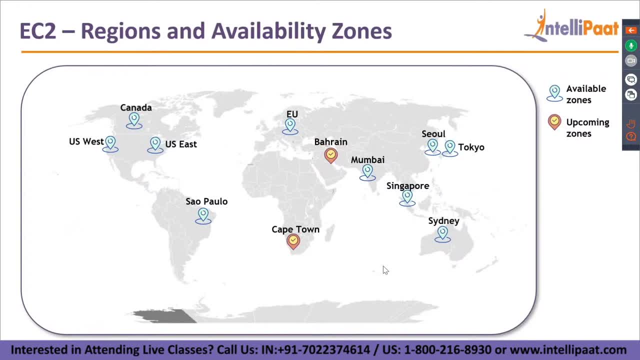 obviously there are a lot of restrictions. You'll have to get a place, you'll have to set up servers and you'll have to proceed with it. But if it is AWS, it's pretty simple. You can just choose the region, create the servers. 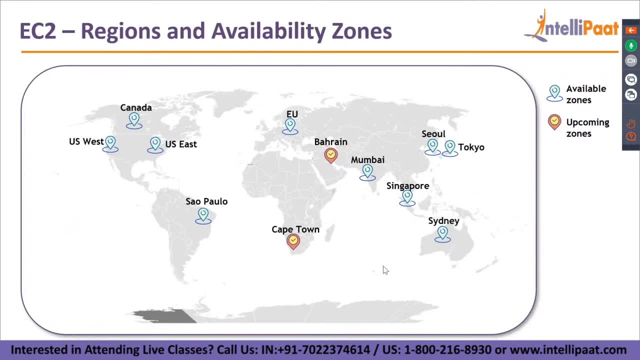 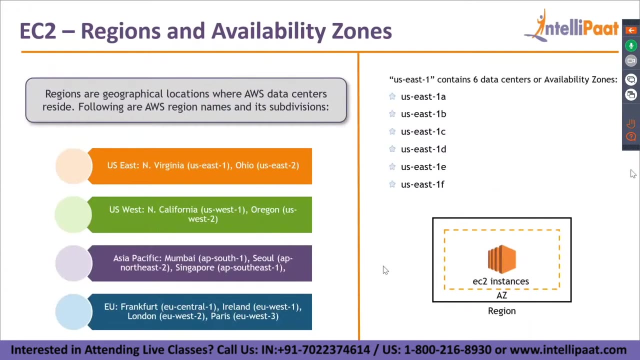 upload your code and your setup. So it's pretty simple. You move your application across multiple regions and availability zones. Okay, so I've explained about the regions. One more thing I wanted to introduce is the availability zones. So there are multiple availability zones within one region. 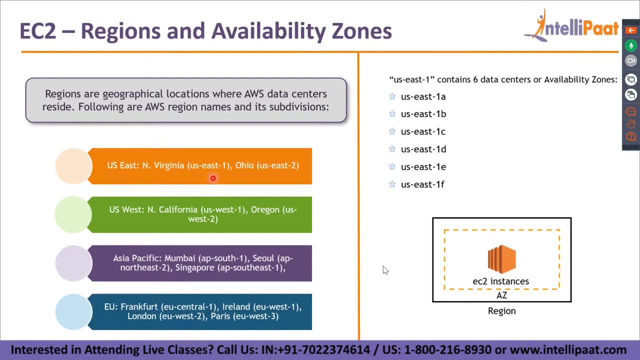 That basically means there are multiple data centers. So if you take US East one in North Virginia, there are six different availability zones or six different data centers within that one region itself. So you can host your data or you can host the code in all of these availability zones. 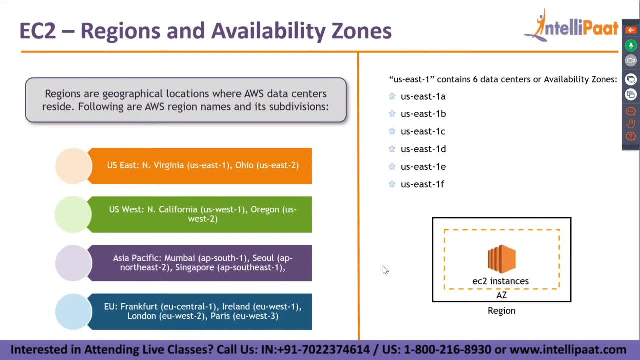 or one of these, or two or three of these. So I'm just giving you an example. These are the geographical regions and these are the availability zones. So it is not that there are six availability zones in all of the regions. You will just have to look into each. 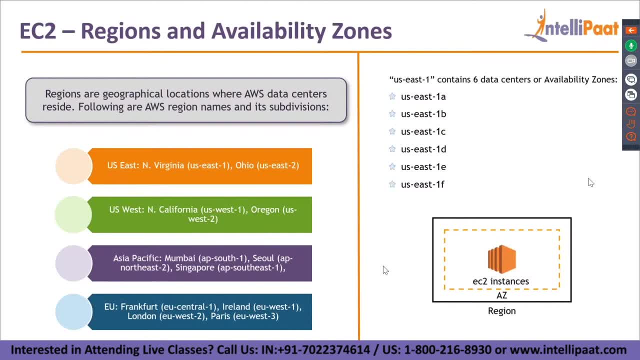 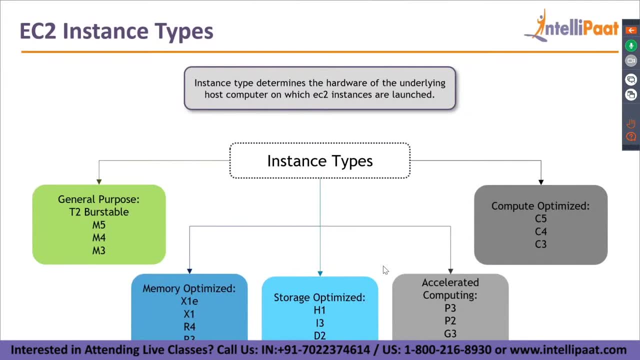 of the region to check the number of data centers which are available within them. Okay, now coming down to EC2 instance types. So this again: there are multiple instance types which can be grouped, each region grouped together in these five different types. 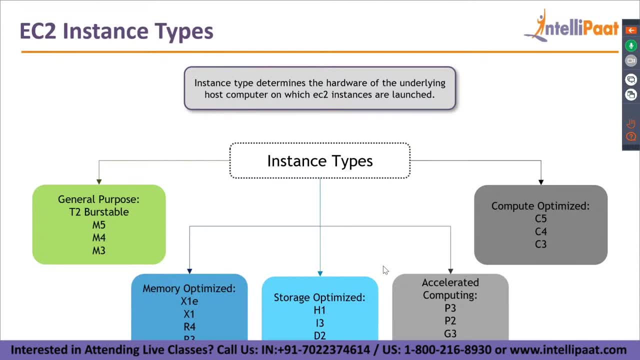 One is general purpose. one is memory optimized, storage optimized, accelerated computing and compute optimized. So general purpose are the instance types which you can use for any usage. It can be for a simple server usage. You can basically store something, you can run simple code in it. 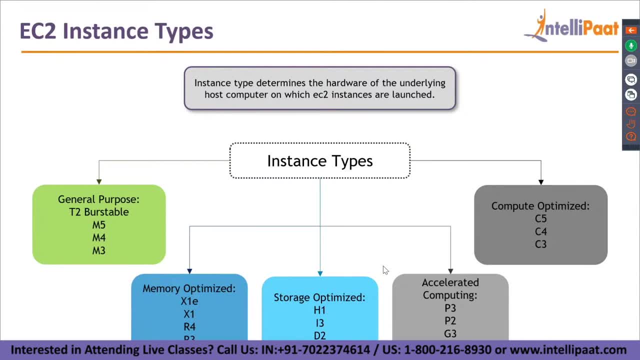 You can. basically, you understood the word right, The sentence general purpose. it's basically for that. Going to memory optimized, you get an increase in the RAM more than the virtual CPU. So you get CPU and RAM in each of these instance types. 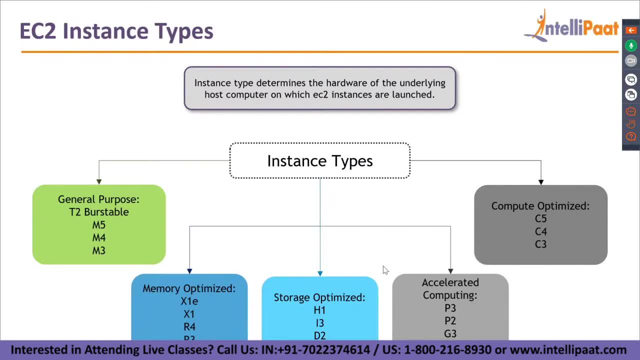 So the RAM comparing to the virtual CPU will be a higher number. So, for example, you might get 100 GB of RAM and 20 virtual CPUs. that is computing power Coming to storage optimized. in this case you will get an increase in storage. 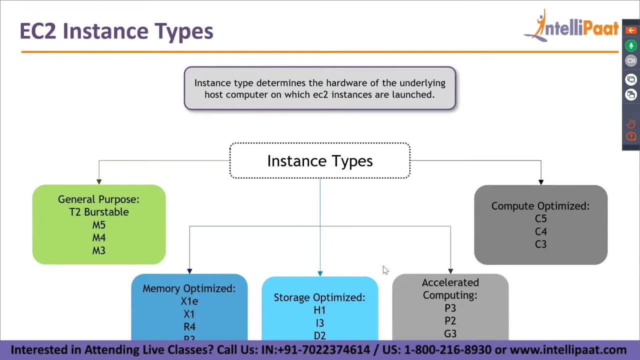 and also you get SSD storage, That is, your storage is faster but it does have more RAM and more data than all the other instance types. So if your application, which you're going to host in your Easy2 server, require a lot of read and write, 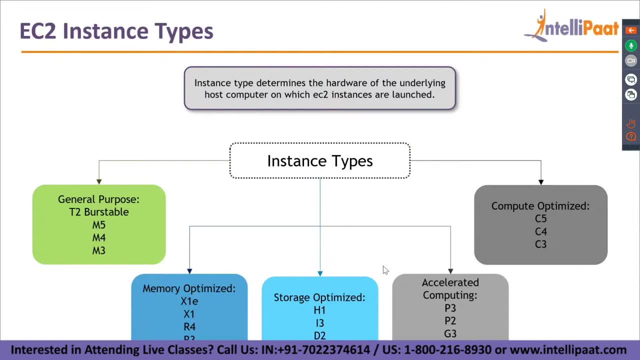 in that case, what you can do is you can use storage optimized instances because they give you an increase in the read and write throughput so that you can retrieve data and upload data to your Easy2 instance, or you can retrieve data from a database which is running inside the server. 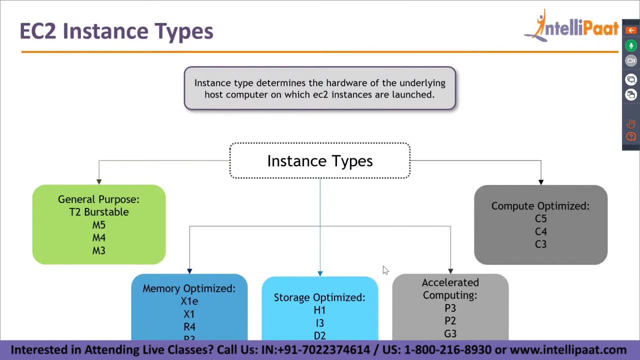 basically faster than the other EC2 instances. Sorry guys. Now coming to accelerated computing. in this case, these instances basically provide you a burstable performance. Let's say you are running an application in these instances which have a baseline performance of 20%. 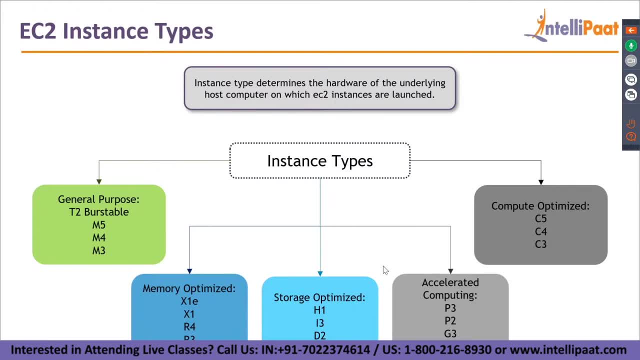 And suddenly an algorithm starts to run and your CPU goes to 90%. If it is a normal general purpose instance, there will be some. it might slow down, but accelerated computing has the power to handle that much, So it can handle high performance computation. 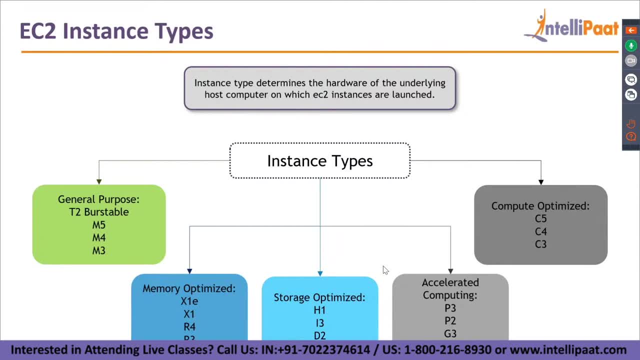 Coming to Compute Optimized, it is basically the vice versa of Memory Optimized. In Compute Optimized, you get more. basically, you can, for example, as I told you, in Memory Optimized, if you have 100 GB of memory. 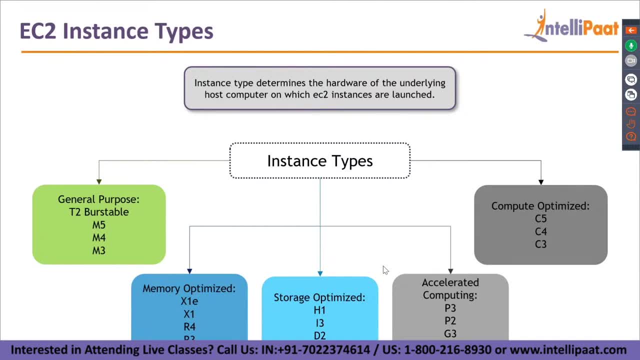 and 20 virtual CPUs. in Compute Optimized you might have 50 virtual CPUs and around 120 GB of RAM. So the Compute Optimized, that is, the virtual CPU numbers, will increase in Compute Optimized. So these are the instance types which you can go with. 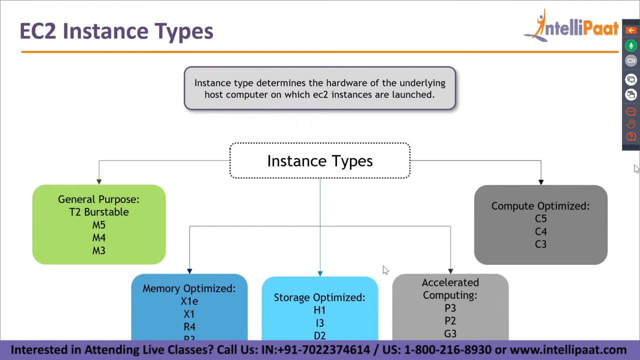 But if you're practicing, if you're starting off with AWS, go with the general purpose instances, because they come under pre-tier. What is meant by M5, M4, X1, E? Okay, so basically they are the names of the EC2 instance types. 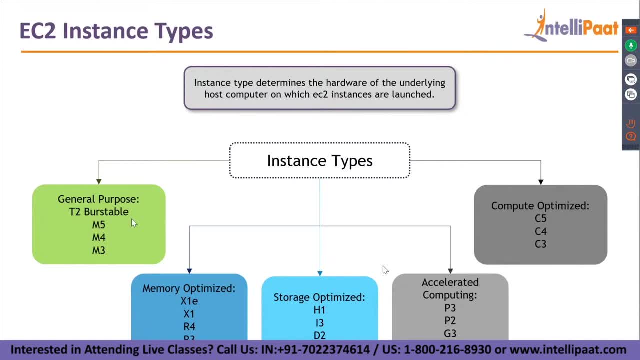 I'll show you while creating the demo. These are, for example, M5. in the sense it'll have a certain number of virtual CPUs and RAM. You'll just have to choose the instance type according to the RAM and virtual CPU you need. 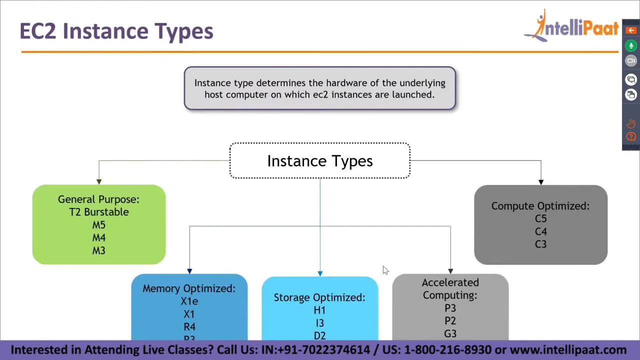 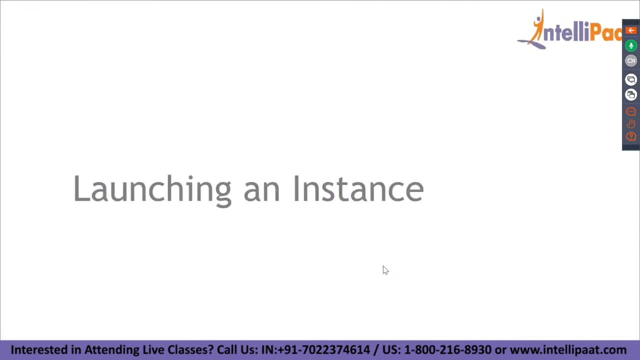 So these are just the names and the group which they belong to. I'll show you once I'm while I'm doing the demo, because the second option is to choose the instance type. Okay, so we've come to the demo and I think you got a basic idea of what EC2 is. 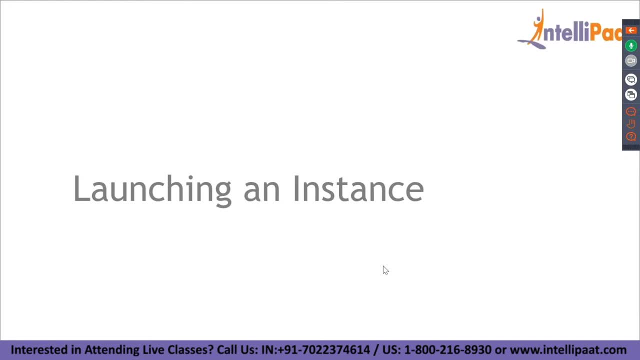 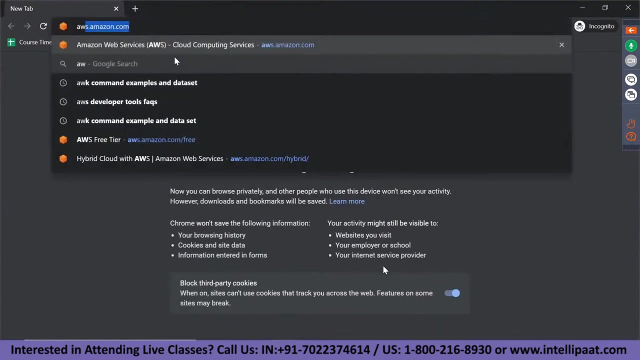 It is basically a server which you can launch on AWS and get access through the internet. Now let me open my management console. So I'm already logged in. So let me show you how to create an AWS account. first, You can just go to awsamazoncom. 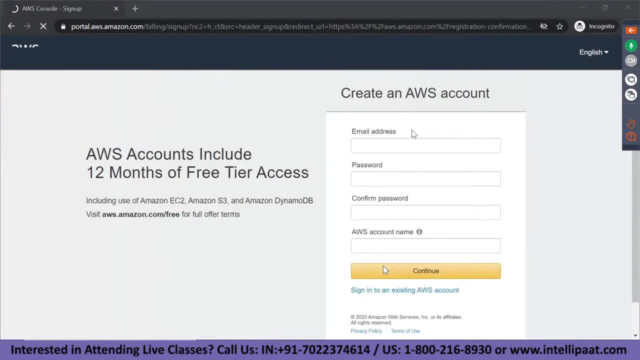 click on create an AWS account, And it's pretty simple to start, guys. You'll just have to provide your email ID password. confirm your password. provide an account name. The next step is basically a payment gateway, where you'll have to give your debit or credit card details. Don't worry about it. You get 12 months of certain free time, So you can just go to the payment gateway. You'll have to give your debit or credit card details. Don't worry about it, You get 12 months of certain free time. 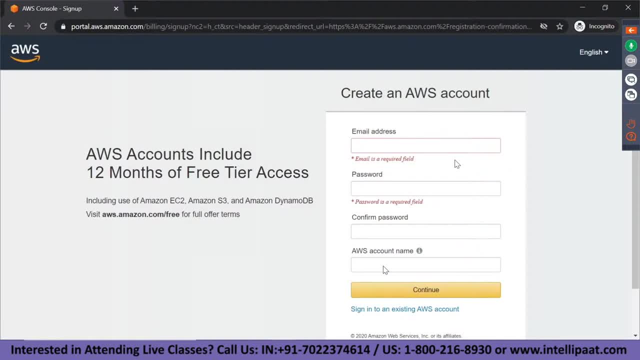 So you'll have to give your debit or credit card details. You can also get free services, which I'll be showing you. So first, it'll take a minimum amount. If you're from India, it'll take two rupees. If you're from US, it'll take a dollar. So I don't know the other country's minimum number, So it'll basically take the minimum currency. Once it takes that, it basically verifies whether your card is real or not, And once it verifies it, they will send back the cash within three to five working days. 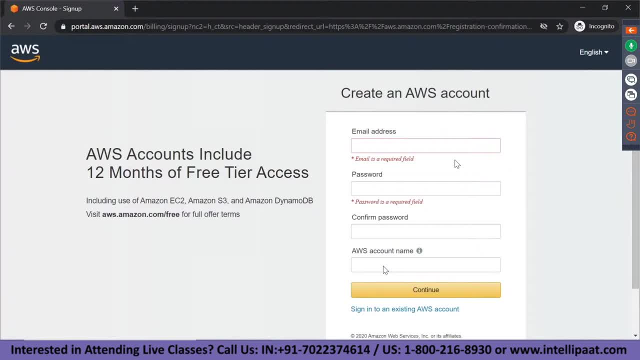 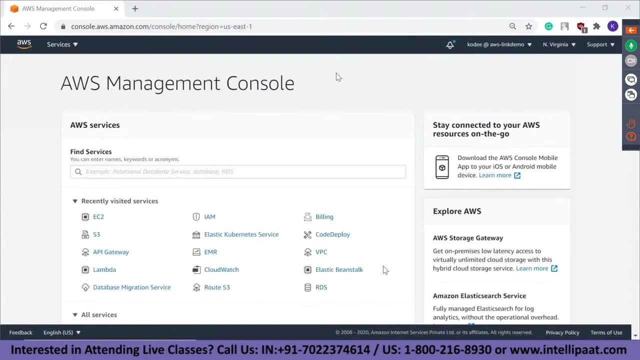 So you don't need to worry about your cash. And once you create it, that's it: Your AWS account would be set up and you can start on AWS off with your work. so once your aws account is set up, it will look something like this: you will have: 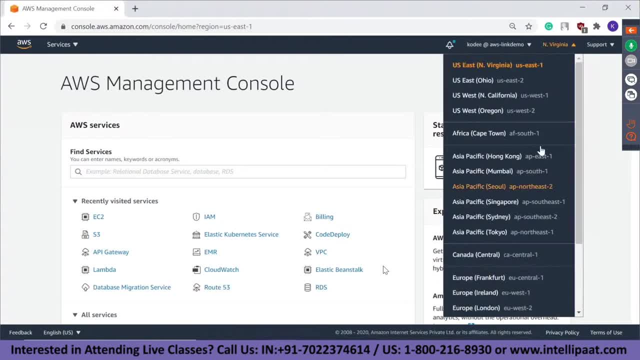 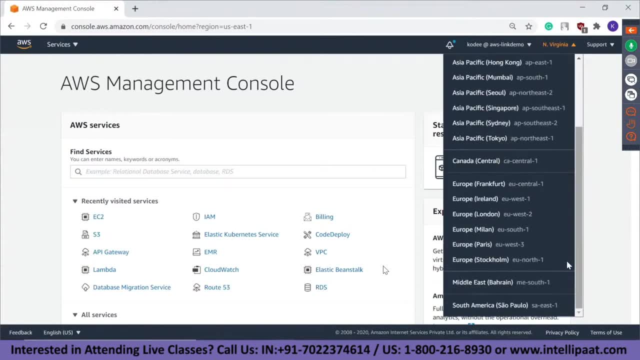 your name over here. uh, here you will have the regions which you can select from. so i'm working on north virginia region. you can choose any of the regions you want. you can choose, uh, south america. you can choose canada. you can choose asia, pacific, mumbai or hong kong sea. also, whichever region you 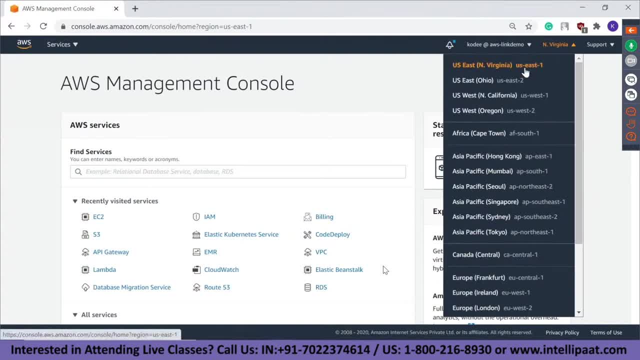 want to work in. but why i work with- uh, the american regions, that is, us east one or us east two- is because whichever new update comes into aws, they always implement it in a region in the us. so that's why i pretty much use the us- uh regions. so if you're a beginner, please start with the us. 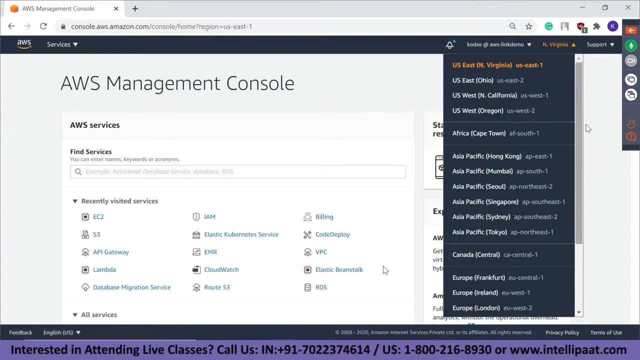 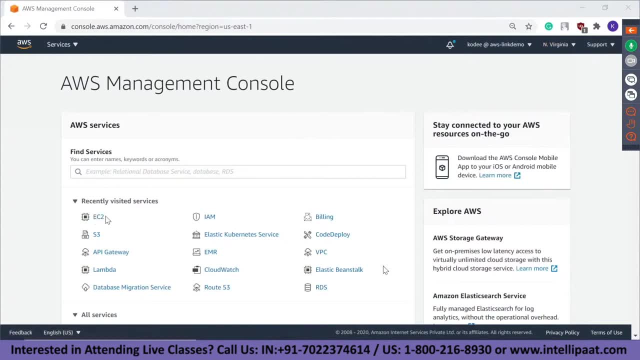 regions. if any new service or if any new feature is coming into a certain service, it will be available in the us region first. next we'll have to start off with the ec2 part. okay, now, to start off with it, you will have to click on ec2. so if you are a beginner, 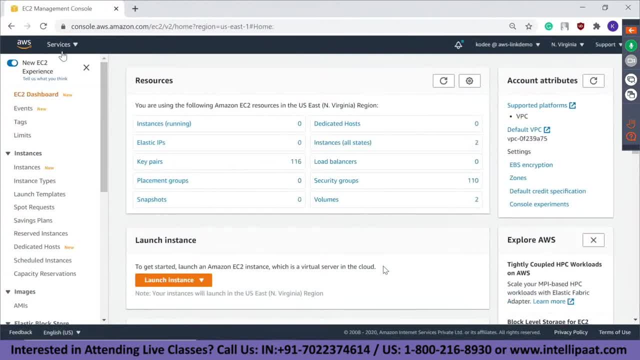 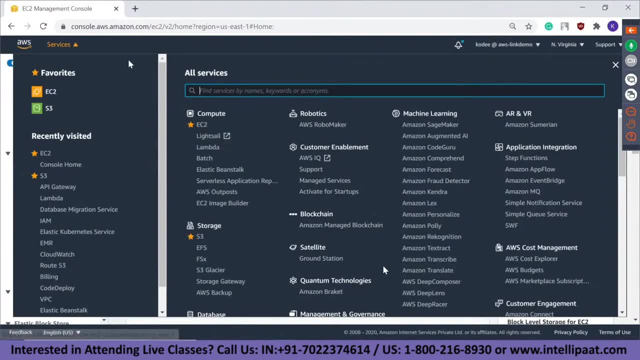 you will have to click on ec2. so if you are a beginner, you will have to click on ec2. so if you, if you, if your account is new, you won't get that option over there, so you'll just have to go to services and search for ec2, or your first option itself would be ec2. so just select it and once. 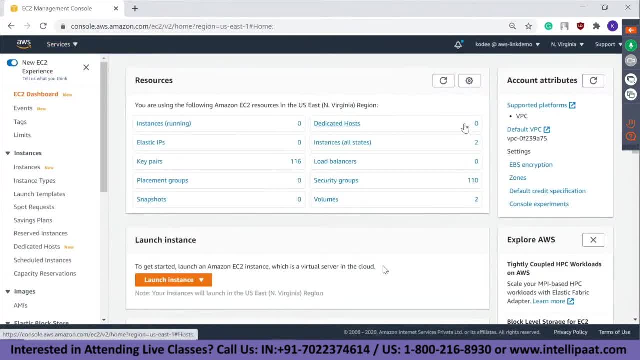 you are in, you will get this dashboard. so once you're new, everything will be zero over here for you. for me, you can see there are 116 key pairs, 110 security groups, two volumes, two instance in all states, but there are zero instances which are running. if you go to these two instances in all, 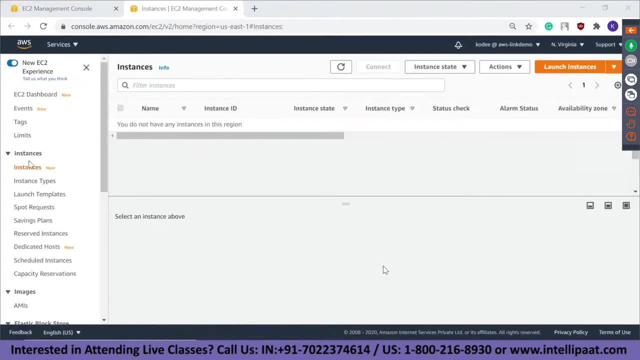 these two instances should be stopped. yeah, so we came into the ec2 instances. so over here right now there are no instances. there are two stopped instances, as i told you. so these two instances are stopped, so you don't get billed for these two instances. uh, whichever instance is stopped, 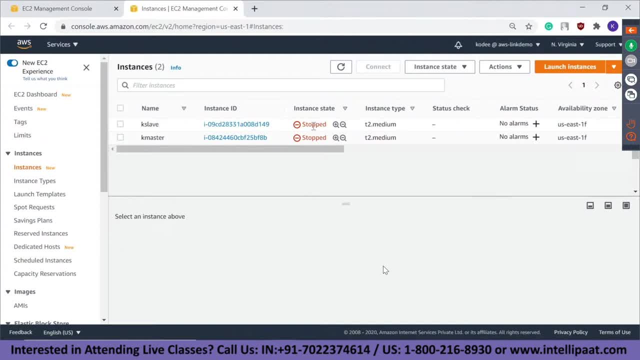 you won't get billed only for the running instances you will get charged. so if you create an instance and then stop it, you only get charged for the minutes that instance was running. so yeah, so this is. i just wanted to show you guys. so now let's start off with the. 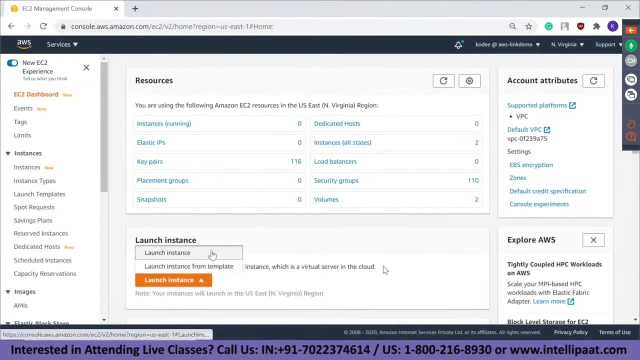 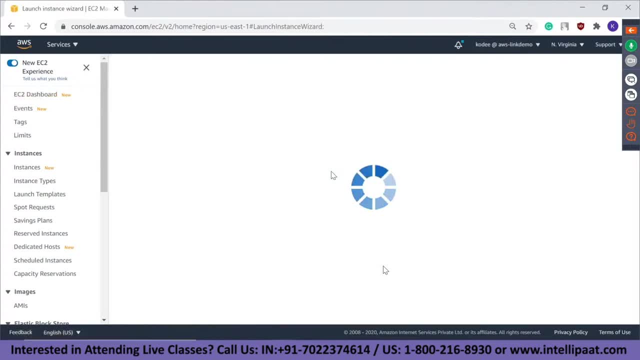 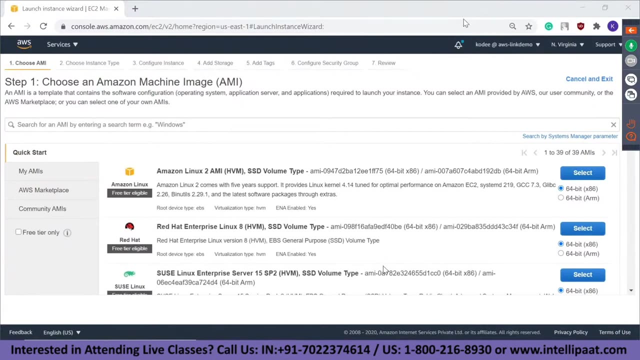 launching an instance part now. click on here so go to launch instance. don't worry about from template so that we'll see. uh, maybe in another session now launch, clicking on launch. once that is done, choose the ami. so let me explain what an ami is. first of all, uh, to launch a virtual. 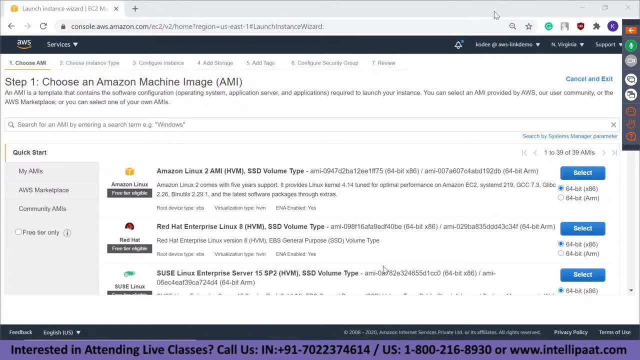 mission in your pc, you will have to basically provide an iso file so that basically contains all the configuration files to launch the operating system in your virtual machine environment. so the same thing goes with an ami. so an amazon machine image consists of the operating system, the application server and the applications which 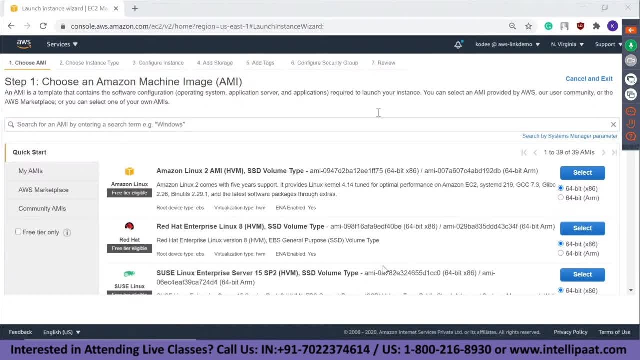 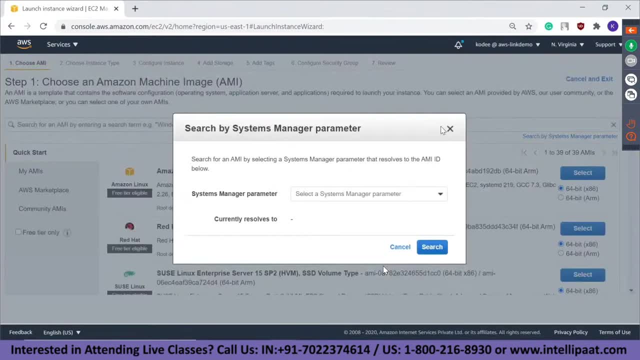 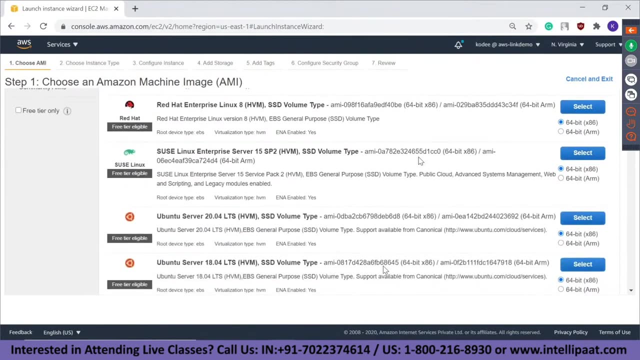 you need to be available within the ami. so if you go with the amis, which are pretty eligible, you can see over here. see, sorry, you have amazon linux 2, you have amazon linux 2. you have red hat enterprise. you have susc linux enterprise. you have ubuntu server. 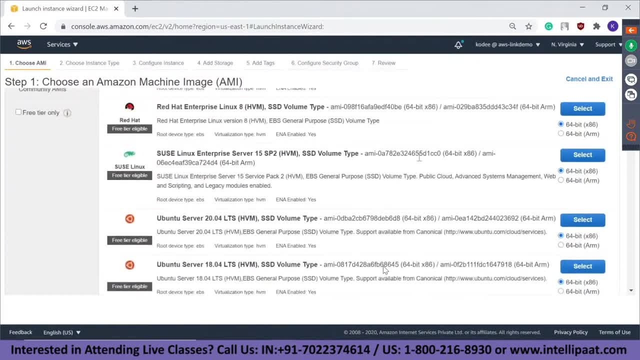 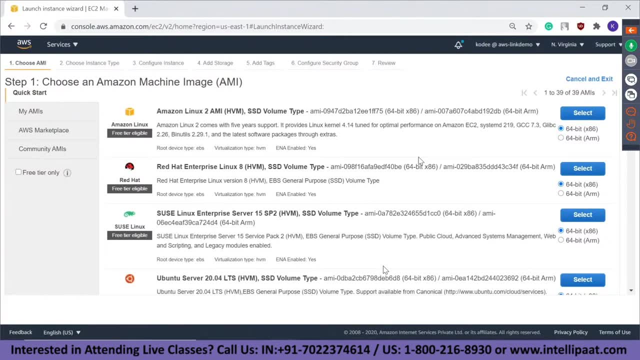 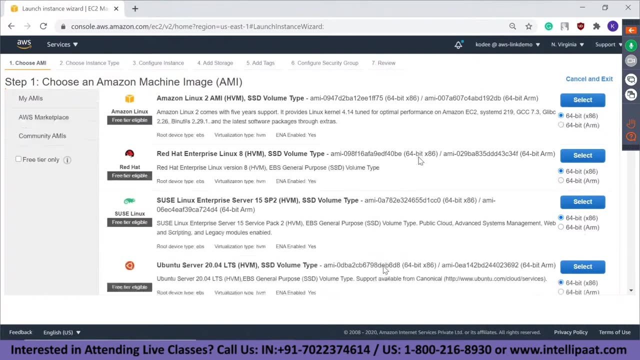 you and you have windows. so these are the six different free tier eligible amis. so now, if you select one of these, you will only get the operating system. then you will have to basically install all the softwares you need for your server. so i'm going to choose the ubuntu server. i pretty much. 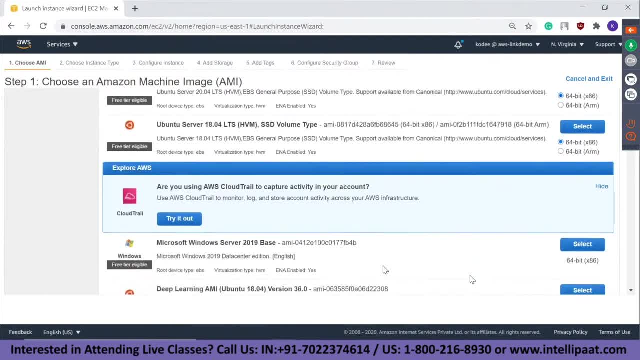 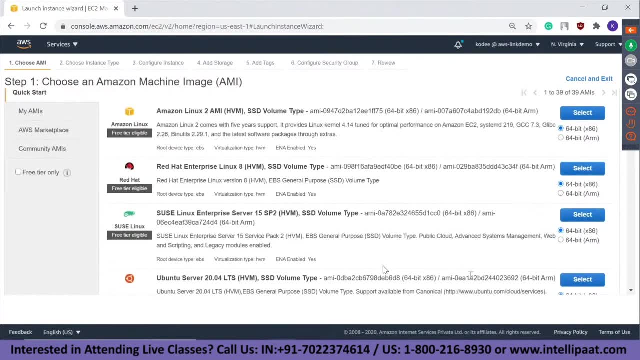 use the ubuntu server. you can choose any of these servers. you can also choose the windows instance. you can choose any server you want to start off with it, to practice off with it. go with a linux because, uh, it will be easier to start off with, so i'm just going to go with the ubuntu 18.04 lts. 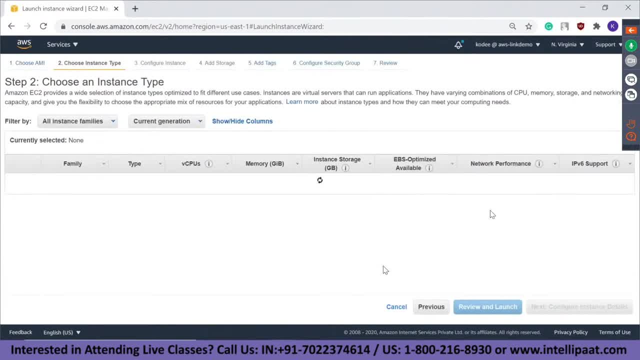 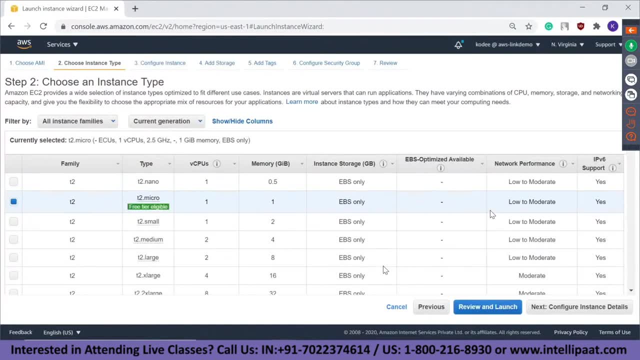 because my i have an virtual mission of it, so i use it often, so i'm just going to go with it. so first we have selected the ami, which basically directly: uh, tells you that we are going to use an ubuntu operating system on our server. next, coming to the instance type, someone asked me: 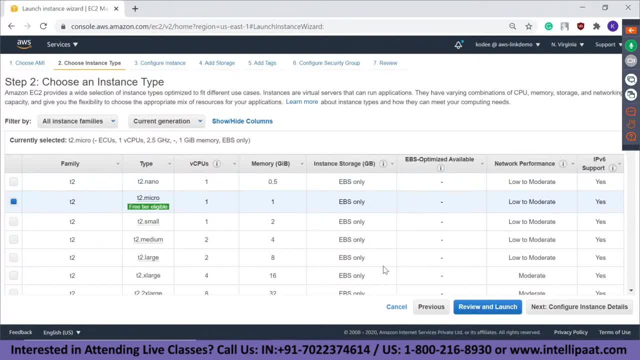 what is m1, m5? uh, what are these? uh, random digits. so that's what i'm going to answer right now. uh, where is it? yeah, so over here you can see, there is one instance, t2.micro, which is under free tier eligible category. so you get the first 12 months. uh, so in the first 12 months you get. 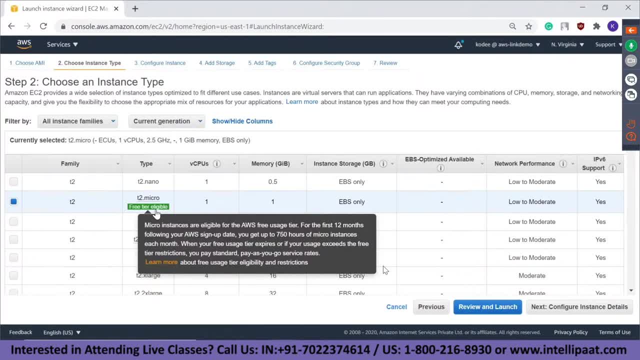 t2.micro instance for free, so you get it for 750 hours per month. that basically means you can run one instance for the whole month and you won't get charged, or you can run multiple instances, but the hours you run these instances, so the total hours of all the instances together should be less. 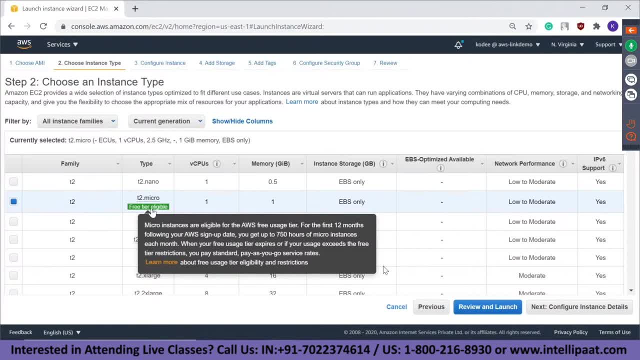 than 750 hours. i'm just introducing you to this so that you get to know which is the free tier eligible instance which you can start off with. so now, as i told you, there are compute optimized instances, there are storage optimized instances coming down. you can see there are. there are very 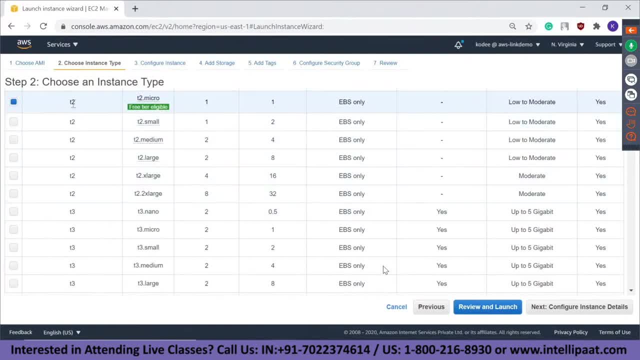 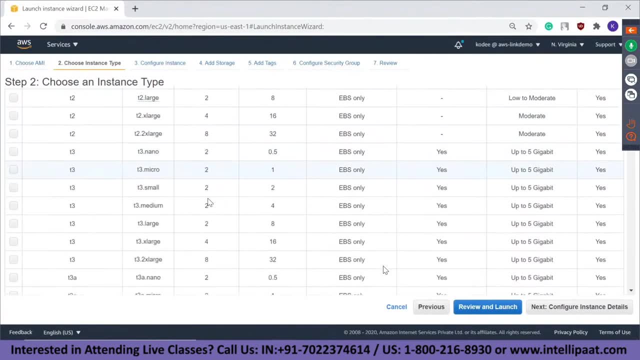 various varieties of instances you can see under t2 itself, t2 family. you have eight virtual cpus and 32 gb of ram. so you can see this is one type. this particular instance type is one type where you get eight virtual cpus and 32 gb of ram. so 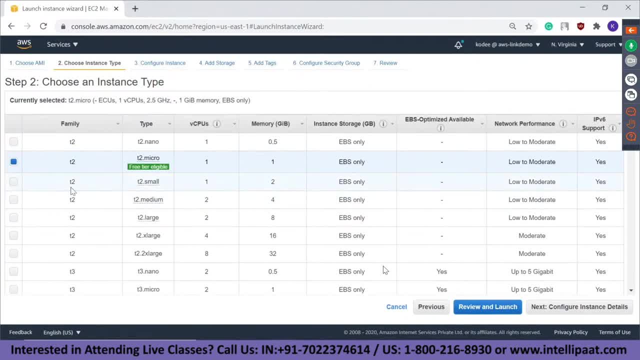 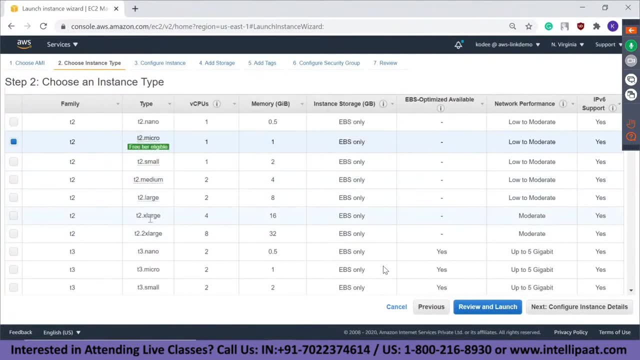 this basically denotes the names which are provided here, that is t2 under t2. you have multiple instances: t2, micro, t2, small, t2, large, t2, uh, t2 into uh, one multiplier, so two multipliers large, which is two, eight over here. then x, large is 416, two into largest, 832.. so now coming down there, 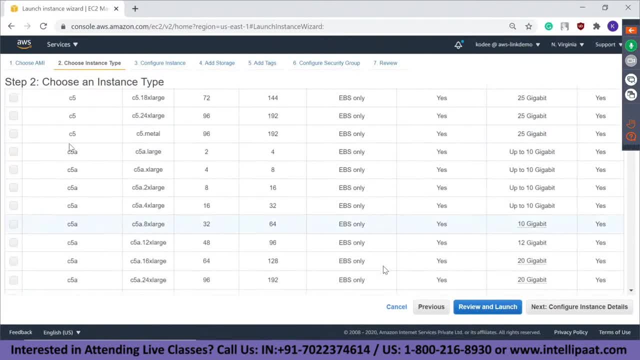 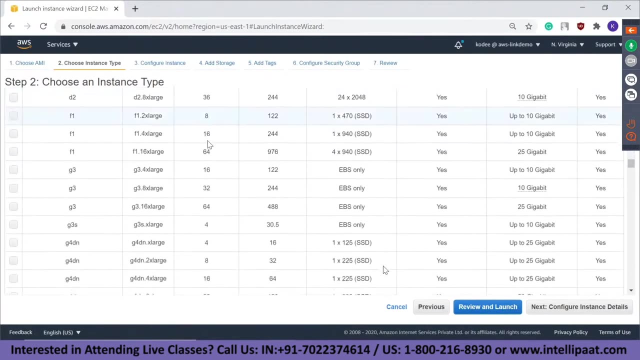 are larger instances. so whenever you go larger the cost will also increase. you can see c5, 96 virtual cpus. that basically means you get the computing capability of 96 virtual cpus and 192 memory, that is, 192 gigs of memory coming down. there are larger instances. uh, larger instance. 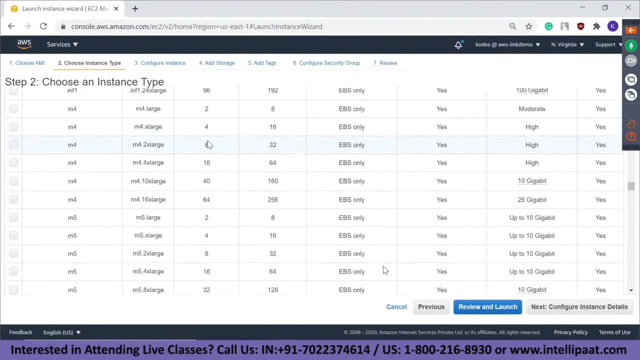 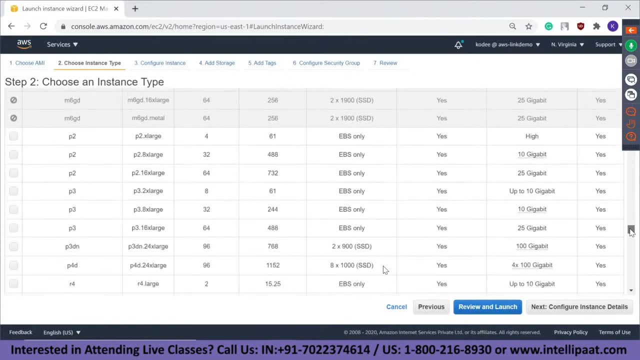 types as well. um wanted to show one which has a 2000 memory. but the thing is, make sure that you don't launch these instances because you don't want to launch these instances, because you don't, they are very expensive and they'll cost you a lot. 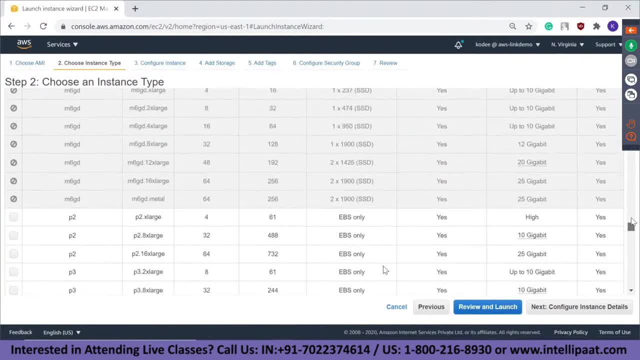 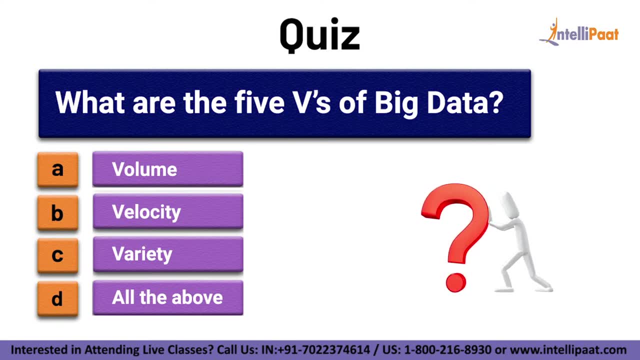 okay, so it's not here, it's over here. i saw it somewhere. just a quick info: guys, test your knowledge of big data by answering this question: what are the five v's of big data? a, volume, b, velocity, c, variety, d- all of the above? comment your answer in the comment section below. 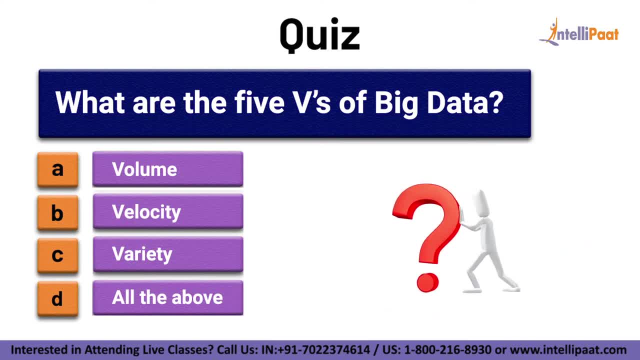 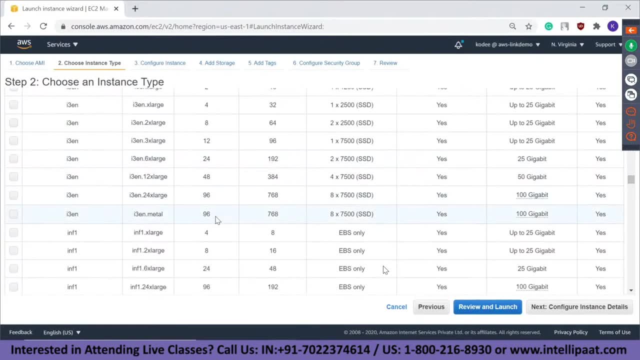 subscribe to intellipaat. know the right answer. now let's continue with the session. you can see there is one instance, i3en, 96 virtual cpus and 768 gigs. so these instances are basically memory optimized instances, where you get a very high increase in the memory, but the virtual cpus 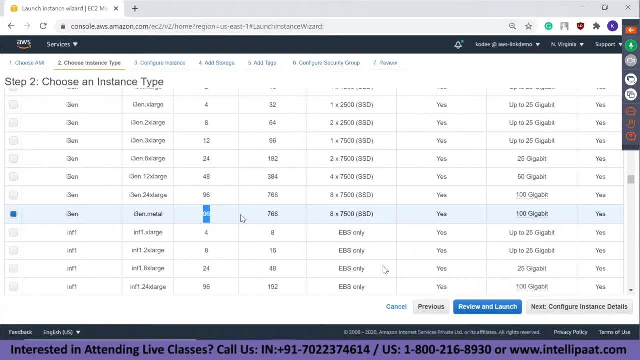 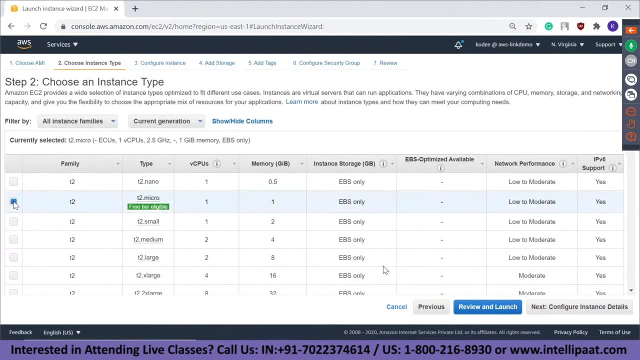 are basically the same as any other instance type which is available. also, you can see storage: optimized instances will have ssd, normal instances will have ebs only. so ebs is the block storage which is attached to your instance type. block storage in the sense, whichever you store or 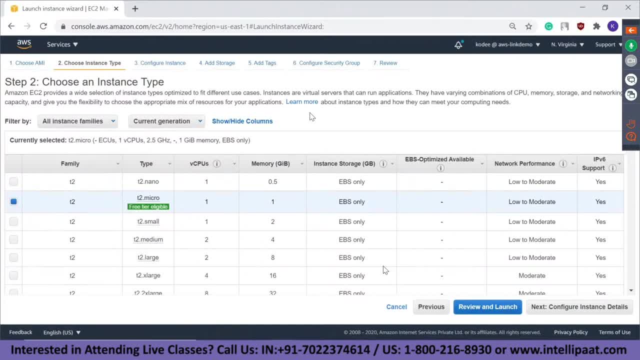 whatever software you install on ec2 server will be stored in the volume attached to it. that is the root volume attached to it and that root volume is basically ebs. so again, we are going going to go much into ebs, but the next you will have. i'll just give you an introduction in the 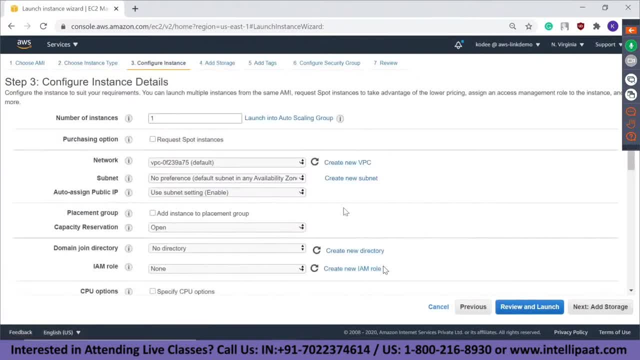 storage part. so i'll select t2.micro. next configure details so you can choose the number of instances which you want. so i just want one instance and next you have network subnet again. you don't need to go into these now because vpcs subnets are completely different module in which you'll 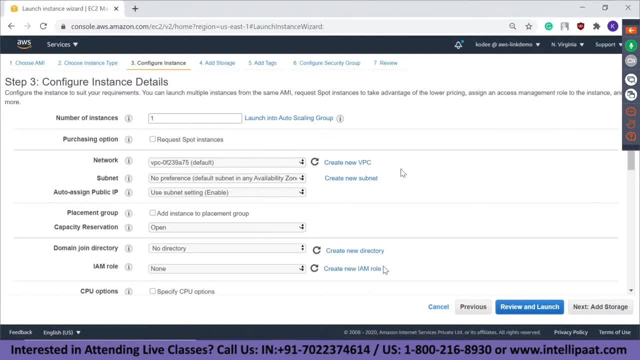 have to go through and understand everything. to put it simply, to uh, to set up a land or to set up a local network, you need multiple systems which you connect together, which forms a network. so right now, if you want to create a network in aws, you can create a vpc which creates a logical 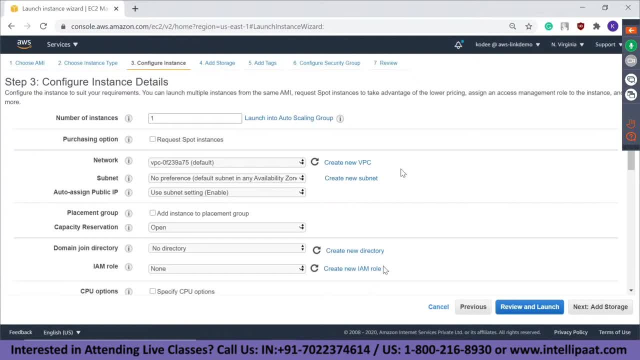 network inside of which you can launch multiple ec2 servers which you can use as a group of servers which are connected together. so it basically denotes a network and subnets are uh. basically you can use a subnet mask where you denote a cider notation which basically is uh. 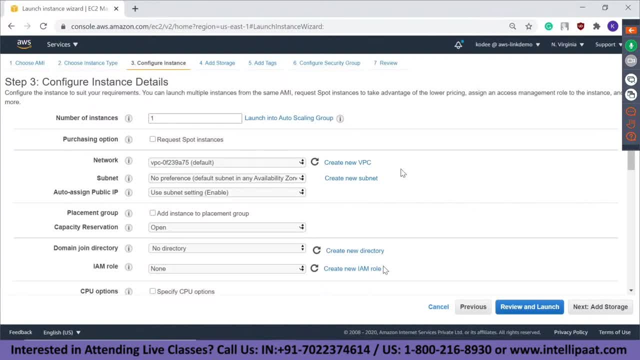 a list of ip addresses which the instances within the subnets can use. it's a little complicated. if you know networking, if you have steady networking and know a little about network masks, you can understand this easily. if not, you'll have to look into this later, so just choose one. 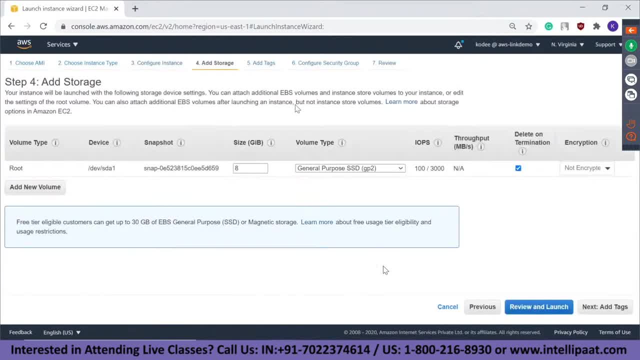 instance, and click on next. next is the root storage: 8 gb is more than enough and also under free tier. that is, for the first 12 months of your aws account, you get 30 gb of ebs storage free. the basically means even if i create a storage uh volume for 100 gb, i won't get charged, but i'll. 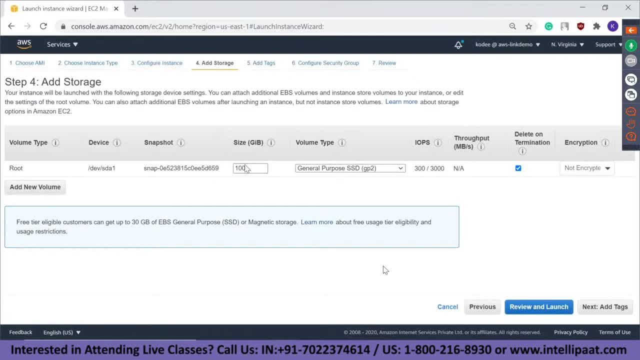 only get charged if i store 30 gb of content inside of this 300 gb uh storage volume. so make sure you don't go more than 30 gb uh for per month, otherwise you will get charged. now i'm just going to go with 8, also this one. if you unselect this, if you delete the ec2 instance after this, this 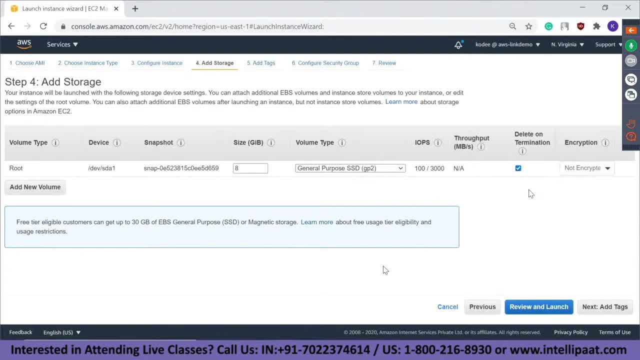 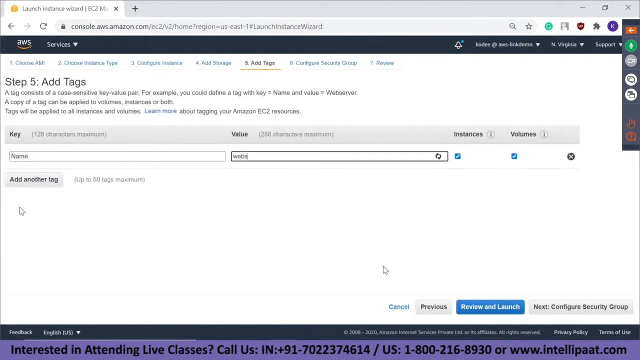 particular volume will not get deleted. if you select this. the volume will get deleted on terminating the ec2 instance. so this is the volume. next coming to tags. so tags are pretty much to track the instance. so if i provide name and web server, so this particular name will be attached to the instance. if i have 10 different servers, 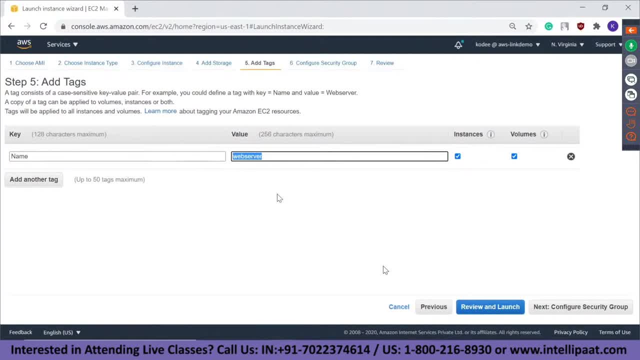 which are running the same web server on the same website. within it, i can name all of those servers with the same tag and if you want to check what, check all of the servers that are running on the same website within it. i can name all of those instances once i can search them with this. 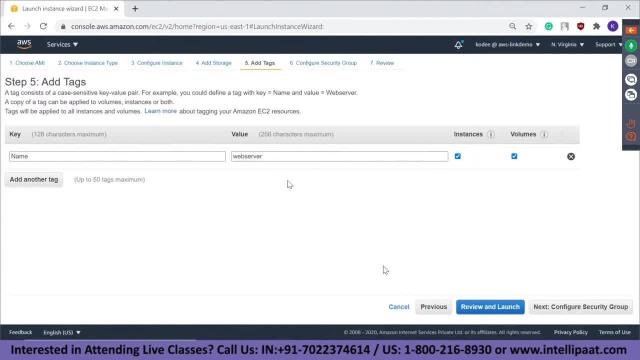 particular tag and i'll get only the servers which have this tag, so other servers will not be shown in the search. let's basically filter and track them nothing much you can. this is optional. you can ignore this as well, going to the next step, which is again important. so again this comes under. 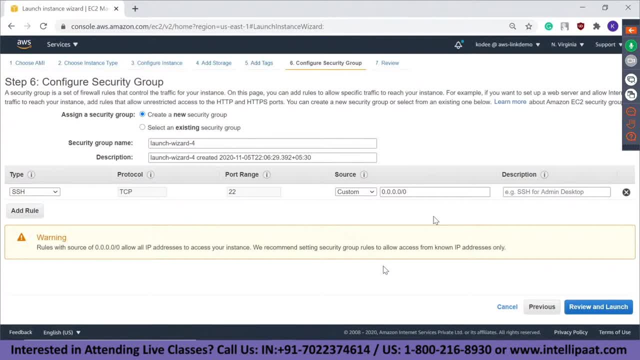 bpc, but this is basically like a firewall which you create. so now, uh, this particular instance can be accessed from any ip address. that basically means even you can access this instance if you have the private key file which i'll create. if you don't have the private key, you will not be able. 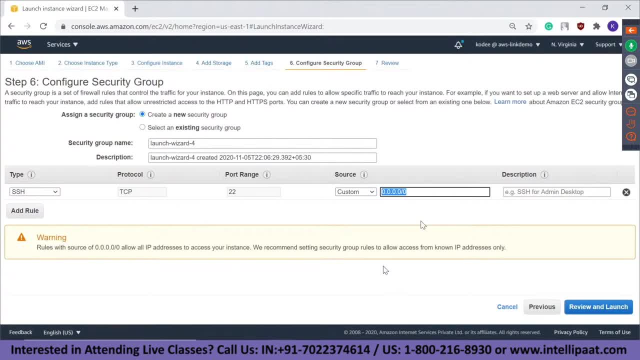 to log in. but if i give you the private key you will be able to log in into the instance which i'm going to create. but if i don't want you to log in, even if you have the private key file, i can change this ip into my own pc's ip address, so only i can log in, even though you have the private key file. i. 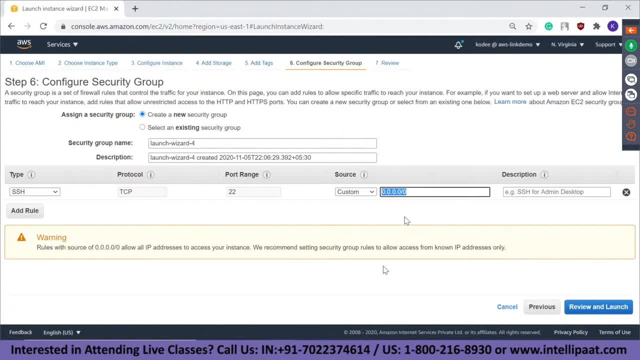 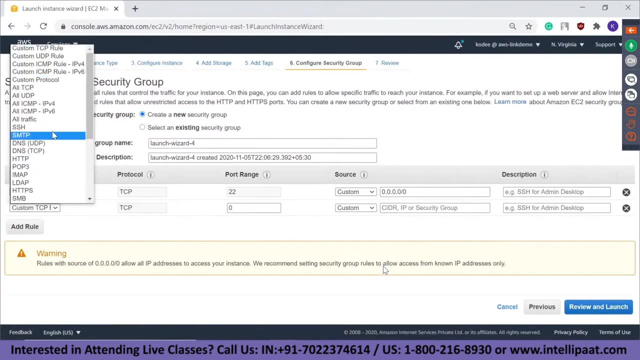 can use the private key to log in into this. so if you want to know what is private key, obviously i'm going to explain it. so now, first go with ssh. ssh means secure shell. it basically lets you log in into the instance securely using the private and public keys. also, add one more rule. so not right, you don't need to add this, i'm just going to add. 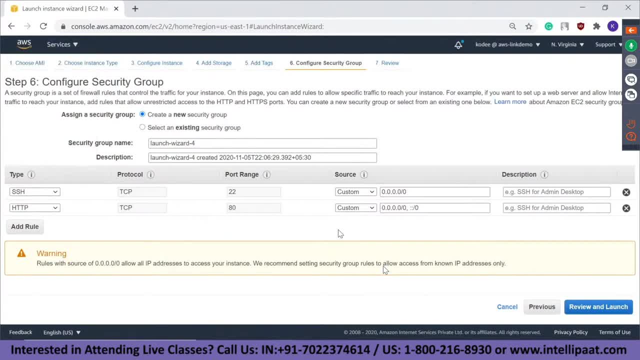 this because i wanted to show you how to create, basically install, software within this. so go with http. uh, i'm just going to go with custom. so anybody should be able to see. even you can. you should be able to see. so i'll launch an instance and i'll give you the ip address of the server so that you 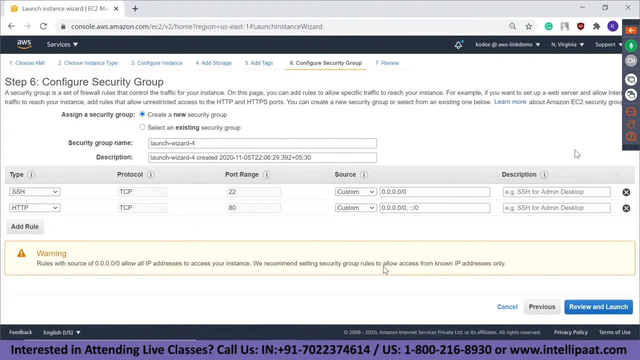 paste it in your computer, if any of you have, and you can see this particular instance which i'm going to launch now, the web server which i'm going to launch. so, right now, everything is done, every particular, every step is provided. next, click on review, on launch, uh, coming down, you can see you. 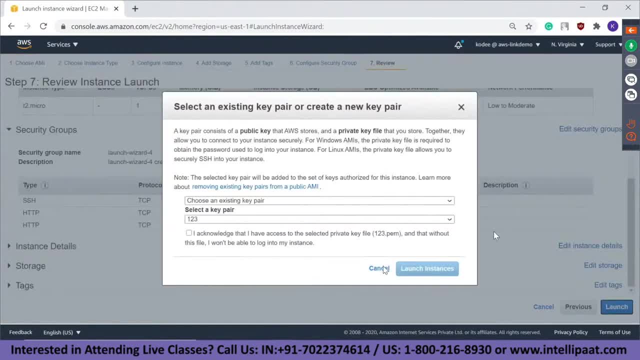 can just check all the details once and click on launch. so once you click on launch it'll ask for a key pair. you can either create one or use an existing key pair. so first let me explain what is a key pair. so key pair has two keys. that's why it's called a pair. you have a public key and a private key. so 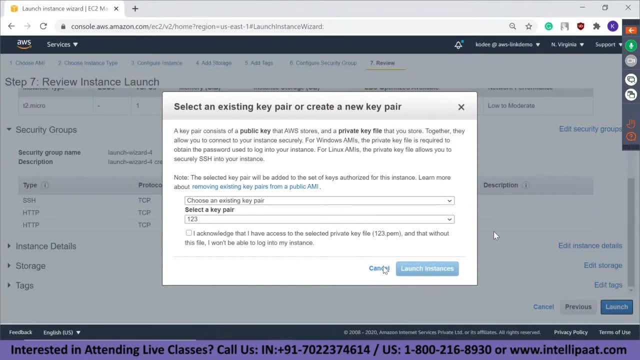 the public key is stored inside the server. the private key is the one which you download to your pc. so now, while logging into the instance, you will have to provide the private key or upload the private key to the server, and the private key will be used to decrypt the public key, if it successfully. 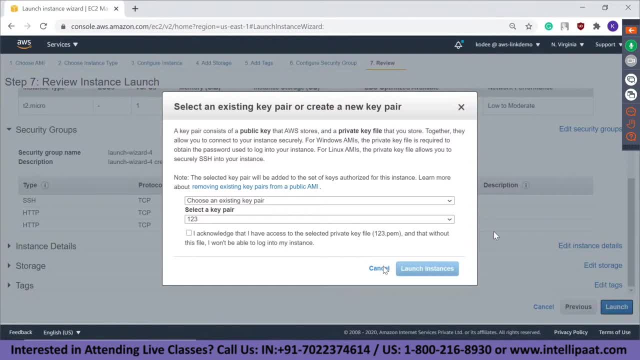 decrypts the public key, then you will be given access to the server. if you use a wrong key, you to login into the instance. it's pretty simple. it's like logging- uh sorry, uh, entering your home. if you use the wrong key, your lock won't open. so the same thing here. it is basically for security. 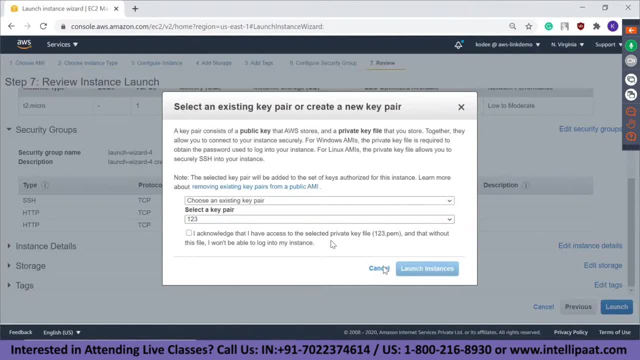 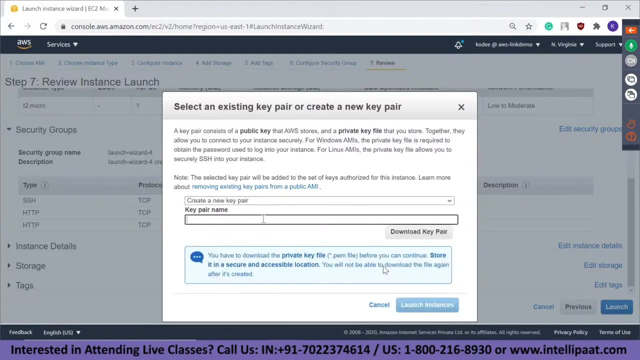 so now i'm not going to use an existing keypad. i already have one, but i'm not going to use it. i just wanted to show you guys how to create one. so click on create a new keypad and type in a keypad name. so i'm just going to type as north virginia. 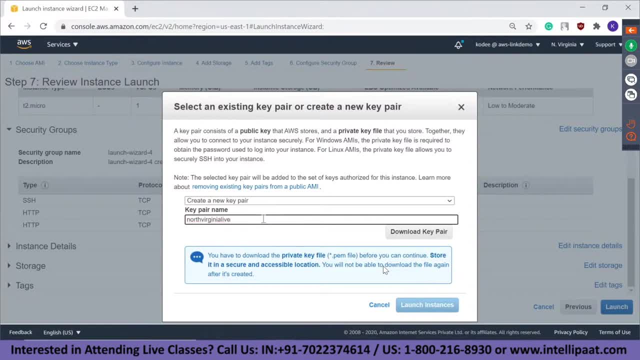 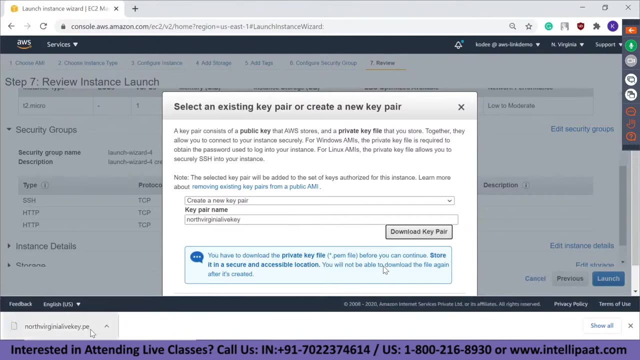 live key. so there's a question creating keypad. i think i explained it. so north virginia live key and once you provided the keypad name, click on download keypad and you will get your keypad downloaded. so it is a dot pem file. you can see over here: north virginia live key, dot pem. so we 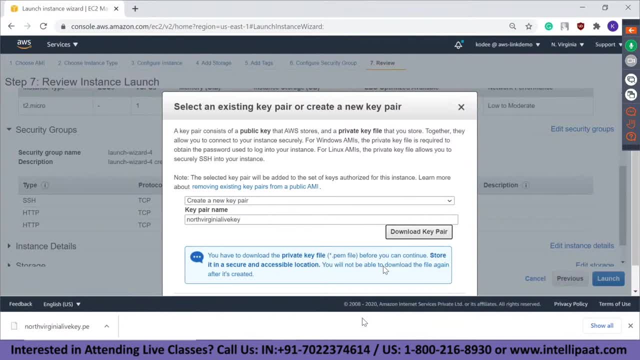 cannot directly use the dot pem file in the windows system, so we'll have- we'll be using a software to do that. so we're going to use a software to do that. so we're going to use a software to log in into the instance if you're in uh, ubuntu or linux operating system. 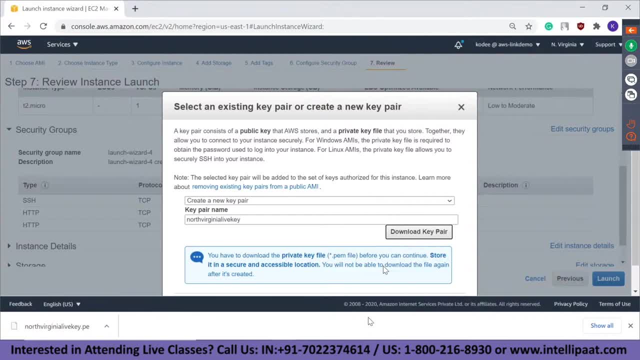 then the login process is a little different. you'll have to use the ssh command. but right now, as we are in the windows pc and most of you watching this might have a windows pv, so i'm just going to go ahead with it. so i've downloaded it. i'll just close this and click on. 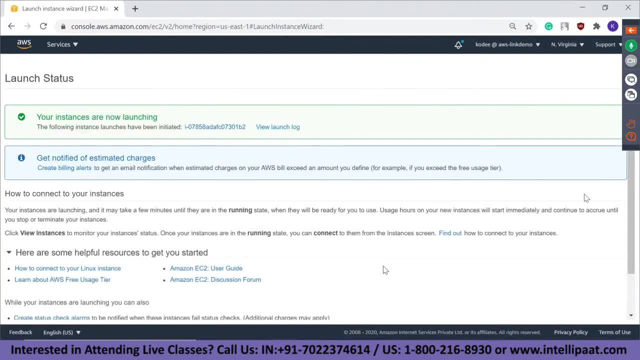 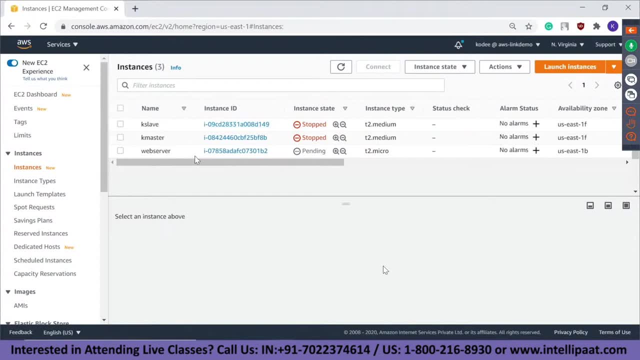 launch instances. so the instance is successfully launched. going to view instances. so just ignore these changes. the next thing you want to do is you want to update the browser. if you do that, so you to these are stopped. so this is the instance which is getting created. you can see the name is web. 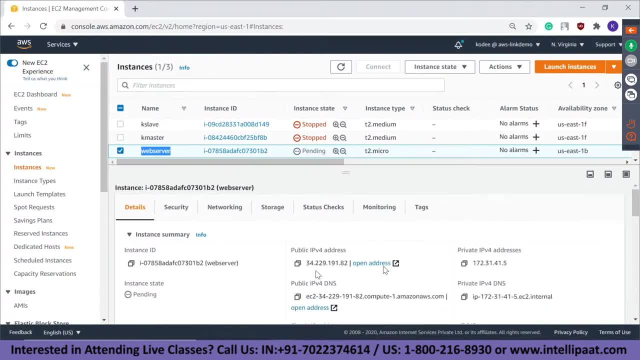 server, which is the tag which i provide. also, you can see a public ip address has been provided. a private ip has been provided. you don't need to worry about the private ip right now, because if you have to learn about the private ip address, you will also have to know about vpcs and subnets. 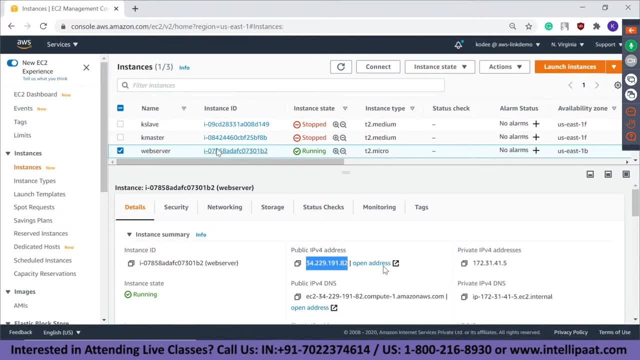 so now the public ip address is the one which we will be using to identify this server, which is unique to this particular server. so this ip address will not be available in any of the pcs or any of the server which is available in the world. it is only for this particular server. so 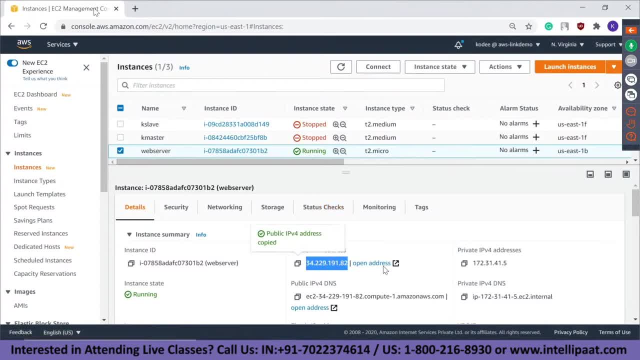 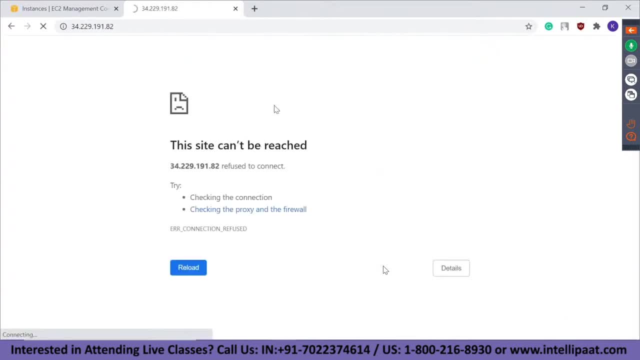 that we can access it. so now, if i copy this- so right now it is running- if i copy this and paste it here, you will not see any output. it will show just an error. so you can see: this site can't be reached because there is no server running inside of this. there is no web server running inside of 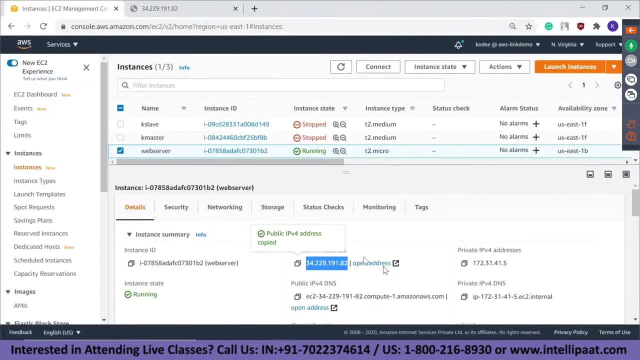 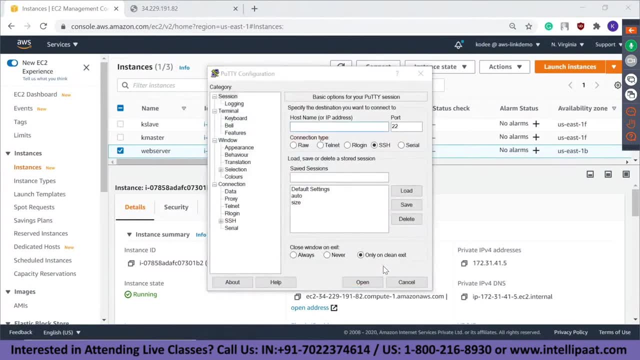 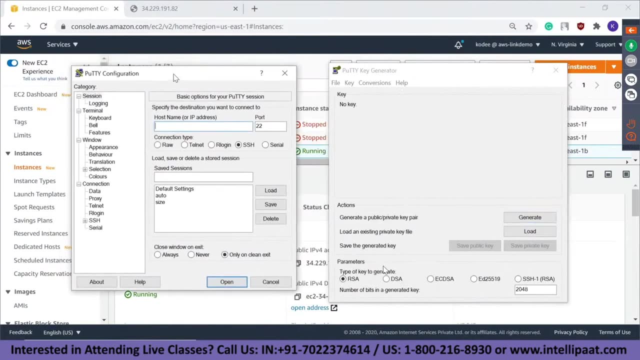 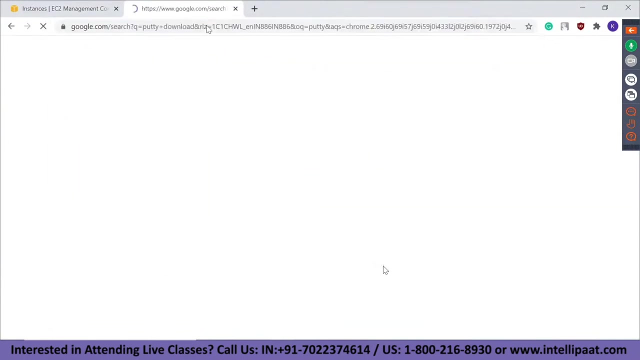 this. yeah, so inside of this easy to instance. so now we'll have to log in into that. okay, now let me show you this particular tool: putty and partition. so you will need these two tools to log in into the ec2 instance. so now, where you can get these? uh, you can just type in putty, download the first option. 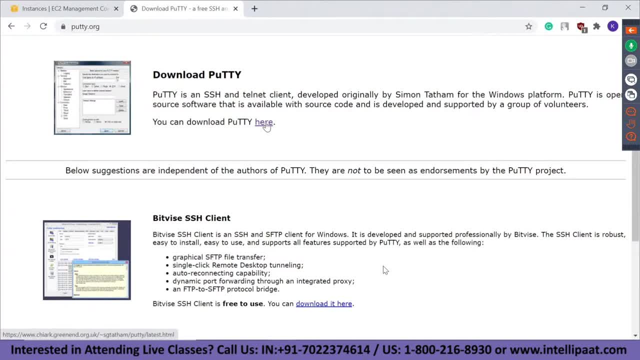 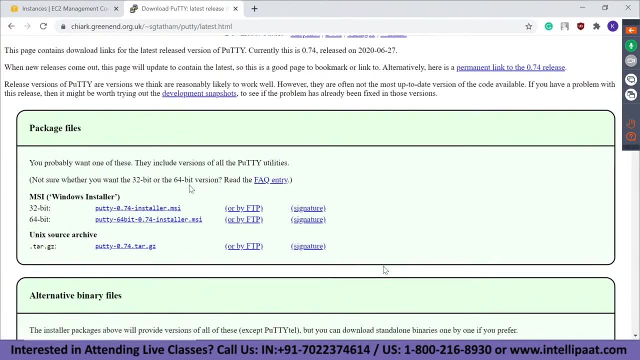 over here is download putty. enter that and over here you can see you can download putty here. click on it. so if you're using windows, just select it from these two options. if you're using a unique source- maybe any unix- you can just download it. 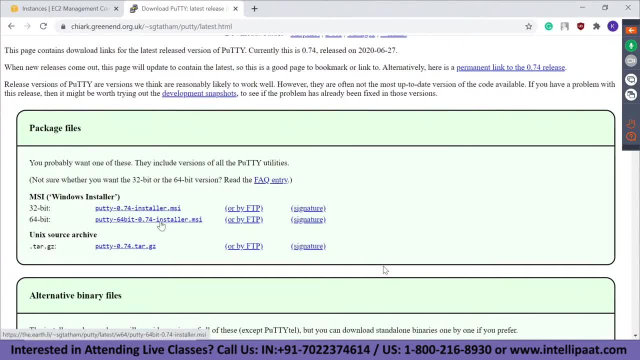 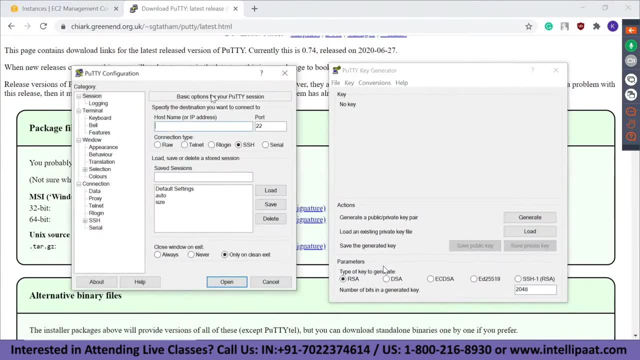 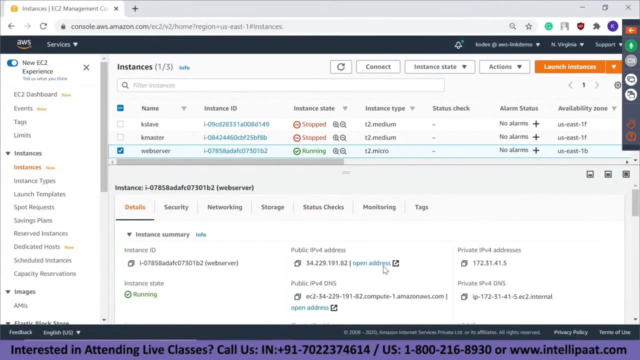 and untar it and start using it. so here i just installed this. you guys also can install this. once you install it, you will get both these tools, that is, putty key generator and putty configuration tool. so these two tools will be available. okay, so i've shown you that. now going. 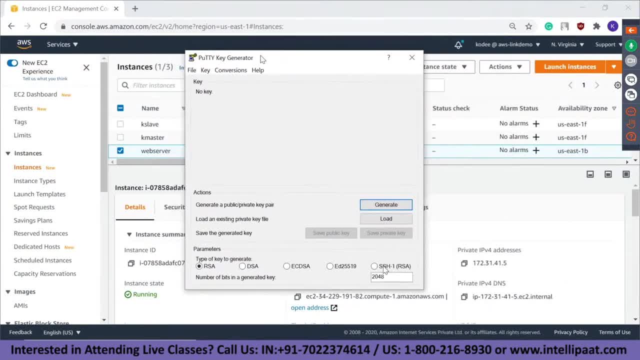 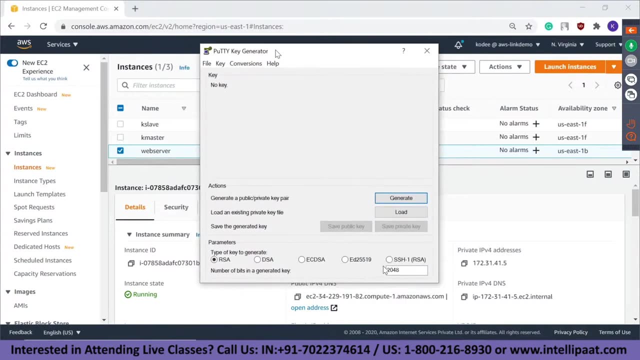 back. so what we'll have to do is we have to convert our pem file into a format which the putty tool will allow. so the putty tool will not accept dot pem files. it will only take a putty private key files. so we'll have to convert it into a putty private key. for that we'll have to. 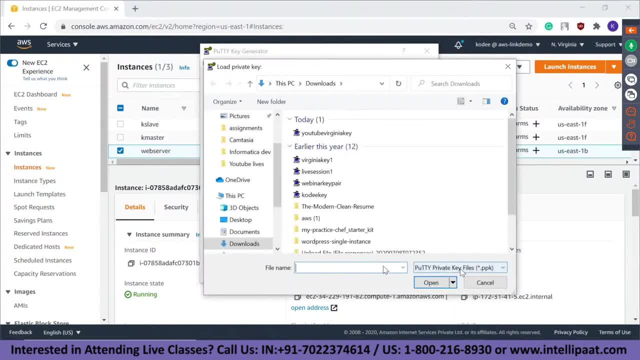 use putty key generator. so clicking on load, so change this to all files, because it only searches for dot, pp, dot, ppk files. you can see i already have some key pairs. i'm not going to use them. clicking on all files, you can see the key pair which i just downloaded is over here. 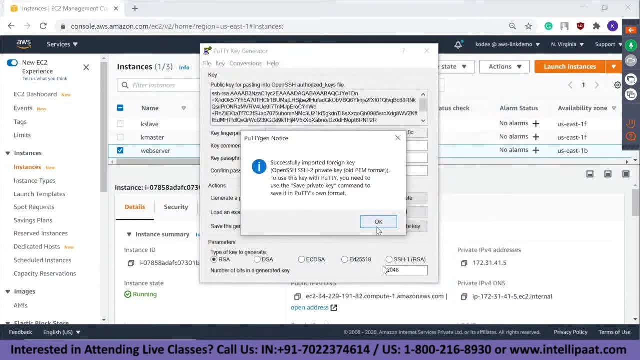 north virginia live key. so i'm going to select this and open. just click on ok. now it has a been converted into a ppk file. that's it. you don't need to do any other hard work. you'll just have to upload the key. the putty generator key will change it into a putty readable format, and 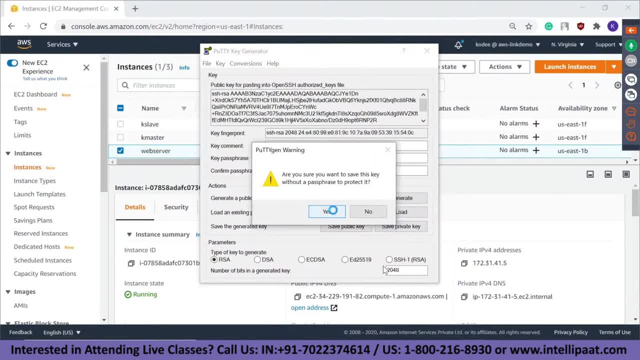 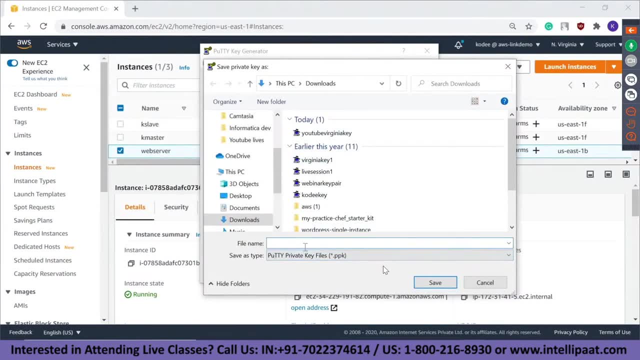 give it to you back. once that is done, click on save private key. click on yes. provide a similar name. what is this? okay, i'll leave that. uh, provide a similar name. i'm just going to provide north virginia live key. oh, sorry, i'm going to provide north virginia. 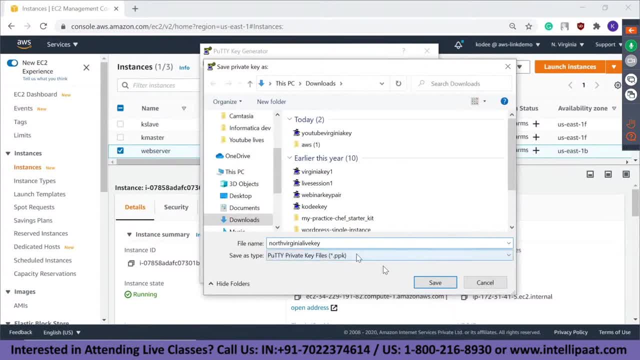 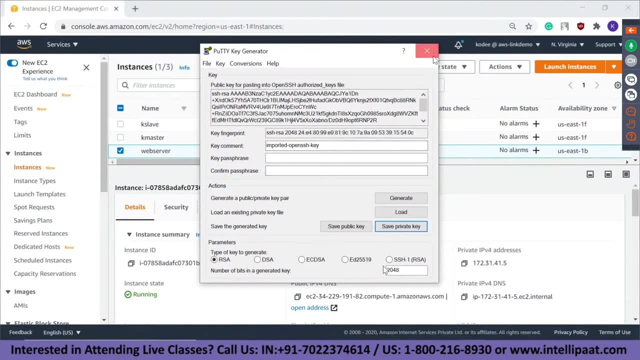 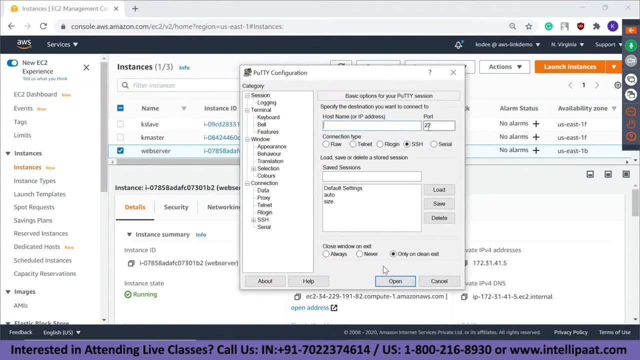 live key, but don't give dot pem, because it will be stored as the stored as a dot ppk file. okay, so now the first step is done. so once this is done, just close it and open putty. so now, guys, uh, you guys know that we created a security group which allowed port number 22 to ssh into the instance. 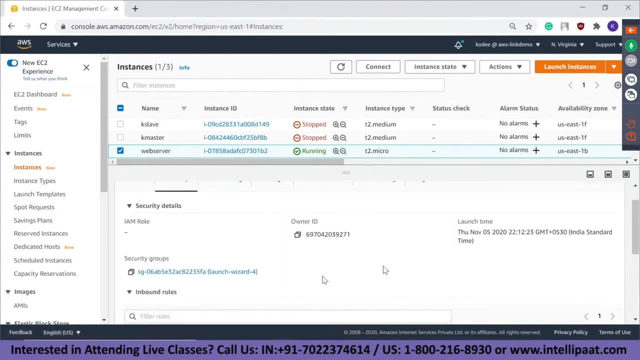 so that is why we need it. so, if you go to security, yeah, so this is the security group which we created and you can see port number 22 and you can see what is this port number 22. it's allowed via a tcp protocol from any ip address. 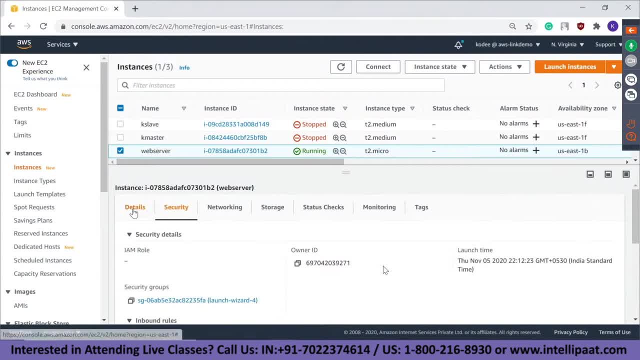 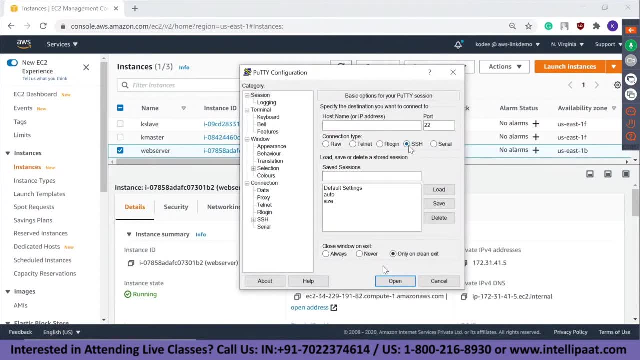 and the protocol which we need is ssh, which is also a tcp. uh, it is under a tcp protocol, so now open butty. so first you'll have to select this, but you don't need to because it is the default option provided here. it's such port number 22, and here you'll have to provide the host name. so i just 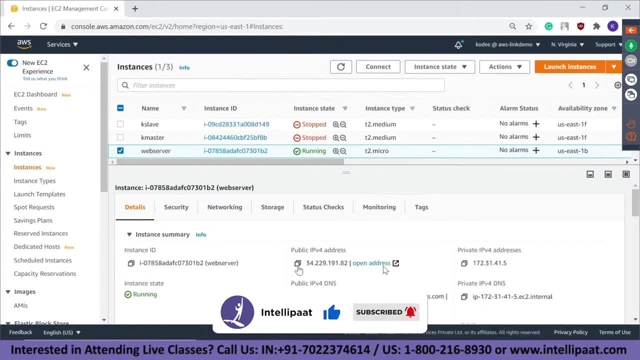 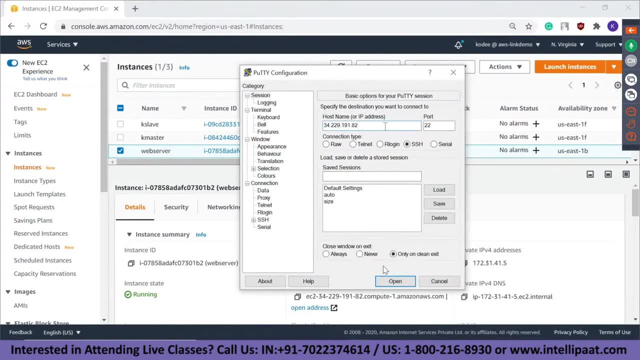 copied the host name from here, sorry, so this is the host name, guys. the public ip address, copy it over here. so now the host name is provided, port number is 22 and the connection type is ssh. so the second step is to upload the private key file. so to upload the private key file, go to ssh. go to. 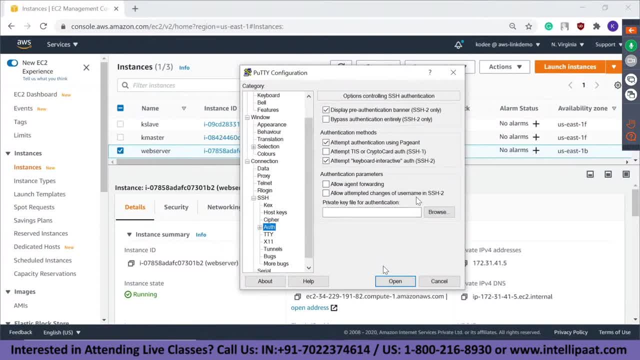 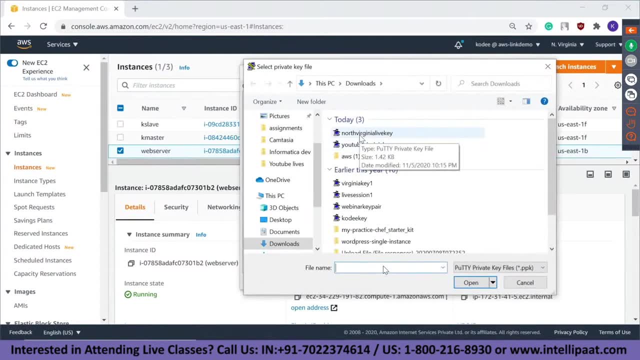 authentication and over here you can see private key file for authentication. click on browse and choose the appropriate key. so if you choose the wrong key and if i'm trying to open it, it won't work, so you'll have to choose the appropriate key, which is not virginia live key. 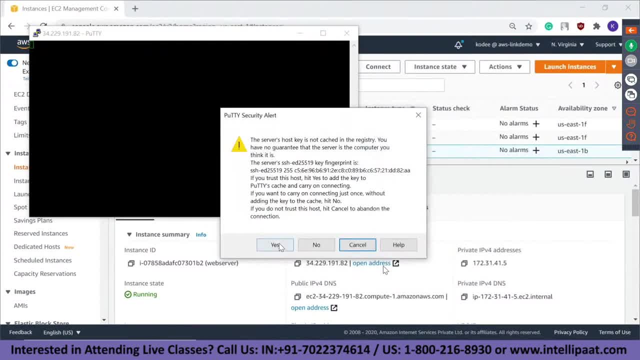 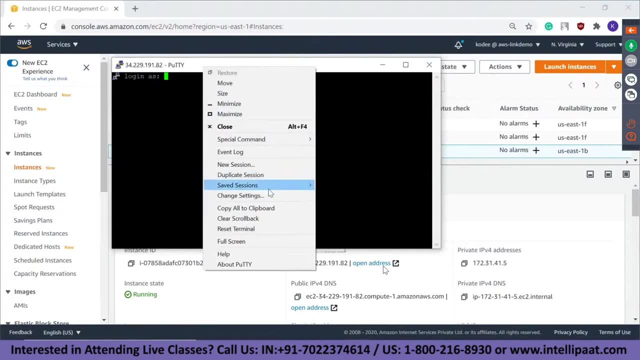 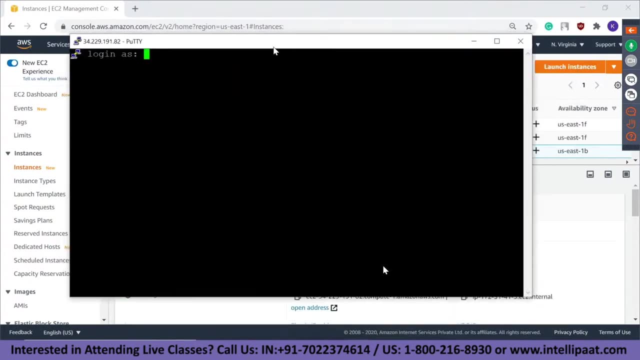 opening it and open. so once this is shown, click on yes and right now you will see there is a login as option. so let me just make the screen a little bigger, okay? so right now you can see there is a login as option. so for an ubuntu instance, the user username. 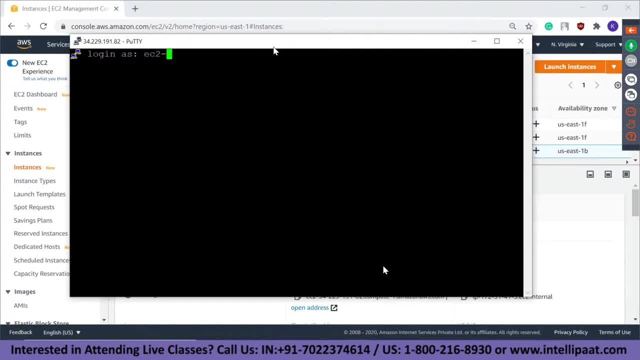 is ubuntu. if it is a linux instance you are using, the username would be ec2 user. so any other linux instance- it can be redhat, it can be its usc, it can be amazon linux, but the username is ec2 user. if you're using ubuntu, the username is ubuntu, so there is no password once you hit enter. 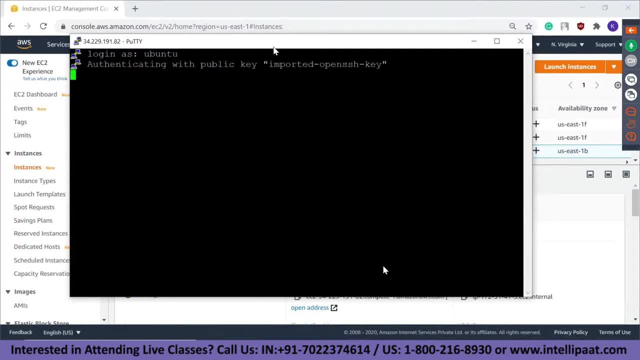 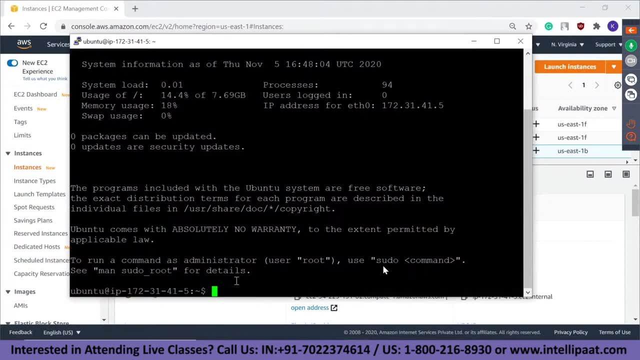 it will basically get the private key file from putty and it will try to authenticate it with the public key. so if it successfully authenticates, you will get the terminal over here. so right now you are successfully logged into the ec2 instance which we just created, guys. okay, so i just put. 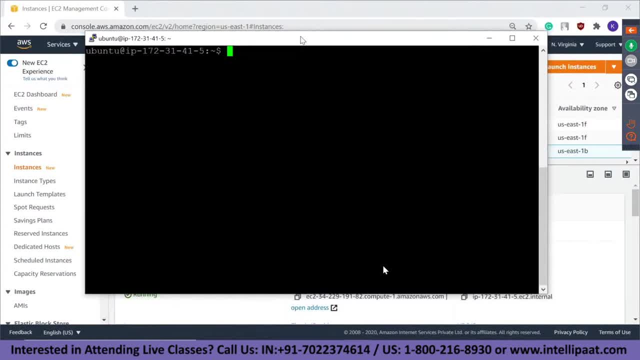 the clear command to show you the terminal. so you can see over here we are basically inside a directory called flash, home slash ubuntu. so we are successfully logged in. so we have created an ec2 instance and we have successfully logged into it. so i wanted to show you how to install certain software. so some of you might not know linux. so 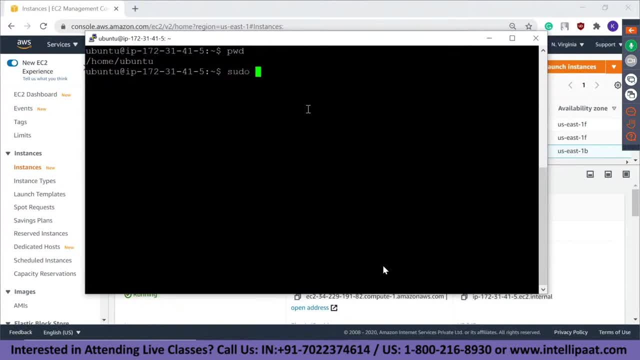 in ubuntu it's pretty simple: you just have to provide sudo- apt-get. so apt-get is a package manager which is basically like an install wizard which lets you install certain software, and the first thing you'll have to do every time you launch an instance is update it, because 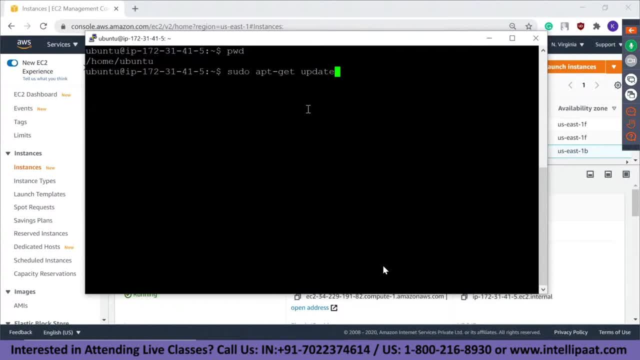 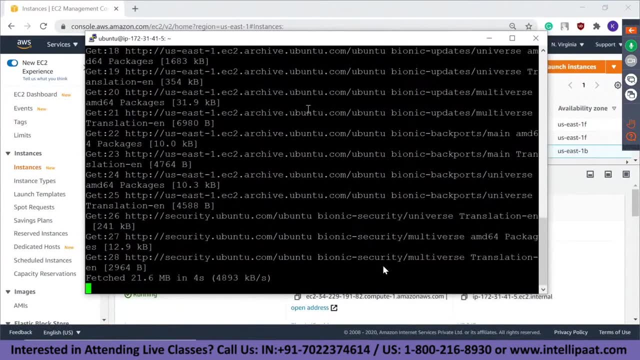 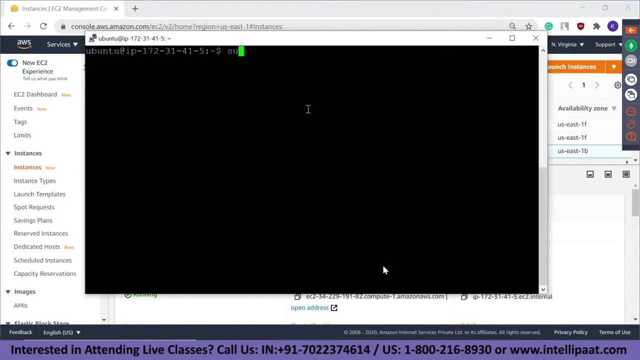 certain softwares might not be updated in the instance which you just launched, so always do an update. so once you update it, you can basically install any other software which you need. so the update is done. so now let me install a web server called apache2. so 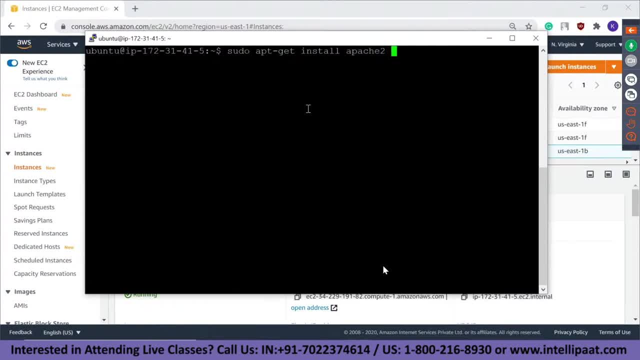 you see, this is the web server which i'm going to install. it's basically a lightweight web server where you can host html and okay, so now. so this is the software which i'm going to install, which will be basically running a default web page in it which i'll be able to see in the browser. 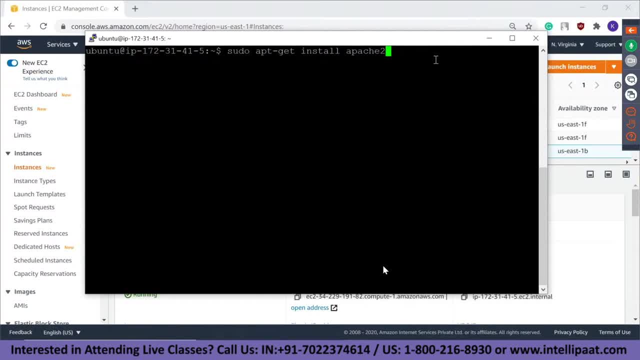 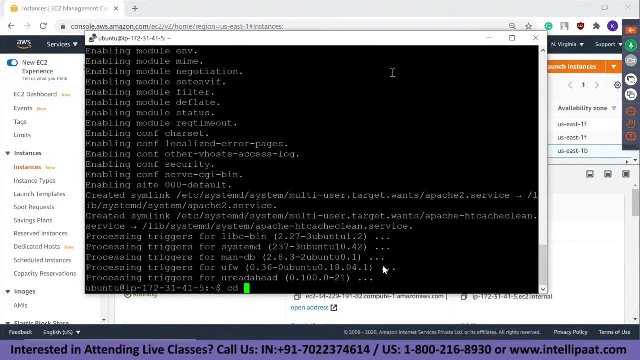 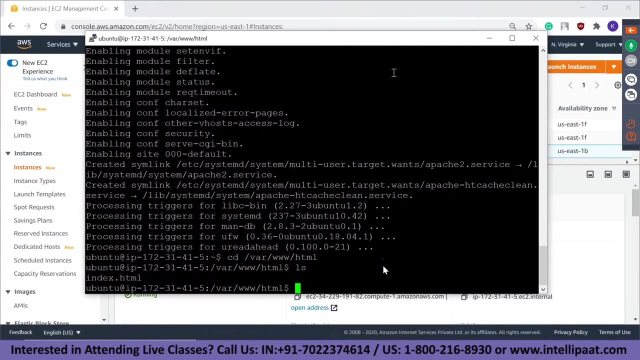 i'll also give you guys the ip address so that you can view it in your browser as well. so now, clicking here and providing yes, the software will be stored in a location called http//wwwvrhtml. if you go to this location and do an ls, you can see there is an indexhtml file. 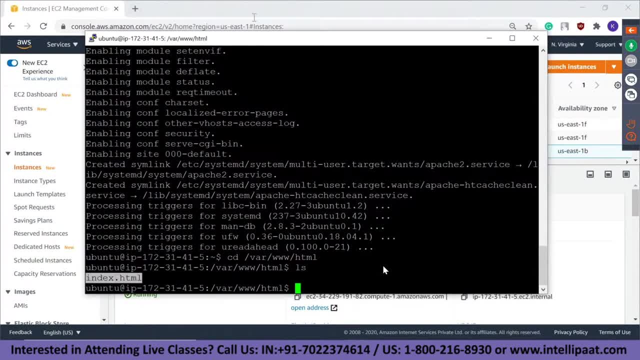 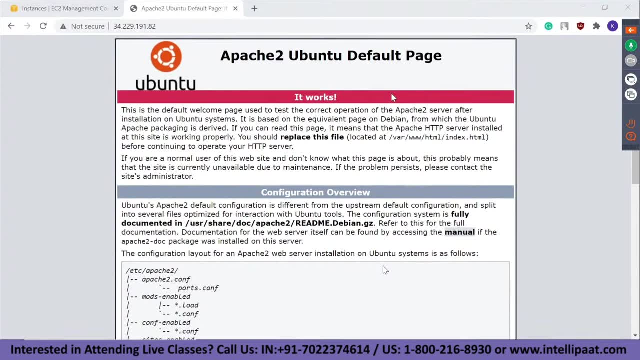 over here. so this is the file which will be shown in the browser right now, in the web page right now, and right now you can see there is an ubuntu default page running in my ec2 server. the last time when i showed you this particular ip address did not have anything inside of it. right now there. 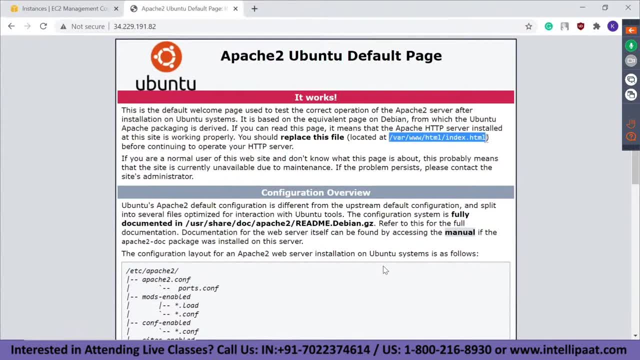 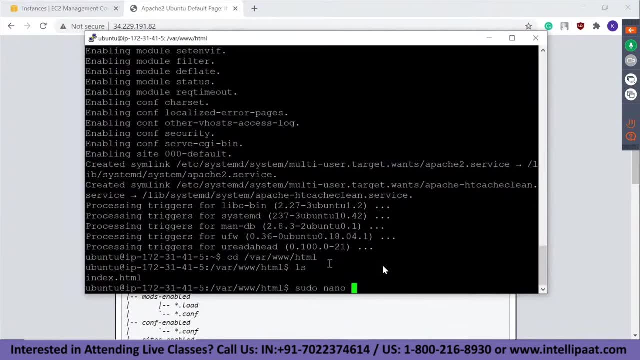 is a default page and you can see it is located at this particular location. so right now, if we go back to my instance and use sudo nano, so nano is an editor where you can edit files, so sudo nano editor. i'm creating a file called 1.html. 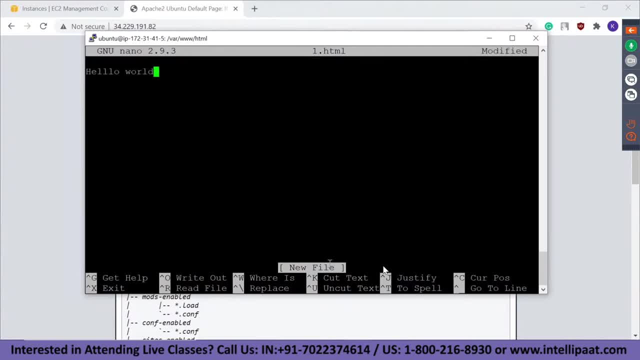 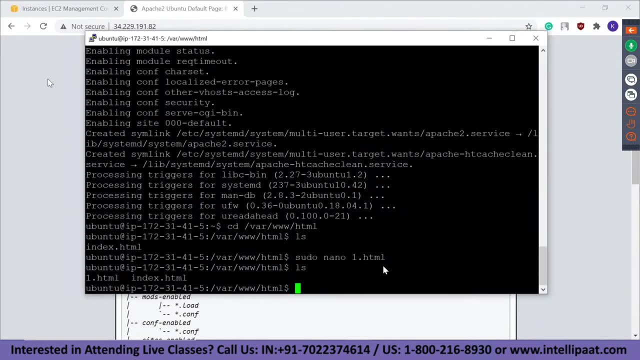 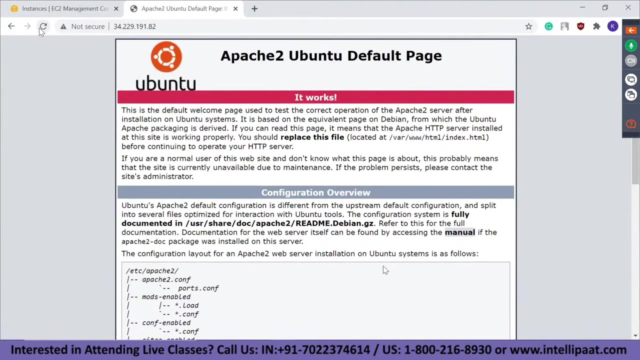 and i'm going to type in hello world and saving this. okay, right now i have two files: indexhtml and 1.html. so if i refresh this, which is the file do you think will open? is it indexhtml or 1.html? so if your answer was 1.html, you're wrong. it basically searches for the indexhtml within. 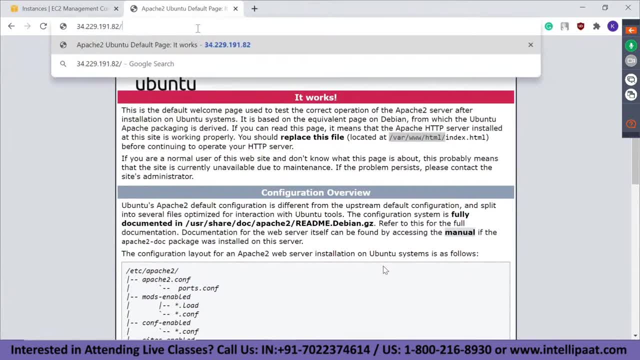 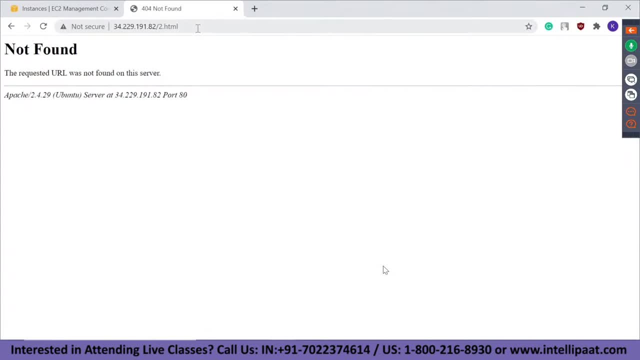 this location. so right now, if i search for a file which is not available in that location- let me search for 2.html- it will show an error because there is no file called 2.html within that particular directory. but if i search for 1.html, you can see it shows the hello world page. so this: 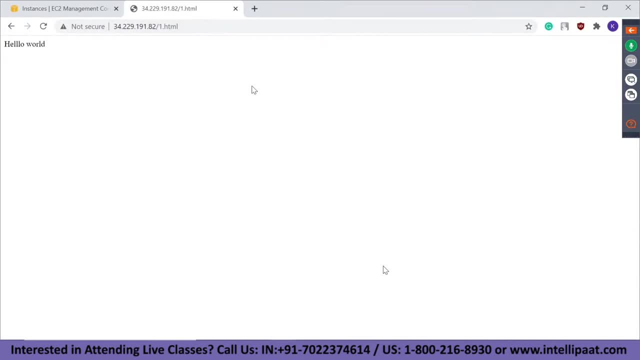 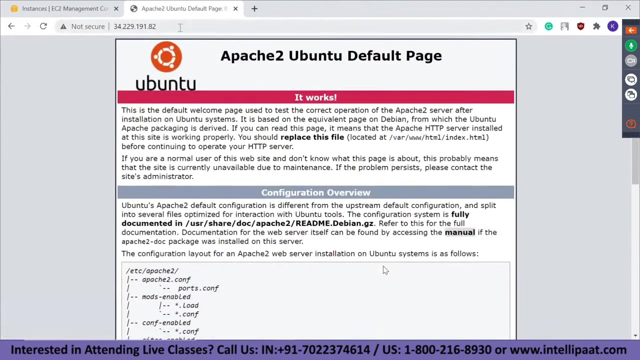 is how you can also host your own web page on the internet using pc2. so pretty much, you're just installing a basic web server in which you are uploading your files. so if you want your website to appear whenever you type in the ip address, in that case what you'll have to do is we'll just have to delete this indexhtml file. 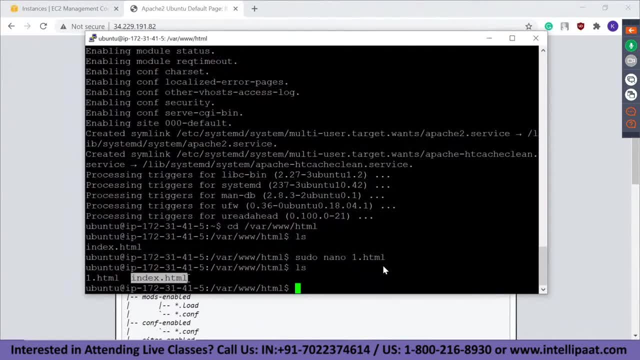 and create a new indexhtml file and put your code inside that indexhtml file. okay, so i think i've covered how to create the uh an instance and how to launch a web server as well. so this was not part of the session, but i just wanted to show you guys so you can basically start off with ac2 at a single go. just a quick. 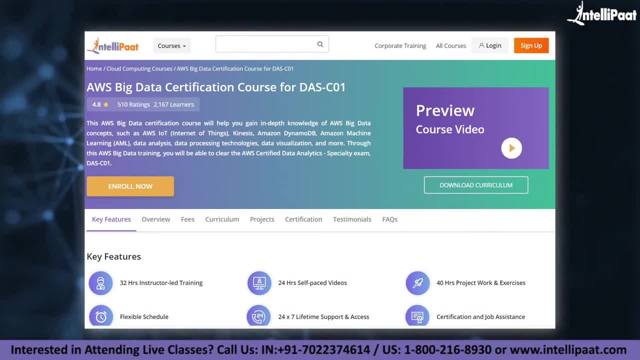 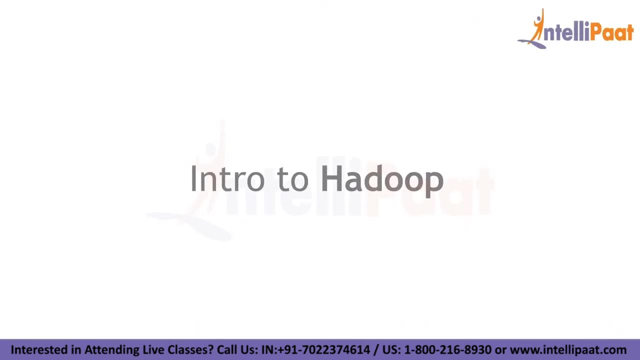 info guys. intellipaat provides aws big data certification course mentored by industry experts, the course link of which is given in the description below. now let's continue with the session. uh, we get to the introduction to how to uh, so we're going to be solving. 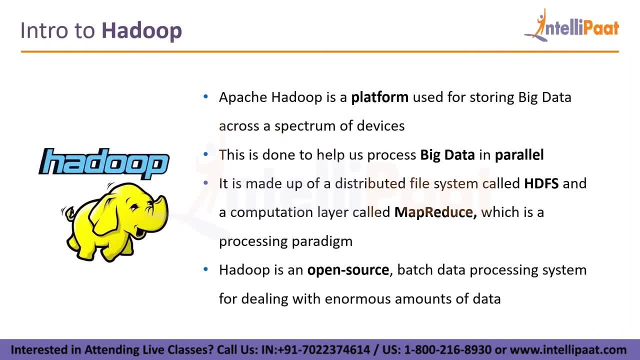 those problems by understanding what hadoop is right. so, uh, big data obviously has a lot of issues when it comes to computing it, when it comes to storing it. right, you cannot store big data on a normal computer that has one terabyte hard drive, obviously, if the 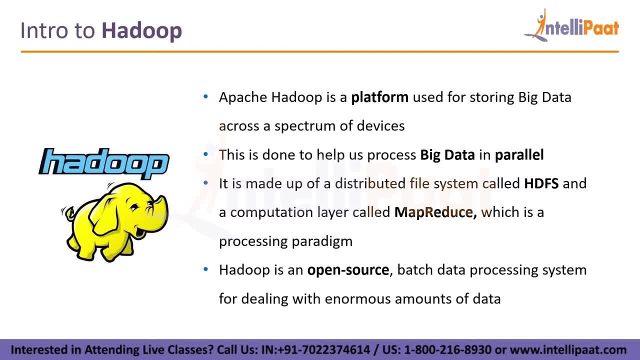 data is above one terabyte, you cannot be storing it on one terabyte hard drive. and even if you manage to uh have a uh combined hard drive of, uh say, five to six terabytes and you're storing that data on it, right then what will happen is what's going to happen in the future. is it's going to turn of processing it at the middle of the night, which is when we do this entire thing, and all of a sudden it just exits. that still, uh, and that's the point of the fan Prose, supernatural, the era. That is got to be at the end for us, because obviously we do a lot of things. but i want to. 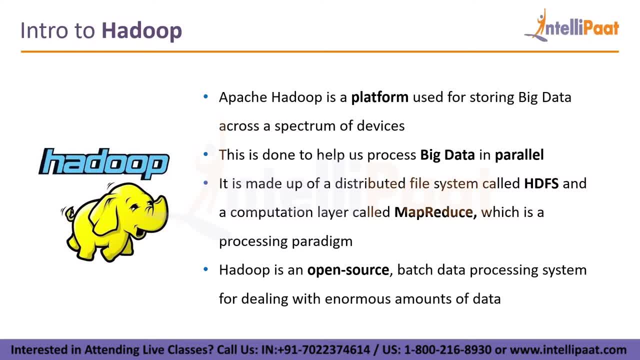 what happens when you try to process it. it will take days, right? if you try to process terabytes of data on your computer with a single i7, even i7 cpu, it will take days to process that amount of data. so the uh alternative to that would be to actually have a lot of computers combined together. 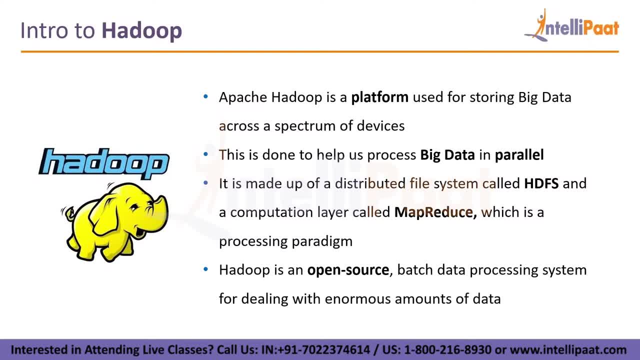 so we'll get to that. apache hadoop is a platform used for storing big data across a spectrum of devices. so instead of one device, apache hadoop as a platform comes in. it's a framework that allows you to combine multiple devices together using lan wires, right or network uh. you combine the multiple. 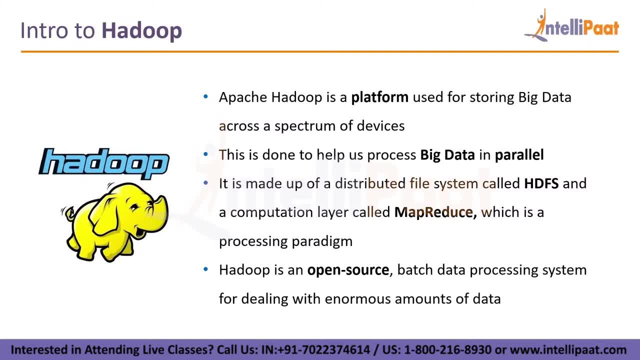 devices together and you store that data across those multiple devices instead of just one device. so this is hell. this is useful to process this big data and store this big data in parallel. so that means that, uh, you divide the data into a certain amount of parts, right, and then the data is put. 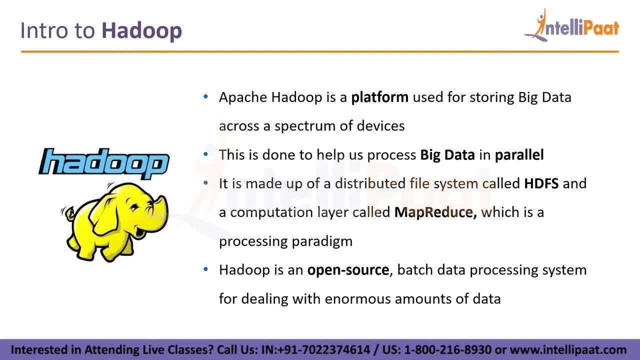 in parallel, so each computing device will process that block of data that it has been assigned. so that is what it means. so when you compute all of that data in parallel, you drastically reduce the time in which the data can be processed. so it is made up of distributed file system called hdfs. 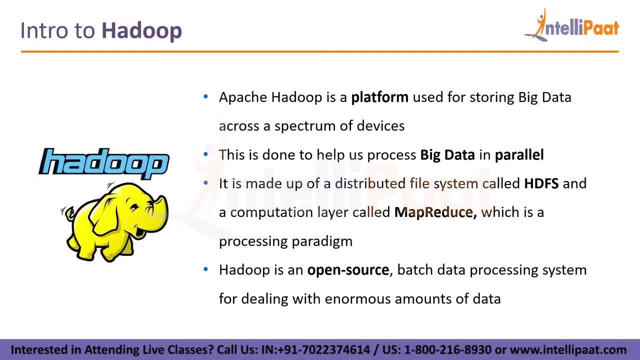 which is the hadoop distributed file system, any computation layer called map reduce, which is hadoop's processing framework. so hdfs stores the files and map reduce processes the files and hadoop is open source. so, obviously, if you want to tinker or tinker with it, if you want to add, 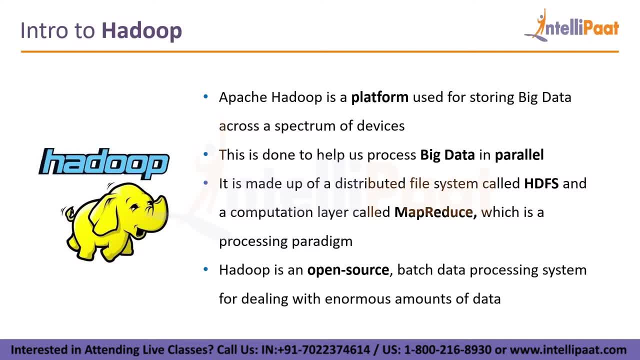 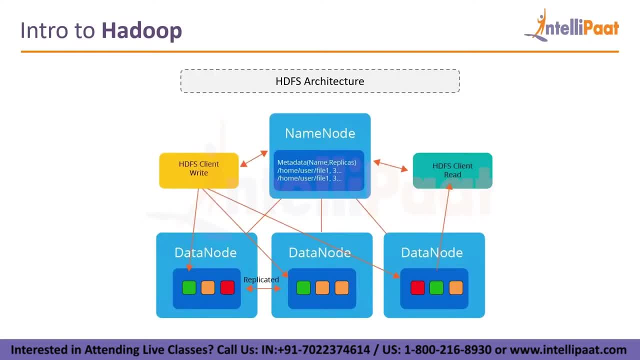 some upgrades to it for your own use case. you can easily look into the source code of the hadoop framework and edit it according to your needs as well. so let's continue. uh, let us look at the hdfs architecture now. uh, follow me here. uh, basically, hdfs is uh comprised of: the name node, data node. 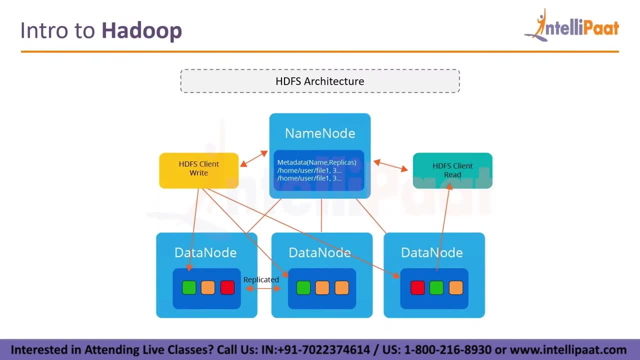 architecture. so what does that mean? uh say, in your hadoop cluster that you have created to store and you have combined eight to nine computers. nine computers, let us assume you have combined, uh, not nine computers, four computers you have combined right, so you have connected them, uh, through lan. 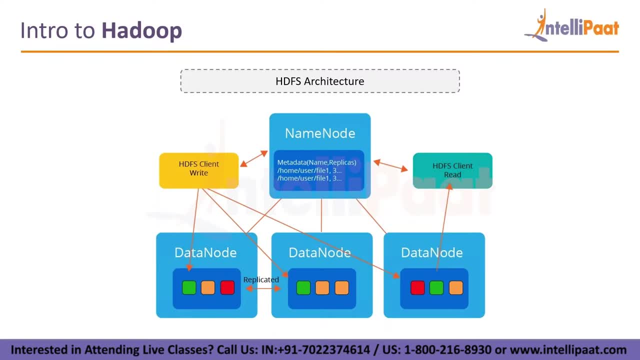 wires, you have created your network. so the computer with the weakest specifications, with the weakest processor, with the weakest, with the lowest ram, with the lowest hard drive space, you will assign as your name node in hadoop, and the computers with decent specs, specifications, you'll assign as data nodes. 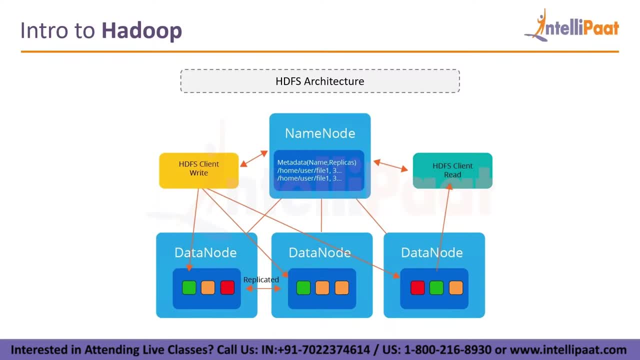 so one you assign as name node and the rest of the, the remaining three you assign as data nodes and you connect them all together, right, and hadoop is installed on top of them. so when you come in and try to store a- uh, five to six terabyte file, right, you come in and try to store that. 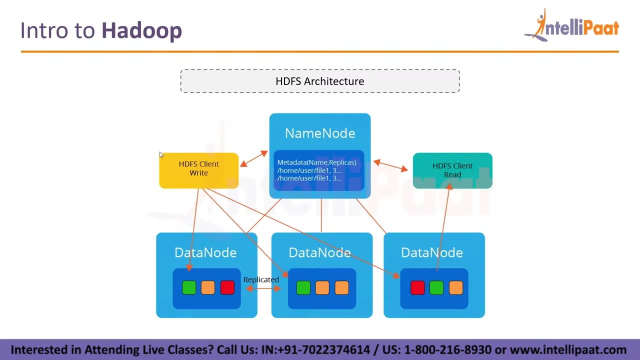 what will happen is the moment. uh, you as a client- as you can see my mouse over here, right, uh, so you as a client, you try to access this hadoop server that comprises of these four nodes. you will contact the name node and you'll say: i want to write a file of this, three terabytes, this. 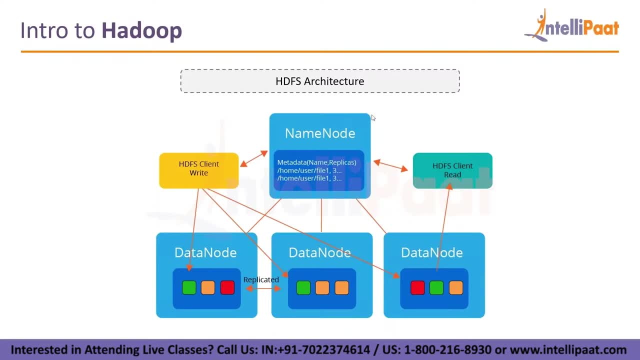 big data file of three terabytes onto this hadoop cluster which comprises of these four nodes. so the name node will then check all of the data nodes. it will check all of the data nodes, it will look for the space present on these data nodes right and it will look of the status of these data nodes. 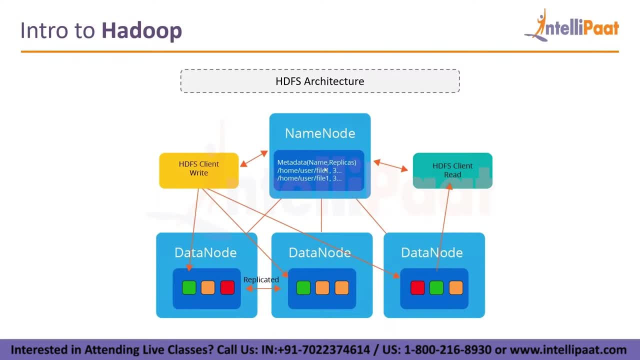 whether they are active or they are not active. once it has determined all of the specifications and the status, it will then divide that file into uh parts, into blocks. right, so these blocks, uh, you can determine the size of this, these blocks, by specifying in the configuration, but it can be. 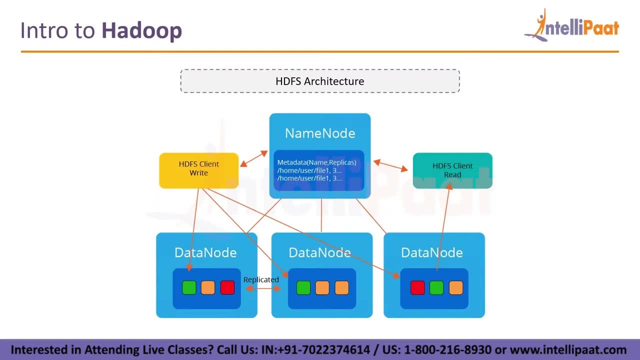 around 120 mb at an average. you can specify blocks. so what this particular uh name node will do? it will divide the file into the block size uh, as many blocks as possible, and then it will start distributing those blocks across these data nodes: one, two and three and uh. 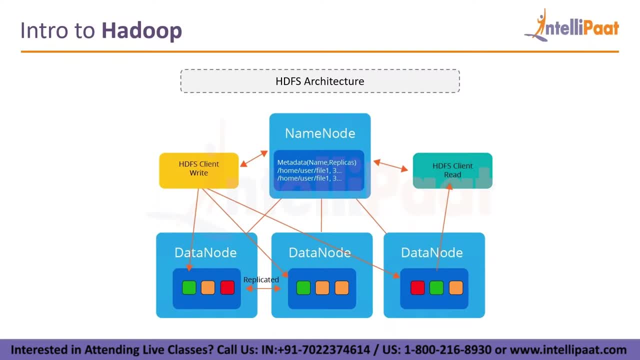 in a relatively proportional amount, depending on the space these data nodes have. it will distribute them and store them on those data nodes. right, the name node will store, uh, the metadata of this data as to where, what part of the block is there? uh, so the part one is on, say, data node one. it will store. 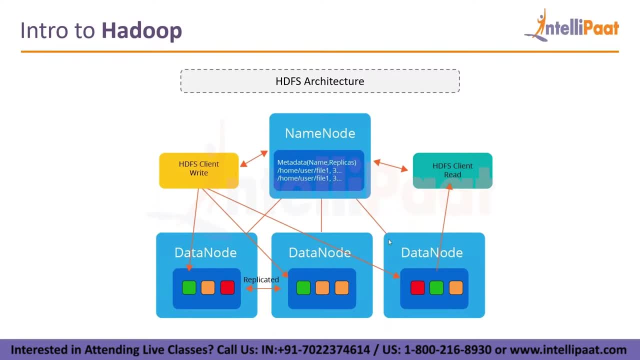 that information. the part two is on over here, the part three is on over here. name node has all of that information, right, so it will do that. then what the data node will do is it will replicate those blocks across all of these, all of uh. depending on the replication factor, it would be two, three, four, depending on how many times it has to. 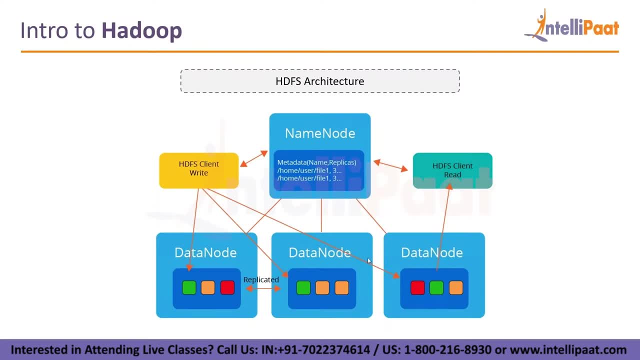 replicate those blocks. it will replicate it across these data nodes. so replication is done to prevent any sort of data loss. so if you store only one copy of the block on one data node, what will happen is if one of the data node fails, right, you lose that block permanently. you don't want that. you want to. 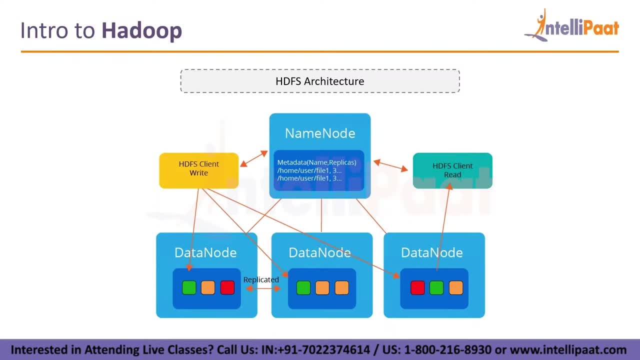 replicate it across the data nodes. so even if one data node fails, you still have a backup of that data, right? so you replicate it across. depending on the replication factor, you replicate it across the data nodes and you have your file stored on the hdfs server, right? you have a really big file. 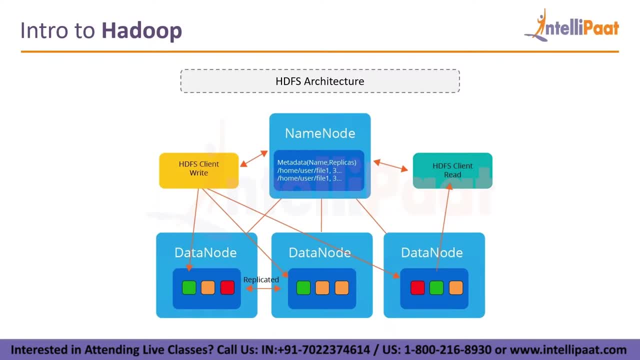 a six terabyte file stored across this entire server right without any issues, without any particular uh data node having to store a lot of data. you have divided it very uh specifically for that purpose and only then say a hdfs client wants to read that data, right, so he'll try to access the. 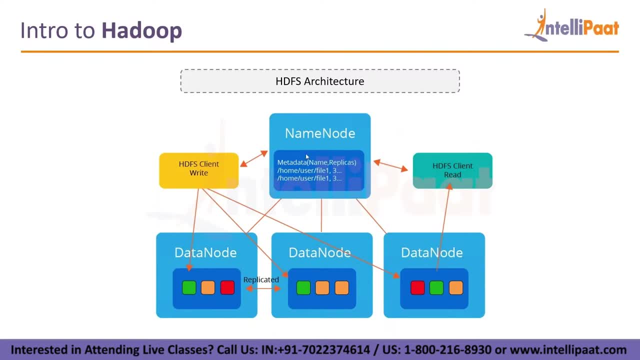 name node again. right, he'll ask: where is this file? the name node will tell that client the file is present. uh, the first part of the file is present on this particular data node. the second file is present on this. third part is present on this right. and, uh, the best thing about the data replication is that the client will read the. 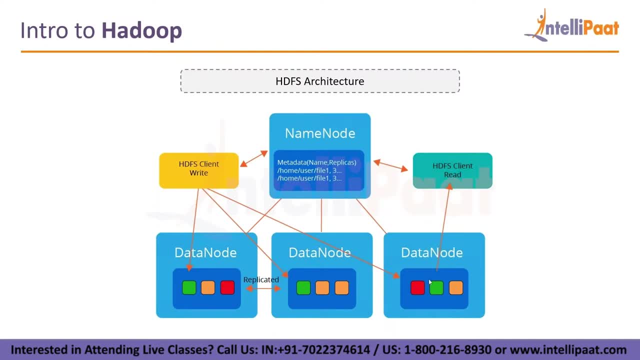 files that are closest to him. so, from a latency point of view, from a closeness of device point of view, where there is the least latency involved, the client will fetch that data from the least latency, causing data node right. so so the closest block that he has, he'll fetch it from this data. 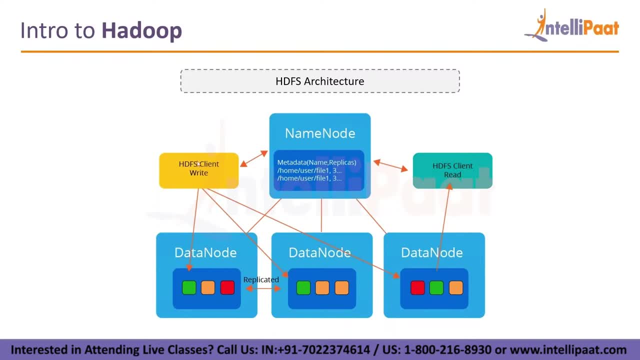 node, even though this green block is over here, the writing. the original green block was over here. it replicated and was stored on data node 3 as well. so the client read it as well from the data node 3 because it is the closest to him right, and similarly he'll read the other blocks as well. 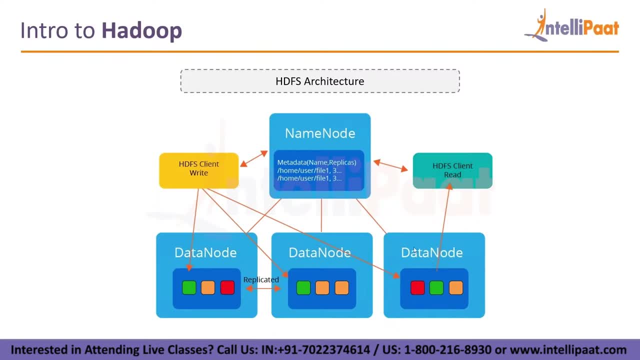 he'll combine all the other blocks. uh, basically, the data nodes will combine all the other blocks and give him the combined view and the client will be able to read the data. so this is how storage works. so let me look at some of the questions that have come up. so, uh, one question is by rupal. 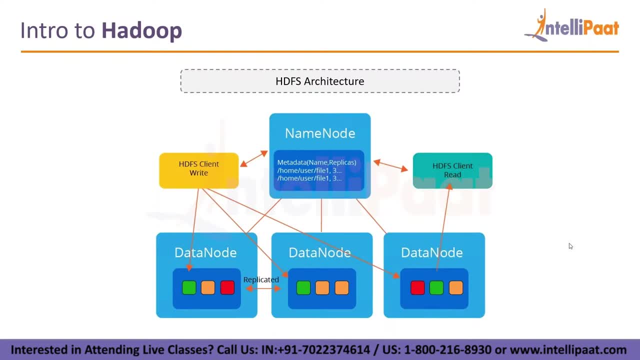 he asks. in that case, three terabyte files will become, uh, about 12 terabyte files, uh, with the replication. so, uh, not exactly. so here i was talking about only four nodes, right, but there can be more nodes, so don't? i actually took a very big size, like a six terabyte, so don't, don't, uh. 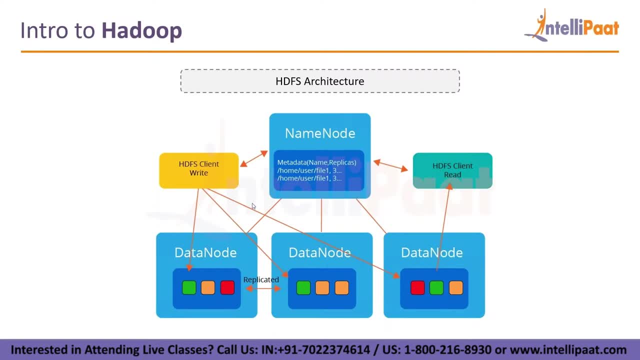 particularly think about that. but imagine this: if you have, say, a hundred nodes on your big data- usually the case for big companies, so you have a hundred nodes, right? so in that case a replication does not uh, multiply your data by that much amount. it will still be there across the data, the size. 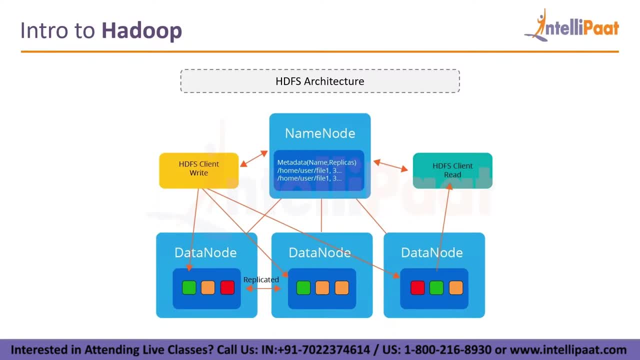 will be increased, obviously so, because you're replicating that data. obviously you're also increasing the size of of that particular data, but it will not cost your hardware as much because it will be stored evenly across those hundred nodes. it doesn't matter, uh, even if you're increasing the. 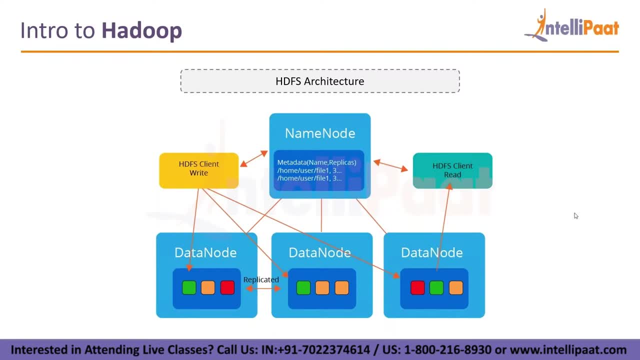 size of those hundred nodes. it will still be there across those hundred nodes. so that's a good, good question that you asked. that was a good doubt that you had, uh, these four data nodes that i have taken here, that there is an example that is not the case with actual live cases, that you will only 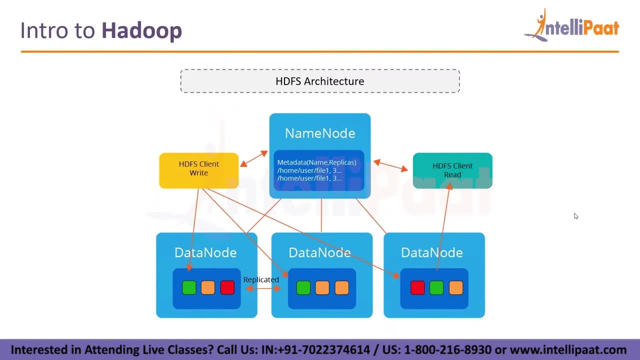 have four nodes. so in that case you're obviously you're uh costing your hardware too much by storing it almost entirely on the hard drive space of those four nodes. you don't have to do that. so one other question: data node have multiple copy to prevent failure, but name node has, uh no, what will? 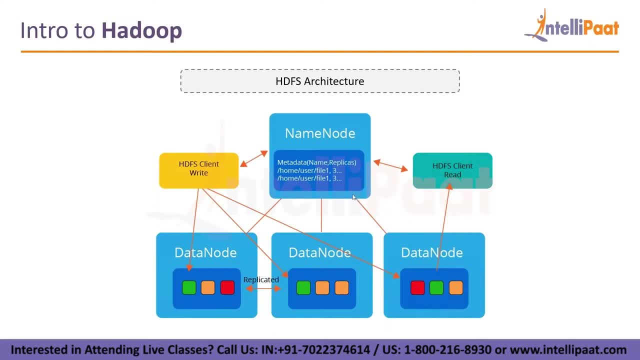 the thing is, you can also configure the name node or to be multiple as well. so in that case you can. you, there's no limitation to how many name nodes you can have. uh, big companies, obviously, where the data is very sensitive in nature and cannot be lost, obviously there is a backup name. there will. 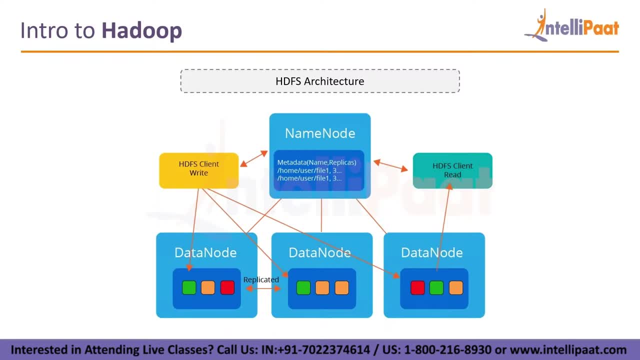 always be a backup name mode and it is impossible for any organization not to have a backup name right. so the data of the name node is also replicated. don't have to worry about that one. so, basically, you can pick a block number. that is in the model. so you can pick a block number. 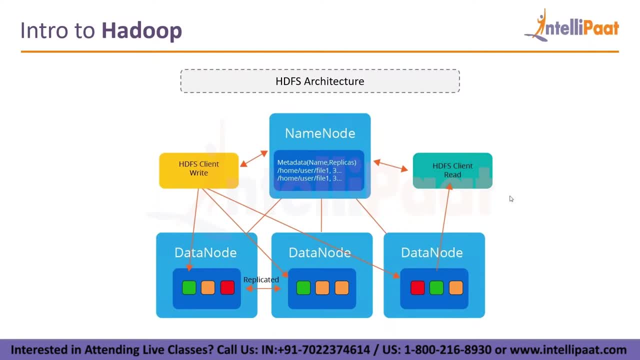 actually it will tell you which data nodes are the closest and the closest to the client number, the sequence of the blocks, the hdfs client is a person or a computer at the client's end. so basically what that happens is, uh, the name node will essentially tell the hdfs client. 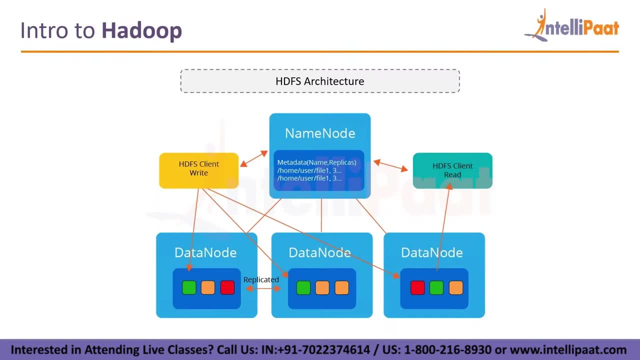 uh, that you can pick uh, depending on the latency that the client has with the name nodes. uh, with the data nodes the name tells you you can pick uh, block number one from this particular data road. you can click that particular doubt. are there any other technologies that like Hadoop to? 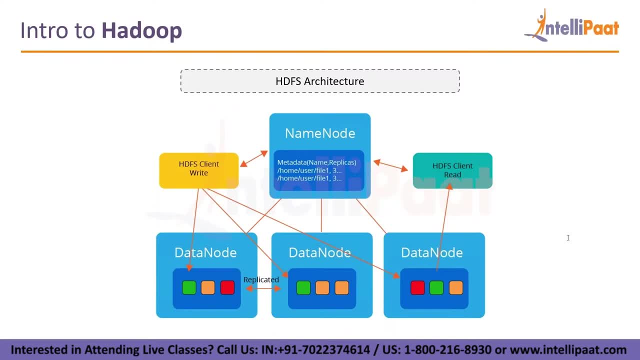 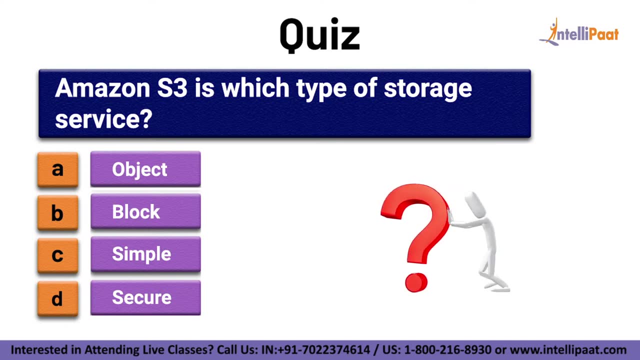 process, big data or is Hadoop the only solution? just a quick info, guys. test your knowledge of AWS by answering this question. Amazon s3 is which type of storage service a object be blocked? see simple D: secure comment. your answer in the comment section below. subscribe to in. 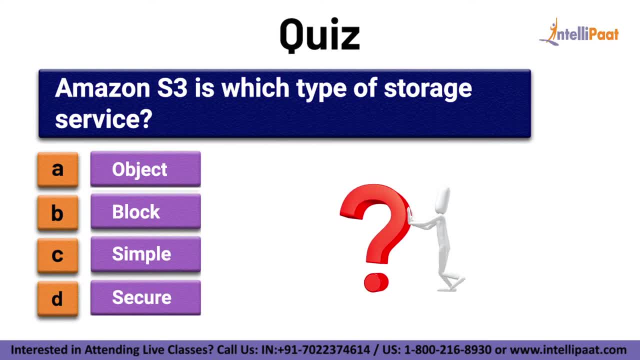 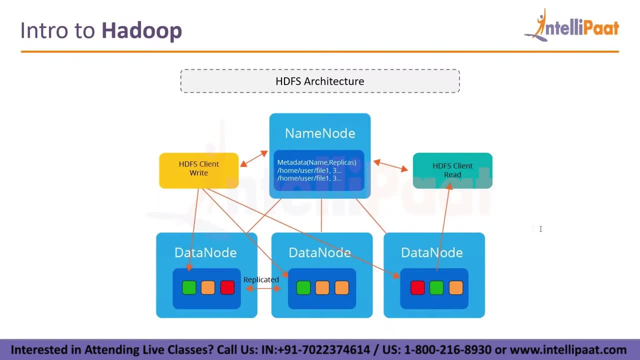 telepath to know the right answer. now let's continue with the session. there are other solutions as well in today's world. obviously we are going to talk about some of the solutions that are available in the world, but obviously there are other solutions. but what? obviously there is a. 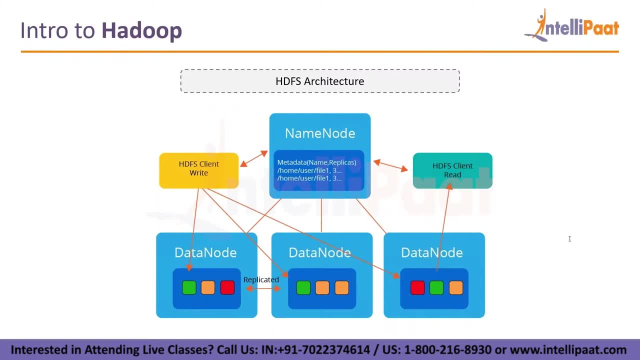 this thing, that Hadoop's map reduce, the processing framework of Hadoop, which we're going to discuss in a moment over here. if the processing framework of Hadoop is now outdated, the map reduce is not used as much anymore. it is used for fundamental concepts, for very custom programs, but it is not used in much. 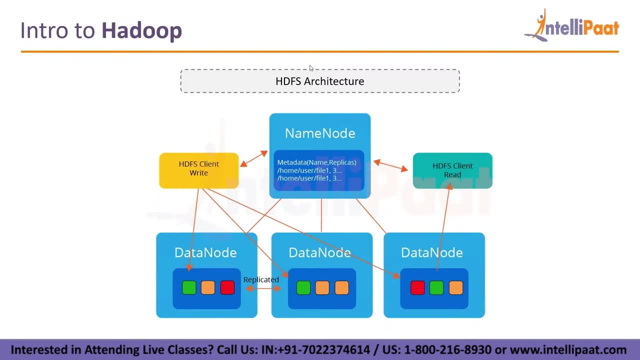 frequency anymore. what we still use, though, is the HDFS. we still use. the technology is based on the HDFS, the Hadoop distributed file system, for our storage. we do that, so how do we still relevant in that way? we use her to for storage today very, very frequently. we do use it. 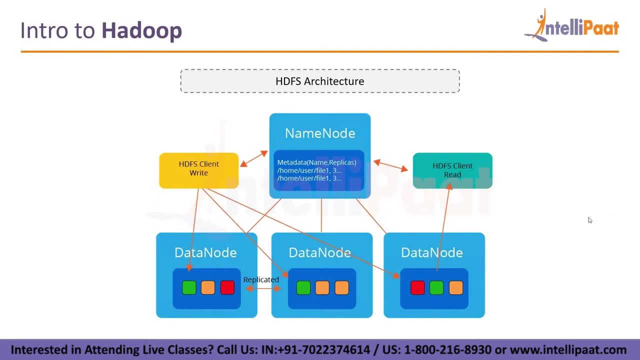 what happens with the name node fields. so I have already answered what happens. so the name node fills in this particular case. obviously, if the name node fails, we will have a lot of problem on our hands. so we'll, in a professional environment, will always have a backup of the name node as well. we'll have another name Routs. 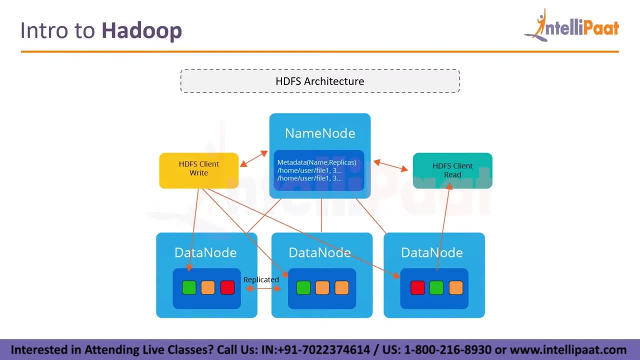 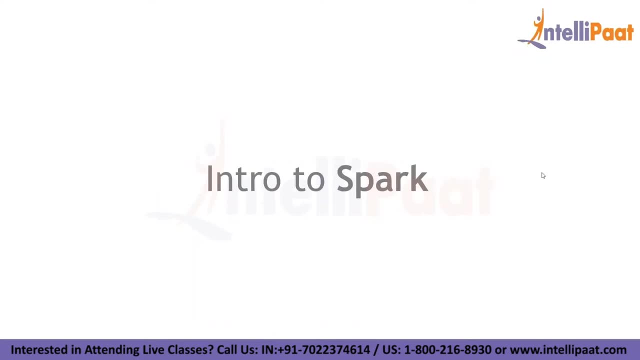 that backs up the data on the first name. so that is there. we don't actually lose the data of the name, no way that happens. so let us look at the next slide. so introduction to spark. so now that we have an introduction to hadoop, right, so we will have an introduction to spark just a moment. 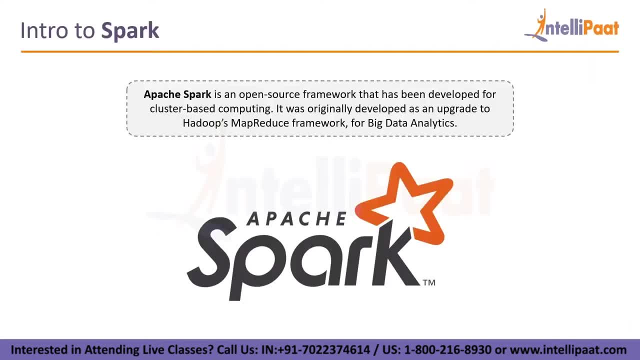 yeah, introduction to spark: apache. spark is it's by apache. again, hadoop is also by apache, spark is also by apache. so these are essentially technologies that are developed in universities and organizations and then apache adopts that particular technology. it becomes open source. so spark is also an open source framework that has been developed for cluster-based programming. 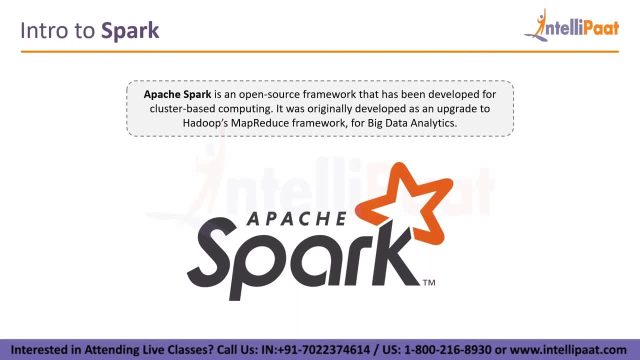 so oftentimes in big data domain you will see this term being used called cluster-based programming. so this term is based on hadoop's original idea to combine a lot of computers together: commodity level hardware, very user user level hardware, not advanced hardware like servers and everything normal computers together create a cluster in a network. 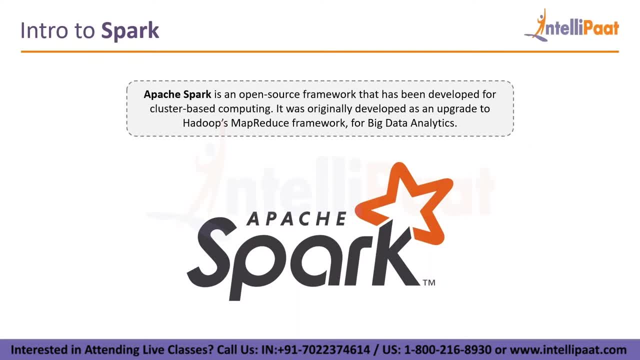 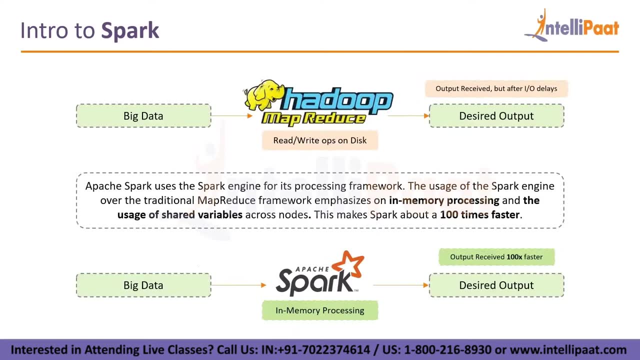 and then install hadoop on top of it. so it was originally developed as an upgrade to hadoop's map reduce framework for big data analytics- hadoop's map reduce framework. i will talk about this. so what happened in map reduce was, uh, you had these file blocks present on various data nodes. 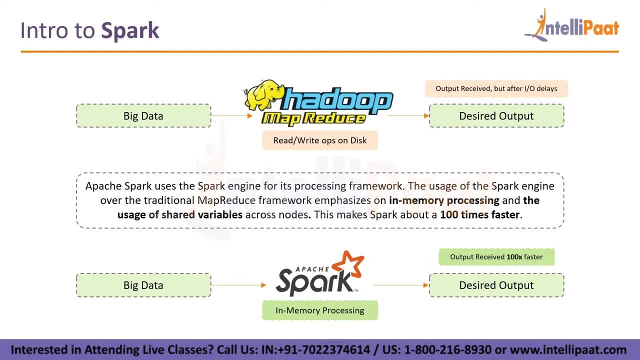 across your cluster. the map of this framework essentially took the big data that was there on the respective block, on the respective node, data node. it took it and then it, uh it- the data was present on the disk, obviously the hard drive, the data was present on the hard. 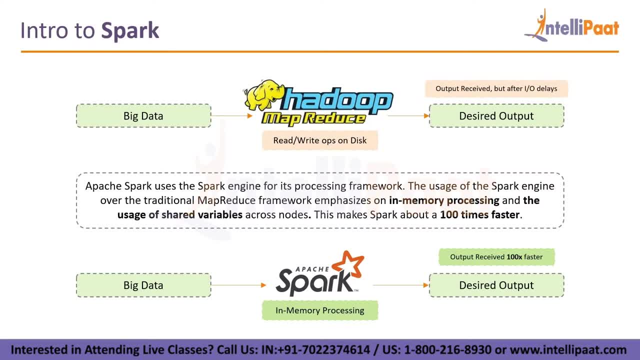 drive. it took it from the hard drive, put it into the ram, then from the ram it was then put it into, put into the cpu. the cpu processed that data and then it output that data, uh, back into the ram, and from there it was back into the disk, right. so the problem with this particular approach, right, when 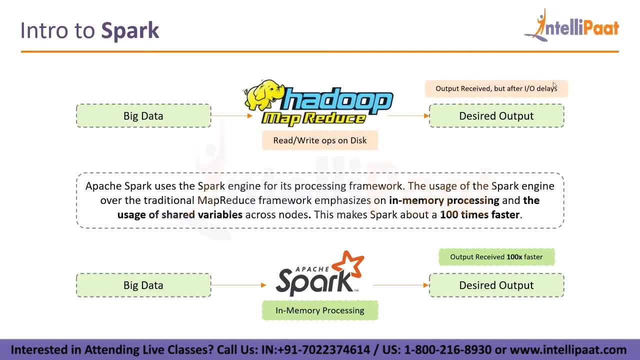 you get the desired output. there are a lot of input output delays. so what does that input output delay mean? so, uh, essentially what that means is that, when you transfer data from your hard drive to your ram in order for it to be processed by your cpu, there is some latency, there's some delay. 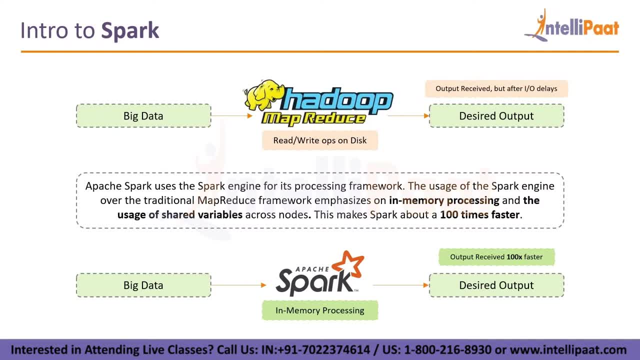 involved to that. so, since you're dealing with big data, right you? what you'll often find yourself doing is transferring it from the data from hard drive to ram and then ram to hard drive data. so what that does is it increases the time in which your processing will happen. 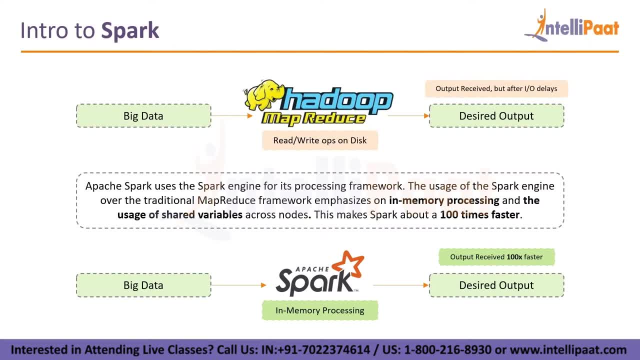 right. so this was the case earlier on, when ram used to be really expensive. right today, ram is really cheap. you get like 64 gbs of ram on your mobile phone, right? that is how cheap it has become. earlier, uh, ram was really expensive, so we used to have like two gigabytes of. 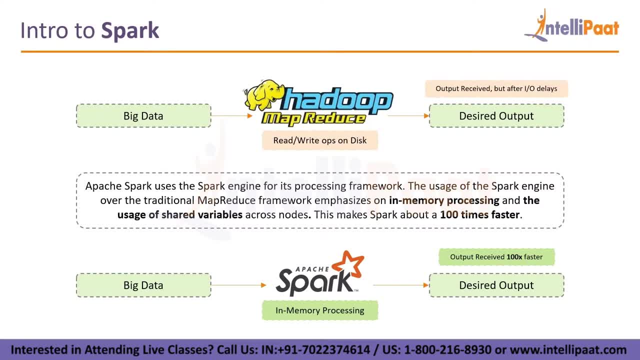 ram at maximum on a computer system, right? uh, that was even on the higher side that you had two gigabytes of and there was a really extremely good computer, right so, to process this data, uh, we were relying on the hard drive more than the ram because we used to store all the intermediate. 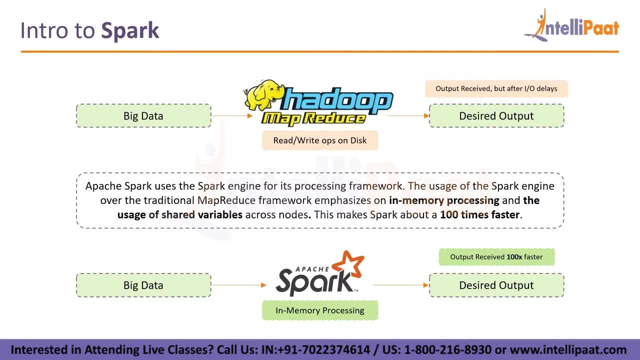 information in the processing on the hard drive and then put it back into the ram. so that caused a lot of input output delays. so as ram became cheaper, right, so we came up with a purchase bar. it uses a spark engine for its processing framework, which is the framework engine. processing engine. 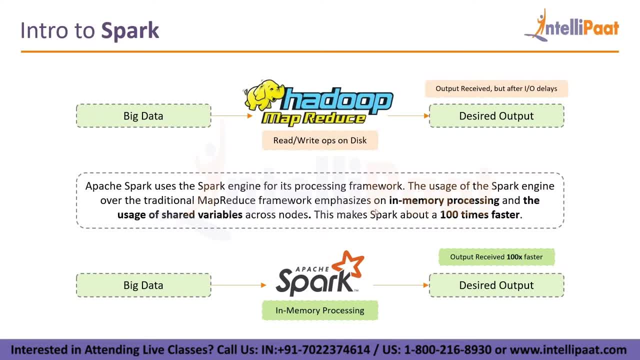 the usage of the spark engine over the traditional map. reduced framework emphasizes on in-memory processing and the shared, your use of variables across nodes, so this makes spark about a hundred times faster. uh, so what that means is, uh, that when you have this huge amount of ram, like 16 to 64 gbs of ram- on your computer, then you 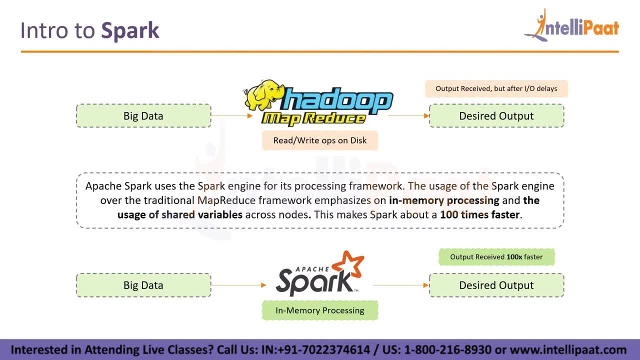 can simply transfer that data from your hard drive once into your ram. ram is what memory means. by the way, for those of you who are not familiar, in memory means ram, right? that is not your hard drive memory memory in memory means a random access memory, right? so this is where the ram is right. so you. 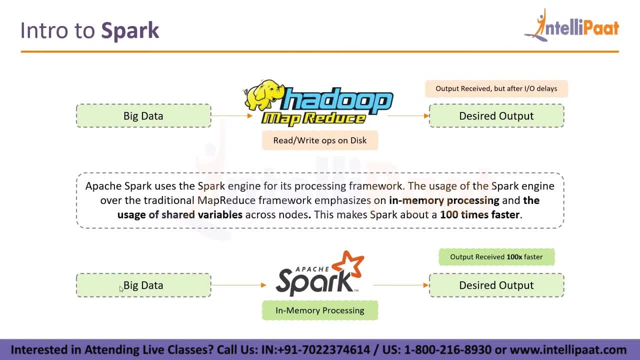 transfer that when you start with your processing job. right, you transfer that data once, once, only once, from your hard drive to your ram and then it stays in the ram until the job is complete. so all of the information that is created, all of the intermediate data that is created, that is still. 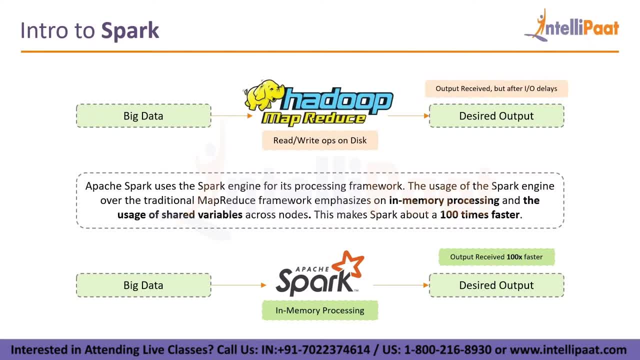 present in the RAM. the hard drive is not contacted again, unless until the output has been created. when the output has been created, you can surely store it in the hard drive or not, depending on what you want. right, yeah, until the output is created, you don't need to store it back in the 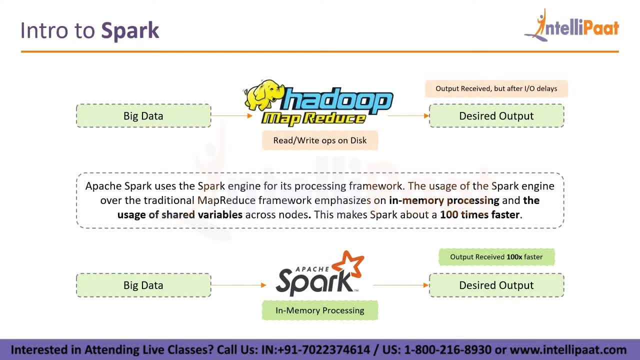 hard drive. so this absolutely decreases the input output delay that you would have from transferring the data back and forth from the RAM and hard drive right. so this makes, in the long run at least when you have a really big task, when, when you compare the efficiency of MapReduce and spark. 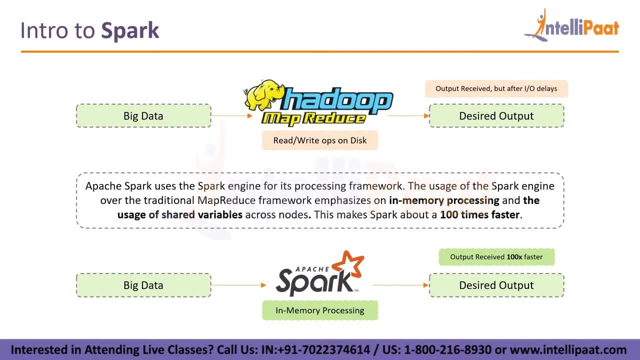 if you have a really big task right. spark is about a hundred times faster than MapReduce in that particular case, so that I hope you understand why that is so. any questions in this particular regard? so there's one question that I can see: can spark work on file system that are not HDFS? yes, spark. 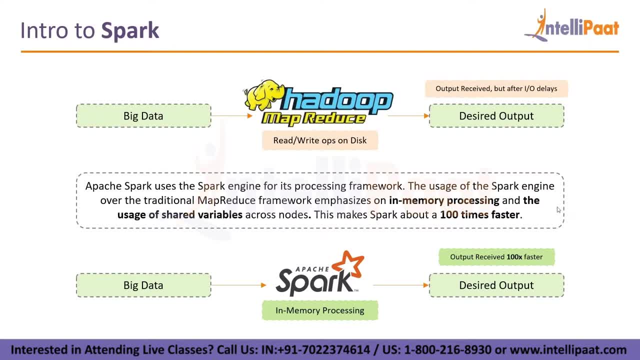 is compatible with file systems that are not HDFS. in fact, that is what we're discussing in the next slide. there's one other question, since spark works in memory, are there computers with terabytes of memory? no, there are not computers with terabytes of RAM, but if you have like six gigabytes to eight, 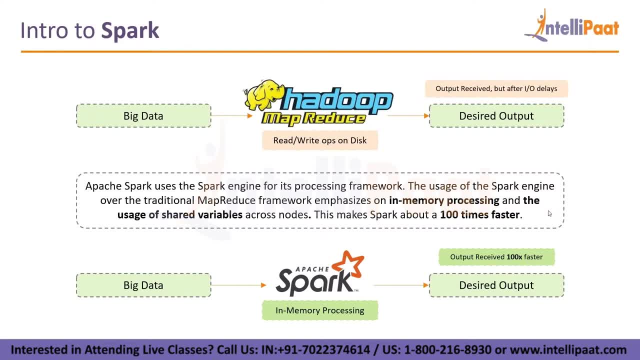 gigabytes of RAM across hundred computers, then across hundred to a thousand to five hundred computers, depending on whatever there is right, you will have a lot of RAM in collective together. right, that works for it. and one other doubt that is there. that is a very valid doubt. what if the size? 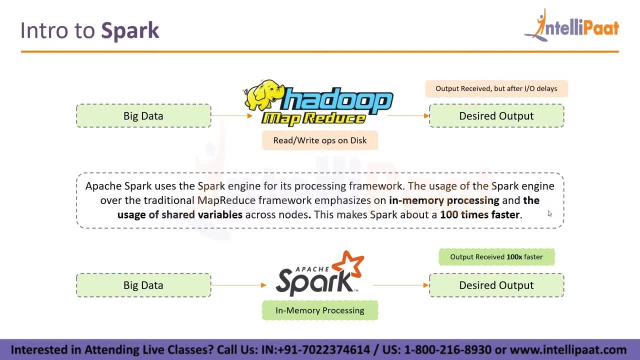 of the data is greater than the RAM on that particular node, which is a very viable case, right? so in that case, what happens is you will have a certain percentage of data still present on the hard drive- right, it will still be there, and as much data as you can, you'll put it onto. 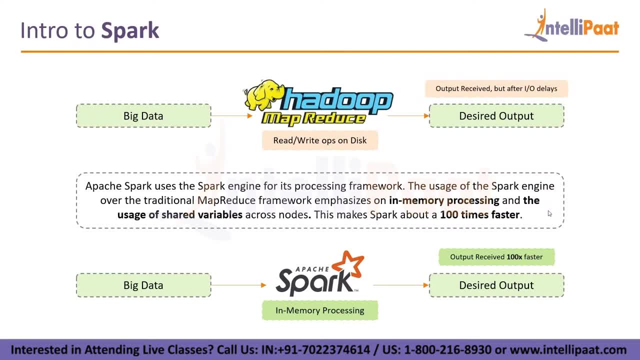 the RAM. you'll process that first and then you'll take the data from the hard drive and process it later, right? so yes, that increases a little bit of latency, but it's still relatively really fast as compared to a MapReduce. obviously, if you don't have space in your RAM, you'll still have to store. 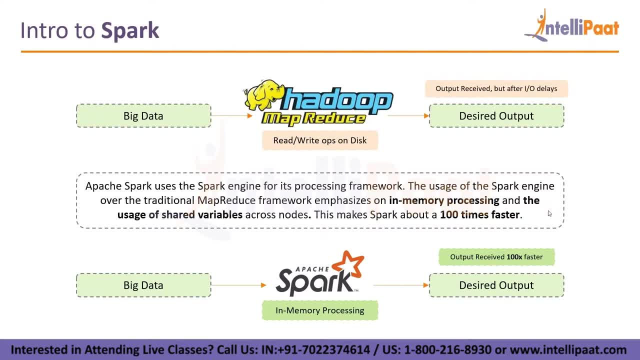 that data in the hard drive? that is not a question. if you don't have as big of a cluster, then that will be the case. if you aren't able to divide your data into very small blocks, that would be the case. yes, what is the minimum RAM? 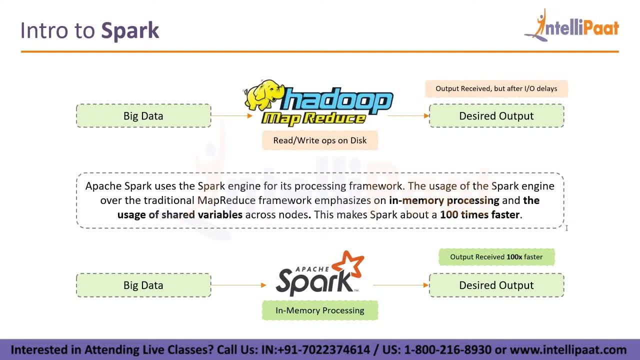 requirement for Spark. so it's generally recommended if you have a large enough cluster. it's generally recommended to have at least four gigabytes of RAM right on your computer as a data node. as a data node, if your computer is attached to a Hadoop cluster, then it's generally 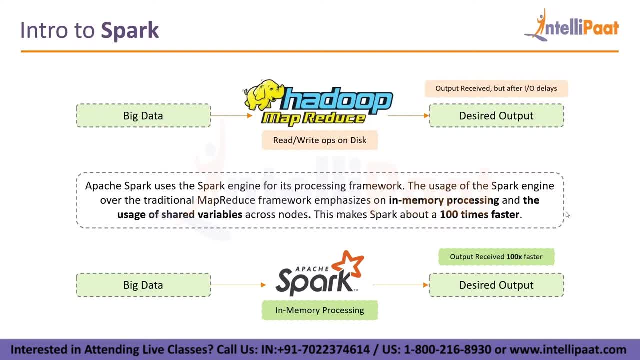 recommended to have four gigabytes of RAM to actually be useful in the big data jobs, but you can have lesser RAM as there's not a minimum requirement. it's just it'll just be that your data node, your particular data node, will not be as effective, so it will be a bad investment in the first place. 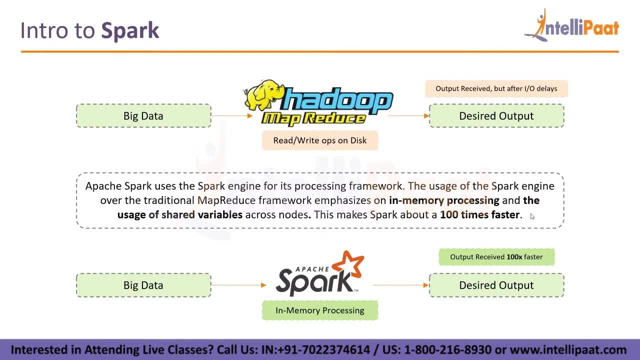 so for data nodes there's not a minimum requirement. obviously, if you're running a single node cluster, which means you don't have any data nodes, you only have, say, a- what do you call it? a name node and data node combined together, because you're doing it for practice purposes, then it's recommended. 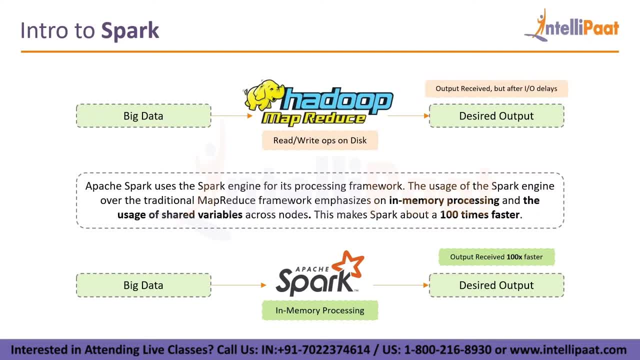 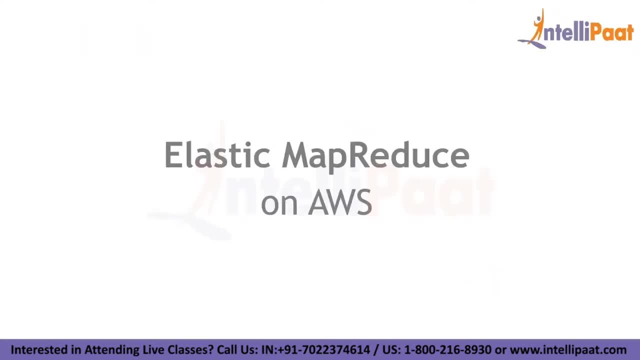 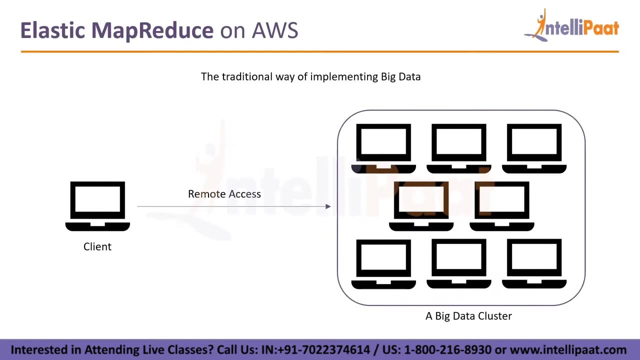 to have eight gigabytes of RAM on your single node system. eight gigabytes of RAM for practice purposes. so let's look at the next slide. so this, the topic that comes up, is elastic MapReduce on AWS. so usually the traditional way of implementing big data is you have a client and you have a big data cluster. 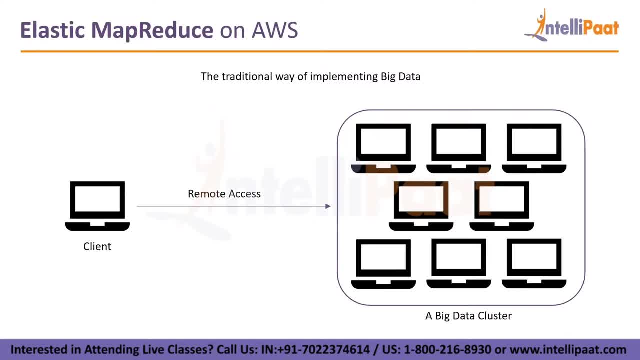 which is a Hadoop cluster. right, you have all of these computers attached together and they are acting as one single unit, which is called the Hadoop cluster. so you remotely access that and then you perform your big data jobs. so this is the traditional way of doing it, offline way of doing. 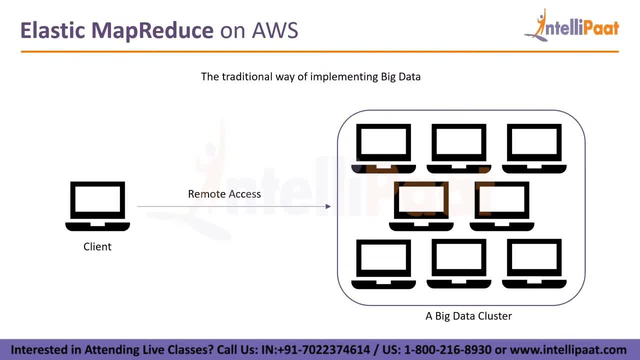 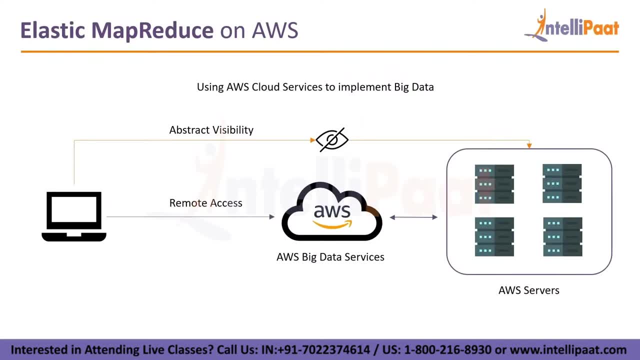 it. essentially, if you're working on a big data cluster, you're going to have a big data cluster working from office where there is a big data cluster. the other way to do it is using AWS cloud services- right, so there are a lot of advantages associated cloud services. so the advantages would 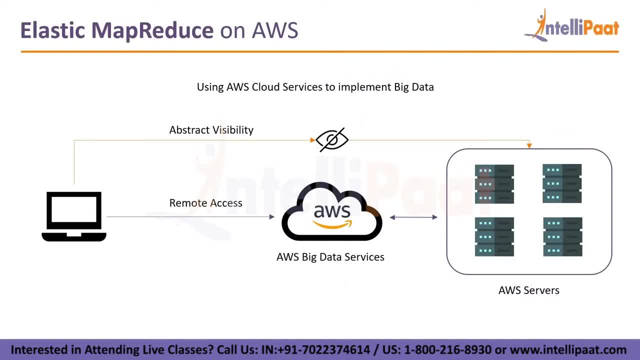 include: you don't have to have an administrative team- administration team that handles your cluster. you don't have to have a team that installs a new node on your cluster or deletes a node from your cluster. they. you don't have to have a maintenance team. you know they provide that long termvida service. you don't have to have to have a mount machine. 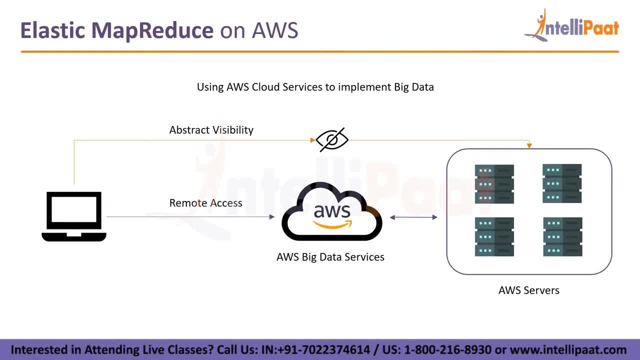 they also have busy dishes. or you don't have to have atra teller. they really package a cluster and baby building WetS cousins you can create so they work the entire cluster. so with AWS big data services members don't have to do so because they're the same person so they can store and 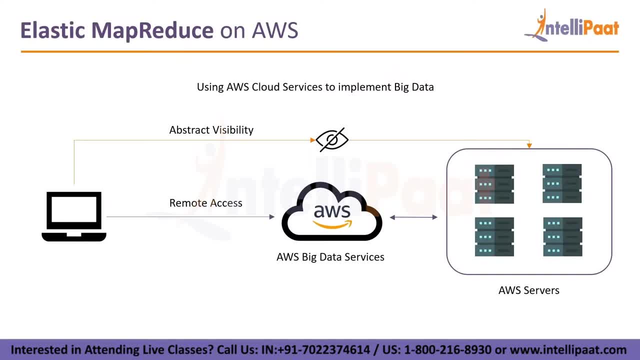 predict accurate data and they have no problem. so because of that, you can have thatlung, Blooms, Mint and things like. you can basically use Azure, LinkedIn and Android. look at the AWS big data services. it's just a click of a button. you can create a as big of a cluster as you want containing 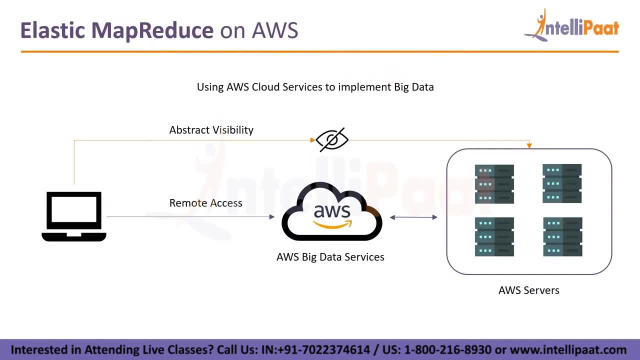 of a good enough size, right? so in that case you can simply take on the auto scaling option and the cluster size will increase or decrease automatically depending on the workload. so you can see how easy this makes the entire Hadoop administration process, right. you don't have to. 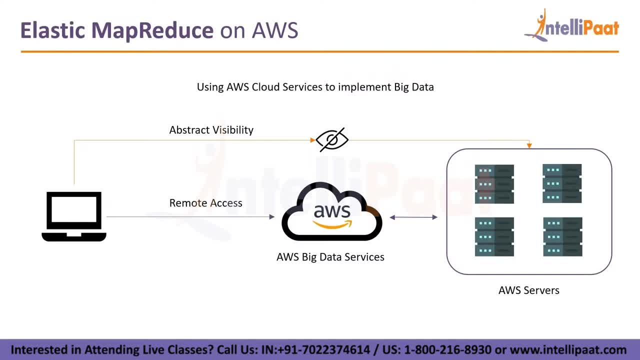 have a team. you don't have to pay a team. you don't have to AWS big data. it's a managed service. if you have it, if you have an issue with it, you can simply contact their customer support. so that is the advantage, essentially, when you're talking about cloud services in general. so AWS is. 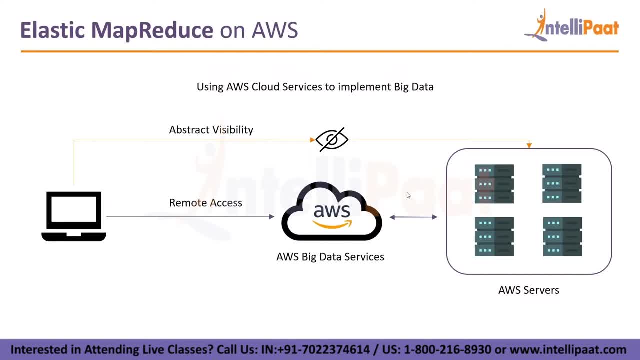 not the only service that provides this, but it's definitely the service with the best features, right? so Microsoft Azure and Google Cloud also provides big data services, but with AWS, you'll find that it is the most convenient way to actually use big data clusters. a lot of big companies use it. a lot of moderate medium companies also use it, because who has the 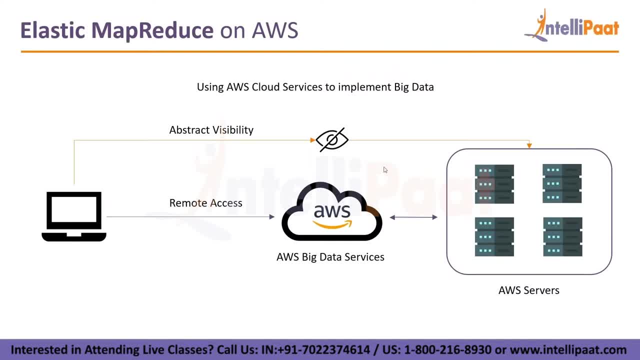 time to actually have a cluster in office, because that's just old today, right? unless you want really really low latency jobs. in that case, say big companies, like multi-billion dollar companies, they usually have these big clusters in their campuses themselves. so there's one question, very relevant question, I believe it means that this will eliminate Hadoop admin jobs in the future. 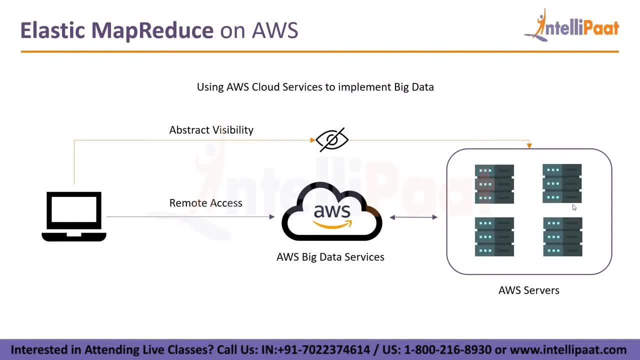 no. so Hadoop admin jobs will always be there, because it depends on the use case. if you want to use Hadoop admin jobs in the future, you can use Hadoop admin jobs in the future. you want to use cloud services or not? so say, I am sitting in India right and I have a Hadoop cluster. 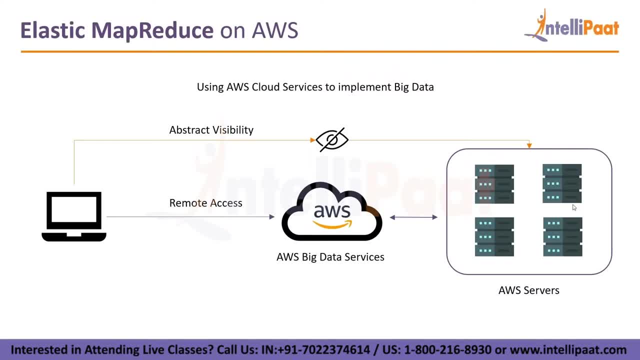 in the United States, so from India to the United States, whenever I try to contact that cluster, it will take me about 250 milliseconds at an average to ping that server right. so that is quite a high latency. and say, if I am working as a stock market broker, right, that is life or death for me, because 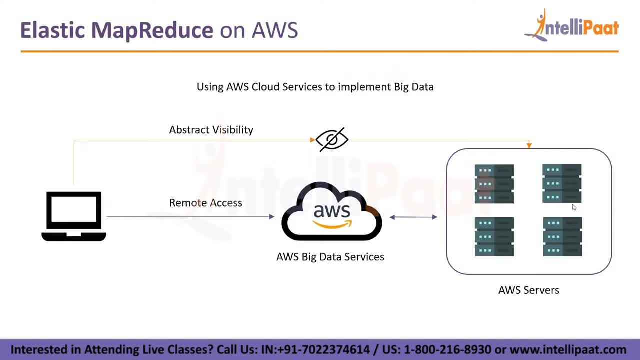 250 milliseconds of delay as a stock market broker can essentially break my trade right. so when you're trying to analyze a lot of amount of stock market data at once, right, and you want that data to be processed really frequently and really fast, that 250 milliseconds of delay can cause you a lot of. 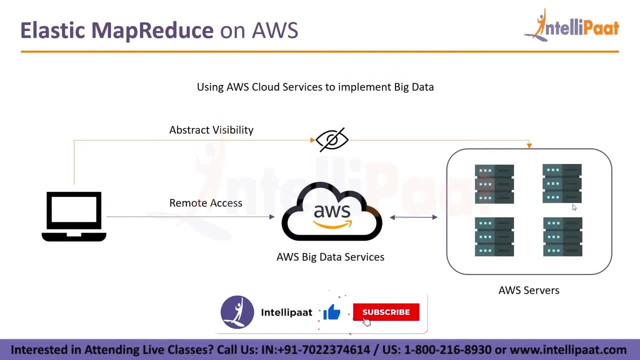 money, right. so that is a stock market example. but if you want low latency, then you will have to install this, these Hadoop clusters, in-house, right, you will have to have the server in-house. you will have to have those commodity hardwares attached in-house. you cannot have them on the cloud because the cloud will always have latency. 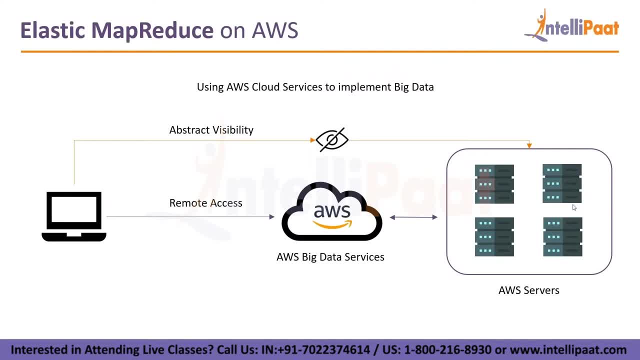 because you will never be close to the cloud, which means you will never be close to the Google servers or the Amazon servers or the Microsoft servers. so I hope that answers that doubt will not eliminate Hadoop admin jobs in the future because somewhere somebody is administrating the. 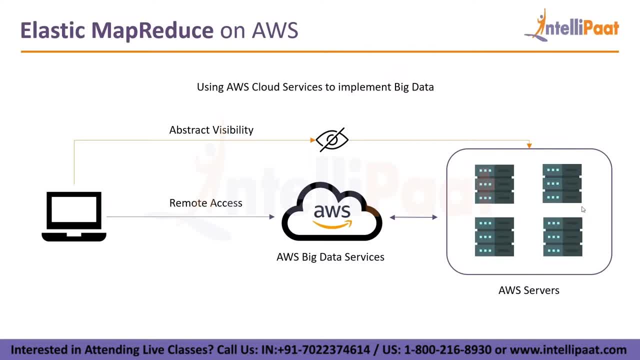 Hadoop right, it's not happening automatically. so even in Amazon somebody is doing that, particularly although it's uh our automatically handled, but there are issues involved with that as well, so you need to be uh provisioned in admin as well for those of you who have that admin job. so how does EMR cost compare? 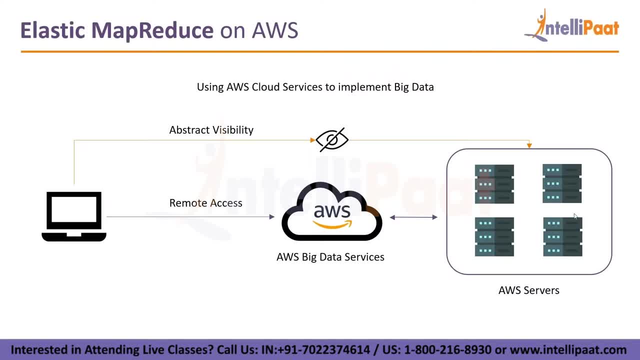 with Microsoft. offering EMR is cheaper than Microsoft's offering uh, so Amazon is the most flexible with price. actually, I have found personally in my experience. uh uh, Google cloud and Microsoft are expensive as compared to Amazon. Amazon also has a lot of options for learners, right, so if you're training uh, then it also gives you a lot of free tier options like 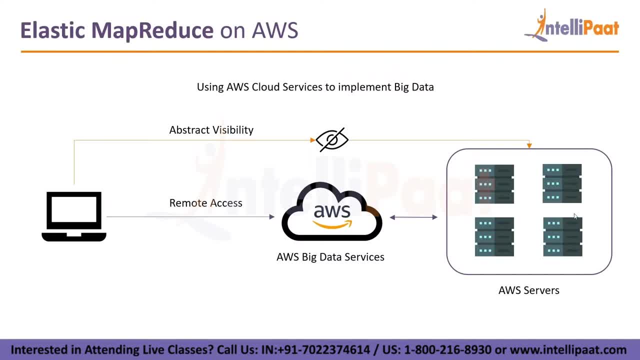 you can use one of their ec2 instances and whatnot for free. so Amazon uh is better in pricing. so while we implement Hadoop and local, do we need of hundreds of computers to do it? uh? it depends on your use case. you might need hundreds of computers to do it uh or uh, instead of having hundreds of. 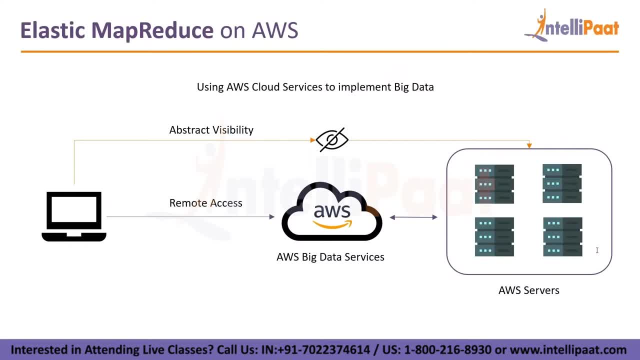 computers specifically for that process. uh, what I mean by hundreds of computers is that you have employees in your office that are in the hundreds. right? you're not actually buying hundreds of computers specifically for your Hadoop cluster. make sure you understand that. what happens is you have hundreds of computers in your office for your employees. you reserve a certain section of that. 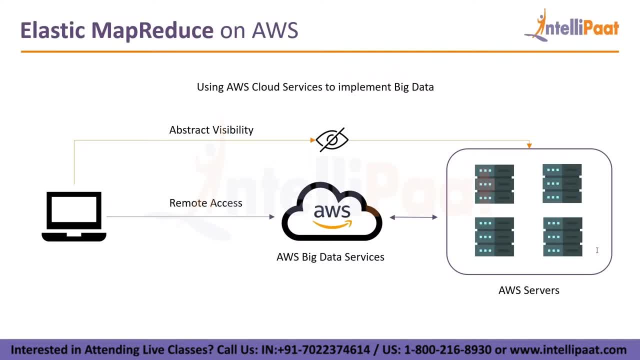 computer. uh, all of those computers are, by the way, connected to the network together. you reserve a certain section of those computers, right, and that is used for your Hadoop cluster. so the employee will work on whatever he is working on. but a certain of the computers, computing resources have been, uh, in used, reserved for the Hadoop cluster. so nobody. 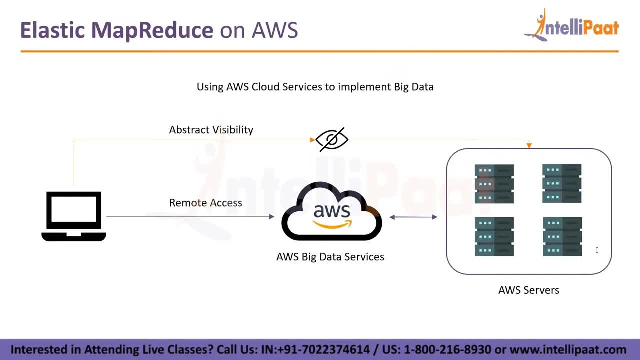 notices any difference. so that is what it means. so that is what commodity hardware essentially means. uh, the second option for that for you, especially when hardware has now gotten a lot of cheap, a lot cheaper: right, you can also have server farms in your office. right, you can have server rooms, which 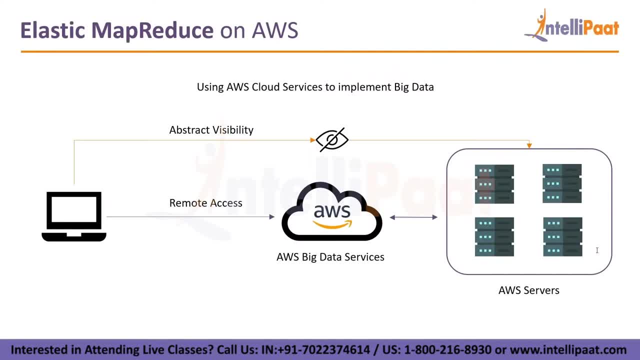 will do the exact same thing. you can install Hadoop on server rooms as well. earlier people used to use a lot of commodity hardware as well, because, uh, I think server farms was a lot expensive. but today hardware is cheap, you can go for server farms as well. so you have two options essentially, depending on how efficiently you want your job, obviously. 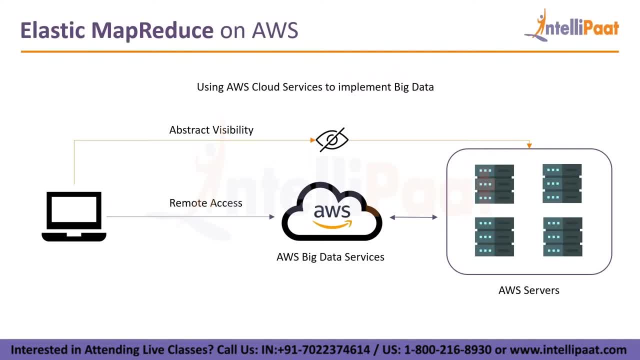 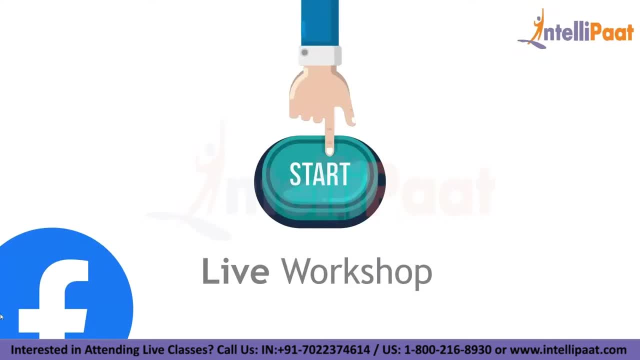 server farms will do it a lot more efficiently. so, uh, let us get to the next part: live workshop. we're going to be analyzing a Facebook pseudo sort of Facebook data set. we're going to be analyzing that with the EMR, so we're just going to run you through the process of that. it's very interesting. 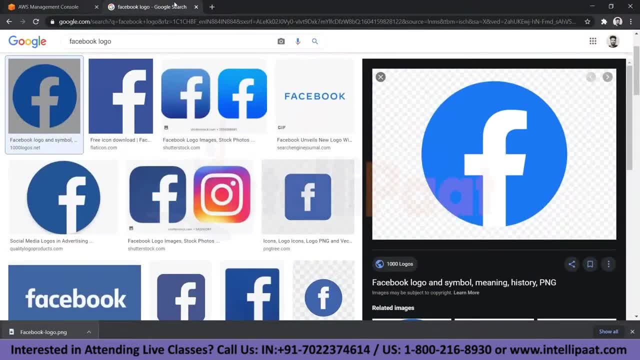 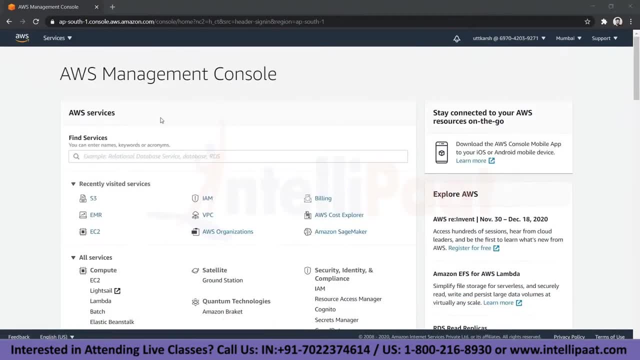 for those of you who are looking at this for the first time, I was looking for a Facebook, don't mind me. so, uh, let me do that. um, yeah, so firstly, uh, this is the AWS management console. so, if you have AWS account, uh, this is how it looks like, right? uh, you have a dashboard and you have 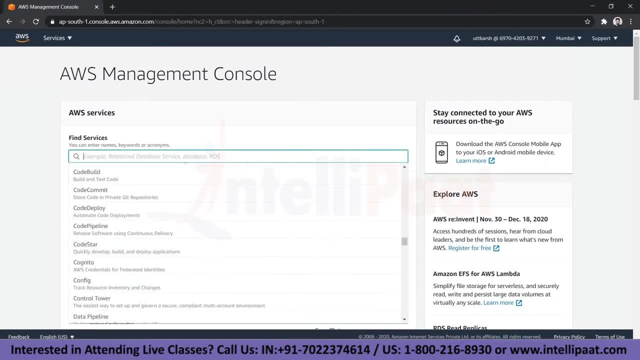 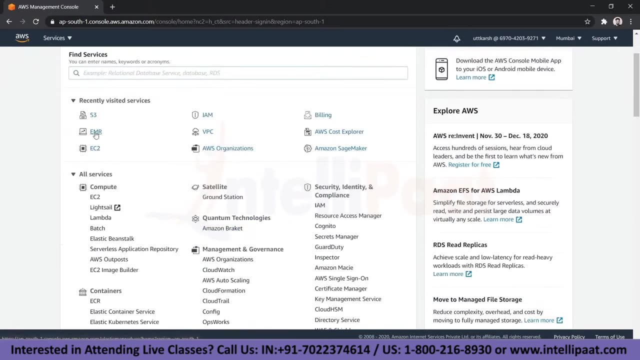 a lot of services available to you, so all of these services accomplish different needs. uh, it depends. if you want to do machine learning, if you want to run a virtual server for your website, you can do that right. what we are concerned with, uh, today, is EMR. so EMR is elastic properties. once you open that, 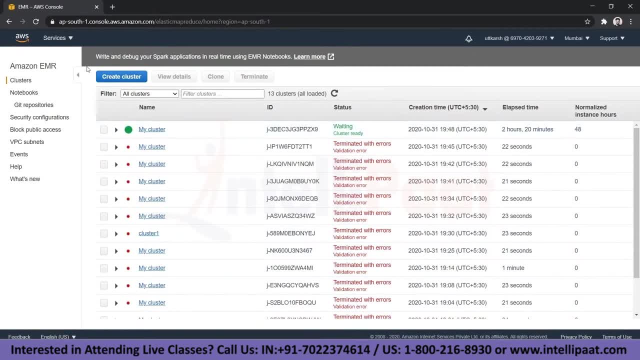 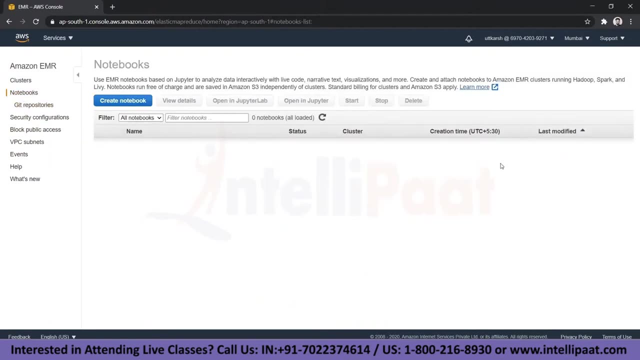 as you can see, I have a lot of clusters that I had opened earlier on as well, so this is how the dashboard for Amazon EMR looks like. so this is used for big data. right, you have a lot of options in this particular case as well. you can create notebooks like these will create Jupiter notebooks. 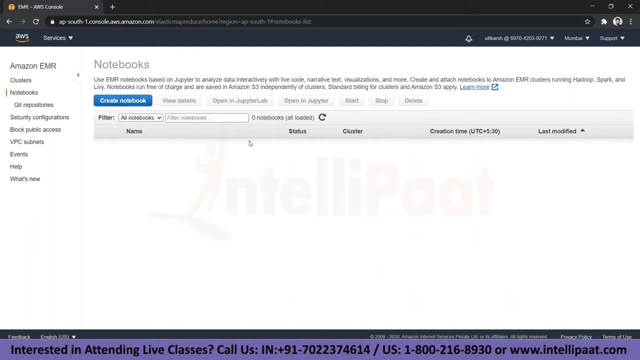 on top of your EMR, right? uh, you can simply go into the UI section. you don't even have to look at a terminal screen. you can simply open up a Jupiter notebook and implement your uh python code or your spark code on that terminal using the big data cluster. right, so you have that option as well. uh, so firstly, I'll go to: 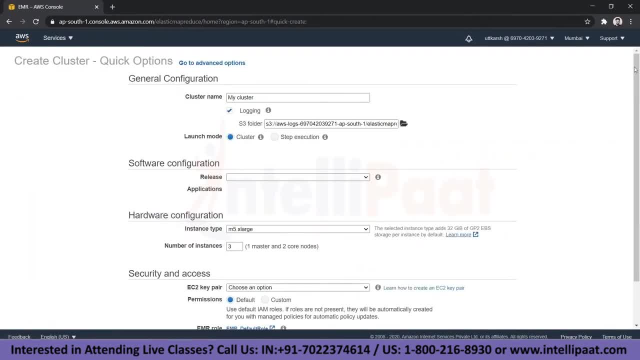 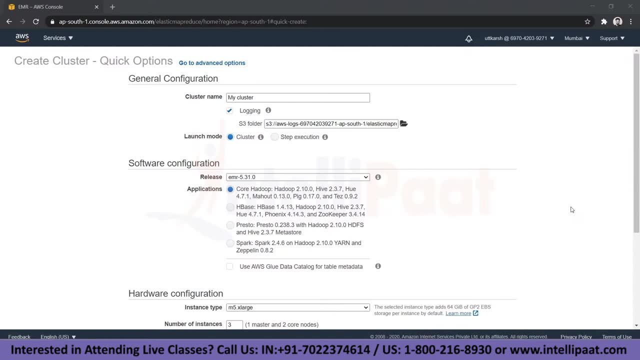 the cluster. I'll click on create cluster, right. so I'll go on. so what is the EMR? it is like map producer. uh, it's called elastic map reduce, but it does not. actually. you don't necessarily have to use map reduce with it, right? so I'll show you what that. 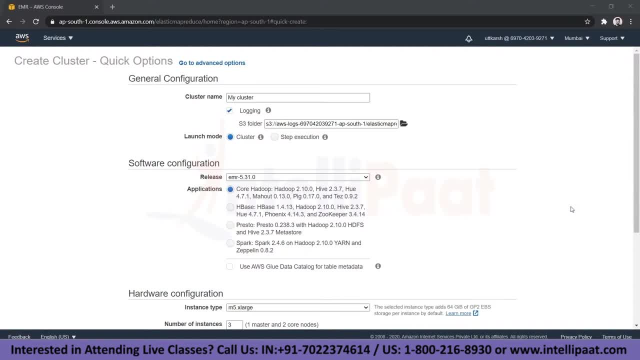 exactly means it's just called elastic map reduce. that doesn't mean we're always, always using map reduce. uh, yes, EMR can use Hadoop and spark at the back end. you can uh. no, you cannot. uh, EMR cluster is not free tier. for those of you who are wondering: with Amazon EMR, creating EMR is not free tier. what? 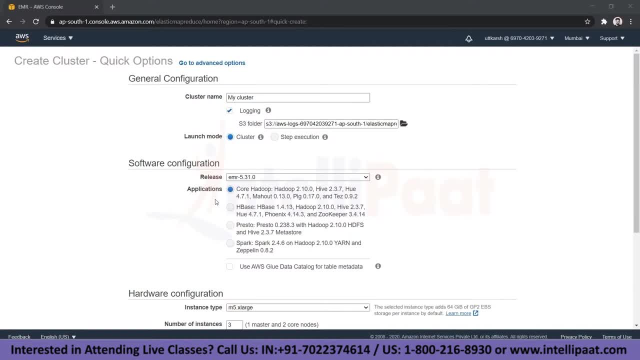 you can do is create ec2 instances, right and uh, then you can attach them together and create your own. you can just install Hadoop on one ec2 instance and then you can go and ec2 is free tier. uh, one of the ec2 machines is free tier. you can go with that, definitely. uh, just I don't think you'll have to pay. 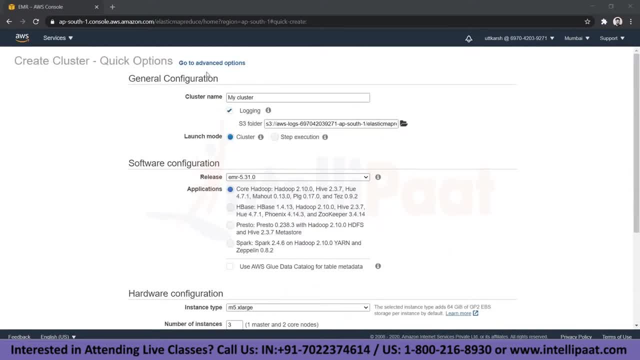 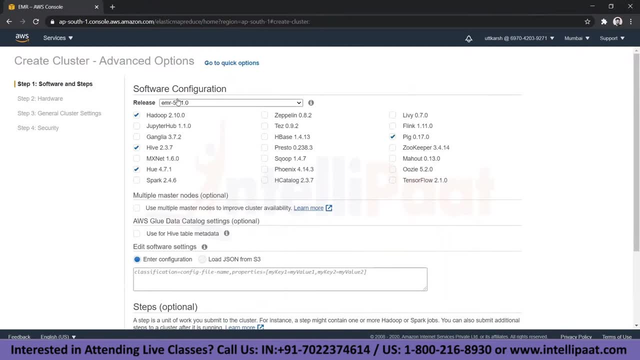 much, uh, if, if you decide the machines, I'll just go through this particular option. so I'll just go to advanced options. right, with advanced options you can select a lot of customizations, right. so firstly, there's the release, the EMR release. so this decides Amazon actually comes up with releases of software. 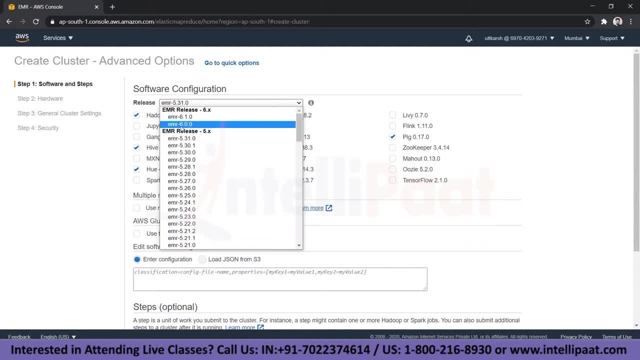 currently there are two unstable releases, which are the 6.1.0 and 6.0.0. uh, the current stable release is this particular version, 5.31. right, so we'll go with that. um, you can then select what softwares you want to install, what frameworks you want to install. very convenient, right? uh, you can. 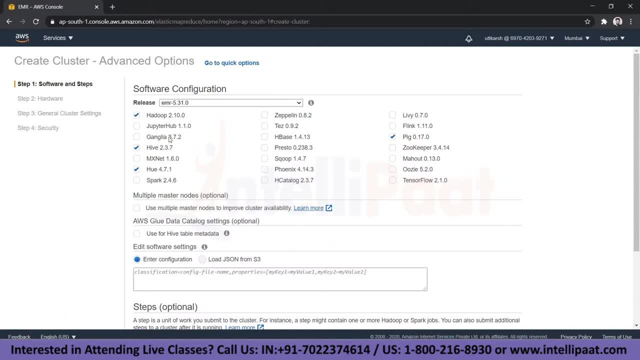 select: uh, Hadoop, obviously we want to install because Hadoop is obviously going to be there. we're going to be using the HDFS for our uh purpose, right? and then we have hive. we don't need hive for uh, we can have you, we don't need you, we need the spark. let us look at other softwares. uh, we don't. 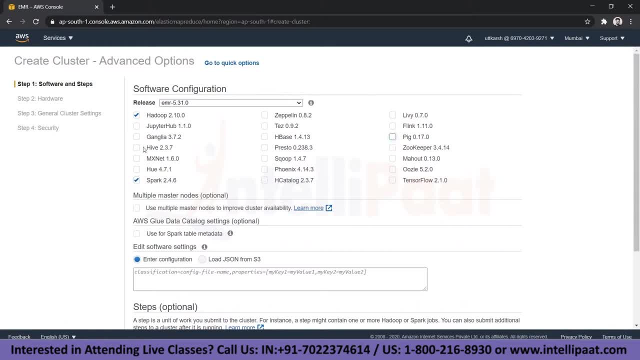 need press to HBS. yeah, so other than that, we don't need anything, right, so we only need for now. I think, uh- and I am no hope I'm not messing this up- yeah, so we don't need anything, particularly other than the softwares we have currently. if we do need, then I'll have to go again and create the cluster again. 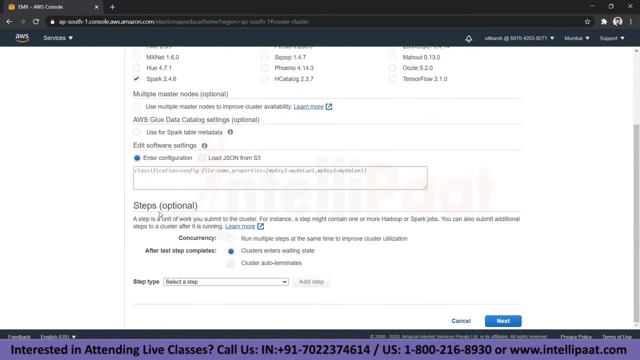 all right. so, um, uh, all of the other configurations are correct, so we don't need multiple master nodes. we can say: we have the option to have multiple master nodes. for our case, we don't need that, uh, because we are only practicing right and, uh, we have steps which are 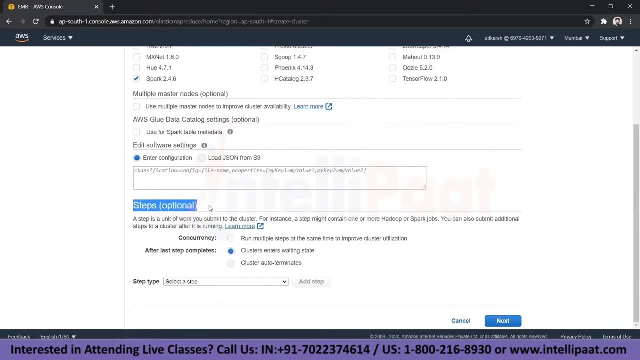 optional. so steps basically means that, uh, if your process has completed, then you can shut down your cluster for the time being, so that you're not priced for anything. so you have that option. we're not going to be doing that. we're going to be going it going slow. we're not going to be adding steps. 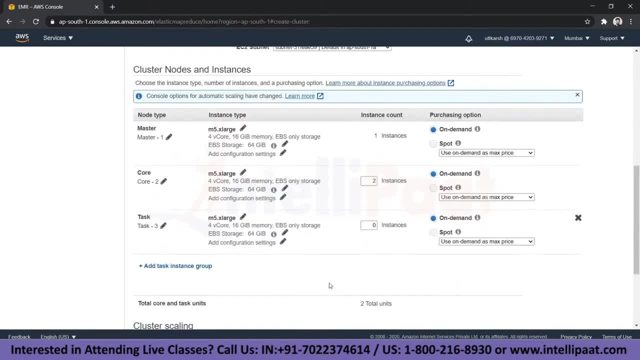 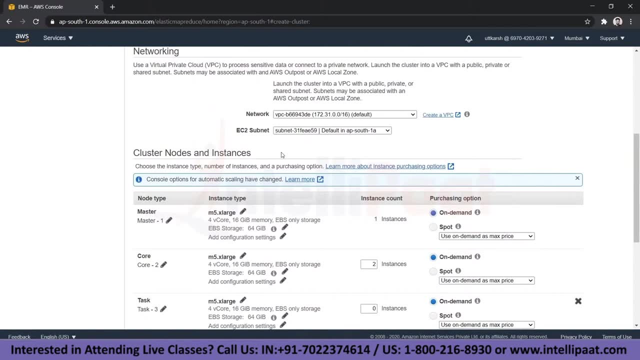 to it, right, so I'll click on next. then, uh, the important part comes up, so we can select our networking settings. so these are related with Amazon security, a very big topic. we don't need to get into that. so here we have clustered nodes and instances, right so? 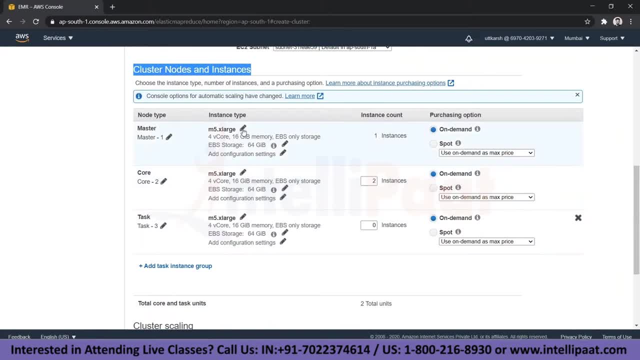 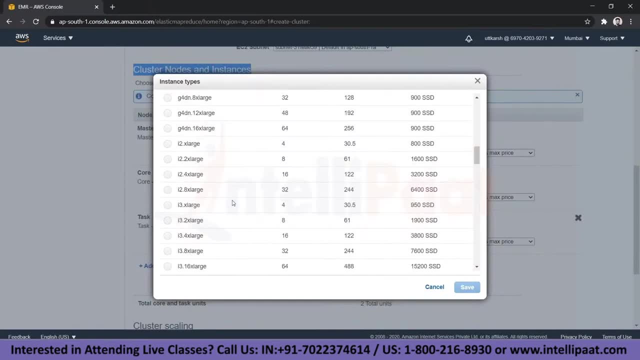 this is where your pricing particular model comes in, right, so in my case, I can select what sort of machine I want to use, right? so, uh, as you can see, it does not have three tier machines, but we can see the size and the RAM, right, the GB, uh, and the course. 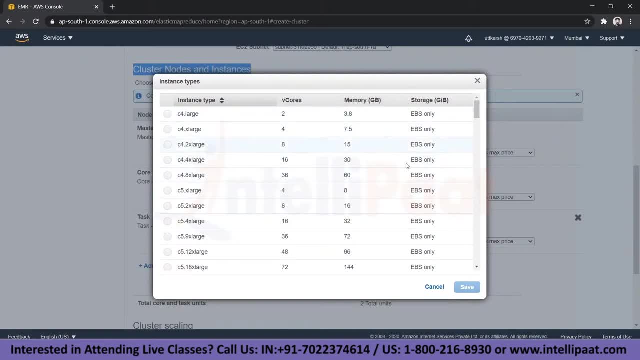 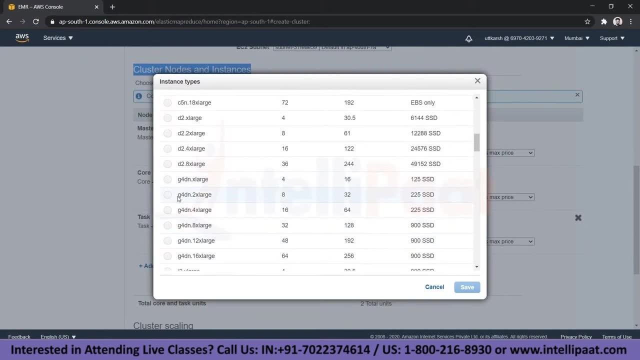 that the processor has for each of these machines, so we can select according to our need what sort of machine. we want the master node to be right, so each of these machines are priced differently. you can look at the prices so you probably wouldn't have to deal with all of this for. 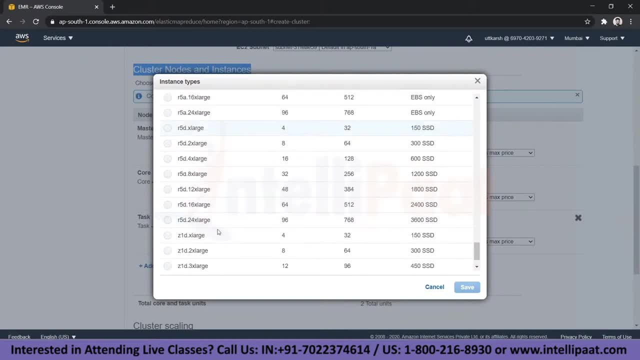 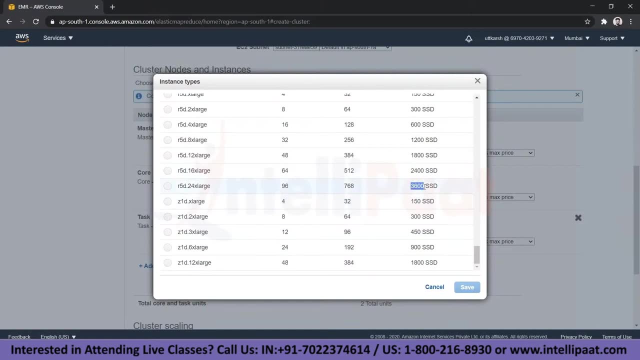 for a training purpose, but the when you're dealing with companies and whatnot. so you'll have to look at pricing and you can see the size of the SSD. so this is a 3.6 terabyte SSD essentially, and you have 768 gigabytes of RAM on one machine. so you can understand how expensive this particular. 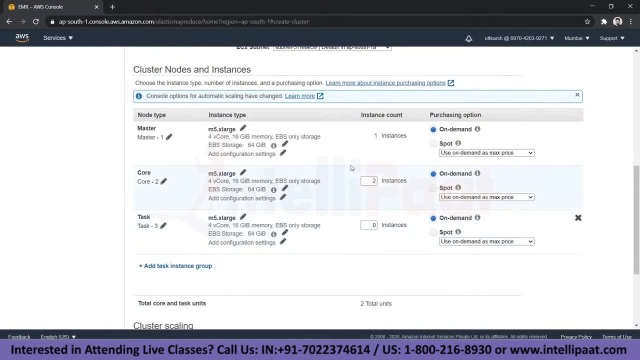 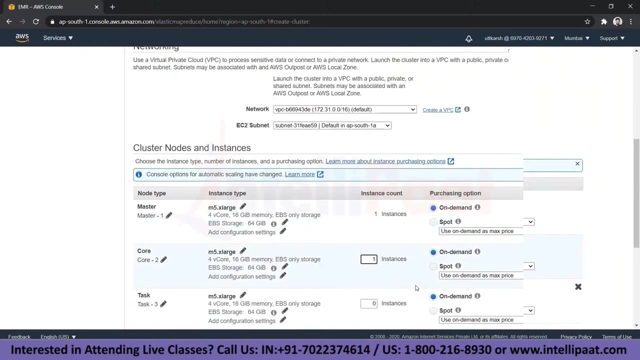 machine would be. so for now, I'm not going to be selecting any custom instances. we're just going to go with the m5x large and uh, we can go with a core node. we don't need two core nodes. core node is what a data node is, essentially. we'll just go with one, right and uh. we can see this configuration. 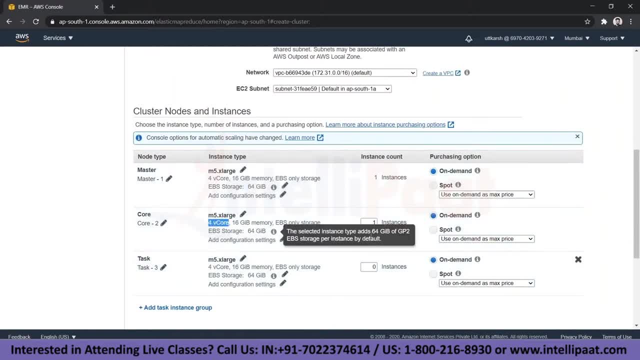 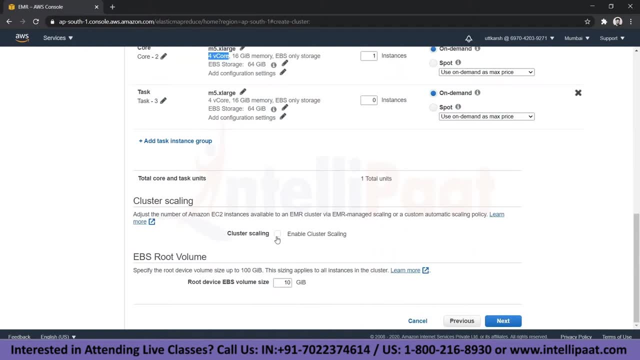 we have a volume of 64 GBs and we have four virtual ports, so we'll go with that. and we also have the option for enable cluster scaling. so this basically means that adjust the number of Amazon ec2 instances available to an EMR cluster. uh, with this custom automatic scaling policy. so that means 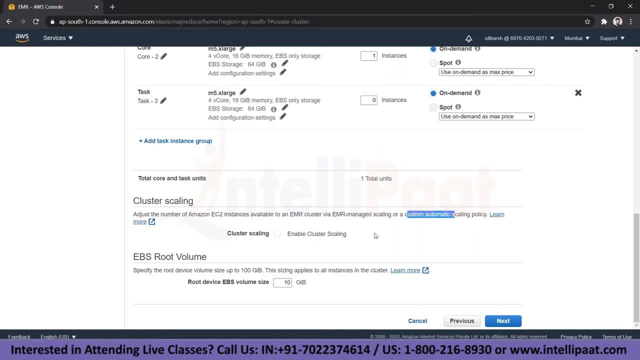 that say, your workload suddenly increases and it's your cluster is not big enough for your workload to be handled in a reasonable amount of time. so in that case, if you have enabled cluster scaling, it will automatically add new instances to your cluster so that your job is done in a reasonable amount of time. when you say MapReduce, is it a? 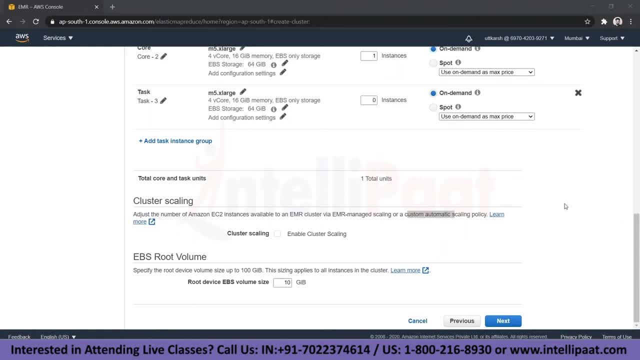 synonym for Hadoop? no, it is not a synonym for Hadoop. MapReduce is a processing framework attached to Hadoop. Hadoop has two elements: HDFS and MapReduce. what else AWS services do we need apart from EMR? uh, you can use a lot. you could use Amazon kinesis. you can use data warehousing tools like uh, you have. 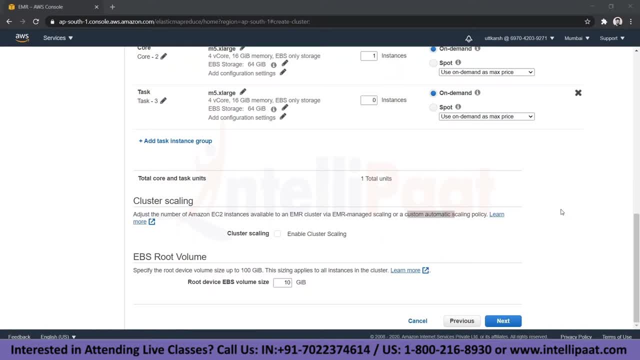 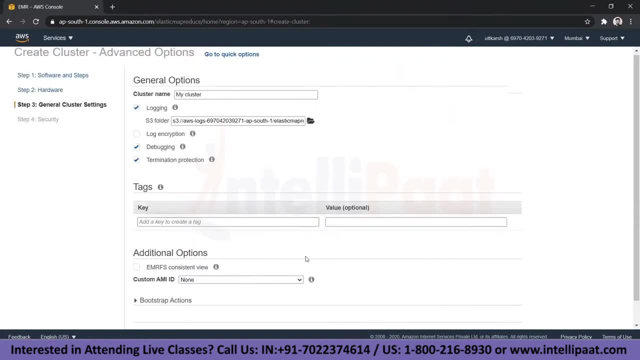 other tools available to you. redshift all of these things. you can use that data visualization, a quick site. all of this is basically covered in an extensive big data course that we actually provided. all right, I'll call the cluster my cluster. no issues with that. next, uh, no security. 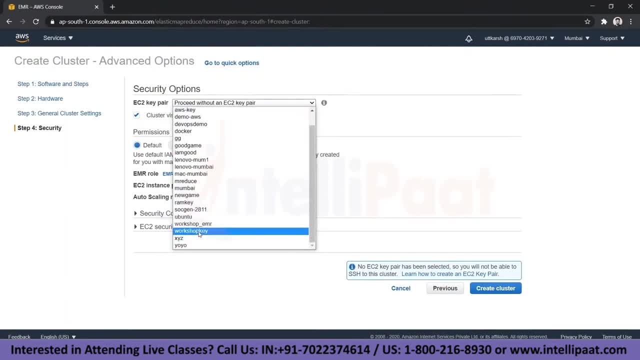 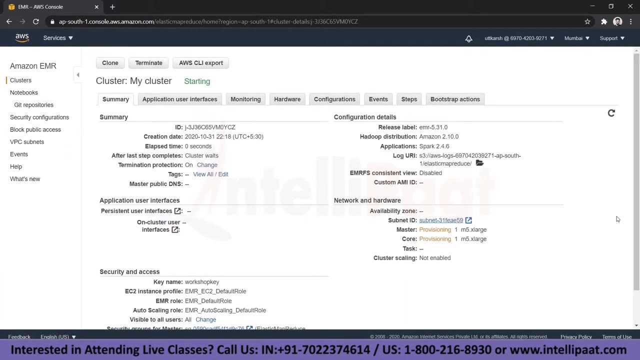 settings. particularly, I have to give a workshop key as my SSH key pairs, because I want to connect my terminal, my masternode. so there's a key that I have created already for that and I'll create the cluster. so this takes some time. I mean, while I'll answer any doubts, also meanwhile what I can. 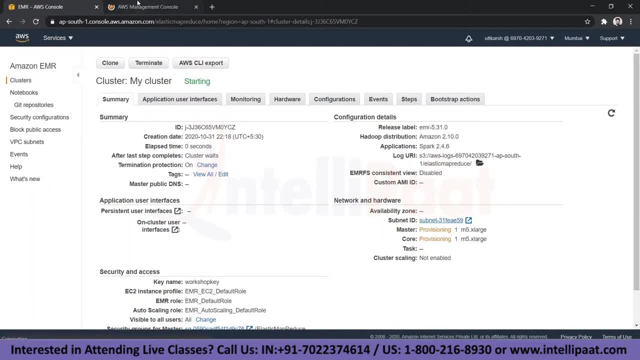 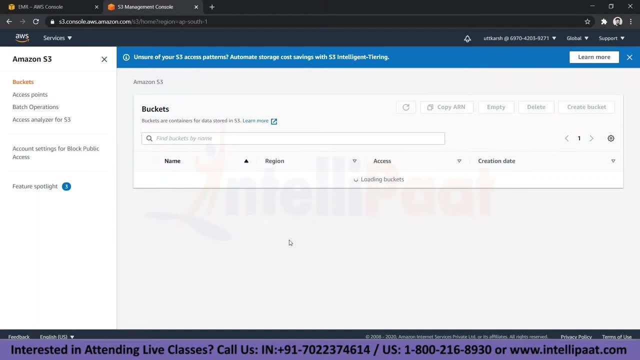 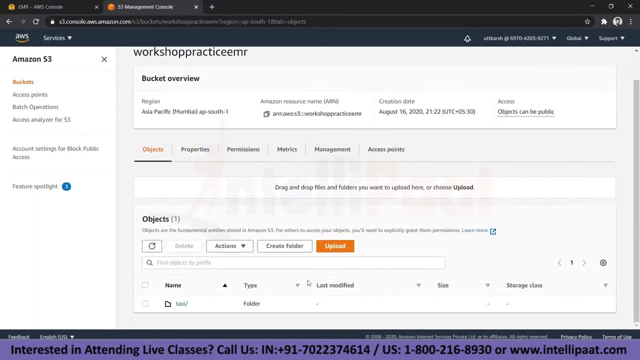 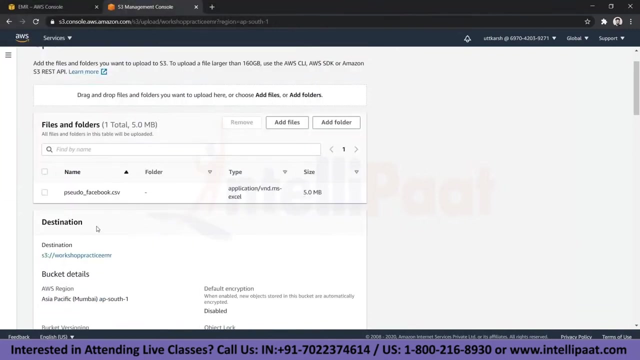 do is actually put our data set on the S3, so we want to actually access our data set. uh, when we run our spark job, we want to put it somewhere, so I'll put it on workshop practice, right? so I already said, I put another click on add file and I'll click on this. so this is the pseudo Facebook CSV. so 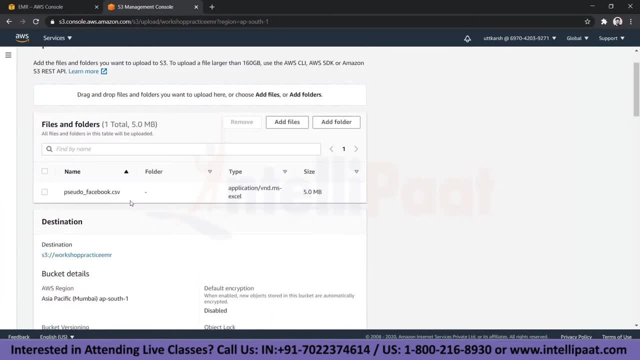 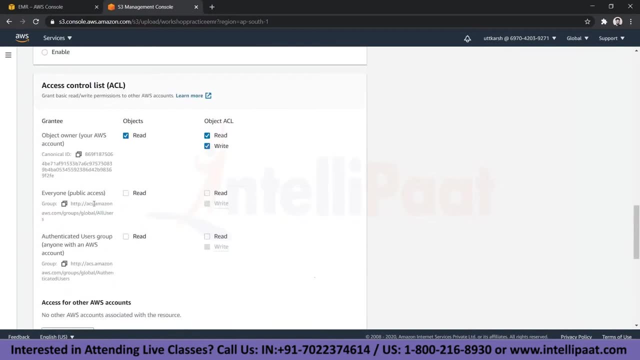 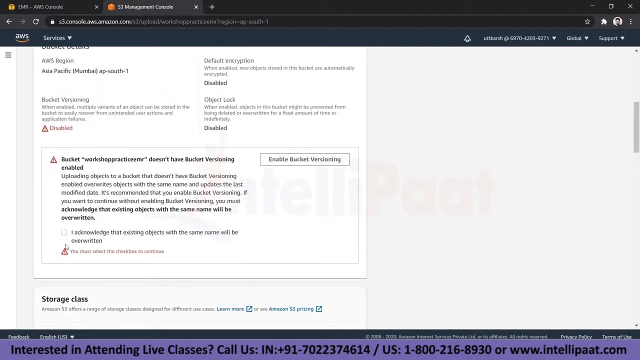 once that is being loaded. I think that has been loaded. uh, yeah, so I'll click on upload. so is there any specific? so I I'll allow public the read access, right, because I want this to be accessed by my cluster actually- and then I'll click on upload. what is the issue? okay, so I'll then click on. 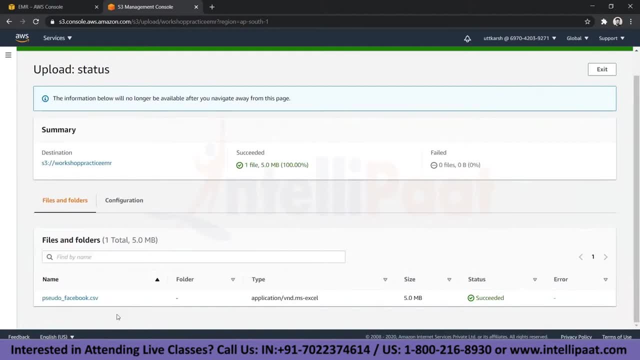 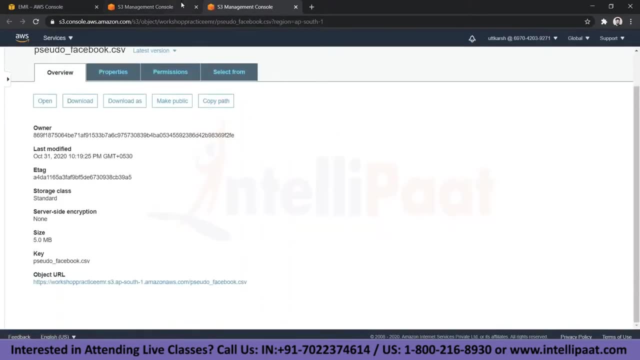 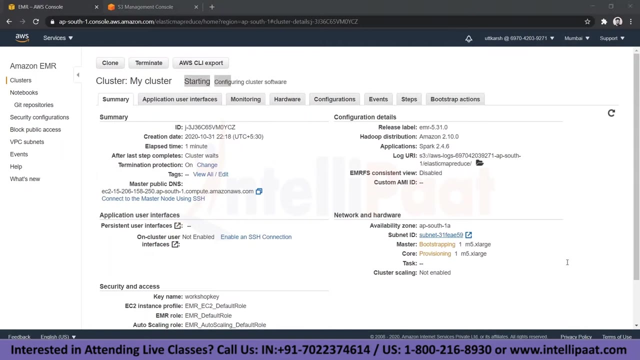 offcode. so the file has been uploaded. uh, yeah, so I'll just keep this address over here. I'll click on the file and I'll keep this particular area, uh, assigned on this tab. right, I'll close this tab and I'll go back over here. it's still on starting. uh, PySpark is uh. why is PySpark recommended it? 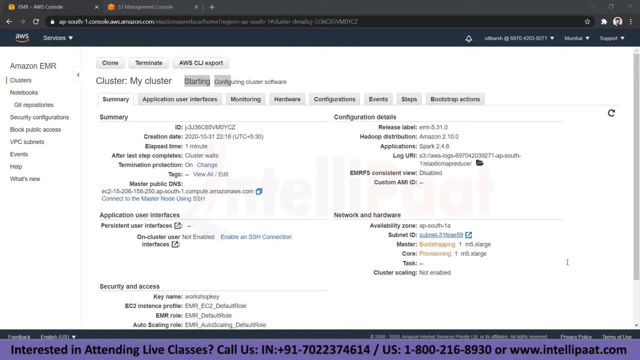 is recommended because of the machine learning libraries. yes, uh, because Python has a very easy integration with data science, plotting, machine learning and artificial intelligence Technologies. how is data loaded on DMR? we'll get into that when we actually do our hands-on section. it takes some time for the cluster to actually start because, uh, the Hadoop. 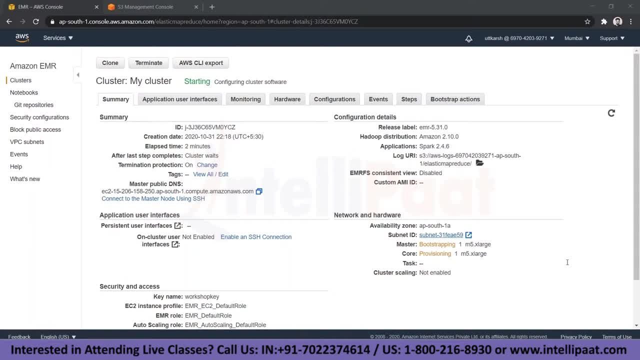 installation is actually happening on both of these clusters as we speak. it's. it's actually slow because you're actually connecting all of the nodes together. it takes a lot of core core coordination but, uh, it generally does not take a lot of time. it's relatively easy for it to relatively 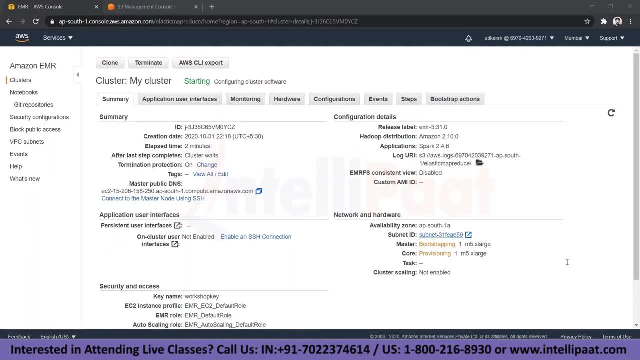 fast compared to the other option that you have, which is actually installing it in house. uh, this particular uh, when we are dealing with a slow uh sort of when we're dealing with a low number of instances, it will take around uh, five to six minutes, uh, five minutes at maximum, uh, but when 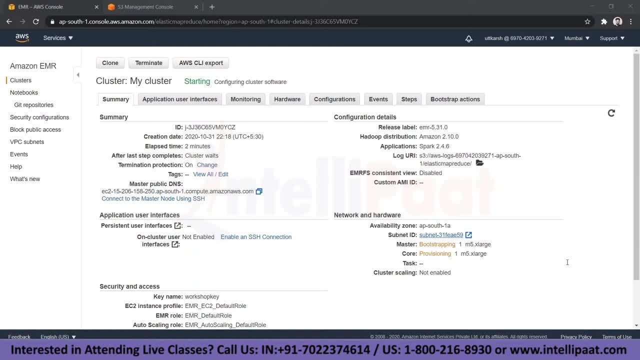 we're dealing with larger uh workloads, then it can take a larger amount of time. it depends on how many instances are there. so what is EBS and SSD? so the difference between EBS and SSD is that SSD is obviously uh, your solid state drive, and EBS is your normal hard drive volume. so 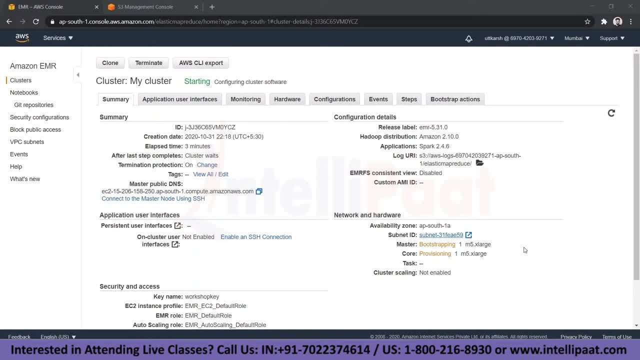 it's the difference between the speeds of a hard drive that you have on your computer and a SSD, which is extremely fast writing and reading. all of this is to essentially decrease the latency, nothing else you are. if you're using SSD, definitely it's faster, can you SSH? 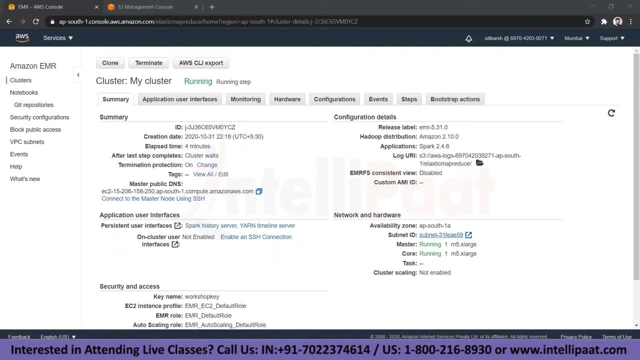 into the master and not the name nodes. uh, the master is the name node, so there are two names for it. you can go with uh, master and uh, your core node, which is the first case you can go with that. the code node is the data node and the master node is the name node. so now the cluster is in running. 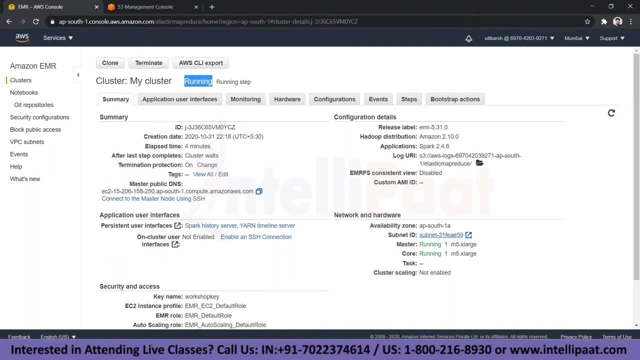 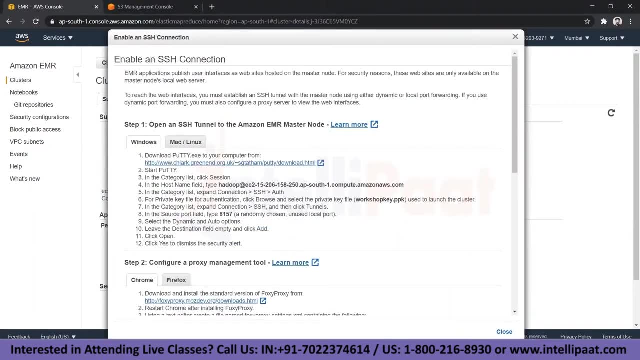 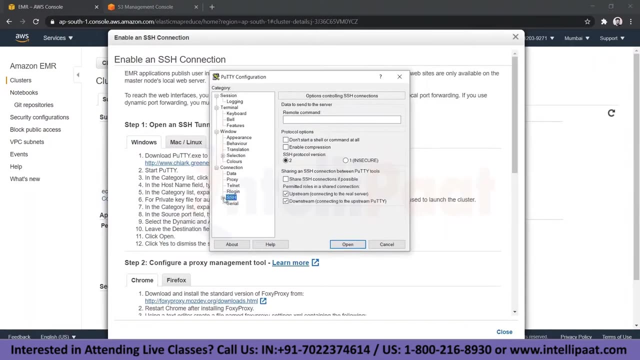 right. so, uh, then now the cluster that is in running. you can simply open up our SSH tool, which is party go and enable an SSH connection. we'll copy the address of the master node, put it over here, right, and then we'll go into SSH. we obviously need our 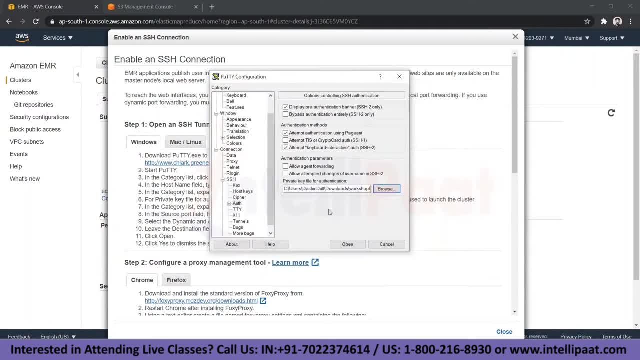 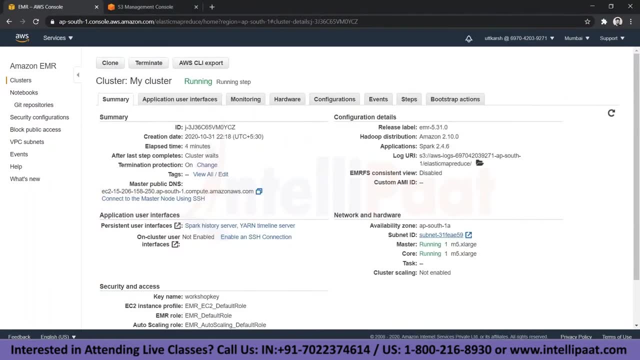 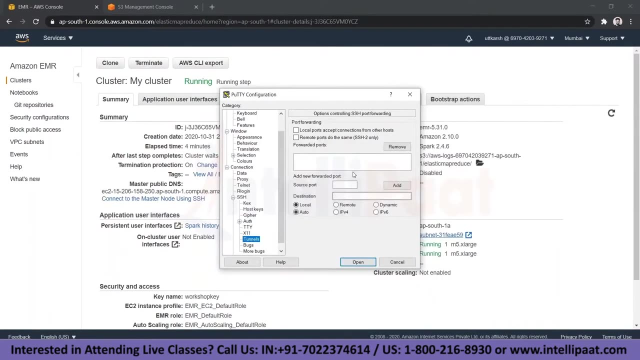 key right, so we'll go and search for the key, which is the workshop key. I think that is the one that I used just a moment. I'll check. is that the one that I use? yeah, it's workshop key. okay, paste it over here. go over here and select workshop key, go with that, go to tunnels and then I think there's a port. 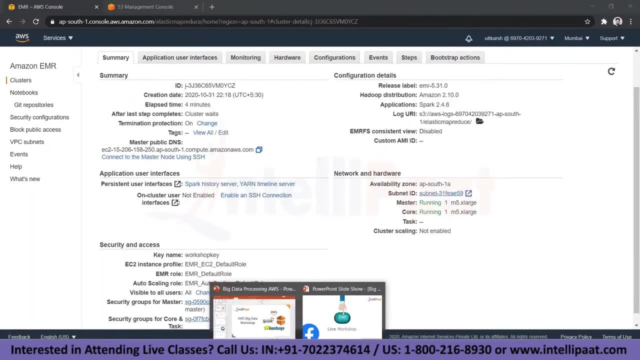 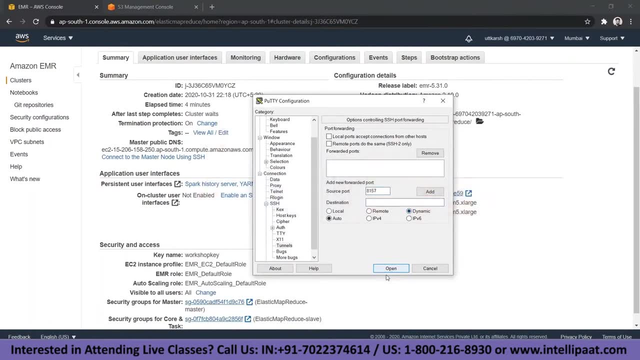 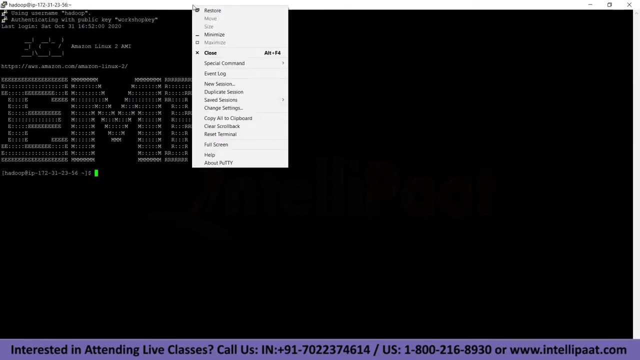 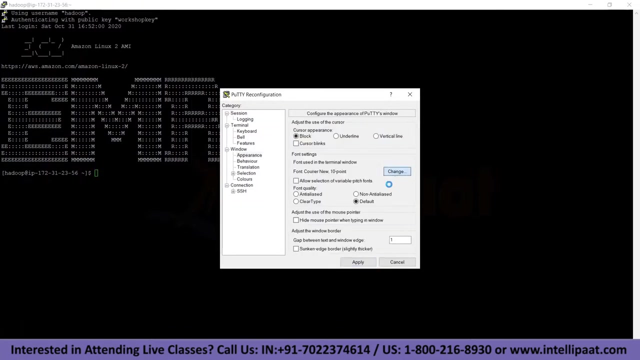 so the port is 8157. we go with that 8157. put that in the source port area, put this to dynamic because it can change and we click on open. so we have successfully remotely gotten into our master node, right. so I'll simply go to the change settings and actually increase the font size for 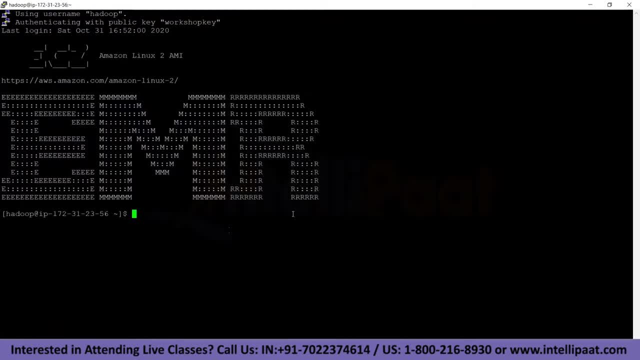 a little bit right, so I'll click on apply so you guys can see better that way for those of you who have a lower resolution. all right, so the first thing that I would do is obviously start the spark shell, so the shell by default starts in Scala. 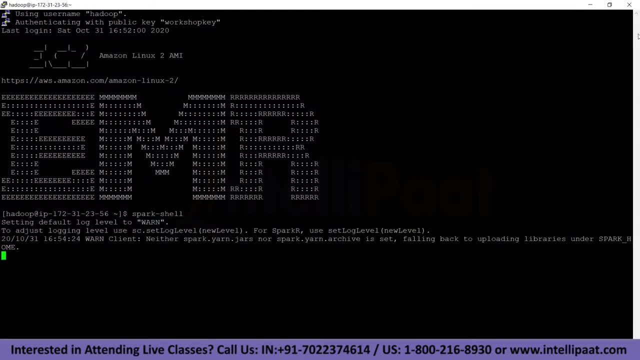 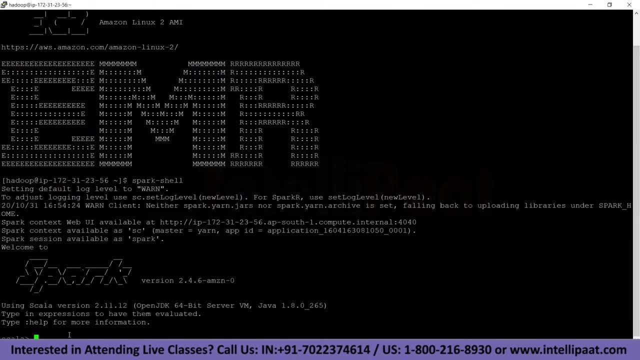 it takes some time for the shell to actually start, and but it when it starts it it's really faster, yeah, so, uh, definitely, the first thing that I would do is actually create a variable that contains the data set that we have uploaded right? so the first thing that I would do- and this could be as big of a data set that you want, right? so the 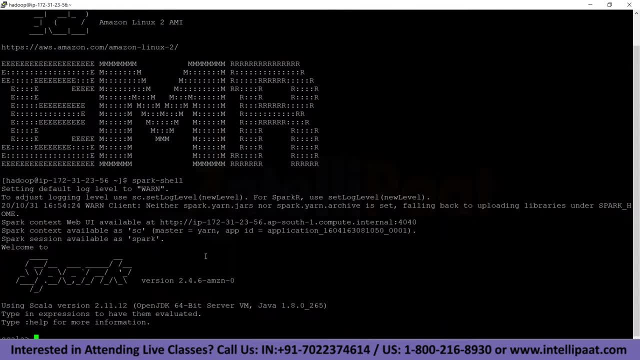 s3 currently has a lower size data set. it could be in terabytes, it could be in petabytes, it does not matter wherever you're taking your data from. you can simply put in the location and spark will do it in a fast amount of time, but depending on the cluster size that you have. so, uh, let us go with. 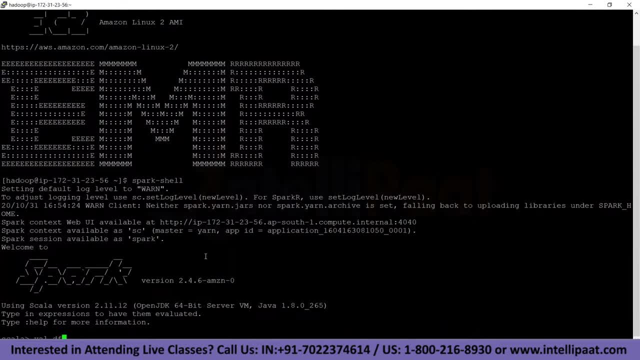 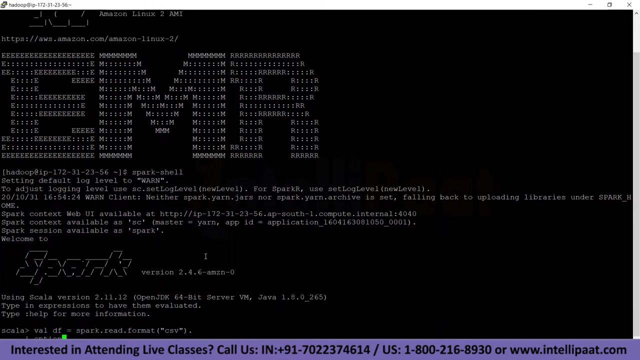 a variable creation where we are going to create our data frame. data frame is something similar to it, right? so spark dot. read dot format and the format is a csv because, uh, the file that I had uploaded was a csv file, right, put in a dot over here. go to the next line option. I want the headers. 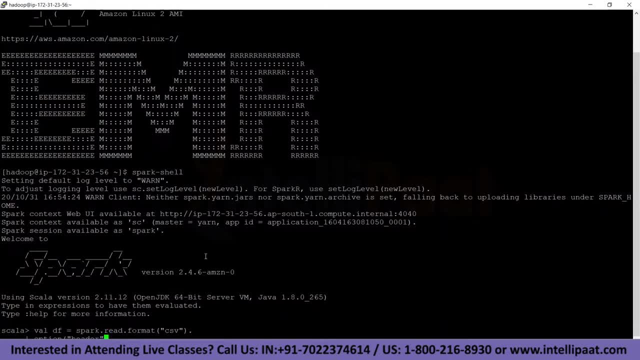 to be included in the column names. uh, the files do have headers. we'll look at how the file looks in a moment, and I want the header to be true because I want the headers uh option and for schema, I want it to be treated like an SQL table, so I'll put this to true as well. 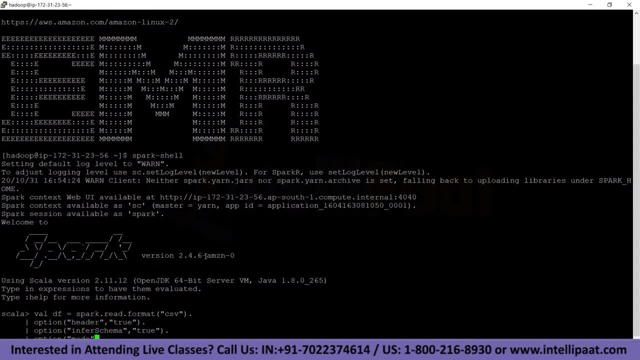 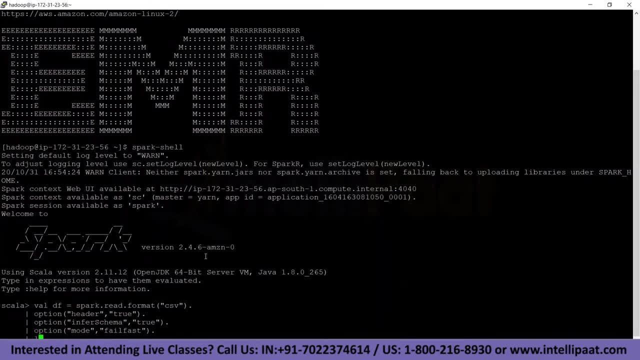 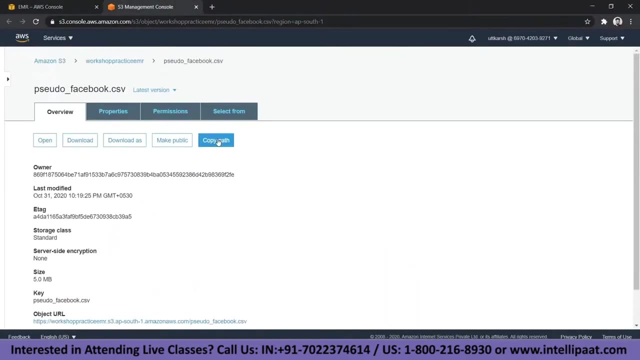 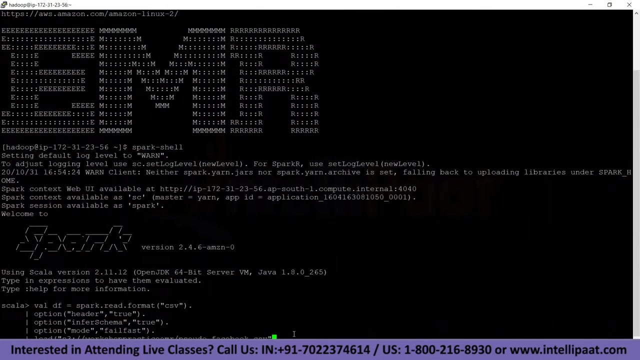 option and finally fail fast for memory management purposes. and then we want to actually specify the address of the file. so load and we'll put in the location. so I'll simply go over here and copy the location to copy paths of the file. go back, paste it over here, put in a double quote and that will create our data frame. 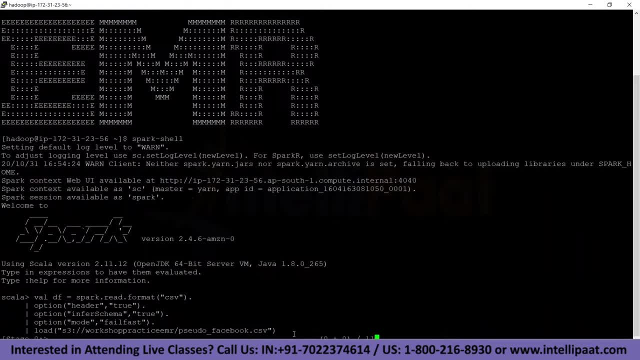 so it will take some time. it connects to the s3 bucket and then it imports the file. but once it has imported it will not take time, because then obviously we have it in the RAM. so, uh, it took some time, but, uh, we have the data set now. so 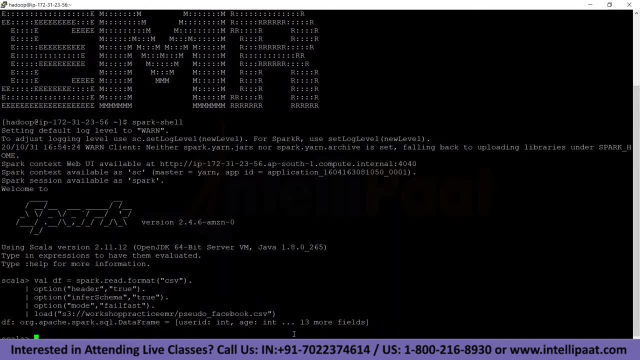 uh, what I will do now is for convenience purposes. we're going to be using spark SQL, so you're going to create a table name for this data frame. we're not going to refer it, to refer to it as DEO, we're going to call it something like FB. let's call it Facebook for the. 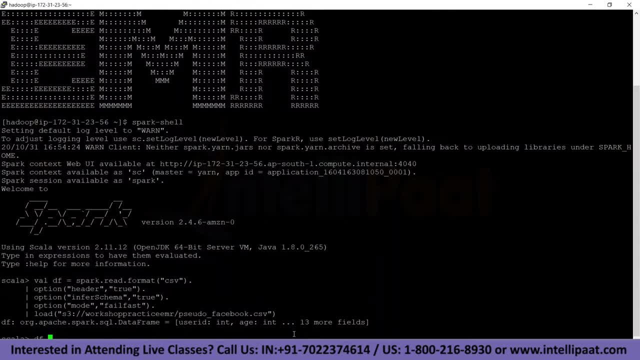 initials. let's call it FB. so, uh, create a temporary view. create or replace temp view. so this is going to be temporarily the name of the SQL table. let's call this FB, right? And we do that. put in a double quote over there and press Enter. 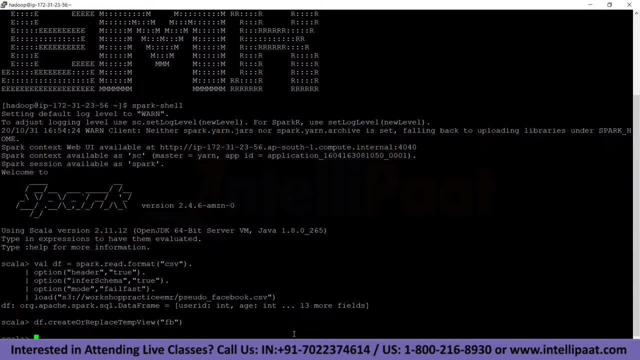 So we have changed the table name to FB. for Spark SQL access It's still DF, but when we're referring to Spark SQL context it's called FB. So we'll type in sparksql and let's look at the data set. 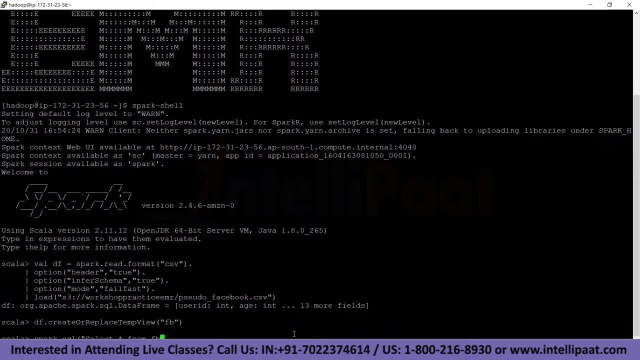 Select start from FB, which is an SQL statement. So if you're coming from an SQL background, you can understand how simple that makes it for you, right? So you simply have to implement. up until here, you have to implement the Scala code or the Python code. 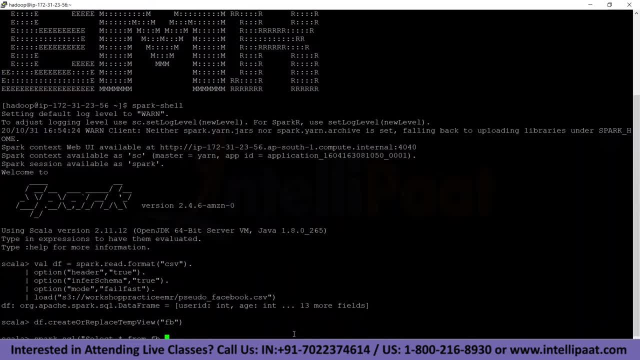 and then you can simply go ahead with your SQL knowledge. That is how easy it is. Now you're simply implementing it for big data, right? You're not implementing it for small data on, like on your MySQL. You're implementing it for big data sets. 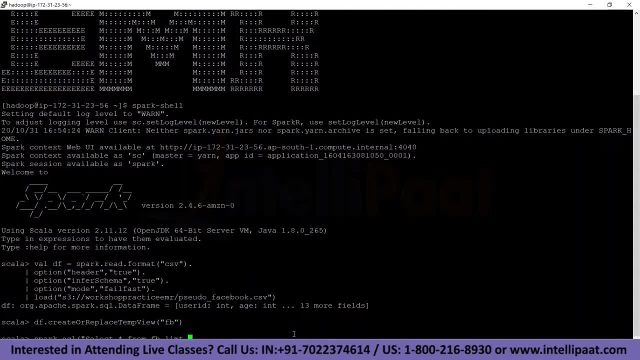 So from FB, and then limit this to like three, because I don't want my entire screen covered with the data, right? So then I'll simply type in show. Now, show is important. If you don't type show, it will not actually give you the output. 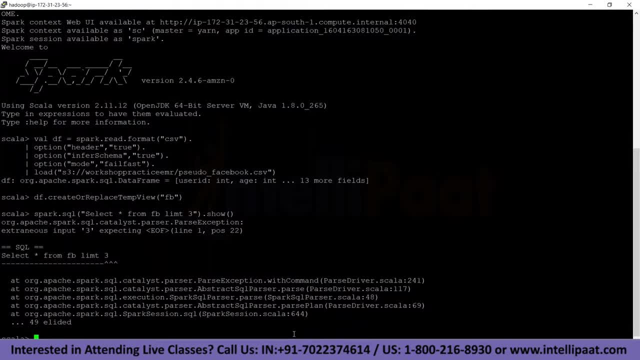 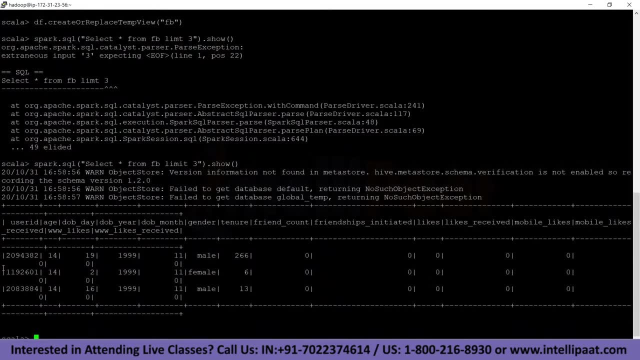 So some error. Okay, I did not spell limit correctly. Just a moment, Yeah. so this is how the table actually looks like, right? So it's a little bit jumbled up, So we'll just look at. there's a user ID. 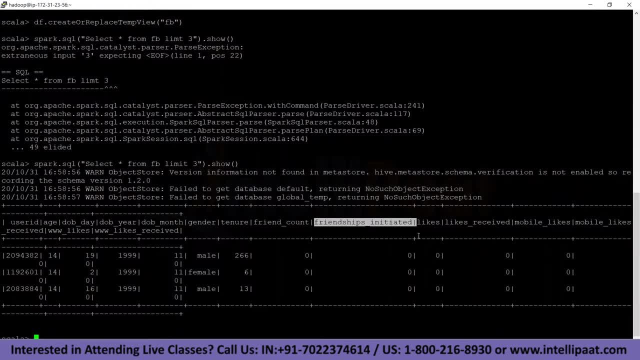 for your Facebook ID account number. primary key You have an age for each of the Facebook users. the friend count of that person. the friendships that the person has actually sent requests for the person's likes. the likes that person has received. 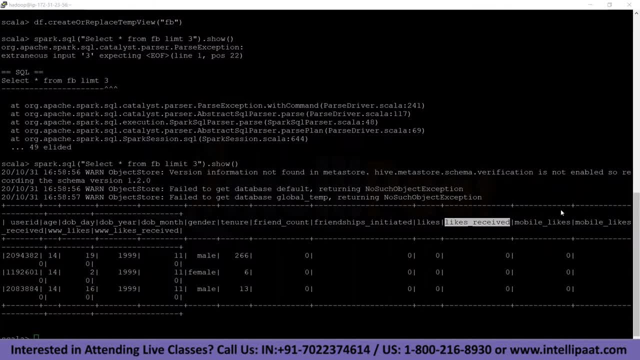 mobile and web browser likes, right. So this is the data set that we have. All right, so let's open that back again and we'll begin with our process. So say, I want to find out the number of rows, the number of records that we have in this particular data. 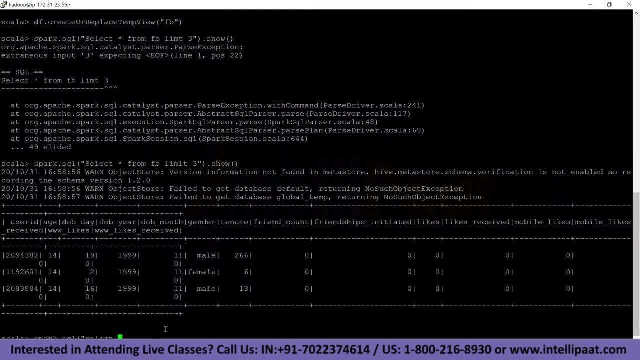 set. So I'll type in SparkSQL, I'll type in select count and then put in an asterisk over there. So this is simple SQL from now. There's no difference between this and SQL. So from FB and putting our double quotes over there. 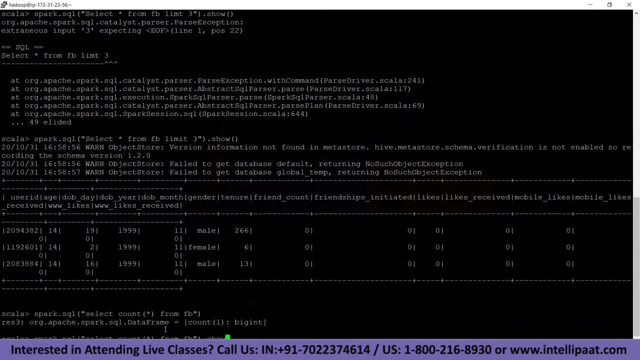 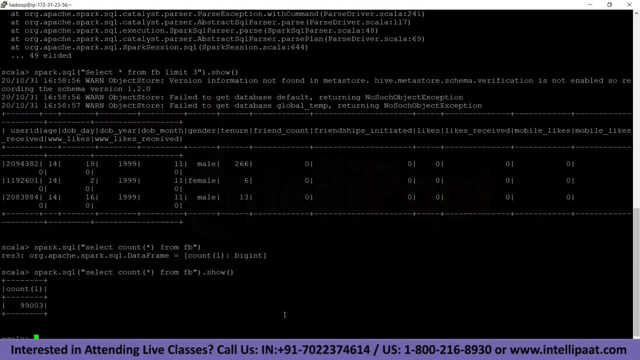 and press Enter. So I didn't actually type in show. I typed in show, then press Enter. It will evaluate the number of records that are there in the data set and then it will give me 99,003.. That's the number of records that are present. 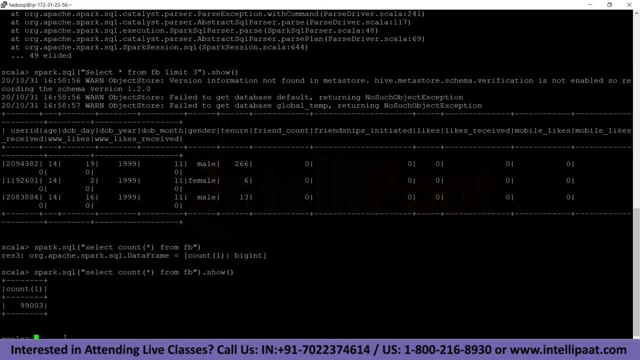 in this particular data set. Obviously, when you're dealing with really, really big data sets, right Like in the terabytes, petabytes- you will get a lot of records, But the advantage that you'll have in that- it took me some time to actually evaluate this thing, right- 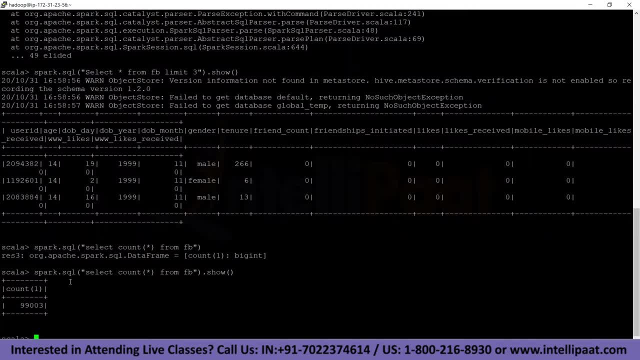 And that was because we actually have a two-node setup over here And we're analyzing a really small data set- right. But if you're dealing with a really big data set, what will happen is it will still take the same amount of time. 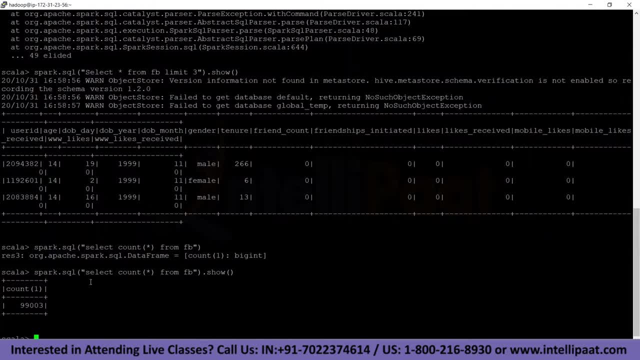 as we just took right, But it will give us the output. So not necessarily for this, because when we're dealing with a small data set, using Spark or any other big data framework is not a good idea to use, right When we're dealing with a big data set. 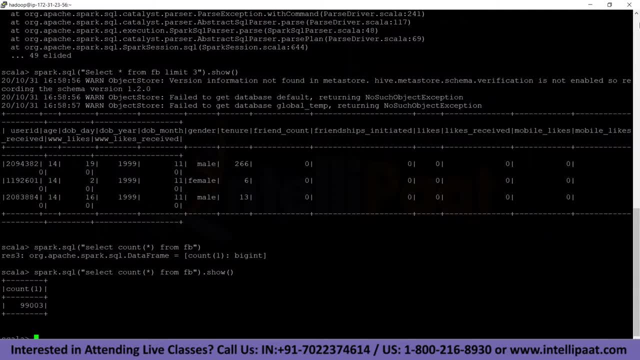 it should still take the same time. So that is the difference there, basically right, OK. so the next thing that we can do is something interesting. We can calculate the average age of a person on Facebook. So sparksql put in and select average. it's called AVG. 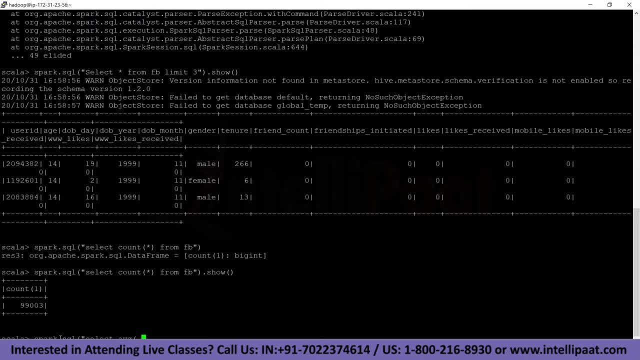 All right, So that's it, Select AVG, and we're going to put in the column name age over there. I think. just a moment. So we're going to put an age over there from FB. I think it should be in double quotes. just a moment. 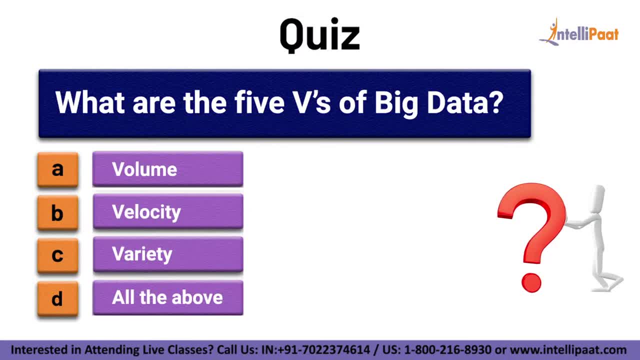 And let's see Just a quick info. guys, Test your knowledge of big data by answering this question. What are the five Vs of big data? A, volume B, velocity C, variety D, all of the above. 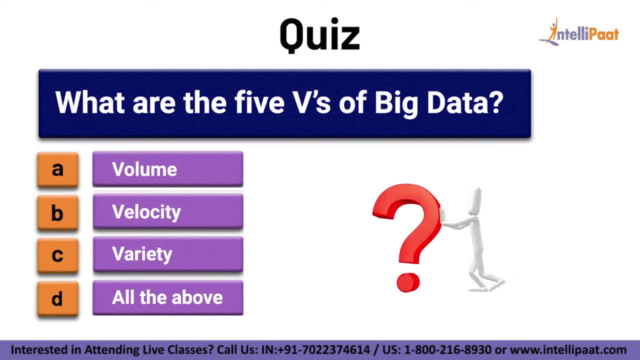 Comment your answer in the comment section below. Subscribe to Intellipaat to know the right answer. Now let's continue with the session. So we'll evaluate that. So the average age of an individual on Facebook is about 37,, depending on the data set. 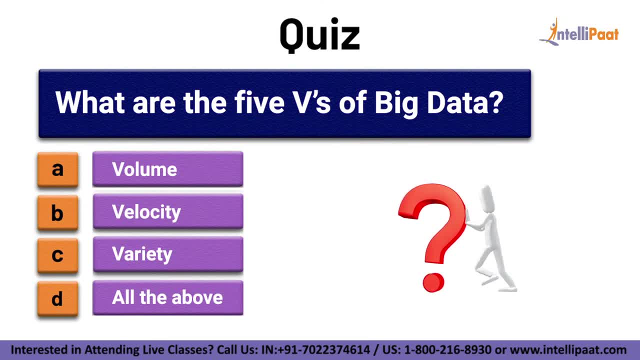 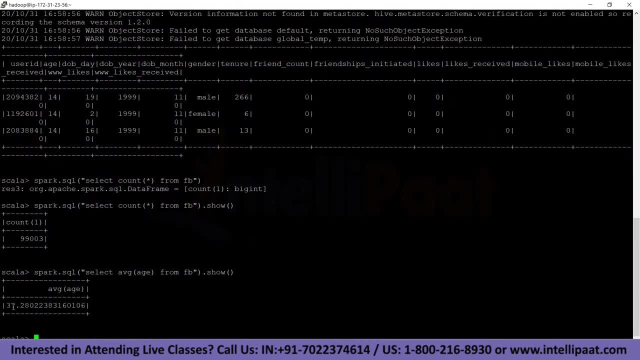 So these are sort of the questions that you will actually be asked. All right, So the average age of an individual on Facebook is about 37, depending on the data set. So these are sort of the questions that you will actually be asked. 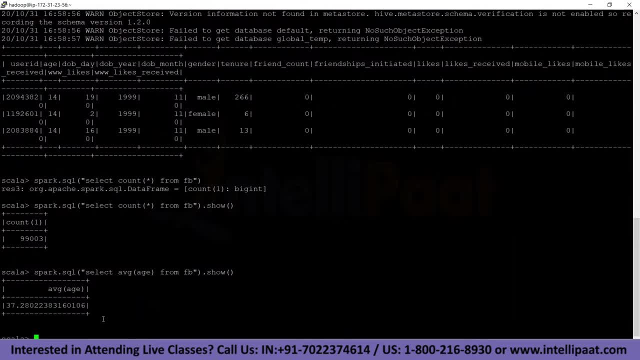 All right, So we're going to put in the column name. So we're going to put in the column name So you'll be given the basic level of questions that you will be asked of when you're actually working in the big data domain. 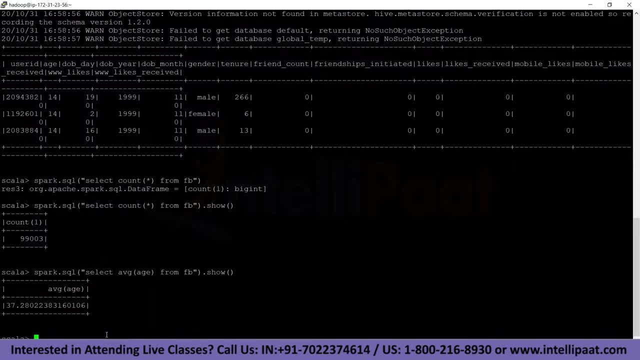 So you'll be given a handful of tasks as to what you have to evaluate and visualize and whatnot. So you'll have these data sets available to you And you'll have to calculate these things and convey this information to the marketing team that you have, the sales team that you have. 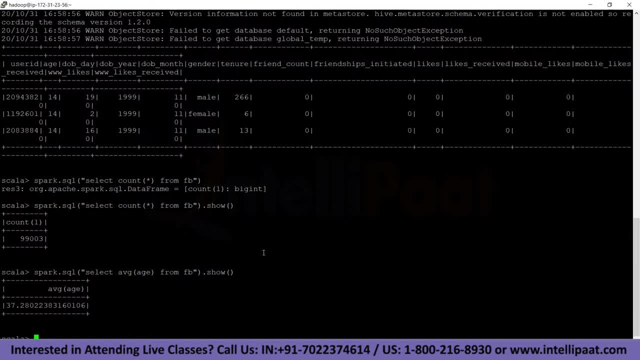 So they can initiate their plans as to how they want to proceed with their business dealings, right? So that is there. Okay, So let's do something interesting. Let us find the average age of an individual, the average age of a male and then average of a female, and order it by that. sparksql select. 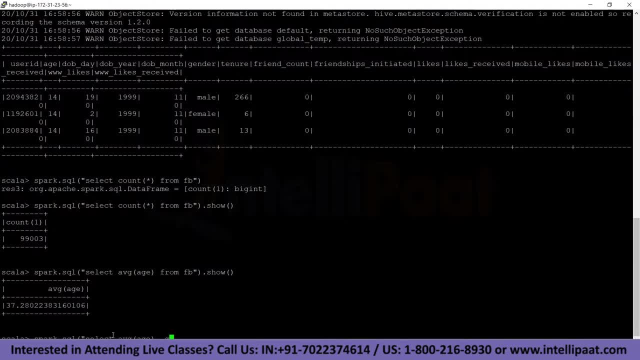 average age and then use the column name of gender as well, because we're going to be ordering it by that from FB and order thing is called order, but group by actually, group by group by gender, and put it over there and if I don't show, so that will be your. it will show me the average age of a. 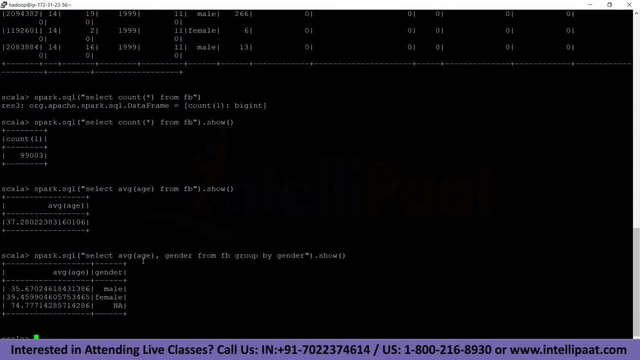 male and an average age of a female on Facebook. So we actually three genders, so the one that's not disclosed right and female and males. female: we have 39 for male, we have 35 for not disclosed. we have 74 right. so this tells a lot about not disclosed as well, because we may have some people. 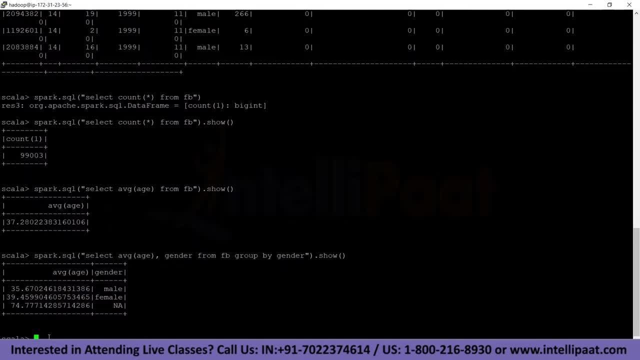 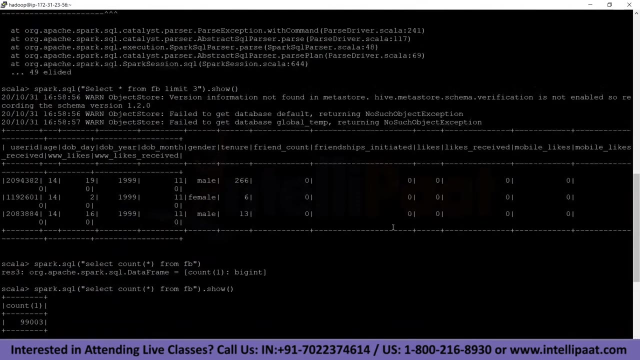 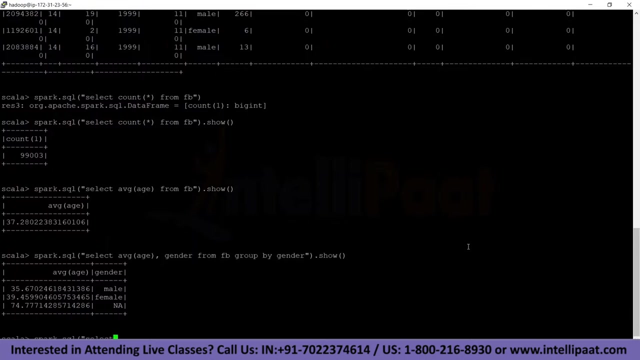 who have actually entered, not disclosed for personal reason, Or we have people who are simply not aware of how that particular aspect works. so let us try something else as well. sparksql, now we can do some. we do anything. essentially, we can analyze anything, particularly for this data set. we can find out something like select average friend. 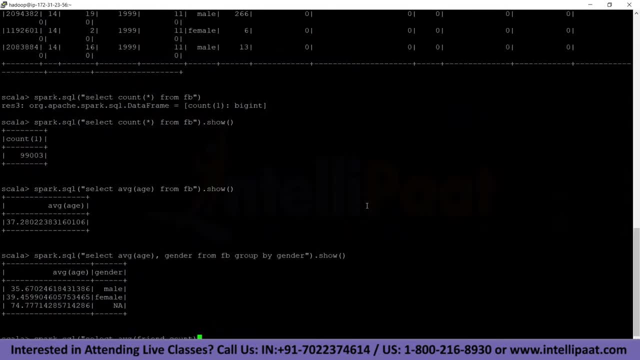 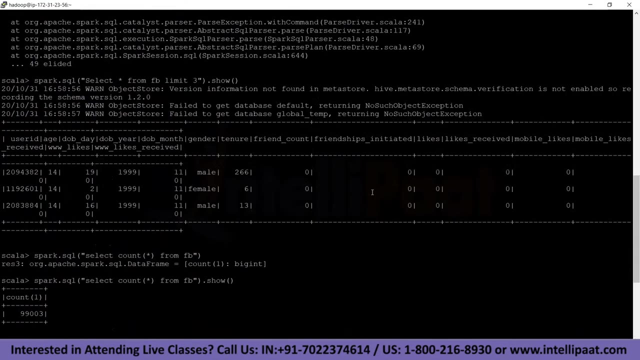 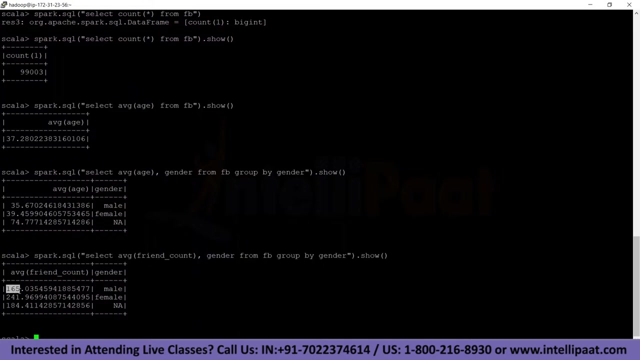 count of genders And then we can simply put in from FB and appropriate by gender. Put in that and we'll get that answer. so meanwhile that is happening. let's look at what we can do next. So we can see that a female has, at an average, higher number of friends than the male, which is 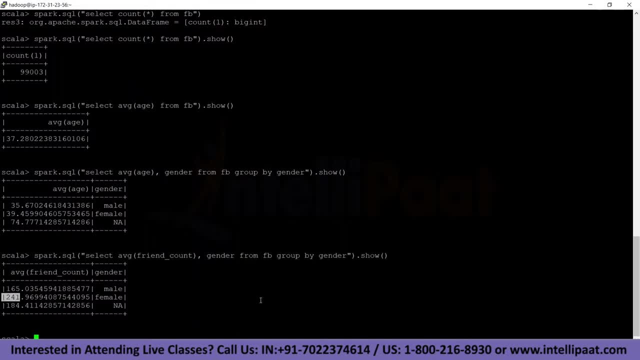 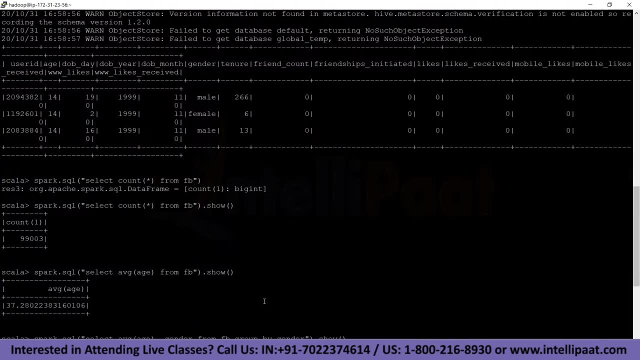 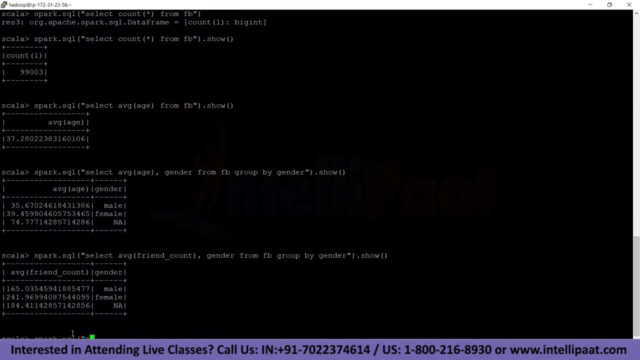 165 compared to 41. so we have that with us, that information with us, whatever we want to do with it. and let us now understand the, the average friends on the age-based demographic right. so let's go with spark dot sql, select average age and average number of likes maybe. so these has this is. 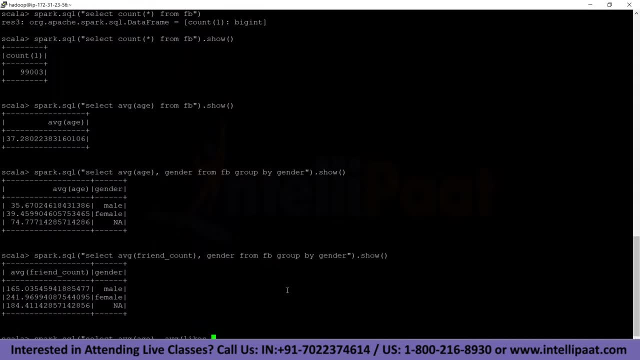 the amount of likes that person likes to receive this code. likes received: Uh, received here. so we'll go with that and go with there from FB and we can go if we click in the image of the DATE APPLICATION Process and go in the environment where it goes and 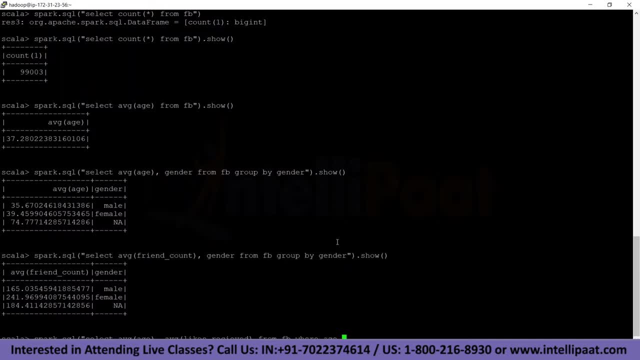 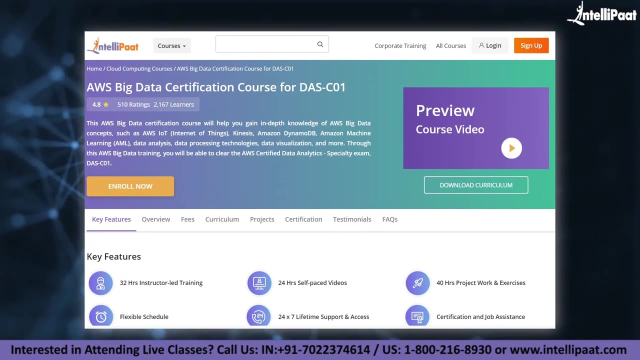 and we can specify where age is greater than equals to 13, which is the minimum age requirement for Facebook. and just a quick info: guys in Telepad provides AWS big data certification course mentored by industry experts, the course link of which is given in the description below. now let's continue with the session. 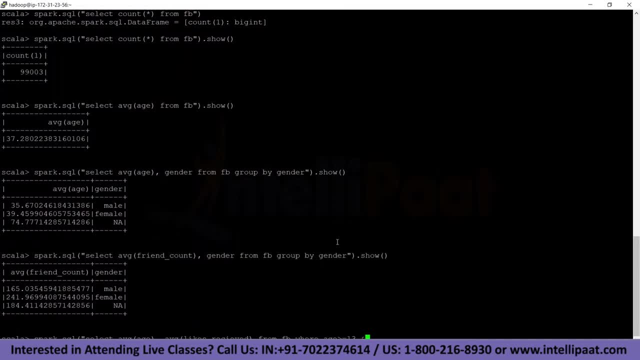 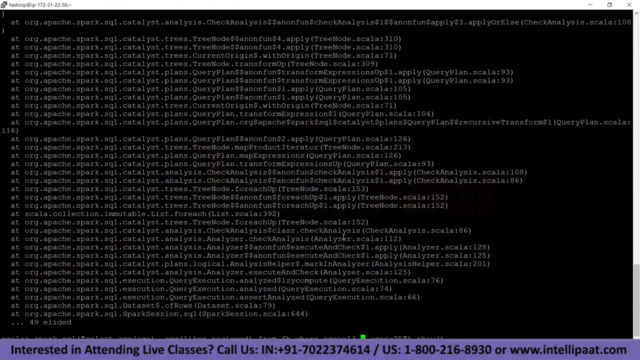 yeah, I'm not entirely sure. and each smaller than equals to say: let's go with 25, right? so the young generation, we go with that and put it over there and I can go to show. okay, so this was an- and pretty sure about that- select average. 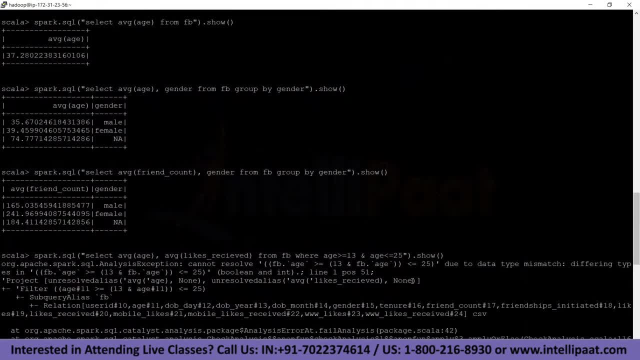 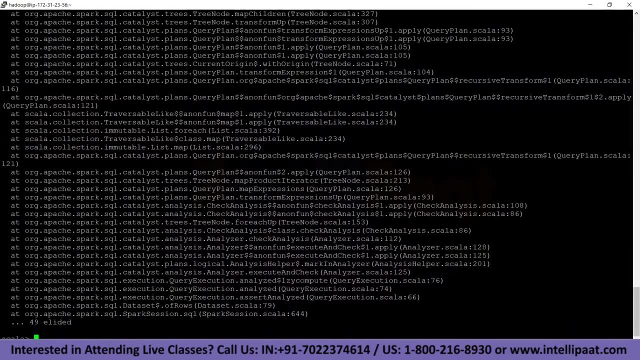 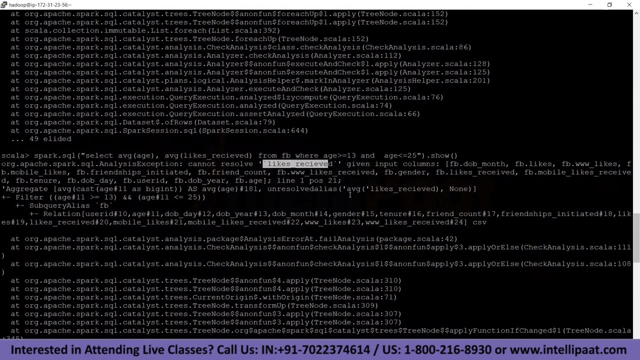 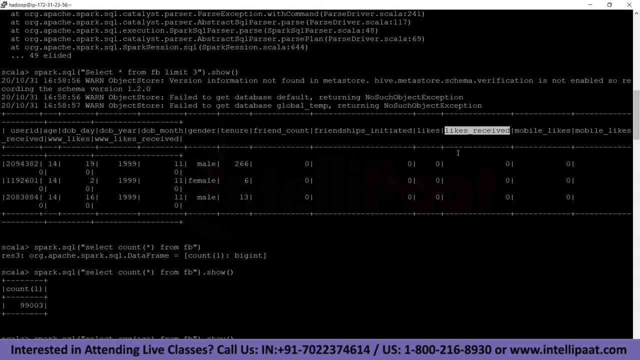 age and like saved, so it's an issue that we had particularly okay. so what exactly did I do wrong over there moment? okay, you cannot resolve Reich's receive, so I think I've mismatched the column sport likes receive. maybe I have, so what? I'll just take this, put it up over here. 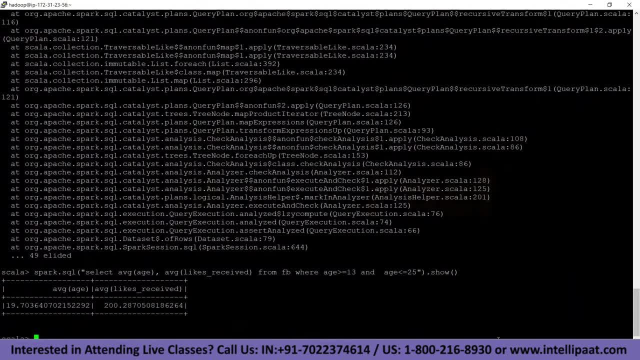 yeah, so was a type of. so we can see that the average age of people work between the age of 14 and 25 is 19. so in the young sort of side, on with P F, 19 of the average age and likes those that those persons have, see our The Area of 200. so 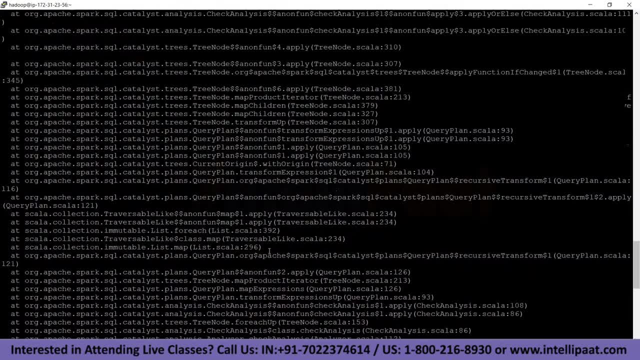 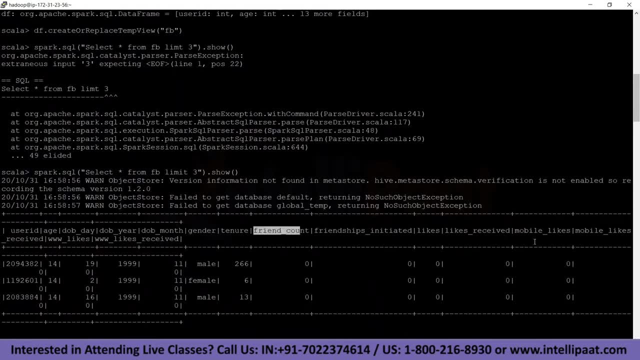 there's that and you go up and look at something else we can do with that. we can cool cat friend, count right and you can also do something interesting with it: mobile likes, so we can understand their usage. like how many? uh, like the usage of mobile phones as? 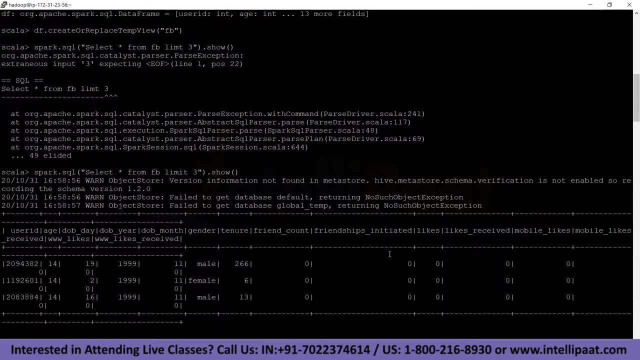 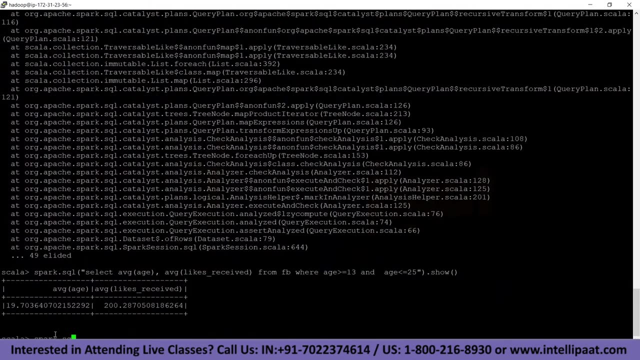 compared to web browsers. we can understand that from this. so, firstly, let's go with the friend count. i think we have already dealt with the fan counters. go with the mobile likes and the website like. so let's go with that spark dot sql. select from average type in mobile. 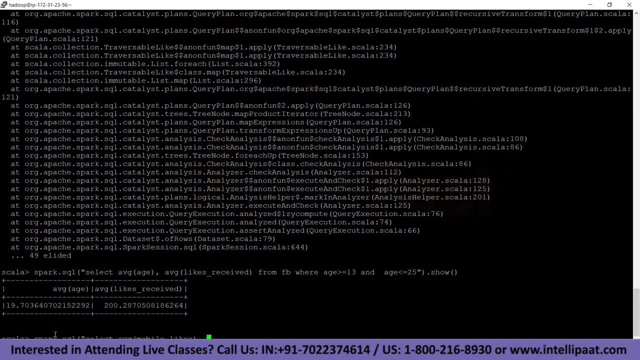 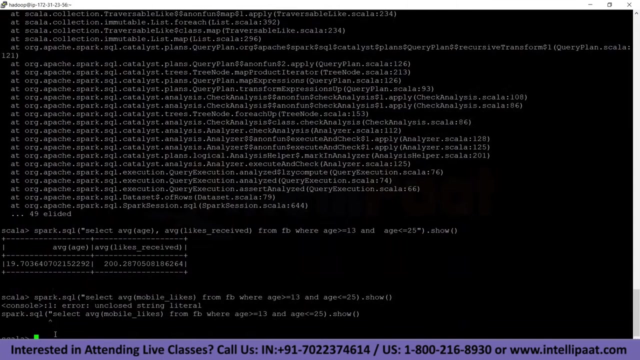 underscore likes and from fb where h is 13 greater than equal to 13 and h is less than equals to 25.. we'll go with that and like not show. put it back over there. so what else did we do wrong over here? unenclosed, we didn't add a double quote. 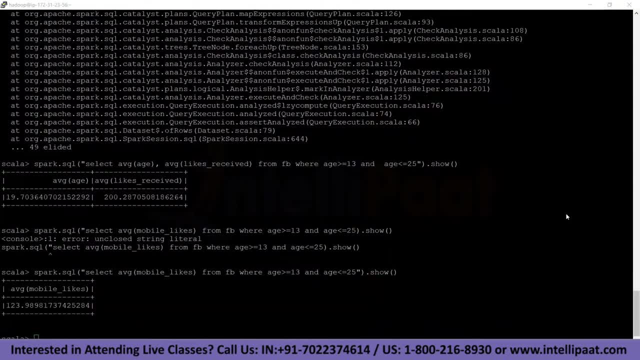 over there. so we put that and we get our output. does it give a squiggly line when the column name is spelled uh incorrectly? no, it does not when you're dealing with the terminal. terminal is very minimalistic in nature so you would not get the squiggly line. uh it, you will get the squiggly. 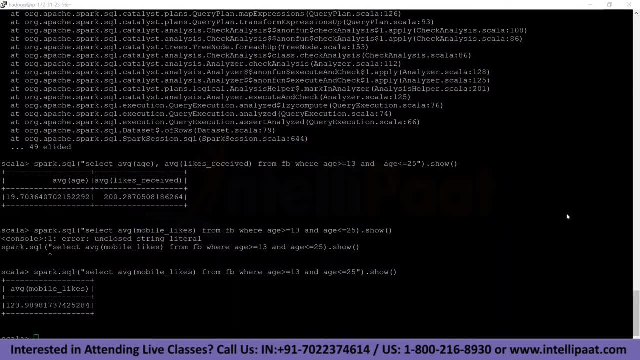 line. if you're using some of the ui based uh implementation of it, like you're using a notebook or something, you will get a squiggly line in that uh. so what are the other questions that we have any more questions about? uh? so sql setup. c È question is: can we access this spark cluster in? 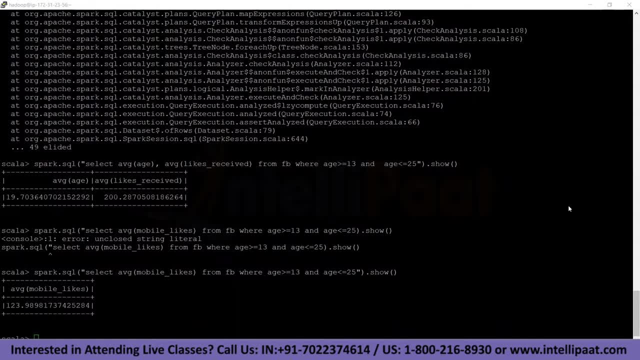 any aws compute engine. so, uh, no, you cannot actually do that. you cannot access the spark cluster. but yeah, you can actually do that. so if you have actually created an emr cluster and you have a separate sort of compute engine like an ec2, ec2 instance running separately, right, 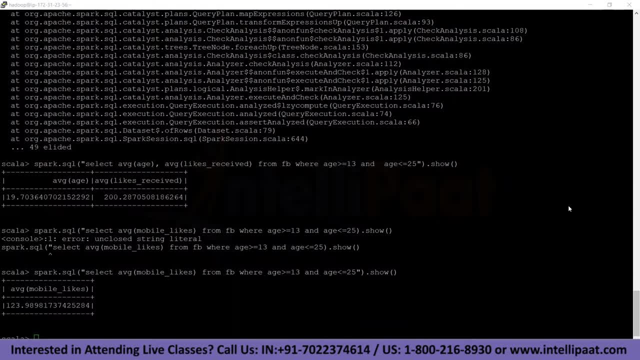 if you have configured the inbound rules correctly, if you've configured the security profiles, µ strings, subnet- correctly, you can actually do that. You can connect your EC2 instance with the Spark cluster and run these jobs remotely as well. That is also possible. So that is mostly something that is possible. No issues with that. 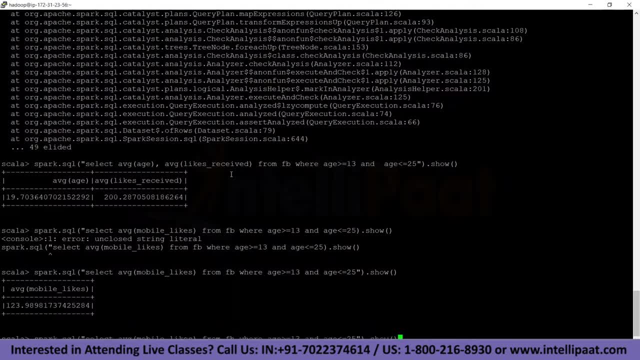 Alright, so this is essentially what we can do with that, and we can check the same for a higher age demographic, say for greater than 25 and above, essentially 25 and above. Let us see for that. So this is the average mobile usage. 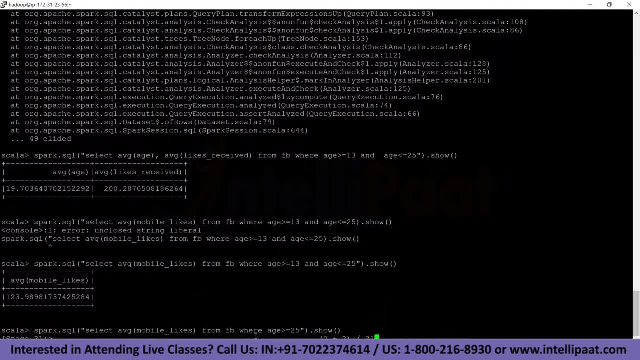 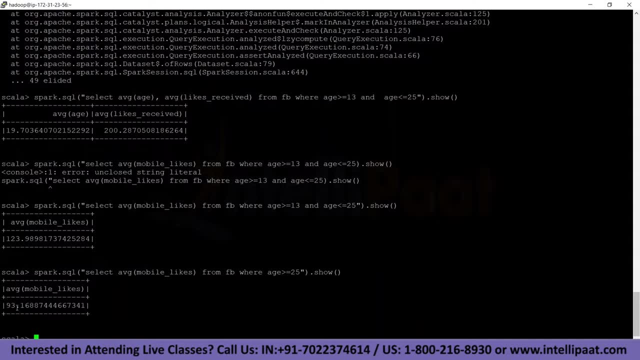 compared. if we compare this with the higher age demographic, let us understand how many, how much activity Understand this from that that the higher age demographic has a generally lower mobile usage than the younger age demographic. Right, but we can also check this for website. so web browser, computer When we 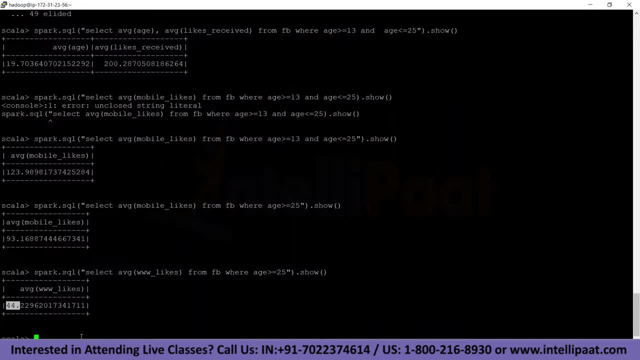 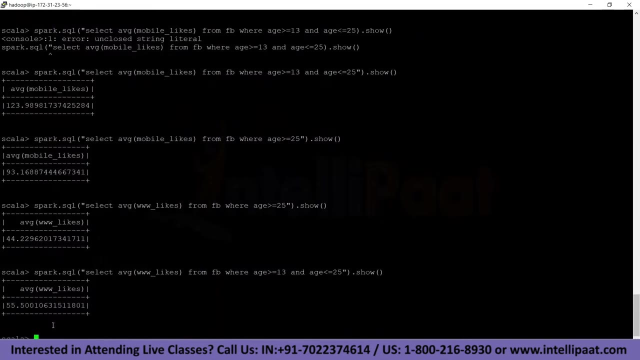 do that, we can see that it's 44 for a higher age demographic and if we simply go ahead and put this back Just a moment and put this back for a younger age demographic, See that it's 55. So we can see that at any age group, the usage of the younger people is higher of. 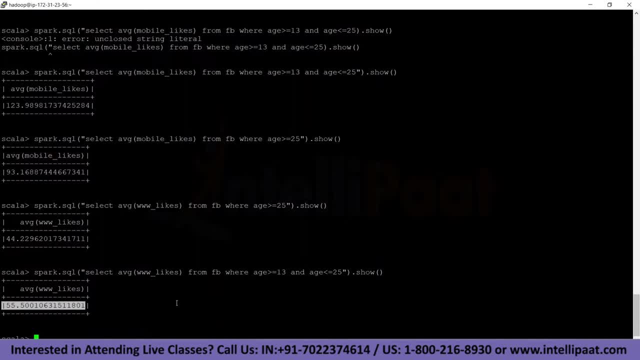 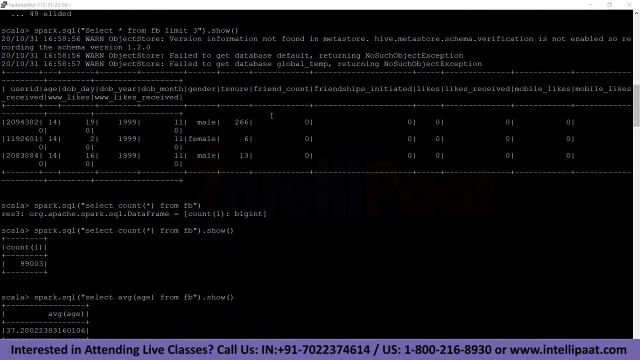 social media accounts, social media websites than older people. So that is there. So that is about. I mean, you get the gist of it right. We can go on and on with creating questions and solving those, but these are the sort of things that you would be actually asked of when you're working in the 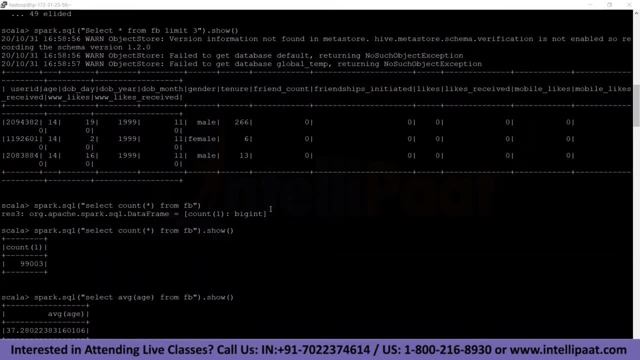 big data domain. So yeah, there's that. So there's one other question: If you want to create this EMR with just EC2 instances, how do we install Hadoop to use one more than one machine? So creating this manually using EC2 instances is. 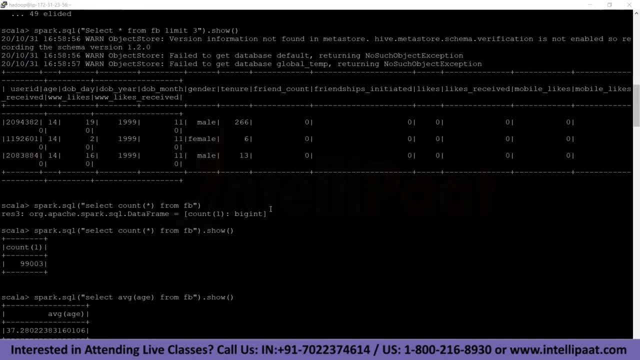 very much possible, but it's a very time-taking task, right. So there are a lot of variables attached to it. Hadoop is not that easy to install. That is why there is a Hadoop administrator course, right. It's a very sort of complex. 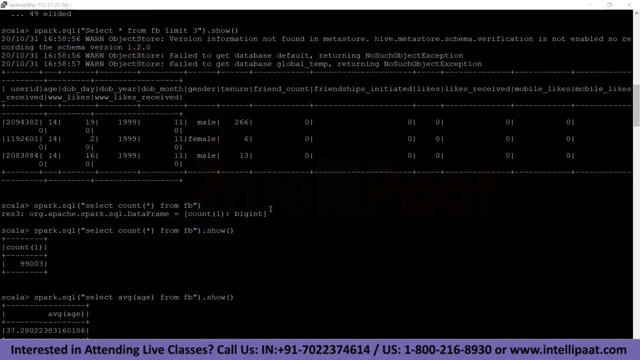 thing to do. So, yeah, but you can go about and do it. So we're not going to actually go over that in this particular course, because I am also not aware of how to do Hadoop administration, Hadoop installation. Well, you'll run into a lot of errors, essentially, when you do that. 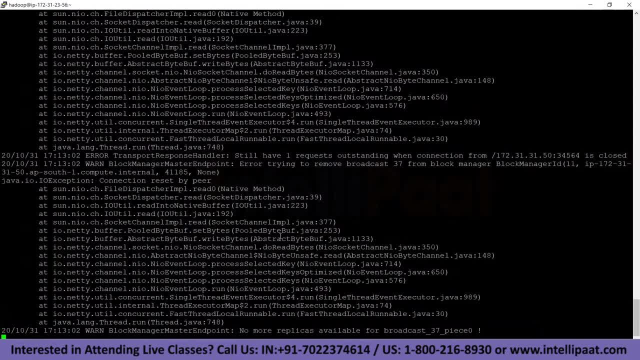 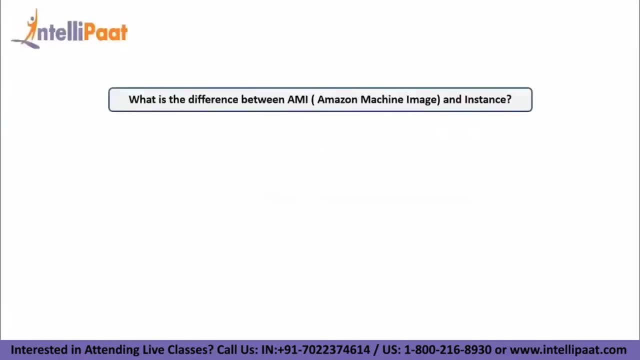 and you'll have to keep solving them as you move ahead with your job, right? So the first question says: what is the difference between an AMI and an instance? So, guys, an AMI is nothing but a template of an operating system. It's a. 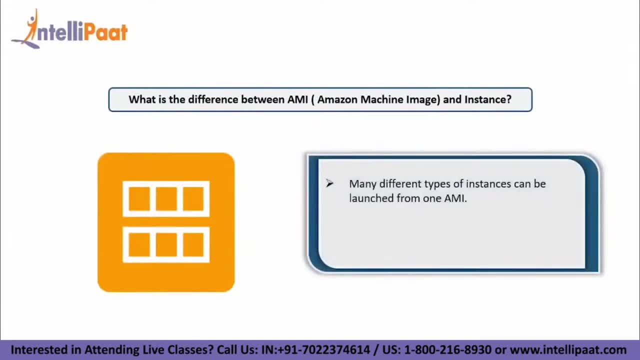 just like a CD that you have of an operating system which you can install on any machine on the planet, right? Similarly, an AMI is a template or is an installation of an operating system which you can install on any servers which fall into the Amazon infrastructure. alright, You have many. 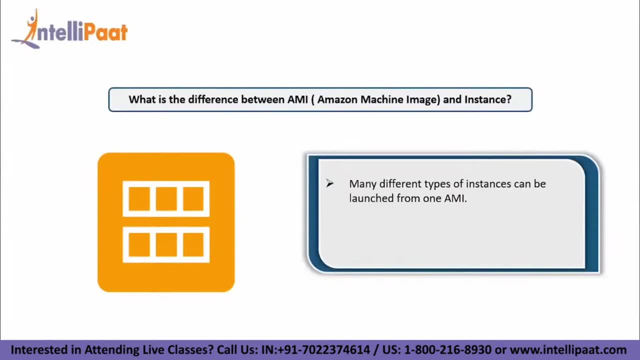 types of AMIs. You have Windows AMI, you have Ubuntu AMIs, you have CentOS AMIs, etc. There are a lot of AMIs that are present in AWS marketplace and you can install them on any server, So it's a very simple and easy thing to do. So 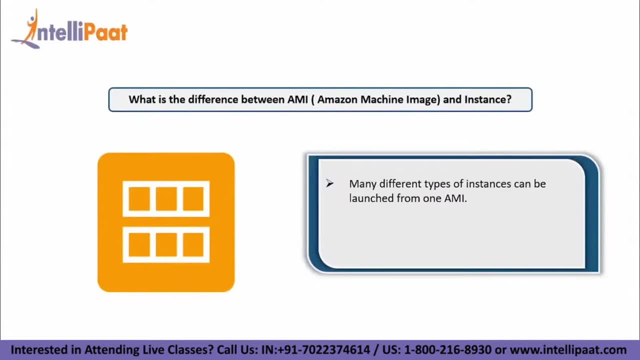 servers which are there in the AWS infrastructure. all right, coming on to instances, what are instances? so, instances are nothing but the hardware machines on which you will install AMI, right? so, like I said, AMIs are templates which can be installed on machines. these machines are called instances. 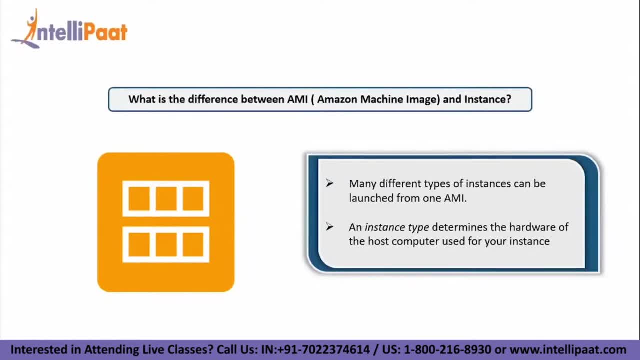 and again, instances also have types based on the hardware capacity. for example, a one CPU and one GB of machine is called t2.micro right. similarly you have t2.large, you have t2.extralarge. then you have IO intensive machines, you have storage intensive machines, you have memory intensive. 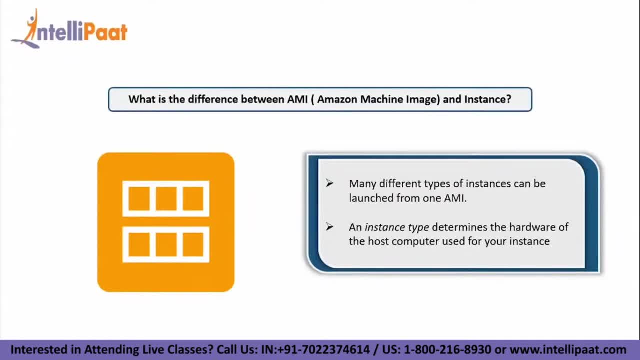 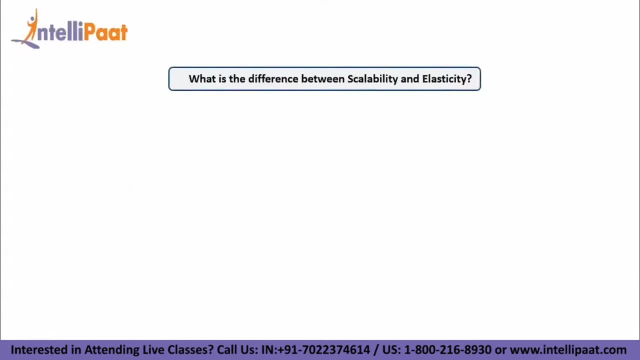 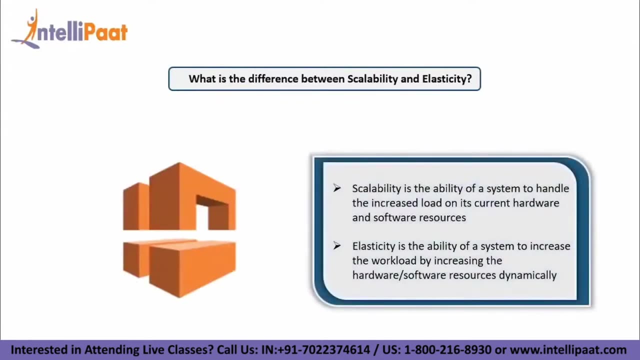 machines, and all of these have been classified in different classes, right, depending on their hardware capability. so this was the difference between an AMI and an instance. our next question asks us: what is the difference between scalability and elasticity? all right, so, guys, scalability versus elasticity is a very confusing topic and if you think about it so, scalability is nothing. 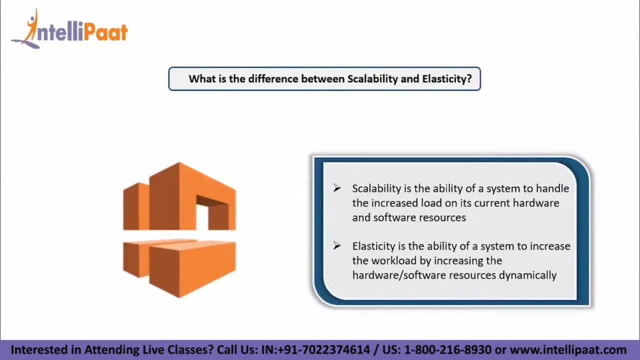 but increasing scalability is nothing but increasing scalability is nothing but increasing the, the machine's resources. for example, if your machine has 8 GB of RAM today, you increase it to 16 GB. therefore, the number of machines are not increasing. you are basically just increasing the specification of the machine, right, and this is called scalability. when we talk about elasticity, 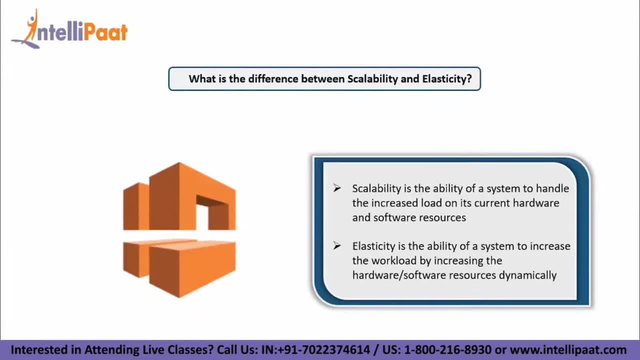 we are basically increasing the number of machines present in an architecture. we are not increasing the specification of any machine. for example, we choose that we require a 3 GB machine with, say, around 8 GB or 10 GB of storage, right, so any replica which will be made or any order scaling which will happen, 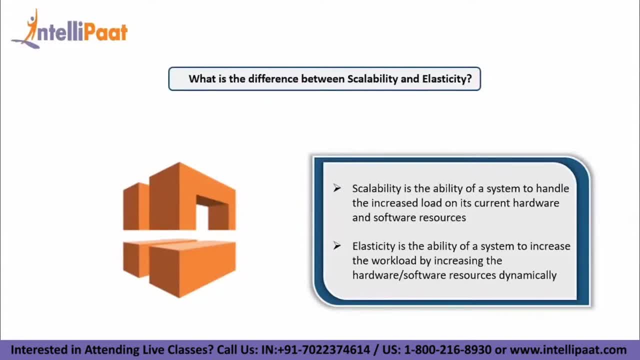 it will only happen to the number of machines. it will no where be related to the specification of the machine. the specification of the machine will be fixed. the number of machines will go up and down, and this is called elasticity. on the other hand, scalability is called is basically termed as the change of the 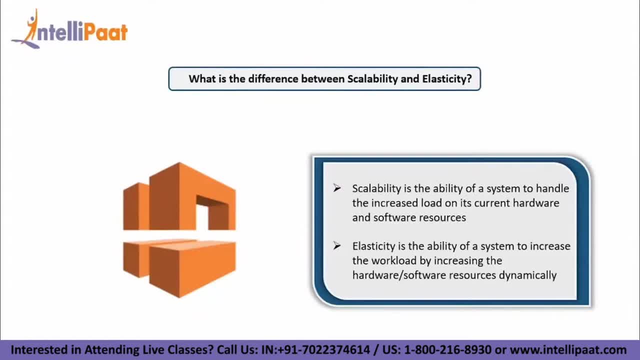 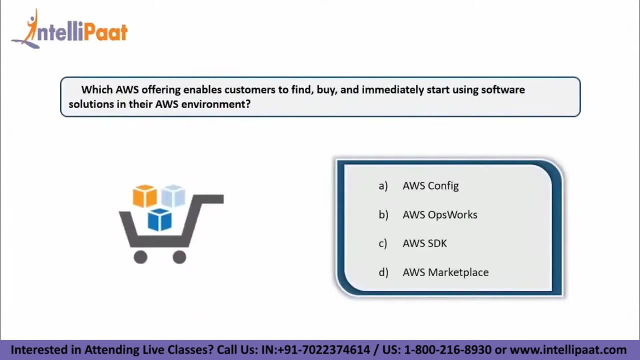 specification of the machine. that is, you're not increasing the number of machines, you're basically just increasing the specs of the machine, for example the RAM, the memory, the hard disk, etc. and this is the basic difference between scalability and elasticity. moving forward, our next question is which AWS offering enables 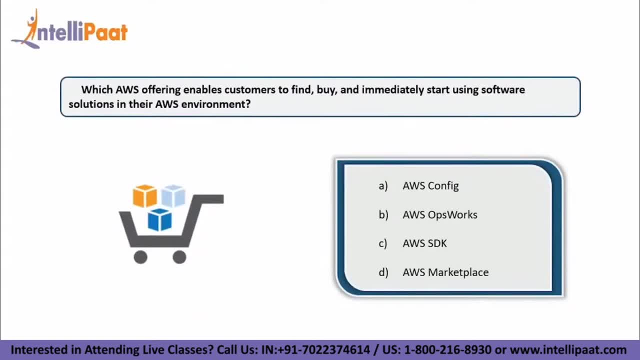 customers to find, buy and immediately start using software solutions in their AWS environment. now you can think of it as, say, you want a deep learning AMI, or you want a Windows Server AMI, which specific software is installed on it, right? so some of them are available for free, but some of them can be purchased. 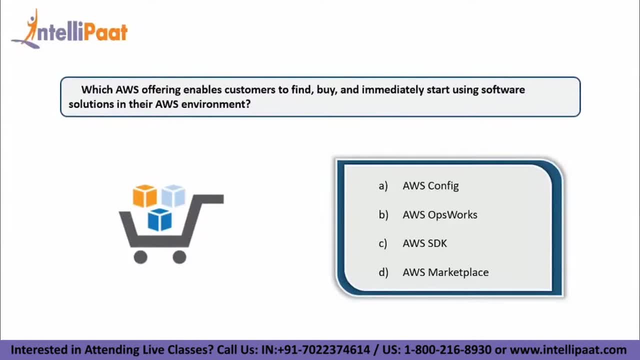 in the AWS marketplace. so the answer for this is AWS marketplace. it's basically a place where you can buy all the AWS systems that you, or all the AWS or non AWS softwares that you require to run on the AWS infrastructure. right, so the answer is AWS marketplace. moving on. 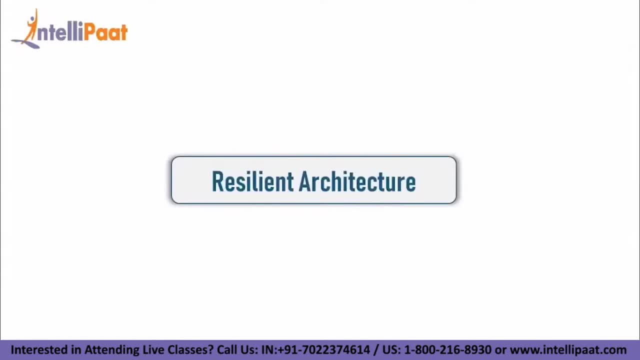 I. the next question would fall under the domain of resilience architecture. so all the questions that will be discussing henceforth in this domain will all be dealing with the resiliency of an architecture. all right, so a customer wants to capture all client connection information from his load. 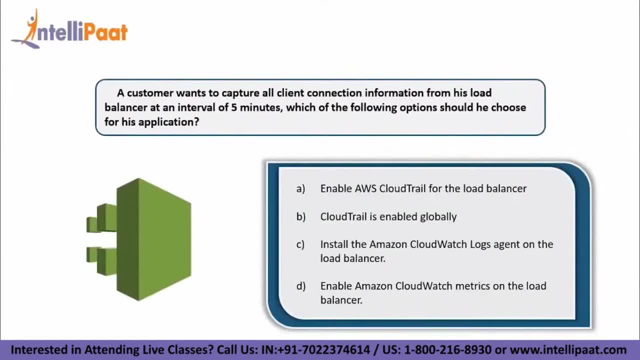 balancer at an interval of 5 minutes, which of the following options should be chosen for his application? all right, so I read out the options for you. the option A says: Enable AWS CloudTrail for the cloud plancer for the load balancer. option B says: 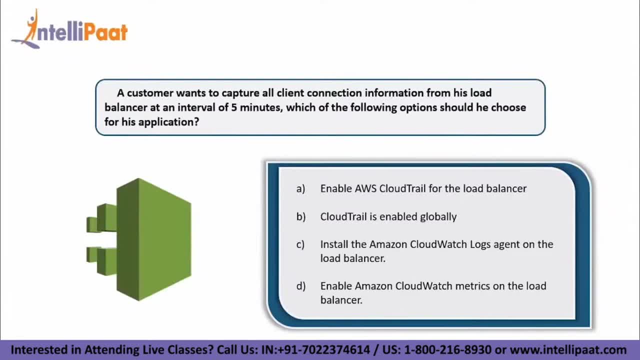 says cloud trail is enabled globally. option c says install the amazon cloud watch logs agent on the load balancer and option d says enable cloud watch metrics on the load balancer. all right now, if you think about it, cloud trail and cloud watch are both monitoring tools, so it's a bit. 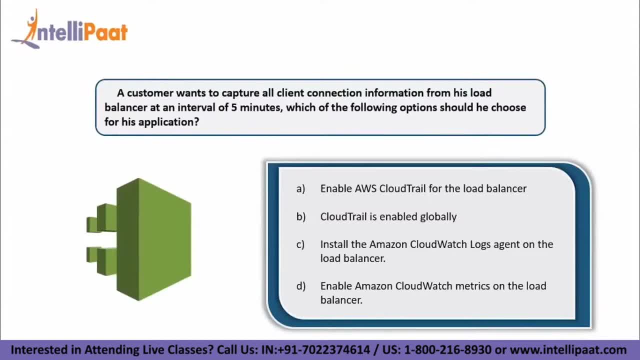 confusing, but if you have studied it deeply or if you understand how cloud trail works and how cloud watch works, it is actually not that difficult, all right. so the answer for this is a, that is, you should enable aws cloud trail for the load balancer, reason being option b is not correct. 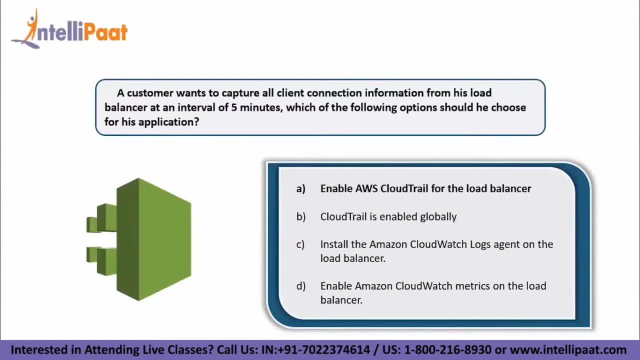 cloud trail is not enabled by default or is not enabled globally to all the services. option c says install amazon cloud watch. so option c and option d you will not even consider reason being that. you're talking about the log of the client information, right? what all people are connecting. 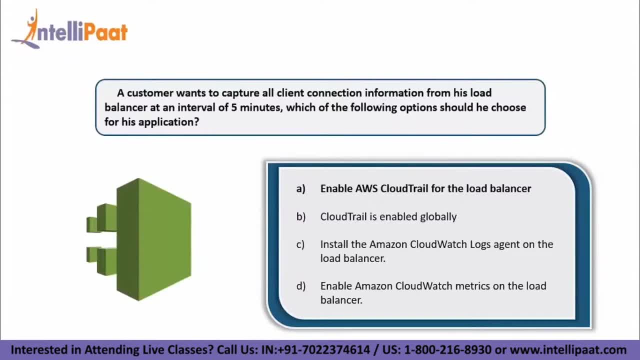 to the load balancer, what ip addresses are connecting to the load balancer, etc. cloud watch deals with the local resources of you, the instance that you are basically monitoring. for example, if you are monitoring ec2 instance, cloud watch can monitor the cpu usage or the memory usage of that particular instance. 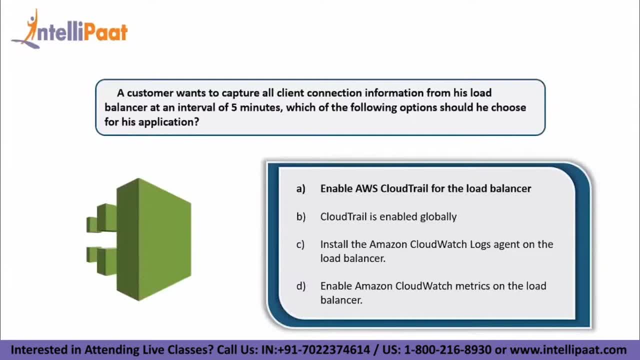 it cannot take into account the connections which are getting connected to your aws infrastructure right. on the other hand, cloud trail deals with all these kind of things wherein client information or any kind of data which can be fetched from a particular transaction. all of that can be recorded. 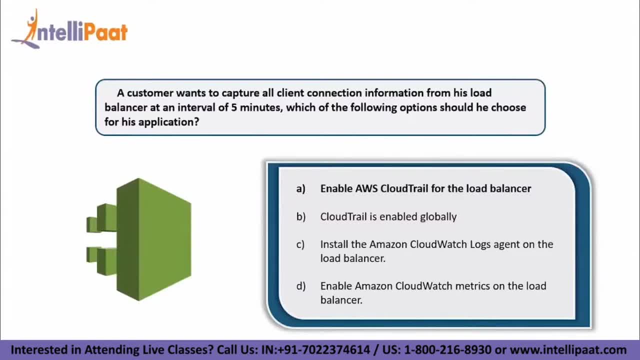 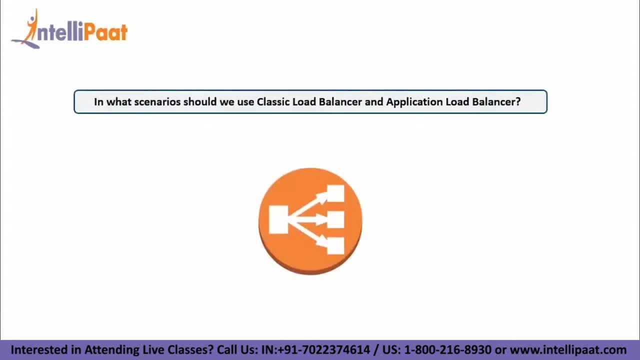 in the logs of cloud trail and hence, for this particular question, the answer is: enable aws cloud trail for the load balancer. moving on, our next question is: in what scenarios should we choose classic load balancer and application load balancer? all right, so, uh, for this question, i think, uh, the 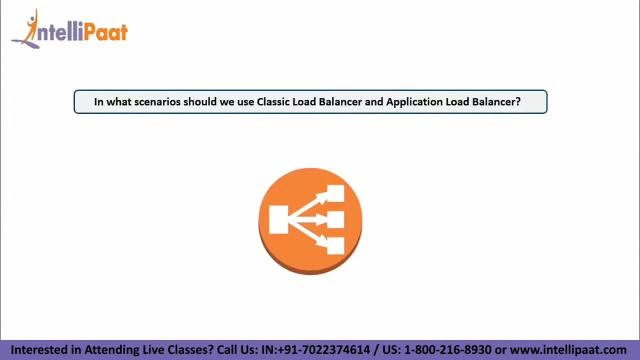 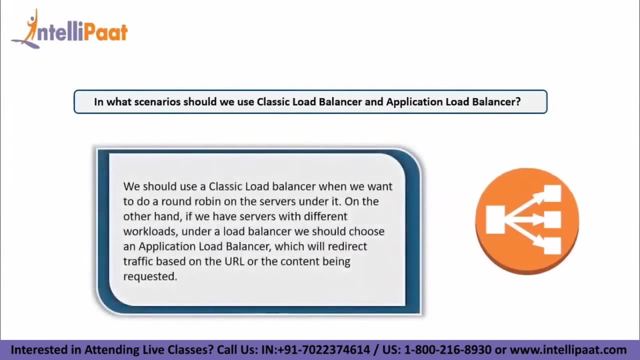 best way to answer this question would be to understand what exactly is classic load balancer and what exactly is application load balancer. all right, so a classic load balancer is nothing, but you know it's changing the load balancer. yeah, so if you're using a load balancer for application catalog, 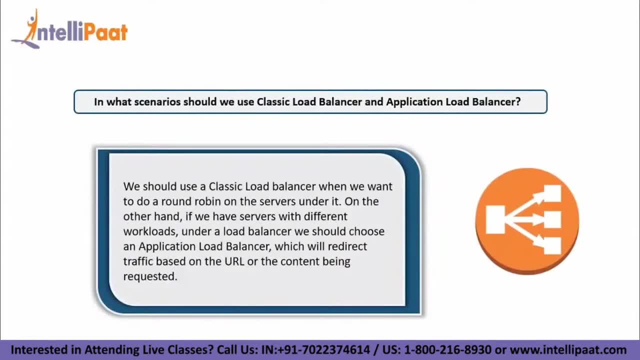 It's an old-fashioned load balancer which does nothing but round-robin based distribution of traffic, which means it distributes traffic equally among the machines which are under it. It cannot recognize which machine requires which kind of workload or it requires which kind of traffic. 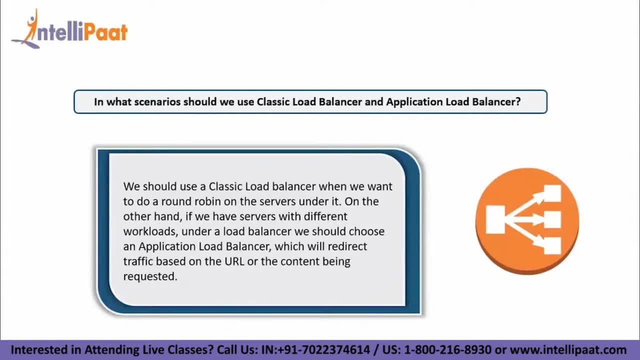 Whatever data will come to, a classic load balancer will be distributed equally among the machines which have been registered to it. On the other hand, application load balancer is a new age load balancer which basically deals with identifying the workload which is coming to it right. 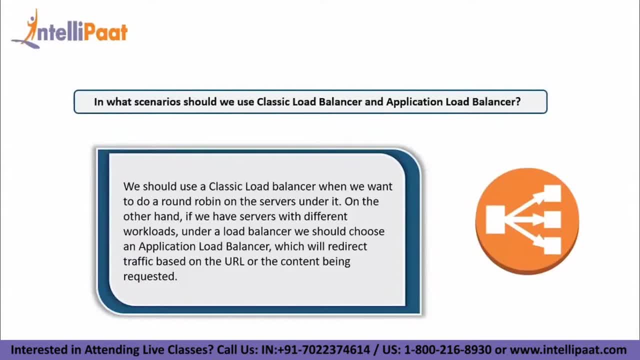 It can identify the workload based on two things. It can either identify it based on the path. For example, you can say that you have a website which deals in image processing and video processing, So you can say it might go to intellipacom slash images or slash videos. 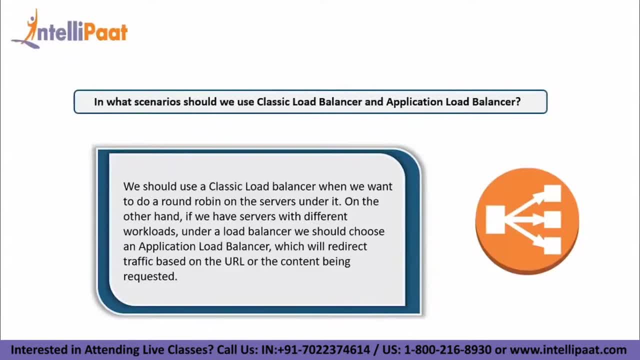 So if the path is slash images, the application load balancer will directly route the traffic to only the images servers, right. And if the path is slash videos, the application load balancer will automatically route the traffic to the video servers. And this is application load balancer. 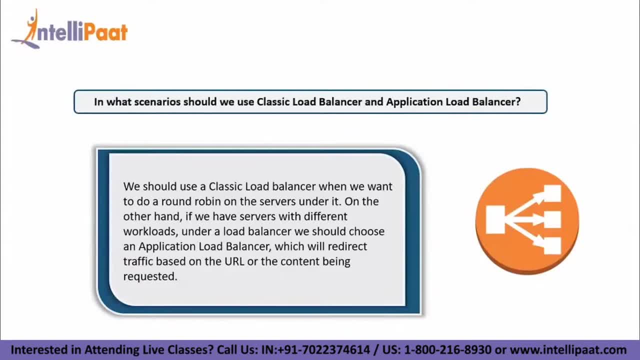 So, whenever you are dealing with multivariate traffic, that is, traffic which is meant for a specific group of servers, you would use application load balancer. On the other hand, if you have servers which do the exact same thing- right, You just want to distribute the load among them equally- then in that case you would use 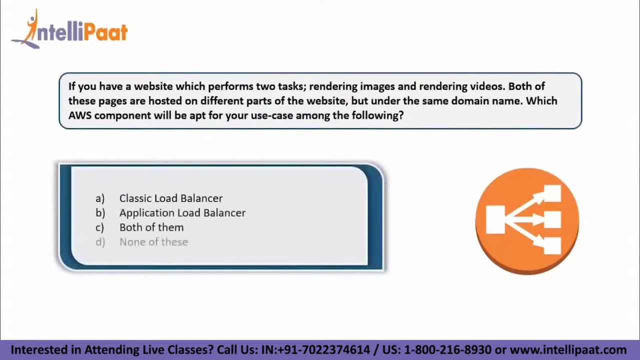 A classic load balancer. Our next question says: if you have a website which performs two tasks, that is, rendering images and rendering videos. both of these pages are hosted on different parts of the web, right, But under the same domain name. 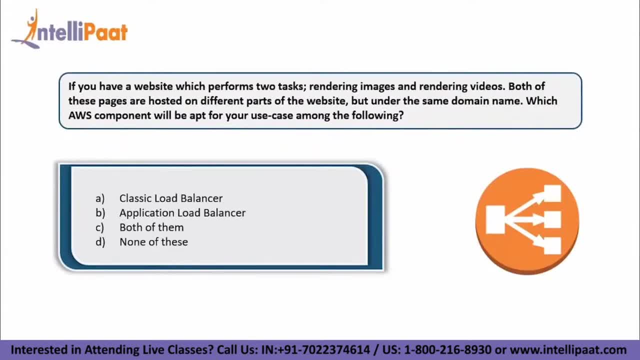 Which AWS component will be apt for your use case among the following. Alright, so this, I think, is an easy question. Reason being: we just discussed this right. So the answer for this is application load balancer. Reason being: the kind of traffic which is coming is specific to its workload. 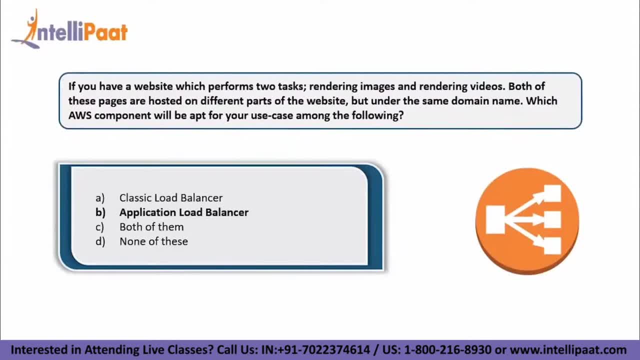 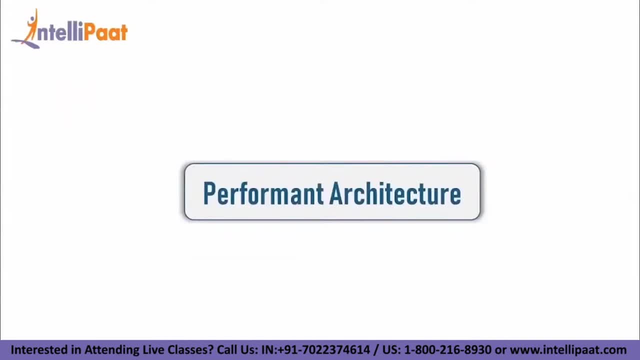 And this can be differentiated easily by an application load balancer. Okay, so we are done with the resilient architecture questions. Now let's move on to the performance architecture domain, Where we will be discussing about how to, about architectures which are performance driven right. 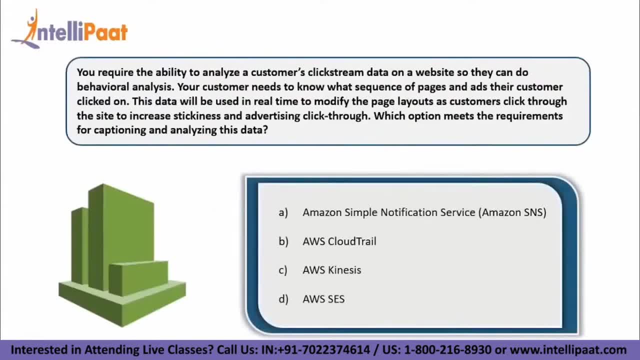 So let's take a look at the first question. So the first question says you require the ability to analyze a customer's clickstream data on a website So they can do behavioral analysis. So your customer needs to know what. 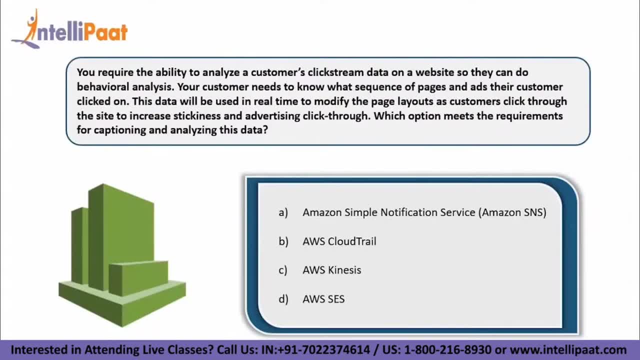 Sequence of pages and ads their customers clicked on. This data will be used in real time to modify the page layouts as customers click through the site. to increase stickiness and advertise, click through Which option meets the requirement for captioning and analyzing this data. 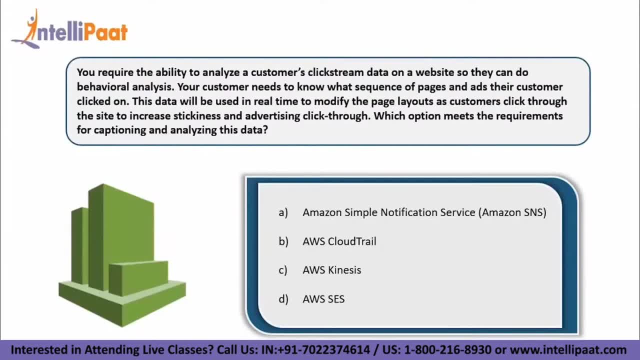 Alright, so the options are Amazon SNS, AWS CloudTrail, AWS Kinesis and AWS SES. So let's first start with the odd one out options, right? So we have Amazon SNS, which deals with notifications. So, obviously, because we want to- basically we want to- track user data, right? 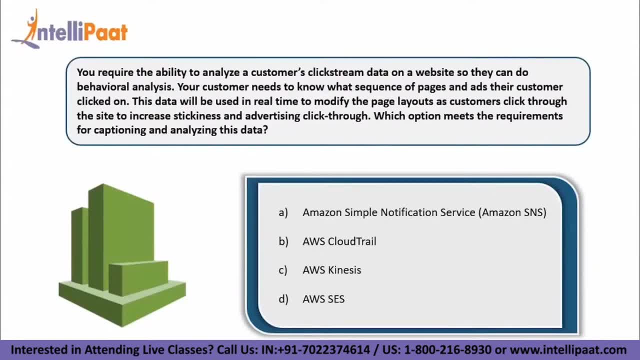 So SNS would not be the apt choice for it, because sending multiple notifications in a short amount of time would not be apt. Similarly, SES would also not be the apt choice, because then we will be getting emails on basically the user behavior, and this would amount to a lot of emails. 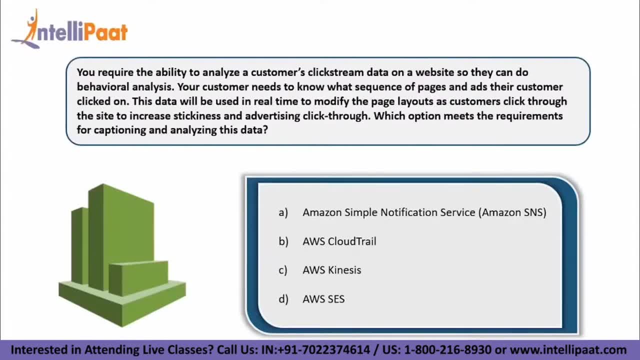 So hence it's not an appropriate solution, I think. Then we have AWS CloudTrail: AWS CloudTrail and AWS Kinesis. Actually, both these services can do this work, But the keyword over here is real time. right, You want the data to be in real time. 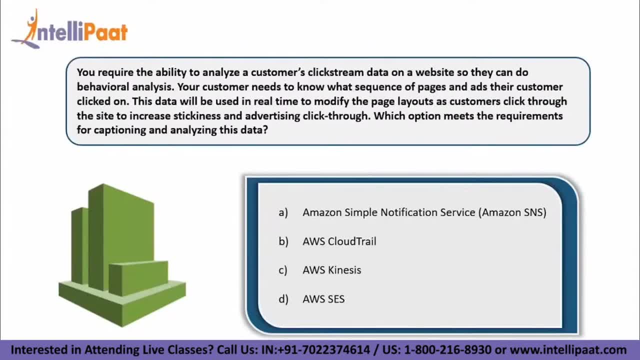 So, since the data has to be in real time, you will choose AWS Kinesis. CloudTrail cannot pass on logs for real time analysis. Kinesis is specially built for this particular purpose And hence, for this particular question, the answer will be AWS Kinesis. 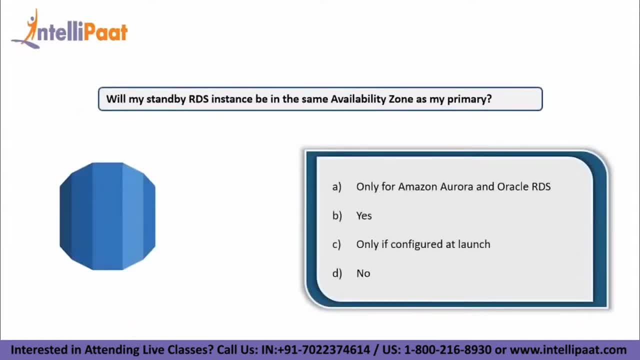 Moving on. Next question is you have a standby RDS instance. Will it be in the same availability zone as your primary RDS instance? Okay, So the options are. it's only true for Amazon, Aurora and Oracle RDS. Second option is: yes. 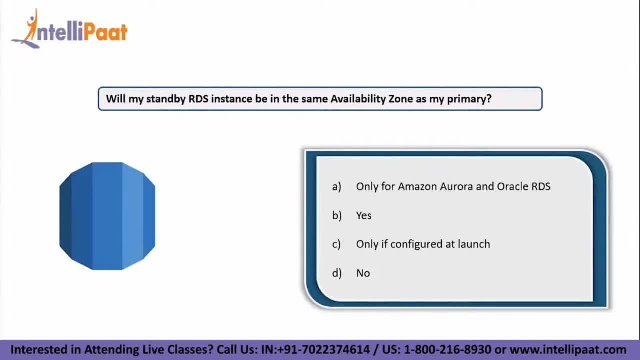 Third option is only if configured at launch, And the fourth option is no, Alright, So the right answer for this? I want you to think about it like this: That whenever you want a standby RDS instance, it will only be there. 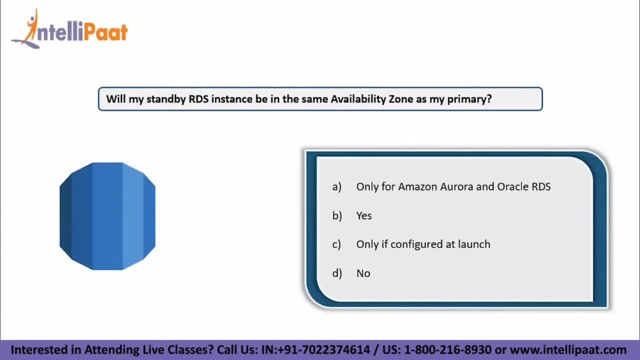 when your RDS instance stops working. now, what could be the reasons that your RDS instance could stop working? probably it could be a machine failure, or it could be a power failure at your, at the place where your server has been launched. it can also be probably a natural calamity, which. 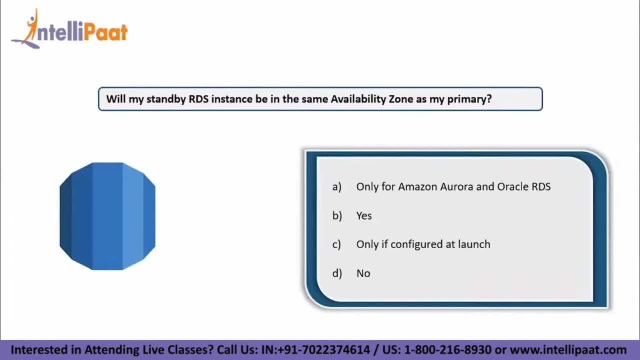 would have struck your data center where your server exists. so all of these could be reasons which could lead to disruption in your RDS service right now, if your standby RDS instance is also in the same availability zone as your primary. these conditions cannot be tackled, or these? 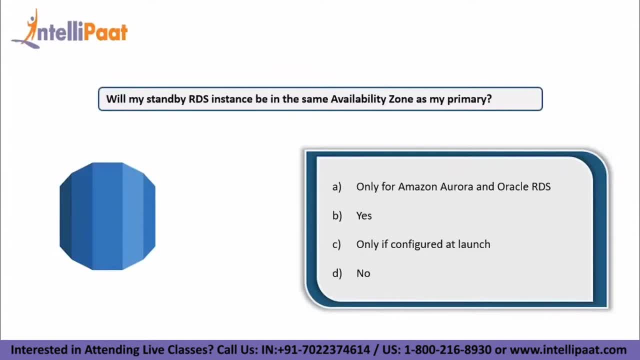 situations cannot be tackled all right. so it is always logical to have your standby machines in some other place right, so that even if there is a natural calamity or if there is a power failure, you, your instance, is always up and ready. and because of that AWS does not give you the option. 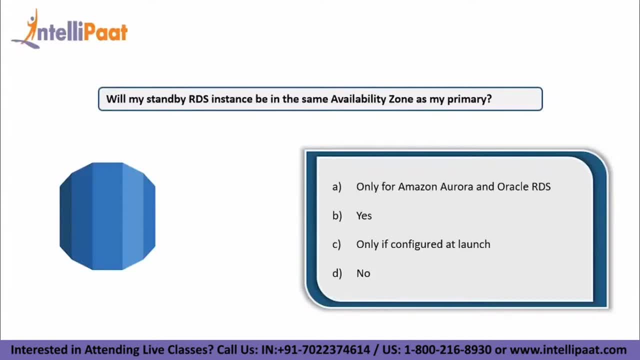 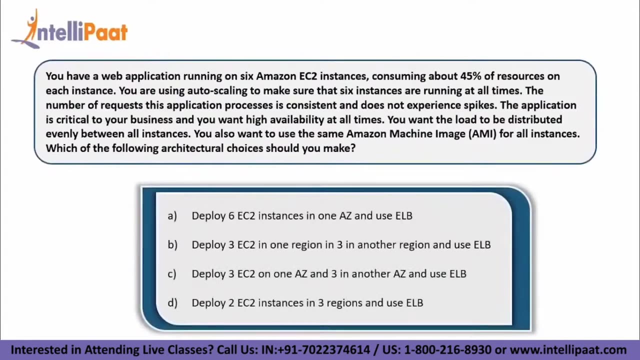 of launching your standby RDS instance in the same availability zone. it always has to be in another availability zones, and that's why the answer is no. your RDS instance will not be in the same availability zone as your primary instance. all right, so our next question is: you have a web. 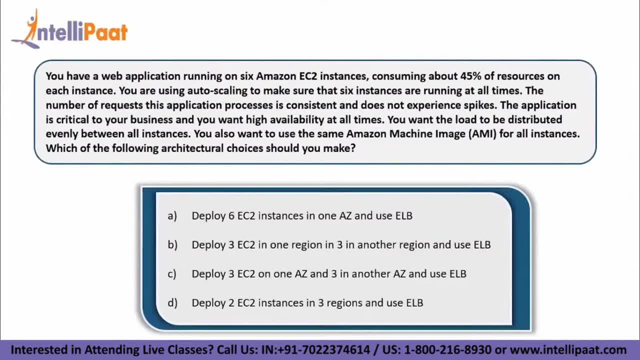 application running on six Amazon EC2 instances, consuming about 45% of resources on each instance. you are using auto scaling to make sure that six instances are running at all times. the number of requests this application processes is consistent and does not experience spikes. all right, so the 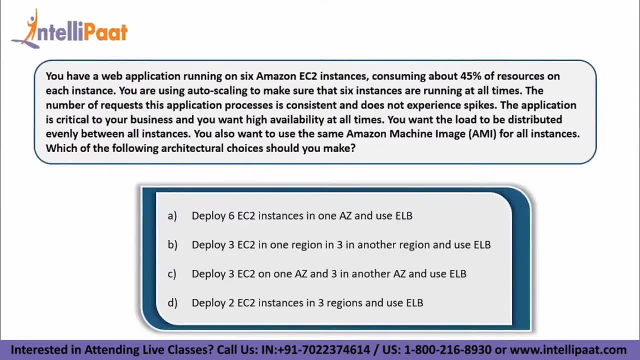 application is critical to your business and you want high availability at all times. you want the load to be distributed evenly between all instances and you also want to use the Amazon AMI for all instances. which of the following architectural choices should you make? all right, so this is a 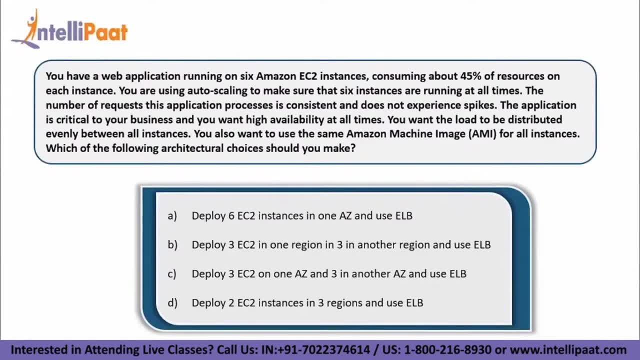 very interesting question. so, basically, you want to run six Amazon ECD instances, six Amazon EC2 instances, and they should be highly available in nature and they would be using an AMI. of course, they are auto scaled. so which among the following would you choose? so you have the options deploy. 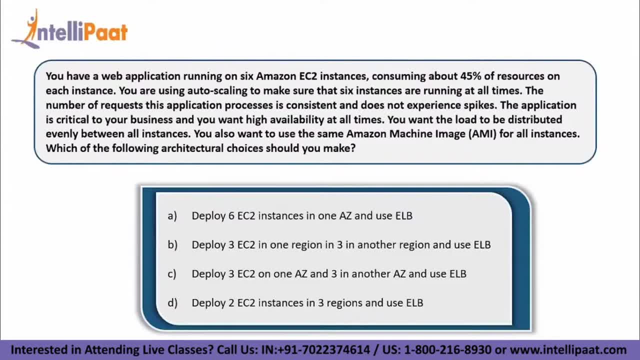 six easy to instances in one availability zone and ELB. deploy three EC2 servers in one region and three in another region and use ELB. you should deploy three easy to on one easy that is availability zone and three in another availability zone and should deploy two easy. 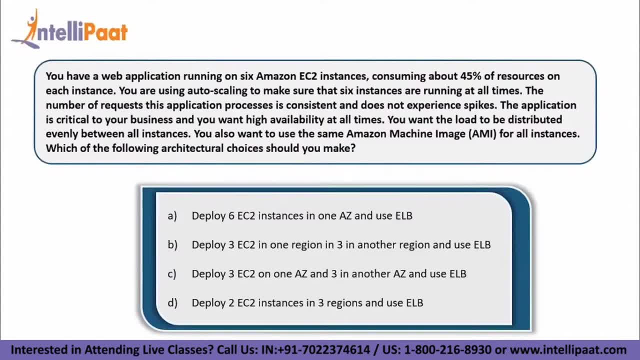 to instances in three regions and use an elastic load balancer. all right now. the correct answer for this would be C, the reason being that AMIs are not available across regions. right, so if you have created an AMI in one region, it will not be automatically available in another region. you? 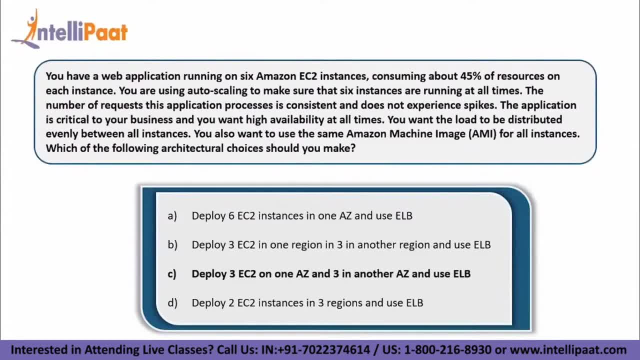 what you will have to do some changes, and only then, or do some operations, and only then it will be available in the another region. so this is reason number one. so the region options mentioned over here get casted out because of this reason. second, if you look at the first, 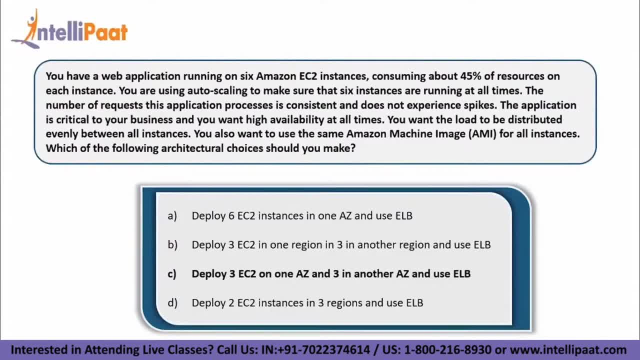 option which says: deploy six easy to instances in one availability zone. that defeats the purpose of high availability because, like I said, if there is any natural calamity or a power failure at a data center, then all your instances will be down. so it's always advisable to have your servers. 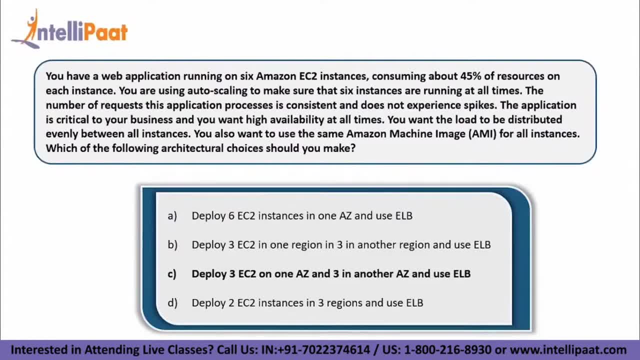 distributed. but since we have that limitation of using an AMI and therefore, and also the limitation that it is not accessible across regions, we would choose distributing our instances among availability zones, and I'd say we have. we just had the option of two availability zone, right, it could be three availability zones and we could. 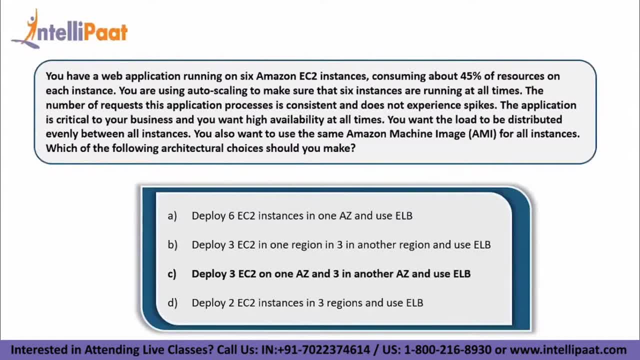 deploy two, two servers in each, and this would also amount to high availability. all right, and, of course, because you want to load balance traffic, if you apply an ELB on top of three availability zones, it will work like a charm. regions across regions, it can become a problem, right and 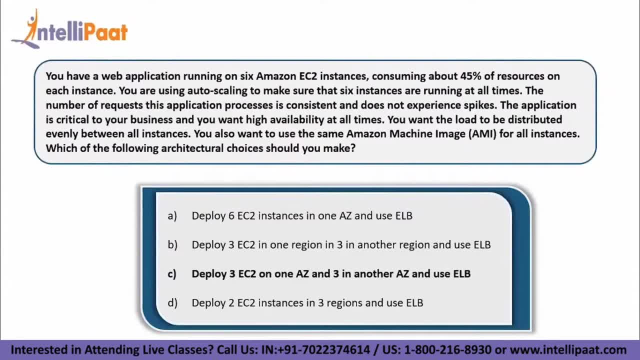 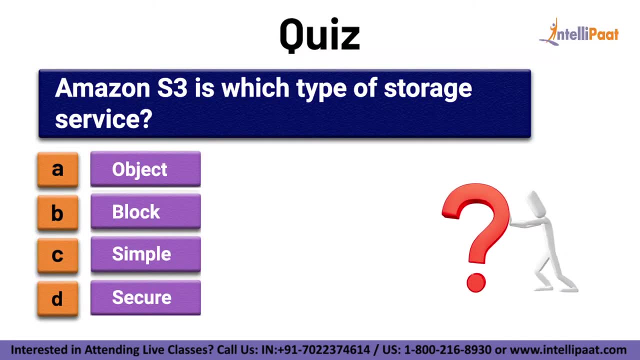 but in availability zones it definitely works and it will work perfectly, all right. so the answer for this question is: you would be deploying ec2 instances among multiple availability zones in the same region across an ELB. all right, just a quick info, guys, test your knowledge of AWS by 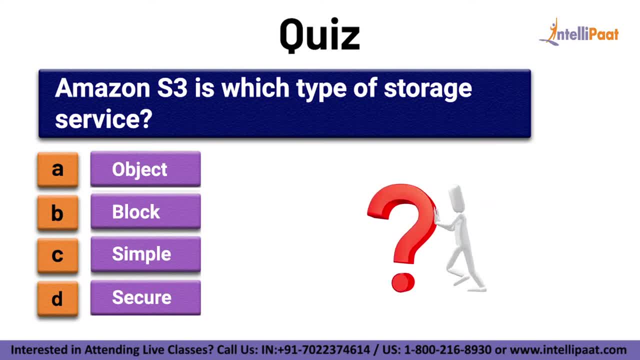 answering this question, Amazon S3 is which type of storage service? a, object B, block C, simple, D, secure. comment your answer in the comment section below. subscribe to Intellipaat to know the right answer. now let's continue with the session. so our next question is: why do we use 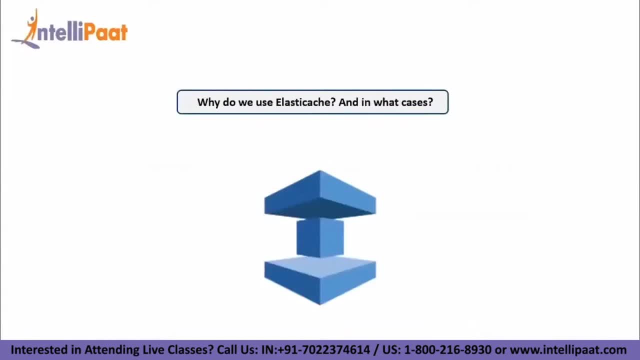 elastic cache and in what cases? all right, so the answer for this is basically related to the nature of the service of elastic cache. so elastic cache has a name suggested. it's basically a cache which can be accessed faster than your normal application. for example, if you talk about a database instance from which you are gathering information, right if you're. 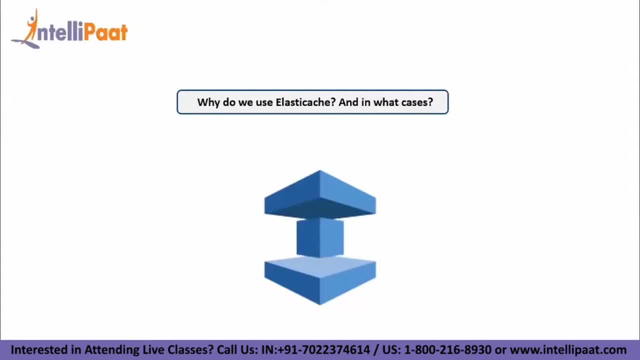 always dealing with the same kind of query. for example, you're always fetching the password for particular users, right? so if you're using an elastic cache, that data can be captured or can be cached inside elastic cache, and whenever a similar request comes in which is asking for that. 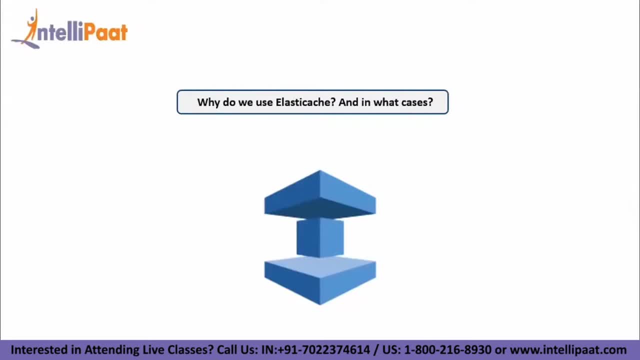 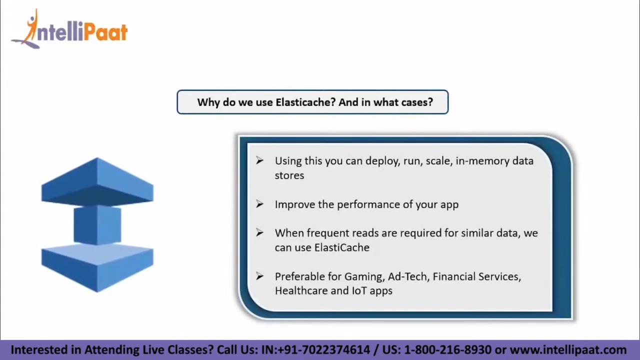 kind of data, your MySQL instance will not be disturbed. the data will directly be relayed from elastic cache. and that is the exact use of elastic cache, right? so you use elastic cache when you want to increase the performance of your systems. right, whenever you have frequent reads of the similar data. so if you 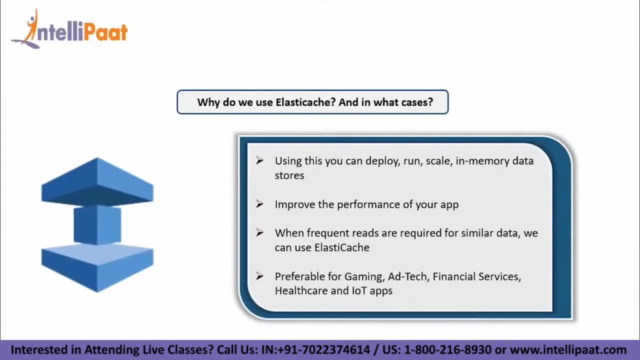 have frequent reads of similar data, we will probably be querying the same kind of data every time and basically that will increase the load on your database instance. but to avoid that you can- you can basically introduce an elastic cache layer between your database and your front-end application, and that would not only. 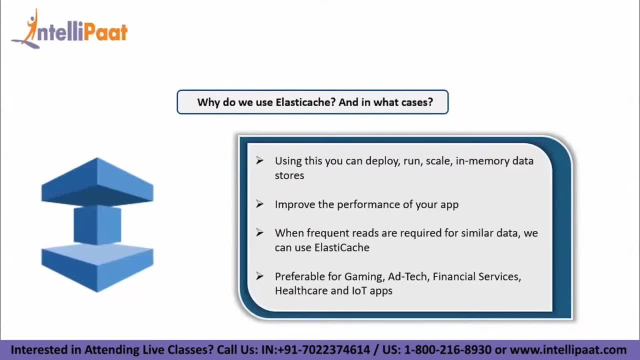 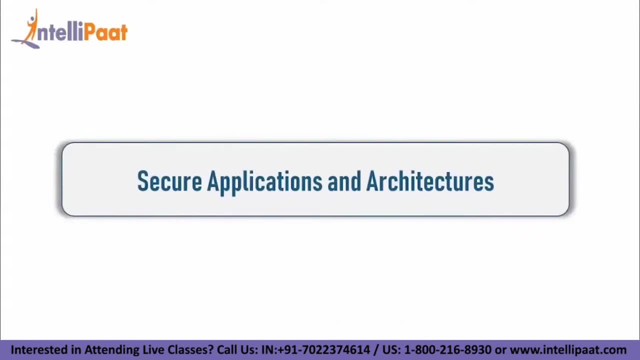 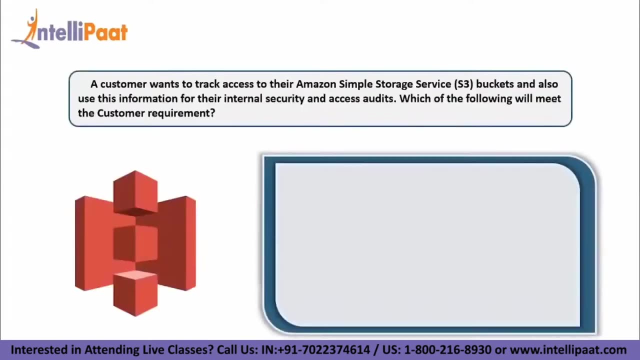 increase the performance but also decrease the load on your database instance, right? so, uh, this was all about performance architectures, guys. our next domain would deal with secure application and their architecture. so let's go ahead and start with the first question of this domain, which talks about a customer wants to track access to their Amazon simple storage service. 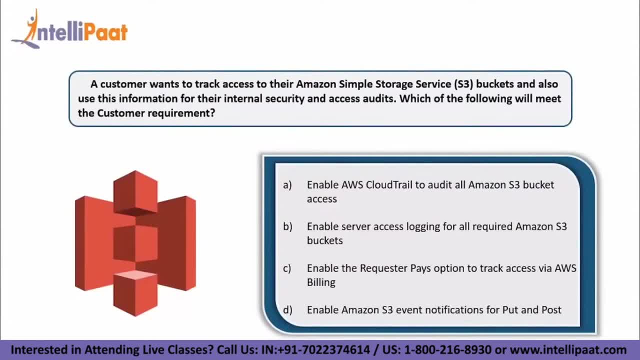 buckets and also use this information for their internal security and access audits. which of the following will meet the customer requirement? so, basically, you want to just track access to the S3 buckets. now, if you want to track access, let's see what are the options so you can enable cloud. 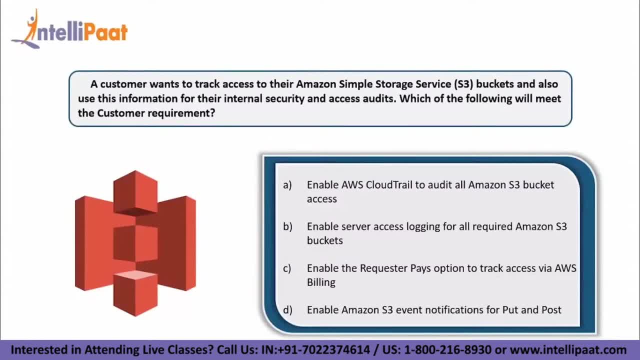 trail to audit all Amazon S3 buckets. you can have enable server access logging for all required Amazon S3 buckets enable the request to pay option to track access via AWS billing or you can enable AWS S3 event notifications for put and post. all right, so I would say the answer is A and reason being why is the answer not B? because 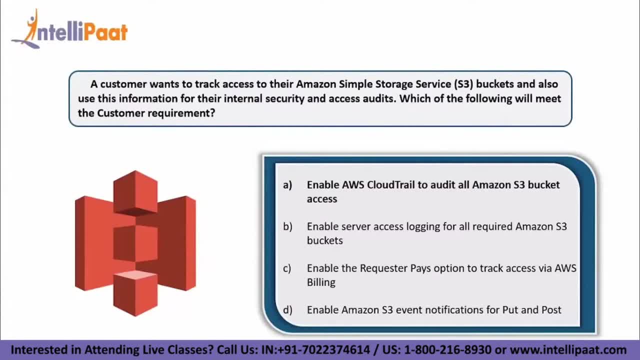 server access logging is actually not required when you want to deal with tracking. access to the objects present in the S3 bucket, a requester pays option to access via AWS billing. again, it's not required because there's a very simple feature of cloud trail which you, which is available to all. 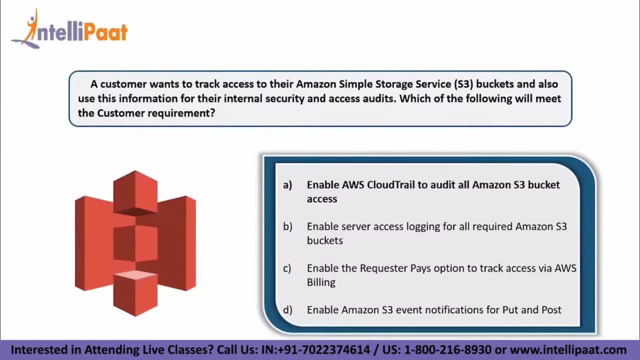 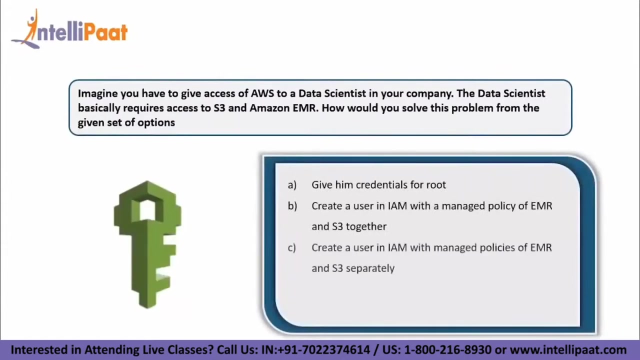 the buckets across S3. so why not use that? and using AWS cloud trail? okay, our next question is: imagine if you have to give access of AWS to a data scientist in your company. the data scientist basically requires access to S3 and Amazon EMR. how would? 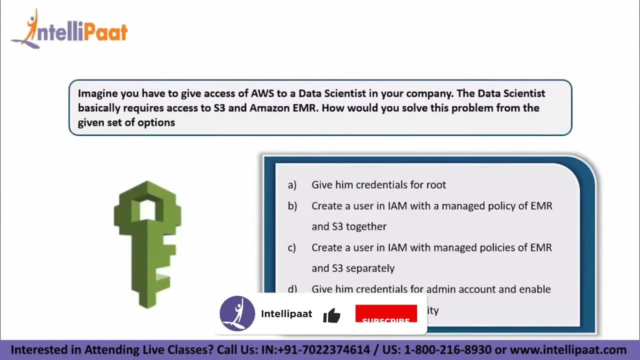 you solve this problem from the given set of options. okay, so you basically want to give a particular services access to an employee and we want to know how would we do that? okay, so the options are: we should give him credentials for root, second option being create a user in IM with. 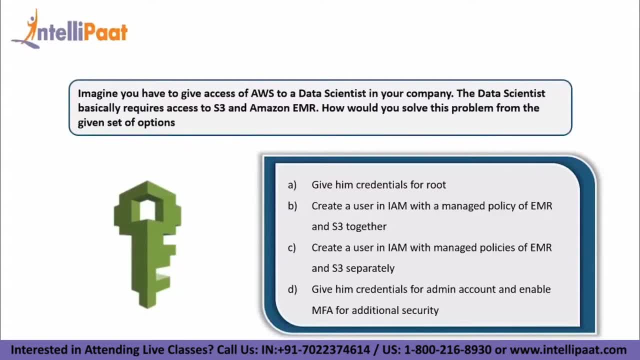 a managed policy of EMR and S3 together. create a user in IM with managed policies of EMR and S3 using credentials for admin account and enable MFA for additional security. okay, so rule of thumb, guys: never give root credentials to anyone in your company. even yourself, you should never use root. 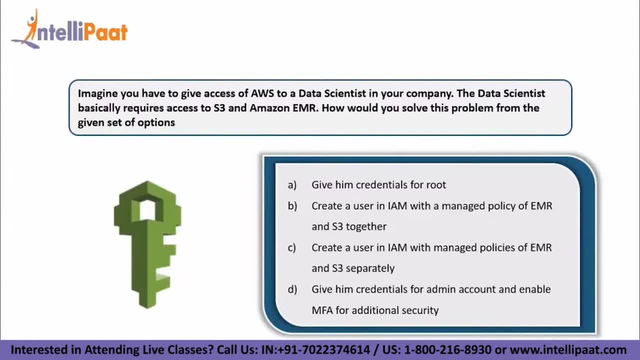 credentials. always create a user for yourself and access AWS through that user. all right, this was point number one. second, whenever you are you want to give permissions to services or permissions of to of particular services to people, you should always create or use policies that pre-exist in. 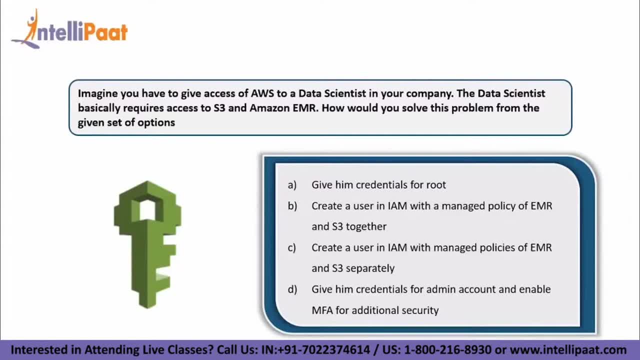 AWS right. so when I say that, I basically mean never merge two policies, okay. so, for example, if you, if you are using EMR and S3 together, that basically means that you create a policy with that gives you, you know, the required access in one document, that is, in one document you mention. 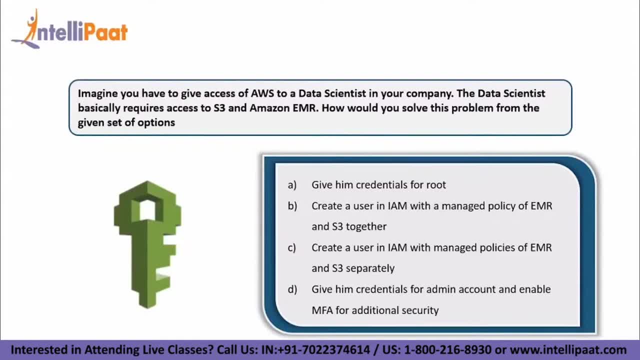 the access for EMR and the in the same document, you mention the access for S3 as well. well, this is not suggested reason being: you have policies created by AWS, which is, which are basically created and tested by AWS, so there is no chance of any leak in terms of security aspect. second, 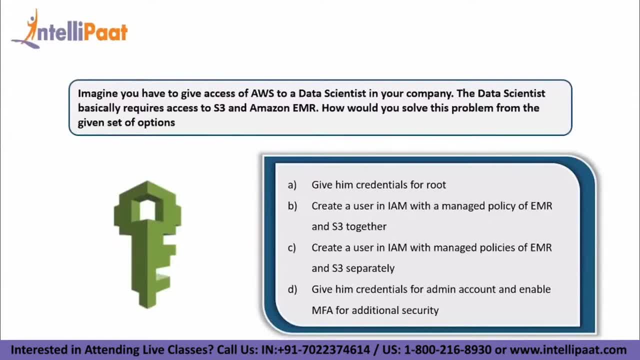 thing is: see needs, change right. so if tomorrow your user says he doesn't want access for EMR anymore, he probably wants access for easy to right. so in that case what will you do? if you had policy in the same document, you would have to edit that document correct. but if you create a document separately, 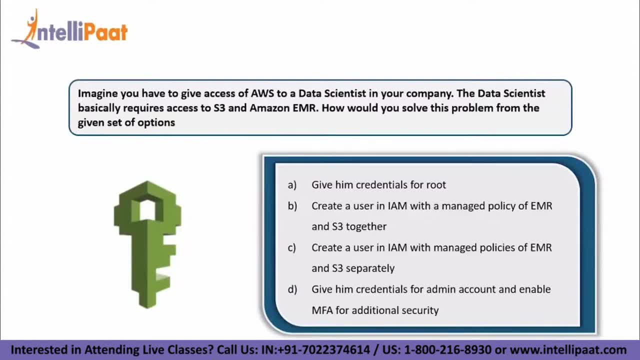 for each and every service. all you have to do is remove the document for EMR and add the document for the other service that he requires. probably easy to you. just add the document for easy to and your S3 document will not be touched right. so this is. 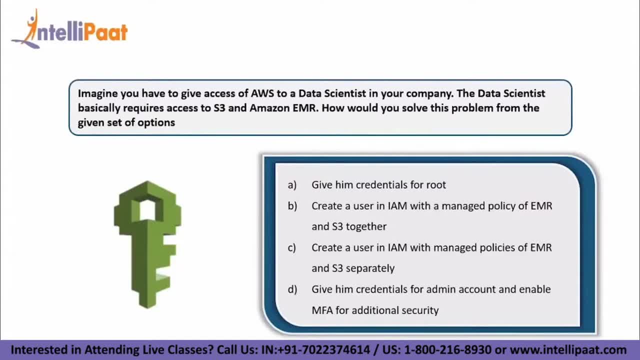 more easier to manage than, to you know, writing everything in one document and editing the code later to give permissions of specific services that he requires. now, right, so that is something that is not much manageable. so the answer for this is: create a user, and I am with a managed 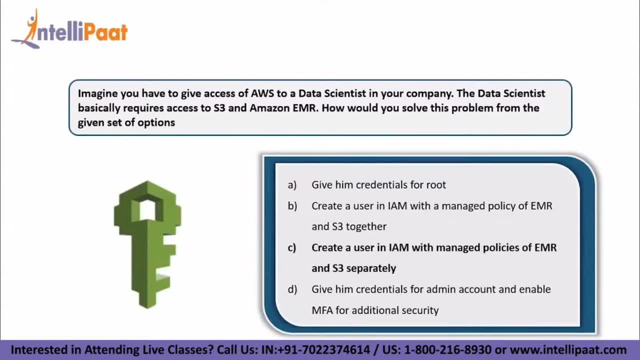 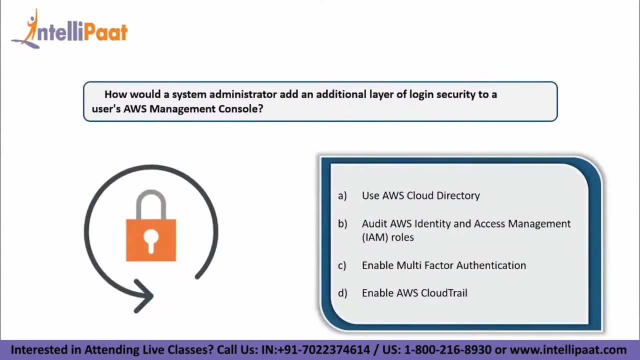 policy of EMR and S3 separately. all right, let's move on to the next question. so how do system administrator add an additional layer of login security to a user's email AWS management console? so okay, so this is a simple question. the answer for this is enable. 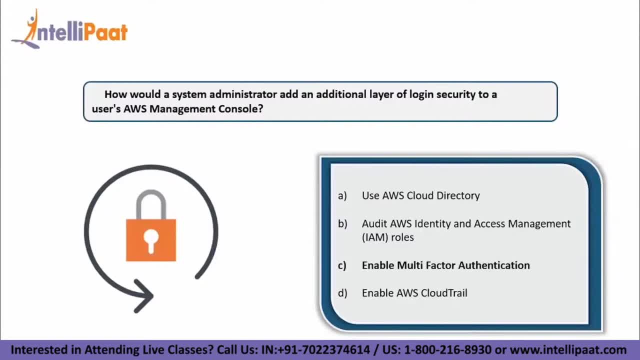 multi-factor authentication. so a multi-factor authentication basically deals with rotating keys. that the keys are always rotating, so every 30 seconds a new key is generated, and this key is required while you're logging in, so once you've entered your email and password, it will not. 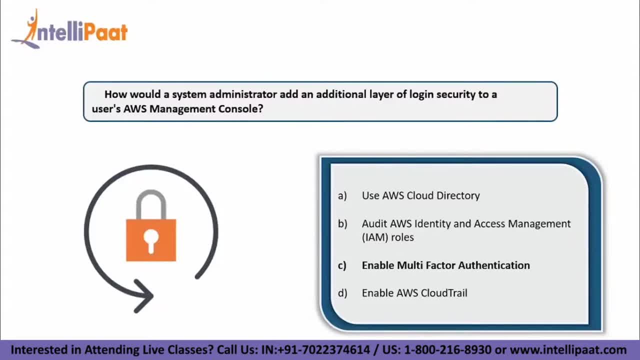 straight away. log you in. it will again give you a confirmation page for a code that you have to enter, which will be valid for those 30 seconds. now, this can be done using apps, so you have a app called. if you have an app from Google, you have apps from other third-party vendors as well, right? so these 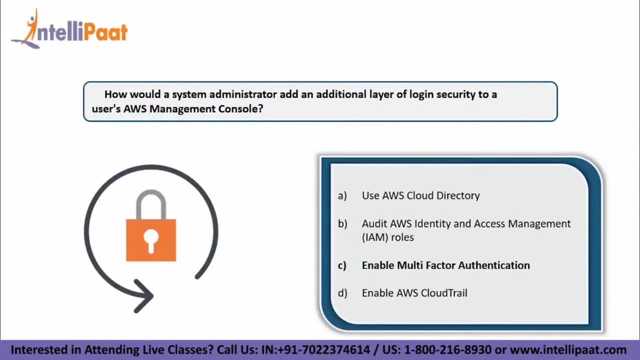 apps are basically compliant with your AWS, right, and you can use them to have access to the keys which are changed at every 30 seconds. all right, so it is better. so if you want to enable multi-factor authentication, then you can do that by logging in, and then you can also enable multi-factor. 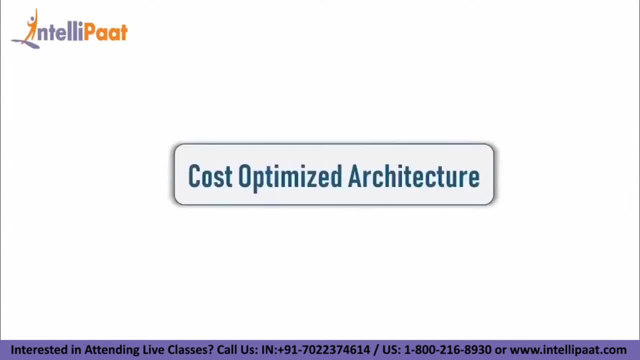 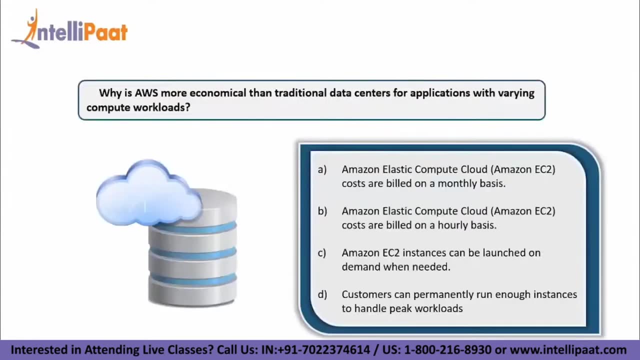 authentication, so this is the best way of adding a security layer over the traditional username and password information that you enter. all right, so our next domain deals with cost optimized architectures, so let's discuss these questions as well. so first question is: why is AWS more economical than traditional data centers for applications with varying compute workloads? 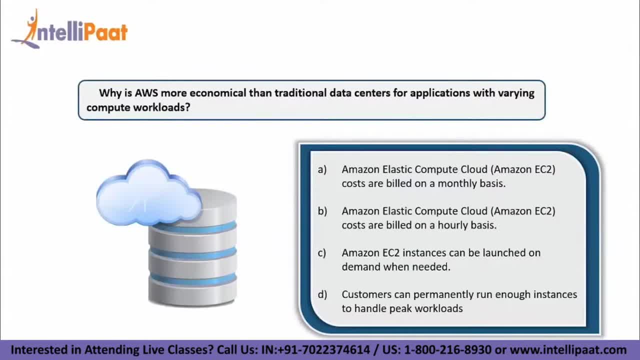 all right, so let's read out the options. so we have Amazon elastic compute costs are billed on a monthly basis- okay. build on an hourly basis, which is true Amazon. easy to instances can be launched on demand when needed. true customers can permanently run enough instances to handle peak workloads. all right, so 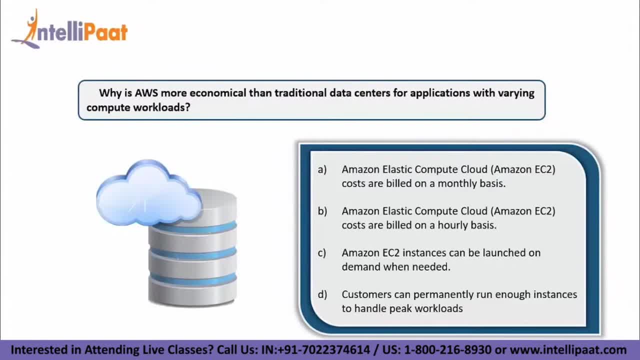 I'll say, because this question is talking about the economical value of AWS, option B and option C are correct. reason being: you're charged according to the hour and at the same time you can have them on demand. if you don't need them after two hours, just pay for two hours and then you can. you don't. 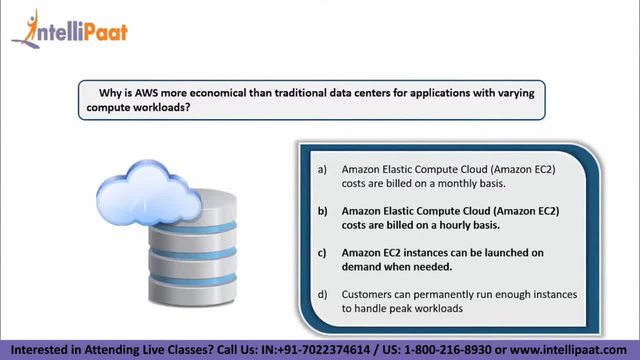 have to worry about where that server went right. so this is very economical as compared to the fact that when you buy servers and their need finishes, say after one or two years, when their hardware gets outdated, so it becomes a bad investment on your part. right, and that is the reason AWS is very much economical. 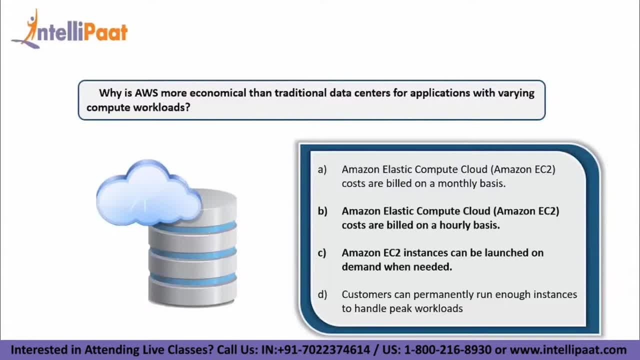 in terms of uh, the reason being that, uh, you know the. it charges you according to the hour and also gives you the opportunity of using servers on the basis of on-demand pricing. all right, so this would be the answer to option B, and option C would be the right answer for this particular. 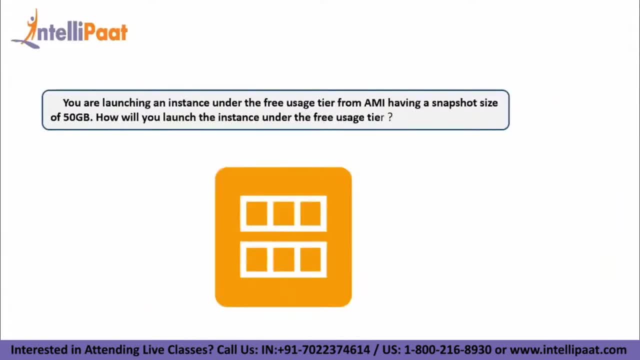 question moving further. uh, our question says you're launching an instance under the free tier usage from EMI having a snapshot size of 50 GB. how will you launch the instance under free usage tier? so the answer for this question is pretty simple: it is not possible, right you? 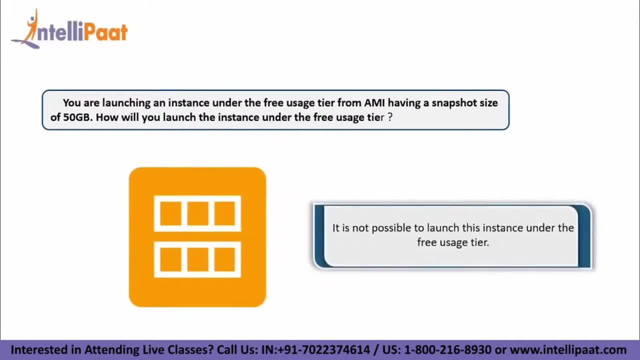 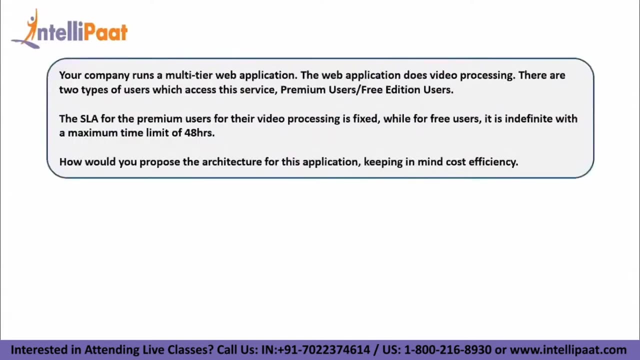 have a limit on how much of size snapshot size you can use. that would fall under the free 50gb, is not. the size is basically a size which will not fall under the amazon free tier rules and hence this is not possible. all right, our next question says: your company runs a multi-tier. 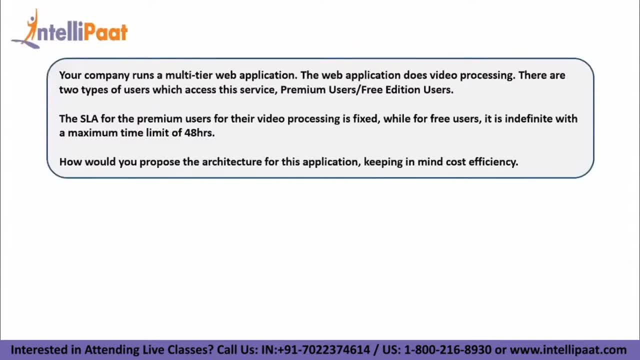 web application. the web application does video processing. there are two types of users which access this service: premium users and free edition users. the sla for the premium users for the video processing is fixed, while for the free users it is indefinite. that is a maximum time limit of 48. 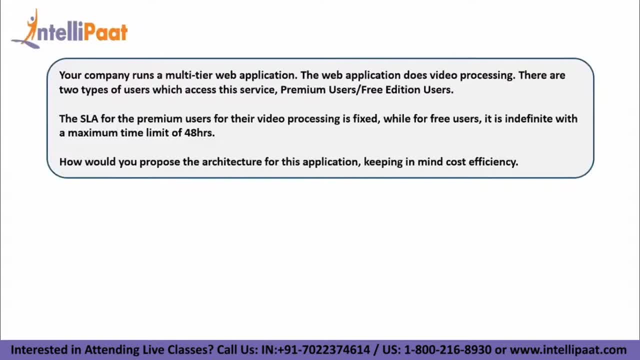 hours. how would you propose the architecture for this application, keeping in mind cost efficiency? all right, so to rephrase this question, basically, you have an application which has two kinds of traffic: one is free traffic and one is premium traffic. the premium traffic has an sla that the 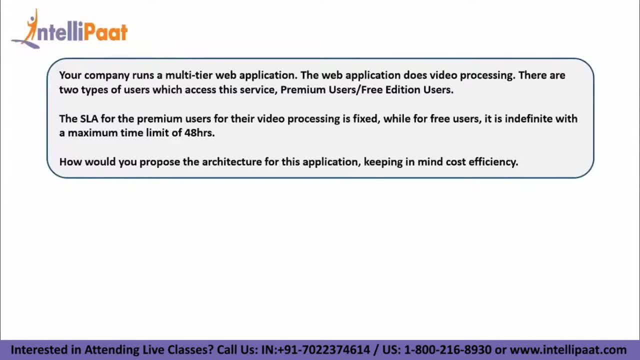 task, say, should be completed in, say, one hour or two hours. the free traffic- they do not guarantee it when it will finish and it has a maximum sla of 48 hours. so if you were to optimize the architecture for this at the back end, how would you design the architecture that you get the maximum cost? 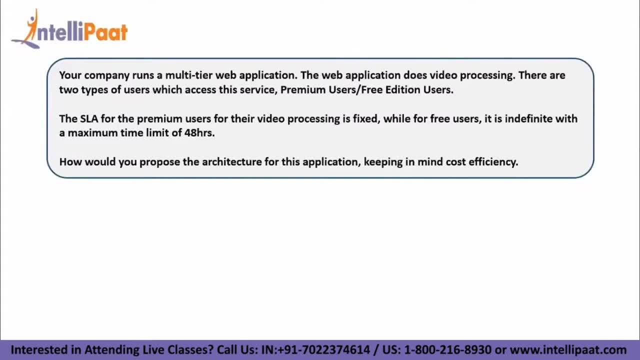 efficiency possible using this architecture. all right. so the way we can deal with it is: there's a thing called spot instances in aws, which basically deals with bidding. so you bid for aws servers in the lowest point of time and you get the maximum cost efficiency possible using this architecture. 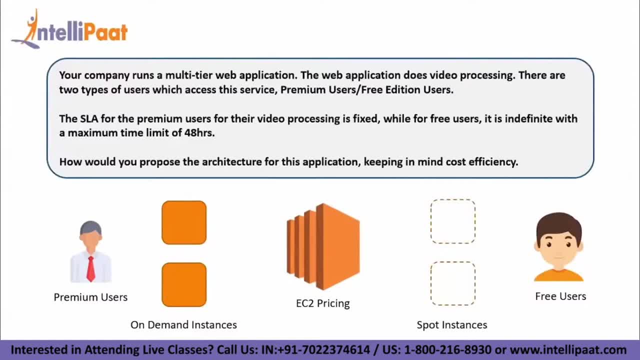 price possible and as long as the server prices are the in in the range that you specify, you have that instance for yourself. so all the free users who are coming to this website can be allotted to spot instances, because there is no sla. so even if the prices go high and the systems are not, 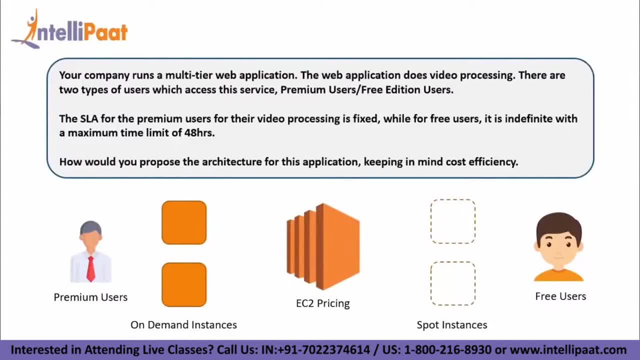 available. it does not matter right. you can wait for the applications for processing if you're dealing with free users. but for premium users, since there is an sla, you can wait for the sla. you have to meet a particular deadline. i would say you use on-demand instances. they are. 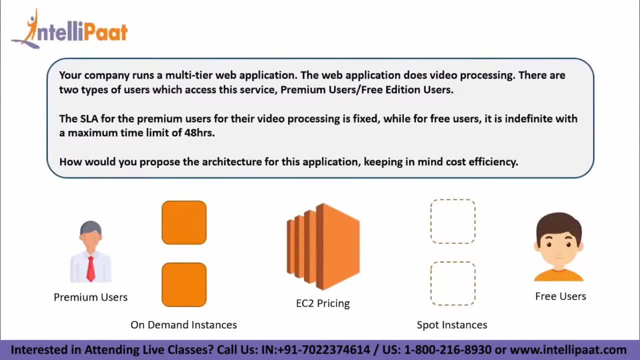 little expensive, but i think, because premium users are paying for their membership, that should cover that part, and spot instances would be the cheapest option for people who are freeloaders or people who are coming free on your website because they do not have any urgency of their work and hence can. 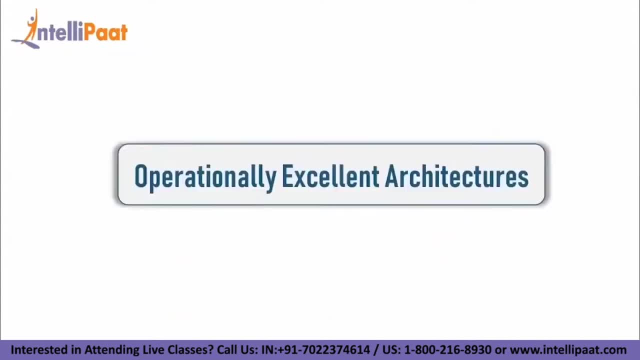 wait, if required, if the prices are too high for you, all right. so our next domain we'll talk about is operationally excellent architectures. so let's see what all questions are covered in this particular domain. all right, so imagine that you have an aws application which is monolithic in 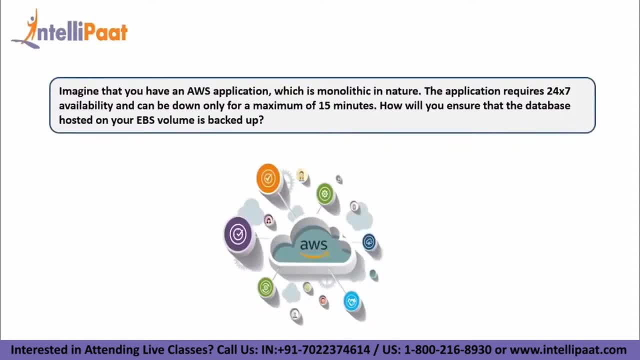 nature. so monolithic applications are basically which do not uh, which, which which have the whole code base in one single computer, right? so if that is the kind of application you're dealing with, it's called a monolithic application. now, this application requires 24: 7 availability and can. 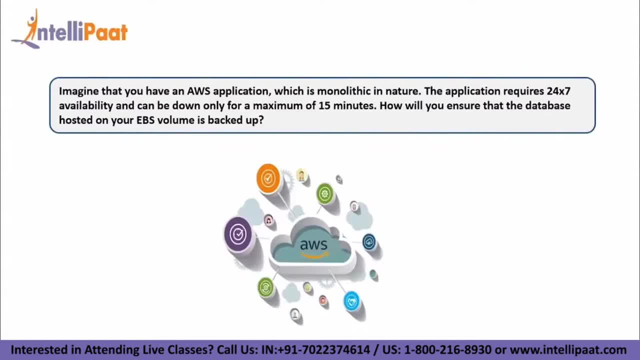 only be down for a maximum of 15 minutes. if had your application been not monolithic, i would say that there would be no downtime, but since it's a monolithic application the question has mentioned, there is an expected downtime of, say, 15 minutes. how will you ensure that the database hosted on your ebs volume is backed up now, since it's a 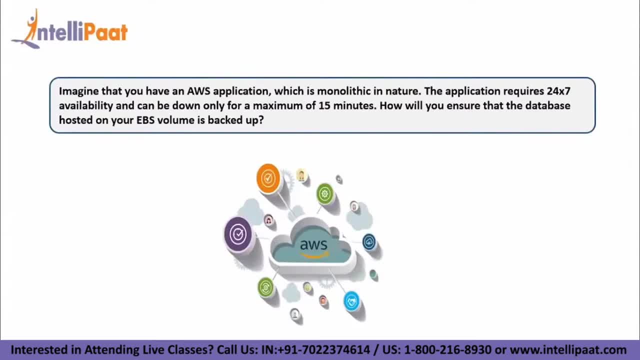 monolithic application, even the database resides on the same server as that of the application. so the question is: how will you ensure that your database is backed up in case there is an outage? so for this answer, i'll say the answer is pretty easy. you can schedule ebs snapshots for. 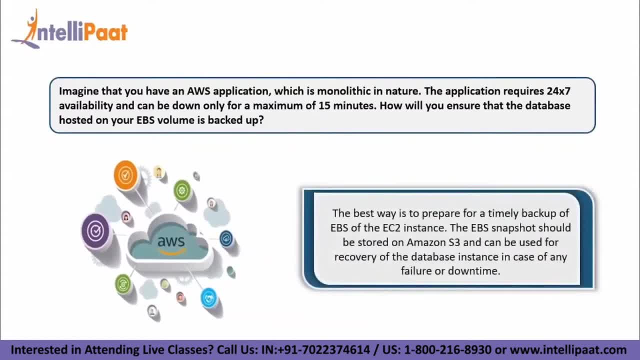 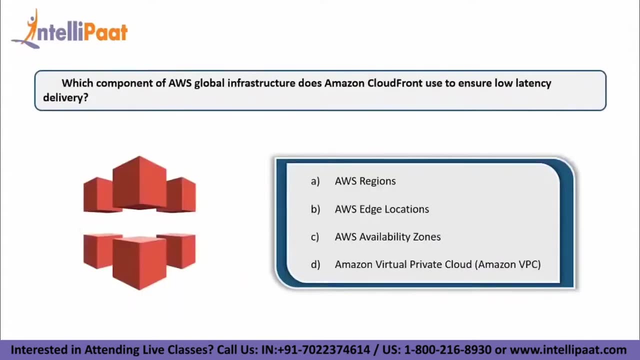 your ec2 instance at particular intervals of time, and these snapshots would basically act as a backup to your database instances which have been deployed on ec2. so hence the answer is ebs instance back snapshots. all right, our next question is: which component of aws global infrastructure does aws cloud fund use to ensure low latency delivery? 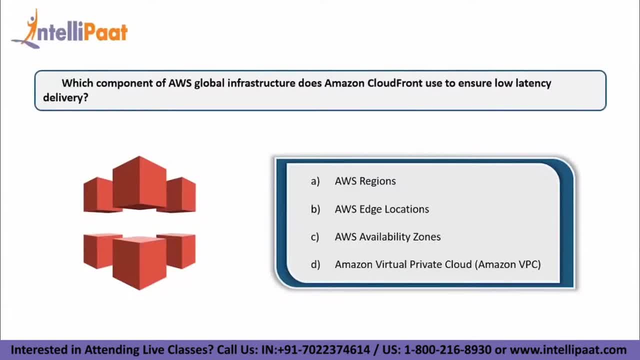 now aws. cloud front is basically a content delivery network, which basically means if you are in the us and the application that you're accessing has servers in india, it will probably cache the application in a us server so that you can access that application faster than to send traffic packets over to india and then receiving them back all right. so this is how. 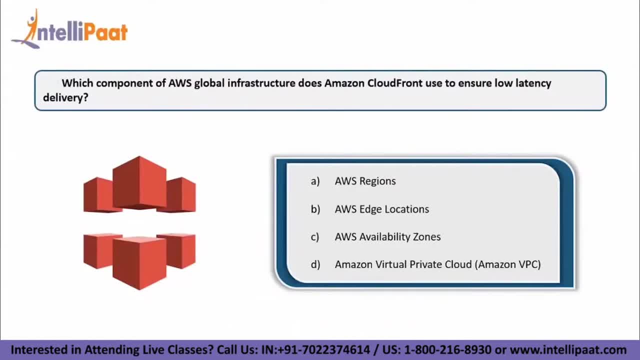 cloud front works. it basically caches the application to your nearest server and so that the maximum latency- sorry, the minimum latency possible and it is possible using aws edge locations- okay, so, as locations are basically the servers that are located to near your, near your place or near a particular availability zone, which basically cache the applications, which. 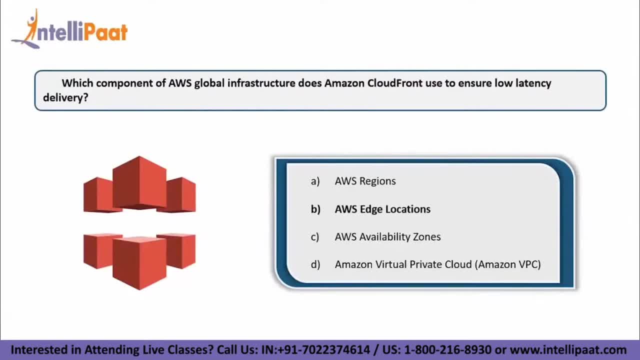 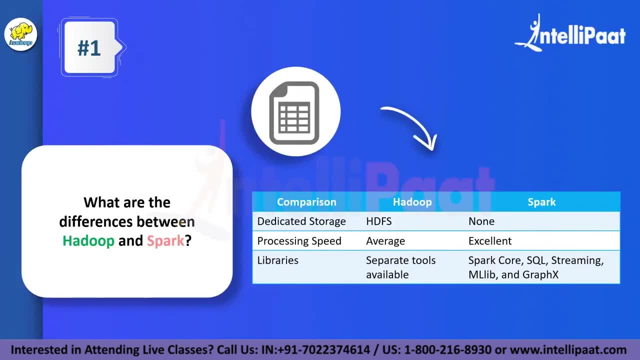 are available in different regions or are at far places. so, coming to the first question on the stop loop interview question set, it is: what are the differences between hadoop and spark? this is a very commonly asked question and it has a very simple answer, to be honest. uh, we'll be comparing. 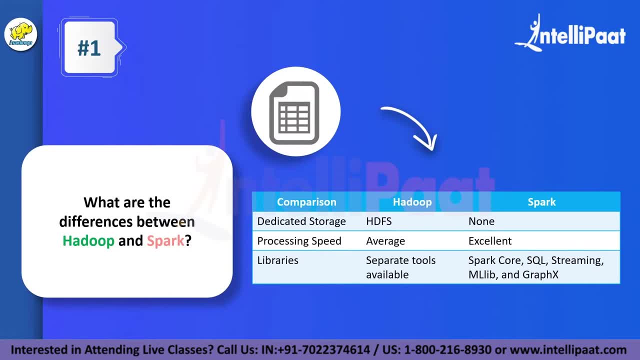 three simple points here. one is how storage is handled in hadoop and spark, the other one is the processing speed and the third one is the availability of libraries. so, in terms of dedicated storage, hadoop has its own file system. right. it has its native file system, called as the. 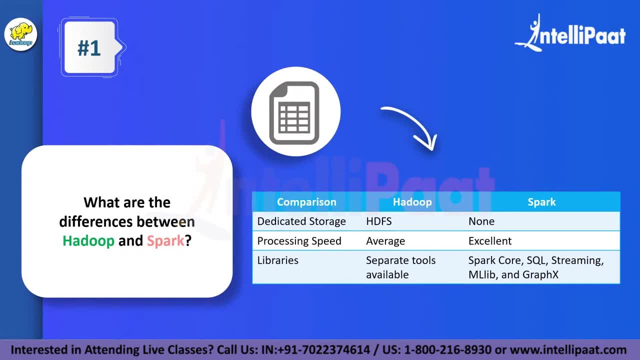 hadoop file system, while while spark lacks a native file system. then you're talking about processing speed. hadoop has an average processing speed. when you compare to uh, you know large amounts of data, because here spark is really very good, uh, at handling large amounts of data without 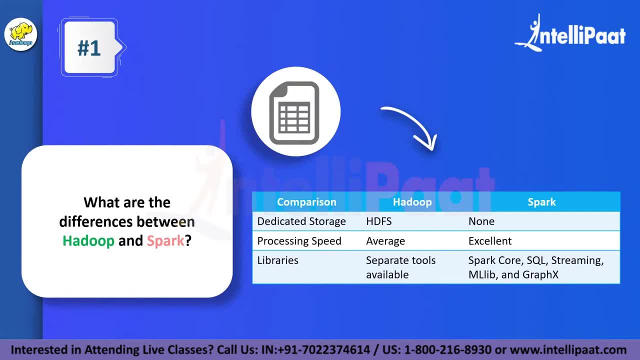 having to do. uh, you know much when you compare it to hadoop. coming to the next point, which is libraries, right, so hadoop has the connection with multiple tools, multiple libraries, and hadoop is pretty much a big tool. but then, when you think about the native availability, where 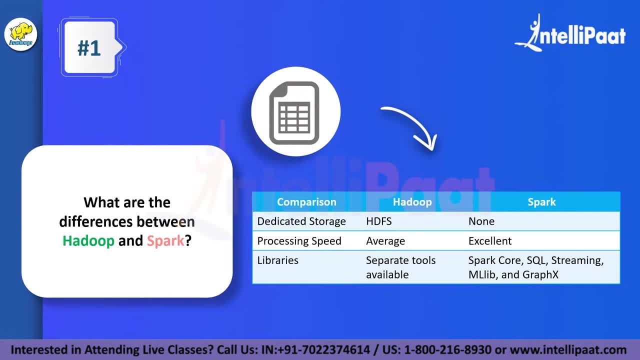 uh, you know a lot of people depend on it. uh, the spark provides the spark core. you have the spark sql, spark streaming, spark graphics, spark ml, liberty- of all of these libraries that come attached with spark. why you will have to learn and integrate these new things in case, if you want to. 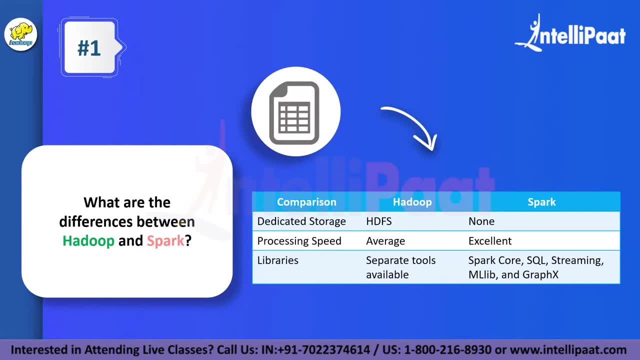 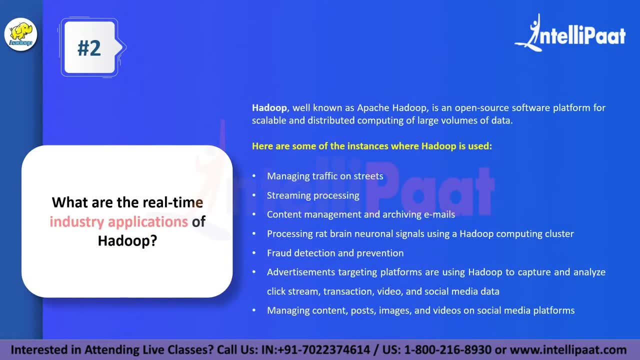 use all of these with hadoop as well, so that extra learning curve in terms of hadoop is required. coming to question number two, it states: what are the real-time industry applications of hadoop? hadoop? as you might know, it is already called as apache hadoop. it's one of the world's most famous 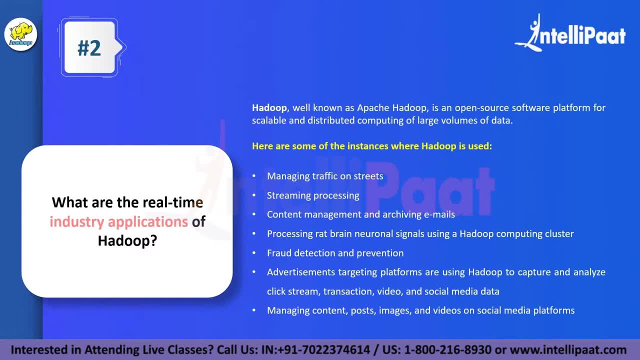 open source program, especially for the world of distributed computing, where we handle, uh, you know, large amounts of data day in and day out. uh, you know, the world generates 2.5 quintillion bytes of data a day, so we needed a solution to handle all of that, and hadoop does just that. so, when you think about the practical applications, 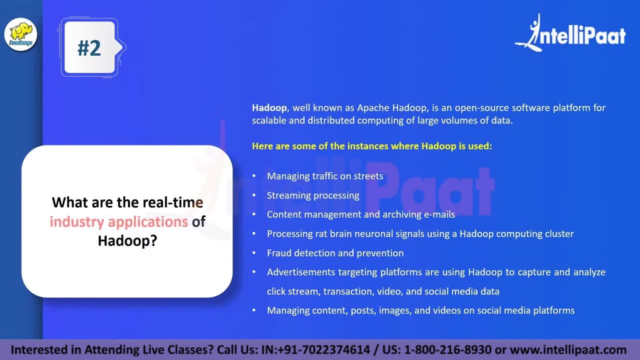 of hadoop all the way from the small scale industries to, you know, handling a little bit of the big boys as well. so think about google, think about yahoo, think about facebook. so all of these guys also have a solution for their big data, because they are generating a lot of data, right? so 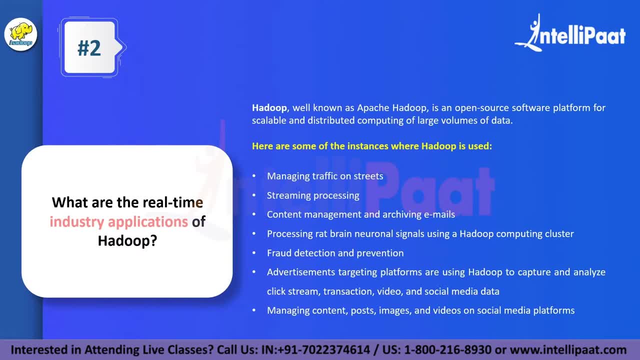 you can use this to do a lot of things, like you know: managing traffic on the street, uh. handling streaming processing- uh. working on content management, how to archive emails, how to save them- uh, you know. working on fraud detection, which is very important in today's world: fraud prevention. 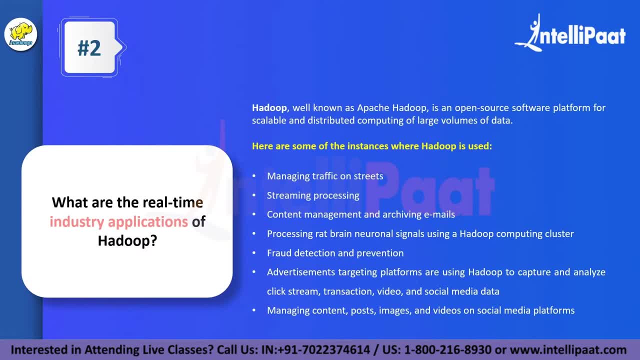 or targeted advertising and guys, uh, you know, you can go on and on and talk about the applications of hadoop for a long time and then make sure to keep your answer concise. uh, do talk about two or three points, or? uh, you know, if you do know some of the applications, then make sure to note at least. 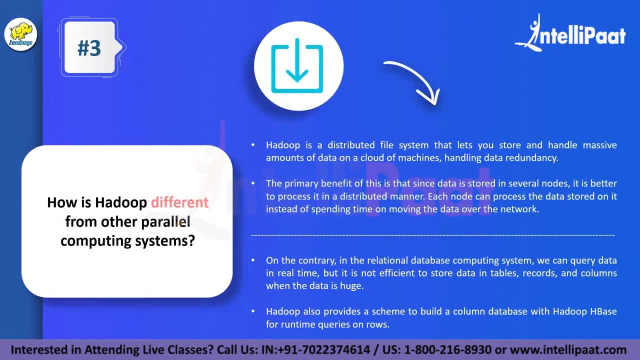 this we can come to the third question that states: how is hadoop different from other parallel computing systems? well, this could very well be the first question through which your interview starts. so hadoop is actually a distributed file system that lets us- uh, you know- handle a large amount. 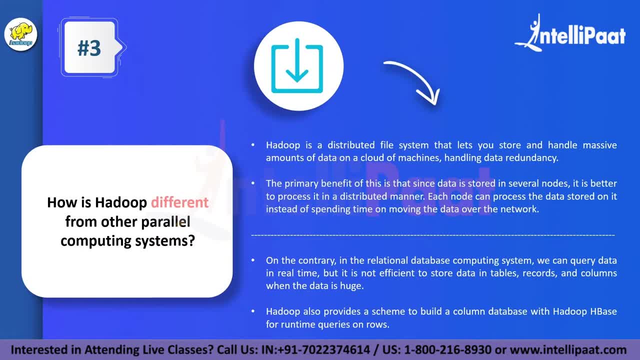 of data, to store it, to work with it on, you know, either local machines, offshore servers or even on clouds as well. so when you think about it, uh, if your data is stored in multiple places rather than on multiple servers, then you can store it on multiple sites, and this is a very good way to 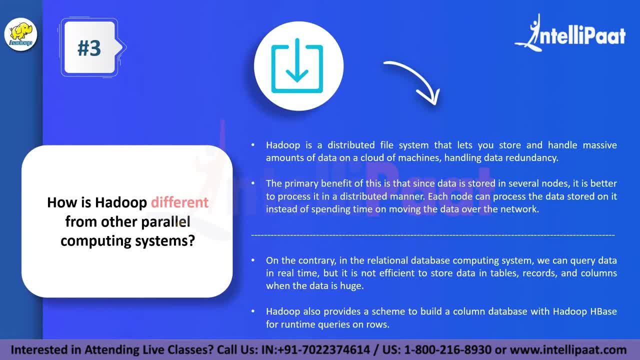 make sure that you know if your data is stored on multiple sites, you can actually use the processing power of multiple machines to actually go on and you know work with your data. so this does not happen in a relational database, because when you think about it right here, so if you have 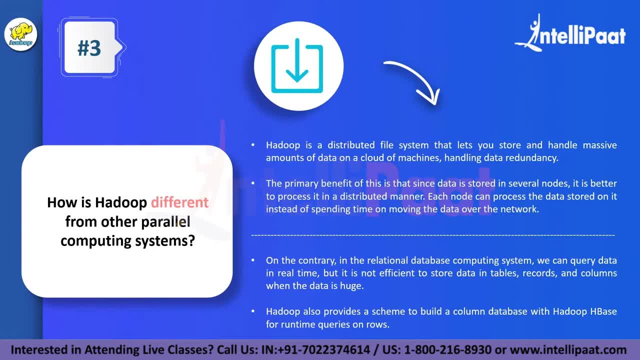 a relational database, you have to query the database. you have to, you know, pick up all the tables, records, columns, and you know, keep in mind that if you have a relational database, you don't have to run it every single time when you think about it. right, you have to, you know. inventory. 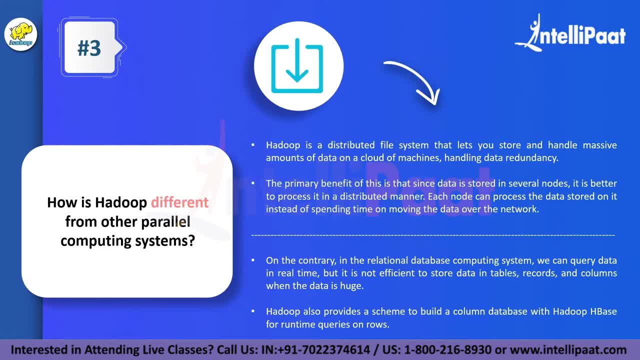 And it'll be a manual task and you really cannot make use of- you know- multiple machines to do this effectively. It is a good enough method, of course, but at the end of the day, it is not as fast as what Hadoop can do. 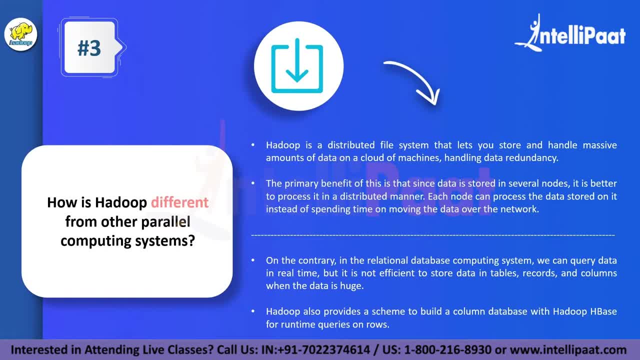 And of course, Hadoop also provides a scheme where you can build your own column databases, And just for this we have the Hadoop HBase. HBase is very similar to SQL And here, you know, we actually go on to run queries on the rows, on the columns, wherever it's required. 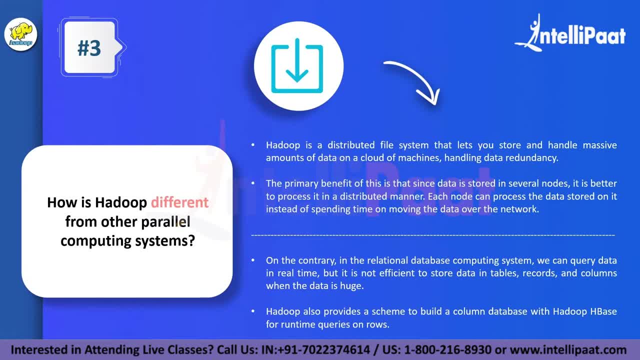 And basically, this is Hadoop's approach to making sure your data storage and access protocols are done easier, And this is how you know Hadoop is different from the other parallel computing systems out there. Coming to question number four, Question number four is a very important one. 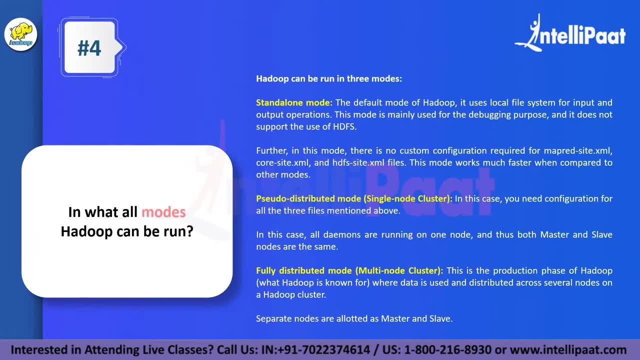 It states: what are all the modes that Hadoop can be run in? Well, it's a pretty simple question with a very straightforward answer. Hadoop can be run in three modes. One is the standalone mode. The second one is the pseudo distributed mode, or what we call as the single node cluster. 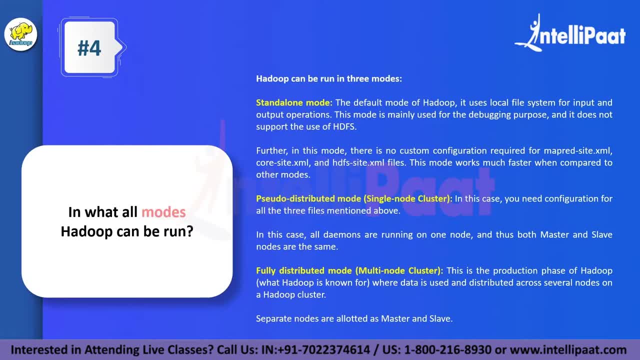 And then we have the fully distributed mode, Which is also called as the multi-node cluster. Coming to standalone mode, Standalone mode is actually the default mode of Hadoop, where it uses the local file system where you're working on for all the input and the output operations. 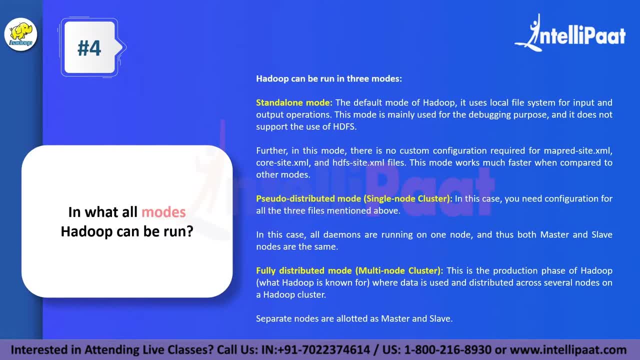 So this is not used popularly in the case of a production environment, but mostly when you're testing or when you're debugging right. So a standalone mode is very important. One highlight you have to talk about when you talk about standalone mode is that it does not support the usage of a Hadoop file system, because it's using the local file system. 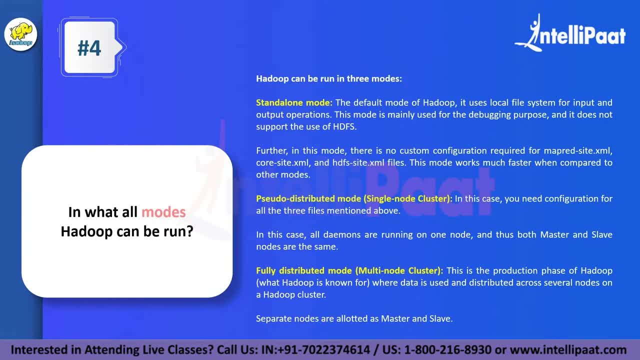 So make sure to mention that. And then when you're thinking about the pseudo distributed mode, right? So what happens in pseudo distributed mode is that you will have to provide three files for configuration. There's the core sitexml, you have the HDFS sitexml and the mapper sitexml. right, 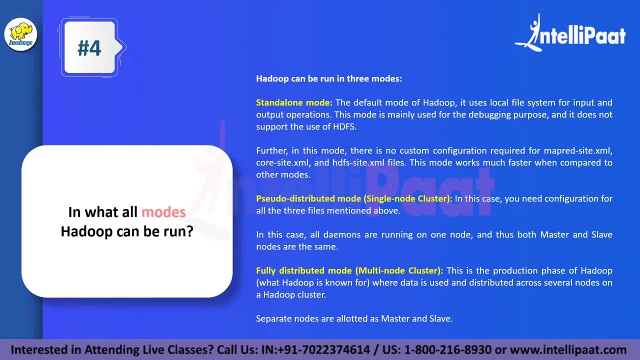 So for MapReduce, for core and for working of HDFS, you have to provide a configuration on which this mode works on. So if you're running on one node, it means that both the node, it means that both. So if you're running 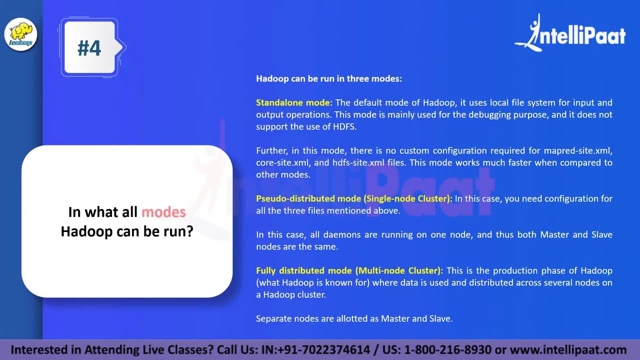 So if you're running pseudo distributed mode on one node, it means that both the nodes are running on one node. So if you're running, So if you're running on one single machine, it means that that machine itself is the master and that machine itself is the slave node as well. 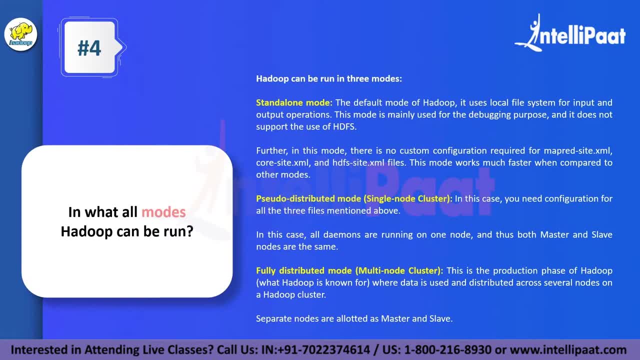 So this is one thing you have to note. And then, coming to the fully distributed mode, Fully distributed mode is, of course, the production phase of Hadoop, where you know, this is where Hadoop is known to be very powerful and this is where it beats all the other tools out there. 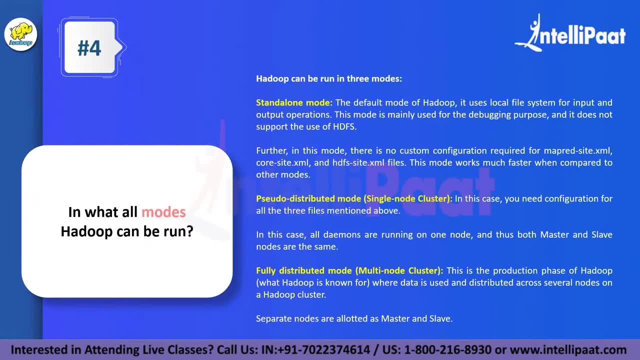 Because here data is used and data is distributed across multiple clusters, multiple nodes, And once you have more than two or three nodes, we call it a Hadoop cluster. And using clusters, you know you, You can have a separate node which is a master node. 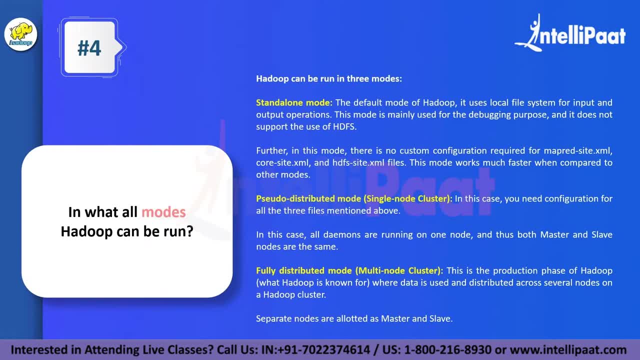 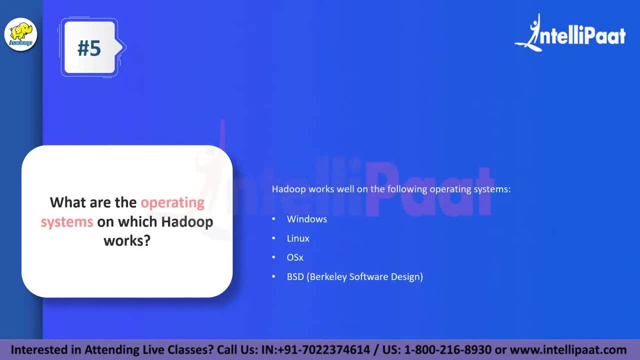 You can assign all the other slave nodes as well, and then you know work with it in a chain of command, in a very structured way. So this is the advantage of the fully distributed mode. Now, moving on to question number five. it says: what are the operating systems on which Hadoop works? 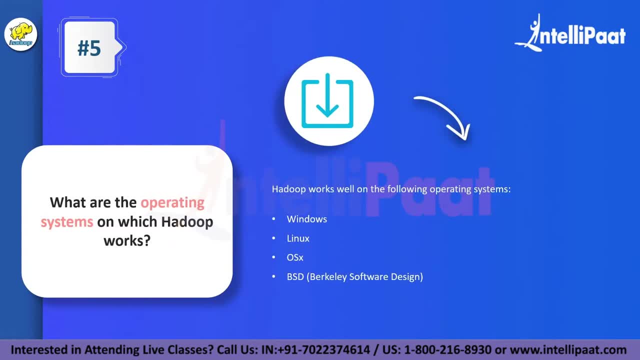 You know, Hadoop supports a lot of operating system. In fact, it's an open source tool and the support for multiple operating systems were being added one after the other. It's mostly preferred to use Hadoop with Windows or Linux, Because 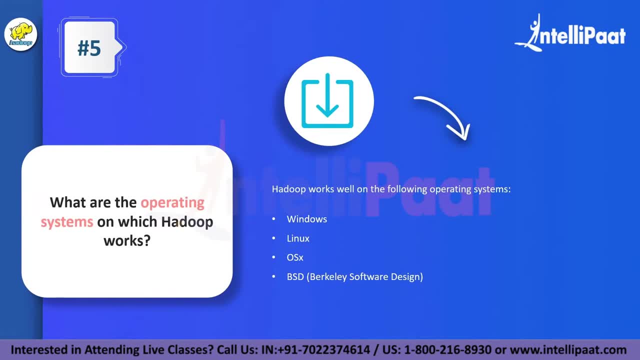 Most of us almost use Windows or Linux, right. But then for the people who are using OSX, for the people who are using Apple's operating system, or let's say even the BSD, which is also called as the Berkeley software design OS, the support for Hadoop is there. 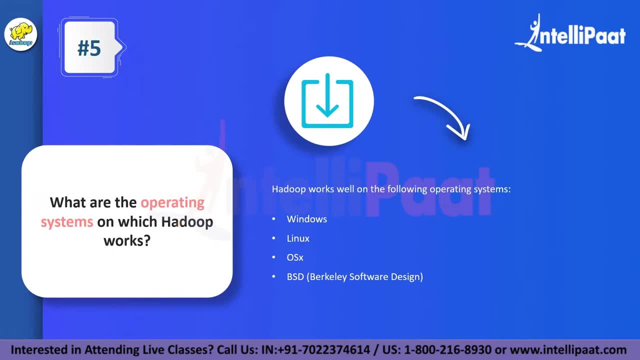 So. so there is a lot of flexibility in terms of what operating system can be used to run Hadoop effectively, So make sure to mention three or four of these when asked. Coming to question number six, it states what is distributed cache. 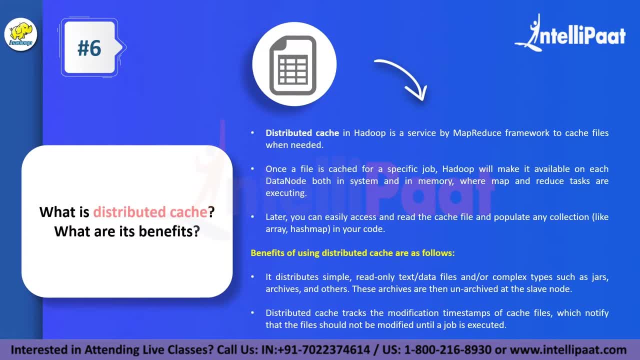 What are its benefits? Distributed cache right In Hadoop is actually a service. So what it does? as the name suggests, it caches files whenever we require it. So let's say there is a file which is cached for a particular job. 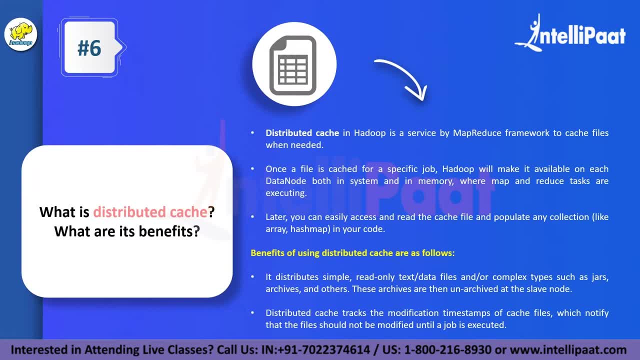 What Hadoop does is that it'll make it available to the data node both in the system memory and the, both in the actual system where it's been accessed from And, of course, in the memory as well, because, at the end of the day, this is where your map operations are happening. 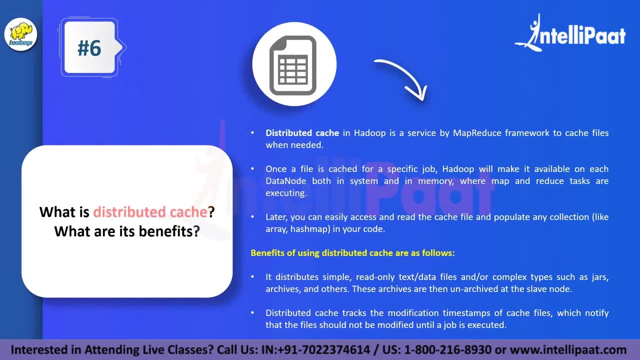 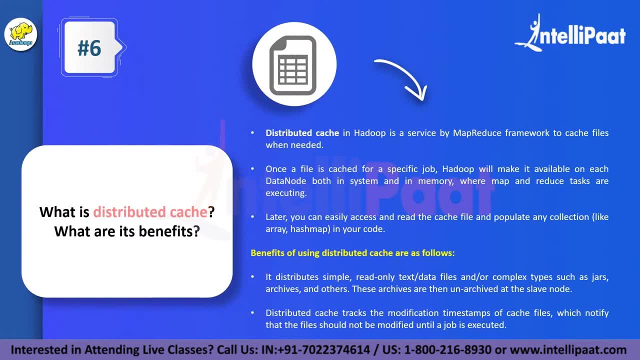 So if you have a caged version there, right. So if you have a caged version there, right. So if you have a caged version there, it's almost like copying it and keeping a temporary sample there where you can use it. 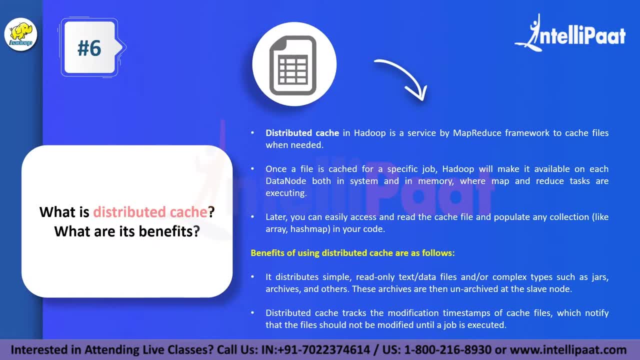 You can populate any collection that you like, right? So think about arrays, think about hash maps and all of that in your code and later use it quickly without having to wait for wait for the pull operation from another node. So what are the benefits of doing this? 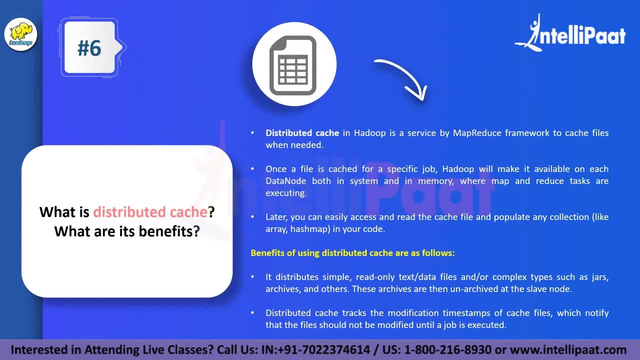 One benefit is that it provides a very simple path of you accessing the data, copying the text file, data file or whatever it is- And it also ensures that there is developer efficiency: Uh, in terms of uh, there is a decrease in terms of access time. 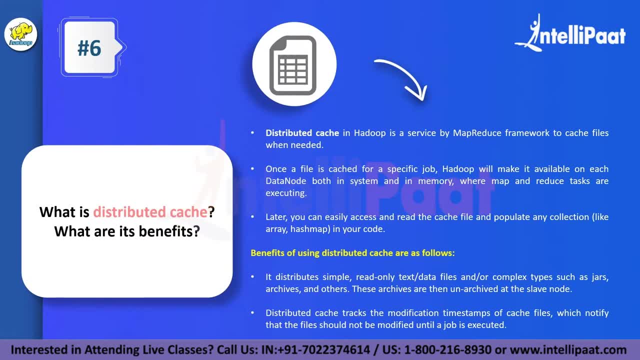 And, of course, what what distributed cage does is that it tracks the modification timestamp for each and every cage file, which means, uh, that you know, the user or the machine or the language itself can have the capability to check if the file has been modified or not. 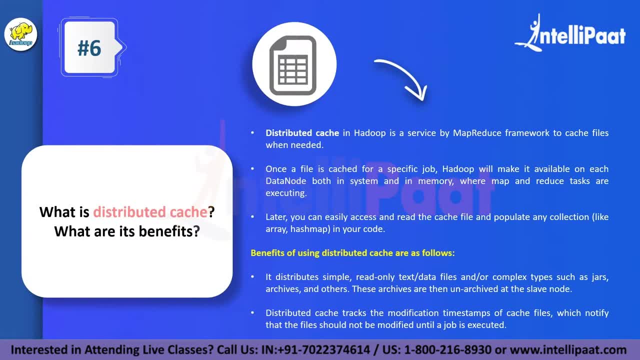 So the general practice is that the file will not be modified until the job is complete, because once the file is changed, it doesn't become a cage file, It becomes a standalone file at the end of the day, because caching is a copy of something. 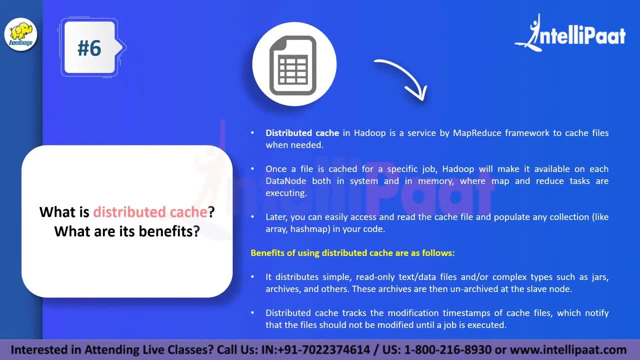 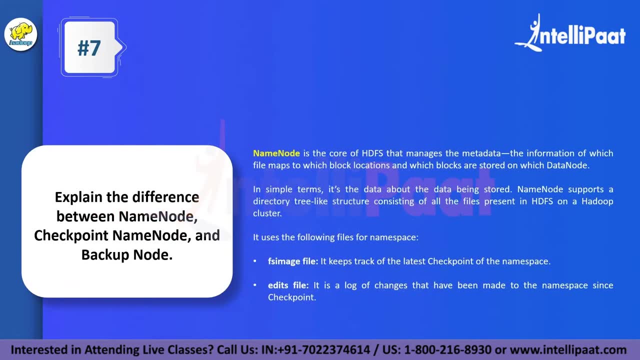 Once you've Copied onto that, it has to remain the same until you work with it, Right? So these are some of the benefits and the working of the distributed gauge in Hadoop. coming to question number seven, This is a big one. 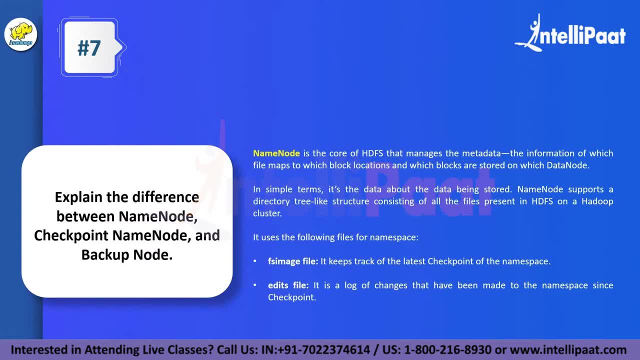 It says, explain the differences between name node, checkpoint name node and backup node. Well, let us check out name node first. I think you would already know this name, Not as one of the most important components, the core components of the Hadoop file system, which is used to handle metadata. 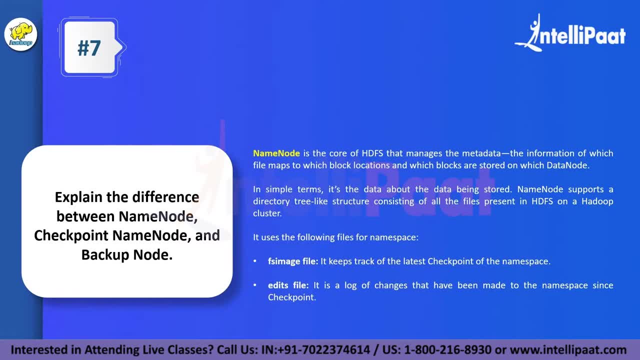 Metadata is what we talk about when we have to describe the Events of files- see, uh, files will have certain information- but then to describe what information these files has. that is exactly what metadata is. So, uh, what we're doing with name node is that we're trying to map all of these files using metadata to check where the block locations are, what blocks are located on which point in the data node right. 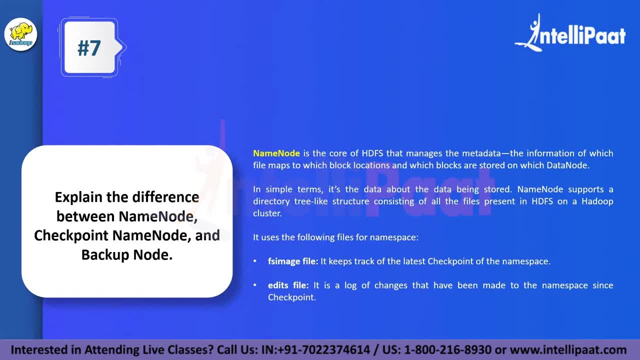 So what we're trying to do here is we're trying to understand and map away on which, uh, you know, think about a tree structure, right? Think about a directory structure where we have all the files arranged one after the other in the Hadoop. 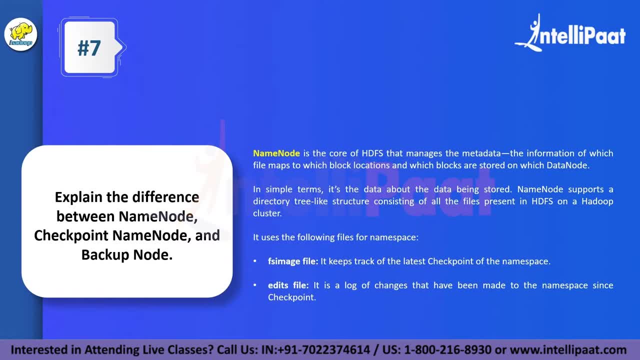 Cluster. Uh, that's the exact purpose of the name node. So to do that we'll actually require- uh, you know- two files. One we have the FSMH file. It's used to check the latest checkpoint of the namespace. 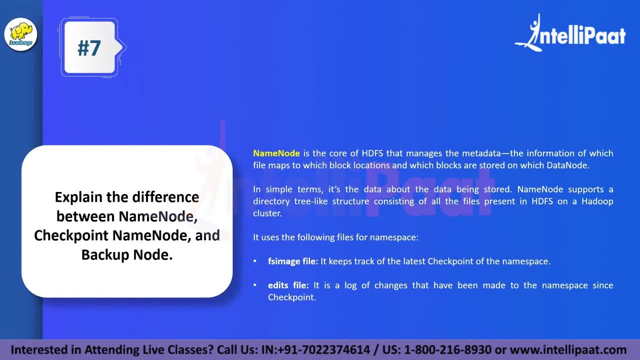 And, of course, we have the edits file. Uh, edits file will give you a log of changes that has been made after the checkpoint has been achieved for every single namespace entry, Because, at the end of the day, whatever changes you do, minor or major, it is very, very important that you keep it in check. 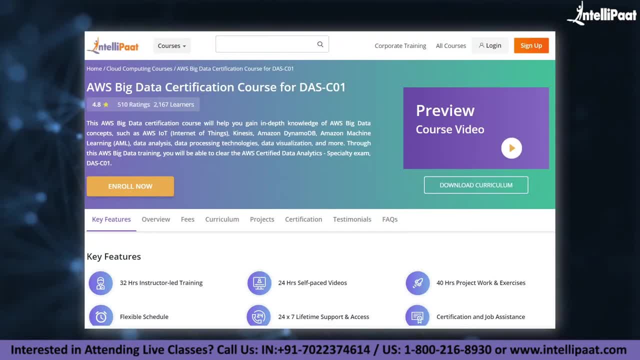 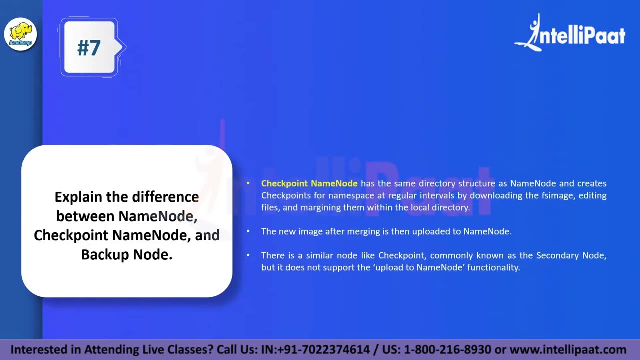 This is name node. Now, just a quick info, guys. Intellipaat provides AWS big data certification codes, mentored by industry experts, The course link of which is given in the description below. Now let's continue with the session. Let's talk about checkpoint, name node. 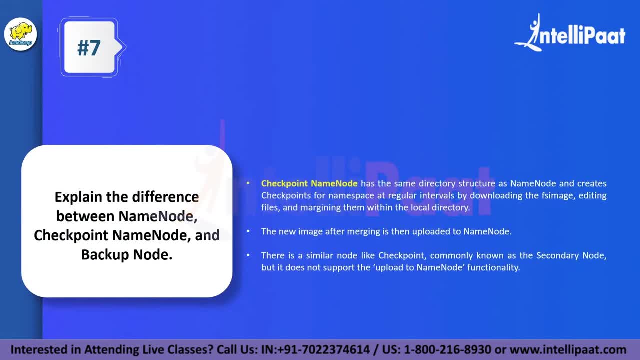 Checkpoint name node is basically very similar to what name node does. And here what we're trying to do is we're trying to create checkpoints for name nodes at regular intervals rather than in randomness. And here, by doing this- uh, you know, what we have to do is if you download the FSMH, you have to edit all the files. 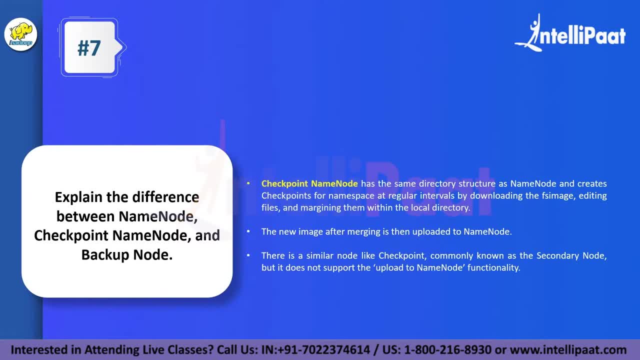 And later, after editing, what we'll do is we'll merge these files into the local directory And after this we'll have a new image, And the new image, after being merged, is basically uploaded to the name node. So, after these checkpoints, after analyzing them, after editing the files, after merging them, is when we created and uploaded it to the name node. 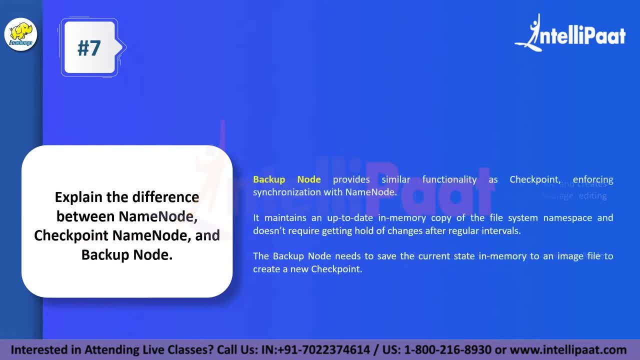 So so this is the checkpoint name node. And then now when we talk about backup node, right, So backup node basically provides the functionality, is very similar to checkpoint, But at the end of the day, here what you're trying to achieve, 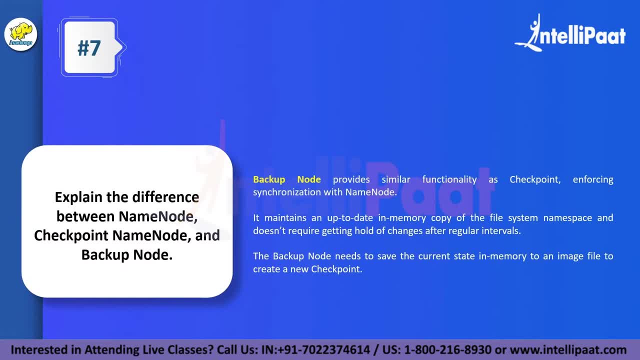 to do is we're trying to achieve a synchronization with the particular name node. uh, it is very vital, as i've been saying that, uh, you know, your file should be up to date. your file should have an in-memory copy. it should not differentiate from each other when it's being cached or when it's. 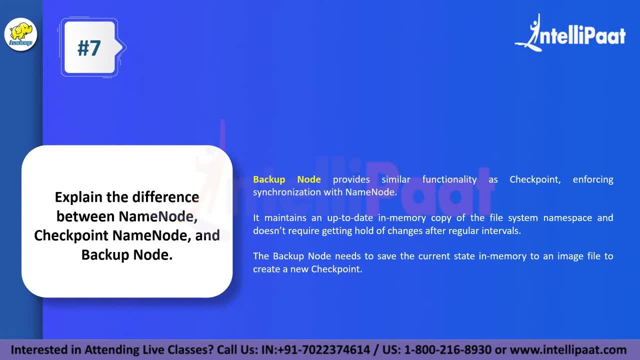 a copy or anything like that. so backup node needs to save the current state in a memory, to an image file- uh, you know, to create a latest checkpoint file as well. so this is what a backup node is. so this is the basic difference that lies in between name node, the checkpoint name node, and 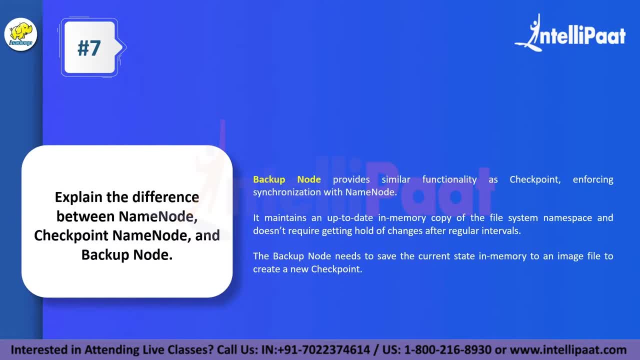 the backup node. so when you ask this, make sure to put the answer out in a clear and a concise way. and, uh, you know, whenever you're answering questions regarding nodes, name nodes and uh, especially data and roads, things get a little messy, right? uh, make sure you put the answer out. 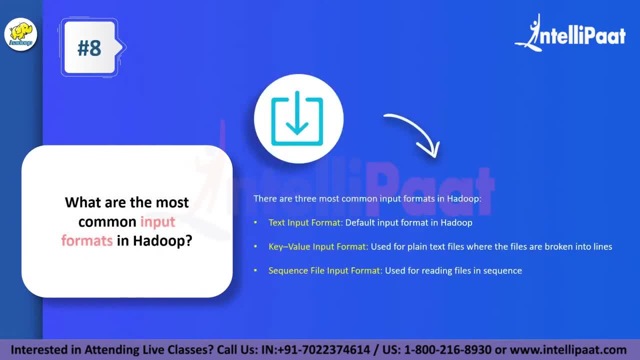 uh, in a very structured way. now, coming to question number eight, let's say it's: what are the most common input formats in hadoop? well, there are three common input formats in hadoop that you should know about. one is the text input. we have the key value input and, of course, we have the 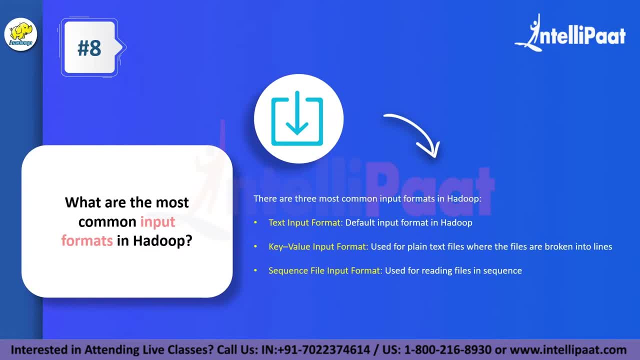 sequence file input. so the default mode, right. so you can have another question here that says: what is the default input format? in hadoop it's actually the text input format. that is the default format, and then we have the key value input. so the key value input format is used for plain text files. 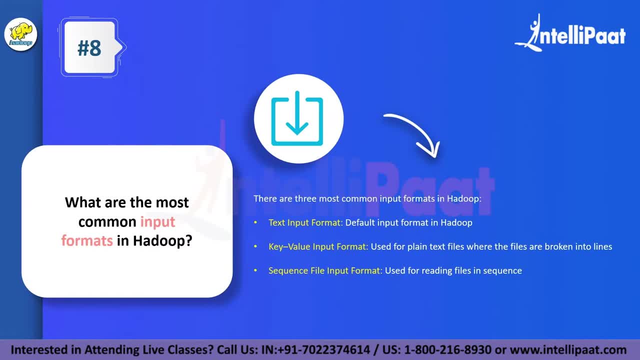 where the files are actually broken down into lines and later used. but in the case of sequence file input, here we make use of this particular format to read all the files in a particular sequence as per requirement. So these are the three common input formats in Hadoop and you have. 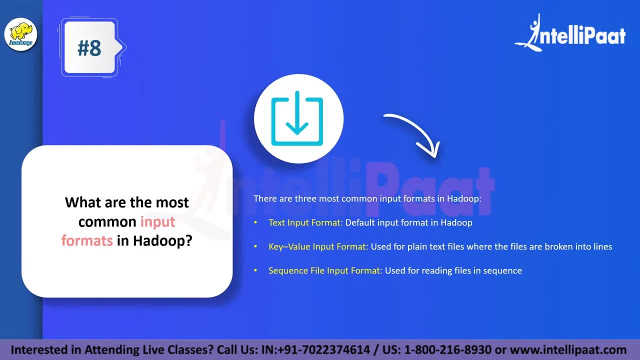 to stay in order, It really doesn't matter. The default one is the text input, and talk about key value inputs And, of course, how you'll be reading files in a sequence using the sequence file input as well. So with this we can come to question number nine. that states define data node. 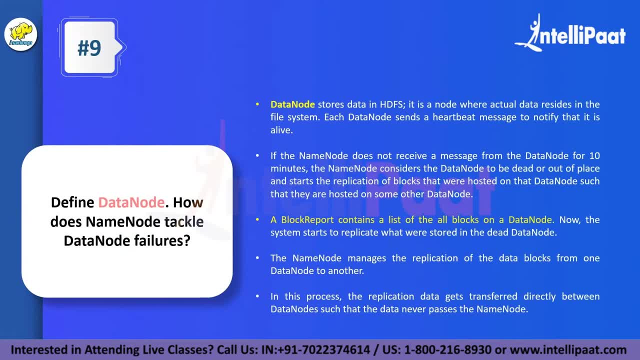 How does name node tackle the data node failures? Well, the name node we've already seen right, But what is data node? Data node is where the data actually gets stored in the Hadoop file system. The data actually resides here in a way where it has the capability to communicate with the 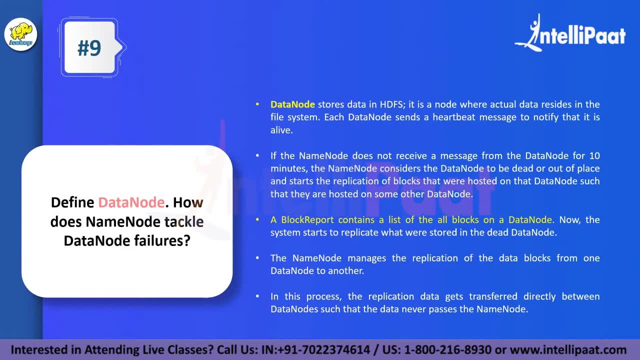 name node. It does this by sending a message called as the heartbeat message. The heartbeat message, literally, is to show that it is alive and that it is working. So what happens is that we have ten-minute integrals and in these ten minutes, if the name node does not receive a 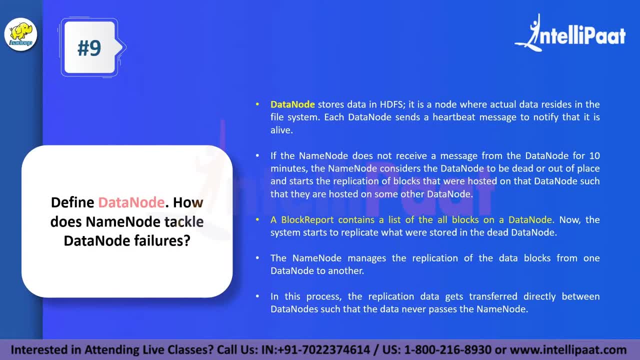 message from the data node: right. So the name node is waiting for the data node to send a message In 10 minutes. so two examples I'm going to share. you know we have a request which says no, we're going to close what you really did to send a message. So I mean actually output test. 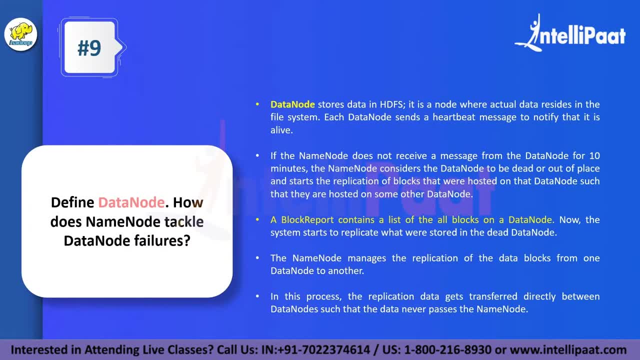 minutes if it doesn't send a message. what the name node thinks is that the data node is either dead or it's out of place or it's not working fine, and the name node actually starts replicating the blocks which are hosted on that particular data node which wasn't responding, and it takes that. 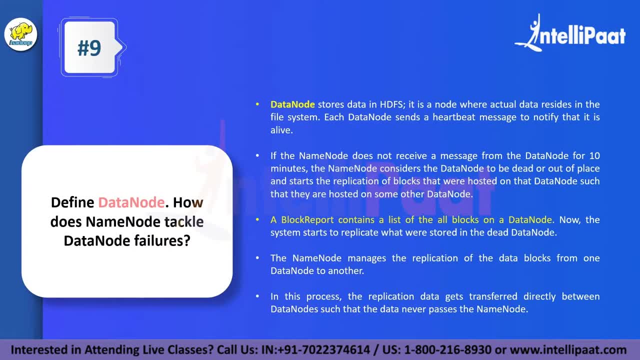 and pushes it on to another data node to make sure that the data replication and data redundancy part of it is maintained well as well. so this is how actually name node tackles data node failures, but then to denote the failure we have something called as a block report. a block report is 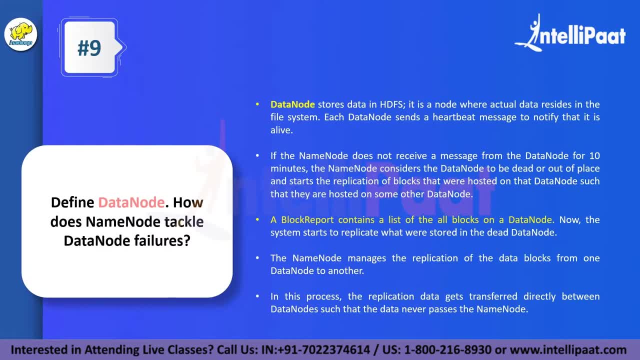 actually consisting of all the lists of blocks that are present on a data node. so whenever the system starts to replicate it right, uh, you will get to know what data was stored in the data node and what data needs to be moved. so this replication of data to, uh, you know, moving from one data node, 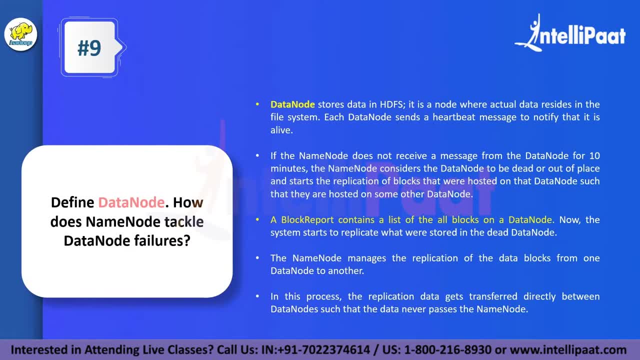 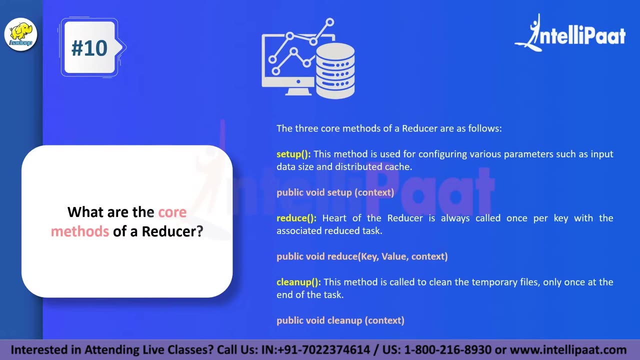 directly into the other by keeping a track, uh, you know, under the name node, by making use of a heartbeat message. this is something which is very important and this is how you know communication happens between the data node and the name node. with this we can come to question number 10. uh, that states what are the core methods of a reducer? well, there, 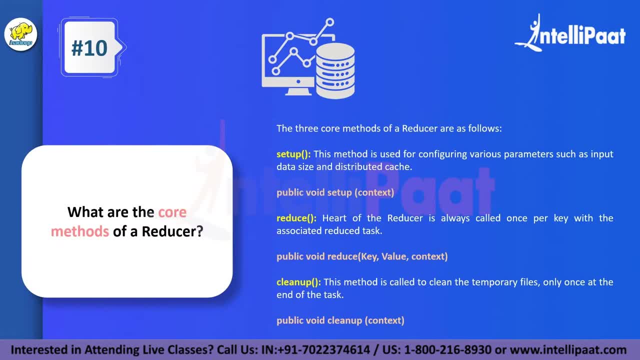 are three core methods. uh, you know, whenever you're talking about a red user. one is the setup. uh, we have the one of the setup method, we have the reduce method and, of course, we have the cleanup method. talking about setup method, setup method is basically used to configure all the parameters. 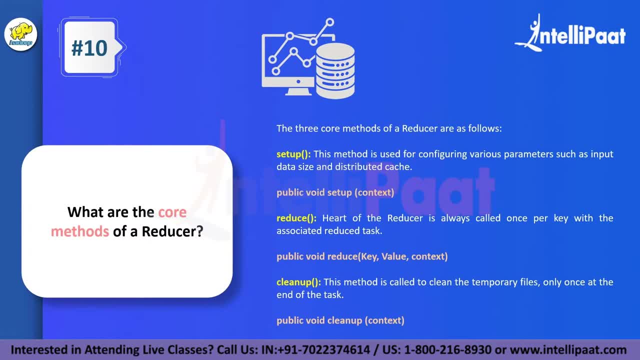 that we have that we have to feed into the network. see, you have the input data size, you have the distributed cache and all of these parameters, right? so to do this, uh, you know you can use public void context as the- uh, you know- parameters to send it in. but then when you talk about reduce, reduce is 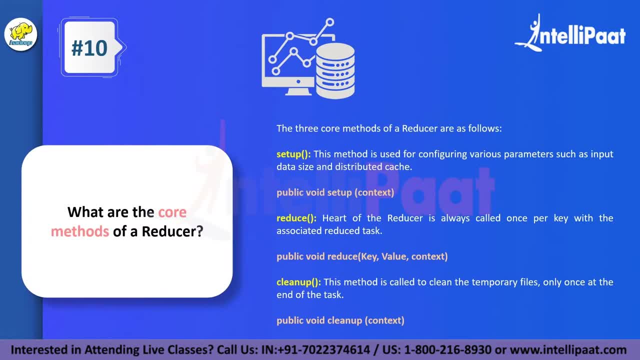 the most important part of the reducer right. as the name says, it is the heart of the reducer. so every time there is a new key that's generated, the reducer is called once with that particular task, the key is given to it, the value and the context is added where- uh, you know this method can run the 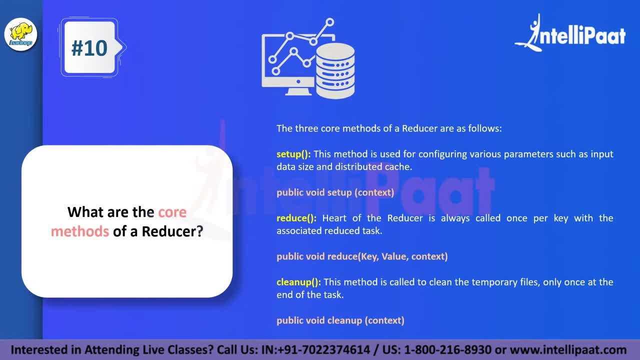 reduction operation and be done with it as well. and then we're talking about the cleanup method. the cleanup method, as the name says it again, is pretty simple. it is used to clean all the temporary files once a task has ended. so you will have certain files which are required to perform the 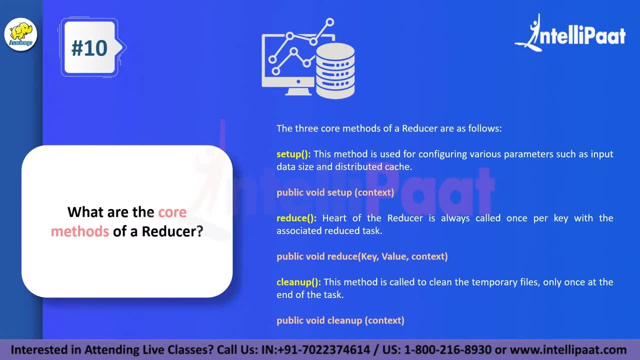 reduction operations, but then, as soon as the operation is done, you will not require them anymore. so in that particular case, it is vital that you keep cleaning the memory then and there to keep it effective. right cleanup method does just that now. uh, do take a look at the syntax. 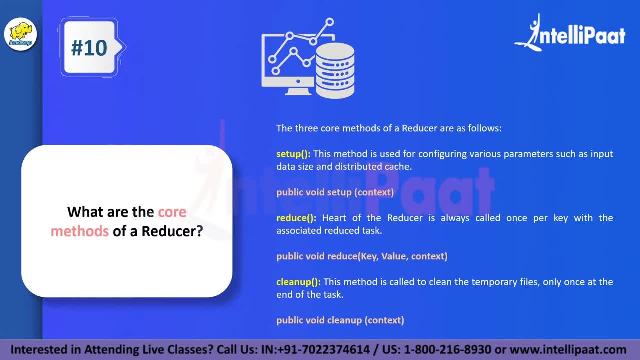 now, do take a look at the syntax and if you have a pen and paper in front of you or your computer in front of you, do make sure to put that down to showcase to the interviewer that you actually have worked on this or that you know it in detail. 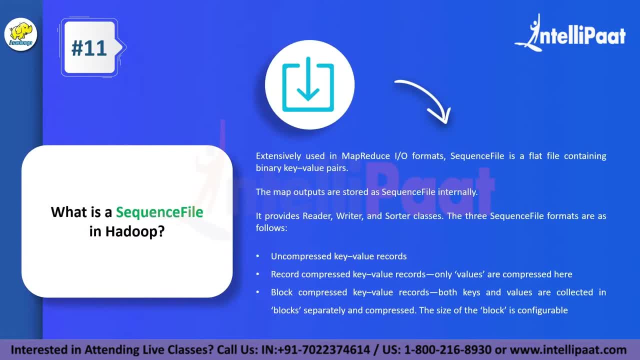 now coming to question number 11. it states: what is a sequence file? in hadoop, a sequence file is basically a flat file. uh, you know, in hadoop so whenever we're talking about flat files, especially here in the case of sequence file, it contains binary key, value pairs and you. 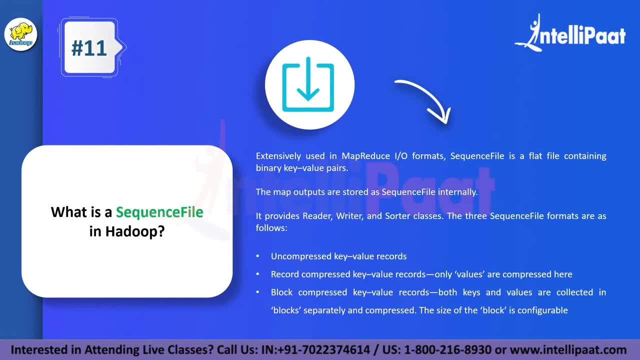 know, we have the map inputs, we have the map outputs, where, uh, the map output actually gets stored, uh, you know, as a sequence file internally here itself. so if you're thinking about, what classes does this uh sequence file provide? it provides you the sorter class, the reader class. 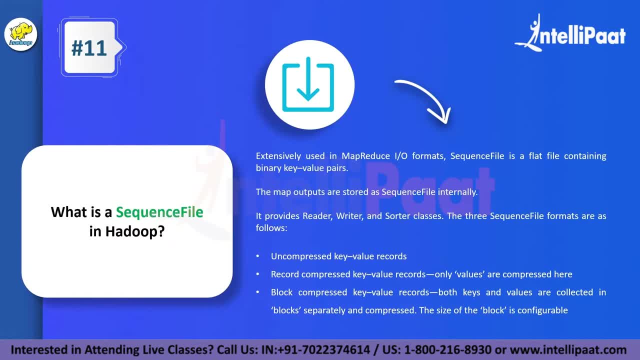 and each of these file formats right. so there's actually three formats that you need to know about. one is the uncompressed key value records. then you have the record compressed key value records, where only the values get compressed. and then you have the block compressed key value records where, uh, you know, it's not just values here, but both the key and the value gets collected. 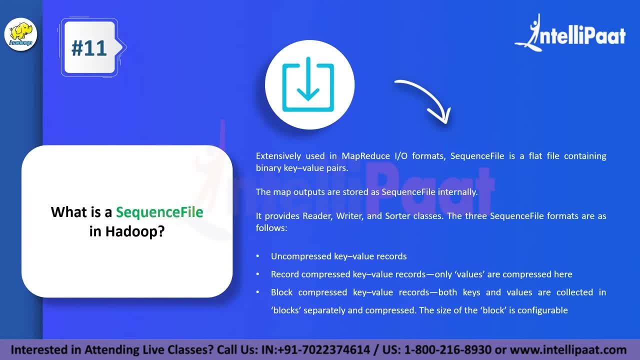 in separate blocks and compressed and the size of these blocks. right, this is assignable to you. so having it uncompressed, compressing only the values or compressing both key and value in the case of sequence files are valid, very important. so these three classes in the binary key value pair- uh, you know, see a lot of. 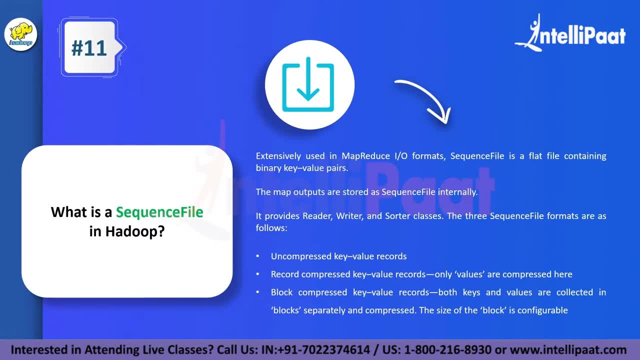 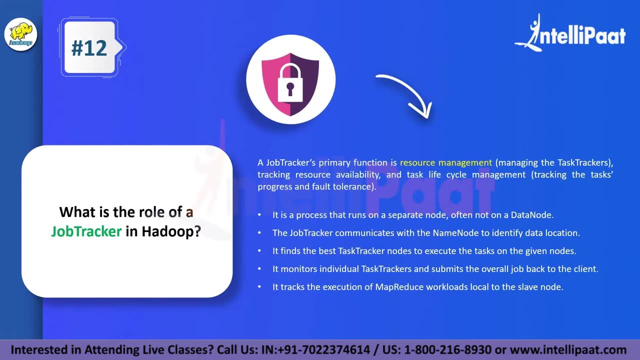 usage in the daily world. so it is very vital that you answer this like that. next, coming to the 12th question, it states: what is the role of a job tracker in hadoop? job tracker, as the name suggests. again, its main function here in hadoop is to basically handle resource management. so we have 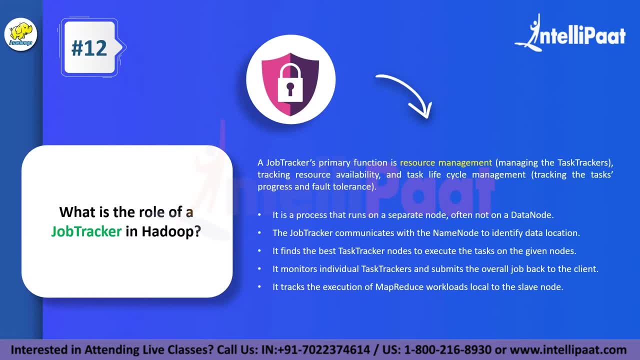 something called as task trackers, where the job tracker actually handles and manages the task trackers. so you'll be checking for our resource availability. it will be checking for task life cycle management. it will be understanding about what's going on in terms of fault tolerance, in terms of the tasks, progress and much more so. 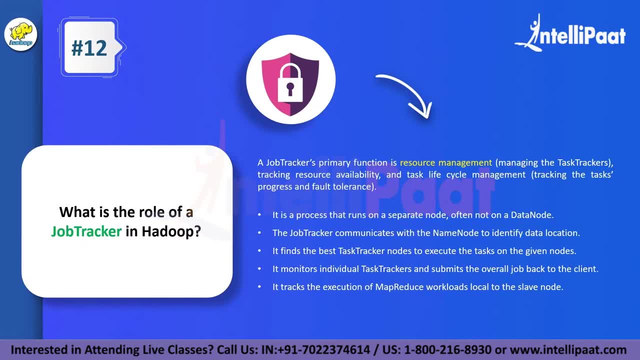 there's a lot of things, uh, that the job tracker does in hadoop, right? so there's basically a process that runs on a separate node and not on a data node, and this is, this is a very important point that, uh, you're supposed to mention- and then, of course, the job tracker communicates with the name. 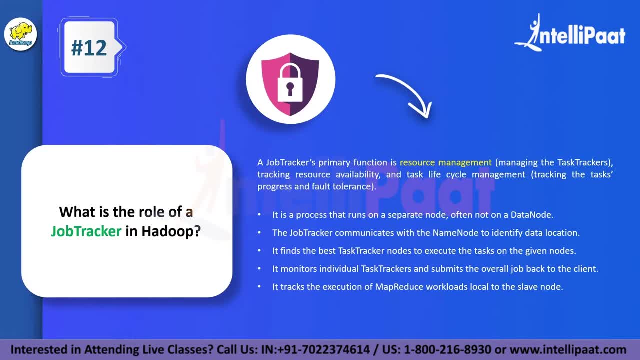 node to identify the data location, and if it finds the data, then it will execute the task. uh, if it finds the data, then of course it goes into redundancy. but then one important thing is that it will monitor all the individual task trackers and submit your overall job back to the client. 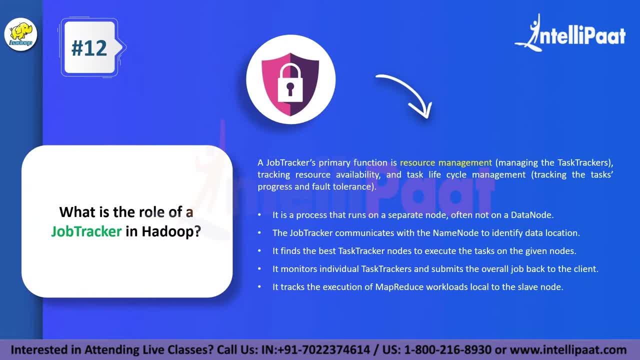 it's like, hey, it takes in all the data, it works with, it executes all the tasks and sends it back in a structured way. so what it does is that it also tracks the execution of the map: reduce workloads, the operation and the tasks are, you know, local to that particular slave node and creates a file. 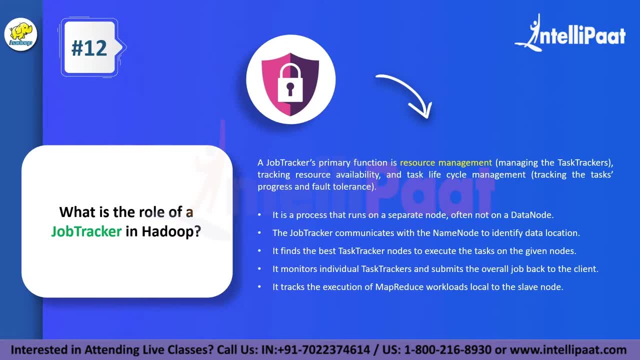 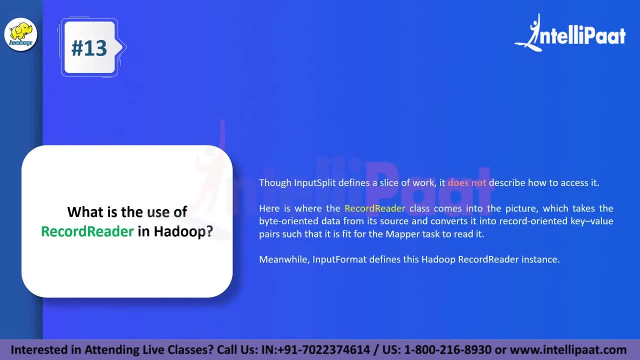 where you can track that as well. so in terms of what job tracker does is, it does a lot of things very effectively. that's the important part here. coming to question, number 13 says what is the use of record reader in hadoop. so when you think about it, we have input split, right. so input split. 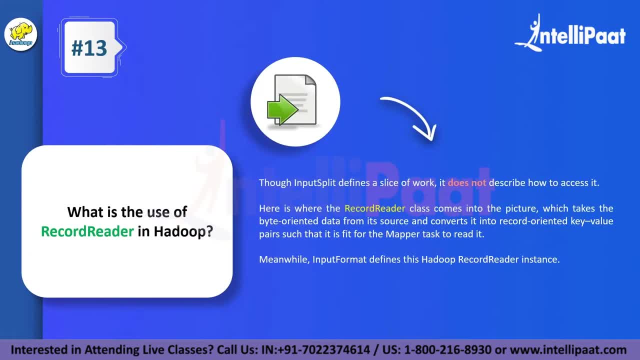 basically defines a slice of data, but then what it does not do is that it does not describe how to access this place of data, right? so what the record reader does is here it is. here is where this class comes into the picture. uh, you know, here we take the byte oriented data from its source. 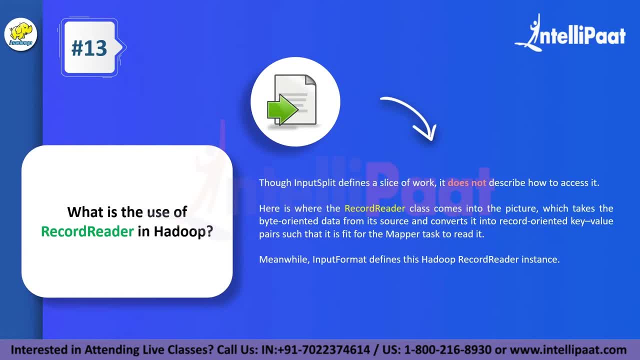 we directly convert it into the record oriented pairs. right, so you already know it. it's the key value pair. and after we convert the byte oriented data into its key value oriented data, then we give it to the mapper, where you know the mapper can handle the task. it can read it and work with it. so, in the background, what happens is that the input format 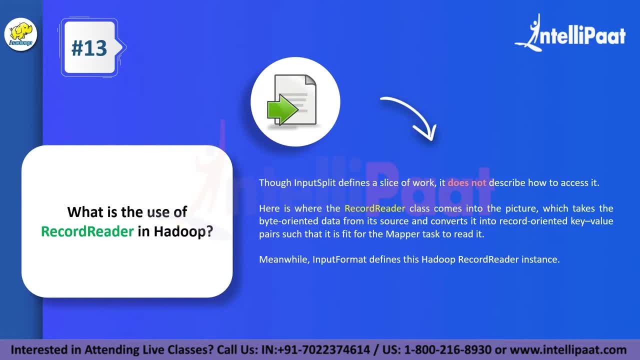 right, it actually defines the hadoop or record reader instance, uh, where, uh, it keeps adding up onto that list about what's going on, what files got converted, and if the mapper is ready to pick it up or not. so in that particular case, uh, you know, even record reader adds a lot of value to. 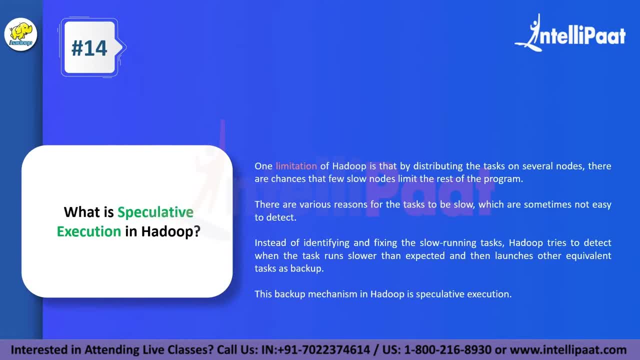 the hadoop. now, coming on to the 14th question, it says: what is speculative execution in hadoop? well, uh, you know, one important limitation we have to talk about every time we uh discuss about hadoop is that whenever you're distributing a lot of tasks on multiple nodes, right uh, sometimes it 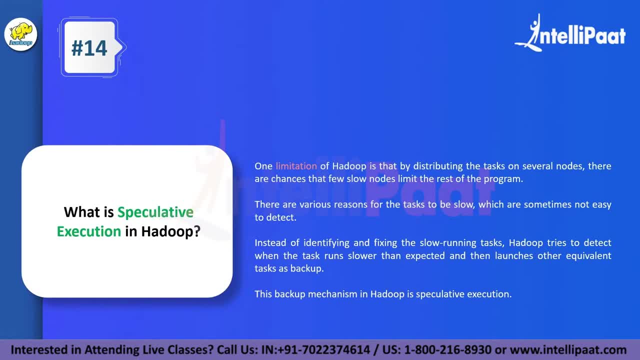 is not always that you have nodes which are really fast, so a few slow nodes will actually limit the execution. it will limit the efficiency of the entire program, right? so when you think about it, there might be multiple reasons of why it's so important that you're distributing a lot of tasks. 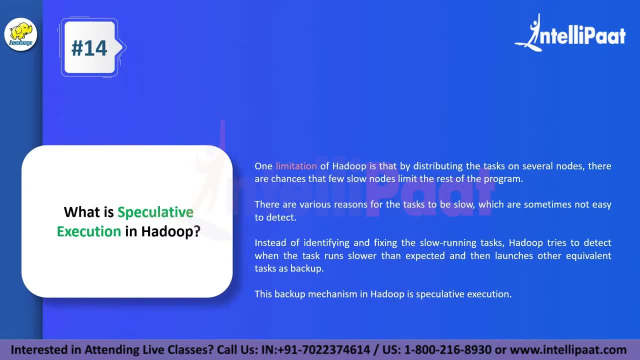 uh, you can go to the network library and find out why a task is slow. uh, in a small, in a small scenario. this is a. this is a very simple thing to find and you can work with it. hunt for the node which is slow and replace it. but when you're thinking about a large scale solution, it is not easy to detect. 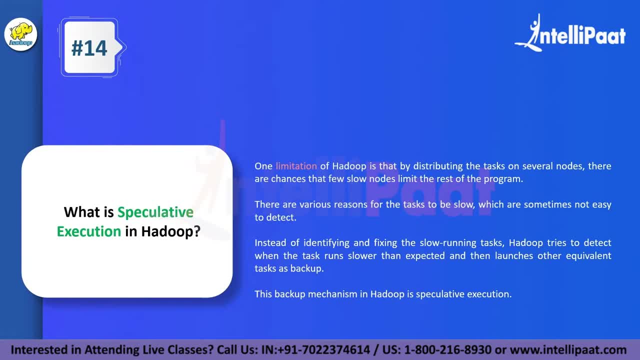 which node is slow. so what we try to do here is, you know, instead of identifying, instead of fixing all of these slow running tasks, hadoop will actually try to detect what tasks run slower than an expected time. it will have an expected time through which the task has to finish. it will see. 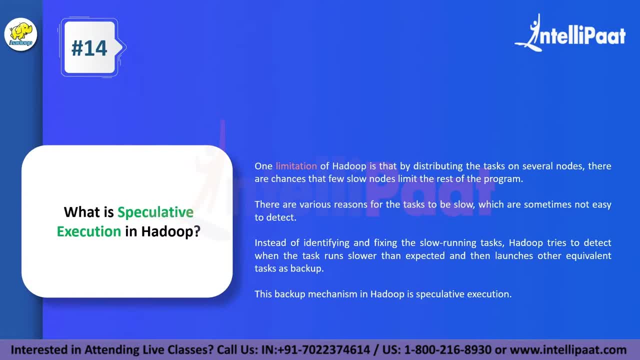 than the expected time And it launches other tasks, you know, as a backup in case if this is taking more time. So this backup mechanism that exists in Hadoop right, this is exactly what we call as speculative execution. This is a very important thing to maintain high efficiency. 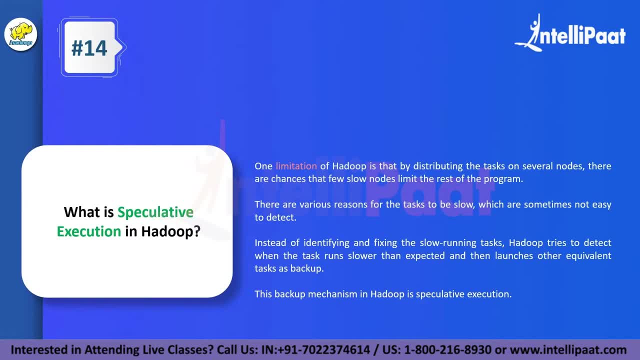 throughout the execution of our task. you know, getting closer to our big data handling goals, whatever it is, speculative execution is definitely one of the most important things. you know. that's adding a lot of value in the community of distributed computing. So 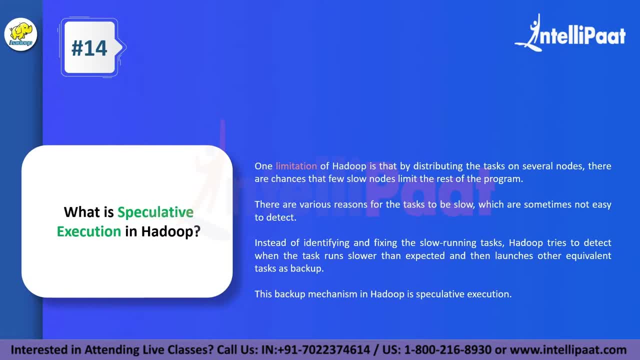 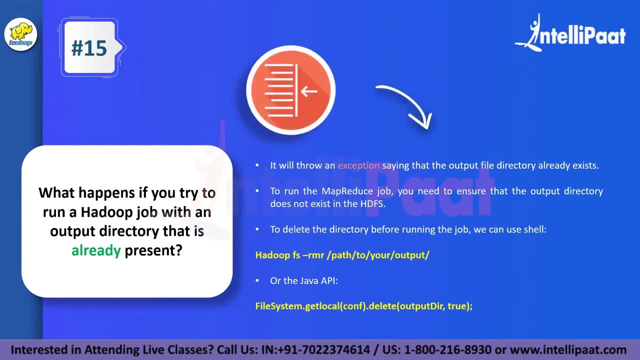 when you ask this question, you know make sure to give it out in a concise way. Coming to the 15th question, it says what happens if you try to run a Hadoop job with an output directory that is already present. Just a quick info, guys. test your knowledge of big data by answering this. 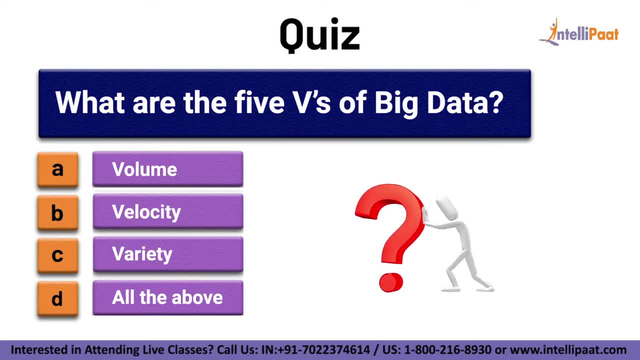 question: What are the five V's of big data? A, volume, B, velocity C, variety D. all of the above. Comment your answer in the comment section below. Subscribe to Intellipaat. know the right answer? Now let's continue with the session. Well, if your directory is already. 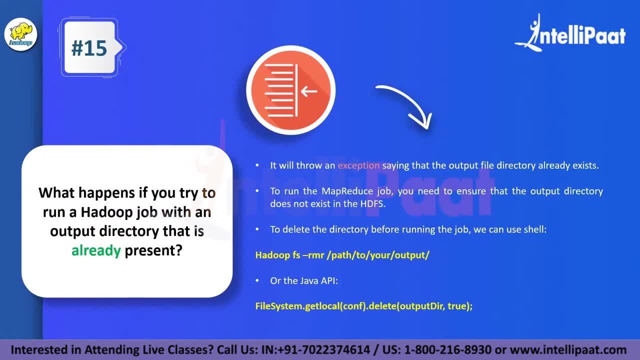 present what Hadoop does. it's a very simple thing: it'll give you an exception saying it already exists, Because you really cannot create a directory when already one is created, right? So a Hadoop job requires either the creation of brand new directory or you know, working with it as 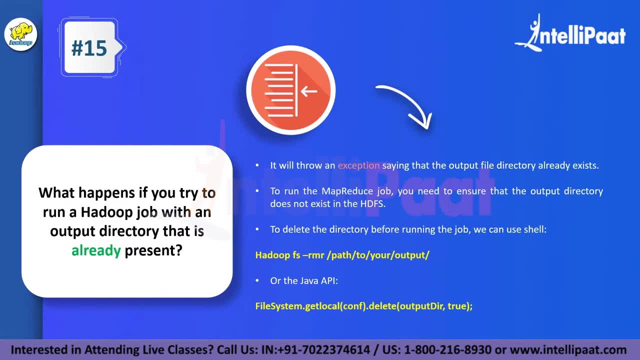 well, Make sure that the Hadoop directory will not exist, because if it does, it will not work. it will give you an exception. So in case, if it exists, but then you want to delete it and run your Hadoop job fresh, make sure to use the file structure command Hadoop FS RMR, which will 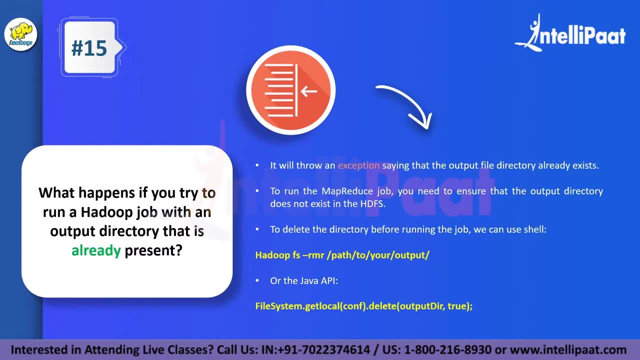 basically remove it, put the path to your output And as soon as you're done with it, you know you will delete a directory. or you can make use of a Java API as well: get local contour. delete will actually make sure that your directory gets deleted And later, as soon as you run the job, 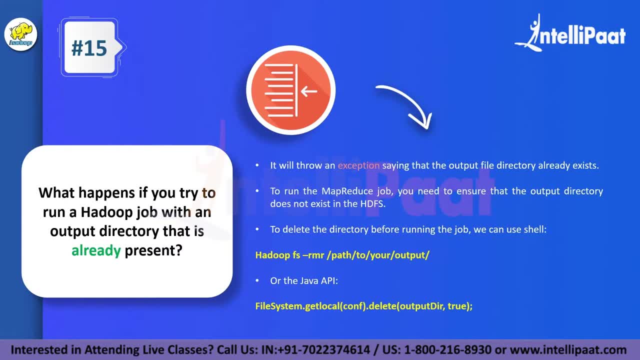 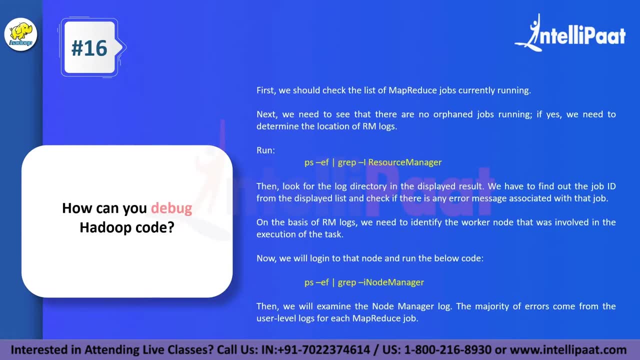 again. this time you will not be able to create a directory, So if you do that, you will not be have an exception, but this time the job will run as expected. Now coming to question number 16, it states: how can you debug Hadoop code? See: to debug Hadoop code, one very important step- you. 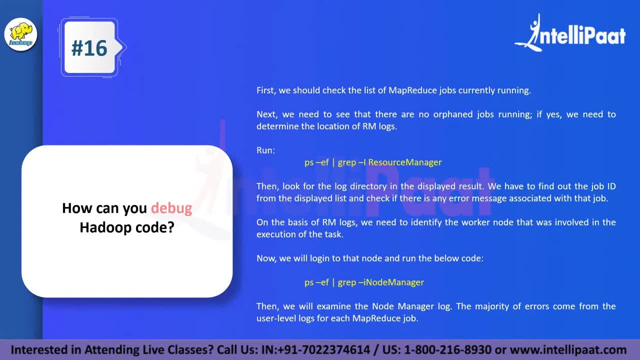 always have to check is to check the list of the MapReduce jobs that are currently running And once you see the logs, once you see all the jobs that are being run there, you have to make sure that there are no orphan jobs which are running. If they're running, make sure find the. 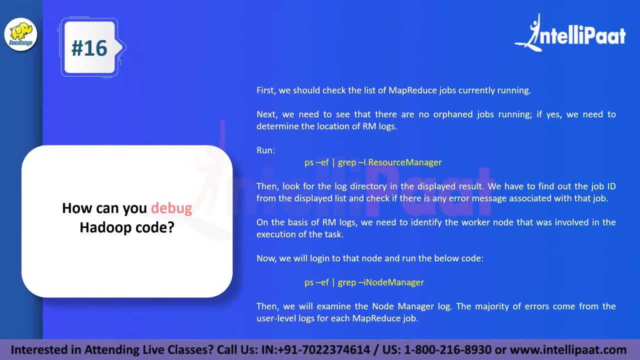 location of the RM logs, make sure to check it out And if you see that there are no orphan jobs, you know, especially when you run the command that's given on your screen right with the resource manager. So what it does is look for the log directory. It is very important that there. 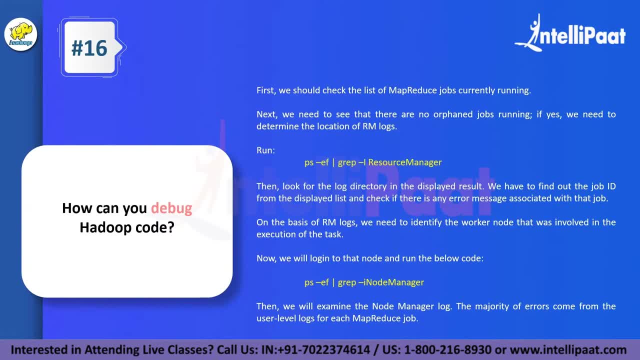 should be no orphan jobs running. So, based on what we find on the RM logs- right, we have to check if the worker node was involved in the execution of task or not. To do that we have to log into that particular node, right? Because without logging into that node we cannot see if a worker node 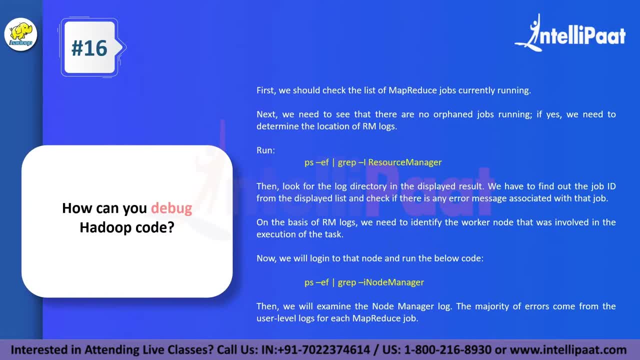 was involved in the execution of a task. To do that you can use PSEF, grep inode manager And you know you can log into the node to see if it is, if it is the worker node that was involved. So later, after doing this, what you'll actually do is examine the node manager log where you know. 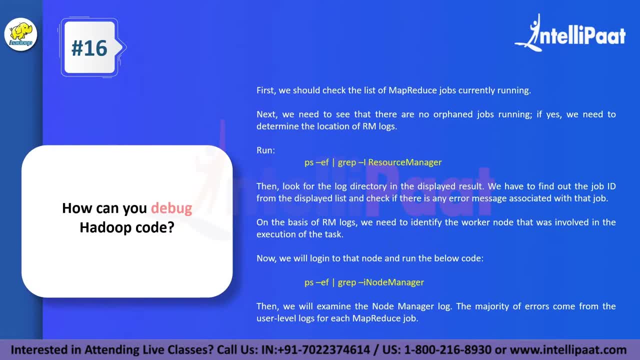 the majority of the user level logs come from here, you know, for every single MapReduce job out there. So this is a structured way, an ordered way of how you know you can simplify and debug Hadoop code If you have a Hadoop structure running on your machine, if you have a standalone. 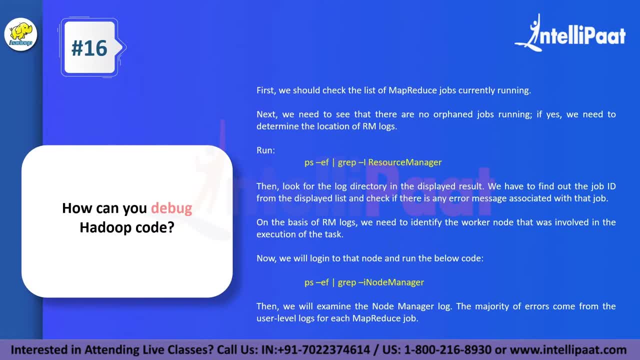 structure. or let's say, if you're connected to a, you know if you're connected to a, you know a multi-node structure as well. open up your laptops to show all the working of this practically to the interviewer. that will add a lot of value to your candidature and that particular company. 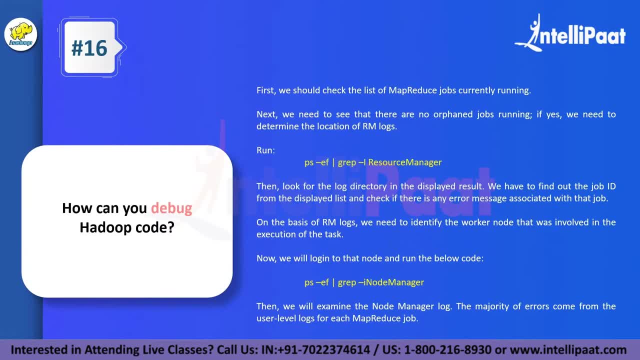 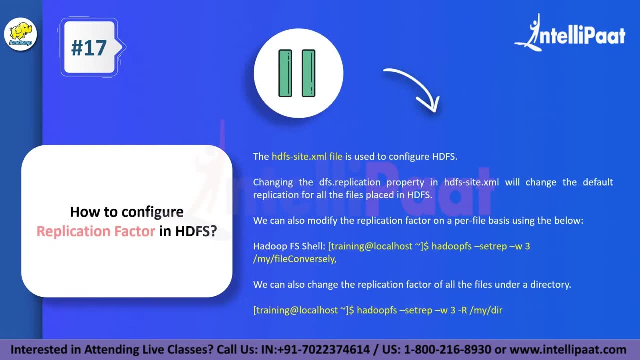 not just this question among all the questions we discussed. wherever it is possible, do show you know it practically. So with that we can come to question number 17 that states how to configure replication factor in HDFS. See to configure HDFS, you remember. 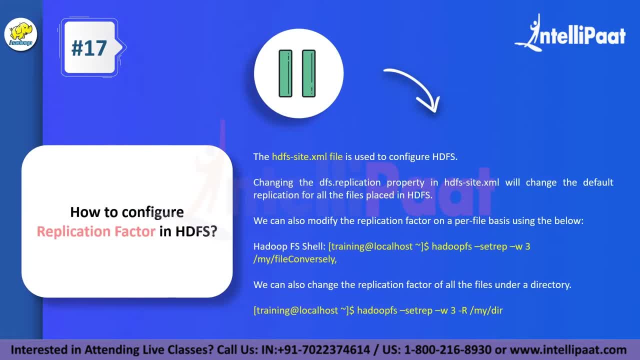 we spoke about three files and one of those files are HDFS site dot XML right. So this is a very important file which we use to configure the file system. So, basically, to change and configure the replication factor, we have the DFS dot. 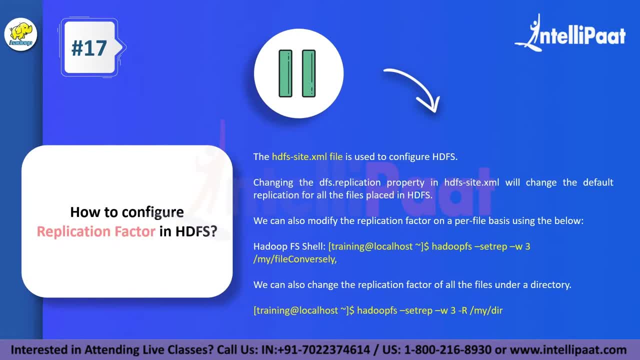 replication property. It's present in this particular file, So by changing that we can modify it. but then if we change it on a file basis, right per file basis, where you're checking out each, each and every individual file and working with it, for that you have a Hadoop. 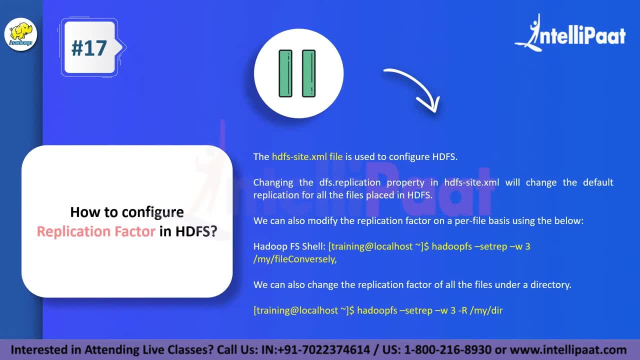 shell command, you know, Hadoop set rep, where you can put in the file name and work with it. But then if you have to change the replication factor of all the files at a time, but then not like each one of them individually, you can modify it. So you can modify it, but then if you have to, 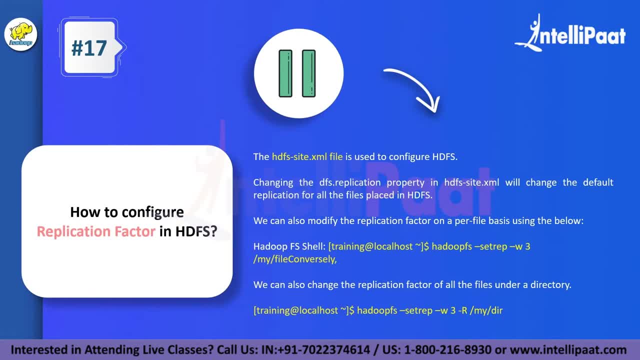 change the replication factor of all the files at a time, but then not like each one of them individually. then of course we have another Hadoop command for that as well. Uh, you know there are certain subtle differences. You have the capital R in the second one. that denotes that you'll be rep. 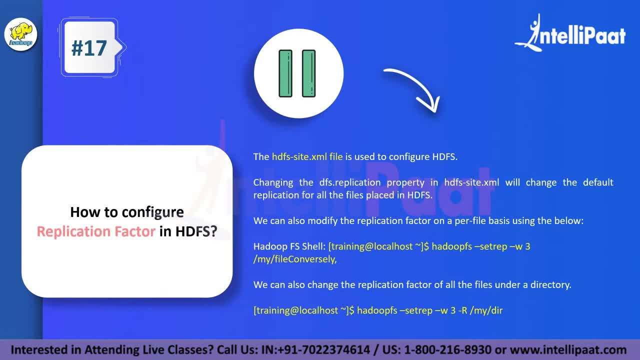 you'll be adjusting the replication factor for all the files in the directory And of course, for the first one it's only the individual file. So here it's very important that you talk about- uh, you know- replication factors on individual files and, of course, replication factor changing. 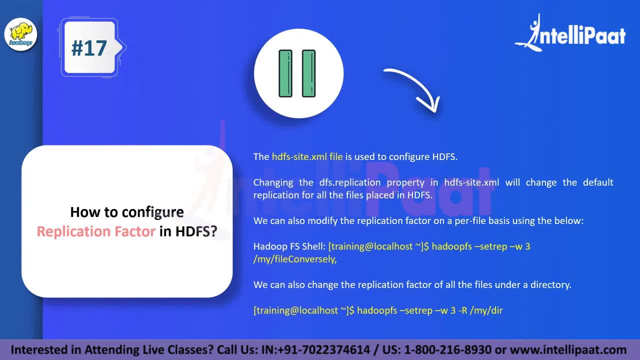 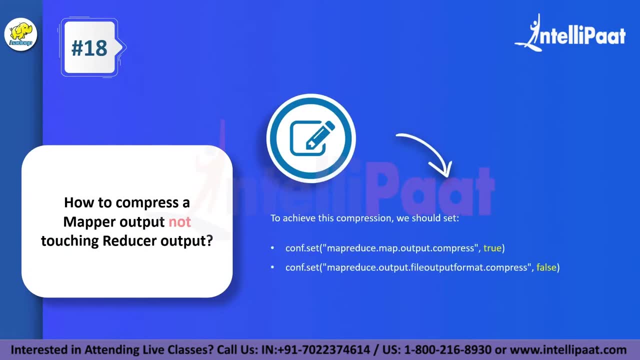 on all the files that are present in a single directory as well. So make sure to mention this. moving on to the 18th question, It states how to compress a mapper output- uh, you know, not touching the reducer output- to basically compress a mapper output which is not in touch in the reduction process. 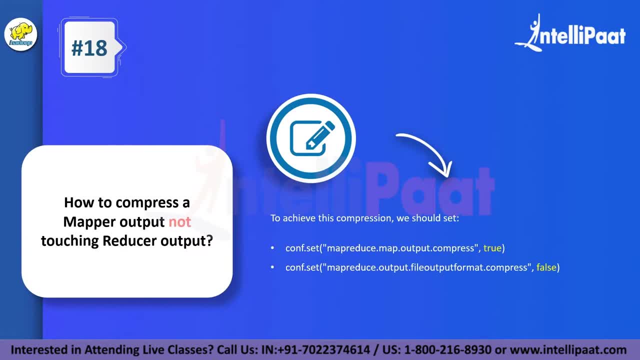 What we try to do is we set two things. to achieve the compression, We have con dot set where we're trying to set the output compressed to be true, And what we're trying to do is we're trying to keep the file output format to be false. So after setting these two parameters, 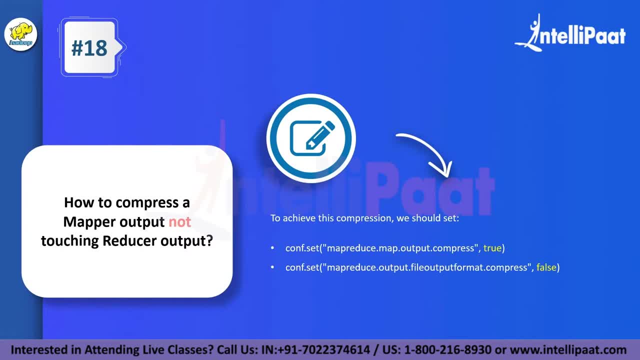 right, this is how compression can be achieved. It's a simple question, It's a very straightforward answer. And then, uh, you know, if you have a pen and paper, rather than spelling it out, make sure to write it down and show that you'll be setting the bitch to be true in the case of the map output, But in case 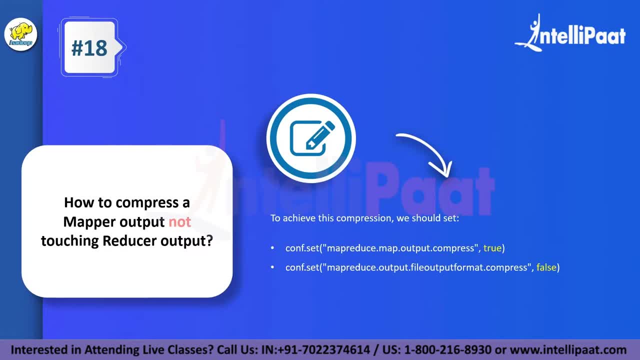 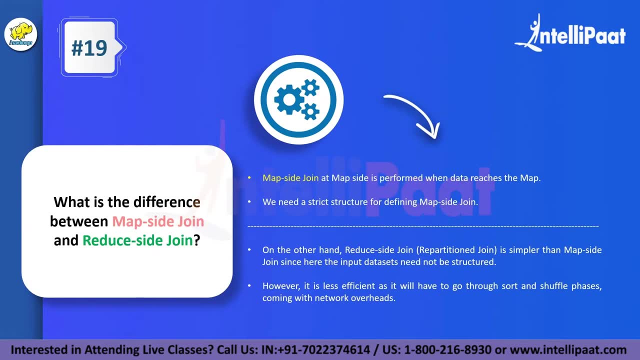 of the file output format, we'll be putting it to false. Now, coming to the 19th question, it states: what is the difference between map site join and reduce site join? Well, map site join happens at the map site right, As the name suggests. So whenever your data reaches the map, this is where. 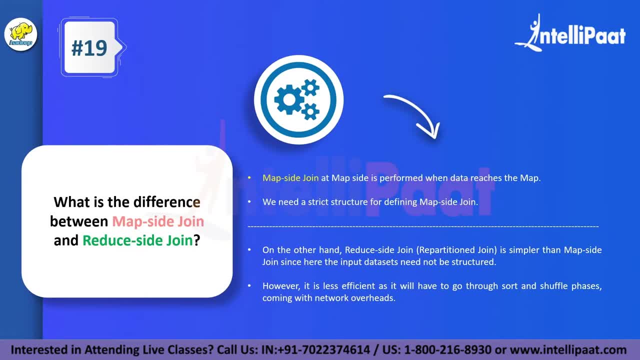 the join operation takes place. So then I'm sure you're already aware of this, but then to do this you have to have a strict structure, right? So, uh, especially when you're defining your map site joints, you really need that. But then when we talk about the reduced site joints, it's also called as: 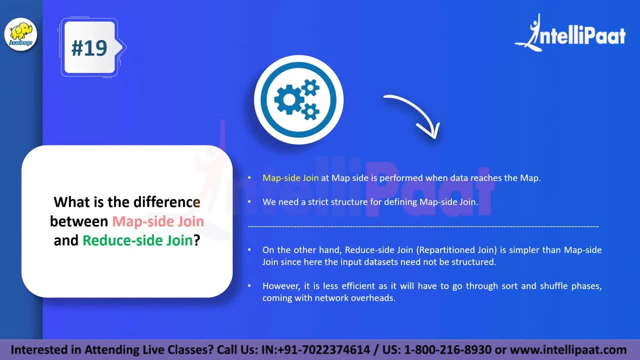 the repartition joints. So here, uh, you know, it's a little simpler when you compare it to map site joints, because here all we're trying to do, uh is, uh, you know, map the files rather than the. 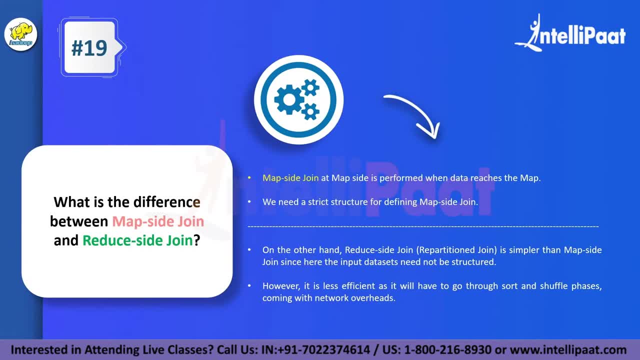 input data sets. The input data sets need not be structured out here. So, uh, when it comes to that, uh, you know so. but then when you talk about efficiency, right map site joins are more efficient here, because in this case you're not going to have to have a strict structure. So you 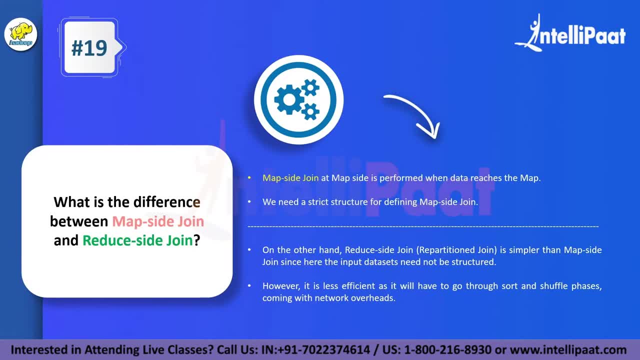 the case of reduced site joints, it'll have to go through a lot of sorting phases. It'll have to go through a lot of shuffle phases where, uh, you know, you'll be coming in touch with a lot of network heads and it might take a lot of time and, uh, you know, work power to actually get the job. 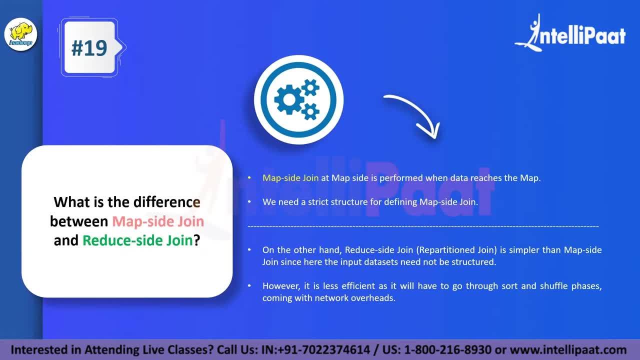 done in the case of the reduced site joints as well. So hence, uh, you know this is one of the reasons why people prefer the map site join, but then to do that, you need the structure, And this is a very important point that you should talk about Now. with this, let's come to the 20th. 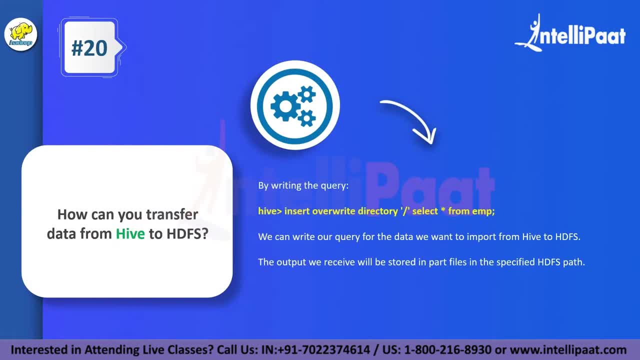 question that states: uh, how can you transfer data from Hive To HDFS? Well, it's a very simple question with a very simple answer. Uh, you just have one query that you have to write: where you can, you know, pick up the data from your Hive and push it onto? 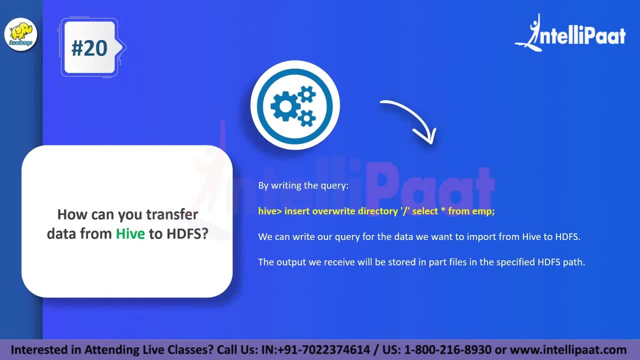 HDFS. It's Hive command is: insert override directory where you have the slash select star from EMP, where, uh, you know, EMP is the directory where EMP is actually the record there And, uh, you know, after you, after you execute this query, you can import whatever files you want from Hive. 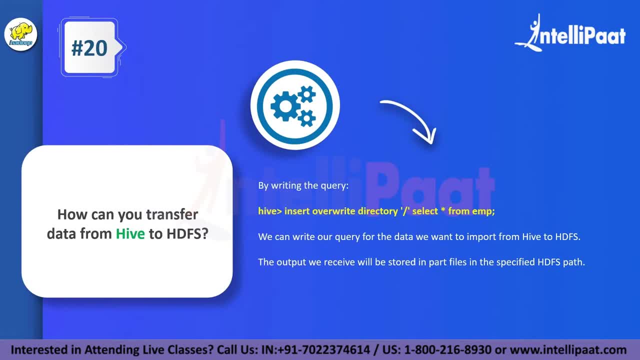 to HDFS. So the output that we get here is actually stored in part files in this specified file system structure as well. So that's one very important thing too. So if you are expecting a very complex process of transferring files from a Hive to HDFS, well, sorry to disappoint you. 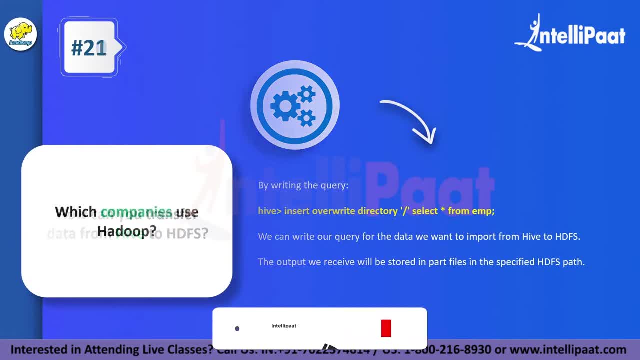 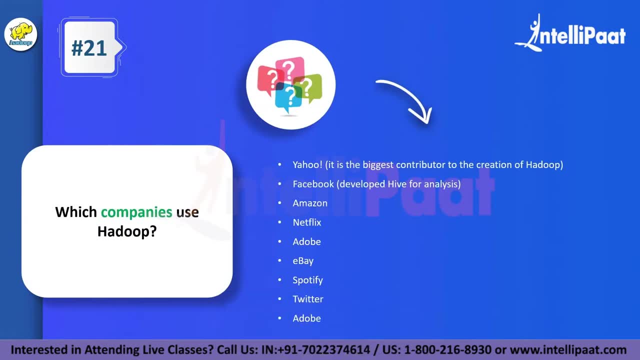 because it is pretty simple, as you can see on the screen. Coming to question number one, it states what companies make use of Hadoop. Well, there's a lot of companies that make use of Hadoop. In fact, there's thousands of companies right now making use of Hadoop. Uh, you know, even when? 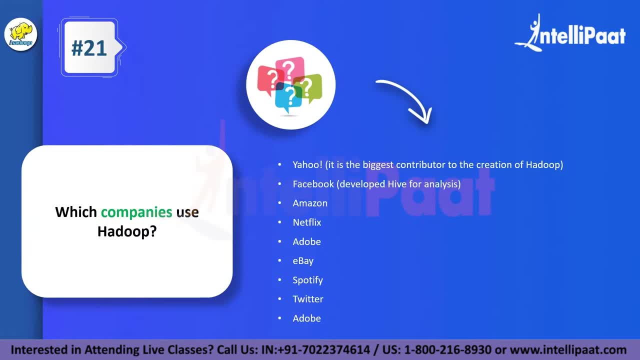 you're watching this particular video. uh, the big boys are Yahoo and Facebook, because Facebook developed Hive to perform analytics And we have Yahoo- is one of the biggest contributors in the creation, in the entire creation, of Hadoop. We have Amazon, we have Netflix, we have Adobe. 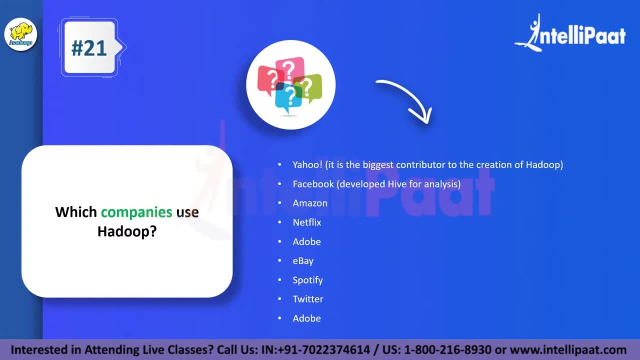 we have eBay, we have Spotify, we have Twitter, we have, uh, you know, a lot of other companies where each of these products have one particular or multiple- uh you know- use for Hadoop. So it it can be a very small scale solution that they're trying to implement, or, in fact, 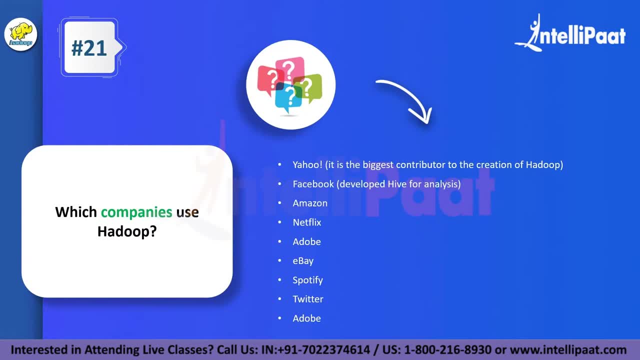 it can be a very huge thing. uh, you know that they're trying to add on to their company by making use of Hadoop as well. So in that particular case, right? Uh, Hadoop is very, very well regarded and used a lot, uh, in many companies out there today. 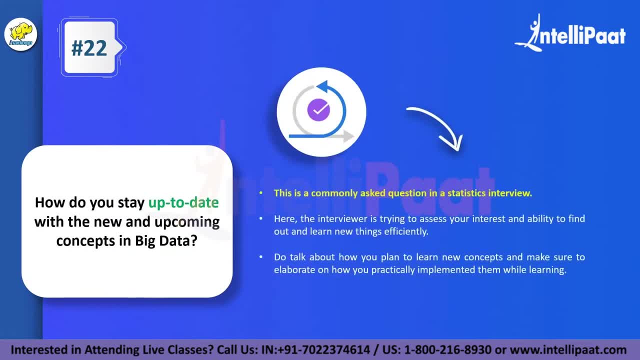 So question number 22 stays: how do you stay up to date with the new and upcoming concepts in big data? So the 22nd question states: uh, how do you stay up to date with the new and the upcoming concepts in big data? You have to know one thing is that this is a very commonly asked question. 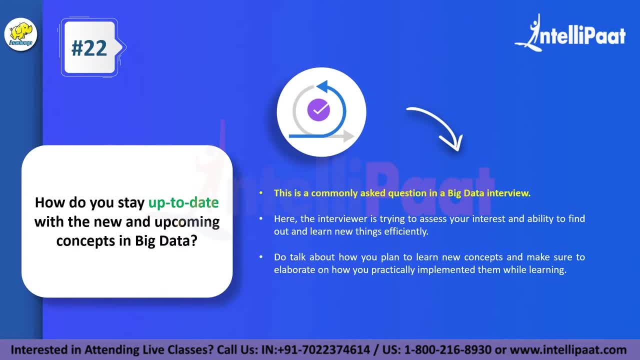 here because, with this right, the interviewer wants to understand what your interest is, where your interest lies. And, uh, you know you have to know about the possibilities of learning something new and how can you learn it. well, So, talk about how you've learned things in the past. talk about how you're planning to. 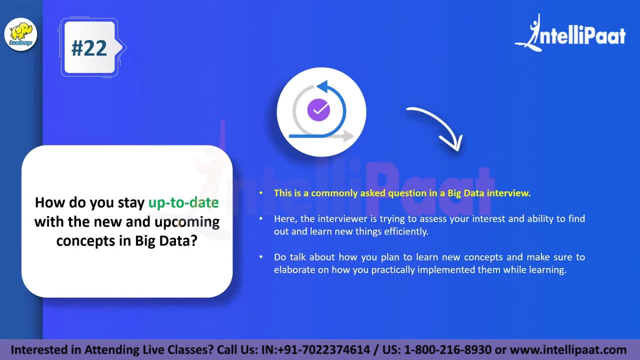 uh, you know, use these past learnings. uh, probably you could have taken an easier way to learn, a more structured way to learn, or, you know, there are many other concepts which keep coming out right. So the tool of today will become obsolete tomorrow. And, uh, it is very. 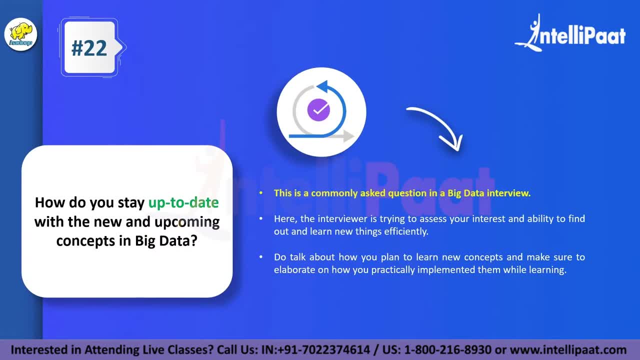 vital that you know the latest versions of the software, you know what are the changes that happen. And it's not only that. it's about how you change yourself with these new changes, or how you plan to- uh, you know- impart these new changes in a 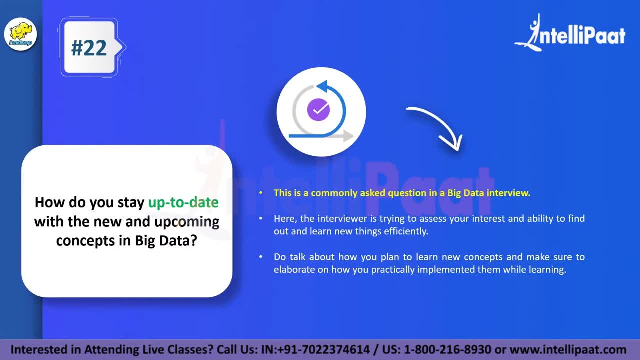 very simple way, in a fashionable way, in your particular project, uh, or whatever you're handling. So the interviewer wants to understand this. uh, you know he or she wants to understand your interest, your ability to actually find and how you will learn new things, because in 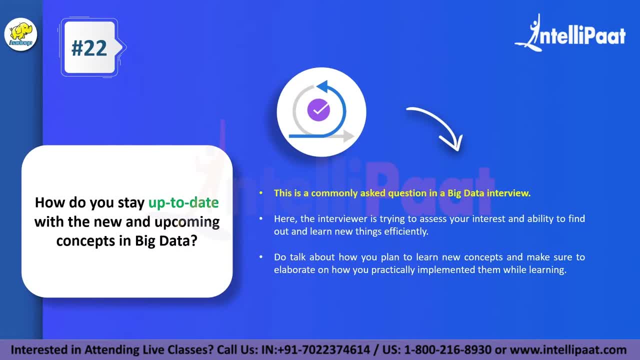 a production environment. when you're looking for a job, uh, it becomes very vital that you have to pace yourself and learn new things rapidly. So make sure to keep this answer concise, but then put it out in a clear way, Uh. 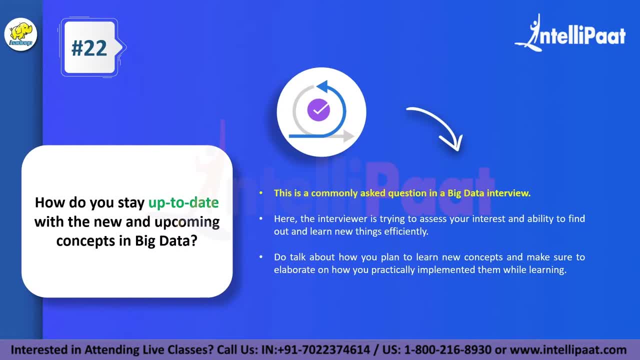 you know, if, uh, if you have a path, uh, it can be very different from what I told you. You might, you know, go on the internet, check a couple of YouTube videos, pick up a certification program or whatever it is. Uh, you know, you really have to mention your way on how you plan to learn new. 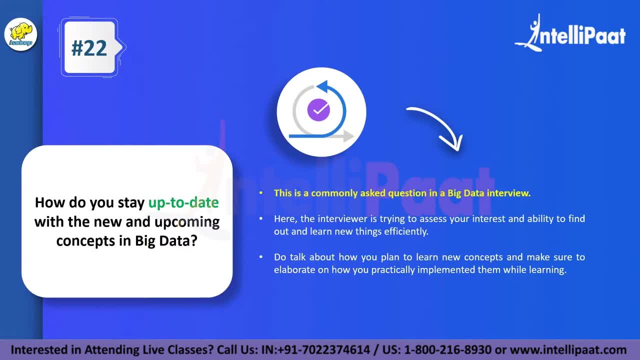 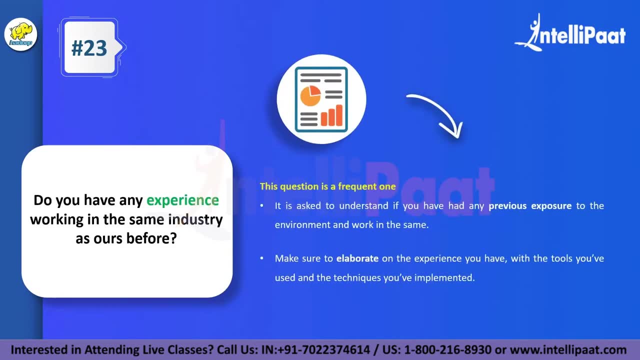 things as an added bonus. Talk about how you've used these new things as well. Coming to the 23rd question: uh, you know, if you're a fresher or if you're, uh, if you're an intermediate user. 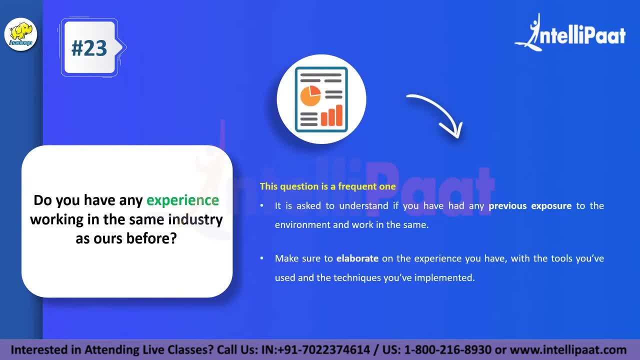 or, let's say, if you're an advanced developer, there's a good chance. uh, you know this question is asked. It's a very frequent one. Uh see, uh, you know Hadoop is used in multiple different uh kinds of so Hadoop is used in: 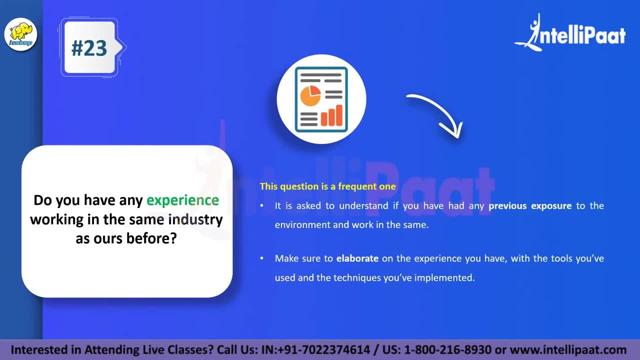 multiple industries, right? So you might be working at Facebook, which is a social media company. Uh, you know there's many other companies, right? There's Google. uh, you know, there's Yahoo and Adobe, which do a lot of different things compared to social media. So, uh, based on the industry, 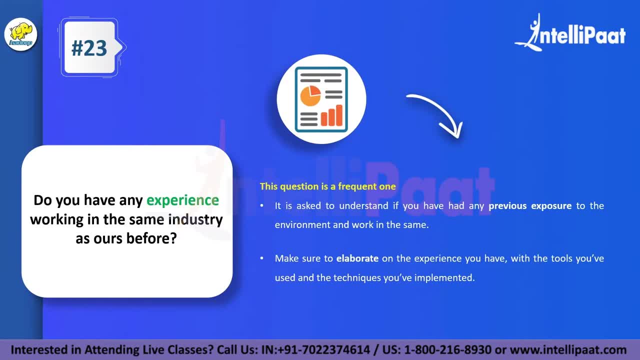 that you have worked in before. if you're a fresher, of course you can say you're a fresher and, uh, you know you'll move on to the next question. but then if you're an intermediate developer, uh, you know who's looking forward for this interview? uh, if you've had any 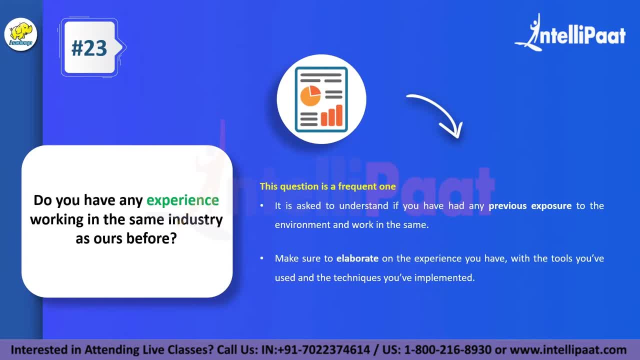 any experience in that industry right? So make sure to elaborate about it. talk about the industry experience that you have, because, at the end of the day, you can talk about the tools you've used, You can talk about the techniques that you've used and how you've made a change in the 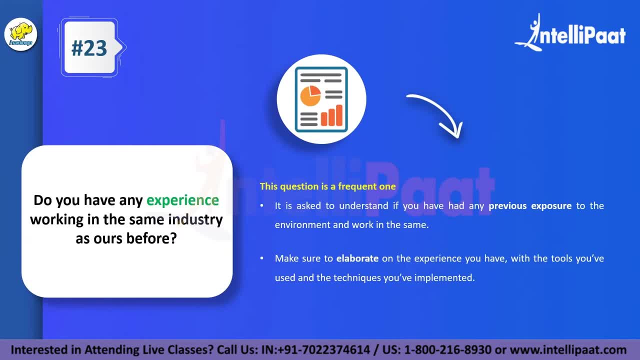 same industry before and basically what you bring to the table as well. So it is very important: if you have the industry, do talk about it, but then if you do not have it, uh, talk about how you plan to bring the learning from the industry that you belong to into this particular one, So you might. 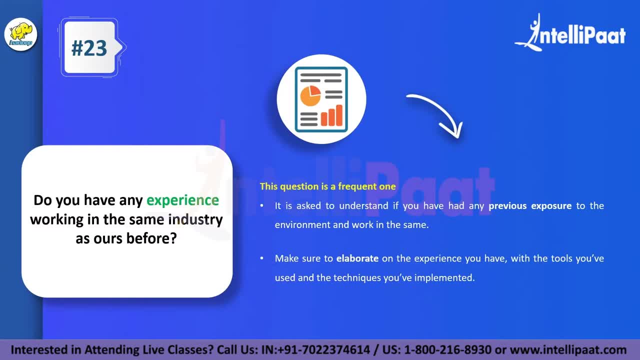 be moving from social media to another industry, but then talk about how you plan to make that switch of what you'll carry along with you from that, uh, different industry, to see to it that, if it works or not, or how better- uh, you know- it can be implemented. 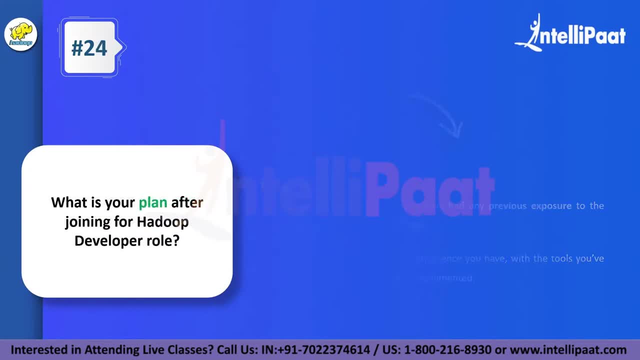 in this particular industry as well. So this is a very important question. And then the 24th question stays: what is your plan after joining for the Hadoop developers role? Well, the first thing you have to talk about is when you asked for any plans in the future. right, So talk about how. 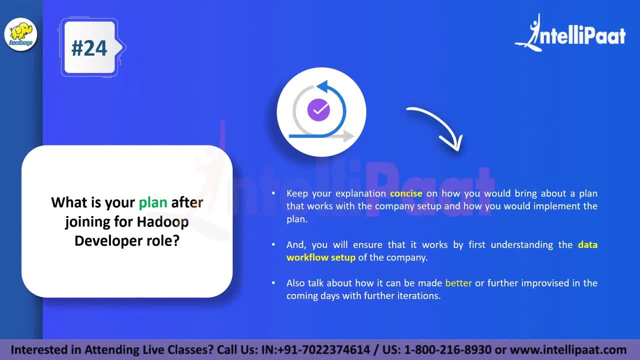 you're planning to understanding the complete data workflow setup In the company, because once you understand the workflow of the company, then you can have a plan of action. You can work on the plan of action, discuss it, implement it and verify it to see. 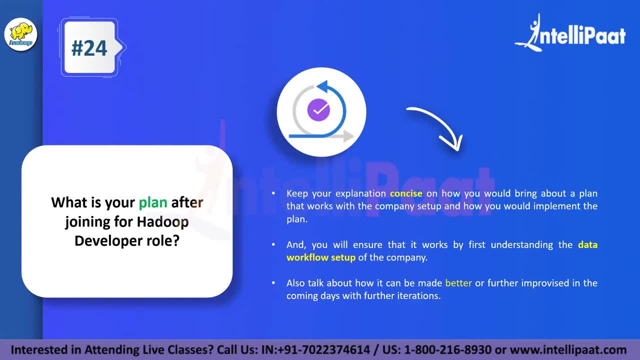 if it's working or not. Uh, you know, don't just say, uh, that you're going to step into the company and start changing things around, because that definitely wouldn't work in a production environment. So you yourself have to get very familiar with what's going on, what's already. 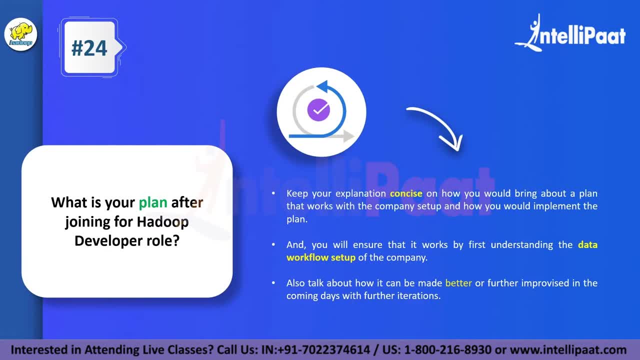 existing and then you can work on seeing what can be changed, what can be made better. Or, in fact, if you feel like you're going to be able to do it, then you're going to be able to do it, So you 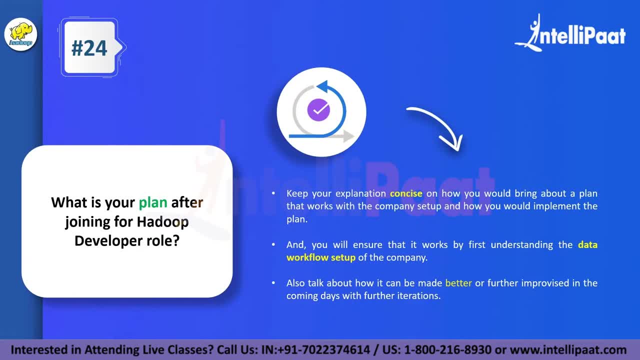 can get into, uh, the actual requirement that is already there and you will not have to change anything. So in multiple cases like that, it is very vital that you state out a plan of action, right? You joining, you learning new things, you talking to the people who have done it. 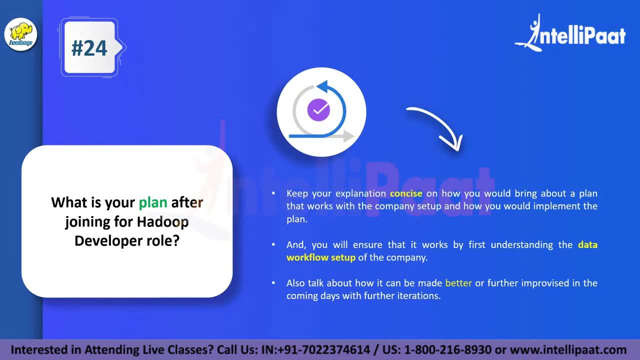 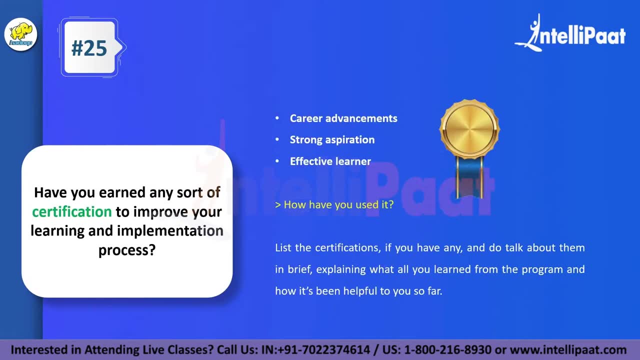 see what can be done better, verifying if it can actually be done better and doing it better. So this is something that would add a lot of meaning to your particular interview as well. So with this we can come to the last question, The 25th question. that says: 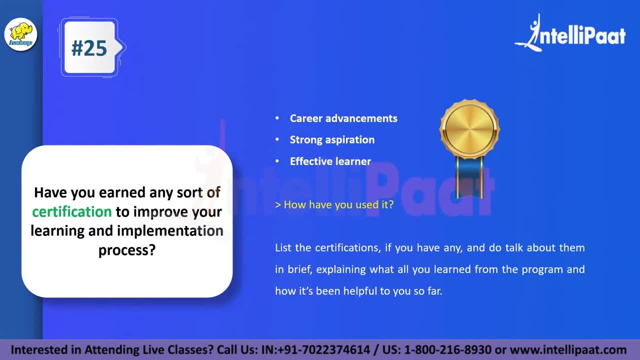 have you earned any sort of certification to improve your learning and implementation process? Well, uh, I'm sure if you're at this point of time- uh, you know, if you're at the 25th question, you will already know the value for the certification program would bring to you right? 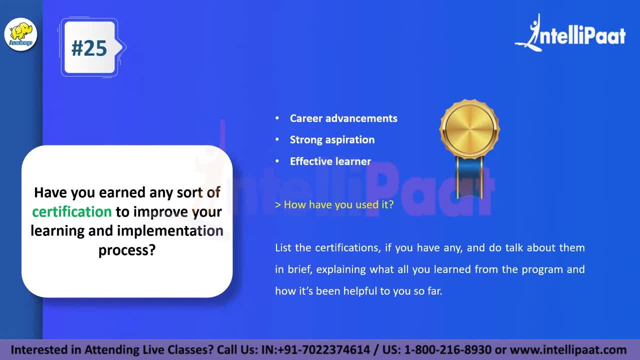 So you will have a lot of uh experts teaching you a lot of content over a couple of months. Uh, you'll be picking up industry level projects. You'll be working on real time projects. You'll be uh given thorough training where, basically, you have learned all the concepts thoroughly. A good 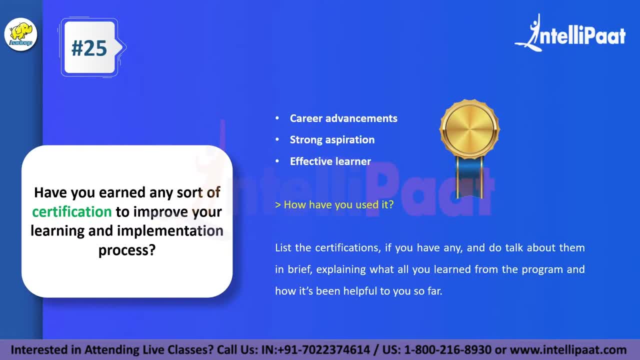 certification program will also give you industry level projects where you can actually implement your learning to see and improve. Uh, you can actually implement your learning to see and verify if you have actually learned, because, at the end of the day, what you put on your resume is: 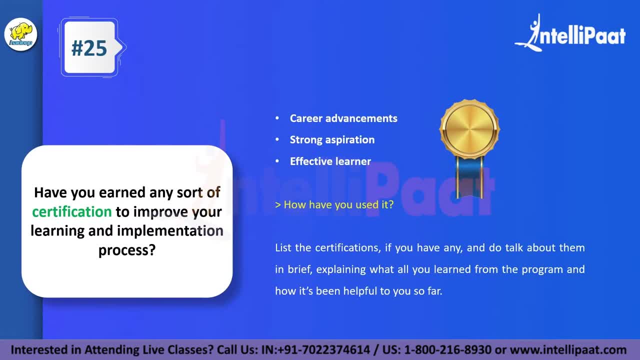 your projects right. So if you put on a certification, well, it's well and good. but in an interview, as soon as they talk about the certification, the first thing the interviewer is going to ask is: what did you learn and how have you solved problems using that? Because when you 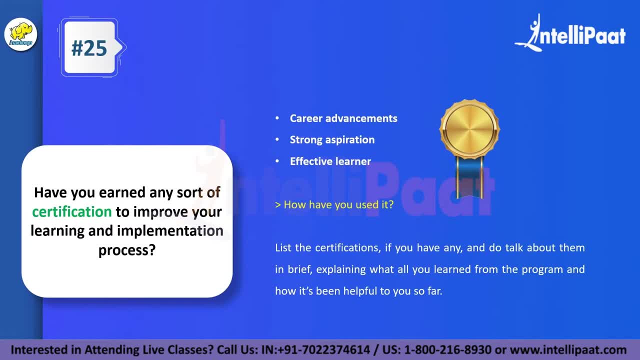 think about it: all the IT problems that exist out there today, right, Are being solved, and we have solutions for that. See, the entire process of big data handling itself is a problem, and handling that is is the solution right. So we had a lot of data that's being generated. 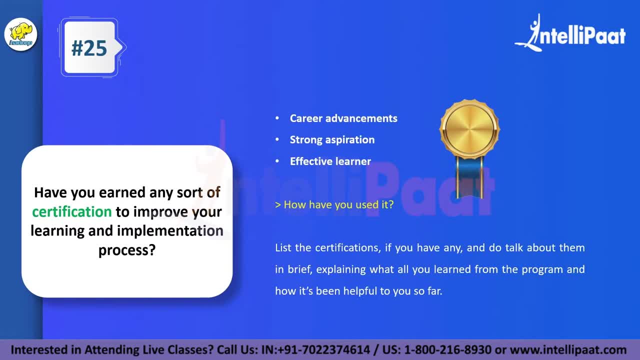 every day, and now we know how to handle it and work with it. In fact, that is one thing that you could state about what you learned in that particular program, but then me. but then make sure to elaborate about how you learned it and how you've planned to use it in the near future. 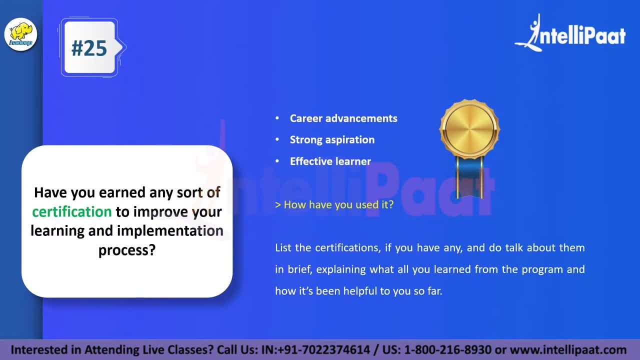 or how you already used it in the past to solve a real life problem. So all of these- uh you know, will give the interviewer an impression that you are very good at advancing your career, that you've put in your time, your money, your effort into, uh you know, working on Hadoop or 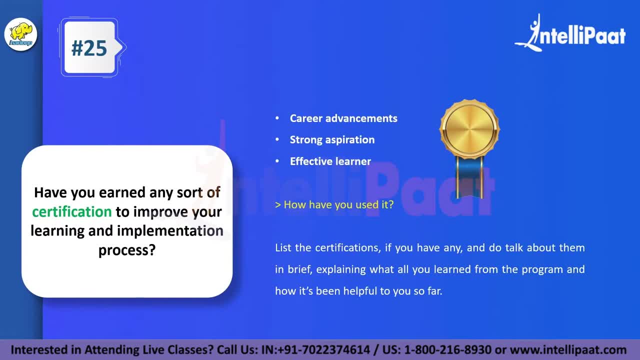 big data. In fact, it also shows that you are an effective learner and that you have strong aspiration to pick up a certification program, to learn to it, to see through it thoroughly and become an expert at the end of it as well. So certification program adds a lot of value to you. 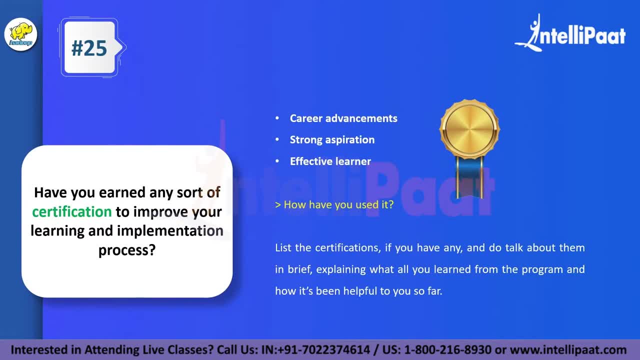 as well as the interviewer, because, uh, you know all of that. the knowledge that you carry is very important for the company there as well. So, in terms of job prospects, in terms of impressing the interviewer, uh, in terms of, uh, working well at the job, that you do anything right. 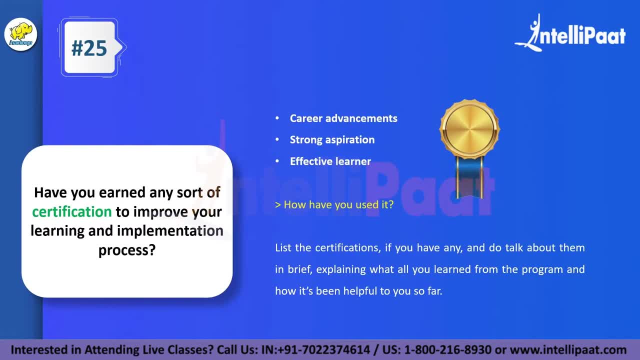 Certification program definitely helps. So with this, uh, we come to the end of the top. uh Hadoop interview questions set. Uh, I take this opportunity to wish you guys all the very best for all the interviews out there. Uh, you know you can use this as a guide to see how you can approach each. 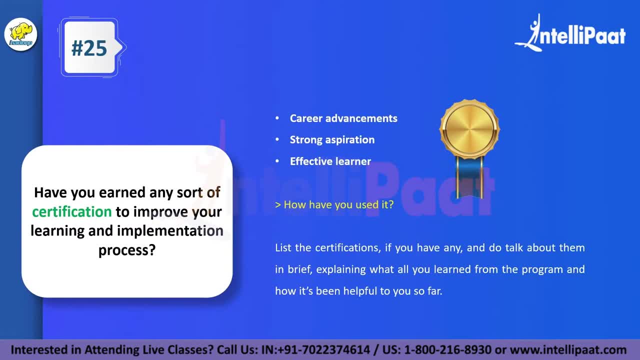 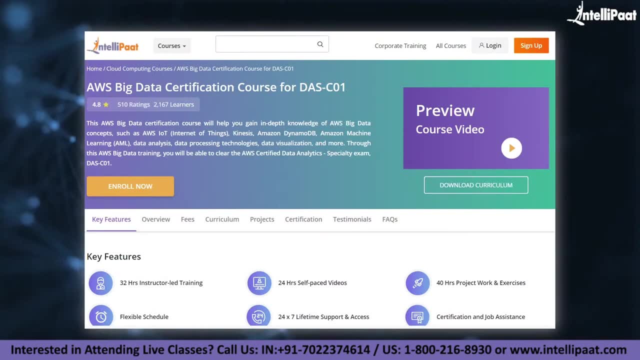 of these questions in an effective way and how you can answer them in a clear and a concise way too. So with this, I wish you all the best and I'll see you on the next one. Just a quick info, guys. Intelipaat provides AWS big data certification code.